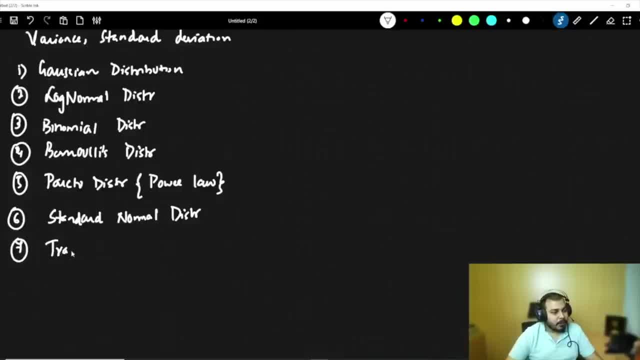 have different, different techniques. We'll be discussing about transformation, We'll be discussing about standardization, We'll be discussing about different kind of transformation, And this all will be with the help of Python. also, We'll try to see, We'll distribute. 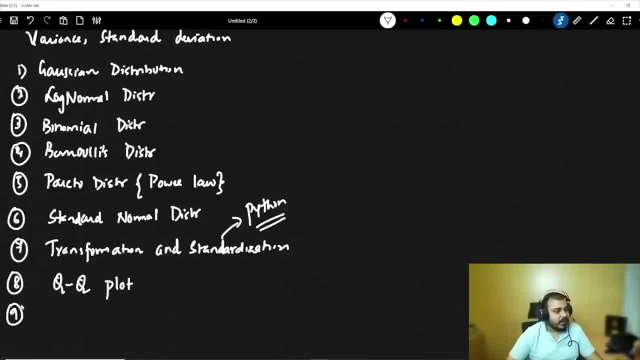 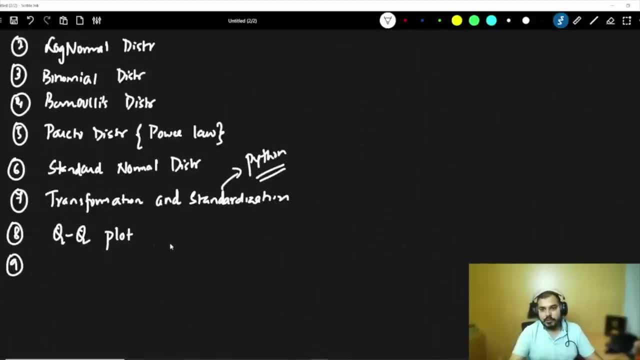 We'll discuss about something called as QQ plot. We'll try to find out, Find out how to determine whether a distribution is a normal distribution or not. That all things will try to discuss. These are some other topics that I have written. 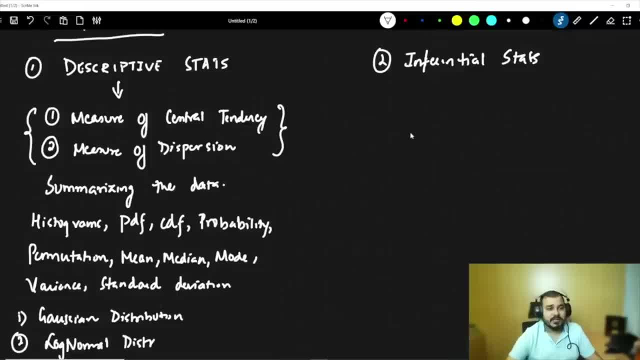 There is also very something, very much important, which is called as inferential stats. Now, in inferential stats, our main focus is basically like Z-test, T-test, ANOVA-test, chi-square test. If I just consider some example with respect to Z-test, there are multiple ways. 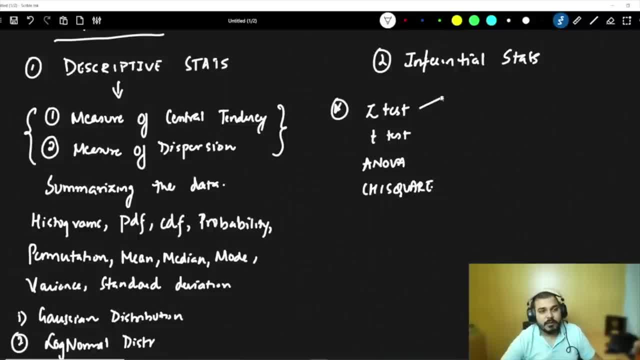 to actually perform Z test. So in Z test probably you will be having different ways, and this I will also try to show you by executing in Python T test. also I'll be showing you by using Python programming language: Chi-square test, ANOVA test. so ANOVA test is also called as something called as F test. we will be. 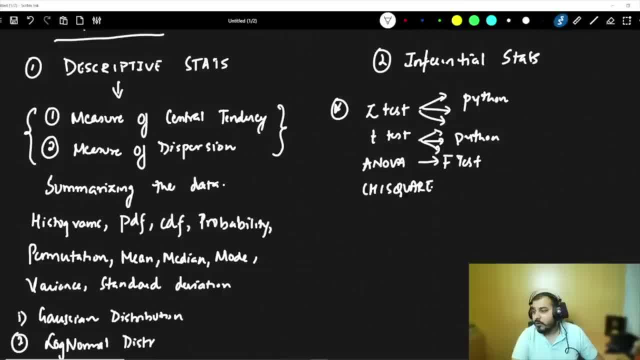 discussing about this, like factorial ANOVA, different kind of ANOVAs that we are going to discuss. Most important thing, we forgot right, which is called as hypothesis testing. how can I forget this? okay, so we are also going to discuss about hypothesis testing, right in hypothesis testing. how do you? 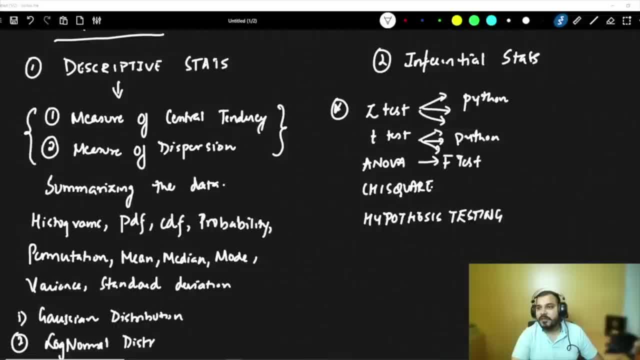 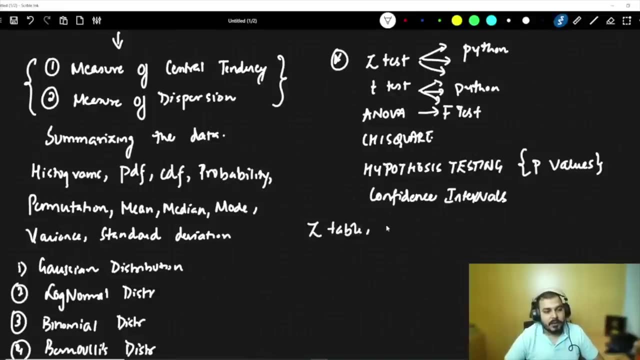 determine your null hypothesis, alternate hypothesis- everything will probably get covered in this. Here we are specifically going to understand about p-values. one very much important thing is something called as confidence intervals- confidence interval- then I'll also teach you how to see Z table. you know which is. 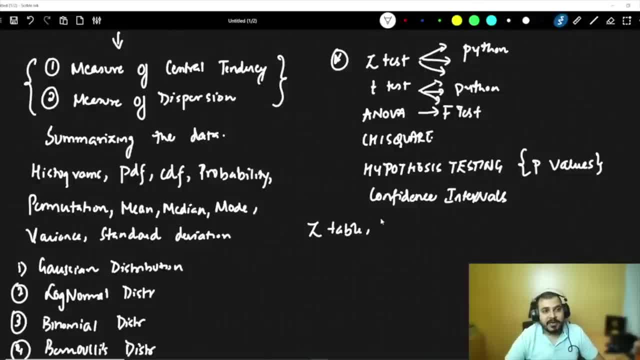 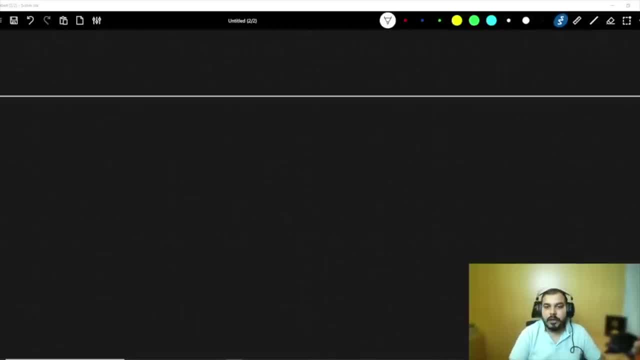 a kind of sheet where you can directly get the values over there. similarly, T table is there? chi-square table is there? many things will basically be there. Let's start the first topic. the first topic that obviously anybody needs to understand is that: what is statistics? okay, we really need to understand, because whatever I'm discussing right it. 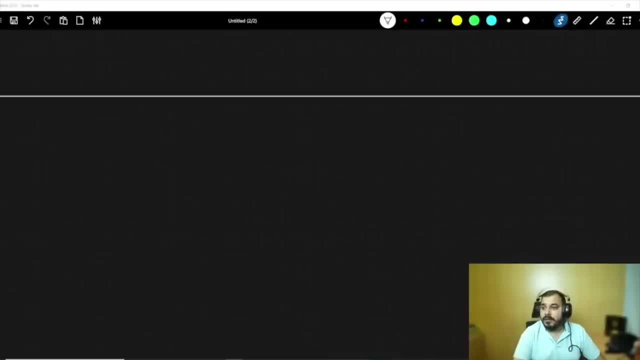 is very much important in terms of interview. in terms of interview, I'm actually going to teach so that you will definitely be able to understand many things. so the first thing: we will understand what exactly statistics. many people have different kind of definition with statistics, but I really want to. 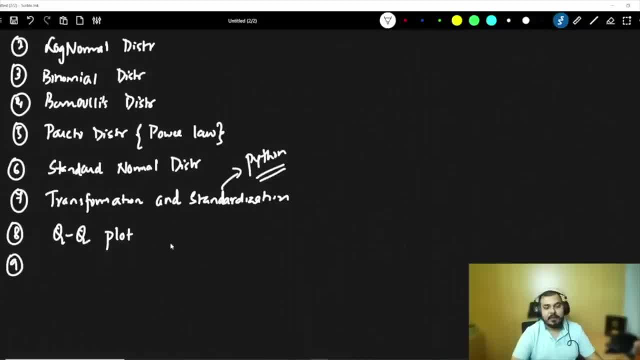 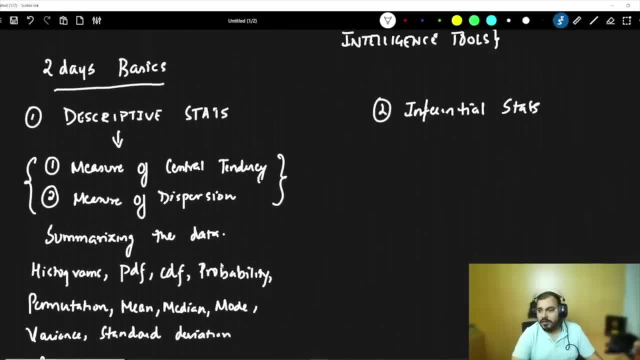 find out how, how to determine whether a distribution is a normal distribution or not. That all things we will try to discuss. These are some of the topics that I have written. There is also very something, very much important, which is called as inferential stats. Now, 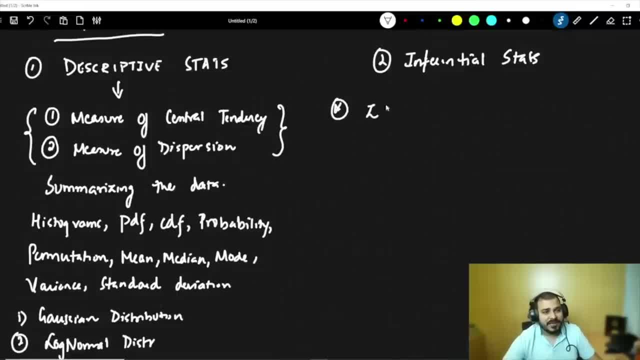 in inferential stats. our main focus is basically like z test, T test, ANOVA test, chi-square test. If I just consider some example with respect to z test, there are multiple ways to determine And this is important because we are currently looking at a very, very high level of information. 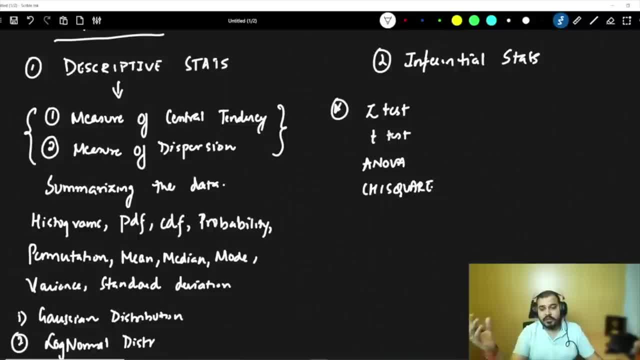 I will have to understand this, especially in terms of these two, x, y, z and t. These are just example of Bisquery. Now, for example, I am going to try to talk about differential statistics, multiple ways to actually perform z test. so in z test probably you will be having different ways. 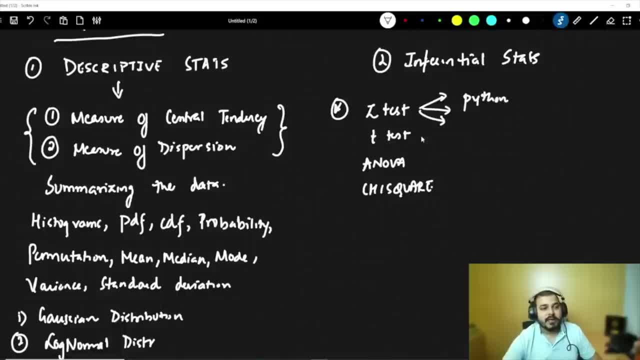 and this i will also try to show you by executing in python t test. also i'll be showing you by using python programming language: chi-square test, anova test. so anova test is also called as something called as f test. we will be discussing about this um like factorial anova, different kind of anovas. 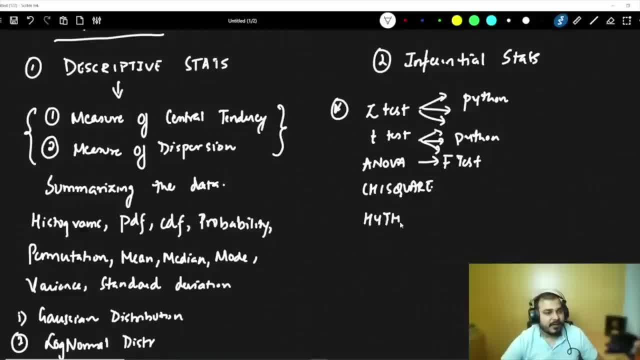 that we are going to discuss most important thing we forgot right, which is called as hypothesis testing. how can i forget this? okay, so we are also going to discuss about hypothesis testing. right, in hypothesis testing, how do you determine your null hypothesis, alternate hypothesis- everything will probably get covered in this uh. here we are specifically going to understand about. 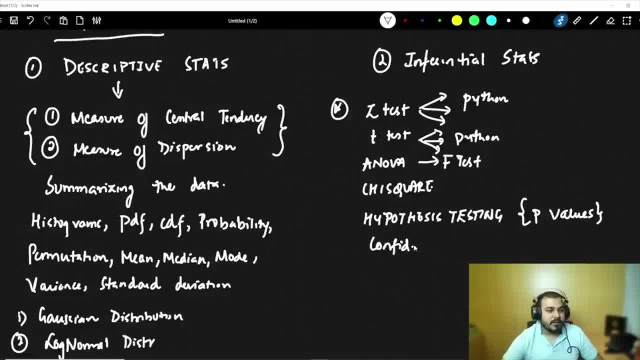 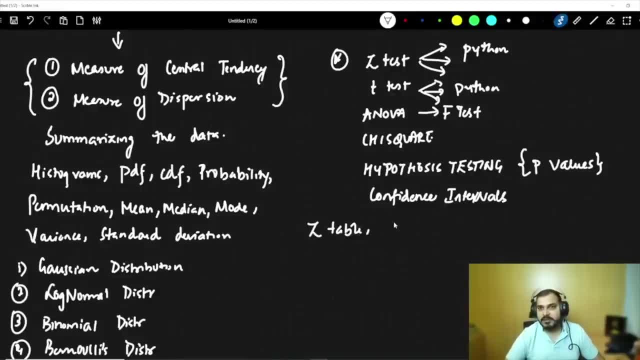 p values. one very much important thing is something called as confidence intervals. confidence intervals, and i'll also teach you how to see z table, you know, which is a kind of sheet where you can directly get the values over there. similarly, T table is there? chi-square table is there? many things will basically be there. let's start the. 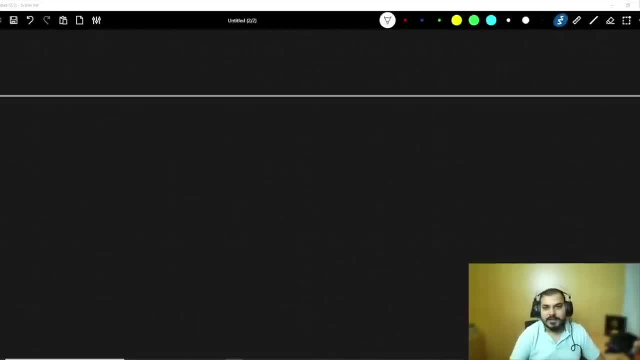 first topic. the first topic that obviously anybody needs to understand is that: what is statistics? okay, we really need to understand, because whatever I'm discussing, right, it is very much important in terms of interview. in terms of interview, I'm actually going to teach so that you will. 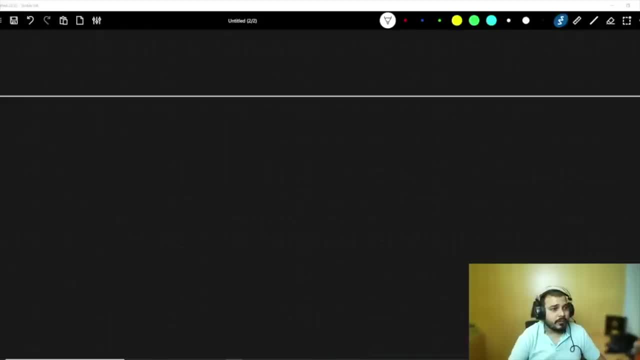 definitely be able to understand many things. so the first thing: we will understand: what exactly statistics? many people have different kind of definition with statistics, but I really want to give a very simple definition, which is from Wikipedia. so I'm going to say: statistics is the science of collecting, organizing and analyzing data. now you know. 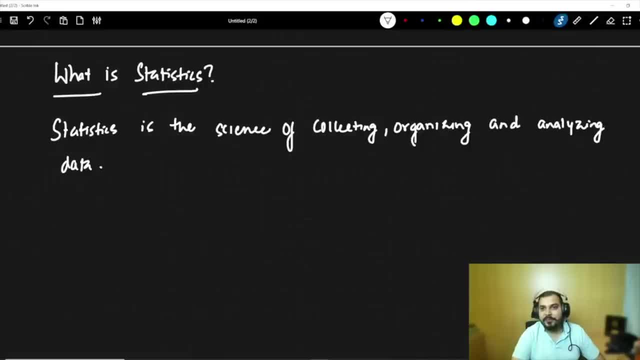 based on the amount of data that is getting generated. now you can just understand directly like how important stats is. you have tons and tons of data. you have huge amount of data and definitely you can actually utilize this particular data to make sure that there is improvement in your products, there is improvement in your business goals and that actually helps. 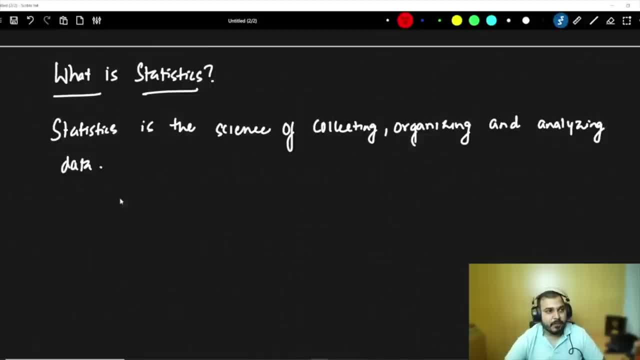 you to finally make a very good decision. so, finally, why why we are doing this? for why we are doing this? for better decision-making. so we are specifically doing this for better decision-making. everything that is basically getting covered on this and if I try to now this, define statistics or the types. 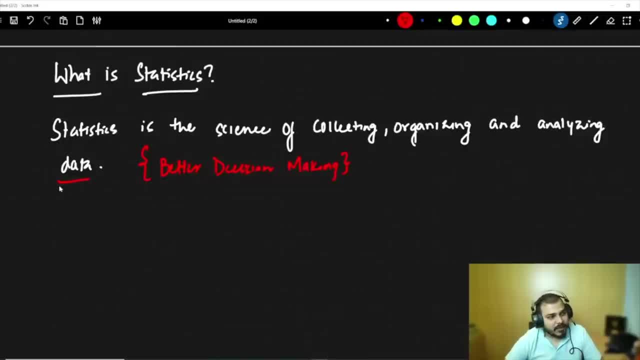 of statistics. first of all, there is one very important thing, which is called as data. so data over here is nothing but facts or pieces of information that can be measured. so what is data in short? a fact or a piece of information that can be measured. so what is data in short? a fact. 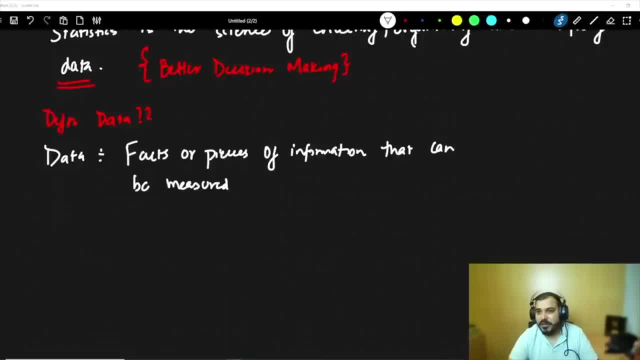 so pieces of information that can definitely be measured, and let's go ahead and let's see some of of data examples. basically I saying between 0 to 100.. Suppose let's say that I am getting this one, I'm getting this, I'm getting 55,, I'm getting 75,, I'm getting 65. So this is one example of 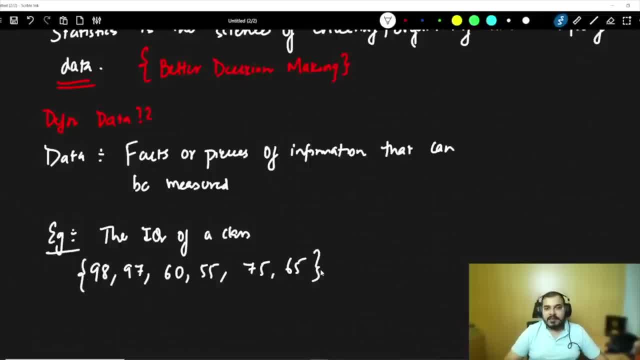 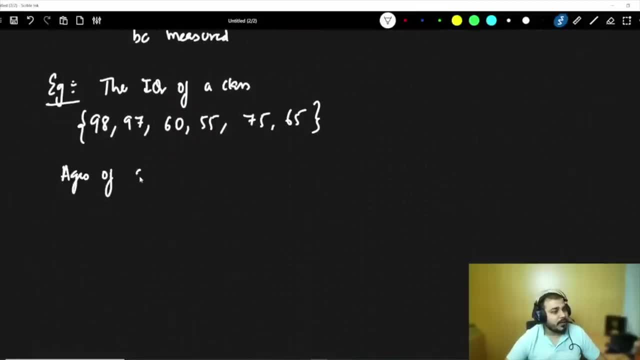 data Here we can basically measure, and the example is IQ of a class. Suppose I want to give one more example. Okay, the age, the ages of student of a class. I may have different ages, like 30,, 25,, 24,, 23,, 27,, 28.. What is this? This is specifically. 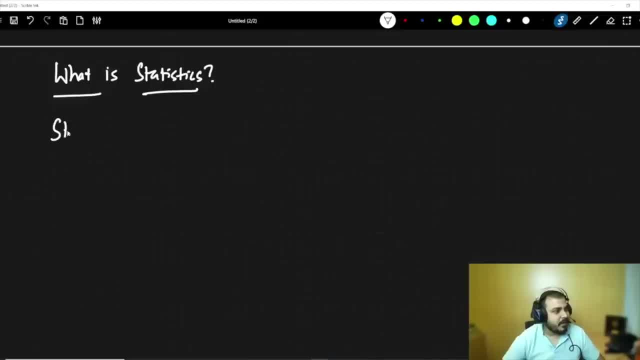 give a very simple definition, which is from Wikipedia. so I'm going to say statistics is the science of collecting, organizing and analyzing data. now you know, based on the amount of data that is getting generated, now you can just understand directly, like, how important stats is. You have tons and tons of. 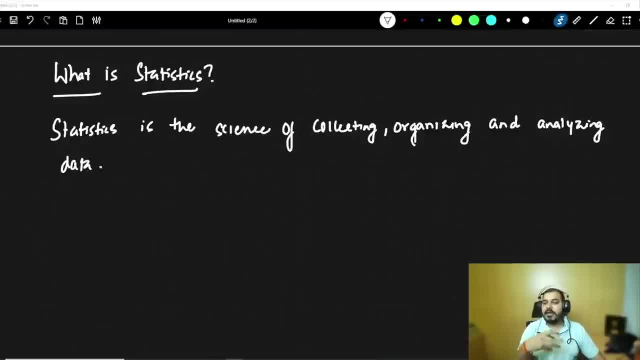 data. you have huge amount of data and definitely you can actually utilize this particular data to make sure that there is improvement in your products, there is improvement in your business goals, and that actually helps you to finally make a very good decision. so, finally, what? why we are doing this for. 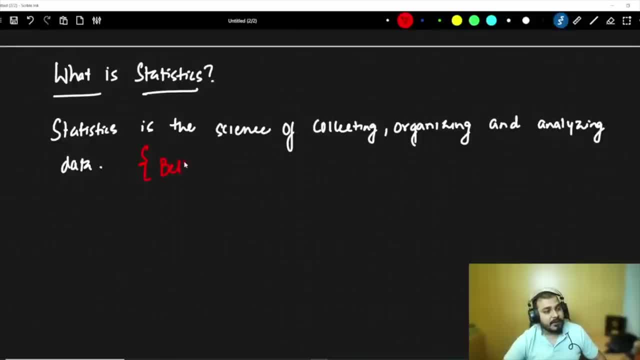 why we are doing this. we are doing this for better decision-making. so we are specifically doing this for better decision-making. everything that is basically getting covered on this. and if I try to now define statistics or the types of statistics, first of all there is one very important thing which is called as data. so data. 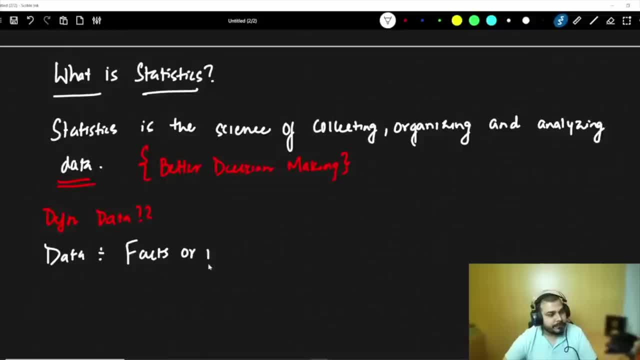 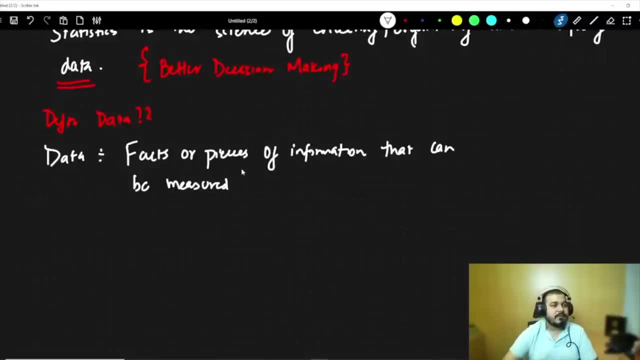 over here is nothing but facts or pieces of information that can be measured. so what is data in short? of facts or pieces of information that can definitely be measured, and let's go ahead and let's see some of the examples. what do you think about data? definitely. 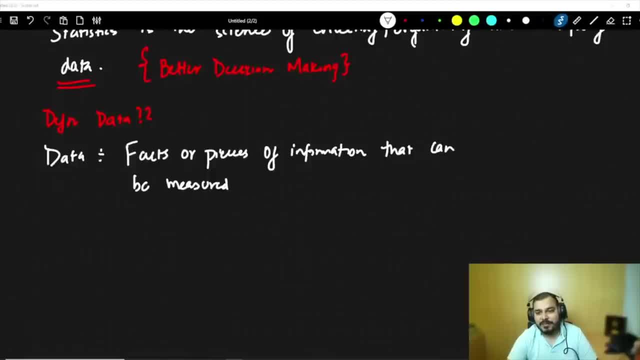 if I, if I say that, okay, let's, let's consider one very simple example. I am basically going to say that, fine, with respect to the data, I can give you some lot of examples. so one example: I can say that let's see if I want to measure the. 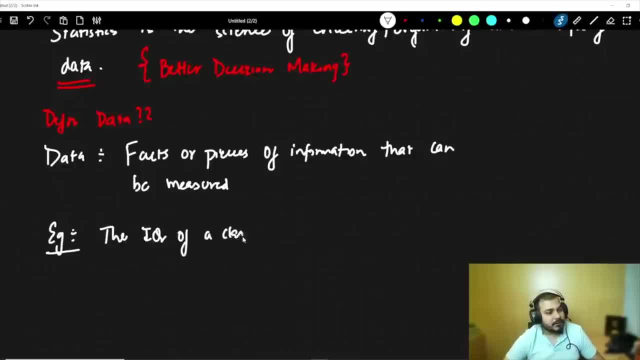 IQ of a class of the students. right, I want to measure the IQ of the students of the class, so I may probably get values between 0 to 100. suppose let's say that I am getting this one, I'm getting this, I'm getting 55, I'm getting. 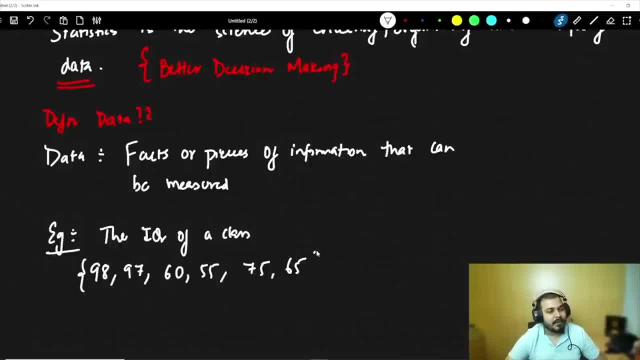 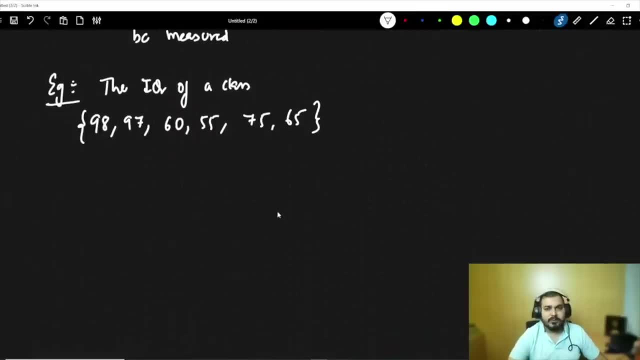 75, I'm getting 65. So this is one example of data here we can basically measure, and the example is IQ of a class. suppose I want to give one more example. okay, the age, the ages of student of a class. I may have different ages, like 30, 25. 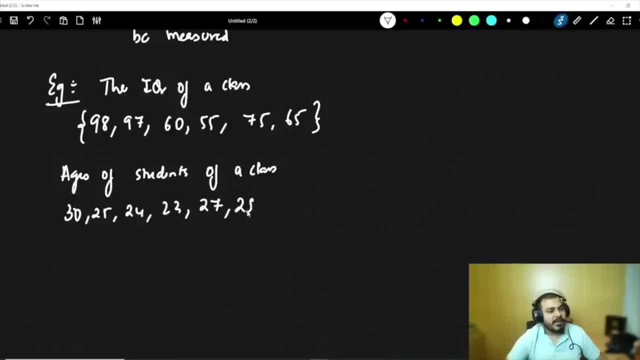 24, 23, 27, 28. what is this? this is specifically data, and always remember the most intrinsic meaning of data is that it can be measured. that is the most important thing. types of statistics and, third of all, it can be measured. if a specific mass is luckily measured, it does appear to have a potential which 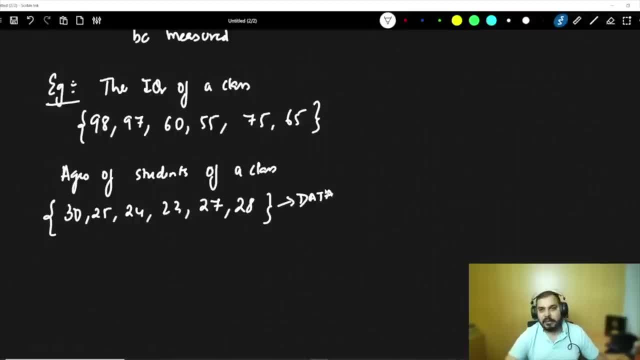 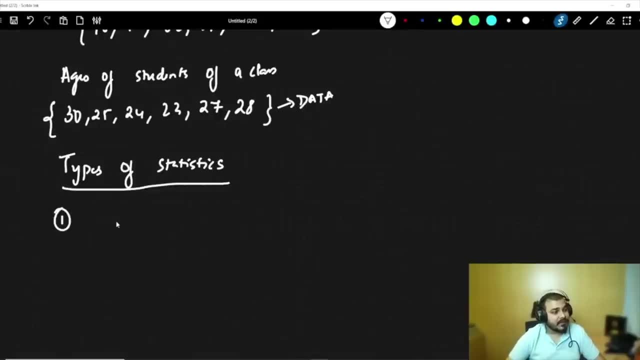 data and always remember the most intrinsic meaning of data is that it can be measured. That is the most important thing. Types of statistics: The first type, as I said, is called something called as descriptive, So the first type is basically called as descriptive stats. Now, how do you define descriptive stats? 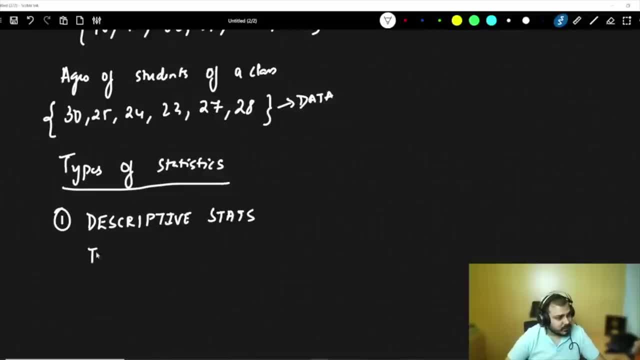 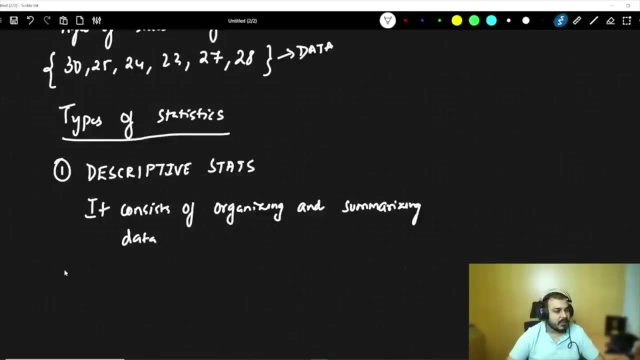 Descriptive stats. I'll just say that it consists of organizing and summarizing of data. It consists of organizing and summarizing data. That's it Very simple, If I really want to understand. I'll probably make you understand more about what is descriptive stats, but let's go. 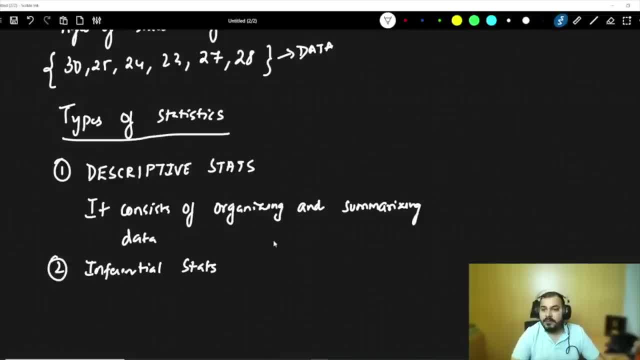 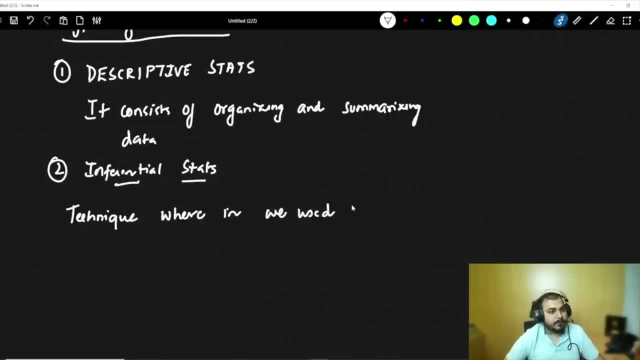 towards the definition of influential stats. Now, the influential stats? you can basically say that it is. it is a technique wherein we use the data that we have measured to form conclusions. Now, if I talk about two important things, One is conclusion and one is about data. 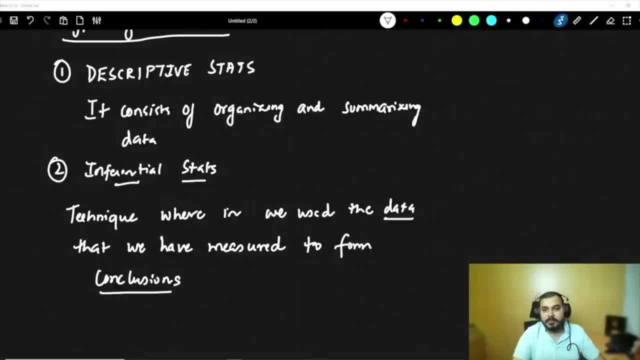 First of all, we will understand about descriptive stats and then probably, I'll give you a very good example. Okay, I'll try to give you a very good example And, based on that particular example, what is the type of question that may come up in descriptive stats? So let's let's consider that. 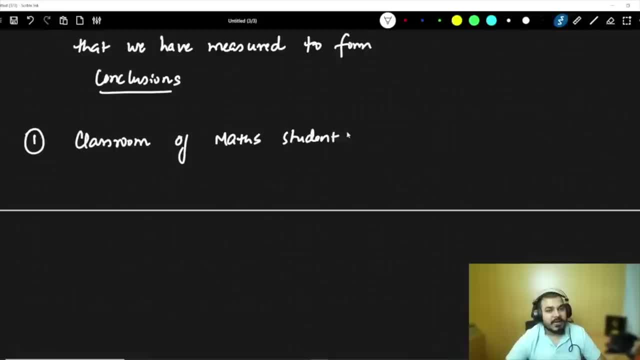 I have a classroom of math students and in this classroom let's consider that there are around 20 people. And now I want to find out the marks. marks of the first sem, let's say Now here probably, the marks with respect to percentage are like this: 84,, 86,. 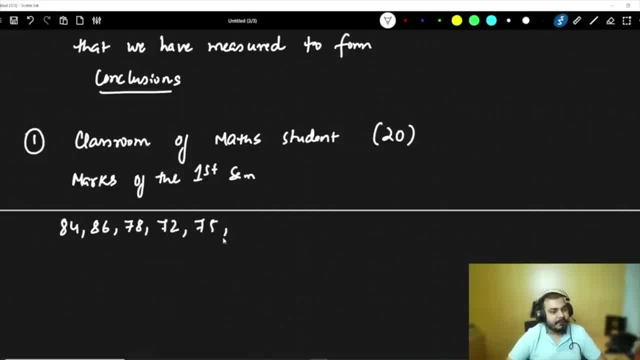 78,, 72,, 75,, 65,, 80,, 81,, 92,, 95,, 96,, 97. So over here you can see how many data are there: 1, 2, 3,, 4,, 5,, 6,, 7,, 8,, 9,, 10,, 11, 12.. Let's consider that we have around 20 data. What is the average? 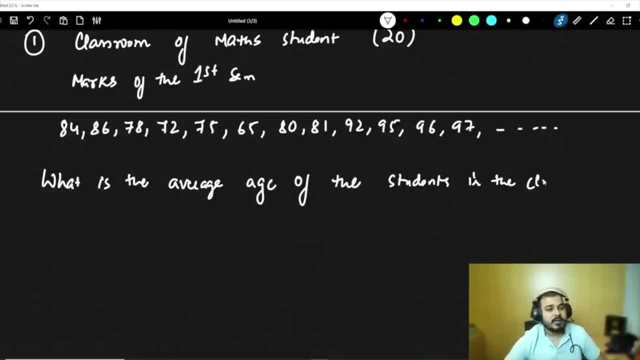 age of the students in the class. student in the class. So this may be a perfect example of descriptive stats. Now, here I've just told about the average. It can be anything. It can be standard deviation, It can be mean, it can be mode, It can be different. 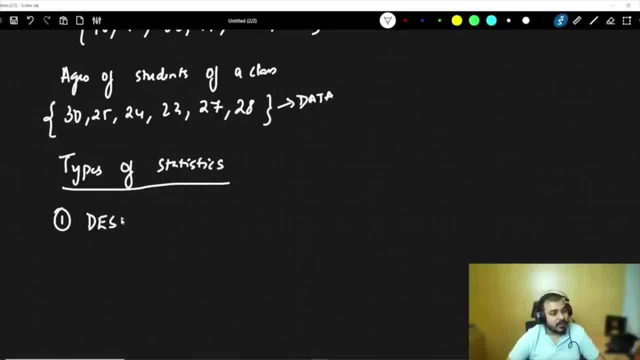 statistics. the first type, as i said, is called something called as descriptive, so the first type is basically called as descriptive stats. now, how do you define descriptive stats? descriptive stats? i'll just say that it consists of organizing and summarizing of data. it consists of organizing and 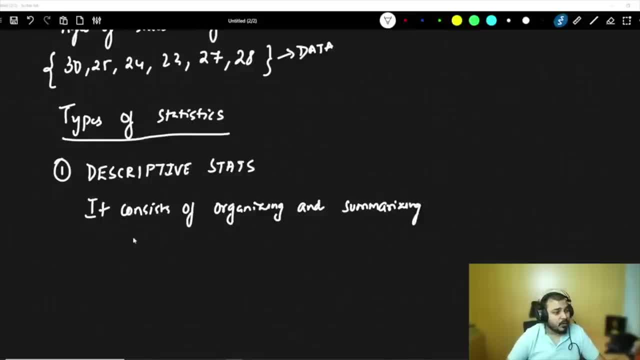 summarizing data. that's it very simple. if i really want to understand, i'll probably make you understand more about what is descriptive stats, but let's go towards the definition of inferential stats now. in inferential stats, you can basically say that it is. it is a technique. 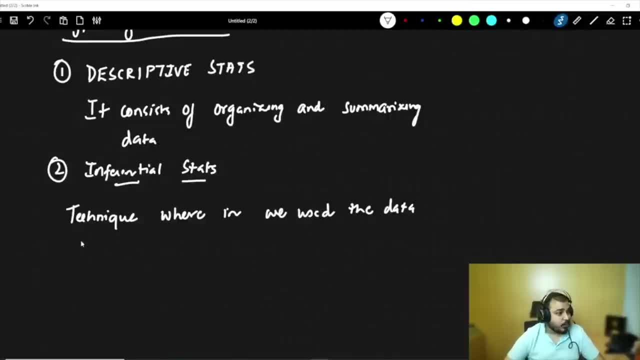 wherein we use the data that we have measured to form conclusions. now, if i talk about two important things, one is conclusion and one is about data. now, first of all, we will understand about descriptive stats and then probably- and i'll give you a very good example, okay, 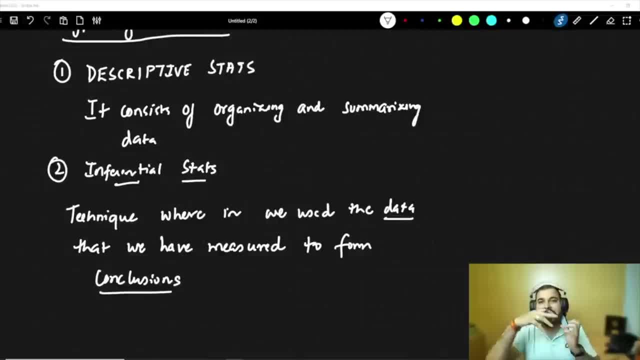 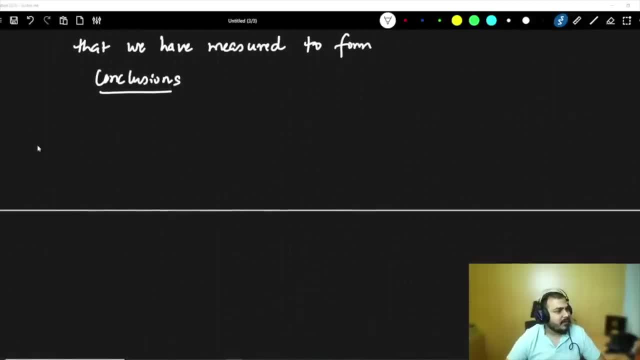 i'll try to give you a very good example and, based on that particular example, what is the type of question that may come up in descriptive stats? so let's let's consider that i have a classroom of math students and in this classroom, let's consider that there are around 20 people. 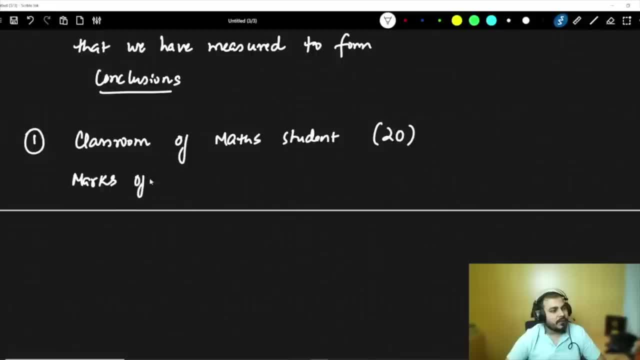 and now i want to find out the marks, marks of the first stem, let's say now, here, probably, the marks with respect to percentage are like this: 84, 86, 78, 72, 75, 65, 80, 81, 92, 95, 96, 97. so over here you can see how many data are there: 1, 2, 3, 4, 5, 6, 7, 8, 9, 10, 11, 12. 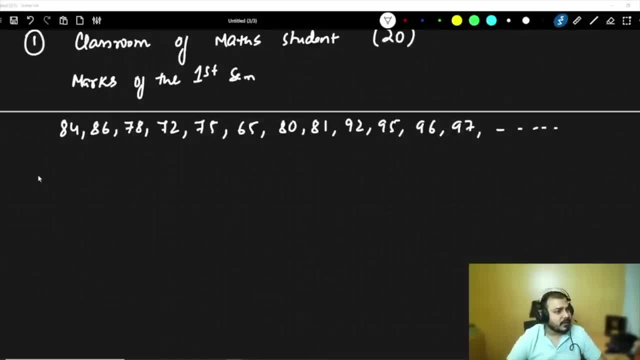 let's consider that we have around 20 data. what is the average age of the students in the class? student in the class. so this may be a perfect example of descriptive stats. now here i've just told about the average. it can be anything. it can be standard deviation. 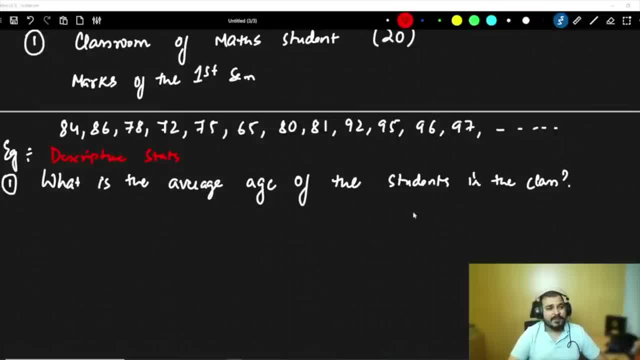 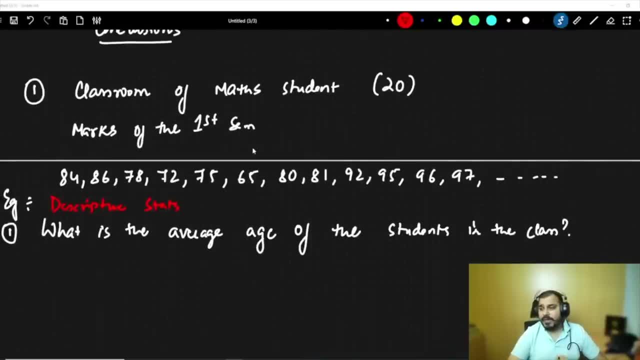 it can be mean, it can be mode, it can be different, different things. so here you can see that i've taken a very simple example. i have, uh, our math students- like 20 people over here and probably you can basically understand over here that we are trying to find out what is the average age. 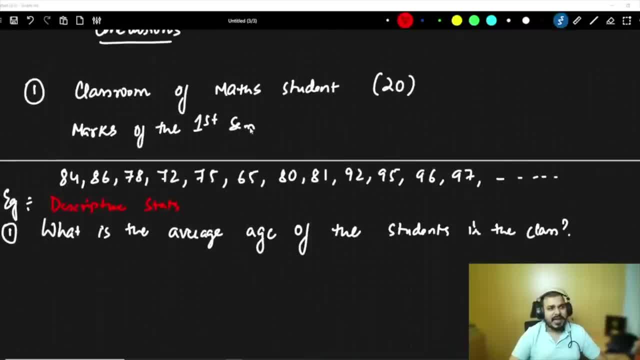 different things. So here you can see that I've taken a very simple example. I have our math students- like 20 people over here And probably you can basically understand. over here we are trying to find out what is the average age of the student in the class. You may also say that: 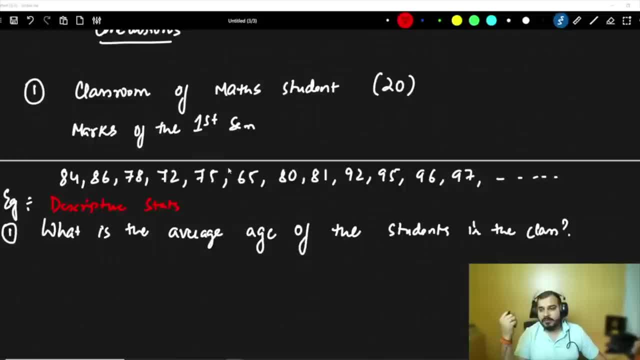 what is the percentage of the people passing out from the class? You can also say that different, different examples. probably you'll be able to understand when I talk about percentiles and all. Now let me go ahead and let me find out and let me tell you the other example of. 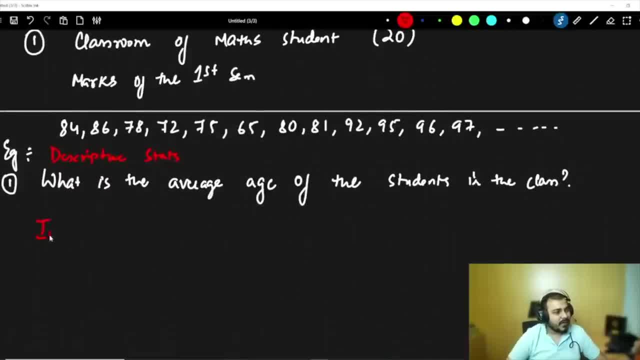 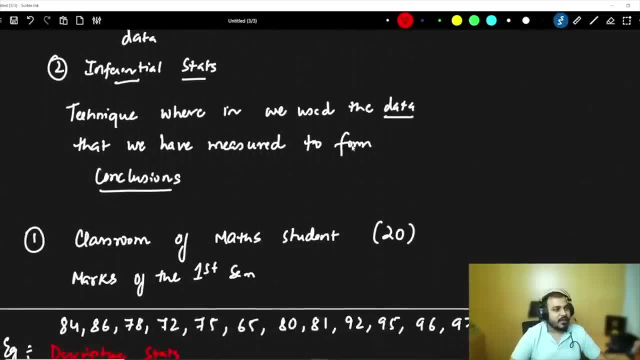 inferential stats Based on this, what kind of thing, what kind of question you can ask with respect to inferential stats? I've told you the definition: what? what inferential stats, what kind of inferential stats, what kind of inferential stats, what kind of inferential stats? 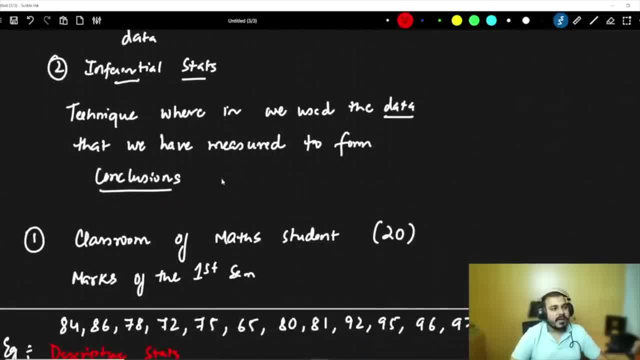 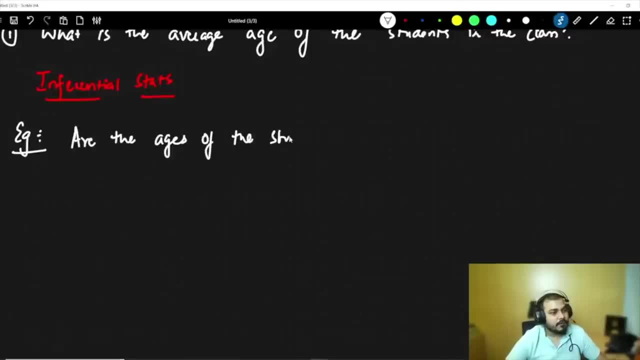 basically consists of. it is a technique wherein we use the data that we have measured to form conclusions. I may say that are the ages of the students of this classroom similar to the age of the college? similar, and that's the age of the college, but age of the maths classroom in the 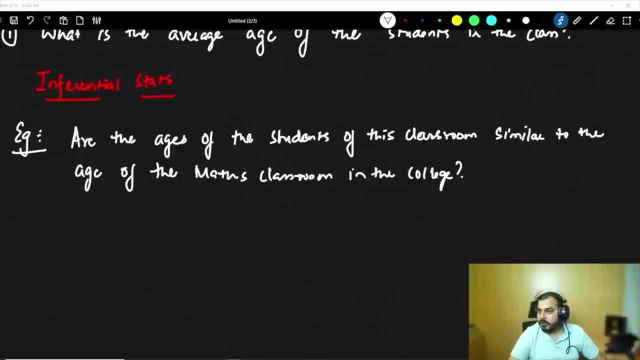 college. So this is basically my question. My question basically says that are the ages of the students of this classroom similar to the age of the maths classroom in the college? So here maths classroom in the entire college is my population And probably just a classroom student's age is just. 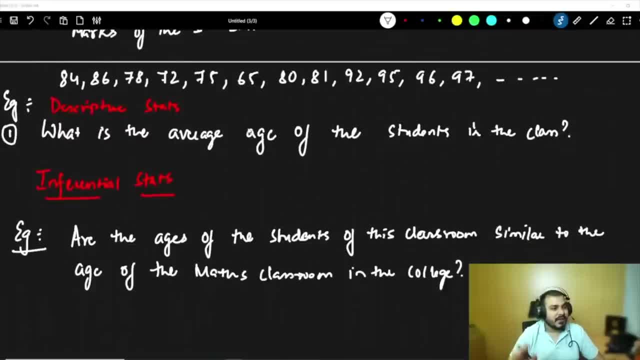 like my sample. Sorry, did I discuss about maths? Okay, sorry, I'll not say age, but average marks. I'll just try to change over here. Just a second, guys. I'm extremely sorry. So this is not age. 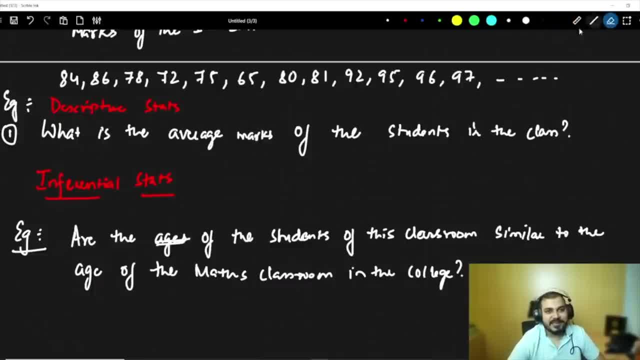 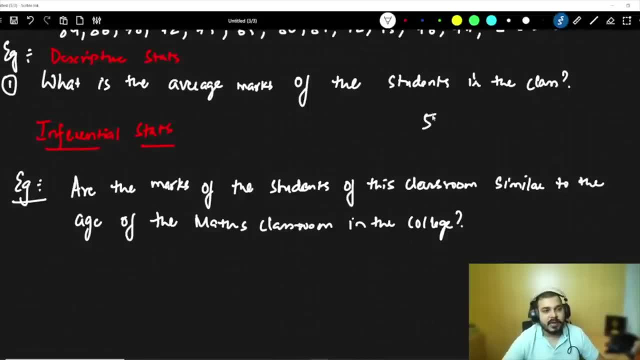 this is marks, So I'll not say This as ages, let me, but you can also take ages as an example. I will say it as marks, Like that. let's consider the maths classroom. There are different, five different classrooms, and I've 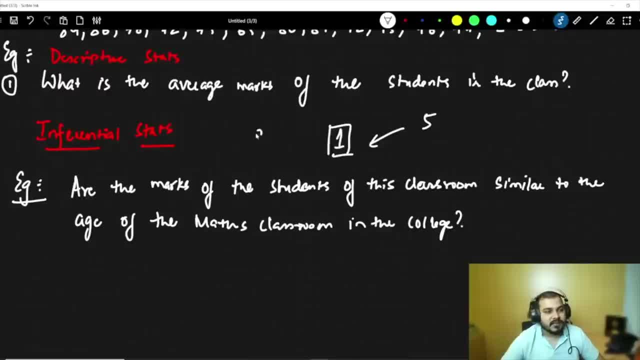 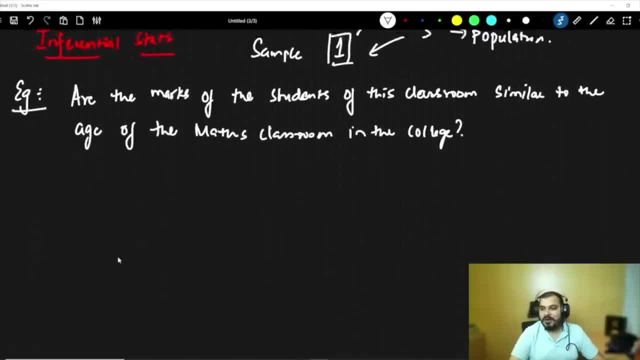 actually taken the data of only one classroom And from this this is basically called a sample And this is my entire population. Now, since we have discussed about population and sample, and I'll be coming more on making you understand about descriptive when we are deep diving into 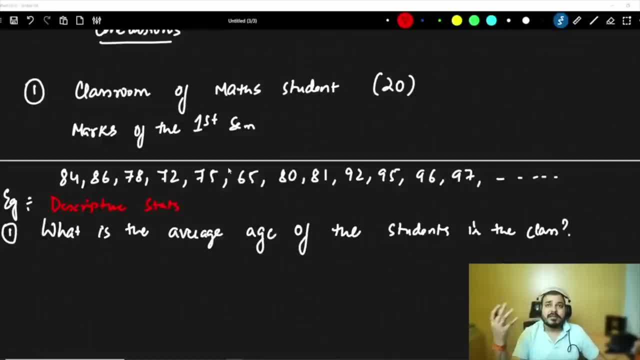 of the student in the class. you may also say that: what is the percentage of the people passing out from the class? you can also say that different, different examples. probably you'll be able to understand when i talk about percentiles and all. now let me go ahead and let me find out and let me tell you the other example of. 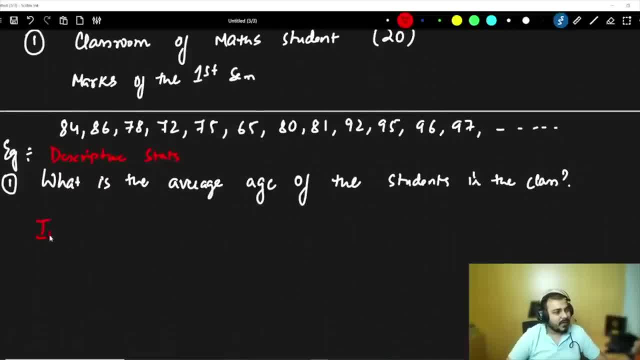 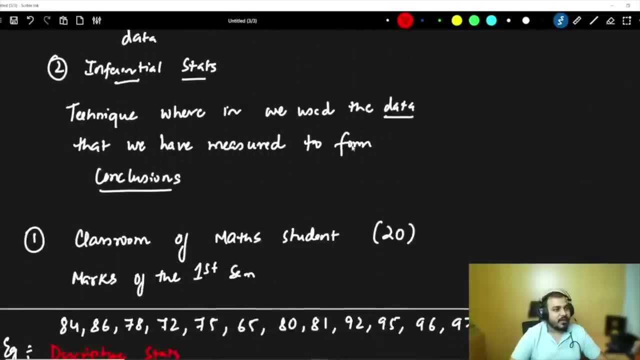 inferential stats based on this, what kind of thing, what kind of question you can ask with respect to inferential stats? i've told you the definition: what what inferential stats basically consist of. it is a technique wherein we use the data that we have measured to form conclusions. i may say that 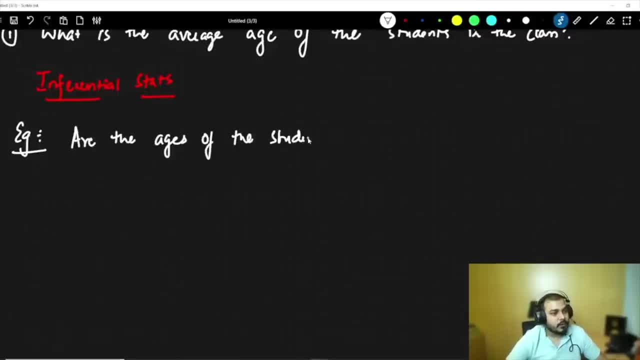 are the ages of the students of this classroom similar to the age of the college? familiar, and it's an age of the college, but delivery �翻역 since 2019 age of the math classroom in the college. so this is specifically my question. 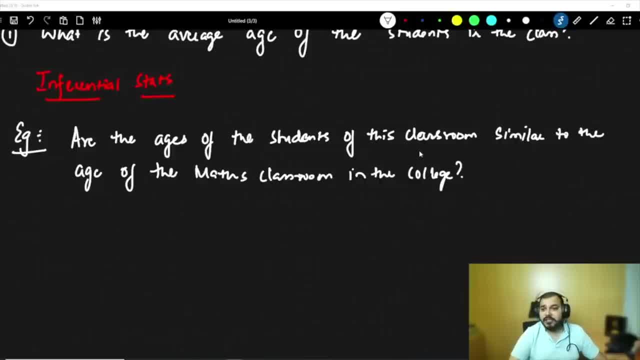 my question basically says that are the ages of the student of this classroom similar to the age of the maths classroom in the college. so here, maths classroom in the entire college is my 所以现在 m制 Still twelve students who school in my school population And probably just a classroom student's age is just like my sample, Sorry. 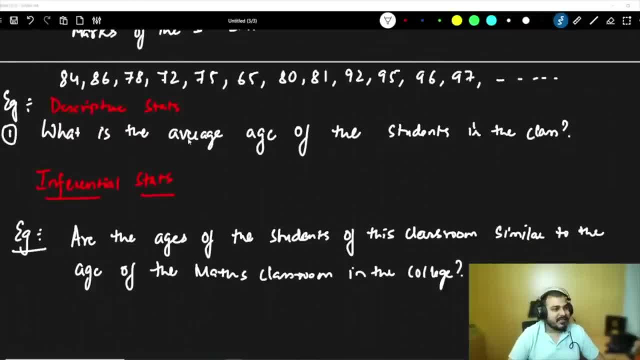 did I discuss about maths? Okay, sorry, I'll not say age, but average maths. I'll just try to change over here. Just a second, guys, I'm extremely sorry. So this is not age, this is maths. So I'll not say this as ages, But you can also take ages as an example. I will say it as: 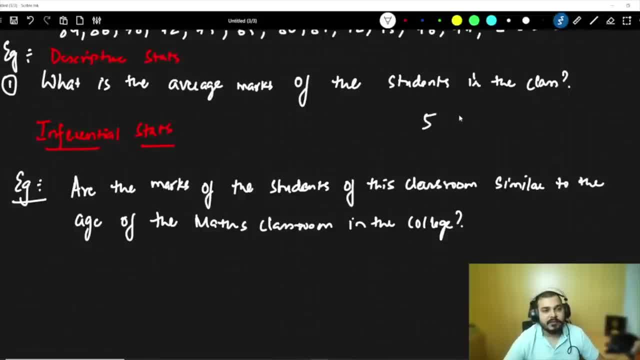 Like that. let's consider the maths classroom. there are different, five different classrooms, and I've actually taken the data of only one classroom And from this this is basically called a sample, And this is my entire population. Now, since we have discussed about population and 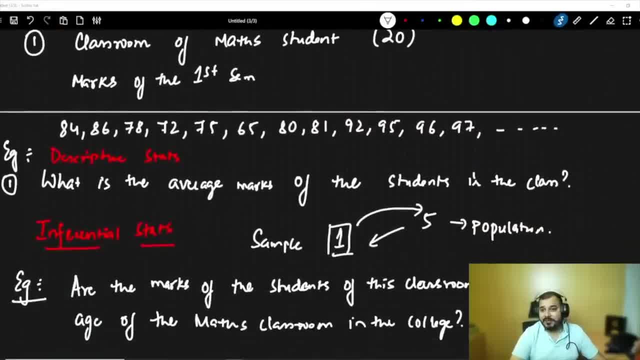 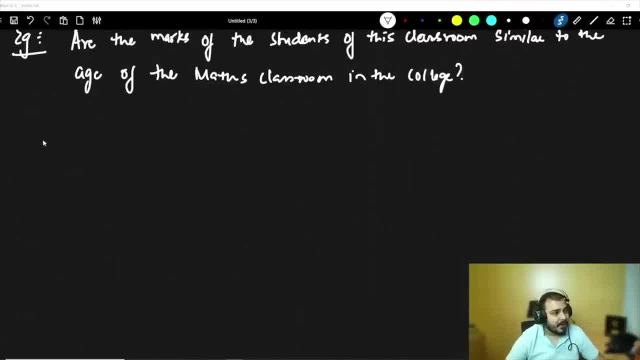 sample, and I'll be coming more on making you understand about descriptive when we are deep diving into various topics. Now it is time that we really understand about population and samples. So coming over here is basically population and sample. What exactly is population? Now, population basically means: let's consider one. 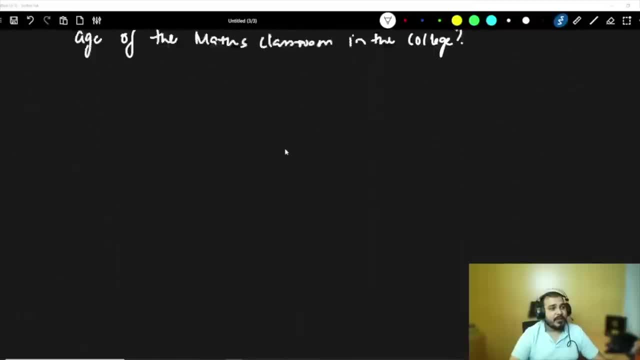 various topics. Now it is time that we really understand the difference between the two. So let's start with population and sample. So coming over here is basically population and sample. What exactly is population? Now, population basically means? let's consider one example. 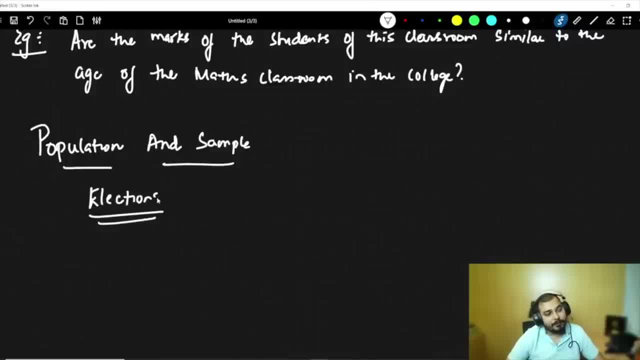 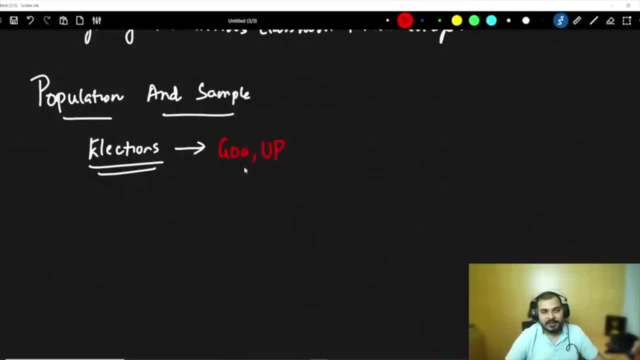 you may be talking about Goa, you may be talking about UP. Let's consider this two states. So obviously it is not possible. Probably, let's consider that the election has finished And we really need to find out the exit poll. Now, exit poll: what usually this press, reporters and 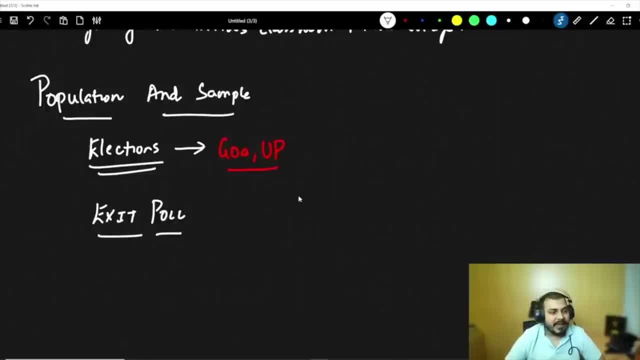 all will do. what they will do is that they cannot go and ask each and every person. Suppose the Goa population is this big. Let's consider It is not possible for every reporter to go and ask each and every person. Let's consider It is not possible for every reporter to go and 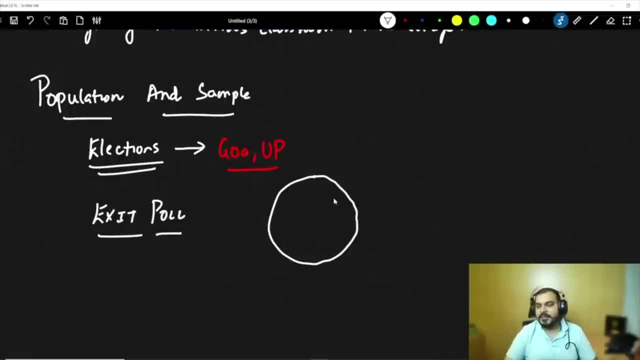 ask each and every person that whom you have voted, because it is not possible. You may not find some people, some people may be traveling, some people may be doing different, different things at all. So it is not possible at all. So what happens in this exit poll? this reporters. 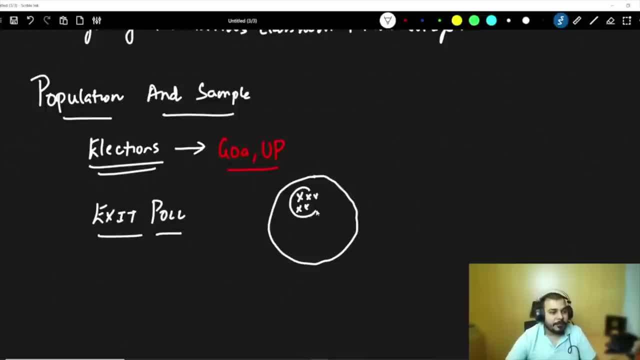 what they do is that they take up sample of population from different, different region- And again they are different, different kinds of sampling techniques. They take up different, different samples, And then what they do is that they ask that: whom did you vote? 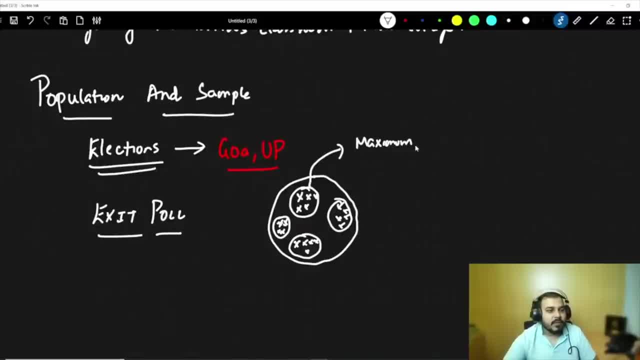 And, based on that maximum number of people, whom did they vote? They basically say: based on that, they actually create their exit poll. Now, in this particular case, what is my population data? My population data is this entire population of Goa. So this specifically thing is my population data And this round circles that I have actually 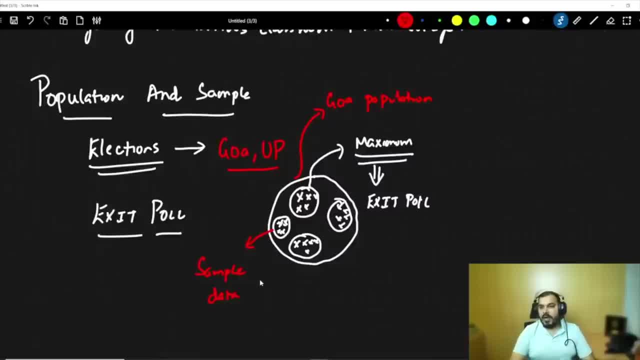 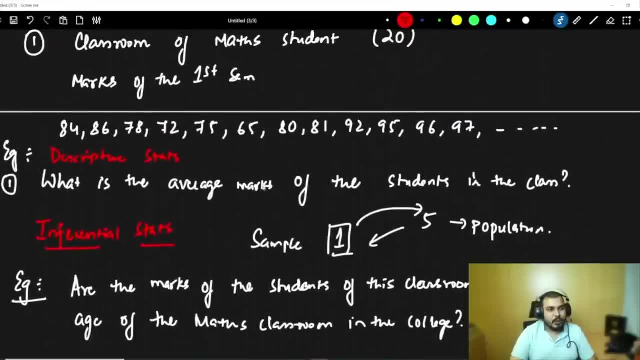 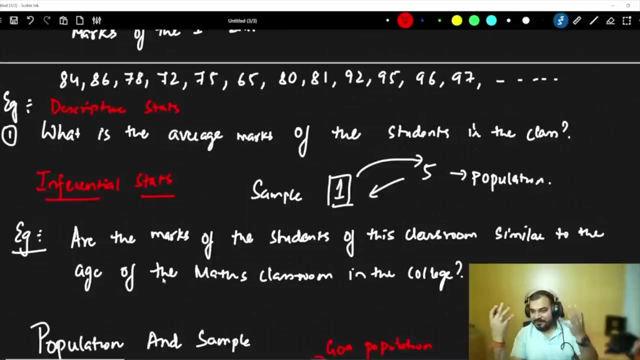 done is basically my sample data, So I hope you have basically got some, some examples with respect to that. Guys, I hope everybody's clear with this. I basically told age over here, So don't get confused. Sometime When I'm teaching, sometimes students may come, ages may come or marks may come, So you'll not get. 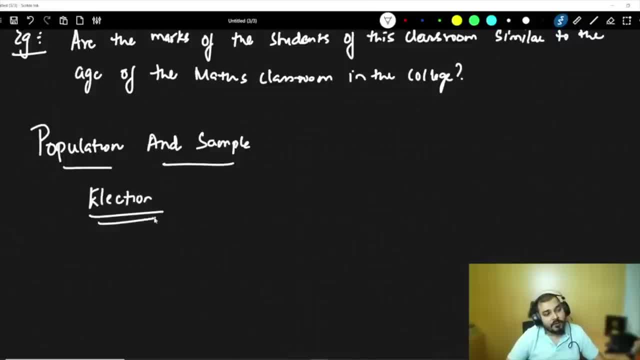 example again. See, guys, I will definitely give you a lot of examples. The reason why I'm giving you examples is that because understand, if we learn statistics in such a way that we have examples in mind, we will be able to explain the interviewer in a very good way. So let's take an 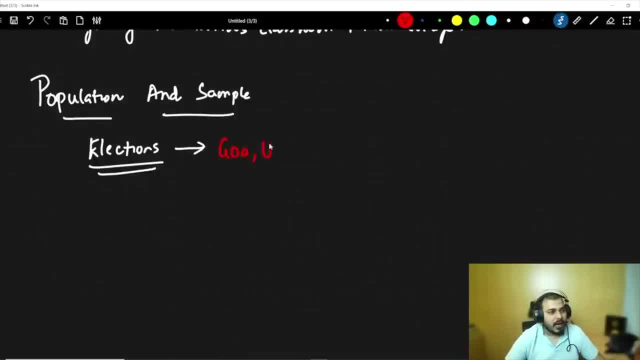 example of elections. Probably you may be talking about Goa, you may be talking about UP. Let's consider this two states. So obviously it is not possible. probably let's consider that the election has finished And we really need to find out the exit poll. Now, exit poll- what usually this press, reporters and all 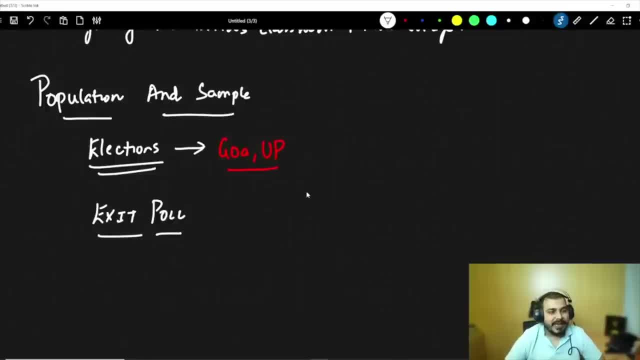 will do. what they will do is that they cannot go and ask each and every person. suppose the Goa population is this big, Let's consider. it is not possible for every reporter to go and ask each and every person that whom you have voted, because it is not possible. you may not find some person who is. 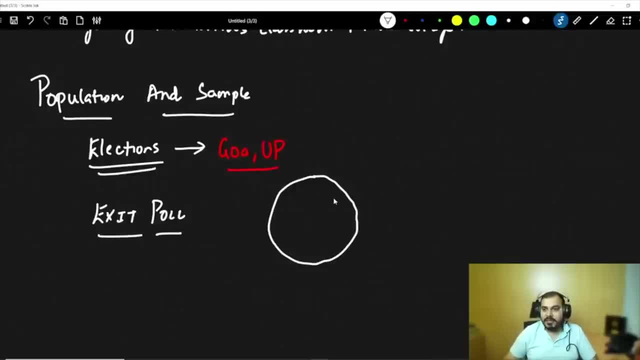 voting some people, some people may be traveling, some people may be doing different, different things, and also it is not possible at all. So what happens in this exit poll? this reporters? what they do is that they take up sample of population from different, different region, And again they are. 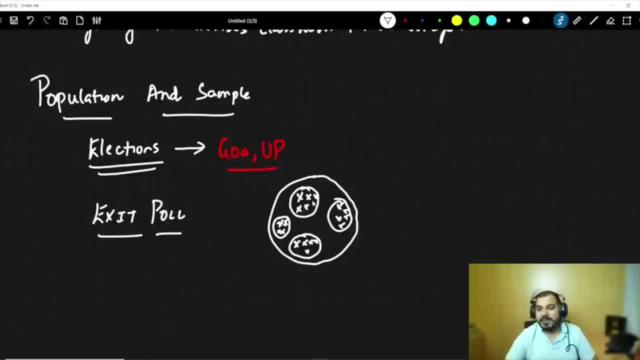 different, different kinds of sampling techniques. they take up different, different samples And then what they do is that they ask that whom did you vote? And based on that maximum number of people, who, whom did they vote? they basically say: based on that, they actually create their exit poll Now in. 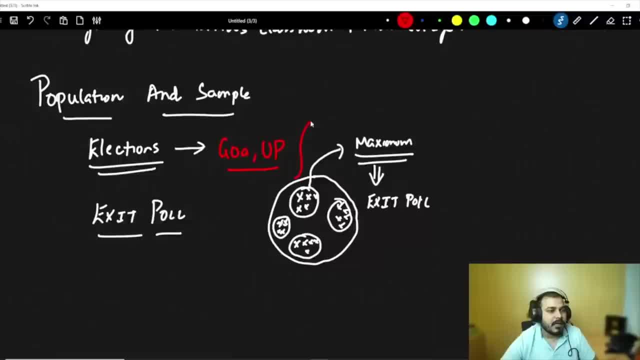 this particular case, what is my population data? my population data is this entire population of Goa. So this specifically thing is my population data And this round circles that I have actually done is basically my sample data. So I hope you have basically got some, some examples, with respect. 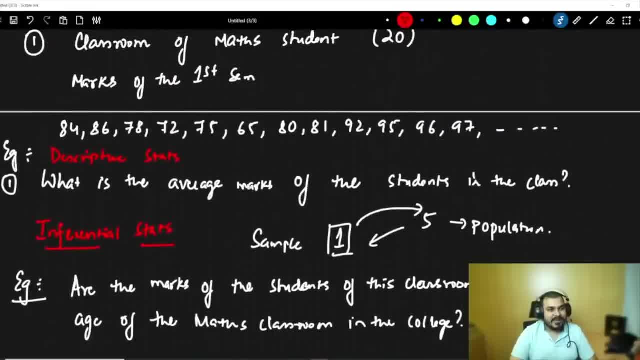 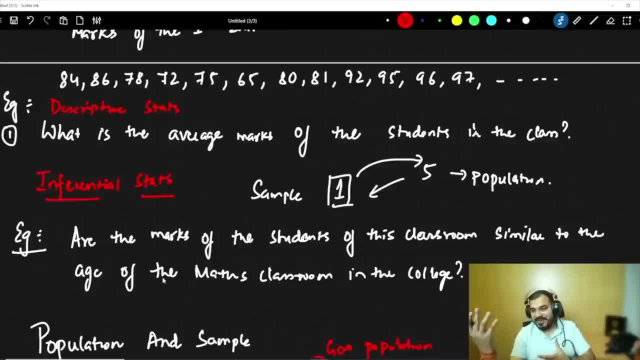 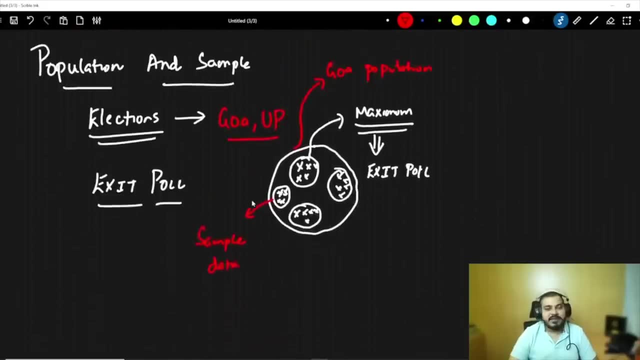 to that. Guys, I hope everybody is clear with this. I basically told age over here, So don't get confused. Sometime when I'm teaching, sometimes students may come, ages may come or marks may come, So you'll not get confused, Don't worry. So here is one example. Now let's go ahead and let's try to. 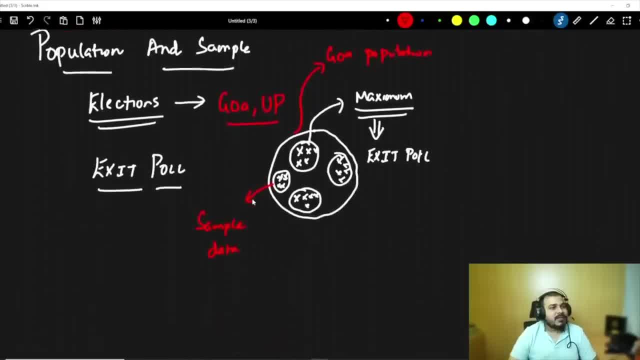 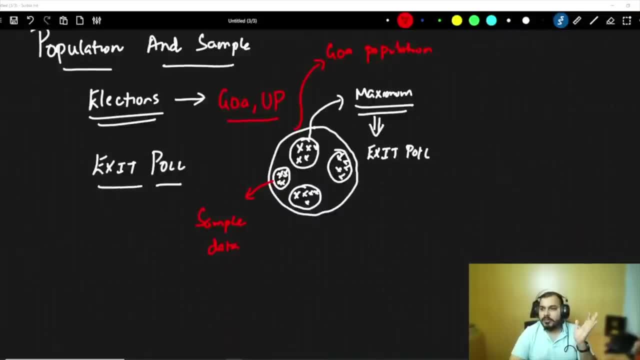 confused, Don't worry. So here is one example. Now let's go ahead and let's try to understand one thing Now, in this particular scenario, in this particular example- many people have told about Krish- why are you just considering- okay, you're considering- samples to solve a particular 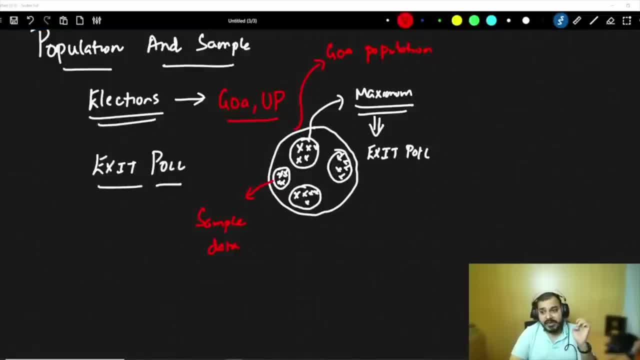 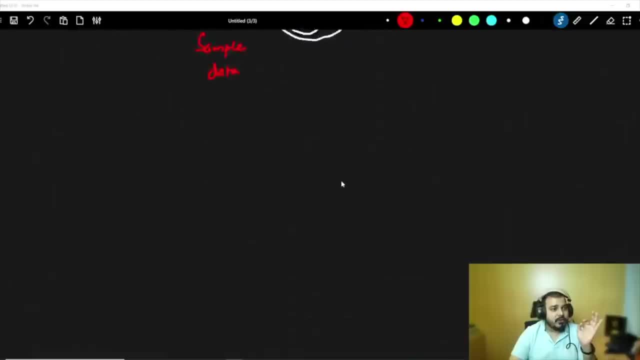 problem. What are the different sampling techniques? You nearly need to understand or tell us that, because they are different. different sampling techniques. What are the different kinds of sampling techniques? But before I go ahead, usually population. if I talk about population, you 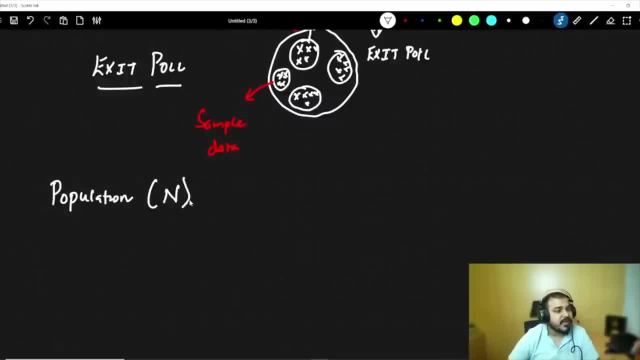 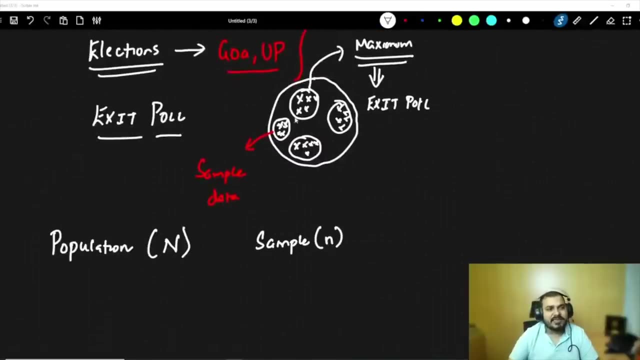 really need to understand about some of the notation. Population is basically given by capital N, and sample is basically given by small n. So this is how we basically denote population. This is how we basically denote sample. Now the next question comes, that Krish, why you have selected. 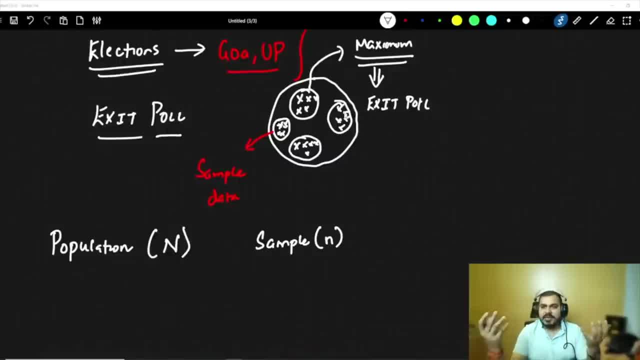 samples randomly. Is there any better ways to do sampling also, or just we need to? we need to do the sample randomly. I would like to say that, guys, this entire sampling takes place based on various scenarios, And for that I will be showing you some of the examples. So let's go and 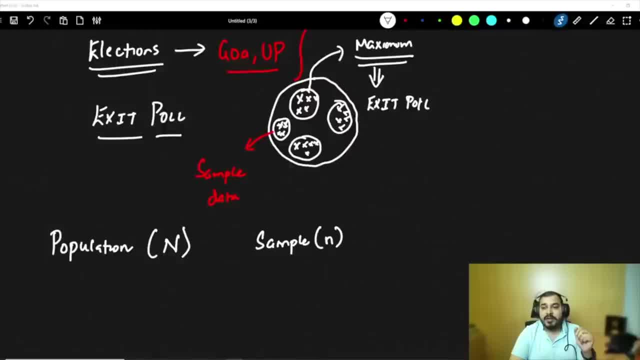 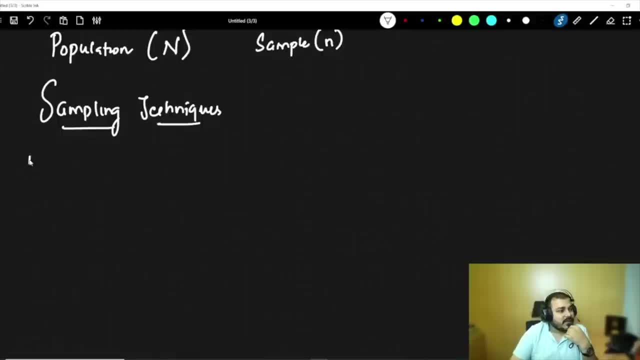 understand about some of the sampling techniques and what are different different sampling techniques. we basically have The first sampling techniques. let me write it down for you Now. the first sampling techniques which is most of the time used. it's called a simple random. 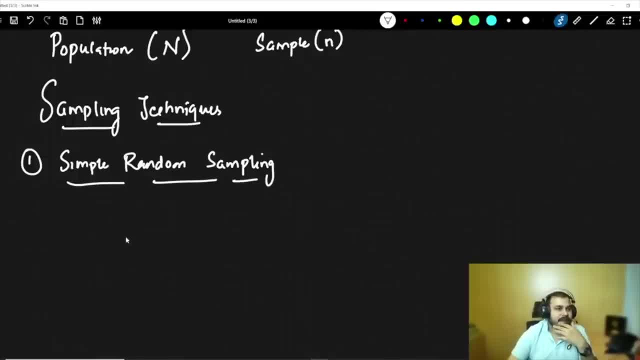 sampling: Simple, random sampling. very simple, very important. Suppose I have some data, I have some, I'm sorry- I have some population. Suppose this is my population: simple, random sampling will be just like you go and pick up some people like this, anyhow you want, There is no. 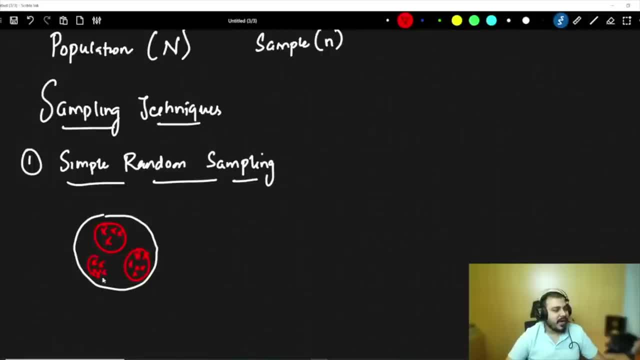 there is no such confusion as such. You just go and randomly pick up people- Simple, random sampling- and simple random sampling is basically used in many of the scenarios, probably in exit scenarios. You can use simple random sampling, Suppose, if you want to use some kind of medicines. 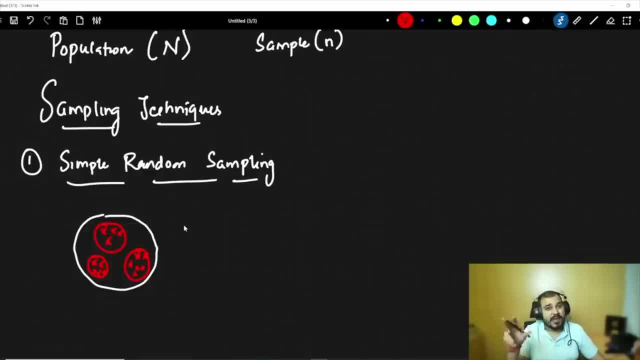 right, You do some kind of test for the medicines. At that point of time you cannot use simple, random, simple, random sampling. You have to pick up some people probably have to check their medical history. Based on that, you have to apply. But simple, random sampling it's all about. I can. 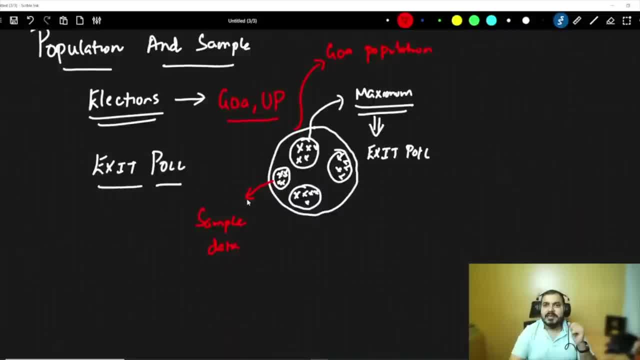 understand one thing Now, in this particular scenario, in this particular example- many people have told about Krish- why are you just considering- okay, you're considering- samples to solve a particular problem? What are the different sampling techniques? You nearly need to understand or tell us that. 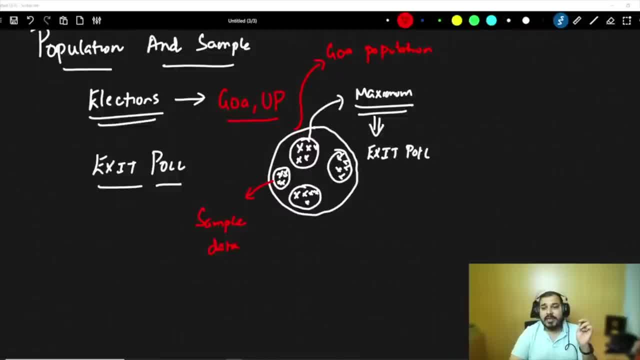 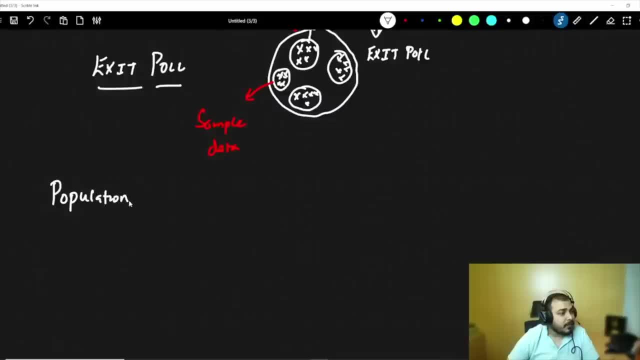 because they are different. different sampling techniques. What are the different kinds of sampling techniques? But before I go ahead, usually population. if I talk about population you really need to understand about some of the notation. Population is basically given by capital N and sample is basically given by small n. So this is how we basically denote population. This: 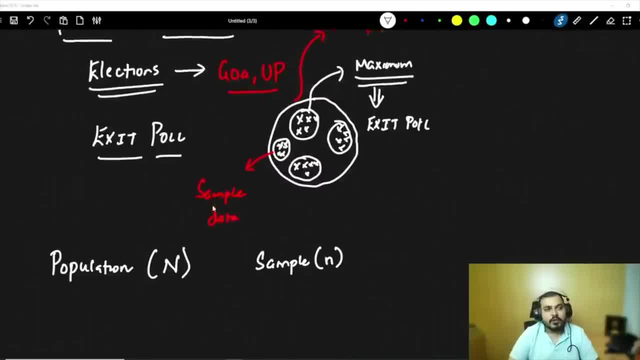 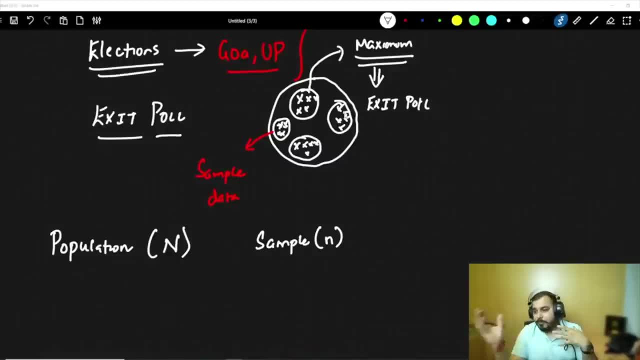 is how we basically denote sample. Now the next question comes, that, Krish, why you have selected samples randomly. Is there any better ways to do sampling also, Or just we need to do the sample randomly? I would like to say that, guys, this entire sampling takes place in the same way, So 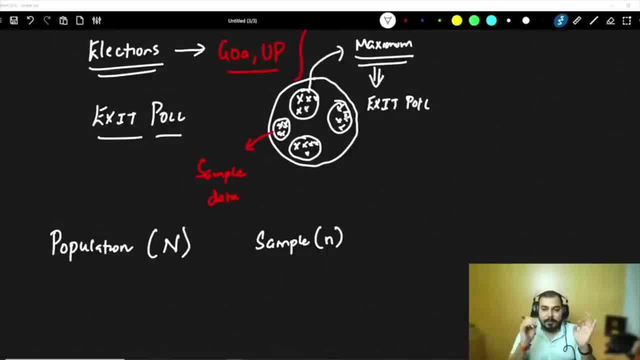 it takes place based on various scenarios And for that I will be showing you some of the examples. So let's go and understand about some of the sampling techniques and what are different, different sampling techniques. we basically have The first sampling techniques. let me write it. 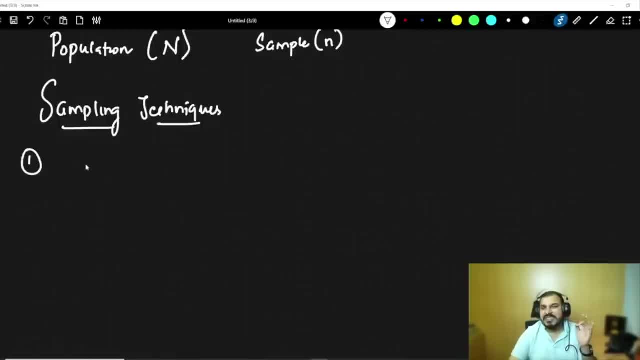 down for you Now. the first sampling techniques, which is most of the time used, is called as simple, random sampling. Simple, random sampling, Very simple, very important. Suppose I have some data, I have some, I'm sorry- I have some population. Suppose this is my population. 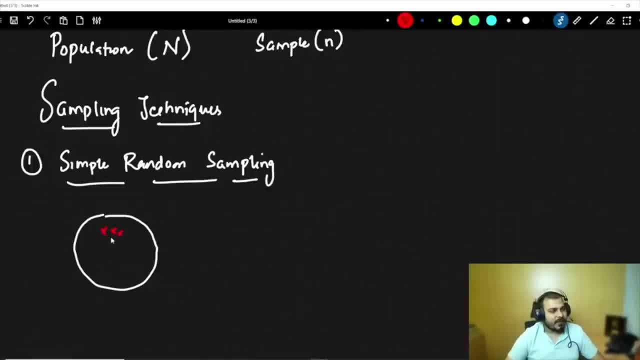 Simple random sampling will be: just like. you go and pick up some people like this, anyhow you want. There is no, there is no such confusion as such. You just go and randomly pick up people- Simple random sampling. And simple random sampling is basically used in many of the scenarios, Probably. 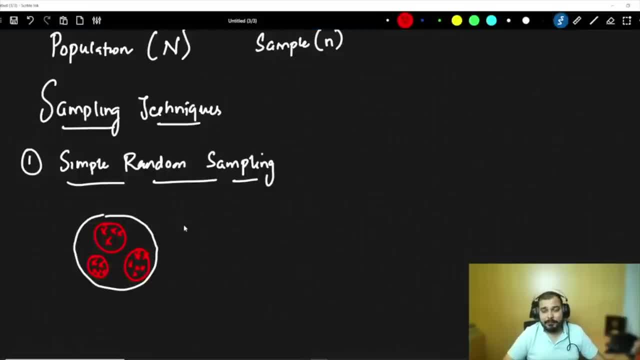 in exit poll you can use simple, random sampling. Suppose, if you want to use some kind of medicines, right, You do some kind of test for the medicines. At that point of time you cannot use simple random, simple, random sampling. You have to pick up some people, Probably. 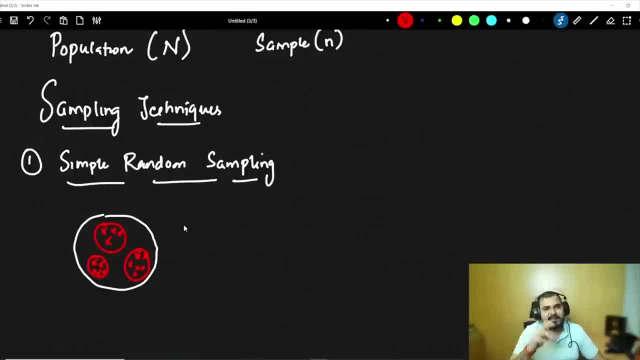 you have to check their medical history. Based on that, you have to apply. But simple random sampling it's all about. I can basically say that I'll just give you a small definition over here. When performing simple random sampling, every member of the population has an equal chance of being. 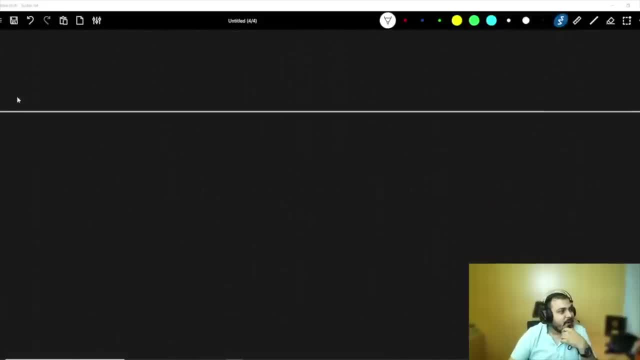 stratified. And now coming to the second type, the second type of sampling is called as stratified sampling. Let's let let me give you a definition. Stratified sampling is a technique where the population, that is, capital N, is split into non-overlapping groups. So one example. I'll be 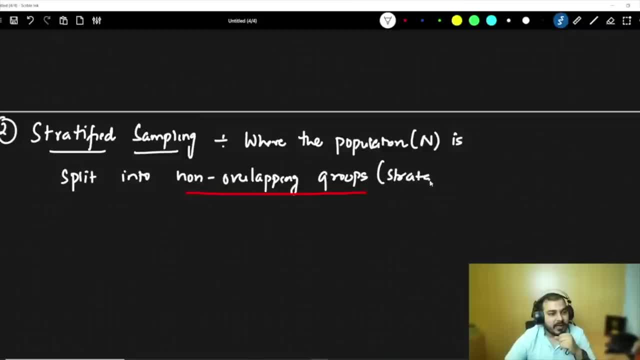 talking about it. Don't worry, This is also called as strata. Strata basically means layering, Stratified layering, like that. we basically say: This is what a stratified sampling basically means. Let me give you one example. Let's let's consider gender. I want to do this sampling based. 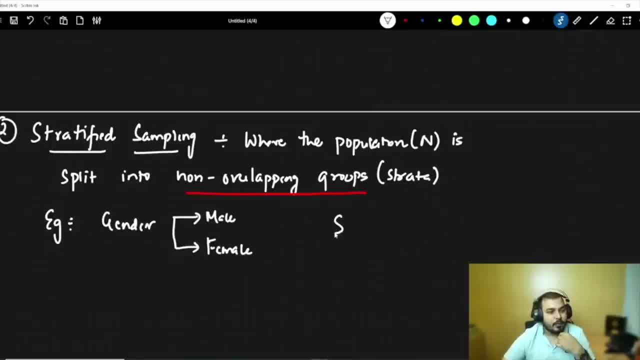 on two things. One is male and female. Let's consider that I want to do a survey And for a survey obviously I will be requiring some people And based on that, my samples will basically be divided right, Based on male and female. Male people will give different kind of a survey. 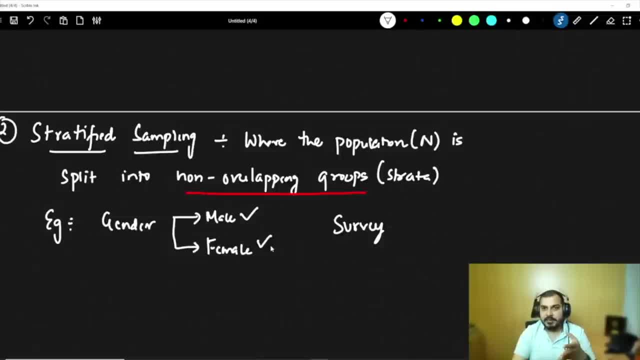 Female people may give different kind of survey. Okay, So something like this. So this is definitely one example. Any other examples that you would like to say? Obviously, wherever you can see that there can be non-overlapping groups, Obviously you can do it. Let me give you one more example. 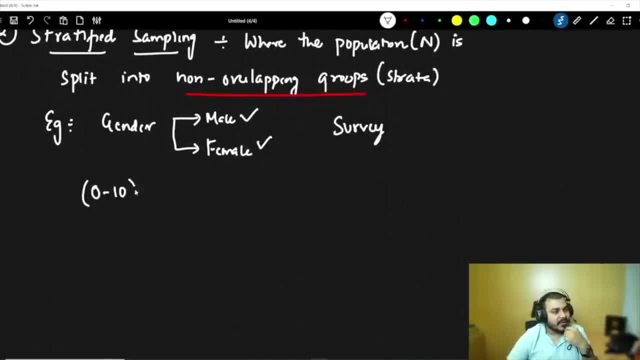 Suppose I want a survey to be done by 0 to 10 years of kids, I want the next probably. I'll try to make this kind of layering based on age. Probably 10 to 20 will be one age group, Probably. 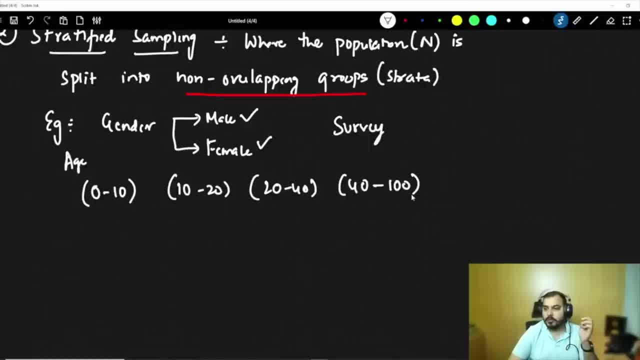 40 to 100 will be another age group, So based on different, different age group. I can also do a sampling. Understand one thing: This terminology is very much important: Non-overlapping. It should not overlap Over here. there is no chance of overlapping Based on profession. can I do? 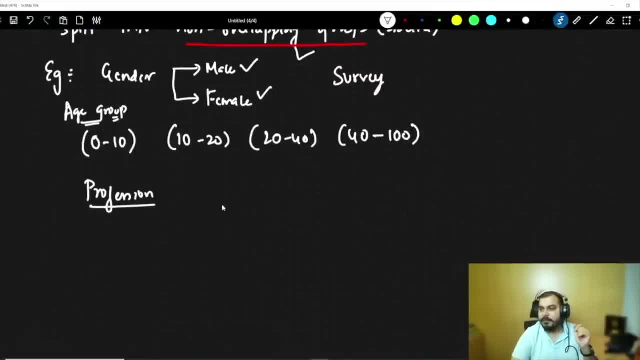 stratified sampling Based on profession. can I do stratified sampling? See, a profession may be that. let's say that this profession is with respect to different, different, different, different people. Suppose a person is a NET developer, A person is a PHP developer, A person is a? you know? 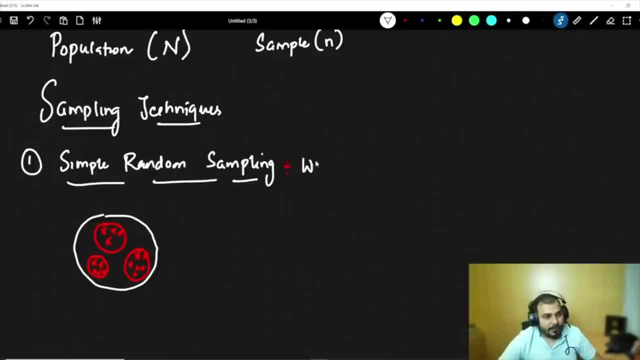 basically say that. I'll just give you a small definition over here. When performing simple random sampling, every member of the population has a certain number of people. every member of the population has a certain number of people. every member of the population has a certain number of. 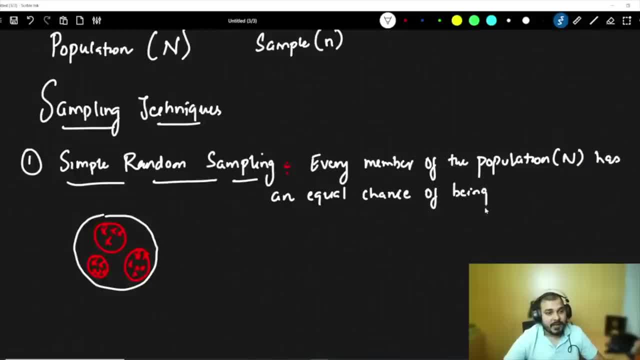 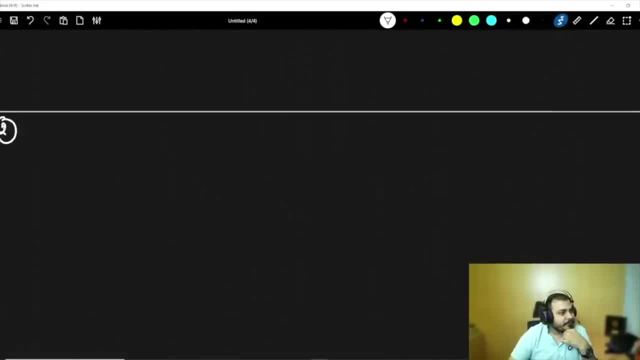 people. every member of the population has an equal chance of being selected for your sample N. Now coming to the second type, The second type of sampling is called as stratified sampling. Let's let let me give you a definition. Stratified sampling is a technique where the population 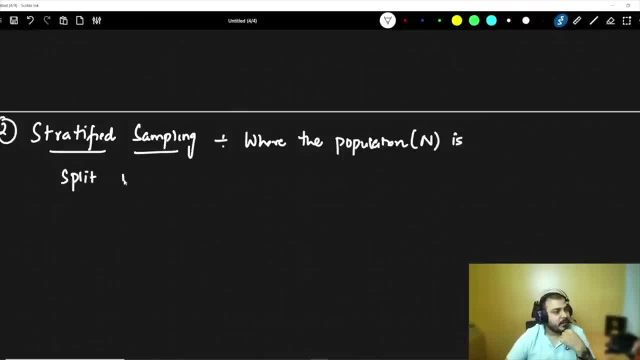 that is, capital N is split into non-overlapping groups. So one example: I'm just talking about it, don't worry. this is also called as strata. Strata basically means layering, stratified layering. like that we basically say: This is what a stratified sampling basically means. 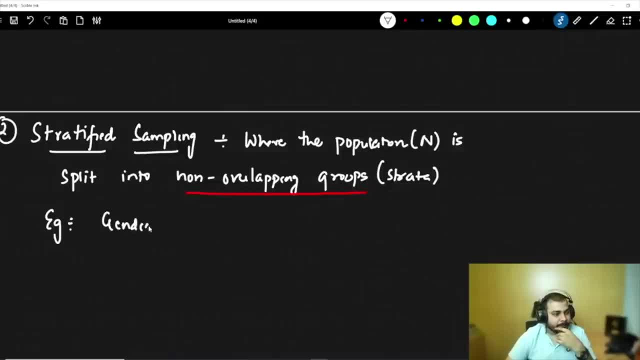 Let me give you one example. Let's let's consider gender. I want to do this sampling based on two things: one is male and female. Let's consider that I want to do a survey and for a survey, obviously I will be requiring some people And based on that, my samples will basically be divided And 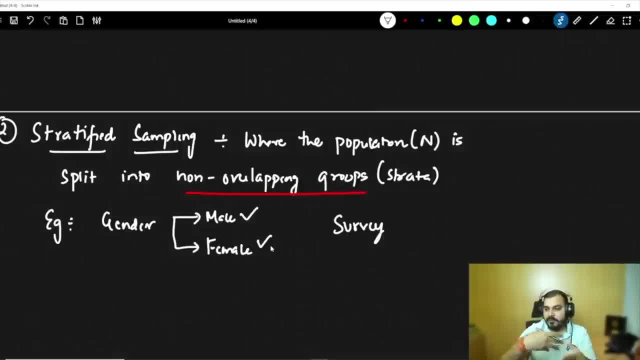 Right Based on male and female. Male people will give different kind of a survey. Female people may give different kind of survey. OK, so something like this. So this is definitely one example. Any other examples that you would like to say? 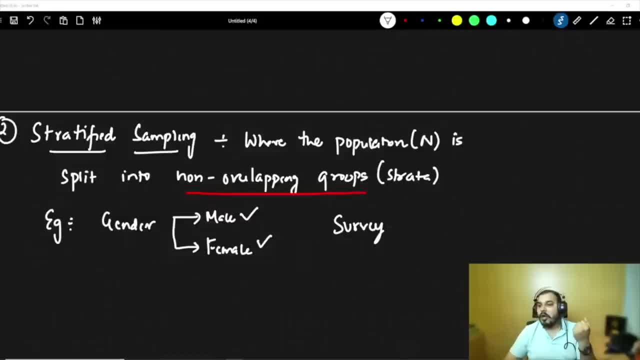 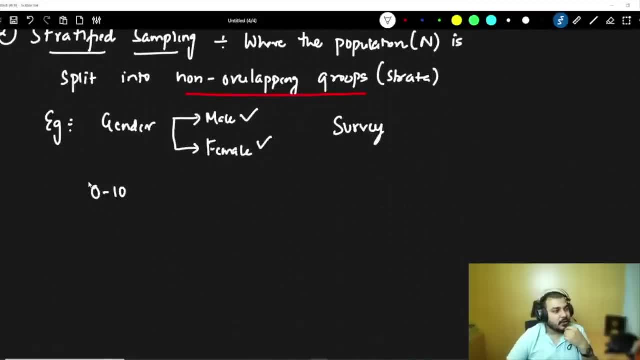 Obviously, wherever you can see that there can be non-overlapping groups, obviously you can do it. Let me give you one more example. Suppose I want a survey to be done by 0 to 10 years of kids. Next I want the next, Probably I'll try to make this kind of layer based on age. 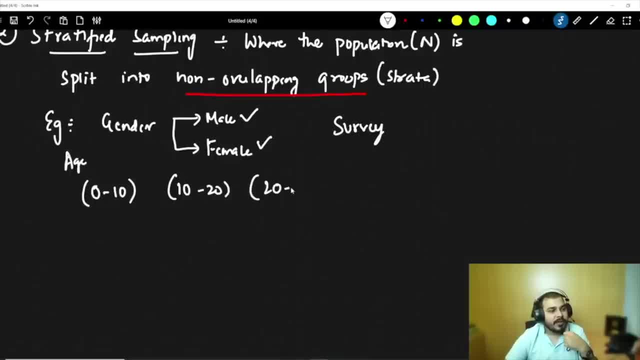 Probably 10 to 20 will be one age group, Probably 20 to 40 will be another age group And probably it will be 40 to 100 will be another age group. So based on different, different age group, I can also do a sampling. 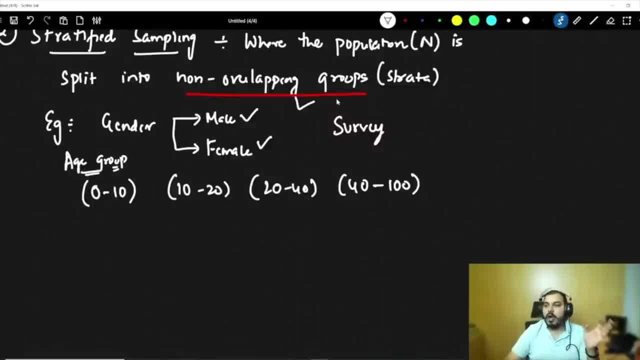 Understand one thing. This terminology is very much important: Non-overlapping. It should not overlap Over here. there is no chance of overlapping Based on profession. can I do stratified sampling Based on profession? can I do stratified sampling? 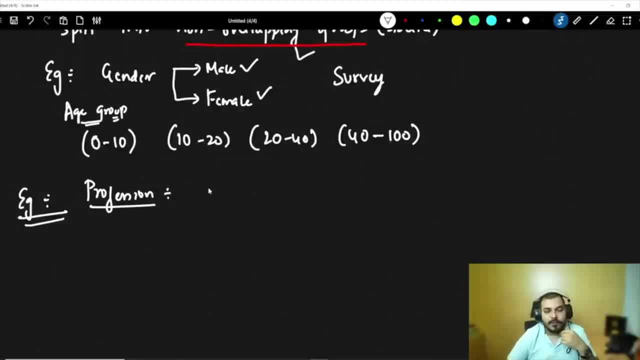 See, a profession may be that, let's let's say that this profession is with respect to different, different, different, different people who are working. OK, suppose a person is a NET developer, A person is a PHP developer, A person is a- you know- data scientist, or he's working specifically in Python. 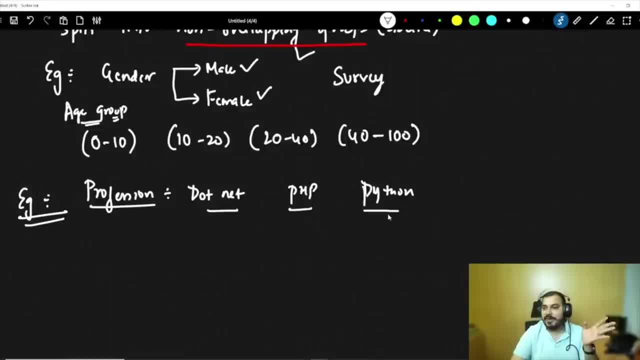 Over here. definitely, you can see that they have different, different stratified layers, But there may be some scenarios that it may overlap. A PHP person may know NET, A NET person may know Python, So both the scenarios will be there. 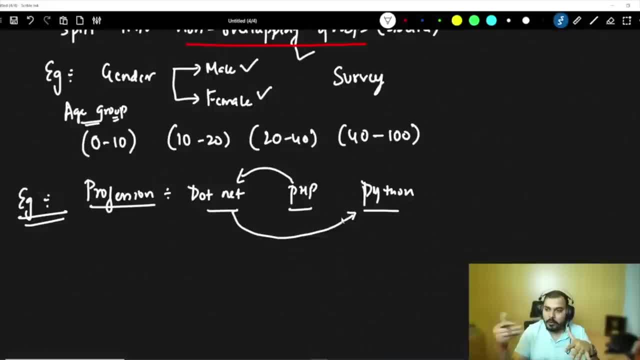 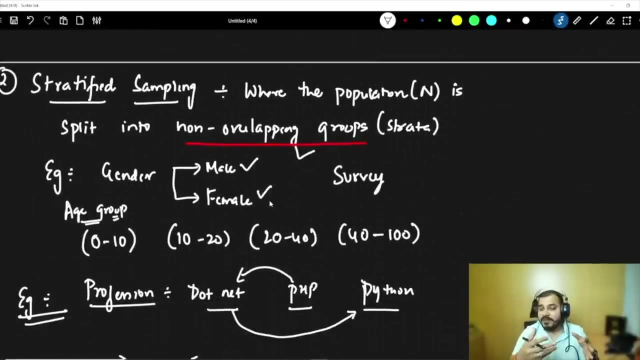 If a person is highly experienced and he says that- no, I don't know NET, then it will not become overlapping, But definitely we can apply it for doctors, engineers, doctors, engineers, different, different survey can be there. So just understand that in some of the cases we can do stratified sampling. 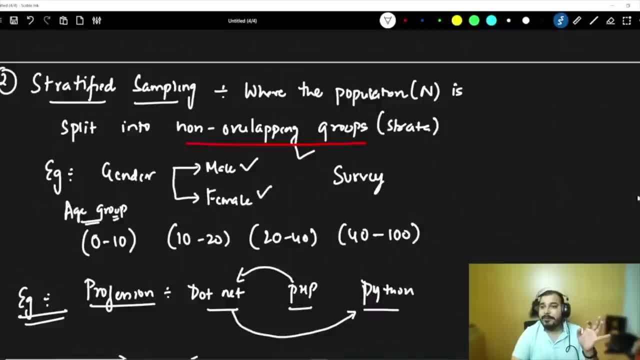 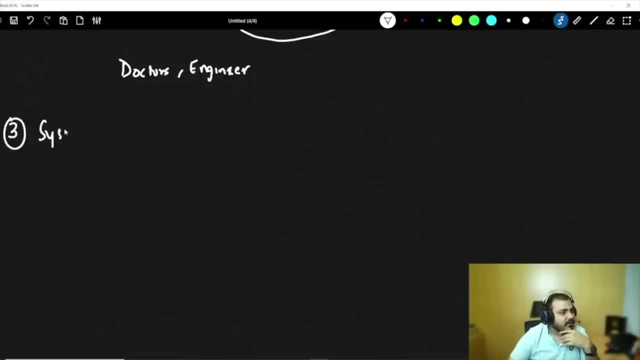 But by applying some other conditions we can make sure that that sampling satisfies all the conditions. Coming to the third one, The third technique is basically called as systematic sampling. The third technique is called as systematic sampling Here from the population N what we do? we just pick up every Nth individual. 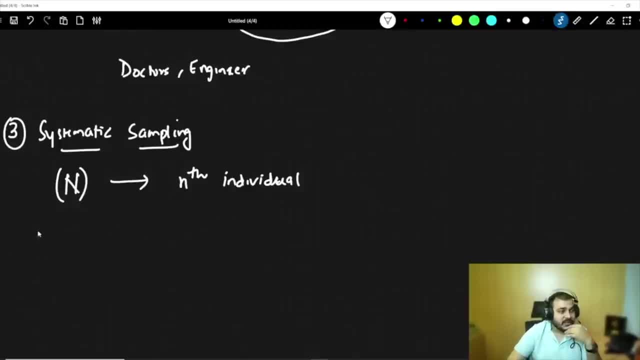 I'll give you a very good example. Nth individual from this population. What does this basically mean? Let's consider that I'm outside the mall and I want to do a survey regarding COVID. So what I'm doing Every 7th or 8th person. 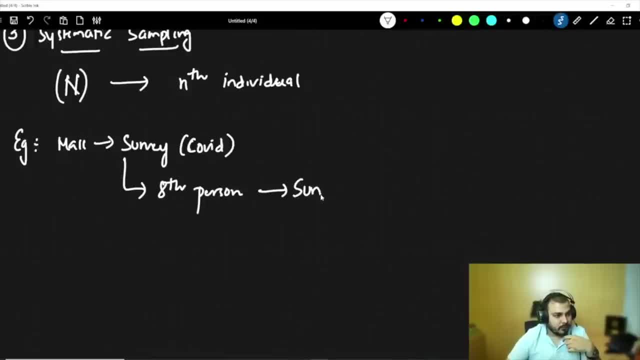 That I see. I am saying that for this person. do the survey. So in systematic sampling you consider any 8th person. I'm just saying as an example, every 8th person, I mean every first person that I see, every 5th person that I see, or every 10th person that I see in front of my eyes. I'll just tell him to do the survey. 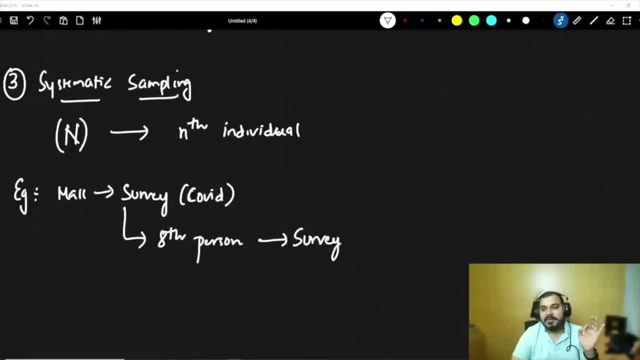 So this is what systematic sampling is all about. In systematic sampling, there is no reason why you're selecting the 8th or the 9th person. You just said that. OK, it is my personal duty What I'm actually going to do. whichever person that I see on the 7th time, I'm just going to catch him and I'm going to basically ask him about this survey. 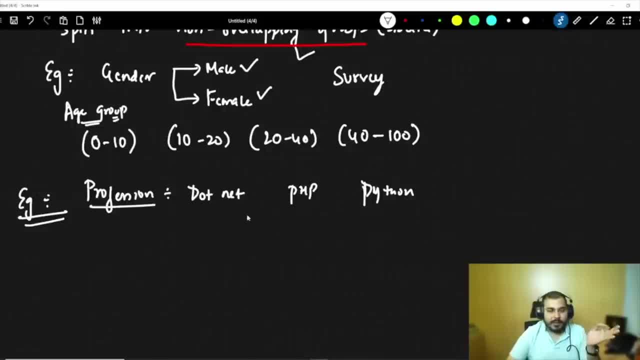 data scientist or he's working specifically in Python Over here. definitely, you can say that they have different, different stratified layers, But there may be some scenarios that it may overlap. A PHP person may know NET, A NET person may know Python, So both the scenarios will be. 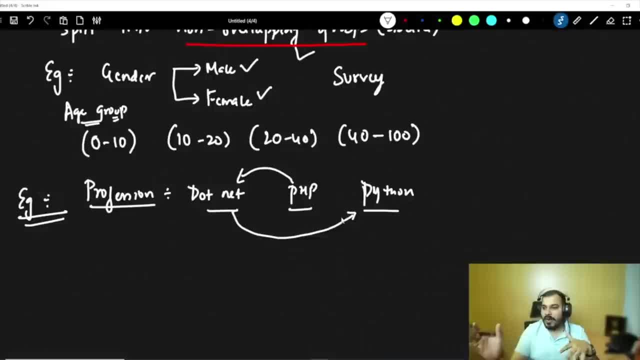 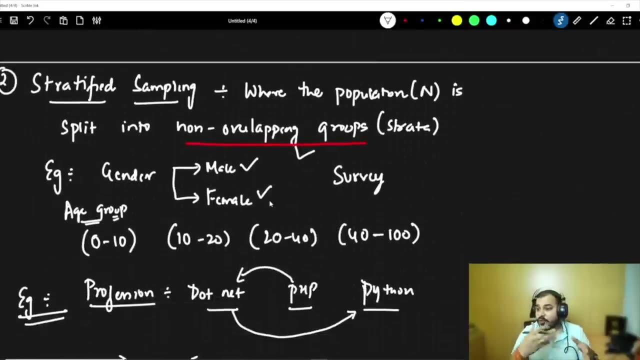 there. If a person is highly experienced and he says that no, I don't know NET, then it will not overlap. So definitely we can apply it for doctors, engineers, doctors, engineers, different, different survey can be there. So just understand that in some of the cases we can do stratified. 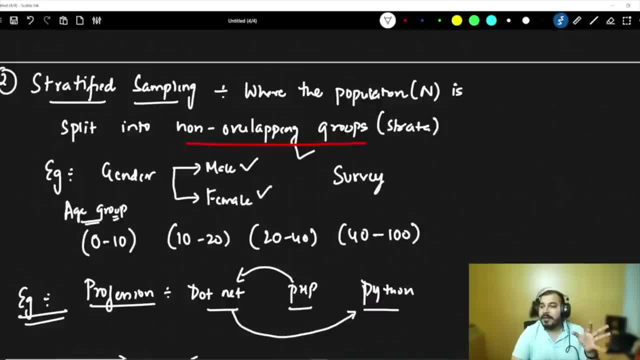 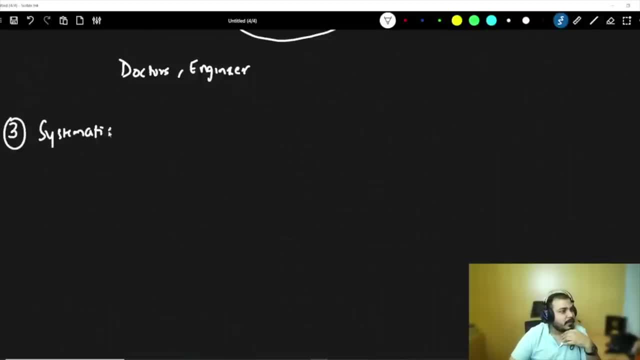 sampling, but by applying some other conditions we can make sure that that sampling satisfies all the conditions. Coming to the third one, The third technique is basically called as systematic sampling. The third technique is called as systematic sampling. Here, what we do, we just pick up every nth individual. I'll give you a very good example: Nth individual. 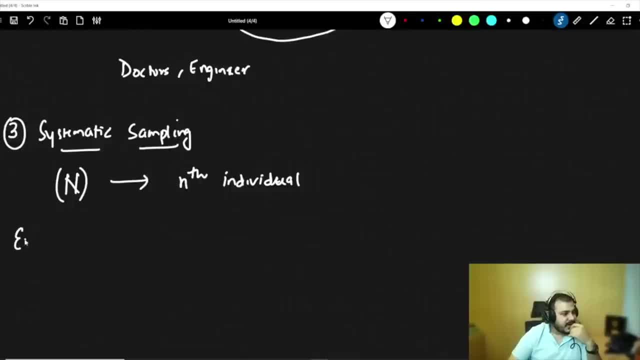 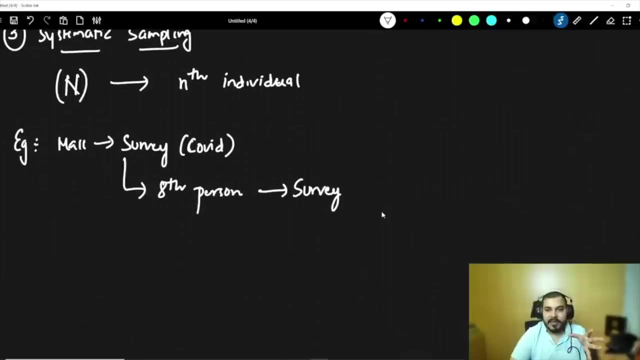 from this population. What does this basically mean? Let's consider that I'm outside the mall and I want to do a survey regarding COVID. So what I'm doing- every seventh or eighth person that I see, I am saying that for this person- do the survey. So in systematic sampling. 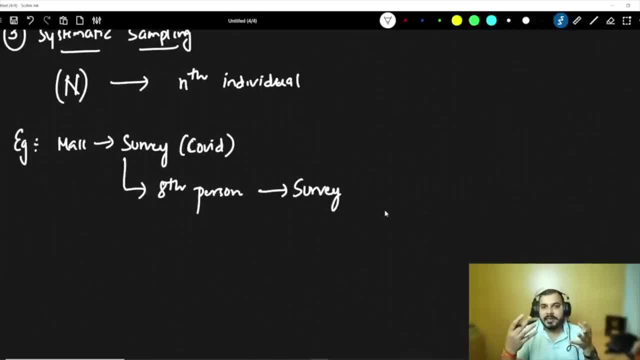 you consider any eighth person. I'm just saying as an example, every eighth person. I may take every first person that I see, or every fifth person that I see, or every 10th person that I see in front of my eyes. I'll just tell him to do the survey. So this is what systematic 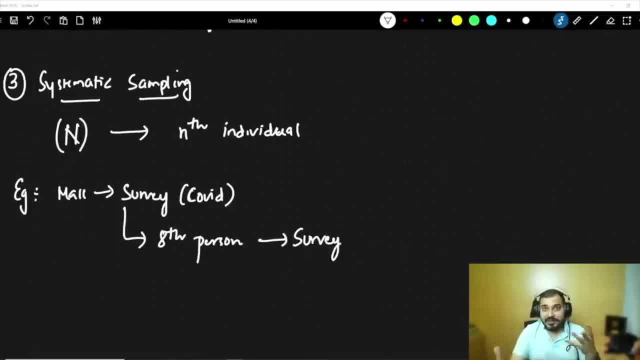 sampling is all about. In systematic sampling, there is no reason why you're selecting the eighth or the ninth person. You just said that. okay, it is my personal duty What I'm actually going to do. whichever person that I see on the seventh time, I'm just going to catch him and I'm going to. 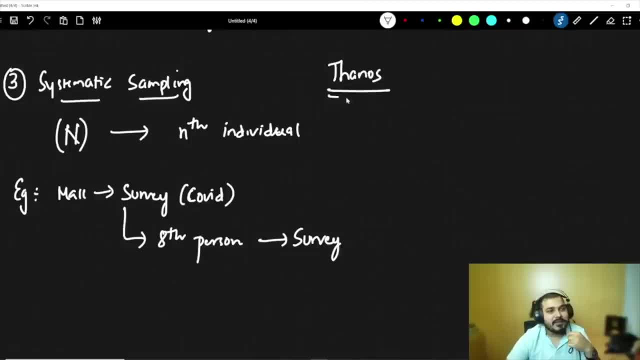 basically ask him about this survey. So, Thanos, when he snapped the, when he snapped his finger, what do you think what kind of sampling techniques may have used? do you think random sampling is basically getting used because you could see right, probably random sampling may have been used. 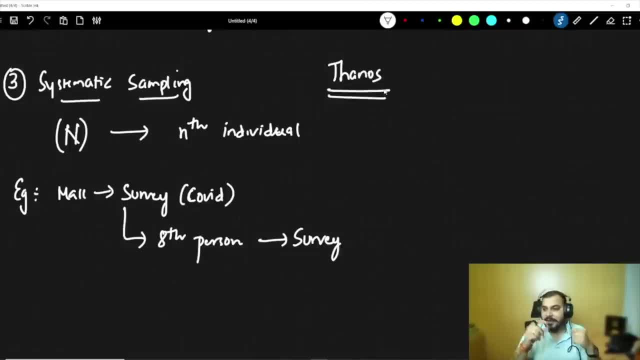 So, Thanos, when he snapped his finger, what do you think? what kind of sampling techniques may have been used? Do you think random sampling is basically getting used? Because you could see right, Probably random sampling may have been used. OK, now let's come to the next sampling, which is called, as you can say it, as convenience sampling. 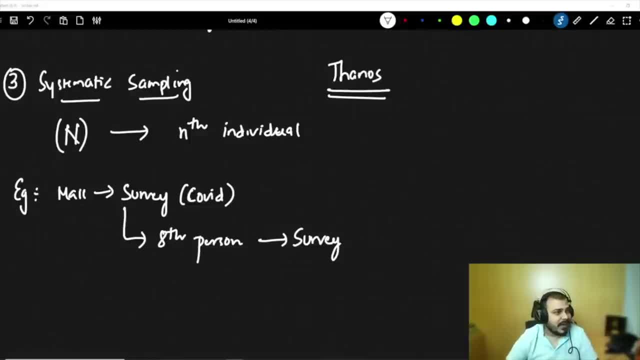 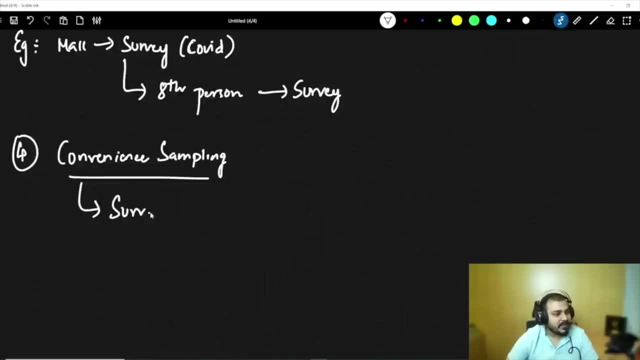 You can say it as voluntary response sampling. I'll just say it as the fourth technique, I'll say it as convenience sampling, This kind of samples, suppose. let's consider that I'm doing a survey. Only those people who are, who are a domain expertise in that particular survey will be doing, will be participating in that particular survey. 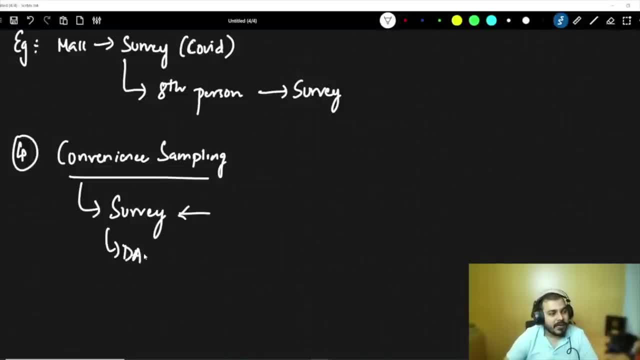 Suppose, let's say, consider that I am doing a survey related to data science, I will say that any person who is probably interested in data science and has the knowledge of data science, if you consider only those people, only those people, then it basically becomes a convenience sampling only those people who are 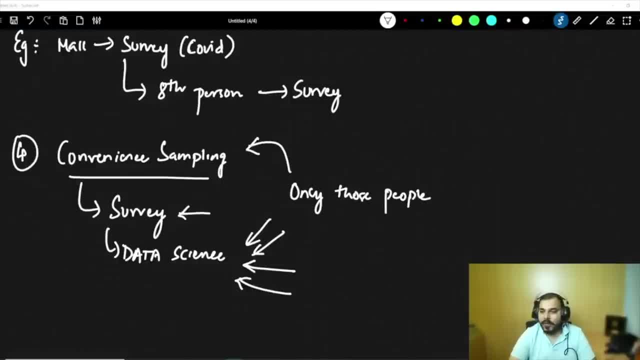 basically interested in this will basically be doing it, or who are expert in that will definitely be doing it, because this is a specific topic which requires domain knowledge, which require some amazing things in that, basically, he should be knowing, based on this survey, because those surveys will be important. through surveys, you take out some kind of information. you, you will. 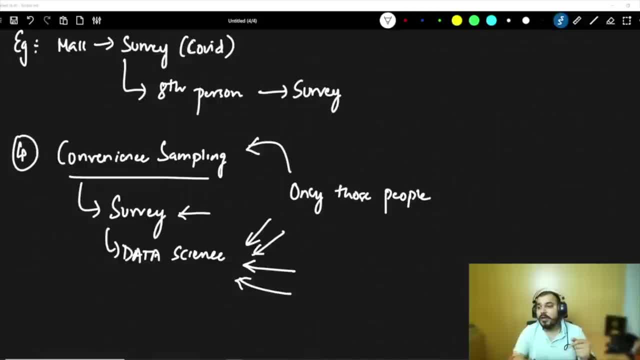 be able to make some kind of decisions, so that is very much important. who is taking the survey? like many people also. how do you generate your data set? that is also said. like in many companies, what they do is that they make sure that the people actually try to put some kind of surveys. 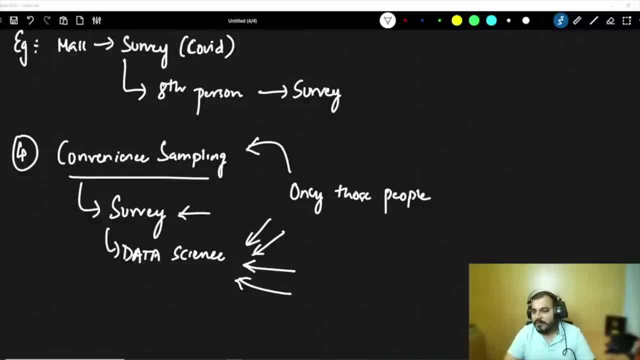 in front of the people and they basically use that data for doing different, different things. again, i'm going to repeat what is convenience sampling. let's consider that i am doing a survey related to a specific topic, in this particular example, data science. obviously i will not go to. 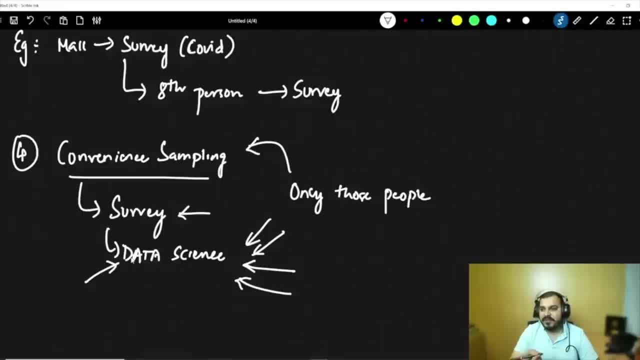 some other people who don't have the knowledge of data science to do that specific survey. so i may collect my sample in a bit different way, where we'll focus on people who's giving the survey should have knowledge on that specific topic. okay, now let me give you some of the examples. let's say 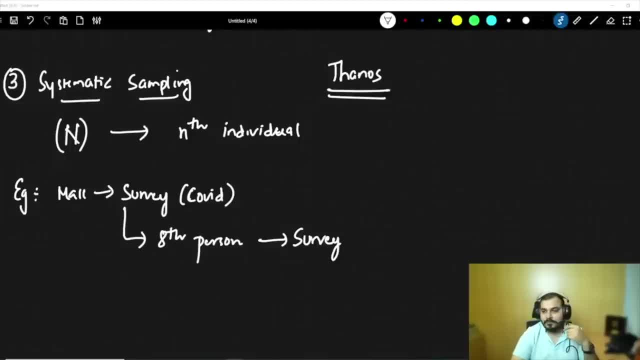 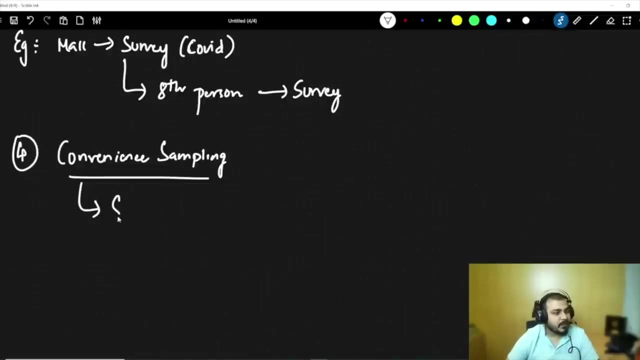 okay, now let's come to the next sampling, which is called as: uh, uh. you can say it as convenience sampling, um, you can say it as voluntary response sampling. i'll just say it as the fourth technique. i will say it as convenience sampling, this kind of samples, suppose let's consider that i'm doing. 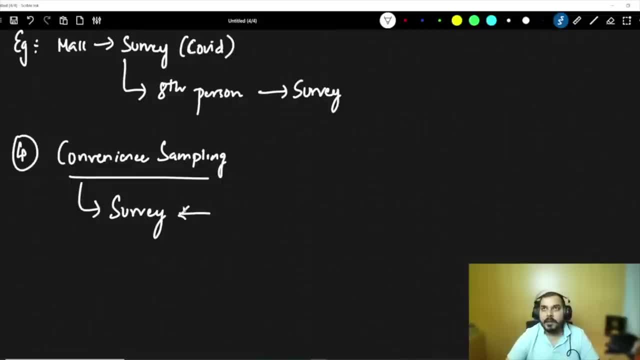 a survey, only those people who are who are a domain expertise in that particular survey will be doing, will be participating in that particular survey. suppose, let's say, consider that i am doing a survey related to data science- i will say that any person who is probably interested in data science and has the knowledge of data science- if you consider only those people- 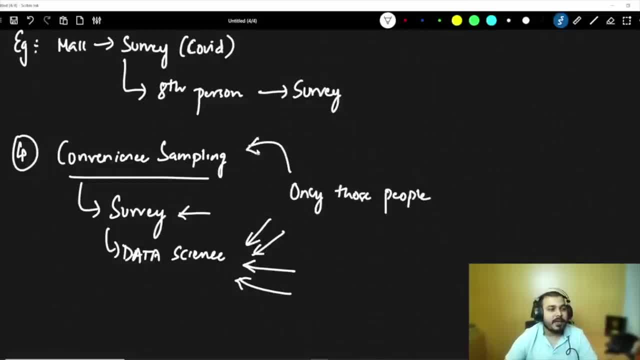 only those people, then it basically becomes a convenience sampling. only those people who are basically interested in this will basically be doing it or who are expert in that will definitely be doing it, because this is a specific topic which requires domain knowledge, which require some uh amazing things in that basically he should be knowing based on this survey, because those surveys will. 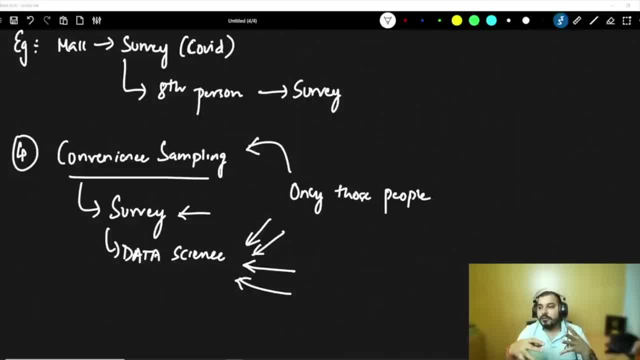 be important. through surveys, you take out some kind of information. you you will be able to make some kind of decisions, so that is very much important. who is taking the survey? like many people also. how do you generate your data set? that is also said. like in many companies, what they do is that they make sure that the people 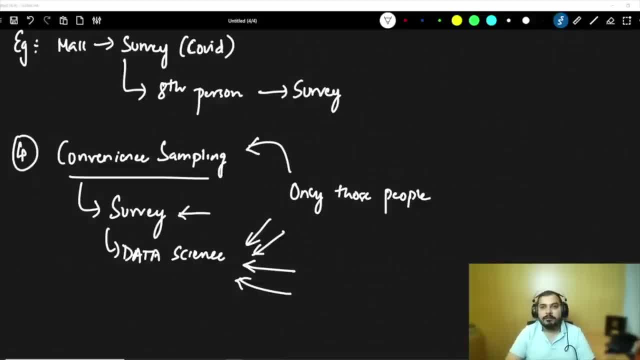 actually try to put some kind of surveys in front of the people and they basically use that data for doing different, different things. again, i'm going to repeat what is convenience sampling. let's consider that i am doing a survey related to a specific topic. in this particular example, data. 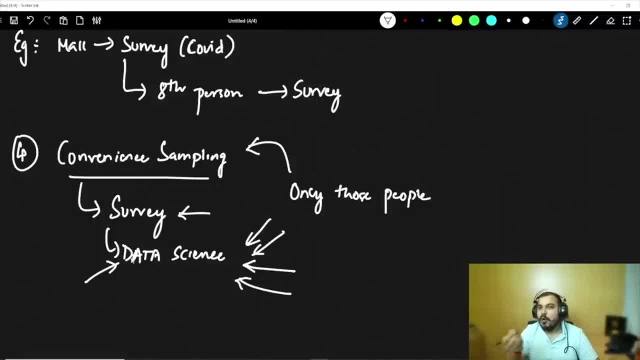 science. obviously i will not go to some other people who don't have the knowledge of data science to do that specific survey. so i may collect my sample in a bit different way, where we'll focus on people who is giving the survey should have knowledge on that specific topic. okay, now let. 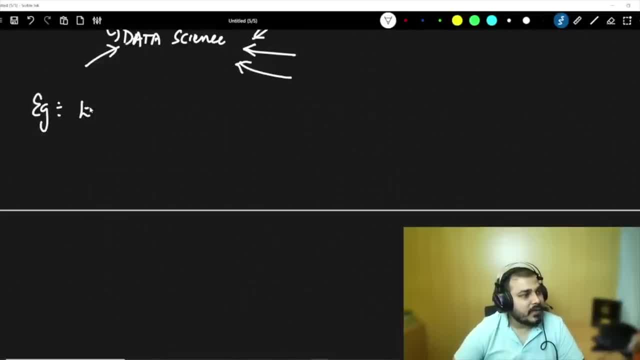 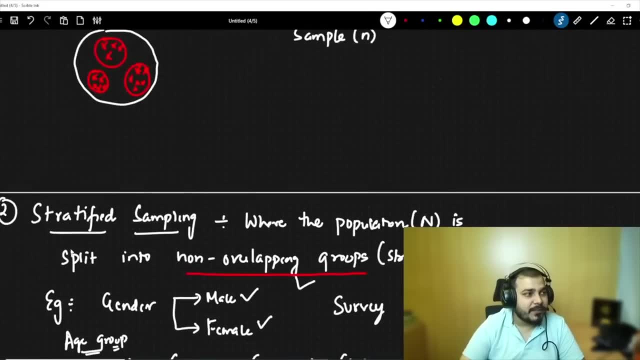 me give you some of the examples. let's say that there is an exit poll. what kind of sampling we would be better? see guys again. people are getting confused with respect to system and stratified sampling and this sampling in convenience sampling. we are just specifically considering a domain. 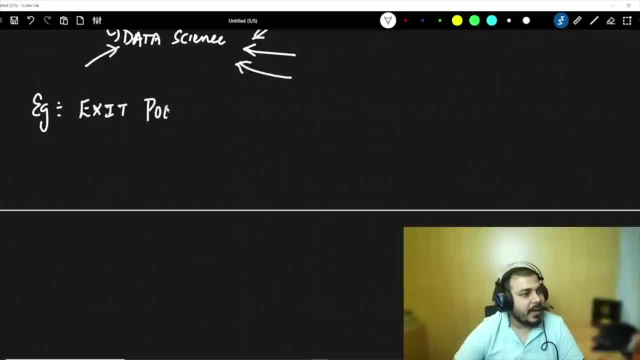 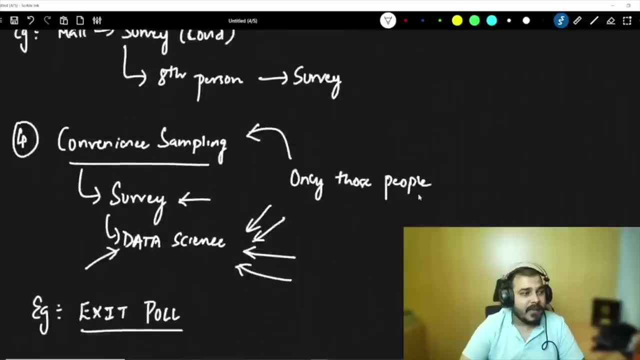 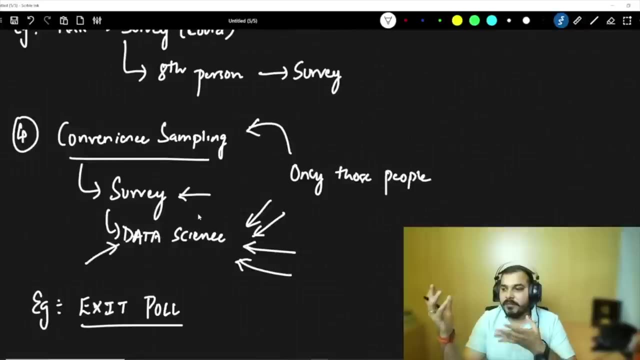 that there is an exit poll. what kind of sampling we would be better. see guys again. people are confused with respect to system stratified sampling and this sampling in convenient sampling. we are just specifically considering a domain. there we are dividing groups based on something. so tell me the. 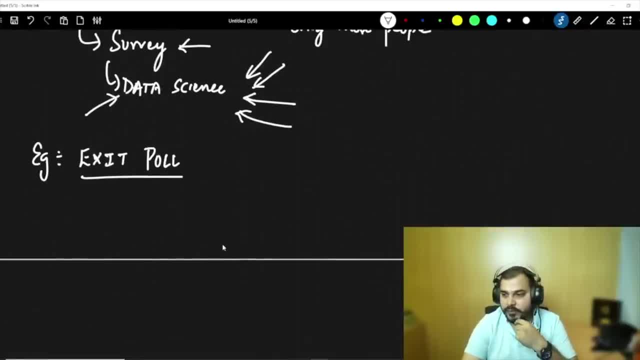 examples of exit poll. what kind of sampling technique we may use? so obviously we will be using over here as random sampling, see rbi. i hope everybody knows rbi. they do something- survey with respect to household, household surveys for this, household surveys. what kind of sampling probably? 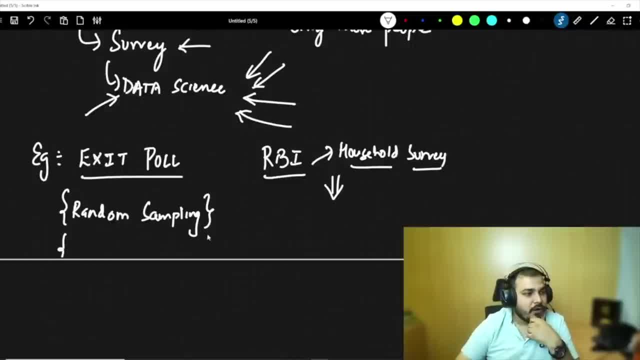 they may use. hey guys, you may also consider that over here you need to follow some stratified random sampling. obviously we can do, but over here most of the time random sampling is basically done in household surveys. rbi, make sure that they have to fill the survey from a woman, where probably 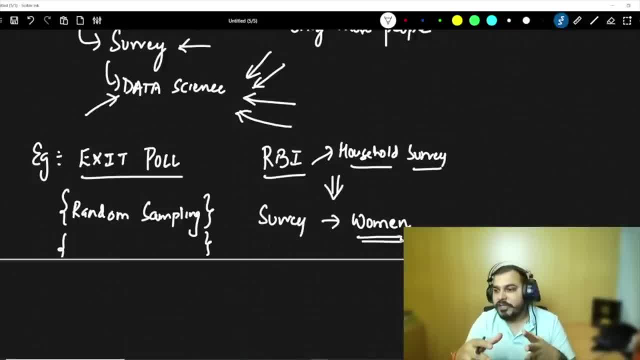 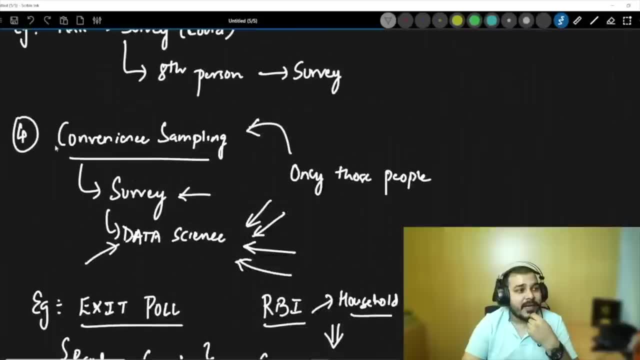 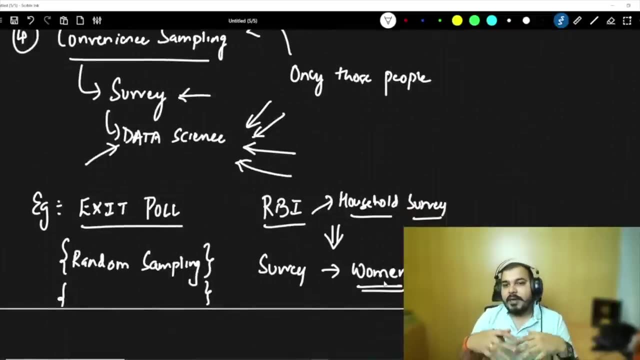 they are trying to find out, like what is the cost expenditure in running a house. so here you can probably consider stratified sampling. if you don't want to consider stratified sampling, we can also do convenient sampling, only women. you can basically consider over there and you can do it now. 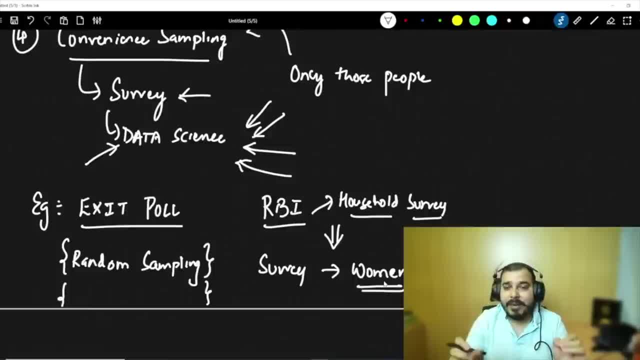 understand, sampling techniques may be different. it is completely dependent on the use case that we are following, based on the use case that you really want to do. based on that you will do and it is not like we will just be dependent on one kind of data. we try to use different, different. 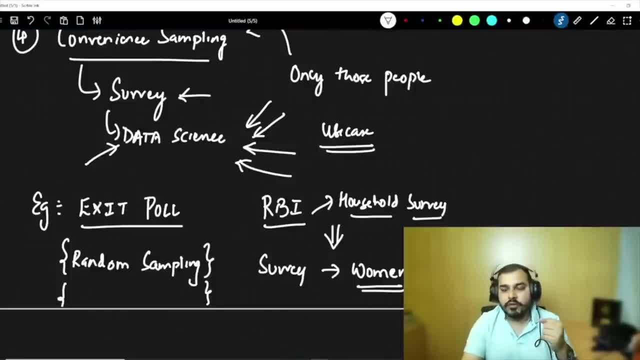 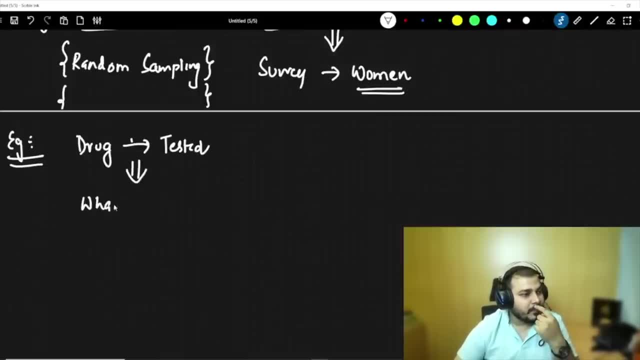 sampling techniques and finally, we try to come to a conclusion on the same. let me give you one more example. a drug needs to be tested, so for this, what kind of samples we may take? now, here i can bring up multiple use case. first of all, to whom this drug needs to be tested, if i get that specific. 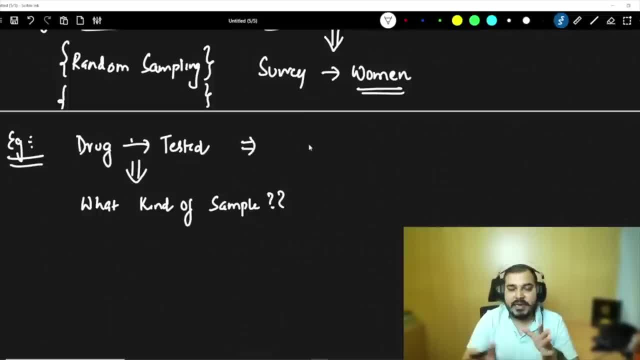 information. i will basically do the age groupings and then i may probably apply. let's consider that this drug is for everyone. probably then i may consider picking up some samples, but at least i'll put a condition that at least it should be greater than 15 years, because we cannot just 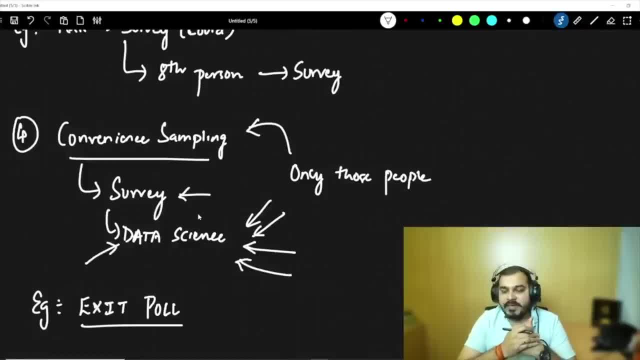 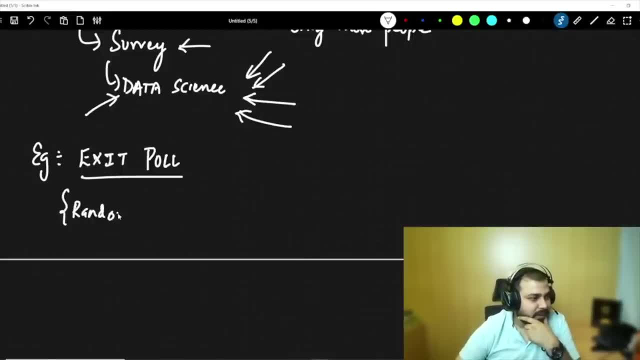 there we are dividing groups based on something. so tell me the examples of exit poll, what kind of sampling technique we may use? so obviously we will be using over here as random sampling- see rbi. i hope everybody knows rbi. they do something. survey with respect to household. 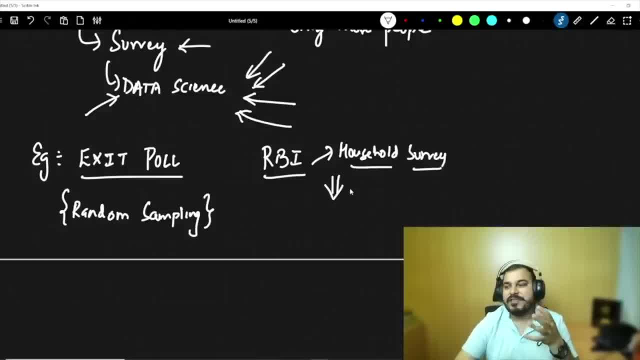 household surveys for this. household surveys: what kind of sampling probably they may use? hey guys, you may also consider that over here you need to follow some stratified random sampling. obviously we can do, but over here most of the time random sampling is basically different. so we are dividing groups based on something. so tell me the examples of exit poll. 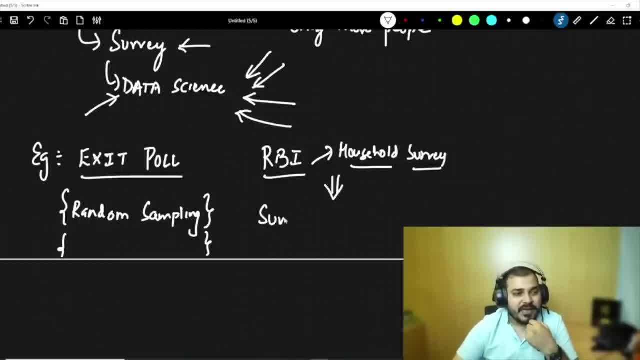 done in household surveys. rbi make sure that they have to fill the survey from a woman where probably they are trying to find out, like, what is the cost expenditure in running a house. so here you can probably consider stratified sampling. if you don't want to consider stratified sampling, we 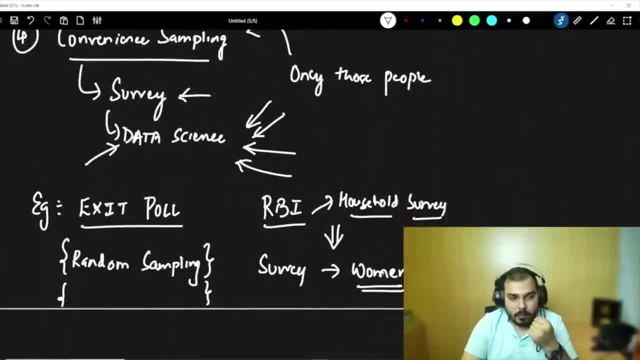 can also do convenient sampling, only woman. you can basically consider over there and you can do it. now understand, sampling techniques may be different. it is completely dependent on the use case that we are following, based on the use case that you really want to do. based on that, you will do and 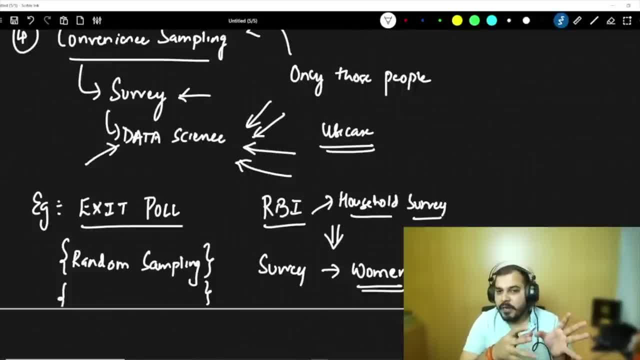 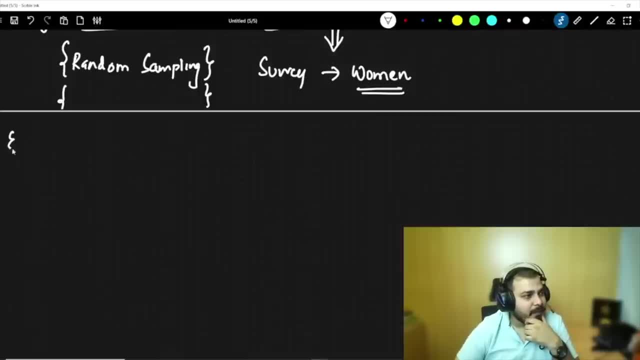 it is not like we will just be dependent on one kind of data. we try to use different, different sampling techniques and finally we try to come to a conclusion on the same. let me give you one more example. a drug needs to be tested, so for this, what kind of samples we may take? now, here i can bring up. 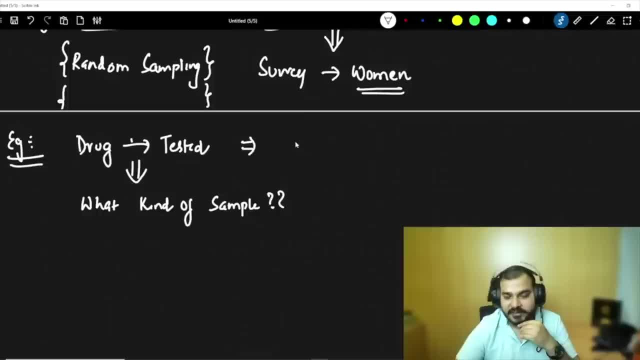 multiple use case. first of all, to whom this drug needs to be tested. if i get that specific information, i will basically do the age groupings and then i may probably apply. let's consider this drug is for everyone. probably then i may consider picking up some samples, but at least i'll put a condition that at least it should be greater than 15 years. 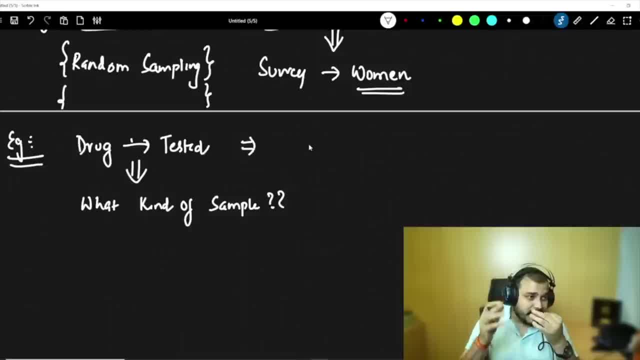 because we cannot just directly use a specific drugs on kids. so different, different. it depends on the use case that you are probably trying to do and based on that you will probably try to select it. and again, there may be many things, many, many questions that may come. is that okay, krish? why not this? why not that? why not this? 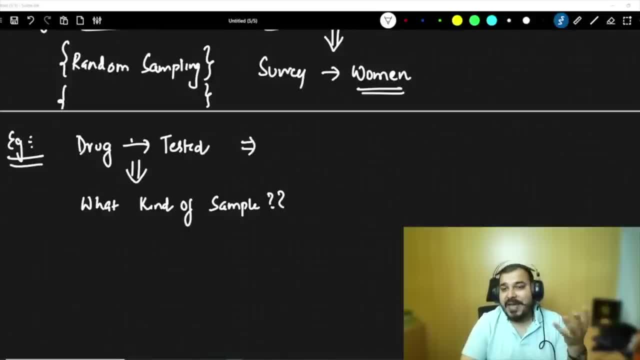 why not that right? this kind of questions may come. that is where we basically experiment with multiple things. so in the real world scenario also, when you are probably collecting the data, you will find this kind of scenarios a lot. now let's go with the next topic: what is called as variables. now, what is a? 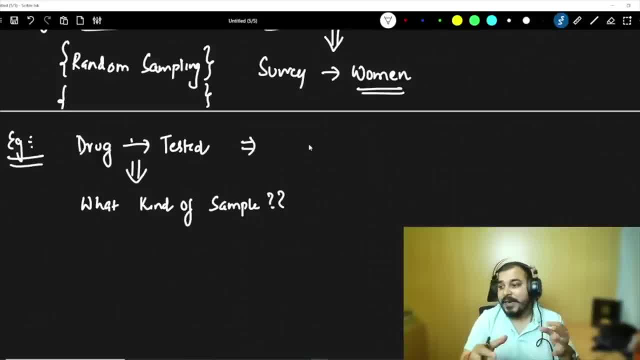 directly use the specific drugs on kids. so different, different people. we may not have this particular increase in possibility within one year. so we don't have that many break down and we have to think of one specific. you know that we don't have to do that, but we don't have to deal with that. anyone species. 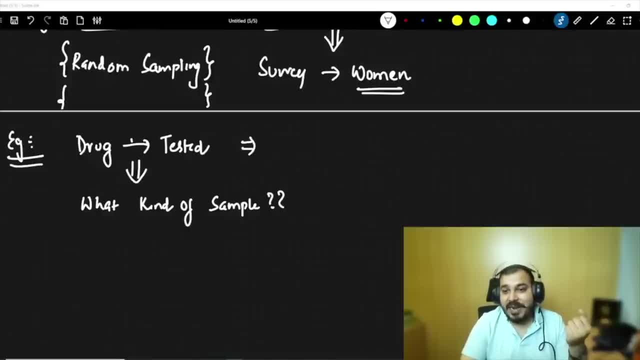 is diferentes, then it is up to you what to tend to be present or what to expect. it depends on the use case that you're probably trying to do and, based on that, you will probably try to select it and, again, there may be many things, many, many. 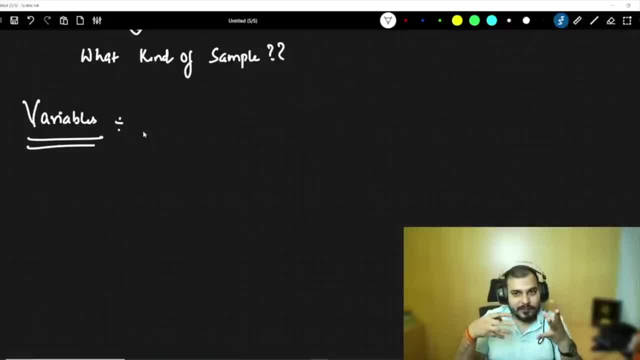 questions that may come. is that a variable? Obviously, if you are a coder, you obviously know that what is a variable? So I will just give you a definition that is much more related to you. I'll say that a variable is a property that can take on any value. A variable is a property that can take any value. Let's say: 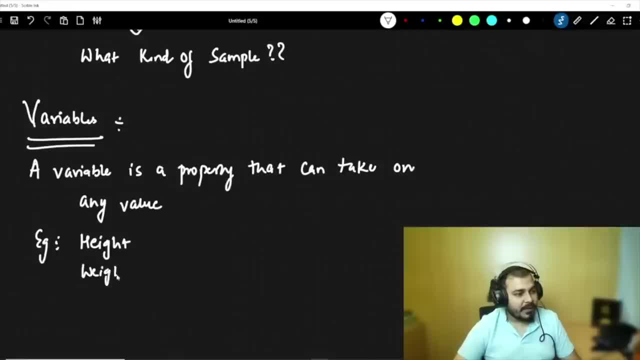 an example, I'll say height, I may say weight. These are variables. We can have any value. We can have 170 centimeters, 172 centimeters, 185 centimeters, 190 centimeters, anything. I can have different, different values with respect to height: 182, 178, 168, 150, 160, 170, anything. 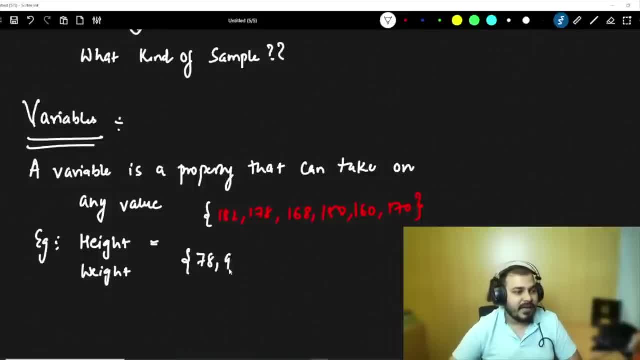 Similarly, with respect to weight, I can have any values like 78,, 99,, 100,, 60,, 50, anything that I want. So this is a simple definition with respect to a simple variable, with a lot of examples. 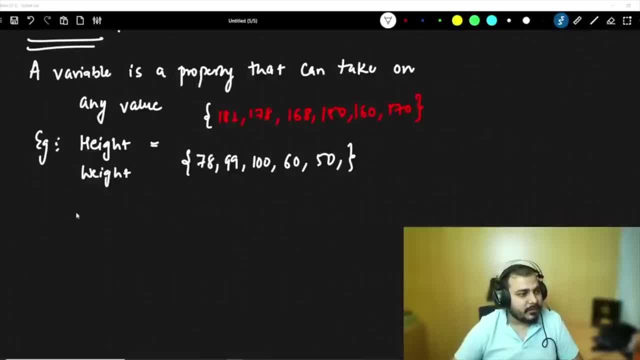 Now understand. there are two kinds of variables. So let me go ahead and let me teach you this. There are two kinds of variables. The first kind is basically quantitative variable- quantitative variable. The second type is basically: you just say me the answer. I'll pause for five seconds. The second type is something: 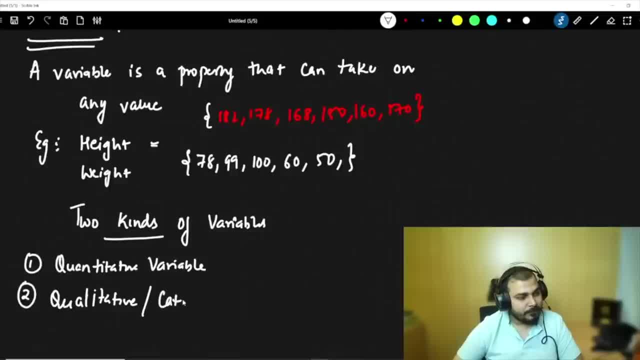 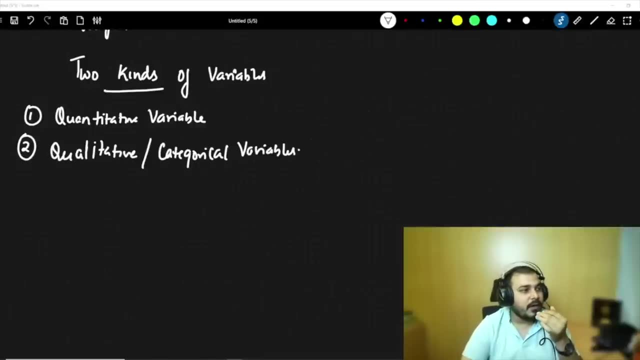 called as qualitative variable, qualitative or categorical variables. So these are the two types of variables that we specifically use. Now I will try to divide this into many types and we'll try to understand these variables, because these are also very much important. Now, first of all, 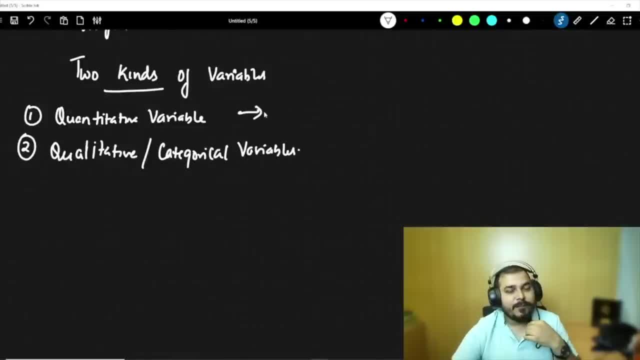 coming to the quantitative part, This quantitative part will have some properties. it can be measured numerically, so we can measure them by putting numbers. We can perform lots of operations like add, subtract, divide, multiply, right, We can perform any kind of operations that we want. So one example of this: 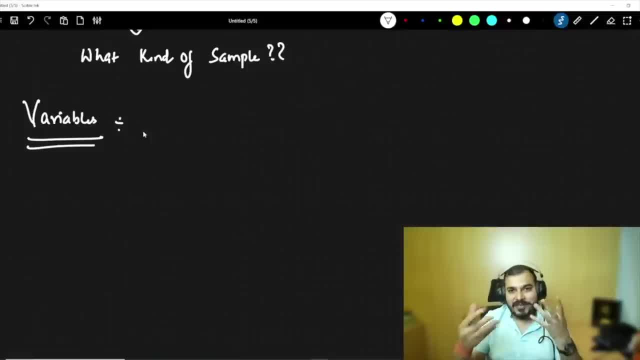 variable. obviously, if you are a coder, you obviously know that what is a variable? so i will just give you a definition that is much more related to you. i'll say that a variable is a property that can take on any value. a variable is a property that can take any value. let's say an example. i'll say height, i may say weight. these are 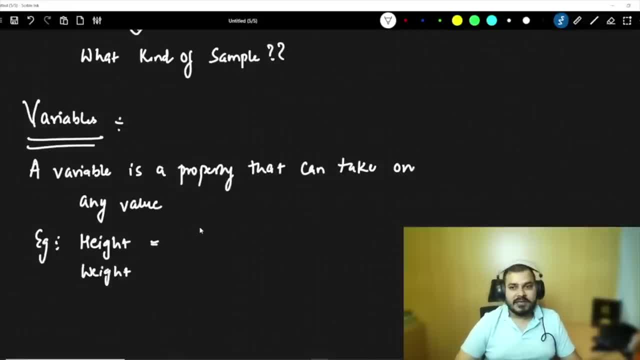 variables. we can have any value. we can have 170 centimeters, 172 centimeters, 185 centimeters, 190 centimeters, anything. i can have different different values with respect to height: 182, 178, 168, 150, 160, 170, anything. similarly, with respect to weight, i can have any values like 78, 99 hundred or 60. 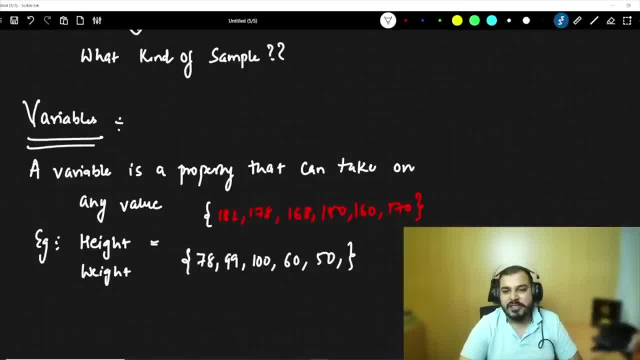 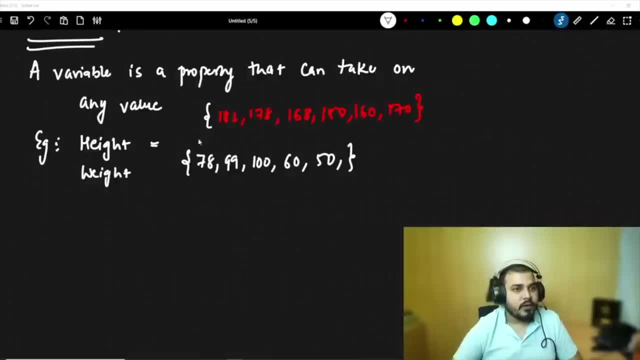 or 50, anything that i want. so this is a simple definition with respect to a simple variable, with a lot of examples. now, understand there are two kinds of variables, so let me go ahead and let me teach you this. there are two kinds of variables. the first kind is basically quantitative variable: quantitative variable. the second type is basically- you just say me the answer. i'll pause for five seconds. the second type is something called as qualitative variable. qualitative or 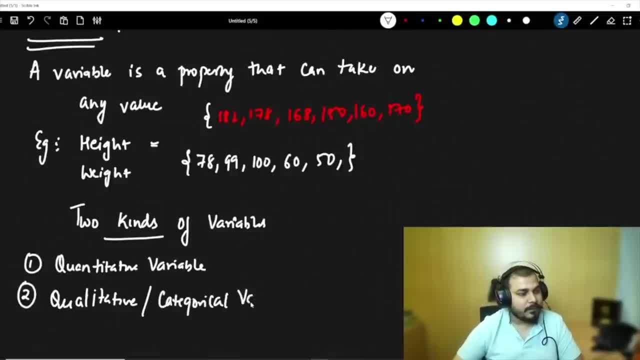 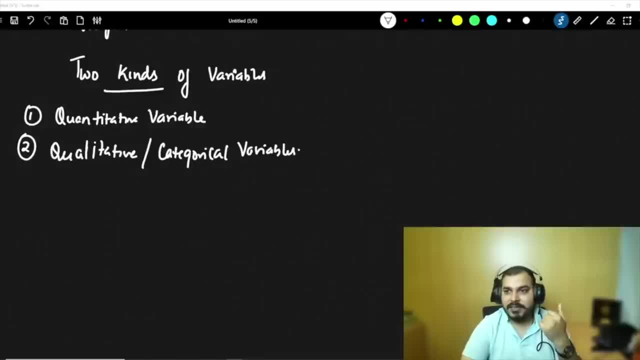 categorical variable. so these are the two types of variables that we specifically use. now i will try to divide this into many types and will try to understand this variable, because this are also very much important. now, first of all, coming to the quantitative- but this quantitative part, we'll have some properties. it can be measured numerically, so we can measure them by putting numbers. we can perform lot of operations like add, subtract, divide and multiply. right, we can. we can perform any kind of operations that we want. 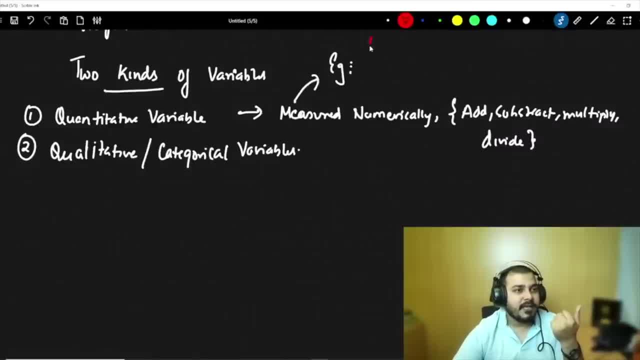 So one example of this is: I may consider age, I may consider weight, I may consider height. Some of the examples with respect to quantitative variable, If I say that, okay, age is a quantitative variable In qualitative and categorical variables. if I specifically take an example, let's consider gender. 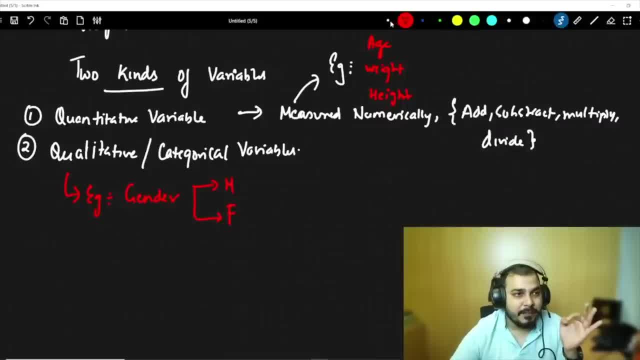 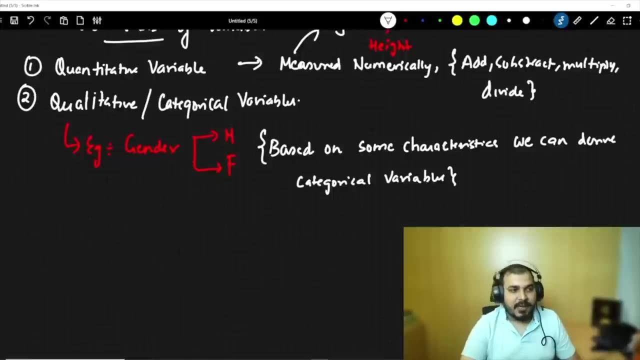 In gender. I have male and female. Now what does this basically mean? Based on some characteristics. based on some characteristics we can derive some categorical variable Or we can derive categorical variable. That basically means we have categories in categorical variable. Here we cannot add, subtract or do some kind of mathematical equations, because here we don't have that option. 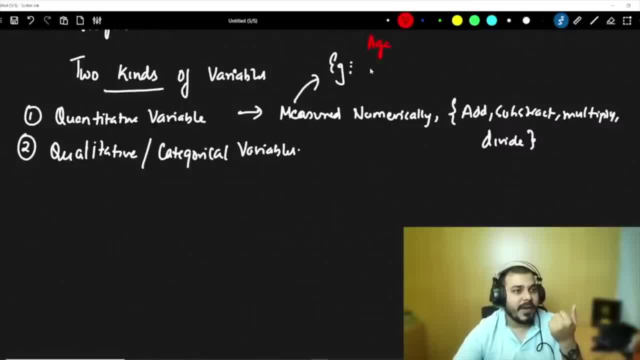 is. I may consider age, I may consider weight, I may consider height. some of the examples. with respect to quantitative variable, If I say that, okay, age is a quantitative variable In qualitative, qualitative and categorical variables. if I specifically take an example, let's consider: 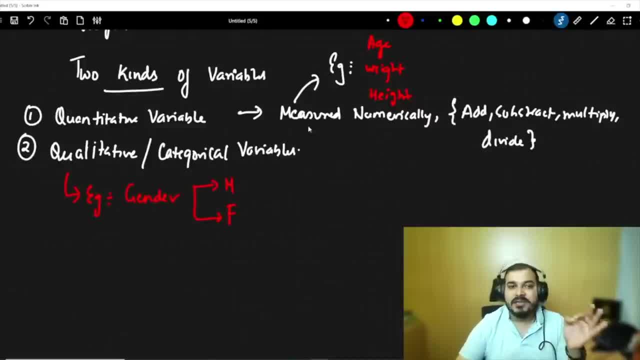 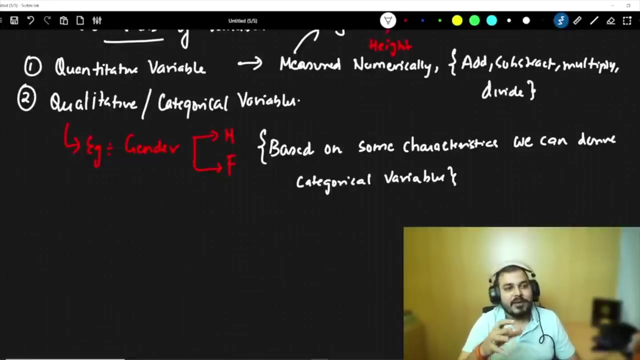 gender. in gender I have male and female. now what does this basically mean? based on some characteristics. based on some characteristics we can derive some categorical variable or we can derive categorical variable. that basically means we have categories in categorical variable. here we cannot add, subtract or do some kind of mathematical equations, because here we don't. 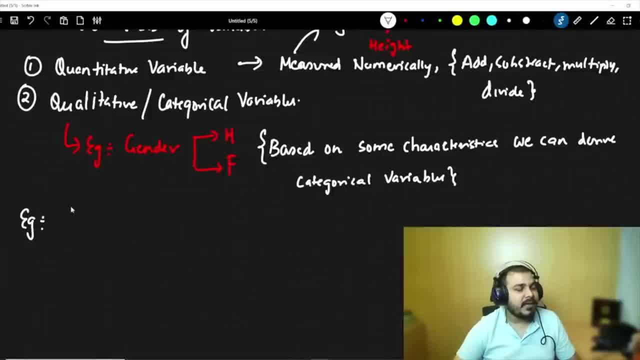 have that option. another example: I may basically say that I may say: okay, I may have categories of let's. let's consider that I have IQ, IQ. if I say 0 to 10, I will divide this IQ 10 to 50 and 50 to 100. 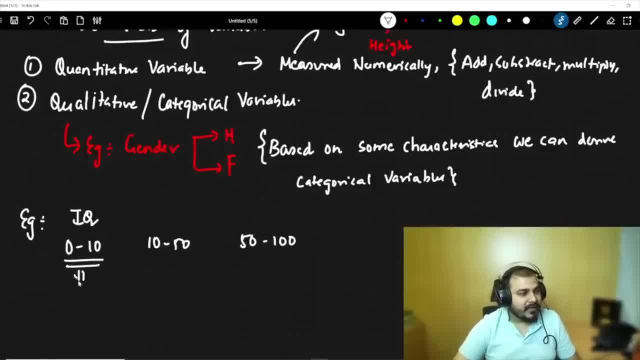 wherever the values are between 0 to 10, I may say that less IQ. whenever I say 10 to 50, I may say that medium IQ. suppose I say this: 50 to 100, I may say good IQ. I'm just saying it this as an example. 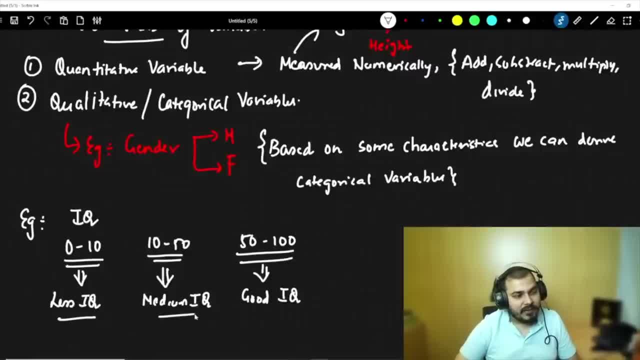 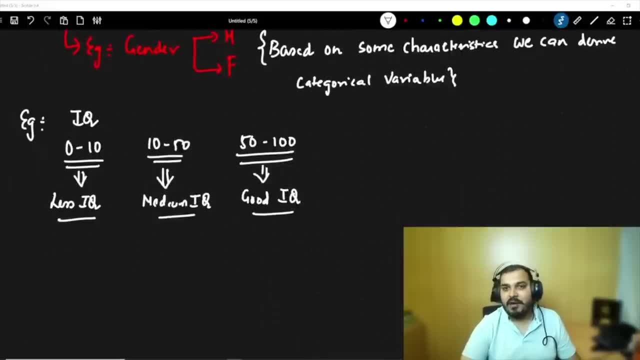 now, based on some characteristics I have derived, or I have classified this into multiple categories, which is called as IQ. here don't tell me, sir Krish, how sir, like, how Krish, more than 50. you are saying that good IQ, then probably every. I'm just taking another example over here. blood group is another example. 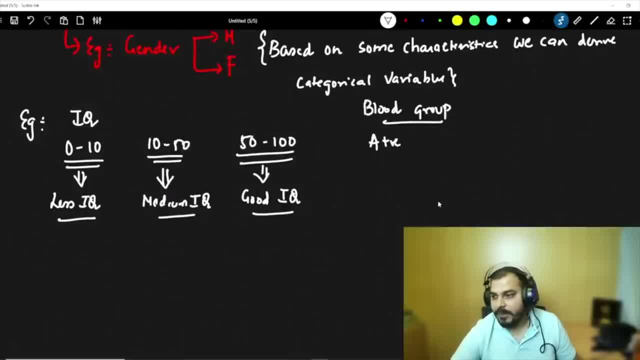 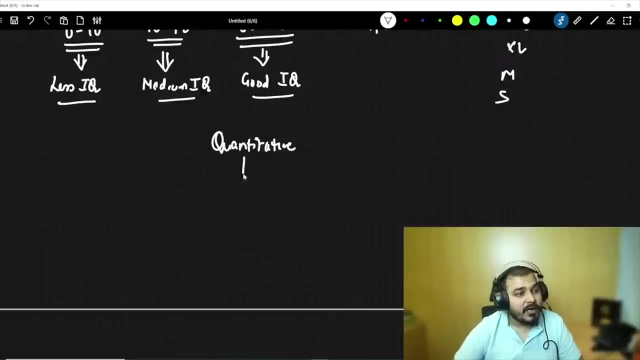 I may have a positive, a negative, like that. I may have a lot of IQs. I may also say t-shirt size based on the properties. you know. we may have large, excel, medium, small, this kind of things. now coming to the quantitative part, quantitative also has two. 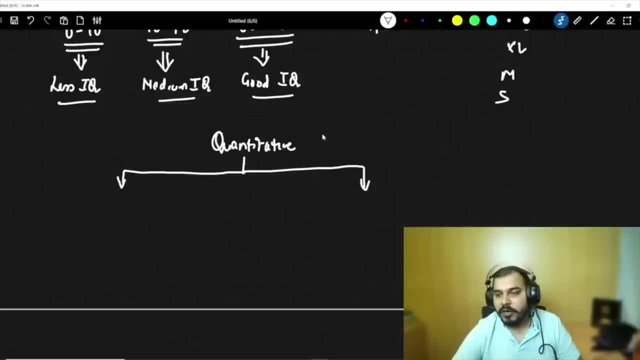 different kind of categories. obviously we know continue. quantitative basically means we have some numerical values here. I'm going to divide this into two one one is the discrete variables and one is the continuous variable. so discrete variables and continuous variable. in discrete variable you will specifically have a whole number. let me just talk about some of the examples. 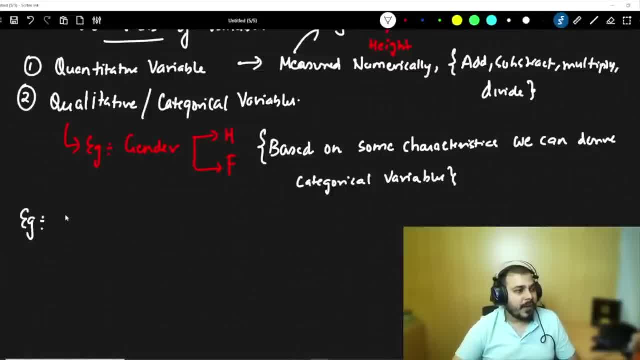 Another example. I may basically say that I may say: okay, I may have categories of, let's consider that I have IQ, IQ, if I say 0 to 10, I will divide this IQ 10 to 50 and 50 to 100. 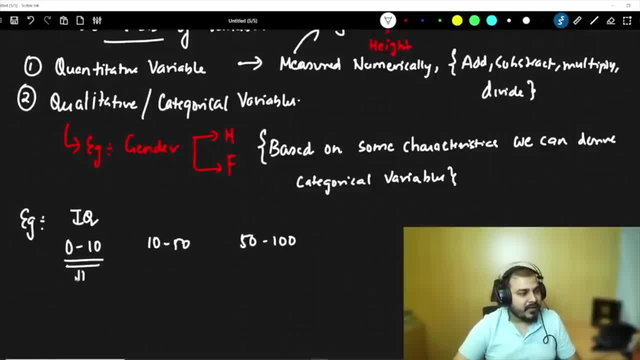 Whenever the values are between 0 to 10, I may say that less IQ. Whenever I say 10 to 50, I may say that medium IQ. Suppose I say this 50 to 100, I may say good IQ. 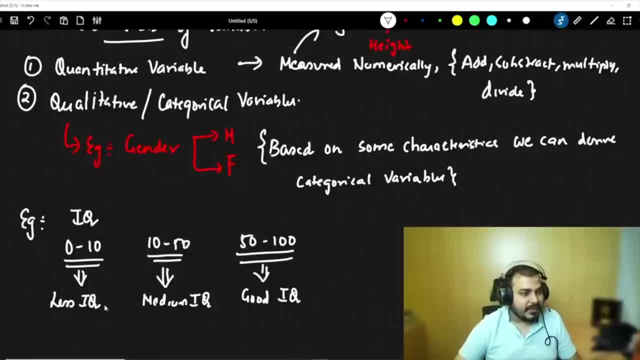 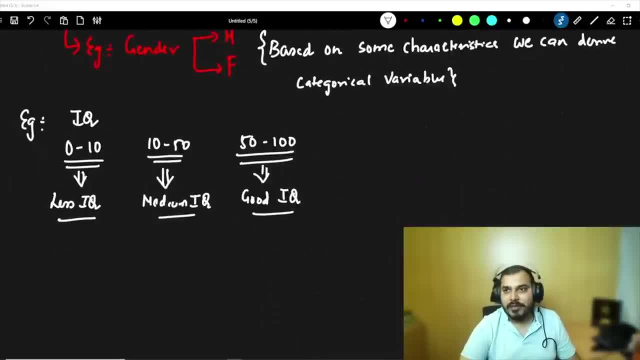 I'm just saying this as an example. Now, based on some characteristics I have derived, or I have classified this into multiple categories, which is called as IQ Here. don't tell me, sir Krish, how sir, like, how Krish, more than 50, you are saying that good IQ. 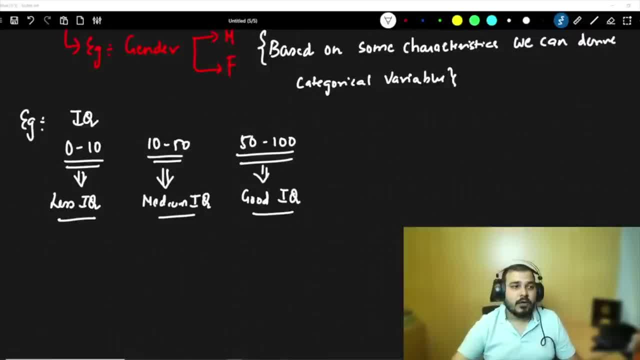 Then probably- I'm just taking it as an example over here. Blood group is another example. I may have A positive, A negative like that. I may have a lot of IQs. I may also say t-shirt size Based on the properties you know. we may have large, XL, medium, small, this kind of things. 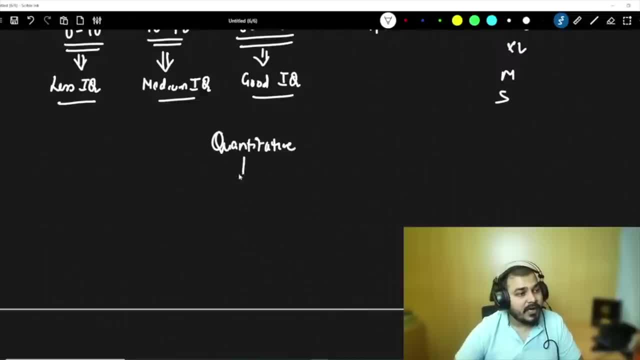 Now coming to the quantitative part, Quantitative also has two different kind of categories, Obviously, we know. quantitative basically means we have some numerical values Here. I'm going to divide this into two One. one is the discrete variables and one is the continuous variable. but discrete variables and continuous variable in discrete variable you will specifically have a whole number. 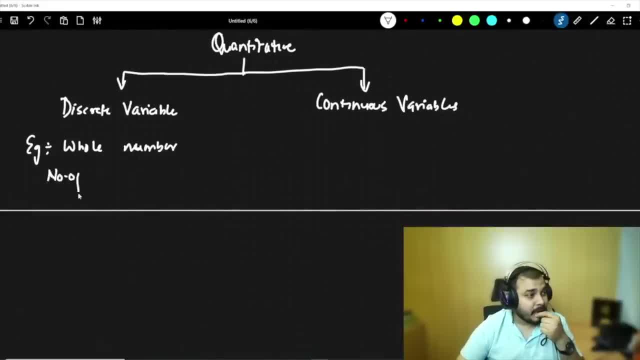 Let me just talk about some of the examples. Number of bank accounts of a person. in this particular case, The example is that you'll say that I have two bank account, three bank account, four, five, six bank account, seven bank account. 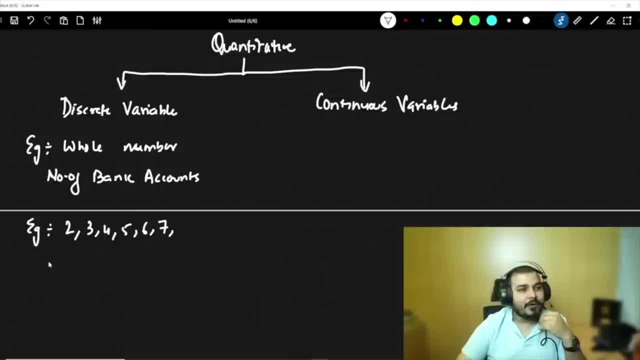 You can say that you have two point five bank account. Another example that I would like to give: a number of children in a family. So this is why another example here: you obviously will say that, okay, there are two children, three children, four children, five children, but you cannot say it is two point five children or three point five children. 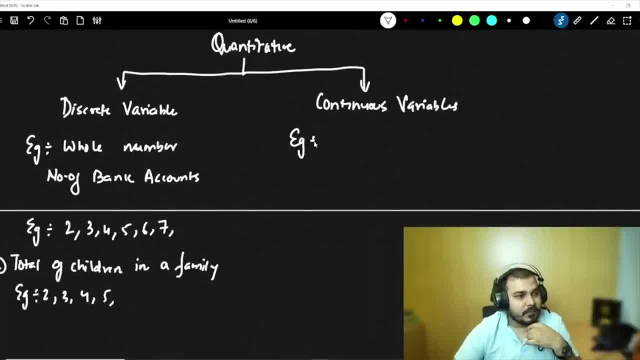 Right now let's go with respect to continuous variable- here We have already discussed that- any values it can have. Okay, Suppose I say height, I can say that the person is one seventy two point five centimeters. I can say that the person is one sixty two centimeters. 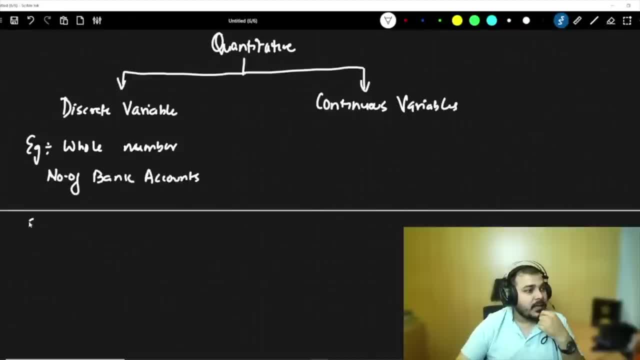 number of bank accounts of a person. in this particular case, the example is that you'll say that I have two bank account, three bank account, four, five, six bank account, seven bank account. you can't say that you have 2.5 bank account. another example that I would like to give: number of children in a family. so this is why- another example here- you obviously you'll say that, okay, there are two children, three children, four children, five children, but you cannot say it is 2.5 children or 3.5 children, right? 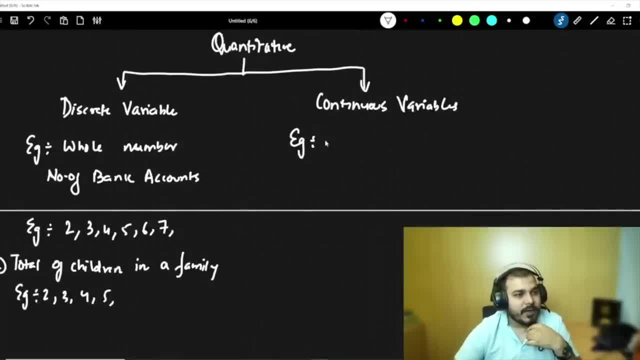 now let's go with respect to continuous variable- here we have already discussed that- any values it can have. okay, suppose I say height. I can say that the person is 172 point five centimeters. I can say that the person is 162 centimeters. I can say a person is 163 point five centimeters- any value that can come. 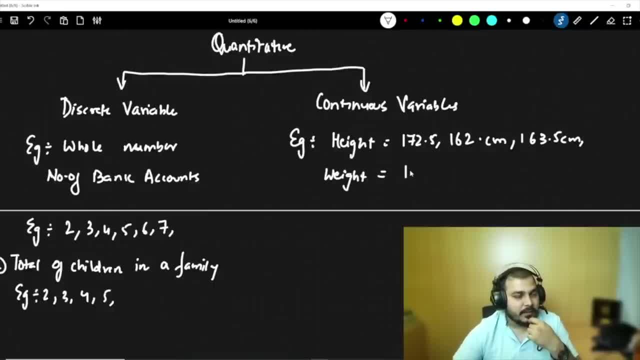 away. similarly, with respect to weight, here I can say the person is hundred kgs, I can say 99 point 5 kg, I may say 99 point 75 kgs. I can also talk about amount of rainfall, which is measured in inches. suppose I say it is one point one. 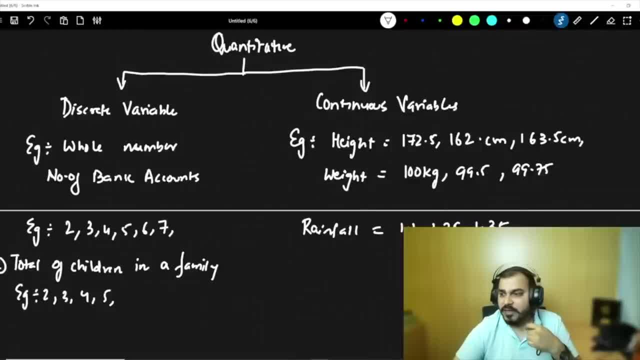 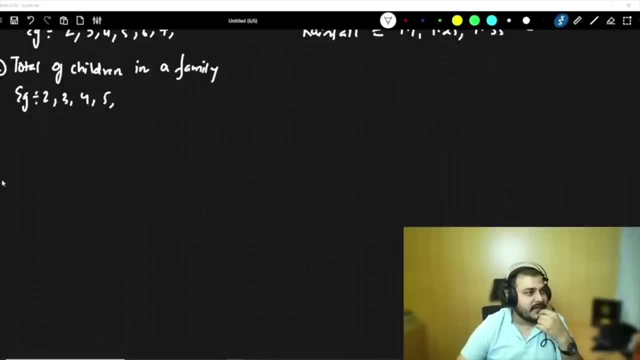 inches, 1.25 inches, 1.35 inches, right, all these things are basically there. so this was an example. with respect to continuous variables, i'll give you some examples. what kind of variable gender is? what kind of variable? marital status is? what kind of variable? river length is what kind of variable? 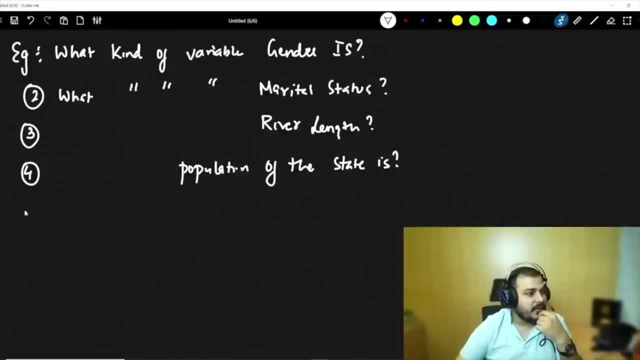 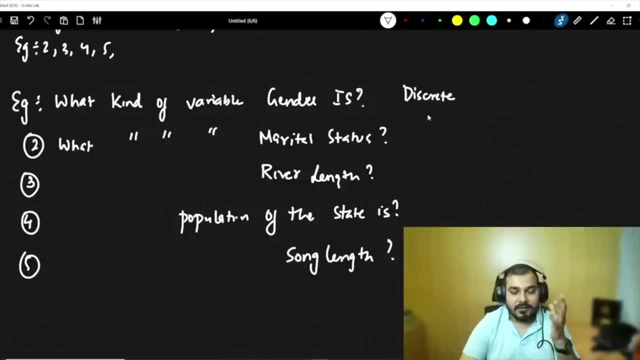 the population of a status. what kind of variable song length is so? gender is obviously a discrete one. um, i'll not say discrete, but i'll say categorical. sorry, not discrete. okay, so it is a qualitative or categorical variable. marital status: again same thing. river length: continuous, if i want. 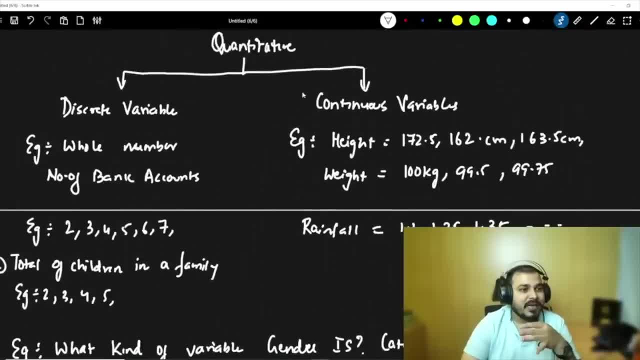 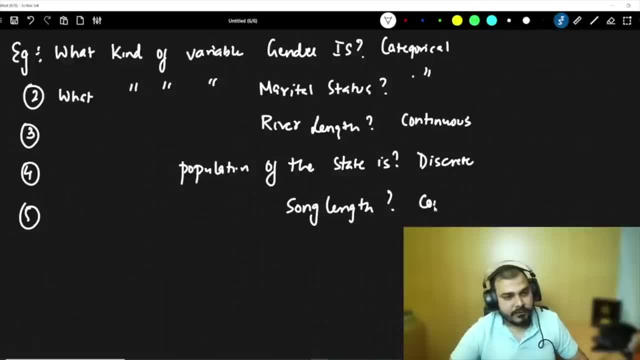 to say discrete, continuous or normal. continuous: it will be a continuous quantitative variable. population of the state: it will be discrete. and song length is what kind of variable marital status is what kind of variable song length is will also be continuous. what kind of variable blood pressure is blood pressure? it will also be. 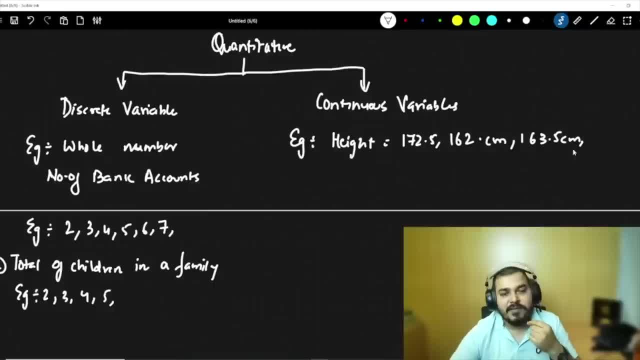 I can say a person is one sixty three point five centimeters, Any value that can come over here. Similarly, With respect to weight, here I can say the person is one hundred kgs. I can say ninety nine point five kgs. 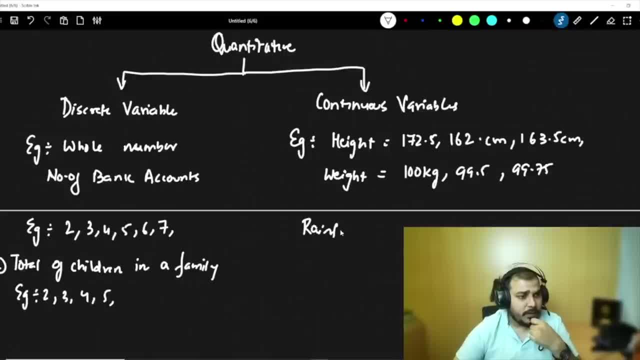 I may say ninety, nine point seven, five kgs. I can also talk about amount of rainfall which is measured in inches. Suppose I say it is one point one inches, one point two, five inches, one point three, five inches. Right, All these things are basically. 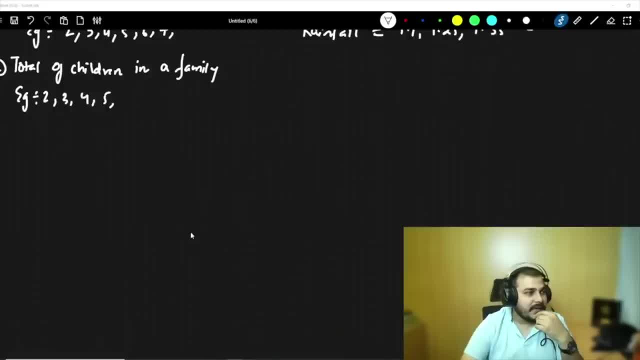 So this was an example with respect to continuous variables. I'll give you some examples. What kind of variable Gender is? What kind of variable Marital status is? What kind of variable River length is? What kind of variable The population of a status? 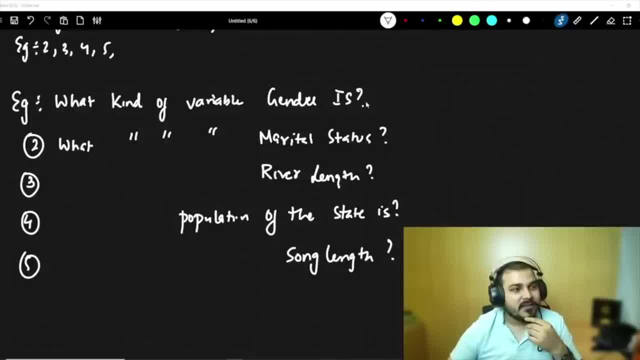 What kind of variable Song length is? So gender is obviously a discrete one. I'll not say discrete, but I'll say categorical. Sorry, not discrete. Okay, So it is a qualitative or categorical variable. Marital status: Again same thing. 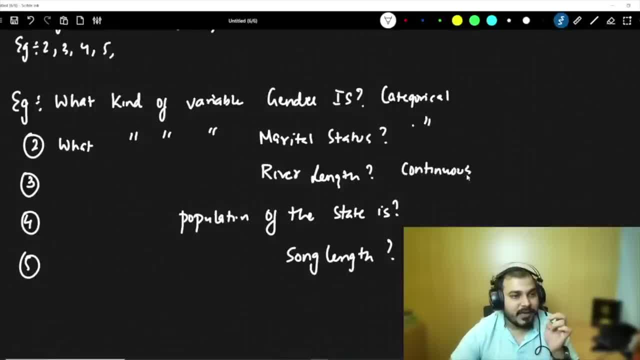 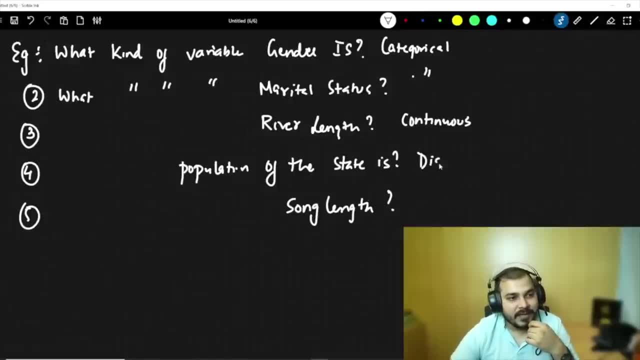 River length Continuous. If I want to say Discrete continuous or normal continuous, it'll be a continuous quantitative variable, Population of the state, It will be discreet and song length will also be continuous. What kind of variable blood pressure is? 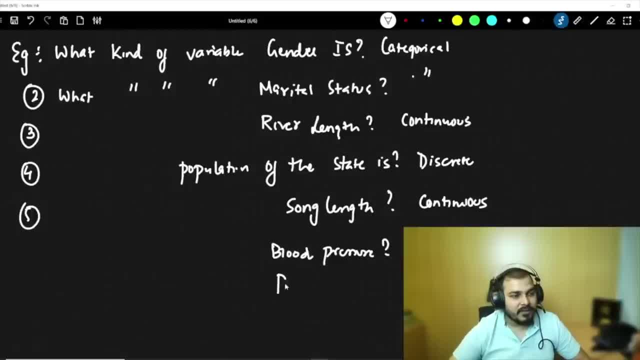 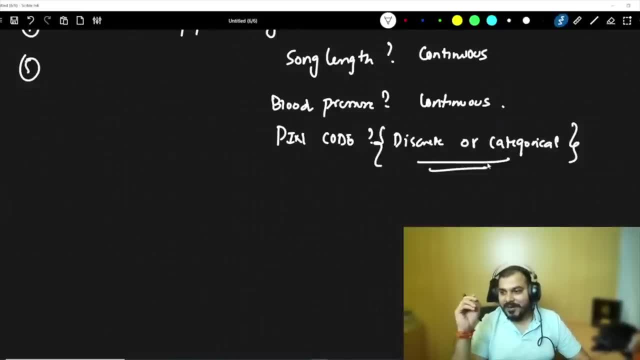 Blood pressure. It will also be continuous. What kind of variable is PIN code? discrete or categorical? Don't worry, As we go ahead in some of the classes, you'll be able to understand this. That is where, when you will be getting a problem statement in data science, where you will be. 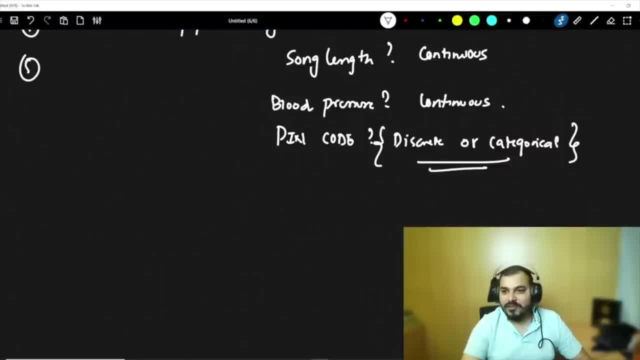 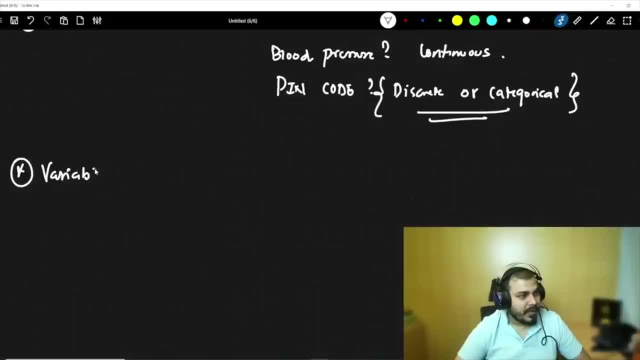 Get a problem statement in data science where you will be able to understand this. Okay, have specifically PIN code in a data set how you are going to handle those. Okay, now let's go to the next one. next topic: Variable measurement. So here we are, probably. 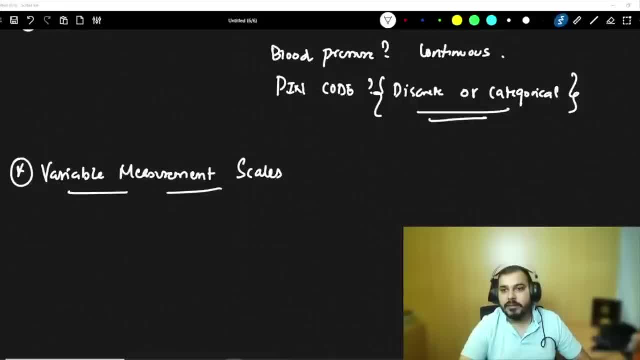 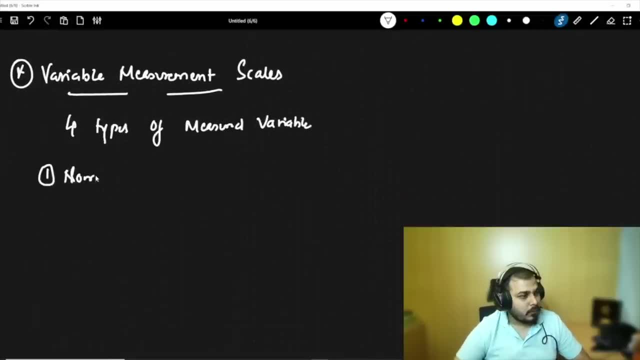 going to understand how do we measure variables. So over here we basically have four different types of measured variable. The first type is nominal, the second type is ordinal, the third type is something called an interval and the fourth type is something called as a ratio. 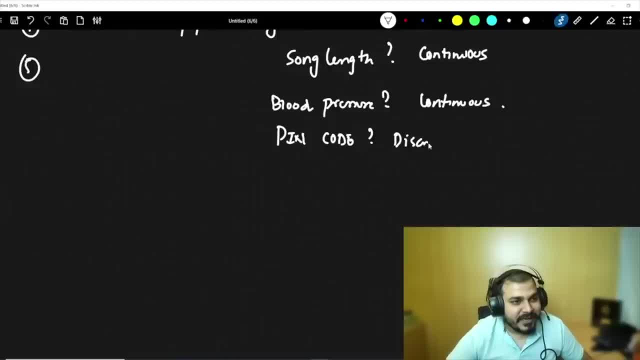 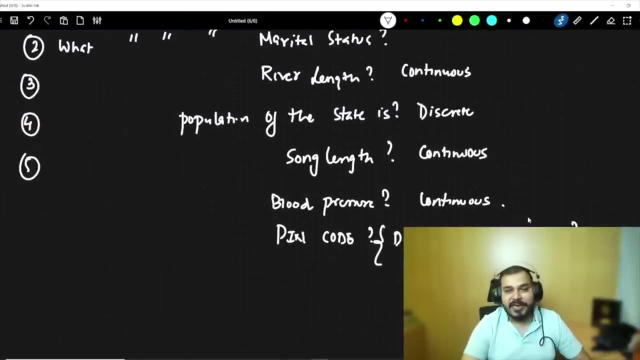 continuous. what kind of variable is pin code? discrete or categorical? don't worry, as we go ahead in some of the classes, you will be able to understand this. okay, that is where, when you will be given a problem statement in data science where you have specifically pin code in a data set, how? 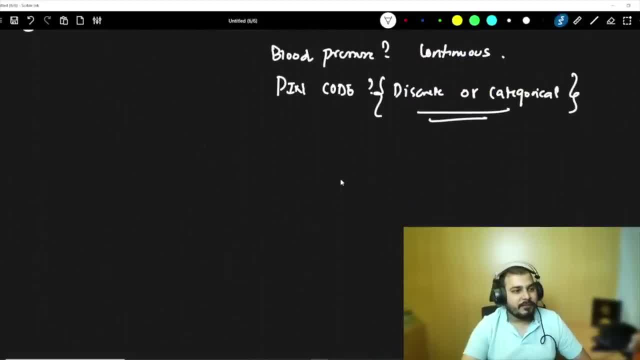 you are going to handle those. okay, now let's go to the next one. next topic: variable measure measurement. so here we are probably going to understand how do we measure variables. so over here we basically have four different types of measured variable. the first type is nominal, the 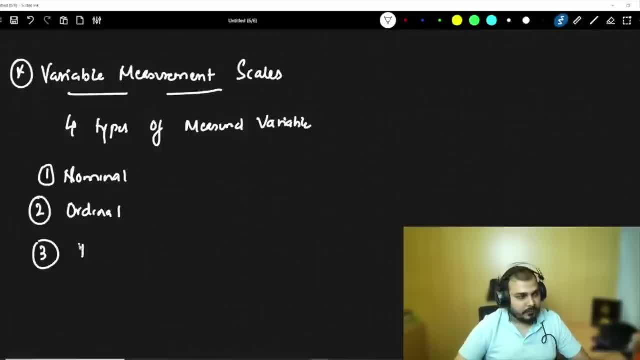 second type is ordinal, the third type is something called an interval and the fourth type is something called as a ratio. now, first of all, we'll try to understand about nominal. probably i'll here also i'm i'm going to give you a lot of examples and why. why it is very much similar to the previous one. 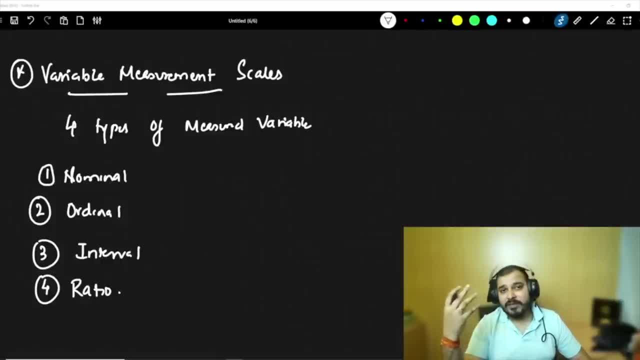 because it is very much necessary to know this kind of measured variables, four type of measurement variables, because your data set will also have this kind of variables. you'll have nominal data, you'll have ordinal data, you will have internal data. it's for interval data ratio related data. 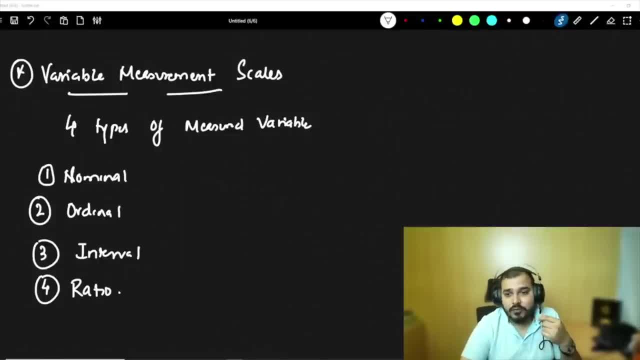 so that you'll be able to do a good data analysis. okay, so you basically use this kind of variables. so if i talk about nominal variable, so nominal uh data also, i can say these are specifically categorical or qualitative data. when you talk about categorical data, you know that it is split into different, different classes. 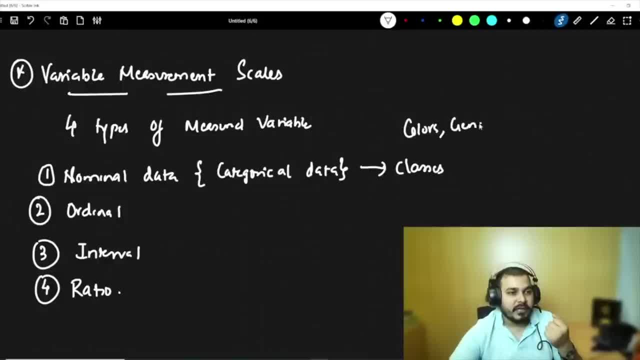 colors. color is one example. you have example. gender, you have example. different, different things, type of flower. these are some of the examples with respect to the nominal data, because the first thing i've heard this: a interviewer asking what is the difference between ordinal and nominal data. now let's go ahead and let's discuss about ordinal data in order to 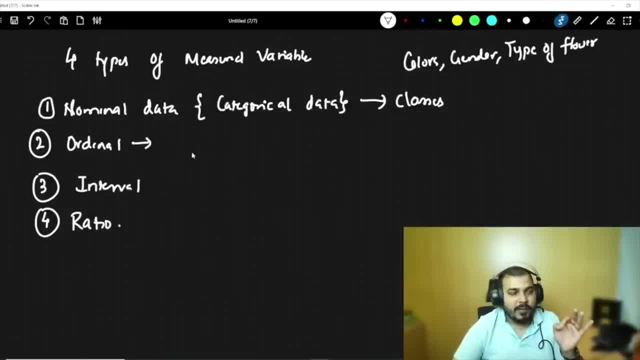 understand ordinal data. i'd like to say some example here over here. in this particular data, the order of the values, the order of the data matters, but value does not. i'll talk about it why i'm saying value does not. let's say that i have five students and here the marks of 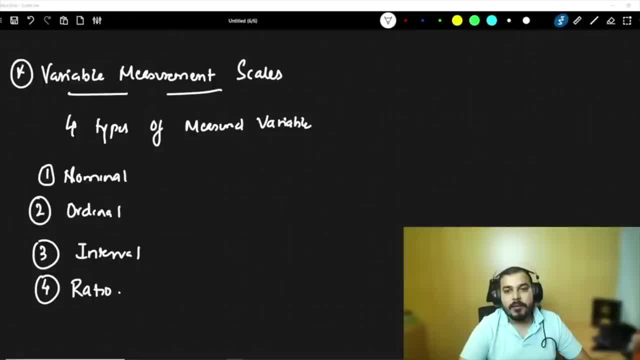 Now, first of all, we'll try to understand about nominal Probably here also I'm going to give you a lot of examples and why. why it is very much necessary to know this kind of measured variables, four type of measured variables, Because your data set will also have this kind of variables. 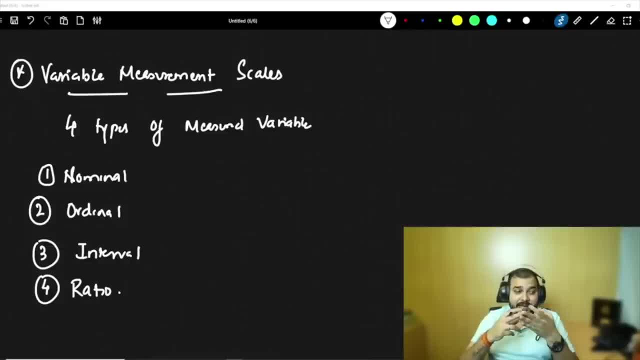 You'll have nominal data, you'll have ordinal data, you'll have internal data- it's or interval data, ratio related data, so that you'll be able to do a good data analysis. Okay, so you basically use this kind of variables. So, if I talk about nominal, 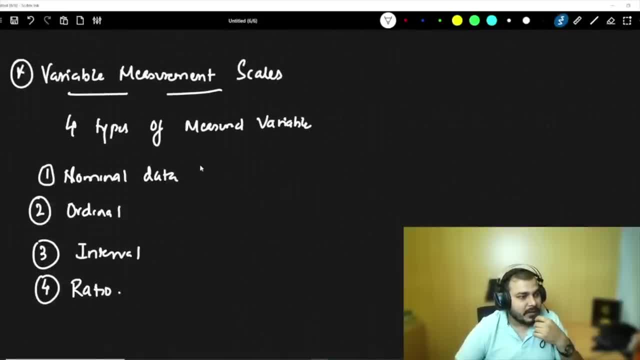 variables. so nominal data also, i can say these are specifically categorical or qualitative data. so whenever i say categorical data, you know that it is split into different, different classes: colors, color is one example. you have example. gender, you have example different different things, type of flower. these are some of the examples with respect to the nominal data, because the first thing i've 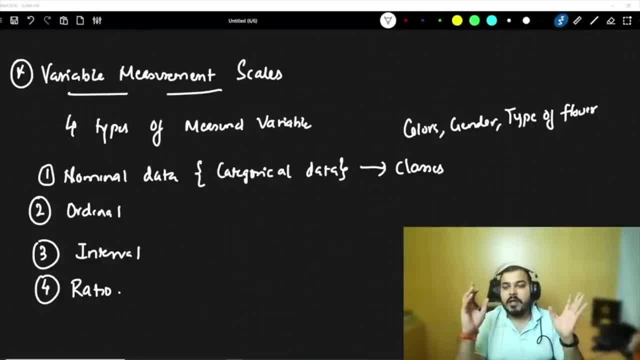 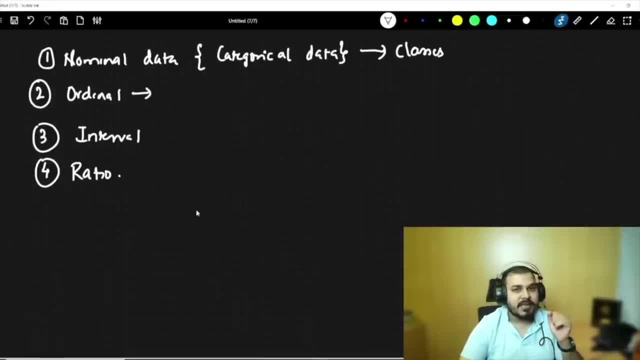 heard this interviewer asking what is the difference between ordinal and nominal data. now let's go ahead and let's discuss about ordinal data. in order to understand ordinal data, i would like to say some example here over here, in this particular data, the order of the values, the order. 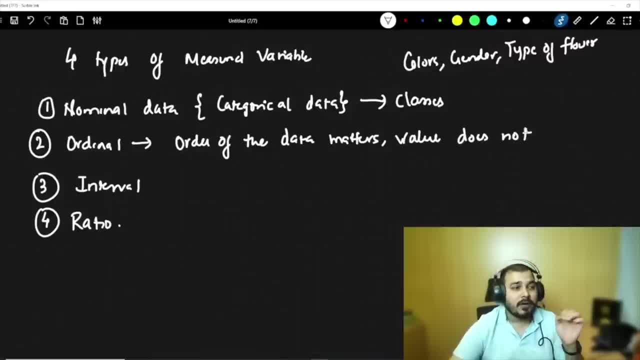 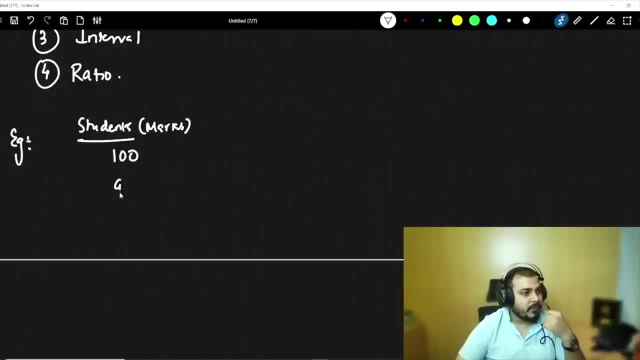 of the data matters, but value does not. i'll talk about it why i'm saying value does not. let's say that i have five students and here the marks of the students are like 100, 96, 57, 85, you and 44. now tell me over here if i just try to find out the rank. rank basically means who is. 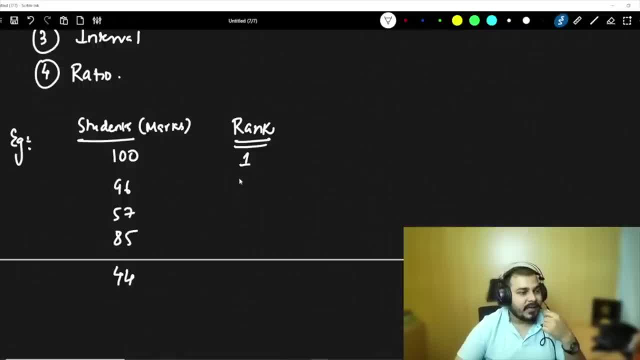 having the highest marks will get the first rank. 96 will then get second, this 85 will get third and this we will get as fourth and this finally will get as fifth. this data that we specifically have is my ordinal data. here we focus more on the order, not on the values. here we mostly focus on 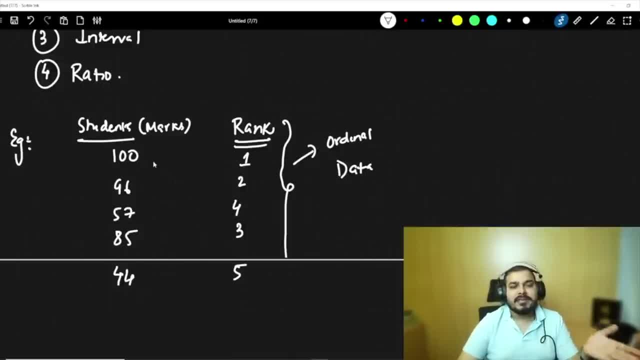 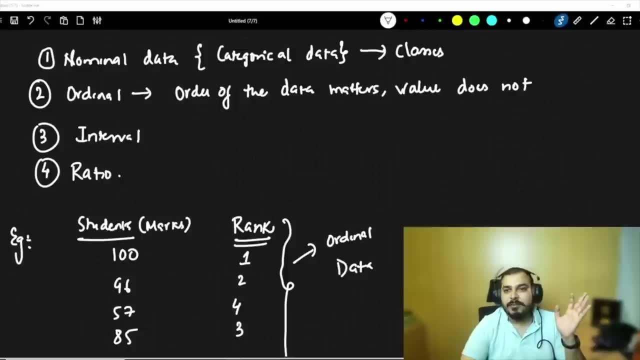 this ranks. we are not worried like what marks that particular person has got. yes, he has got the first rank. so this was with respect to the ordinal data. now let's me let me come towards the so over. here you can basically say that ordinal data will be present and we also use a different technique to analyze. 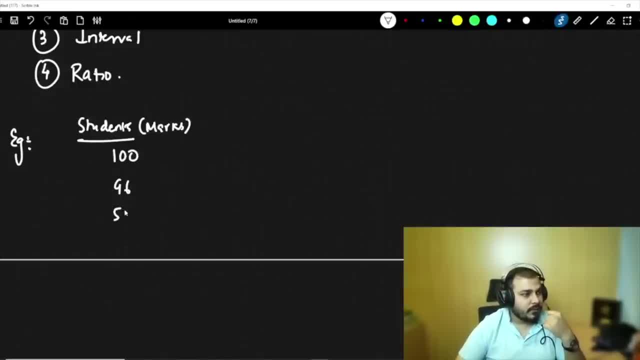 the students are like 100, 96, 57, 85 and 44. now tell me over here if i just try to find out the rank. rank basically means who is having the highest marks will get the first rank. 96 will then get second, this 85 will get third and this we will get as fourth and this, finally, will get as fifth. 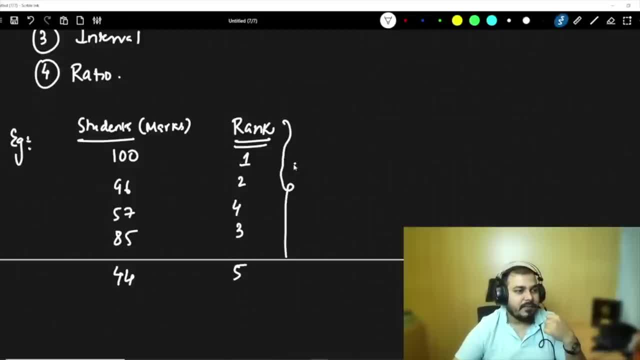 this data that we specifically have is my ordinal data. here we focus more on the order, not on the values. here we mostly focus on this. ranks- we are not worried like what marks that particular person has got. yes, he has got the first rank. so this was with respect to the. 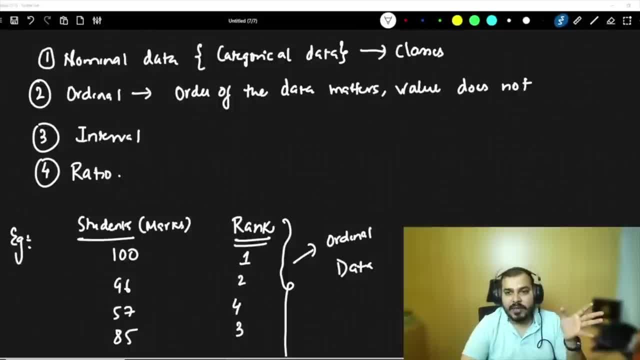 ordinal data. now let's me, let me come towards the so over here you can see that i have a rank of 85 and this 85 will get third and this we will get as fourth, and this we can basically say that ordinal data will be present and we also use a different technique to 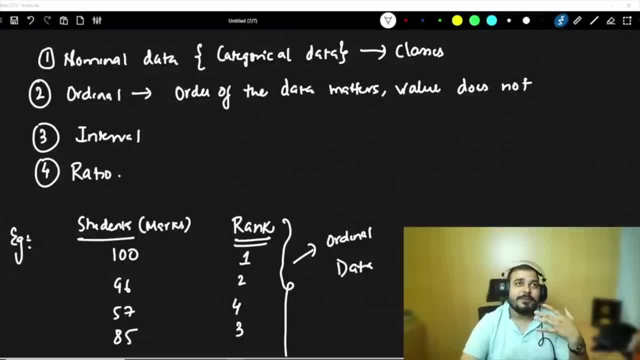 analyze those data and probably we try to. probably, when we'll be seeing some data set in the future, we will probably try to see that. okay scenarios also. now, interval, interval data. here the order matters, here the value also matters, and one thing is that your natural zero is not present. what is? 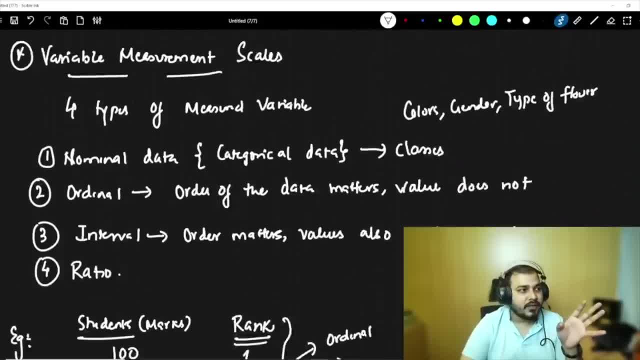 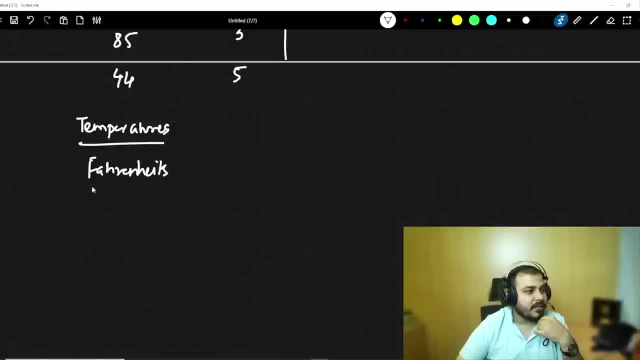 natural zero here. order also matters, values also matter. so if i take an example of interval, let's say that i have an interval of temperatures and let's consider fahrenheit- fahrenheit temperature i'm just talking about. i may have values like this: 70 to 80 fahrenheit. 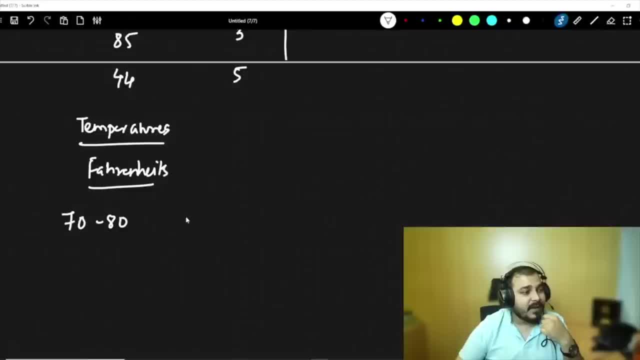 into 80 to 90 fahrenheit, or i may have 70 to 80 fahrenheit, 80 to 90 fahrenheit. here interval, is there definitely some kind of values? are there 90 to 100 fahrenheit, but if i say zero fahrenheit? 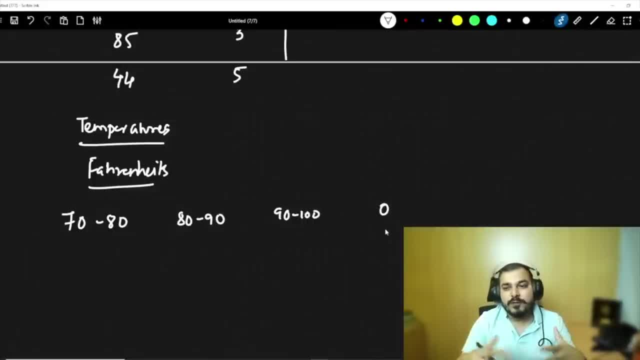 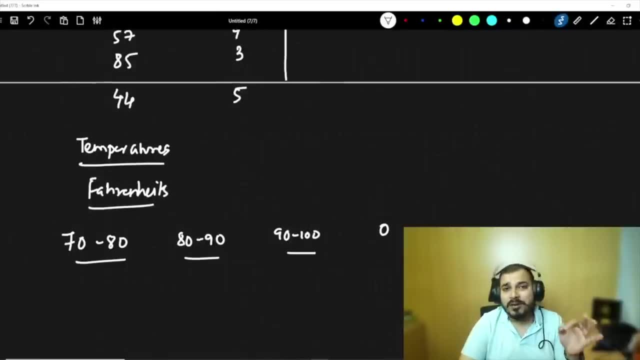 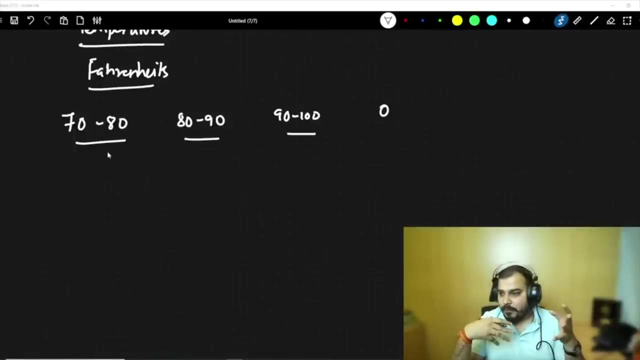 it won't. it won't basically make a useful meaning in this. so definitely. this is basically called as an interval. you can here, You have some range of values between them and the order also basically matters a lot. I may also have distance- 10 to 20,, 20 to 30,, 30 to 40, where probably this interval data. 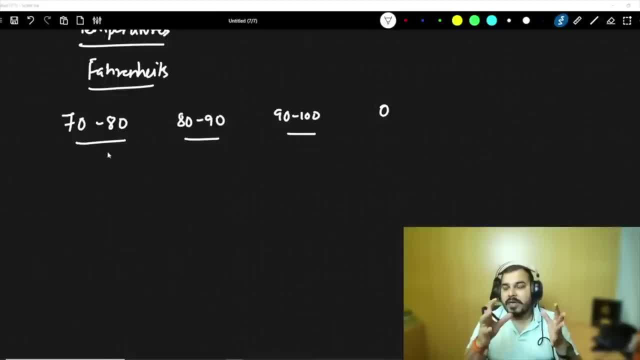 may be used In OLA. I think you have probably booked cabs. You book the cab for, let's say, you're booking the cab for six hours there. they'll be saying that you can actually go till zero to 60.. 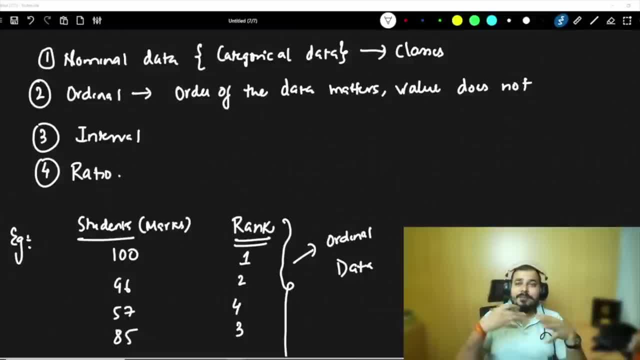 those data and probably we try to. probably, when we'll be seeing some data set in the future, we will probably try to see that. okay scenarios also now, interval interval data. here the order matters, here the value also matters, and one thing is that your natural zero is not present. what is? 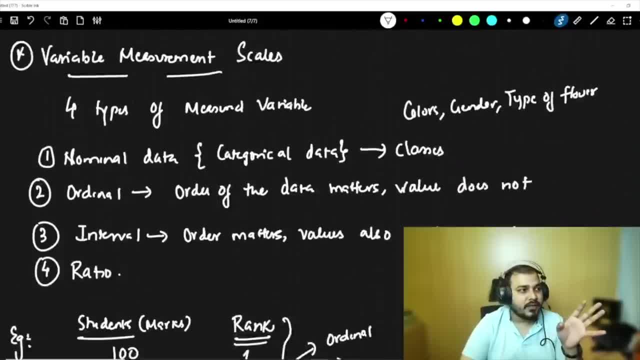 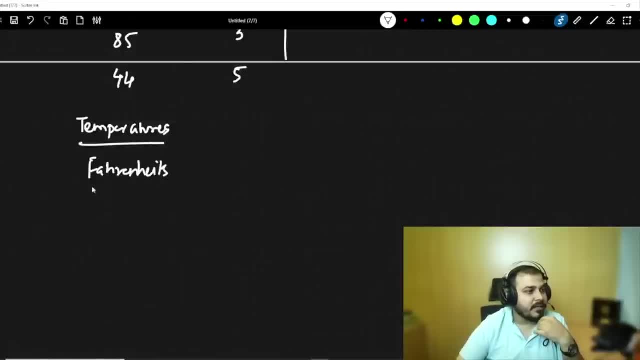 this natural zero here. order also matters, values also matter. so if i take an example of interval, let's say that i have an interval of temperatures and let's consider fahrenheit, fahrenheit temperature i'm just talking about. i may have values like this: 70 to 80 fahrenheit, 80 to 90 fahrenheit, or i may 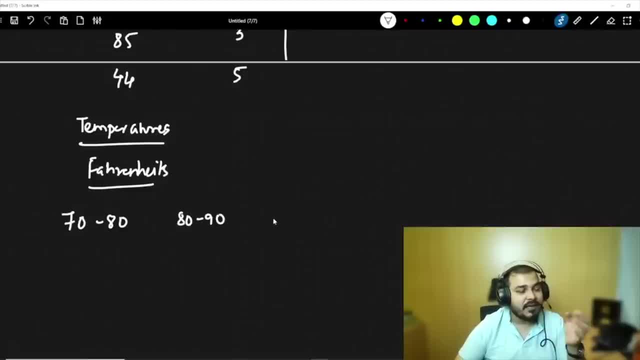 have 70 to 80 fahrenheit, 80 to 90 fahrenheit here interval is there definitely some kind of values? are there 90 to 100 fahrenheit? but if i say zero fahrenheit it won't, it won't basically make a useful meaning in this. so definitely, this is basically called as an interval. you have some. 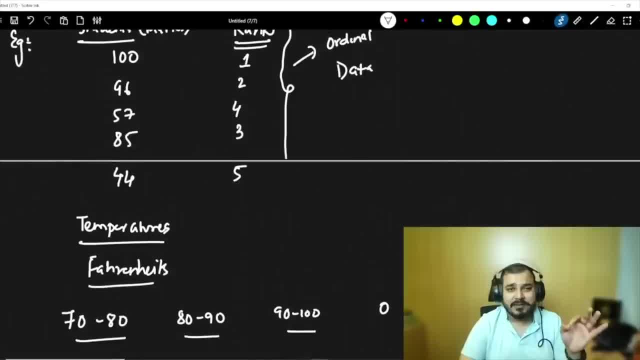 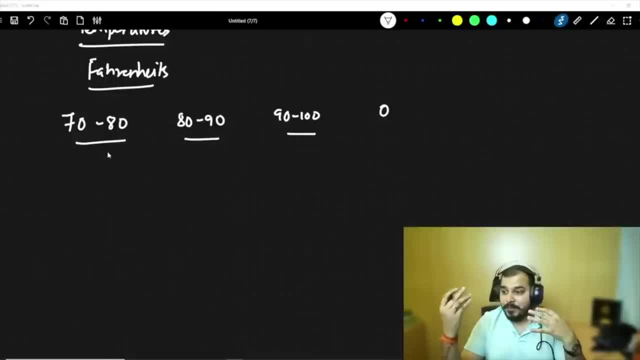 range of values between them and the order also basically matters a lot. i may also have distance- 10 to 20, 20 to 30, 30 to 40- where probably this interval data may be used in ola. i think you have probably booked cabs you book the cab for. let's say you are booking the cab for six hours. 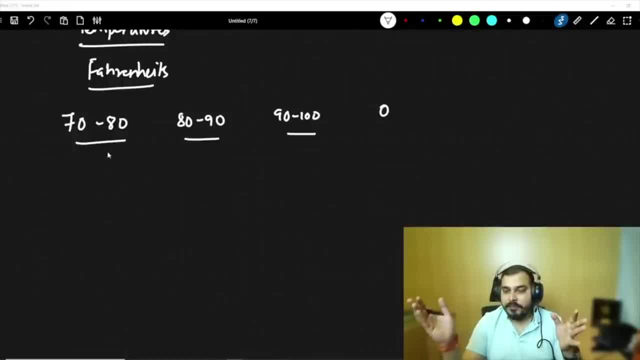 there they'll be saying that you can actually go till 0 to 60, and then you can probably- uh, if you are more than 60, that time you have to pay more. natural zero. zero will not be present, right? zero fahrenheit will not make any difference. now, ratio data will be an assignment for you. let me go ahead. 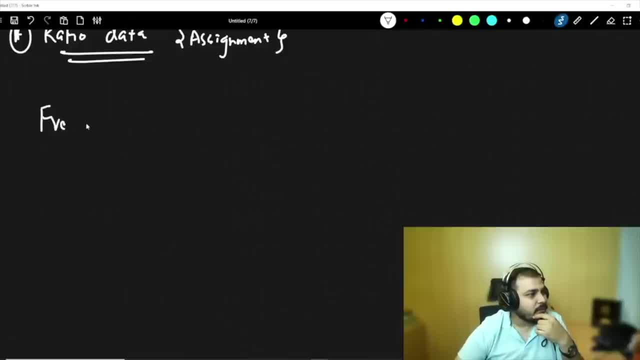 and let me take another topic which is called as frequency distribution. now, this is pretty much important because in the later stages you'll be understanding about histogram and all. let's say that i have a sample data set and suppose in this particular data set i have three types of flowers. 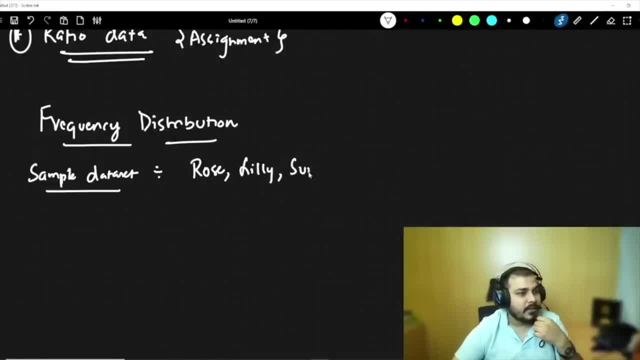 rose, lily and sunflower. now, similarly, in this particular data set i have a lot of flowers like rose, lily, data sunflower, then again i have rose, then again i have lily, then again i have lily. okay, so suppose let's consider that this is my entire data set now, usually for showcasing this. 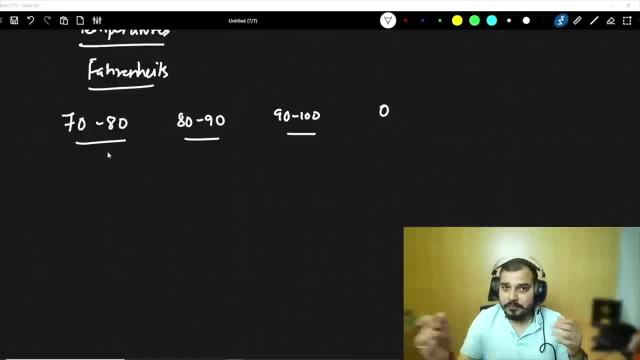 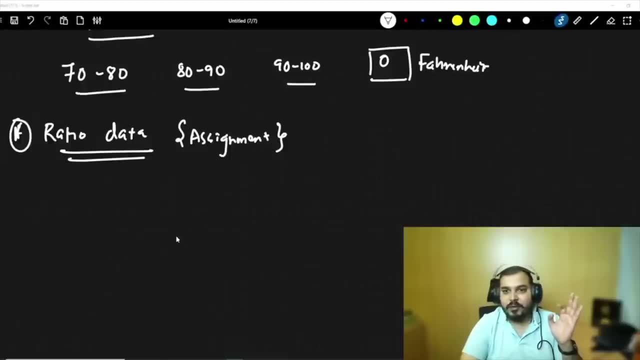 And then you can probably, if you are more than 60, that time you have to pay more money. Natural zero. Zero will not be present, right, The Fahrenheit will not make any difference. Now, ratio data will be an assignment for you. 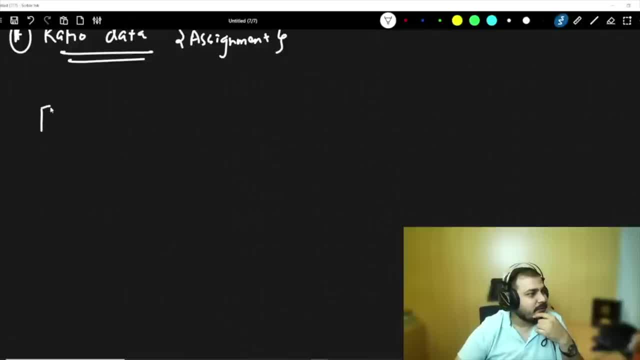 Let me go ahead and let me take another topic, which is called as frequency distribution. Now, this is pretty much important because in the later stages you'll be understanding about histogram and all. Let's say that I have a sample dataset and suppose in this particular dataset I have 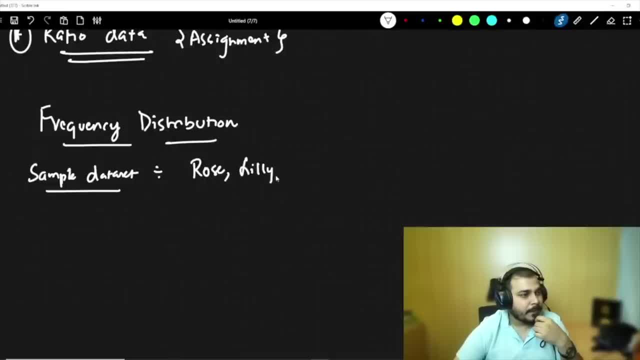 three types of flowers: rose, lily and sunflower. Now, similarly, in this particular dataset, I have a lot of flowers like rose, lily, sunflower, then again I have rose, then again I have lily, then again I have lily. 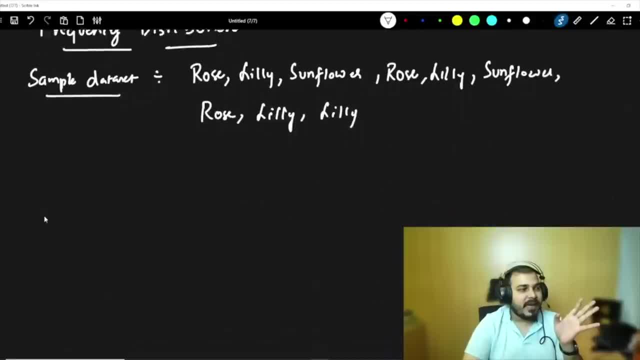 Okay, So suppose let's consider that this is my entire dataset. Now, usually for showcasing this dataset in some kind of visualized manner, we can basically use this frequency distribution table based on the flower type and how much is the frequency. Okay, And this will be very much important. 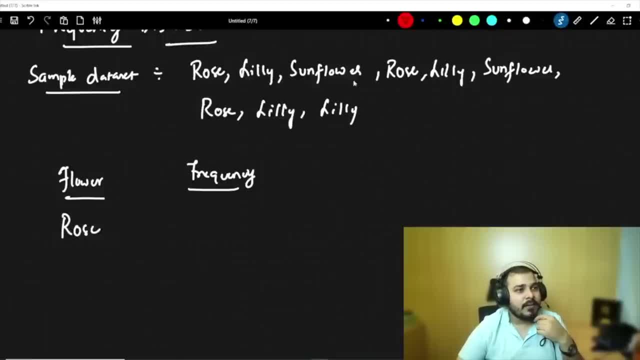 Suppose, if I say rose In rose, how many types I have? One, two, three, Okay, Okay. So three is the count of rose If I consider lily, so lily, what is the basic count? I'm basically having one, two, three, four. 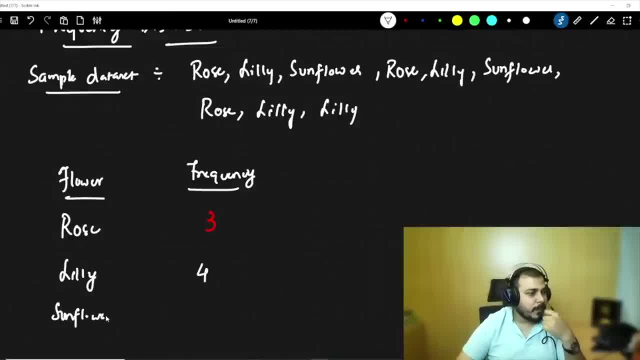 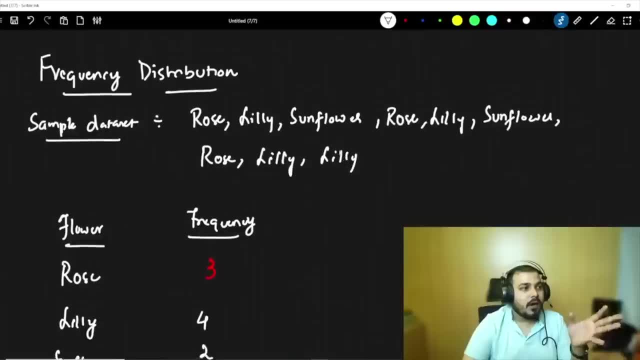 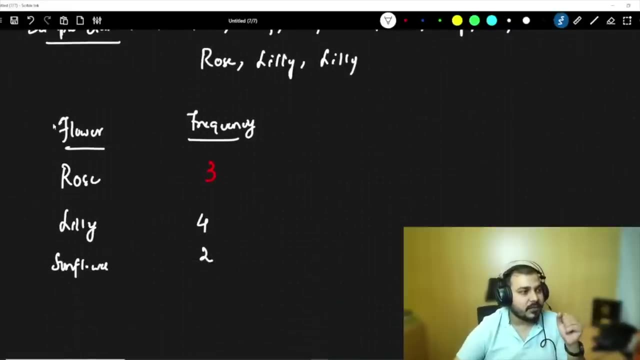 So four is the count. If I consider sunflower, what is the count? One and two. So this is the frequency of this particular values, of this particular dataset with respect to different, different categories. Okay, So here you can see that I this is entirely frequency distribution table. 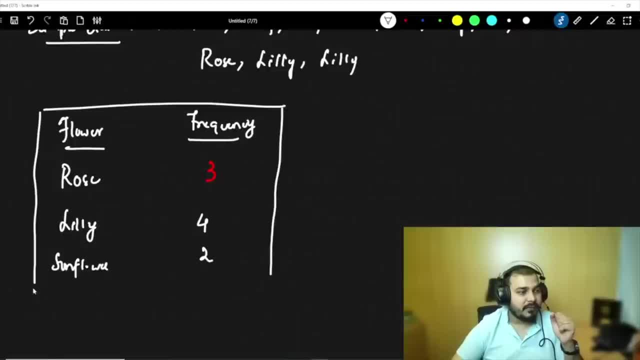 And from this table you can derive bar charts, You can derive pie charts, You can derive different, different things. Now one more topic. Now this: you know that it is a frequency distribution, but there is something called us cumulative frequency. 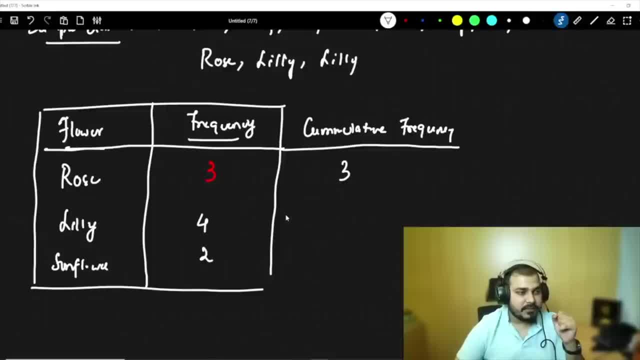 Cumulative frequency basically says that initially I have rose, three flowers, Then I'm going to add this to this, So it will be seven, Then I'm going to add this to this, It will be nine. At the end of the day, when we go with respect to cumulative frequency and when we go to 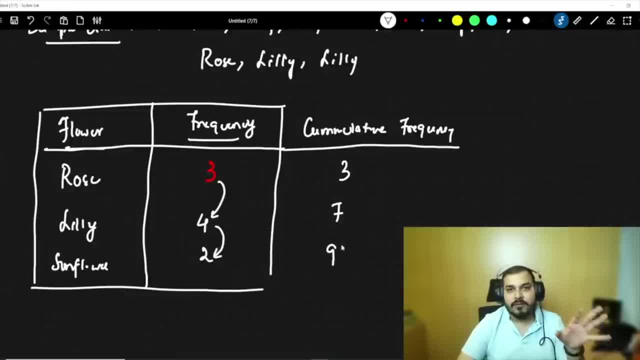 the last category, We'll be able to find out how many total number of flowers are present. This is basically the cumulative frequency. The frequency is getting added And finally you'll be able to see the cumulative frequency of it Now, what we can basically derive from this. I'll just show you an example. 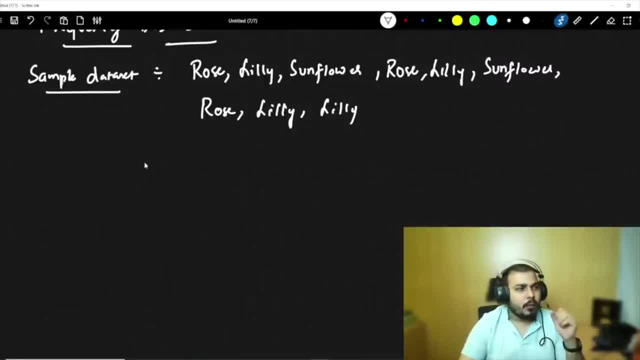 uh, data set in some kind of visualized manner. we can basically use this frequency distribution based on the flower type and how much is the frequency? okay, and this will be very much important. suppose if i say rose in rows are how many types i have: one, two, three. so three is the. 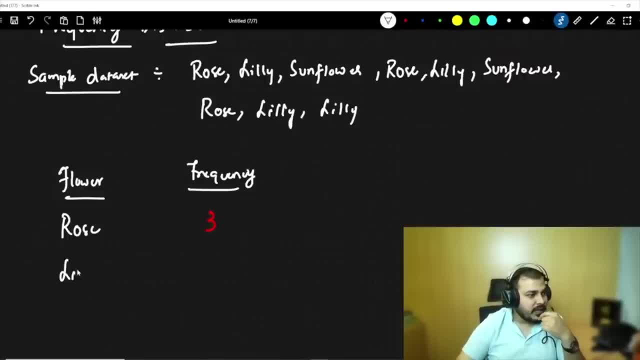 count of rows. if i consider lily, so lily, or what is the basic count? i am basically having one, two, three, four. so four is the count. if i consider sunflower, what is the count? one and two. so this is the frequency of this particular values. 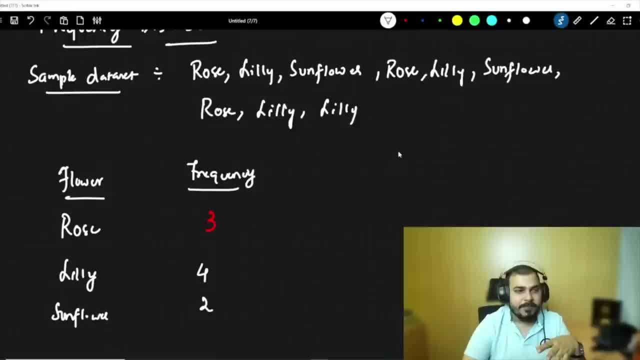 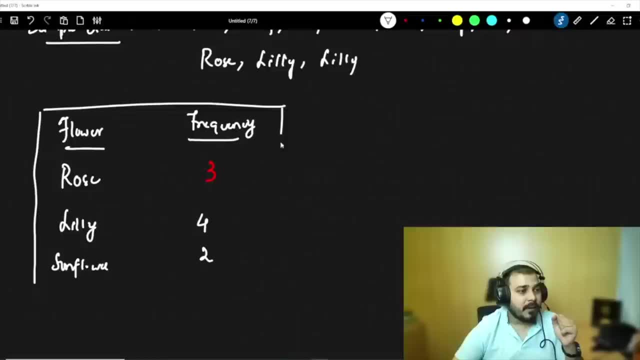 of this particular data set with respect to different, different categories. okay, so here you can see that i this is entirely frequency distribution table, and from this table you can derive bar charts, you can derive pie charts, you can derive different, different things. now one more topic, now this: you know that it is a frequency distribution, but there is something. 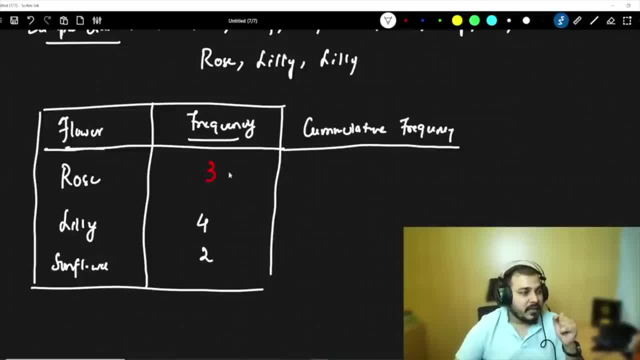 called as cumulative frequency. cumulative frequency basically says that initially i have rose, three flowers. then i am going to add this to this, so it will be seven, then i am going to add this to this, it will be nine at the end of the day when we go with respect to cumulative 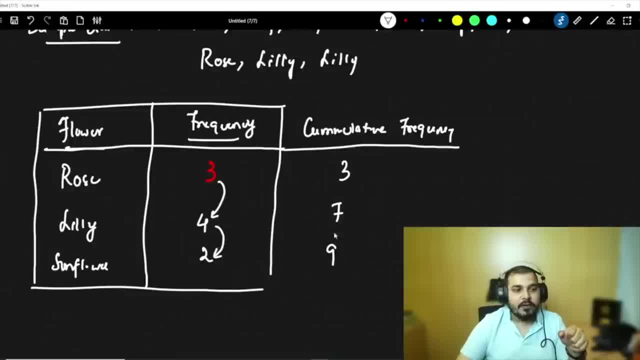 frequency, and when we go till the last category, we will be able to find out how many total number of flowers are present. this is basically the cumulative frequency. the frequency is getting added and finally you will be able to see the cumulative frequency over here. now what we can. 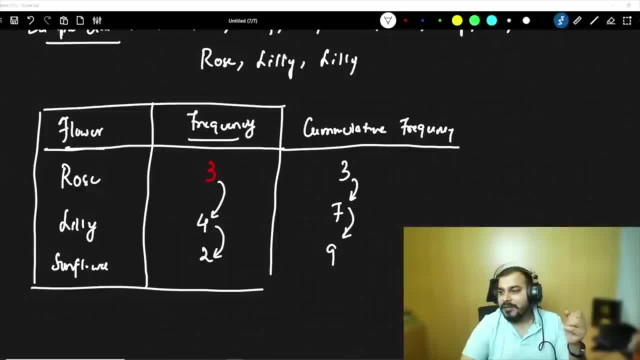 basically derive from this. i'll just show you an example. there is something called as by uh, bar, bar graphs and pie charts. so that particular part now we'll try to draw from this and we'll try to see that. how does it look like in the case of discrete variable? we 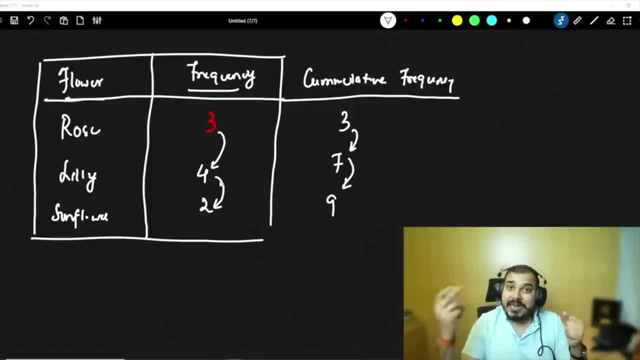 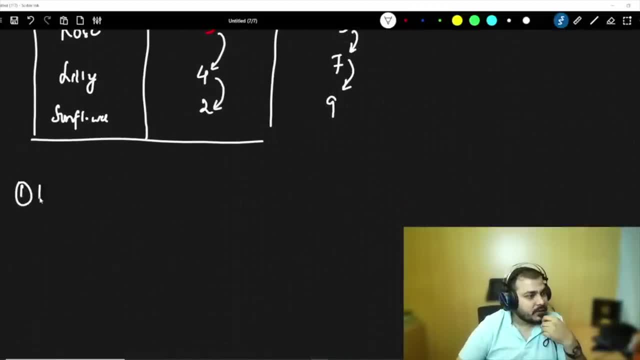 can definitely draw a bar chart. if the variable is continuous at that point of time, we can draw a continuous, we can draw a histogram. so let me just talk about bar graph. so first one is the bar graph. in bar graph, in the x-axis i will probably have all my flowers, so this is rose. 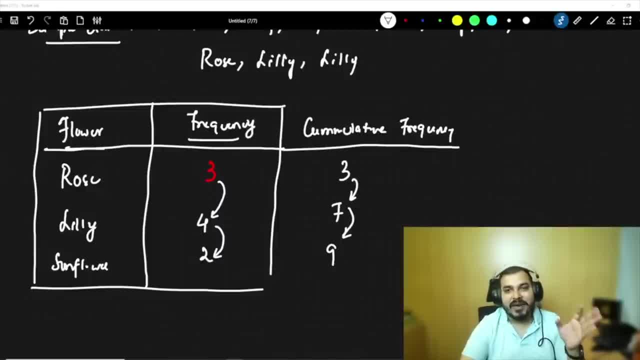 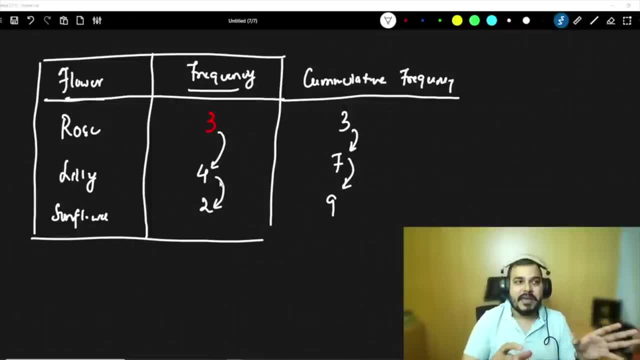 There's something called as bar graphs and pie charts. So that particular part now we'll try to draw from this And we'll try to see that. how does it look like? In the case of discrete variable, we can definitely draw a bar chart. 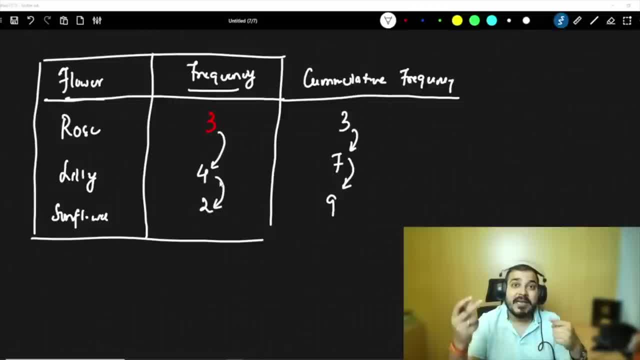 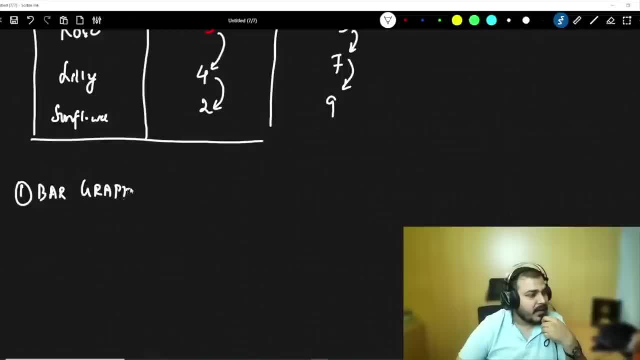 If the variable is continuous, At that point of time we can draw a continuous, we can draw a histogram. So let me just talk about bar graph. So first one is the bar graph In bar graph in the x-axis. I will probably have all my flowers. 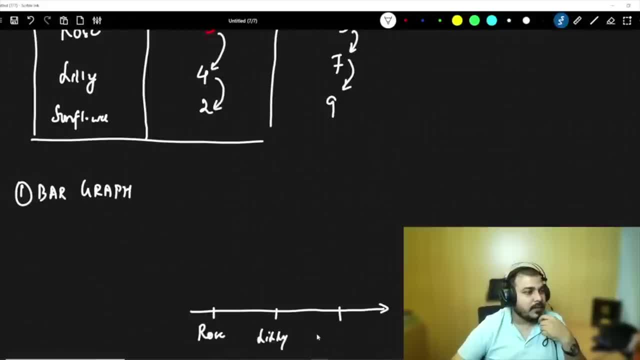 So this is the rose, this is lily and this is sunflower In the y-axis. I will probably have frequency, So this will be my value: one, two, three. Obviously, I know how many roses are there. Roses are three. 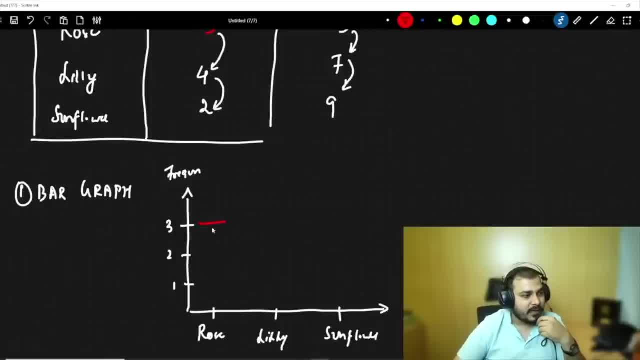 So I'm just going to create this graph over here which will be looking like this. So this is my bar chart for rose. Lilies are obviously four, So I'm going to basically lilies. I may use blue color and this will be my four value. 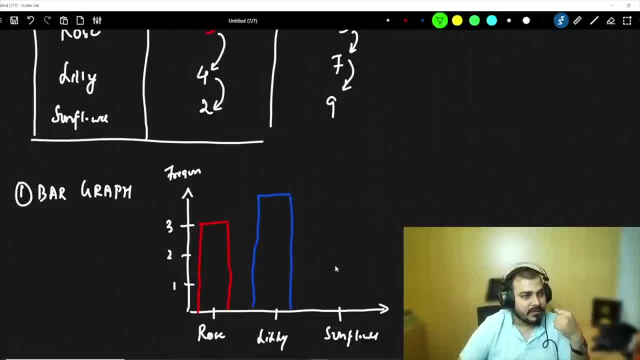 And finally you'll be able to see sunflower. This will be sunflower. Let's say, sunflower is only two, So I'm going to create this. This specific diagram is basically called as bar chart From this. why do we use it? 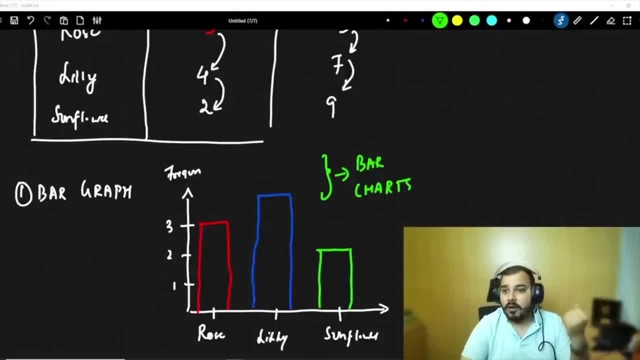 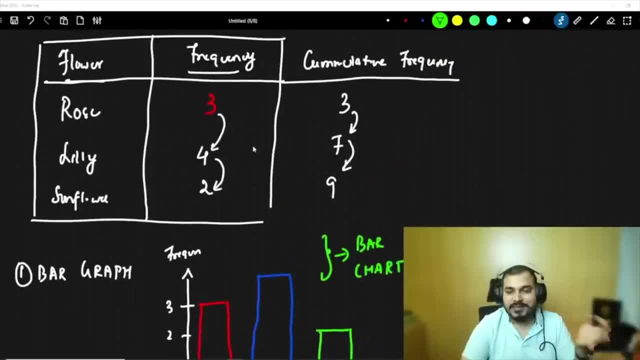 As I said, summarizing the data. This is still the part of descriptive statistics, So this is how you basically define it. Here you can see that the values is discrete variables. Now what if I consider the next example, which is called as histograms? 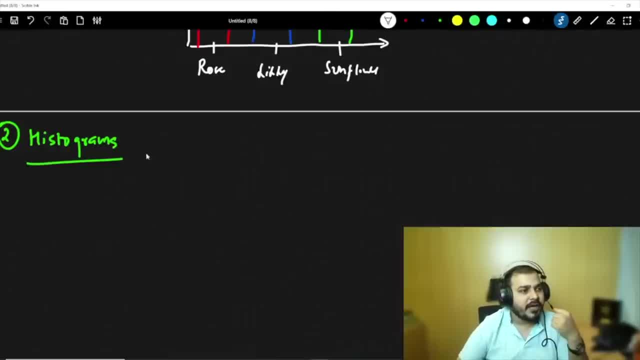 Now, in the case of histogram, how do we define? First of all, your data should be continuous. It can be discrete continuous. It cannot be discrete continuous. Let's take one example of age. Suppose I have a data set of ages and I have values like 10,, 12,, 14,, 18,, 24,, 26,, 30,, 40,. 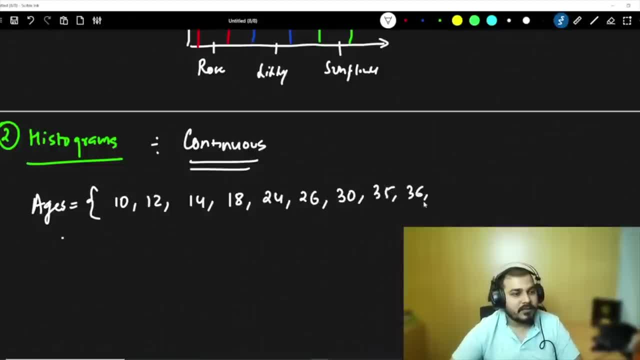 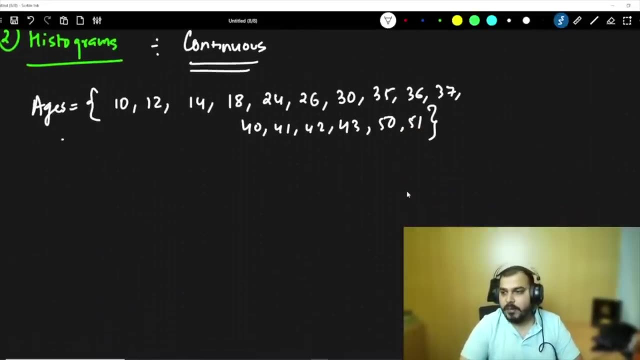 50, 60, 70.. 30,, 35,, 36,, 37,, 40,, 41,, 42,, 43 and 50, 51. So suppose, if I have this specific ages Now here, you know that it is a continuous value. 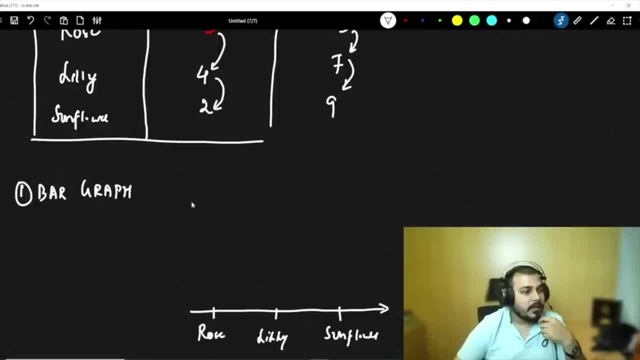 this is lily and this is sunflower in the y-axis. i will probably have frequency, so this will be my value: one, two, three. obviously i know how many roses are there. roses are three, so i'm just going to create this graph over here which will be looking like: so this is my bar chart for rose. 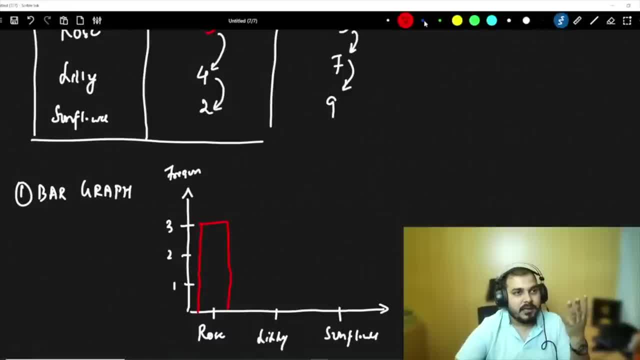 lilies are obviously four, so i'm going to basically lilies. i may use blue color and this will be my four value and finally you'll be able to see sunflower. this will be sunflower. let's say, sunflower is only two, so i'm going to create this. this specific diagram is basically called as: 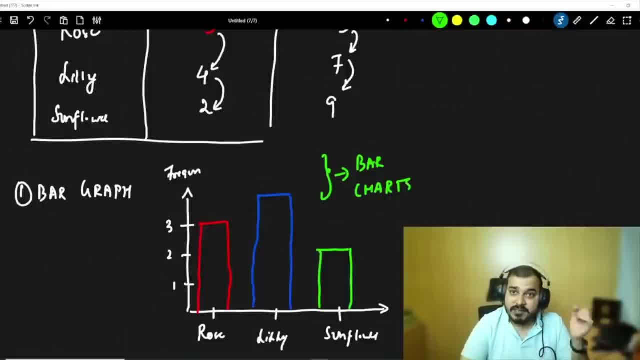 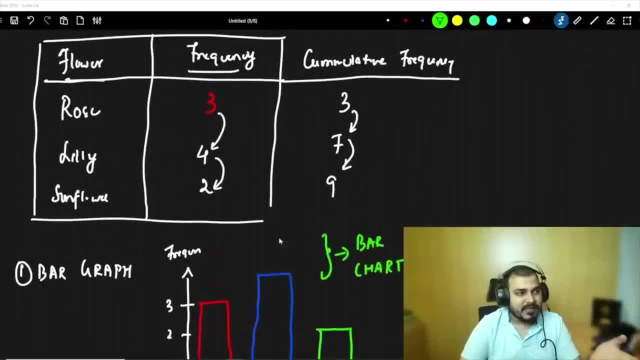 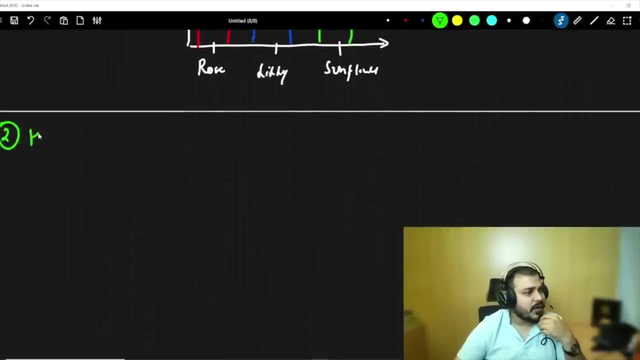 why do we use it? as i say, summarizing the data, this is still the part of descriptive statistics- descriptive statistics. so this is how you basically define it. here. you can see that the values is discrete variables. now, what if i consider the next example, which is called as histograms? 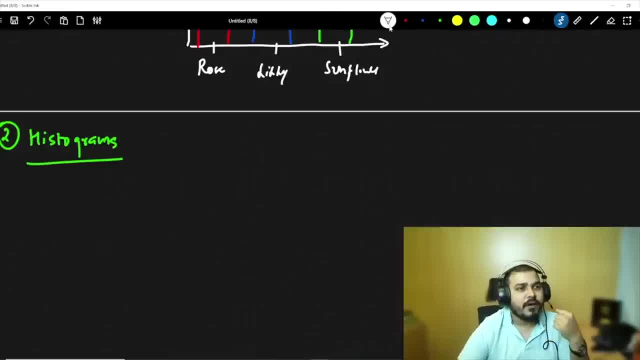 now, in the case of histogram, how do we define? first of all, your data should be continuous. it can be discrete continuous. it cannot be discrete continuous. let's take one example of age. suppose i have a set of ages and i have values like 10, 12, 14, 18, 24, 26, 30, 35, 36, 37, 40, 41, 42, 43 and 50, 51. okay, 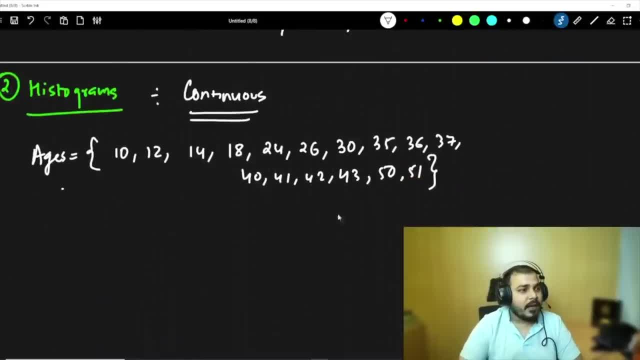 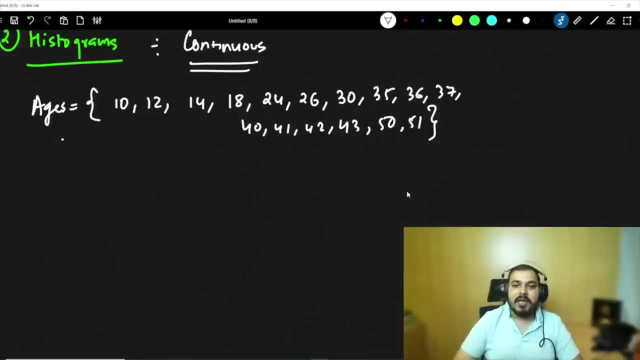 so suppose, if i have this specific ages, okay, now here you know that it is a continuous value. now, in the case of continuous value, if you want to represent it through some diagrams for the data, you can basically use something called as histograms. you can basically use histograms. so 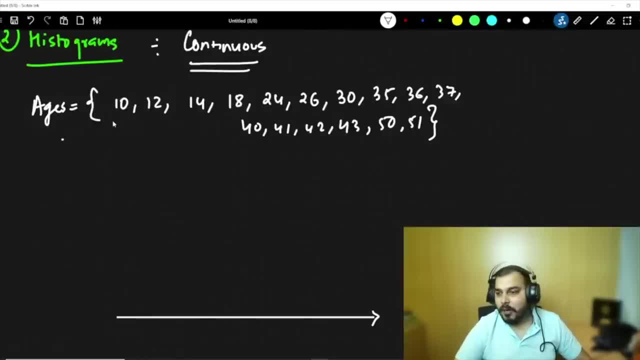 the histogram will have like this: now understand one very important thing: in histogram we make something called as bins. bins basically means we make some kind of grouping. by default, the bin size is usually 100, sorry, 10.. now, if i really want to make this bins, what i'll do in the y-axis: 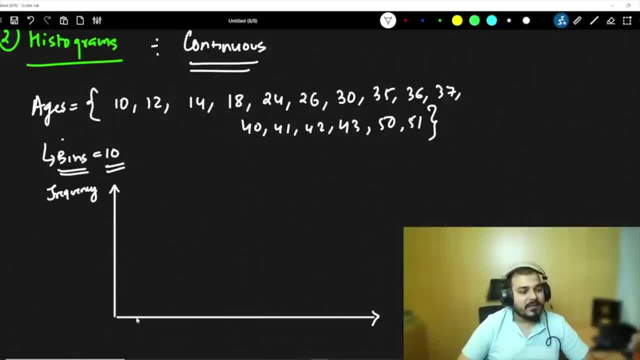 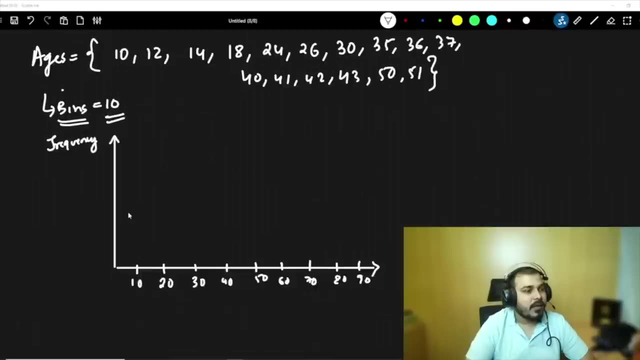 i will be having the frequency. obviously you will know this. now let's make the bin. i told you 10 will be the bin size: 30, 40, 50, 60, 70, 80, 90. you can change the bin value also between 0 to 10. 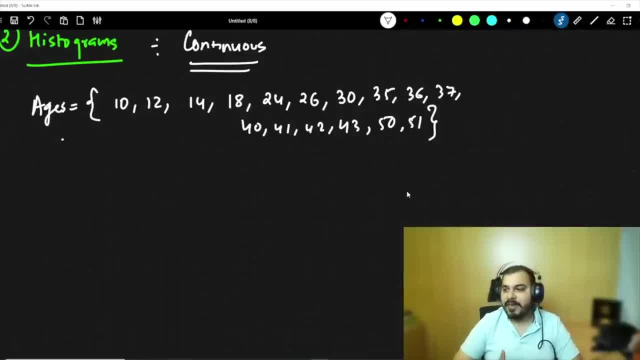 Now, in the case of continuous value, if you want to represent it through some diagram for the data analysis purpose, you can basically use something called as histograms. You can basically use histogram. So the histogram will have like this: Now understand one very important thing. 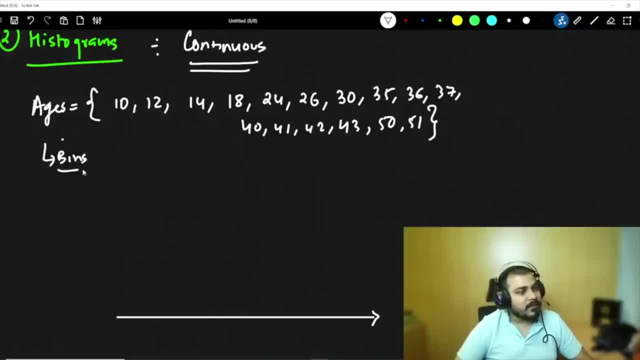 In histogram we make something called as bins. Bins basically means we make some kind of grouping. By default, the bin size is usually 10.. Now, if I really want to make this bins, what I'll do in the y-axis I will be having 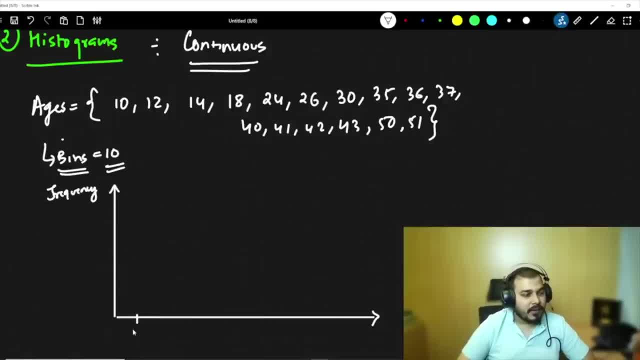 the frequency. Obviously, you'll know this. Now let's make the bin. I told you 10 will be the bin size: 30, 40, 60.. 50, 60, 70,, 80,, 90.. 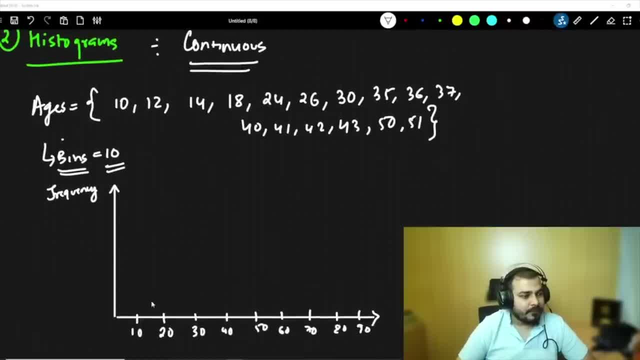 You can change the bin value also Between 0 to 10, between 0 to 10,. I don't have any value, So I'm not going to create it. So let's see that 1 is there, 2 is there, 3 is there, 4 is there and 5 is there. 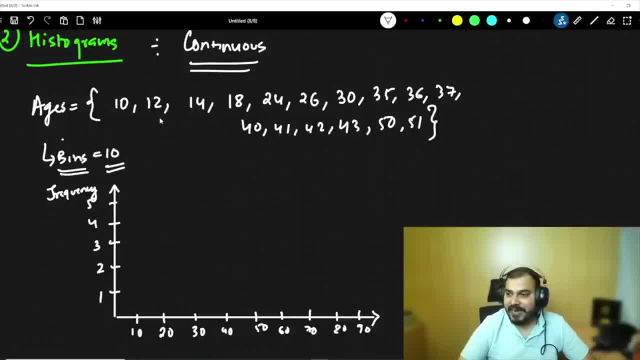 Okay, so this is my frequency count. Now, between 10 to 20, I have how many values? 1,, 2,, 3, 4.. So 4 values. I'm going to create a diagram over here. Between 10 to 20, I have 4 different values. 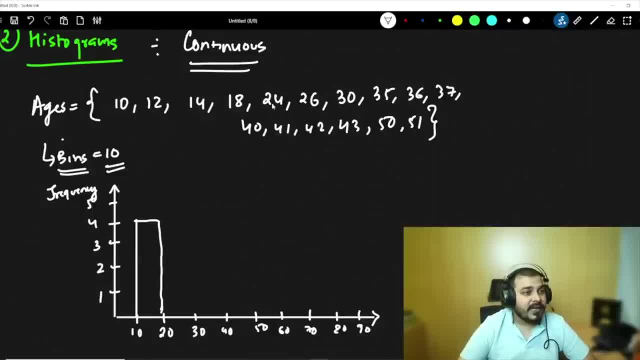 I have 4 different values And then 20 to 30, I have 3 different values: 1,, 2, 3.. Let's consider, I'm going to draw my next diagram. Then I have between 30 to 36, I have 1,, 2, 3.. 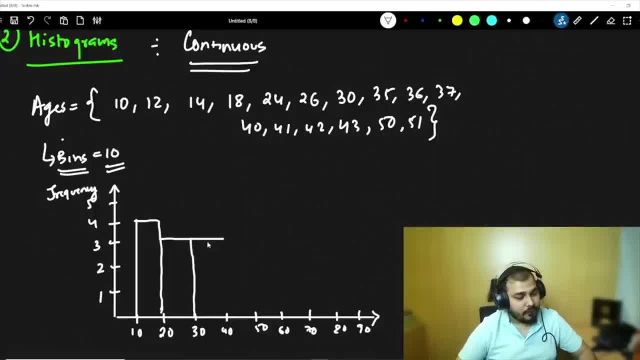 Again, I have 3.. Between 30 to no, sorry, I have 4. Because I'm also going to count 1,, 2,, 3, 4.. Okay, So I'm going to draw my another building over here. 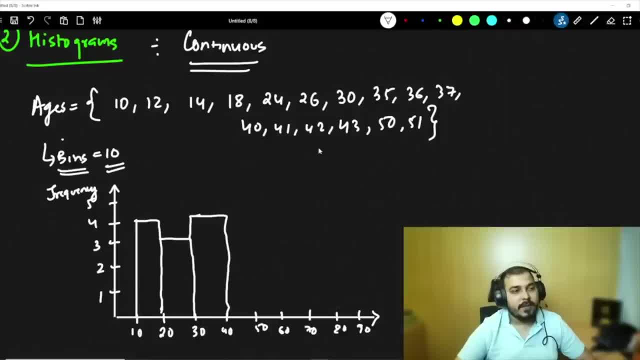 And this building is going to be 4.. Okay, So this building is basically called as histograms. Okay, And then between 40 to 50, I have 1,, 2,, 3,, 4.. Okay, So again I have 4 over here. 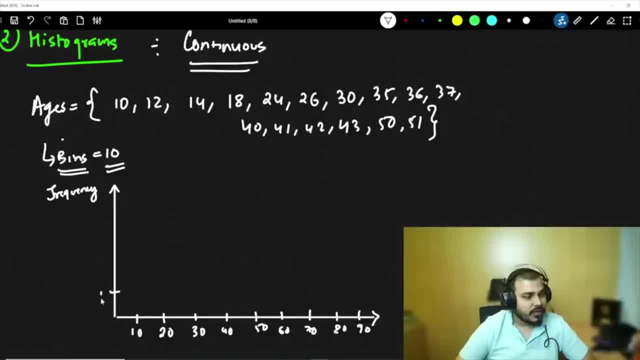 between 0 to 10. i don't have any value, so i'm not going to create it. so let's see that 1 is there, 2 is there, 3 is there, 4 is there and 5 is there. okay, so this is my frequency car now, between 10 to: 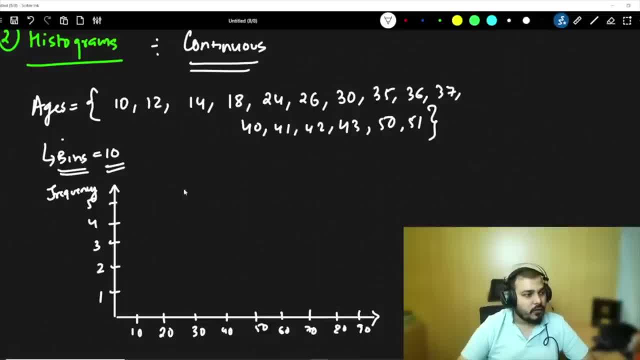 30, i have how many values: 1, 2, 3, 4. so 4 values. i'm going to create a diagram over here. between 10 to 20, i have 4 different values. i have 4 different values, and then 20 to 30, i have 3 different values. 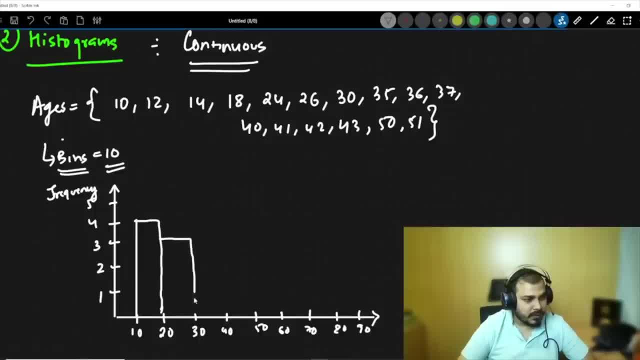 1, 2, 3.. let's consider, i'm going to draw my next diagram. then i have between 30 to 36. i have 1, 2, 3.. again, i have three, between 30 to no, sorry, i have four, because i'm also going to count one, two. 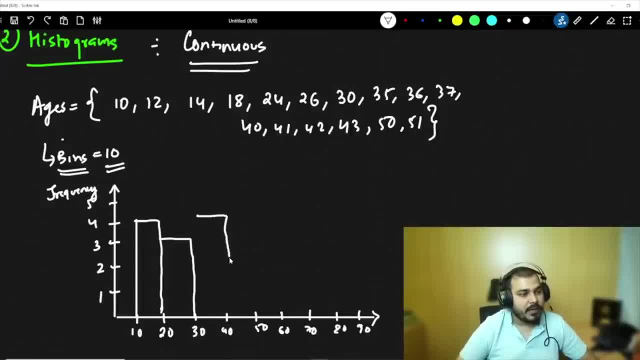 So I am going to draw my another building over here and this building is basically called as histograms. And then, between 40 to 50, I have 1,, 2,, 3,, 4.. So again I have 4 over here. and finally, between 50 to 60, I have 1.. 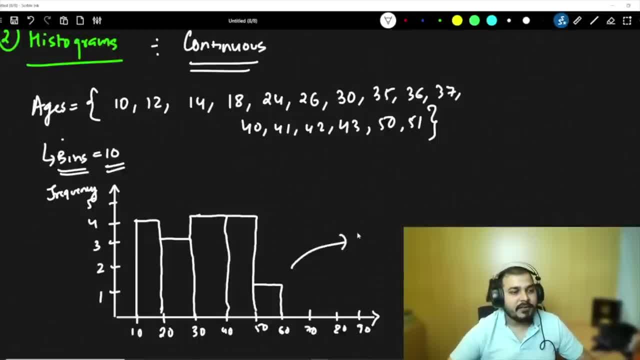 This buildings that you see is basically called as histograms. This building that you basically see is called as histograms And in this histogram your values will be continuous. Now one amazing thing, because people ask about what is PDF. I say that PDF is smoothening of histograms. 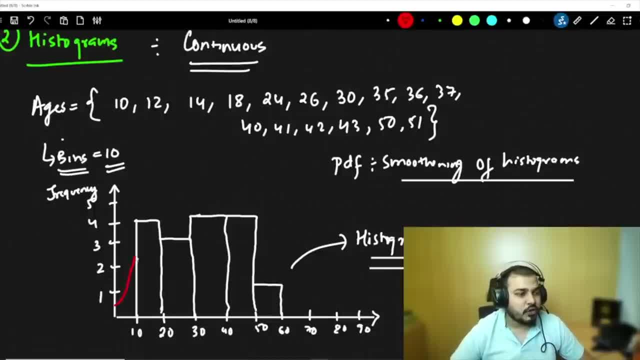 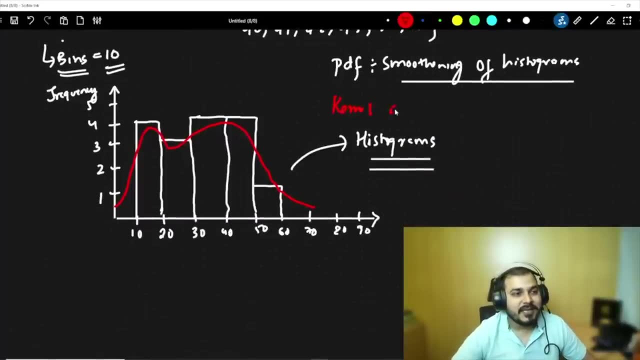 So I will just tell you one example. If I smoothen this histogram, my PDF function will look something like this. Now you may be considering: Krish, how is this basically getting created? Ok, how is this basically getting created? I will say that there is something called as Kernel Density Estimator. 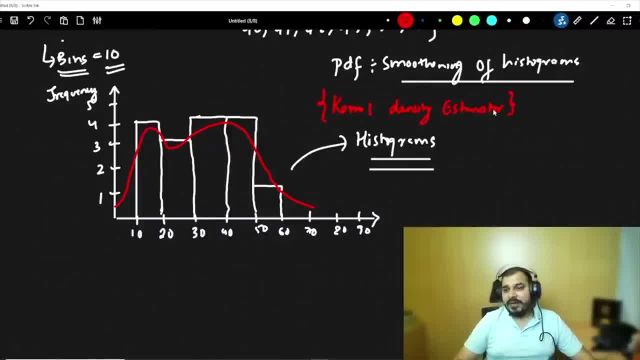 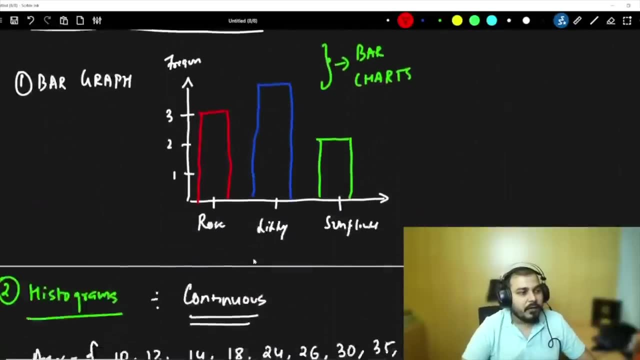 Now this Kernel Density Estimator, how it is done. we will try to understand that in the upcoming classes. Probably that is little bit in the advanced side, But I hope everybody got an idea about histograms. Everybody got an idea about bar graph. Definitely only for ok. tell me what is the difference between bar versus histogram? 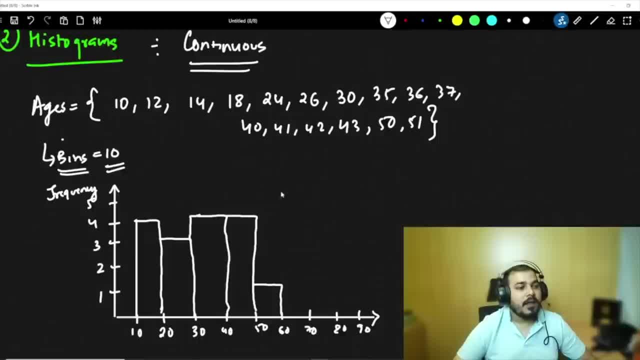 And finally, between 50 to 60, I have 1. This building that you see is basically called as histograms. This building that you basically see is called as histograms, And in this histogram, your values will be continuous. Now one amazing thing. 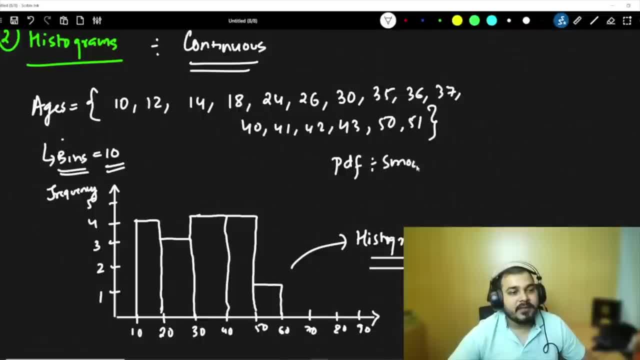 Because people ask about what is PDF. I say that PDF is smoothening of histogram. So I'll just tell you one example. If I smoothen this histogram, my PDF function will look something like this: Now you may be considering: Krish, how is this basically getting created? 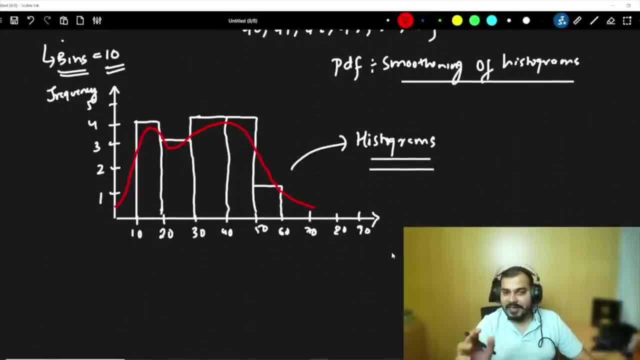 Okay, How is this basically getting created? I'll say that there is something called as Kernel Density Estimator. Now, this Kernel Density Estimator, how it is done, we will try to understand that in the upcoming classes. Probably that is little bit in the advanced side. 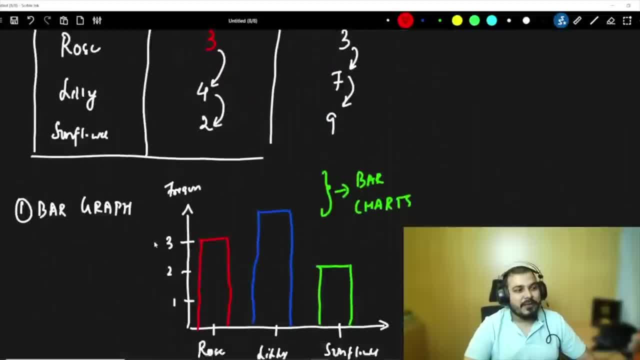 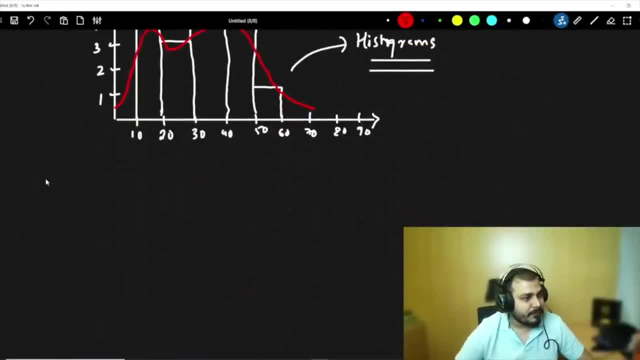 But I hope everybody got an idea about histograms. Everybody got an idea about bar graph. Definitely only for Okay. Tell me, what is the difference between bar versus histogram, Bar versus histogram, Why do we use bar graph and why do we use histogram? 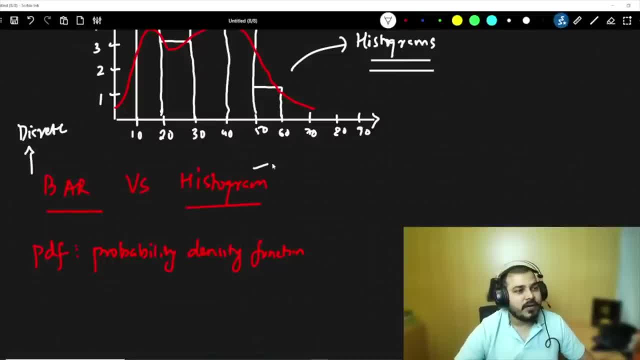 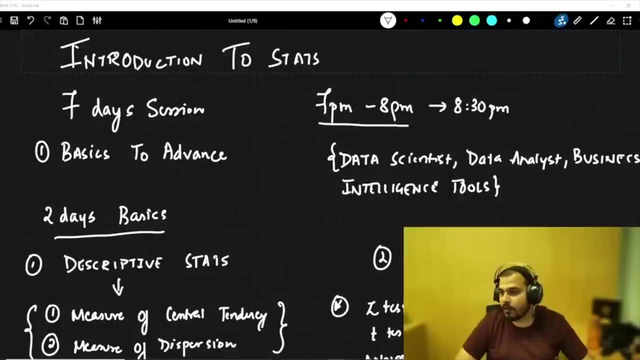 Bar is specifically used for discrete. This is used for continuous. Now, if somebody asks you what exactly is probability density function, you're just smoothening the histograms. Hello guys, So yesterday, if you remember, we have discussed all the basic things. 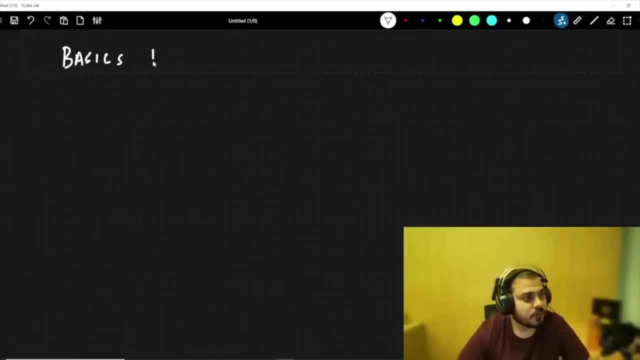 Today we will be moving from basics to intermediate stats, specifically for data science. So this is what we are going to discuss, and there are so many topics that I am probably going to cover Today. we are basically going to cover measure of central tendency. measure of central tendency. 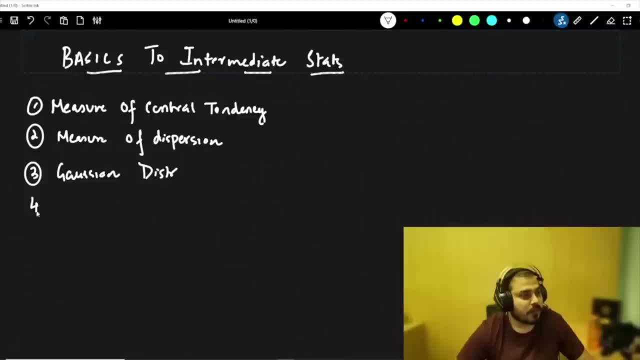 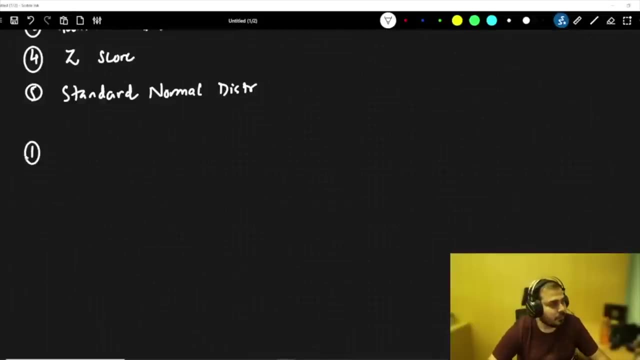 measure of dispersions, Gaussian distribution. Okay, Then fourth, we are going to understand Z-score, Then we are going to understand standard normal distribution, standard normal distribution, and there are some more topics that we really need to cover. So the first topic that probably we are going to discuss is something called as arithmetic. 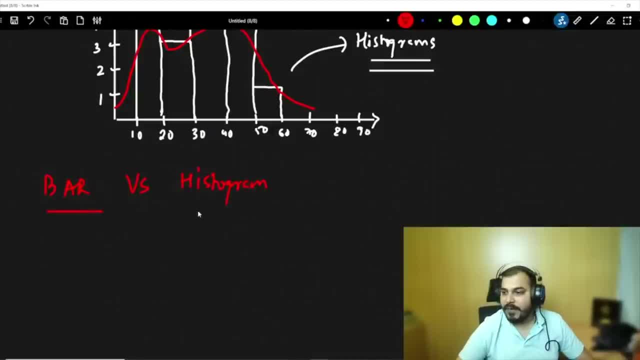 Bar versus histogram. Why do we use bar graph and why do we use histogram? Bar is specifically used for discrete. This is used for continuous. Now, if somebody asks you what exactly is probability density function, you are just smoothening the histograms. 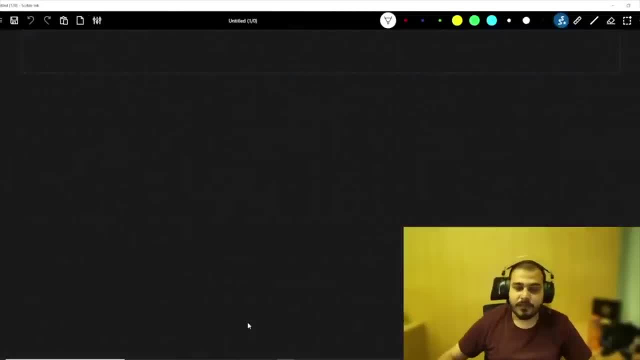 Hello guys. So yesterday, if you remember, we have discussed all the basic things. Today we will be moving from basics to intermediate stats, specifically for data science. So this is what we are going to discuss, and there are so many topics that I am probably going to cover. 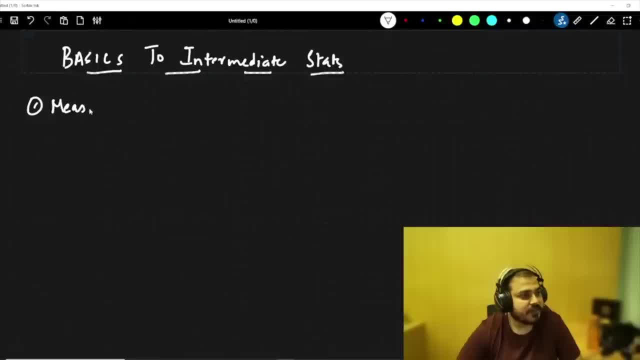 Today we are basically going to cover measure of central tendency. So this is what we are going to discuss, and there are so many topics that I am probably going to cover Measure of central tendency, measure of central tendency, measure of dispersion, Gaussian distribution. then, fourth, we are going to understand Z score, then we are going to understand standard. 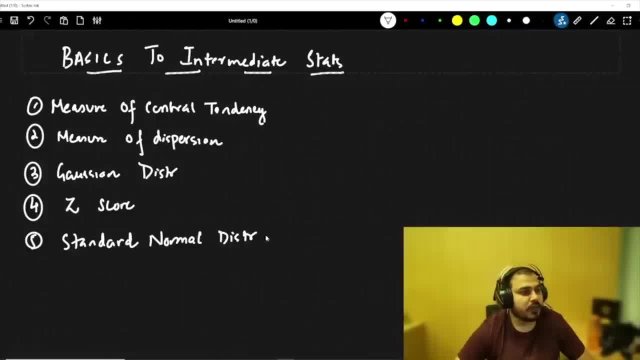 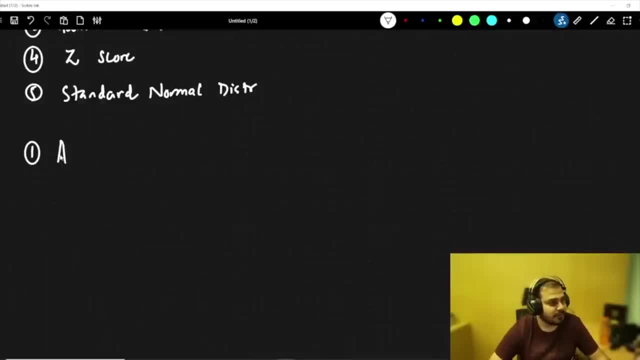 normal distribution, standard normal distribution, and there are some more topics that we really need to cover. So the first topic that probably we are going to discuss is something called as arithmetic mean for population and sample Mean, for population and sample Mean basically means over. here, specifically, we are talking about average. 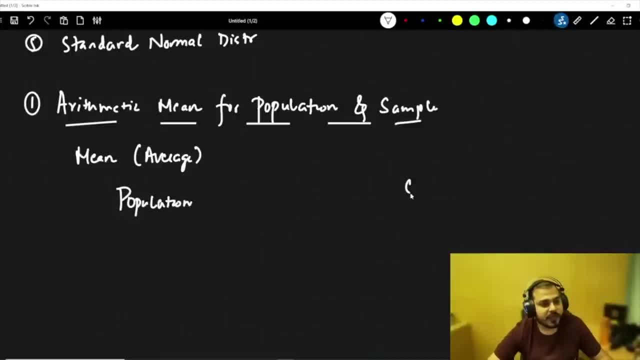 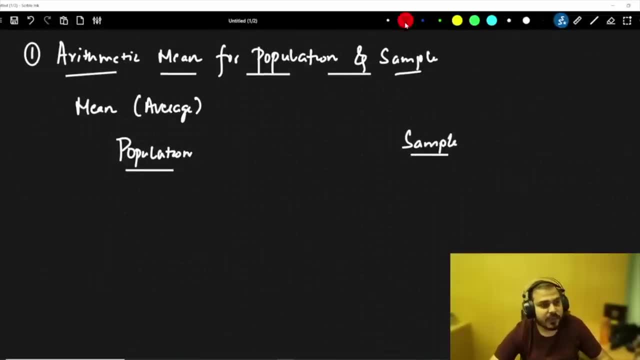 Now, with population and with sample, we really need to understand the formulas of mean, and we will try to understand in this specific way. population is basically given by capital N. sample is given by small n. Now, coming to the first thing, whenever we are probably discussing about mean, you need 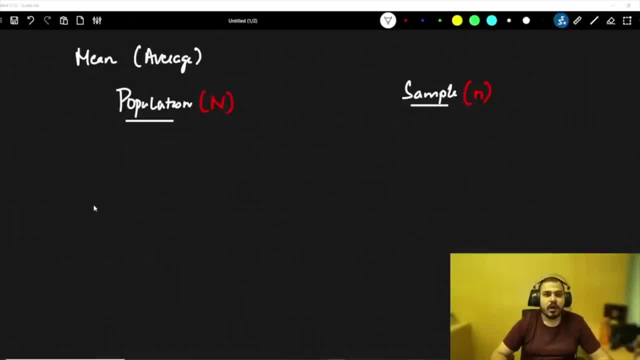 to remember that we are trying to find out the average of a specific distribution. So let's say that my data set looks something like this: 3,3,4,5,5,6. so if I really want to find out the mean of this population, mean of this population, I can basically give by: 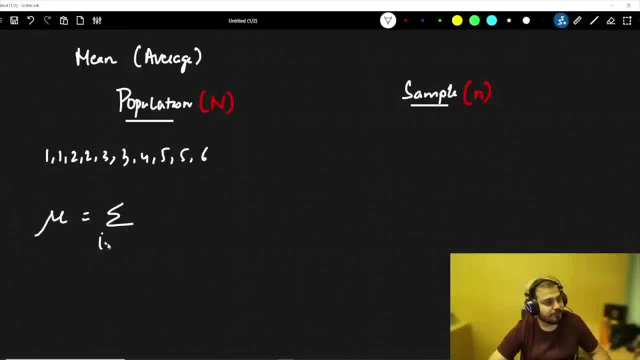 a symbol which is mu, and I will say: summation of i is equal to 1 to capital N, x of i divided by n. Now, what is this x of i? let's consider that this is my random variable x, and probably I have so many different values inside my data set: 1,1,2,2,3,3,4,5,5,6. so if I really 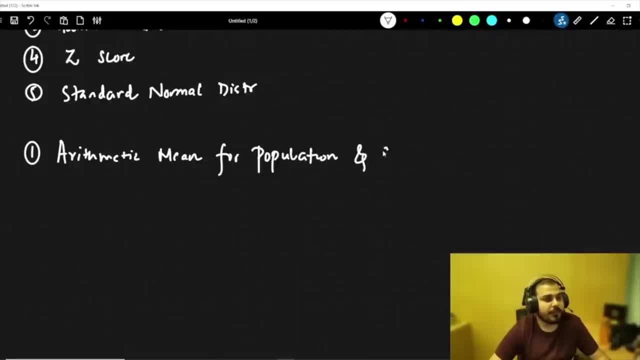 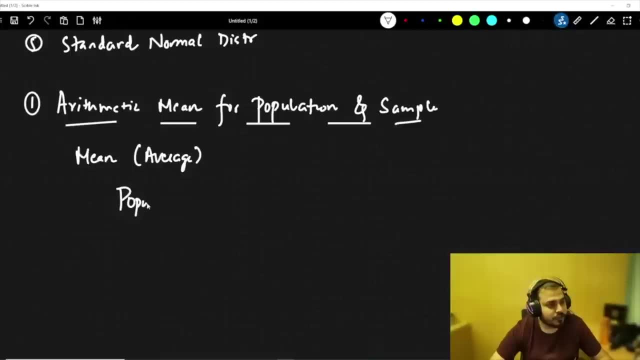 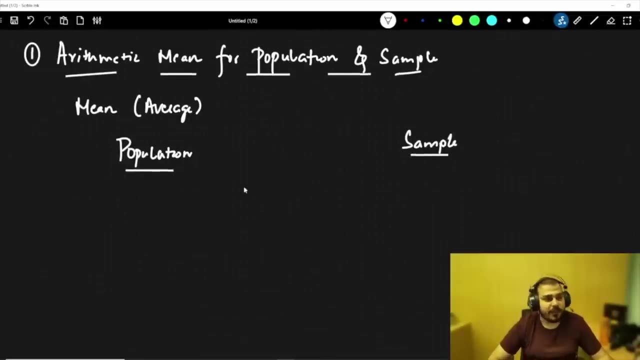 mean for population and sample. Mean basically means over here specifically, we are talking about average. Now, with population And with sample, we really need to understand the formulas of mean and we will try to understand in this specific way. Population is basically given by capital N. Sample is given by small n. 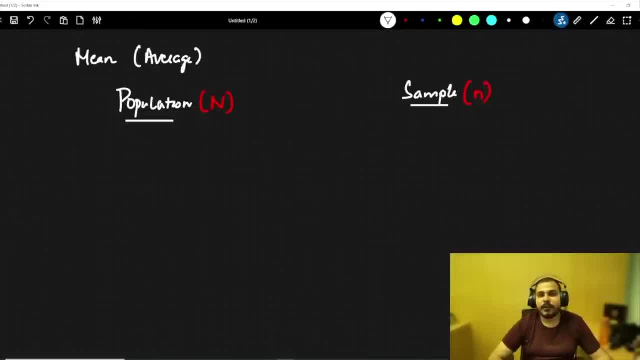 Now, coming to the first thing. whenever we are probably discussing about mean, you need to remember that we are trying to find out the average of a specific distribution. So let's say that my data set looks something like this: 3, 3,, 4,, 5,, 7,, 8,, 9,, 10,, 11,, 12,, 13,, 14,, 15,, 16,, 17,, 18,, 19,, 20,, 21,, 22,, 23,, 24,, 25,, 26,, 27,. 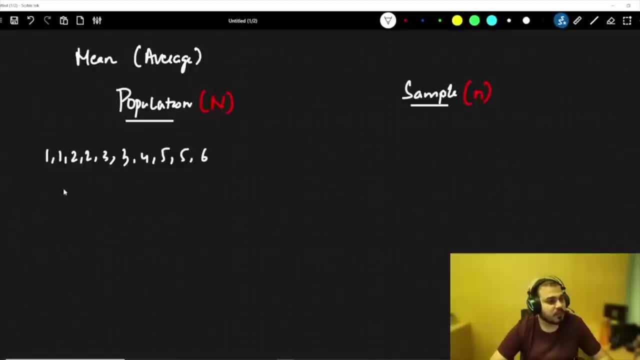 28,, 28,, 29,, 30,, 31,, 32,, 33,, 34,, 35,, 35,, 36.. So if I really want to find out the mean of this population, mean of this population, 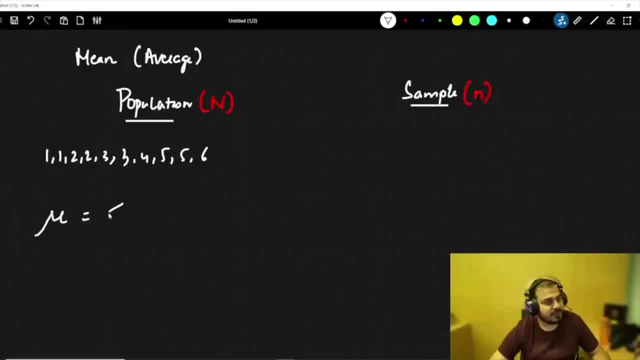 I can basically give by a symbol, which is mu, and I'll say: summation of i is equal to 1 to capital N, x of i divided by n. Now, what is this x of i? Let's consider that this is my random variable x, and probably I have so many different values. 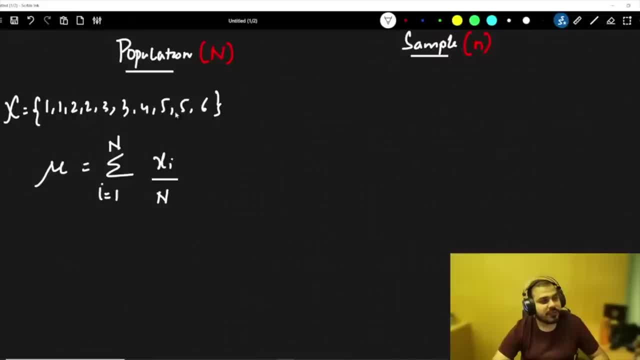 inside my data set: 1, 1,, 2,, 2,, 3,, 4,, 5, 6.. So if I really want to expand this thing x of i, basically we are going to iterate through all these n elements. 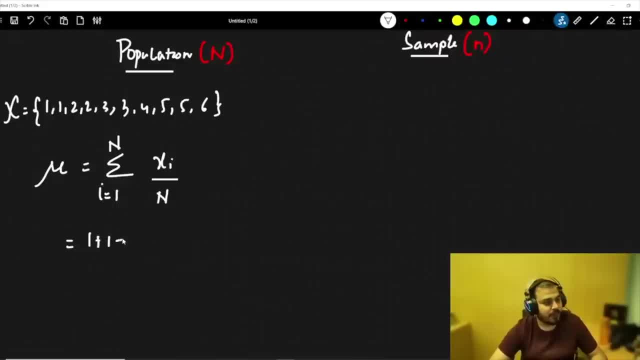 So I may write: 1 plus 1 plus 1 plus 2 plus 2 plus 3 plus 3 plus 4 plus 5 plus 5 plus 6 divided by capital N Over here. capital N is what? 1, 2, 3, 4,, 5, 6, 7,, 8, 9, 10,, so 10 elements. 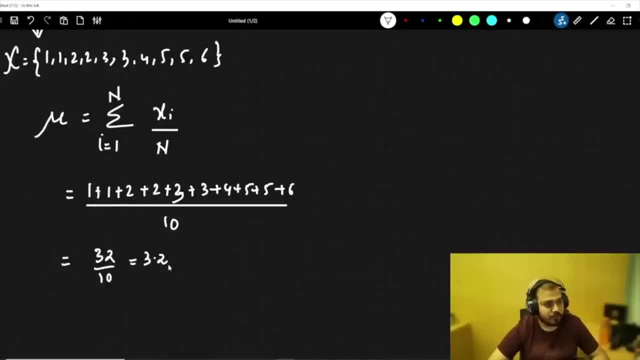 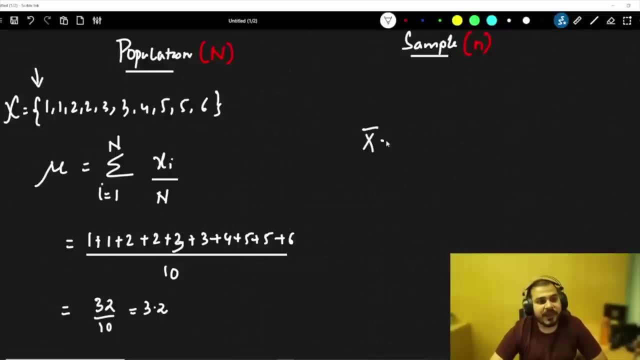 So it is 32 by 10, which is nothing but 3.2.. So 3.2 is basically my average. Now, with respect to population, always remember how the symbol is basically given. We can write x bar, which is specified by sample mean. 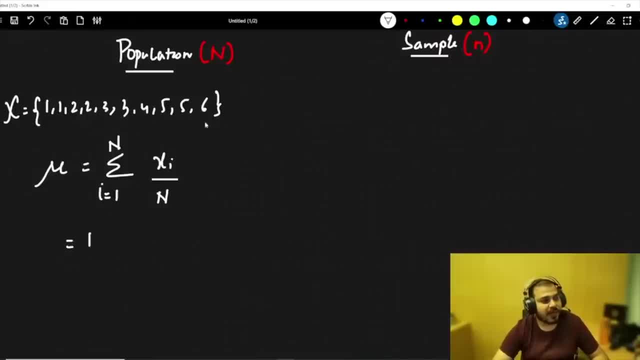 want to expand this thing x of i. basically, we are going to iterate through all these n elements, so I may write 1 plus 1 plus 1 plus 2 plus 2 plus 3 plus 3 plus 4 plus 5 plus 5 plus 6 divided by capital N. 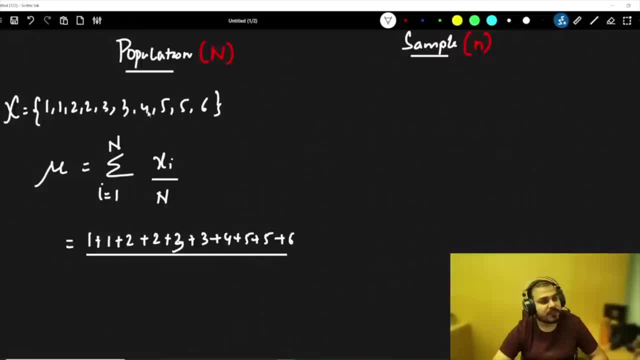 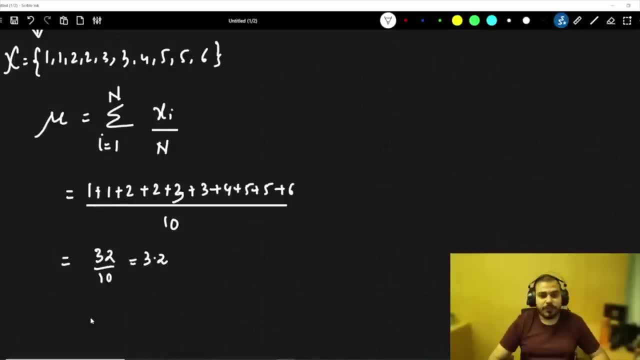 Over here. capital N is what? 1,2,3,4,5,6,7,8,9,10, so 10 elements. so it is 32 by 10, which is nothing but 3.2, so 3.2. 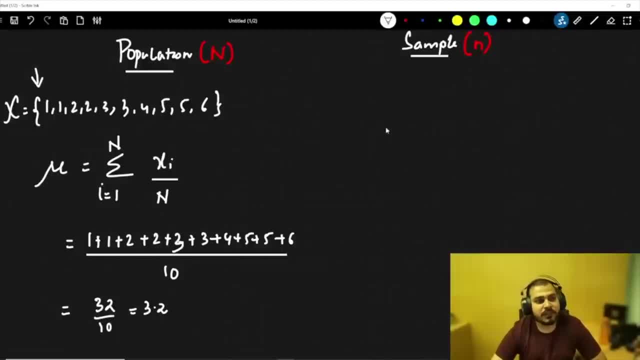 is basically my average now with respect to population. always remember how the symbol is basically given. we can write x bar, which is specified by sample mean. here I am going to write: summation of i is equal to 1 to small n. and here I can basically write x of i divided. 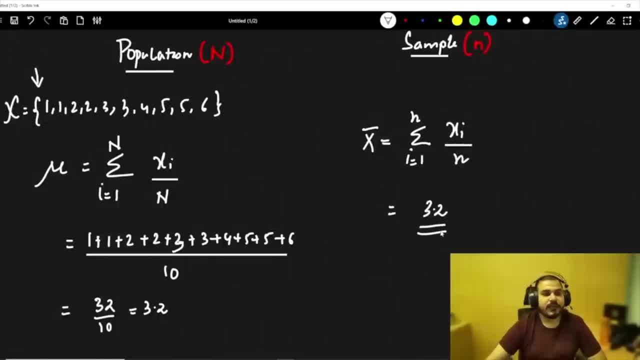 by n, obviously we will get the same answer because we are going to take the same data set. So this was the example with respect to arithmetic. mean always understand that notation. the notation is quite important over here, the reason why I am saying your notations over here in this. 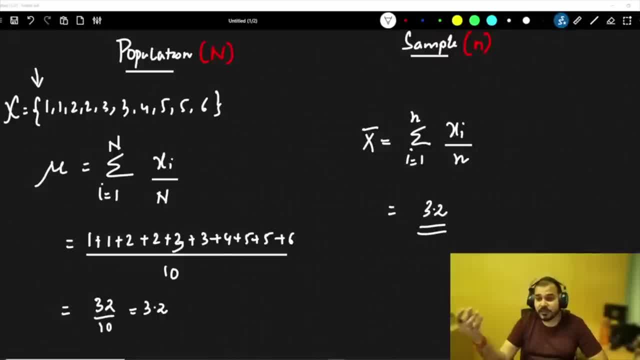 way. because I want? because in the real world industry, when you are working, when you explaining someone as a data scientist, you really need to use this well-known notation. you can use your own notation whatever you like, but think of a larger point of view here. you really 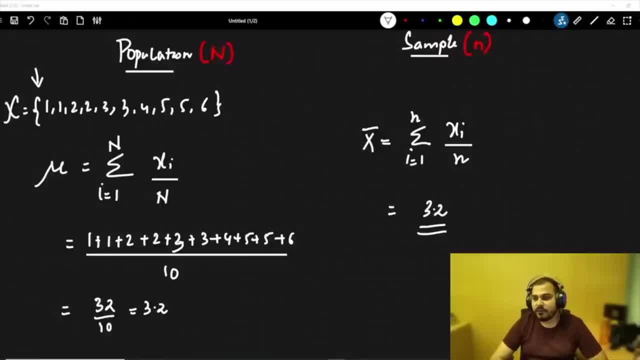 need to make sure that whatever standards is being followed, we need to try to follow in that specific way. So this was the basic things. with respect to mean, mean is the part of central measure of tendency. apart from mean, there are two more things, so let me just define what is. 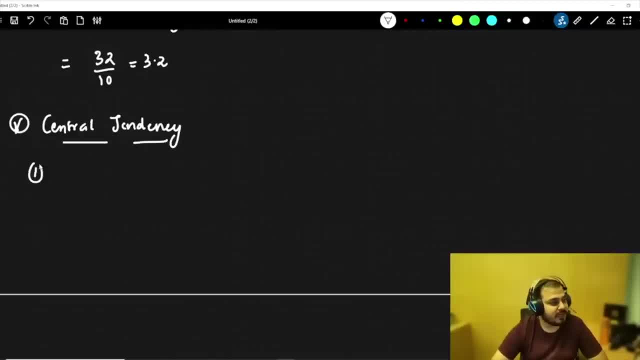 central tendency, which we basically say central measure of tendency, there are three main things: one is mean, second one is median and third one is mode. now, if I really want to make you understand, because it is a very important interview question, if someone says you that, what is? 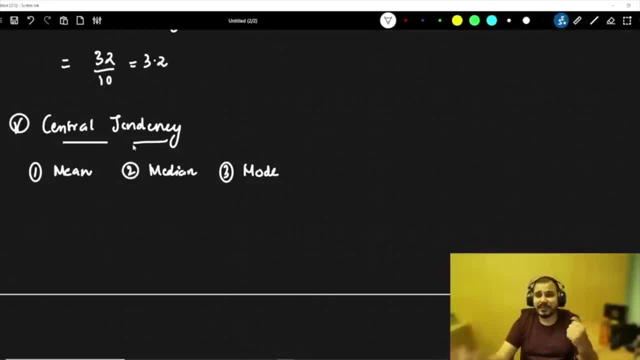 Central tendency, or so what is measure of central tendency? you can just say that it refers to the measure of measure used to determine the center of the distribution of the data. so that basically means whenever I have a data, if I really want to find out the center. 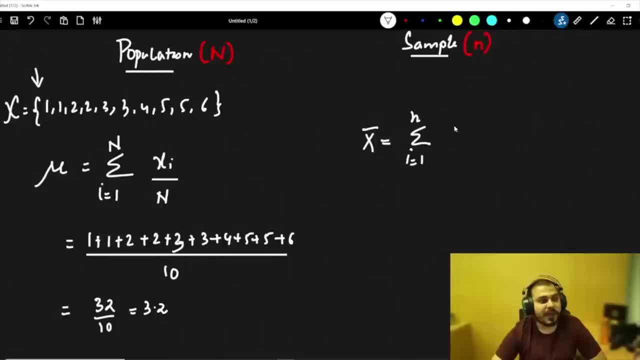 Here I'm going to write: summation of i is equal to 1 to small n. and here I can basically write: x of i divided by n. Obviously, we'll get the same answer because we are going to take the same data set. So this was the example with respect to arithmetic mean. 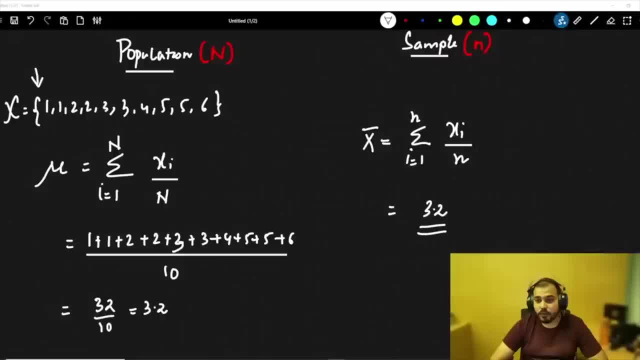 Always understand that notation. The notation is quite important over here. The reason why I'm saying your notations over here in this way: because I want, because in the real world, industry, when you are working, when you're explaining someone as a data scientist. 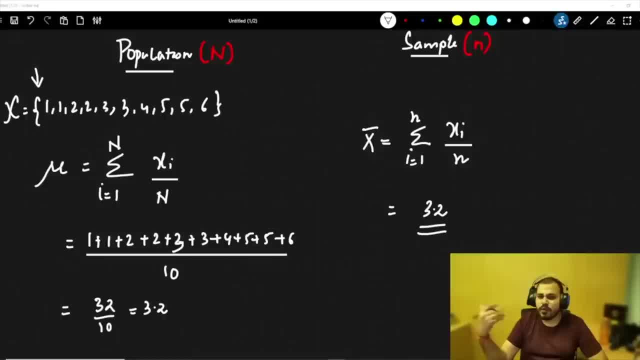 you really need to use this well-known notation. You can use your own notation whatever you like, but think of a larger point of view Here. you really need to make sure that whatever standards is being followed, we need to try to follow in that specific way. 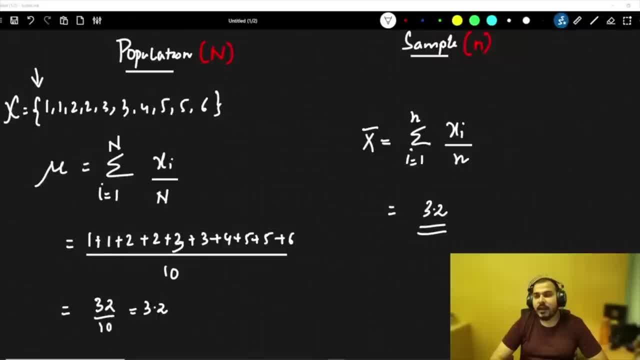 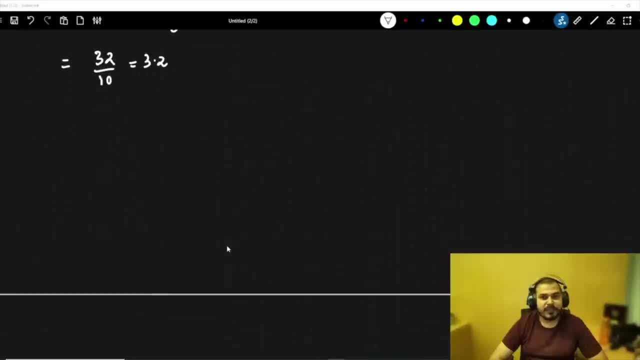 So this was the basic things with respect to mean. Now, mean is the part of central measure of tendency. Apart from mean, there are two more things, So let me just define what is central tendency, which we basically say central measure of tendency. 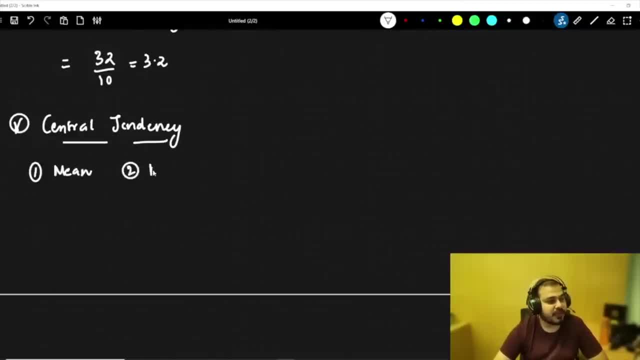 There are three main things: One is mean, second one is median and third one is mode. Now, if I really want to make you understand, because it is a very important interview question, If someone says to you that what is central tendency or what is measure of central tendency, 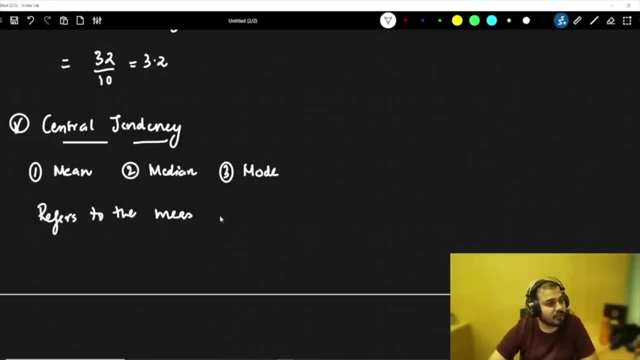 you can just say that. The point is this means that it refers to the measure used to determine the centre of the distribution of the data. So that basically means whenever I have the data, if I really want to find out the centre part of that particular distribution, I can use mean median mode. 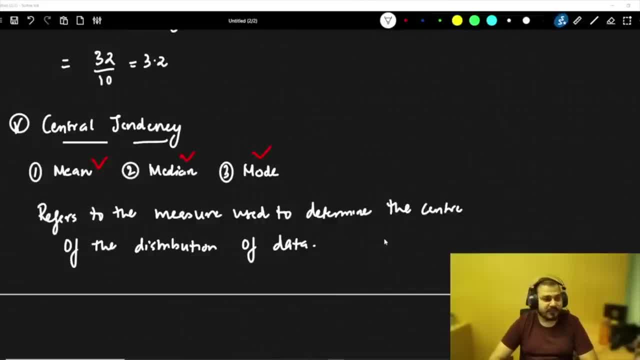 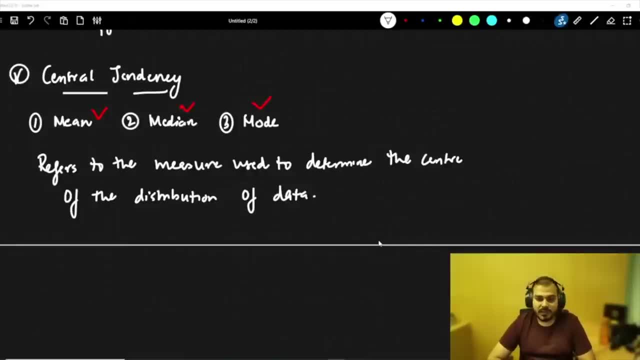 Why specifically will be using it. that is all I will be talking about, But I hope everybody got the definition till here. Everybody clear with this definition. It referring to the measure used to determine the center of the distribution of data. determine the center of the distribution of the data. so average and mean are one in the same guys. 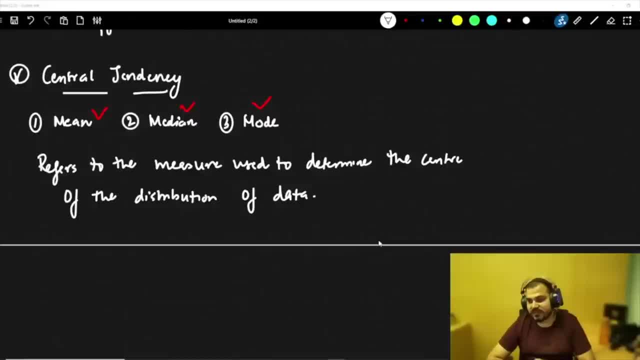 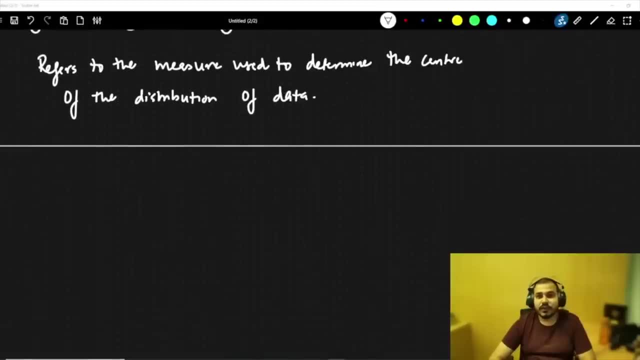 understand average mean. okay, we use the same formula that is basically used. okay, so this was the part with respect to central tendency. now let's go ahead and let's try to solve some problems, right? obviously, i have given you a lot of examples with respect to mean, but now let's go ahead and 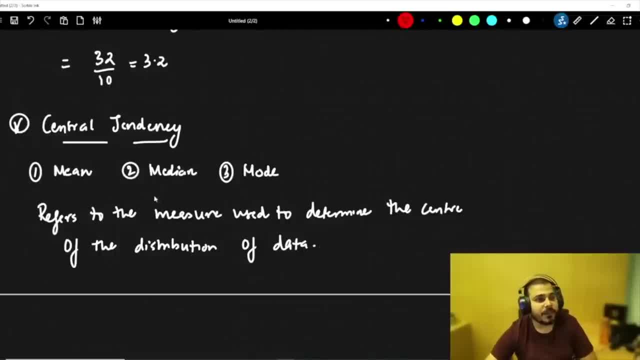 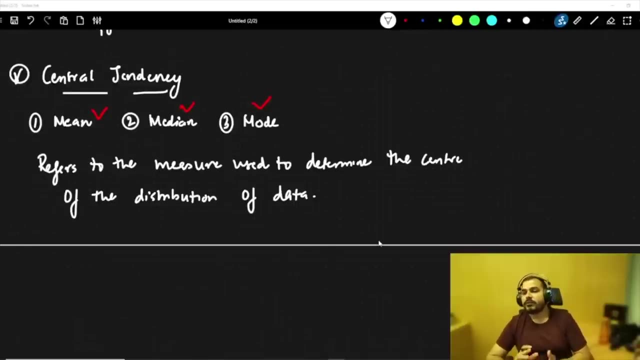 part of that particular distribution. I can use mean median mode. why specifically we will be using it. that all I will be talking about. but I hope everybody got the definition Till here. everybody clear. with this definition it refers to the measure used to determine the center of the distribution of the data. so average and mean are one in the same guys. 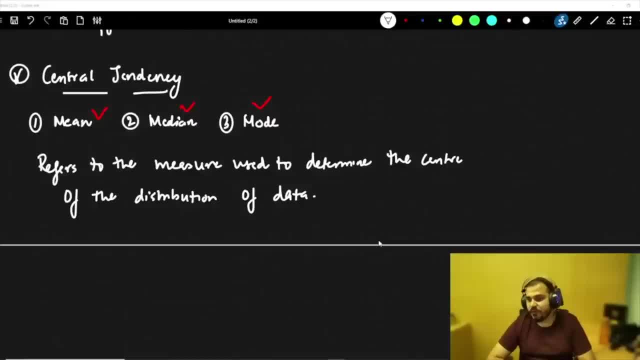 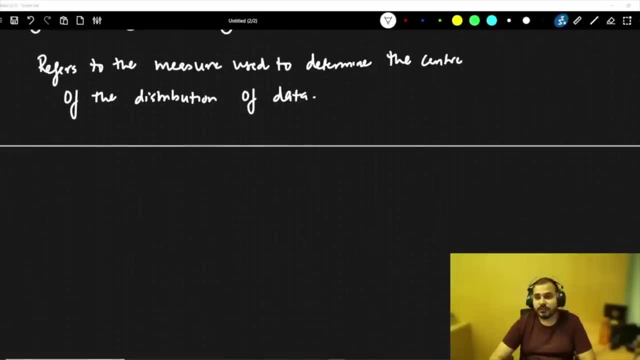 understand average mean. okay, we use the same formula that is basically used, okay, so this was the part with respect to central tendency. now let's go ahead and let's try to solve some problems, right? obviously, I have given you lot of examples with respect to mean, but 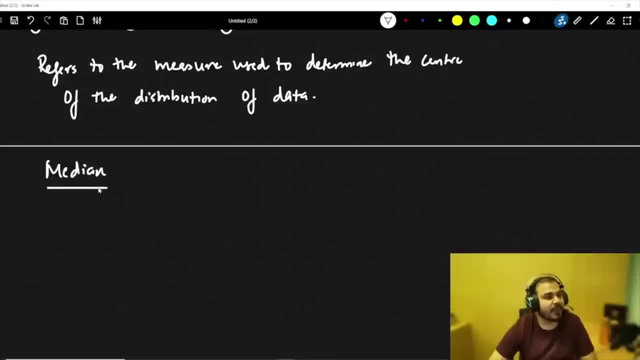 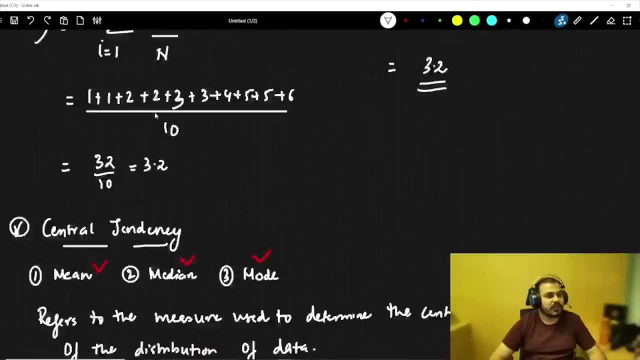 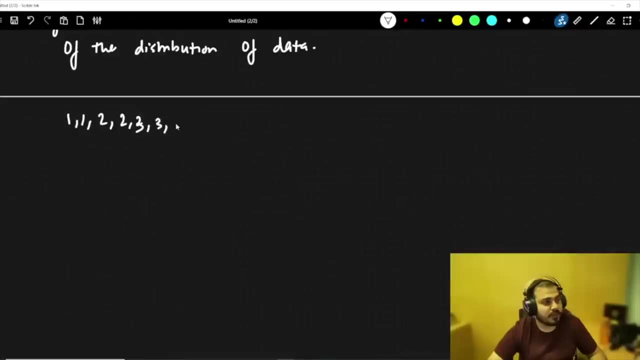 now let's go ahead and try to understand median. And why do we specifically use median? so I am going to take the same data set, whatever data set I have used over here, that is, one, one, two, two, three, three, four, five, five, six. okay, so one comma one comma two comma two, comma three comma three, comma four. and what? 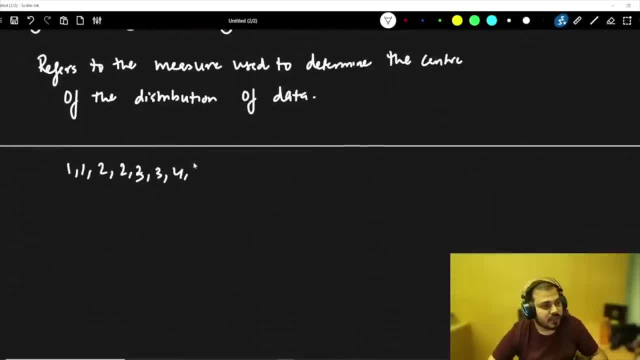 was the data. then you had five, five, six, right? so here I am basically going to take five, five, six. so suppose, if this is my data, obviously the mean we found out was nothing but three, two. now what if I tell you that in this distribution you add one more element like hundred? so when 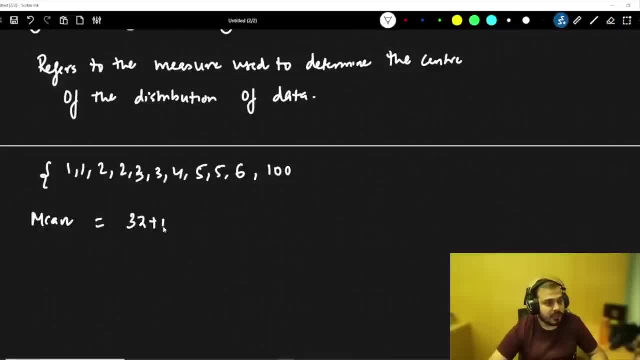 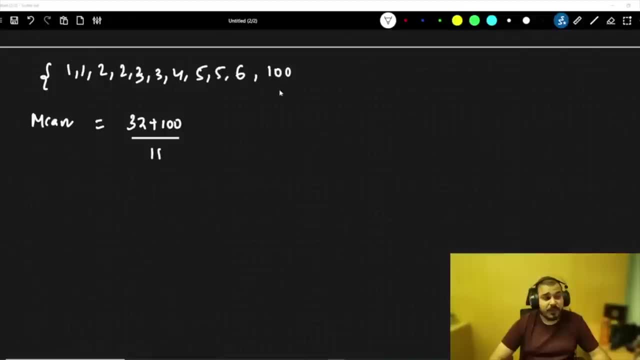 you add hundred, then it will become thirty two plus hundred, divided by eleven. thirty two is basically from the sum of all the numbers that we have done or taken previously, plus hundred, which is a new element that is basically added and we are just going to divide by eleven. 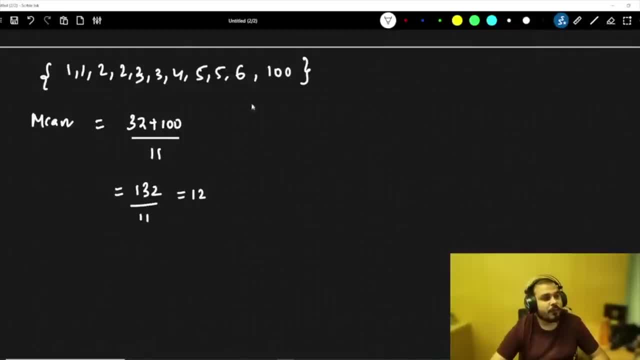 so once I do one thirty two by eleven, we are getting twelve. before when hundred was not added. So if one element was not added at that time, my mean was three point two. but after adding hundred in that specific distribution my mean became twelve. now here you can see that there. 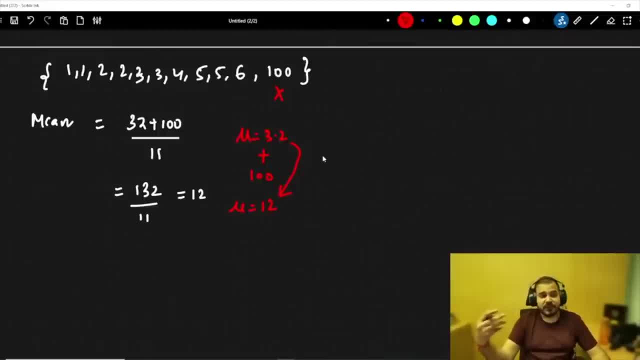 is a huge movement of mean. there is a huge difference with respect to this mean and why it is basically added because of this number. we consider this number as outliers. outliers really have a adverse impact on the entire distribution, so that is the reason why we should be very much careful about this. 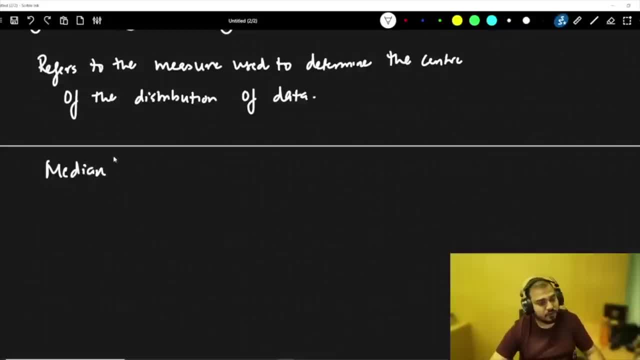 try to understand median and why do we specifically use median? so i'm going to take the same data set. whatever data set i have used over here, that is one, one, two, two, three, three, four, five, five, six. okay, so one comma, one comma, two comma, two comma, three comma, three comma, four. and what was the data? 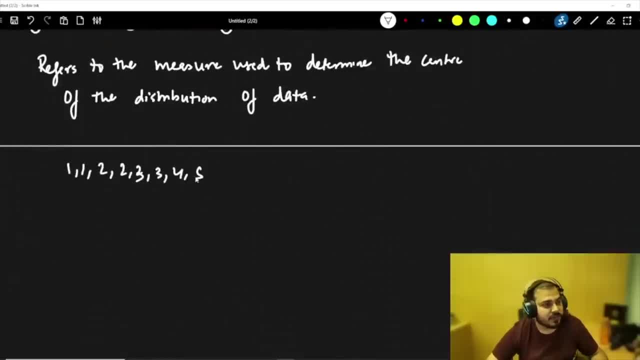 then you had five, five, six, right? so here i'm basically going to take five, five, six. so suppose, if this is my data, obviously the mean we found out was nothing but 3.2. now what if i tell you that in this distribution you add one more element? 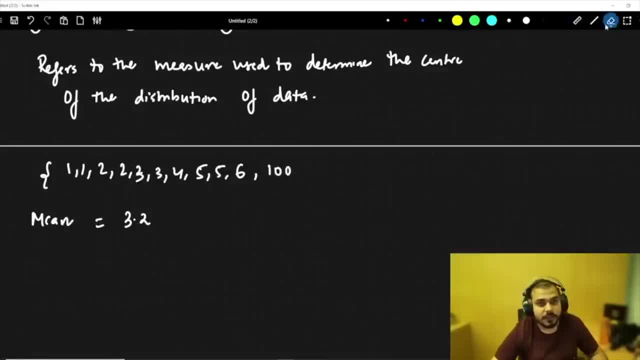 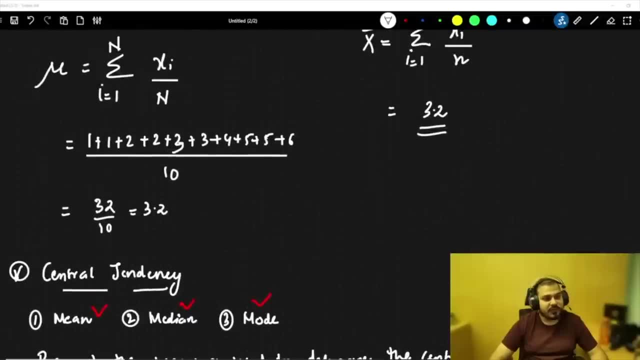 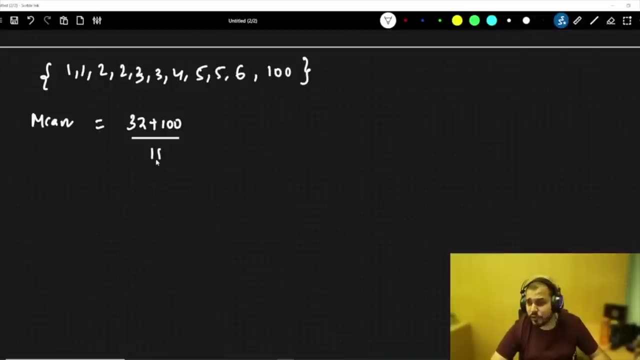 like 100. so when you add 100 then it will become 32 plus 100. divided by 11, 32 is basically from the sum of all the numbers that we have done or taken previously, plus 100, which is a new element that is basically added and we are just going to divide by 11. so once i do 132 by 11, we are getting 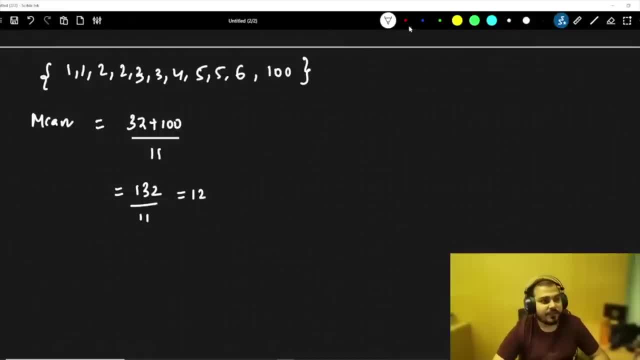 12 before when 100 was not added. when this element was not added, at that time my mean was 3.2, but after adding 100 in that specific distribution, my mean became 12.. now here you can see that there is a huge movement of mean. there is a huge difference with respect to this mean, and why. 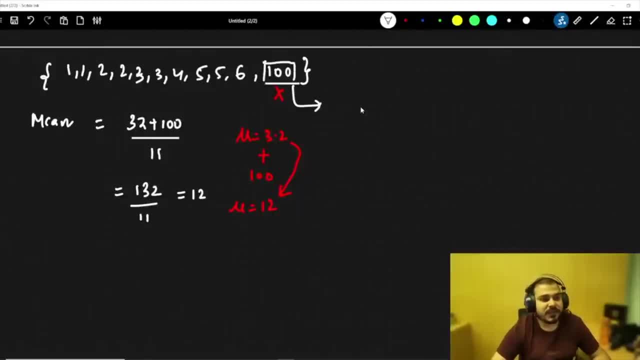 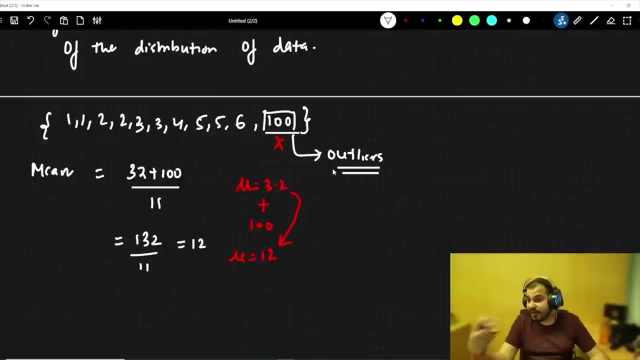 it is basically added because of this number. we consider this number as outliers. outliers really have a adverse impact on the entire distribution, so that is the reason why we should be very much careful with outliers. in data science also, in statistics also, we use different techniques to remove the outliers, which also i'll be discussing today when we are going to discuss about. 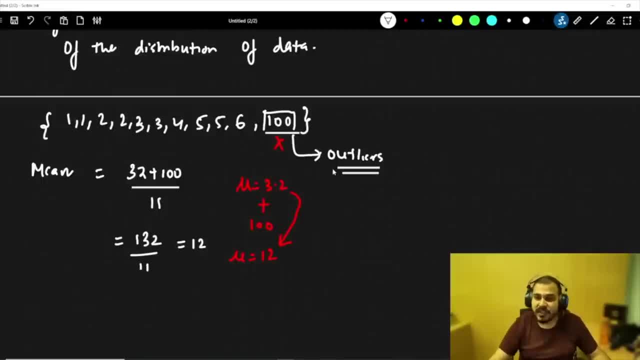 percentiles and all so remember outliers- has a major impact because here you can see that the entire distribution of the central data is basically moving and the difference is quite huge for this particular case, what we do, we can definitely use median now in median, if i take 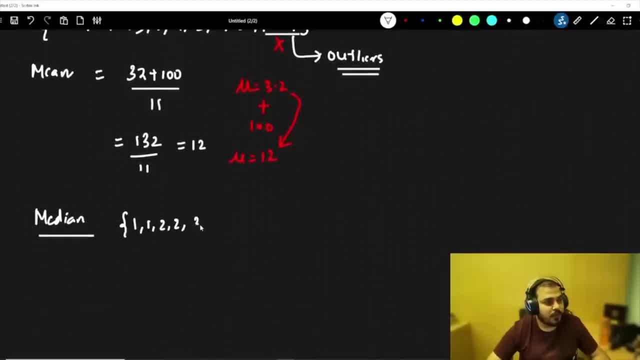 the same number, like one, one, two, two or three, three, four, five, five, six, and then probably i have 100. always understand in median. the first thing that you really need to do is sort the numbers. so first step is sort the numbers. so over here you can see that the numbers are already sorted. if your numbers 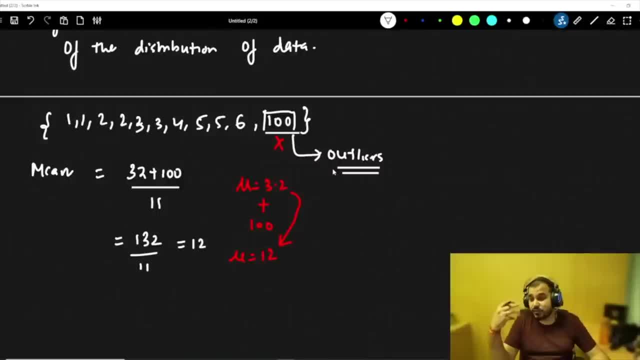 In data science also, in statistics also, we use different techniques to remove the outliers, which also I will be discussing today, when we are going to discuss about percentiles and all. So remember, outliers have a major impact because here you can see that the entire distribution of the central data is basically moving and the difference is quite huge for this particular 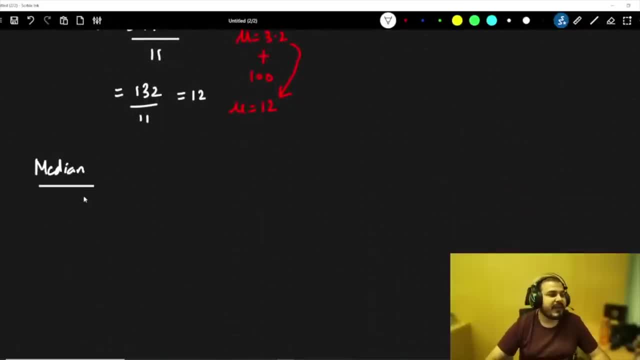 case what we do. we can definitely use median. now, in median, if I take the same number like one, one, two, two or three, Three, three, four, five, five, six, and then probably I have hundred, always understand in median. the first thing that you really need to do is sort the numbers. the first step is sort 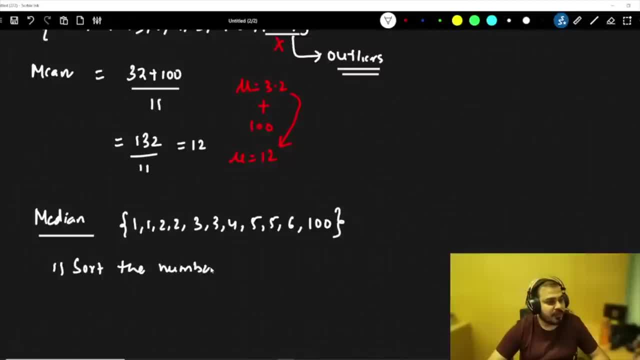 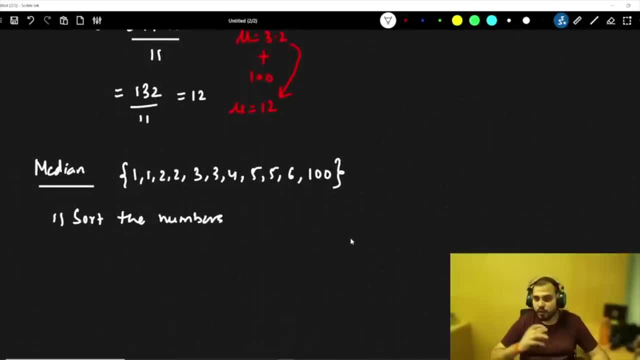 the numbers. so over here you can see that the numbers are already sorted. if your numbers is not sorted at that point of time, you will be able to see that. you know you probably have to sort it right now by default. I have made sure that the number is already sorted. 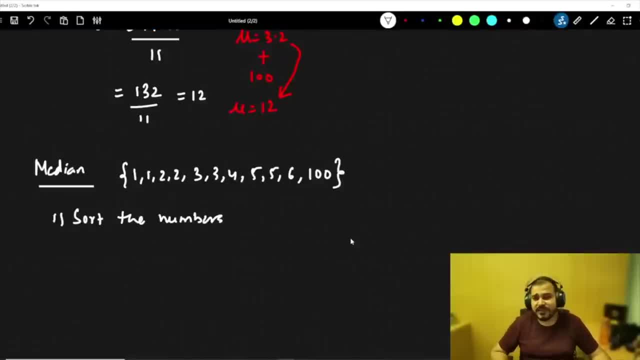 so do you define distribution in statistics? The statistical term distribution basically means that how your data looks. see what is distribution. okay, how do you see how your data is basically distributed? there are various ways. we use PDF, we use histograms, we use different, different techniques. so I will be coming in. 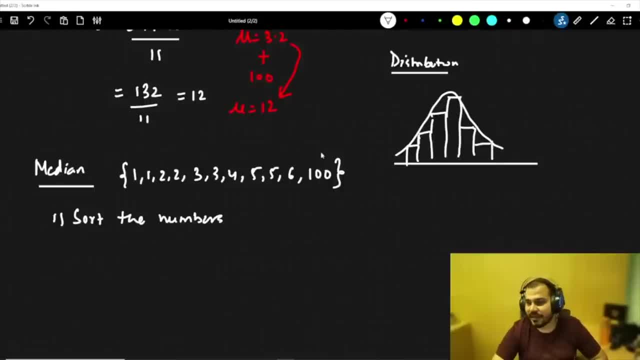 making you understand about different distributions. still, I have not started that now. first step is always sorting the numbers. I have sorted the numbers. after sorting the numbers, what I am actually going to do is that I am basically going to take the central element. a central element means which one? 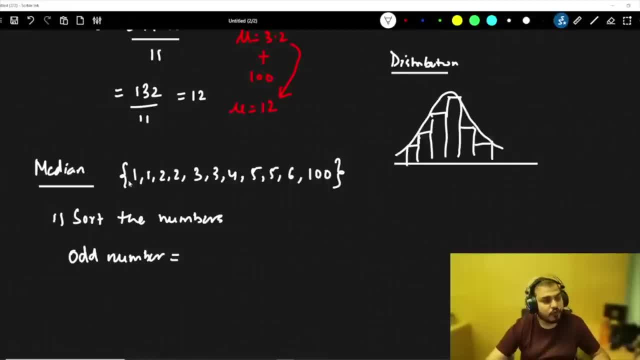 Suppose if I have odd number of elements. so over here, what is the count? one, two, three, four, five, six, seven, eight, nine, ten, eleven. so eleven is the count. in order to find out the central element. okay, we will probably find out the center: one. so one, two, three, four. 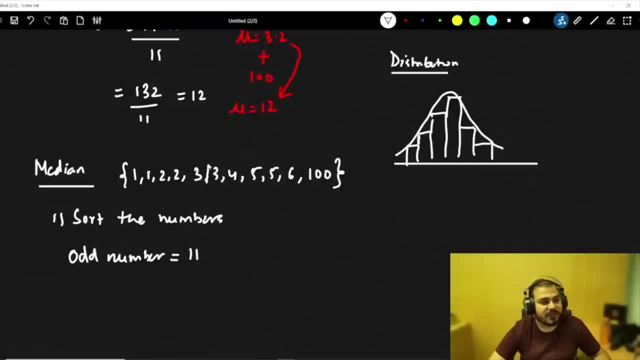 five: one, two, three, four, five. so this will basically be my central element. this will be my central element because it is the middle element. now, in this particular case, I can definitely say that my mode is nothing but three. Now understand, even though the outlier is added. see outlier basically means what outlier? 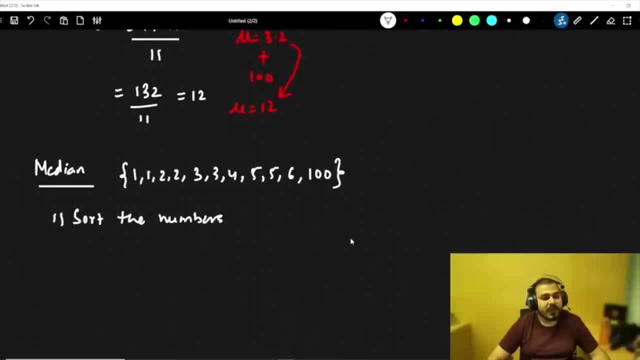 is not sorted, at that point of time you will be able to see that. uh, you know you probably have to sort it right now by default. i have made sure that the number is already sorted. so do you define distribution in statistical term? distribution basically means that how your data looks, see. 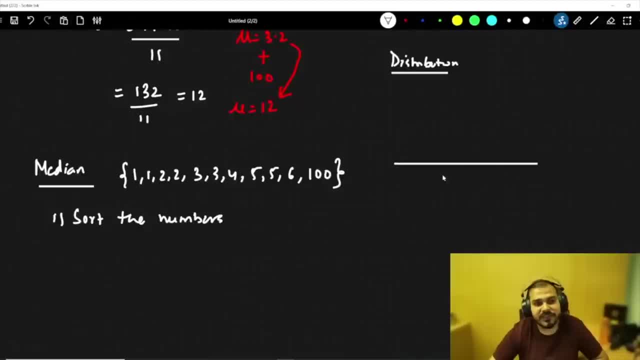 what is distribution? okay, how do you see how your data is basically distributed? there are various ways. we use pdf, we use histograms, we use different, different techniques. so i will be coming in making you understand about different distributions. still, i have not started now. first step is always sorting the numbers. i have sorted the numbers. after sorting the numbers, what i am? 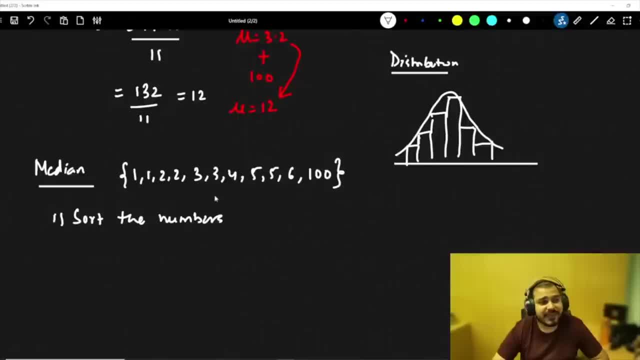 actually going to do is that i am basically going to take the central element. a central element means which one suppose, if i have odd number of elements, so over here, what is the count? one, two, three, four, five, six, seven, eight, nine, ten, eleven, so eleven is the count. in order to find out, 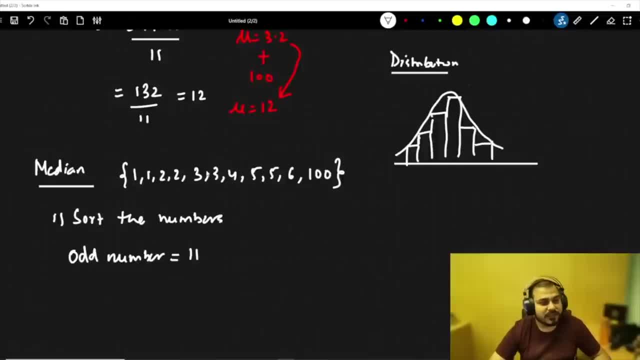 the central element. okay, we will probably find out the center one. so one, two, three, four five. one, two, three, four five. so this will basically be my central element. this will be my central element because it is the middle element. now, in this particular case, i can definitely say that my 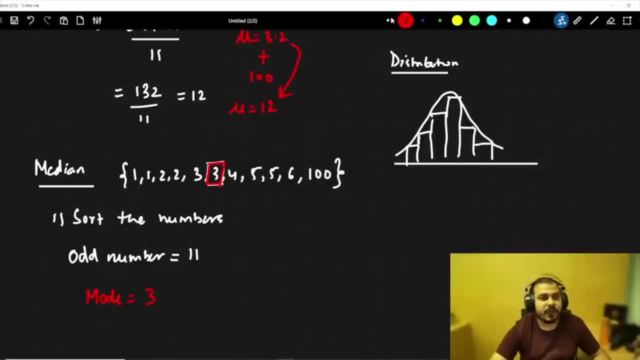 mode is nothing but three. now understand, even though the outlier is added, see outlier. basically, what outlier is a number which is completely different from the entire distribution over here you can see that 100 is a completely different from the entire distribution. now, what if? now your question may rise that okay, krish. what if i have one more number like this? let's say that i have. 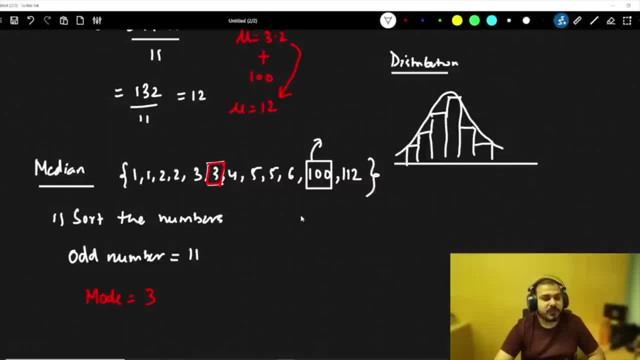 one more number: 112.. now, in this particular case, you told to pick up the central element now in this case, which will be my central element now in this case, my total number of elements are 12.. so, in order to find out the central element, 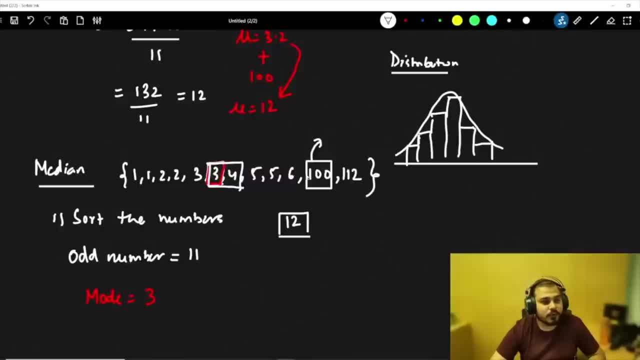 what i will do. i will take up the middle two elements: one, two, three, four, five. one, two, three, four, five. so the middle elements is basically present over here. now, here i will take this middle element, which is my three and four, and i will do the average of them. so three plus four divided by 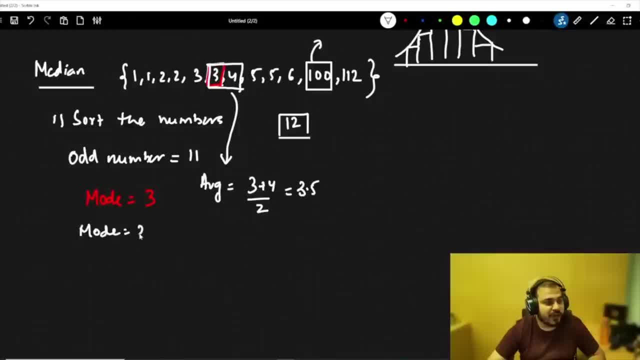 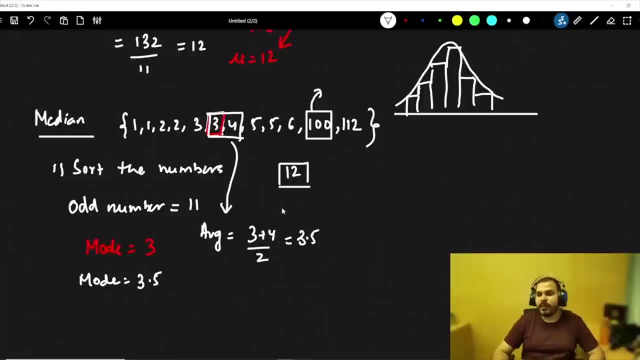 two. so in this particular case i can say that my mode is 3.5, even though i had two different outliers. but yes, if i keep on increasing the number of outlines, then the distribution will become normal. now understand one thing: why mode acts differently from the average of the outliers. 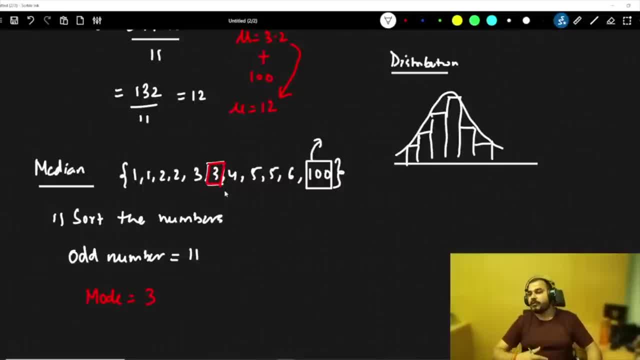 is a number which is completely different from the entire distribution over here. you can see that hundred is a completely different from the entire distribution. now, what if? now your question may rise- that okay, Krish. what if I have one more number like this? let's say that I have one more number, hundred and twelve. now, in this particular case, you told 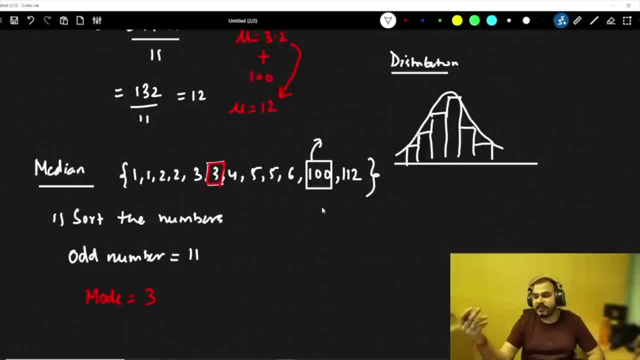 to pick up the central element Now in this case, which will be my central element Now in this case. my total number of elements are twelve. so, in order to find out the central element, what I will do? I will take up the middle two elements: one, two, three, four, five. 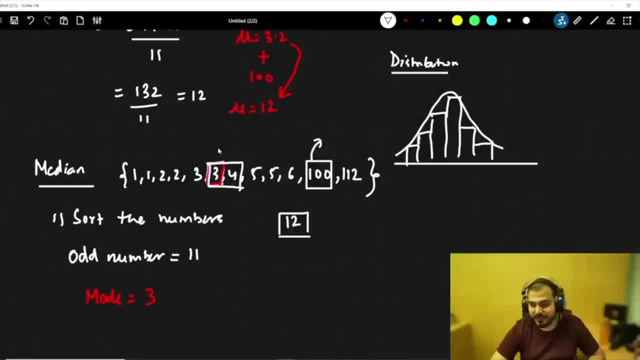 one, two, three, four, five. so the middle elements is basically present over here. Now, here I will take this middle element, which is my three and four, and I will do the average of them, so three plus four divided by two. so in this particular case I can say that 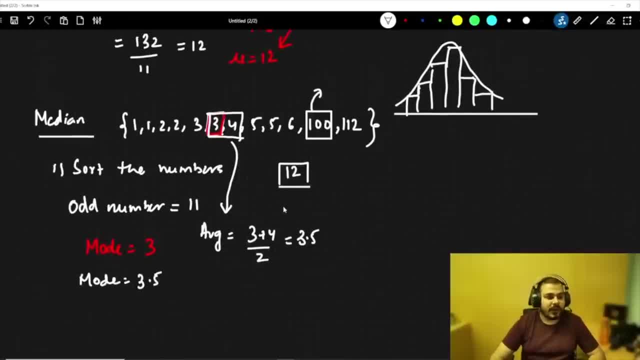 my mode is three point five, even though I had two different outliers. but yes, if I keep on increasing, If I increase the number of outliers, then the distribution will become normal. now understand one thing why mode actually works in a better way before: because of this outlier, my mean. 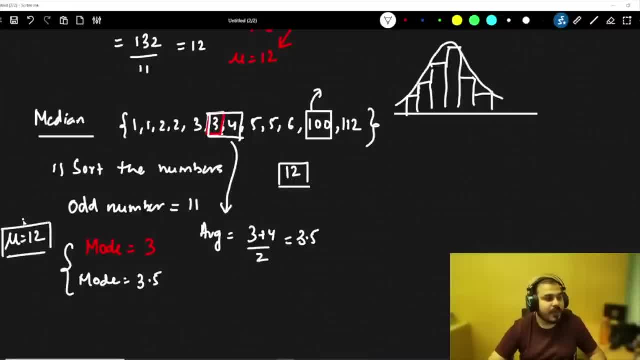 was twelve, even though, after adding the outlier, my mean was twelve. but now here you can see that, even though I added two outliers, my mode, which is again a measure of central tendency, okay, which is again a measure of central tendency, there is highly any difference, a very less. 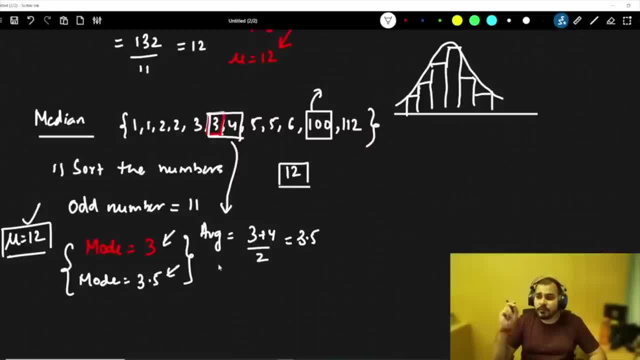 difference. So that is the reason why we use Median. did I say mode? oh sorry, sorry, it is median. I by mistake I wrote mode. it should not be okay median, okay, So median. I hope everybody understood what exactly is median. we basically take the central. 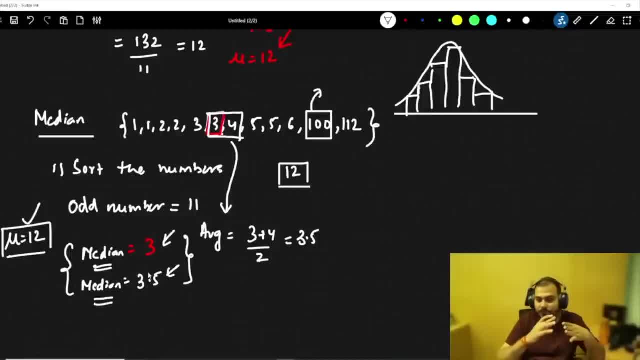 elements. if the number of elements is even, then we probably take the central two elements. we try to find out the average and we try to calculate it. But understand one thing over here: what is the main purpose? initially, when we did not add outlier, Then we try to calculate the mean. at that time I got three. point two, when I try to calculate, 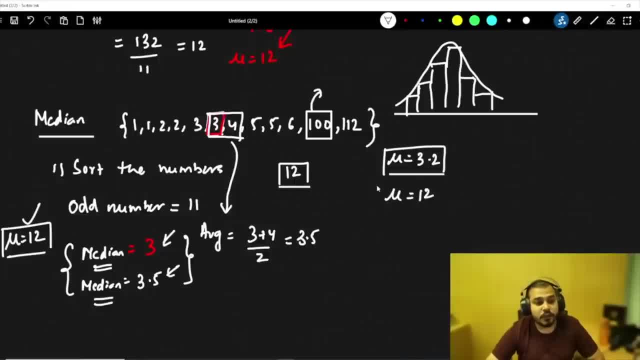 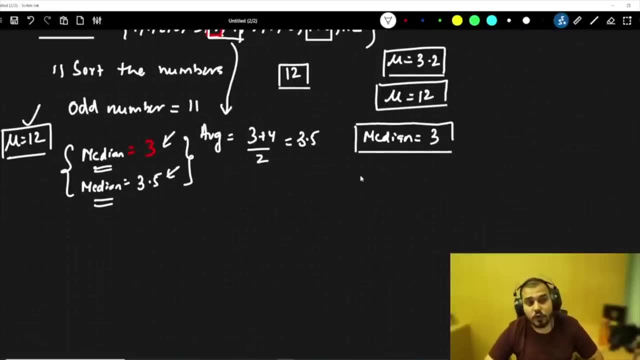 by adding an outlier. my median was twelve. sorry, my mean was twelve. when I try to do this with respect to median, even though I had outlier added the outlier, it came as three and finally, you will be able to see that when I probably used two outliers and then probably 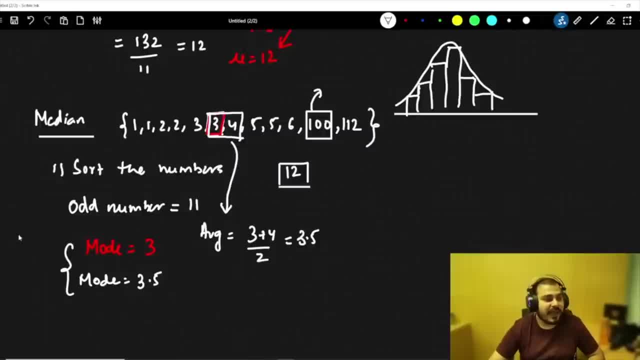 actually works in a better way. before, because of this outlier, my mean was 12, even though, after adding the outlier, my mean was 12.. but now, here you can see that, even though i added two outliers, my mode, which is again a measure of central tendency, okay, which is again a measure of. 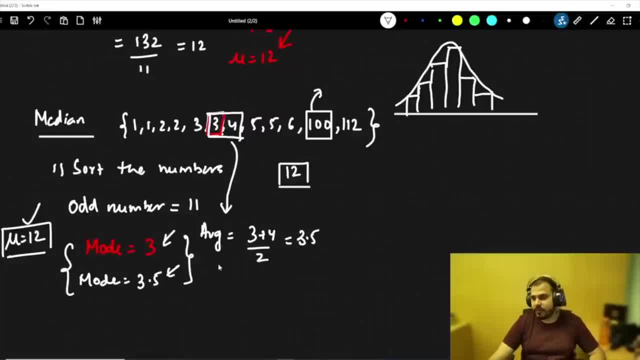 central tendency. there is highly any difference, a very less difference. so that is the reason why we use median. did i say mode? oh sorry, sorry, it is median. i mistake, i wrote mode. it should not be okay median, okay, so median. i hope everybody understood what exactly is median. we basically take the central elements. if the number of elements is even, then 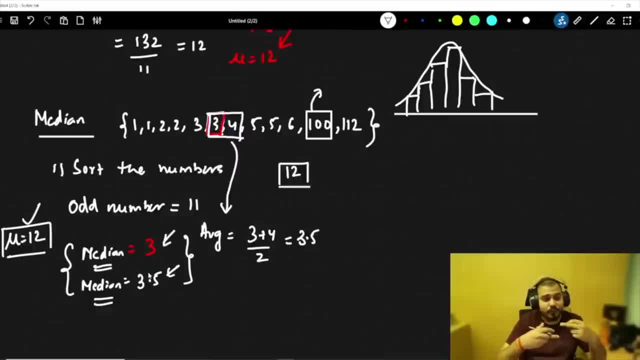 we probably take the central two elements. we try to find out the average and we try to calculate it. but understand one thing over here: what is the main purpose? initially, when we did not add outlier and we tried to calculate the mean, at that time i got 3.2. when i tried to calculate by 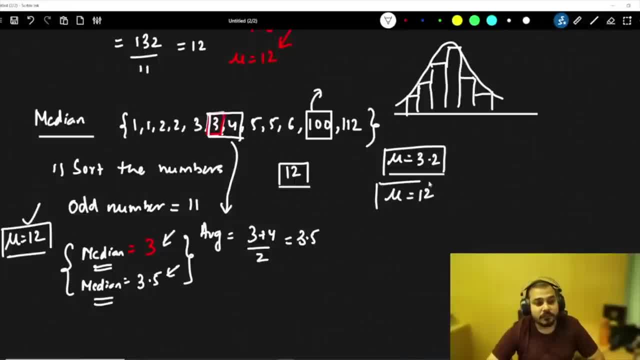 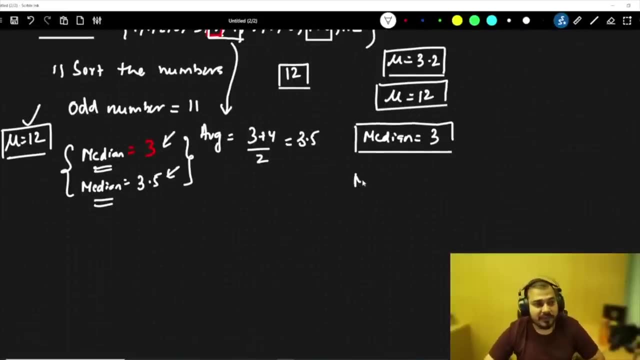 an outlier, my median was 12.. sorry, my mean was 12.. when i tried to do this with respect to median, even though i had outlier added the outlier, it came as 3 and finally, you will be able to see that when i probably used two outliers and then probably i got the median as 3.5. now here you can basically. 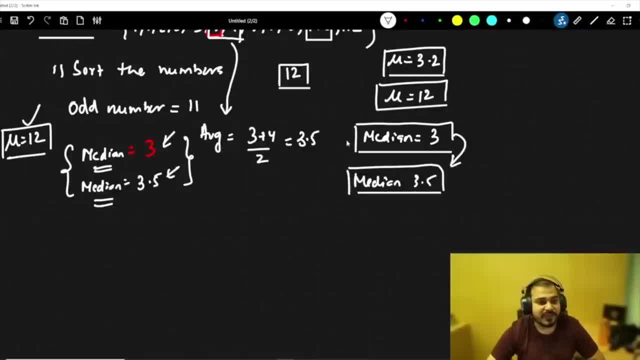 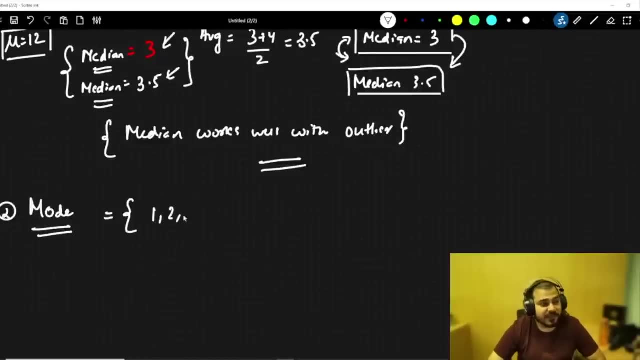 see that there is less difference, right, less difference when compared to this. if i talk about median, it works well with outlier, so this is the proper statement that i want to consider now in the case of mode, the third topic. now suppose if i have a specific data set like this: one, two, three, four, five, six, 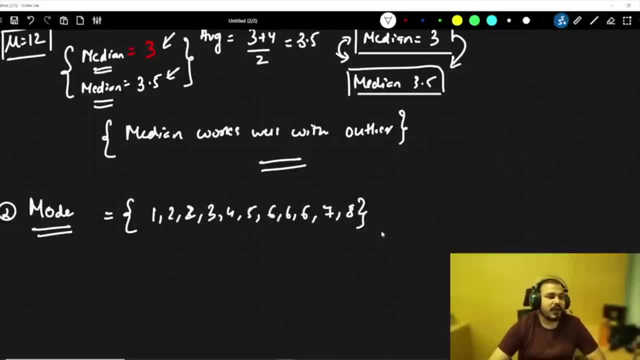 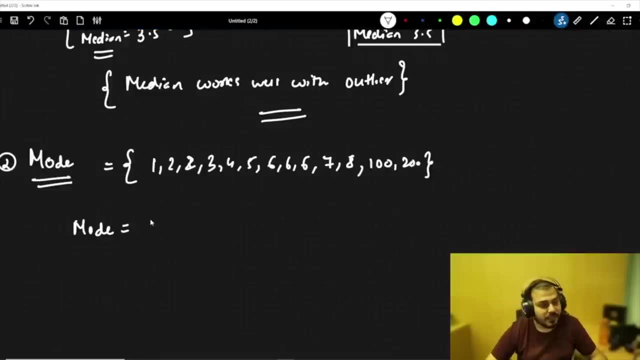 six, six, seven, eight now, even though i have some outliers like 100, 200 now in this particular case, what should be our mode, which is again taken as a measure of central tendency over here, in this particular case, in mode, we find out the most frequent element, mode: most frequent element. 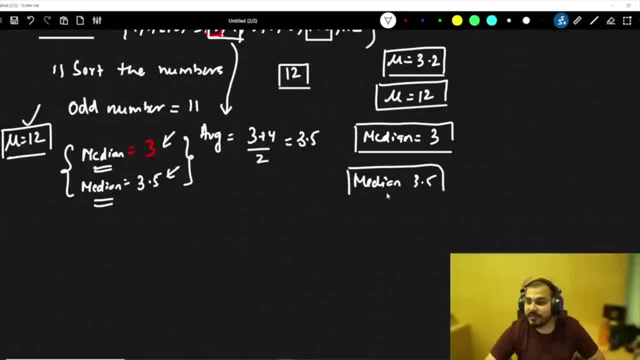 I got the median as three point five. Now here you can basically see that There is Less difference, right, less difference when compared to this. if I talk about median, it works well with outlier, So this is the proper statement that I want to consider. 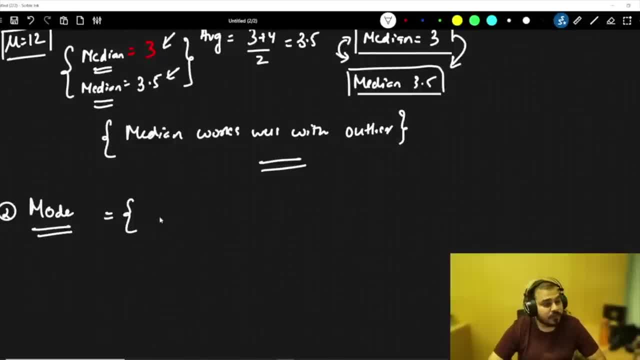 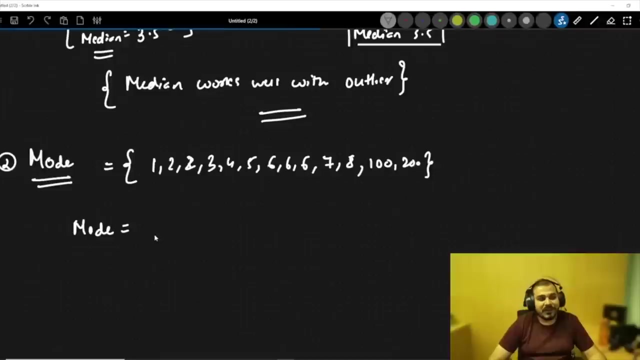 Now, in the case of mode, the third topic now, suppose, if I have a specific data set like this: one, two, three, four, five, six, six, six, seven, eight, Now, even though I have some outliers like hundred, two hundred nine, this particular case, That should be our mode, which is again taken as a measure of central tendency. 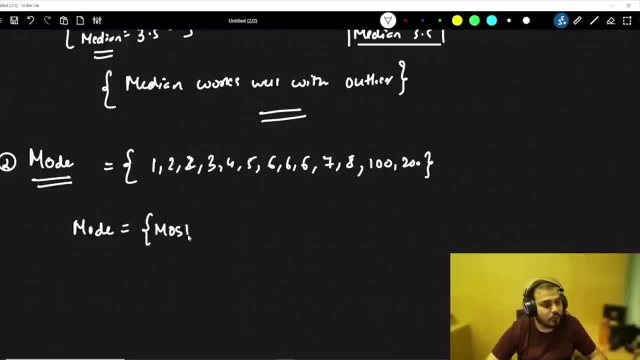 Over here, in this particular case in mode, we find out the most frequent element, mode most frequent element. Now, in the most frequent element we just try to count and we try to see that which element is having the maximum number of elements. So over here you can see six is basically having three. the count is three. 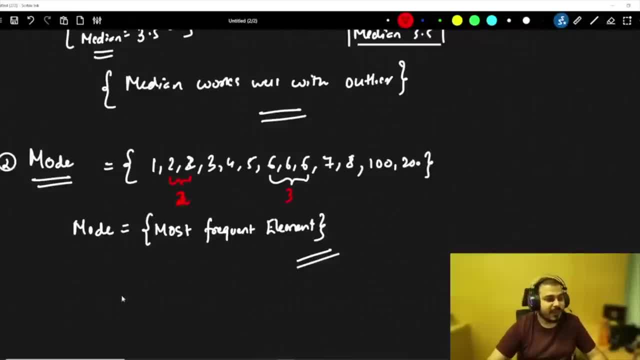 If you see two, the count is two. So in this particular case, My mode should definitely be six. My mode should be definitely six, which is again the measure of central tendency. Now, see guys, now in this particular case there is one disadvantage, even though, suppose let's. 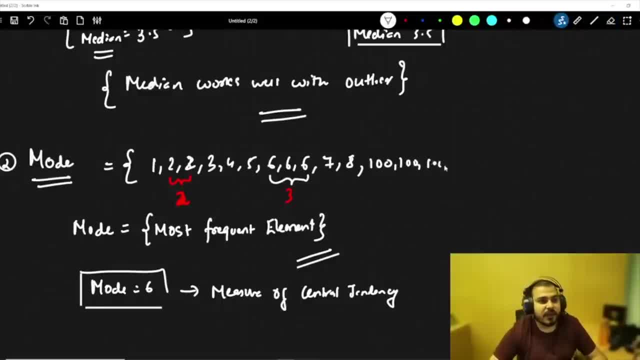 consider that I have many, many outliers like this: hundred, hundred or one more hundred. let's consider Now in this particular case. since we find out the most frequent element, we try to take this as an outlier. So usually in most of the outliers that we specifically use, 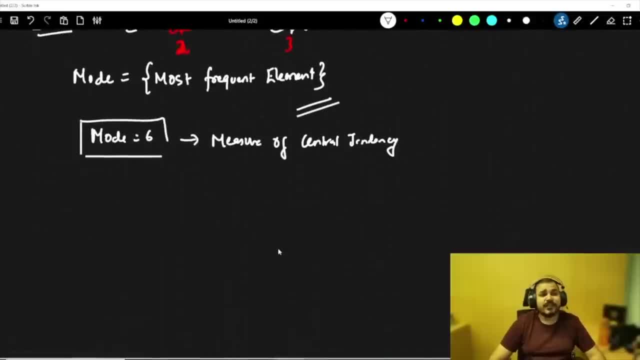 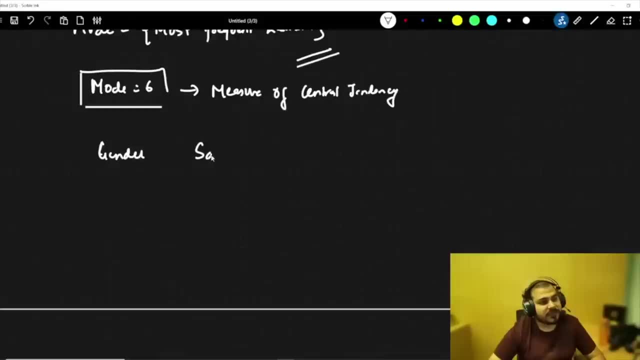 We basically use median Now where specifically mode is used. Let's consider one data set. Let's say that I have a data set which is called as gender salary. Let's consider- I have this In gender. you will probably find out: male female. male female. 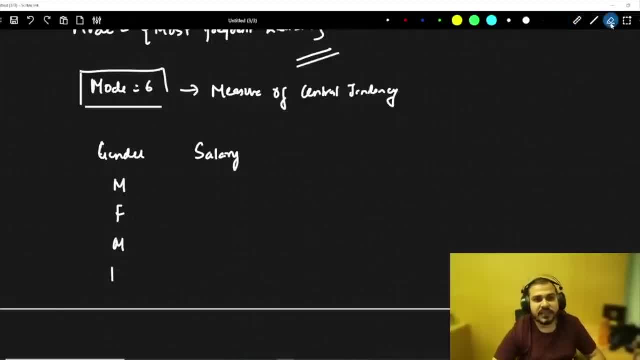 Some different, different values may be there. or let me just change this data set and make it in a simpler way. Why, specifically, we use mode in mode? also, we use it in both integer and categorical variables. Well, with categorical variables, Let's say that this is a type of flower. 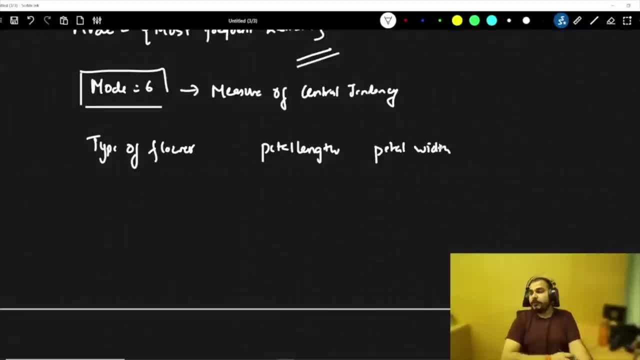 Type of flower, and this is petal length and petal width. Now over here, you will be able to see different, different flowers like rose, lily, sunflower, and you have some flowers. Let's consider that you have some missing data over here. 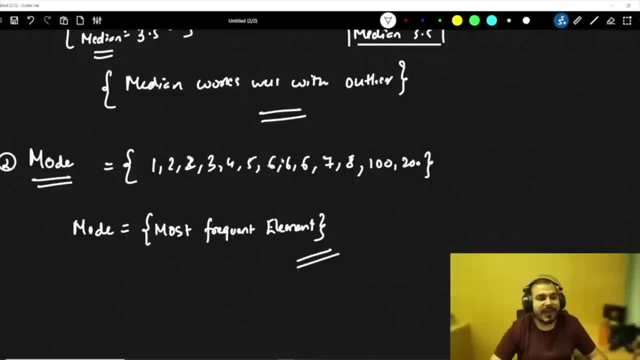 now in the most frequent element, we just try to count and we try to see that which element is having the maximum number of elements. so over here you can see 6 is basically having 3. the count is 3. if you see 2, the count is 2. so in this particular case my mode should definitely 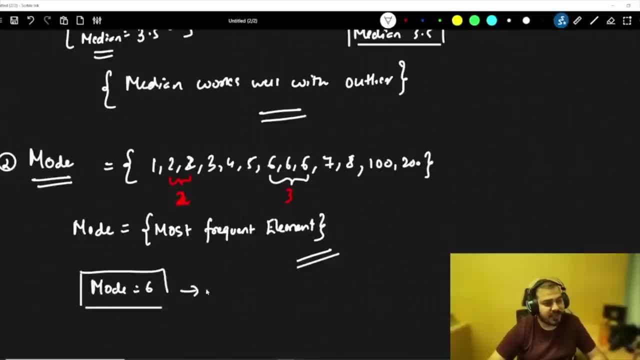 be 6, my mode should be definitely 6, which is again the measure of central tendency. now, see, guys, now, in this particular case there is one disadvantage, even though, suppose let's consider that i have many, many outliers like this: hundred, hundred or one more hundred. let's consider: 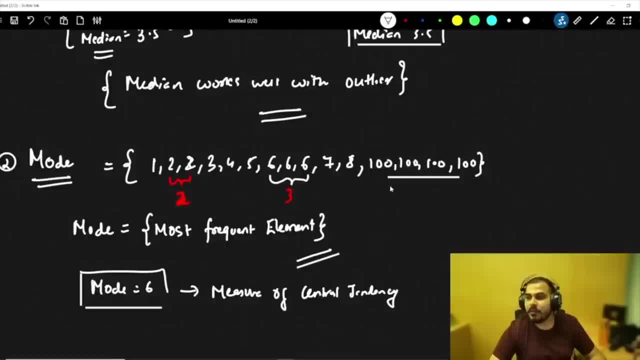 now, in this particular case, since we find out the most frequent element, we try to take this as an outlier. so usually in most of the outliers that we specifically use, we basically use median. now where specifically mode is used, let's consider one data set. let's say that i have 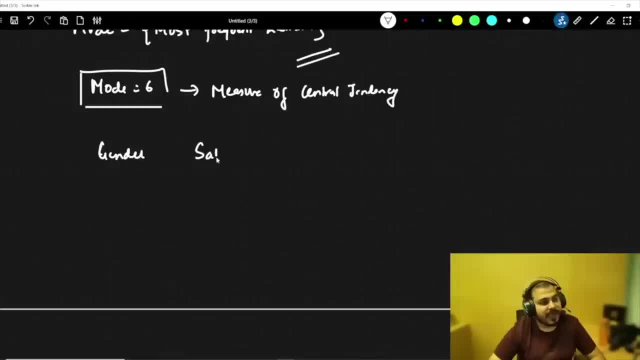 a data set which is called as gender salary. let's consider: i have this in gender. you will probably find out: male female, male female. some different, different values may be there. or let me just change this data set and make it in a simpler way. why specifically we use mode in mode also. 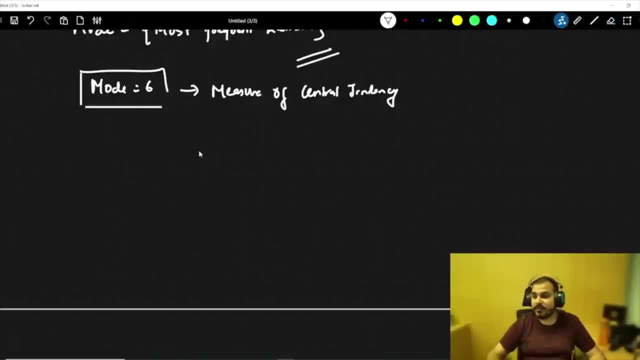 we use it in both integer and categorical variables, but it works well with categorical variables. let's say that this is a type of flower, type of flower, and this is petal length and petal width. now, over here, you will be able to see different, different flowers like rose, lily, sunflower and 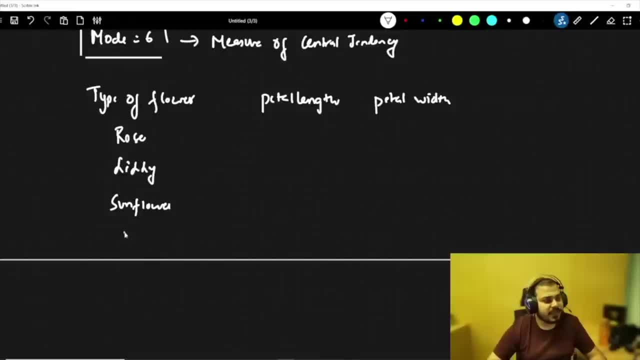 you have some flowers. let's consider that you have some missing data over here and, based on this missing data, now this particular data set has come to me and let's say, consider that i i've seen in this particular data there are 10 missing data. now what do you think in order to handle this missing? values. in order to handle this value, missing values is given settle for 10.5 percent. 10.5 percent, that's the number. four million percent. missing data are about 10.4 percent missing. now, what do you think? in order to buy half a country, form am. 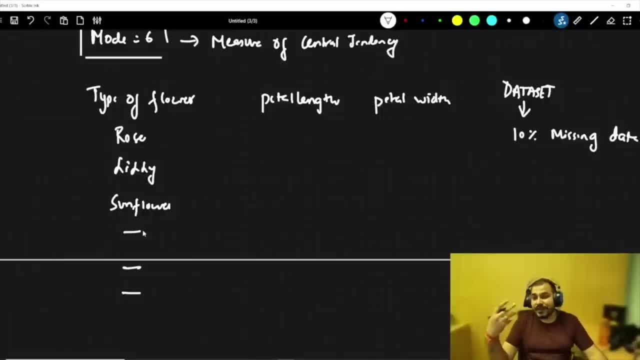 values, what type of things we can definitely use from mean median mode. don't you think i can definitely use mode over here, because the most frequent occurring flower can be replaced with this missing value. so the what i'm saying: the missing value will be replaced with most frequent. 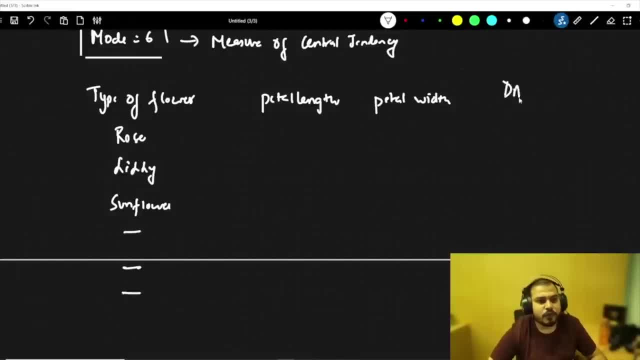 And based on this missing data. now this particular data set has come to me And, let's say, consider that I have seen in this particular data there are around 10% missing data. Now, what do you think In order to handle this missing values, what type of things we can definitely use from? 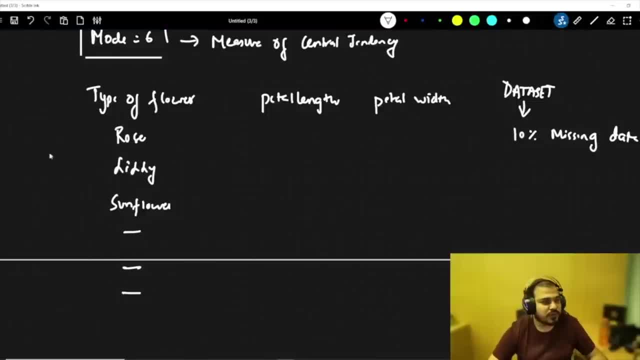 mean median mode, Don't you think? I can definitely use mode over here, Because the most frequent occurring flower can be replaced with this missing value. So what I am saying: the missing value will be replaced with most frequent occurring element, So we can definitely say that most frequent element. 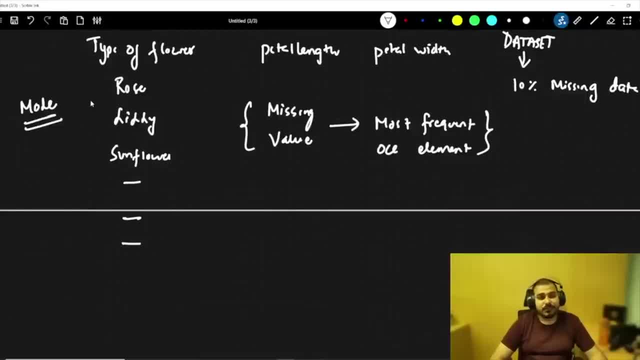 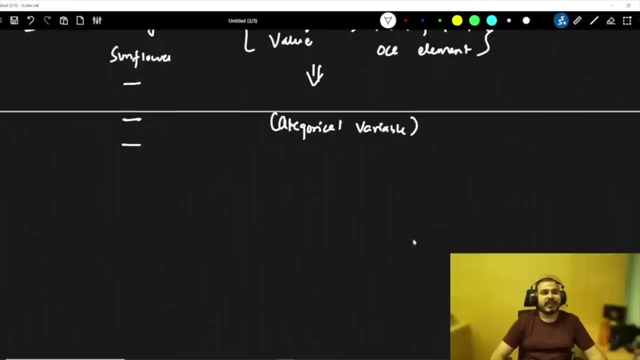 You can actually get it by using mode Which is most frequently used, and this specifically works well with categorical variable. Now let's take another example. Suppose I have a feature age- Age. I have values like 25,, 26,, dash, dash, dash, dash, 32,, 34,, 38. 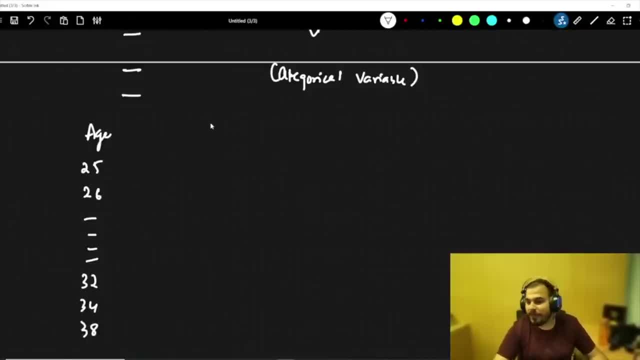 Now, in this particular case, what do you think what may be a suitable thing? Suppose let's say that these are my ages of students. Should I apply categorical variables? Yes, I have mean median or mode. Which do you think, based on this scenario, that is, ages of students? we should definitely. 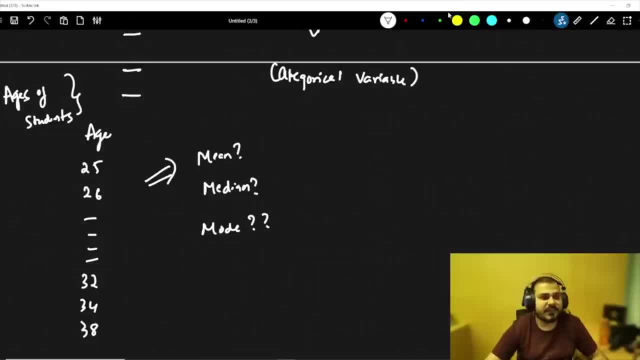 apply? Just tell me this answer. In this particular case, definitely. I would suggest let's go with mean, Because I know students age will basically range from one value to one value. It won't extend more than that specific value. So here a domain knowledge will also come into existence. 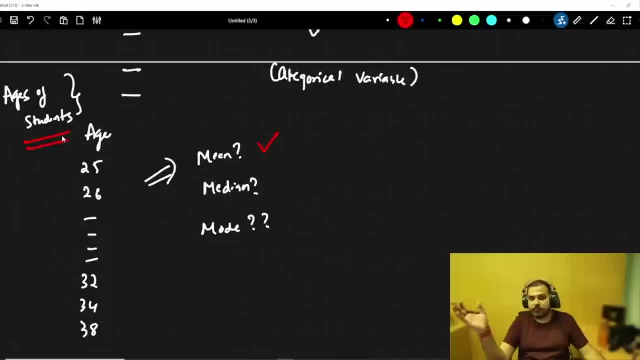 If I say that this is probably the ages of all the parts Of all the population throughout the world, probably I will not go with mean So something like that, you know. So this is a very good example, Very good understanding with respect to various use cases that we can actually take. 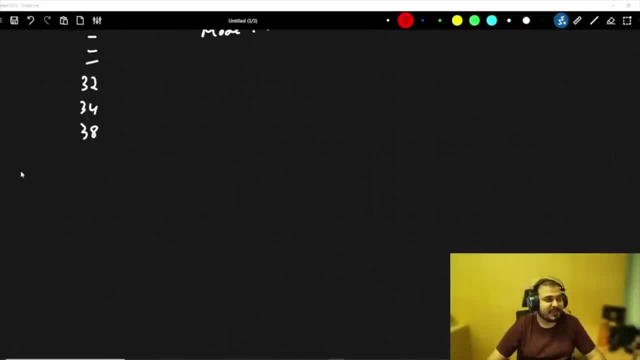 Now let's go and discuss about the next major topic, which is called as measure of dispersion. Now, in measure of dispersion, what all things we specifically discuss? We discuss about two main topics: One is variance, And the second one is something called as standard dispersion. 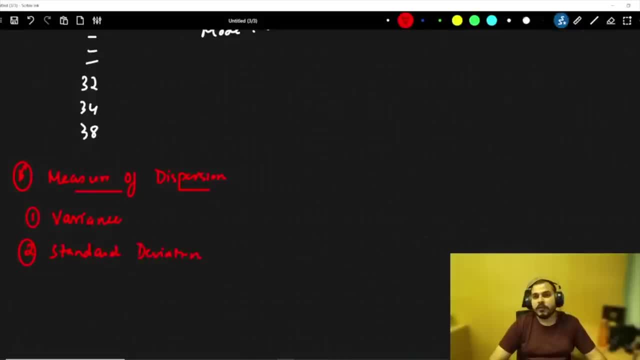 So what are the things we specifically discuss? We discuss about two main topics. One is variance And the second one is something called as standard dispersion. So let's go ahead and let's discuss about this Now. first topic is basically with respect to variance. 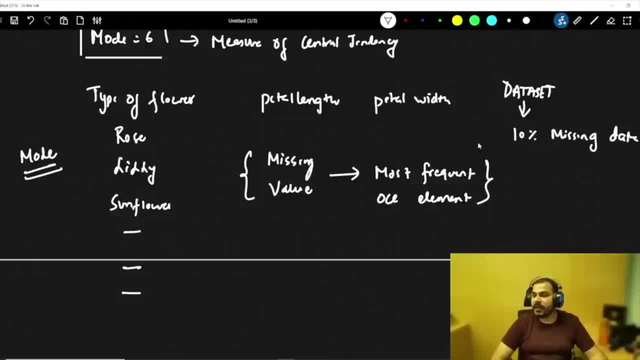 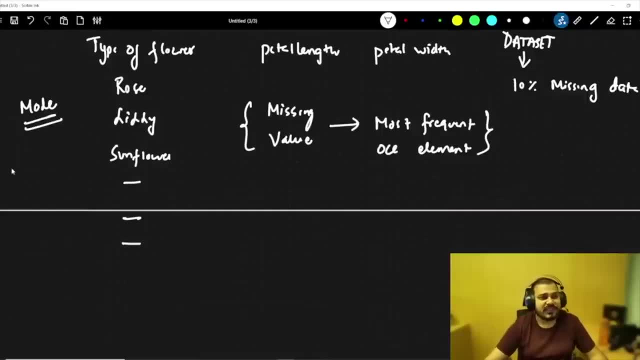 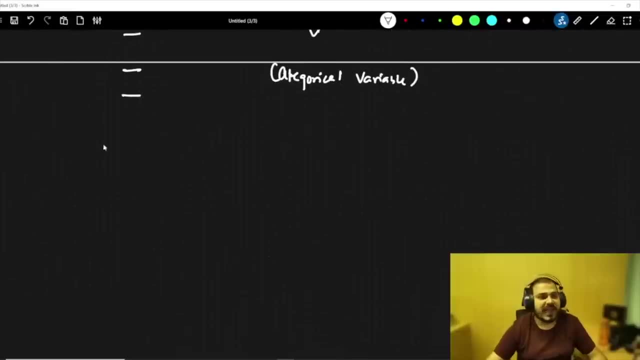 occurring element, so we can definitely say that most frequent element. you can actually get it by using mode which is most frequently used and this specifically works well with categorical variable. now let's take another example. suppose i have a feature age, age i have values like 25, 26. 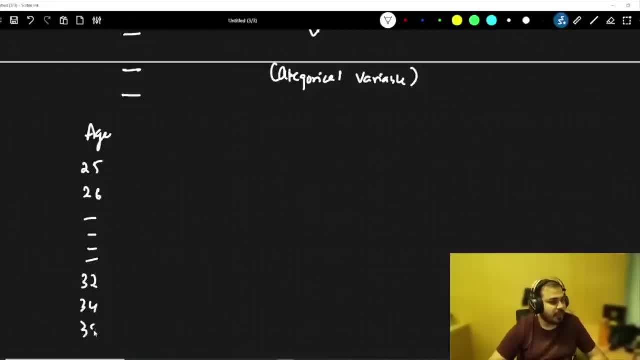 dash, dash, dash, dash, 32, 34, 38. now, in this particular case, what do you think? what may be a suitable thing? suppose let's say that these are my ages of students. should i apply mean median, median or mode? which do you think, based on this scenario, that is ages of students? 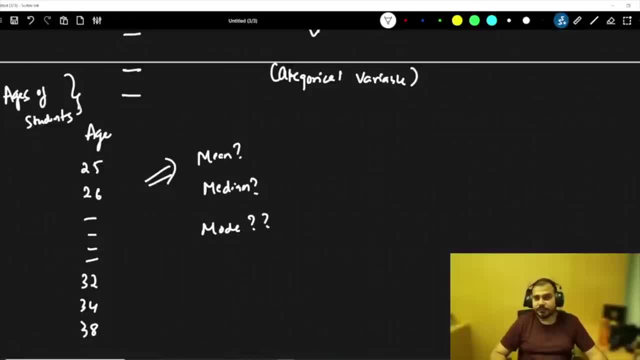 we should definitely apply. just tell me this answer. in this particular case, definitely. i would suggest let's go with mean, because i know students age will basically range from one value to one value. it won't extend more than that specific value. so here a domain knowledge will. 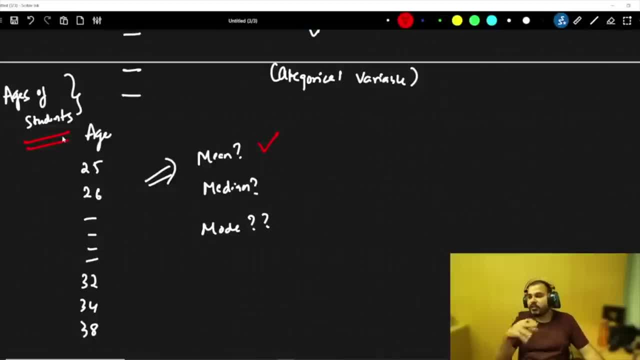 also come into existence. if i say that this is probably the ages of all the population throughout the world- probably the ages of all the population throughout the world, probably the ages of all the population of the world- will be smaller than that and it will also look a little bit confusing. 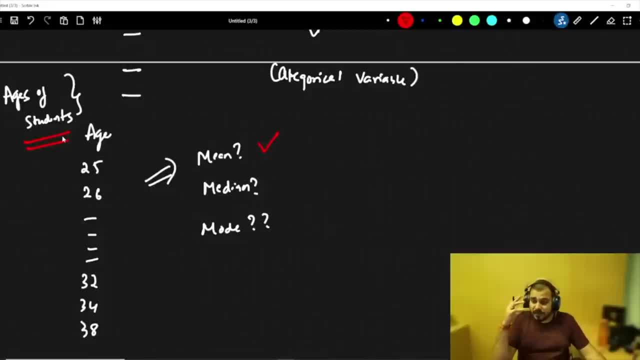 to me also, and i also know that so far in the country, so probably i will not go with me, so something like that, you know. so this is a very good example, very good understanding with respect to various use cases that we can actually think. now let's go and discuss about the next. 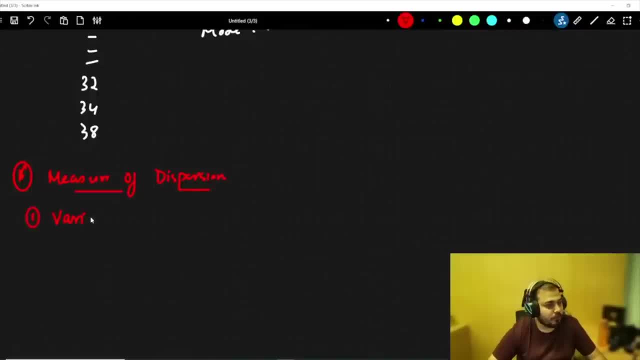 major topic, which is called as measure of dispersion. now, in measure of dispersion, what all things we specifically discuss? we discuss about two main topics: one is variance and the second one is topics that we are probably going to discuss. so let's go ahead and let's discuss about this. 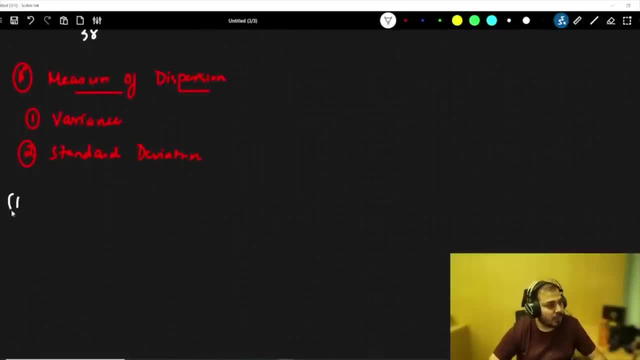 now, first topic is basically with respect to variance. now, how do we define variance? variance is a concept of measure of dispersion and probably for an interviewer also, this may be a confusing question. they may ask candidates, you know, and they may probably make them understand different, different things and they may again confuse you. but when i say dispersion, dispersion, 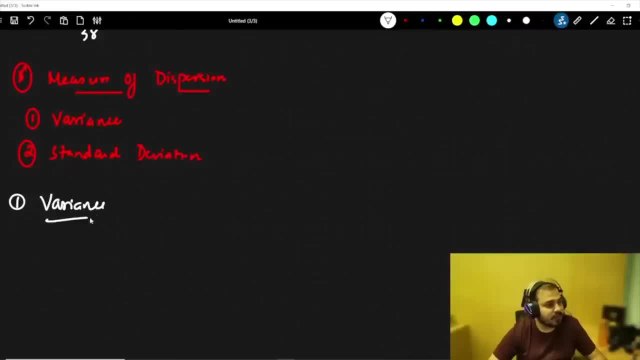 Now, how do we define variance? Variance is a concept of measure of dispersion And probably for an interviewer also, this may be a confusing question. they may ask candidates, you know, And they may probably make them understand different, different things, and they may again confuse you. 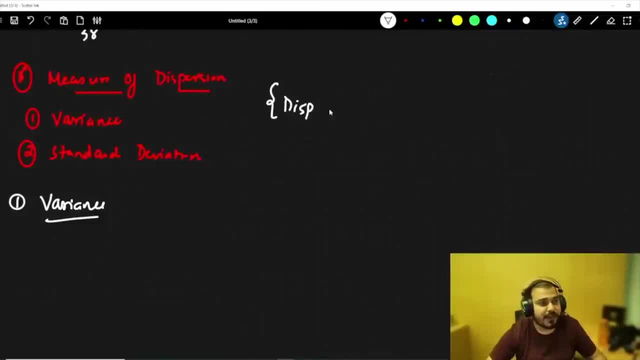 But when I say dispersion, Dispersion Basically means spread. Please make sure that you remember this word. This basically means spread, Okay, spread, How spread, How well spread your data is With the mean? obviously? see, Let's say that I have two data sets. 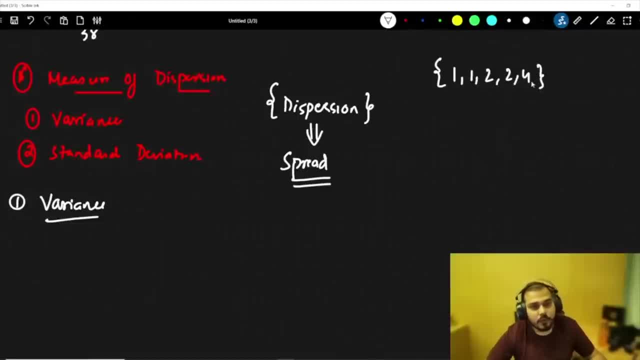 I have data set like 1, 1, 2, 2, 4.. What is the mean? 10 divided by 5 is 2.. Now let's consider that I have another distribution which looks like this: 2, 2, 2, 2, 2.. 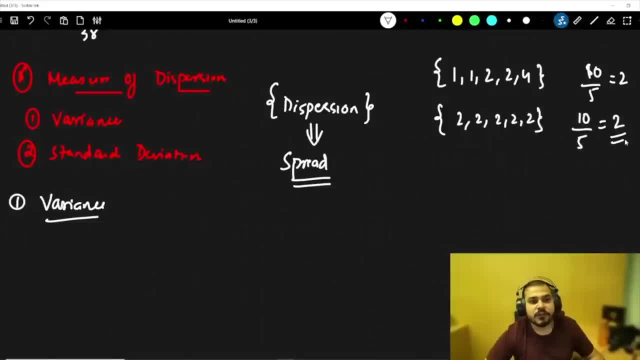 This is my next distribution. If I try to find out the average, then also it is 2.. So for both this distribution we are getting the same average or mean. I'm getting the same mean, right? So if I'm getting the same mean, then how do I identify that this two distributions are different? 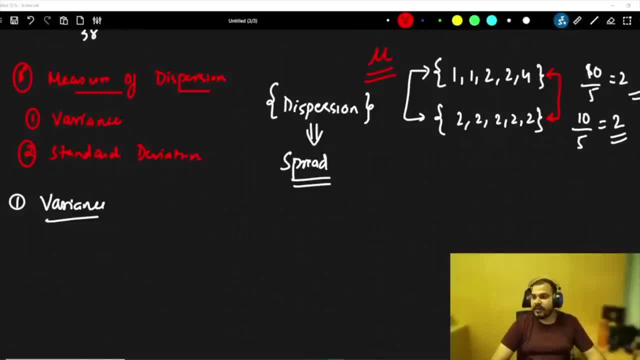 Because we need to think about it right. How do we basically come up Like with this? is that how this two distribution is different? We really need to understand. Okay, and probably interviewer may say you- And he may confuse you- in dispersion, What is variance? 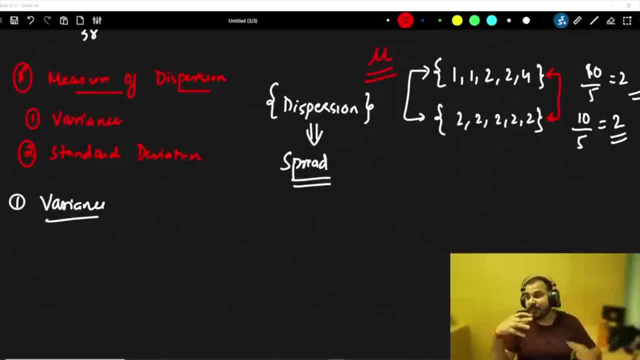 He may definitely confuse you. So for that specific reason, if you really want to identify how two distribution are different, At that point of time we may use variance and standard deviation. Now let's go ahead and let's try to understand the formula with respect to variance and standard deviation. 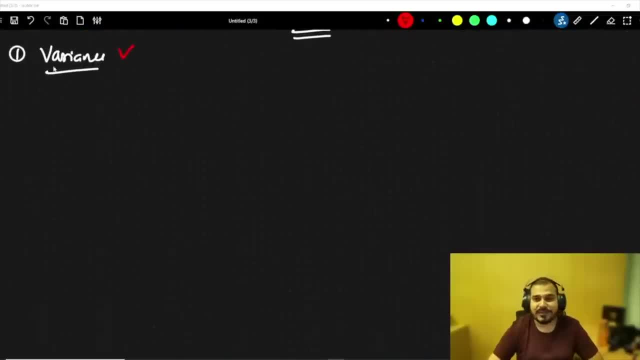 And here also I will probably talk about two different things. And here one very, very important interview question will come. One is population variance And one is About sample variance. So this two things why I'm teaching you with respect to population sample, it will all make sense. 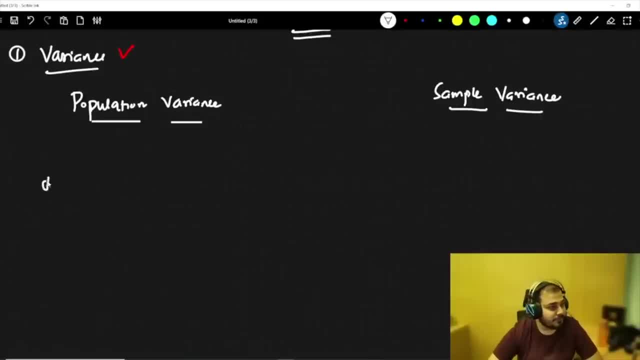 So usually population variance is given by something called as sigma square. Here you basically use as summation of: i is equal to 1 to capital N, X of i minus mu, whole square divided by N. Sample variance is basically given by Small s square. 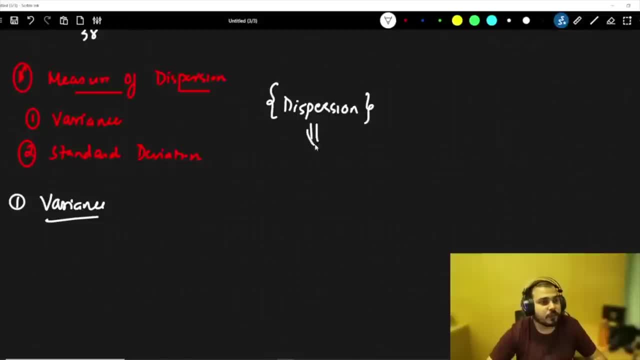 basically means spread. please make sure that you remember this word. this basically means spread. okay, spread, how spread, how well spread your data is with the mean, obviously. see, let's say that i have two data sets. i have data set like one, one, two, two, four. what is the mean? 10 divided by 5 is 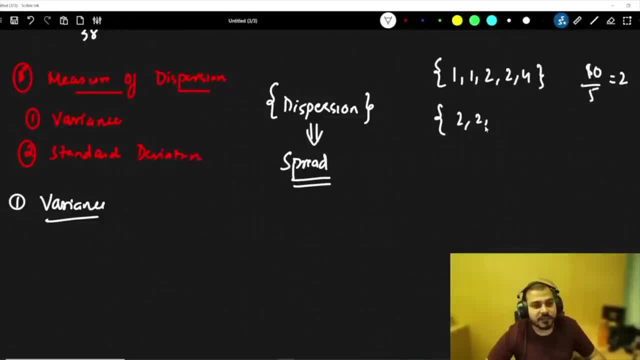 2. now let's consider that i have another distribution which looks like this: 2, 2, 2, 2, 2. this is my next distribution. if i try to find out the average, then also it is 2, so this is my next distribution. what is variance? he may definitely confuse you, so for that specific. 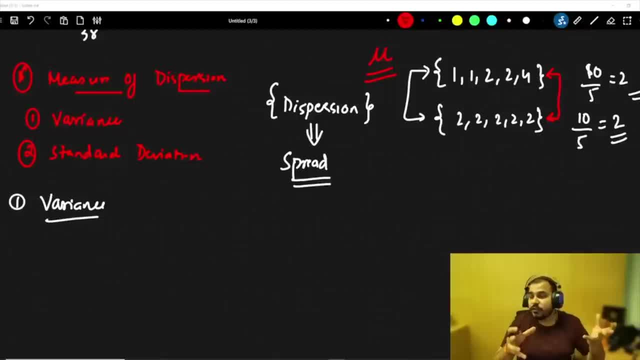 reason. if you really want to identify how two distribution are different, at that point of time we may use variance and standard deviation. now let's go ahead and let's try to understand the formula with respect to variance and standard deviation, and here also i will probably talk. 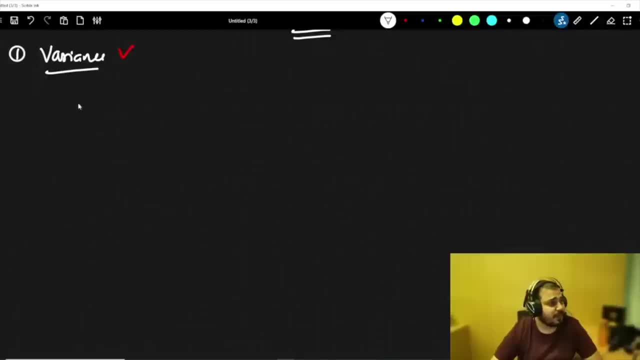 about two different things, and here one very, very important interview question will come. one is population variance and one is about sample variance. so this two things why i am teaching you. with respect to population sample, it will all makes sense. so usually population variance, ah, is given by something called as sigma square. here you 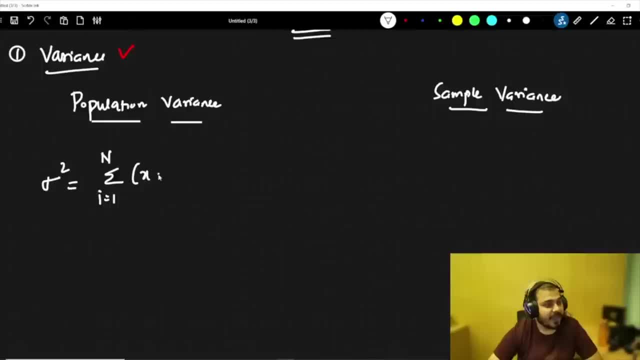 basically use as summation of i is equal to 1 to capital n X of i minus mu. whole square divided by n. sample variance is basically given by small s square. summation of i is equal to 1 to small n x of i minus x bar. x bar basically means sample mean. 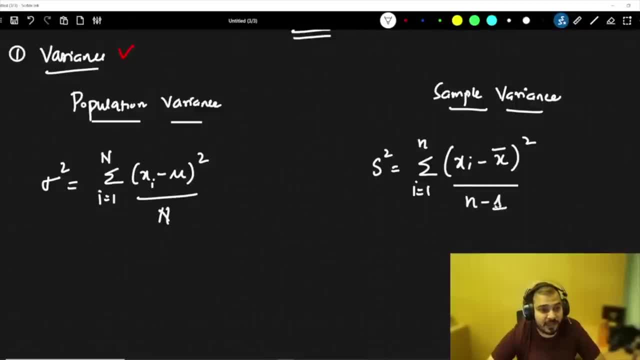 divided by n minus 1. now many people will say: so why n minus 1? n minus 1? yes, this is an interview question. uh, i will talk about it. okay, i will talk about it, don't worry. so let's let's take one very good example, probably, and uh, we'll try to solve this specific problem. let's consider that i have 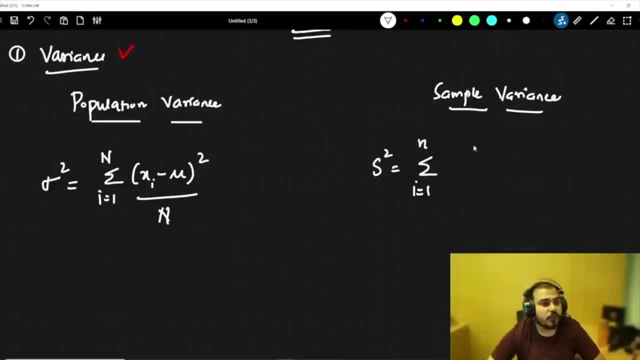 Summation of Summation of i is equal to 1 to small n X of i Minus X bar. X bar basically means sample mean Divided by N minus 1.. Now many people will say: so why N minus 1, N minus 1.. 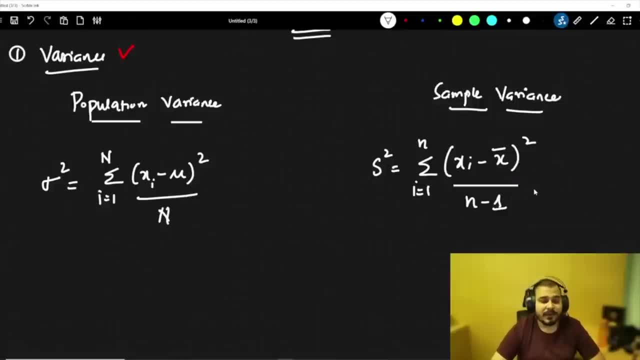 Yes, this is an interview question. I will talk about it. I will talk about it, Don't worry. So let's let's take one very good example, probably, and we'll try to solve this specific problem. Let's consider that I have my 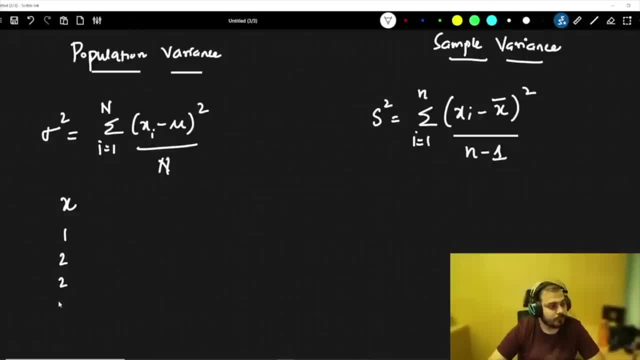 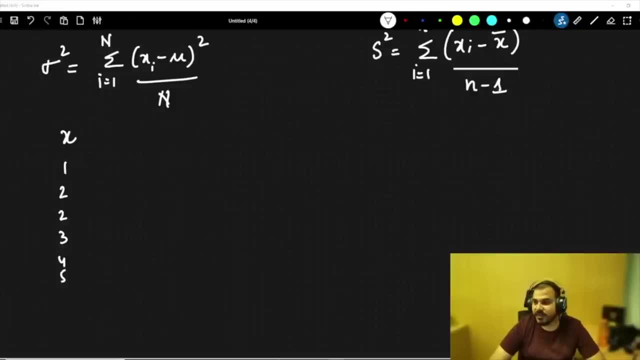 X value as 1, 2, 2, 3, 4, 5.. So this is my distribution. So probably over here this is basically my data set. So first thing, first let's go and calculate. Now we'll go and calculate. So, with respect to population, we'll go and calculate the mu: 2.83.. 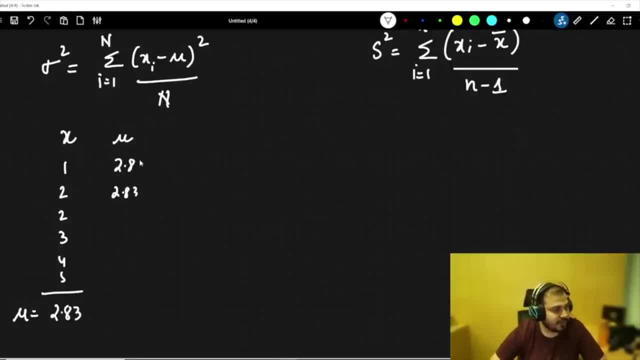 So here mu is basically 2.83, 2.83, 2.83, 2.83, 2.83, 2.83.. The next thing is that From this equation I will try to calculate X minus mu. So what is X minus mu over here? 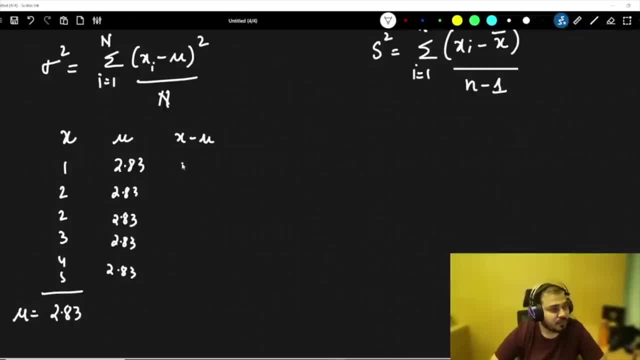 Just do the calculation, and it is good that you do the calculation. So here I get minus 1.83.. Here I get minus 0.83.. This will basically become 0.17.. This is plus, And over here you'll be able to see that this will become 1.17.. 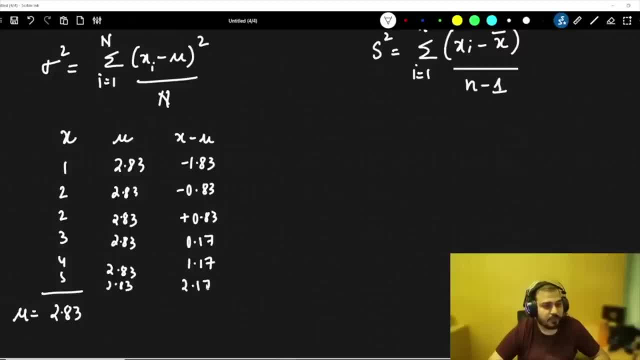 And then for the 5, you have this and it will become 2.17.. Now the next step: you basically do the squaring. Now, if you do the squaring, that is X minus mu whole square. you just have to do the square of this: 3.34.. 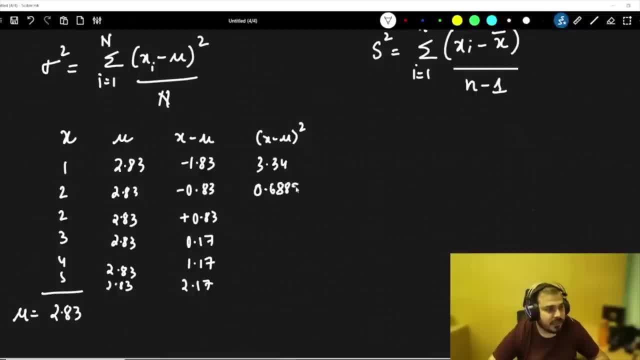 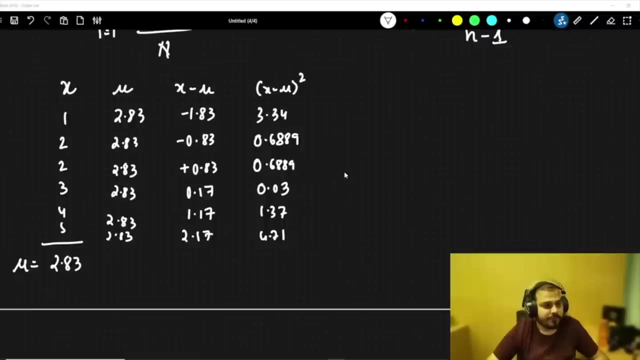 So here you can see 0.6889, then here also I can see 0.6889, and then for the remaining one you can do the calculation. So here it will be 0.03, 1.37 and finally you'll be able to see 4.71.. 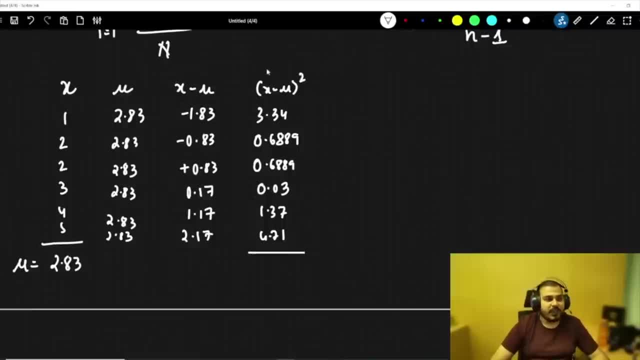 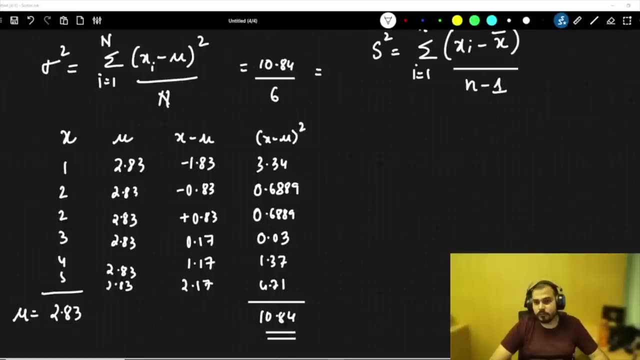 Then what we do? we do the addition of this, because summation of this is there right. So once we do the addition, probably, then we probably calculate it. If I do the addition, this is nothing but 10.84. 10.84 divided by 1, 2, 3, 4, 5, 6, 1.81.. 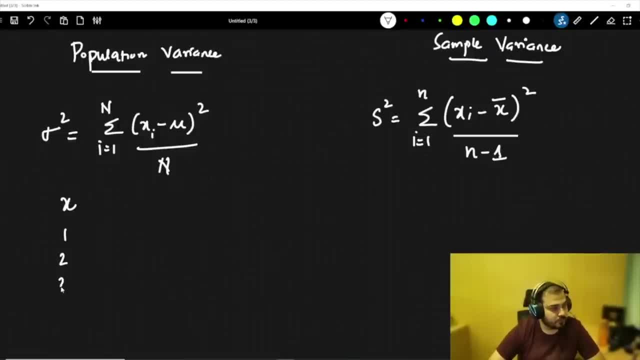 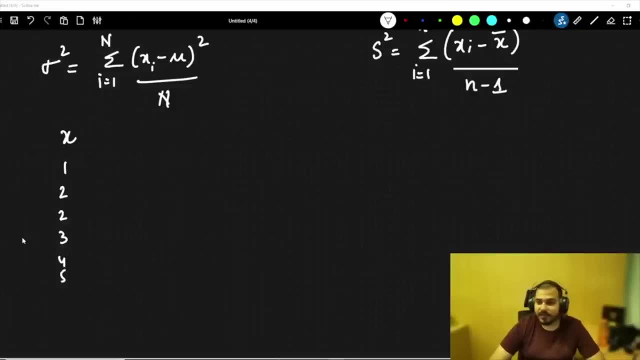 my x value as 1, 2, 2, 3, 4, 5. so this is my uh distribution. so probably over here this is basically my data set. so first thing, first let's go and calculate. now we'll go and calculate. so with respect to population, we will go and calculate the mu: 2.83. so here mu is basically 2.83, 2.83. 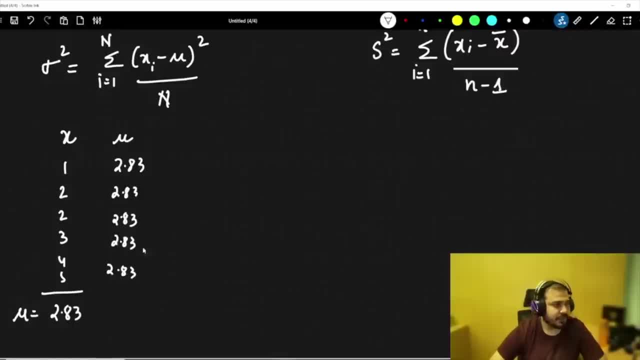 2.83, 2.83, 2.83. the next thing is that from this equation i will try to calculate x minus mu. so what is x minus mu over here? just do the calculation, and it is good that you do the calculation. so here i get minus 1.83. here i get. 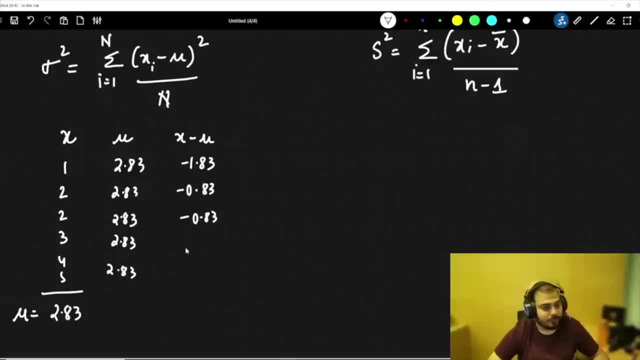 minus 0.83, this will basically become 0.17. this is plus, and over here you will be able to see that this will become 1.17, and then for the 5, you have this and it will become 2.17. now the next step. 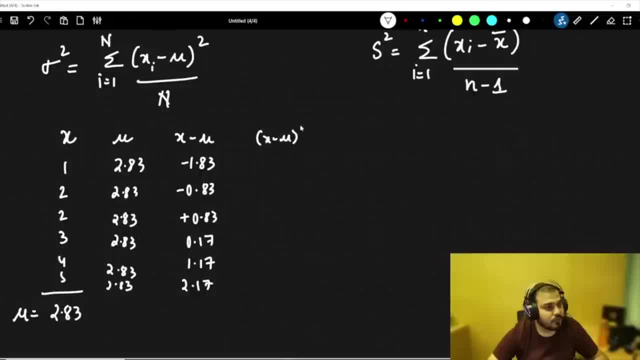 now, if you do the squaring, that is x minus mu whole square, you just have to do the square of this 3.34. so here you can see 0.6889, then here also i can see 0.6889, and then for the remaining one you 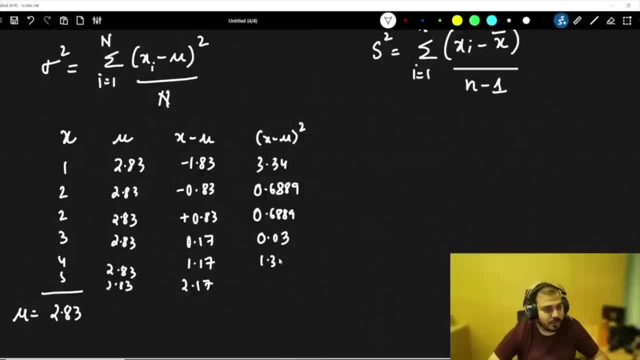 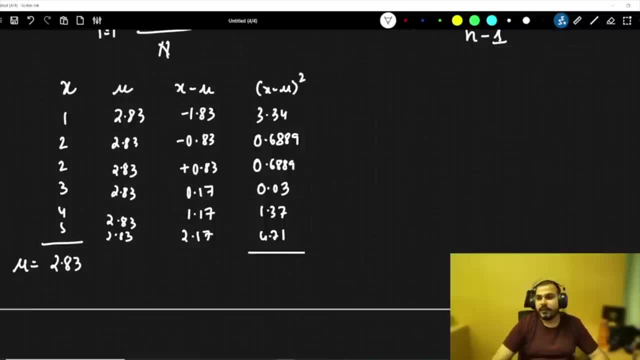 can do the calculation. so here it will be 0.03, 1.37 and finally you will be able to see 4.71. then what we do? we do the addition of this, because summation of this is there right. so we do the addition probably, then we probably calculate it. if i do the addition, this is nothing. 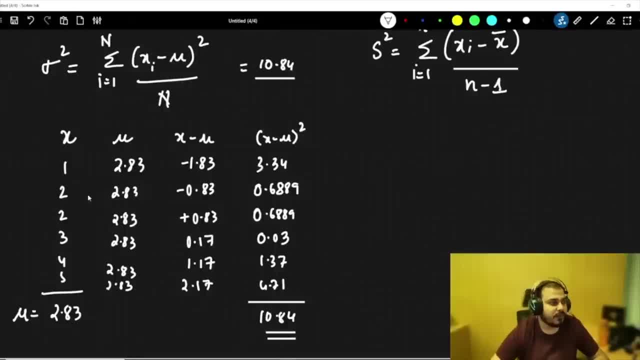 but 10.84. 10.84 divided by 1, 2, 3, 4, 5, 6, 1.81. now understand one thing. let's say, if i have a data set which looks something like this and if i have a data set which looks something like this: 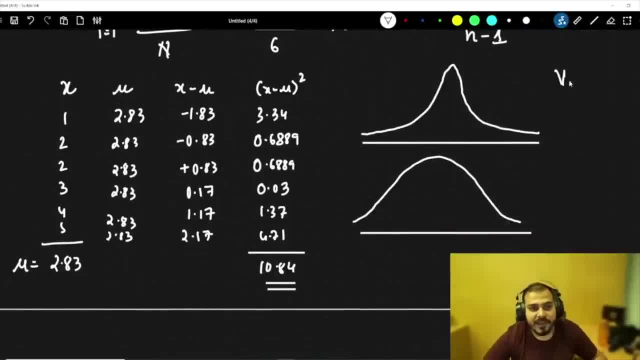 comparing these two data. where do you think the variance is? more variance, understand variance, variance. whenever your things comes into mind, it should be talking about spread. so over here in the second picture, definitely variance will be higher. let's consider that. i'm just going to take this. 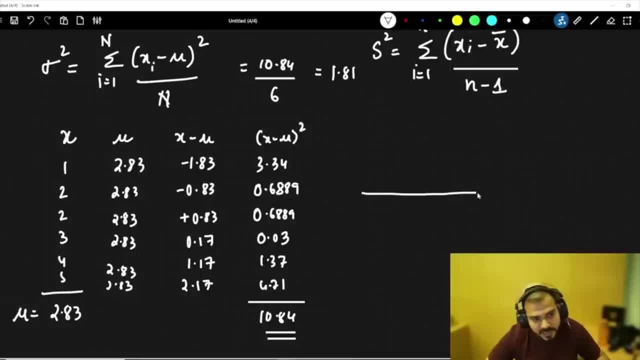 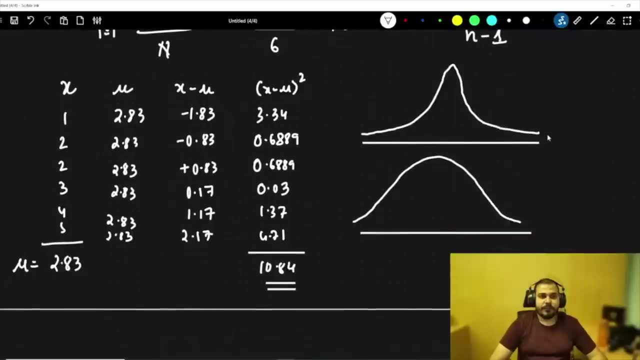 Now understand one thing. let's say, if I have a data set which looks something like this And if I have a data set which looks something like this, Comparing this two data, where do you think the variance is? more Variance, understand variance. 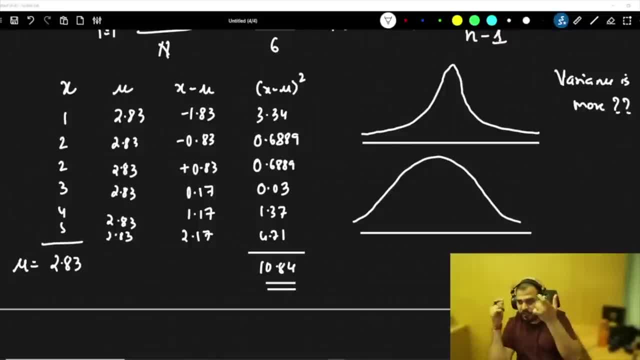 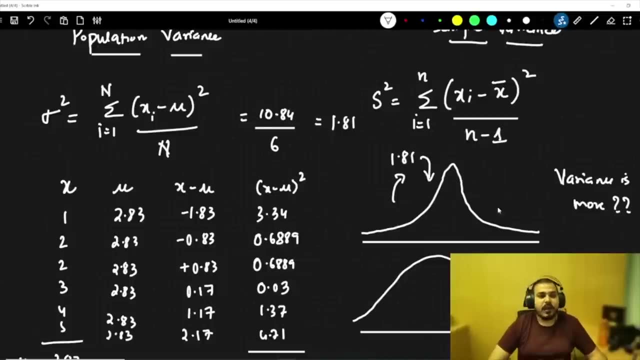 Variance. whenever your things comes into mind, it should be talking about spread So over here in the second picture, definitely variance will be higher. Let's consider that I'm just going to take this example here. my variance is 1.81.. Let's consider that this is 1.81.. 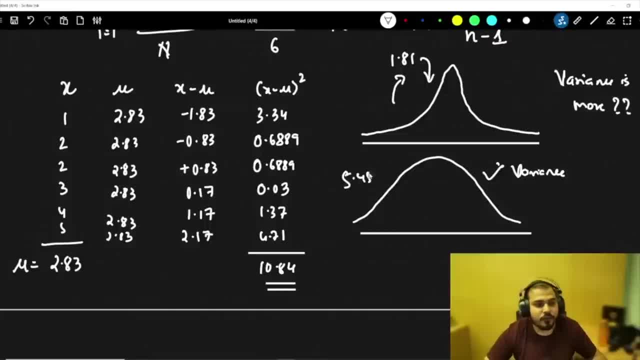 And tomorrow, if I probably get 5., 4, 5. can I say that it may belong to this particular distribution? yes, so the variance will be definitely higher because the spread is quite high spread when. when we say spread is basically high, that basically means the elements that is present in the central region is more. 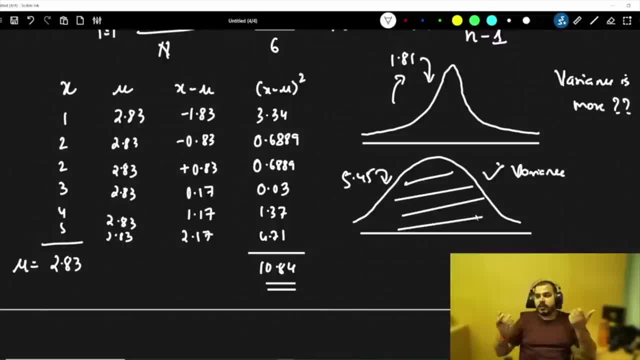 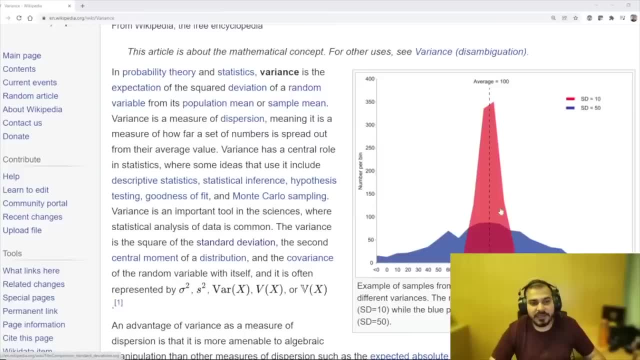 Whenever I talk about more variance, that basically means the data is more dispersed. Let me talk about this also to you, so that you can understand. Okay, Now Let's forget about standard deviation, for right now. now, in this particular image, let's see: 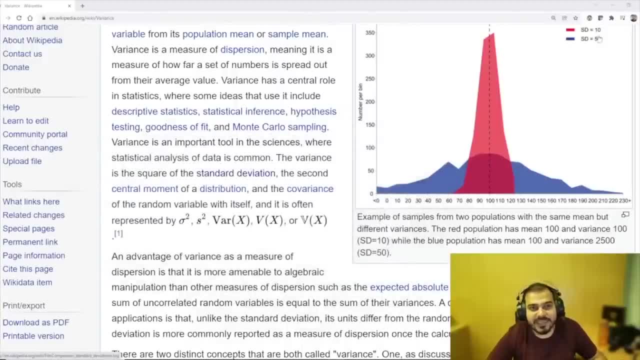 In this particular image. what do you see over here? You can see over here: standard deviation is 10, standard deviation is 50. Now, if you see standard deviation formula, it is nothing but root of variance. Now, here you can see: when the standard deviation is smaller, that basically means you're, you're. 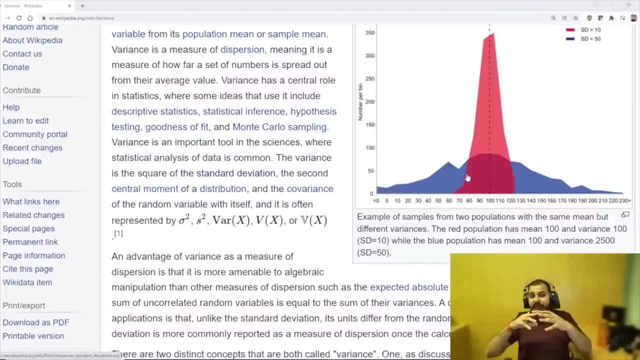 having a very huge curve. that basically means- the graph- that the data is not that much distributed. When You Have a standard deviation like 50, 60 and all you can see, your data is highly distributed. So this is very much important to understand why variance is more for dispersed data, because 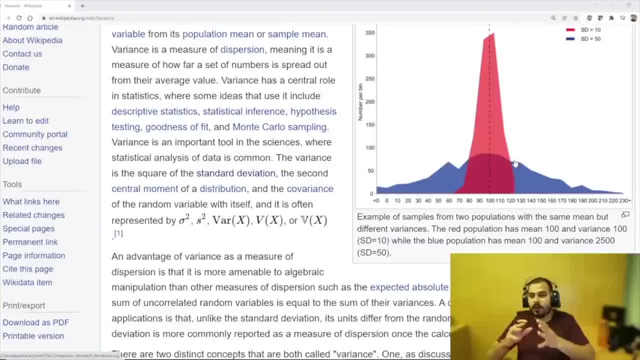 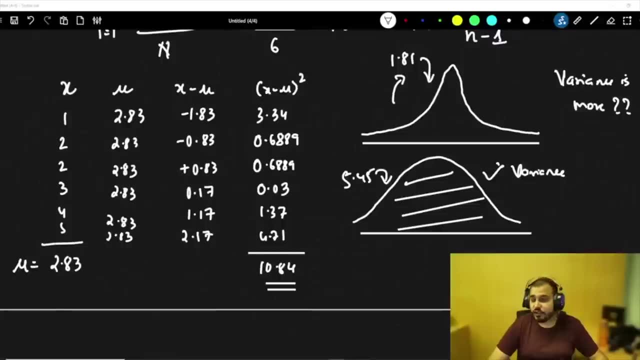 the only you can see, right guys? Okay, let me- when, when you probably calculate, I'll show you some of the problem statements over here. but just understand this graphical, okay. Later on I'll just show you one example where probably I will talk about it and let's try. 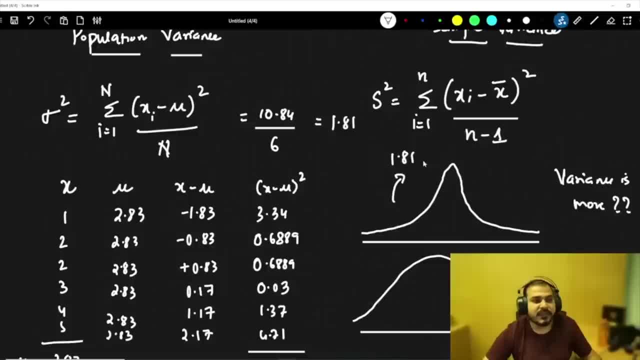 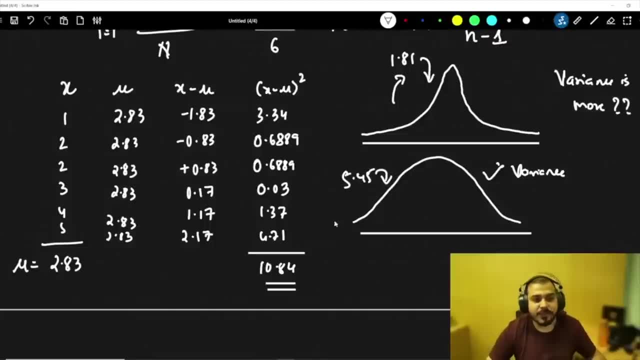 example. here my variance is 1.81. let's consider that this is 1.81 and tomorrow, if i probably get more, variance will be higher here because of the spread of the different set elements. can i say that it may belong to this particular distribution? yes, so the variance will be definitely. 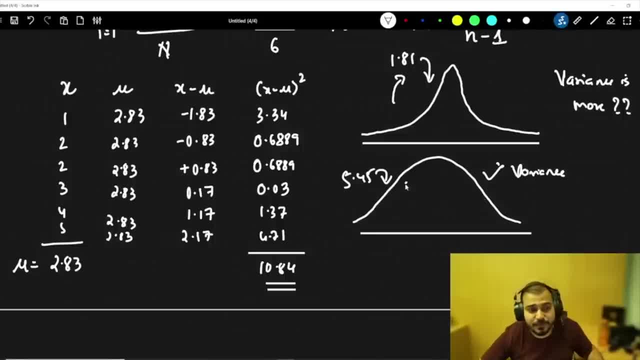 higher because the spread is quite high spread. when when we say spread is basically high, that basically means the elements that is present in the central region is more. whenever i talk about more variance, that basically means the data is more dispersed. let me talk about this also to you. 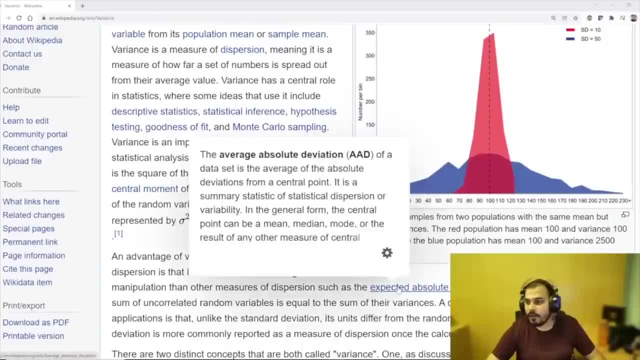 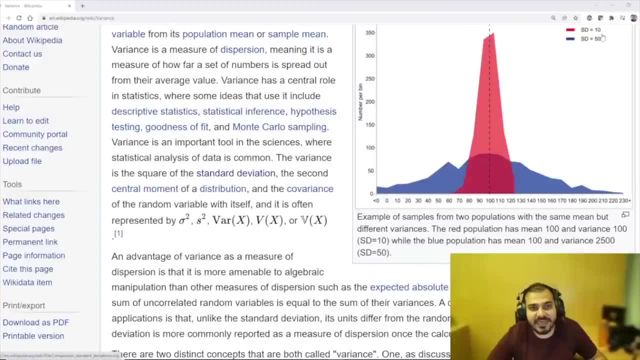 so that you can understand. okay, deviation for right now. now, in this particular image. let's see in this particular image. what do you see over here? you can see over here: standard deviation is 10, standard deviation is 50. now, if you see standard deviation formula, it is nothing but root of variance. now, here you can see when. 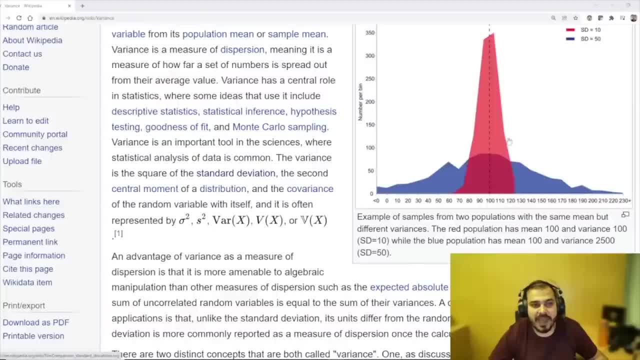 the standard deviation is smaller. that basically means you're you're having a very huge curve. that basically means the graph, the data, is not that much distributed when you have a big standard deviation, like 50, 60 and all you can see your data is highly distributed. so this is very much. 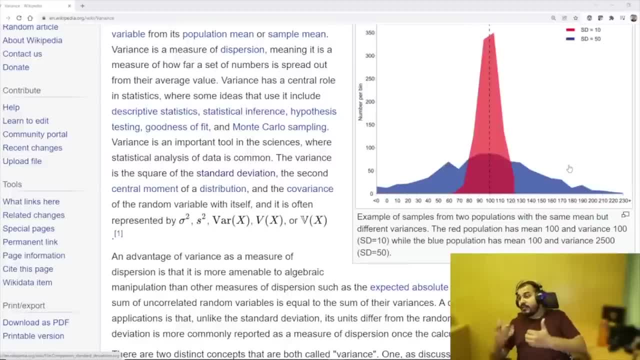 important to understand why variance is more for dispersed data, because over here you can see, right guys. okay, let when, when you probably calculate, i'll show you some of the problem statements over here. but just understand this graphically, okay, later on i'll just show you one example where 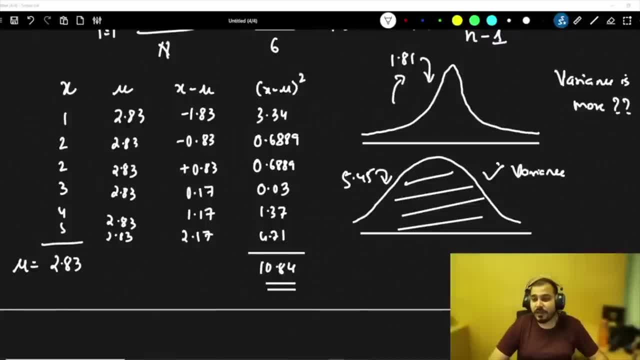 probably i will talk about it and let's try to solve that particular example and then we can definitely understand it. but some idea you basically got, because obviously the variance needs to be spreaded high. if the variance is high, right, the dispersion becomes high because you have more number of values inside it. 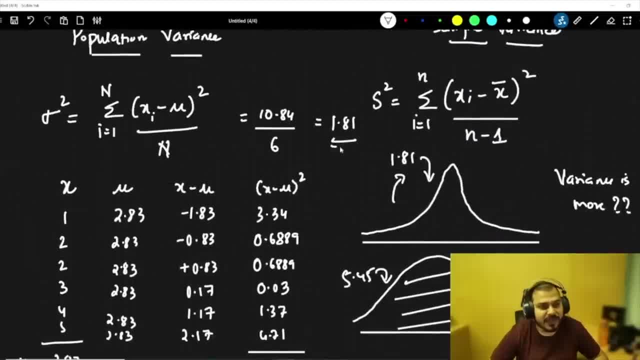 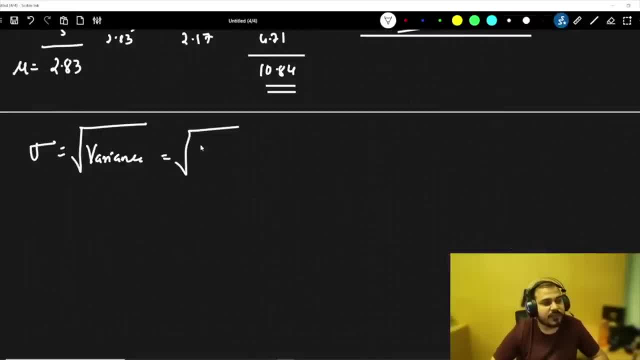 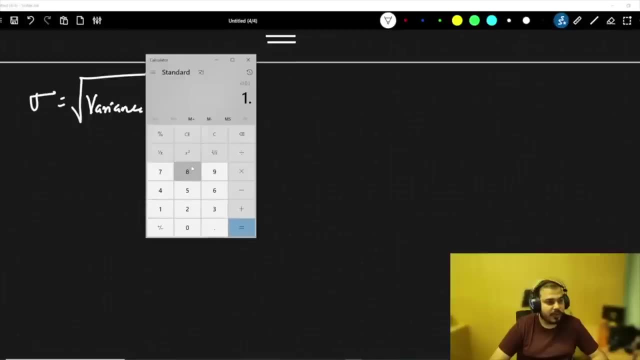 now let's go ahead and let's try to see. now i got my variance as 1.81. now my standard deviation is nothing but root of variance. root of variance, that basically means it is nothing but root of 1.81. so if i go and open my calculator, i'll just say root of 1.81. 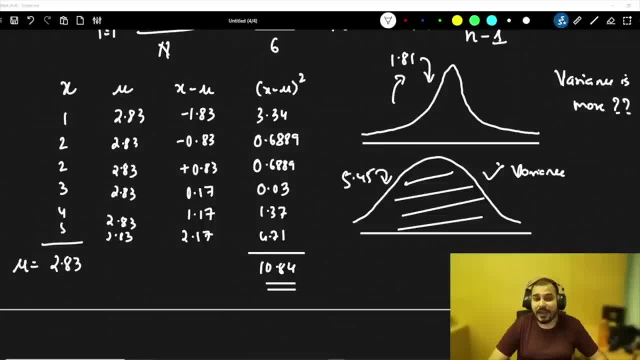 to solve that particular example and then we can definitely understand it. But Let's say you have some idea, you basically got, because obviously the variance needs to be spreaded high. if the variance is high, right, the dispersion becomes high because you have more number of values inside it. 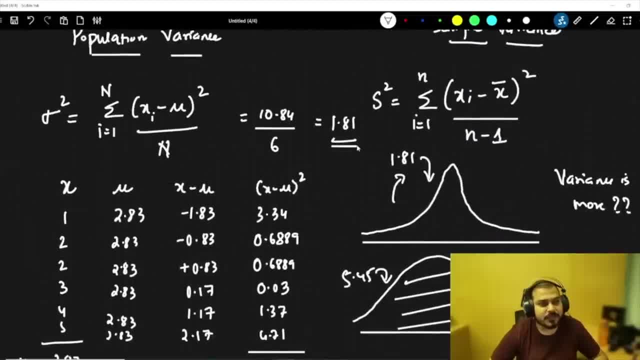 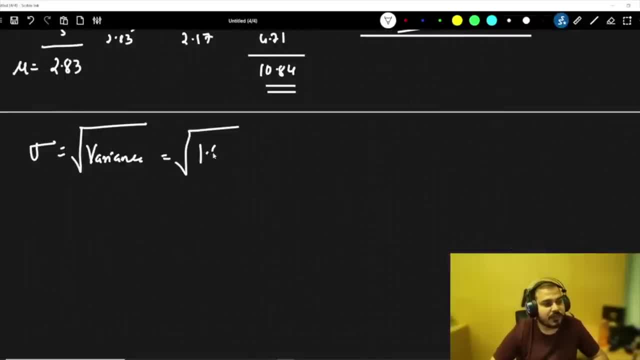 Now let's go ahead and let's try to see. now I got my variance as 1.81.. Now my standard deviation is nothing but root of variance. root of variance, that basically means it is nothing but root of 1.81.. So if I go and open my calculator, I'll just say root of 1.81.. 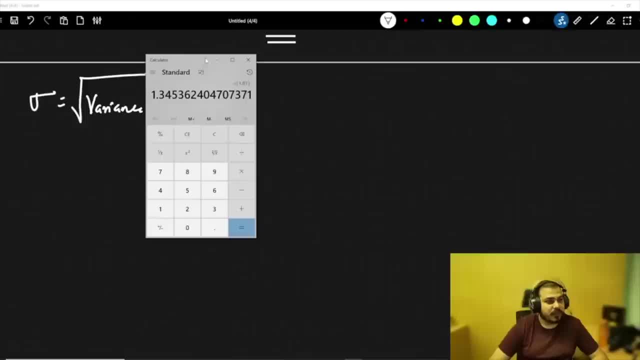 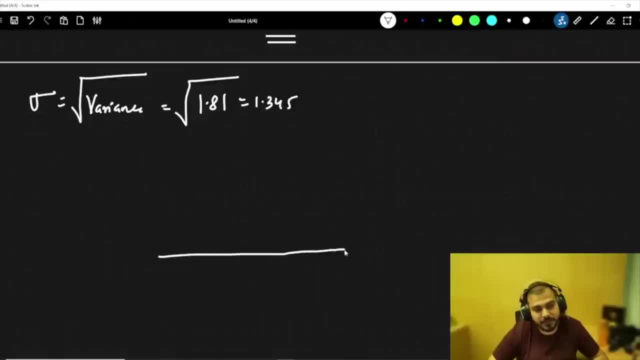 Okay, And there I'm actually getting is nothing but 1.345.. So 1.345.. Now see what does standard deviation basically mean? What is the mean in this particular case? What is the mean? Mean is nothing but 2.83, right. 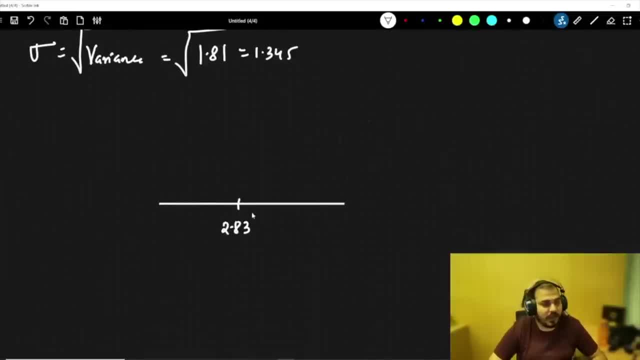 Let's consider this one. The mean is 2.83.. Now, from this mean your data will be distributed, because mean is basically specifying your measure of central tendency, basically says that where the center is there, Therefore that specific distribution. So from here, if I go one step right, one standard deviation to the right, 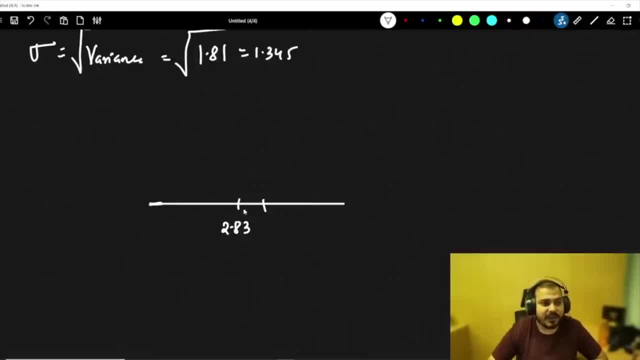 You have seen standard deviation formula. The next element that may probably fall between the one standard deviation will range between: Let's consider that this is my first standard deviation to the right. Then it will basically have 2.83 plus 3.4.. 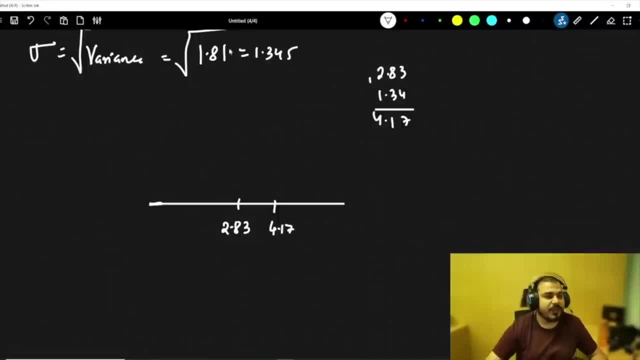 So this is nothing but 4.17.. That being said, Okay, That basically means in this distribution, whatever elements are basically present between 2.83 to 4.17 will be falling within the first standard deviation. And if I consider the same thing towards the left, 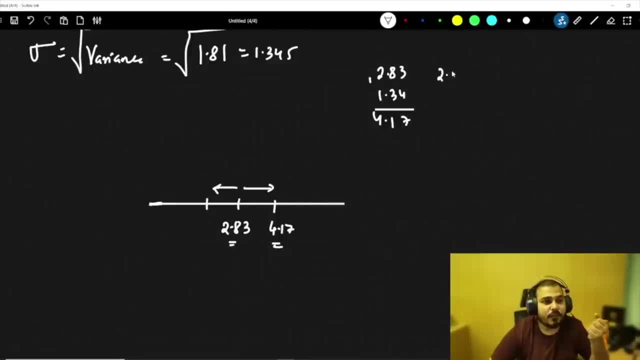 That, basically, is one standard deviation towards the left. Then what I'll do? I'll just subtract 1.34.. So this will basically be 9741.. So it will basically become 1.49.. Now here it basically says that Any elements that falls between 1.49 to 2.83 will be falling in this region. 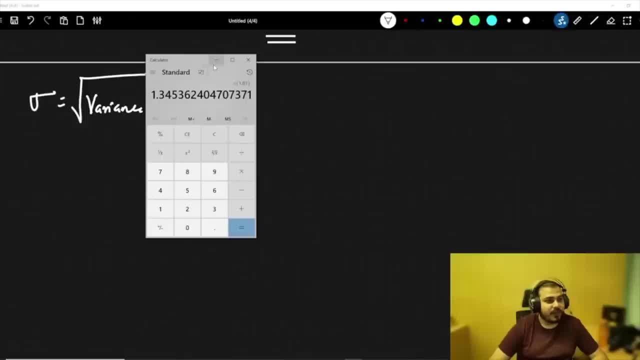 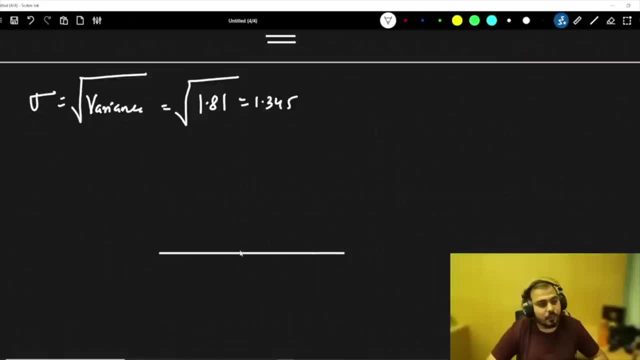 and there i'm actually getting is nothing but 1.345. so 1.345 now see what does standard deviation basically mean? what is the mean in this particular case? what is this mean? mean is nothing but 2.83. right, let's consider this one. the mean is 2.83. now, from this mean, your data will be: 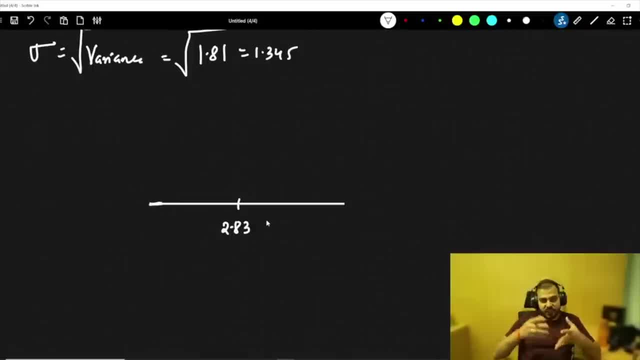 distributed, because mean is basically specifying your measure of central tendency basically says there for that specific distribution. so from here, if i go one step right, one standard deviation to the right, you have seen standard deviation formula. the next element that may probably fall between the one standard deviation will range between: let's consider that this is my first. 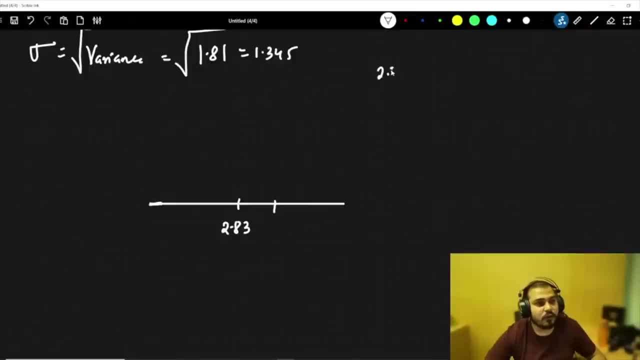 standard deviation to the right, then it will basically have 2.83 plus 3.4. so this is nothing but 4.17. that basically means in this distribution, whatever elements are basically present between 2.83 to 4.17 will be falling within the first standard deviation. and if i consider the same thing towards the left, 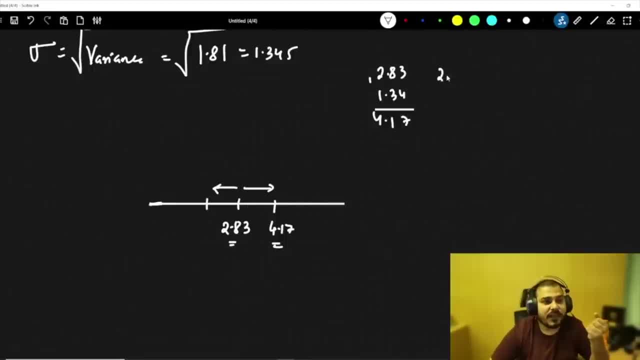 that basically, is one standard deviation towards the left. then what i will do? i'll just subtract 1.34, so this will basically be 9741, so it will basically become 1.49. now here it basically says that any elements that falls between 1.49 to 2.83 will be falling in this region. that is one standard deviation to the. 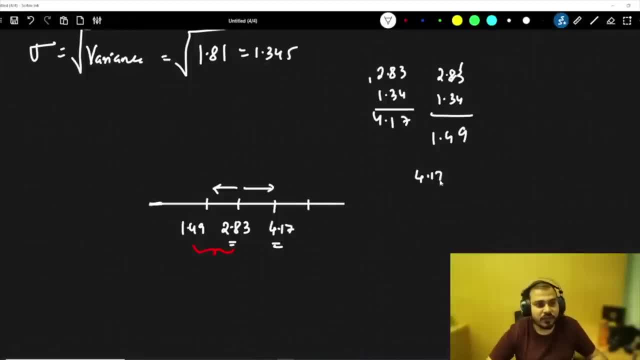 left. similarly, we'll go with the second standard deviation now. in this particular case, it will be 4.17, 1.34, 5, 5, 5.51, similarly. you go and calculate similarly. you go and calculate similarly. now, your standard deviation is a very small number. still, i'll say that this is a small number. 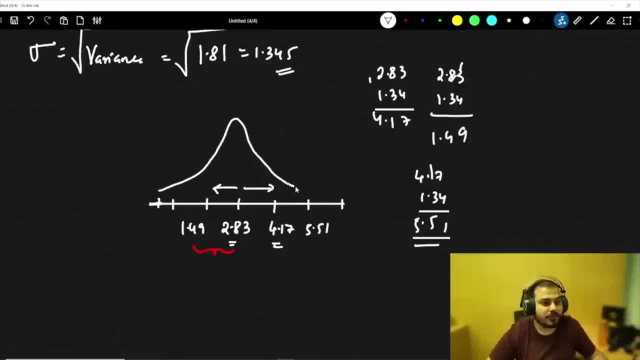 and if i probably try to construct a graph, it will look something like this: the tip right, this, this region that you probably will see. this is basically called as a bell curve and, based on the standard deviation and variance, you'll be able to decide two important things with 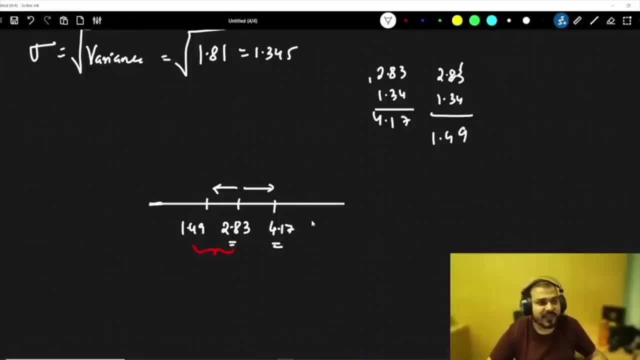 That is one standard deviation to the left. Similarly, we'll go with the second standard deviation Now. in this particular case, it will be 4.17,, 1.34,, 5,, 5, 5.51.. Similarly, you go and calculate. 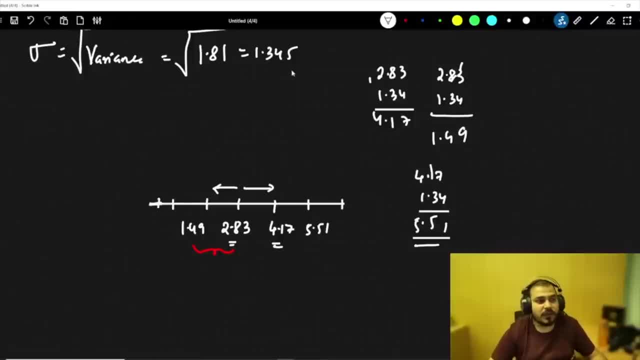 Similarly you go and calculate. Similarly you go and calculate: Now, your standard deviation is a very small number. Still, I'll say that this is a small number And if I probably try to construct A graph, it will look something like this: The tip. 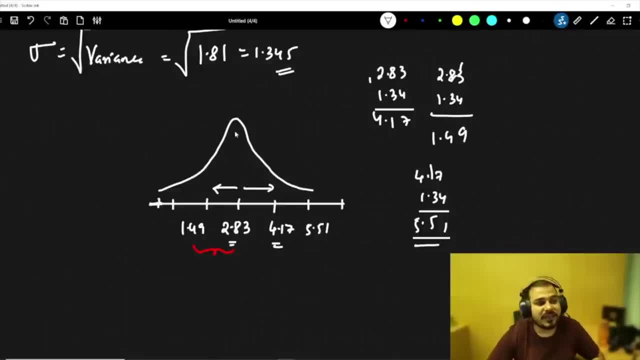 Right, This region that you probably will see. This is basically called as a bell curve And, based on this standard deviation and variance, you'll be able to decide two important things With the help of variance, definitely, you'll be able to understand how the data is spread. 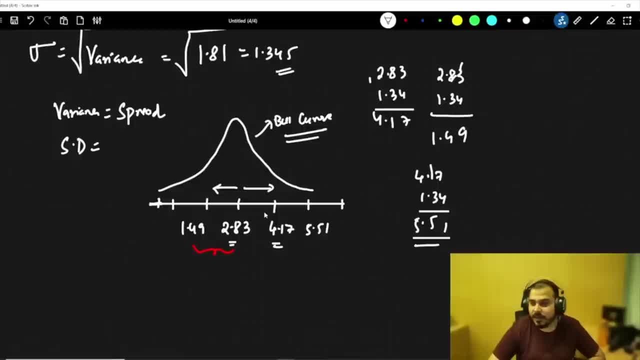 And with standard deviation you'll be able to understand that between one standard deviation to the right and the left, what may be the range of data that may be falling? So standard deviation is nothing, But it is the root, square root of variance. That basically means from the mean right, how far an element can be. 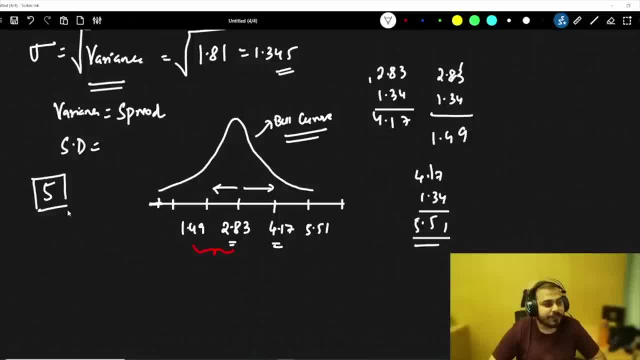 Let's consider that if I consider 5.. Now for 5. if you try to calculate it may fall somewhere here. So how you're going to represent 5.? You will say that it falls in 1.5 standard deviation from the mean. 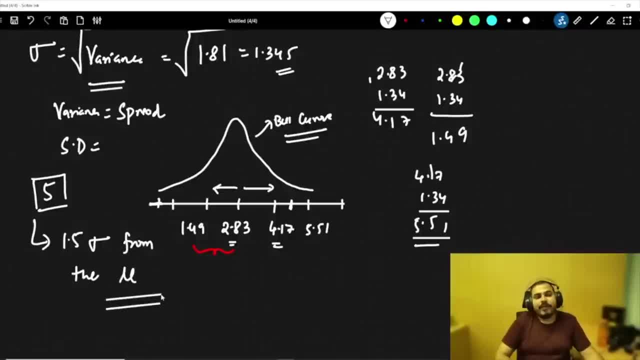 So this kind of definition you will be able to tell them. So that basically means from the mean how far a specific number falls. So that basically means from the mean how far a specific number falls. So that basically means from the mean how far a specific number falls. 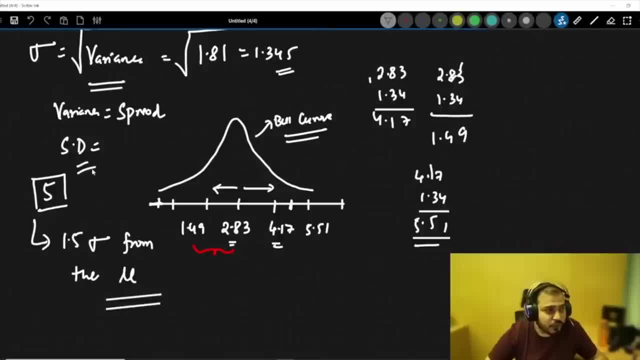 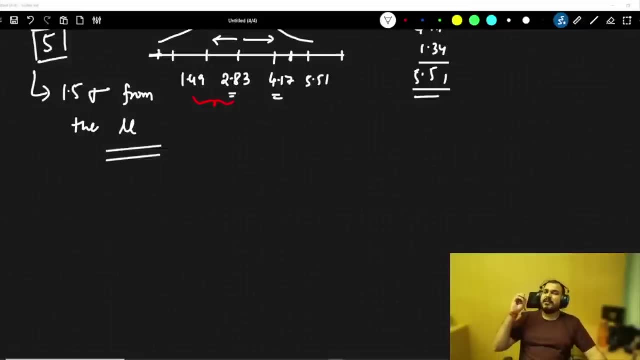 A specific number is with respect to standard deviation. You're calculating, you are using a unit called as standard deviation for saying that. And variance, specifically talk about spread. If the variance is high, the data spread that is there is very, very high. Now let's understand some amazing basic things, which is called as percentile and quartiles. 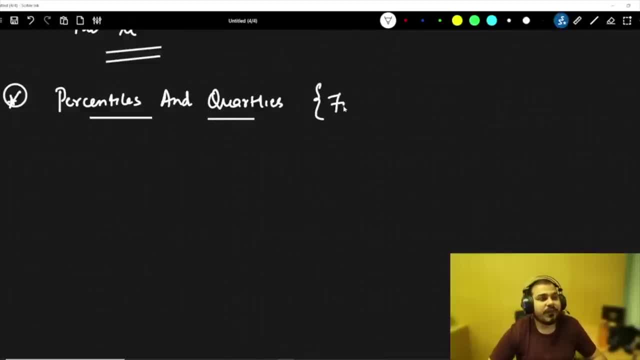 This is the first step: to find outliers. How do we find outliers, an outlier? So probably we are going to discuss in this the first and with the help of code also, you can basically do. Now, with respect to percentiles, let's try to understand what is. 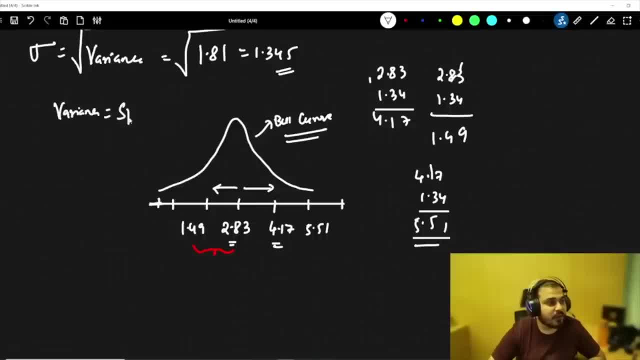 the help of variants, definitely, you'll be able to understand how the data is spread and with standard deviation, you'll be able to understand that, between one standard deviation to the right and the left, what may be the range of data that may be falling? so standard deviation is nothing. 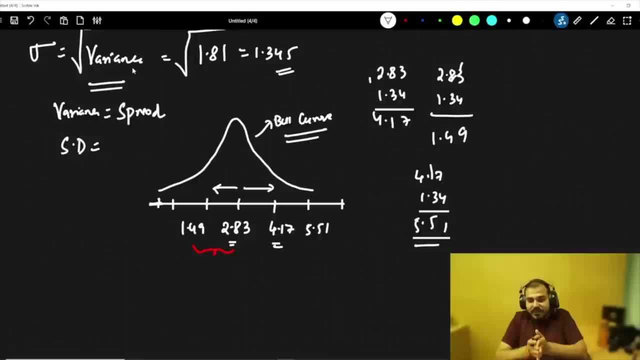 but it is a root, square root of variance. that basically means from the mean right how far a element can be. let's consider that if i consider 5 now for 5, if you try to calculate it may fall somewhere here. so how you are going to represent 5, you will say that it falls in 1.5 standard deviation from the mean. 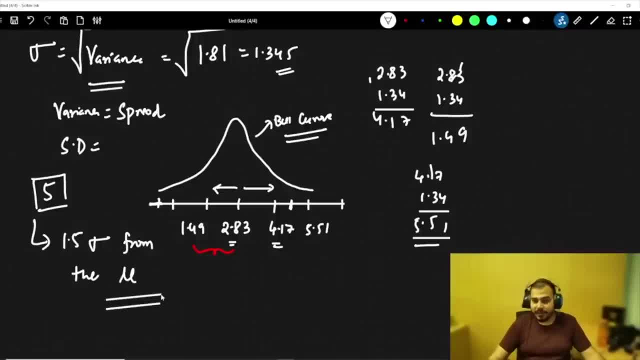 so this kind of definition you will be able to tell them. so that basically means from the mean, how far a specific number is with respect to standard deviation you're calculating, you're using a unit called as standard deviation for saying that. and variance, specifically talk about spread. if the variance is high, the values, the data spread that is there is very, very high now. 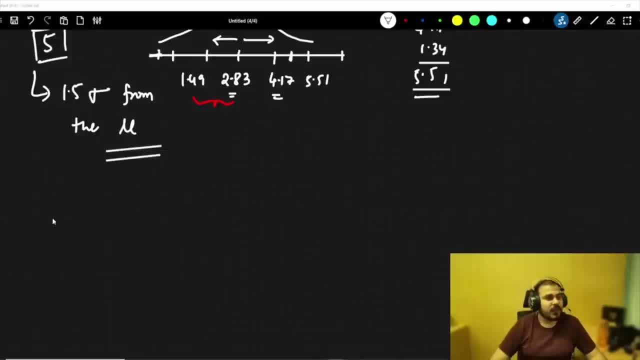 let's understand some amazing basic things, which is called as percentile and quartiles. this is the first step to find outliers. how do we find an outlier? so probably we are going to discuss in this the first, and with the help of code also, you can basically do now with respect to percentiles, let's try to understand what is. 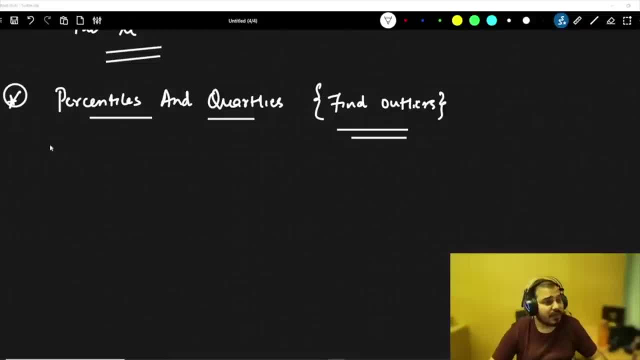 percentile and how do you find out percentile? now, before understanding percentile, you basically need to understand about percentage. suppose, if i have a distribution, i say 1, 2, 3, 4, 5. now i my question is that what is the percentage of numbers that are odd? 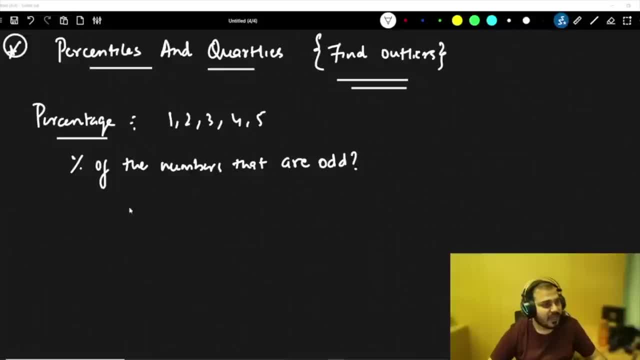 so how do you basically apply a formula over here so i can basically say: percentage is equal to number of numbers that are odd divided by total numbers. so if i really try to calculate how many numbers are odd- 1, 2, 3- so 3 divided by 5 is nothing but how much 0.6, which is nothing but 60 percentage. 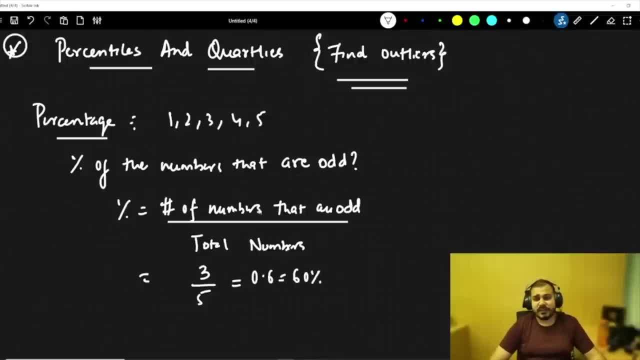 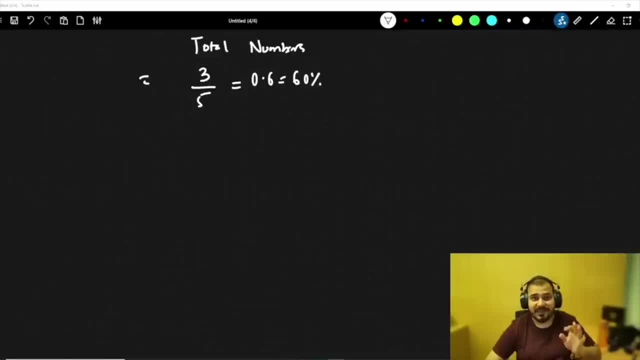 very simple. this is how we basically calculate percentage now, and i hope everybody knows this. now let's understand a very, very important topic, which is the percentage of numbers that are odd, which is called as percentile. now, i probably think you have heard about percentiles in lot of things. 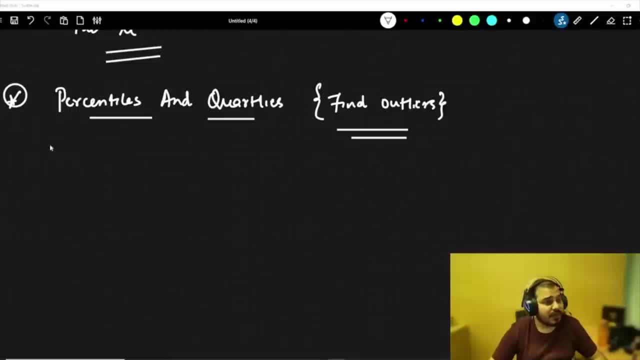 percentiles and how do you find out percentiles? Now, before understanding percentile, you basically need to understand about percentage. Suppose, if I have a distribution, I say 1, 2, 3, 4, 5.. Now my question is that what is the percentage of numbers that are odd? So how do you basically? 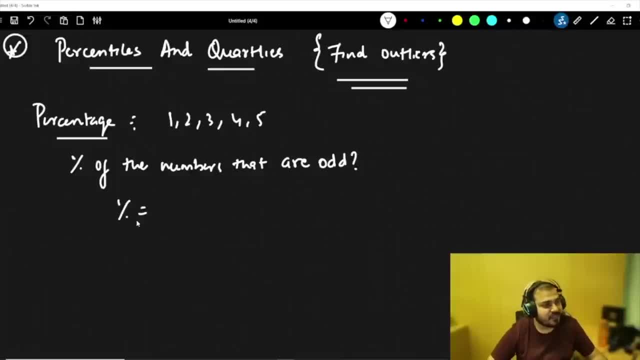 apply a formula over here. So I can basically say: percentage is equal to number of numbers that are odd divided by total numbers. So if I really try to calculate how many numbers are odd- 1, 2, 3.. So 3 divided by 5 is nothing but how much 0.6, which is nothing but 60 percentage. 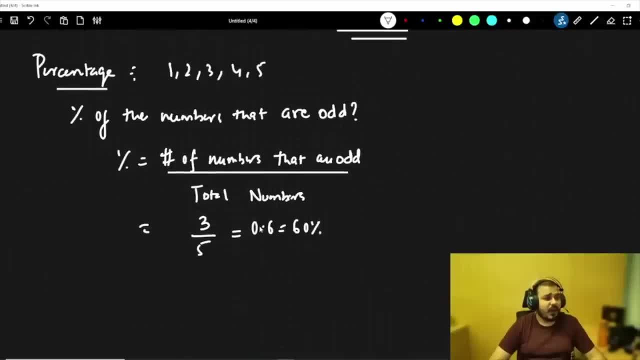 Very simple. this is how we basically calculate percentage. Now let's see how we can calculate percentage. So, if I have a distribution of 0.6, which is now- and I hope everybody knows this- Now let's understand a very, very important topic, which is 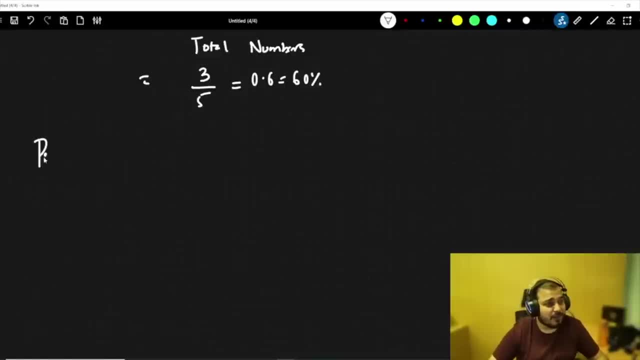 called as percentile. Now I probably think you have heard about percentiles in lot of things, Percentile probably. if you have given GATE exam, CAT exam, GMAT exam, SAT exam, One real example, I will show it to you. that is related to my YouTube ranking also. You can see my YouTube ranking social. 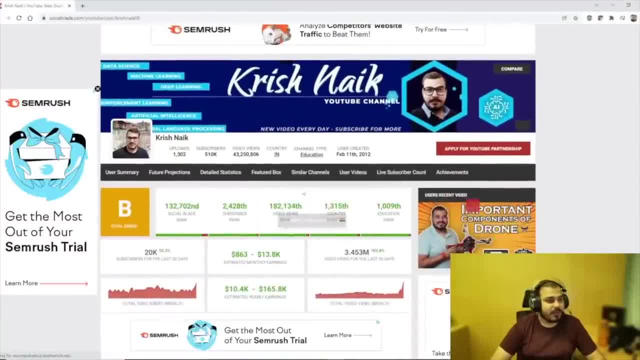 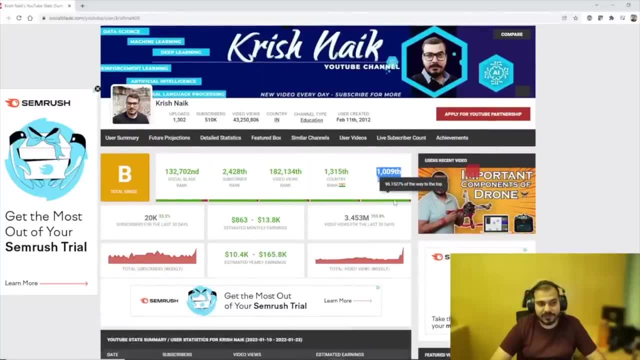 blade. So here, if I show you one example here, you can see that you can see education rank Here. if you hover over here it shows 96.1527 percentile. If I hover over here, it shows 94.98 percentile. Over here, if I hover, it shows 94.958 percentile. So we'll try to discuss about this percentile. 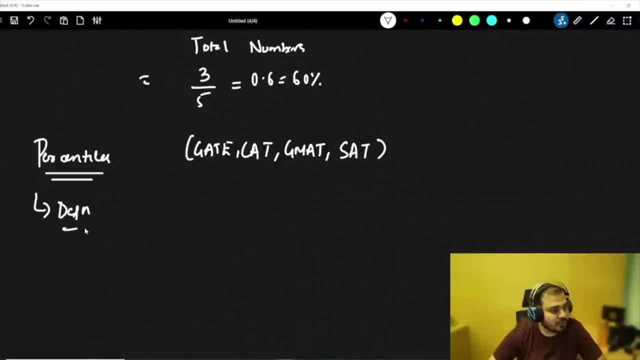 right now. First of all, we will give the definition. What is a percentile? So percentile is a value Below which a certain percentage of observations lie. So this is the definition of percentile. It is basically saying it is a value. If I say, okay, this number is the 25 percentile, This basically. 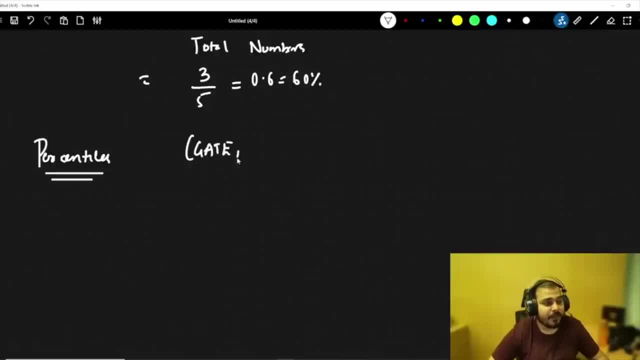 percentile, probably if you have given gate exam, cat exam, gmat exam, sat exam. okay, one real life example i'll show it to you. that is related to my, my youtube ranking also, if you can see my youtube ranking, social blade. so here, if i show you one example, here you can see that you can see education. 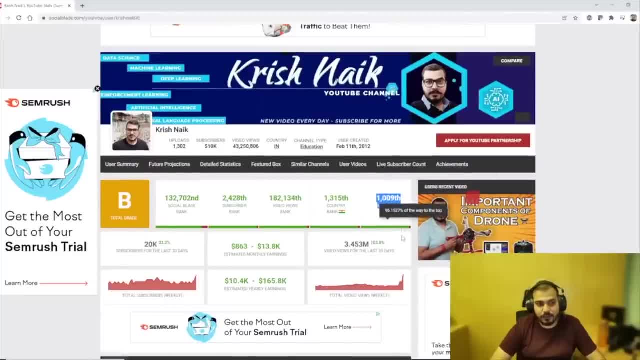 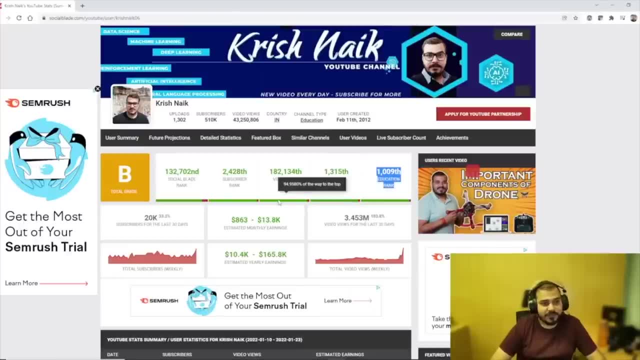 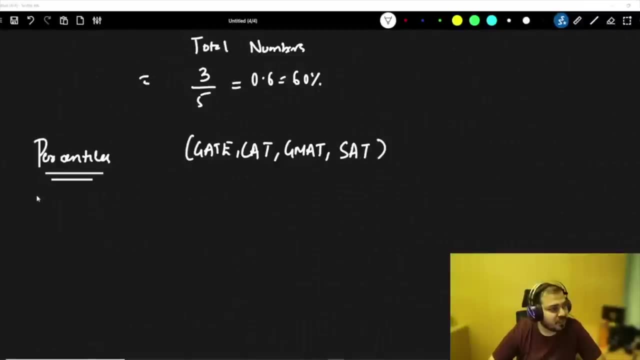 rank here. if you hover over here, it shows 96.1527 percentile. if i hover over here, it shows 94.98 percentile. over here, if it's. if i hover, it shows 94.958 percentile. so we'll try to discuss about this percentile right now. first of all, we will give the definition: what is a percentile? so 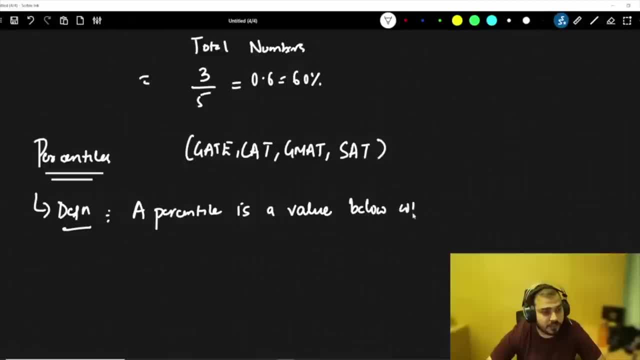 percentile is a value below which a certain percentage of observations lie. so this is the definition of percentile. it it is basically saying it is a value. if i say, okay, this number is the 25 percentile, this basically says that 25 percentage of the entire distribution is less than that particular value. so percentile is a value below which a certain 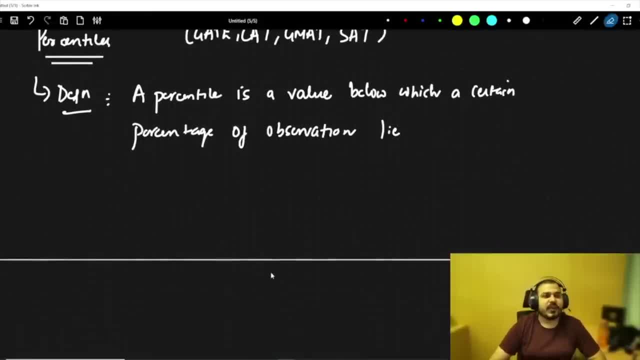 percentage of observation lie. let me take a very good example and show it to you. suppose i have a data set and inside this data set i have elements like two comma two, three, comma four, comma five, comma five, six comma, seven, comma, eight, comma eight, one more eight. one, two, three, four. 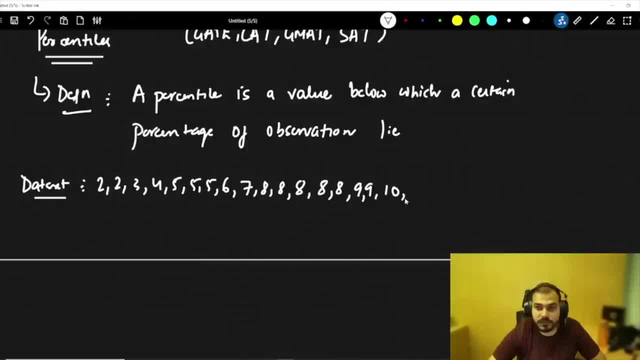 five, nine, nine, ten, eleven, eleven, twelve. so let's consider that, this many number of elements that i actually have. now, in this specific number of elements, i want to find out what is the percentile. let's consider this one. my question is: what is the percentile ranking of 10? so this is my question. we solve this problem by using a simple 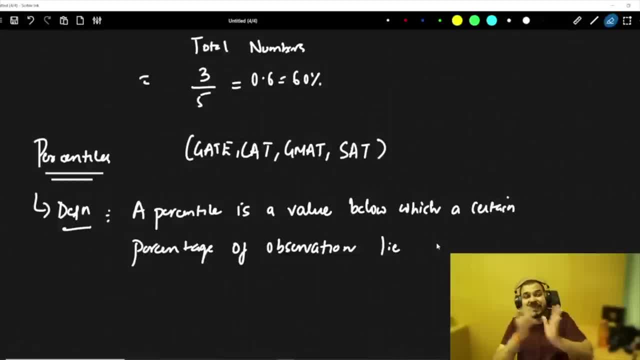 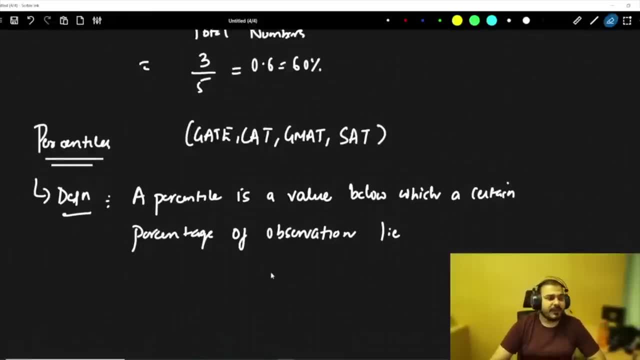 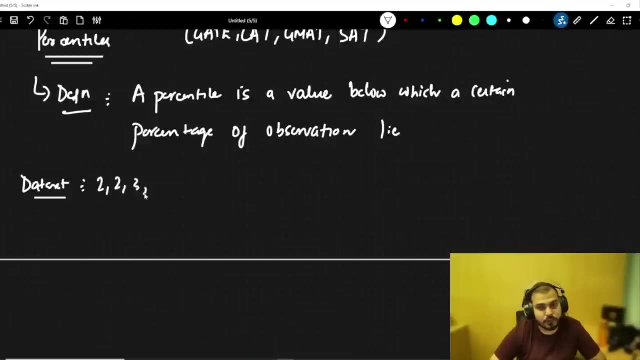 says that 25 percentage of the entire distribution is less than that particular value. So percentile is a value below which a certain percentage of observation lie. Let me take a very good example and show it to you. Suppose I have a data set and inside this data set I have elements like 2, 2,, 3,, 4,, 5,, 5,, 6,, 7,, 8,, 8,, 1 more 8, 1,, 2,, 3,, 4,, 5,, 9,, 9,, 10,, 11,, 11, 12.. 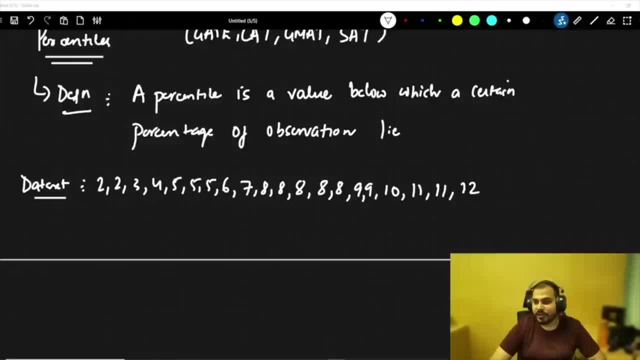 So let's consider that, this many number of elements that I actually have. Now, in this specific number of elements, I want to find out what is the percentile. Let's consider this one. My question is: what is the percentile ranking of 10.. So this is my question. We solve this problem by using a simple formula. I want to. 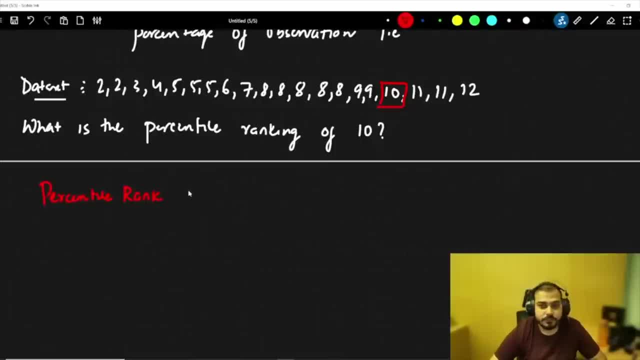 find out the percentile rank of 10, right? So my formula, let's consider this: x is equal to 10.. Okay, so here I am specifically going to write x. So this will basically be number of values below x divided by small n, which is my sample, multiplied by 100. 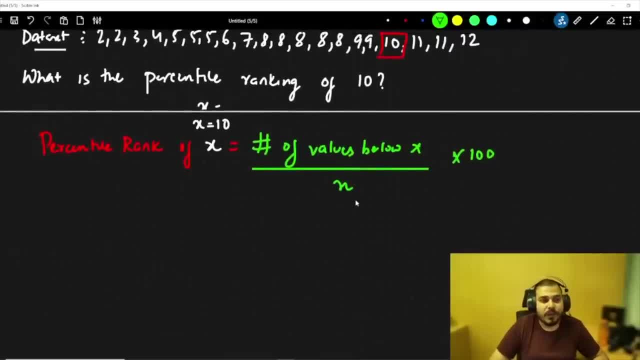 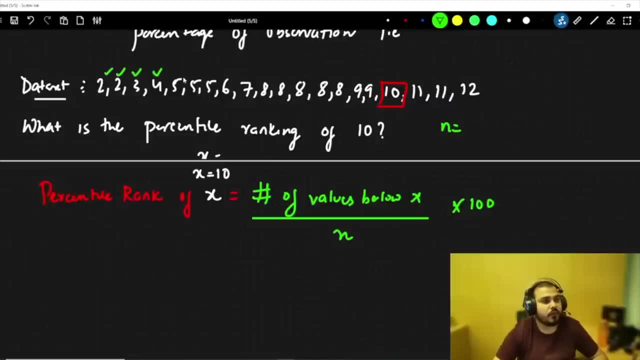 So if you try to calculate this number of values below x divided by n, What is n over here? n size is sample size: 1, 2, 1, 2,, 3,, 4,, 5,, 6,, 7,, 8,, 9,, 10,, 11,, 12,, 13,, 14,, 15,, 16,, 17,, 18,, 19,, 20.. 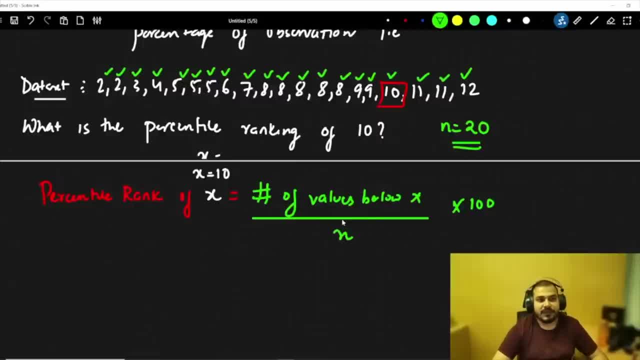 So 20 is basically my sample size. So here I am going to say number of values below x. So how many number of values X is 10.. How many number of values are below x? 1,, 2,, 3,, 4,, 5,, 6,, 7,, 8,, 9,, 10,, 11,, 12,, 13,, 14,, 15,, 16.. 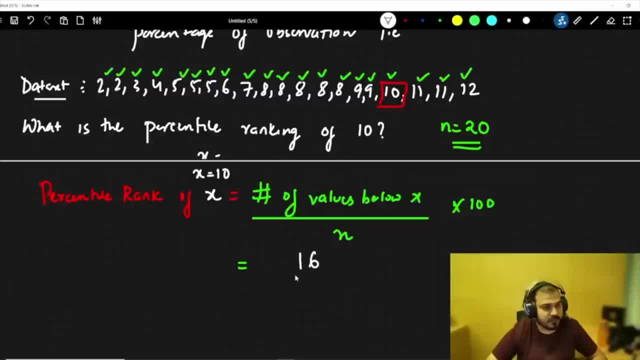 So this will basically become 16.. 16 divided by 20, multiplied by 100.. In short, this will become four. fours are 16,, 4,5,, 17,, 18.. So this will basically become 16.. 16 divided by 20, multiplied by 100.. In short, this will become 4. fours are 16,, 5, 6.. 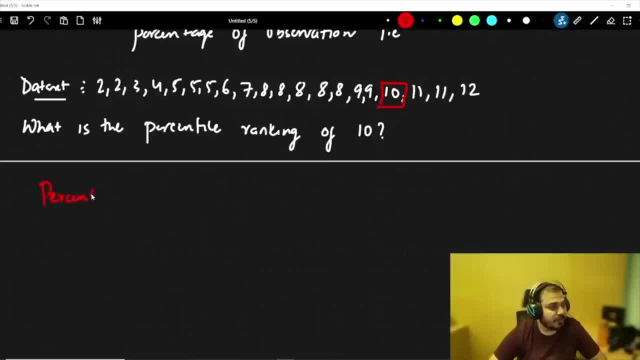 formula. i want to find out the percentile rank of 10, right? so my formula, let's consider this: x is equal to 10, okay, so here i'm specifically going to write x. so my formula will basically be number of x divided by small n, which is my sample, multiplied by 100. so if you try to calculate this number of 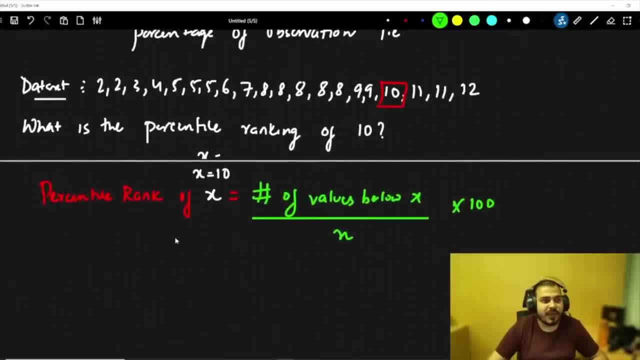 values below x divided by n, what is n over here? n size is sample size: 1, 2, 1, 2, 3, 4, 5, 6, 7, 8, 9, 10, 11, 12, 13, 14, 15, 16, 17, 18, 19, 20.. so 20 is basically my sample size. so here i'm going to say: 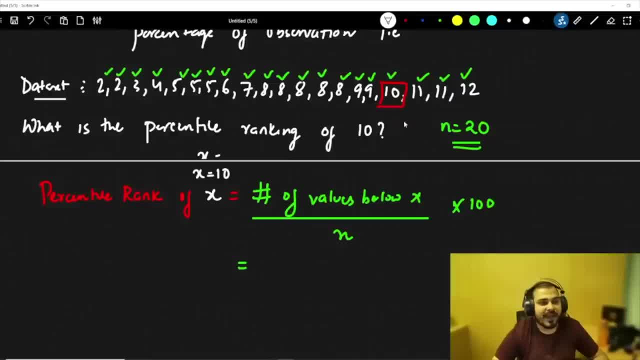 number of values below x. so how many number of values x is 10? how many number of values are below x? 1, 2, 3, 4, 5, 6, 7, 8, 9, 10, 11, 12, 13, 14, 15, 16. so this will basically become 16, 16 divided by 20. 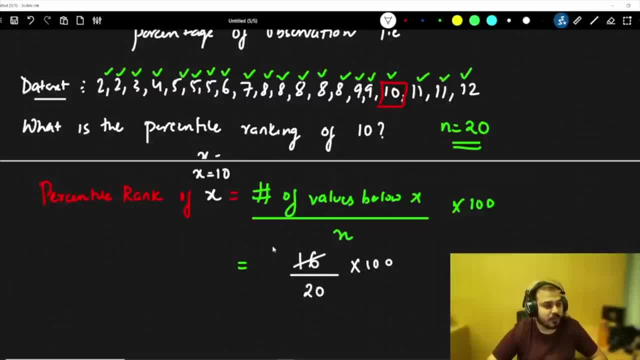 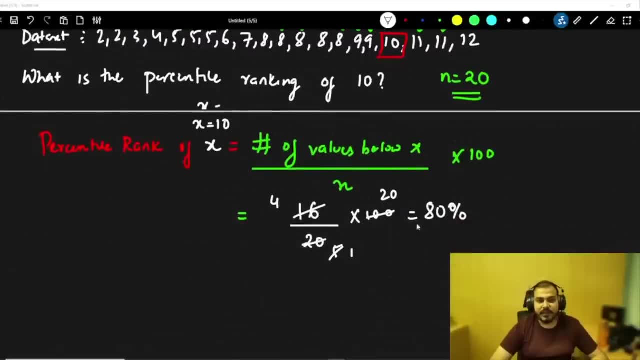 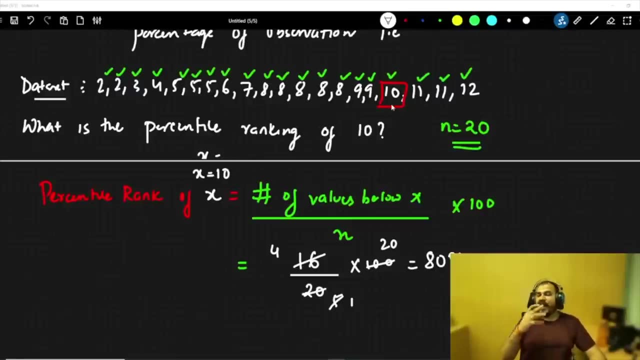 multiplied by 100. in short, this will become 4. 4s are 16, 4 5s are 1s are 20s are so 80 percentile is my answer for this. that basically means, if i really want to find out what this 10 value. 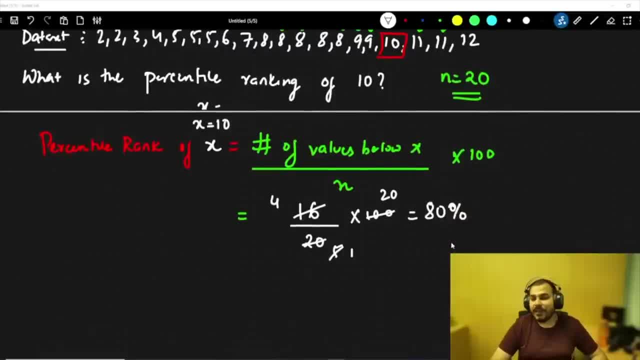 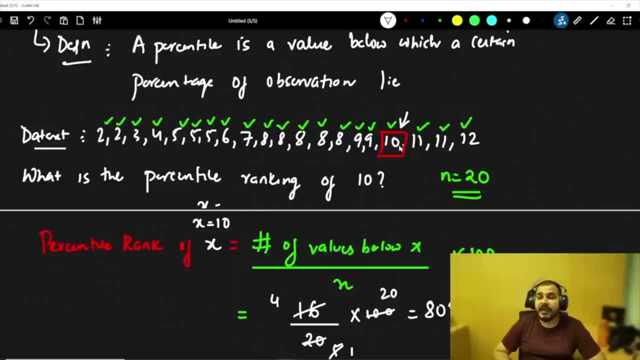 percentile is. it is 80. now understand what is the main meaning out of it. the main meaning is that 80 percentage- please listen to me very, very carefully- 80 percentage of the entire distribution is less than 10. this is the real meaning that you can probably understand from it now quickly. 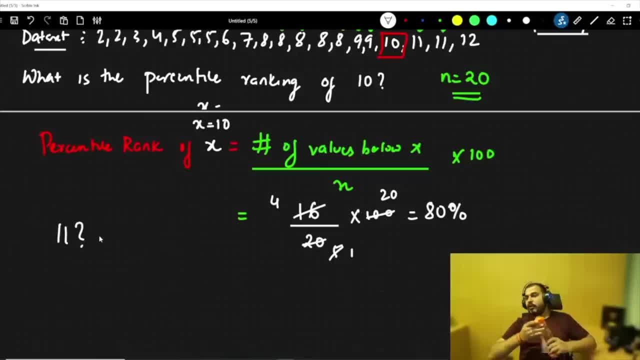 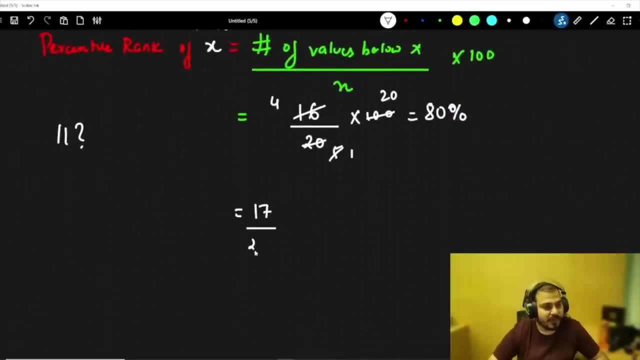 what is the percentile ranking of 11, of value 11? so, uh, how many elements are present below 11? i'll say 17 divided by 20, multiplied by 100, 1s are 5s are 85 percent. let's do the reverse of this. so, from this particular distribution, what? 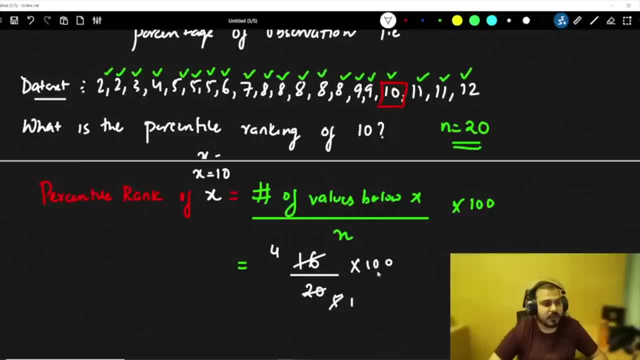 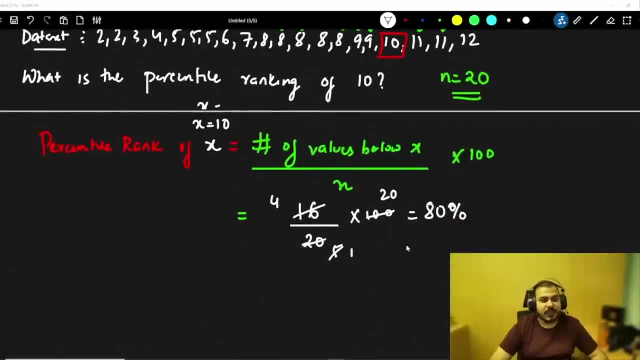 In short, this will become 4. fours are 4, five and 5 small ns yangs zha, 1 zha, 20 zha. So 80 percentile will basically be my answer for this. That basically means, if I 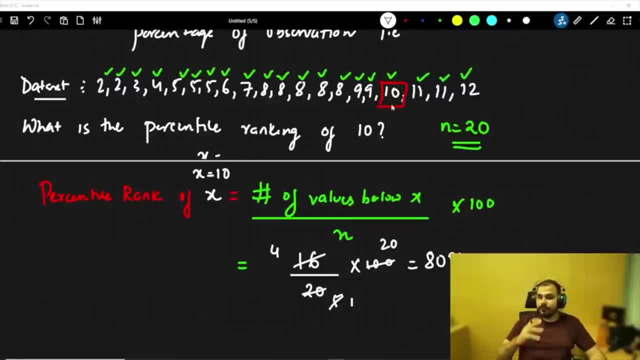 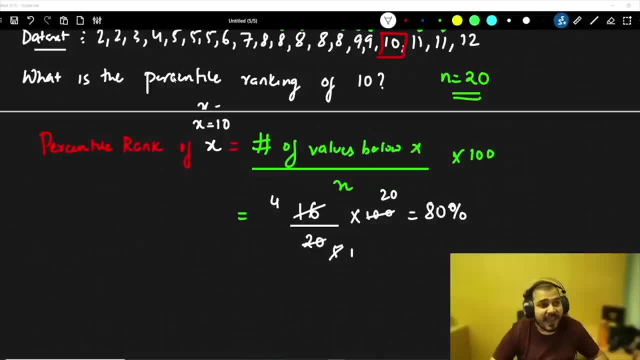 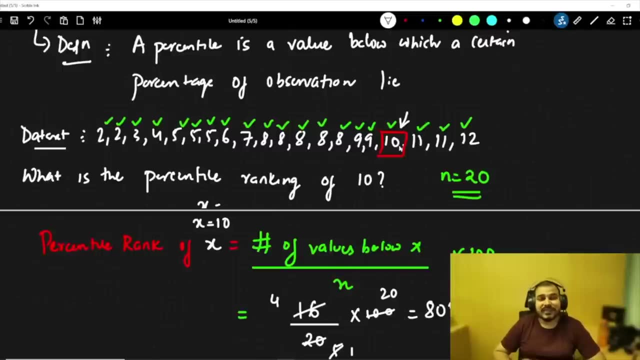 really want to find out what this 10 value percentile is. it is 80.. Now understand what is the main meaning out of it. The main meaning is that 80 percentage- please listen to me very, very carefully- 80 percentage of the entire distribution is less than 10.. This is the real meaning that you 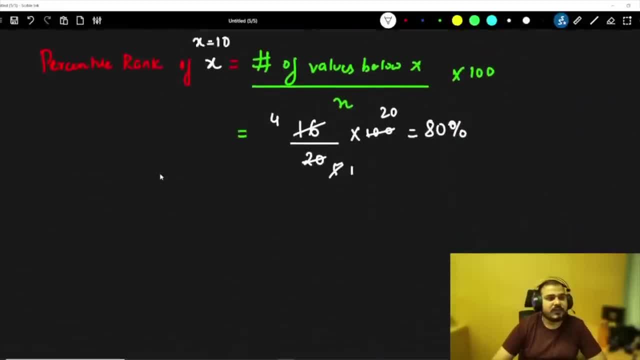 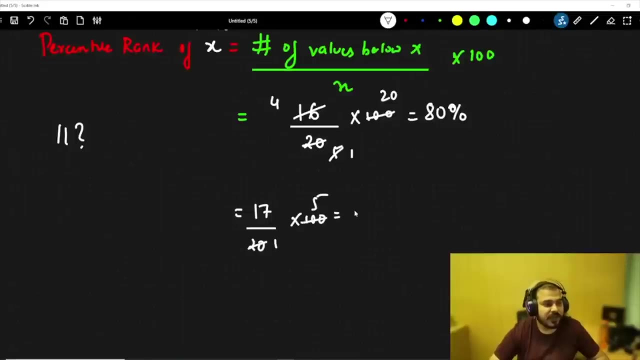 can probably understand from it Now quickly, what is the percentile ranking of 11, of value 11.. So how many elements are present below 11?? I'll say 17 divided by 20, multiplied by 100.. 1 zha, 5 zha. 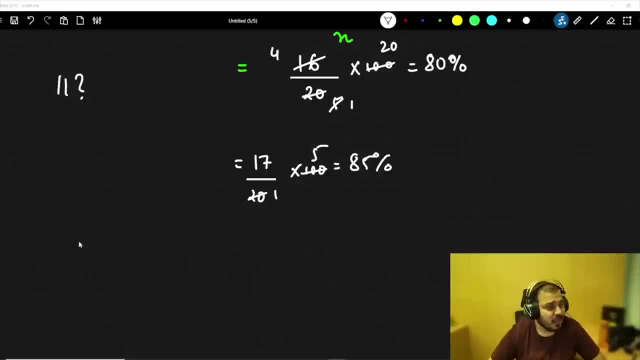 85 percentile. Let's do the reverse of this. So from this particular distribution, what value exists at percentile ranking of 25 percentile? So how do you calculate this? For this you use a very simple formula And the formula is something like this: Value is equal to percentile divided by 100, multiplied by n plus 1.. 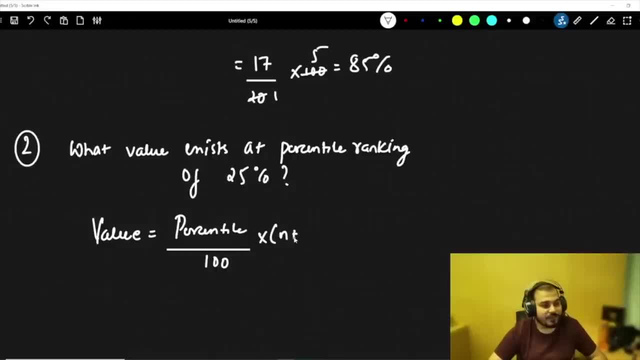 Now see, guys, I'm not going to derive the formula why it is n plus 1, why it is n minus 1, why it is this For sample variance. I'll discuss about why n minus 1.. But understand, we really need to. 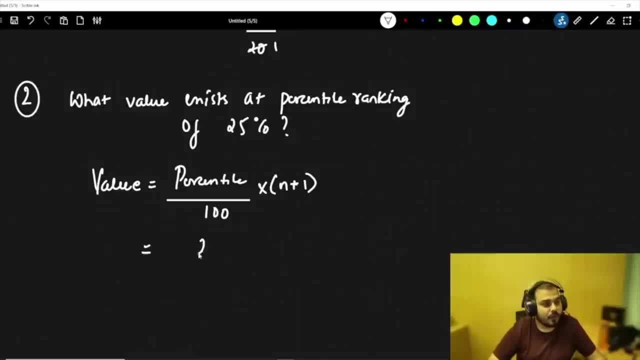 understand how we are using it in some specific purpose. So percentile over here is 25 by 100 multiplied by 21.. Now understand this. this 5.25 is the index position. It is very much important to understand. This is not the value, the index position. Now I will go and find out which is 5.25.. 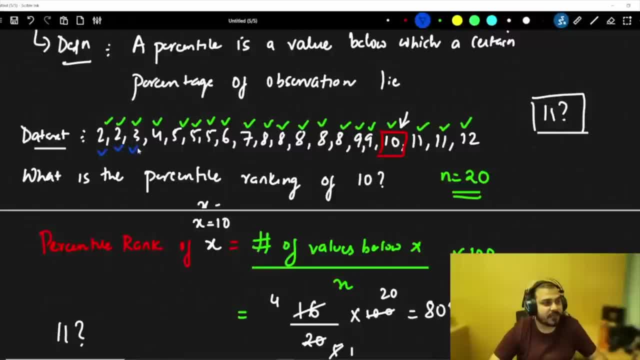 So this is my first element: first index, second index, third index, fourth index, fifth index and 5.25.. 5 will be in between this, But right now I don't see any element between this, So what we do is that. 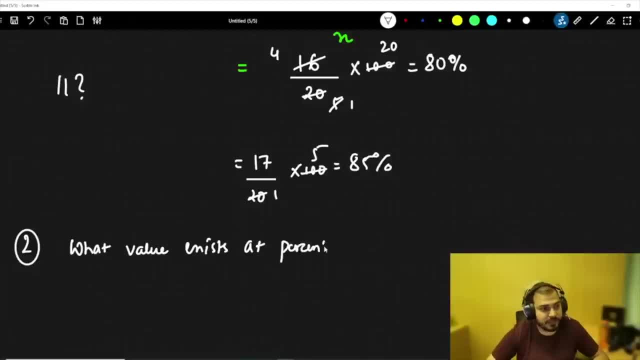 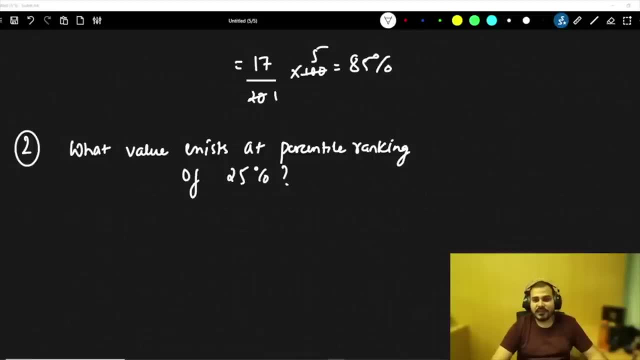 value exists at percentile ranking of 25 percent. so how do you calculate this? for this you use a very simple formula and the formula is something like this value is equal to percentile divided by 100, multiplied by n plus 1. now see, guys, i'm not going to derive the formula why it is n plus 1, why it is n minus 1, why 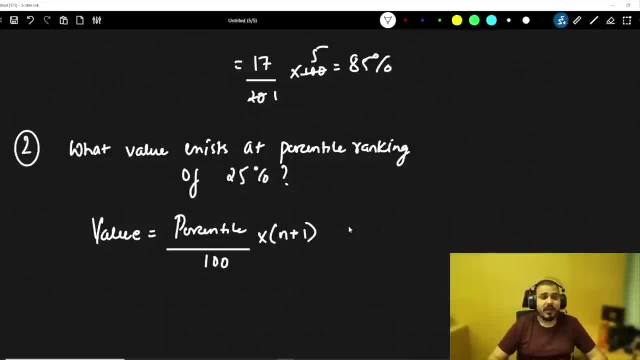 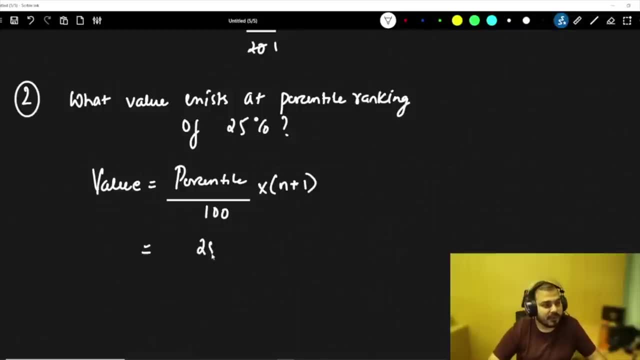 it is this for sample variance. i'll discuss about why n minus 1, but understand- we really need to understand- what things we are doing and how we are using it in some specific purpose. so percentile over here is 25 by 100 multiplied by 100 and the formula is something like: this value is equal to. 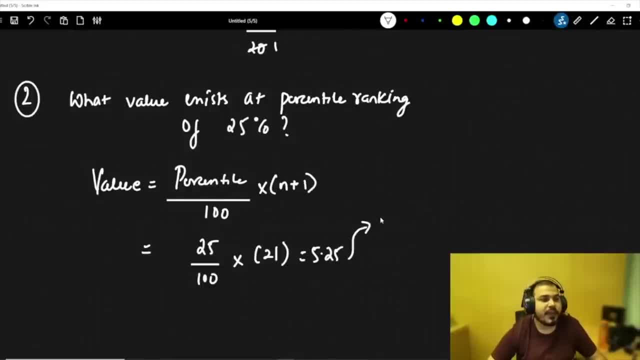 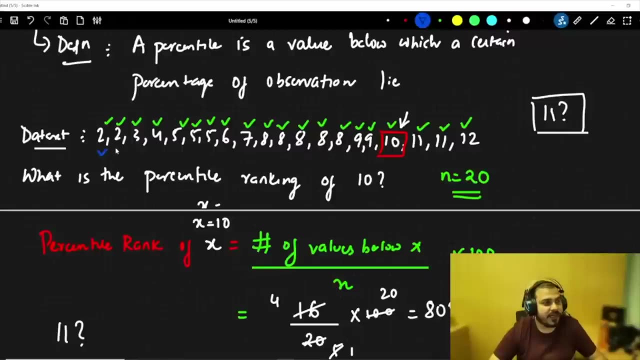 5.25 multiplied by 21.. now understand this. this 5.25 is the index position. it is very much important to understand. this is not the value, the index position. now i will go and find out which is 5.25. so this is my first element. first index. second index, third index, fourth index, fifth index. 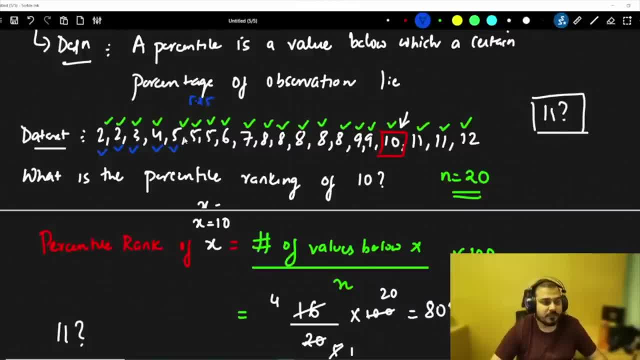 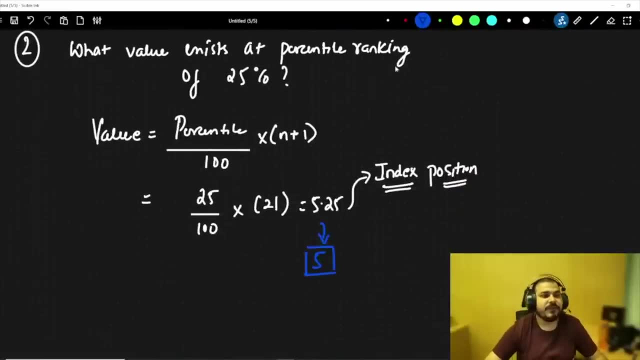 and 5.25 will be in between this, but right now i don't see any element fine between this. So what we do is that we take 5th and 6th index and then we do the average and we calculate the value. In this particular case, my answer will be 5.. So 5 is the value for 25 percentile. 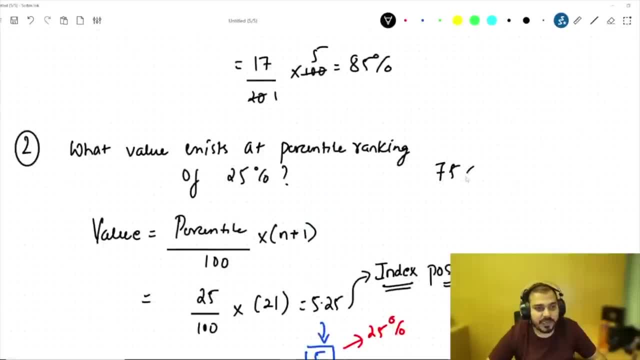 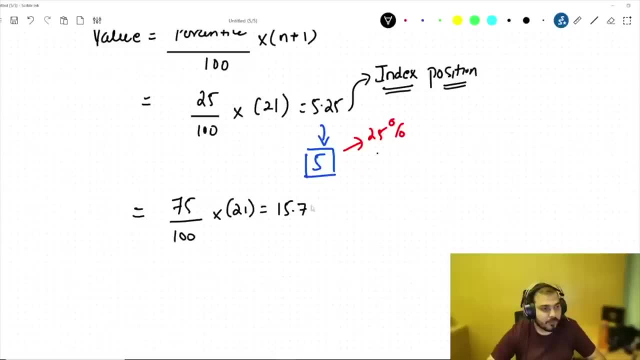 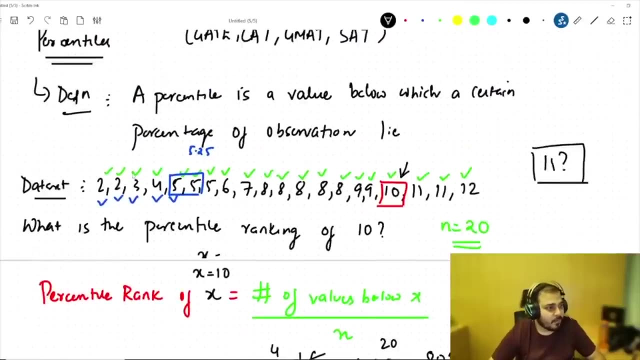 Try to find out what is 75 percentile. So if I use 75 divided by 100, multiplied by 21,, 15.75 is the index position. Now go and count which is 15.75 from the top: 1,, 2,, 3,, 4,, 5,, 6,, 7,, 8,, 9,, 10,, 11,, 12,, 13,, 14,, 15.. 15.75 is the sum of these two numbers. 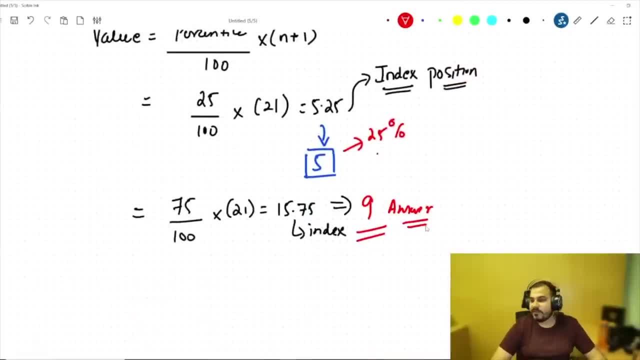 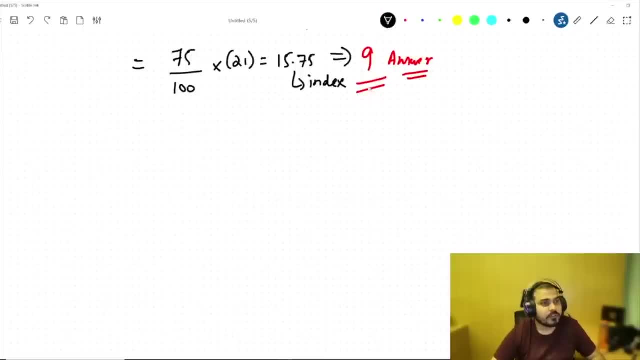 So my answer is 9.. 15.75 is the index position. So here I am basically getting the 9 answer. Now let's go and discuss about a new topic which is called as 5 number summary. In 5 number summary we need to discuss about something called as: 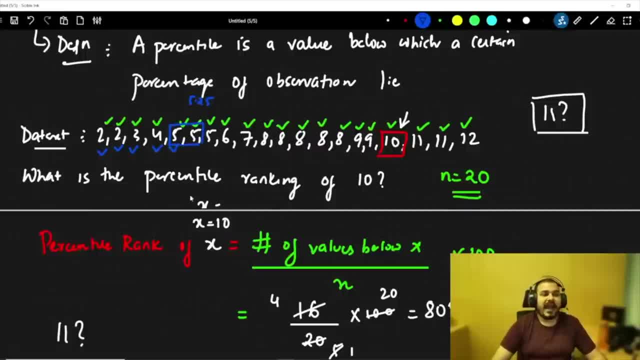 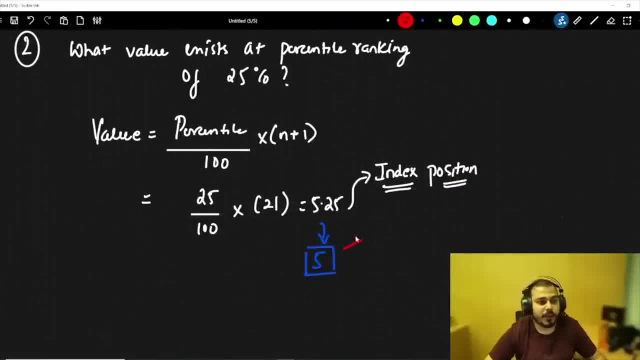 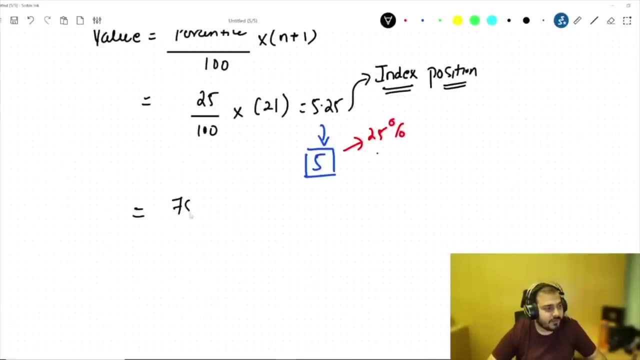 we take fifth and sixth index and then we do the average and we calculate the value. In this particular case, my answer will be 5.. So 5 is the value for 25 percentile. Try to find out what is 75 percentile. So if I use 75 divided by 100, multiplied by 21,, 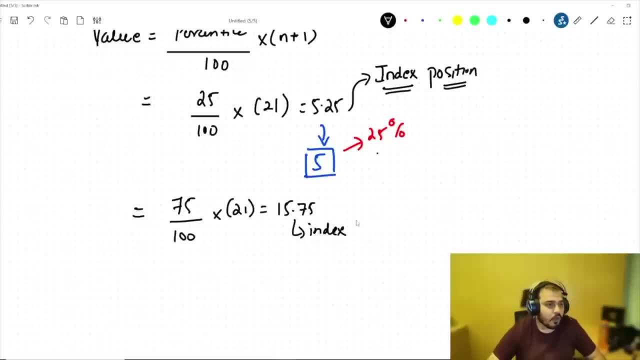 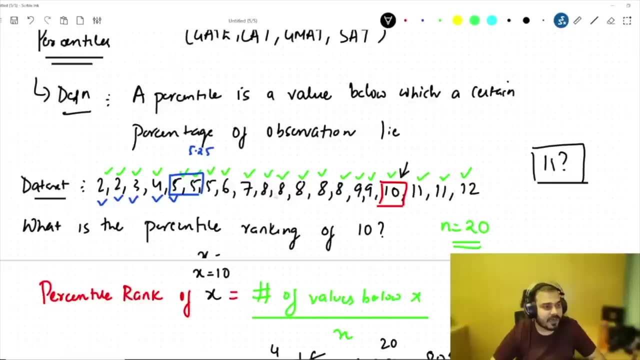 I will get 15.75.. So 15.75 is the index position. Now go and count which is 15.75 from the top 1, 2, 3, 4, 5, 6, 7,, 8,, 9,, 10,, 11,, 12,, 13,, 14, 15.. 15.75 is the sum of these two numbers. 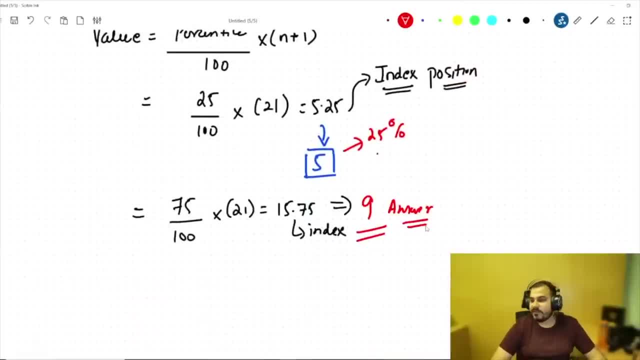 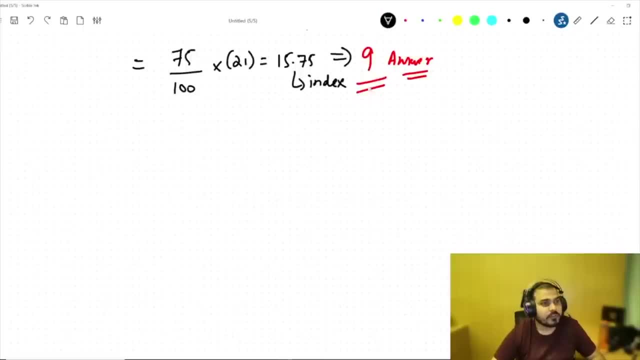 So my answer is 9.. 15.75 is the index position. So here I'm basically getting the 9 answer. Now let's go and discuss about a new topic which is called as 5 number summary In 5 number. 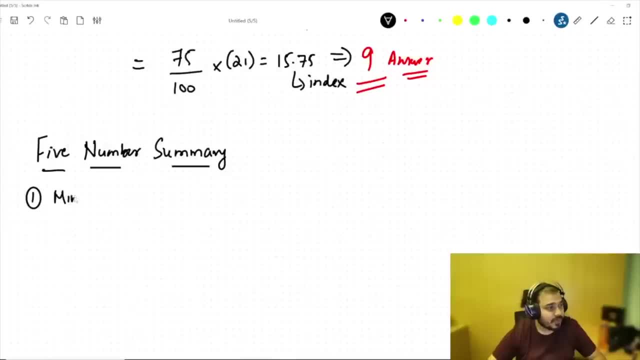 summary, we need to discuss about something called as first one is something called as minimum. The second topic that we should discuss about is something called as first quartile, which is also denoted by Q1.. The third topic that we must discuss about is something called as. 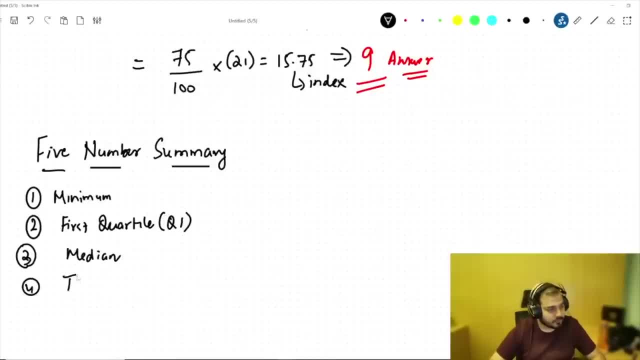 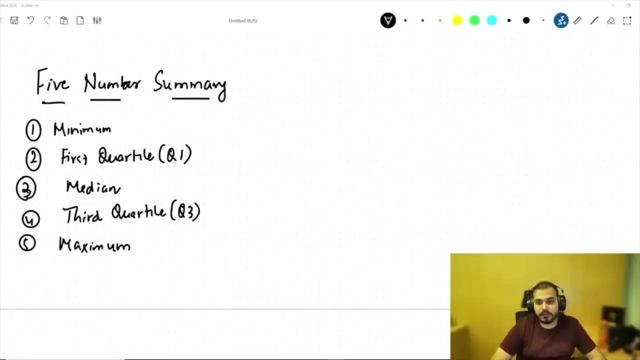 median. The fourth topic that we should discuss about third quartile, which is also said as Q3. And the fifth topic we basically discuss about maximum And with the help of this, we will be using these values to basically remove the outliers. So let's take one example And let's see that by the help of 5 number summary. 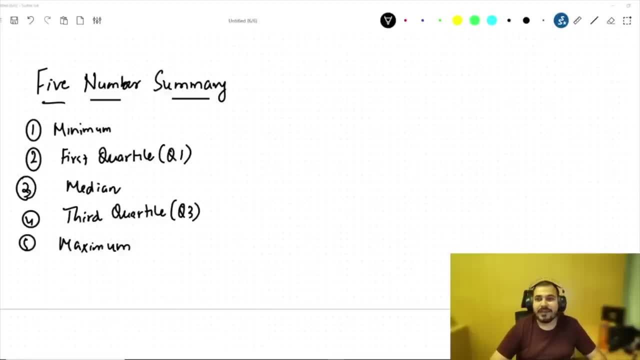 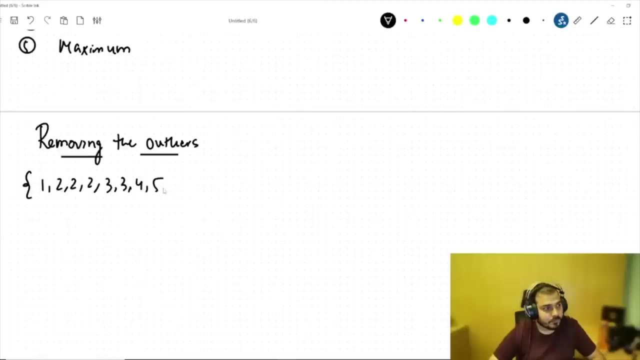 how do we remove an outlier? So, removing an outlier, a very important thing, which is also called as IQR. So here we are going to discuss about removing the outliers. Now, removing the outliers, let's consider that I have one data set which is like this: 1, 2, 2, 3, 3, 4, 5, 5, 5, 6, 6, 6, 6, 7, 8, 8, 9, 27.. 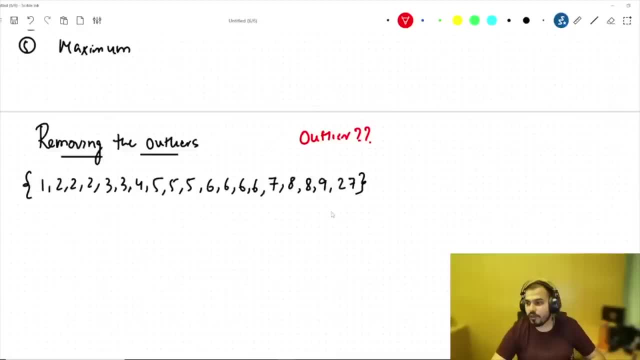 Now, from this distribution, guys, what do you think is? what do you think which is the outlier? So obviously you'll be saying that 27 is the outlier. Always understand, guys. whenever we need to remove an outlier, we really need to define a lower fence. Let's consider that. 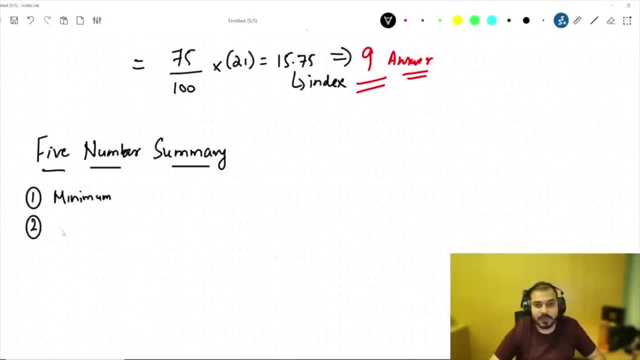 first one is something called as minimum. The second topic that we should discuss about is something called as first quartile, which is also denoted by Q1.. The third topic that we must discuss about is something called as median. The fourth topic that we should discuss about. 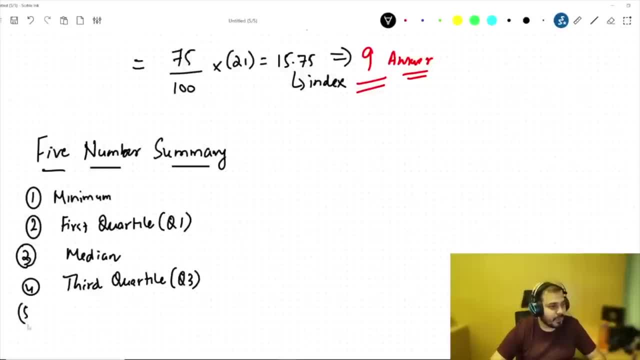 third quartile, which is also read as Q3.. And the fifth topic: we basically discuss about maximum And, with the help of this, we will be using these values to basically remove the outliers. So let's take one example And let's 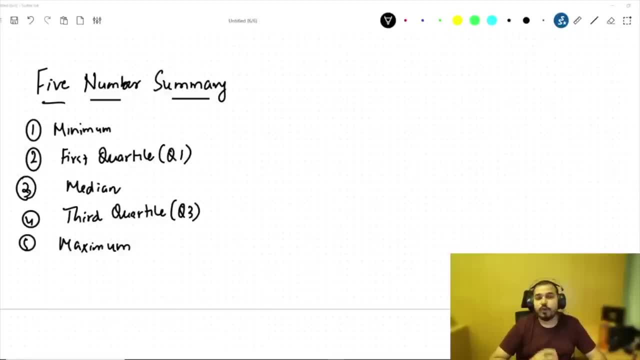 see that by the help of 5 number summary. how do we remove an outlier? So, removing an outlier, a very important thing, which is also called as IQR. So here we are going to discuss about removing the outliers. Now, removing the outliers, let's consider that I have one data set. 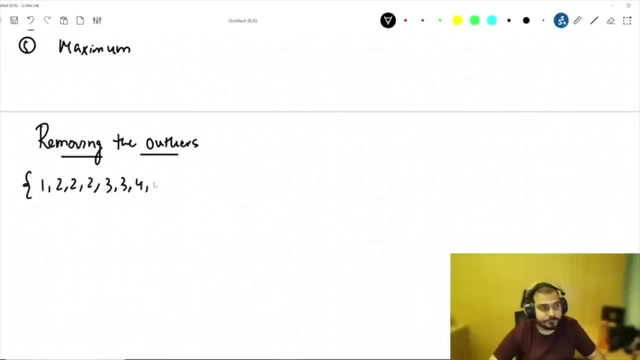 which is like this: 1, 2, 2, 3, 3, 4, 5, 5, 5, 6, 6, 6, 7,, 8, 8, 9, 27.. Now, from this distribution, guys, what do you think is—what do you think? 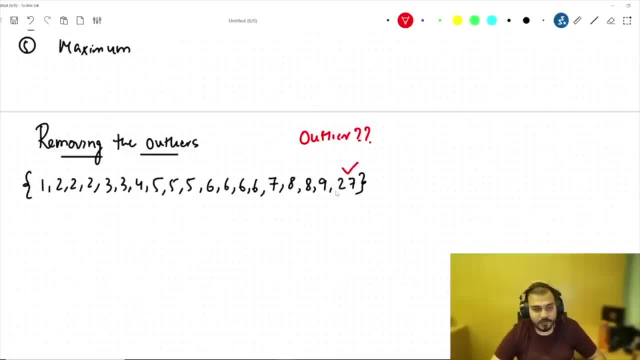 which is the outlier. So obviously you'll be saying that 27 is the outlier. Always understand, guys. whenever we need to remove an outlier, we really need to define a lower fence. Let's consider that I'm going to define a lower fence And then I'm going to define a higher. 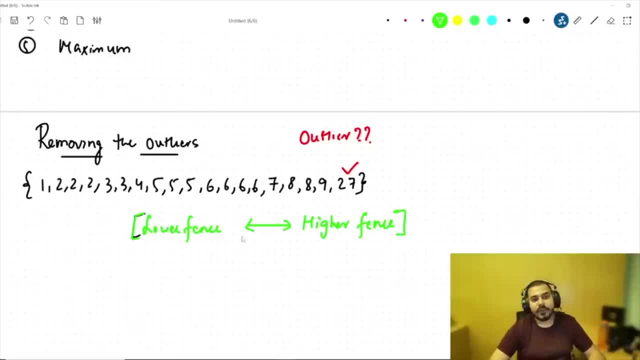 fence. The values that you have over here will be between… lower fence to higher fence. that basically means, after a greater number, all the numbers above that number will be an outlier. after a smaller number, all the number below that particular number, below this lower fence, will be actually treated as an outlier. it should also have higher. it should also. 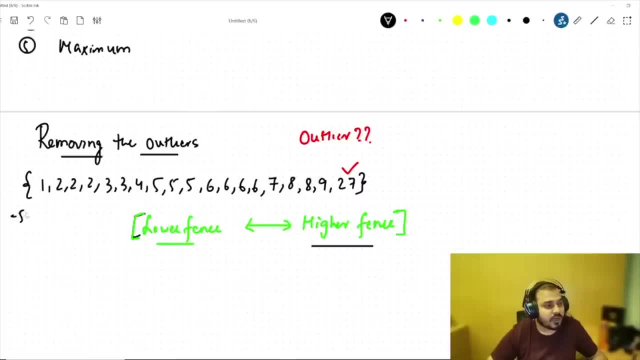 have lower. if i consider that i had one element which is called as minus 50. is minus 50 an outlier for this distribution? yes, the answer is definitely yes. right, if you have minus 50 over here, that is probably in the lower fence side, below the lower fence side, and it can be treated as an outlier. 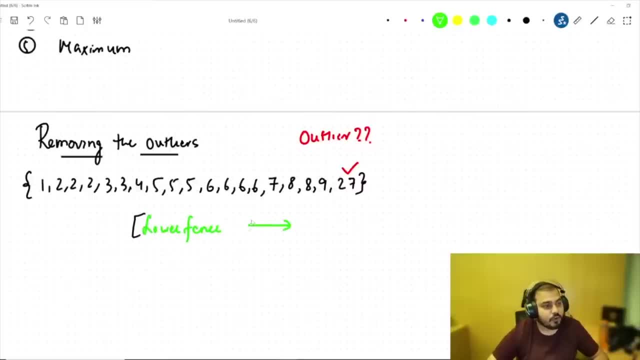 I'm going to define a lower fence and then I'm going to define a higher fence. The values that you have over here will be between lower fence to higher fence. That basically means, after a greater number, all the numbers above that number will be an outlier. After a smaller number. 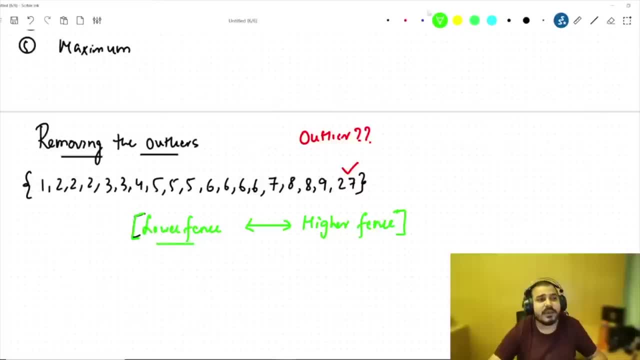 all the number below that particular number, below this lower fence, will be actually treated as an outlier. It should also have higher. it should also have lower. If I consider that I had one element which is called as minus 50. Is minus 50 an outlier for this distribution? 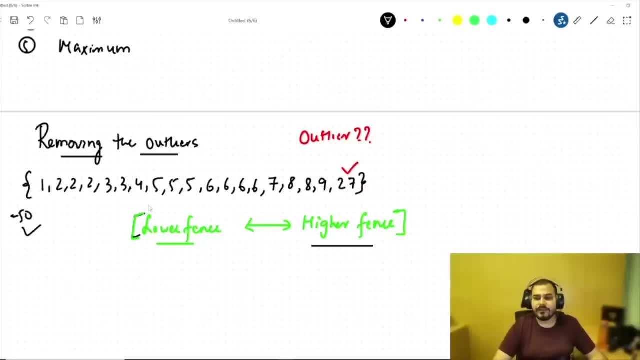 Yes, the answer is definitely yes. right, If you have minus 50 over here, that is probably in the lower fence side, below the lower fence side, and it can be treated as an outlier. So in order to define the lower fence, we write a very simple formula, and the formula looks something like this: 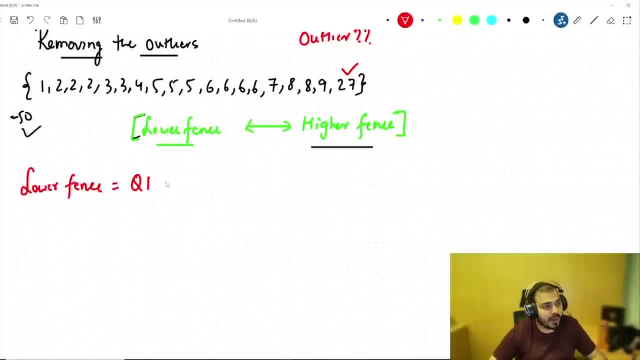 So here you can define: lower fence is equal to Q1 minus 1.5 multiplied by IQR. I'll talk about what is IQR. An upper fence is basically defined as Q3 plus 1.5 multiplied by IQR. These two things are basically there. Now, what exactly is IQR? You will need to understand. 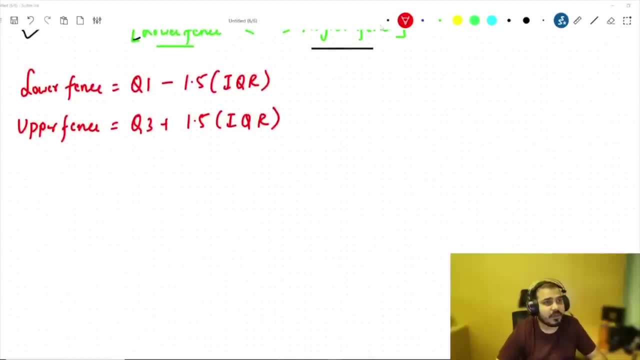 about IQR. What exactly is IQR? IQR is nothing, but it is called as interquartile range. Interquartile range is basically IQR And it is given by the formula Q3 minus Q1.. Q3 is nothing but 75 percentile and Q1 is nothing but 25 percentile. 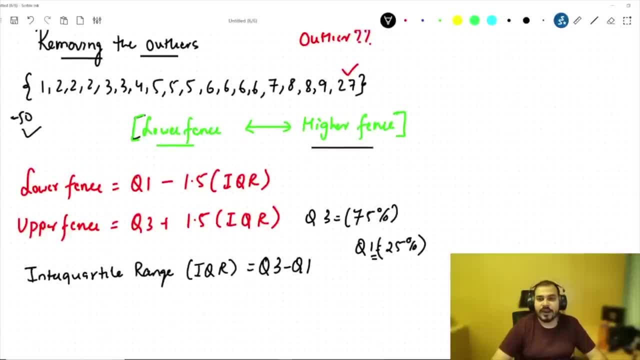 Now quickly check this distribution and try to find out the 25 percentile. So what exactly is 25 percentile? is 75 percentile? Simple formula: 25 multiplied by 100, multiplied by small n. Small n is 1,, 2,, 3,, 4,, 5,, 6,, 7,, 8,, 9,, 10,, 11,, 12,, 13,, 14,, 16,, 17,, 18,, 19.. 19 plus 1.. 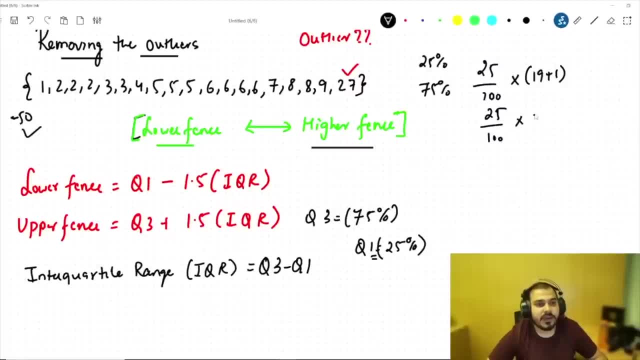 Right. so this is nothing but 25 by 100 multiplied by 20, which is nothing but 5.. This 5 is nothing but index index position. So what is the fifth element index position? So this five is nothing but index position. So what is the fifth element index position? 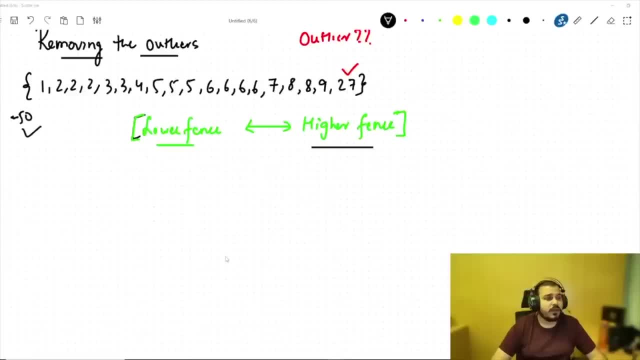 so, in order to define the lower fence, we write a very simple formula and the formula looks something like this. so here you can define: lower fence is equal to q1 minus 1.5 multiplied by iqr. i'll talk about what is iqr- an upper fence. 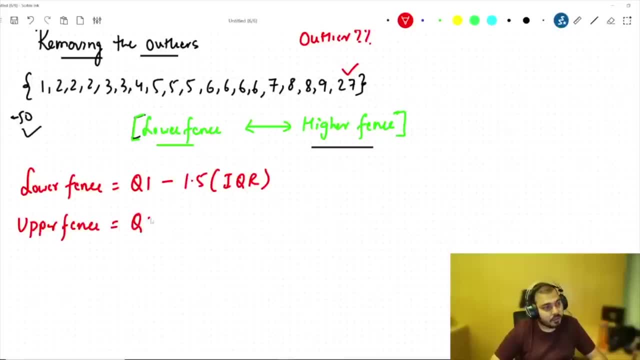 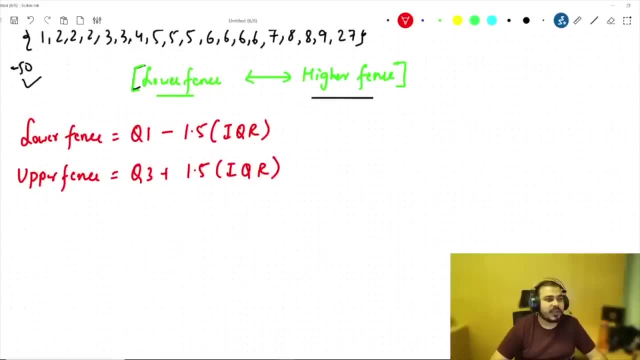 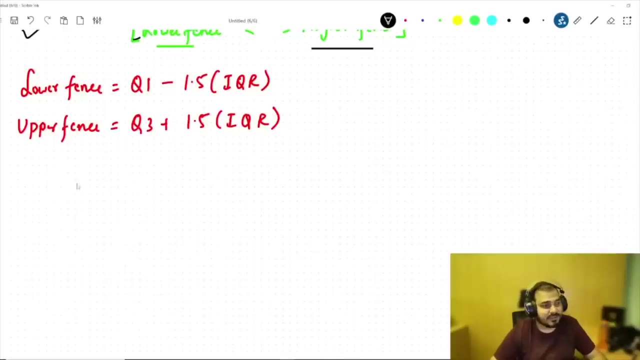 is basically defined as q3 plus 1.5 multiplied by iqr. this two things are basically there. now, what exactly is iqr? you need to understand about iqr. what exactly is iqr? iqr is nothing, but it is called as interquartile range. interquartile range is basically iqr and it is given by the formula q3. 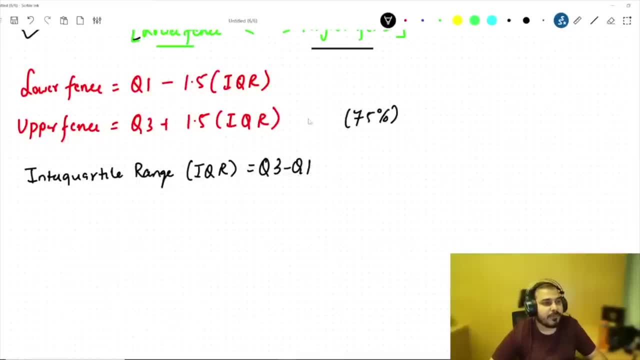 minus q1, q3 is nothing but q1 minus q2 minus q3 minus q3 minus q2 minus q3 minus q3 minus q1 is nothing but 75 percentile and q1 is nothing but 25 percentile. now quickly check this distribution. 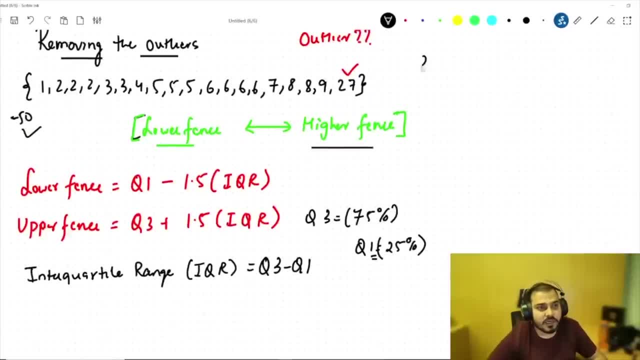 and try to find out the 25 percentile. so what exactly is 25 percentile? what exactly is 75 percentile? simple formula: 25 multiplied by 100, multiplied by small n. small n is 1, 2, 3, 4, 5, 6, 7, 8. 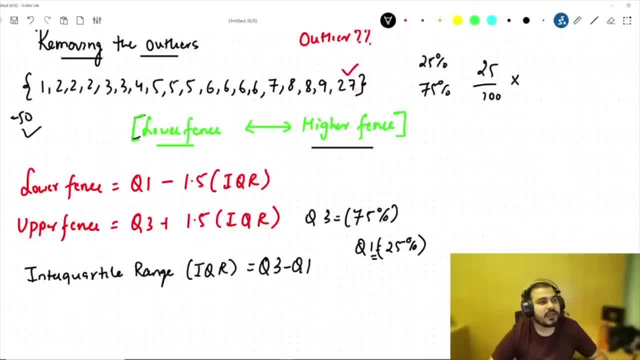 9, 10, 11, 12, 13, 14, 16, 17, 18, 19, 19 plus 1. right. so this is nothing but 25 by 100 multiplied by 20, which is nothing but 5. this 5 is nothing but. 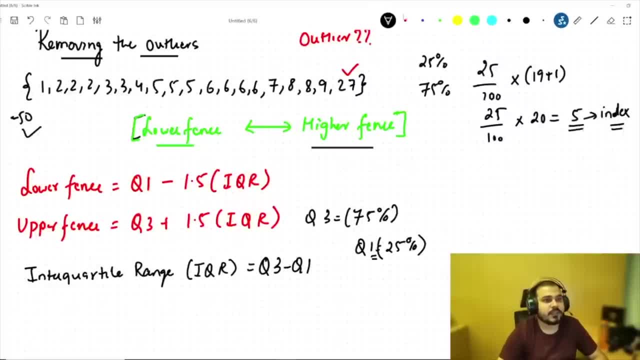 index index position. so what is the fifth element? index position: 1, 2, 3, 4, 5. is everybody getting 25 percentile is nothing but 3? is everybody getting 25 percentile or q1 is equal to 3? similarly, if you try to find out q3, you will be able to get that it is 7. q3 is 7. 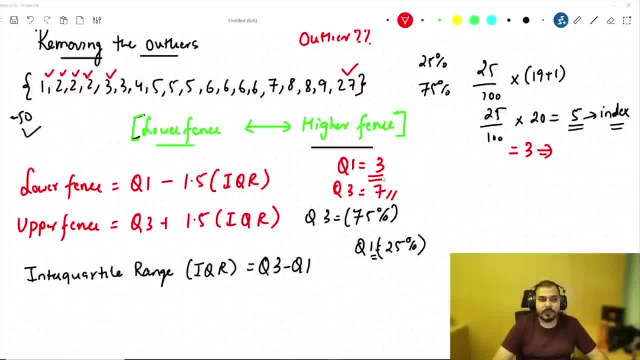 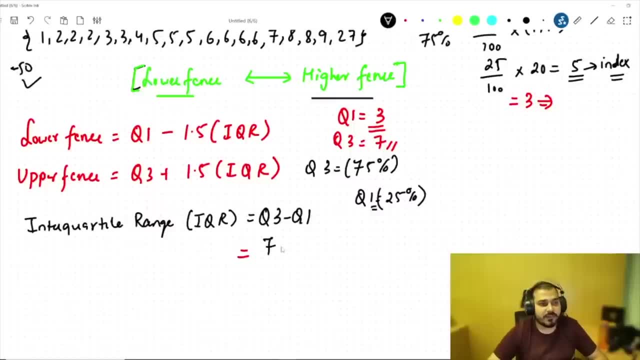 you will get the 15th index for q3. so you are basically going to get 7. now, if i go and compute the interquartile range, what is interquartile range? 7 minus 3, which is nothing but 4 now you. 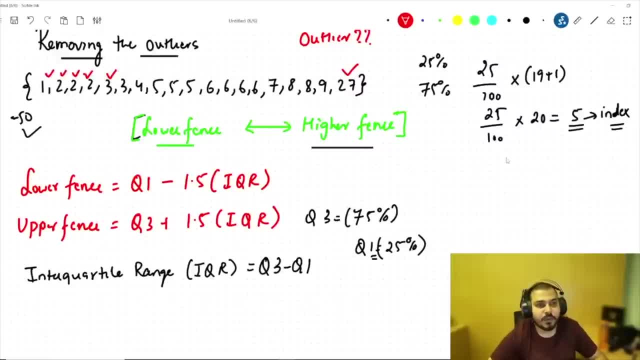 1,, 2,, 3,, 4, 5.. Is everybody getting 25 percentile is nothing but 3?? Is everybody getting 25 percentile or Q1 is equal to 3?? Similarly, if you try to find out Q3,, you will be able to get that it is 7.. 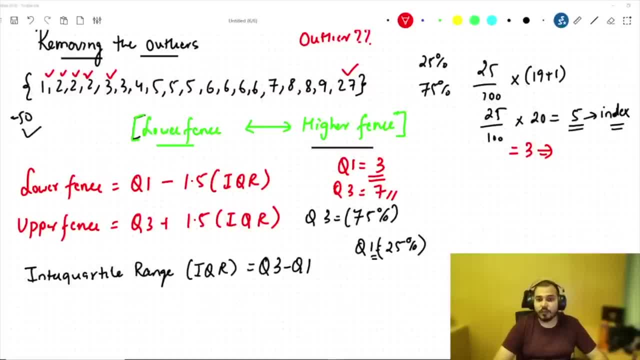 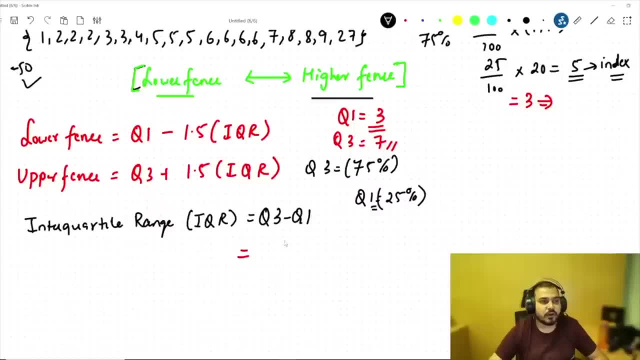 Q3 is 7.. You will get the 15th index for Q3.. So you are basically going to get 7.. Now, if I go and compute the interquartile range, what is interquartile range? 7 minus 3, which is nothing. 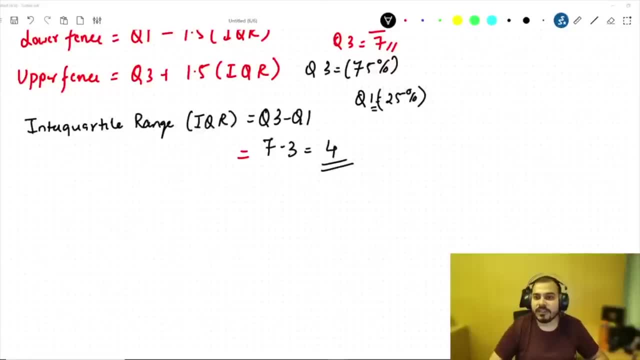 but 4.. Now you have calculated the IQR. So what? all things? we have calculated The IQR, Q3,, Q1, everything has been computed. Now let us go ahead and compute the lower fence. Now the lower fence basically say Q1 minus 1.5 multiplied by IQR. right, This is what lower fence formula is. 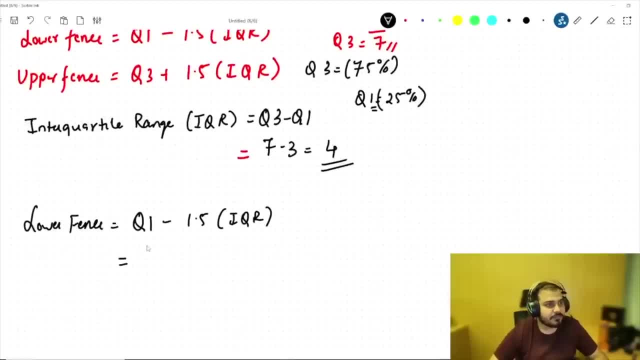 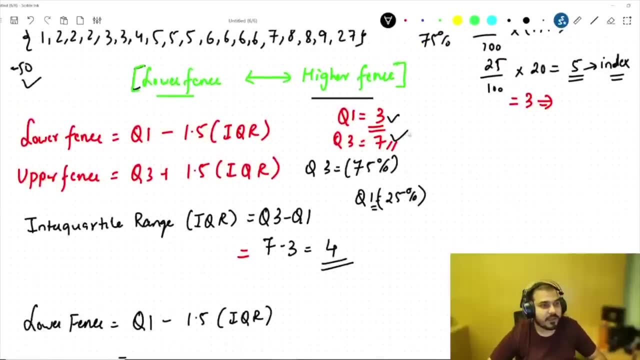 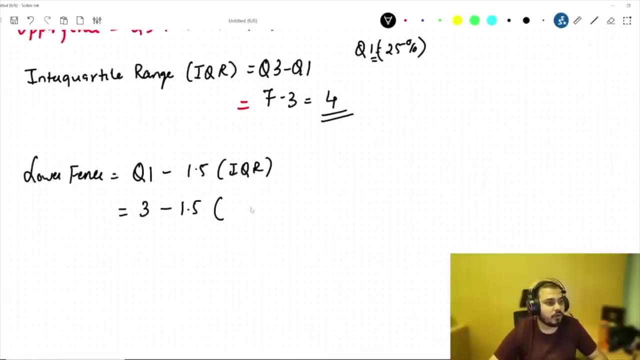 So what is Q1? Q1, basically, is nothing. but what is Q1 in this particular case? I have computed it: It is 3.. You can see over here, Q1 is 3 minus 3, Q3 is 7.. So I am going to write 3 minus 1.5.. What is IQR? 4.. So 3 minus 6, which is 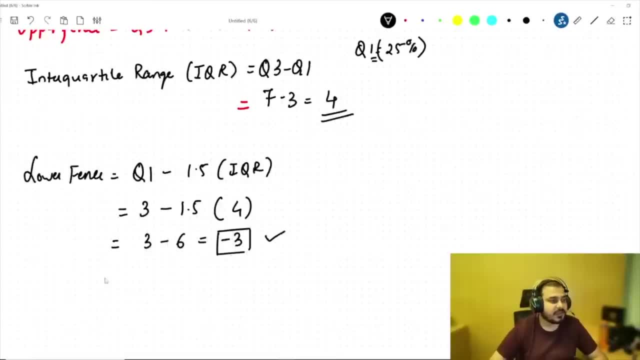 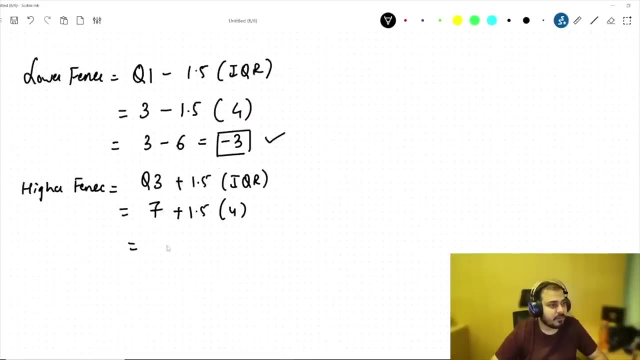 nothing but minus 3.. So the lower fence value is minus 3.. Now let us go and compute about the higher fence. Higher fence, basically say Q3 plus 1.5. multiplied by IQR, Q3 is 7.. 10 plus 6 is equal to 13.. So my lower fence to higher fence range is between minus 3 to plus 13.. 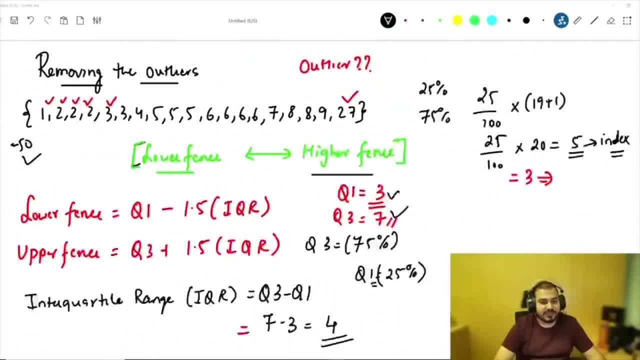 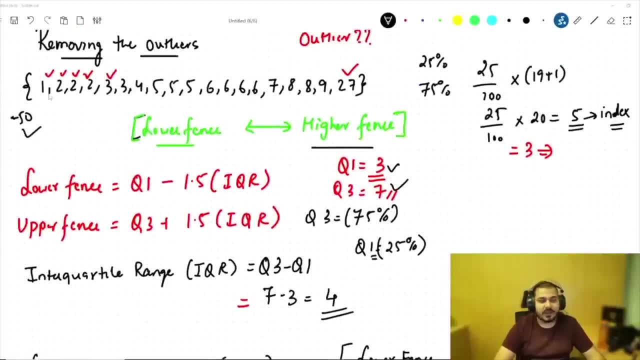 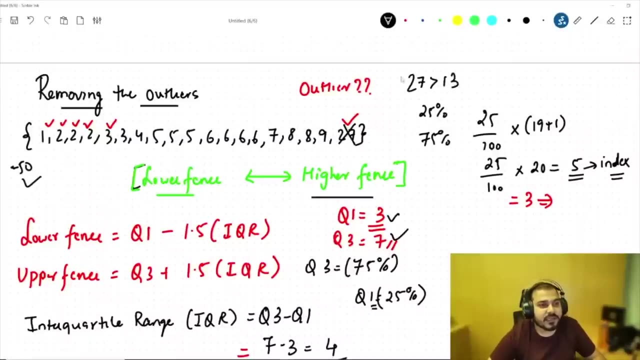 Now tell me which is the outlier from here, Minus 3 to plus 13.. Anything that is greater than 13 is considered as an outlier. Anything lesser than minus 3 is considered as an outlier. So which number should we remove? We should remove 27.. Why 27 is greater than 13,, which is 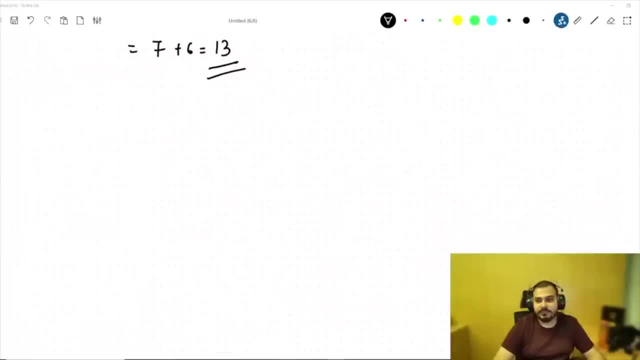 from the higher fence. Now let me write the distributions once again for all of you. Let me write the distribution after removing the 13.. So the remaining data, what I have: 1, 2,, 2,, 3,, 3,, 4,. 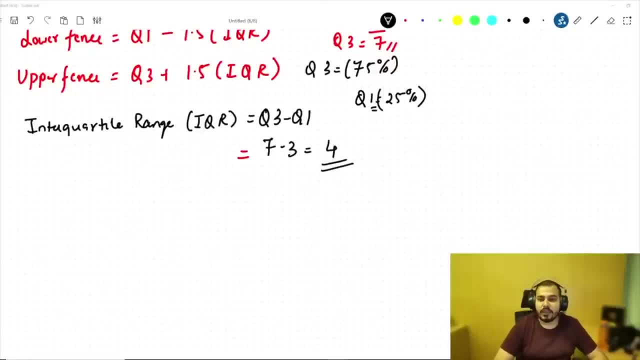 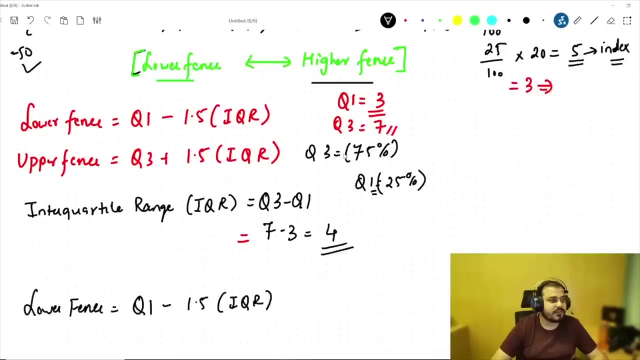 have calculated the iqr. so what, all things? we have calculated the iqr, q3, q1, everything has been computed. now let's go ahead and compute the lower fence. now the lower fence basically say q1 minus 1.5 multiplied by iqr. right, this is what lower fence formula is. so what is q1? q1 basically is nothing, but what is q1 in. 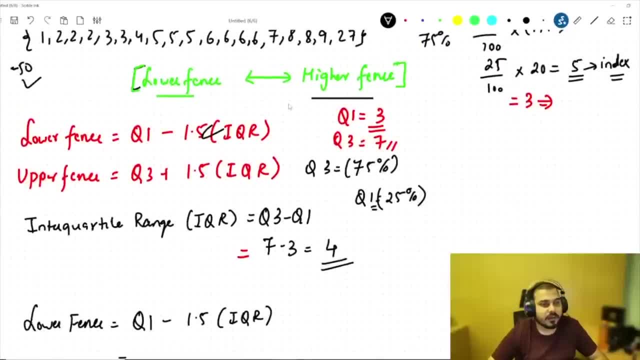 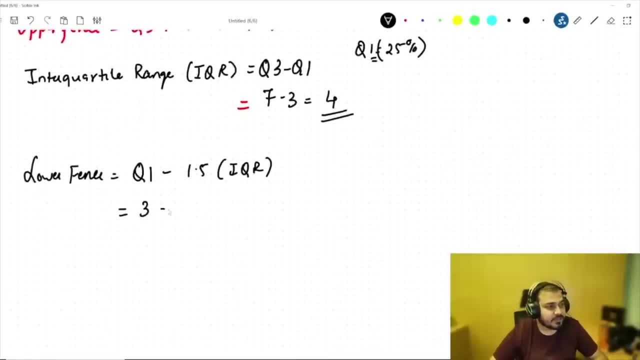 this particular case. i have computed it, it is 3. you can see over here: q1 is 3, q3 is 7. so i am going to write 3 minus 1.5. what is iqr 4? so 3 minus 6, which is nothing but minus 3. so the lower fence. 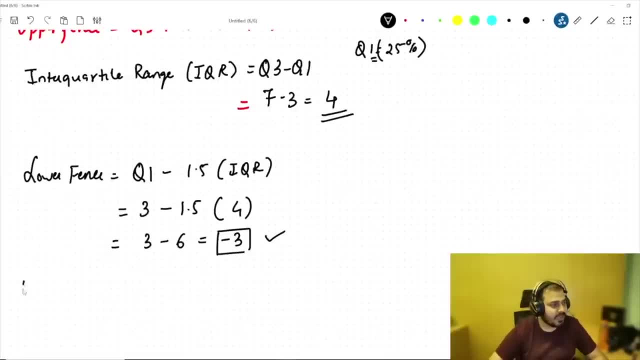 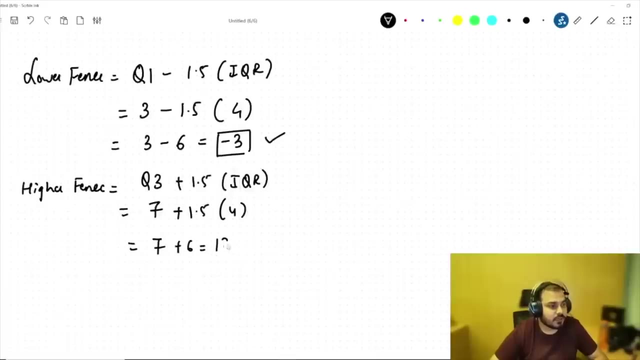 value is minus 3. now let's go and compute about the higher fence. higher fence basically say q3 plus 1.5 multiplied by iqr, q3 is 7. 7 plus 6 is equal to 13. so my lower fence to higher fence range is between minus 3 to plus 13. now tell me which is the. 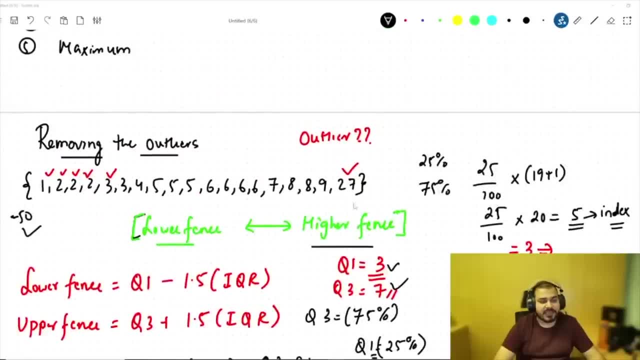 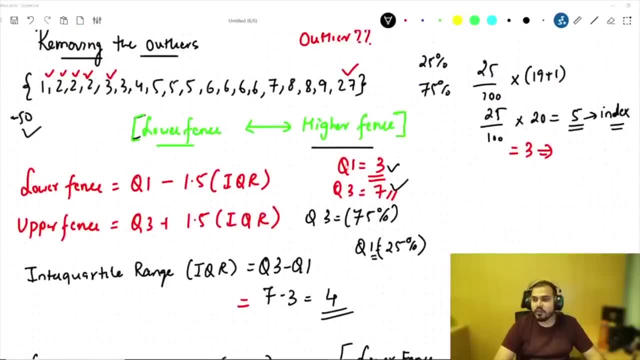 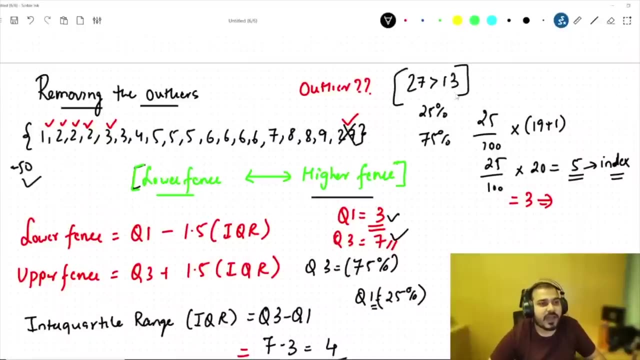 outlier from here minus 3 to plus 13. anything that is greater than 13 is considered as an outlier. anything lesser than minus 3 is considered as an outlier. so which number should we remove? we should remove 27, why 27 is greater than 13, which is from the higher fence. now let 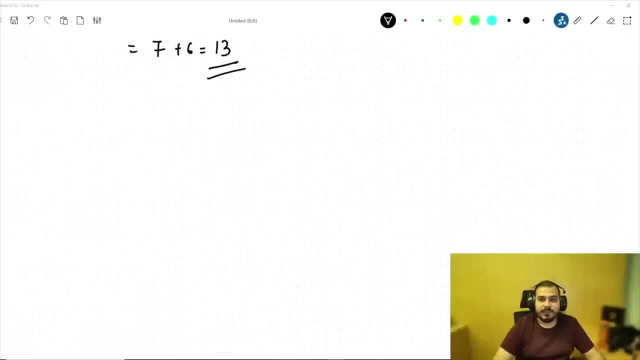 me write the distributions once again for all of you. let me write the distribution after removing the 13, so the remaining data, what i have: 1, 2, 2, 3, 3, 4, 5, 5, 5, 6, 6, 6, 6. 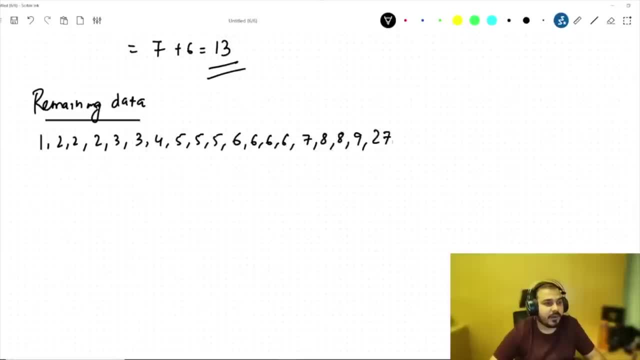 7, 8, 8, 9, 27, but i told you we are removing 27, right? so 27 is removed because it is an outlier. now you know what is the. what is the minimum value out of all these numbers? minimum value is 1. what? 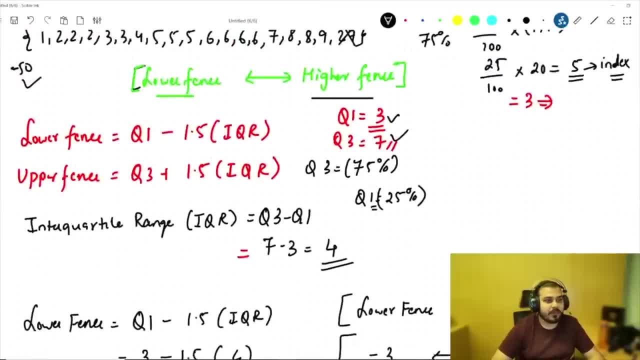 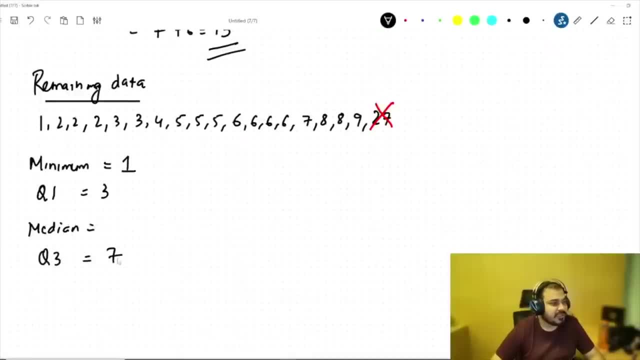 is q1, my first quartile we have computed over here. q1 is nothing but 3 median. you calculate and tell me quickly. then you have q3. q3 is 7 and the maximum number after removing the outlier is nothing but 9. so here you are getting your five number summary. now quickly compute. 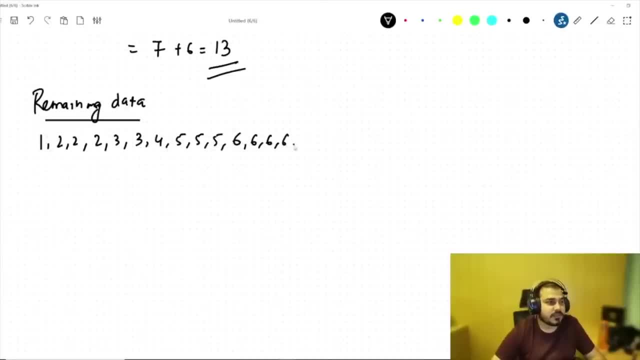 5,, 5,, 5,, 6,, 6,, 6,, 6,, 7,, 8,, 8,, 9,, 27.. But I told you we are removing 27, right, So 27 is removed. 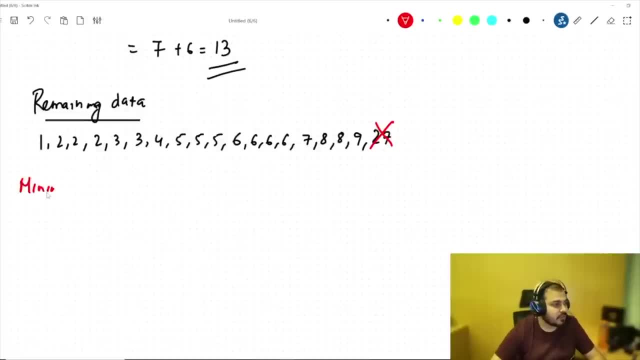 because it is an outlier. Now you know what is the. What is the minimum value out of all these numbers? Minimum value is 1.. What is Q1? My first quartile we have computed over here. Q1 is nothing but 3.. Median you calculate and tell me quickly. 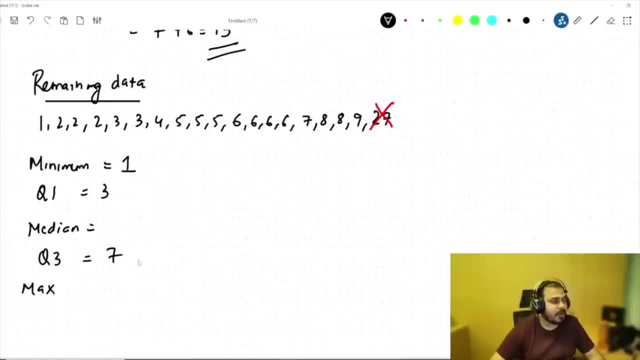 Then you have Q3.. Q3 is 7. And the maximum number, after removing the outlier, is nothing but 9.. So here you are getting your 5 number summary. Now quickly compute median and tell me What is median. Median is nothing but 5.. 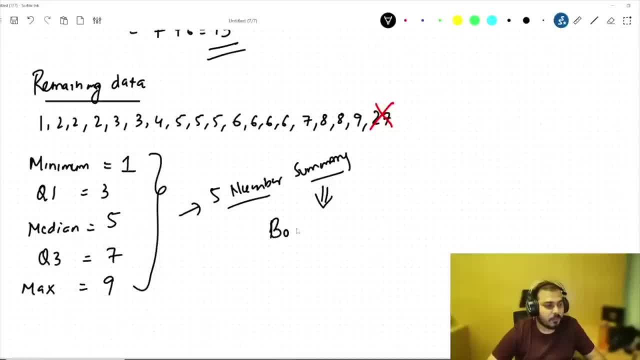 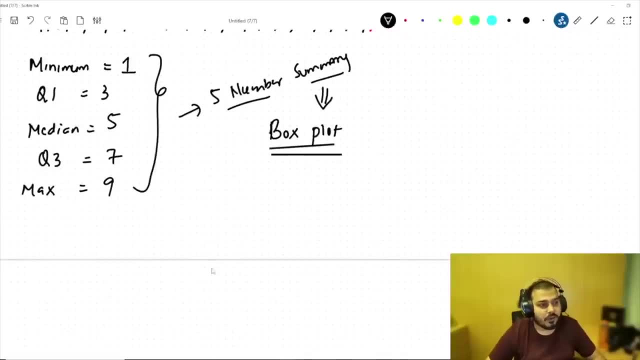 Now let's draw a plot which is called as box plot. By this specific data, you can definitely draw a box plot. Now, how does a box plot basically get drawn? So you will be having x-axis, And let's consider that in this. 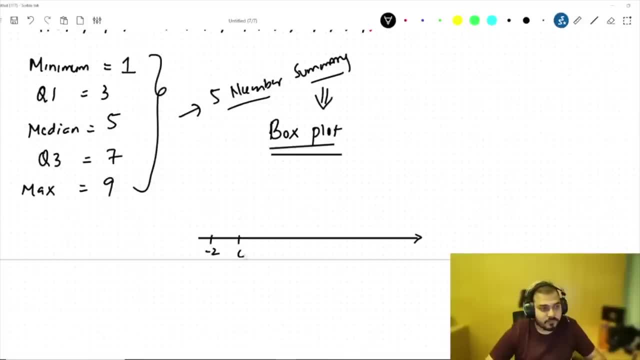 particular x-axis. you have values like minus 2,, 0,, 2,, 4,, 6,, 8, 10.. So this is your x-axis. Now just go and find out where is minimum element. So, basically, you will be having x-axis And let's go and find out where is minimum element. 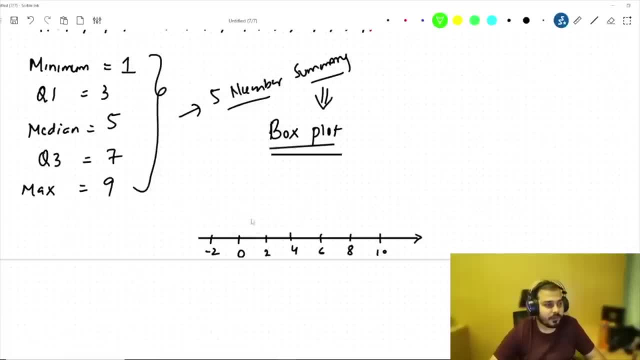 Minimum element will probably fall over here, That is, in 1.. Q1 will basically fall at 3.. So this will be your 3.. Median is basically 5.. So this is basically your 5.. Q3 is nothing but 7.. So this is your 7.. 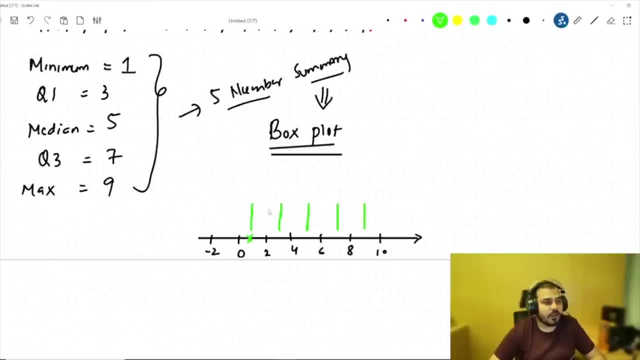 And max is nothing but 9.. So this is your 9.. Now all you have to do is that join these lines. So this exactly is your box plot. as an element, i would have to extend this line this much big and probably put 27 somewhere here. 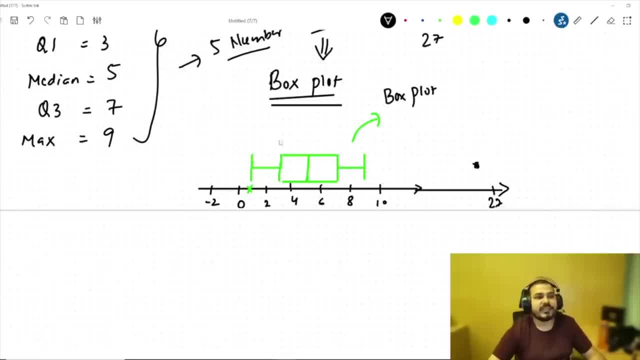 and this used to be one dot over here. have you seen this kind of plot? this value is nothing but minimum. this is my q1, this is my median, this is my q3 and this is my max. and this technique of removing an outlier, we basically say, with respect to lower fence and higher fence, 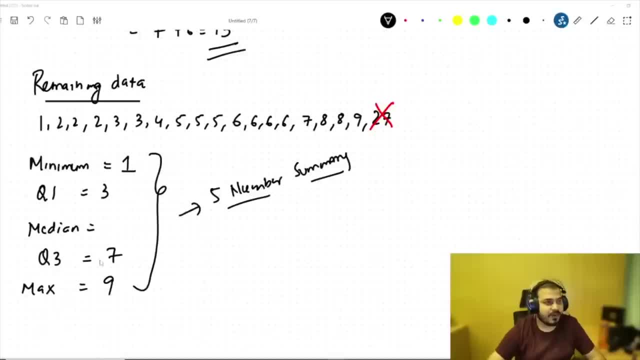 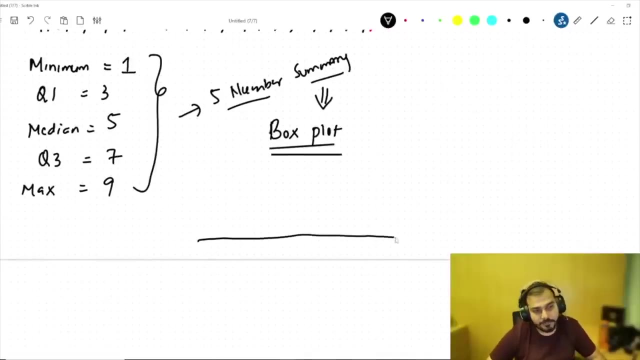 median and tell me what is median? median is nothing but 5. now let's draw a plot which is called as box plot. by this specific data, you can definitely draw a box plot. now how does a box plot basically get drawn? so you will be having x-axis and let's consider that in this particular 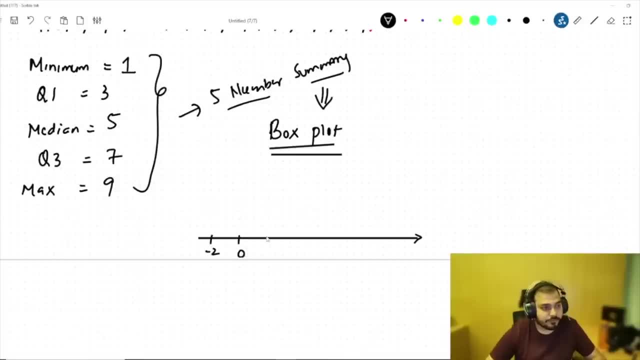 x-axis. you have values like minus 2, 0, 2, 4, 6, 8, 10. so this is your x-axis. now just to go and find out: where is minimum element. minimum element will probably fall over here, that is, in 1 q1 will. 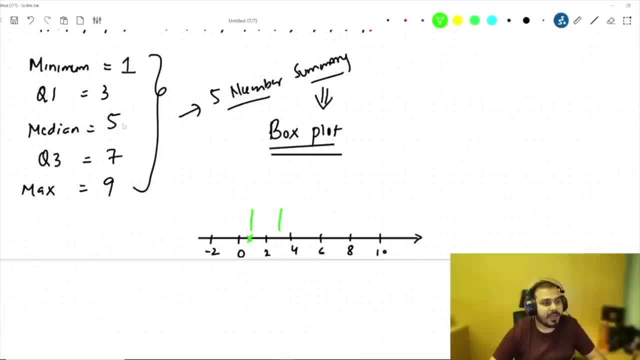 basically fall at 3, so this will be your 3. median is basically 5, so this is basically your 5. q3 is nothing but 7. so this is your 7, and max is nothing but 7. so this is your 7, and max is nothing but 7. 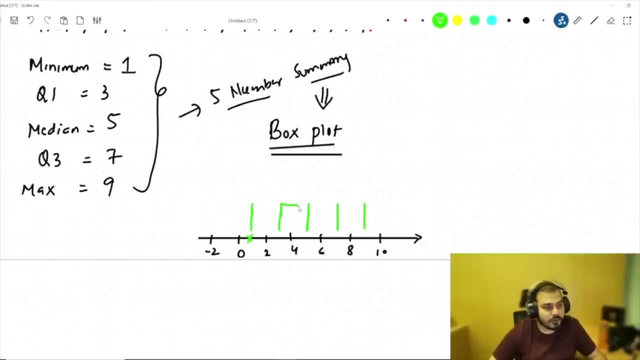 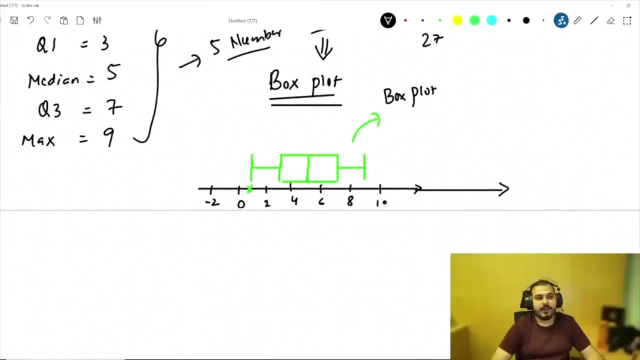 so this is your max. now all you have to do is that: join these lines. so this exactly is your box plot. if I had kept 27 as an element, I would have to extend this line this much big and probably put 27 somewhere here, and this used to be one dot over here. have you seen this kind of plot? this value is 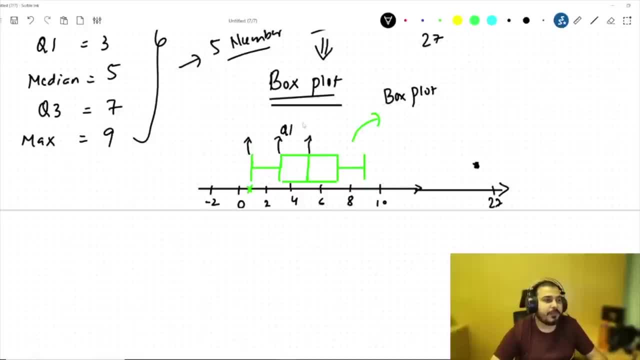 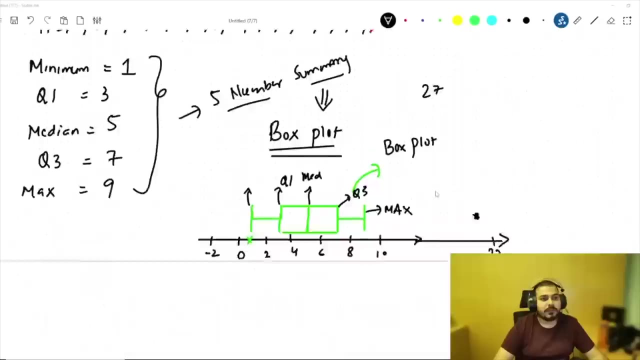 nothing but minimum. this is my q1, this is my minimum, this is my minimum, this is my basic value. median, this is my Q3, and this is my max. And this technique of removing an outlier, we basically say with respect to lower fence and higher fence, and we also use something called as 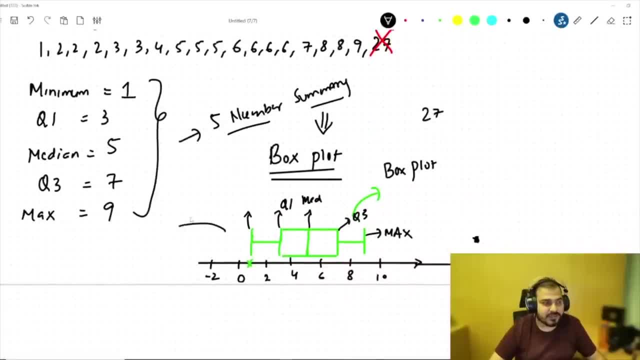 IQR, The first application that I've shown you here. this is also used extensively in data visualization, So you really need to know all these things. I've drawn it in front of you. I can also do this with code. I have to just install a library In matplotlib. you have a. 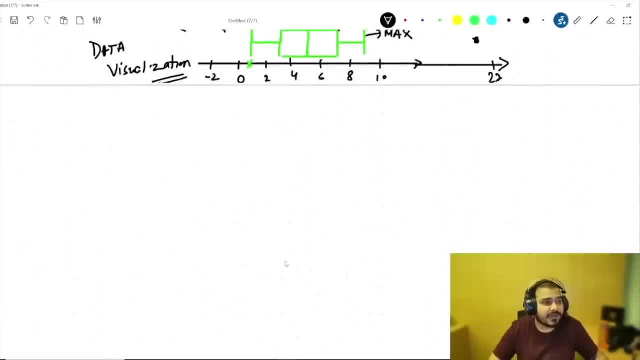 library, where you can probably do all these things. Now let's come back to understand about variance. Summation of i is equal to 1 to n x of i minus x, bar whole square divided by n minus 1.. This n minus 1, why we do it. it is also called as basal correction. We also say it as degree of. 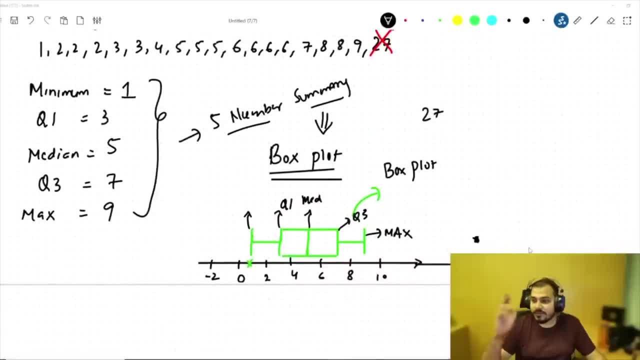 and we also use something called as iqr, the first application that i shown you here. this is also used extensively in data visualization. so you really need to know all these things. i've drawn it in front of you. i can also do this with code. i have to just install a library in matplotlib you have. 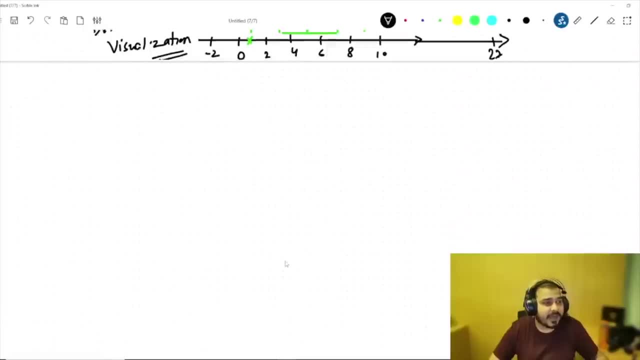 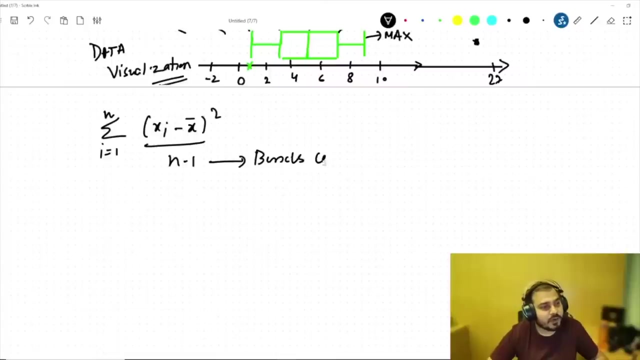 a library where you can probably do all these things. now let's come back to understand about variance. summation of i is equal to one to n x of i minus x, bar whole square divided by n minus one. this n minus one. why we do it? it is also called as basal correction. we also say it as degree. 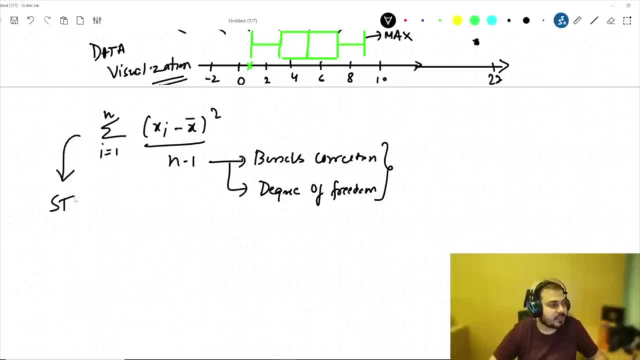 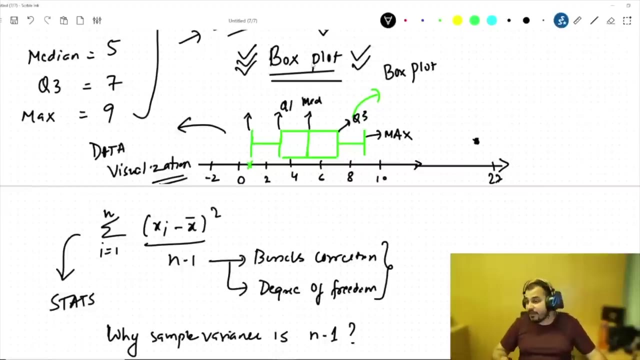 of freedom and i have probably made this video in my stats playlist. why sample variance is divided by n minus one? you can go and search for that. you can definitely understand this thing now. now tell me one interview question may come that: what is the application of box plot? box plots can be used to determine outliers. 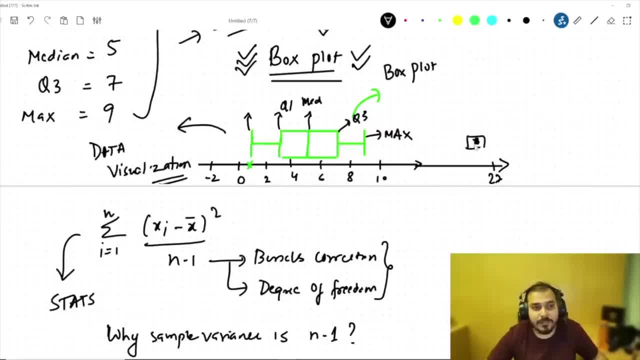 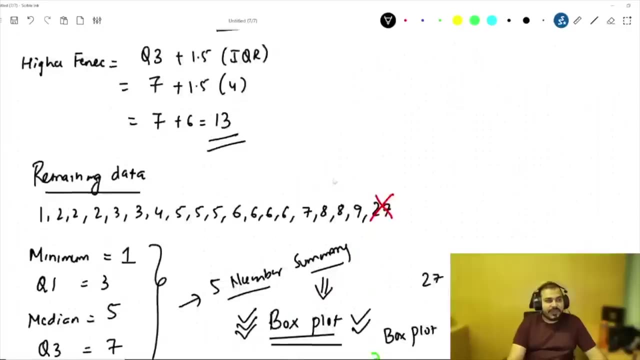 because i just told you that if i was giving 27 over here, my element would have come over here. so box plot actually gives you a visualization way to basically see where an outlier is actually present. if someone asks you how do you create or how do you determine an outlier, you can explain. 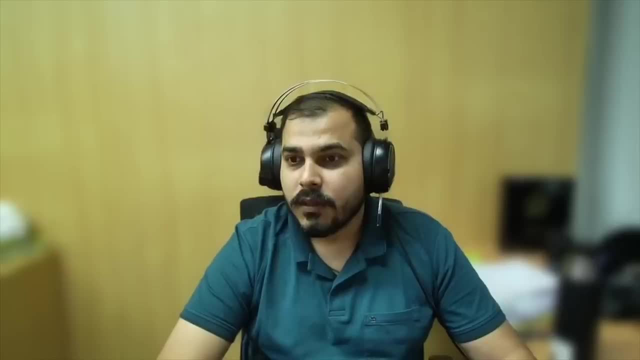 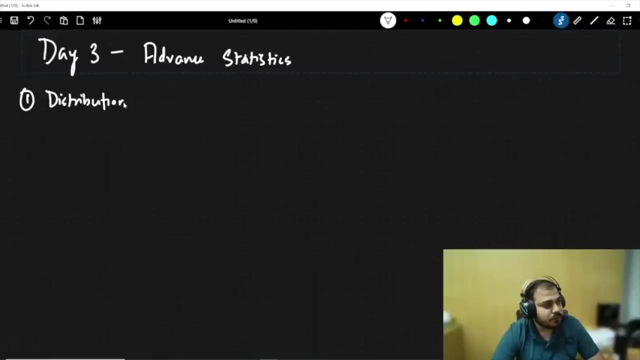 this entire concepts, whatever i have explained with respect to percentiles, hello guys. uh, regarding the agenda, first of all i'm going to talk about, we're going to discuss about lot of distributions now. in this distribution, you will specifically have something called as normal distribution or gaussian distribution. then we will try to discuss. 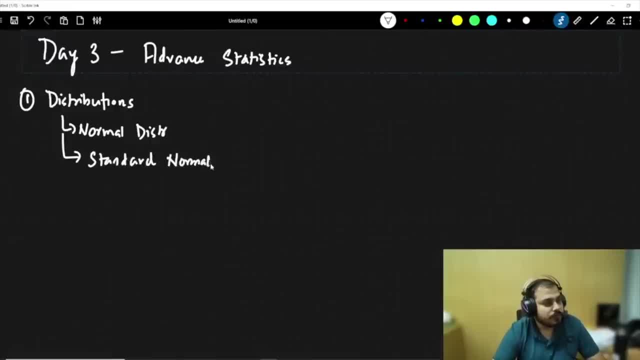 standard normal distribution, standard normal distribution. then probably one more example on z screes. we'll try to see z zscores both with a- uh, you know, z table- there is a concept called a z table- and y realizent scores are actually use. then we will discuss about log normal distribution. then probably we will also discuss 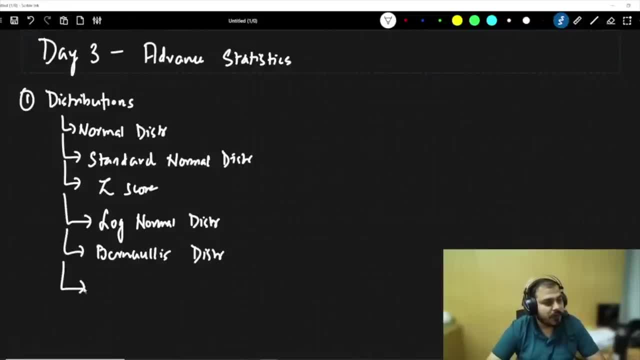 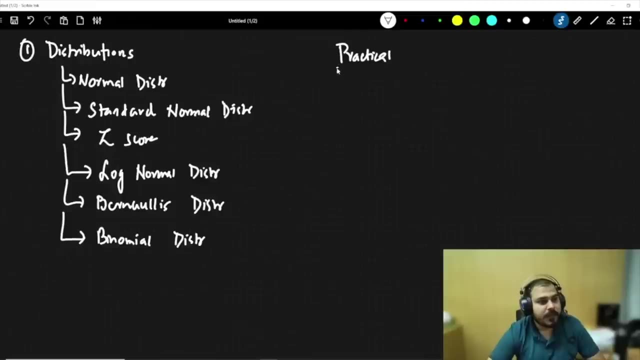 about Bernoulli distribution. then, finally, we will discuss about binomial distribution and we will see some examples, we will solve some examples and then whatever practical part is left that we have not covered till now like mean median mode, everything will. 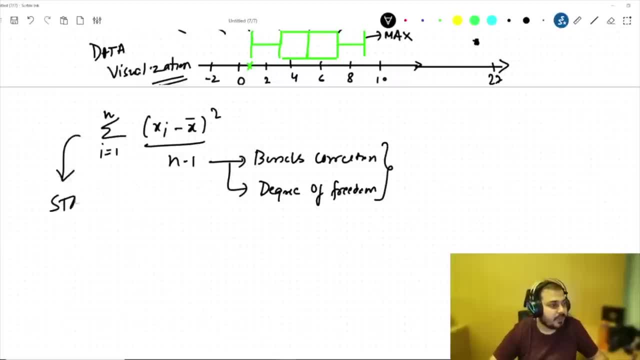 freedom, And I have probably made this video in my stats play- Why sample variance is divided by n minus 1.. You can go and search for that. You can definitely understand these things now. Now tell me- one interview question may come that: what is the? 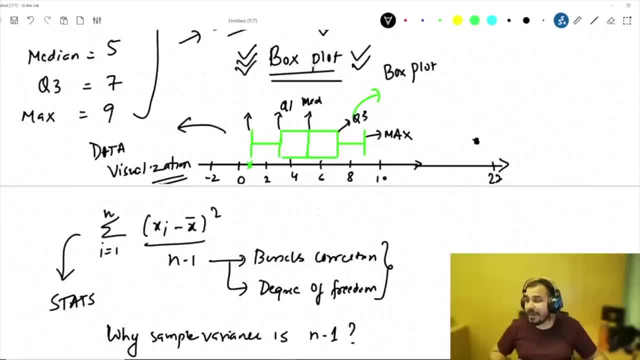 application of boxplot. Boxplots can be used to determine outlier, because I just told you that if I was giving 27 over here, my element would have come over here. So boxplot actually gives you a visualization way to basically see where an outlier is actually present If someone asks you. 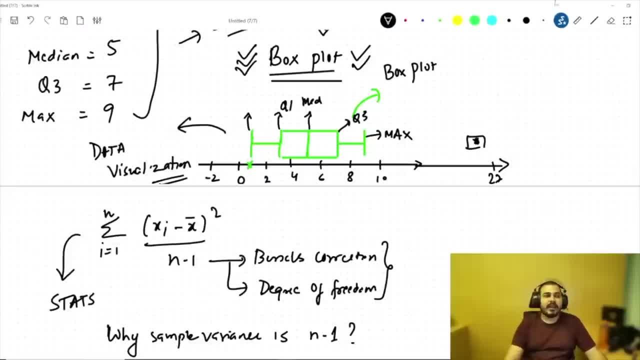 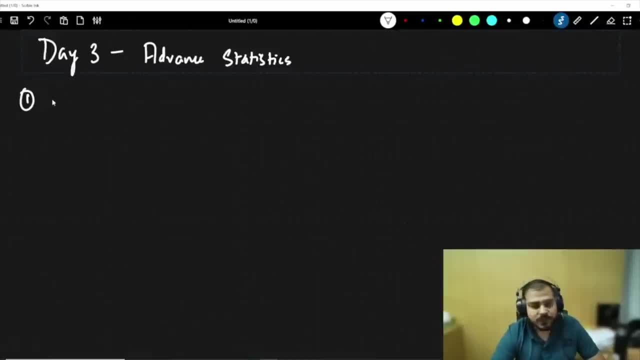 how do you Create or how do you determine an outlier? You can explain this entire concepts, whatever I've explained with respect to percentiles. Hello guys, regarding the agenda, first of all I'm going to talk about, we're going to discuss about a lot of distributions. Now, in this distribution, you will 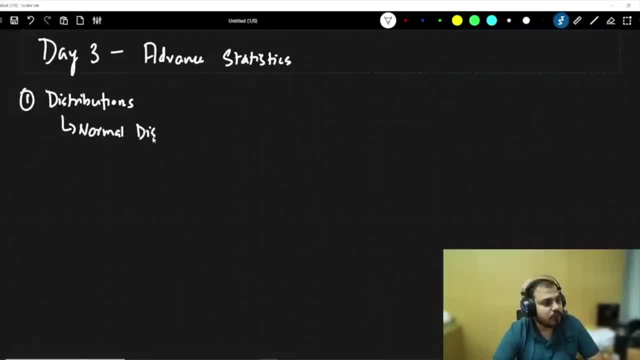 specifically have something called as normal distribution or Gaussian distribution, Then we will try to discuss about standard normal distribution, standard normal distribution. Then probably one more example on z-scores. We'll try to see z-scores both with. you know z-table. There is a concept called a z-table. 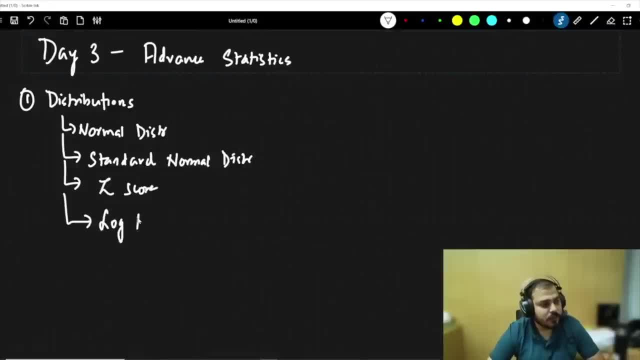 and why z-scores are actually used. Then we will discuss about log normal distribution. Then probably we will also discuss about Bernoulli distribution. Then, finally, we'll discuss about binomial distribution And we'll see some examples, we'll solve some examples And then 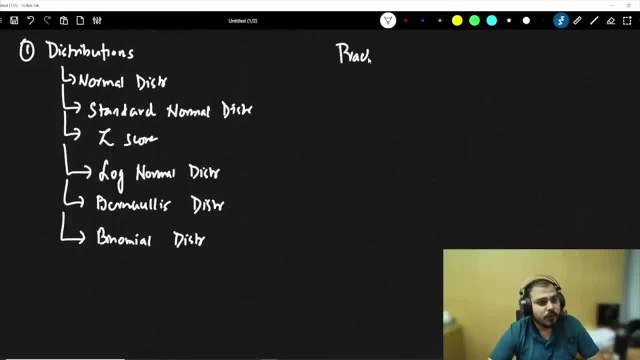 we'll talk about the other practical parts of that That we have not covered till now. Like mean median mode, everything will get covered over here. So if you want to do mean median mode, we'll try to do with Python programming language Okay, And we'll also do variance. 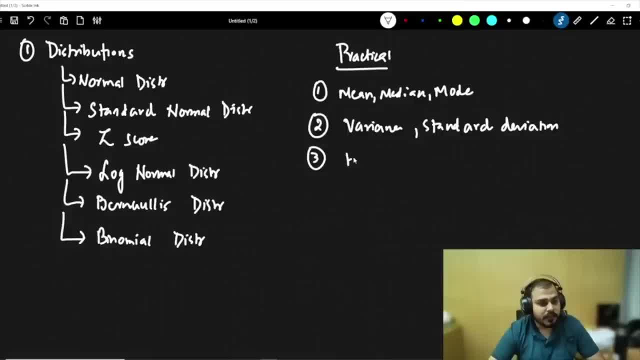 standard deviation. The third thing: we'll try to create histograms, We'll try to create PDFs, probability, density functions. We'll try to understand how does a distribution, this normal distribution- will look in code. We'll try to find out how to find out this. IQ are using code And we'll see all these things. 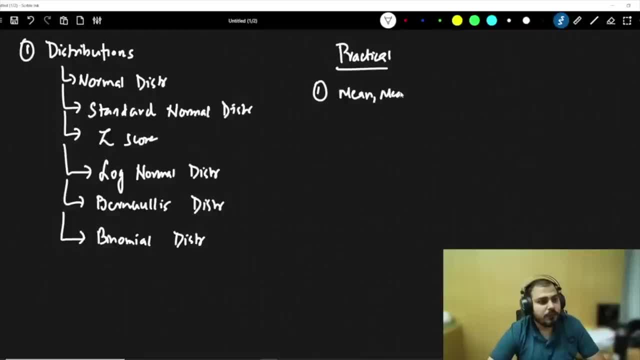 get covered over here. so if you want to do mean median mode, we will try to do with python programming language. ok, and we will also do variance standard deviation. the third thing: we will try to create histograms. we will try to create pdf. probability density. 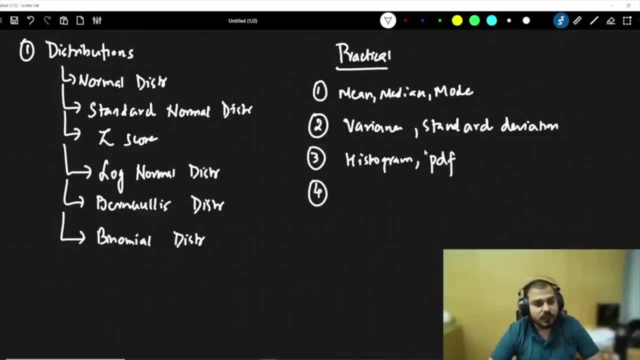 functions. we will try to understand how does a distribution, this normal distribution, will look in code. We will try to find out how to find out this IQ are using code and we will see all these things and some examples of log normal distribution we are going to see. ok, I can also discuss. 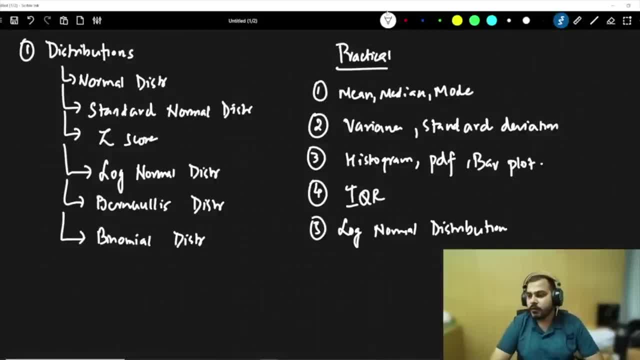 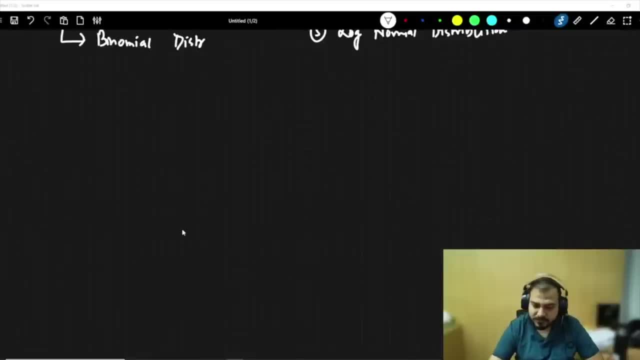 about bar plot, not to worry, that also we will try to discuss about it. ok, I can also discuss about violent plot. so whatever things will come, we will discuss about it Now. first thing first. today we are going to discuss about distribution. now, what exactly? 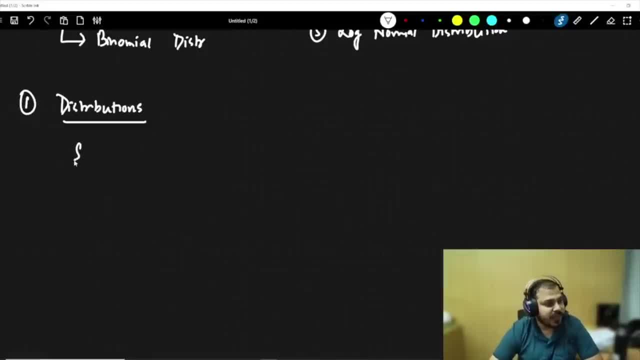 is distribution. Understand distribution of data. when I say I have a data set, let's say that I have a data set of ages like 24,, 26,, 27,, 28,, 30,, 32, you know, so we have lot of data set. 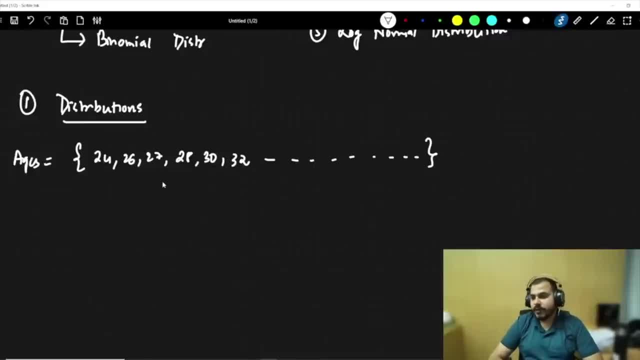 Now, when we have this particular data set- always ok, always in the first thing that we need to focus on is that: how do we basically see this data set in a visualized way, because obviously this is a continuous data. We always, we already know that this is a discrete continuous data in this particular 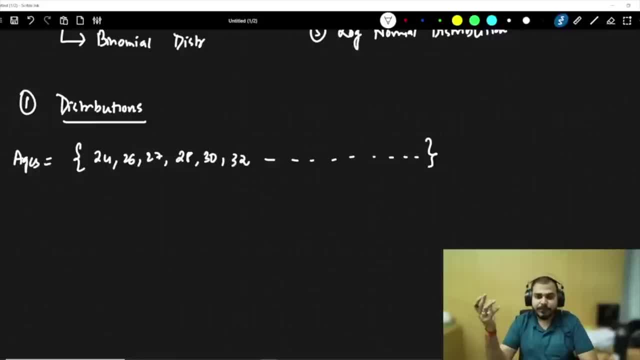 case age. I am just going to consider as discrete continuous data. Now, in the case of continuous data, what kind of graphs do you see? probably you will be able to understand about that specific data. So if I really want to get one analysis or if I really want to start my analysis, I really 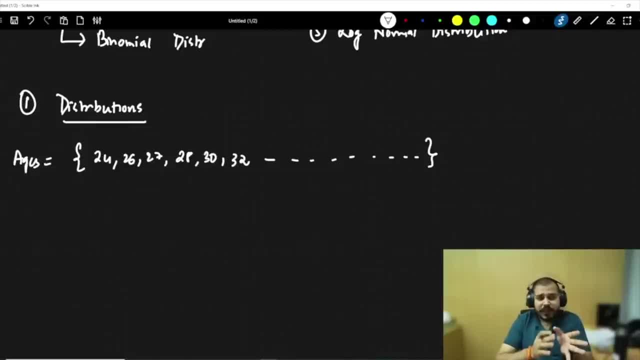 need to see lot of visualized diagrams, And that is where, when I consider this entire distribution, there are multiple ways to visualize this data through various graphs, And these graphs can really play a very important role whenever, probably, we are discussing about. 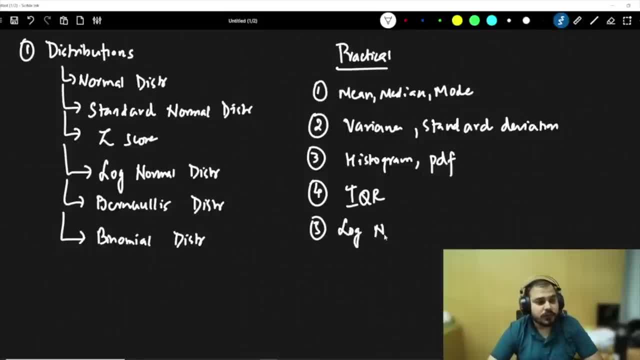 And some examples of log normal distribution we are going to see. Okay, I can also discuss about bar plot, not to worry, That also we'll try to discuss about it. Okay, I can also discuss about violent plot. So whatever things will come we'll discuss about Now. first thing first. 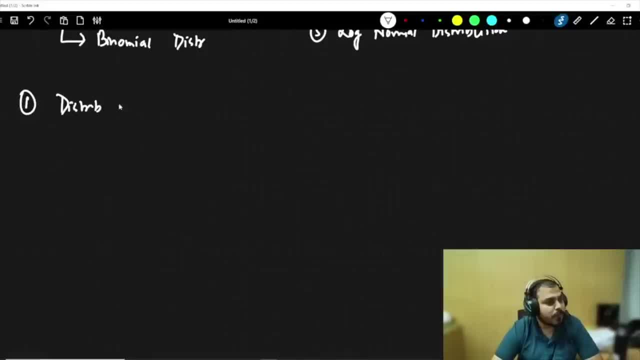 today we are going to discuss about distribution. Now, what exactly is distributions? Understand, distribution of data. When I say I have a data set, let's say that I have a data set of ages like 24,, 26,, 27,, 28,, 30,, 32, you know, So we have a lot of data set. Now, when we have this, 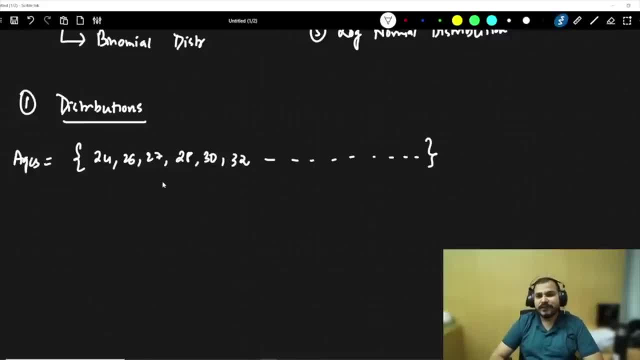 particular data set always, okay, always. in. the first thing that we need to focus on is that: how do we, how do we really see this data set in a visualized way, Because obviously this is a continuous data. We always, we already know that this is a discrete continuous data. In this particular case, age, I'm 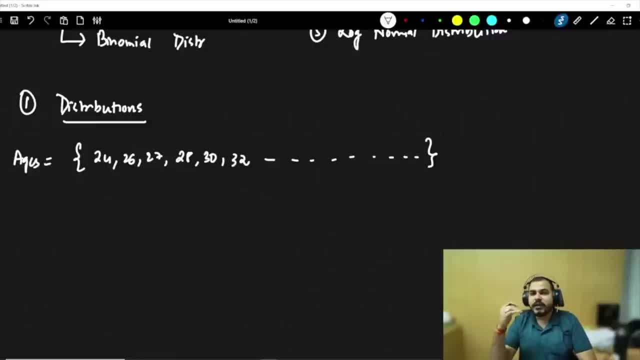 just going to consider as discrete continuous data. Now, in the case of continuous data, what kind of graphs do you see? Probably you'll be able to understand about that specific data. So if I really want to get one analysis, or if I really want to start my analysis, I really need to see a. 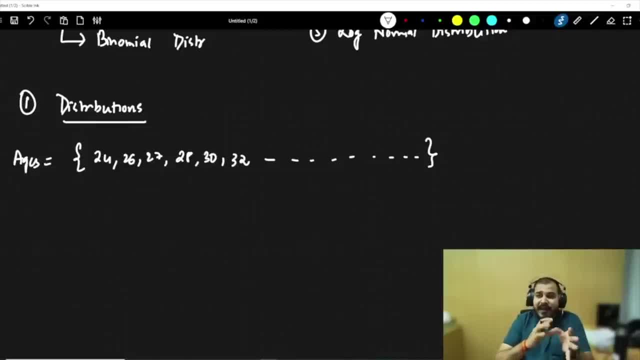 lot of visualized diagrams. So this is where, when I consider this entire distribution, there are multiple ways to visualize this data through various graphs, And these graphs can really play a very important role whenever probably we are discussing about, whenever probably we are creating reports. 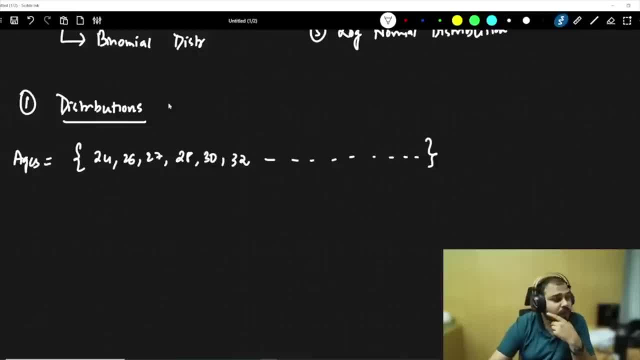 where we are doing exploratory data analysis and many things. So let's go towards distribution. Suppose I have a specific distribution of data, I probably want to plot this data through some way. Let's consider that Okay, So that I want to probably plot this data through some way, And the best and the easy way that you 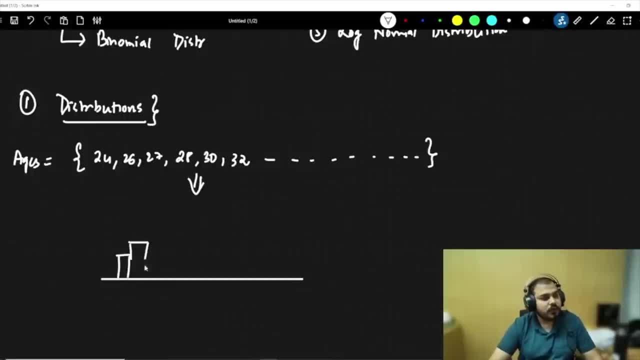 can probably think about. is your histogram right? So we have already seen how to create histograms. You will be able to create diagrams like this. buildings like this- right, So you will be able to get buildings like this. And finally, what you do? you smoothen this histogram to get some 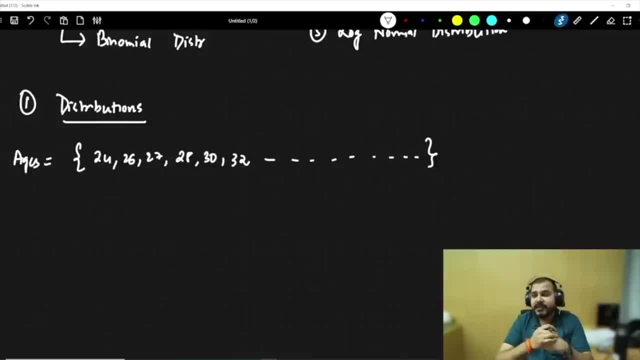 whenever, probably, we are creating reports where we are doing exploratory data analysis and many things. So let's go towards distribution. Suppose I have a specific distribution of data, I probably want to plot this data through some way. Let's consider that I want to probably plot this data through some way. 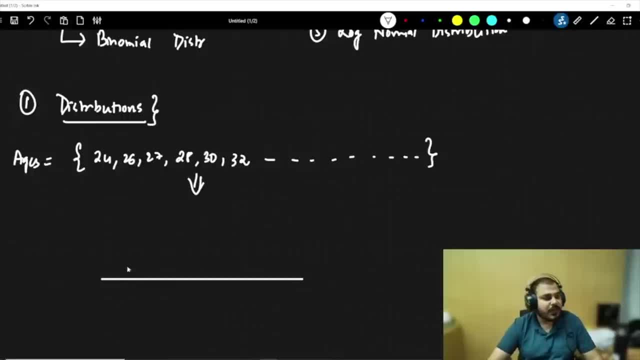 And the best and the easiest way to do that is. let's consider that I want to plot this data through some way, And the easiest way that you can probably think about is your histogram. So we have already seen how to create histograms. you will be able to create diagrams like this: 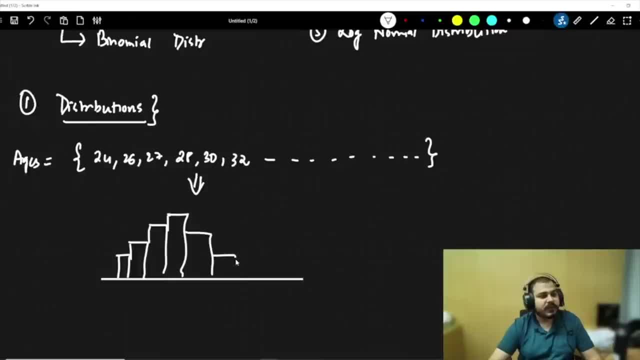 buildings like this. So you will be able to get buildings like this. And finally, what you do? you smoothen this histogram to get some kind of curve, And this curve right now looks like a bell curve. So, considering this, let's go to the first distribution. 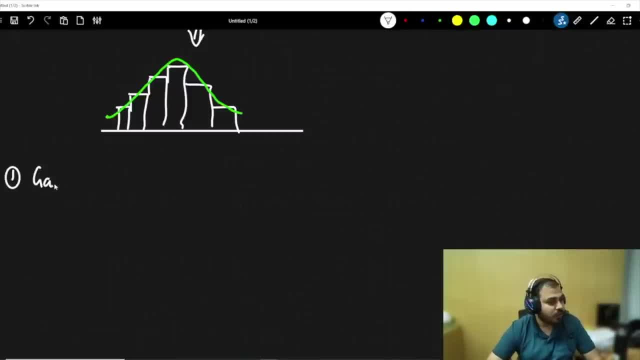 The first distribution that I'd like to focus on is something called a bell curve. This is something called a Gaussian or normal distribution. Now, as I said, why distribution is basically used. Distribution's main purpose is to why these different, different kinds of distributions. 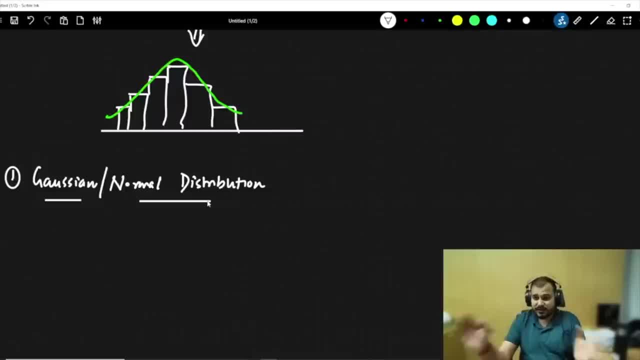 are there So that we can basically have some idea about a data set. Now, first of all, when we discuss about Gaussian or normal distribution, most of the time you have seen this kind of distribution in this specific way, So here probably, you have seen a bell curve. 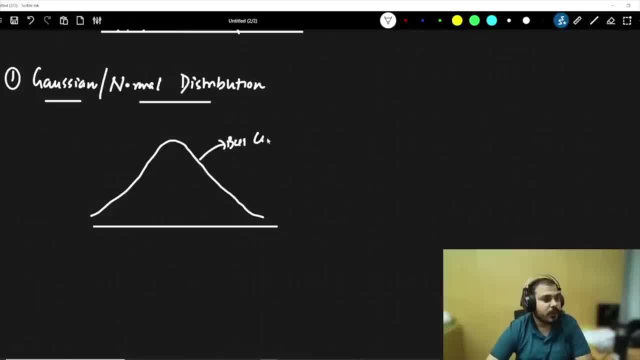 Now this bell curve is a bell curve, This is my bell curve. Now they are very important information. when I probably talk about this bell curve, This will basically: this can be your center line that you see, can be your mean, it can. 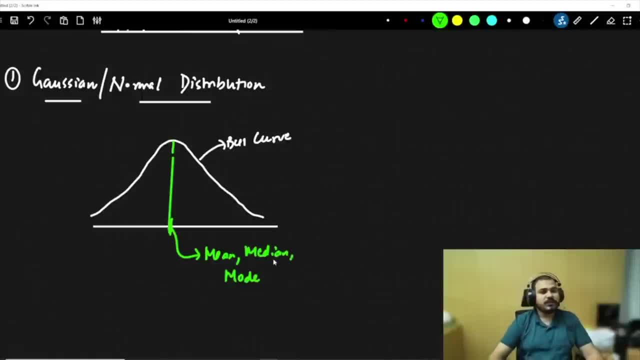 be your median, it can be your mode. So what does this basically mean? If I have a distribution, and probably this distribution follows this kind of bell curve, and one important property of this bell curve is that this side, This side, is exactly symmetrical to this side. 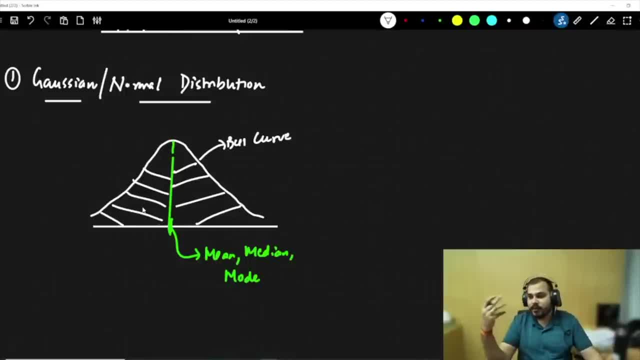 So there are many inferential statistics that we will probably be discussing about in the future, About this bell curve, about this entire distribution or Gaussian distribution. here you can see that it is exactly similar. I mean it is exactly symmetrical. The right part of the curve, when I say consider this particular path, is equal to this part. 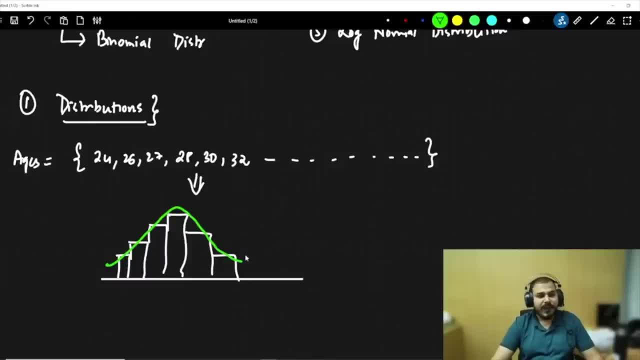 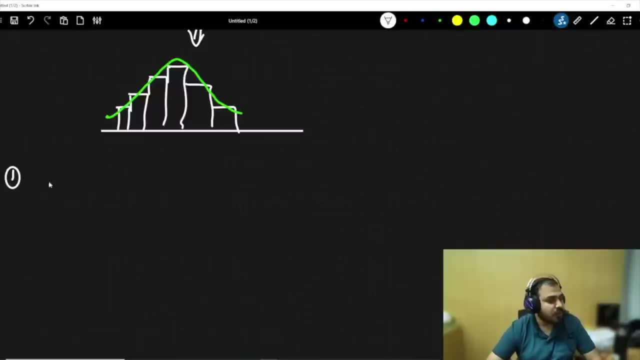 kind of curve, And this curve right now looks like a bell curve. Okay, So, considering this, let's go to the first distribution. The first distribution that I'd like to focus on is something called as Gaussian or normal distribution. Now, why? as I said, why distribution is basically. 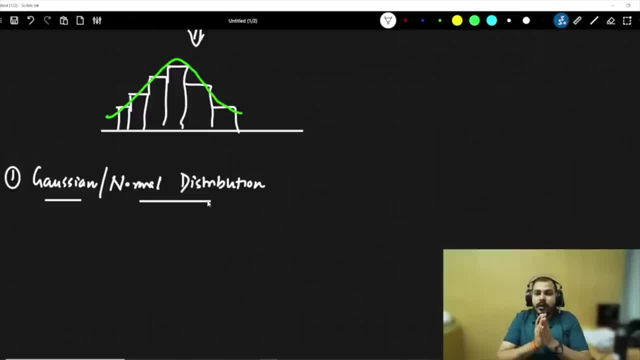 used Distribution. main purpose is to why. why this different, different kinds of distributions are there, So that we can basically have some idea about a data set. Now, first of all, when we discuss about Gaussian or normal distribution, most of the time you have seen this kind of distribution. 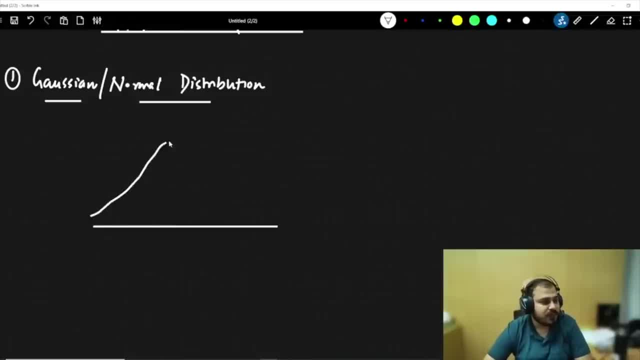 right In this specific way. So here probably you have seen a bell curve. Now this bell curve, this is my bell curve. Now they are very important information. When I probably talk about this bell curve, this will basically: this can be your center line that you see, can be your mean, It can be your. 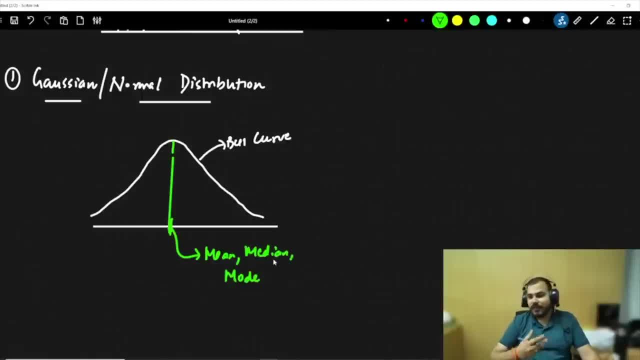 median. It can be a mode. So what does this basically mean? If I have a distribution- and probably this distribution follows this- This kind of bell curve, and one important property of this bell curve is that this side is exactly symmetrical to this side. So there are many inferential statistics that we will probably be 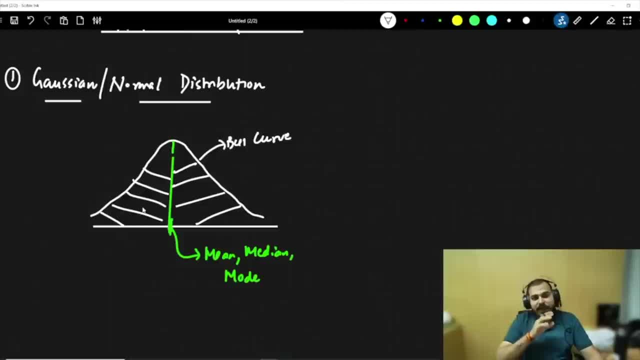 discussing about in the future, about this bell curve, about this entire distribution or Gaussian distribution. Here you can see that it is exactly similar. It is- I mean, it is- exactly symmetrical. The right part of the curve when I say consider this particular particular path is equal to. 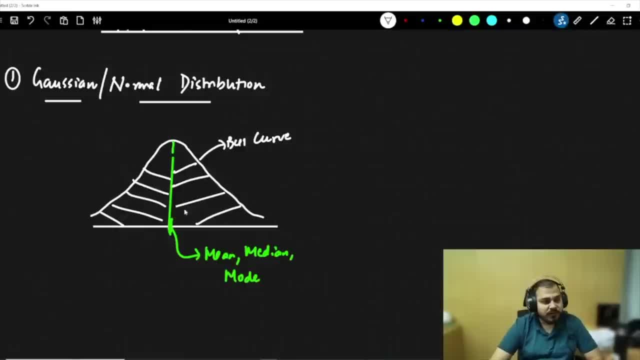 this part. That basically means that the amount of data that is present in this particular part will also be equal to the amount of data that will be basically present in this part. So here you can basically see that exactly this forms a bell curve, And whenever we have a specific distribution, 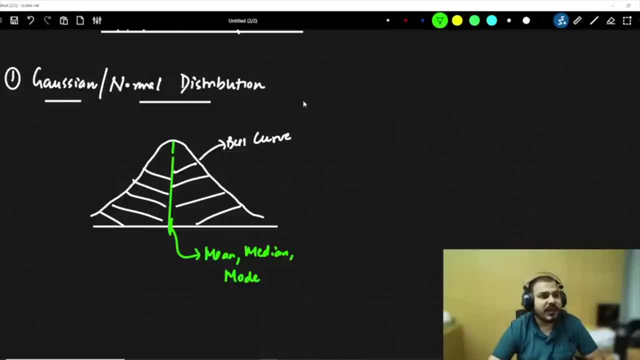 which exactly follows this kind of bell curve. we can definitely say this has a normal or Gaussian distribution. So this is basically my normal distribution. Now why we are specifically focused on this distribution? This distribution is very much important because from this we can derive a lot of conclusions. What are different kinds of conclusions we can derive? 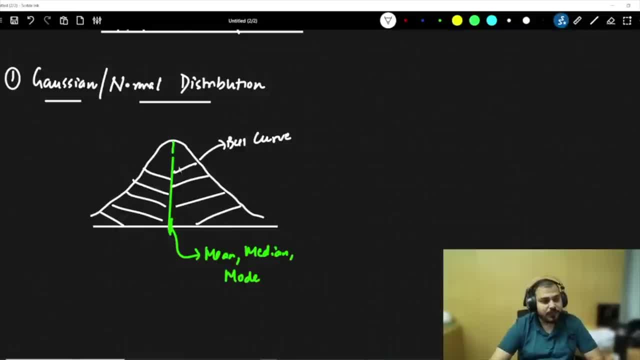 That basically means that the amount of data that is present in this particular path is very similar to the amount of data that is present in this particular part. The amount of data that is present in this particular part is also equal to the amount of data that is present in this particular part. 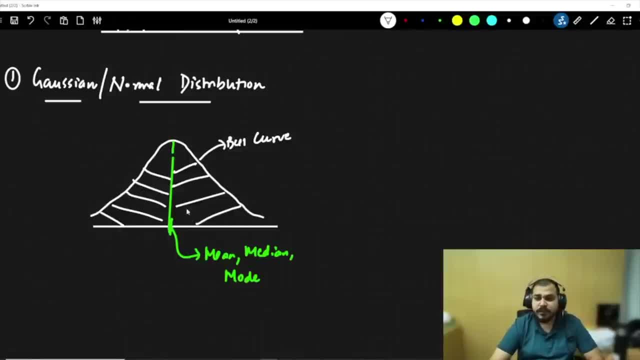 So here you can basically see that exactly this forms a bell curve, And whenever we have a specific distribution which exactly follows this kind of bell curve, we can definitely say that this is a normal or Gaussian distribution. So this is basically my normal distribution. 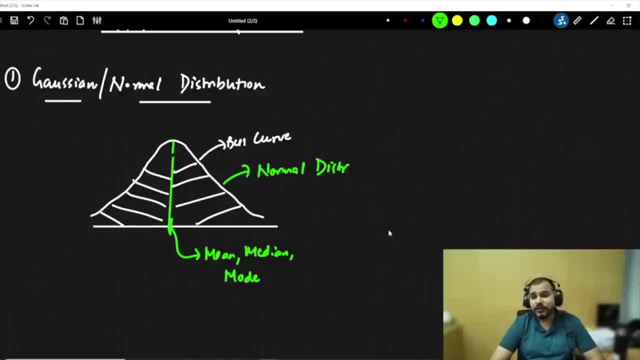 Now why we are specifically focused on this distribution. This distribution is very much important because the value of the distribution is very important. Why? because from this we can derive a lot of conclusions. What all different kind of conclusions we can derive. that I'll just talk about it Now let's go ahead and let's discuss. 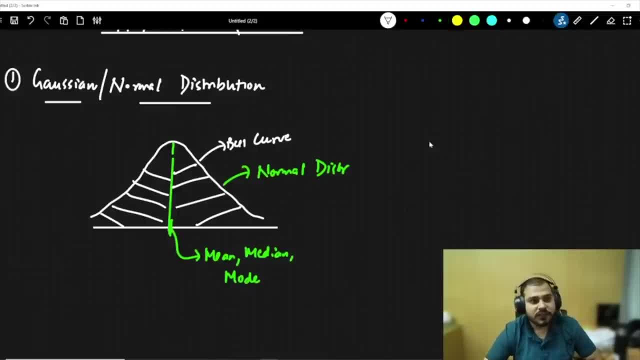 about this distribution, Always understand whenever let's draw this distribution once again. now suppose this is my distribution, so this will be a mean median mode. then you can go one step towards right, second step towards right, first step towards right. So what is this exactly called? 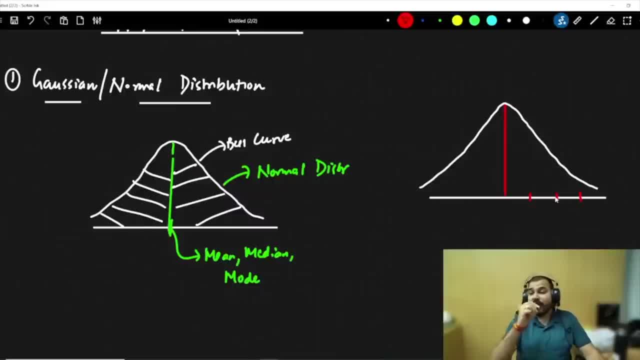 standard deviation. One step towards the right. one step, one step or one standard deviation towards the right. two standard deviation towards the right. three standard deviation towards the right. Similarly, I may have one standard deviation to the left, second standard division to the left and finally, I can also have one more standard deviation to the left. This will be very, very. 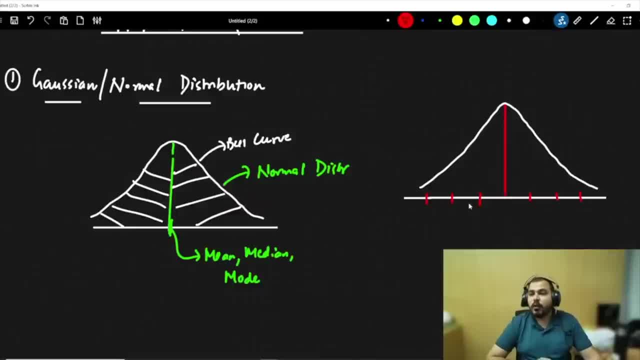 much important guys. Now, what kind of different conclusions or what kind of things we can actually conclude from this kind of graph? This side is symmetry. Now let's go ahead and discuss about some of the important things in this Suppose. if I draw this line, can I say this is my first standard deviation towards the right and second standard deviation towards the left? 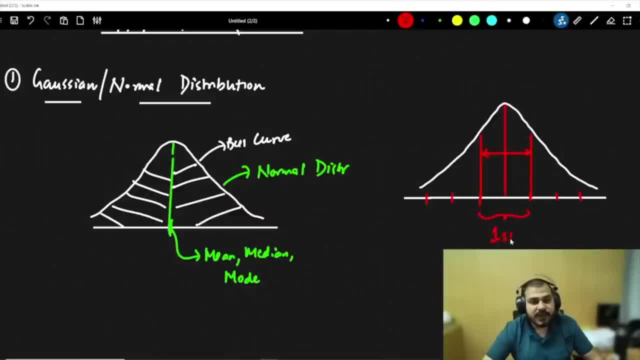 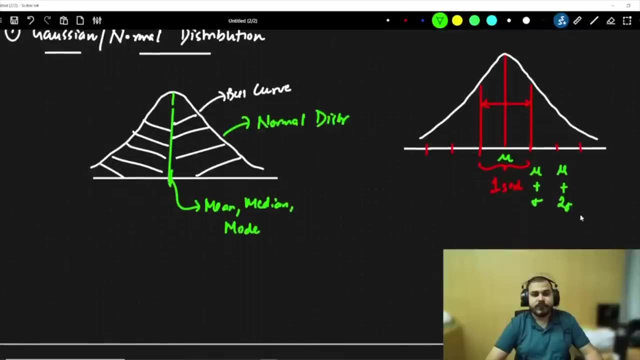 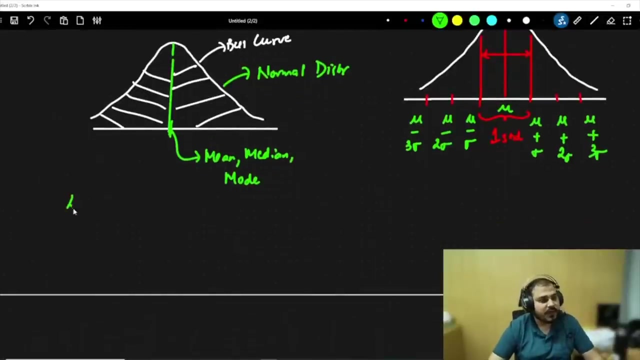 So this is my region of my first standard deviation, The center one over. here I can basically write it as mu. This will basically become mu plus sigma, mu plus two sigma, and this will be mu plus three sigma. Similarly, here I can write mu minus sigma, mu minus two sigma, mu plus mu minus three sigma. Because of less space, I'm just trying to include it in this particular way. Now, the first thing that we will probably come up with is called as empirical formula. Now, this is very much important: Empirical formula. Now, this empirical formula basically says that 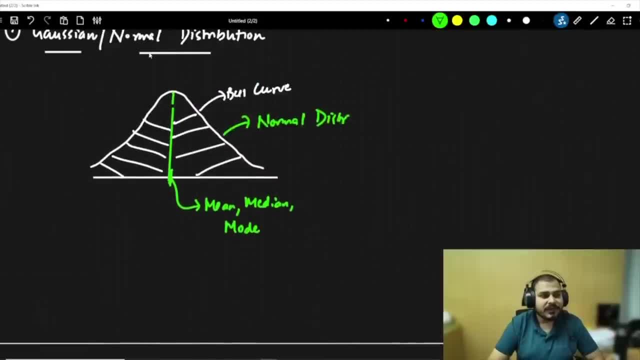 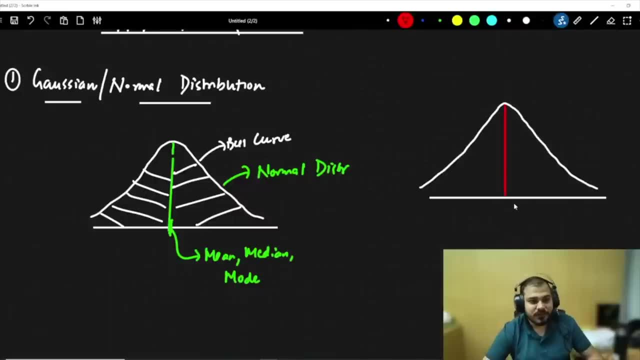 That I'll just talk about it. Now. let's go ahead and let's discuss about this distribution. Always understand whenever let's draw this distribution once again. now suppose this is my distribution, so this will be a mean median mode. Then you can go. 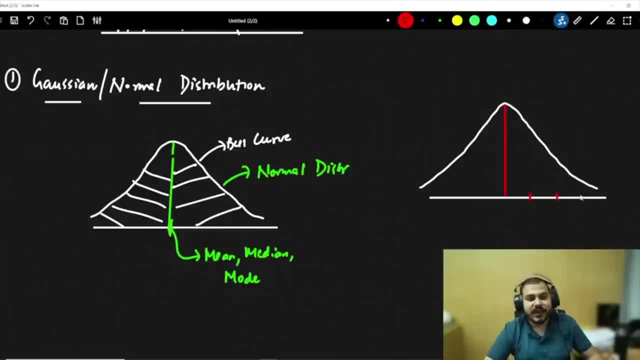 one step towards right, second step towards right, First step towards right. So what is? is this exactly called Standard deviation? One step towards the right, one step. one step or one standard deviation towards the right. two standard deviation towards the right. three: standard deviation towards the right. Similarly, I may have one standard. 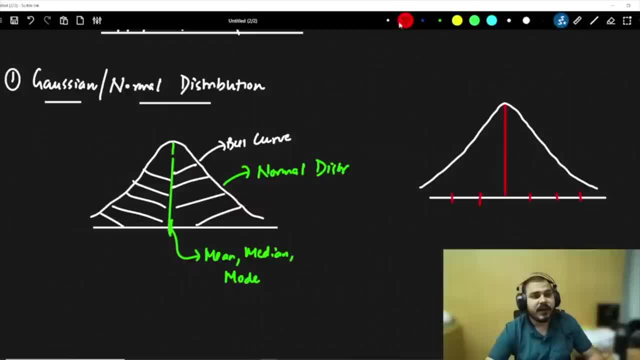 deviation to the left, second standard deviation to the left and finally, I can also have one more standard deviation to the left. This will be very, very much important, guys. Now, what kind of different conclusions or what kind of things we can actually conclude from this kind of graph? This side is symmetrical to this side. Now let's go ahead and discuss. 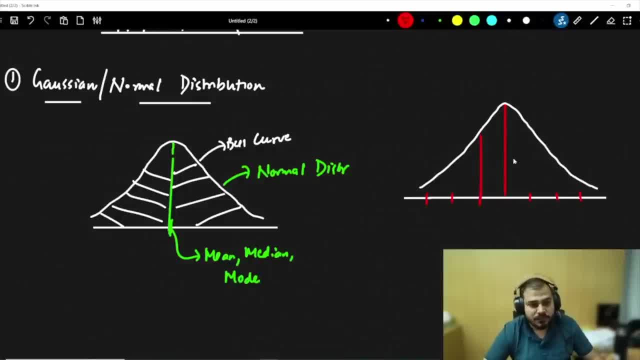 about some of the important things in this Suppose. if I draw this line, can I say this is my first standard deviation towards the right and second standard deviation towards the left. So this is my region of my first standard deviation, The center one over here. 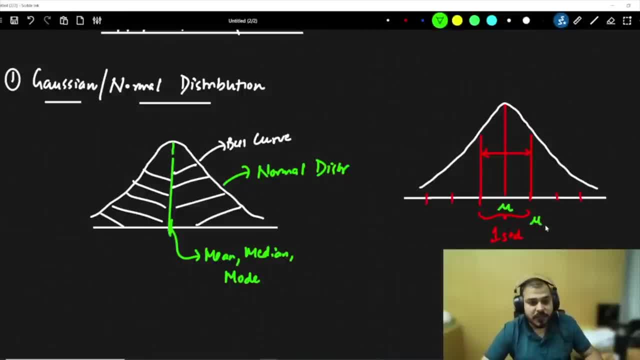 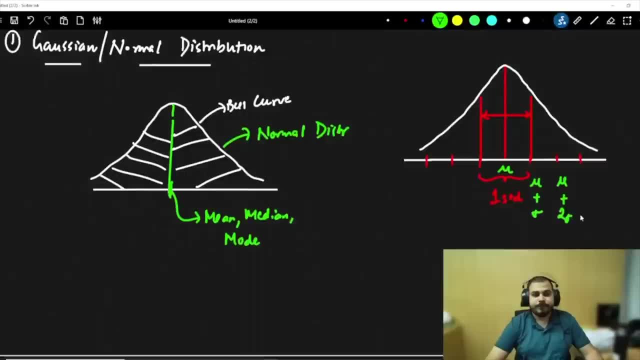 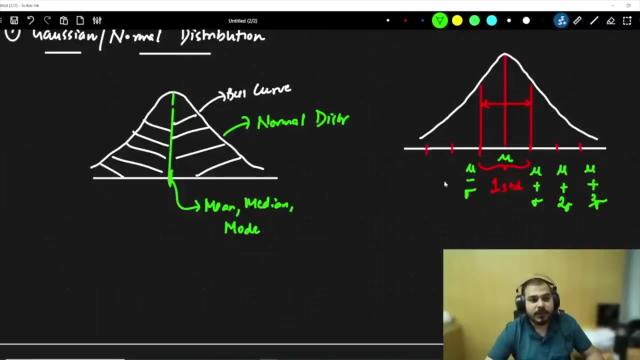 I can basically write it as mu. This will basically become mu plus sigma, mu plus two sigma, and this will be just a second mu plus three sigma. Similarly, here I can write: mu minus sigma, mu minus two sigma. mu plus sorry, mu minus three sigma Because of less. 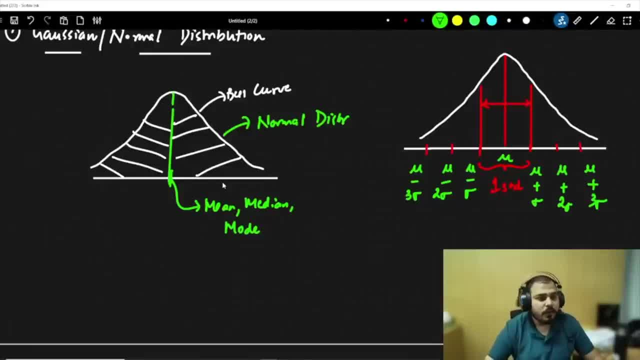 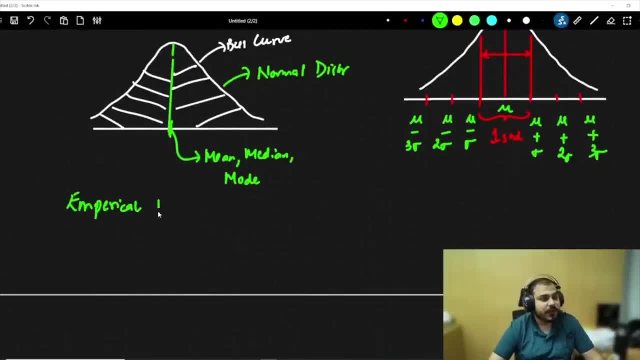 space. I am just trying to include it in this particular way. Now, the first thing that we will probably come up with is called as empirical formula. Now, this is very much important- empirical formula. This empirical formula basically says that you really need to understand this Sixty-eight. 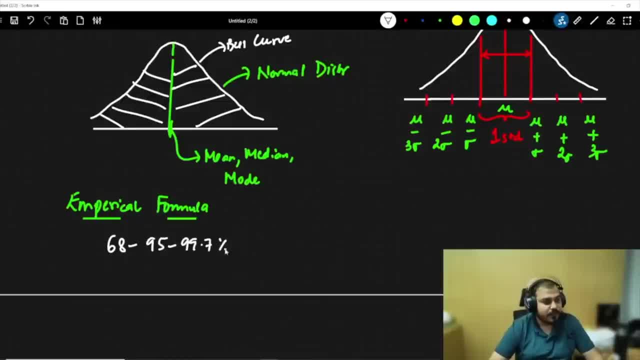 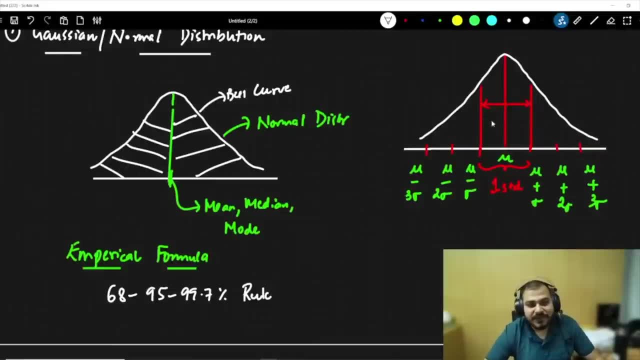 ninety-five, ninety-nine point point seven percentage rule. Now what does this basically mean? This basically indicates that let's go with sixty-eight Within the first standard deviation around, suppose if I have some distribution data. Let's consider that I have a data set. 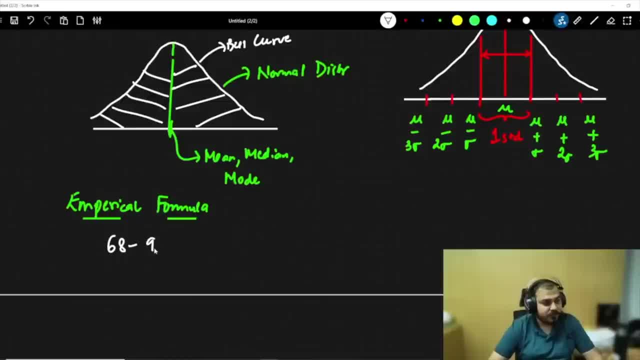 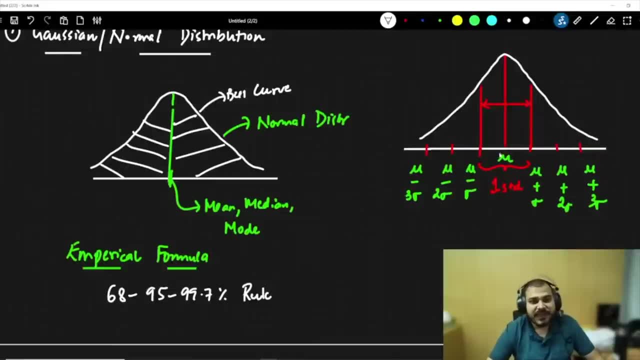 you really need to understand this 68,, 95,, 99.7 percentage rule. Now what does this basically mean? This basically indicates that let's go with 68. Within the first standard deviation around. suppose, if I have some distribution data. Let's consider that I have a data set which have 100 data points. Now what does this basically indicate? is that between the first standard deviation between this. 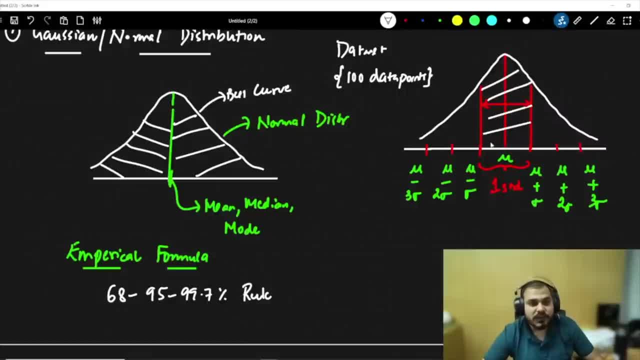 region, in this entire region, around 68 percentage of the distribution is present. That basically means out of this 100 data point, 68 data points will be present in this region. That is the reason it is basically called as a bell cup. That specific region, in that central area, you have a lot of data. So 68 percentage of the entire data set lies in this region, within the first standard deviation. Now coming to the second standard deviation, 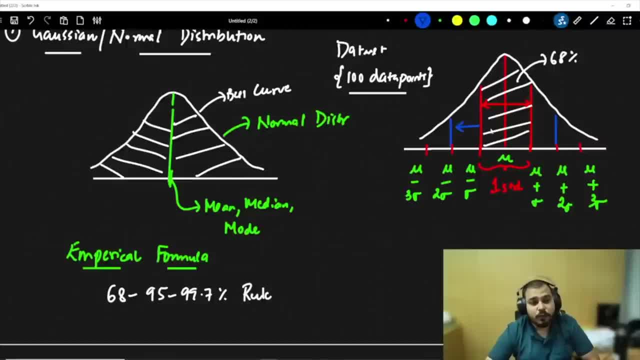 This is something very, very important. I'll also talk about what you can derive from all these things. Between the second standard deviation around, let's come to the 68, percentage is clear. Then, within the second two standard deviation, right within the two standard deviation region, which is this specific region, around 95 percentage of the entire data lies in this region. And similarly, if I go and consider with respect to the third standard deviation, 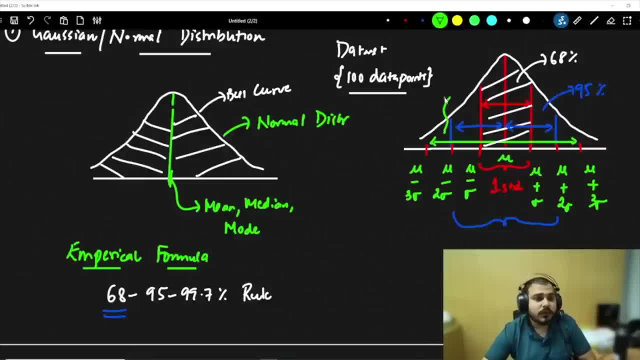 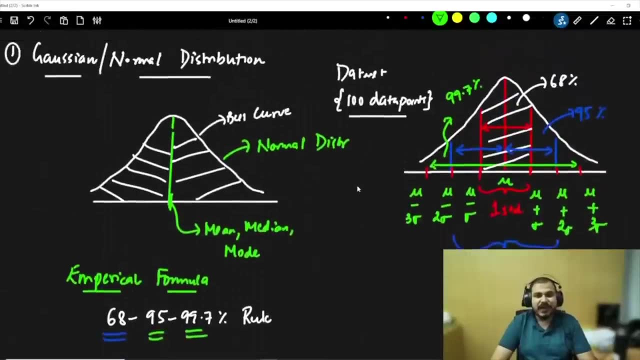 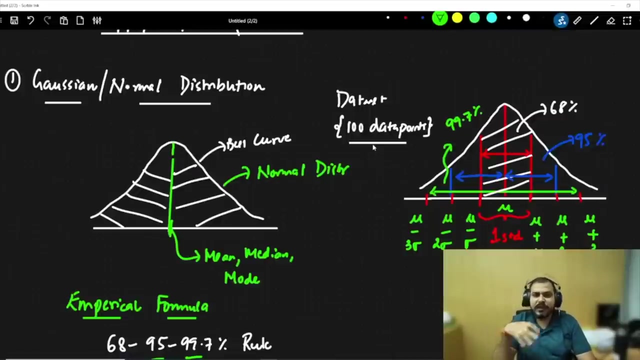 Which is, from here to here, around 99.7 percentage of the entire distribution will fall in this region. So that is the reason why it is basically called as 68, 95 and 99.7 percentile. So everybody is clear. That basically means now, if you have a distribution which is Gaussian or normally distributed, then this conclusion can definitely made that within the first standard deviation. 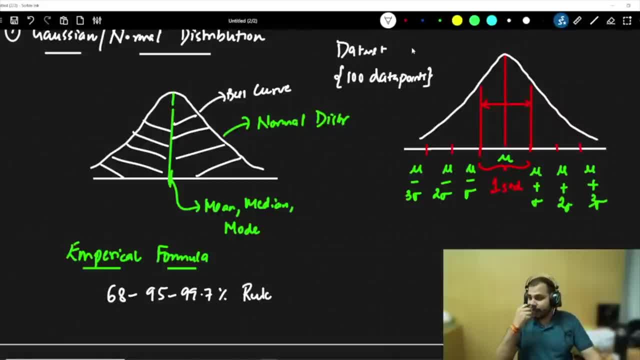 which have hundred data points. Now what does this basically indicate is that, between the first standard deviation and the second standard deviation, the first standard deviation is between this region. in this entire region, around sixty-eight percentage of the distribution is present. That basically means, out of this hundred data point, sixty-eight data points. 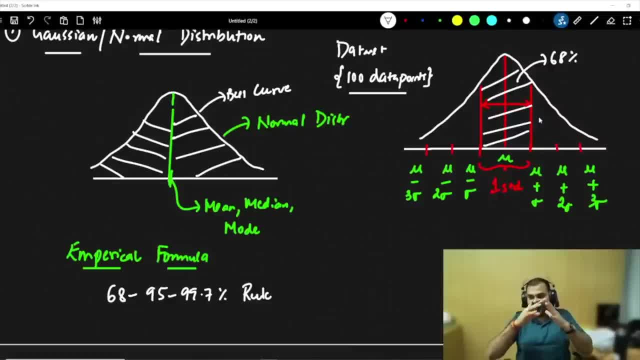 will be present in this region. That is the reason it is basically called as a bell curve, That specific region. in that central area you have lot of data, So sixty-eight percentage of the entire data set lies in this region, within the first standard deviation Now coming. 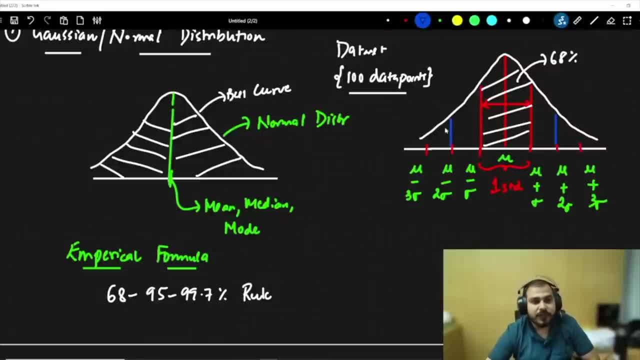 to the second standard deviation. This is something very, very important. I'll also talk about what you can derive from all these things. Between the second standard deviation around, let's come to the sixty-eight percentage. is this clear? then, within the second two, 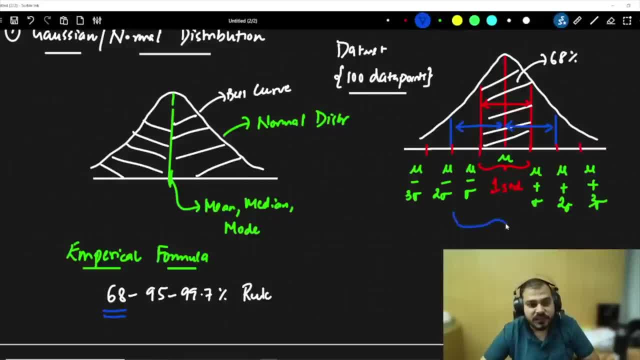 standard deviations right within the two standard deviation region, which is this specific region. around ninety-five percentage of the entire data lies in this region And, similarly, if I go and consider with respect to zero and one or my example right now, it should: 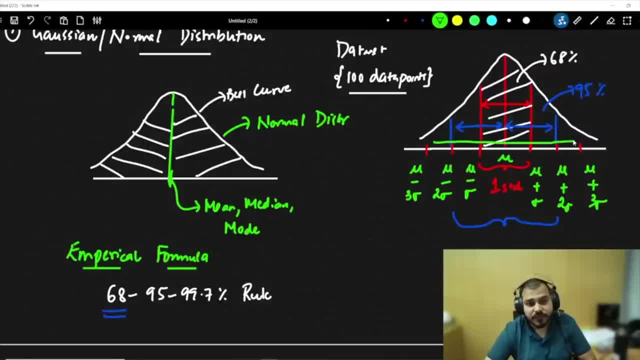 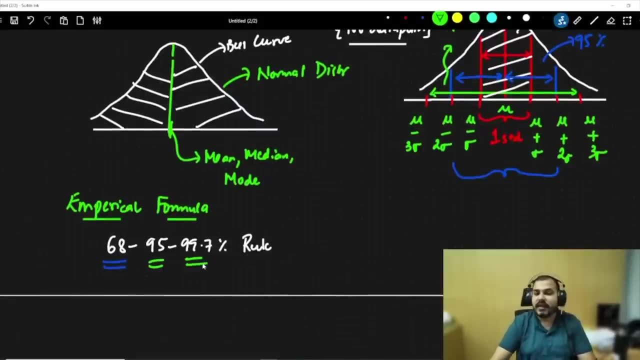 be six hundred eight percentage of the entire data is present in this region. Then now to the third standard deviation, which is from here to here. around 99.7% of the entire distribution will fall in this region. So that is the reason why it is basically called as 68,, 95 and 99.7 percentile lose. 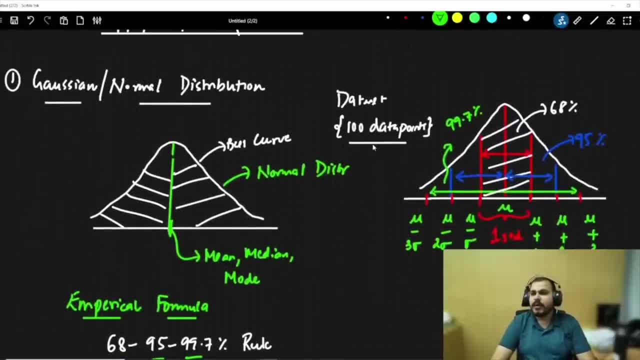 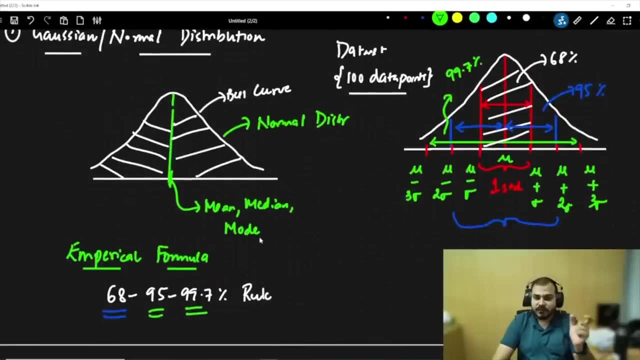 So everybody is clear. That basically means that now, if you have a distribution which is Gaussian or normally distributed, then this conclusion can definitely made that within the first standard deviation, how much data is basically falling. within the second standard deviation, how much data is falling? and within the third standard deviation, how much data is basically falling? 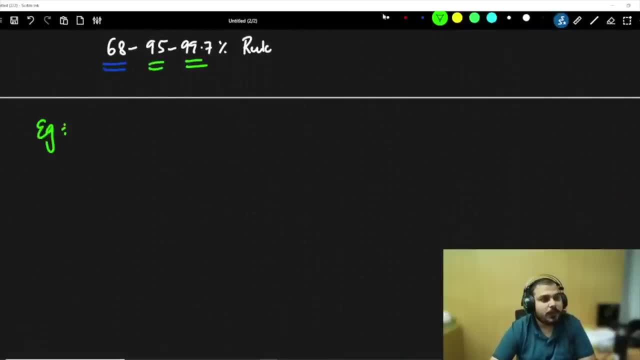 Now let's see some examples, Some of the examples if I talk about, like height. height is basically normally distributed. Who is saying this? I am not saying it. The domain expert is basically saying it. Now, who is the domain expert in this particular case? 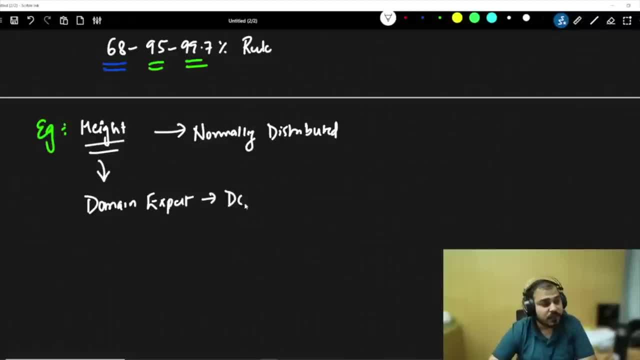 In this particular case, the domain expert is the doctor. Doctor have taken various samples from different, different places and whenever the doctor was constructing this bell curve, it was forming something like this And from that he was able to understand, he was able to derive right. he or she was able. 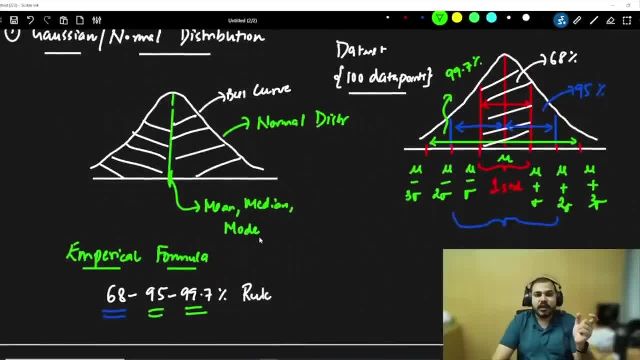 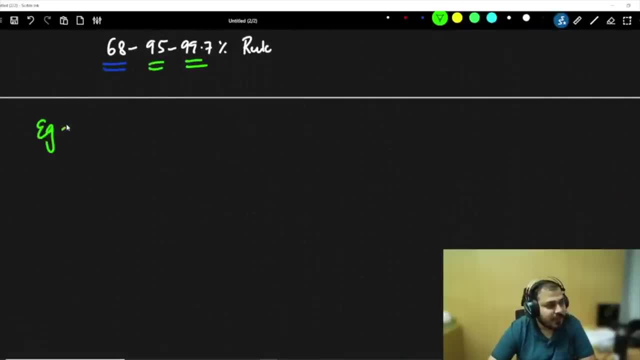 How much data is basically falling. within the second standard deviation, How much data is falling. and within the third standard deviation, How much data is basically falling? Now let's see some examples, Some of the examples. if I talk about like height, Height is basically normally distributed. Who is saying this? I'm not saying it. The domain expert is basically saying it. Now, who is the domain expert in this particular case? In this particular case, the domain expert is the doctor. Doctor have taken various 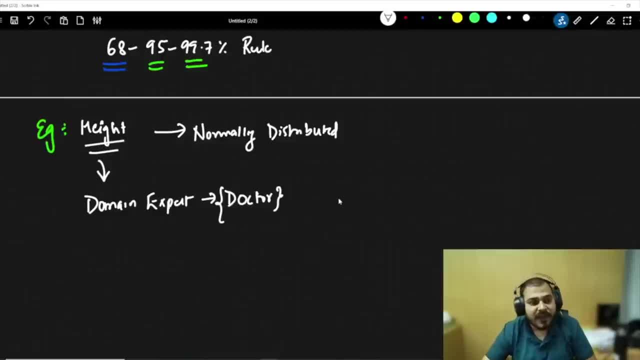 samples from different, different places. and whenever the doctor was constructing this bell curve, it was forming something like this And from that he was able to understand, He was able to derive Right. He or she was able to derive that within the first standard deviation, How much data is basically falling? within the second standard deviation, How much data is falling? and within the third standard deviation, How much data is falling? Second example: if you consider weight, Weight will also follow a Gaussian distribution. Third, I hope everybody knows about this- 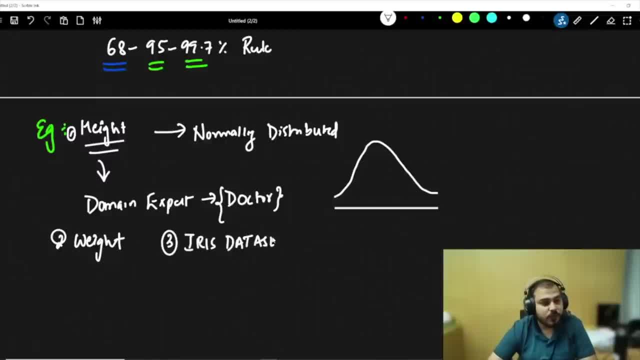 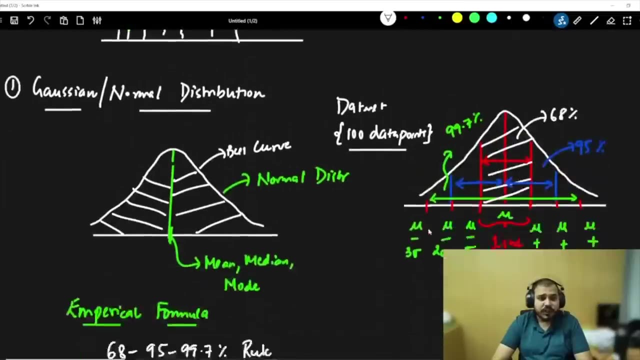 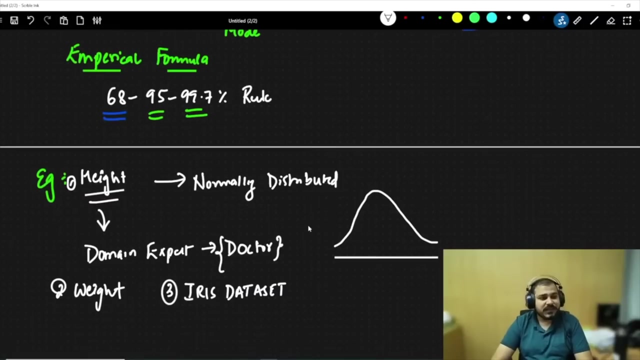 Is this data set In iris data set? if you talk about petal length, sepal length, it actually follows Gaussian distribution. I will show you practically, Don't worry about that. Does that following the empirical rule necessarily imply that it is distributed? See, whenever you have a Gaussian distributed data, at that time it will follow this: 68, 95, 99 point seven percentile. So this was the thing with respect to Gaussian or normally distributed. Now let's go ahead and try to see this. Let's take a look at this. 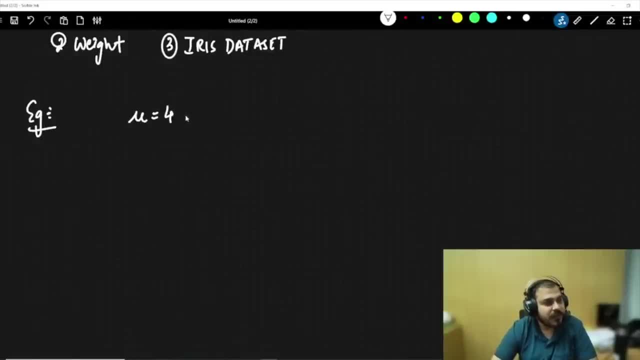 an example. suppose my i have a data set where my mean is 4 and my standard deviation is 1. if i have this two information, can i construct a distribution? suppose this is 4. then in the next step, what it will come? 5, 6, 7, 8, right, and then 3, 2, 1 and 0. so i will be able to create this. and let's 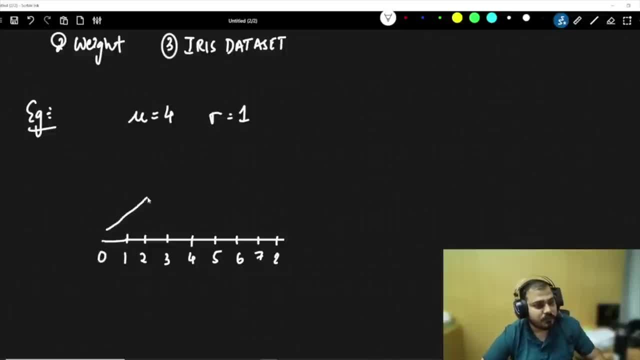 consider that this is basically following this kind of distribution. so this basically follows the this kind of distribution. now understand this middle one is basically your mean and standard deviation. sorry, mean is 4 and standard deviation is 1.. now see one thing, guys, if i talk, 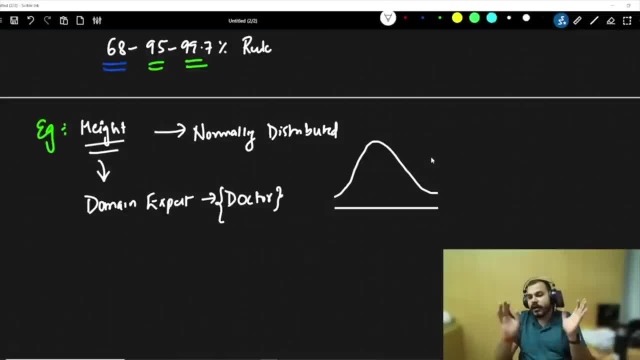 to derive that within the first standard deviation, how much data is basically falling? within the second standard deviation, how much data is falling, and within the third standard deviation, how much data is falling? Second example: If you consider weight, weight will also follow a Gaussian distribution. 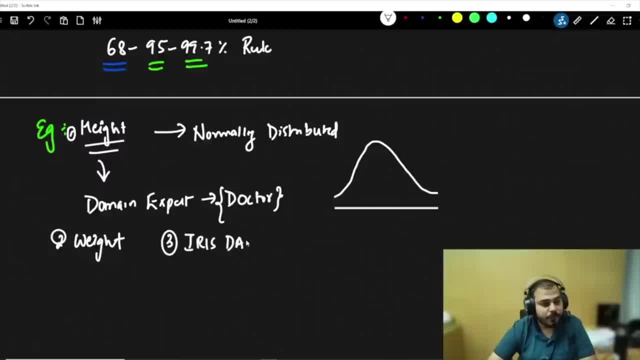 Third, I hope everybody knows about IRIS dataset. In IRIS dataset if you talk about petal length, sepal length, it actually follows Gaussian distribution. I will show you practically don't worry about that. Does that, following the empirical rule, necessarily imply that it is distributed? 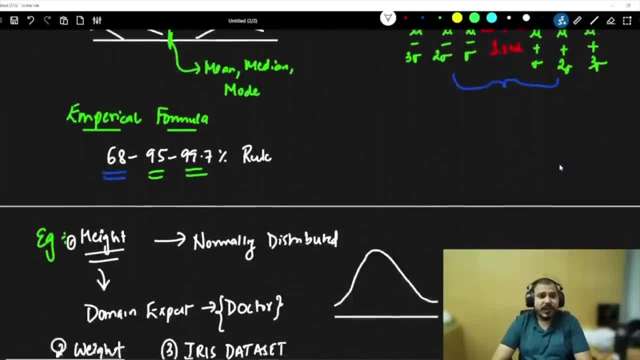 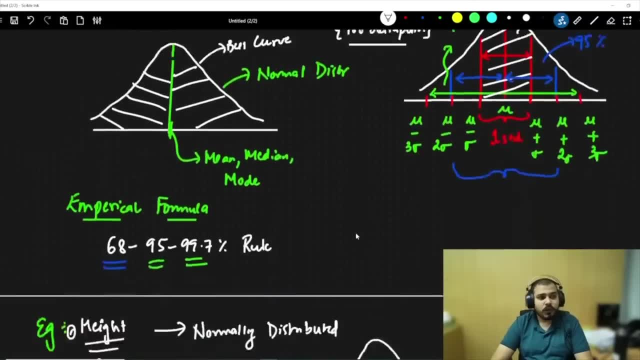 See, whenever you have a Gaussian distributed data, at that time it will follow this 68,, 95,, 99.7 percentile rule. So this was the thing with respect to Gaussian or normally distributed. Now let's go ahead and try to see this. 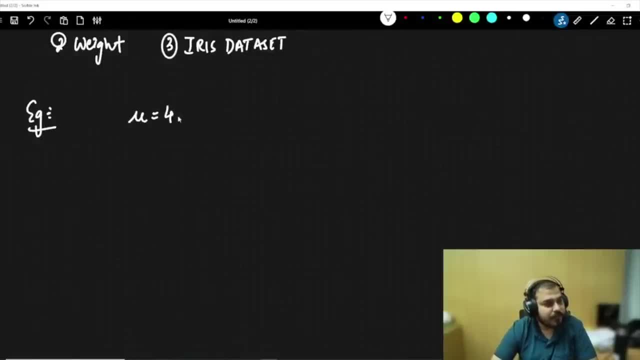 Let's take an example. Suppose my I have a dataset where my mean is 4 and my standard deviation is 1.. If I have this two information, can I construct a distribution? Suppose this is 4, then in the next step, what it will come: 5,, 6,, 7,, 8,, right and then. 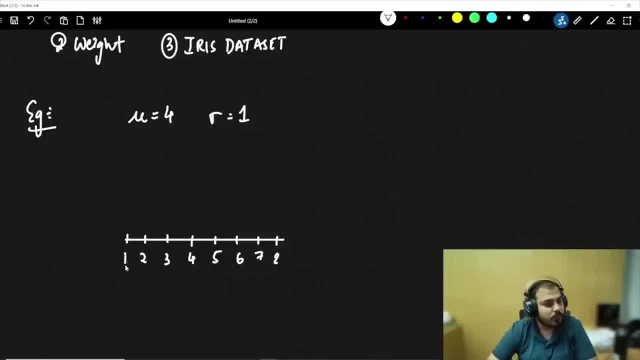 3,, 2,, 1, and 0.. So I will be able to create this And let's consider that this is basically following this kind of distribution. So this basically follows this kind of distribution. Now, understand, this middle one is basically your mean and standard deviation. sorry, mean. 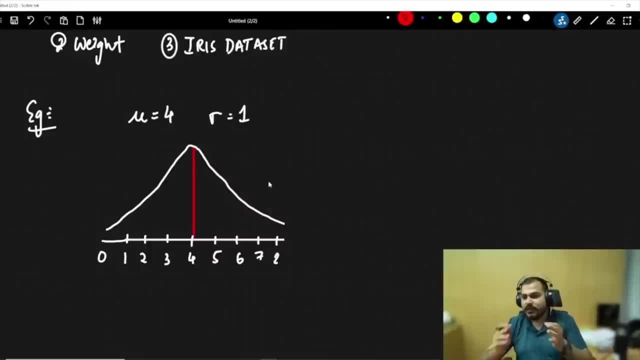 is 4 and standard deviation is 1.. Now see one thing, guys, If I talk about 4.5.. My question is that: where does 4.5 fall? Where does 4.5 fall? Where does 4.5 fall? 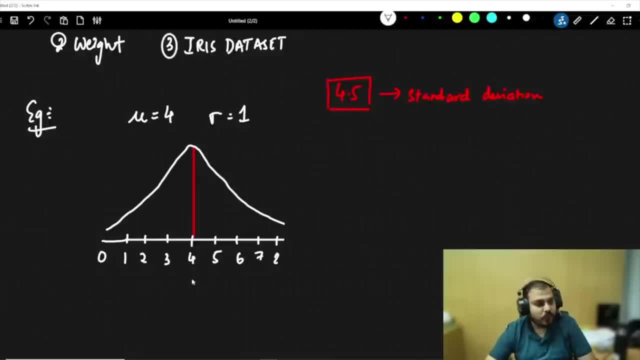 In terms of standard deviation. So you may be thinking: okay, 4.5, where exactly it is? it is somewhere here. Obviously, when I say 5 is first standard deviation to the right, that basically means 4 will be plus 0.5 standard deviation to the right. 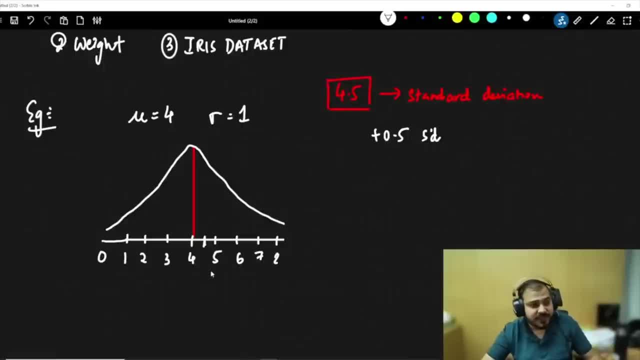 Understand 0.5 standard deviation. if you say 1 standard deviation, it is basically coming to 5. It is 0.5 standard deviation. Now. similarly, if I say where does 4.75 fall, Then how you will be able to see it. 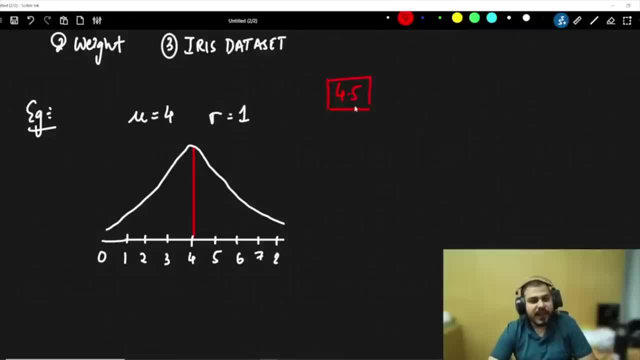 about 4.5. my question is that: where does 4.5 fall in terms of standard deviation? so you may be thinking: okay, 4.5, where exactly it is? it is somewhere here. obviously, when it is 4.5, i say five is first standard deviation to the right. that basically means four will be plus. 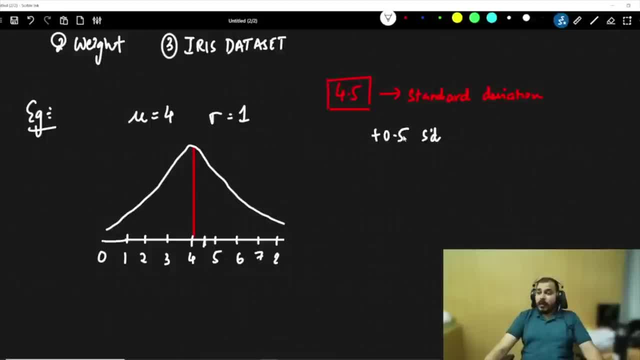 0.5 standard deviation to the right. understand point five standard deviation. if you say one standard deviation, it is basically coming to five. it is point five standard deviation. now, similarly, if i say where does four point seven, five fall, then how you will be able to see it? see point. 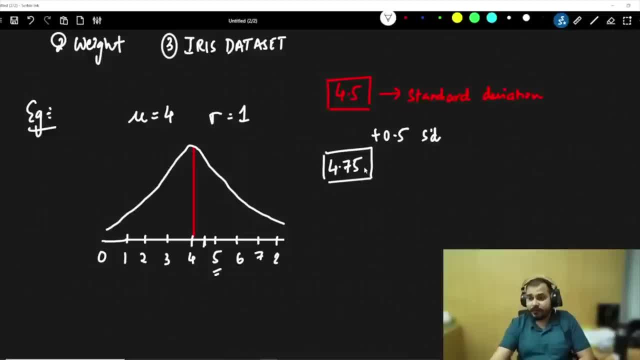 the standard deviation was one. i told four point five. so four point five will be something falling over here, and this is like 0.5 standard deviation. But in the case of 4.75, it will be very much difficult for you to do the calculation. So that is the reason. what we can do is that we 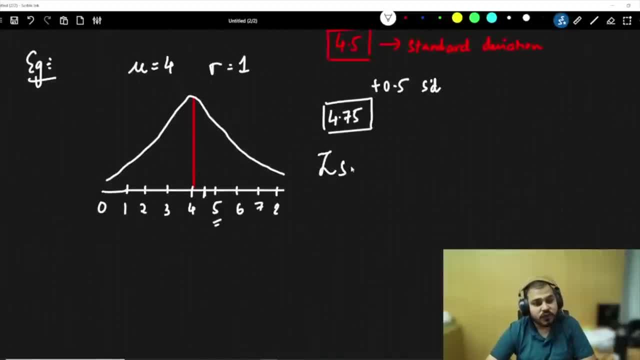 can use a concept which is called as Z-score. Now Z-score will basically help you find out, whenever I talk about a value, how much standard deviation away it is from the mean. So this formula is x of i minus mu divided by standard deviation. Now I need to find out for 4.75.. I will 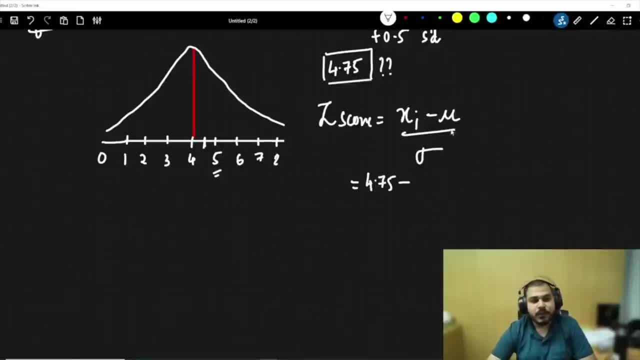 just write: 4.75 minus mu is what Mu is: 4.. 4 divided by standard deviation is 1.. So here I am actually getting 0.75.. So now I can see that it is 0.75 standard deviation to the right. Why it is. 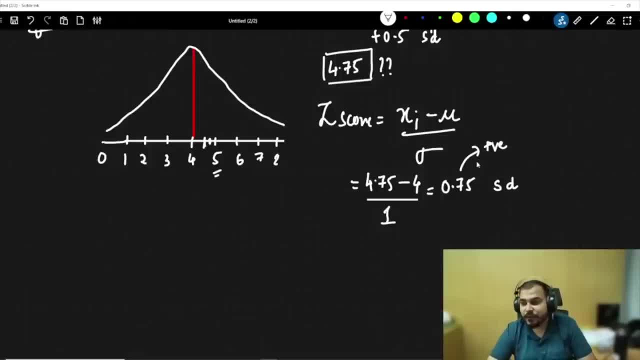 saying right, Because this is positive value. Now, if I give you the same question: try to find out where does 3.75 fall? Like how many standard deviation, whether what should be the standard deviation with respect to 3.75? Then you go and apply the same formula. So here I will. 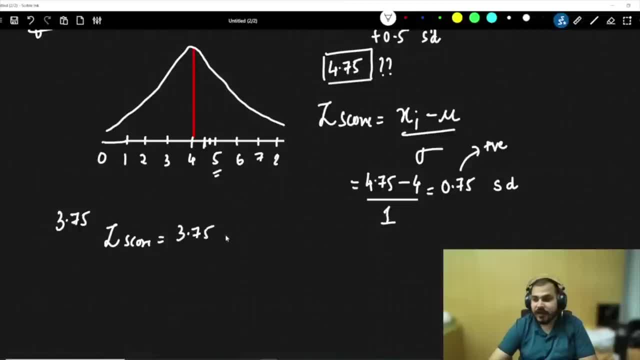 say, Z-score is equal to 3.75 minus 4 divided by 1,, which is nothing but minus 0.25.. So whenever minus comes, that basically means you have to check in this sign And it is basically saying that 3.75 is equal to 3.75 minus 4 divided by 1, which is nothing but minus 0.25.. So whenever 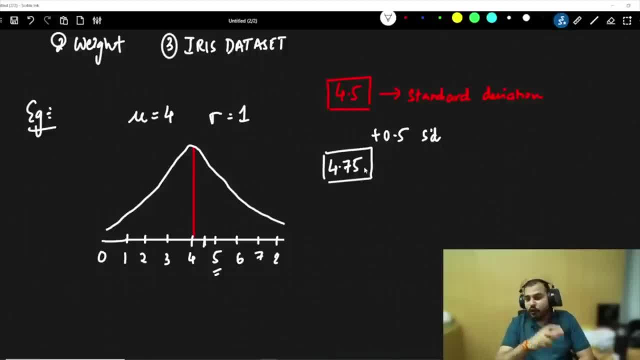 See point. the standard deviation was 1.. I told 4.5. So 4.5 will be something falling over here and this is like 0.5 standard deviation. But in the case of 4.75, it will be very much difficult for you to do the calculation. 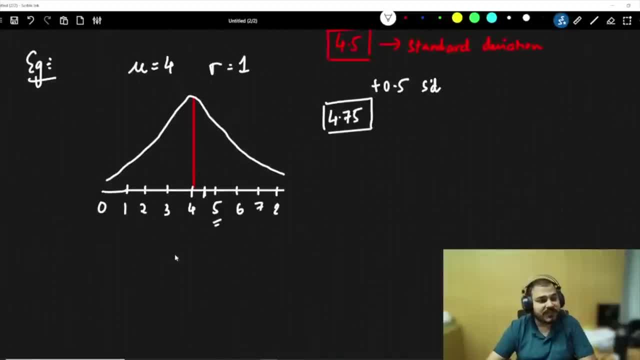 So that is the reason. what we can do is that we can use a concept which is called as Z-score. Now, Z-score will basically help you find out, whenever I talk about a value, how much standard deviation away it is from the mean. So this formula is x of i minus mu divided by standard deviation. 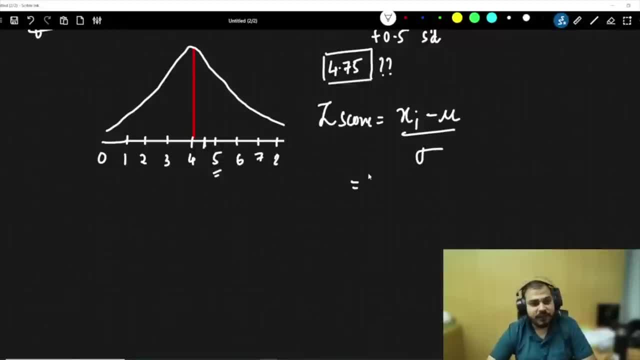 Now I need to find out for 4.75.. I will just write: 4.75 minus mu is what Mu is, 4.. 4 divided by standard deviation is 1.. So here I am actually getting 0.75.. 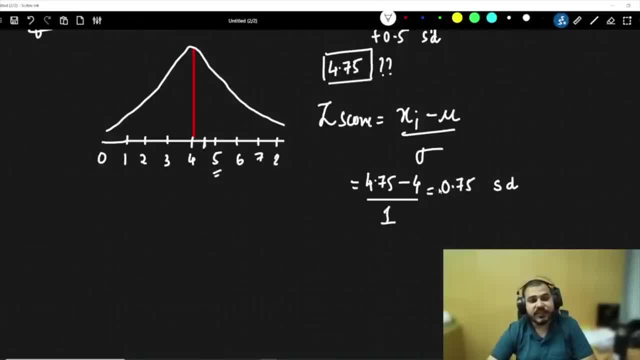 So now I can see that it is 0.75 standard deviation to the right. Why it is saying right? Because this is positive value. Now, if I give you the same question, try to find out. where does 3.75 fall? 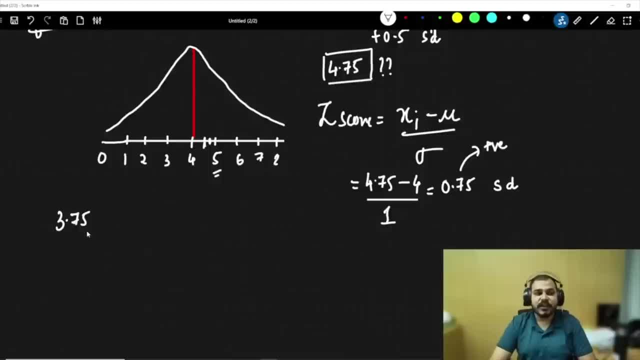 Like: how many standard deviation, whether what should be the standard deviation with respect to 3.75.. Then you go and apply the same formula. So here I will say: Z-score is equal to 3.75 minus 4 divided by 1, which is nothing but. 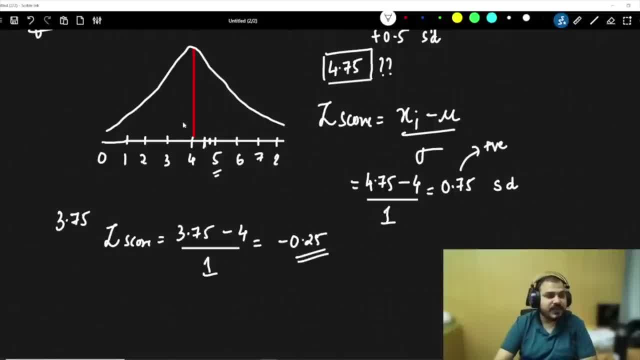 minus 0.25.. So whenever minus comes, that basically means 0.75.. So that is the standard deviation. That means you have to check in this sign And it is basically saying that 3.75 will be falling somewhere here. 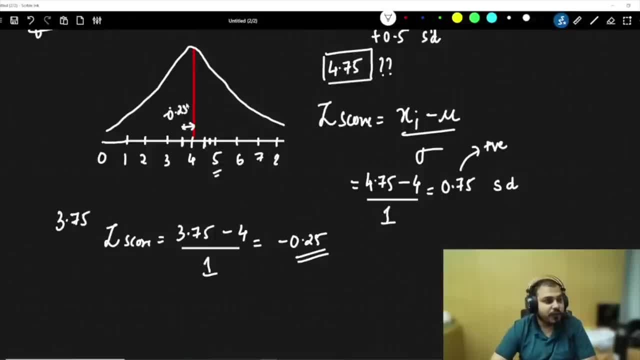 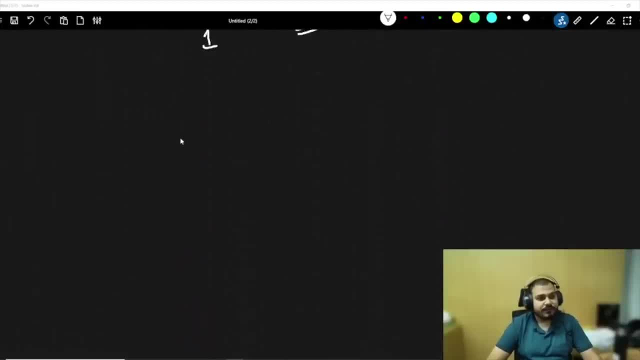 That is nothing but minus 2 point 0.25 standard deviation to the left. Now let's go to the next thing. Suppose I consider this same graph. Now you understood If I really want to find out how many standard deviation to the right or the left I need. 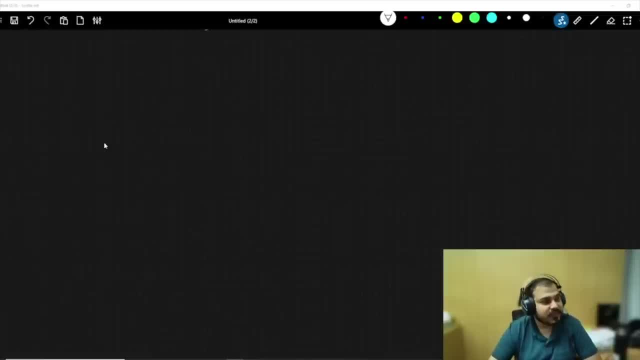 to find out. I can definitely use Z-score. Let's consider this thing. I will use the same graph. I am using the same bell curve. This is my 4.. This is my 5.. This is my 6.. This is my 3.. 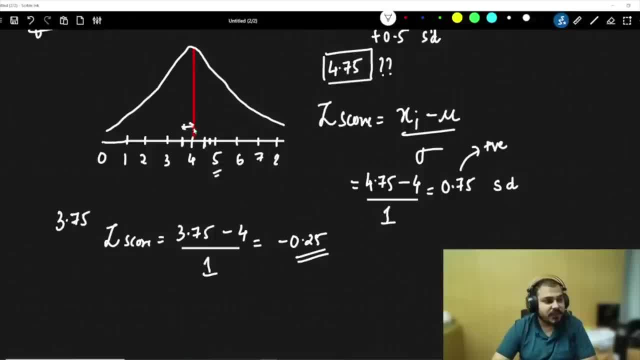 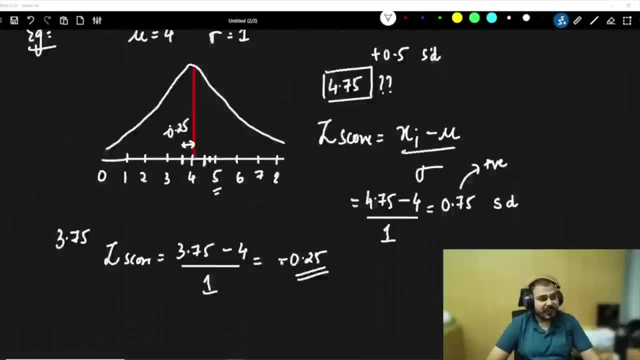 minus comes. that basically means you have to check in this sign And it is basically saying that 3.75 will be falling somewhere here. That is nothing but minus 2 point 0.25 standard deviation to the left. Now let us go to the next thing. Suppose I consider this same graph. Now you understood. 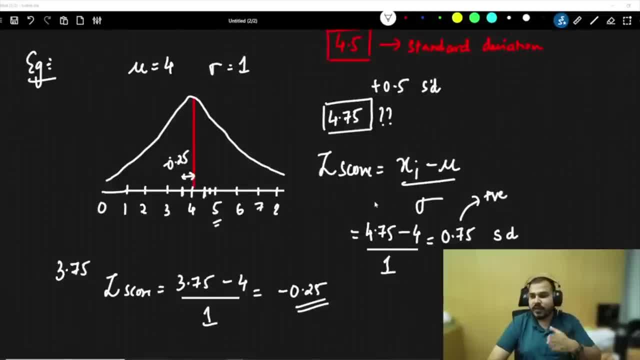 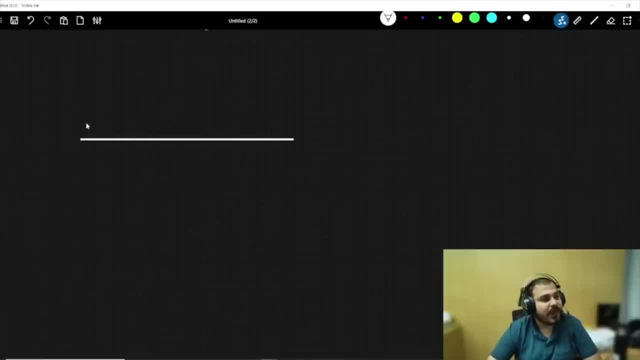 If I really want to find out how many standard deviation to the right or the left I need to find out, I can definitely use Z-score. Let us consider this thing. I will use the same graph. I am using the same bell curve. This is my 4.. This is my 5.. This is my 6.. 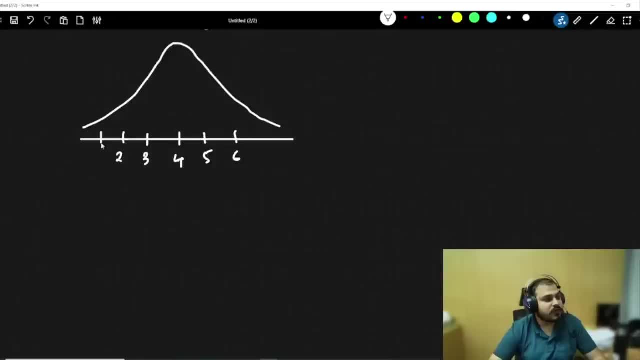 This is my 3.. This is my 2.. This is my 1.. Here you know that my mean is 4 and standard deviation is 1.. Understand one thing over here. I will talk about Z-score again. Don't worry, Now let us apply Z-score. 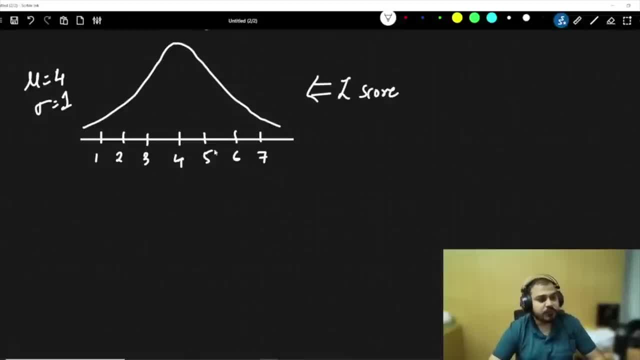 to every values. What will happen If I apply Z-score to every values? what will happen? What is Z-score? formula X minus mu divided by standard deviation? Okay, when I apply Z-score to every values, What will happen? Okay, What will happen in this case? 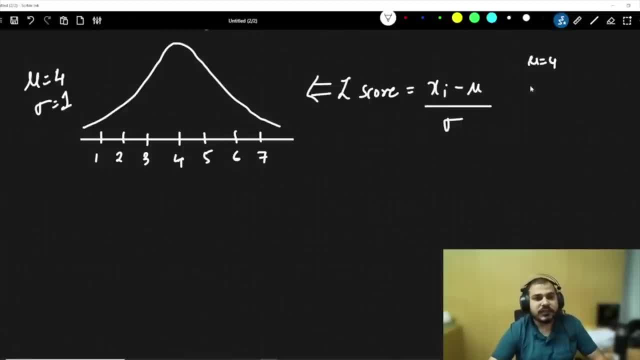 okay, you know. the mean mean is nothing but 4, standard deviation is 1. now, if i apply z score to everything, initially my distribution was like this: 1, 2, 3, 4, 5, 6, 7. now, this was my distribution initially. now, after applying z score to this, what will be my distribution that will be coming? 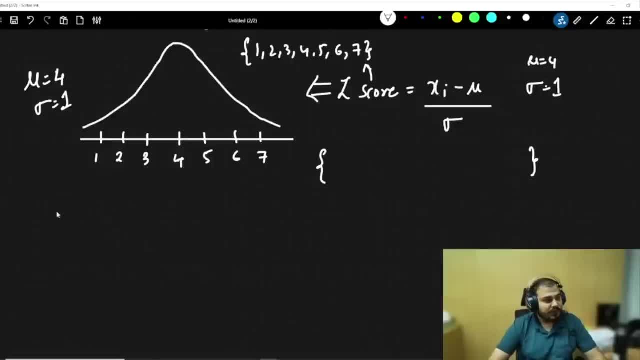 apply. apply for 1 first of all. so if i apply z score to 1, then what will happen? 1 minus 4 divided by 1, this is minus 3. can i say this? 1 is getting converted to minus 3. 1 is converted. 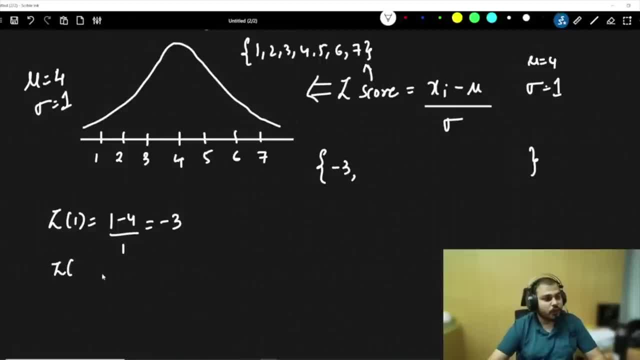 to minus 3. then if i apply this z to the next element, 2, then what is 2 minus 4? my 1? it is nothing but minus 2. so here i am actually getting minus 2. then if i go and apply the z score to 3, 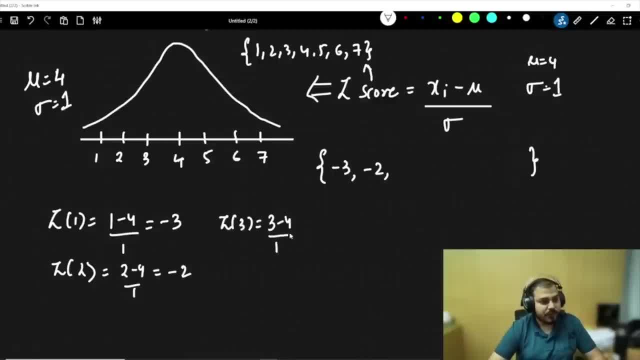 then what will happen? z of 3, so 3 minus 4, divided by 1? what will happen? minus 1, so minus 3, will now get converted to minus 1. then 4 will get converted to 0. then it will get converted to 1, 2, 3. now understand the main magic in this, with the help of z score. 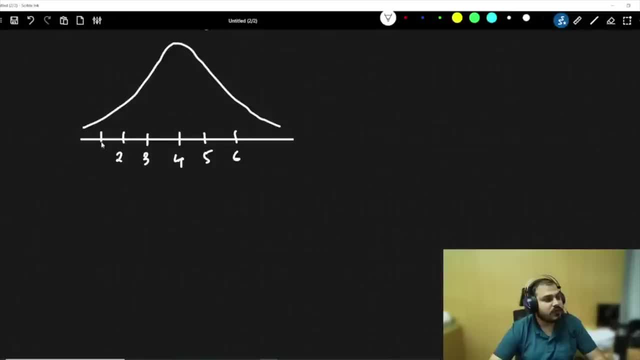 This is my 2.. This is my 1.. Here, you know that my mean is 4 and standard deviation is 1.. Understand one thing over here. I will talk about Z-score again, Don't worry. Now let's apply Z-score to every values. 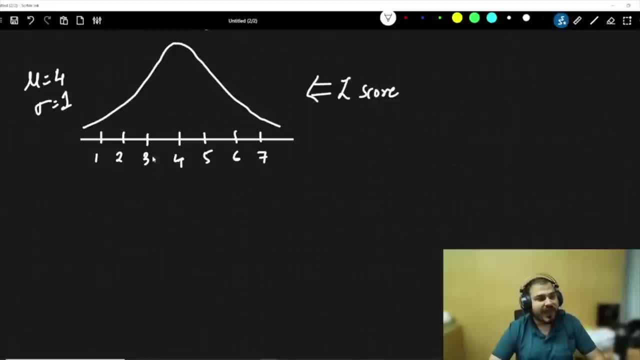 What will happen If I apply Z-score to every values? what will happen? What is Z-score formula? Let's see X of I minus mu divided by standard deviation. You know, the mean Mean is nothing but 4, standard deviation is 1.. 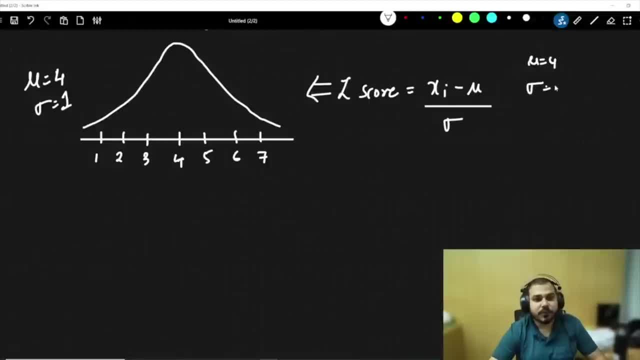 Now, if I apply Z-score to everything, initially my distribution was like this: 1, 2, 3,, 4,, 5, 6, 7.. Now, this was my distribution initially. Now, after applying Z-score to this, what will be my distribution? 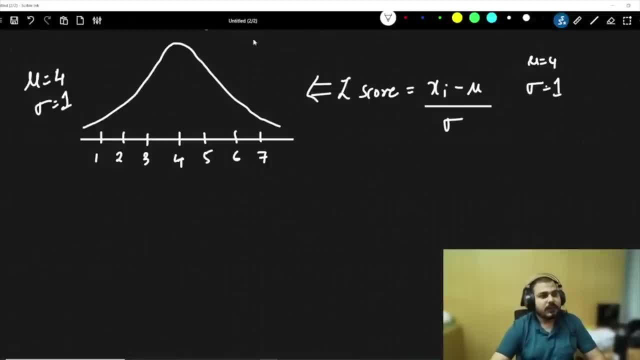 That will be coming. Apply for 1 first of all. So if I apply Z-score to 1, that will be coming. I will apply Z-score to 2.. That will be coming. I will apply Z-score to 1.. 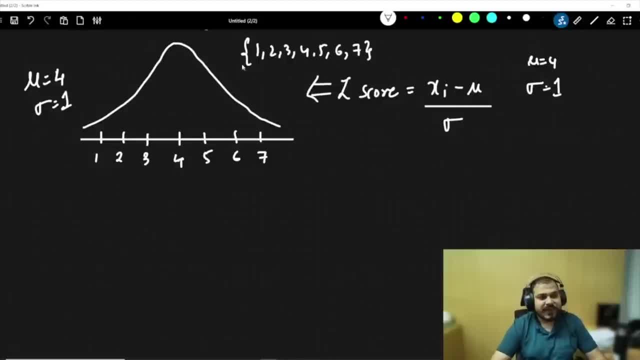 Now, what will happen? Now, I have applied Z-score to 1.. I am applying Z-score to 2.. So what will happen? I am applying Z-score to 1.. Now, after applying z-score to this, what will be my distribution That will be coming Apply. 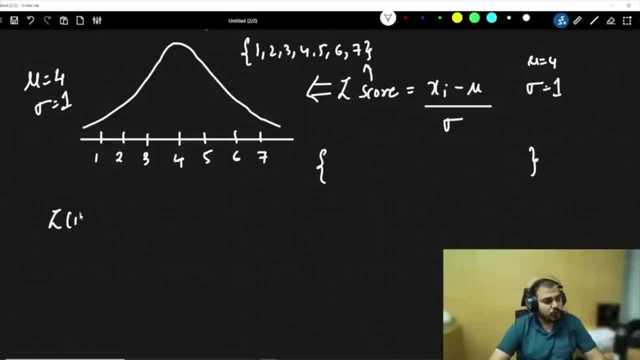 Apply for 1 first of all. So if I apply z-score to 1, then what will happen? 1 minus 4 divided by 1. This is minus 3.. Can I say this: 1 is getting converted to minus 3?. 1 is converted to minus 3.. 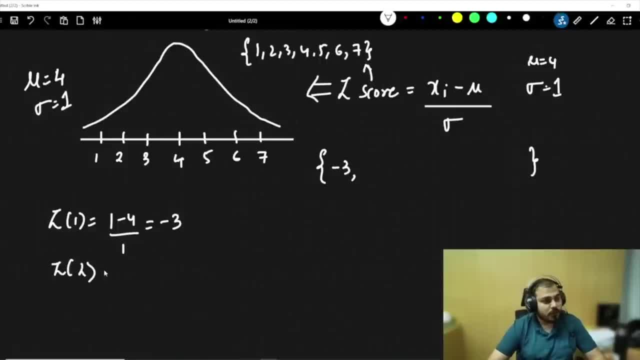 Then if I apply this z to the next element, 2,, then what is 2 minus 4 by 1? It is nothing but minus 2.. So here I am actually getting minus 2.. Then if I go and apply the z-score to 3,, 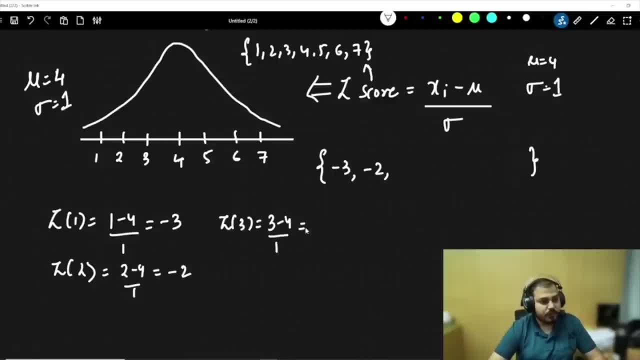 then what will happen? z of 3.. So 3 minus 4 divided by 1.. What will happen? Minus 1.. So minus 3 will now get converted to minus 1.. Then 4 will get converted to 0.. Then it will get converted to 1,. 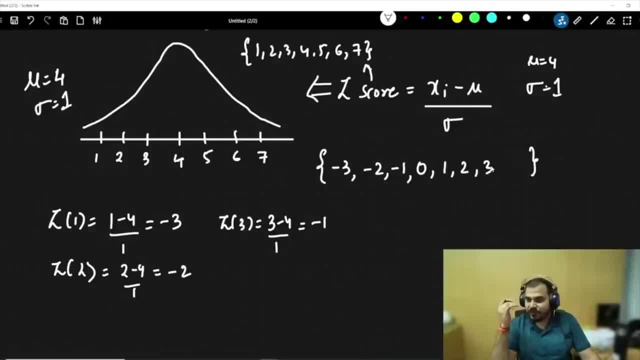 2, 3.. Now understand the main magic in this With the help of z-score. is this not the standard deviation of the same elements that we got over here? Is this not the standard deviation of these elements That we got after applying the z-score? After we applied this initially, my data set was like: 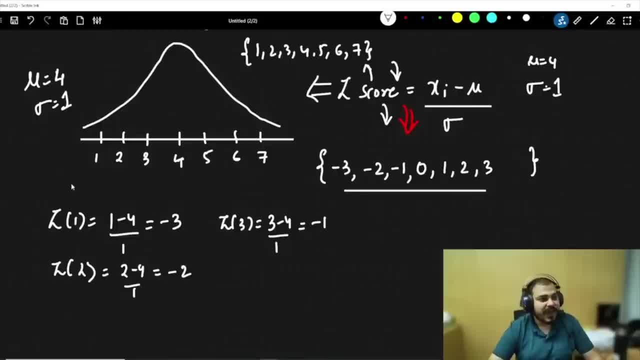 this. Then I got this. This element falls at minus 3 standard deviation. This element falls at minus 2 standard deviation. So here you can definitely see that I am able to get the standard deviation. Now what is happening? See over here One beautiful thing that is basically happening. 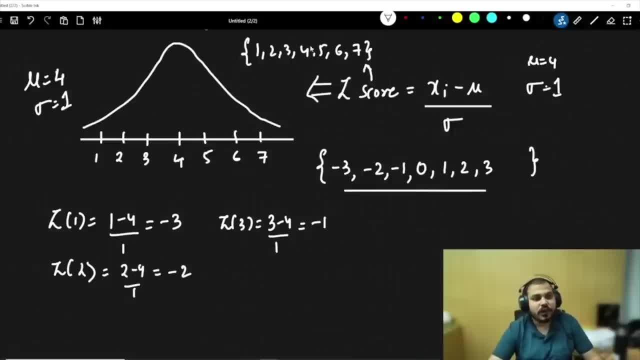 is this not the standard deviation of the same elements that we got over here? is this not the standard deviation of this? all elements that we got after applying the z score? after we applied this initially, my data set was like this. then i got this. this element falls at: 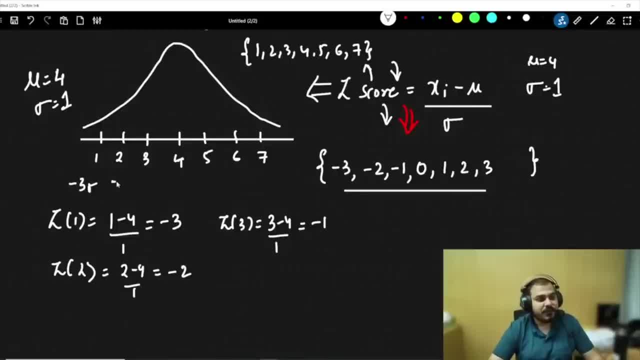 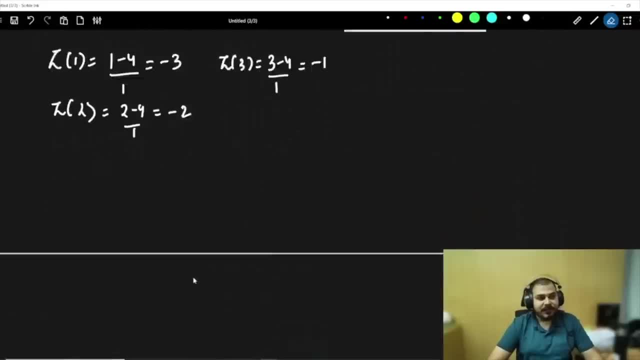 minus 3 standard deviation. this elements fall at minus 2 standard deviation. so here you can definitely see that i am able to get the standard deviation. now what is happening? see over here one beautiful thing that is basically happening. i had a distribution which was 1, 2, 3, 4, 5, 6, 7. after i applied a z score, this got converted to minus 3 minus 2, minus 1, 0, 1, 2, 3. 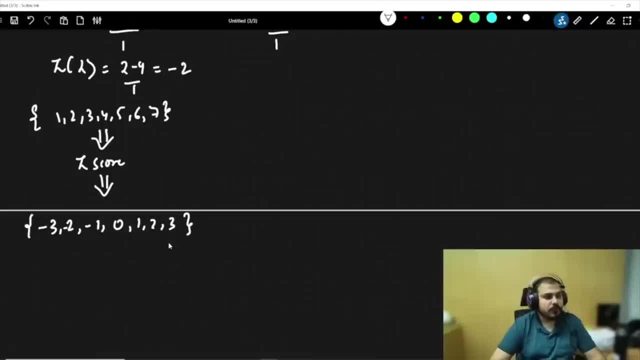 and probably: uh, yeah, right, i got this. now what is this distribution then called? what this was initially a normal distribution, a normal distribution or a gaussian distribution? after i applied a z score? what kind of distribution we are actually getting, and what is this basic distribution called as? so this distribution? 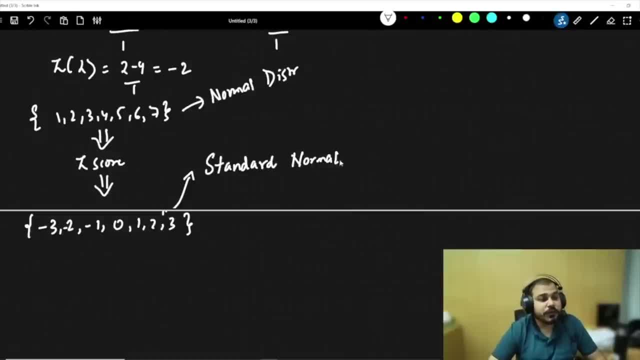 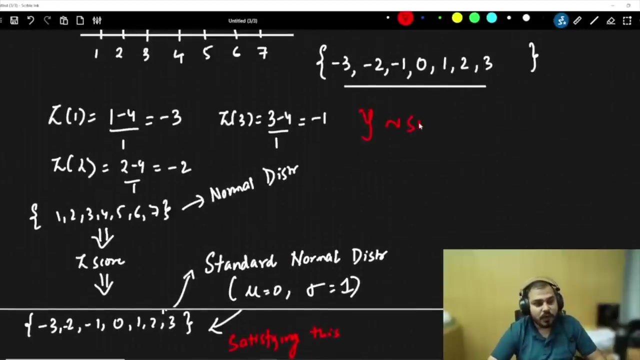 is called as standard normal distribution. so one of the most important property with respect to standard normal distribution is that your mean and your average mean and your average mean and your standard deviation is zero and standard deviation is one. is this satisfying this property or not? it is being satisfied, right. so can i write? can i write a random variable? x or y will belong to. 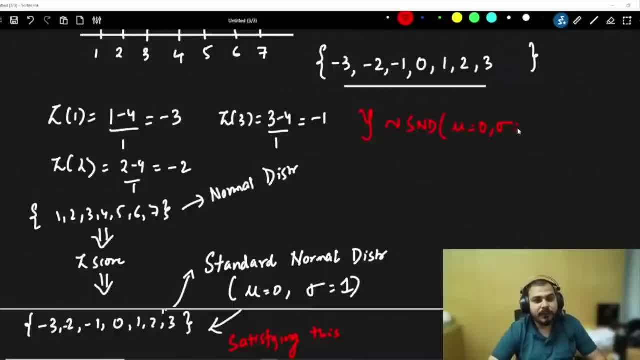 standard normal distribution where, specifically, your mean will be zero and standard deviation will be one. so, after applying a z score, we are able to get into a different distribution, which is called a standard normal distribution. now the question rises: why do we do this? what is the use of doing this? let's go ahead with one practical application. 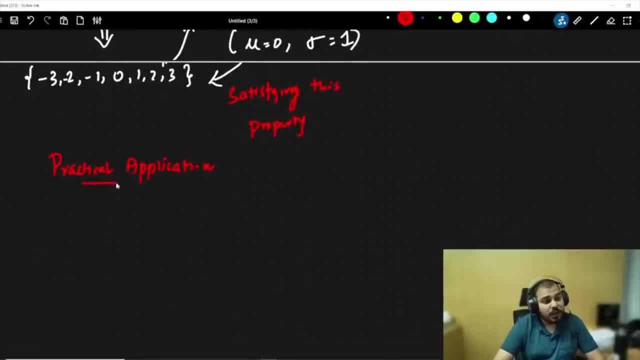 and we do this in machine learning. we do this in most of the algorithms. now let's go ahead and try to see the practical application. suppose i have a data set. let's consider that i am solving a machine learning problem statement. i have a data set: age. i have features like salary. i have features like 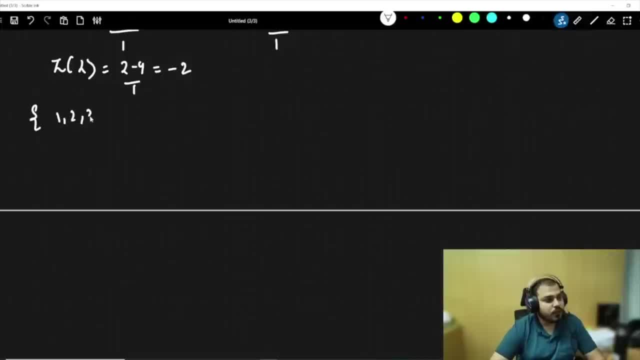 I had a distribution which was 1,, 2,, 3,, 4,, 5,, 6,, 7,, 8,, 9,, 10,, 11,, 12,, 13,, 14,, 15,, 16,, 17,, 18,, 19,, 20,, 21,, 22,, 23,, 24,, 25,, 26,, 27,, 28,, 29,, 30,, 30,, 31,. 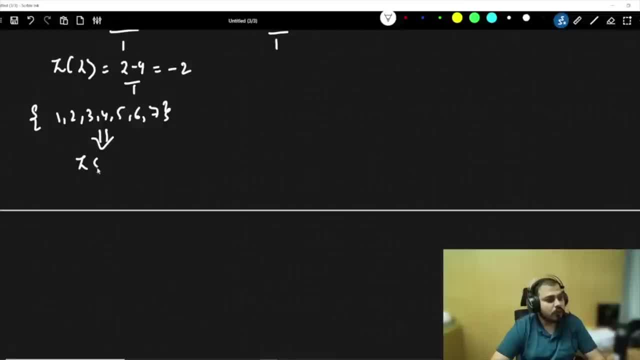 32,, 32,, 33,, 34,, 35,, 36,, 37.. After I applied a z-score, this got converted to minus 3, minus 2, minus 1, 0, 1, 2, 3.. And probably: yeah, Right, I got this. Now, what is this distribution then? 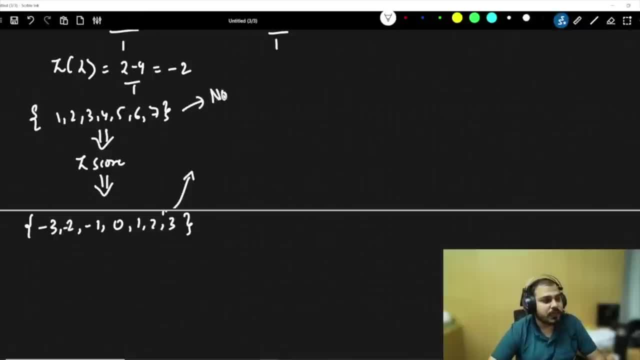 called. This was initially a normal distribution or a Gaussian distribution. After I applied a z-score. what kind of distribution we are actually getting? This is a normal distribution, And what is this basic distribution called as? So this distribution is called as standard. 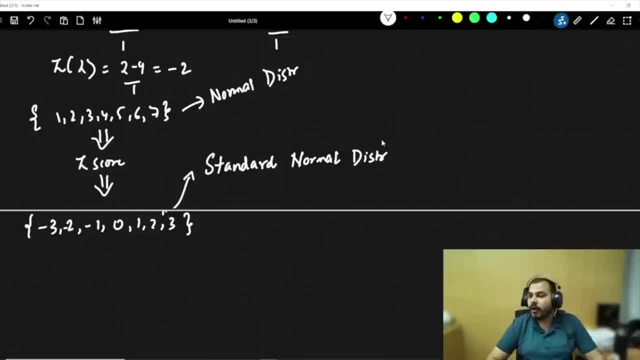 normal distribution. So one of the most important property with respect to standard normal distribution is that your mean is 0 and standard deviation is 1.. Is this satisfying this property or not? It is being satisfied, right. So can I write a random variable? x or y will belong to. 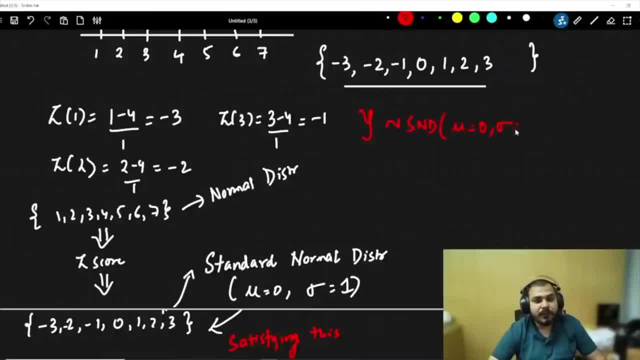 standard normal distribution where, specifically, your mean will be 0 and standard deviation will be 1.. So, after applying a z-score, we are able to get into a different distribution, which is called a standard normal distribution. Now the question rises: why do we do this? What is the use of doing? 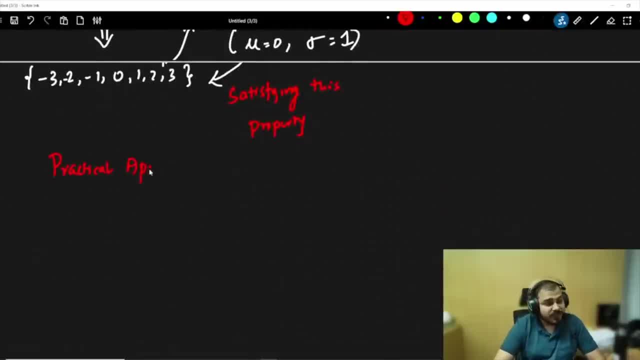 this. Let's go ahead with one practical application. And we do this in machine learning. We do this in most of the algorithms. Now let's go ahead and try to see the practical application. Suppose I have a data set. Let's consider that I am solving a machine learning problem. statement: I have a data set. 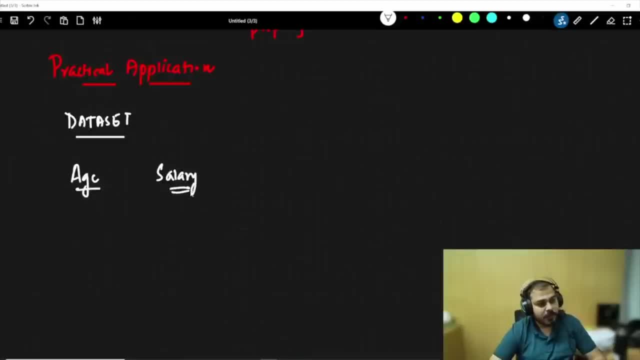 Age. I have features like salary. I have features like weight. Suppose in this particular data set. I have these three columns. Now understand one thing: Age. by what unit? we will calculate By years. Salary: we may calculate by rupees or dollar. Weight: we may calculate in kgs. Understand. 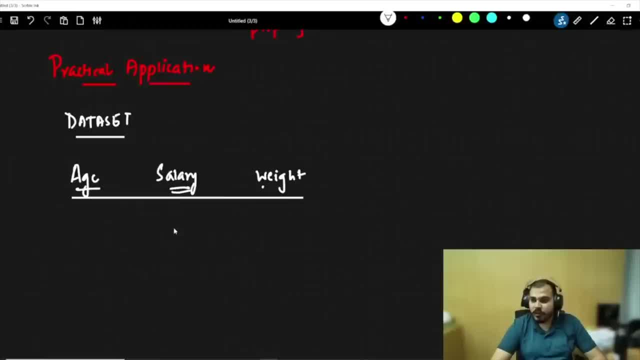 weight, suppose, in this particular data set. i have these three columns. now understand one thing: age, by what unit? we will calculate by years. salary: we may calculate by rupees or dollar. weight: we may calculate in kgs. understand this. units, these are, these are what these are basically. units, units of 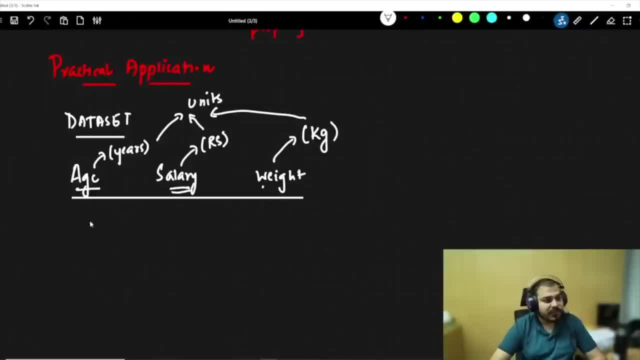 calculation now, whenever i have some values like this, like 24, 25, 26, 27- salary may be 40 k, 50 k, 60 k, 70 k something. weight may be 70 kg, 80 kg, 80 kgs, 55 kgs, 45 kgs. 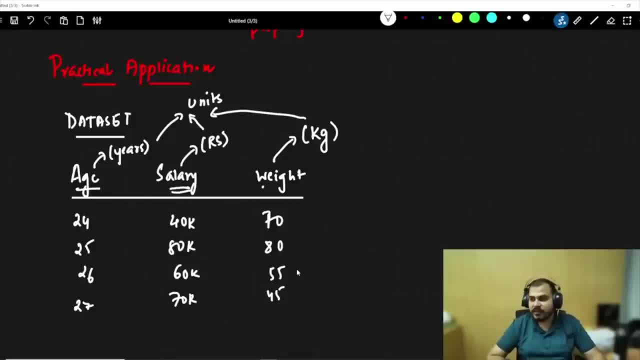 Now here, when you have this kind of data, always understand. Now in this data, obviously you can see the units are completely different. Our main target should be that we should try to bring up in a form, probably in this particular form, where my mean is 0 and standard deviation equal to 1.. 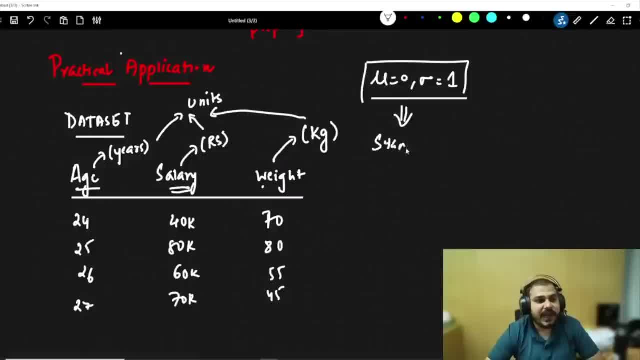 At that point of time, I can definitely apply standard normal distribution. That basically means I can take up this entire data and apply z-score and convert this into standard normal distribution. Similarly, I can go ahead and take up this particular data set, I can apply z-score and I can basically convert this into standard normal distribution. 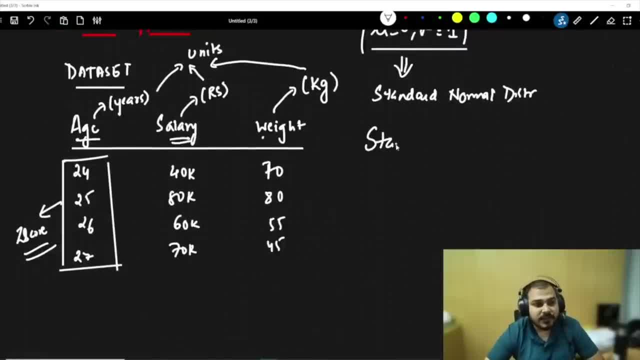 This process is basically called as standardization, Very, super important. Many people will talk about normalization. I will talk about the difference between standardization and normalization. Whenever we talk about standardization, in short, internally there is a z-score formula getting applied. 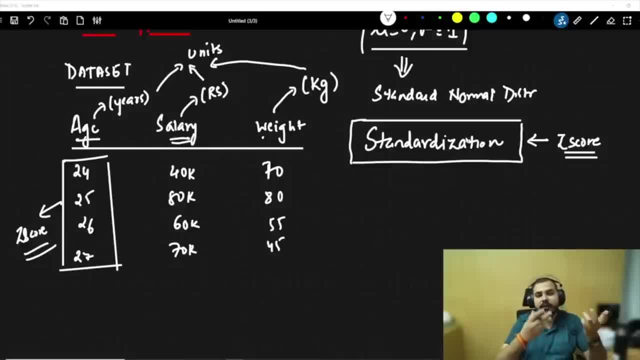 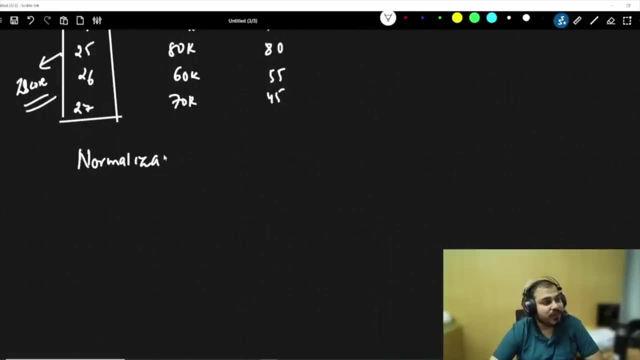 So standardization is a process where I am basically trying to convert a distribution into standard, normal distribution. The property is that the mean is 0 and the standard deviation is 1.. Now let's go ahead towards something called as normalization. Now, what exactly is normalization? 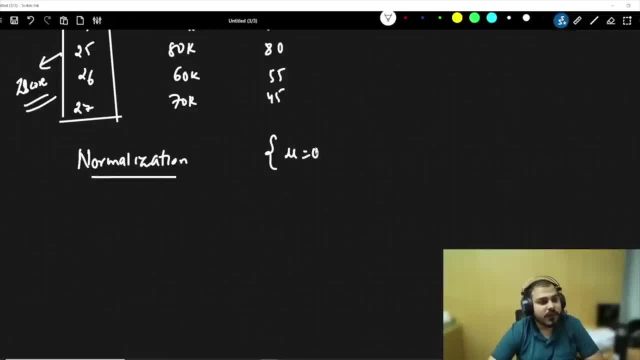 In standardization, whenever we talk about here, we are getting converted as mean is equal to 0 and standard deviation equal to 1.. Now in normalization, you have an option. You will say that I want to shift this entire values, or whatever values that I have, between 0 to 1.. 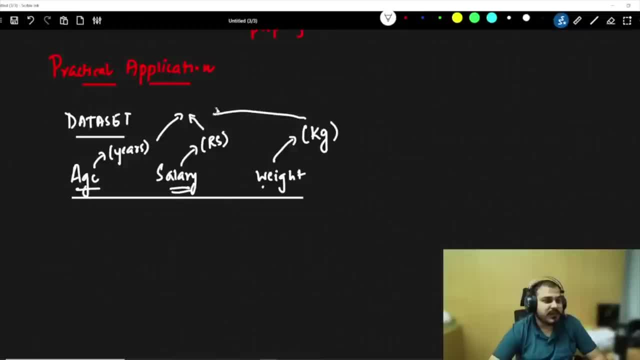 these units, these are, these are what. These are basically the units that we are calculating, Basically, units, units of calculation. Now, whenever I have some values like this, like 24,, 25,, 26,, 27,. salary may be 40k, 50k, 60k, 70k something. Weight may be 70 kgs, 80 kgs, 55 kgs, 45 kgs. 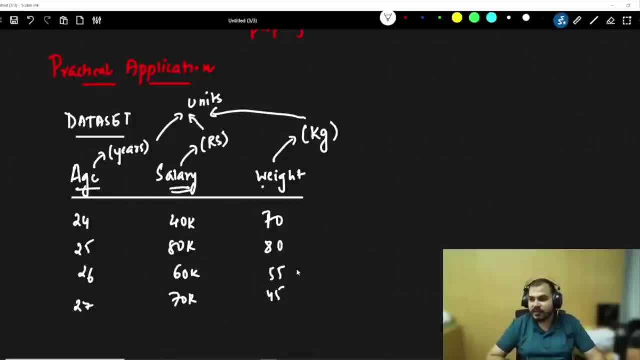 Now here, when you have this kind of data, always understand. Now, in this data, obviously you can see the units are completely different. Our main target should be that we should try to bring up in a form, probably in this particular form where my mean is 0 and standard. 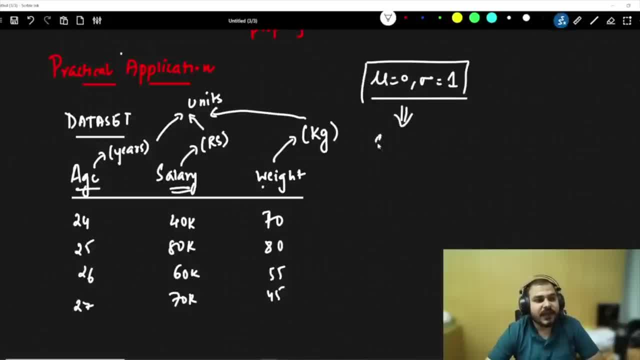 deviation equal to 1.. At that point of time, I can definitely apply standard normal distribution. That basically means I can take up this entire data and apply z-score and convert this into standard normal distribution. Similarly, I can go ahead and take up this particular data set. 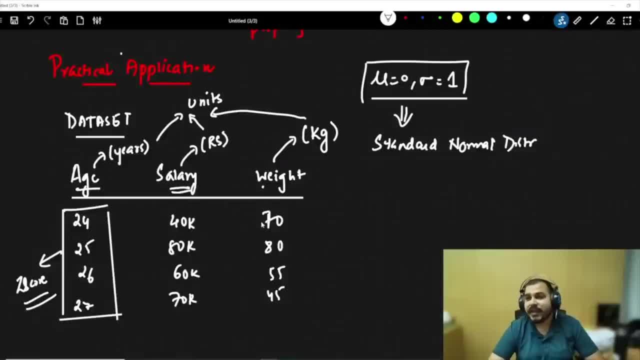 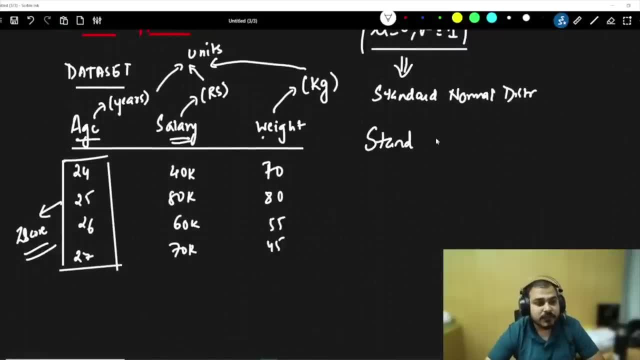 I can apply z-score. I can basically convert this into standard, normal distribution. This process is basically called as standardization- Very super important. Many people will talk about normalization. I'll talk about the difference between standardization and normalization Whenever we talk about standardization. in short, internally there is a z-score formula getting 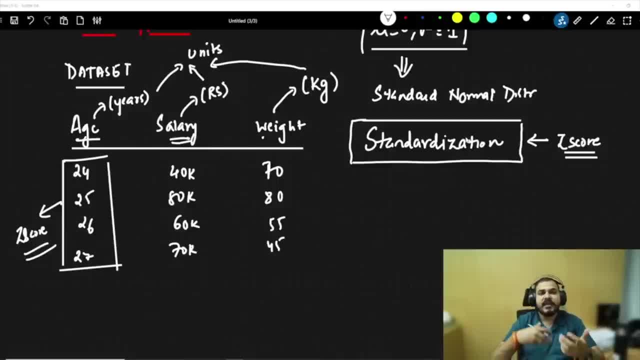 applied. So standardization is a process where I'm basically trying to apply z-score. I'm trying to convert a distribution into standard, normal distribution. The property is that the mean is 0 and the standard deviation is 1.. Now let's go ahead towards something. 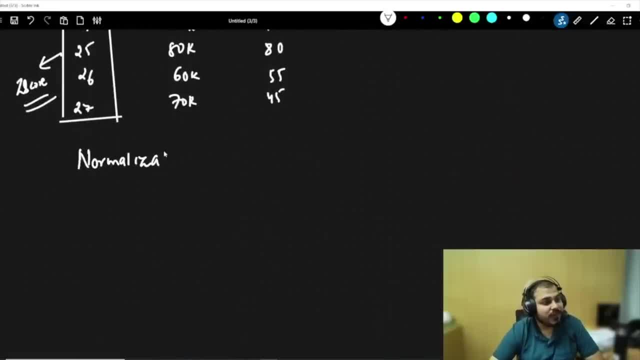 called as normalization. Now what exactly is normalization? In standardization, whenever we talk about here, we are getting converted as mean is equal to 0 and standard deviation equal to 1.. Now, in normalization, you have an option. You will say that I want to shift. 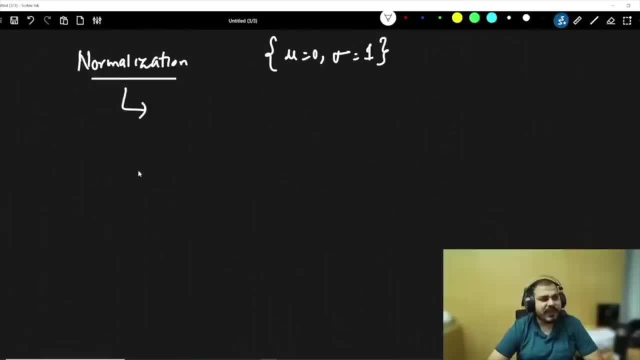 this entire values, Or whatever values that I have between 0 to 1.. Let's consider it like this: I want to change all these particular values between 0 to 1.. So in this particular case, I may definitely apply normalization. Now, how do we do normalization? There is a very important formula which is called 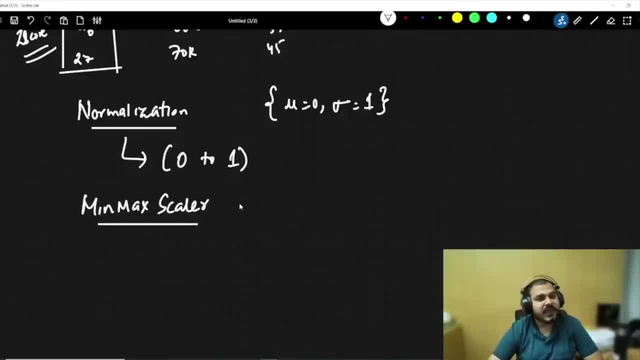 as min-max scalar. In the min-max scalar you just have to provide 0 to 1 and automatically this kind of normalization will happen. And yes, I will show you practically. also, Don't worry, If I want to simply shift this between minus 1 to plus 1, I can basically apply this. So normalization. 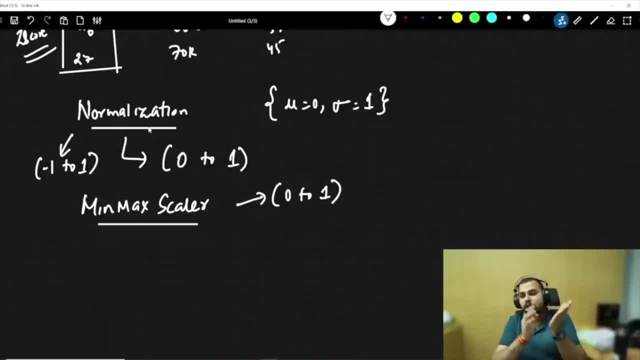 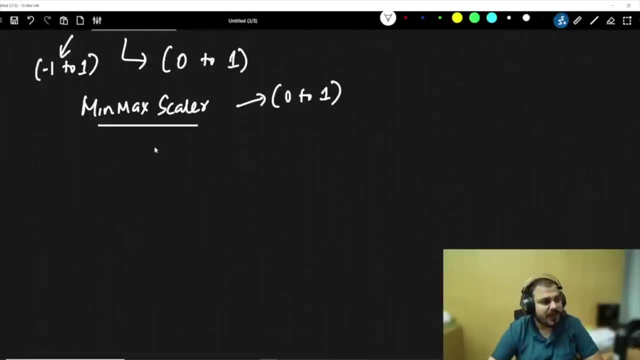 gives you a process where you can basically define the lower bound and upper bound and you can convert your data between them. Now, very important thing, Where do we use normalization? I hope everybody knows about deep learning In CNN whenever you are doing image training. 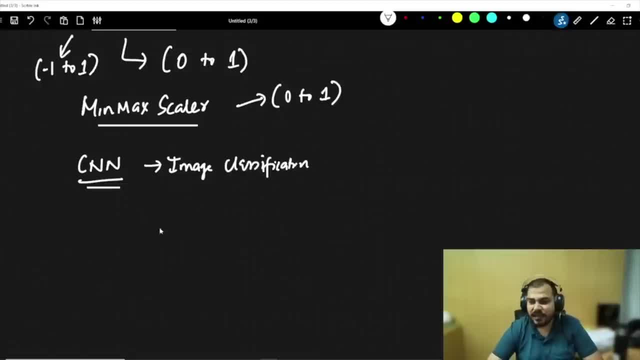 image classification or object detection. in this particular case, understand. every image has a pixels. Suppose I have a pixel. Let's say I have a pixel. Let's say I have a 4 x 4 image. 1,, 2,, 3, 4.. 1,, 2,, 3, 4.. Each and every pixel ranges between 0 to 255.. Now, 0 to 255,. 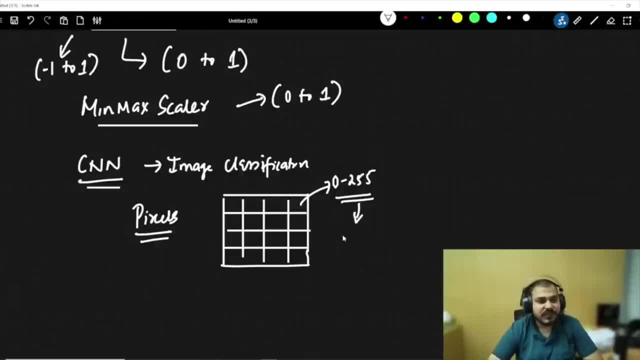 what we do before we start training. this can be applied with min-max scalar and it gets converted between 0 to 1, where the minimum value 0 is assigned to 0 and the maximum value 255 is converted to 1.. So when we do this automatically, we can apply this kind of min-max scalar or 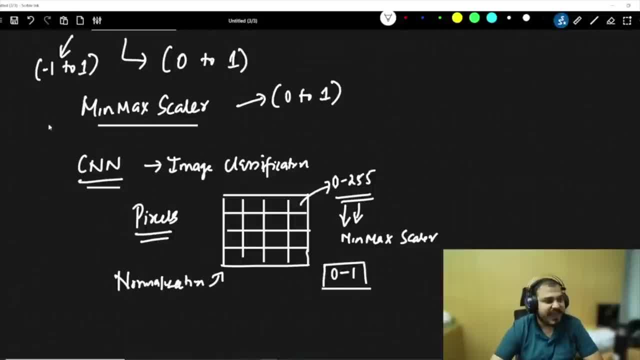 normalization. So in this particular case, I will definitely not use min-max scalar, because min-max scalar has a different formula. I will take each and every pixel divide by 255.. So when we do this specific division by divide by 255, all your values will be. 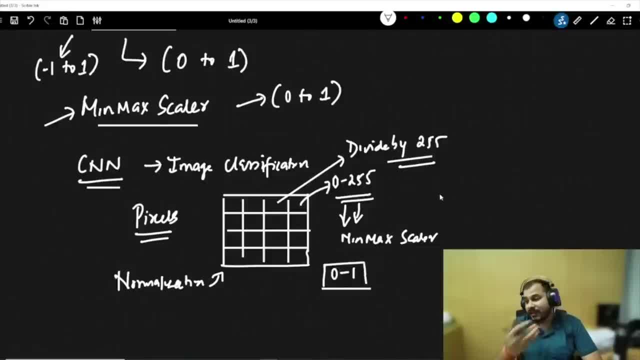 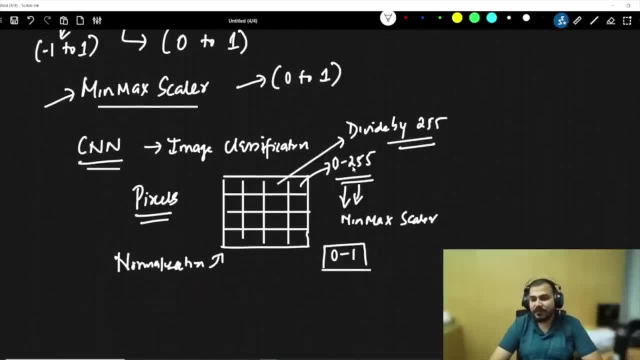 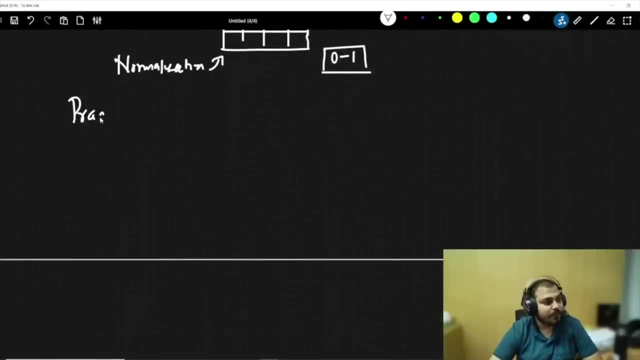 getting changed between 0 to 1. And this is another type of normalization process. So till here, we have discussed about min-max scalar, We have discussed about normalization, standardization. Now let's solve one practical example for z-score: Recently, India versus South. 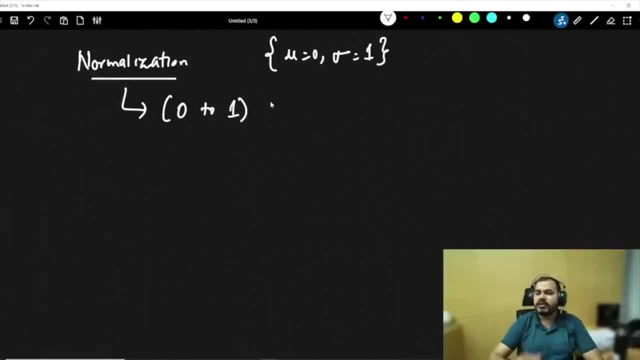 Let's consider it like this: I want to change all these particular values between 0 to 1.. So in this particular case, I may definitely apply normalization. Now, how do we do normalization? There is a very important formula, which is called as min-max scalar. 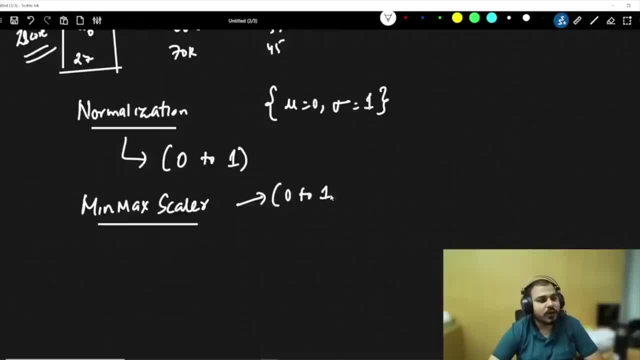 In the min-max scalar. you just have to provide 0 to 1 and automatically this kind of normalization will happen. And yes, I will show you practically. also, Don't worry, If I want to probably shift this between minus 1 to plus 1, I can basically apply this. 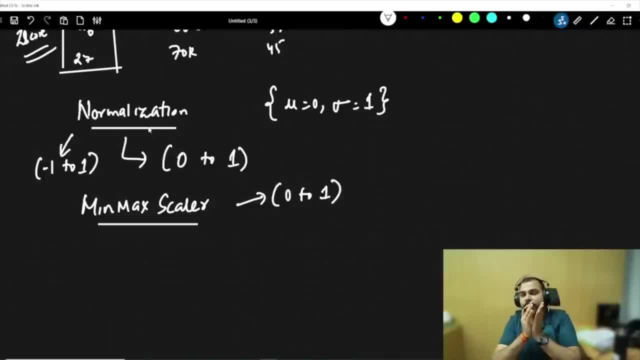 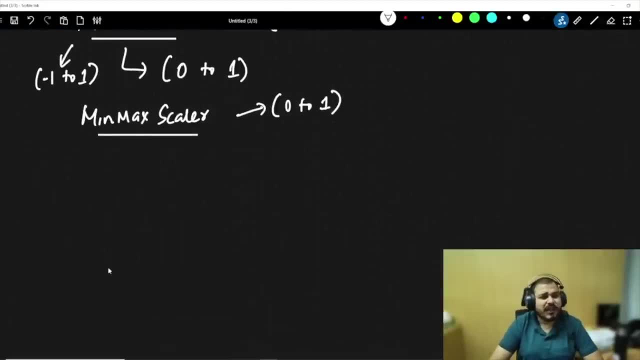 So normalization gives you a process where you can basically define the lower bound and upper bound and you can convert your data. Now, very important thing, Where do we use normalization? I hope everybody knows about deep learning In CNN whenever you are doing image training, image classification or object detection. 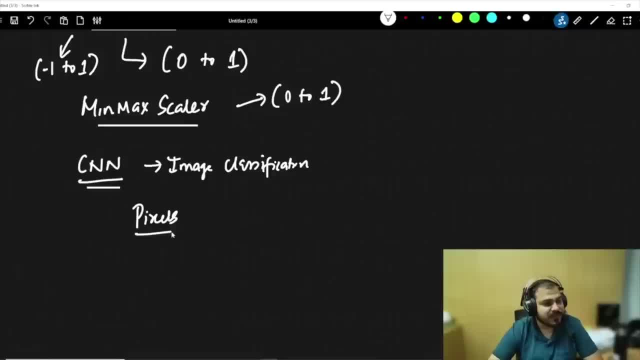 in this particular case, understand. every images has a pixels. Suppose I have a 4x4 image. 1, 2,, 3, 4.. 1,, 2,, 3, 4.. Each and every pixel ranges between 0 to 1.. 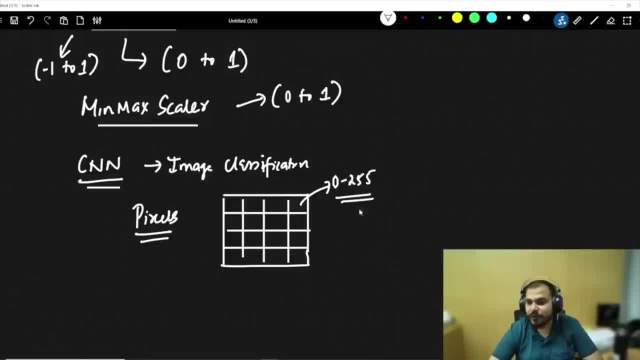 0 to 255.. Now, 0 to 255, what we do before we start training. this can be applied with min-max scalar and it gets converted between 0 to 1.. Where the minimum value 0 is assigned to 0 and the maximum value 255 is converted to 1.. 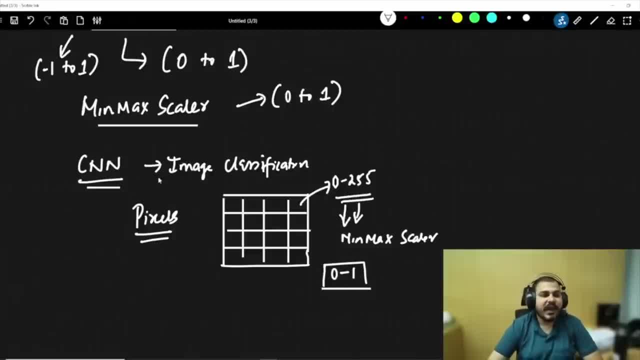 So when we do this, automatically, we can apply this kind of min-max scalar or normalization. So in this particular case, I will definitely not use min-max scalar. I will definitely not use min-max scalar, Because min-max scalar has a different formula. 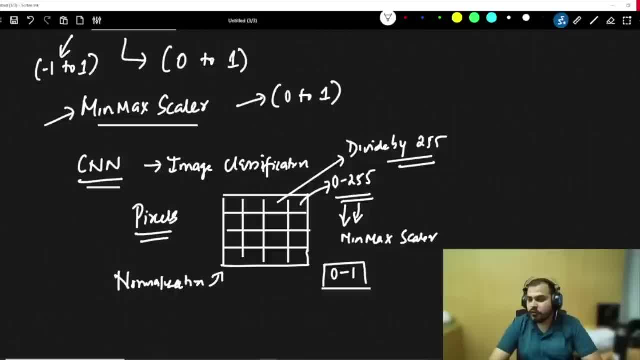 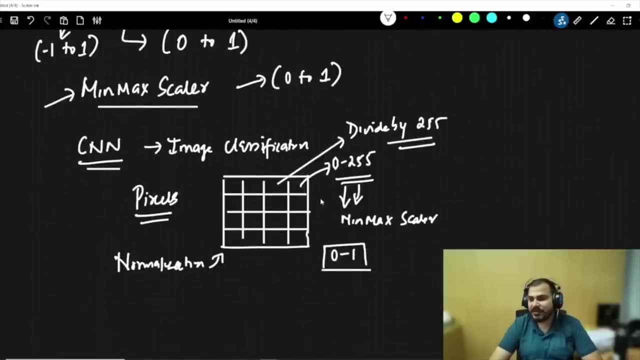 I will take each and every pixel divide by 255.. So when we do this specific division by divide by 255, all your values will be getting changed between 0 to 1. And this is another type of normalization process. So till here we have discussed about min-max scalar. 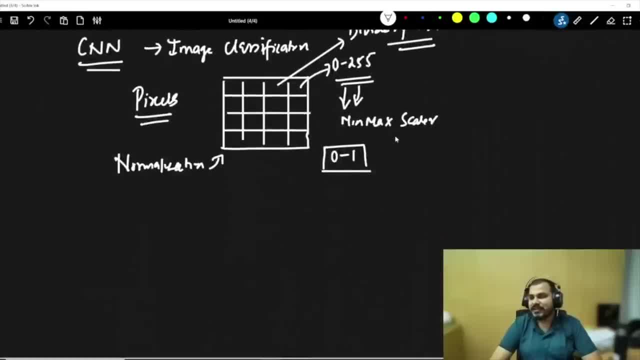 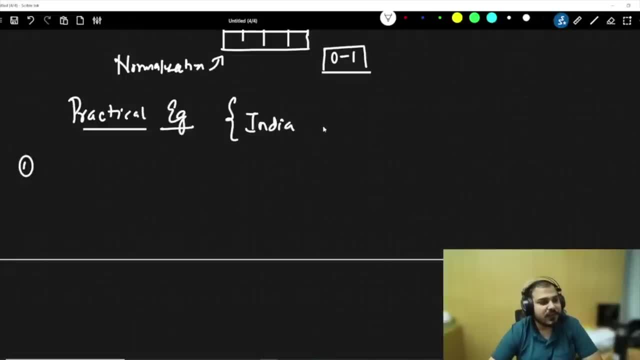 We have discussed about normalization, standardization. Now let us solve one practical example for z-score. Okay, recently, India versus South Africa, where India lost it obviously. Now let us consider that. If I consider ODI series, let us say: 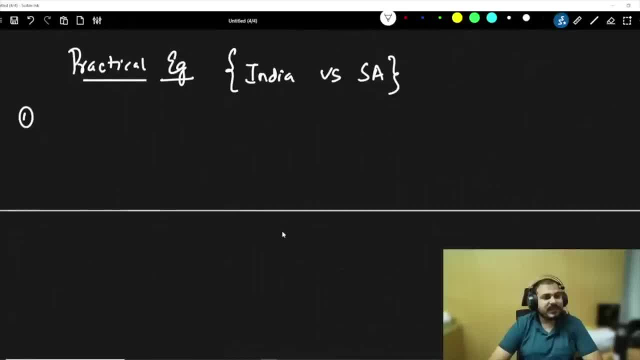 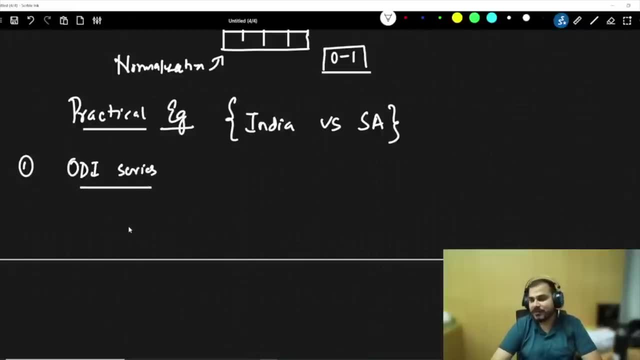 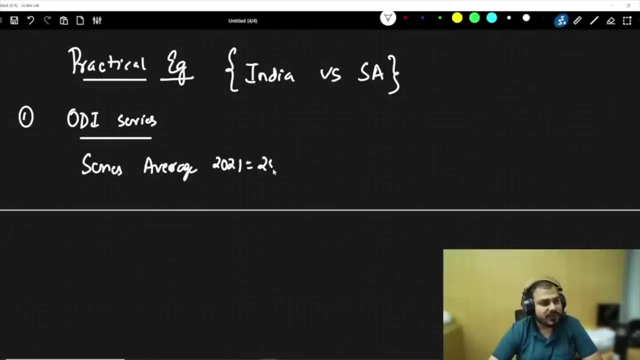 Africa, where India lost it obviously. Now let's consider that. If I consider ODI series, let's say- and every time in last year also, ODI series happened. this year also it happened. The series was somewhere around, let's say, 250.. The standard deviation of the score was somewhere. 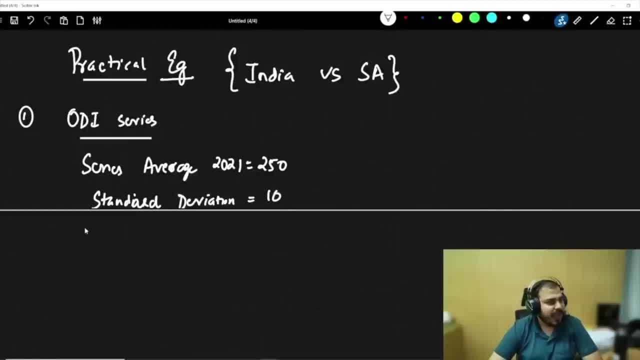 around 10.. And Rishabh Pant, let's say Rishabh Pant, final score was 70.. So this was the series information for 2021.. Let's consider Now. similarly, I have a data for 2020 series. 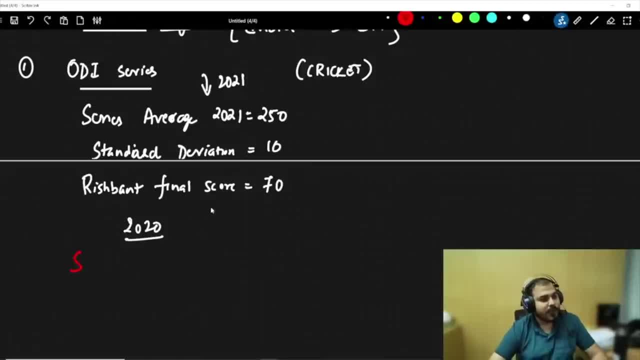 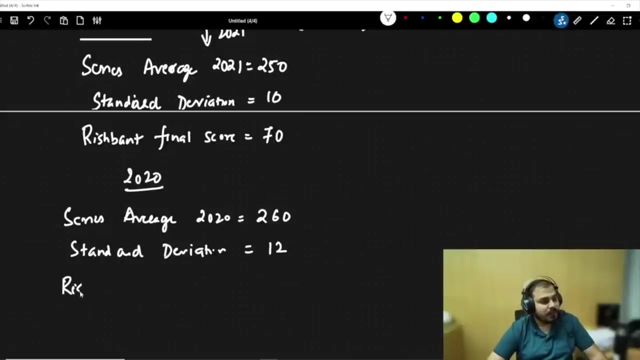 Let's say the series average in 2020,. let's say that the series average is little bit different In 2020, the series average of the team scoring in 2020 was 260.. The standard deviation of the score of all the matches is 12.. And then, over here, probably, Rishabh Pant, final score. 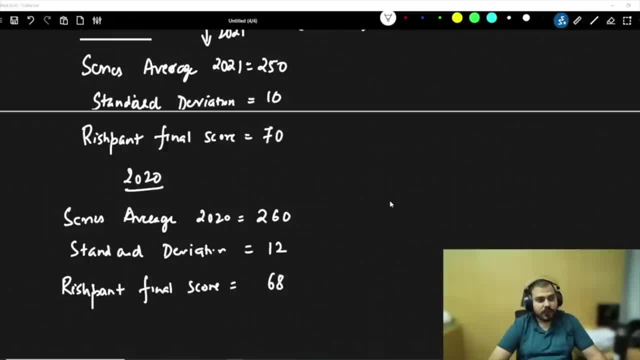 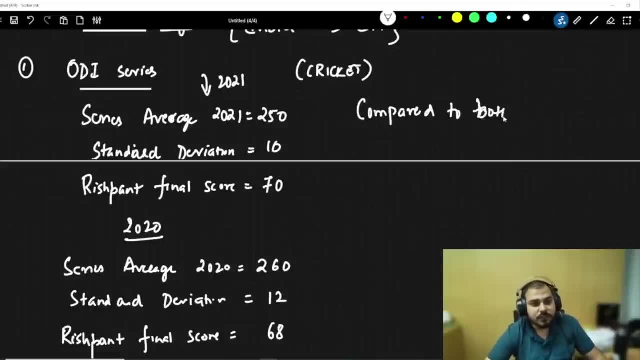 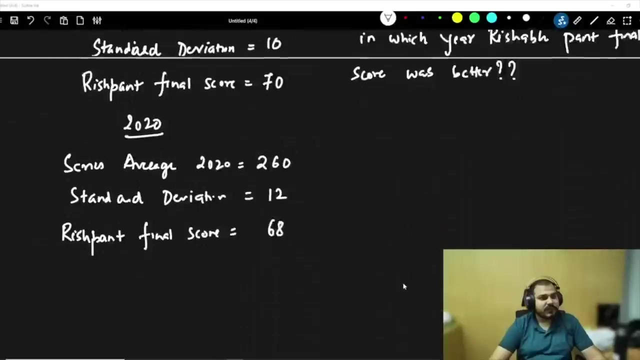 is 68.. Okay, my question is that these two data I have compared to both the series In which year Rishabh Pant final score was better? So for checking this, obviously many people will say 2020, 2021, lot of confusion will be there, So we will just try to apply for Z score. Now for the 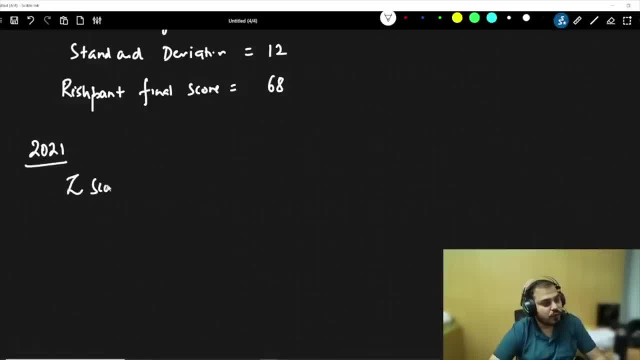 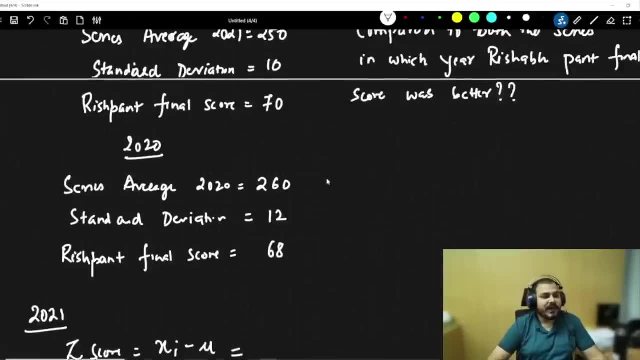 2021, we will apply the Z score, So Z score will be nothing, but it will be X of I minus mu, divided by standard deviation. We know what is X of I. in this particular case, X of I is nothing but. 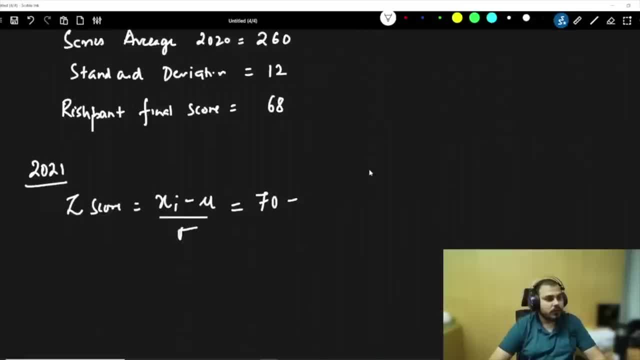 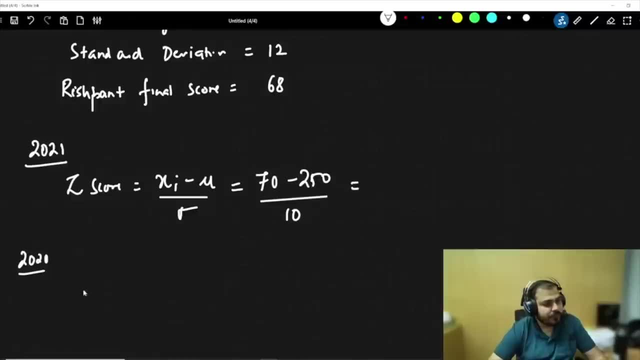 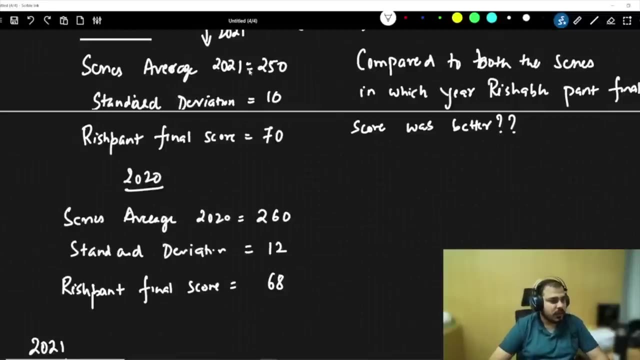 so 70 minus 250 divided by 10.. So what we are getting over here? similarly, for 2020, my Z score will be X of I minus mu divided by standard deviation. So first one, you know this properly. this values may not be coming. Let me change this data a little bit. Okay. Rishabh Pant, final. 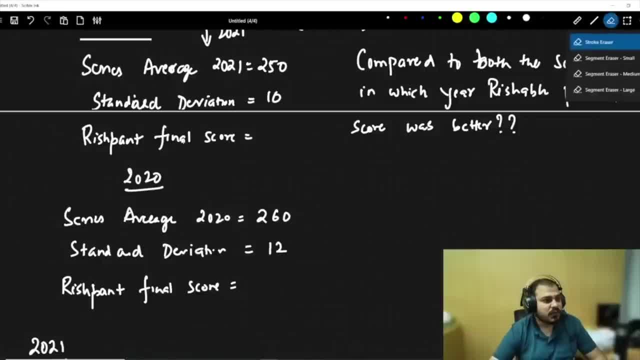 I will say average score, not final score, So that we change this data a little bit, Otherwise the data will be very, very bad. Okay, Rishabh Pant average score: let us consider that it is 240.. Okay, And Rishabh Pant average score is somewhere. 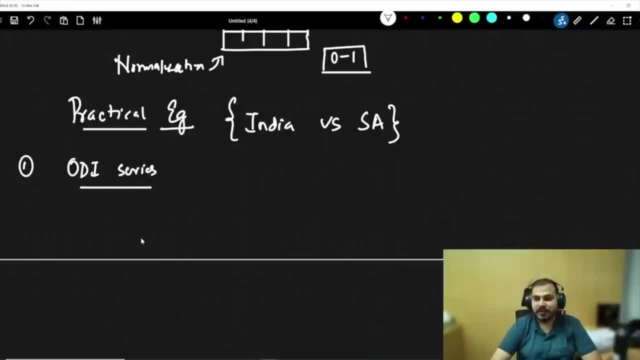 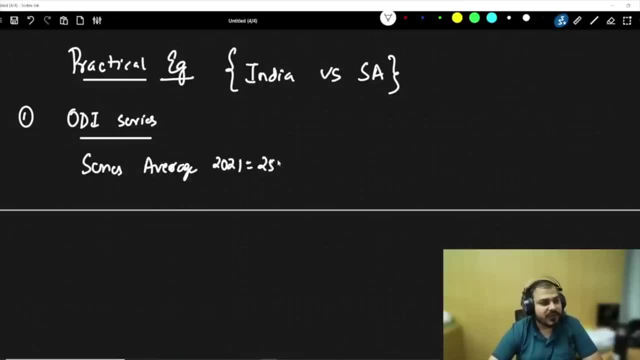 And every time- last year also, ODI series happened. this year also, it happened. The series average of 2021 was somewhere around, let us say, 250.. The standard deviation of the score was somewhere around 10.. And Rishabh Pant- let us say Rishabh Pant. 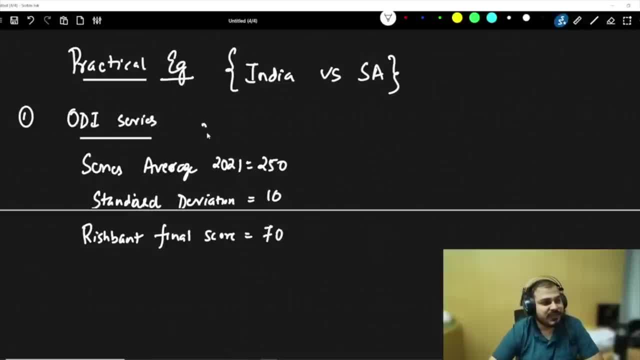 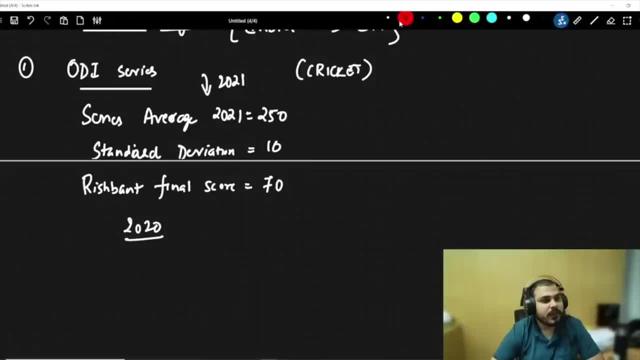 final score was 70.. So this was the series information for 2021.. Let us consider Now, similarly, I have a data for 2020 series. Let us say the series average in 2020, let us say that the series average is a little bit different. 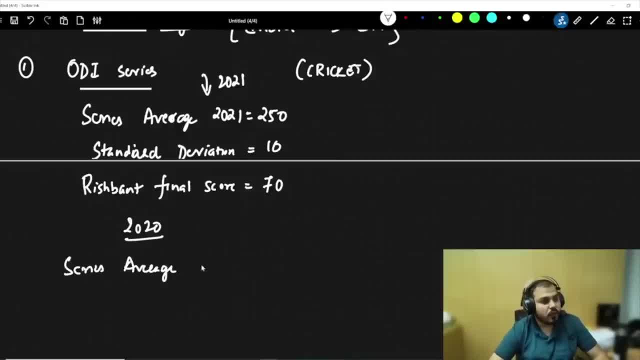 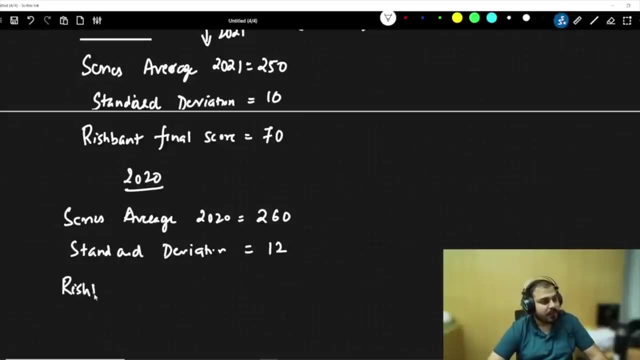 In 2020, the series average of the team scoring in 2020 was 260.. The standard deviation of the score of all the matches, let us say Rishabh Pant, is 12.. And then over here, probably, Rishabh Pant- final score is 68. 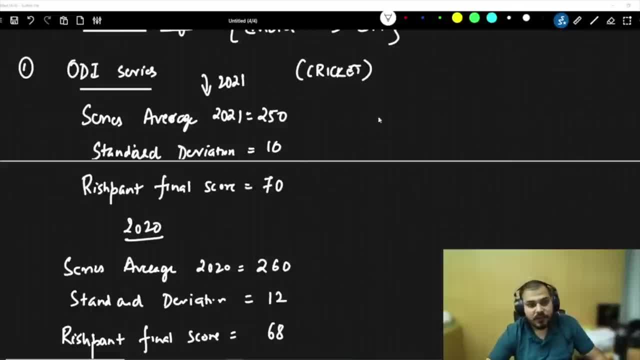 Okay, my question is that these two data I have compared to both the series in which year Rishabh Pant final score was better. So for checking this, obviously many people will say 2020, 2021, lot of confusion will be there. 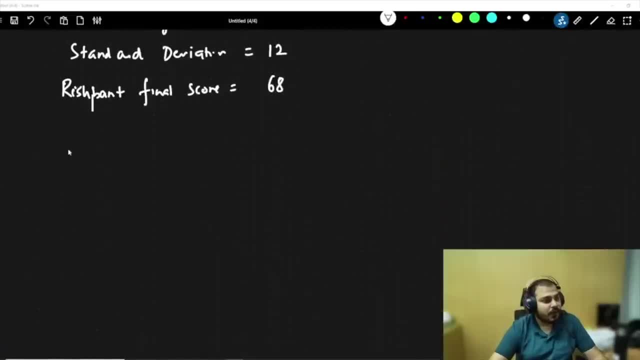 So we will just try to apply for Z-score Now for the 2021, we will apply the Z-score. So Z-score will be nothing, but it will be X of I minus mu divided by standard deviation. We know what is X of I in this particular case. 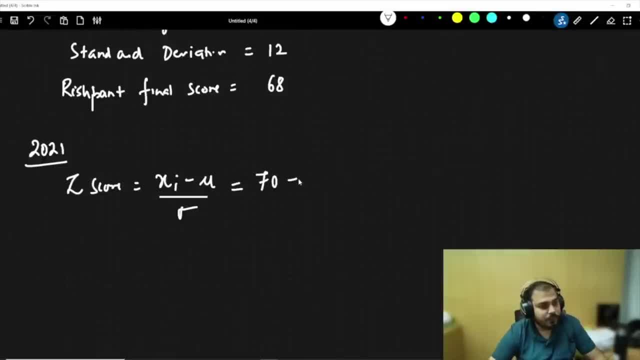 X of I is nothing but so 70 minus 250 divided by 10.. So what we are getting over here? Similarly, for 2020, my Z-score will be X of I, X of I minus mu, divided by standard deviation. 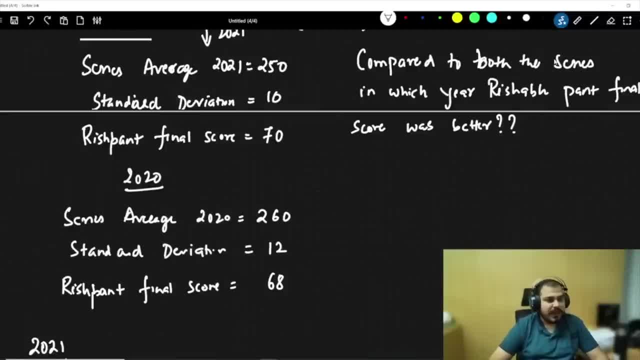 So first one, you know this properly- this values may not be coming. Let me change this data a little bit. okay, Rishabh Pant final. I will say average score, not final score, so that we change this data a little bit. 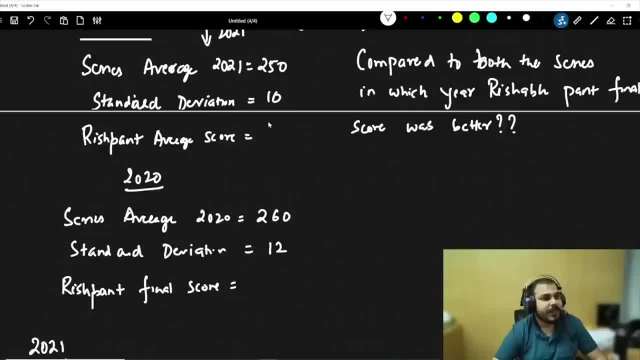 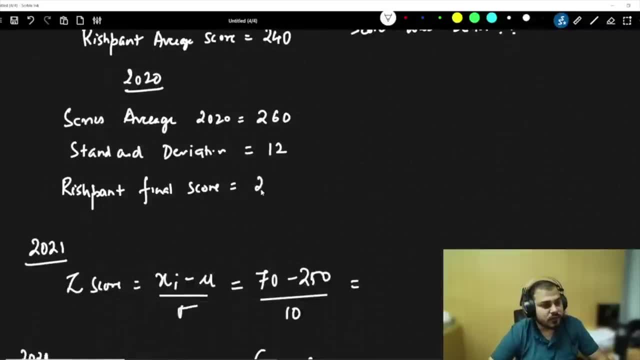 Otherwise, the data will be very, very bad. okay, Rishabh Pant average score. let us consider that it is 240.. Okay, And Rishabh Pant average score is somewhere around. Let us consider like this: Okay, 240 and 245. 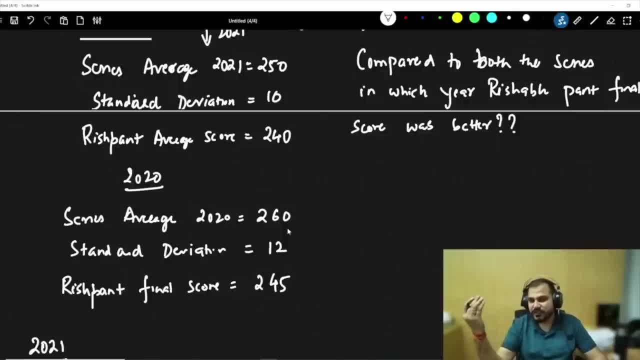 Because I gave one score. so that is the reason a huge standard deviation is basically coming At that point of time. I am just taking average score. Average score of the series: guys Rishabh Pant. this player's average score of the series. 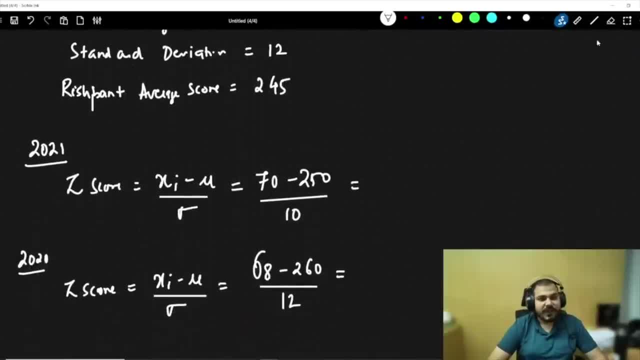 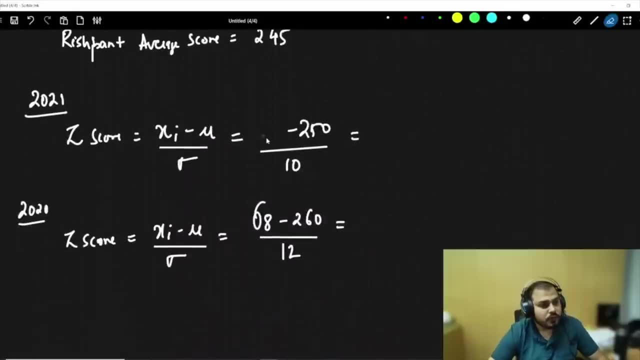 Average score of the series. Okay, Now let me just make some changes And let me put somewhere over here as 240. So 240.. 240 minus average score of the series. guys, Three match, Three match series. So 240 minus 250 is nothing but minus 10 divided by 10.. 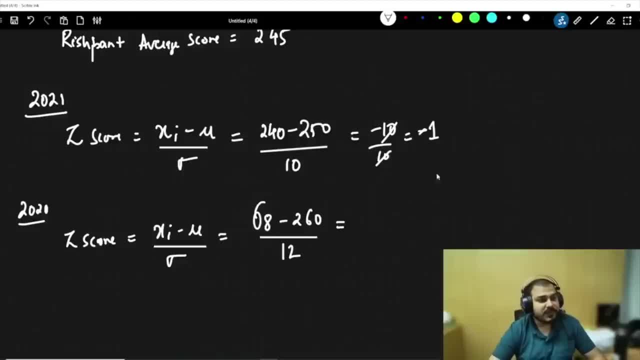 So this is minus one standard deviation, And this data will now change to 245.. So 245, this will be minus 15 divided by 12,, which is nothing but 15 by 12,, which is nothing but minus 1.25.. 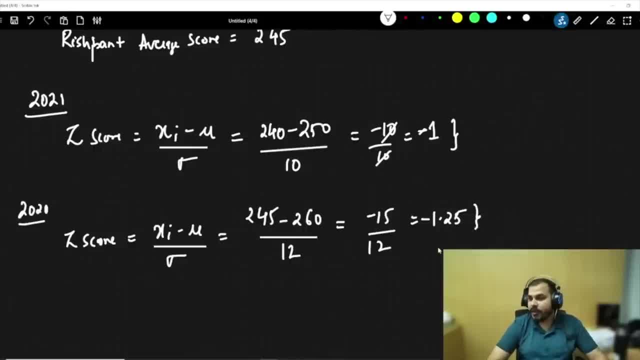 Okay, Clear Everybody. Okay, Akash Singh, if you hit 80 in all three matches, then it is 240.. So understand, along with the not out rule something, 240 is the average. Okay, Let us consider in that specific way. 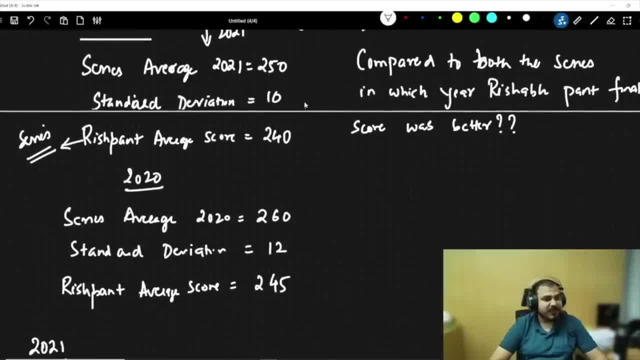 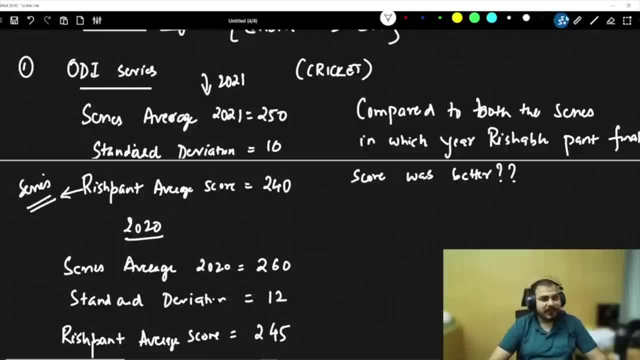 I could have team average score. Okay, Team average score, And probably team played well, probably in the last match or the first match, Like that. Okay, In which series they played well? That also you can basically say Over here: instead of Rishabh Pant, I could write team average score. 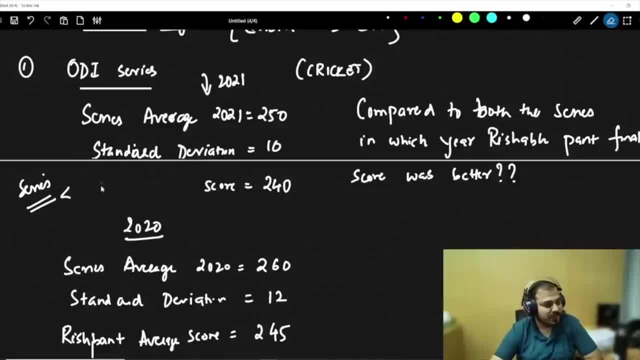 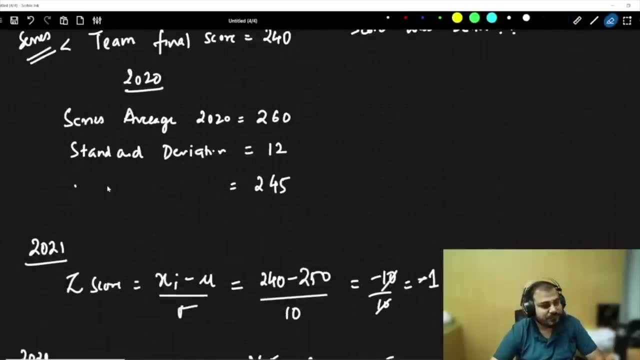 Team score in final match. I messed up with the problem statement Because I was just thinking something: Score, final match score Like that. Okay, Team average, Team final score. Here also I can say team final score. This will probably be more problematic. 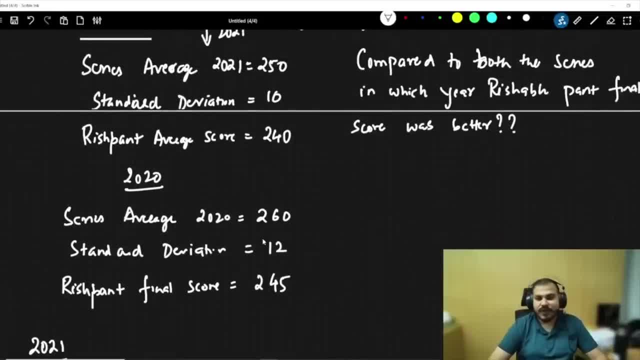 around 245.. Let us consider like this: Okay, 240 and 245. Because I gave one score. so that is the reason a huge standard deviation is basically coming At that point of time. I am just taking average score. Average score of the series. guys: Rishabh Pant: this player's average score. 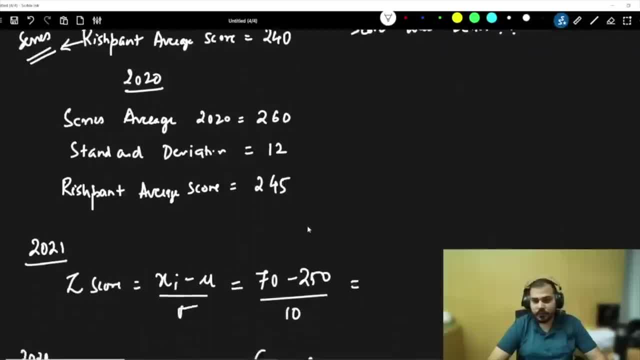 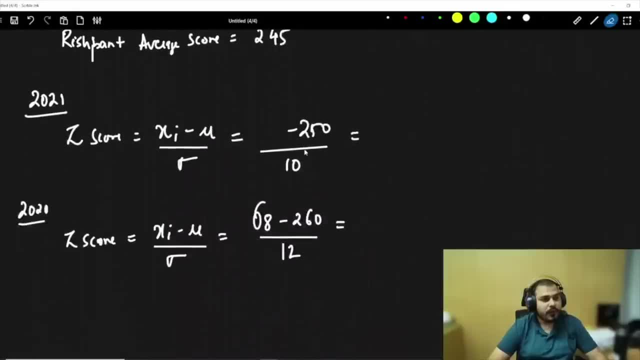 of the series. average score of the series. Okay, Now let me just make some changes And let me put somewhere over here as 240.. So 240 minus average score of the series. guys, Three match, three match series. So 240 minus 250 is nothing but minus 10 divided by 10. So this is minus one standard. 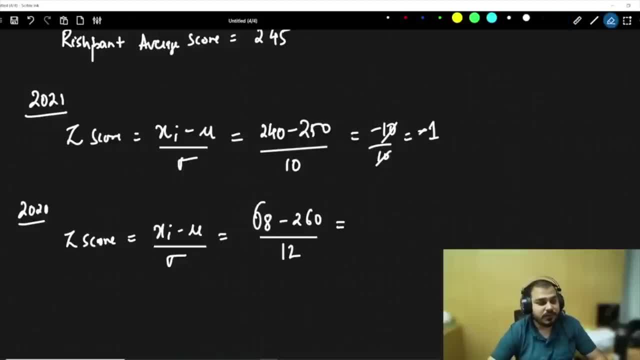 deviation And this data will now change to 245.. So 245, this will be minus 15 divided by 12, which is nothing but 15 by 12,, which is nothing but minus 1.25.. Okay, Clear Everybody. Okay, Aakash Singh: if three matches, 80 is given. 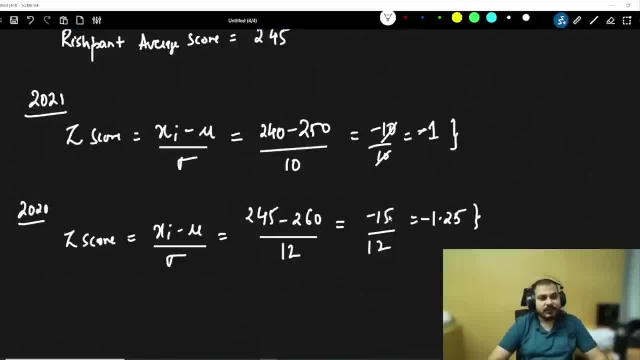 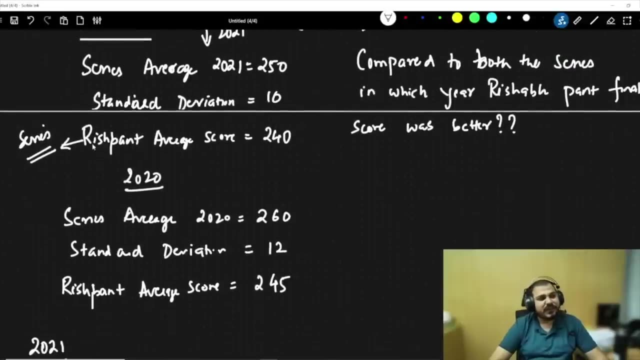 then the average is 240.. So understand, along with the not out rule, something, 240 is the average. Okay, Let's consider in that specific way. I know the data is not approximately right, But I could also, instead of Rishabh Pant, average score, I could have team. 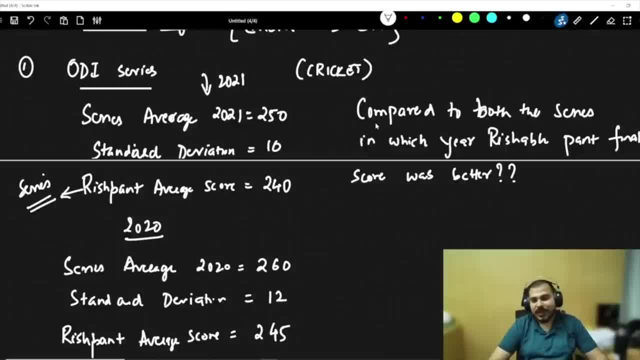 average score. Okay, Team average score. And probably team played well, probably in the last match or the first match, Like that. Okay, In which series they played well? That also you can basically say Over here. instead of Rishabh Pant, I could write team average score. 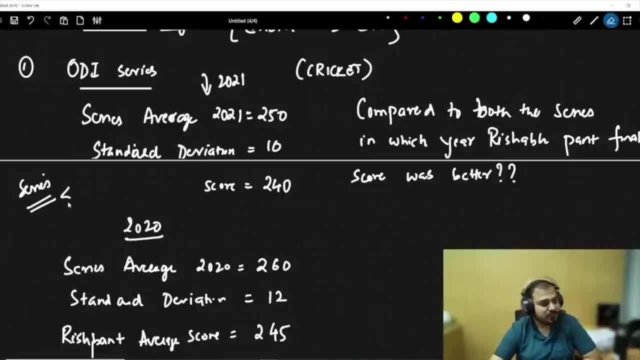 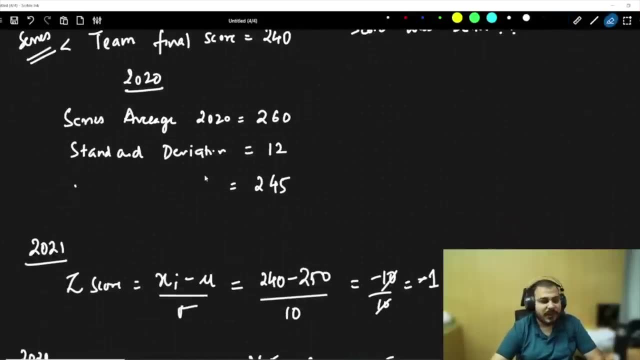 Team score in final match. I messed up with the problem statement Because I was just thinking something: Score, final match score Like that. Okay, Team final score. Here also I could say team final score. This will probably be more problematic. Team final score. 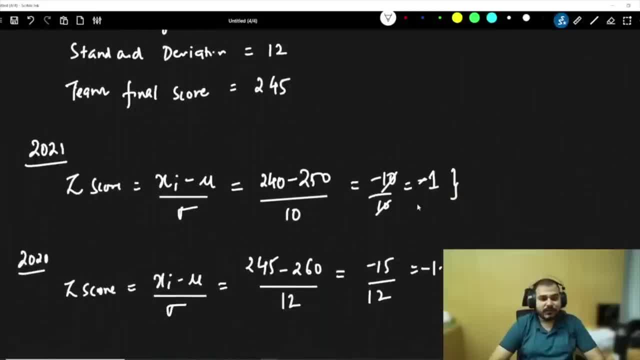 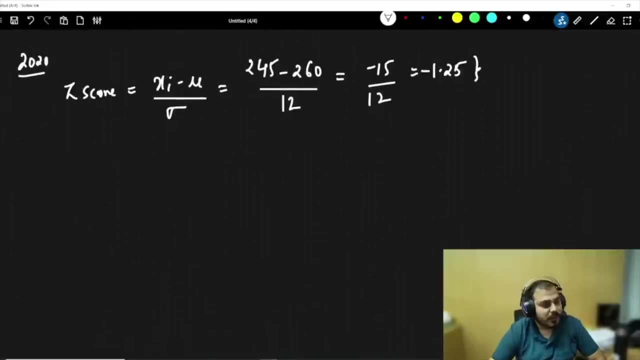 Now, based on this, I have always again. this is an example, guys, Just think of it. Okay, So here I have got minus 1.. Here I got minus 1.. Here I got minus 1.25.. Now see, I have seen that. 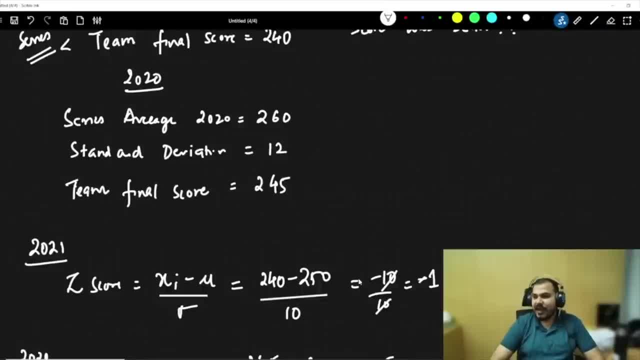 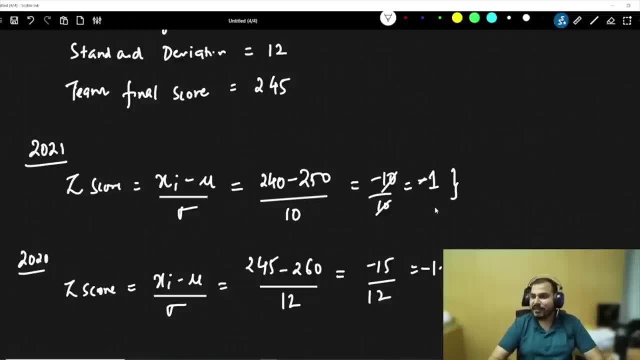 Team final score. Now, based on this, I have always- Again, this is an example, guys. Just think of it. The main idea is to teach you something so that you can apply that anywhere. Okay, So here I have got minus 1.. 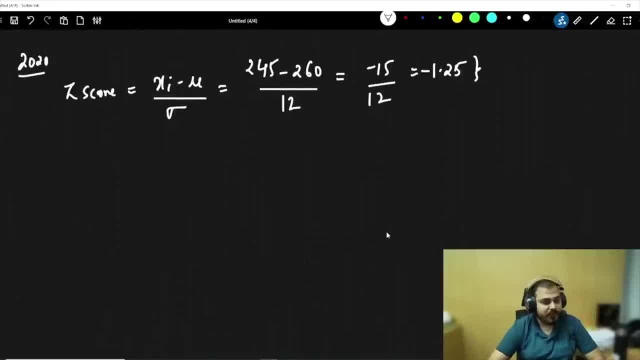 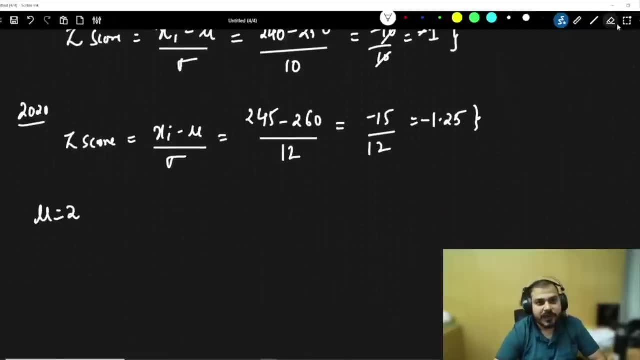 Here I got minus 1.. Here I got minus 1.25.. Now see, I have seen that the mean is 2. In 2021, so let me write it down again for you. So if in 2021, the mean is 250.. 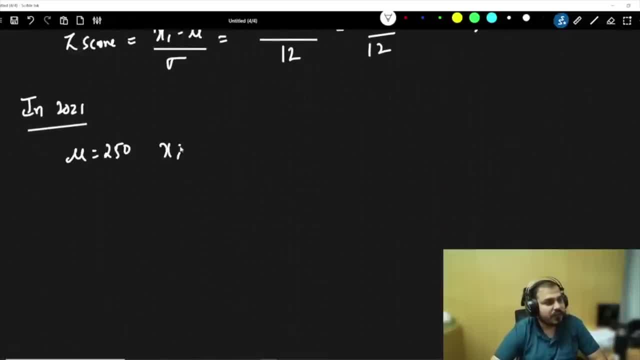 Over here. you can see, the mean is 250.. X of i is nothing but how much. It is nothing but 240.. And the mean is 10.. Sorry, And the standard deviation is 10.. If I have this information, can I draw the bell curve? 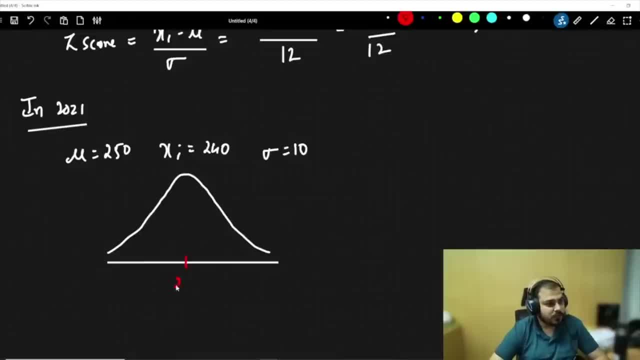 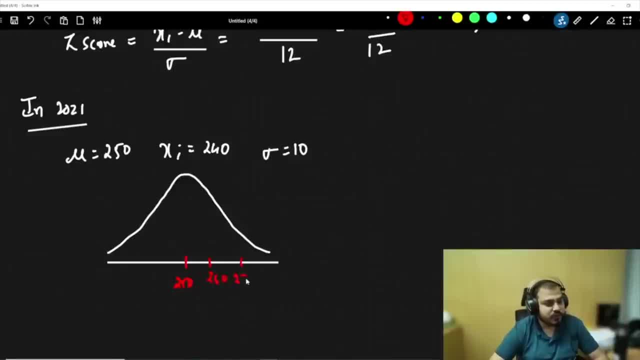 Standard deviation is 10.. Basically means this will come as 260, 270, 280.. Right, This will come as 240, 230, 220.. Right, And this is my mean. Now, where does 240 fall into? 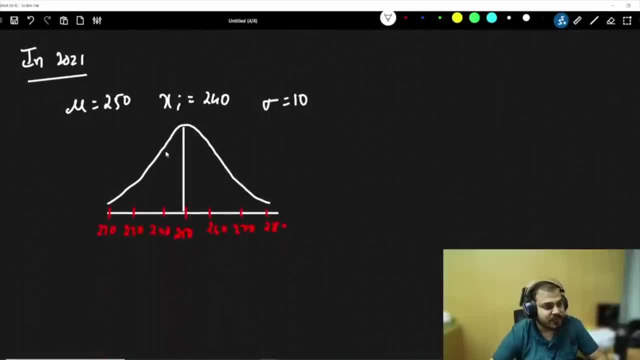 240 is falling into minus 1 standard deviation. So that basically means 240 will fall here Now in 2020.. In 2020.. You know that your mean is how much? 260.. Right, Your mean is 260.. 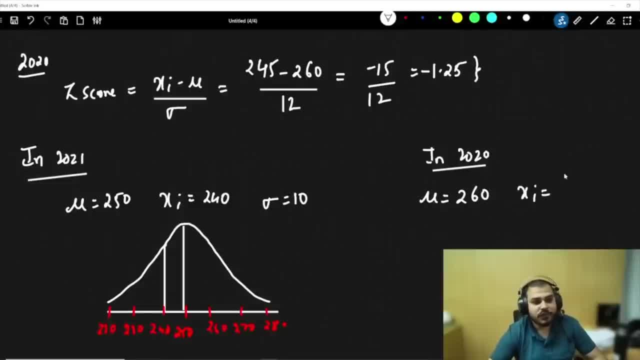 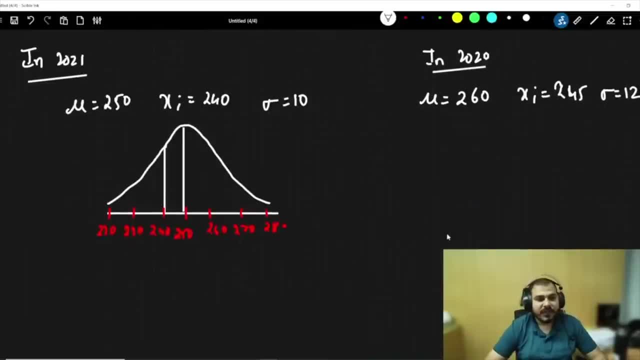 X of i, that is, your final score is 245.. And your standard deviation is nothing but 12.. Now, based on this, I will definitely be able to create another curve which will have this kind of bell curve, And my central element will be 260. 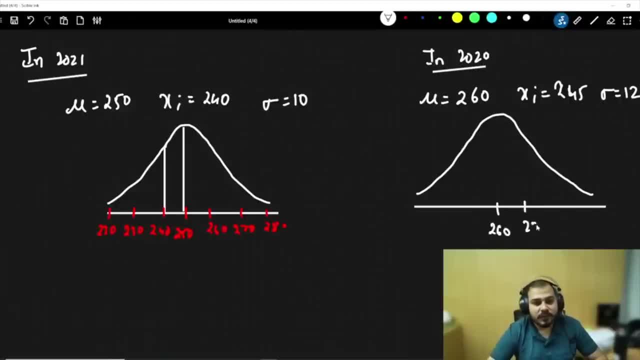 Since my standard deviation is 12,, I will definitely be able to create another curve which will have this kind of bell curve, and my central element will be 260.. This will become 272.. Then it will become 284.. Then it will become 296.. 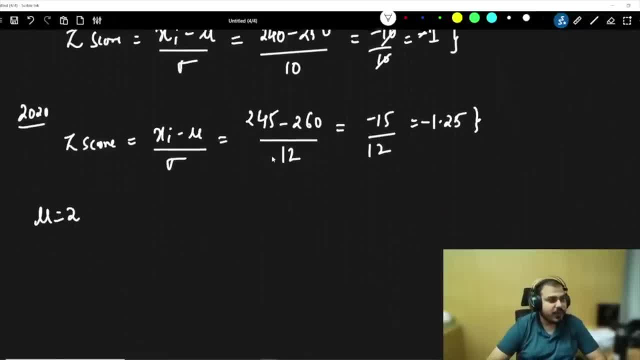 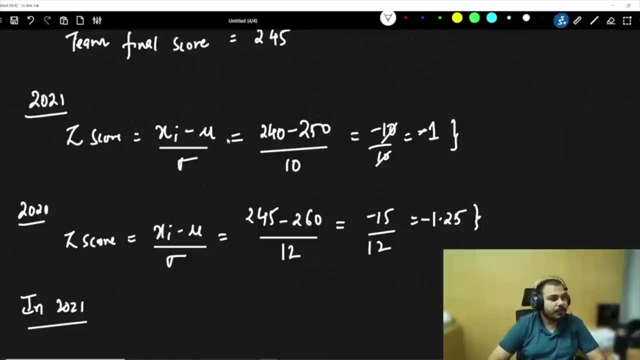 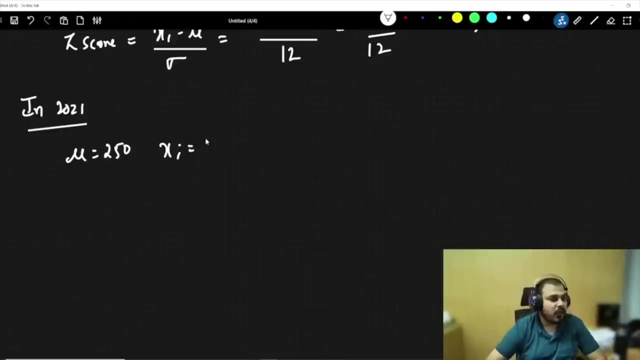 the mean is 2.. In 21,, 2021.. So let me write it down again for you. So if in 2021, the mean is 250.. Over here you can see, the mean is 250.. X of i is nothing, but how much? It is nothing but. 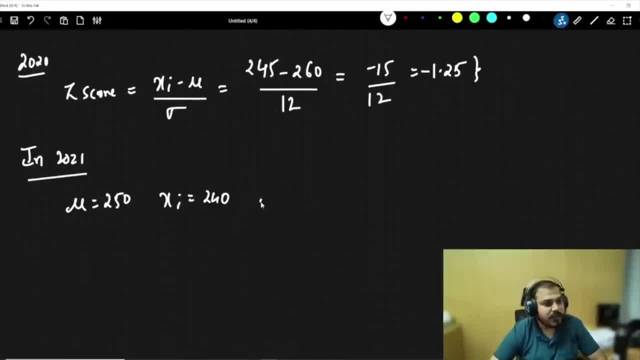 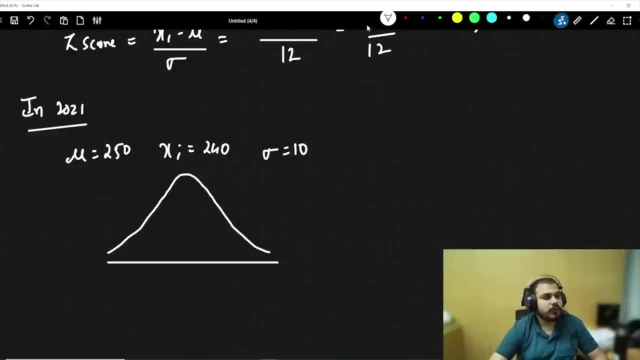 240.. And the mean is 10.. Sorry, And the standard deviation is 10.. If I have this information, can I draw the bell curve? So this is my bell curve. The mean is how much? 250.. Standard deviation is 10.. Basically means this will come as 260,, 270,, 280.. Right, This will come as 240,. 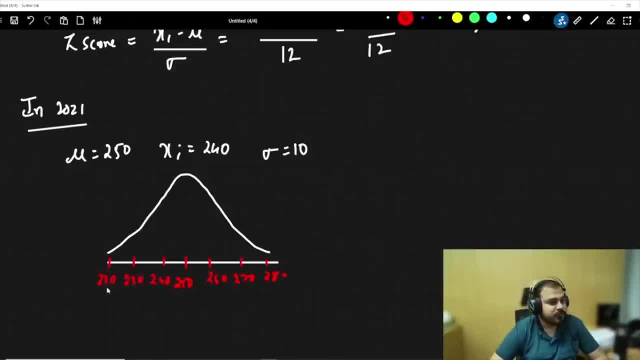 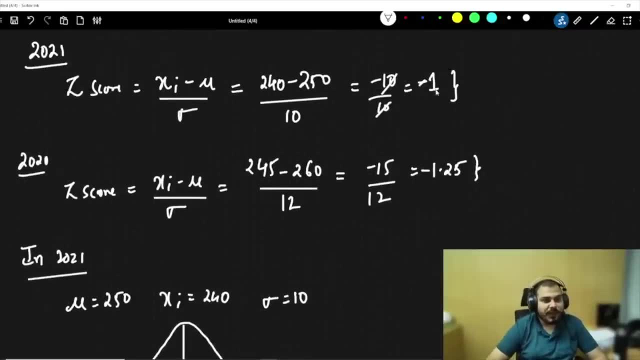 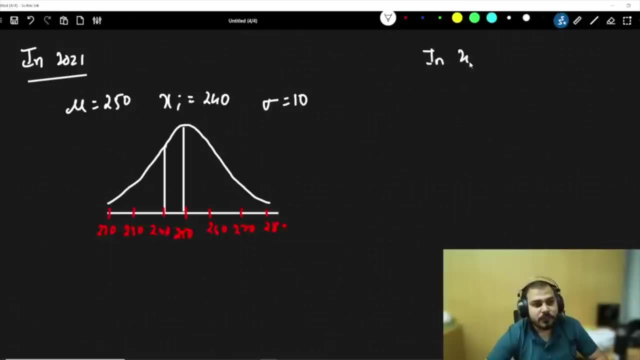 230, 220. Right, And this is my mean. Now, where does 240 fall into? 240 is falling into minus 1 standard deviation, So that basically means 240 will fall here Now in 2020, in 2020, you know that your mean is, how much 260.. Right. 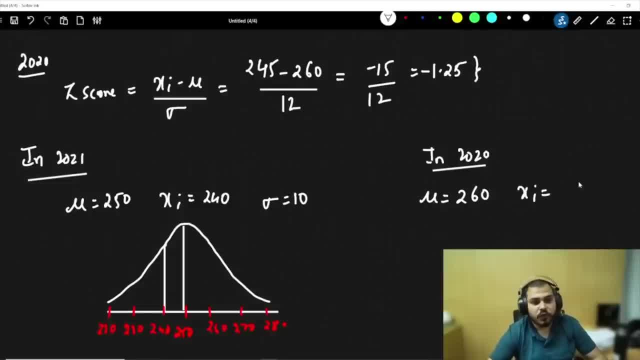 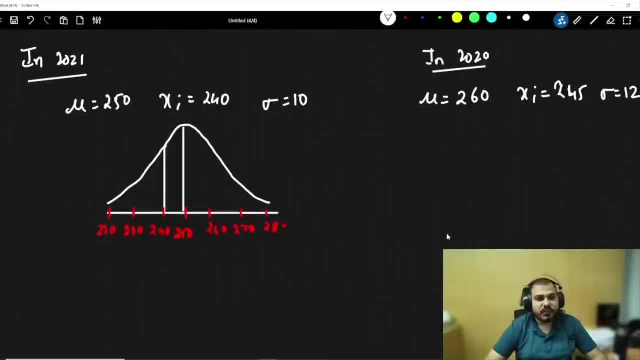 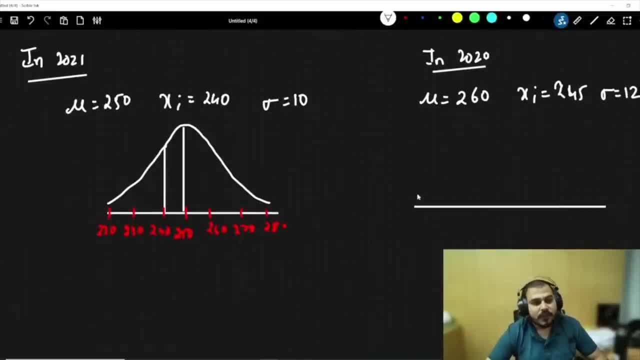 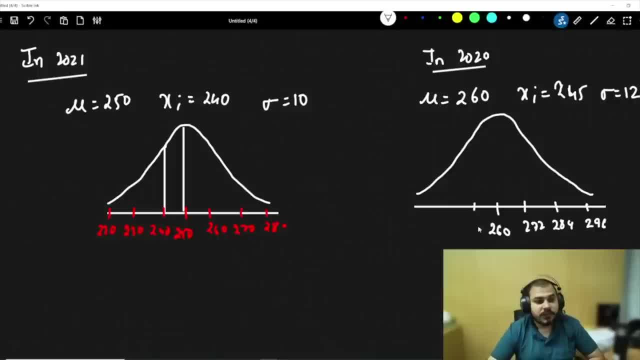 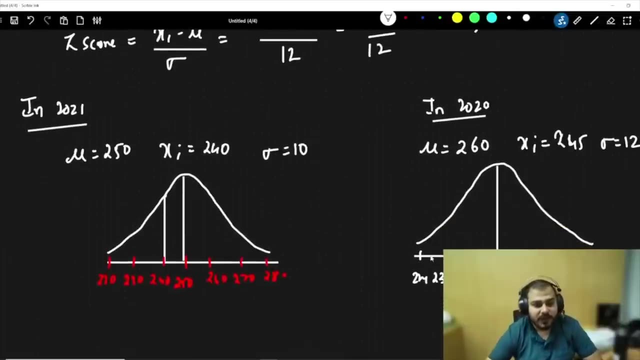 284.. Then it will become 296.. Similarly, over here it will become 248.. Then it will become 236.. Then it will become 224.. So here I have my value over here. And what is the standard deviation? Over here it is 1.25.. So 1.2 minus 1.25, is this specific? 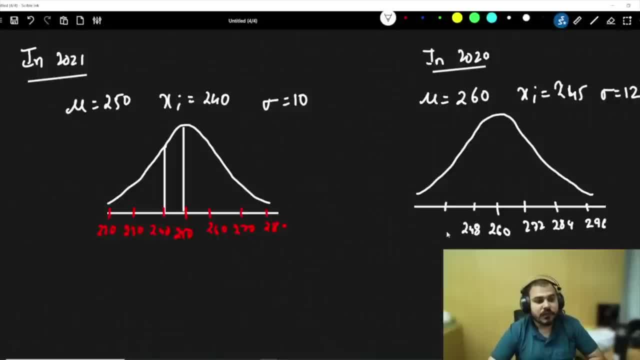 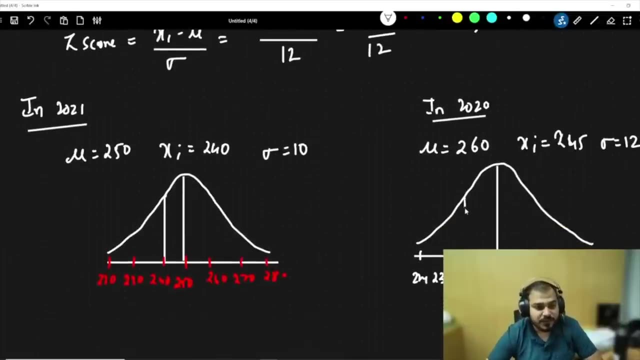 Similarly, over here it will become 248.. Then it will become 236.. Then it will become 224.. So here I have my value over here. And what is the standard deviation? Over here it is 1.25.. So minus 1.25 is this specific standard deviation. 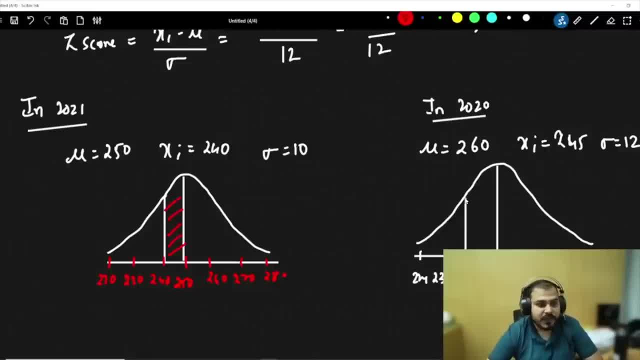 Now here you can see, the area is little bit less. Here the area is little bit less. Here the area is little bit more. So where do you think India has probably performed well in the final match? In the final match, whether India performed well in 2020 or in 2021?? 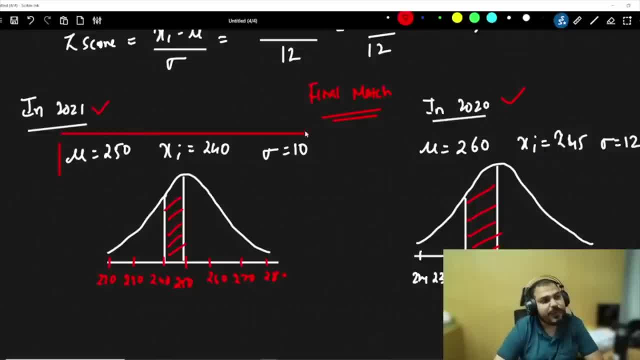 Based on this information. This information basically tells many things about probably the pitch condition. Whenever we say the standard deviation is less, that basically means most of the score was rotating around that much values. So tell me where probably India may have performed well. 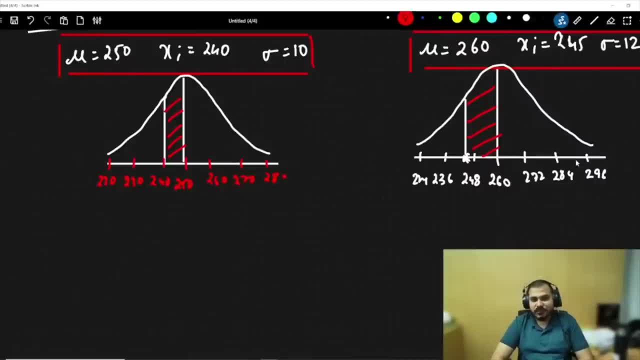 Understand guys. here the standard deviation is more, Here the standard deviation is less. Understand over here. obviously the z-score value is minus 1.. Here the z-score value is minus 1.25, which is greater. Okay, now let's go to one more practical example of z-score. 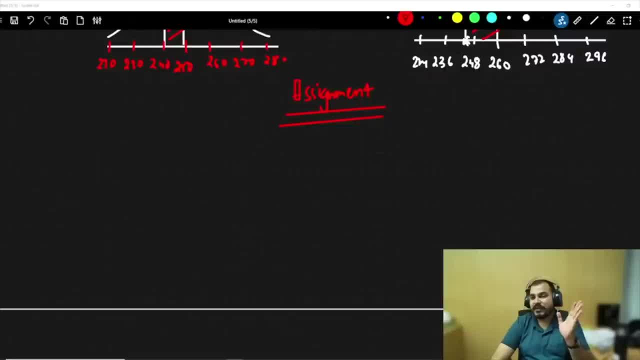 Now this example, most of the time with respect to standard deviation, most of the time with respect to statistics, will come. This may be probably asked in interviews also, And this is a very, very important and important question. I will probably take one very good example and show it to you how to be done. 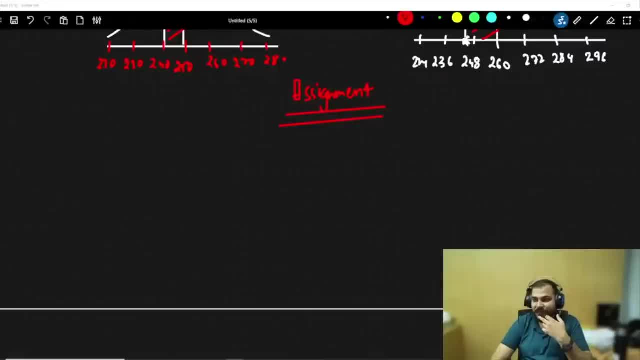 how you can basically do this and how you can actually learn it. okay. So one problem statement that I am actually going to give to you is that one example I will give you. then we will try to see. Let's consider that I have an x random variable. 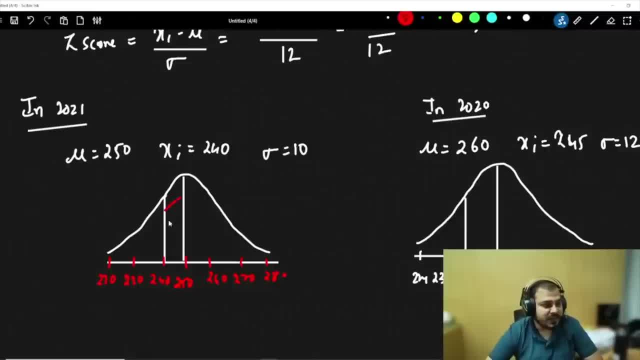 standard deviation. Now, here you can see, the area is a little bit less. Here the area is a little bit more. So where do you think India has probably performed well in the final match? In the final match, whether India performed well in 2020 or in 2021? Based on this information, 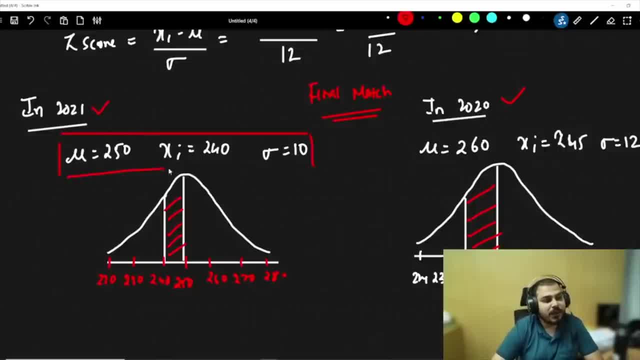 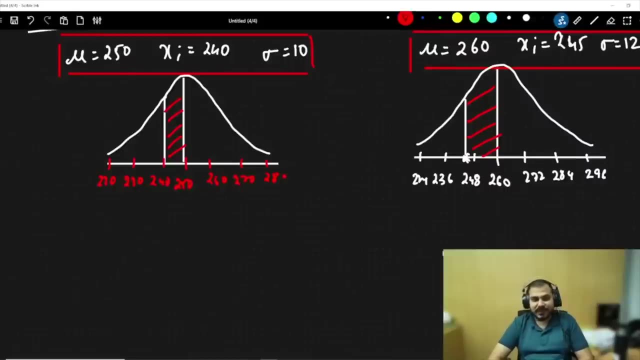 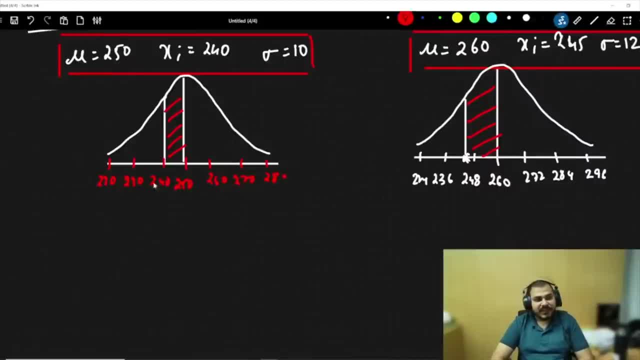 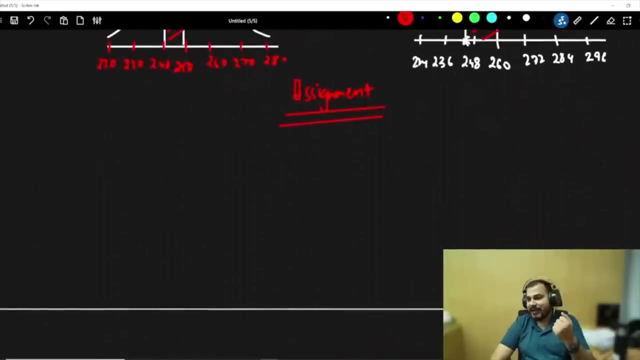 standard deviation is more. Here the standard deviation is less. Understand over. here, obviously, the Z score value is minus 1.. Here the Z score value is minus 1.. Here the Z score value is minus 1.. Here the Z score value is minus 1.25,, which is greater. Okay, now let's go to one more practical. 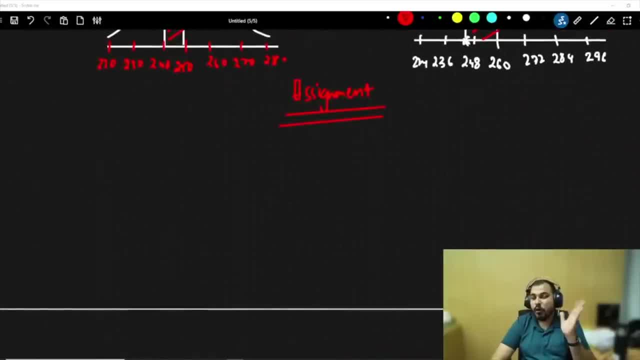 example of Z score. Now this example most of the time with respect to statistics, will come. This may be probably asked in interviews also, And this is a very, very important and important question. I will probably take one very good example and show it to you how to be done. 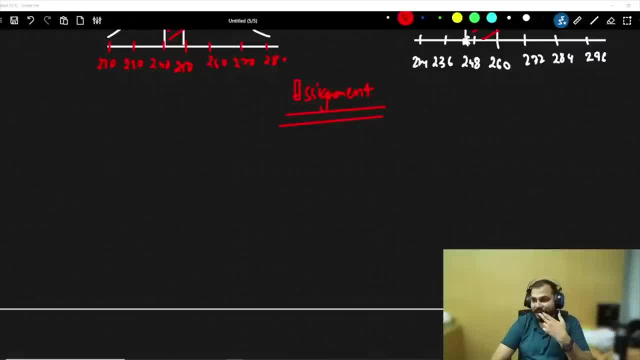 how you can basically do this and how you can actually run it. Okay, One problem statement that I'm actually going to give to you is that. one example I'll give you. then we will try to see. Let's consider that I have an X random variable. I have an X random 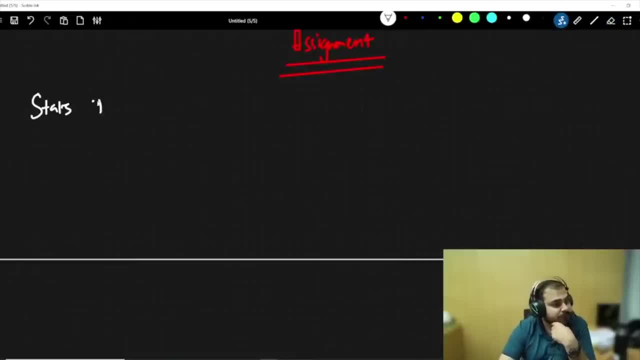 variable. So let's come to the stats interview question Now, in this stats interview question, let's say that I have a random variable X, And let's say that this random variable has this distribution: 4,, 5,, 6,, 7,, 3,, 2,. 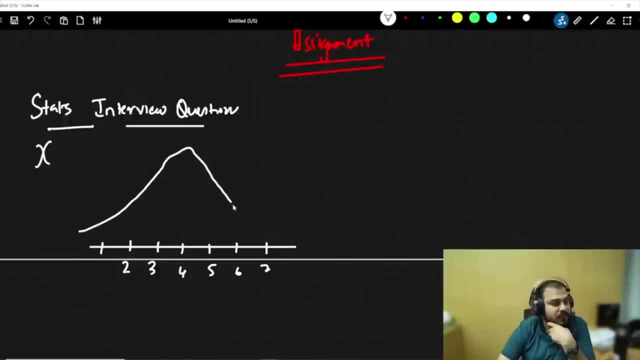 1. And let's say that I have a bell curve which looks like this. Now I want to know. my question is: what percentage of scores fall above 4.25?? Now understand one thing: where does 4.25 fall? 4.25 will fall over here. So this is basically my mean, And 4.25 will fall. 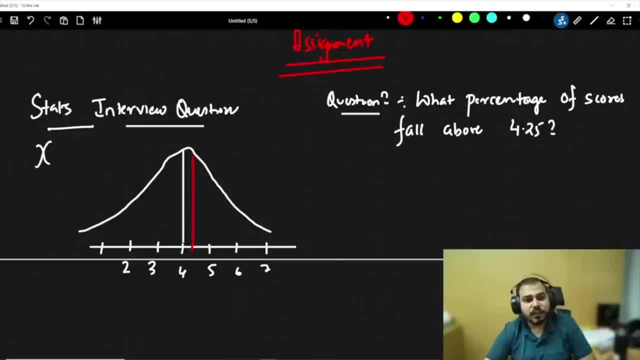 over here. Let's consider that it is falling over here. My question is that: what is the? these are my scores? right, Let's say that these are my scores: 2, 3,, 4,, 5,, 1, like, these are my. 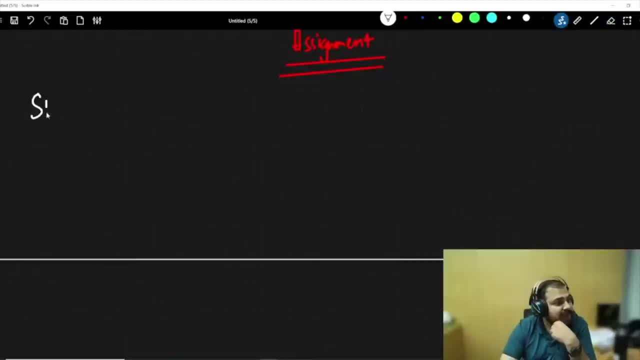 I have an x random variable. So let's come to the stats interview question Now. in this stats interview question, let's say that I have a random variable x And let's say that this random variable has this kind of distribution: 4, 5,, 6,, 7,, 3,, 2, 1.. 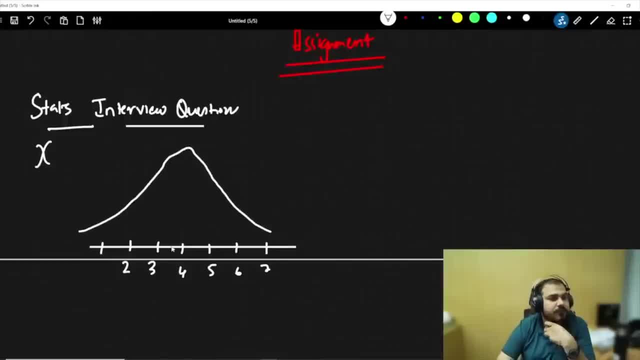 And let's say that I have a bell curve which looks like this. Now I want to know. my question is: what percentage of scores fall above 4.25?? Now understand one thing: where does 4.25 fall? 4.25 will fall over here. 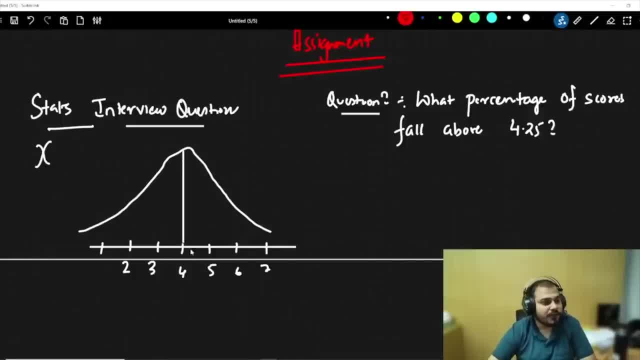 So this is basically my mean, And 4.25 will fall over here. Let's consider that it is falling over here. My question is that: what is the these are my scores. right, Let's say that these are my scores. 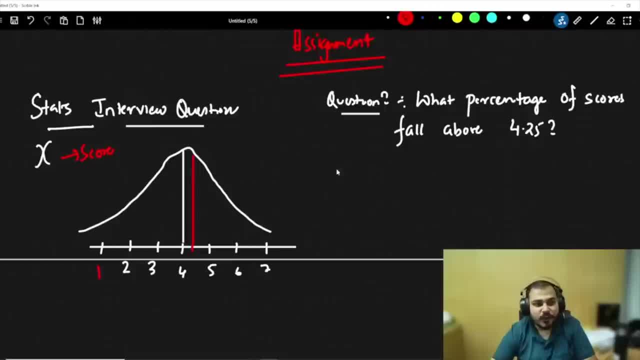 2,, 3,, 4,, 5,, 1, like these are my scores. I need to understand from this distribution, from this my entire data set, what is the percentage of scores that falls above 4.25?? That basically means I am interested in this region. 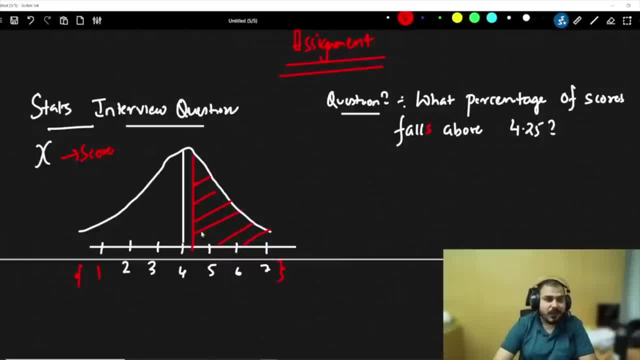 I am basically interested in this region. I am saying that what is the percentage of the scores that are greater than 4.25?? This is my question. Okay, Simple question is this, And now we will try to understand how we can use z-score in this. 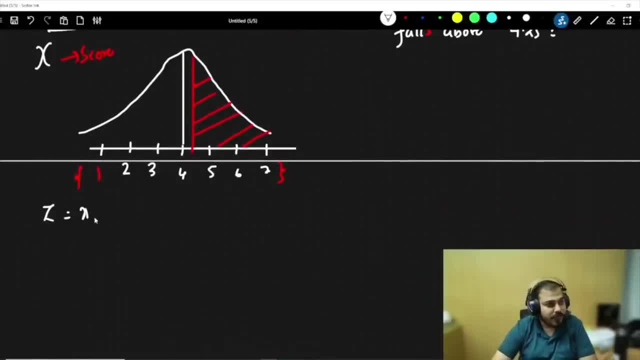 So everybody knows about z-score, Z-score, formula x of i minus mu divided by standard deviation. Here my mu is 4, standard deviation is 1.. What is my x of i? x of i is nothing but 4.25 minus 4 divided by 1.. 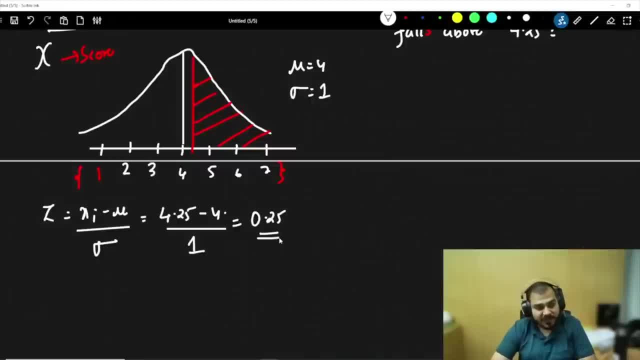 This value is 0.25 standard deviation. 0.25 standard deviation. What does this basically mean? 4.25 falls 0.25 standard deviation from the mean. Okay, From the mean. From the mean, it is basically fall into 0.25 standard deviation. 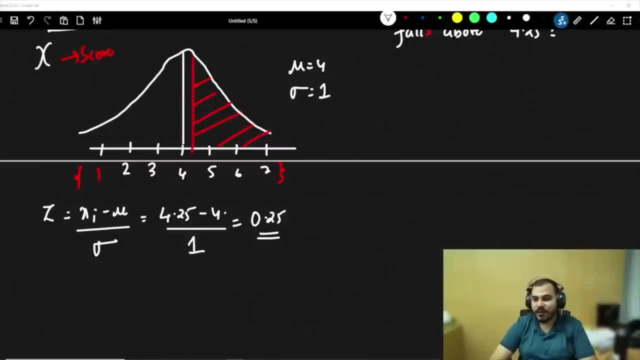 Now I got the standard deviation. This is I got with the help of z-score. But now what is the next very important thing? Obviously, from this we will not be able to understand. Okay, How much? What will be the percentage then? 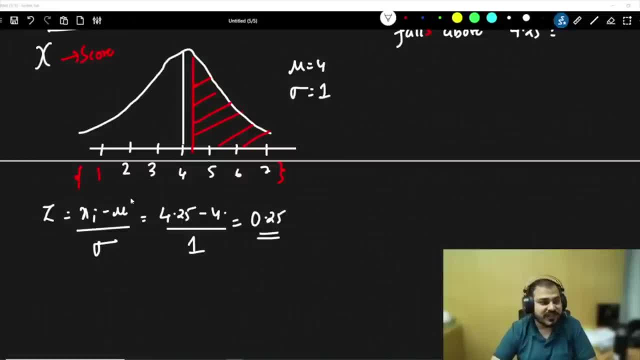 Probably this- I have got that it is 0.25. is my standard deviation or a z-score? My z-score is 0.25.. Now I need- I am interested in this region. How do I come up with the overall percentage from this particular region? 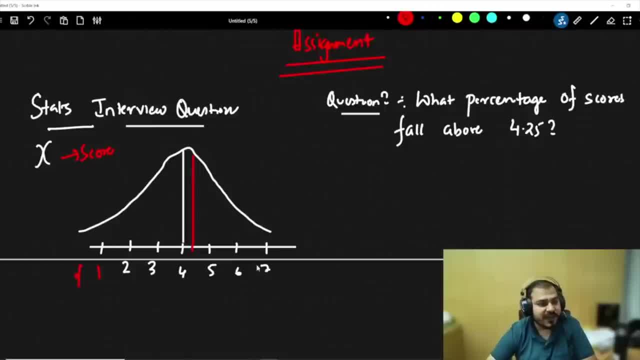 scores. I need to understand from this distribution, from this my entire data set, what is the percentage of score that falls above 4.25? That basically means I'm interested in this region. I'm basically interested in this region. I'm saying that. what is the percentage of the scores? 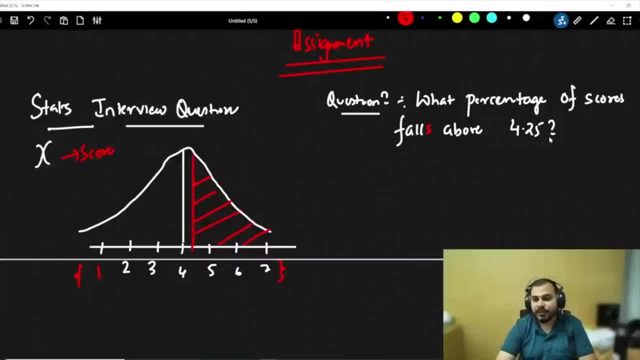 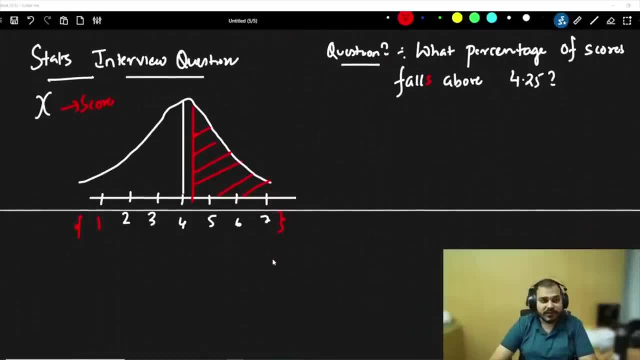 that are greater than 4.25?? This is my question. Okay, The question is this, And now we'll try to understand how we can use z-score in this. So everybody knows about z-score. formula x of i minus mu divided by standard deviation. 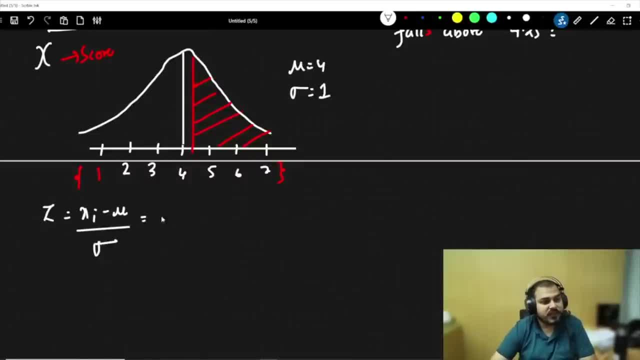 Here, my mu is 4, standard deviation is 1.. What is my x of i? x of i is nothing but 4.25 minus 4 divided by 1.. This value is 0.25 standard deviation. 0.25 standard deviation, What does? 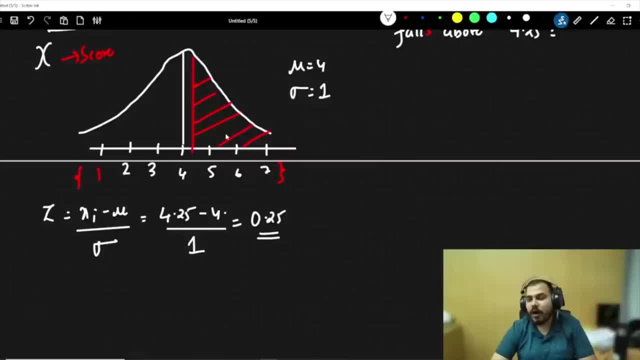 this basically mean 4.25 falls 0.25 standard deviation from the mean. Okay, From the mean. From the mean, it is basically fall into 0.25 standard deviation. Now I got the standard deviation. This is I got with the. 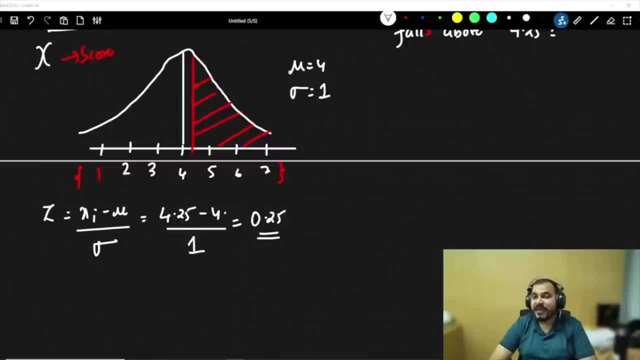 help of z-score. But now, what is the next very important thing? Obviously, from this we will not be able to understand, okay, how much. what will be the percentage then? Probably this: I have got that it is 0.25. is my standard deviation or a z-score? My z-score is 0.25.. 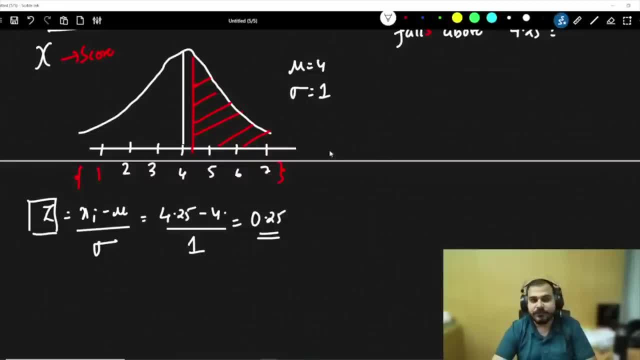 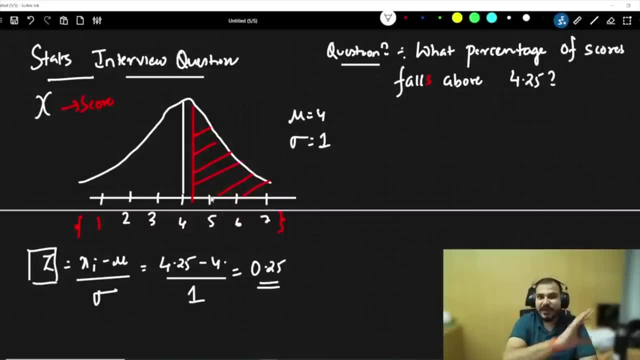 Now I need. I am interested in this region, So how do I come up with the overall percentage from this particular region? Understand one thing: This is a symmetrical bell curve. That basically means the entire area. I can basically consider it as 1.. Now, since I am interested in 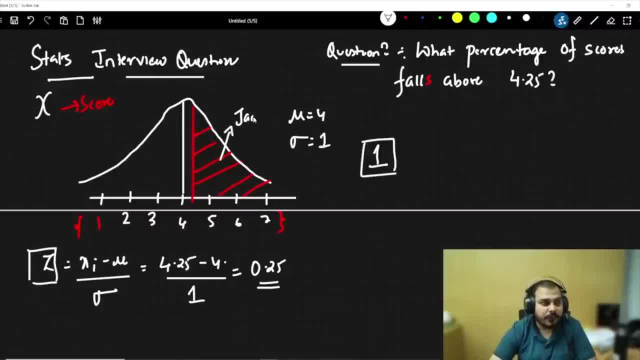 this region. I will say this region as tail Whenever we talk about tail- the region that I am actually interested in. basically, I want the value with respect to this One part of the region that's tail. The other part, that is the remaining portion, I will basically say this as body. 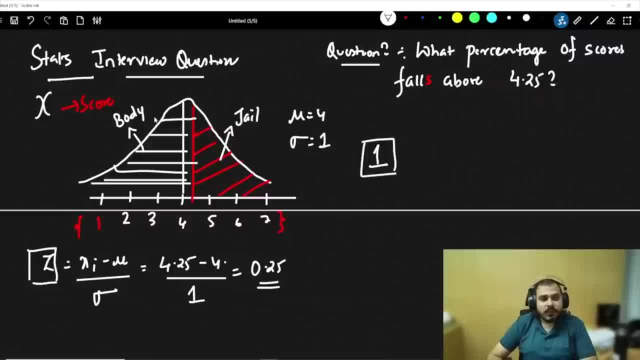 pulled from here to here. So this will basically be my body. Now understand one very important thing: How do I check, Based on this z-score, what should be the value or what should be the body curve, the area of the body curve? I want to find out what is the area of this Z-scores actually. 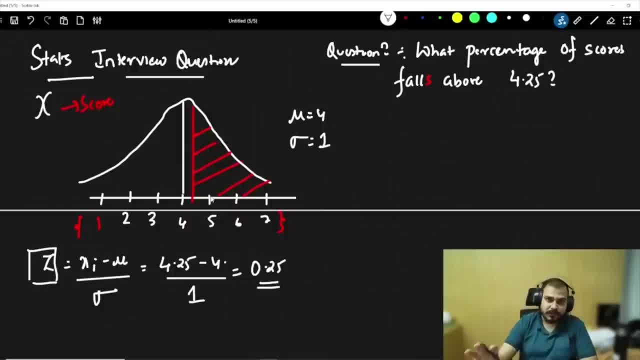 Understand one thing: This is a symmetrical bell curve. That basically means the entire area. I can basically consider it as 1.. Now, since I am interested in this region, I will say this region as tail Whenever we talk about tail- the region that I am actually interested in. basically, I want the value with respect to this. 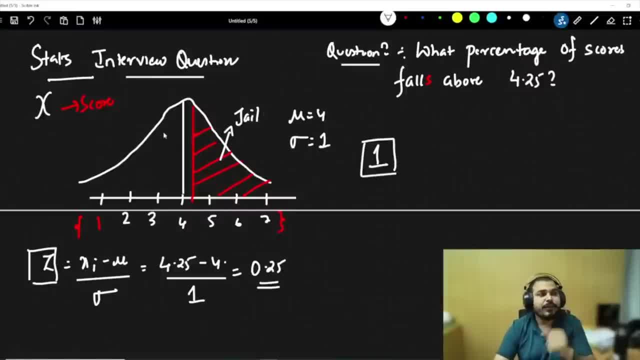 One part of the region, I will say it as tail. The other part, that is the remaining portion. Okay, I will basically say this as body Pulled from here to here. So this will basically be my body. Now understand one very important thing. 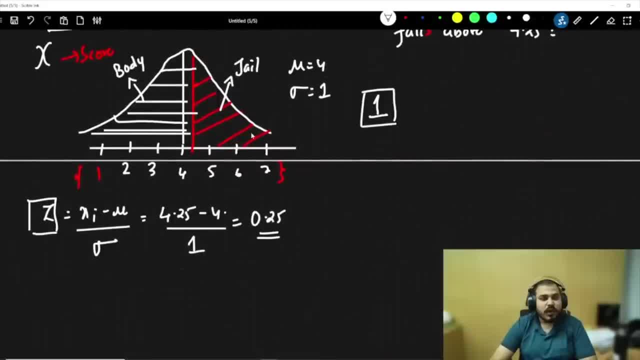 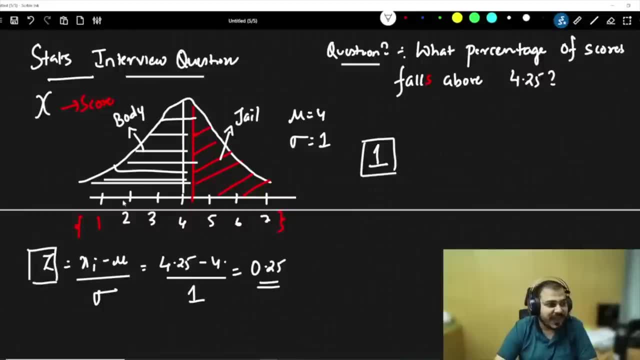 How do I check, Based on this z-score, what should be the value or what should be the body curve, The area of the body curve? I want to find out what is the area of this. Z-scores actually help you to find area of the body curve. 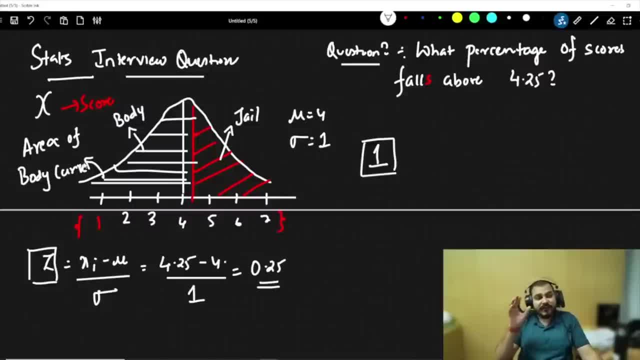 How do we find out? I will talk about it. Z-score will definitely help you to find out the area of the body curve. Now, guys, just think over it. Okay, What do you think this percentage may be? This black, this red region percentage may be. 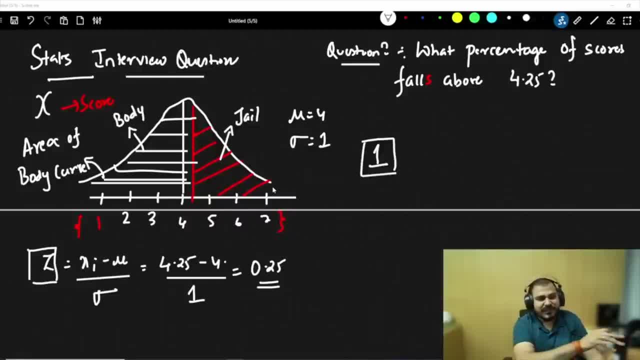 What do you think? Over here, 3 numbers are there. Let's say that total numbers are 7.. And when I say 3 numbers on the right hand side, what may be the percentage? If I say 3 by 7,, what is 3 by 7?? 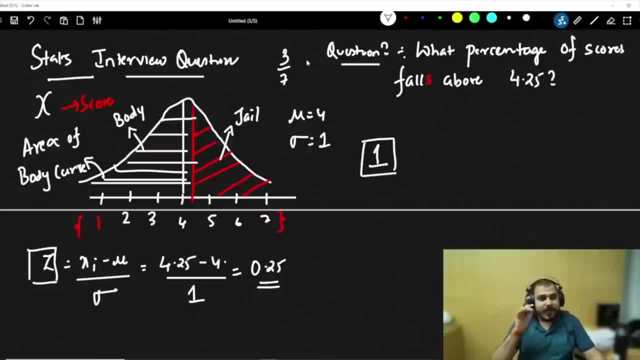 It is approximately around 48 to 49%. Right Now, can we calculate the same thing with the help of z-score? The answer is yes. I have already seen the z-value is 0.25.. Now let me do one thing. 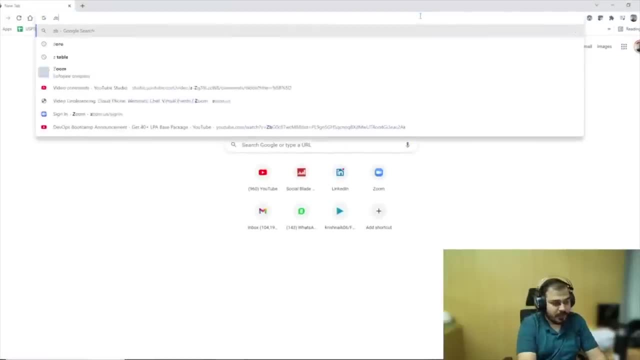 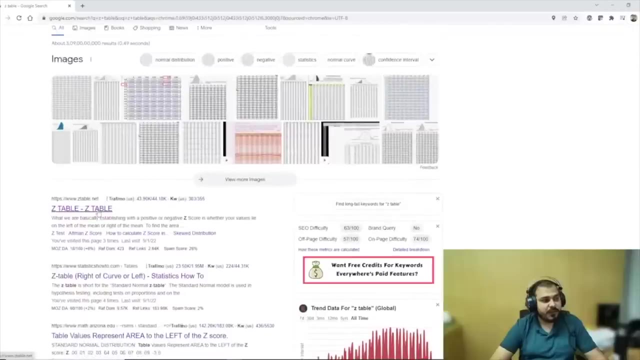 Let me open something called as z-table, Because I want to find out the area of the curve. So, z-table, if I go and search for it, you will be able to see in the first link. You will be able to see in the first link. 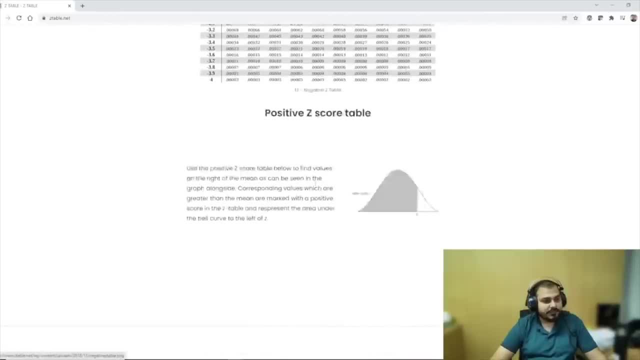 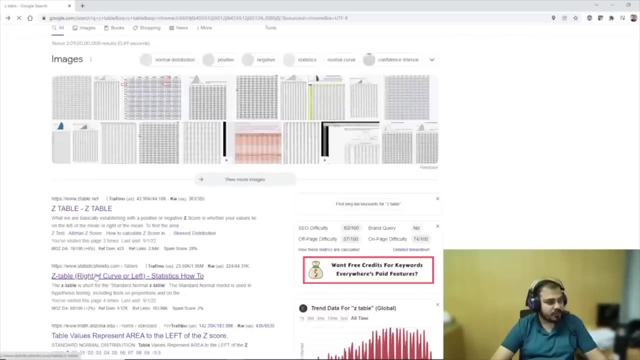 And over here. I will just go over here Now. see, This is how my z-score is. This is how my curves look like Right. See over here z-score. I will just use another table, because this table does not look right. 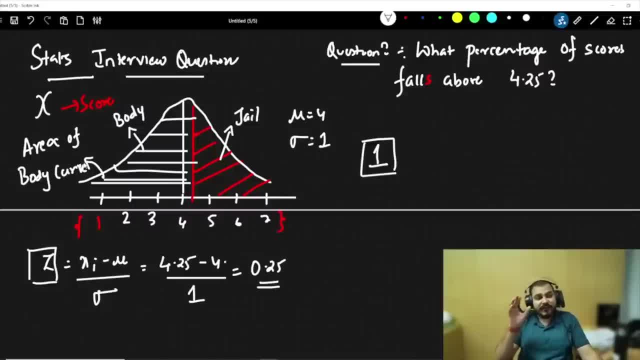 help you to find out. How do we find out. I will talk about it. Z-score will definitely help you to find out the area of the body curve. Now, guys, just think over it. okay, What do you think this percentage may be? this black, this red region percentage may be? What do you think Over here? 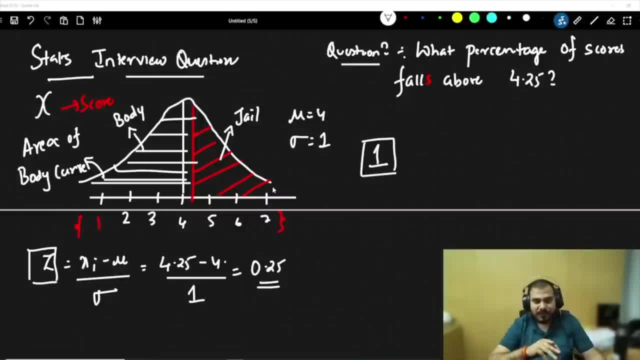 three numbers are there. Let's say that total numbers are 7.. And when I say three numbers on the right-hand side, what may be the percentage? If I say 3 by 7, what is 3 by 7? It is. 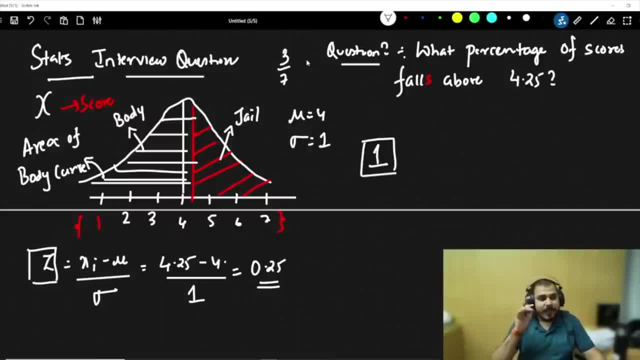 approximately around 48 to 49 percent. right Now, can we calculate the same thing with the help of z-score? The answer is yes. I have already seen the z-value is 0.25.. Now let me do one thing. 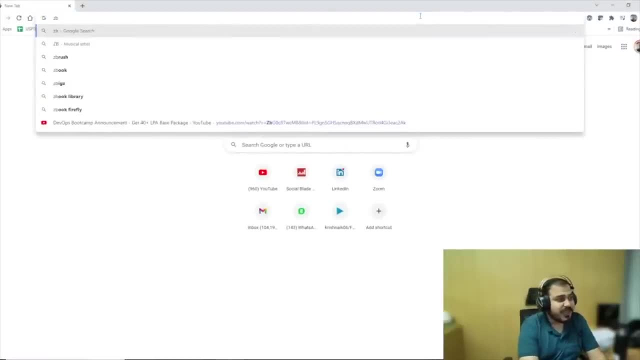 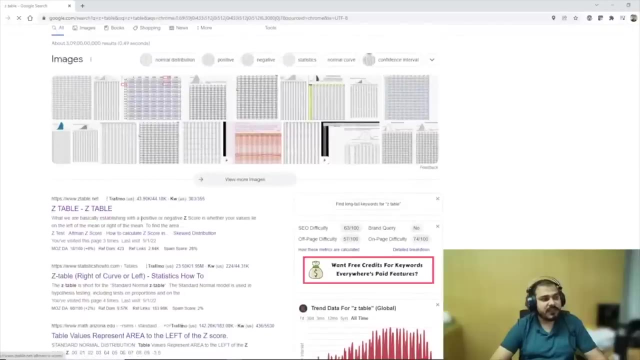 Let me open something called as z-table, because I want to find out the area of the curve. So, z-table, if I go and search for it, you will be able to see in the first link. You will be able to see in the first link And over here. I will just go over here. 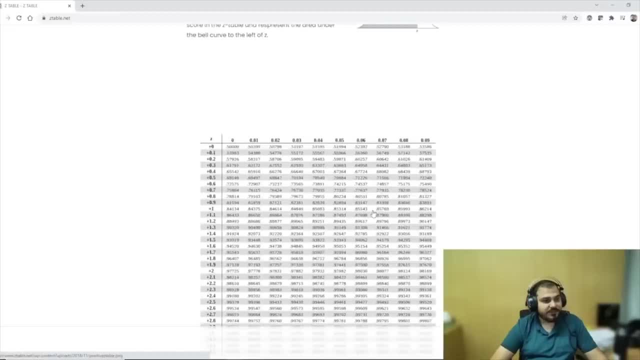 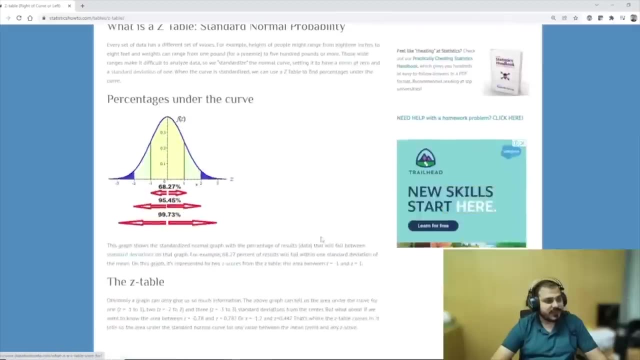 Now see, this is how my curves look like right. See over here z-score. I will just use another table because this table does not look right. okay, So let us consider this table. So always remember three types of z-score we can basically get. One is this type, which, again, I will be. 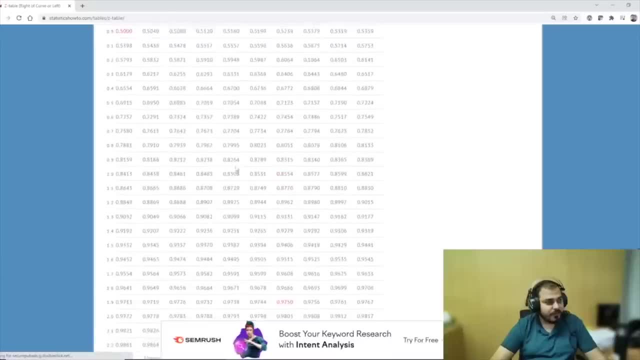 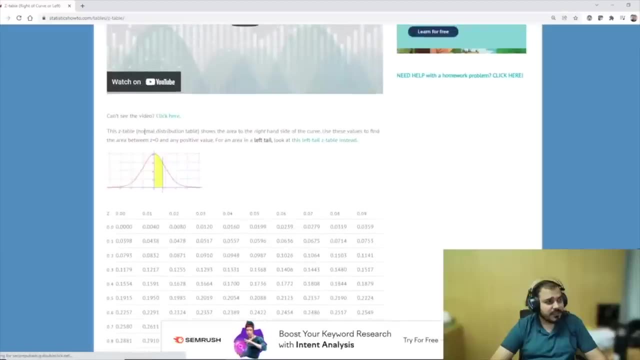 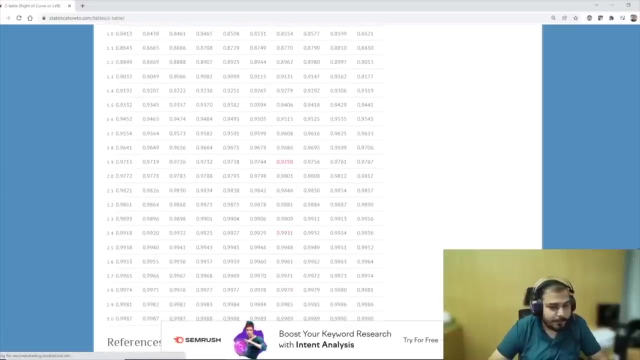 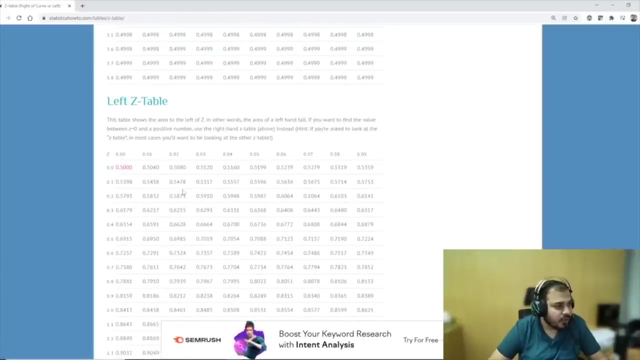 discussing One is in this type. okay, Now see this Left z-table and this is right z-table. okay, Just a second. I will just show you how to make the readings over here: 2.2.. Z is 0.25, right, 0.25.. 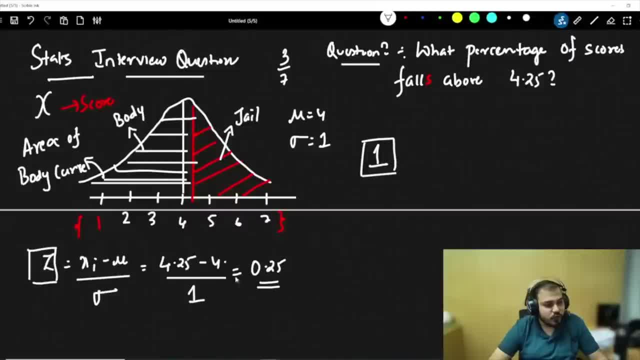 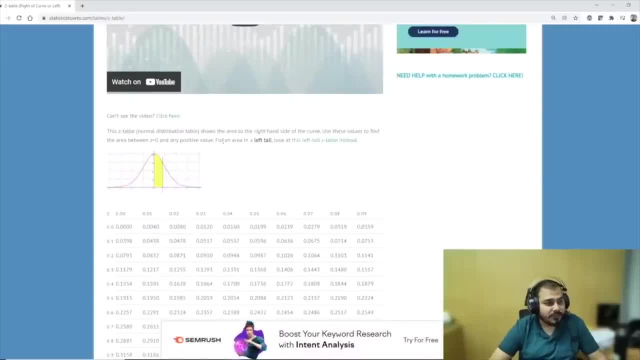 See over here what is my z-score from here. What is my z-score over here: 0.25.. And remember, this z-table will be giving me the area of the body curve. See, a z-table shows the area to the. 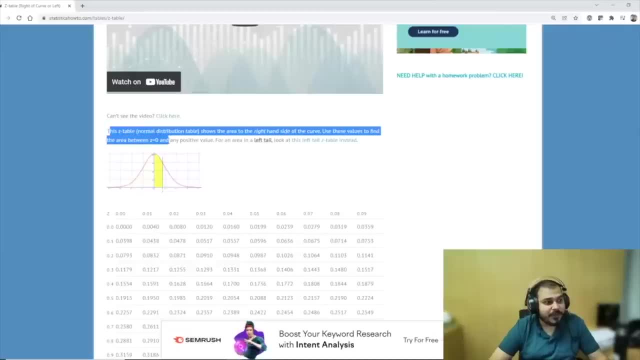 right-hand side of the curve. Use these values to find the area of the body curve. So let us look at: the area between z is equal to 0 and any positive value For area in the left table. look at the left-tail z-table instead. okay, If you want to find out the area in the left-tail search. 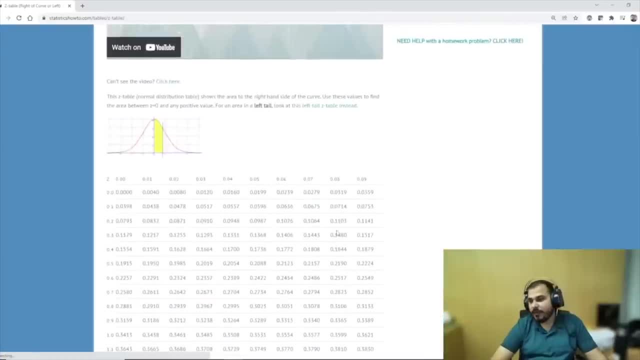 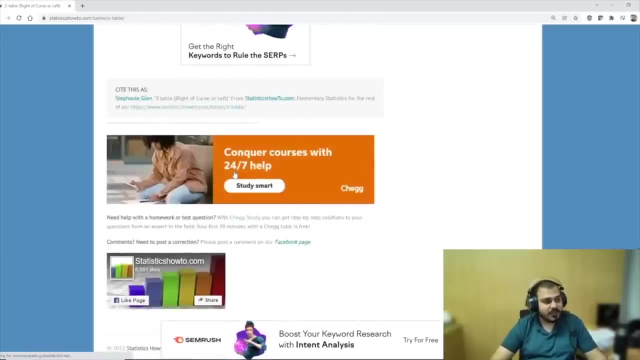 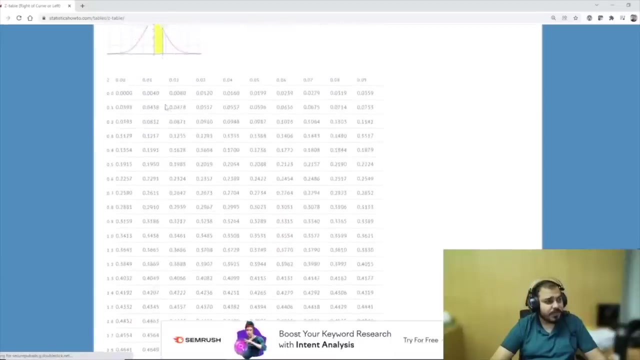 Okay, So let's consider this table. So always remember 3 types of z-score we can basically get. One is this type, which, again, I will be discussing. One is in this type. Okay, Now see this Left z-table and this is right z-table. 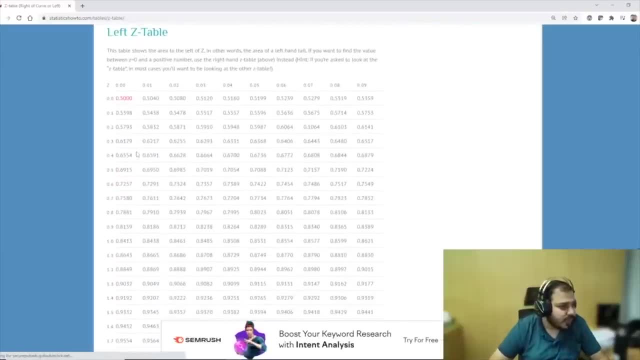 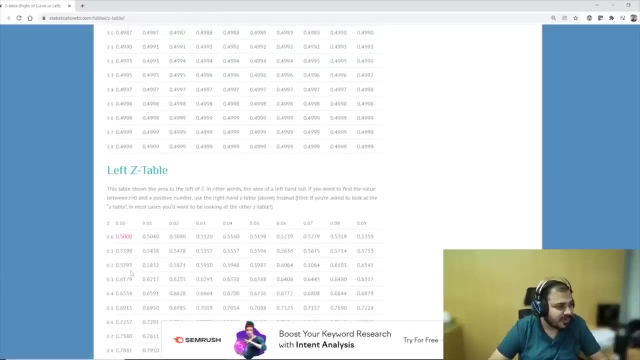 Okay, Just a second. I will just show you how to make the readings over here. 2 point: 2: point z is 0.25.. Right, 0.25.. See over here What is my z-score from here. 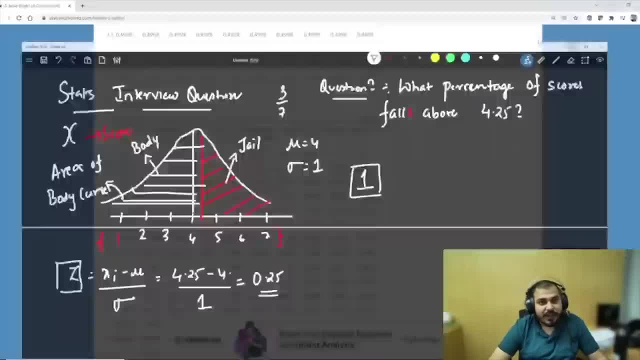 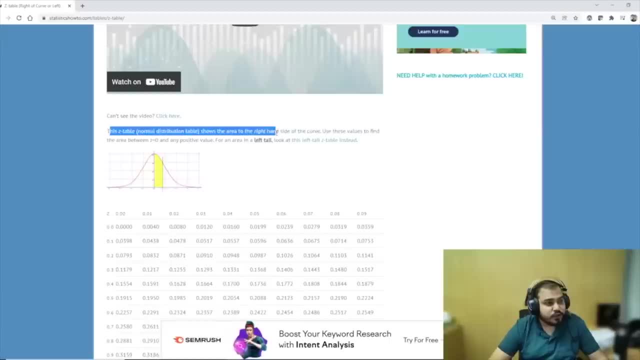 What is my z-score over here? 0.25.. And remember, this z-table will be giving me the area of the body curve. See, A z-table shows the area to the right hand side of the curve. Use these values to find the area between. z is equal to 0.25.. 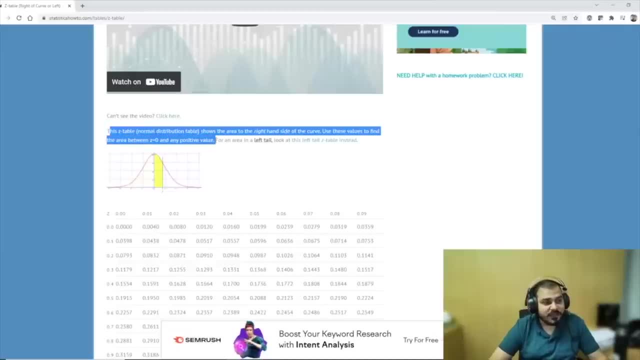 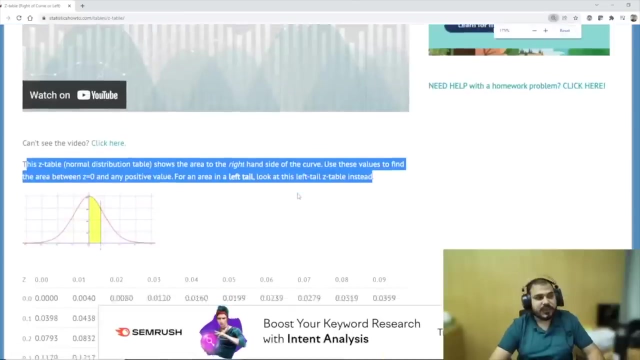 Okay, The area between z is equal to 0 and any positive value For area in the left table. look at the left tail z-table instead. Okay, If you want to find out the area in the left tail, search for it guys. 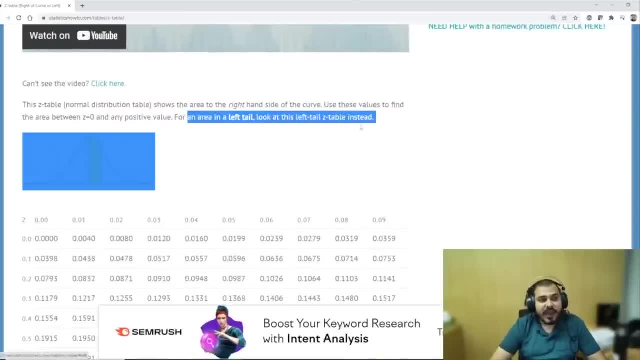 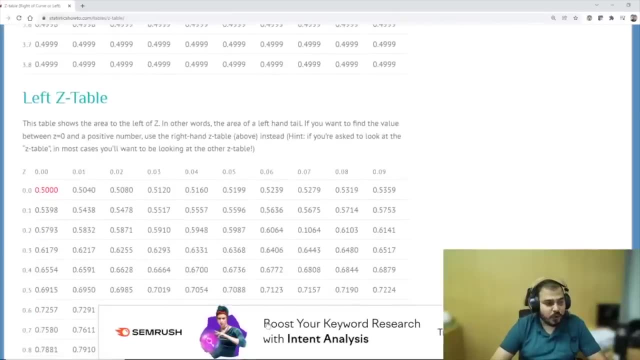 If you want to find an area in the left tail, look at the left tail z-table. instead. In this particular case, let me take left z-table Because I want to look at the area of this. See this, guys: This is the area. 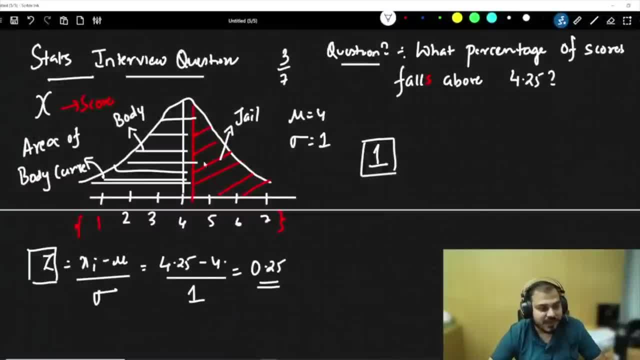 Right now, this area. I want to get the answer Right. If I get the answer of this area, I can just subtract 1 minus the left area. I want to get this particular area. Let me explain once again. Okay, Everybody is able to see this. 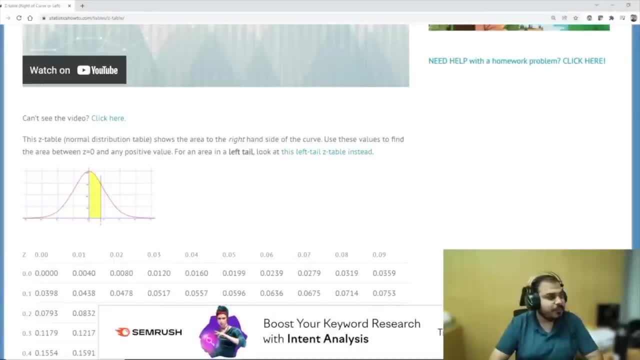 Over here. just see the very, very important thing. The z-table shows the area to the right hand side of the curve. Use these values to find the area between 0 and any positive value. Okay For area in the left tail. look at the left tail z-table instead. 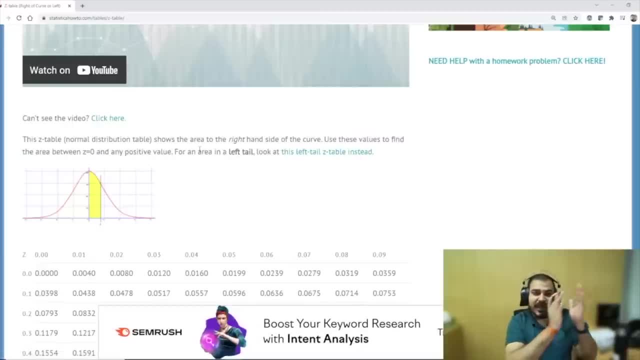 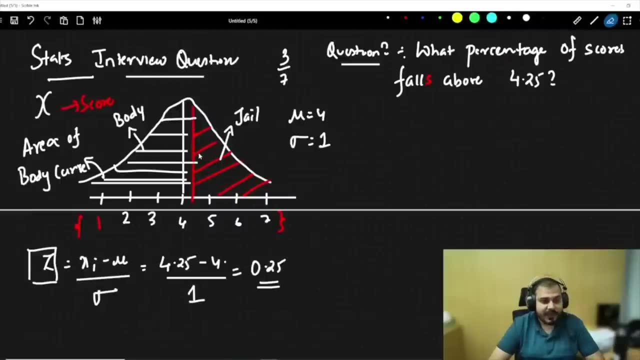 So here you can see that I want to see the left tail or right tail. Okay, What you want to see? Okay, First of all, see that You come to this particular diagram. You want to see this part or this part. 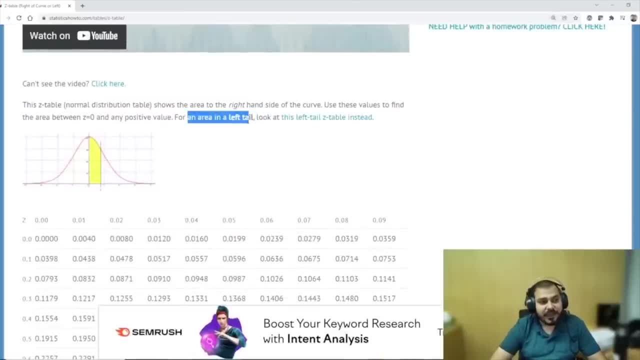 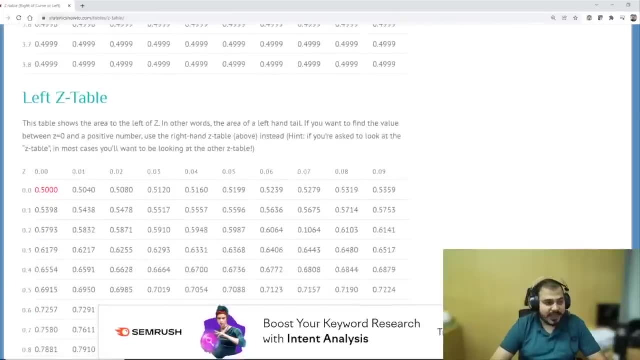 for it guys. If you want to find an area in the left-tail, look at the left-tail z-table. instead, In this particular case, let me take left z-table, because I want to look at the area of this See. 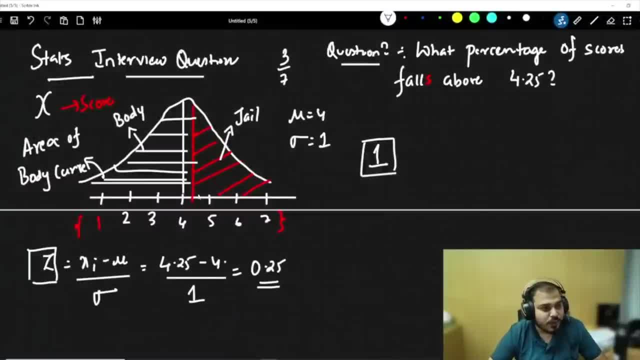 over here. this is the area Right now, this area. I want to get the answer right. If I get the answer of this area, I can just subtract 1 minus the left area. I want to get this particular area. 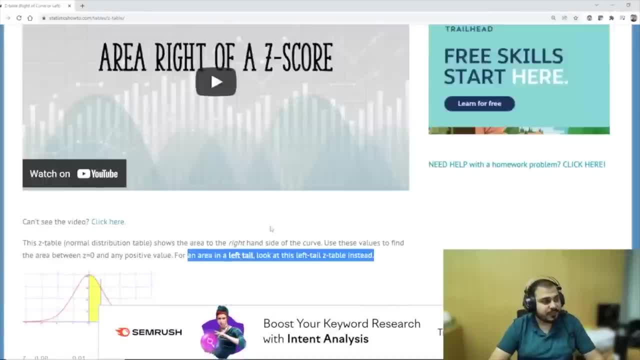 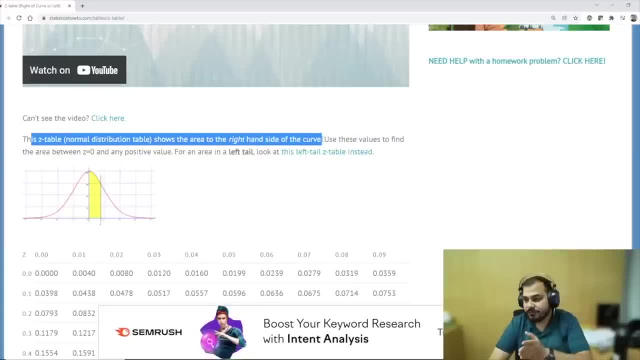 Let me explain once again. Okay, everybody is able to see this Over here. just see very, very important thing: The z-table shows the area to the right-hand side of the curve. Use these values to find the area between 0 and any positive value. 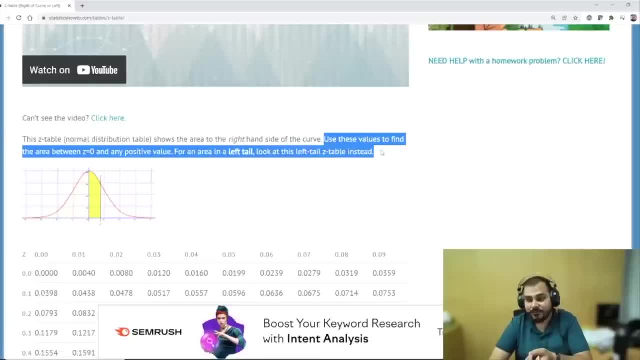 If you want to find out the area in the left-tail, look at the left-tail z-table instead. So here you can see that I want to see the left-tail or right-tail. okay, What do you want to see? 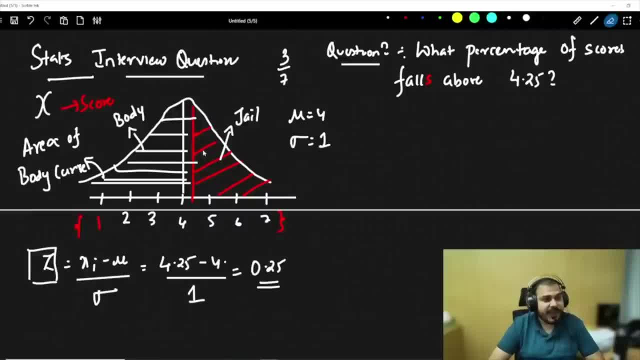 Okay, first of all, see that You come to this particular diagram. You want to see this part or this part. Obviously, you want to calculate this part. But understand one thing: In order to calculate this part, if I get the value of this part, I can just subtract 1 minus. 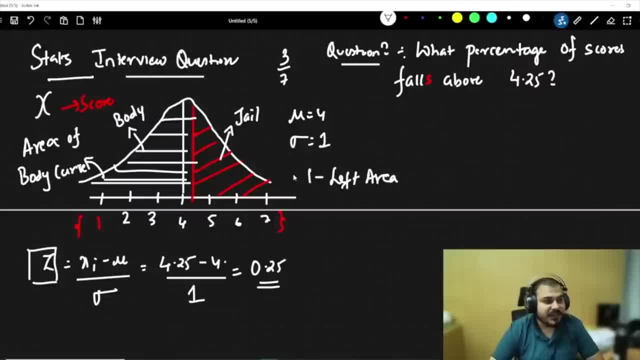 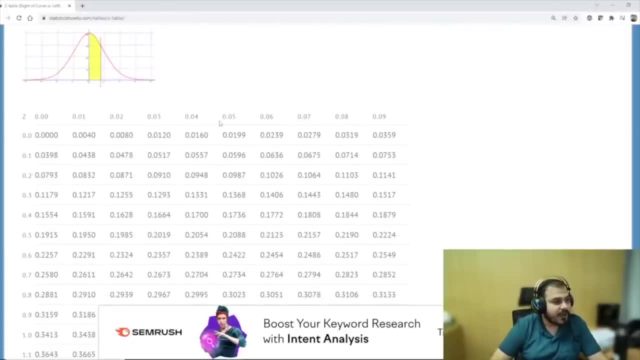 left area right. If I subtract 1 minus left area will I not be able to get the right part. Otherwise you directly go and see in the right-table. Otherwise, directly go and see in the right-table Again. I am showing you Here. you can see 0.25, 0.25, right, So 0.25,. 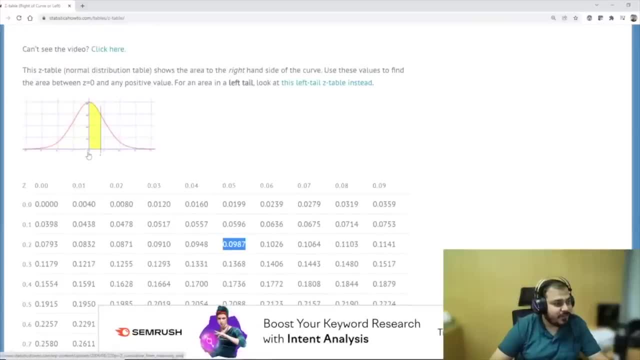 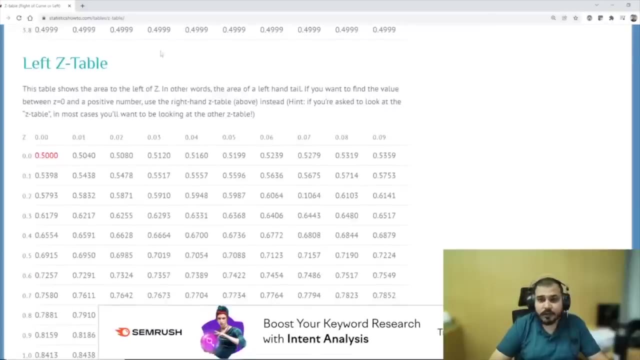 you will be able to see this much. This area will be giving from mean to this standard deviation. Right-table is given. Don't worry, Left-table is also given. See over here. left-table is also given. You can also check this. This table will be giving you the value. 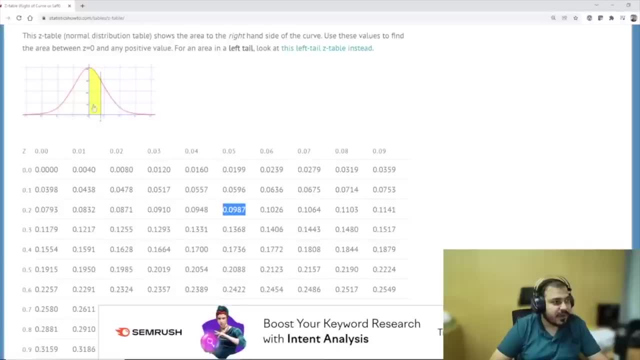 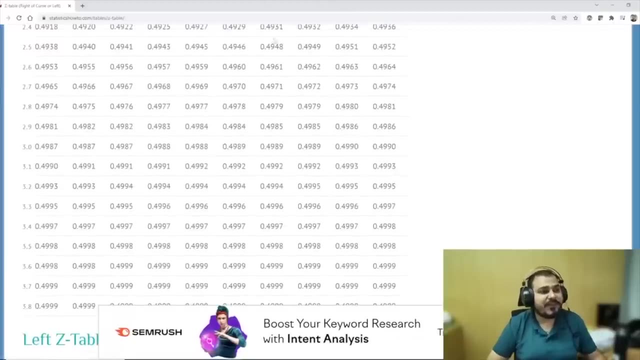 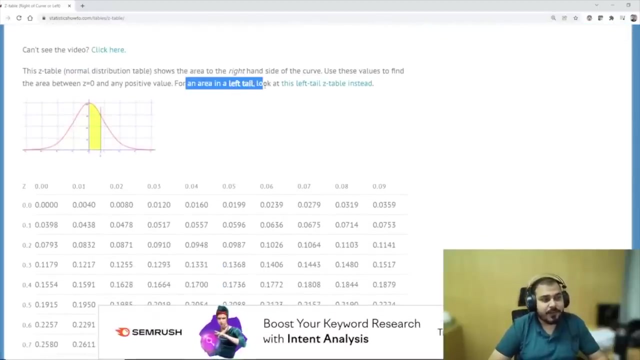 between this to this, Then probably you have to find out this one, or subtract 1 minus this area, Then you will be able to understand it. Now I will go to the left-table Understand Again. I am going to repeat guys Here. clearly it is given that for area in left-table, left-tail, 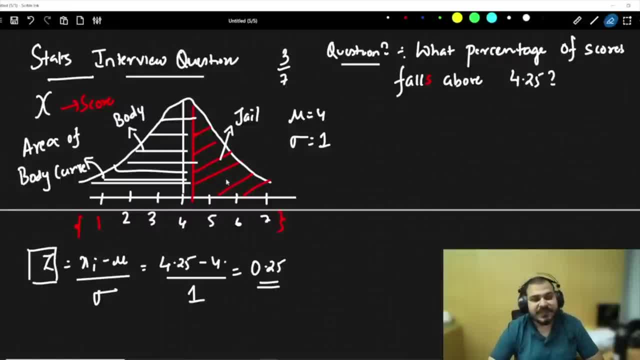 Obviously you want to calculate this part. But understand one thing: In order to calculate this part, if I get the value of this part, I can just subtract 1 minus left area. Right, If I subtract 1 minus left area, will I not be able to get the right part? 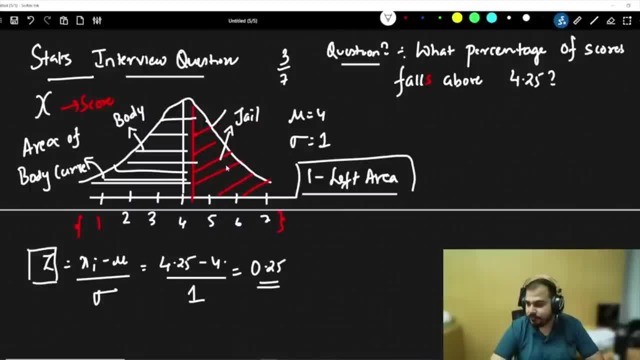 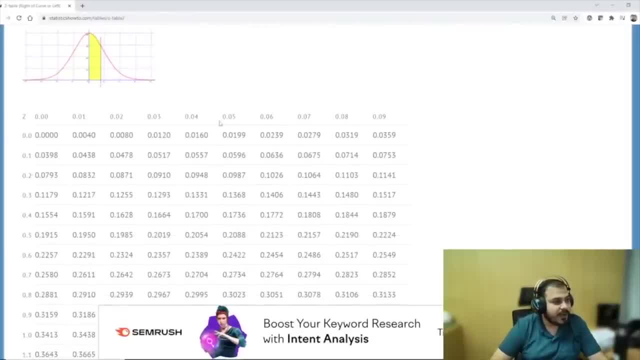 Otherwise, you directly go and see in the right table. Otherwise, directly go and see in the right table. Again, I am showing you Here. you can see 0.25, 0.25.. Right, So 0.25, you will be able to see this much. 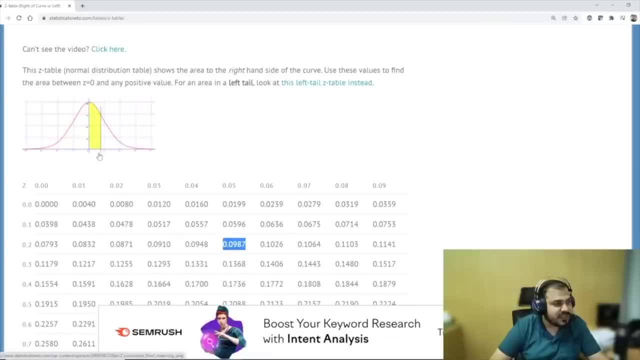 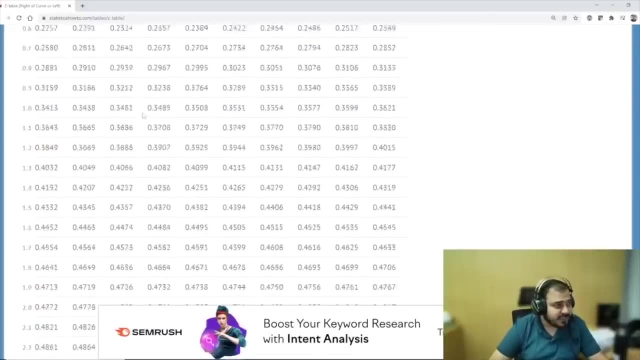 This area will be giving from mean to this standard deviation. Right table is given. Don't worry, Left table is also given. See over here, Left table is also given. You can also check this. This table will be giving you the value between this to this. 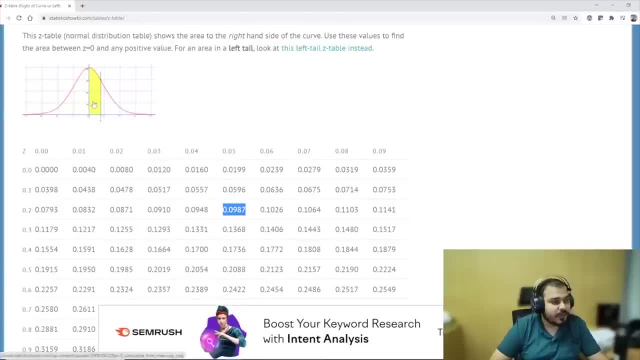 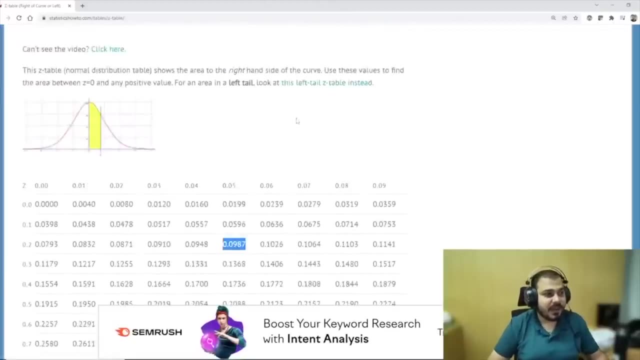 Then probably you have to find out this one, or subtract 1 minus this area, Then you will be able to understand it. Now I will go to the left table. Understand Again. I am going to repeat guys Here. clearly it is given that for area in left table, left tail, look at the left tail. 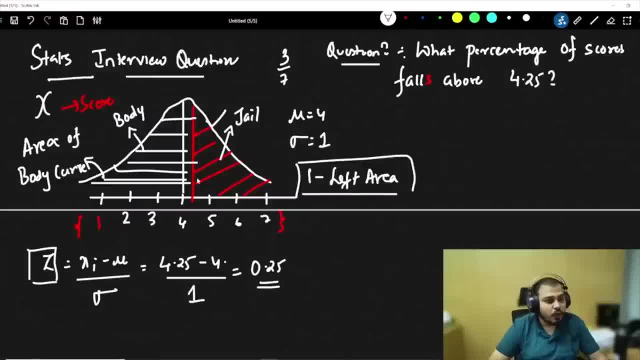 Z table. Why I am seeing left tail? Because if I go over here, this is my right tail, This is my remaining body. Left tail can become this part, So from the entire body. if I subtract 1 minus this, I will be able to get this. 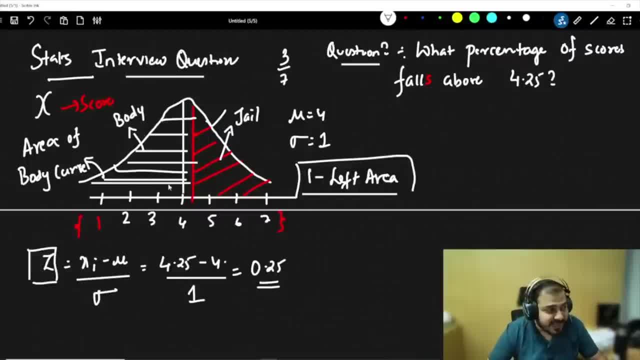 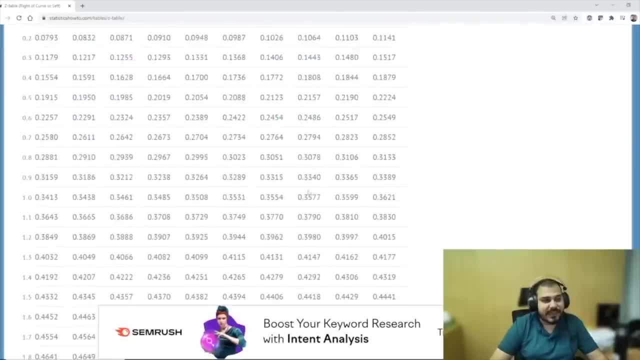 Very much simple. Now how do I check this? I will go over here. It has given me the instruction over here For area in left tail: look at left tail Z table instead. So if I go and see, this is my left Z table. 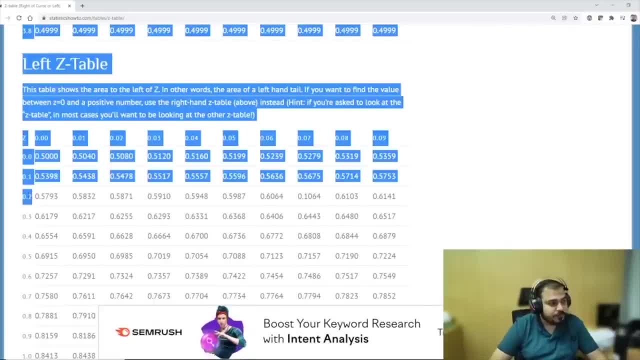 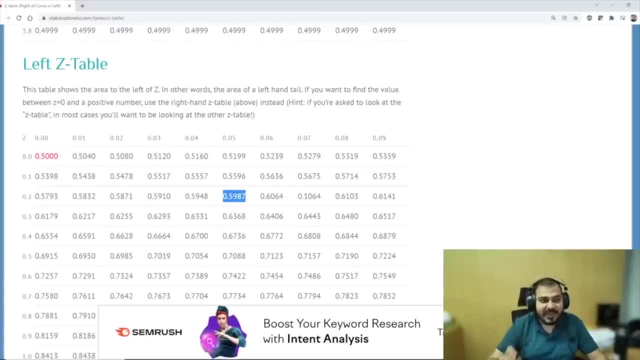 Now I will go and find out the Z value of 0.2 and 0.2 and 5.. So how much? I am getting? 0.5987.. So 0.5987 will be my value of this. 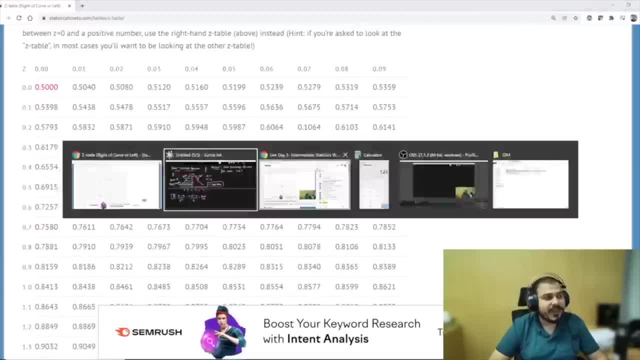 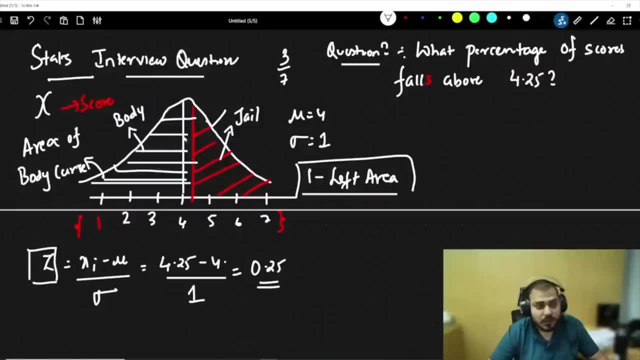 look at the left-tail z-table. Why I am seeing left-tail? Because if I go over here, this is my right-tail, This is my remaining body. Left-tail can become this part, So from the entire body. if I subtract 1 minus this, I will be able to get this Very much simple. 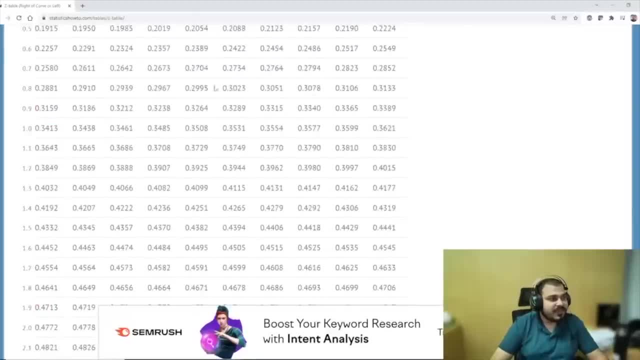 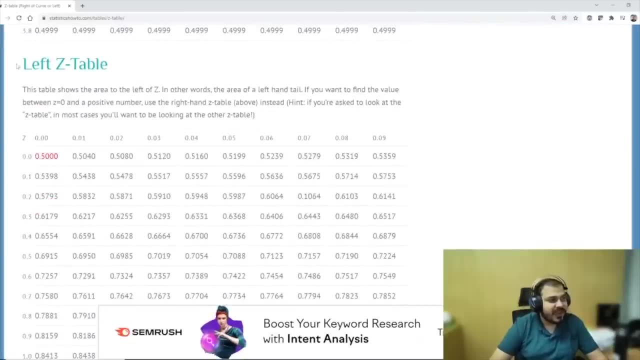 Now, how do I check this? I will go over here. It has given me the instruction over here for area in left-tail: Look at left-tail z-table instead. So if I go and see this is my left z-table, Now I will go and find out the z-value of 0.2 and 0.2 and 5.. 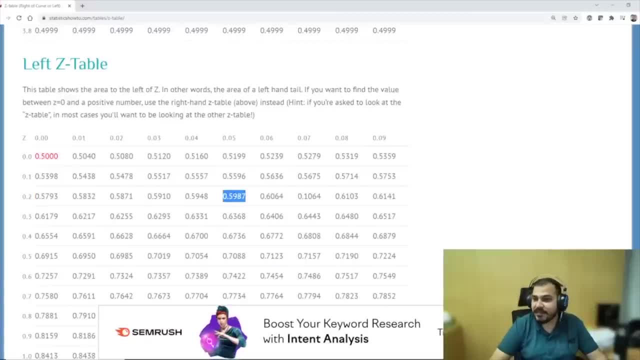 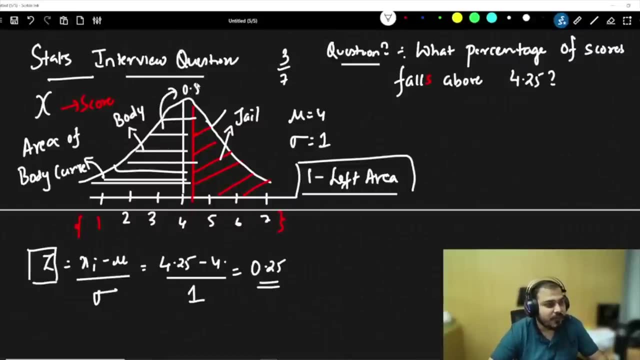 So how much? I am getting 0.5987.. So 0.5987 will be my value of this. My area of the body curve will be 0.5987.. Now, in order to find out this, I will subtract 1 minus 0.5987.. 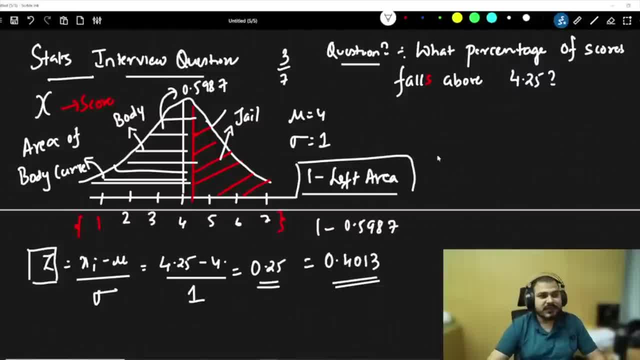 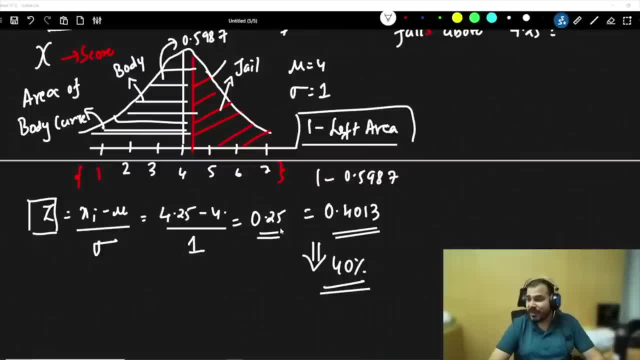 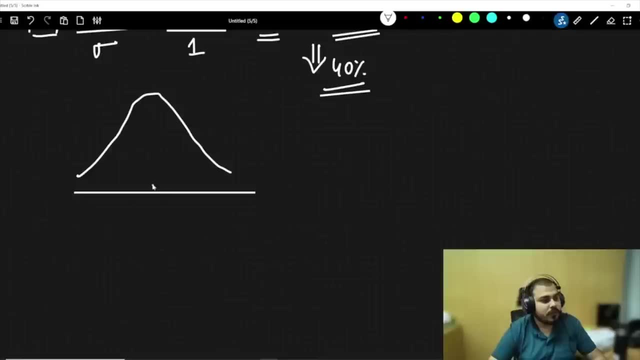 0.4013.. So what is the percentage of scores that fall above 4.25?? It is nothing but 40 percentage. Why subtracting from 1?? It's very simple. no See, guys. again I am talking about this. My question is that this: 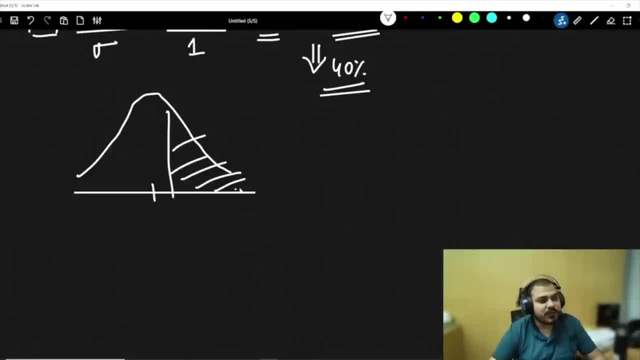 is my mean From this particular curve. I want to find out what is the percentage of the distribution, Then what I can do. if I want to find out this curve, I can take this whole curve subtract with the left one, Then I will be getting this one. So here you are. 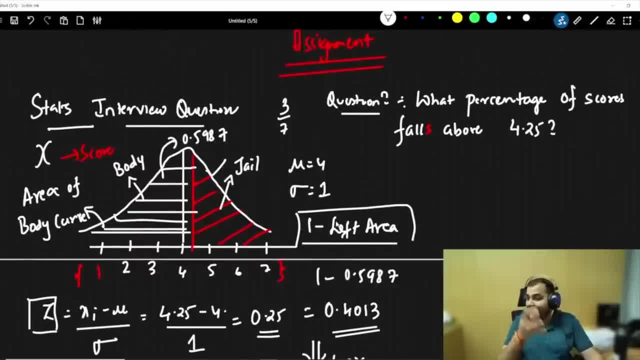 able to get 40%. Now did you understand how important it is basically to understand z-score? Yes, 0.59 is the mean to all the left, this entire region, From this to this, from 0.25 standard deviation to the left part. Now did you find out how? 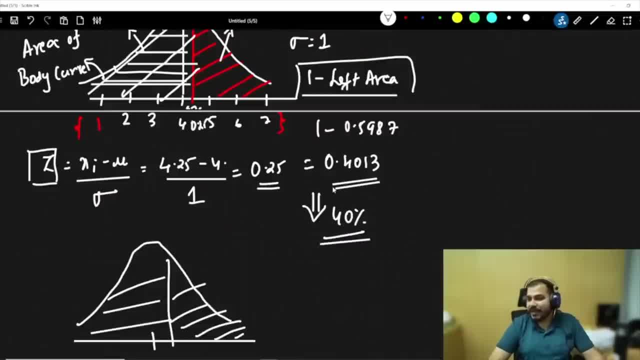 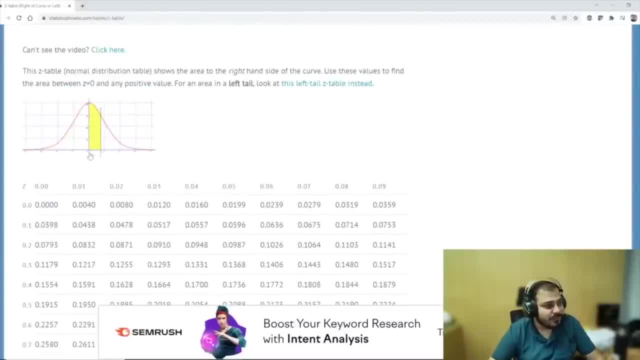 important. this is for the interview questions, guys. Why not directly taking from the right table? Understand, guys: right table is not given. No, This is not right table. This is only given from here to here. If you want to find out from left table, then this is the diagram for this. 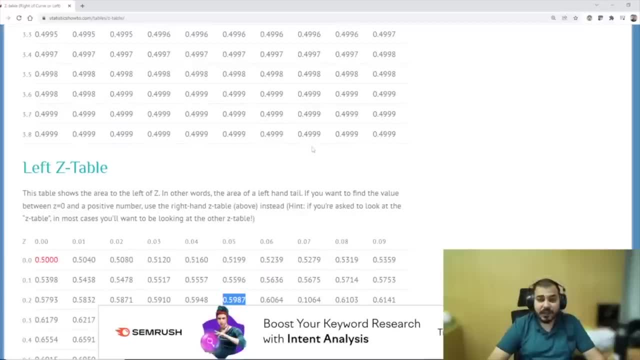 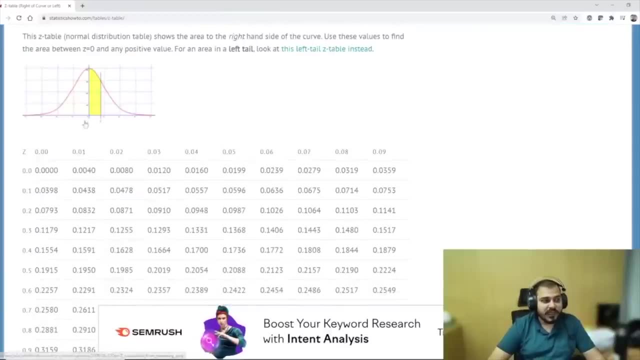 for left z-table. Understand one thing very much important: You cannot take it from right table. Right table there is no information About it. you can see this graph Right. It is only giving information from here to here. In the left table you will be able to get the information of the body of of the area. 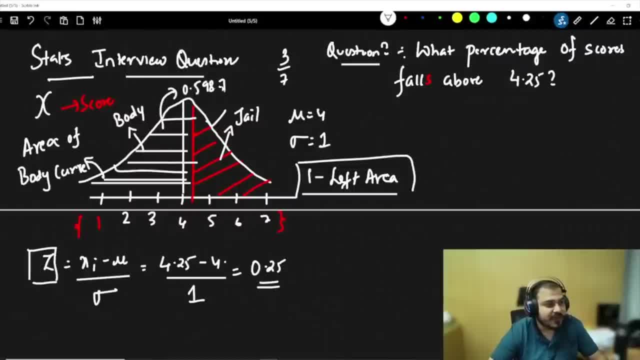 My area of the body curve will be 0.5987.. Now, in order to find out this, I will subtract 1 minus 0.5987.. 0.4013.. So what is the percentage of scores that fall above 4.3?? 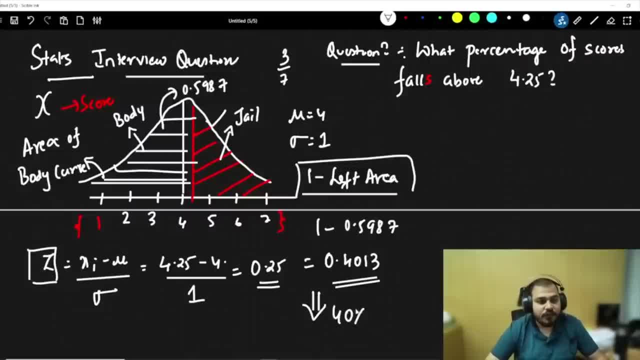 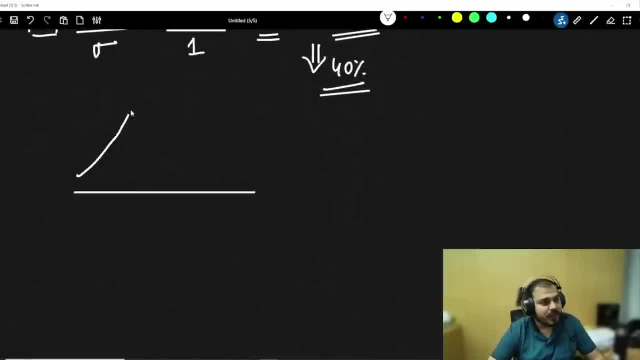 It is nothing but 40%. Why subtracting from 1?? It's very simple. no See, guys. again I am talking about this. My question is that this is my mean. From this particular curve, I want to find out what is the percentage of the distribution. 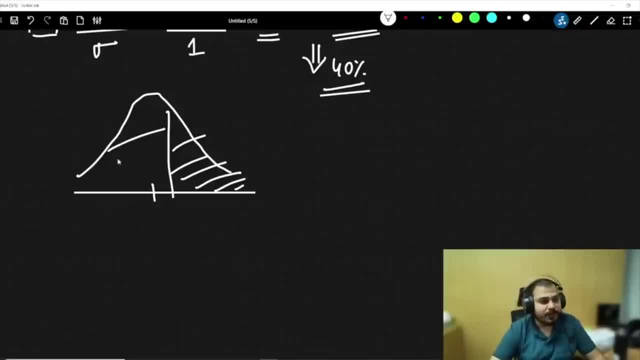 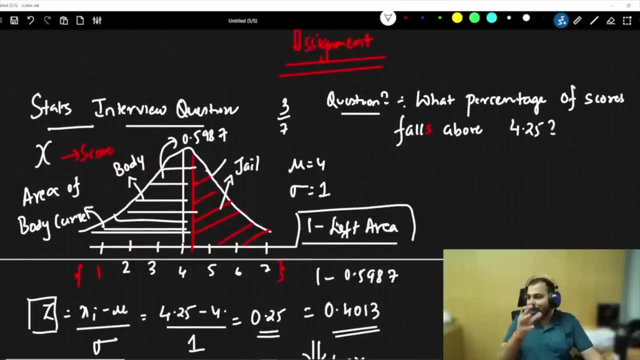 Then what I can do. if I want to find out this curve, I can take this whole curve subtract with the left one. Then I will be getting this one. So here you are able to get 40% Now, did you understand? 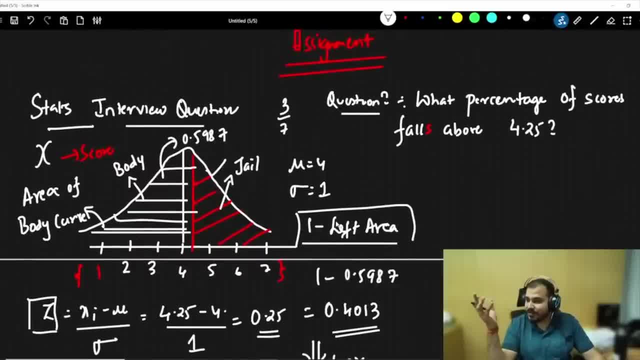 How important it is basically to understand z-score. Yes, 0.59 is the mean to all the left, This entire region, From this to this, From 0.25 standard deviation To the left part. Now did you find out how important this is for the interview questions, guys? 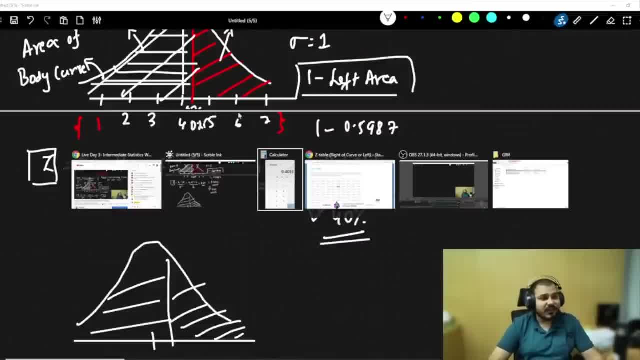 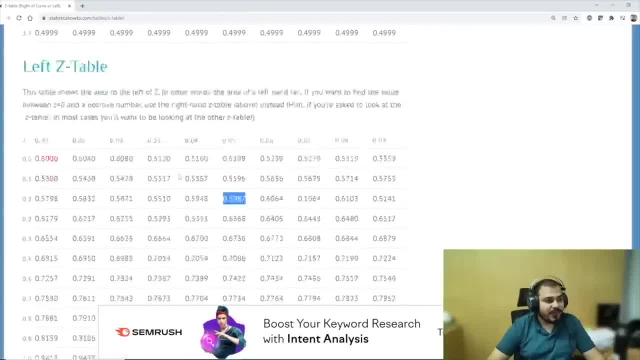 Why not directly taking from the right table? Understand guys, right table is not given. No, This is not right table, This is only given from here to here. If you want to find out from left table, then this is the diagram for this. 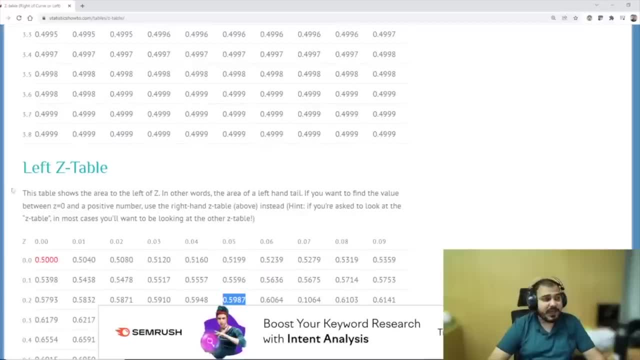 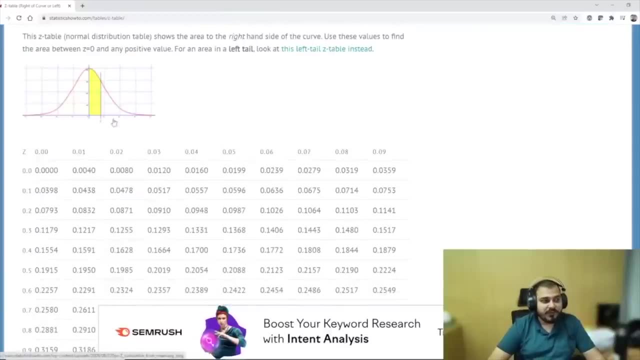 For left z-table. Understand one thing Very much important: You cannot take it from right table. Right table there is no information about it. You can see this graph right. It is only giving information from here to here. In the left table you will be able to get the information of the body of. 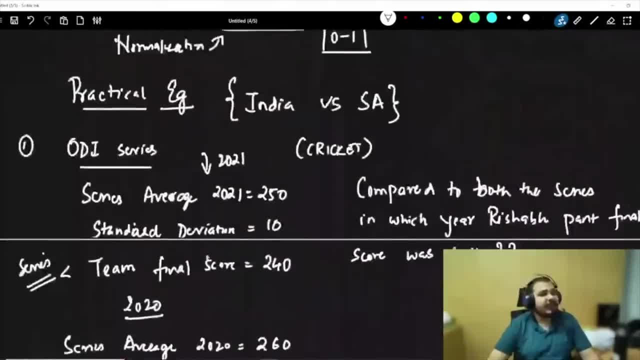 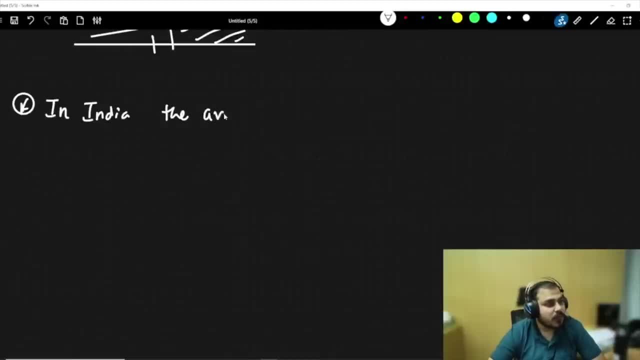 of the area of the body Of this particular part. So this was an example. with respect to z-score standardization, all these things we have probably discussed. So the question is how much the average IQ is 100 with a standard deviation? 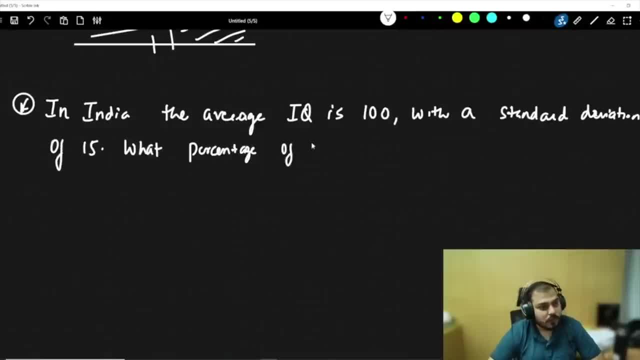 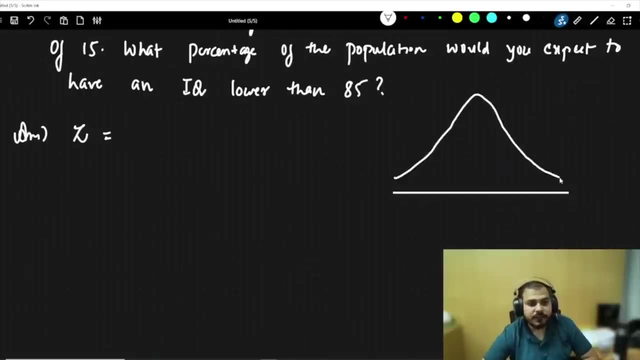 with a standard deviation of 15? What percentage of the population would you expect to have an IQ lower than 85?? So my z-score will be what? So, first of all, let's discuss about this graph. So here you can see that this is my graph. 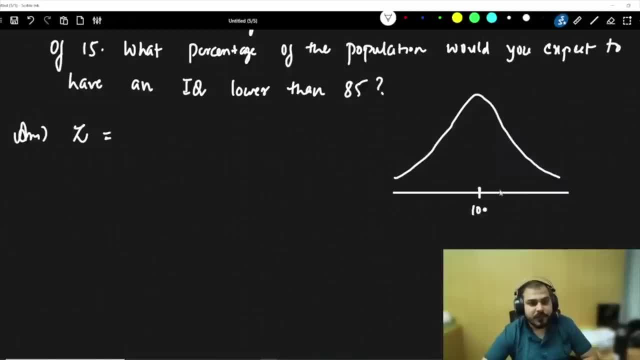 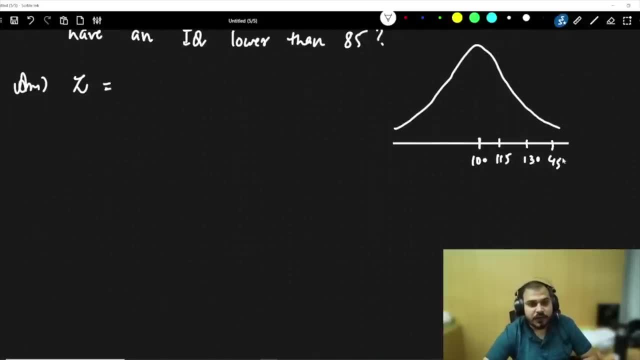 So this particular value is how much. The mean is 100.. My standard deviation is standard deviation is 50. So 115,, 130, 145.. Similarly, I have 85,, 70, 55.. So I have all these values over here. 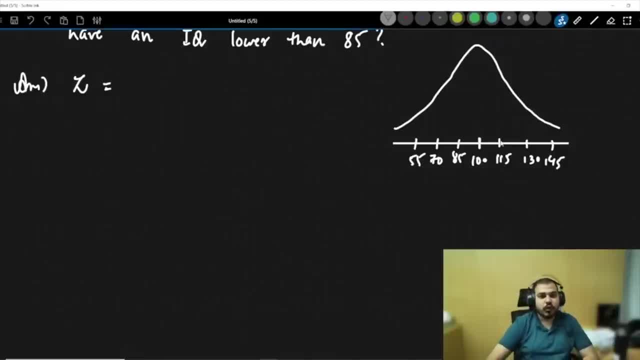 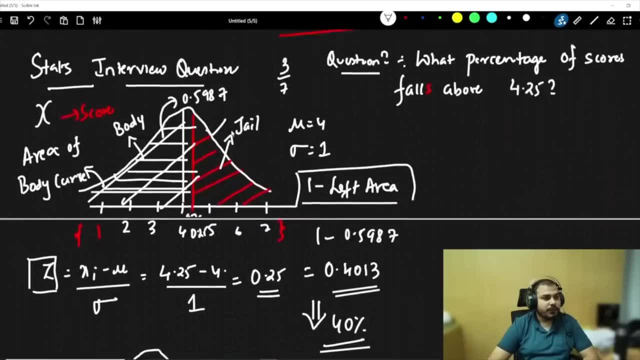 Now, with respect to this, first of all, let's go and compute the z-score. How do you compute the z-score? The same example that what we have done over here. Here, in this particular case, 4.25, falls over. 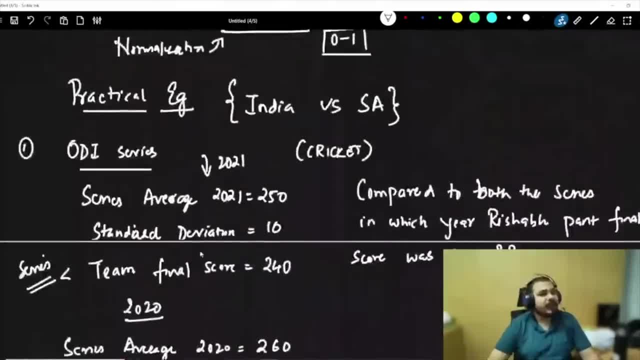 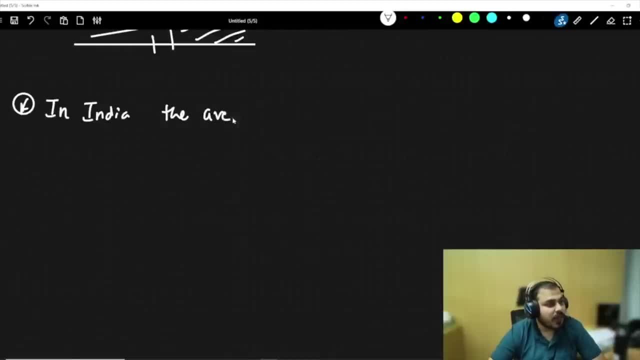 of the body of this particular part. So this was an example. with respect to z-score standardization, all these things we have probably discussed. So the question is: in India, the average IQ is 100, with a standard deviation, with a standard deviation of 15.. What percentage? 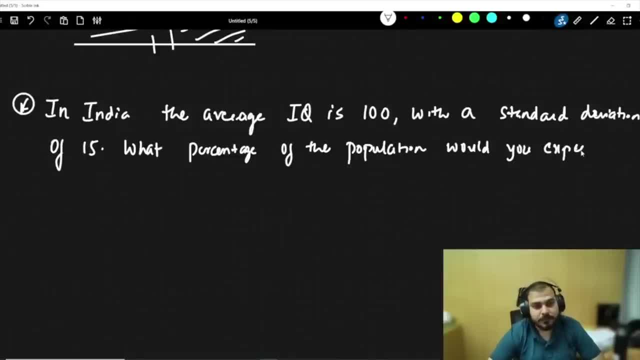 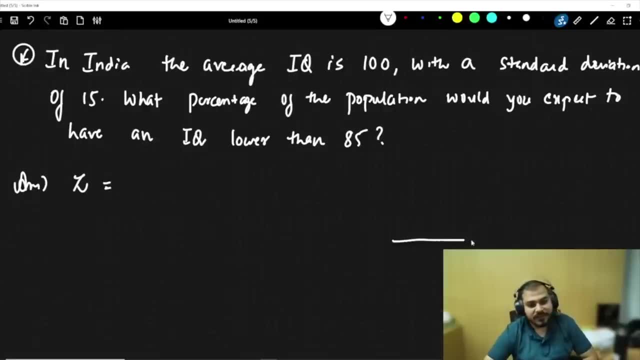 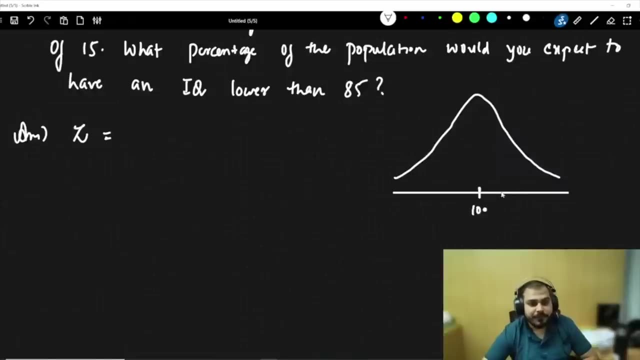 the population would you expect to have an IQ lower than 85. so my Z score will be what? so first of all, let's discuss about this graph. so here you can see that this is my graph. so this particular value is how much? the mean is 100. my. 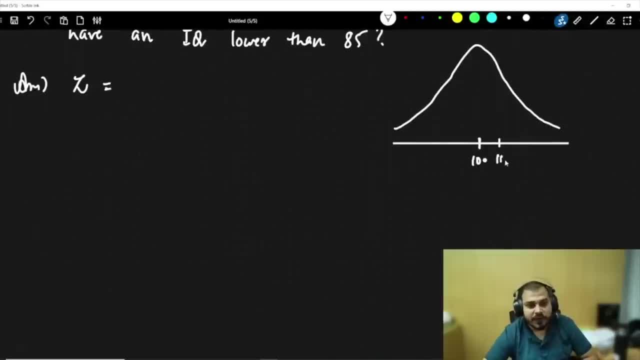 standard deviation is. standard deviation is 50, so 115, 130, 145. similarly, I have 85, 70, 55. so I have all these values over here. now, with respect to this, first of all, let's go and compute the Z score. how do you compute the Z score? the same. 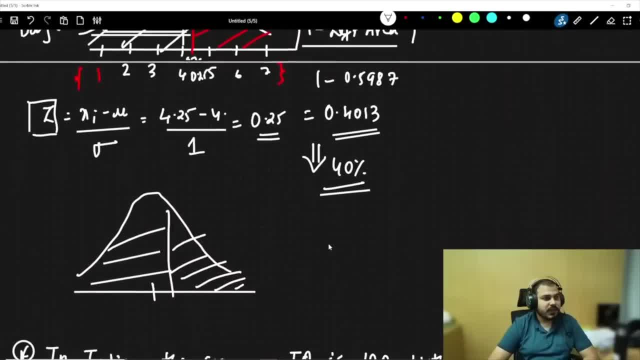 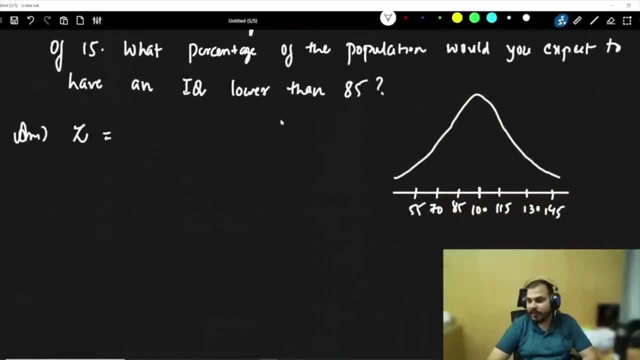 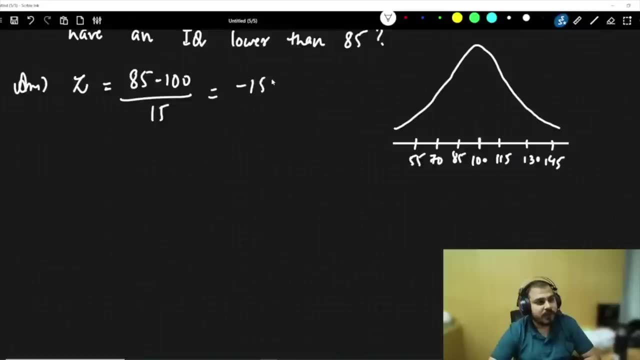 example, that what we have done over here here, in this particular case, 4.25 falls over. we are just taking IQ lower than 85. so what is IQ lower than 85? so it will become 85 minus 100 divided by divided by 15. what it is minus 15 by 15 it is: 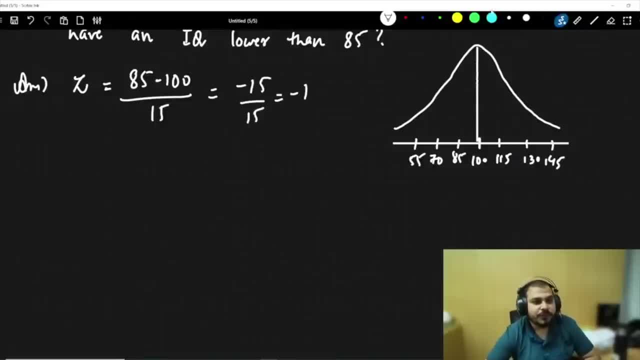 minus 1, so one standard deviation. this is my mean, this is my minus 1 standard deviation. now, this is the area that I want to find out. now, when I want to find out this particular area, this area is already the body part, the left of the curve. so what I will do, I will. 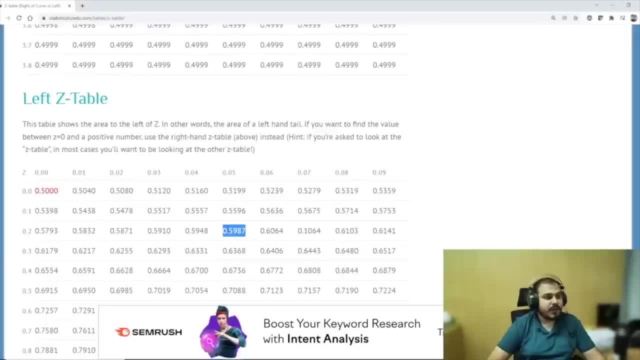 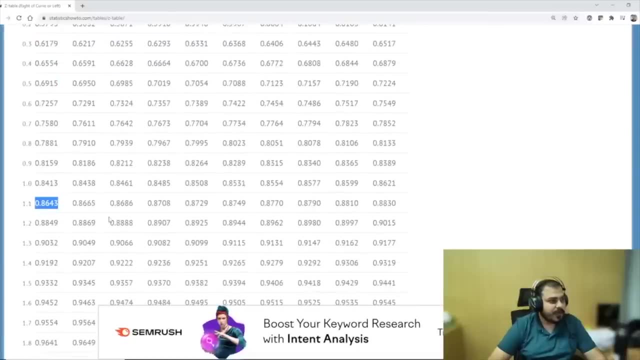 just go and compute for minus 1. now, if I want for minus 1 what it is, go and compute it over here how much it is 1.0. so this is point eight six four. let me just compare the answers or let me just select some different Z table. so 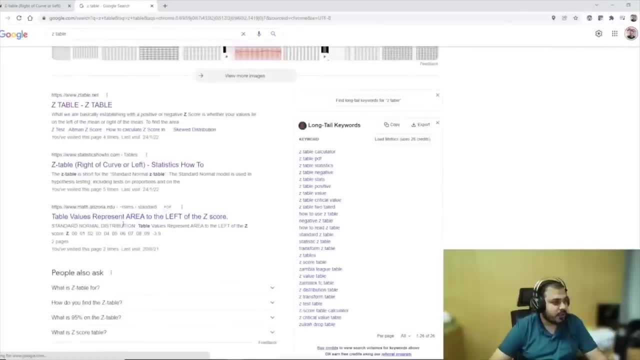 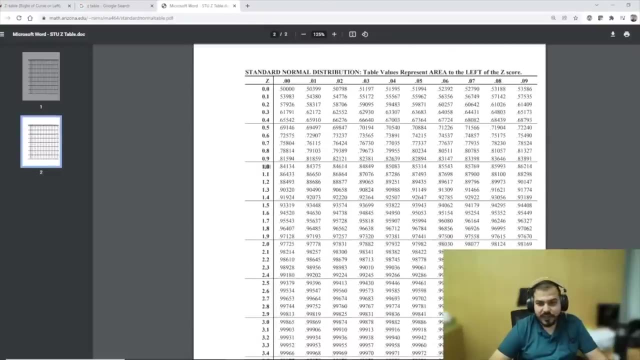 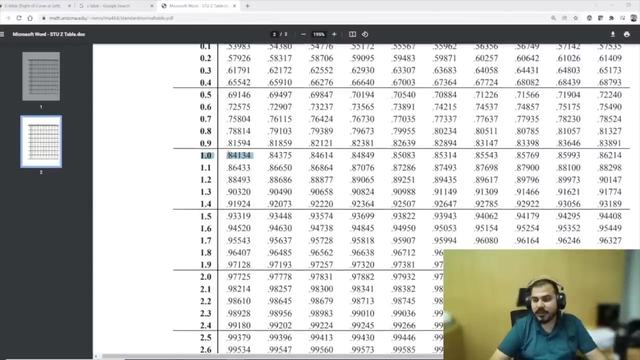 that you will get an idea. I'm actually not able to find the right Z table. yeah, this looks good, so I will give you the link. point eight four. so what I'm actually getting? point eight four, one, three, four. point eight four: one, three, four. this is plus one. understand, this is plus one, plus one when I say understand. 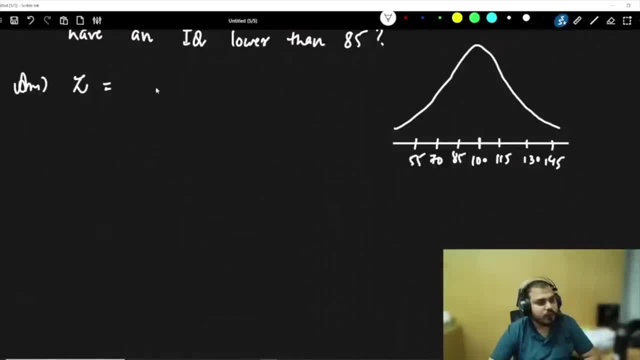 We are just taking IQ lower than 85. So what is IQ lower than 85?? So it will become 85 minus 100 divided by 15.. What it is Minus 15 by 15, it is minus 1.. 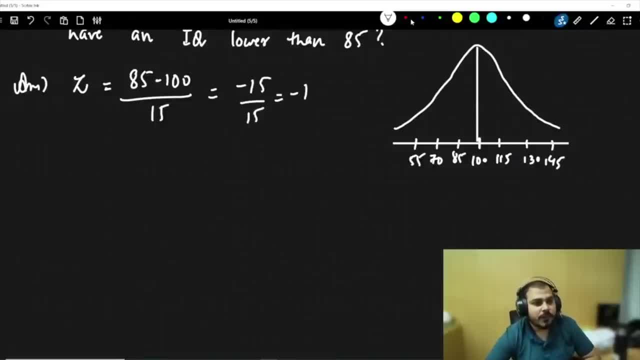 So one standard deviation. This is my mean. This is my minus 1 standard deviation. Now, this is the area that I want to find out. Now, when I want to find out this particular area, this area is already the body part, the left of the curve. 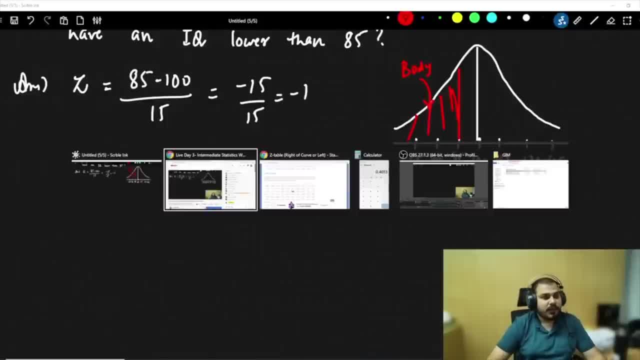 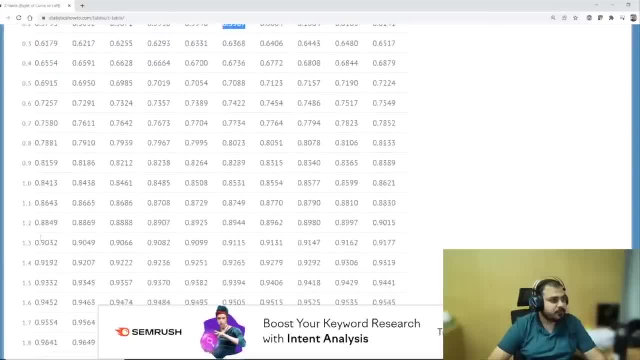 So what I will do? I will just go and compute for minus 1.. Now, if I want for minus 1, what it is, Go and compute it over here How much it is 1.0.. So this is 0.86.. 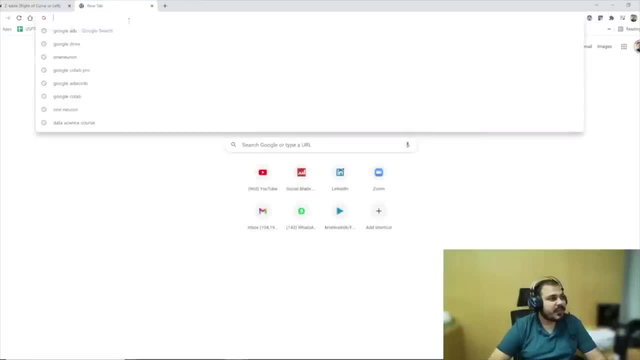 Let me just compare the answers. Let me just select some different z-table so that you will get an idea. I am actually not able to find the right z-table. Yeah, this looks good, So I will give you the link: 0.84.. 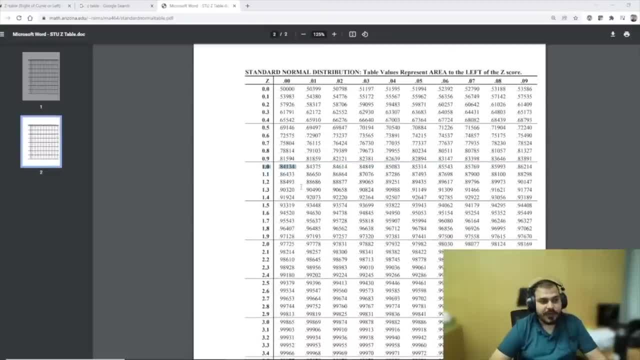 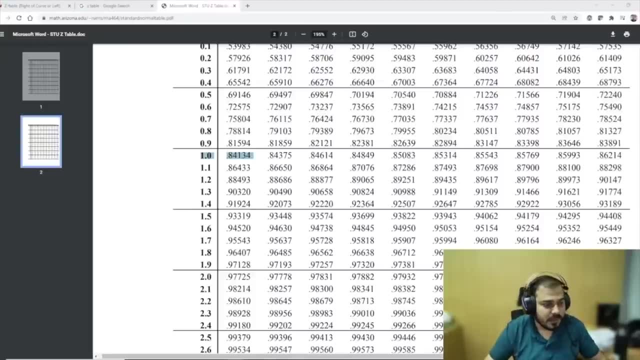 So what I am actually getting? 0.84134.. 0.84134.. 0.84134.. This is plus 1.. Understand, this is plus 1.. Plus 1 when I say: Understand over here. Plus 1 when I say: 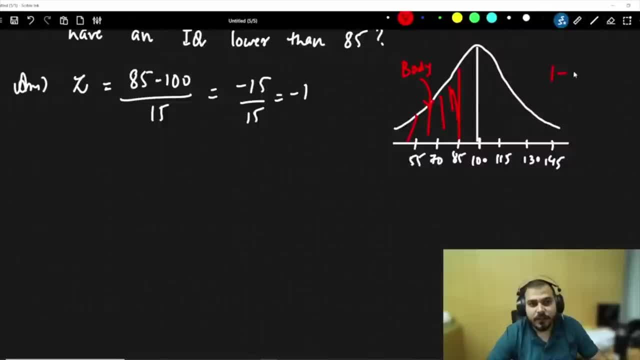 It is basically from this region to this region. Now, if I subtract 1 minus 0.8414.. 0.84134.. That will basically be my values, right. Lower than 85. Understand, lower than 85. Lower. 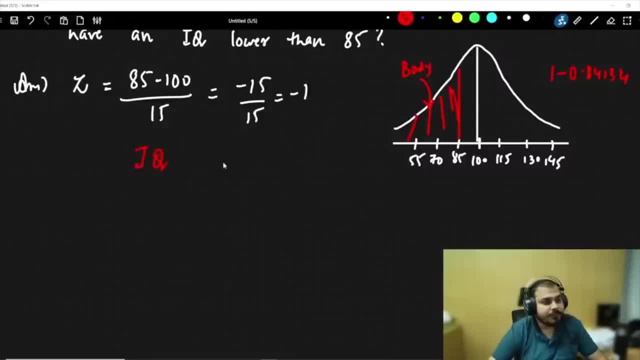 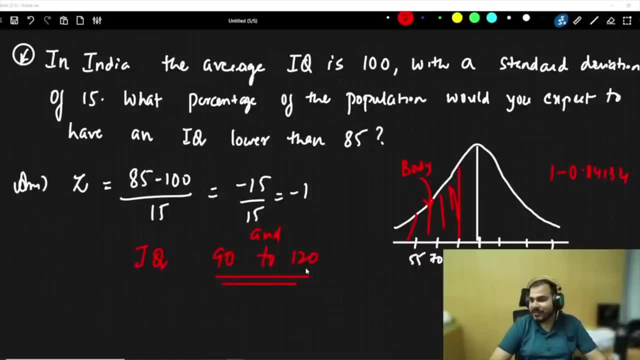 You may also get a question: IQ between 90 to 120. Like this question also, you may get for the same problem statement. So you may get questions like this. At that point of time again, you have to solve it in a different way. 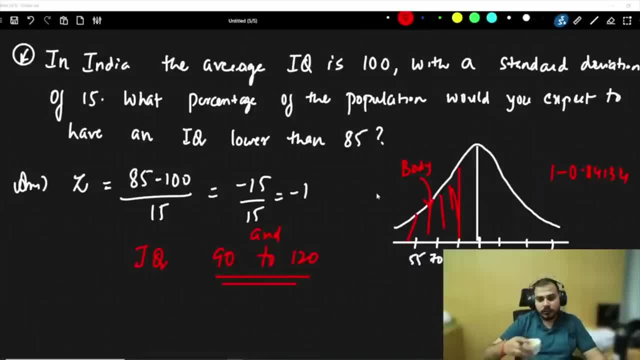 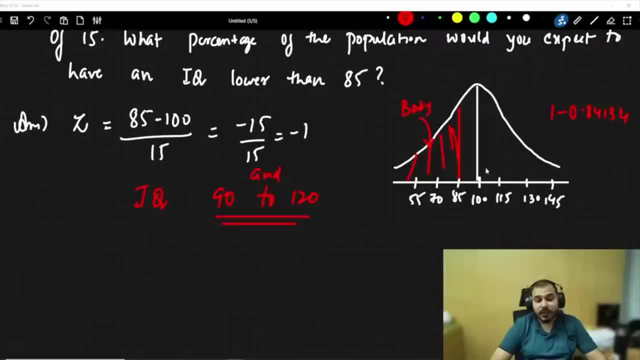 But here is just an idea to talk about. what is body? area of the body. Yeah, negative will not matter. If you say negative, it will come from here. If you say sorry, if you can say negative, it will come from here. If you say positive, it will come from here. 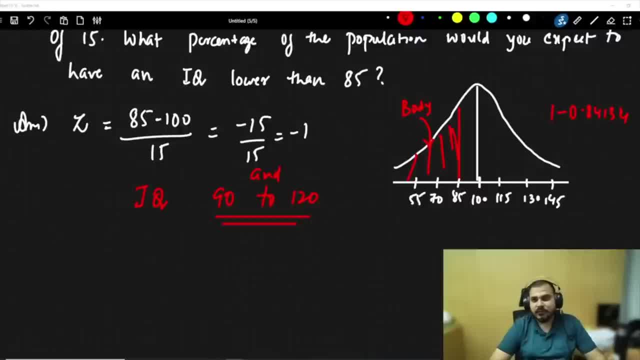 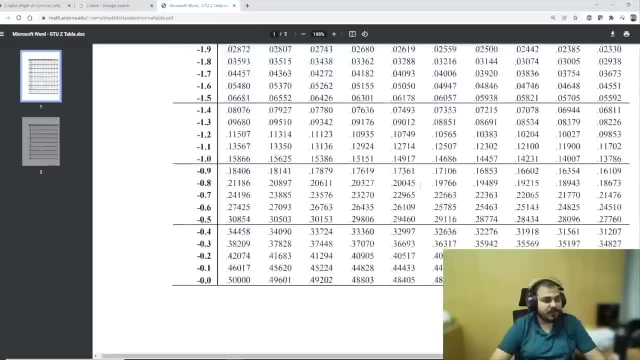 Understand, both the side are symmetric, Minus 1 also. you can look That only I am saying In table. whatever you are able to find out, You can definitely check out for minus 1 also from top, Minus 1.0.. 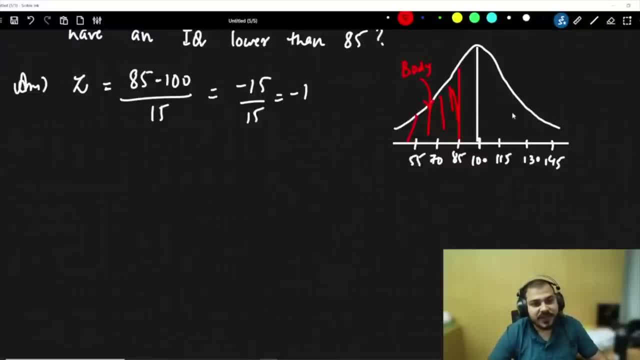 over here, plus one when I say it is basically from this region to this region. now, if I subtract 1 minus point eight, four, one, four, point eight, four, one, three, four, that will basically be my values. right, lower than 85, understand, lower than 85, lower. you may also get a question: IQ between. 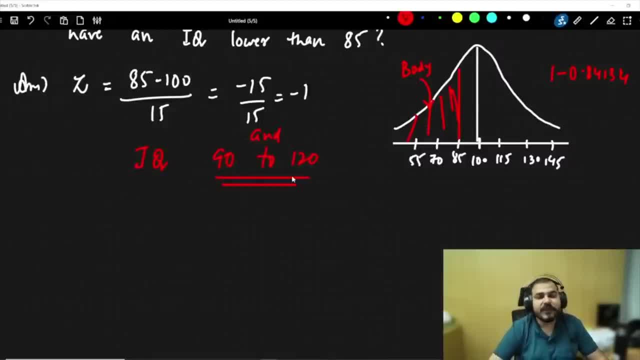 ninety to one, twenty kiw between ninety to one-twenty. like this Question you may get for the same problem statement. so you may get questions like this at that point of time again. you have to solve in a different way. 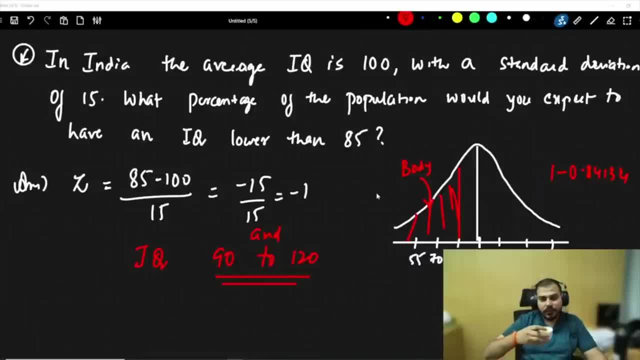 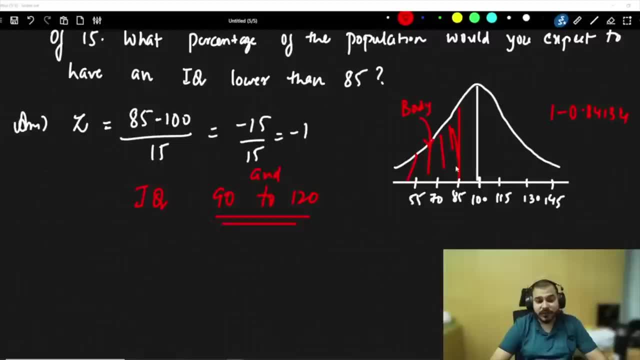 but here is just an idea to talk about. what is body? area of the body. yeah, negative will not matter. if you say negative, it will come from here. if you say sorry, if you can say negative, it will come from here. if you say positive, it will come from here. understand, both the side are symmetric minus. 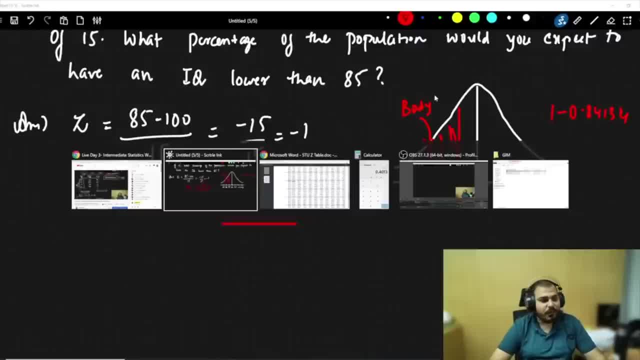 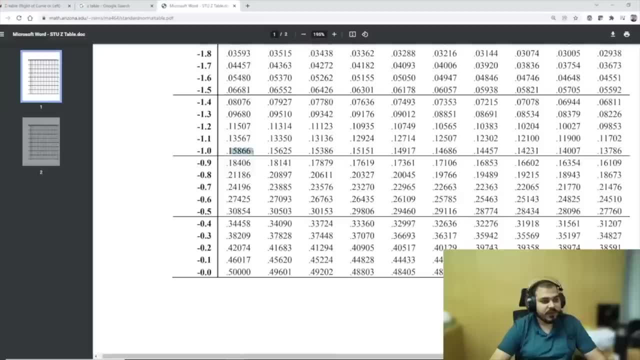 one also. you can look that only i'm saying no in table. whatever you are able to find out, you can definitely check out for minus one also from top. minus 1.0- same thing you'll be getting right. minus 1.0 is 1.15886, which is 1 minus 0.84- right same thing. now let me do one thing guys quickly show. 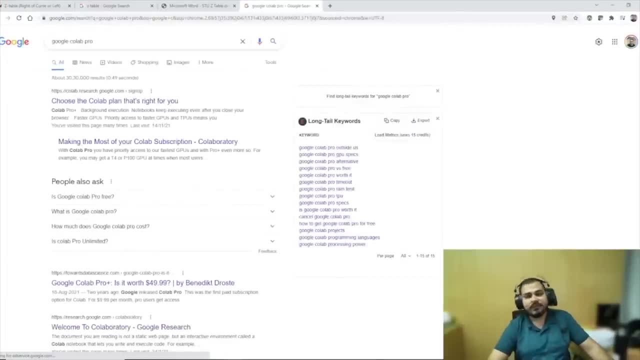 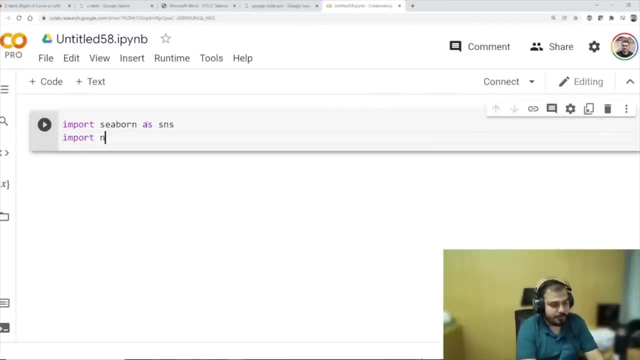 you google collab pro so that we can have some programming sessions. so first of all i'm going to import some libraries as this, import numpy as np, import, import matplotlib, dot, pyplot as plt and then, and then, and then probably i will say matplotlib inline. so all these things we are actually done and then probably i'll. 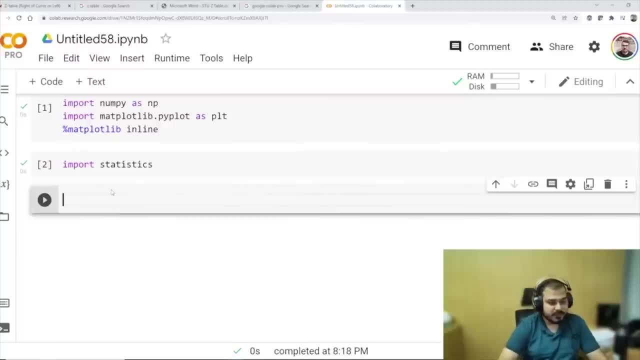 also import statistics. now, first thing first, how to compute mean mean median mode. okay, we are going to see that. first of all, let me load a data set which is called as. i'll load a data set which is called as tips, and this will basically be giving me df is equal to this one, then i'll say df, dot. 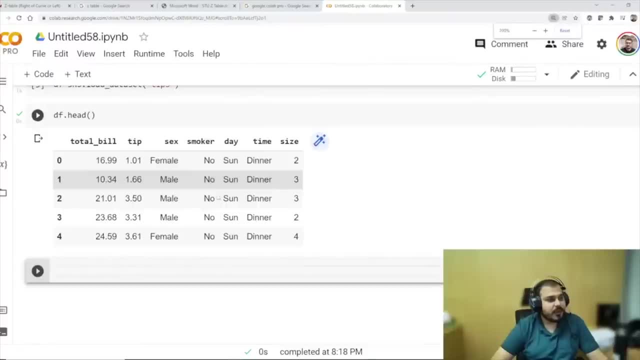 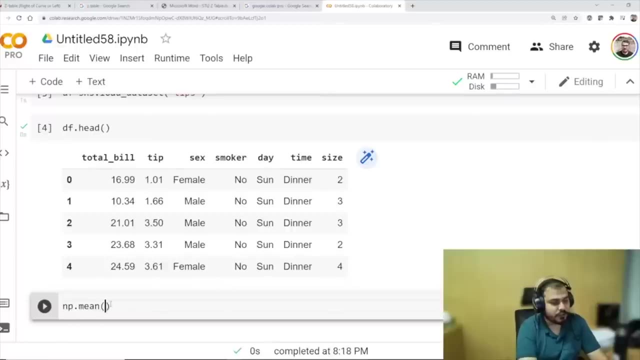 head. so here you can see. this is my entire data set. now, quickly, if you want to see how to do mean for this, let's say that i'm using np dot mean function for finding the total bill mean, total bill of mean. okay, so if i execute this, you will be able to see. 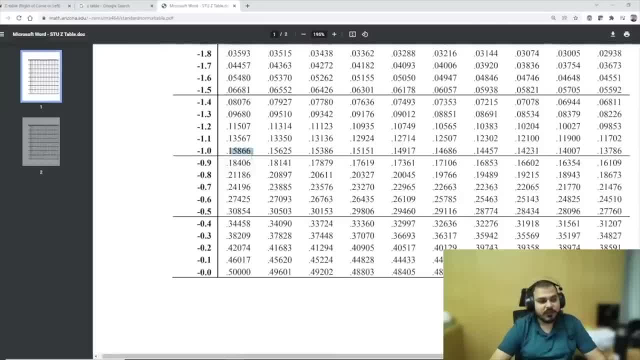 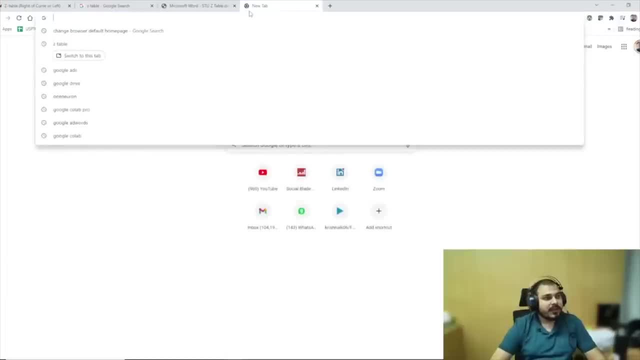 Same thing you will be getting right. Minus 1.0 is 0.15886.. Which is 1 minus 0.84, right, Same thing. Now let me do one thing, guys. Quickly show you Google Collab Pro. 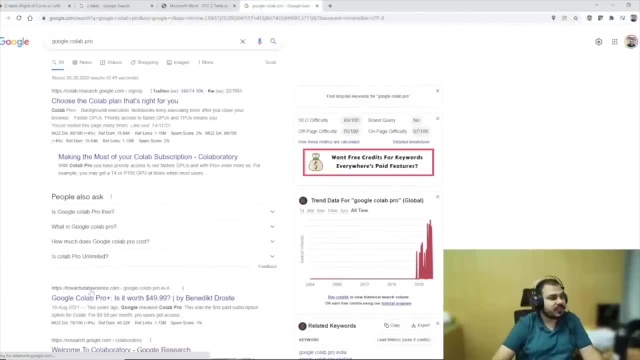 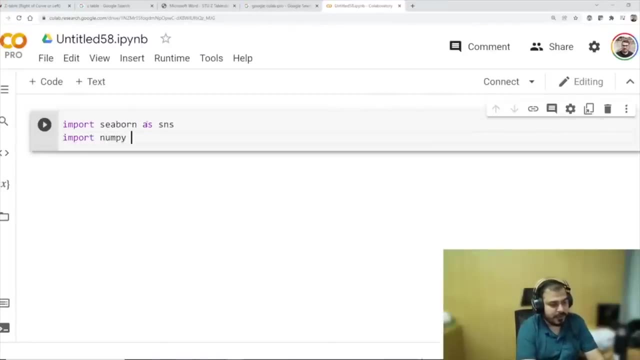 So that we can have some programming sessions. So first of all I am going to import some libraries as this: Import, Import numpy as np, Import, Import matplotlibpyplot as plt And then probably I will say matplotlib inline. So all these things we are actually done. 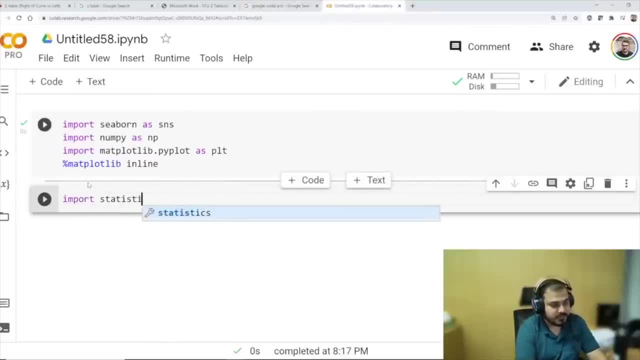 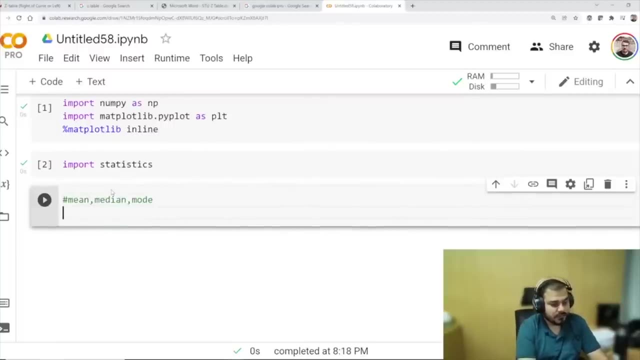 And then probably I will also import statistics. Now, first thing first, How to compute mean Mean median mode. Okay, We are going to see that. First of all, let me load a dataset Which is called as. I will load a dataset which is called as tips. 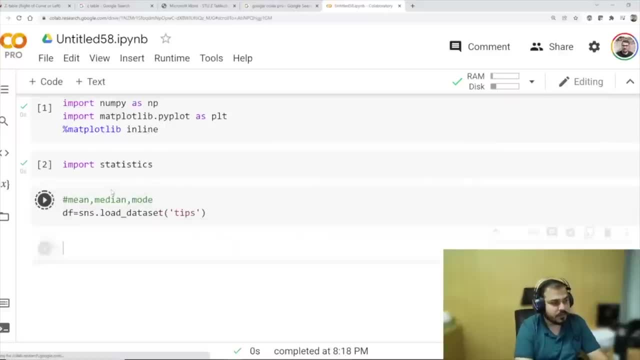 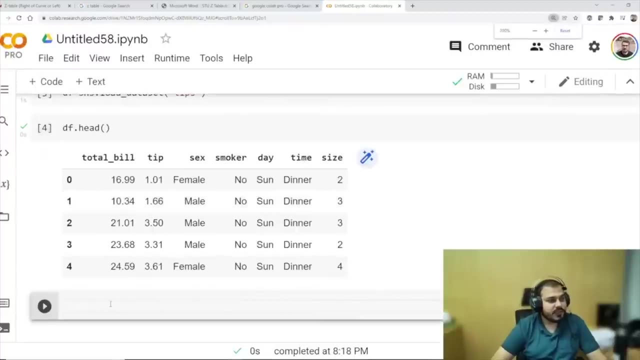 And this will basically be giving me df is equal to this one, Then I will say dfhead. So here you can see. this is my entire dataset. Now, quickly, if you want to see how to do mean for this, Let's say that I am using npmean function for finding the total bill mean. 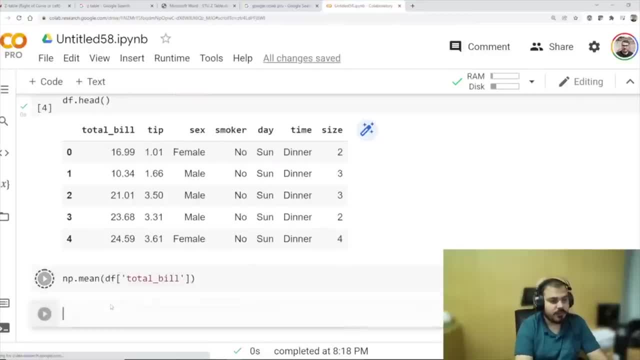 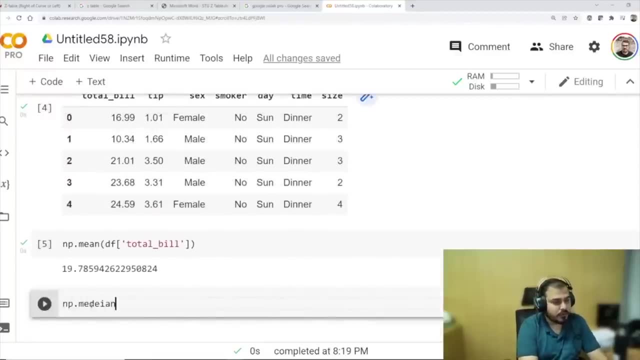 Total bill of mean. Okay, So if I execute this, you will be able to see the answer. So this is the What is the mean of the total bill? If I want to probably find out the median, also, You will be able to find out median. 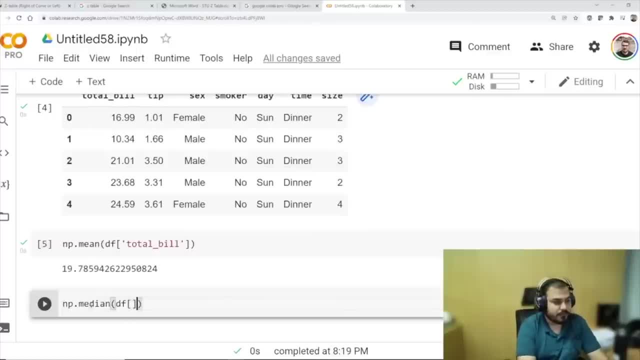 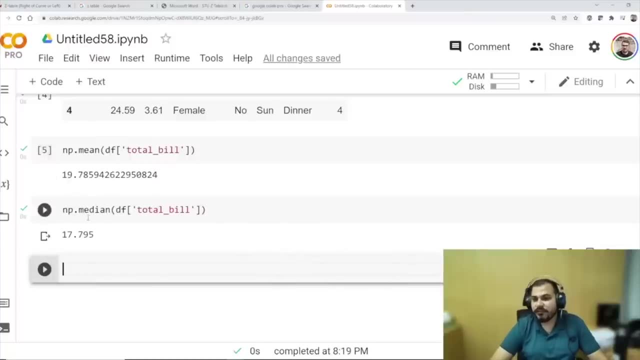 npmedian df of total bill. So here you will be able to see npmedian. So over here you see some differences. If you are seeing some differences, Think that there may be something like Some kind of outliers Also Okay. 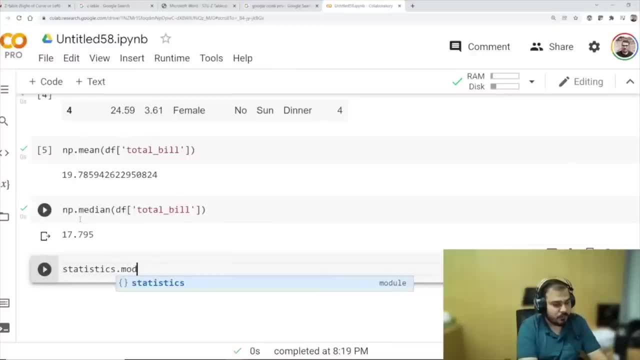 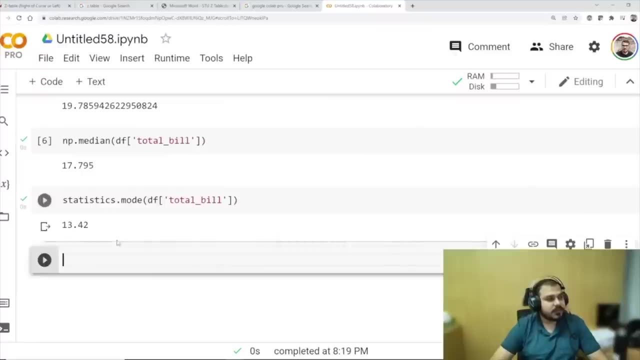 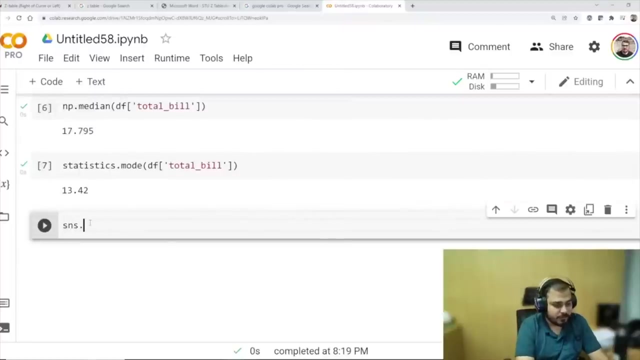 If you want to try for mode, I can use statisticsmode And again I will be using df of total underscore bill. So here you go. This is got. Mode is nothing but 13.42.. Now the thing is that If I want to go and see my box plot, 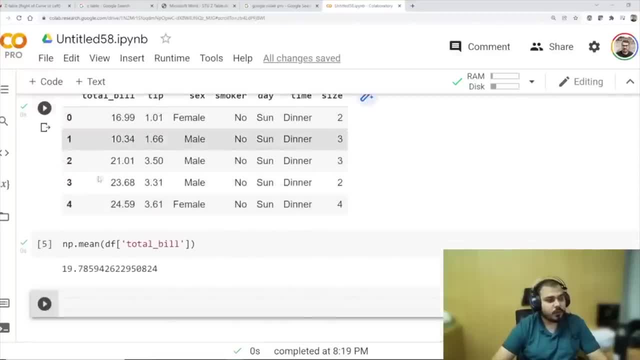 the answer. so this is the. what is the mean of the total bill if i want to probably find out the median? also, you will be able to find out median, np, dot, median, df of total bill. so here you'll be able to see np, dot, median, the median. okay, so now let's see how to do mean for this. let's say that i'm using 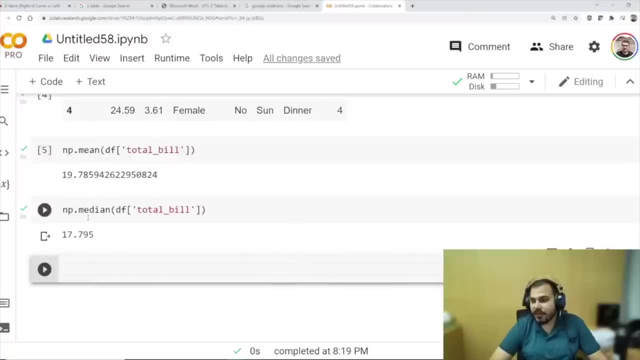 median. so over here you see some differences. if you are seeing some differences, think that there may be something like some kind of uh outliers also okay, uh, if you want to try for mode, i can use statistics dot mode and again i will be using df of total underscore bill. so here you go, this. 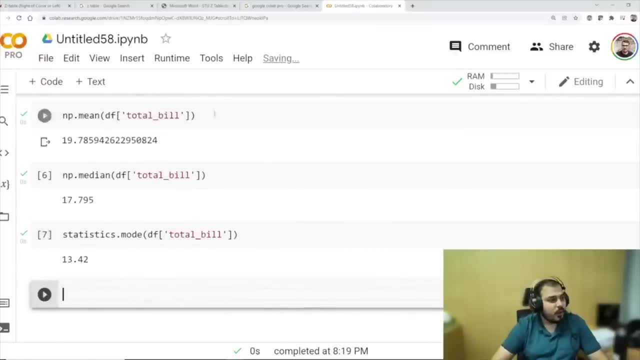 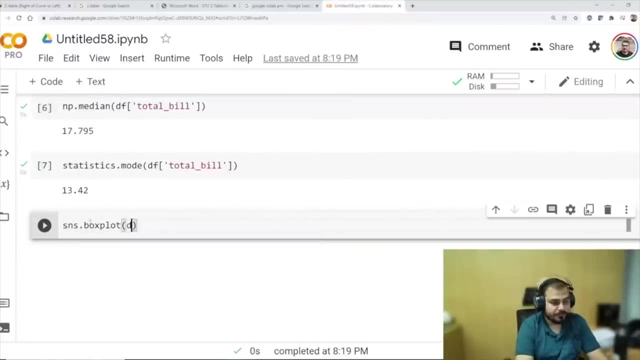 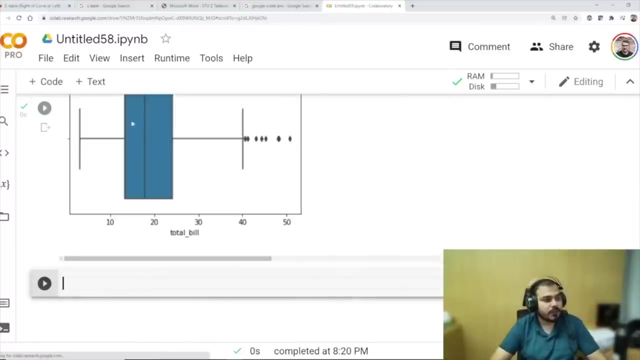 is got mode is nothing but 13.42. now the thing is that if i want to go and see my box plot, which is basically used to see outliers, so if i use df of total bill, total underscore bill, so here you will be able to see my box plot also. so this is one example of box plot. so does this? 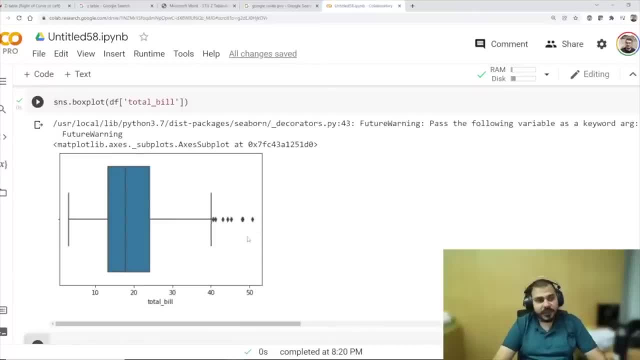 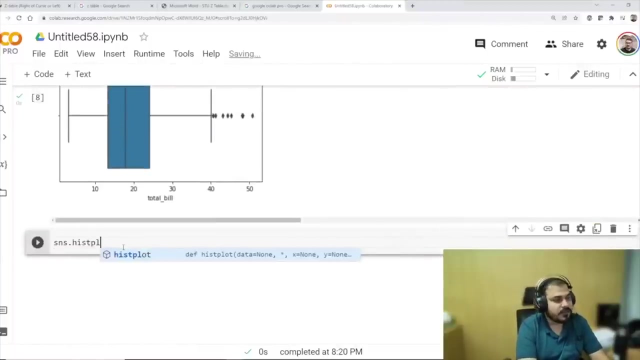 indicate it has an outlier. now, definitely over here outliers is present. but what is this? this is 25, sorry, minimum, 25 percentile, median, 75 percentile and max. so all these things we have calculated. if you write df of sns dot, there is something called as hist plot, which will basically help you to create histograms. 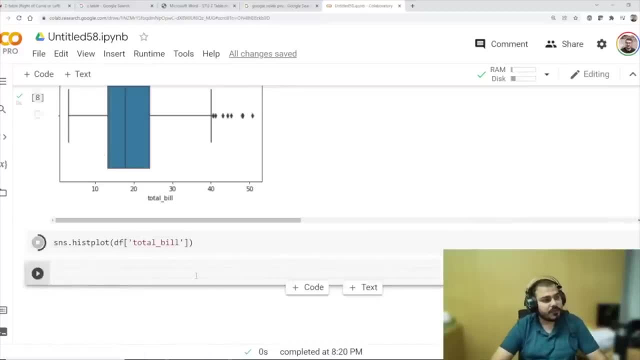 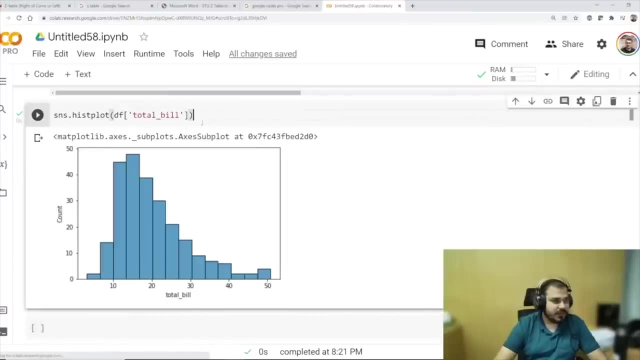 on a specific feature. so if i execute this, you will be able to see one example which looks like this: is this a normal distributed data? i guess no. if you want to see, with uh probability density function, i'll be using. kde is equal to true, so with kd is equal to true. does this look like a? 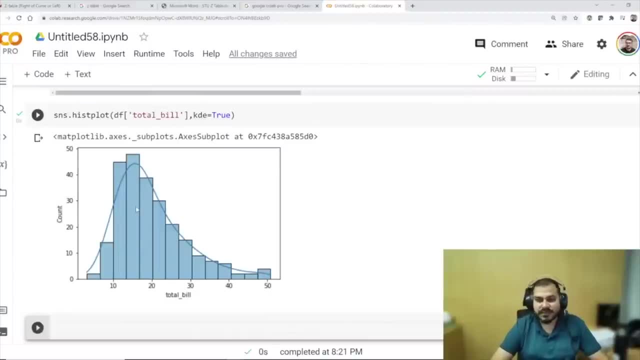 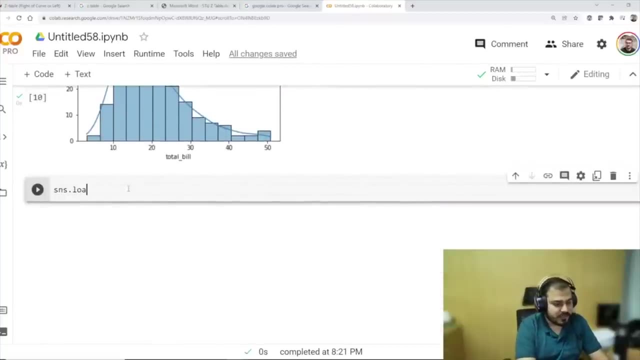 normally distributed. no, it is like a little bit skewed towards the right. i'll also show you some samples with respect to, uh, normally distributed data. so for that i will do snsload underscore dataset. i will be using iris data set, iris flower data set. basically is the data set which will 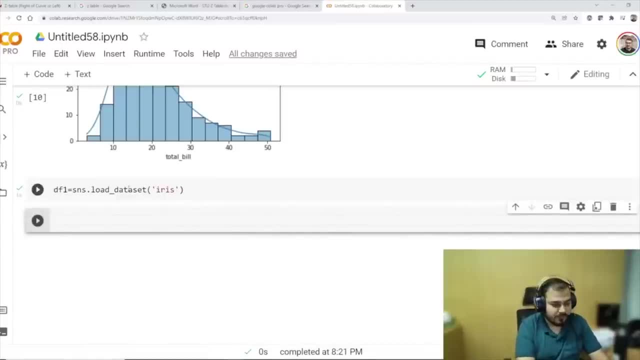 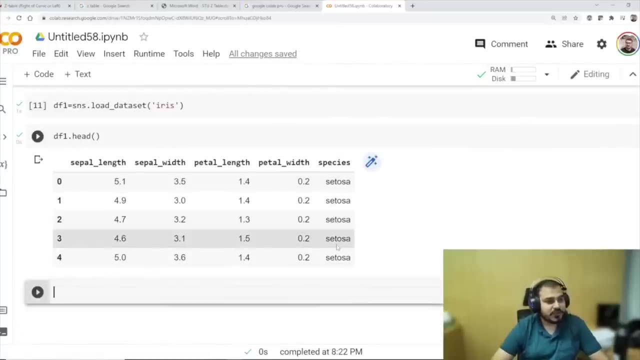 actually help you to give a data of a different types of flowers with respect to iris. so here you will be able to see that df1 dot head. so here you have flowers like setosa versicolor and here you have four features: sepal length, sepal width, petal length and petal width. 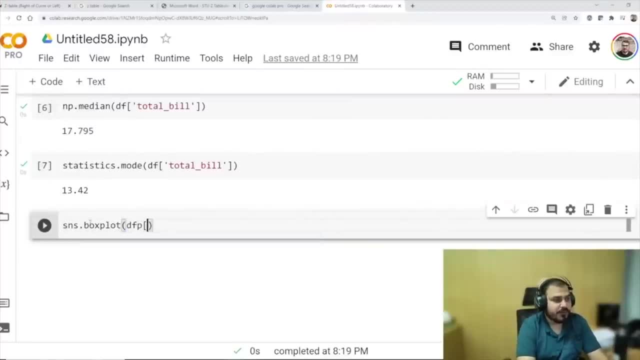 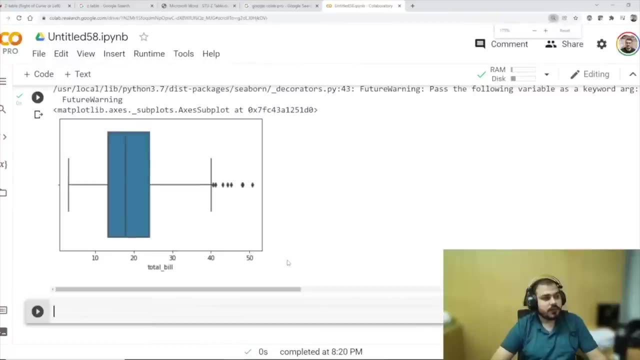 Which is basically used to see outliers. So if I use df of total bill, Total underscore bill, So here you will be able to see my box plot also. So this is one example of box plot. So does this indicate it has an outlier? 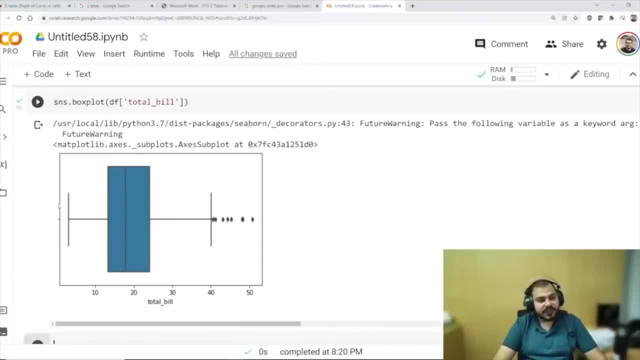 Now, Definitely over here, Outliers is present, But what is this? This is 25 percent, Sorry. Minimum 25 percentile, Median, 75 percentile And max. So all these things we have calculated. If you write df of: 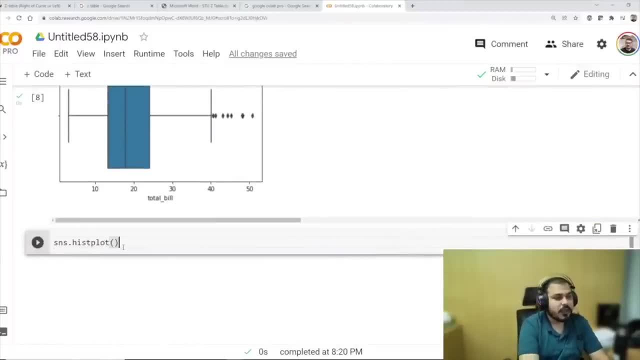 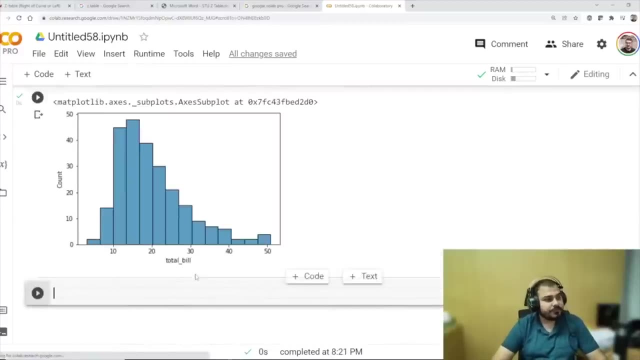 sns There is something called as hist plot, Which will basically help you to create histograms On a specific feature. So if I execute this, You will be able to see One example which looks like this: Is this a normal distributed data? 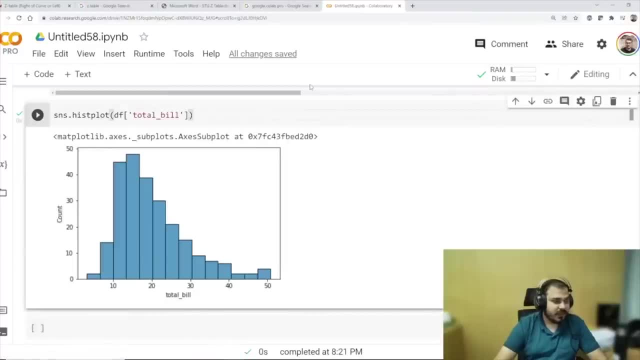 I guess no. If you want to see With probability density function, I will be using. kde is equal to true. So with kde is equal to true, Does this look like a normally distributed No? It is like little bit skewed towards the right. 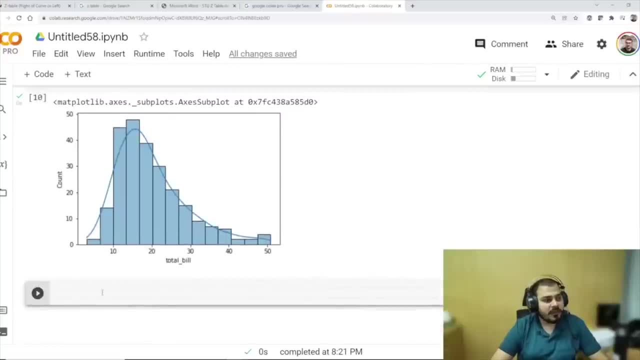 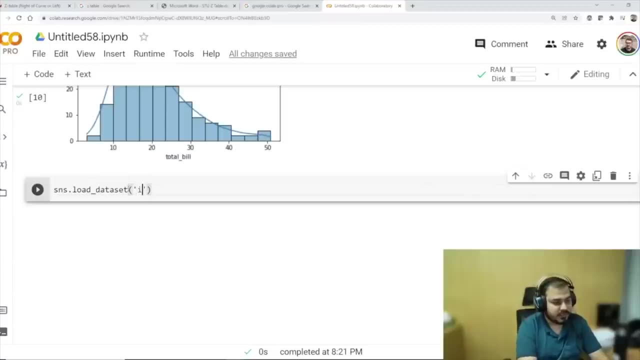 I will also show you some examples with respect to Normally distributed data. So for that I will do sns dot load underscore data set. I will be using iris data set, Iris flower data set basically is the data set Which will actually help you to. 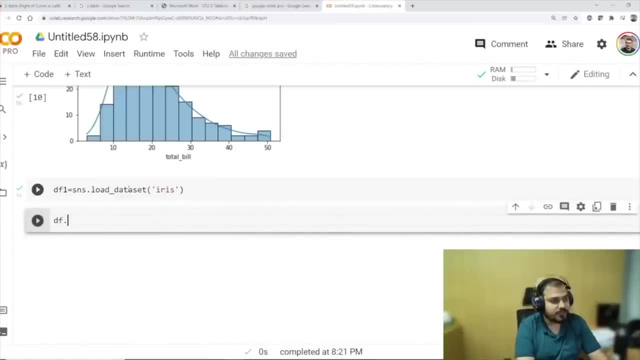 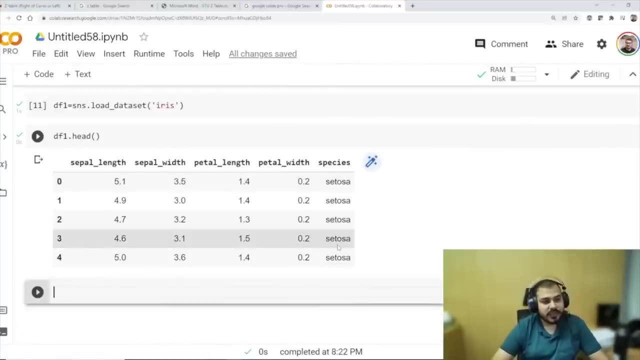 Give a data Of a different types of flowers With respect to iris. So here you will be able to see that df1 dot head. So here you have flowers like Setosa Versicolor, And here you have four features. 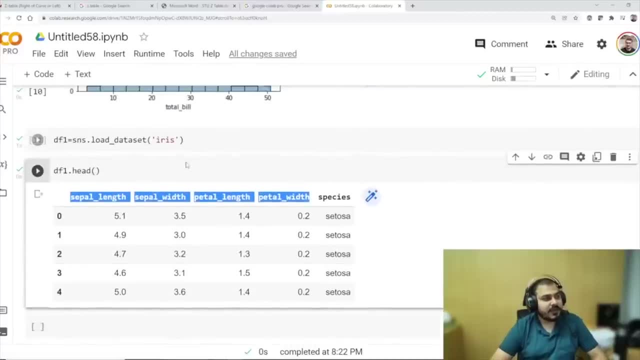 Sepal length, Sepal width, Petal length And petal width. Now let's see, I will just try to plot this same thing With one of the feature. Okay, Let's say that I am doing it with Sepal length. 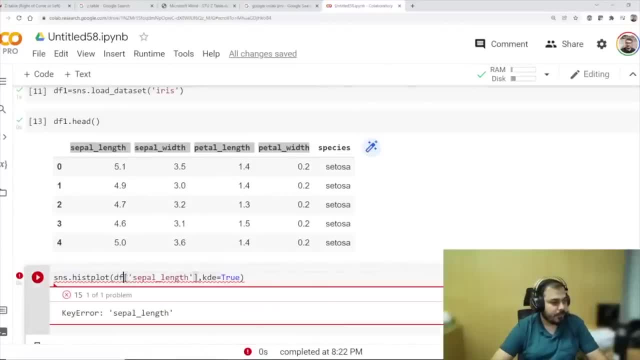 Sepal underscore length: df1.. So here you can see That I am doing it with Sepal length. Sepal underscore length. So here you can see that. Does this follow A Gaussian distribution? Does this follow a Gaussian distribution? 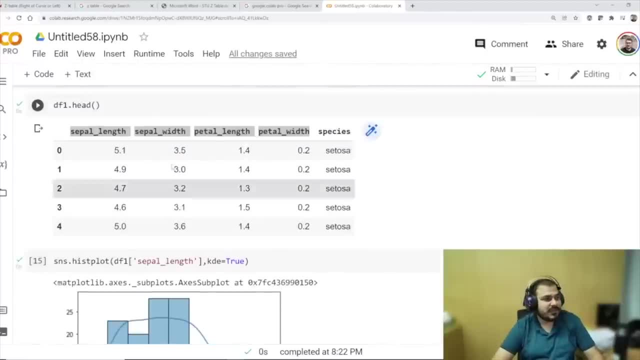 No, I guess Let's try with Sepal width. Finally we will be able to see something. Wow, This follows a Gaussian distribution. Definitely, we can definitely say for this: This is a Gaussian distribution. So this is specifically a Gaussian distribution. 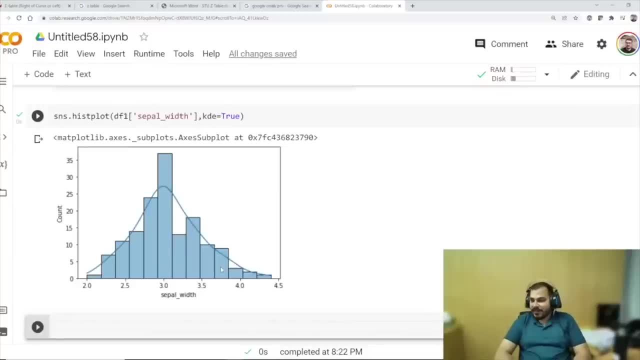 Over here And here you can also apply that Rule, That is, 68., 95., 99., 7. Percentage rule. So all these things you can see Here And here you can also apply that Rule. That is 68., 95., 99., 7., 7., 8., 9., 10., 11., 12., 13., 14., 15., 16., 17. 18.. 19., 20., 21., 22., 23., 24., 25., 26., 27., 28., 29., 30., 31., 32., 33., 34., 35.. 36., 37., 38., 39., 40., 41., 42., 43., 44., 44., 45., 46., 46., 47., 48., 49., 50.. 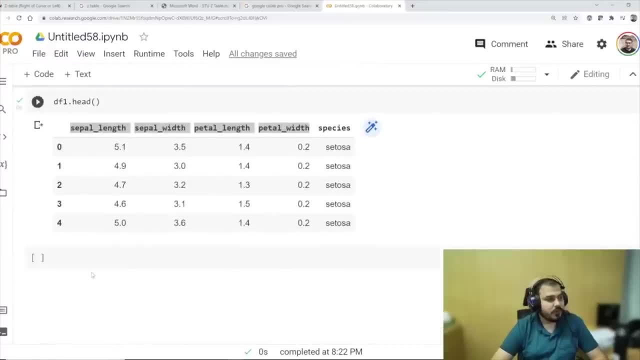 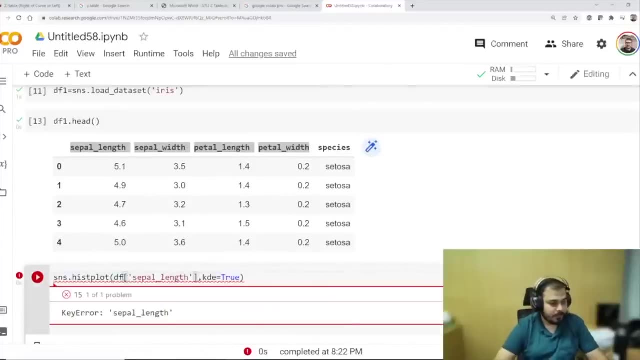 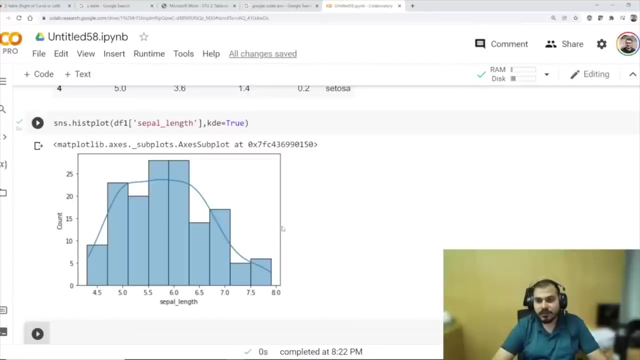 will just try to plot the same thing with one of the feature. okay, let's say that i am doing it with sepal length. sepal underscore length: df1. so here you can see that. does this follow a gaussian distribution? does this follow a gaussian distribution? no, i guess let's try with sepal width. finally we'll be able to see something. 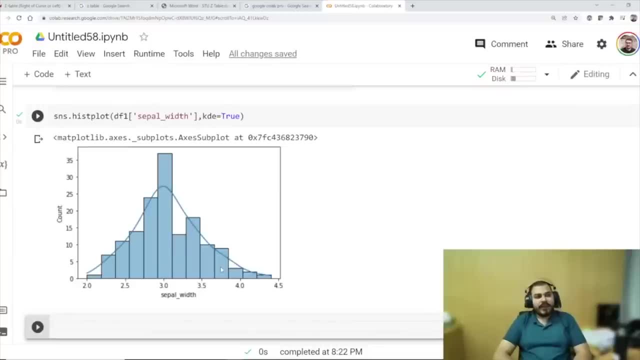 wow, this follows a gaussian distribution. definitely. we can definitely say for this: this is a gaussian distribution, so this is specifically a gaussian distribution over here and here you can also apply that rule, that is, 68, 95, 99.7 percentage rule. so all these things you. 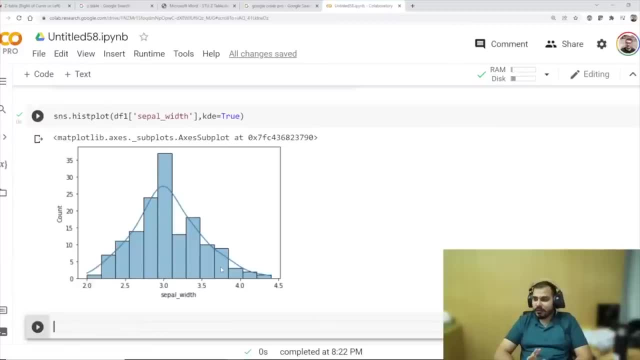 can basically check out over here and you are getting this. i'll also show you how to construct this pdf function and all as we go ahead. okay, it is normally distributed. definitely, we can say that it is normally distributed okay. so this was one example with respect to normally. 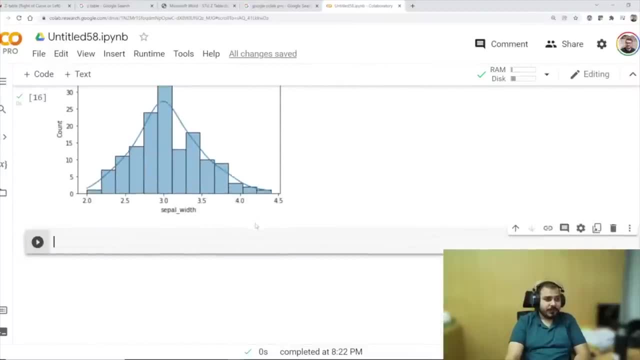 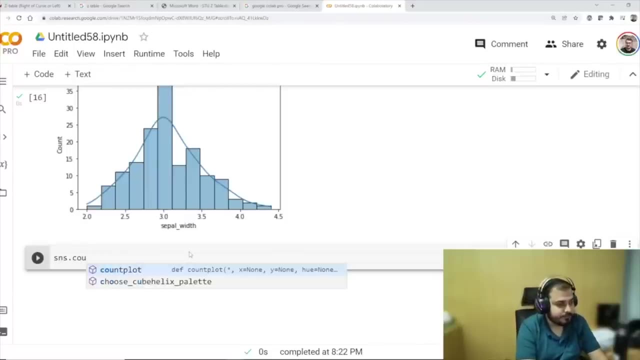 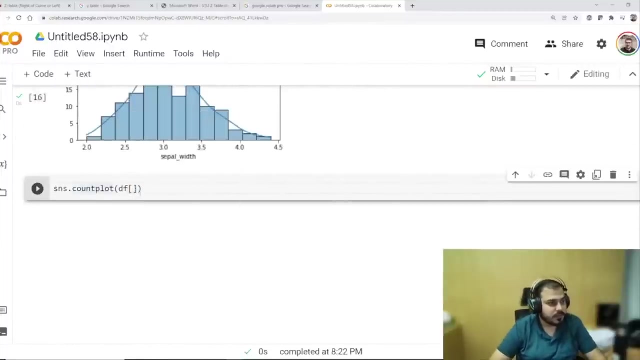 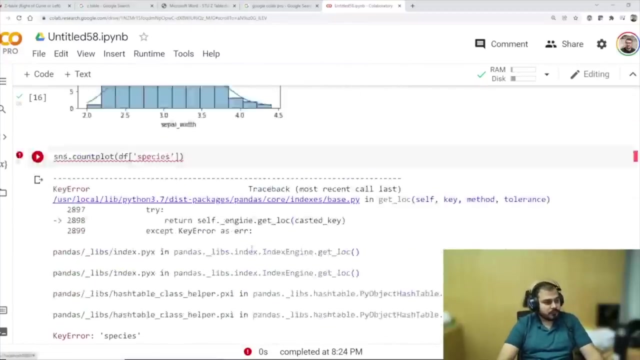 distributed distribution. so let's see how to construct this pdf function, and all as we go ahead. okay, so this is normally distributed. this is not normally distributed. you know sns dot count plot of df of. if i use count plot with respect to species, species spelling is wrong. 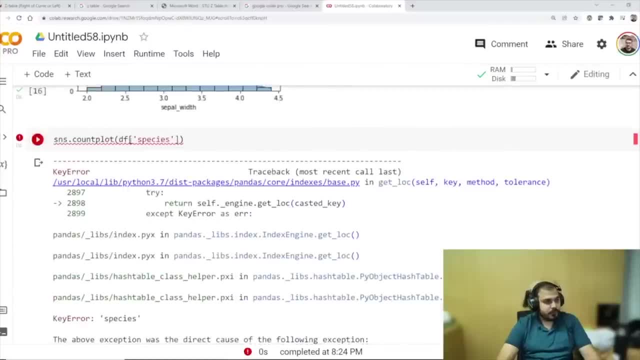 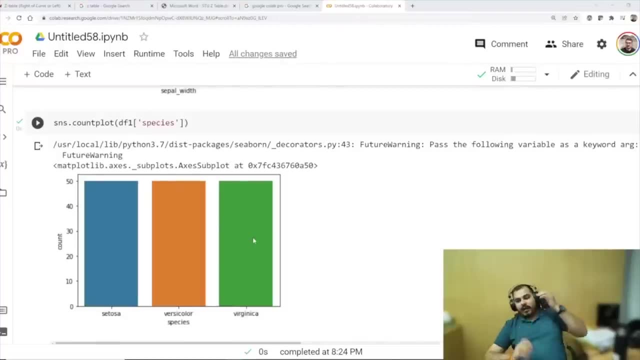 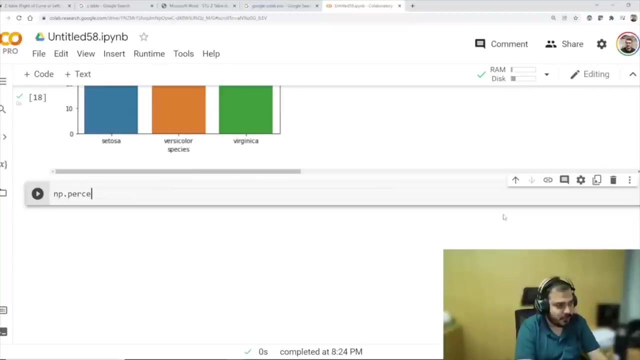 okay, df1. again, i'm writing df. what is this plot? guys, this is a bar graph, bar plot or bar graph, whatever you want. okay, percentiles, let's do for percentile. so for percentile, i can use np, dot, percentile and i can use my df of. let me open one example that i had written for you. so, uh, i will basically use. 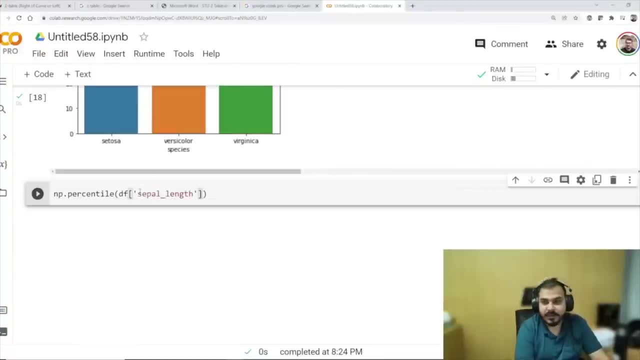 over here like this: let's say i'm going to use say, i'm going to use say, i'm going to use this sepal length, and here i can basically give some parameters, like let's say that i want to get the 25 percentile and 75 percentile. so if i execute it here, sepal length is a df1, so here. 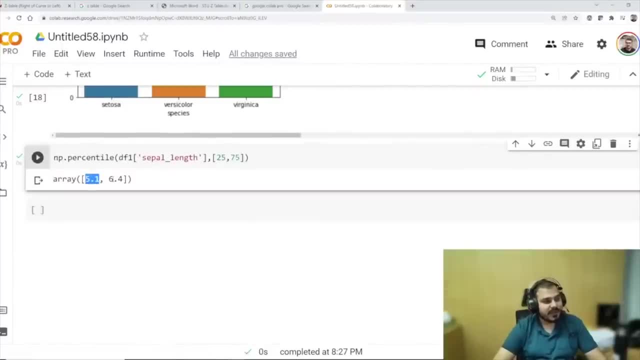 you can see that i'm getting 5.1, as the 25 percentile and 64- 75 percentile is 6.4, so my iqr will be 6.4 minus 5.1. if you want to probably get the 99 percentile also, you can basically write. 51., 52., 53., 54., 55., 56., 57., 58., 59., 60., 61., 62., 63., 62., 63., 64., 65.. 66., 67., 68., 69., 70., 71., 71., 72., 72., 73., 73., 74., 74., 75., 76., 77., 78.. 78., 79., 79., 80., 80., 80., 80., 90., 50., 80., 80., 90., 90., 80., 80., 80., 80.. 90.. 1, 20. 01.. 1., 1., 2., 1, 01.. 1. 0. 1. 1., 1., 7., 1. 8. 8.. 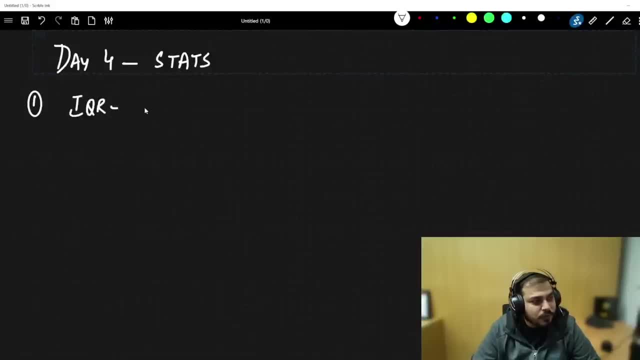 3. 1., 2. 1.. okay, the second topic we are going to discuss about is probability. the third thing that we are going to discuss about is something called as permutation and combination. once we finish this up, the fourth thing that we are going to 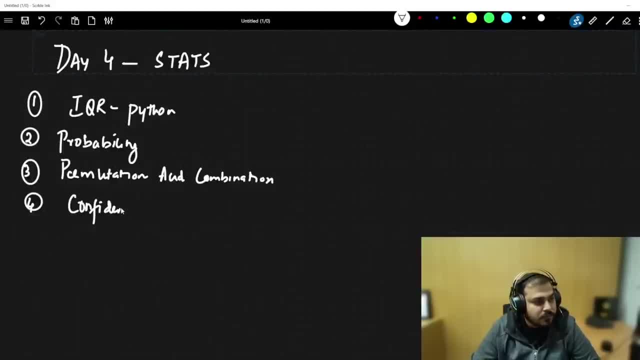 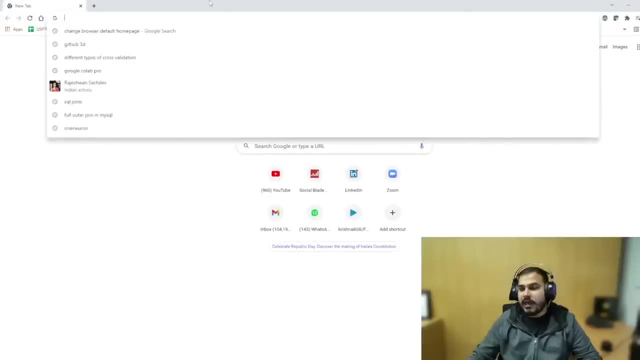 discuss about is something called as confidence intervals. so in confidence intervals then probably, if we get time, we will cover up p-value and then we will start with hypothesis testing. now what we are going to do. first of all, I am going to start with Google collab. you can also open Google collab, okay, so I 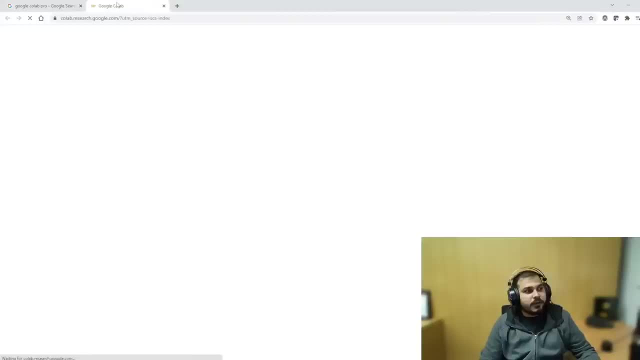 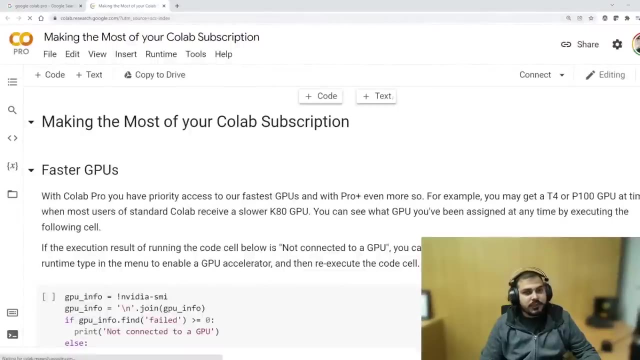 will just make a new notebook. so first of all, we will try to implement z-score and try to find out IQR and with respect to that, we will try to see what all things we can basically implement. other distributions will also come. you can see that we are going to start with z-score and try to find out IQR and we will try to see what all things we can basically implement. other distributions will also come. you. 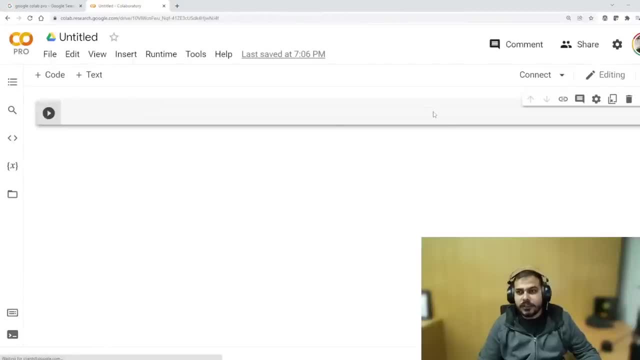 don't worry, Bernoulli. binomial distribution, power law distribution- everything will be discussed. first, let's go in some specific order I have actually decided, and when that is, those distribution will basically come, we'll discuss about it. okay, here you go. so in this session, we 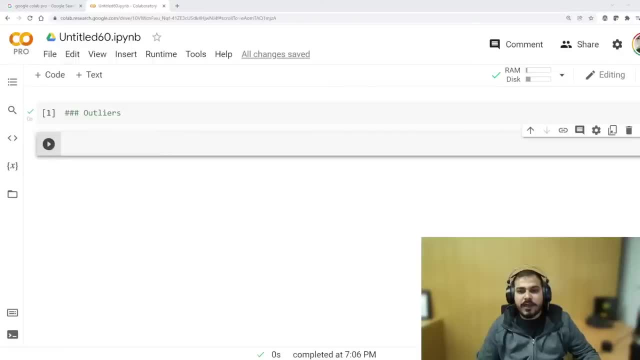 are going to first of all discuss about outliers. now, first of all, what I am actually going to do over here is that I am going to import some libraries, import numpy as np. okay, import matplotlib, dot, pyplot, PLT. then I'm just going to import matplotlib inline. 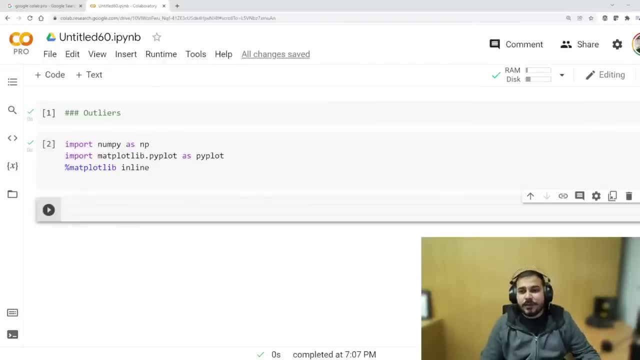 so I'll be executing this now. the next thing that probably we will be discussing about is that let's define our data set. so here I'm going to just define our data set. data set: you can take up anything that you probably want. you can just define your own data set, whatever data set you like. now for for. 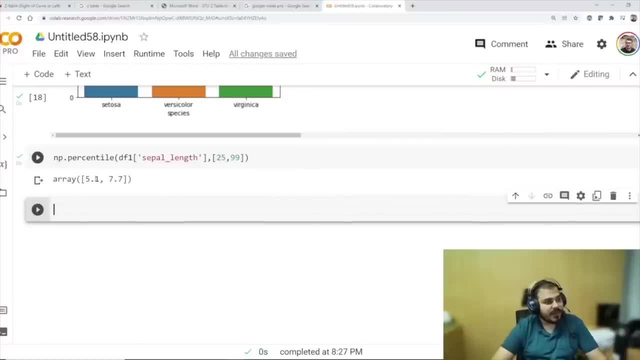 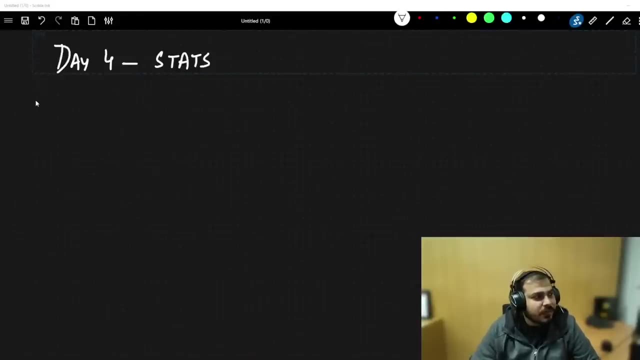 like this, 99, so here you will be able to get the value 5.1 and 7.7. hello guys. so how are you all? i hope everybody is doing well, so let's start today. what all things we are going to do. first of all, we are going to implement this iqr using python. okay, the second topic we are going to 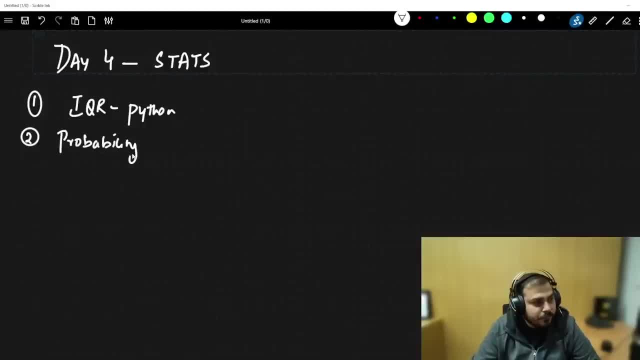 discuss about is probability. the third thing that we are going to discuss about is something called as permutation and combination. once we finish this up, the fourth thing that we are going to discuss about is something called as confidence intervals. so in confidence intervals then probably, if we get time, we will cover up p value and then we will start with hypothesis testing. now what we are 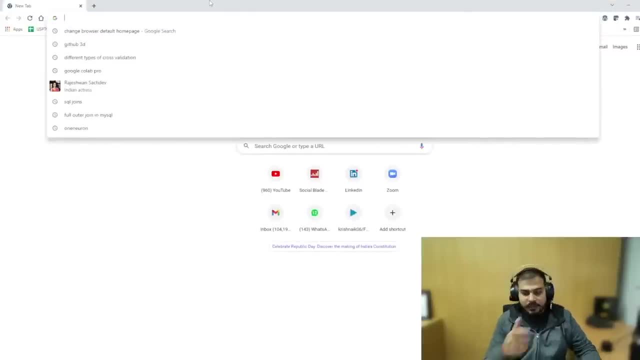 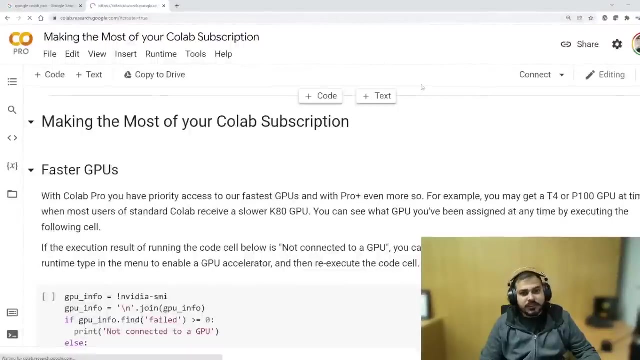 going to do. first of all, i am going to start with google collab. you can also open google collab, okay, so i will just make a new notebook. so first of all, we will try to implement z score and try to find out iqr and with respect to that, we will try to see what all things we can basically implement. 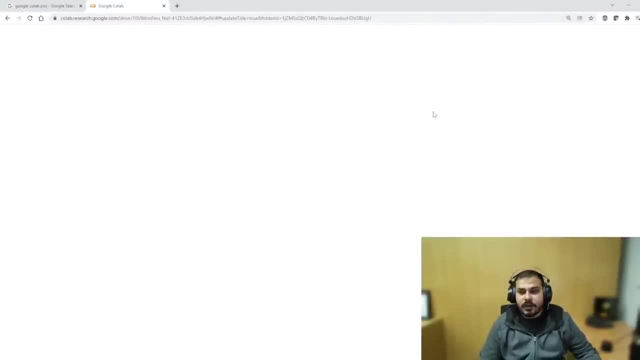 other distributions will also come. don't worry, bernoulli. binomial distribution, power law distribution- everything will be discussed. first, let's go in some specific order i have actually decided, and when that is, those distribution will basically come, we'll discuss about it. okay, here you go. 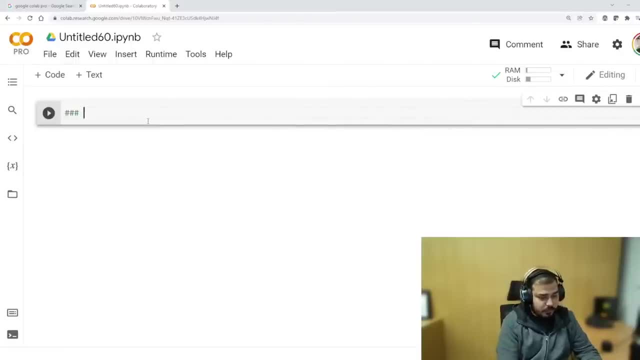 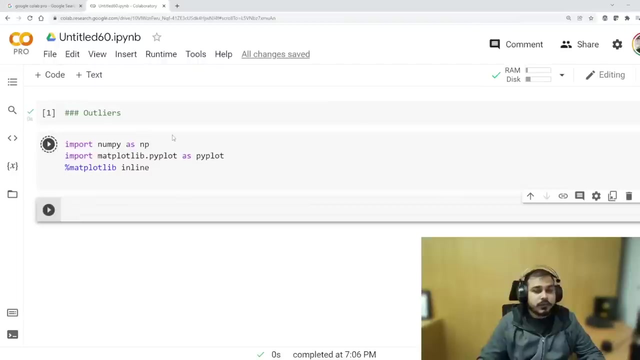 so in this session we are going to first of all discuss about outliers. now, first of all, what i am actually going to do over here is that i'm going to import some libraries, import numpy as np. okay, import matplotlib, dot, pyplot plus plt. then i'm just going to import matplotlib inline, so i'll be. 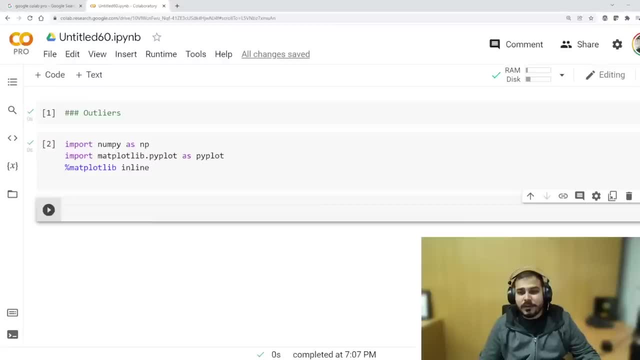 executing this now. the next thing that probably we will be discussing about is that let's define our data set. so here i'm going to just define our data set. data set: you can take up anything that you probably want. you can just define your own data set, whatever data set you. 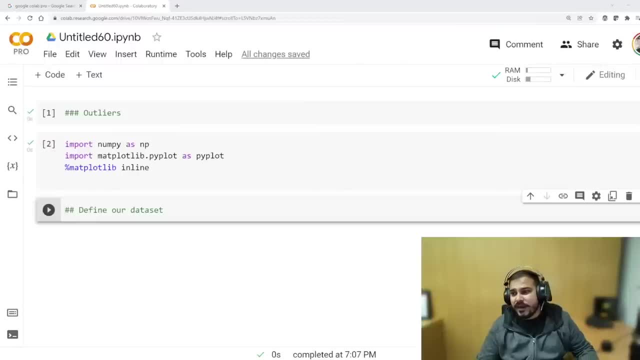 like now, for, for my sake, i have just created one data set over here, so here you will be able to see that this is my data set. can you say some numbers that are like kind of outliers in this? so uh, now the first thing that we are probably going to do is that let's say that. 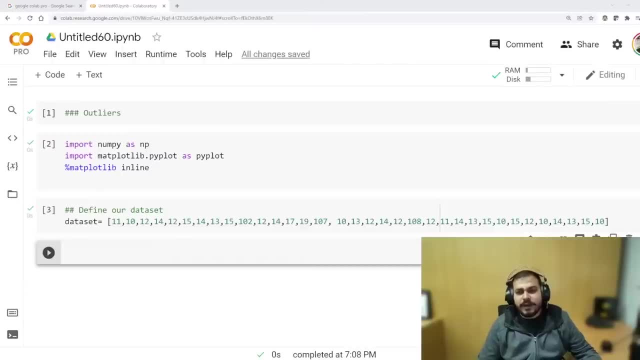 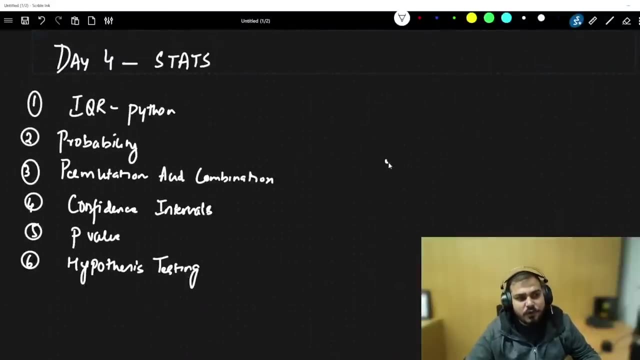 using z score. i probably want to also find out some outliers now using z score. how do you find out some outliers now? let me just go and explain you over here. let's say that you know about normal distribution till now. you have discussed- we have discussed- so many things in normal distribution. 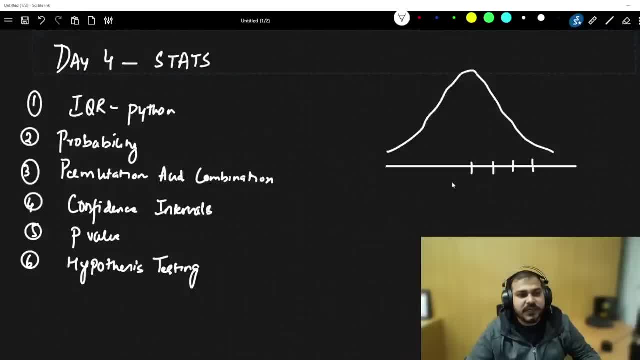 we know that this is the mean. first standard division, second standard division, third standard division, first, second and third standard division to the left. you know that 68 percentage of data, 95 percentage of data and 99.7 percentage of data. can i consider that during some of the scenarios, if my data is normally distributed? 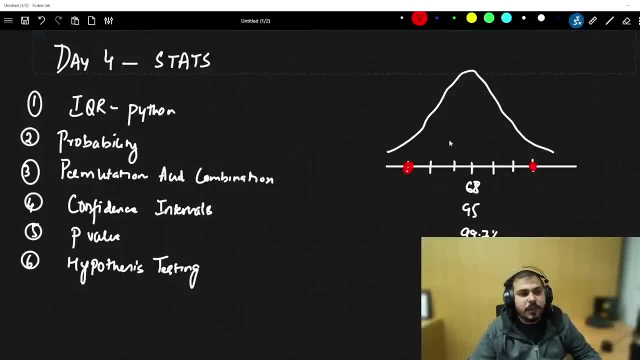 after the third standard deviation, probably the data are outliers, yes or no? yes, after third standard deviation, whatever data is basically present, right, data are outliers, yes or no? just think over it most of the time. if the values are, you know, are outliers, then the data is outliers. and if the values are outliers, then the data is. 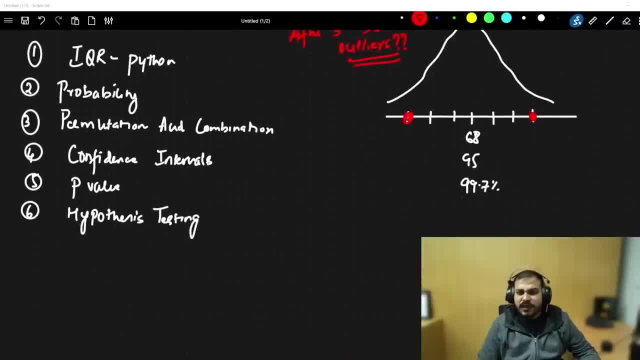 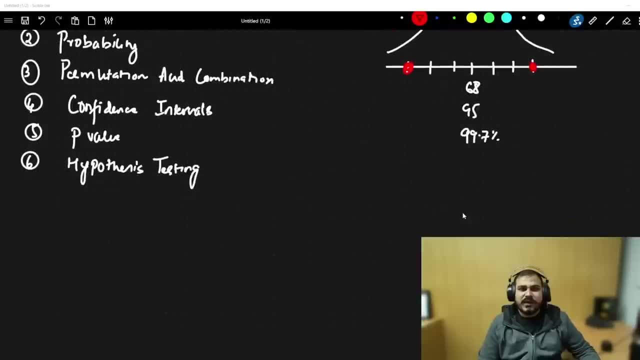 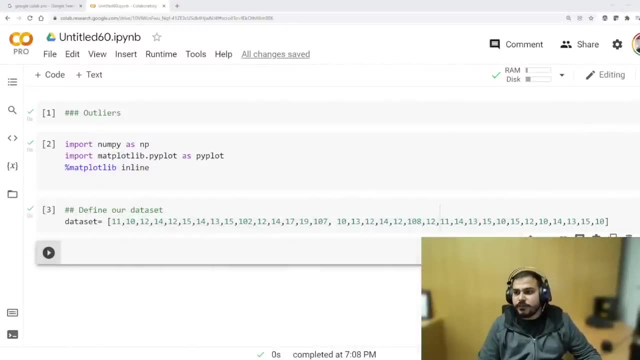 after probably third standard deviation. they are like kind of outliers, yes. so just think over it guys. it can be treated as an outlier, right? if? if data is present after third standard deviation. so first we'll try to implement this. now, what i am actually going to do over here is that, first of 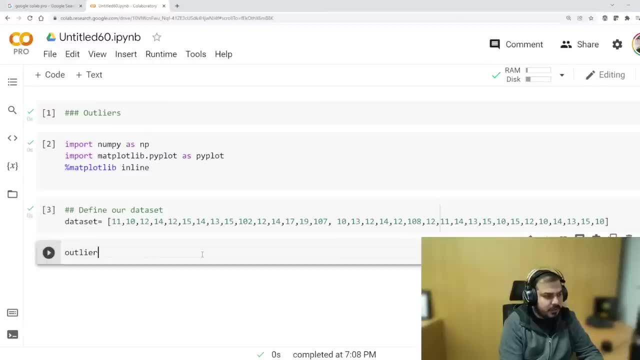 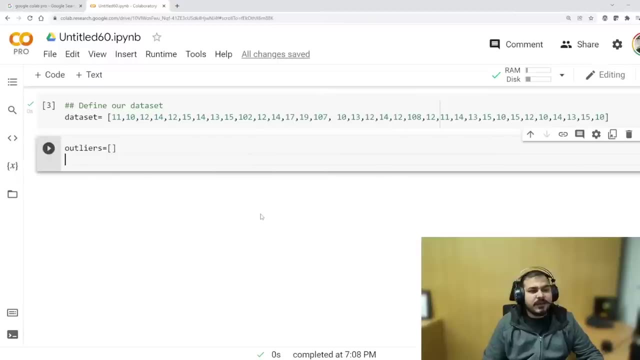 all, let me make a list, okay. so here i'm just saying it is outliers. i'm going to basically create it as a list and put up all outliers inside. let's define: and how do you find out standard deviation? or by using z score right, we can definitely find out z. 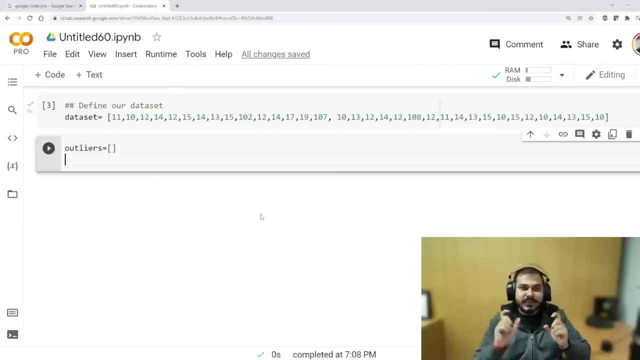 score with the help of z core how many data set or data points actually fall within the third standard deviation. so here i'm actually going to create a function which says define, detect, underscore outliers. so this will be my function, and here i'm going to give my data. now the first: 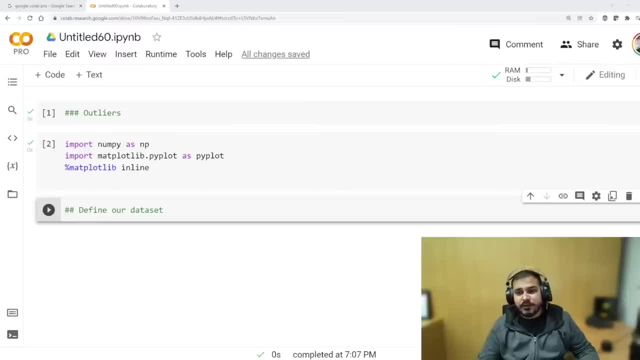 my sake. I have just created one data set over here, so here you will be able to see that this is my data set. can you say some numbers that are like kind of outliers in this? so now the first thing that we are probably going to do is that. 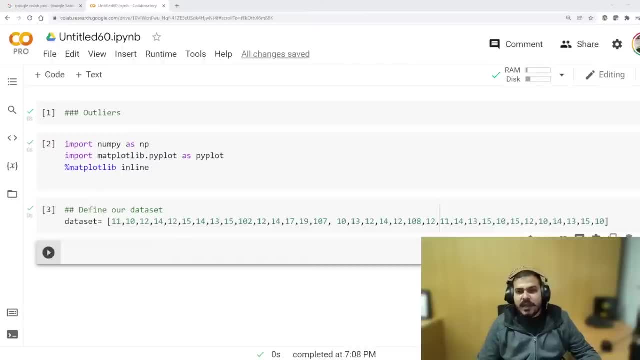 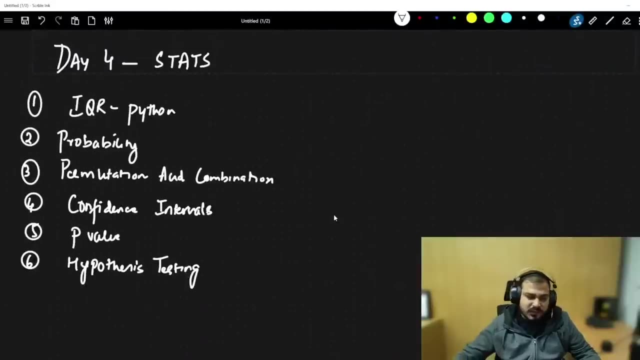 let's say that using z-score, I probably want to also find out some outliers now using z-score. how do you find out some outliers now? let me just go and explain you over here. let's say that you know about normal distribution. till now you have just 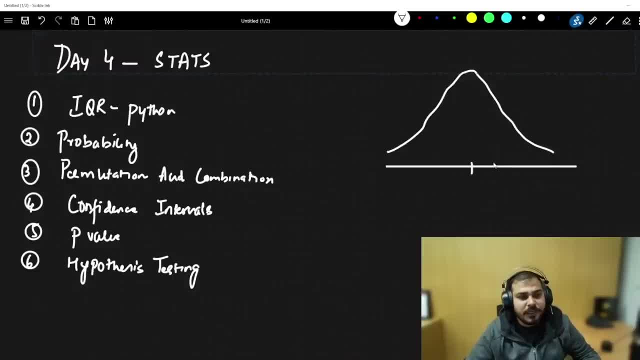 We have discussed so many things in normal distribution. We know that this is the mean: first standard deviation, second standard deviation, third standard deviation: first, second and third standard deviation to the left. You know that 68% of data, 95% of data and 99.7% of data. 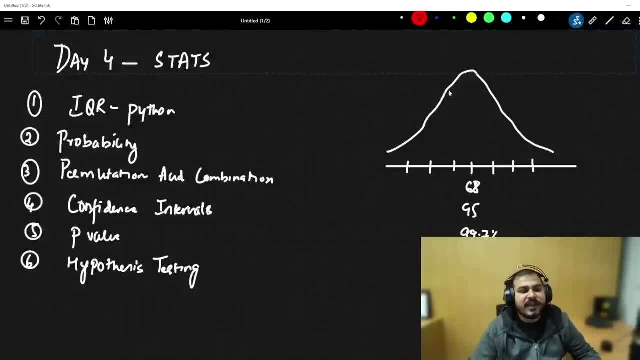 Can I consider that during some of the scenarios, if my data is normally distributed after the third standard deviation, probably the data are outliers, yes or no? Yes, After third standard deviation, whatever data is basically present right, Data are outliers, yes or no? 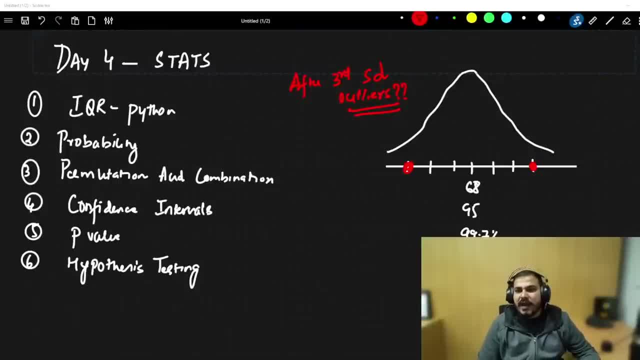 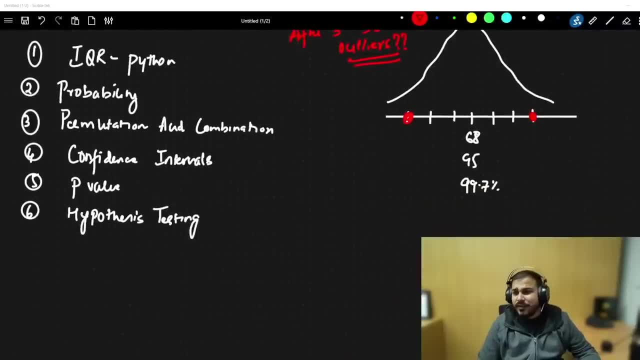 Just think over it. Most of the time, if the values are, you know, after probably third standard deviation, they are like kind of outliers, yes. So just think over it guys. It can be treated as an outlier, right If data is present after third standard deviation. 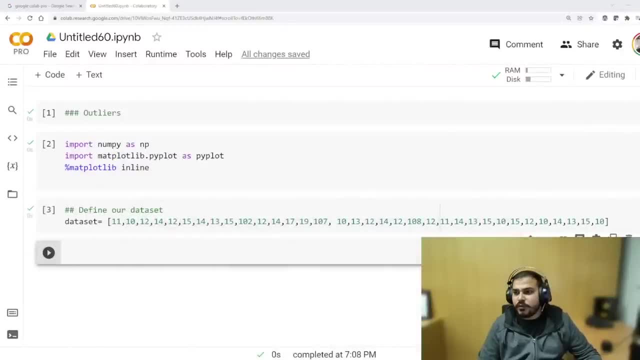 So first we'll try to implement this. Now. what I am actually going to do over here is that first of all, let me make a list. Okay, so here I'm just saying it is outliers. I'm going to basically create it as a list and put up all outliers inside. 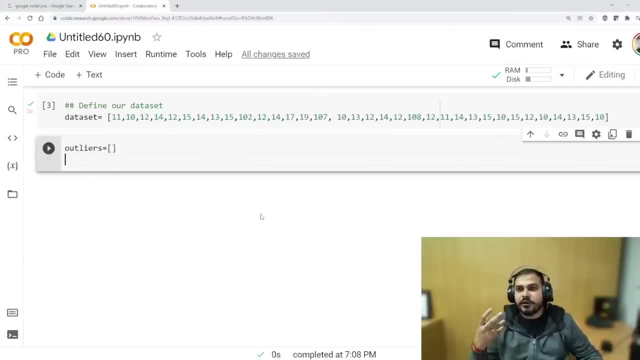 Let's define. and how do you find out? standard deviation? or by using Z-score, right, We can definitely find out Z-score with the help of Z-score, how many data set or data points actually fall within the third standard deviation. So here I'm actually going to create a function which says define, detect, underscore outliers. 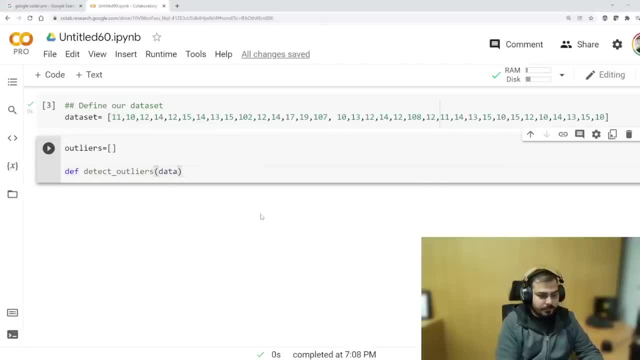 So this will be my function, and here I'm going to give my data. Now, the first thing that I will create a threshold. my threshold will basically be three standard deviation right. Anything that falls away from the three standard deviation I will basically be able to do. 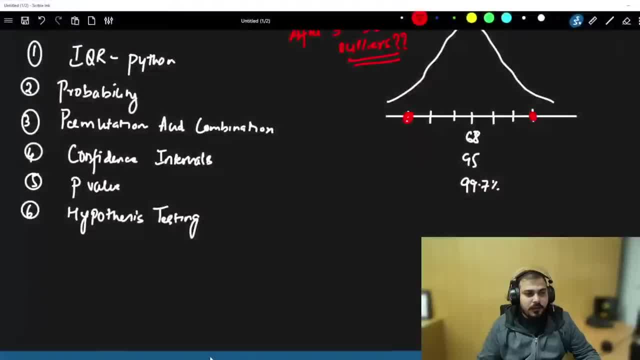 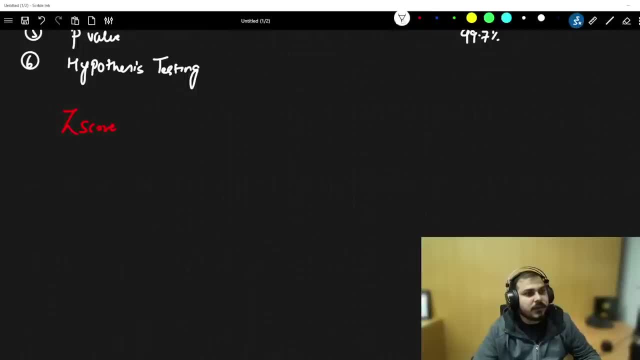 it And I hope everybody remembers the formula. The formula for Z-score is what? if I go and probably define over here, my Z-score formula is nothing, but it is X of I minus mu divided by standard deviation. We usually also write this formula by root n, but I'll talk about it. why specifically? 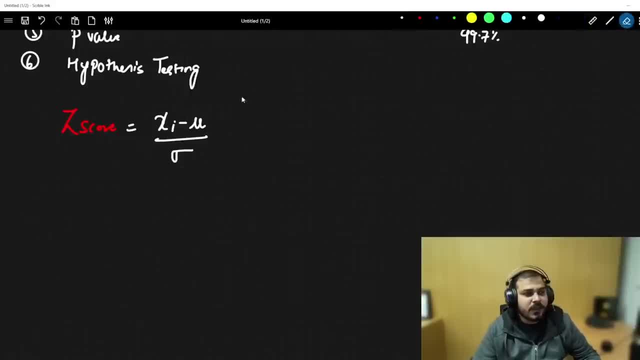 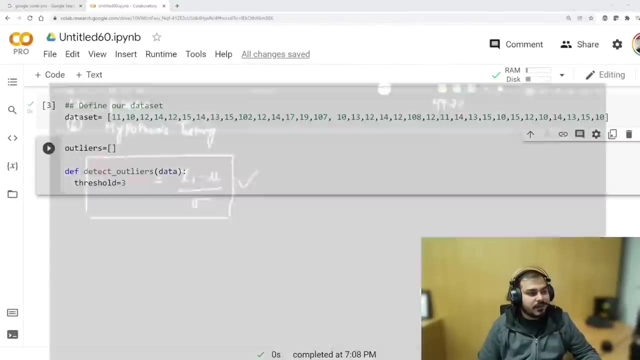 I'm not specifying root n over here. Over here, I'll just try to use this formula. Okay, So this is basically the Z-score formula. Okay, So I have to implement this formula in Python programming language. Okay, So what I'm actually going to do? first of all, obviously in in: in this I need to 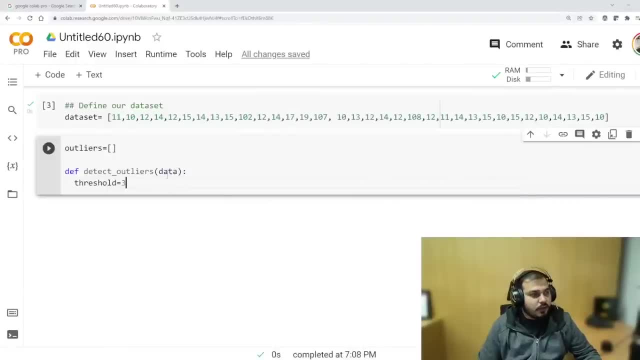 compute mean, I need to compute standard deviation. You know how to compute mean, right? So here I will say: mean is equal to NP dot mean, And here I can actually give my data points which will actually help me to find out mean. 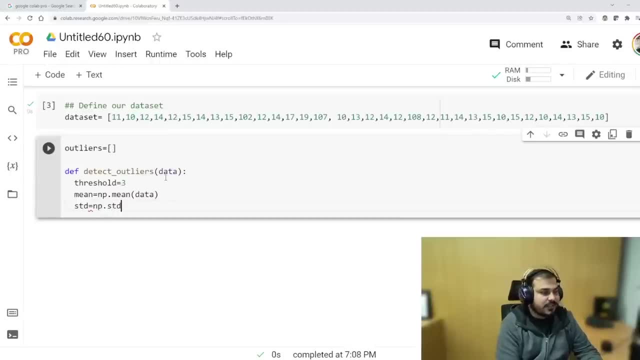 Then my standard deviation. here I can basically write NP dot standard deviation, Okay, And from that specific data I will be able to get the standard deviation. So I have got my mean and standard deviation. Now, for each and every points inside my data set, I will just apply the Z-score formula. 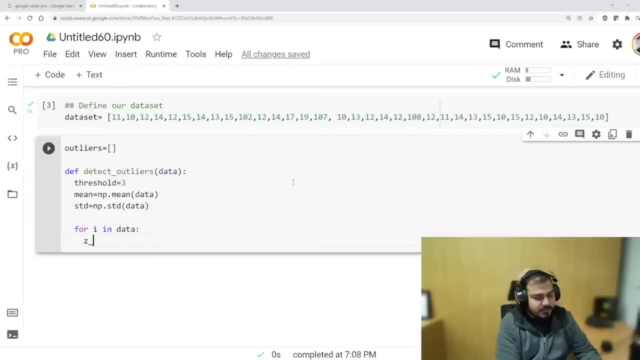 So I'll say for I in data I can say Z-score is equal to I. I is my X of I points right. I'll say X. I minus mean right Divided by standard deviation. So this is my Z-score formula. 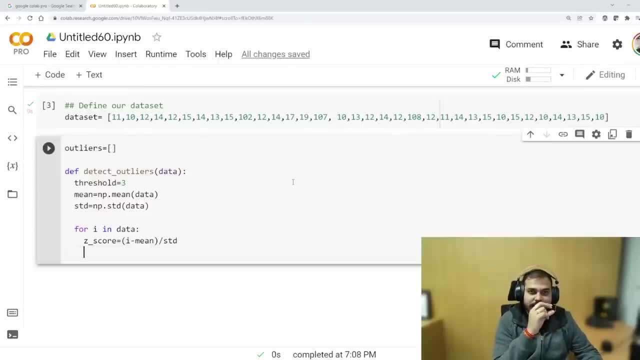 And for every item I'm actually trying to get the standard deviation. Okay, For every item I'm actually trying to find out the Z-score formula. Z-score will basically give you how many standard deviation it is away from mean. So I can write one condition to check whether it falls below the third standard deviation or not. 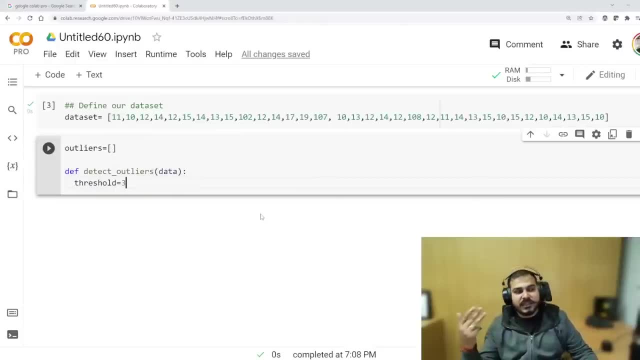 thing that i will create a threshold. my threshold will basically be three standard deviations, right, anything that falls away from the three standard deviation. i will basically be able to do it and i hope everybody remembers the formula, the formula for z score is what if i go, and probably 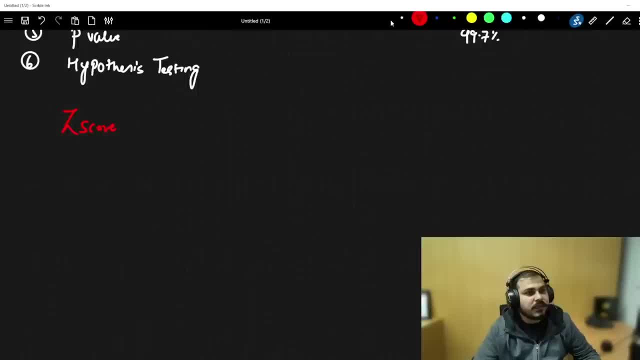 define over here. my z score formula is nothing, but it is x of i minus mu divided by standard deviation. we usually also write this formula by root n, but i'll talk about it why specifically i'm not specifying root n over here. over here i'll just try to use this formula. okay, so this is basically the z score formula. 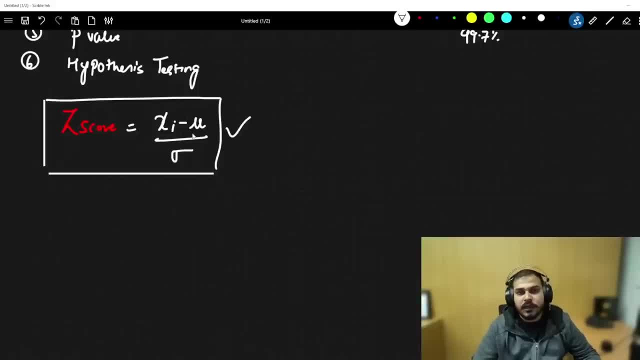 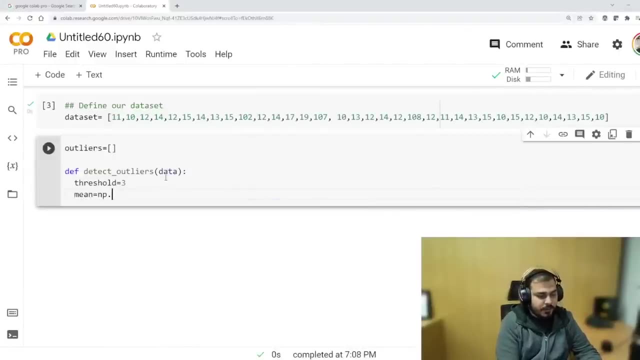 okay, so i have to implement this formula in python programming language. okay, so what i'm actually going to do? first of all, obviously, in in this, i need to compute mean, i need to compute standard deviation. you know how to compute mean, right? so here i will say: mean is equal to np, dot, mean. 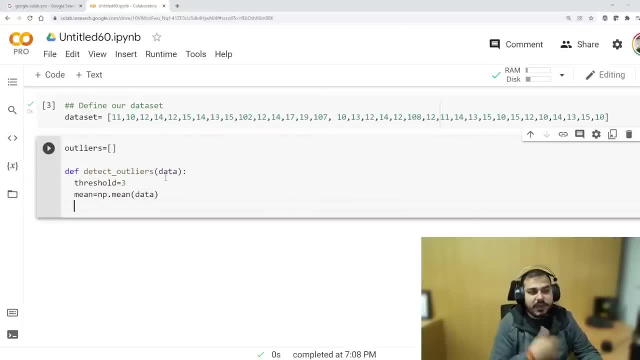 and here i can actually give my data points which will actually help me to find out mean, then my standard deviation. here i can basically write np, dot, standard deviation of that specific data. i will be able to get the standard deviation. so i have got my mean and standard deviation now. 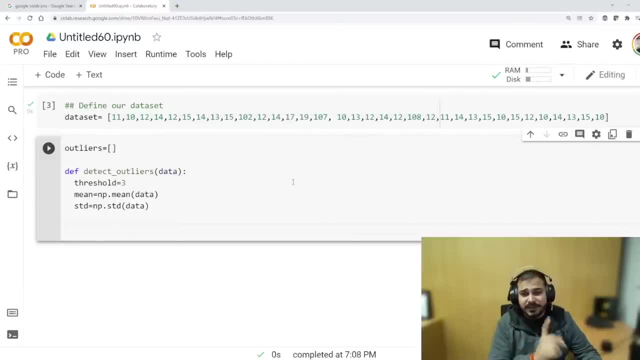 for each and every points inside my data set i will just apply the z score formula. so i'll say for i in data i can say z score is equal to i. i is my x of i points right. i'll say x. i minus mean right divided by standard deviation. so this is my z score formula and for every item i'm actually 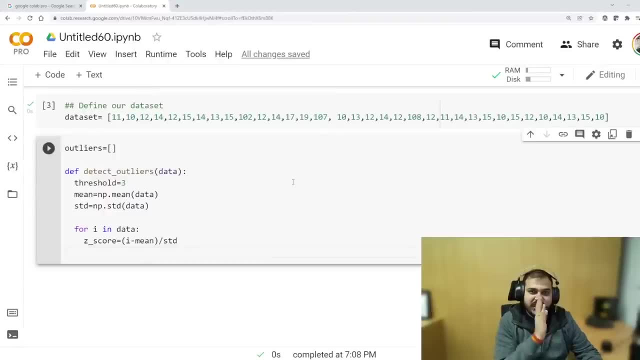 trying to find out the z score formula. z score will basically give you how many standard deviation. it is away from me. so i can write one condition to check whether it falls below the third standard deviation or not. so i can basically use nb dot absolute, which will basically help us to round. 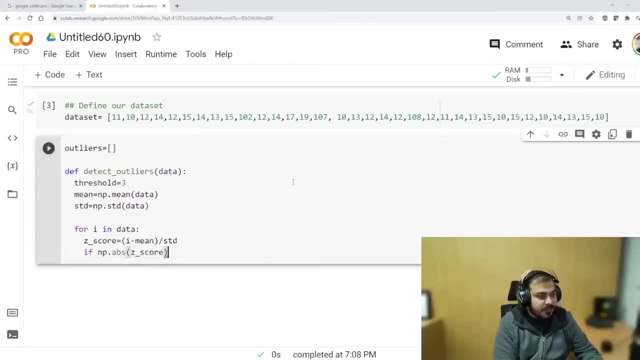 off the z score and i'll say: z underscore score is greater than threshold. if it is greater than threshold, what does this basically mean? let's, let's define threshold over here. i have already defined threshold, right. so if it is greater than threshold, then what does this basically mean? 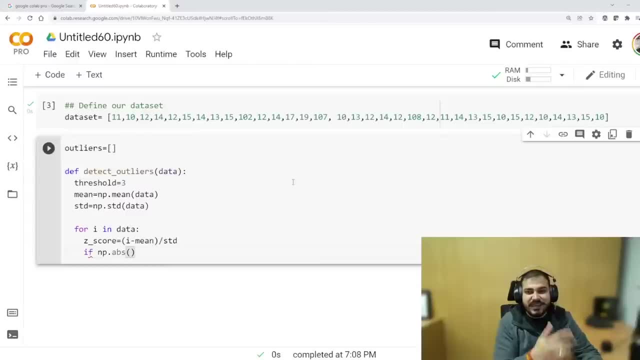 So I can basically use NP dot absolute, which will basically help us to round off the Z-score, And I'll say Z underscore score is greater than threshold. If it is greater than threshold, what does this basically mean? Let's define threshold over here. 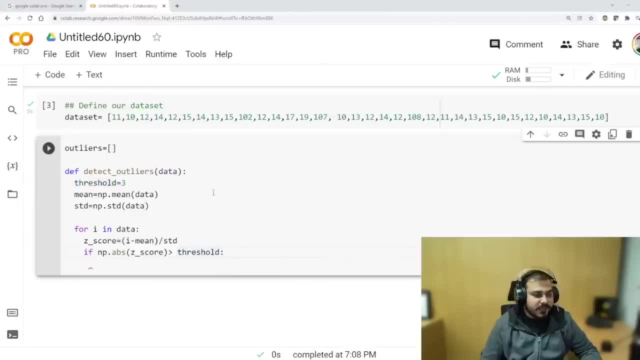 I have already defined threshold, Right. So if it is greater than threshold, then what does this basically mean? Oh sorry, It is dataset. I'm extremely sorry, Dataset. Now tell me, if NP dot apps Z-score greater than threshold, what should I do? 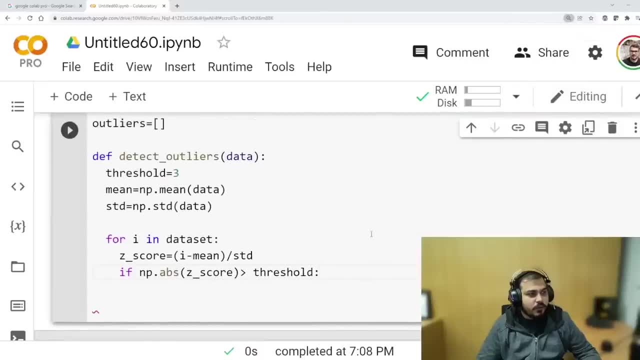 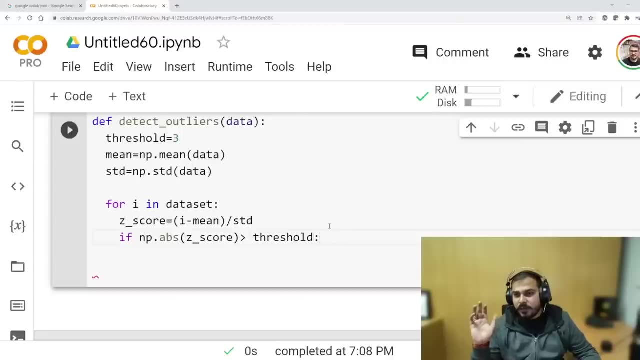 What does this basically mean? Create more clarity, you want, I think. now it is fine, Right. What should we do in this? This basically means that it is an outlier right Because it is falling away from third standard deviation. It is falling below or beyond the third standard deviation. 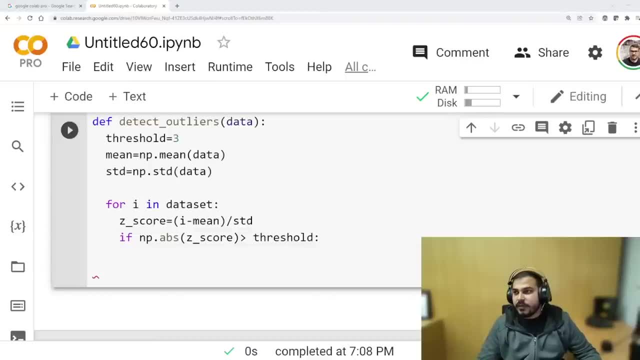 So what I can basically do is that I can just write something like this, because I have created a list, So I'll say outlier dot append, and I'm going to append that specific Z-score value. So I hope it is fine. I'm just going to append this Z-score value, not Z-score. 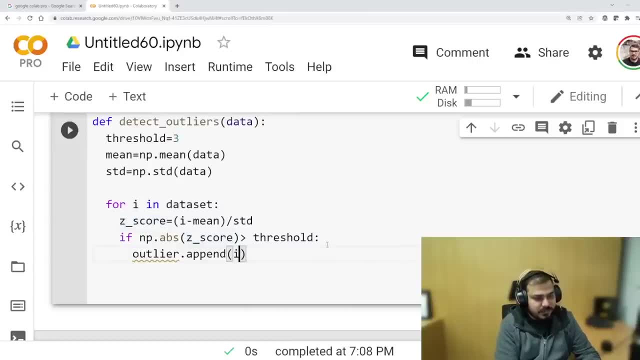 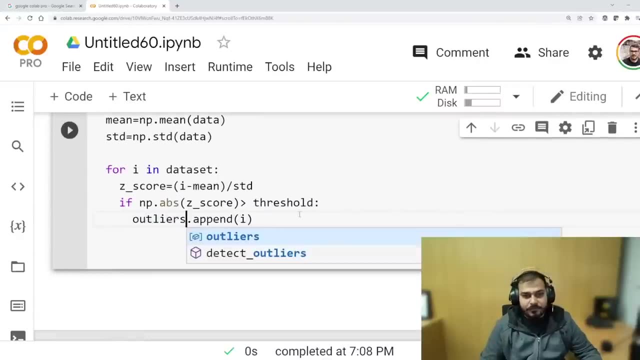 I will append the I value because I in dataset. yes, I'm just going to append this. I. yeah, outliers, Sorry, Outliers dot. append of I. And then, finally, what I'm actually going to do: I'm just going to return the outliers. 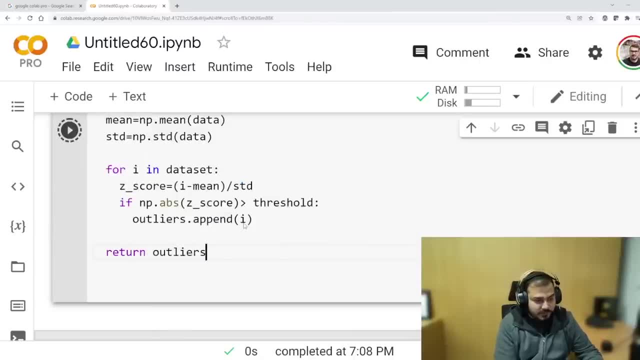 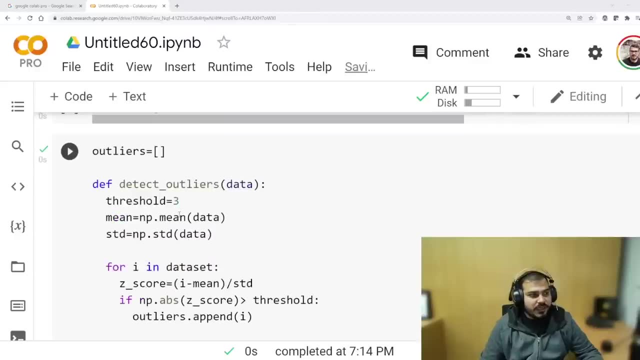 Return outliers. Let's see whether it will work or not. I'm also trying it for the first time, So this is my function. that has got executed. I will just execute one more code. Threshold three basically means this: This defines our third standard deviation, below like beyond. third standard deviation. 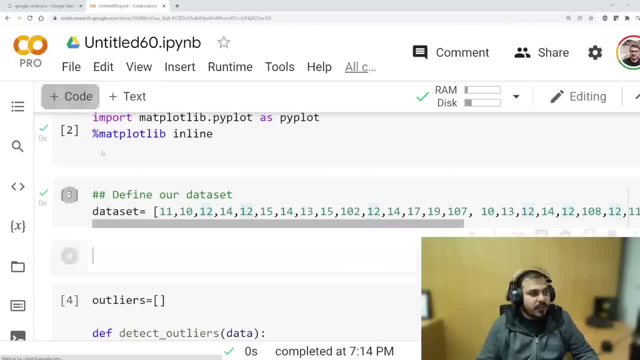 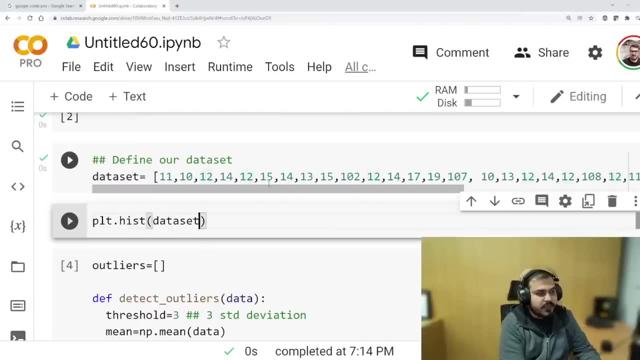 I can basically say that this actually falls on. If you want to probably go and check how this distribution is, So I can write plot dot hist on a specific dataset. PLT is not defined, Why? Okay, This should be PLT. 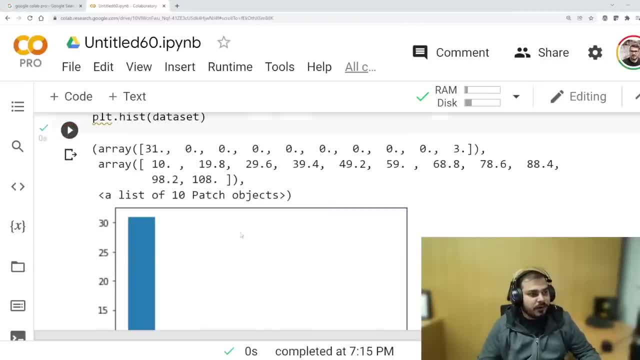 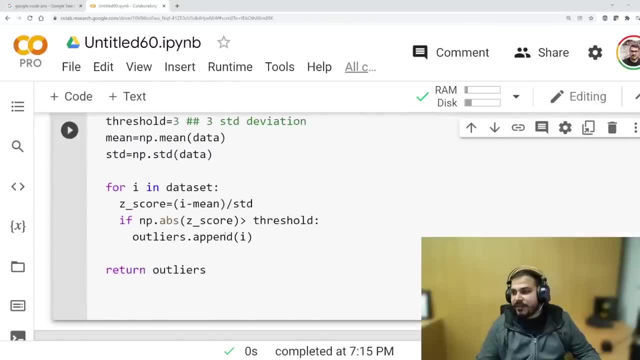 It's okay Whether it is normally distributed or not, but I am actually trying to see this. Okay, There are some definite outliers, but it's okay, Let's see that, whether we will be able to do this or not. What is which arg passed as change dataset, data in for loop. 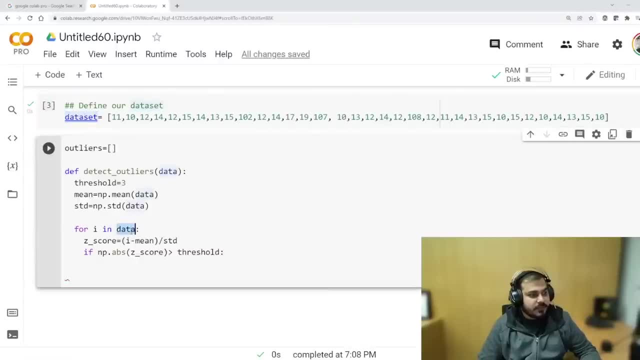 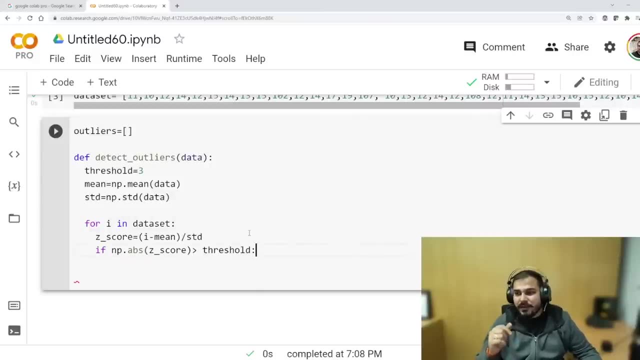 oh, sorry, it is data set. i'm extremely sorry. data set. now tell me: if np dot apps z score greater than threshold, what should i do? what does this basically mean? create more clarity, you want. i think now it is fine, right, what? what should we do in this? this basically means that it is an 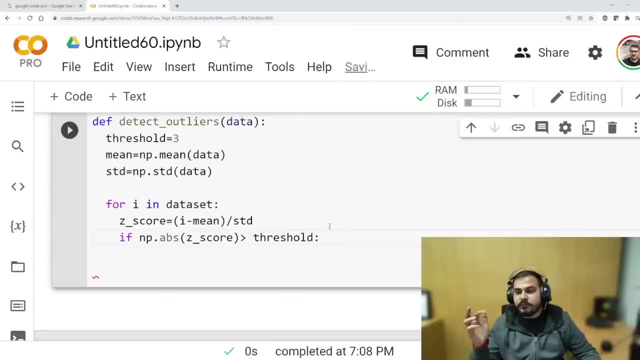 outlier right, because it is falling away from third standard deviation. it is falling below, uh, beyond, the third standard deviation. so what i can basically do is that i can just write something like this, because i have created a list, so i'll say outlier dot append, and i'm going to append that specific z score value. 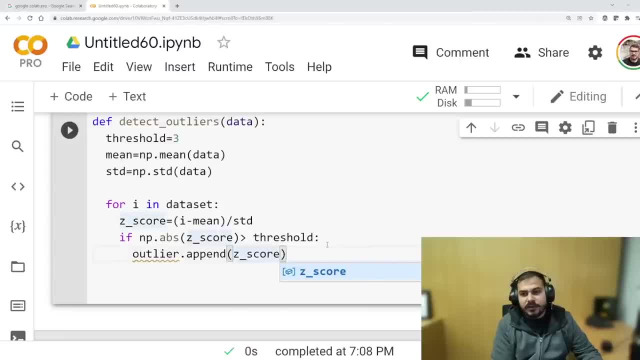 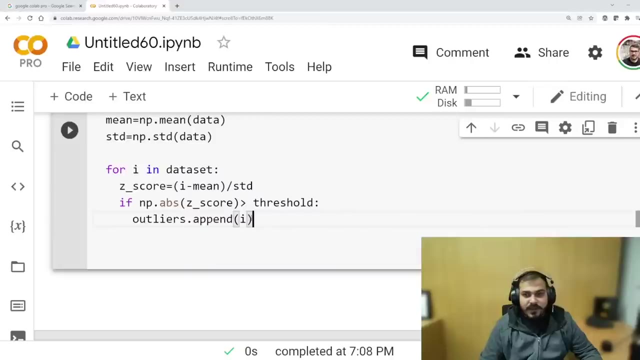 so i hope it is fine. i'm just going to append this z score value, not z score. i will append the i value because i in data set. yes, i'm just going to append this i, yeah, outliers- sorry, it is outliers- dot- append of i and then finally, what i'm actually. 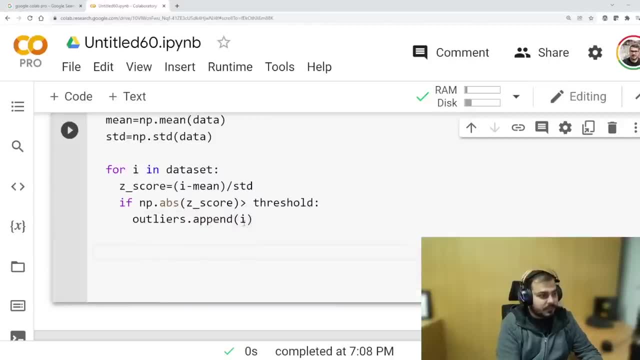 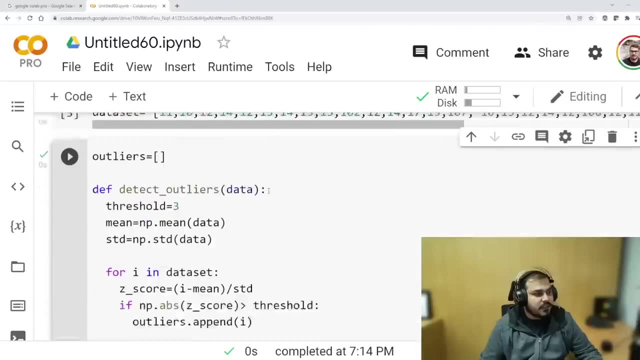 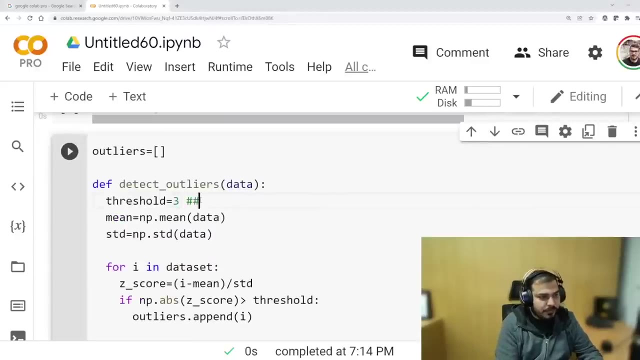 going to do? i'm just going to return the outliers. return outlier. let's see whether it will work or not. i'm also trying it for the first time, so this is my function. that has got executed. i will just execute one more code. threshold three basically means this: this defines our third standard. 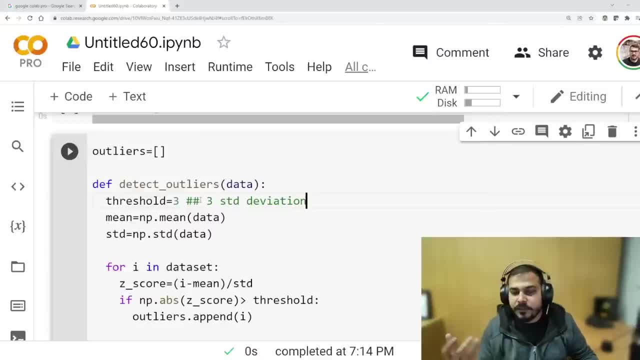 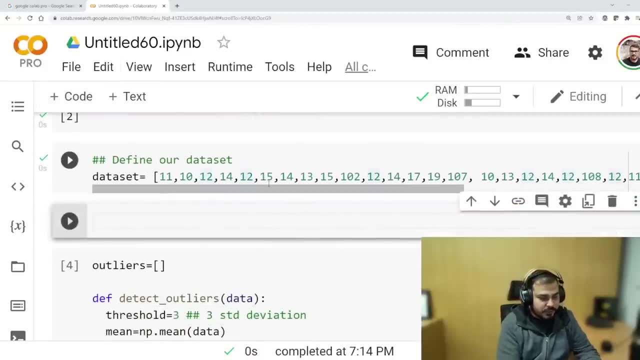 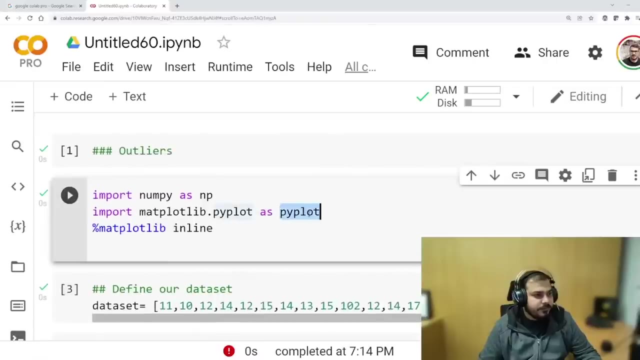 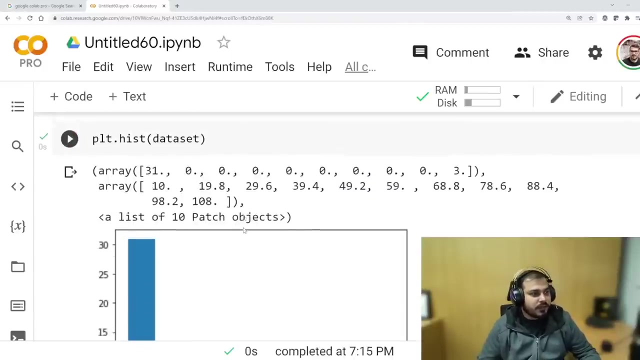 deviation below like beyond third standard deviation. i can basically say that this actually falls on. if you want to probably go and check how this distribution is so i can write plot dot hist. on a specific data set, plt is not defined. why? okay, this should be plt. it's okay whether it is normally distributed or not. but i am actually 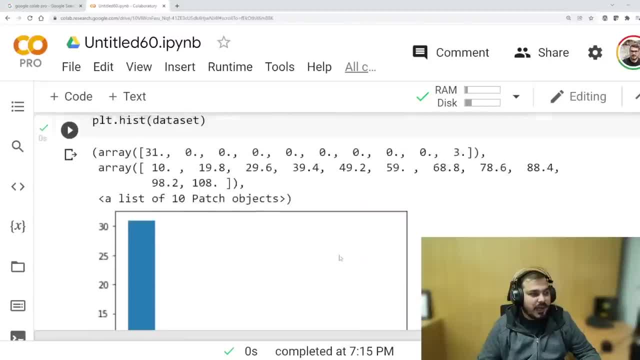 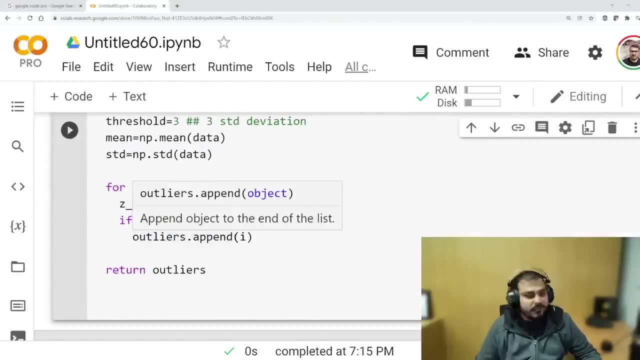 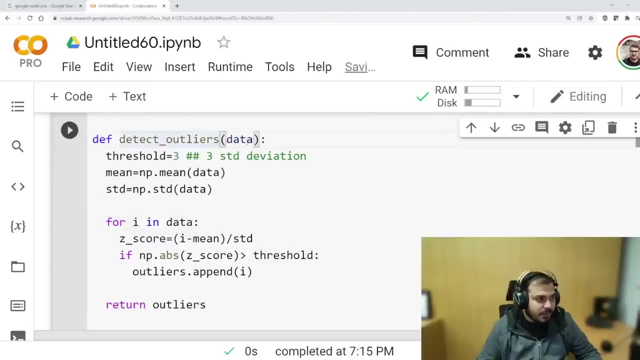 trying to see this. okay, there are some definite outliers, but it's okay, let's see that, whether we will be able to do this or not, what is which are passed has changed data. set data in per loop. it is simple, right, guys? this, this function, everybody understood, or not? oh sorry, this should be data. this data i am actually passing over here, see. 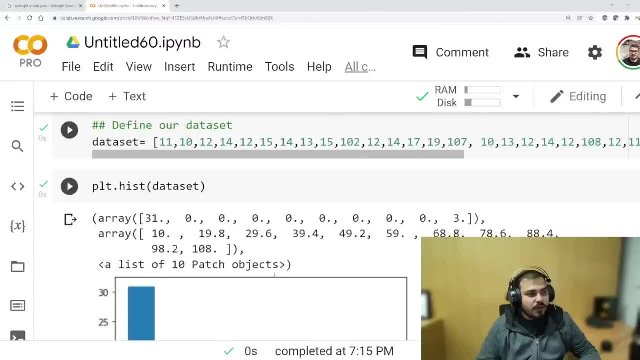 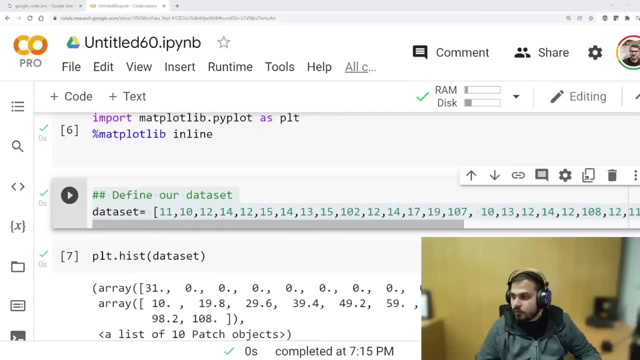 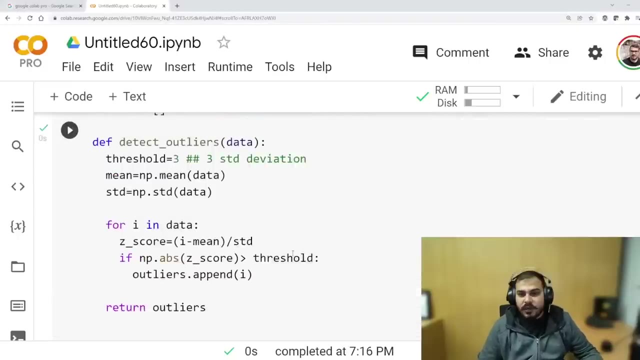 threshold. threshold. here is my third standard deviation. if you want the data set, i can paste this entirely and give in the chat. so this is my chat with respect to the data set. i've already given it to you all. now let's go and execute it now. i have executed this. now what i am actually. 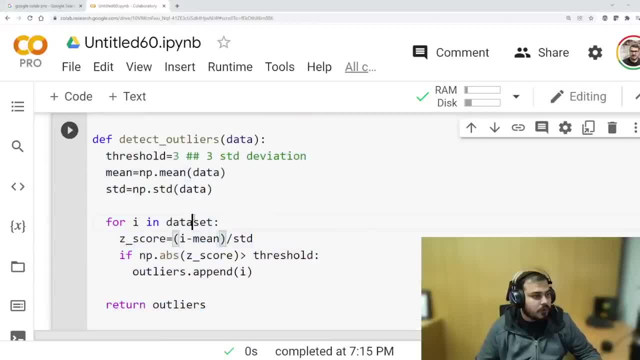 It is simple, right, Guys? this, this function, everybody understood, or not? Oh sorry, This should be data. This data I'm actually passing over here, See threshold Threshold. here is my third standard deviation. If you want the dataset, I can paste this entirely. and, given the chat, 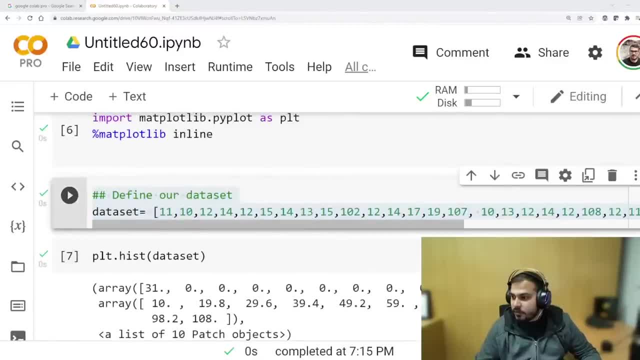 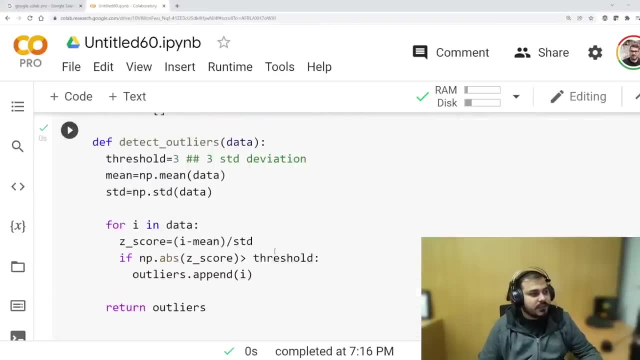 So this is my chat with respect to the dataset. I've already given it to you all. Now let's go and execute it. Now I have executed this. Now, what I'm actually going to do over here, I'm just going to call detect underscore. 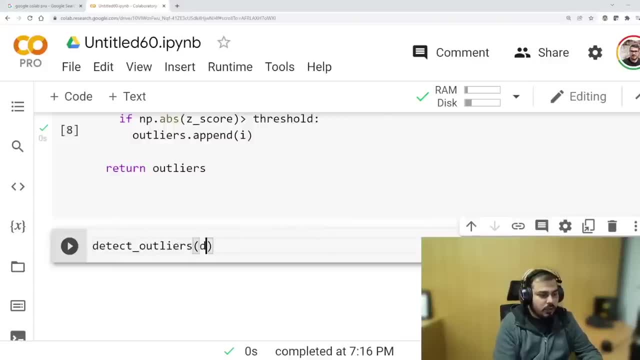 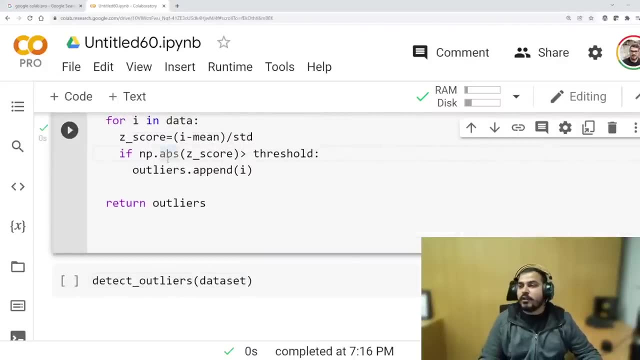 Outliers And I'm going to call this specific dataset The dataset NB dot apps. NB dot apps basically means NB dot, absolute, absolute function. Now, once I execute it here, you will be seeing that it will be returning this three outline: 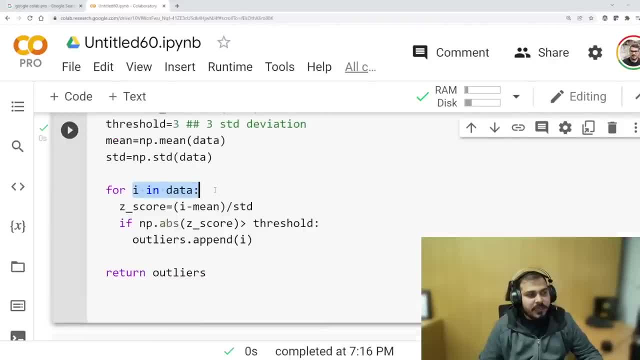 Are these my outliers or not, guys? The for loop is very simple for I. in data, I'm finding for every data which is in the form of list, all the Z score And I'm comparing if the Z score is greater than three or not. 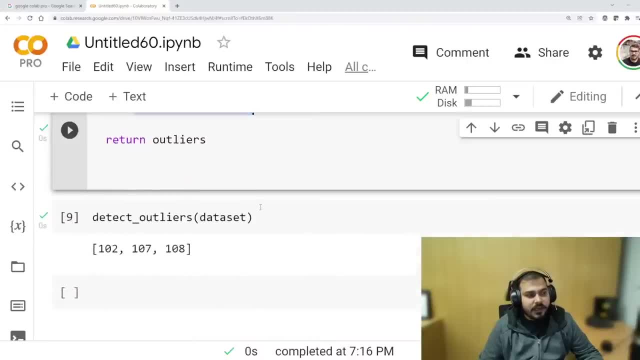 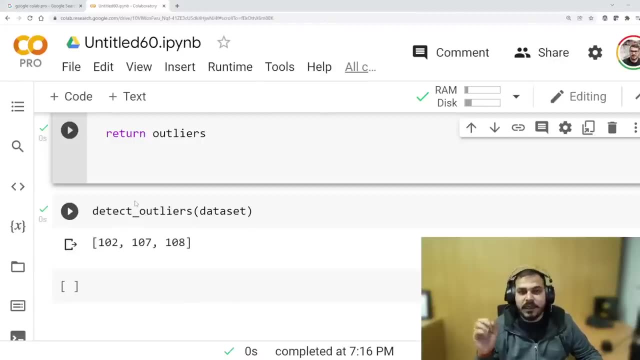 If it is greater than three, I'm considering it as an outlier. Here you can see. all the outliers are there. Outliers means a big number, right? If you have not attended the previous session, guys see. if you have not attended the previous session, you can drop off. 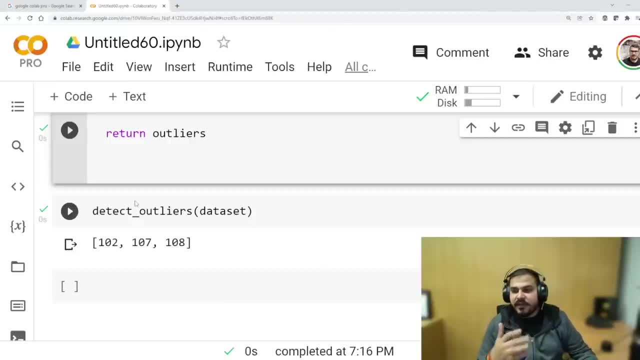 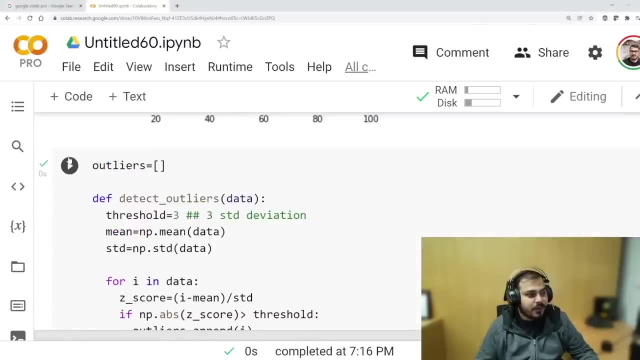 Okay, because you'll not be able to understand. This is a seven days live session. Now I have got the outliers. Now this is one way how we can use Z score. So this was an example of actual Z score, So I'm just going to write it as Z score. 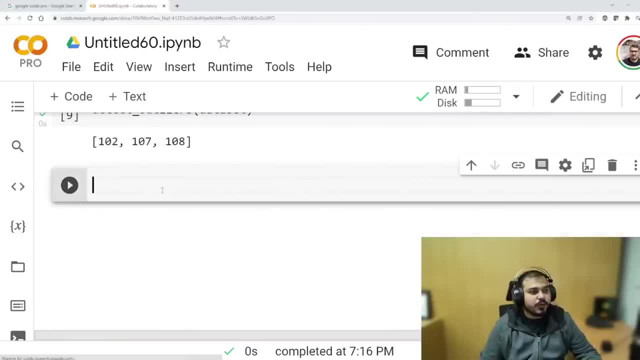 Z score computation And basically we have done it. Now let's go towards the IQR. IQR basically means interquartile range. So for interquartile range, what type of code I will be writing- Always understand- in IQR? what are we discussing in IQR? 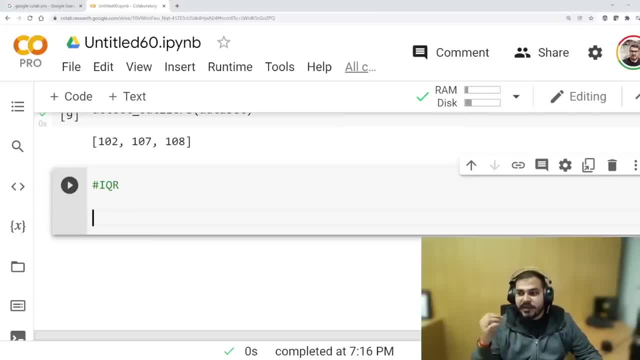 First of all we need to find out Q1. Q1 is 25 percentile. Then we have Q3. Q3 is 75 percentile. Then if I subtract 75 percentile minus 25 percentile, I will basically get the IQR. 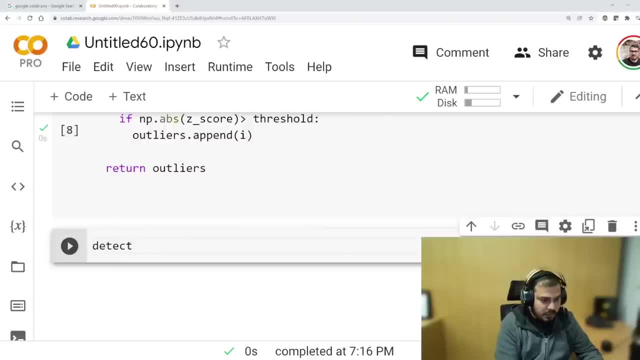 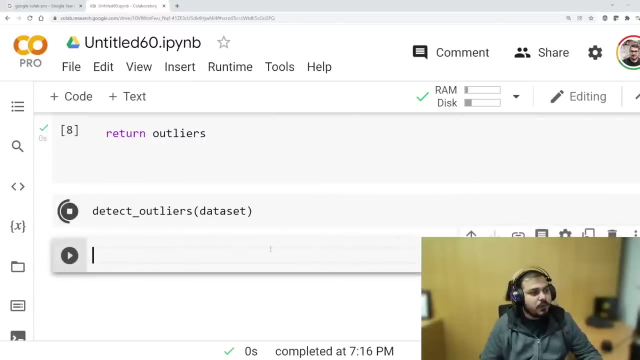 going to do over here. i'm just going to call detect underscore- outliers and i'm going to call this specific data set, the data set nbabs. nbabs basically means nbabsolute absolute function. now, once i execute it here, you will be seeing that it will be returning this three outliers. are these my outliers or not? guys, the for loop is very simple. 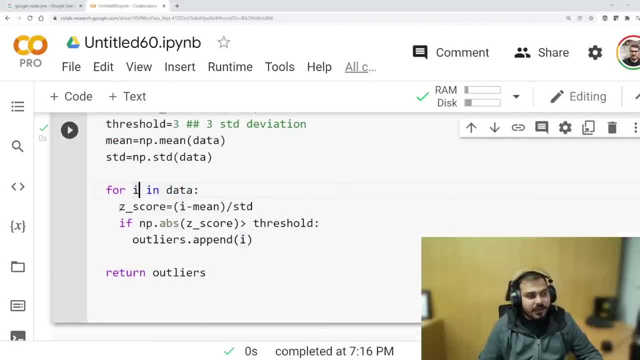 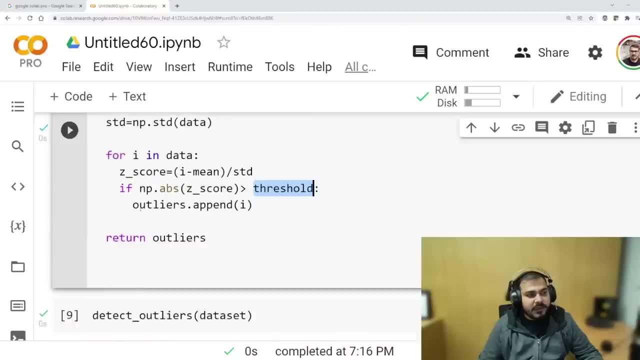 for i in data, i'm finding, for every data which is in the form of list, all the z score and i'm comparing if the z score is greater than three or not. if it is greater than three, i'm considering it as an outlier. here you can see all the outliers are there. outliers means a big number, right, if you? 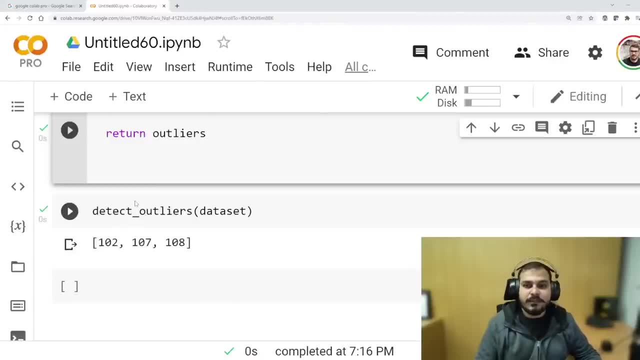 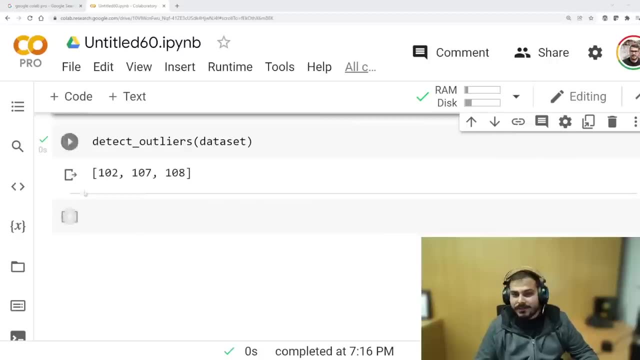 have not attended the previous session. guys see, if you have not attended the previous session, you can drop off, okay, because you'll not be able to understand. this is a seven days live session. now i have got the outliers. now this is one way how we can use z score. so this was an example of actual 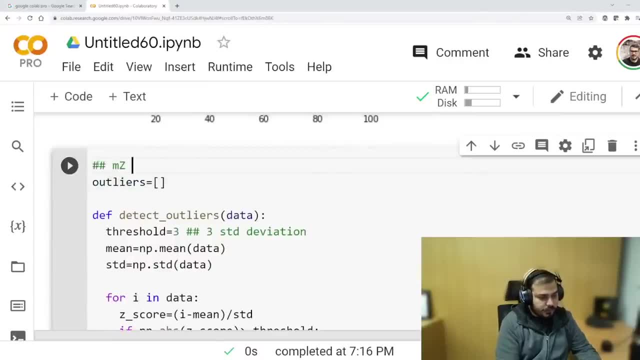 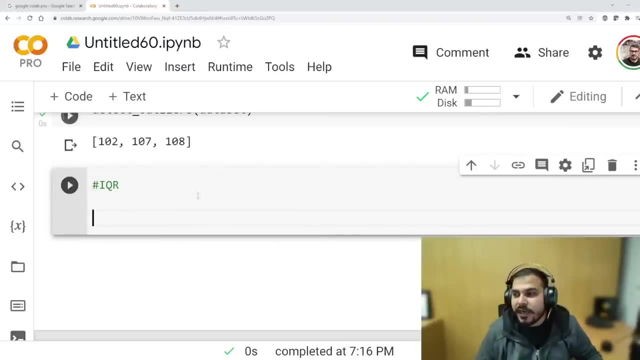 z score. so i'm just going to write it as z score, z score computation and basically we have done it. now let's go towards the iqr. iqr basically means interquartile range. so for interquartile range, what type of code i will be writing? 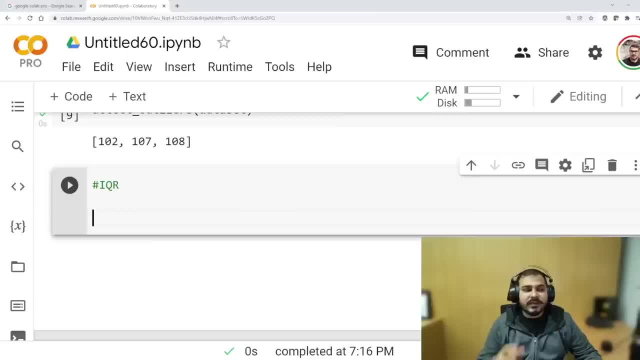 always understand in iqr. what are we discussing in iqr? first of all, we need to find out q1, q1 is 25 percentile. then we have q3. q3 is 20- 75 percentile. then if i subtract 75 percentile minus 25 percentile, 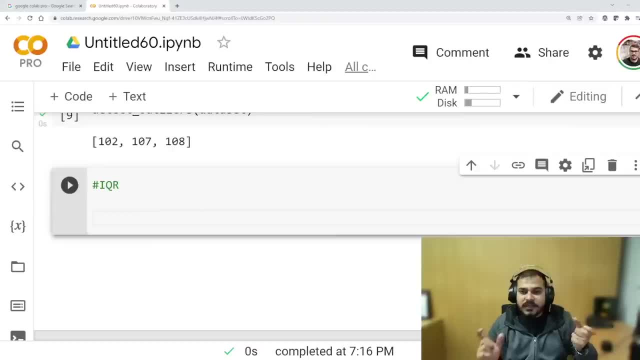 i will basically get the iqr right and always understand in iqr what we do. we basically find out what. what do we do in iqr? in iqr we basically find out the low, the lower fence and higher fence that we really need to find out in case of iqr. so how do i write the code? because this theoretical. 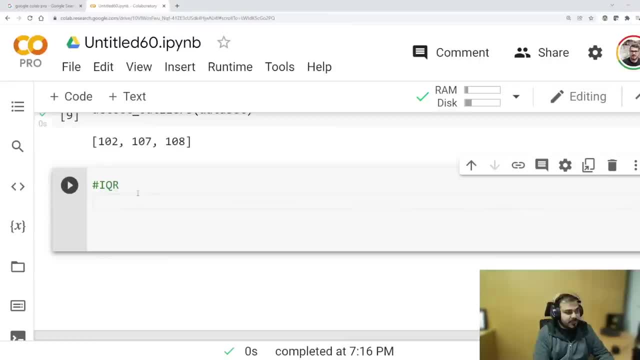 is already explained, so i'll write down all the steps that is required. so the first step is that i want to arrange, i want to sort the data. let's say that i'm sorting the data. okay, this is the first step. the second step is that i will calculate q1 and q3. 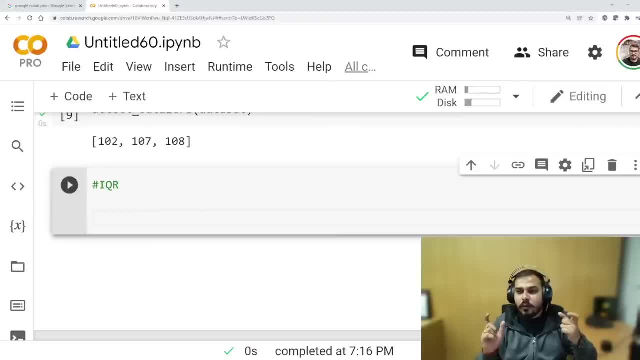 Right And always understand in IQR what we do. We basically find out What do we do in IQR. In IQR, we basically find out the lower fence and higher fence That we really need to find out in case of IQR. 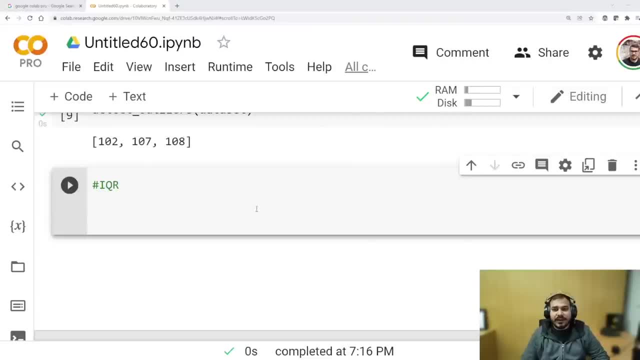 So how do I write the code? Because this theoretical is already explained, So I'll write down all the steps that is required. So the first step is that I want to arrange, I want to sort the data. Let's say that I'm sorting the data. 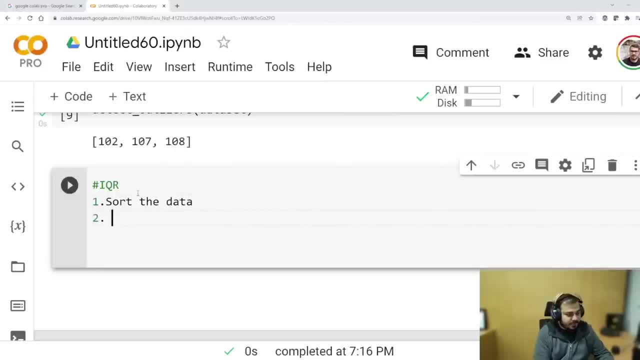 Okay, This is the first step. The second step is that I will calculate Q1 and Q3.. Q1 and Q3 is pretty much important in this particular case, So I need to do it in this scenario. I'll just move this up. 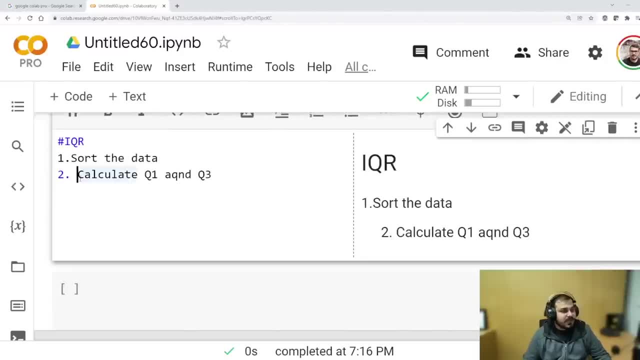 I'll copy and paste it over here. So the first step is basically calculate, sort the data And then calculate Q1 and Q3.. Then we need to find out IQR, which is nothing but the third step, which is nothing but the subtraction of Q3 minus Q1. 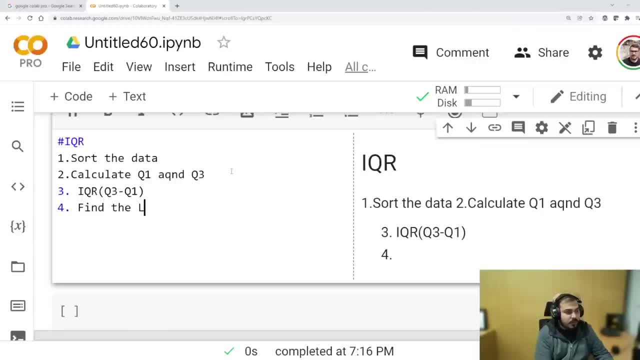 Then we need to find the lower fence. Find the lower fence Now. lower fence formula. I hope everybody knows it. So it is nothing but Q1, Q1, Q1 plus or minus. It is Q1 minus 1.5 multiplied by IQR. 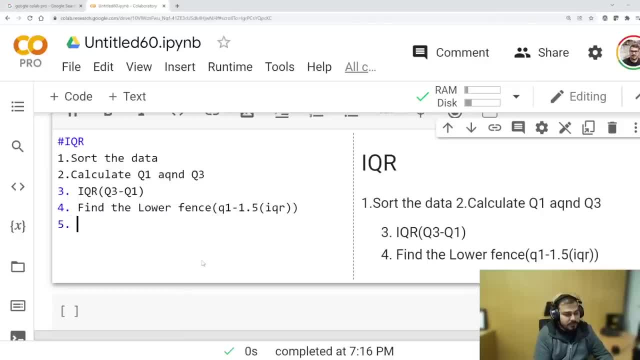 Right, This is the formula to basically find out the lower fence, Then find the upper fence. Here I will basically be using Q3 plus 1.5 multiplied by IQR. So these are the steps that we are probably going to do. 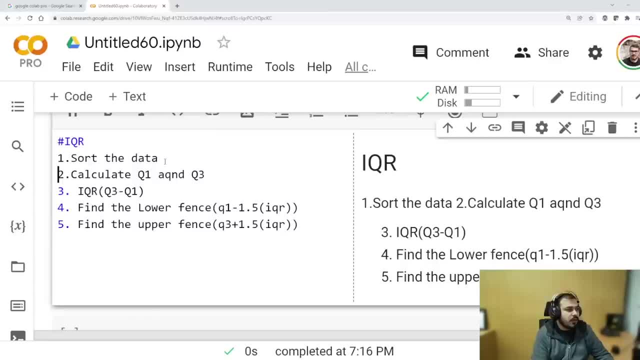 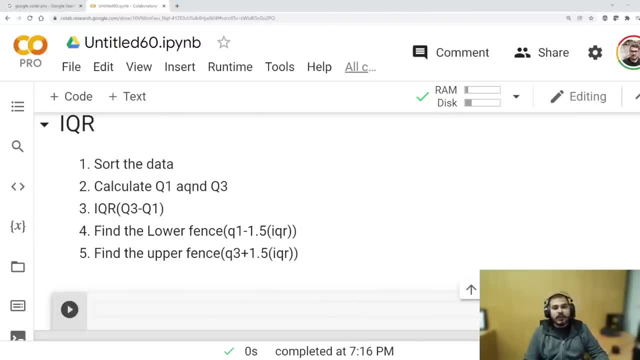 So these are my steps that I am actually going to plan for And, based on these steps, I will be implementing it. So these are the steps that I will be performing in order to find the outliers with the help of IQR. Now, first of all, if I really want to find out the sorted data. 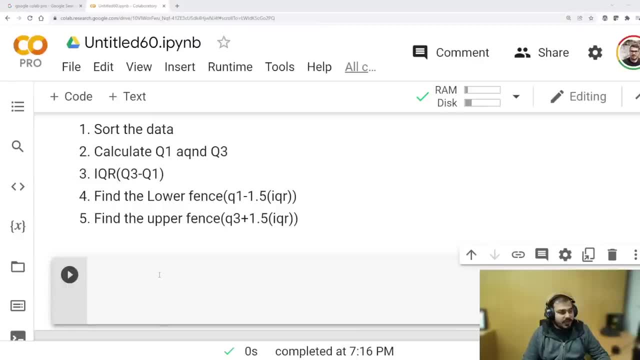 how do I find out the sorted data set? Sorted data set. I will just say this will be my data set And I can use sorted function And in sorted function, if I give you the data set, this will basically be my sorted data set. 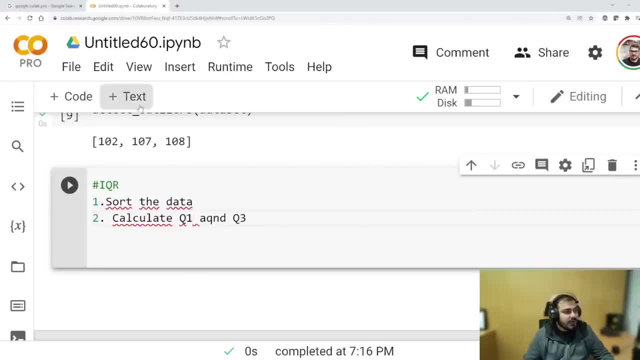 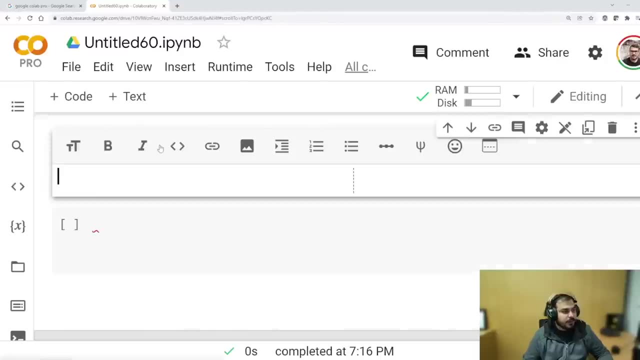 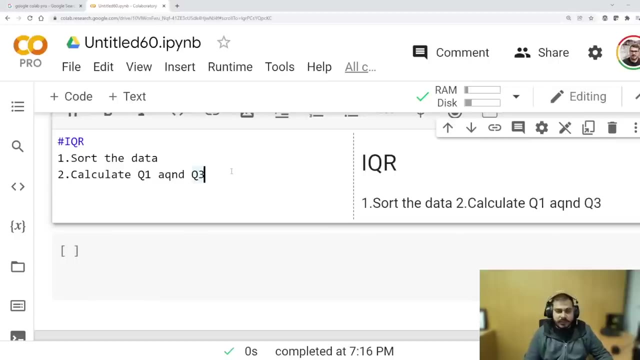 q1 and q3 is pretty much important in this particular case, so i need to do it in this scenario. i'll just move this up. i'll copy and paste it over here. so the first step is basically calculate, sort the data and then calculate q1 and q3. then we need to find out iqr, which is nothing. 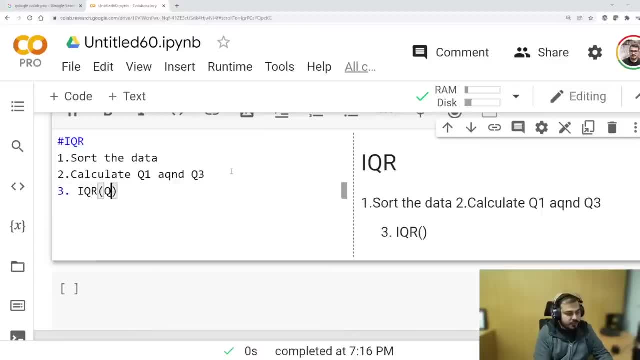 but the third step, which is nothing but the subtraction of q3 minus q1. then we need to find the lower fence, find the lower fence now, lower fence formula. i hope everybody knows it. so it is nothing but q1, q1, q1 plus or minus. it is q1 minus 1.5 multiplied by iqr. right, this is the 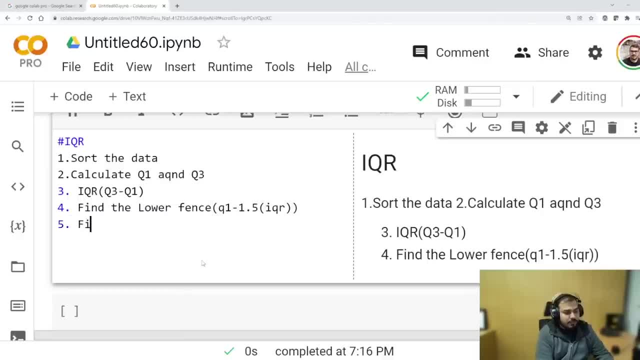 formula to basically find out the lower fence, then find the upper fence, which is nothing but q1. here i will basically be using q3 plus 1.5 multiplied by iqr. so these are the steps that we are probably going to do. so these are my steps that i am actually going to plan for and based on: 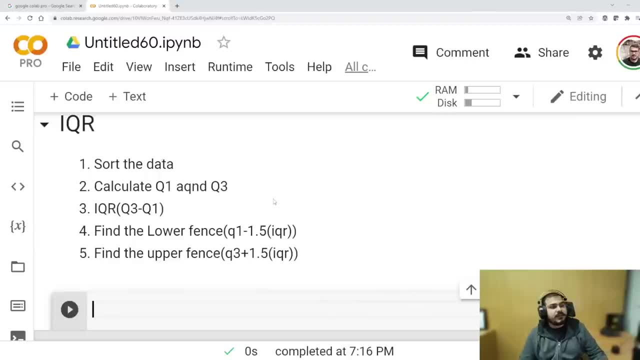 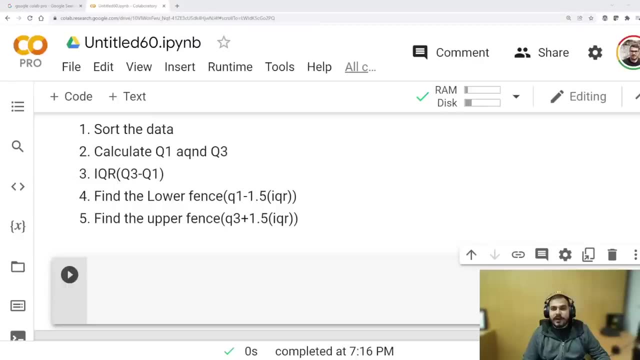 the steps i will be implementing it. so these are the steps that i will be performing in order to find the outliers with the help of iqr. now, first of all, if i really want to find out the sorted data set, how do i find out the sorted data set? so i will first of all find out the sorted data set. 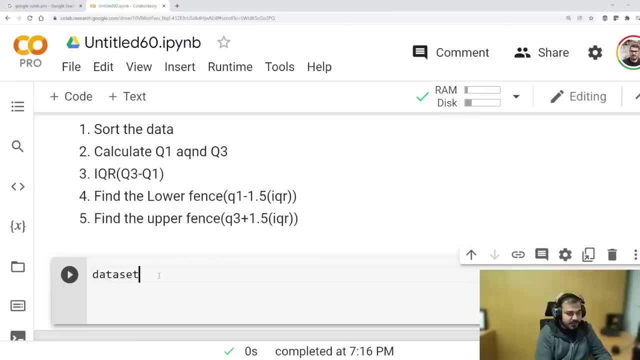 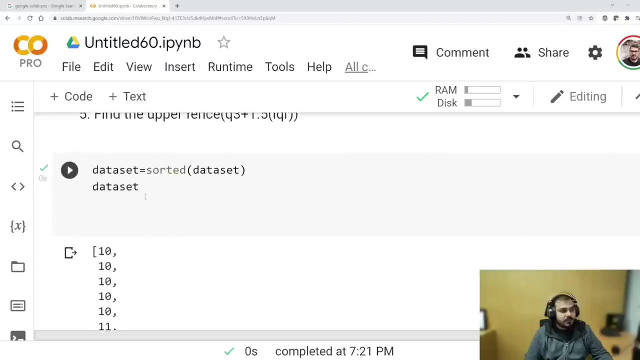 sorted data set. i will just say this will be my data set and i can use sorted function and in sorted function, if i give you the data set, this will basically be my sorted data set. so sorted is an inbuilt function which will actually help you to sort all the numbers. okay, okay, sort all. 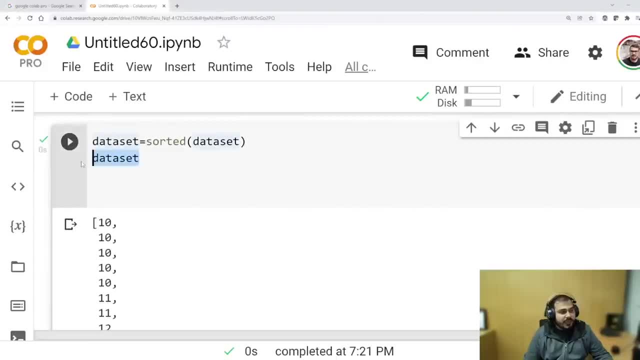 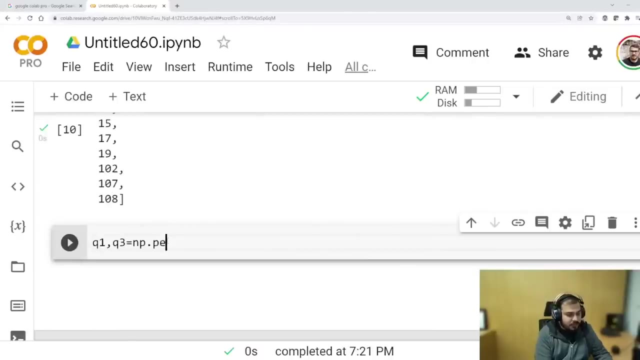 the numbers over here. so right now i have actually created a data set which is completely sorted. so my first step is done. so i am done with my first step. now, second step: i need to calculate q1 and q3. so i will say q1, comma, q3, and here i will basically use np, dot, percentile. i will give my data set over here. 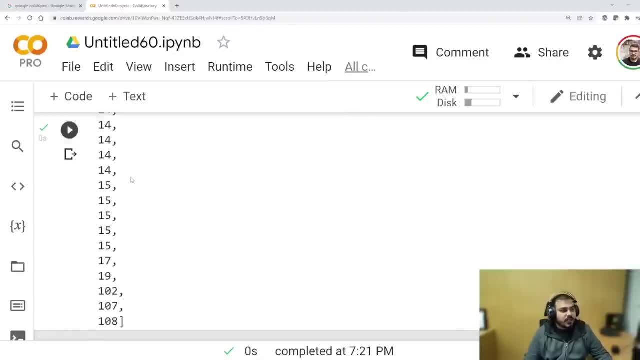 So sorted is an inbuilt function which will actually help you to sort all the numbers. Okay, Okay, Sort all the numbers over here. So right now I have actually created a data set which is completely sorted, So my first step is done. 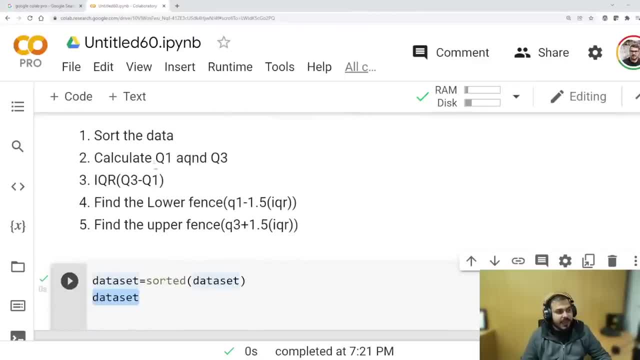 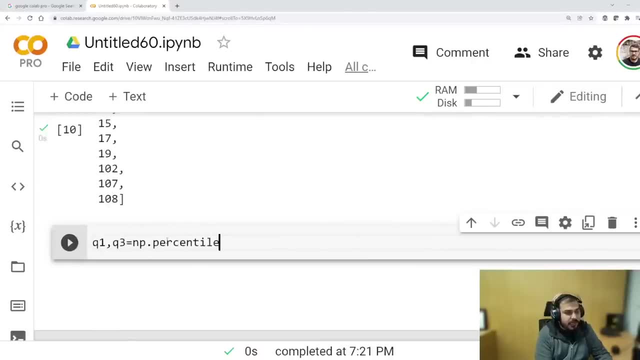 So I am done with my first step. Now, second step: I need to calculate Q1 and Q3.. So I will say Q1 comma Q3.. And here I will basically use np dot percentile. I will give my data set over here. 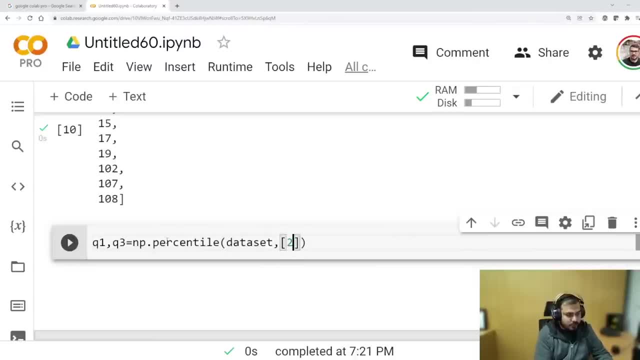 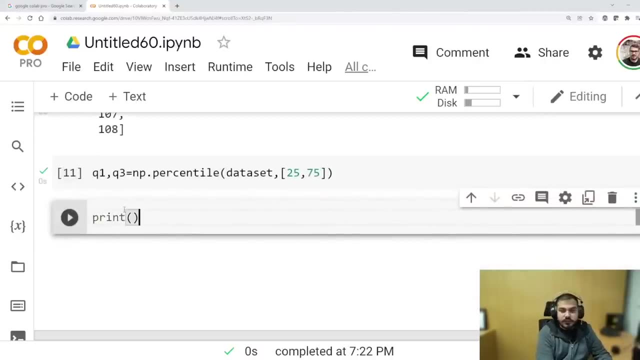 Along with this, I will give two values. One is 25 comma 75.. So once I execute it, you can see that it has got executed. Now I am going to just print Q1 comma Q3.. So here you can see which is my Q1, Q3. 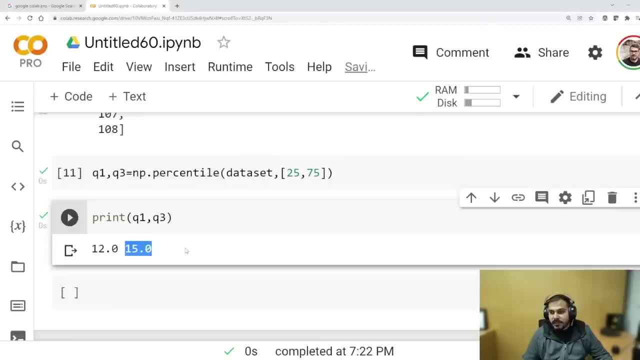 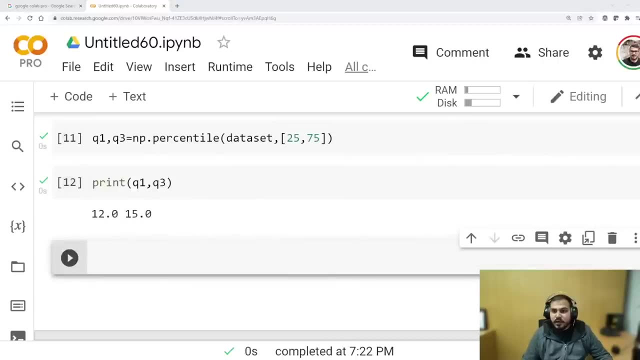 This is my 25 percentile. This is my. this is my what percentile? This is my 75 percentile Now. once we have this, now, let's go ahead and compute the lower fence and the higher fence. Now, in order to compute the lower fence and the higher fence, 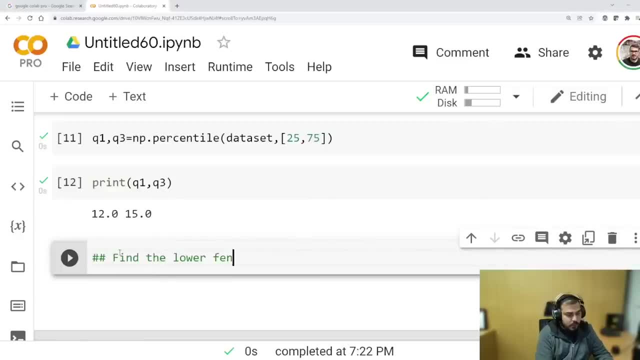 here, I am just going to write the comment. Find the lower fence and higher fence. The lower fence is equal to Q1, right Minus 1.5 multiplied by IQR. And before that I need to compute the IQR. 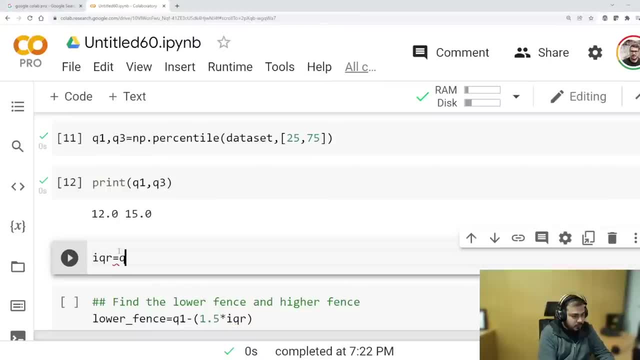 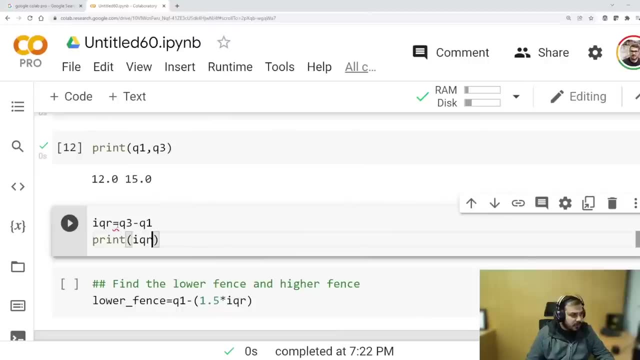 Let's say IQR is equal to Q3 minus Q1.. So if I go ahead and print IQR, What is this error that is coming here Now? if I go ahead and execute this, you will be seeing that IQR is 3.. 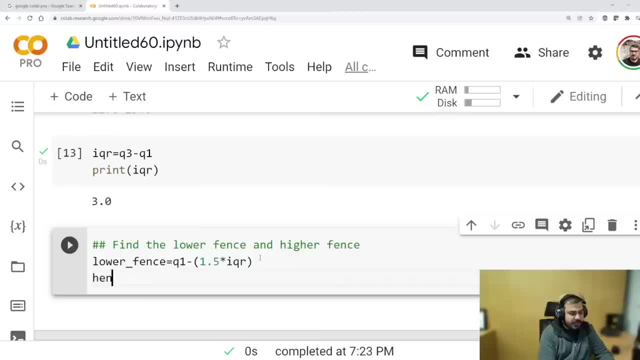 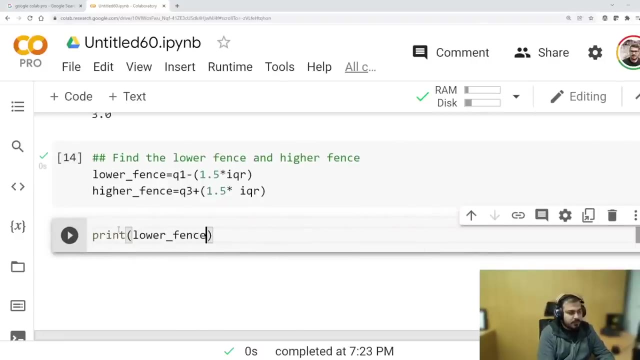 So this is my lower fence. For the higher fence I will basically write: higher fence is equal to Q3 plus 1.5 multiplied by IQR. Once I execute it now I know my lower fence and higher fence. So I am going to print: lower underscore fence. higher underscore fence. 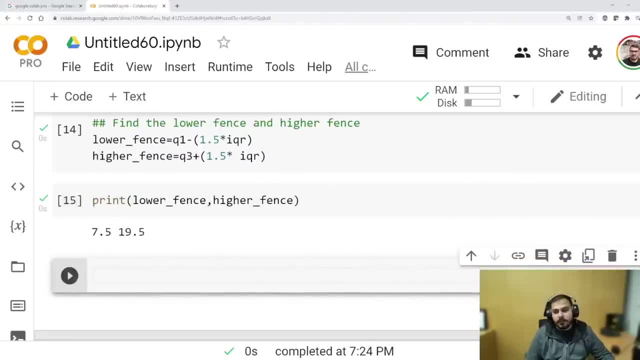 So if I print it, it is 7.5 to 19.5.. Now the further part. I think you can comfortably do it And based on this, higher, lower fence and higher fence, you can write a condition and you can remove all the elements. that is required. 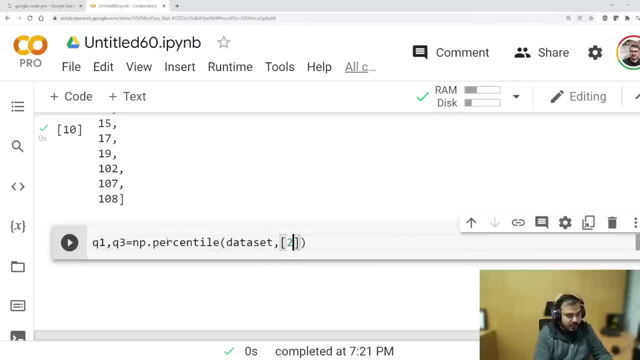 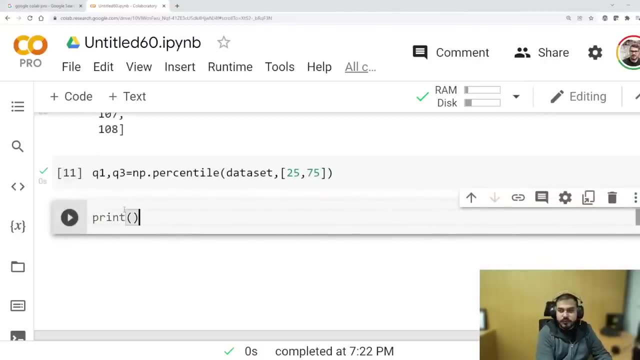 along with this i'll give two values. one is 25 comma 75, so once i execute it you can see that it has got executed. now i'm going to just print q1 comma q3. so here you can see which is my q1- q3. 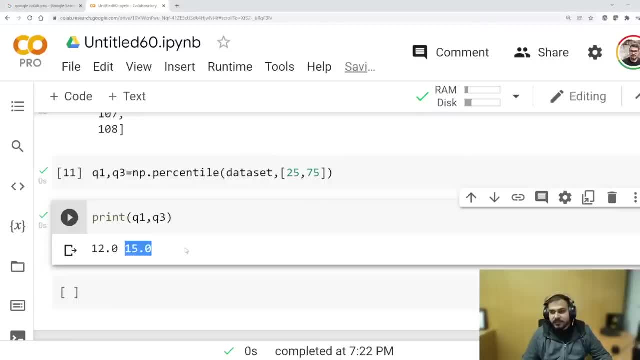 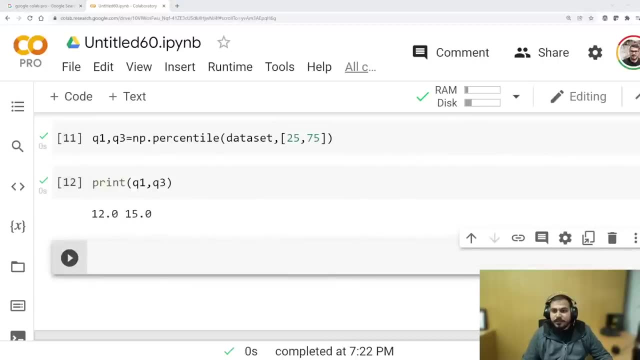 this is my 25 percentile. this is my. this is my what percentile? this is my 75 percent now. once we have this, now, let's go ahead and compute the lower fence and the higher fence. now, in order to compute the lower fence and the higher fence here, i'm just going to write the comment: find the lower fence. 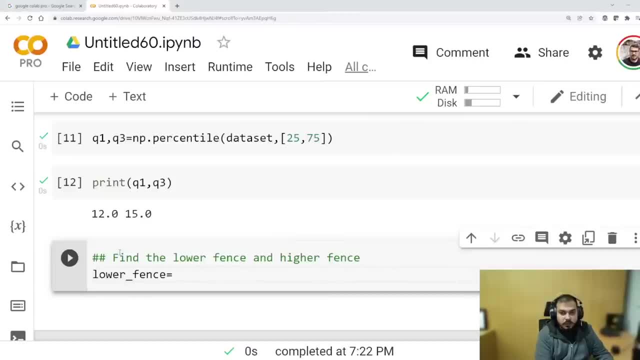 and higher fence. the lower fence is equal to q1 right minus 1.5 multiplied by iqr. and before that i need to compute the iqr. let's say iqr is equal to q3 minus q1. so if i go ahead and print iqr, what is this error? it is: 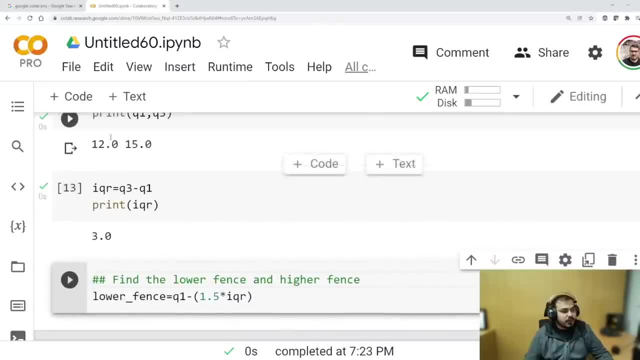 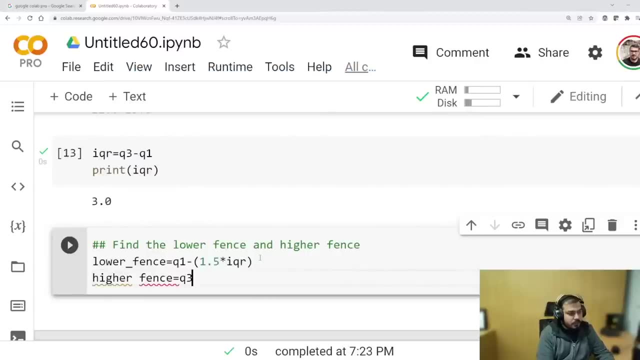 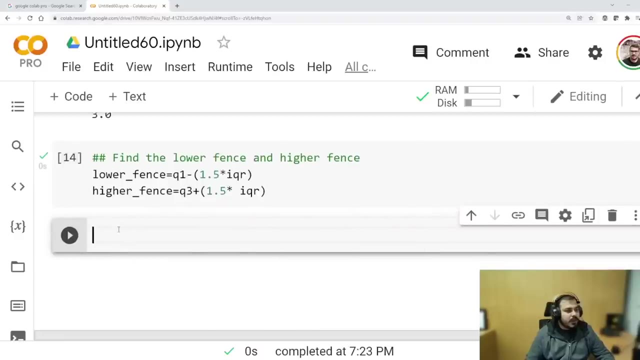 coming here now. if i go and execute this, you will be seeing that iqr is 3, so this is my lower fence. for the higher fence, i will basically write: higher fence is equal to q3 plus 1.5 multiplied by iqr. once i execute it now i know my lower fence and higher, so i'm going to. 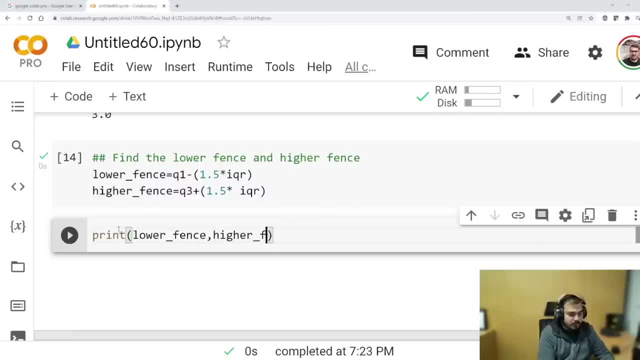 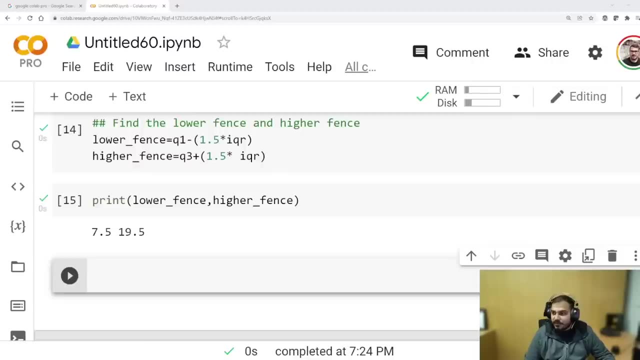 print lower underscore, fence, higher underscore. so if i print it, it is 7.5 to 19.5. now the further part. i think you can comfortably do it and based on this higher, lower fence and higher fence, you can write a condition and you can remove all the elements that is required. so now you can basically 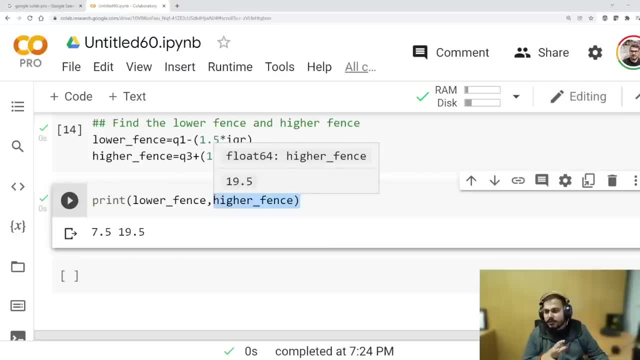 write. don't worry whether the data is normally distributed or not. here what we are doing is that whatever data set you are basically getting is going to be distributed to the higher fence. you are getting what you can actually do. you can basically uh, find the lower fence and higher fence. 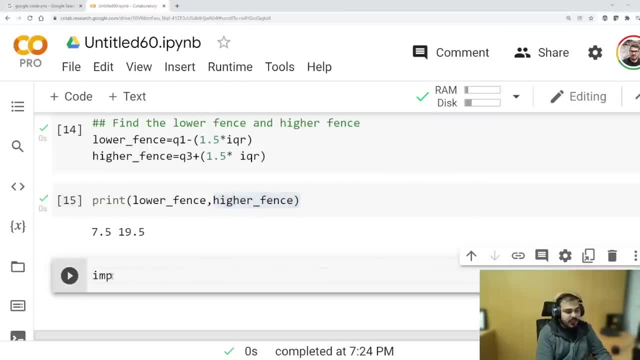 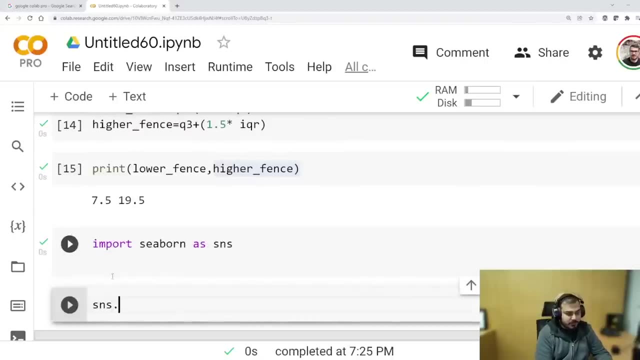 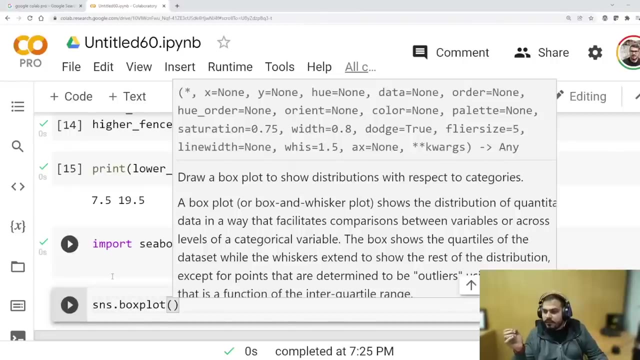 and basically do this thing now instead of doing all these things. if i import cbon as sns, okay and execute it, and there is an option which is called as hist plot, not sorry, box plot. we also saw how to create box plot. if the, if the lower fence is negative, then what you can do is that. 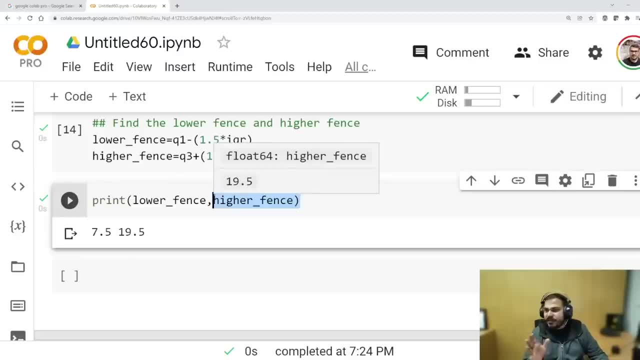 So now you can basically write: Don't worry whether the data is normally distributed or not. Here what we are doing is that, whatever dataset, you are basically getting what you can actually do. you can basically find the lower fence and higher fence and basically do this thing. 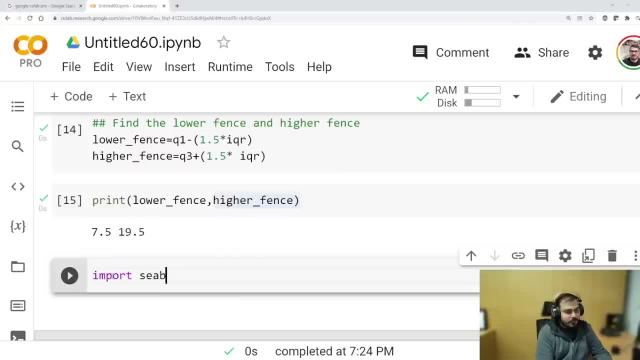 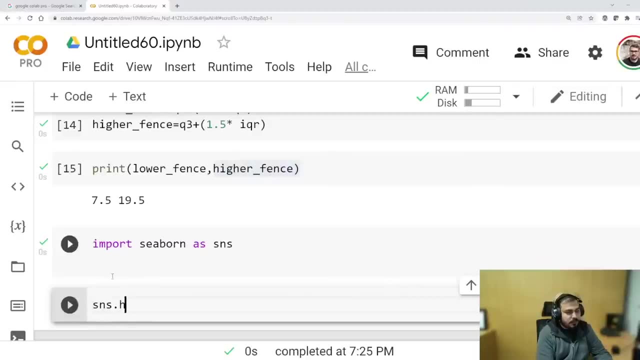 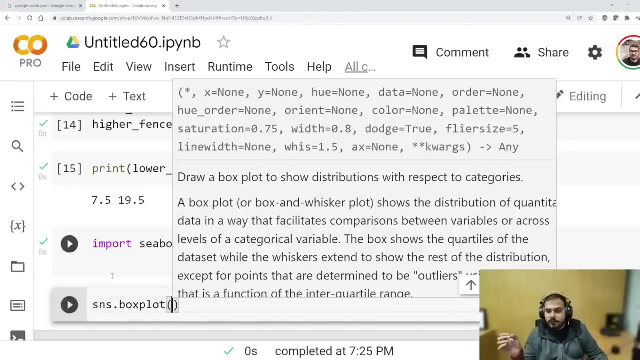 Now, instead of doing all these things, if I import CBON as SNS and execute it and there is an option which is called as boxplot- We also saw how to create boxplot- If the lower fence is negative, then what you can do is that. 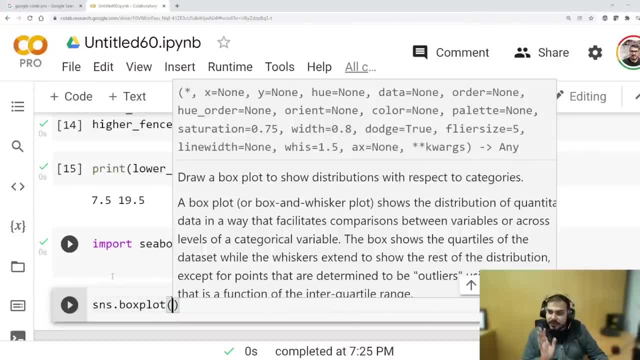 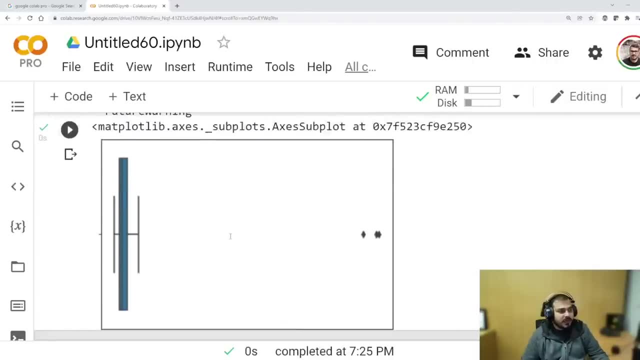 based on that condition, any value lesser than that, you can remove all those things. right. And here, if I give my dataset, you will be able to see that. this will be how a boxplot will be created. Now this looks. you see, that there is a very big outlier. 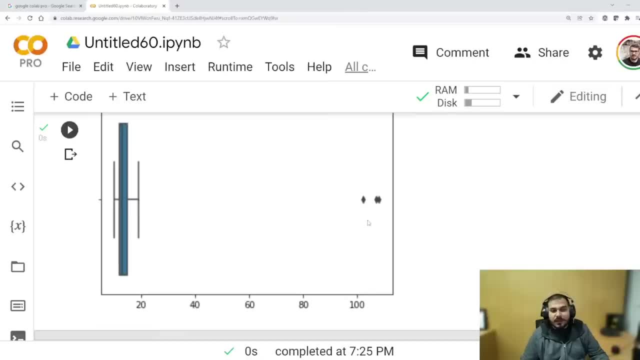 So that is the reason, This same outlier. we found out with the help of multiple things, And here also you can see 7.5 to 19.5.. So most of the data points that will be lying over here will be based on that. 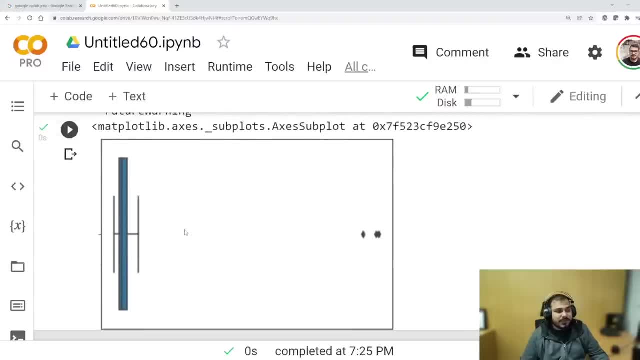 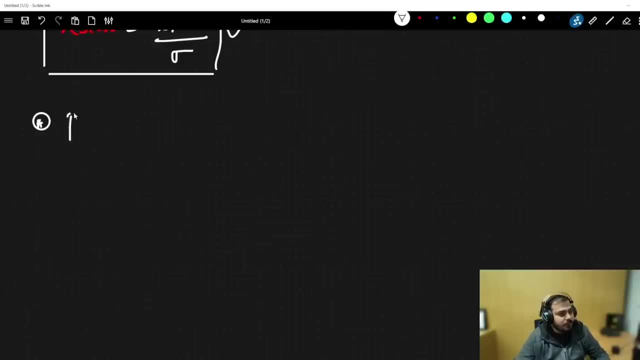 If I probably remove those three elements and try to see that particular dataset, then this boxplot will look bigger. Now let's go ahead and discuss about the next topic, which is called as probability. Probability is super, super important And in this session I will discuss major, major, important things in probability. 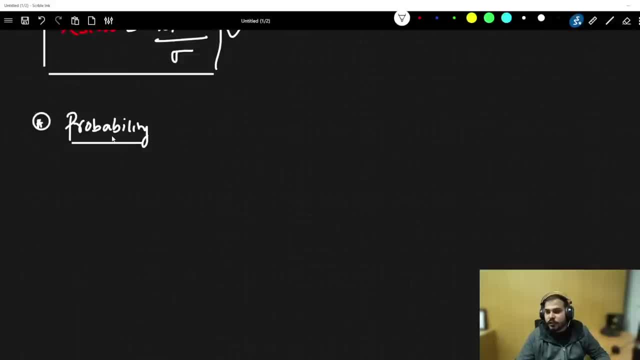 And we will try to see that what all things we can actually do with the help of probability. Probability is by default used in machine learning also, in deep learning, also many places. Let's say one example. okay, Suppose I have two categories of dataset. 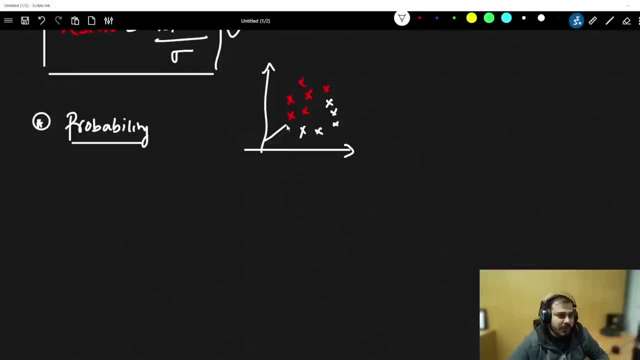 I have another category of dataset. If I try to create a best fit line, you can see that. let's say that this belongs to class A, this belongs to class B. Now, over here, you will be able to see that if I talk about this right when I draw this linear line. 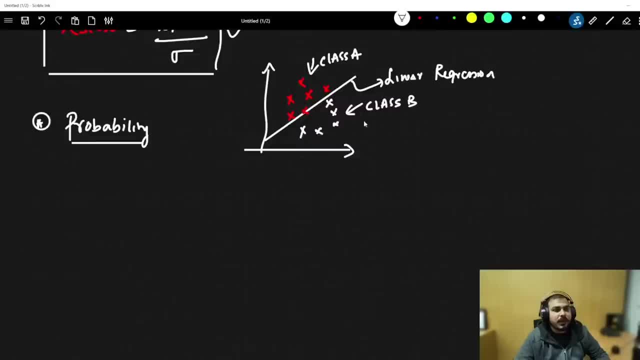 this is basically used in linear regression. let's say Now my question is that what probability of this particular point belongs to class A and what probability of this particular point belongs to class B Because it is passing through the line. So, based on probability, we can definitely get a lot of things. 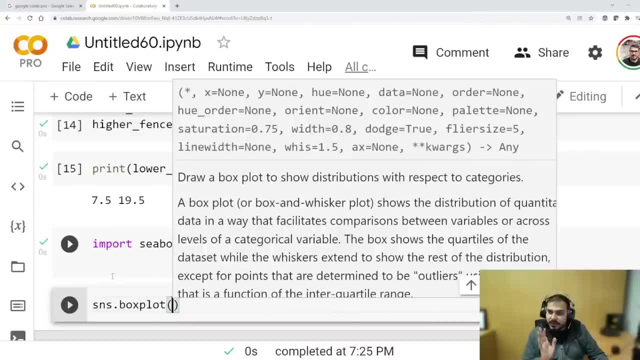 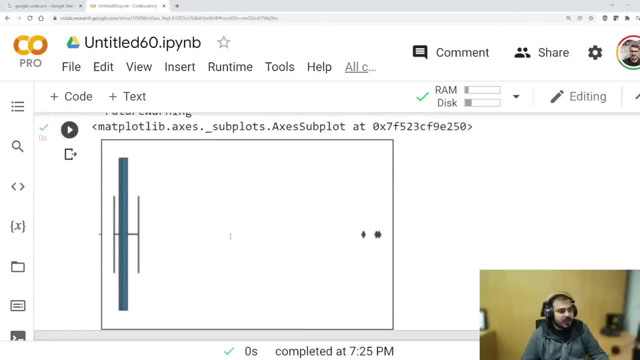 based on that condition. any value lesser than that, you can write a condition and you can remove all those things. right, and here, if i give my data set, you will be able to see that this will be how a box plot will be created. now this looks, you see, that there is a very big outlier, so that 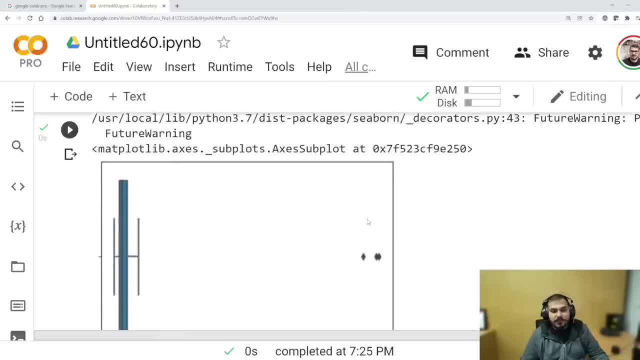 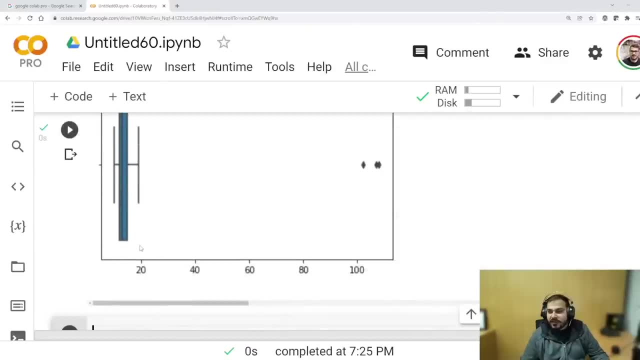 is the reason, this same outlier. we found out with the help of multiple things, and here also you can see 7.5 to 19.5. so most of your data points that will be lying over here will be based on that. if i probably remove those three elements and try to see that particular data set, then this box plot: 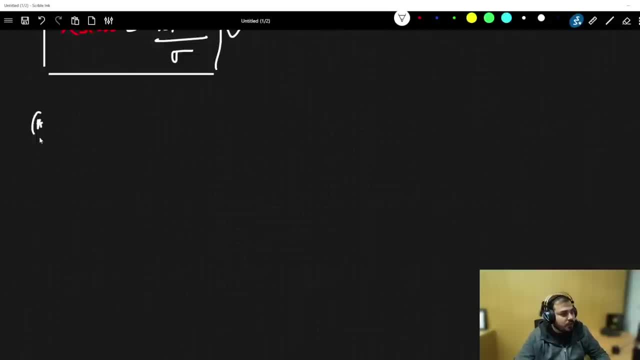 will look bigger. now let's go ahead and discuss about the next topic, which is called as probability. probability is super, super important and in this session i will discuss major, major important things in probability and we will try to see that what all things we can actually do with the help of probability. probability is, by default, used in machine. 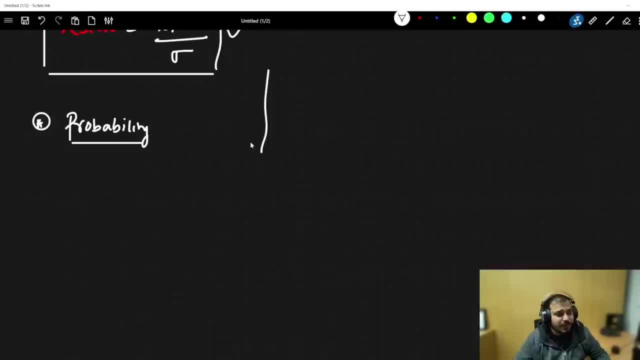 learning, also in deep learning, also many places. let's say one example. okay, suppose i have two categories of data set. i have another category of data set. if i try to create a best fit line, you can see that this is the best fit line and this is the best fit line and this is the best fit line. 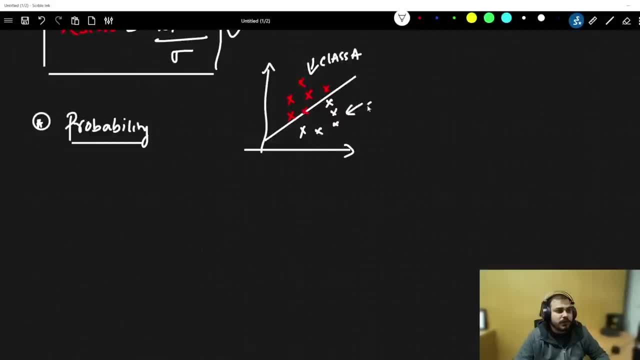 let's say that this belongs to class a, this belongs to class b. now, over here you will be able to see that if i talk about this right when i draw this linear line, this is basically used in linear regression. let's say now. my question is that: what probability of this particular point belongs to? 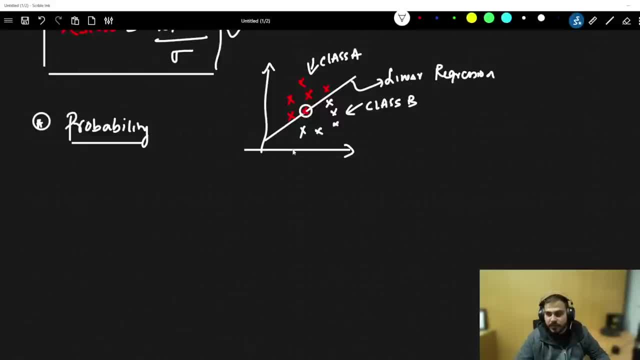 class a and what probability of this particular point belongs to class b because it is passing through the line. so based on probability, we can definitely get a lot of things in linear regression. it is used in, logistically it is used and all. so probability really focuses, uh, like base is basically used over there and different, different. 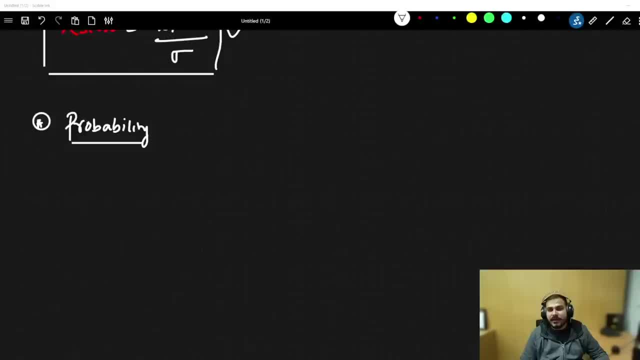 things are used. let's understand what exactly is probability. if you want to give a definition, what exactly is a probability? so here you can say that probability is a measure of the likelihood of an event. probability is a measure of the likelihood of an event, the reason why i am. 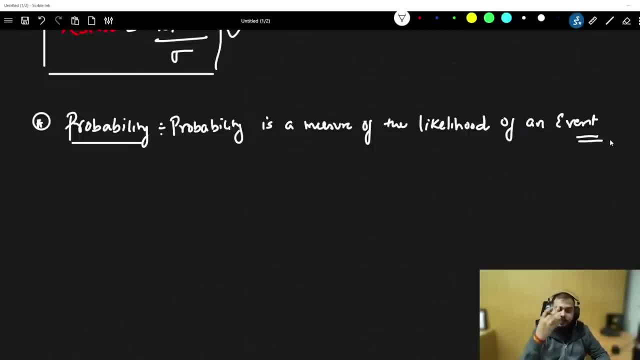 writing you this all definitions. guys, understand, you really need to think. you know what exactly is happening over here. what is the definition? you know if you can remember those definition in an easy way by example. so that is the reason i also give you a lot of examples. let's say that 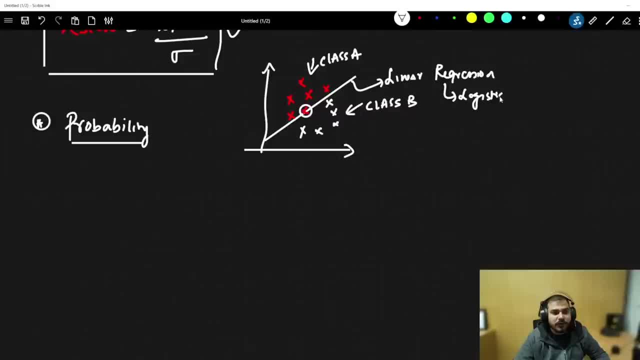 In linear regression, it is used in logistic, it is used and all. So probability really focuses like base is basically used over there And different, different things are used. Let's understand what exactly is probability. If you want to give a definition, what exactly is a probability? 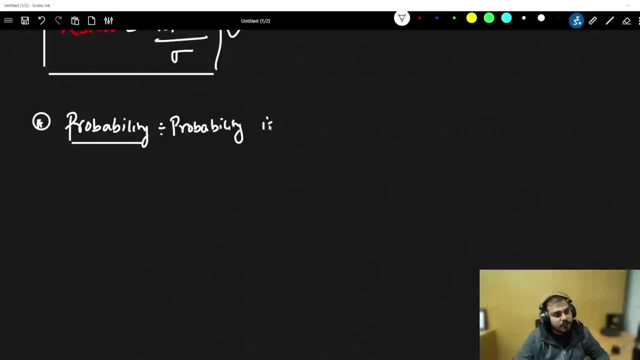 So here you can say that probability is a measure of the likelihood of an event. Probability is a measure of the likelihood of an event, The reason why I am writing you this whole definition, guys, understand. you really need to think. you know what exactly is happening over here. what is the definition? 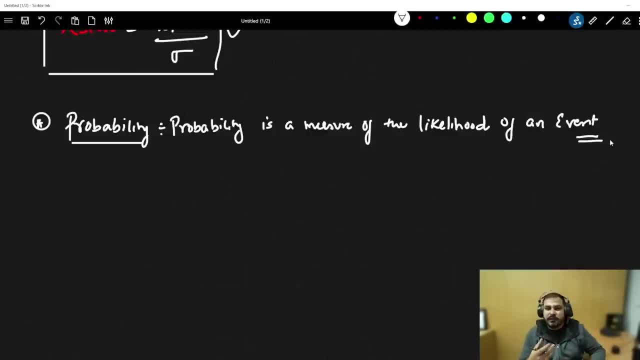 You know, if you can remember those definitions in an easy way by example. So that is the reason I also give you a lot of examples. Let's say that I am flipping a dais In a dais. what are my possible sample events? 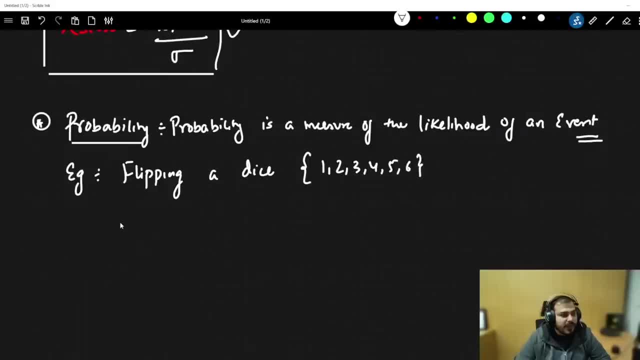 You know that it is 1,, 2,, 3,, 4,, 5, 6.. Now, if I ask you a question, what is the probability when I roll a dais? sorry, roll a dais, not flip. 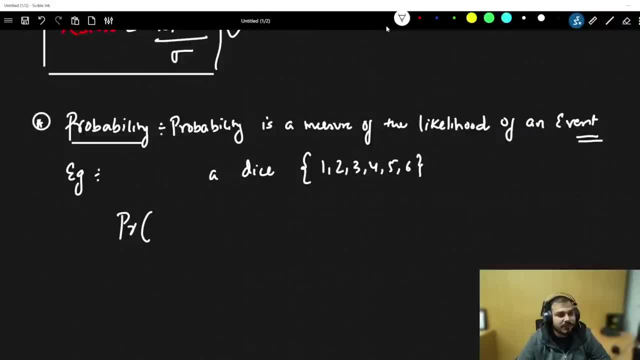 Flipping a coin. it should be. I will say roll a dais. So here I am basically saying roll a dais. So what is the probability of getting 6?? If this is my question, then how probability you will be able to calculate. 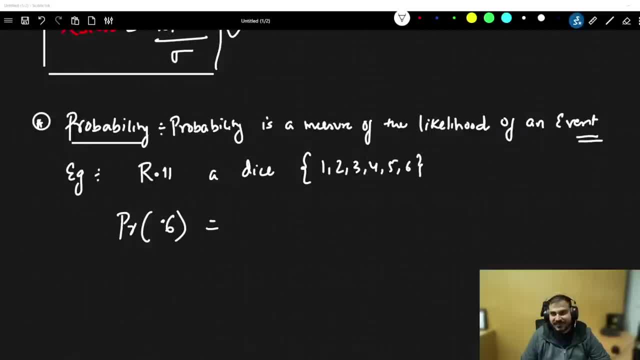 What is the answer? Obviously, you will say 1 by 6, right, It is very simple. So how do we define probability? I will say that number of ways an event can occur divided by number of possible outcomes. So this is the exact definition of this. 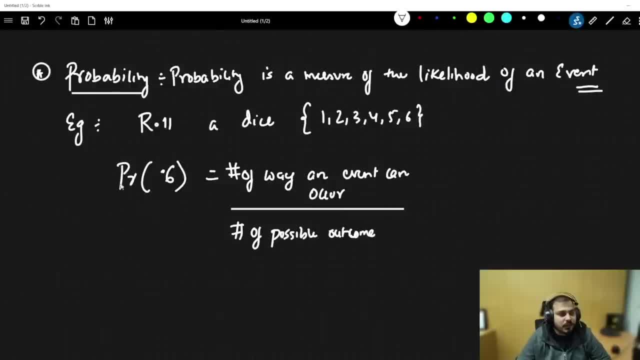 Now, in this particular scenario, number of ways an event can occur. Over here I am trying to find out what is the probability. when I roll a dais, I get a 6.. So how many events can occur? It can only occur as 1.. 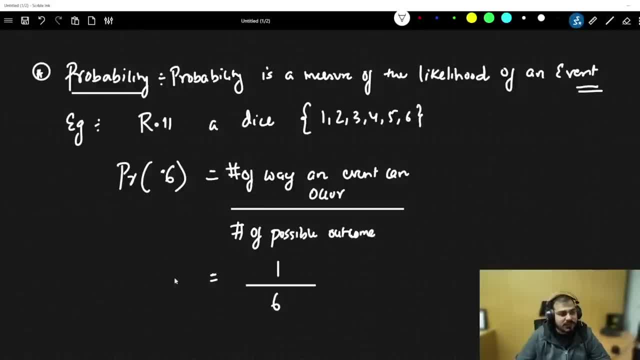 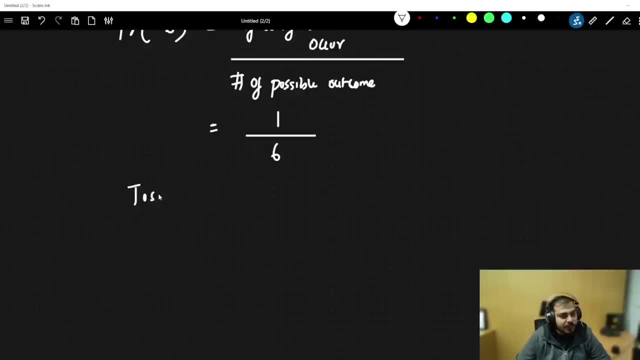 And what is the number of total possible outcomes? It is 6.. So this is how we basically find out. Similarly, if I give one more example, Let's say that I want to toss a coin, Obviously I know what are my sample space, head and tail. 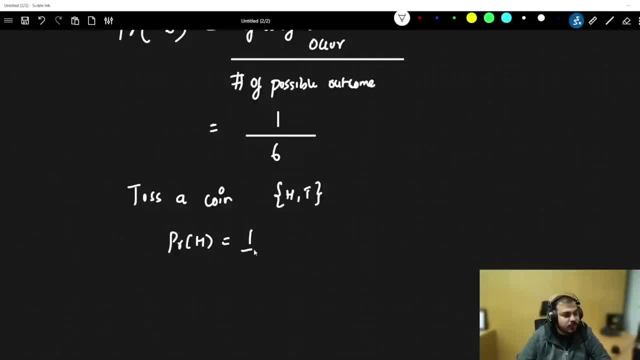 What is the probability of getting head? You will just say that 1 by 2.. Because the sample space is 2 and one number of events that can occur is 1 by 2.. So you basically say this as probability of head, as 1 by 2.. 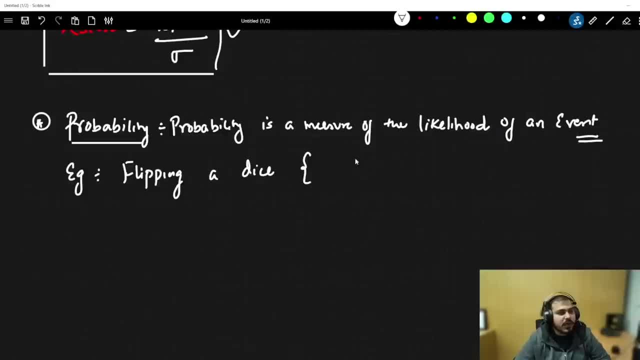 i am flipping a dice in the dice. what are my possible sample events? you know that it is one, two, three, four, five, six. now if i ask you question, what is the probability when i roll a dice? or sorry, roll a dice, not flip flipping a coin, it should be. i'll say a roll a dice, okay. 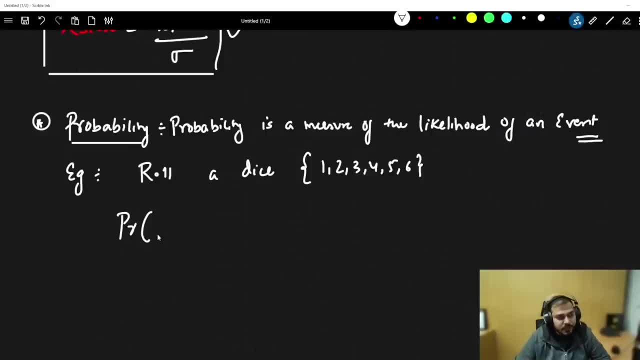 Okay, so here I am basically saying: roll a die. So what is the probability of getting 6?? If this is my question, then how probability you will be able to calculate? What is the answer? Obviously, you will say 1 by 6, right? 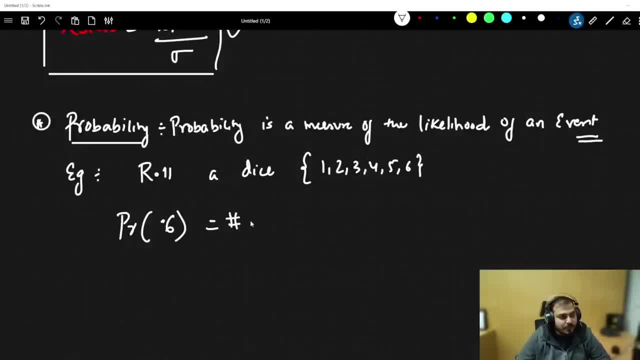 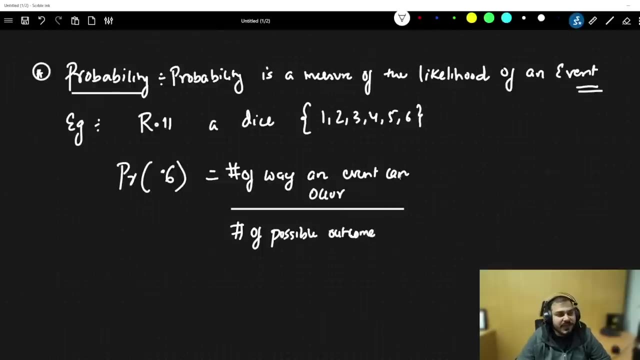 It's very simple. So how do we define probability? I'll say that number of ways, number of ways an event can occur, an event can occur, divided by number of possible outcomes. So this is the exact definition of this. Now, in this particular scenario, number of ways an event can occur. 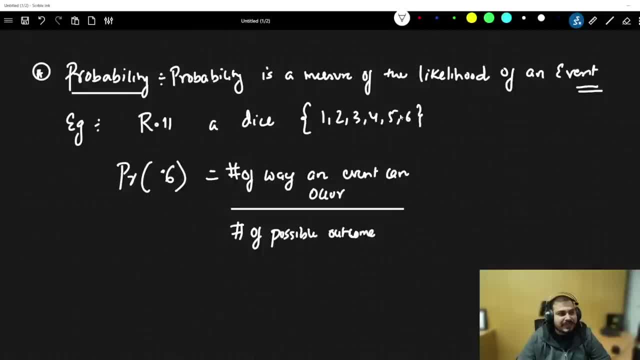 Over here I am trying to find out what is the probability. when I roll a dice, I get a 6.. So how many events can occur? It can only occur as 1.. And what is the number of total possible outcomes? It is 6.. 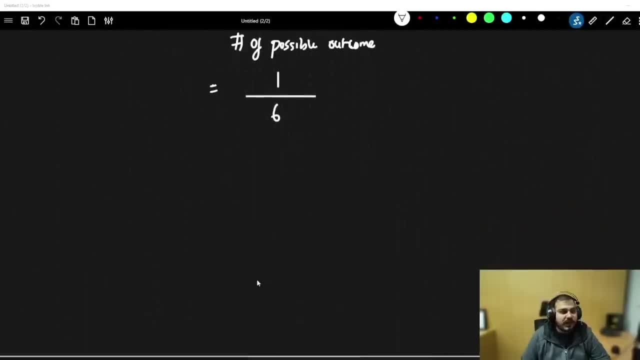 So this is how we basically find out. Similarly, if I give one more example, let's say that I want to toss a coin, Obviously I know what are my sample space: head and tail. What is the probability of getting head? 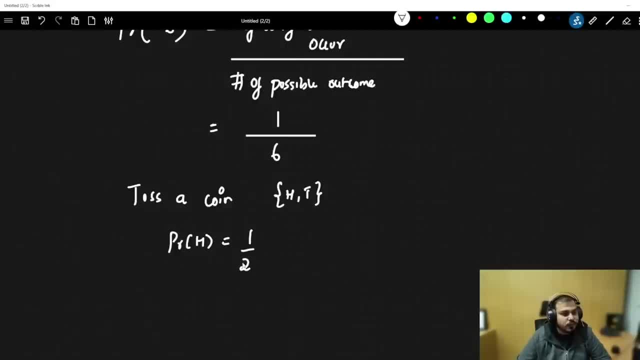 You'll just say that: 1. Because the sample space is 2 and one number of events that can occur is 1 by 2.. So you basically say this as probability of head as 1 by 2.. Now let's go one step above probability, which is called an addition rule. 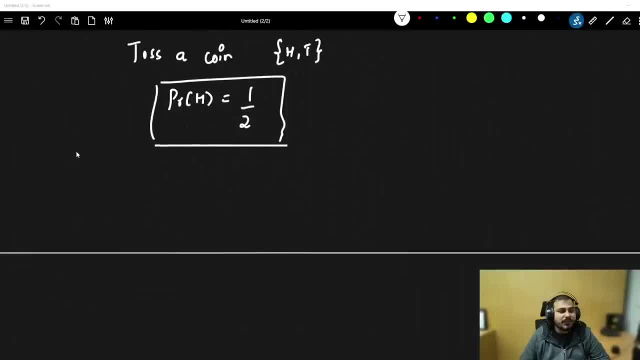 Now here is where you will probably discuss about something called as. So let's go to the next topic Over here. I'm basically going to define as addition rule. This is super important. Probably in your aptitudes You will be using the addition rule, or we also say it as probability, or or, or, or also you say it as like this, or. 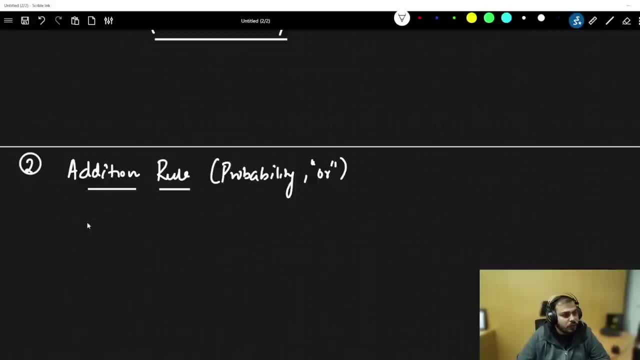 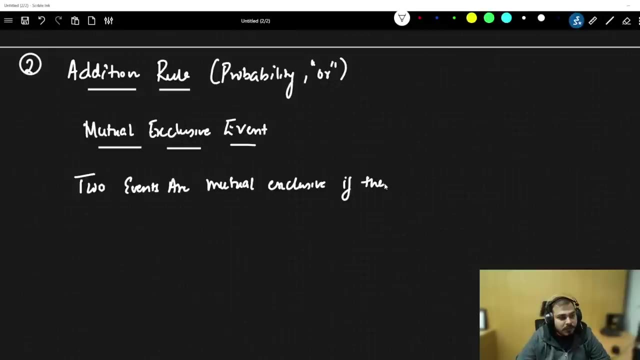 Now, in order to understand additional rule, you need to understand about two things. One is mutual exclusive event. What is this mutual exclusive events? So I can basically define: two events are mutual exclusive. Two events are actually mutual exclusive. They cannot occur at the same. 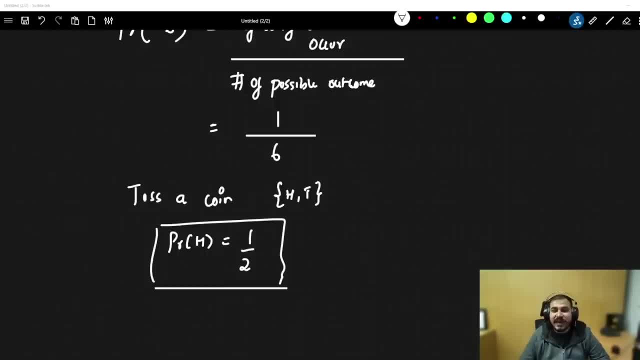 Now let's go one step above probability, which is called as addition rule. Now here is where you will probably discuss about something called as addition rule, So let's go to the next topic Over here. I am basically going to define as addition rule. 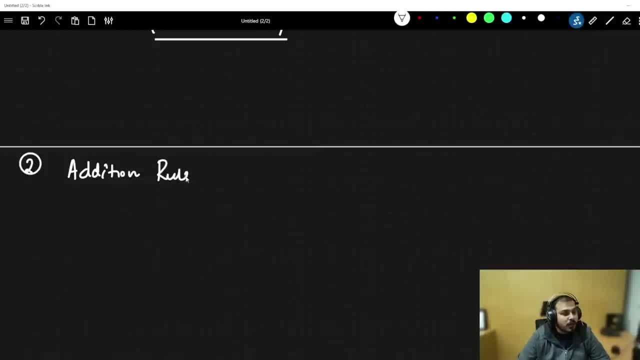 This is super important. Probably, in your aptitudes, you will be using addition rule- Or- we also say it as probability, or or, Or also you say it as like this or Now. in order to understand additional rule, you need to understand about two things. 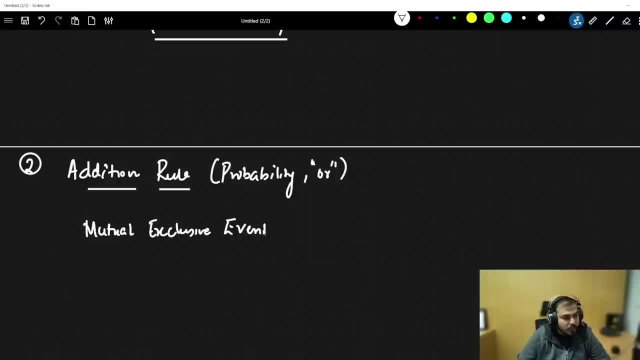 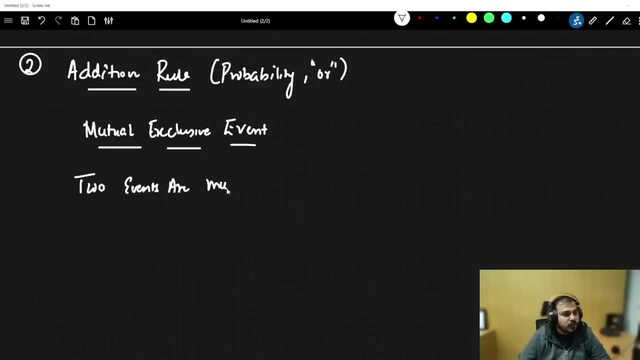 One is mutual exclusive event. What is this mutual exclusive event? So I can basically define: two events are mutual exclusive. Two events are actually mutual exclusive. They cannot occur at the same time. If they cannot occur at the same time, Let's see an example. 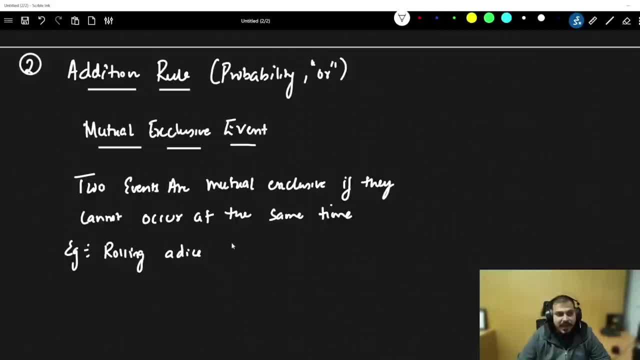 Rolling a dice. Now, when I roll a dice at a specific time, I can either get 1, or I can either get 2, or I can either get 3 or I can either get 4 or I can either get 5 or 6.. 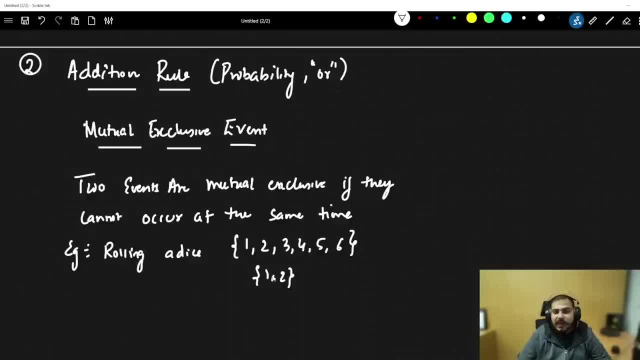 Right, So you can get 1 and 2 at the same time, Or you can't get 1, 2, 3, 4 at the same time. You will only get at one, probably one experiment or one event that you are probably rolling a dice at a single time. 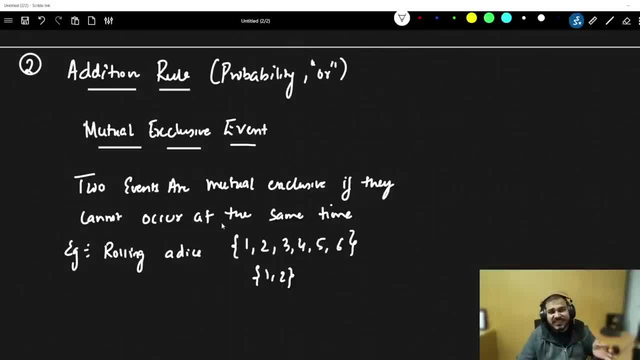 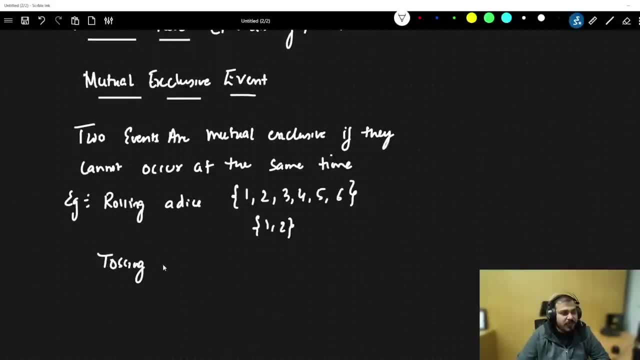 You will only be able to get one number, You will not be able to get two numbers. So this is specifically an example of mutual exclusive. Another example again: tossing a coin. In this particular case also tossing a coin In this particular case also what happens. 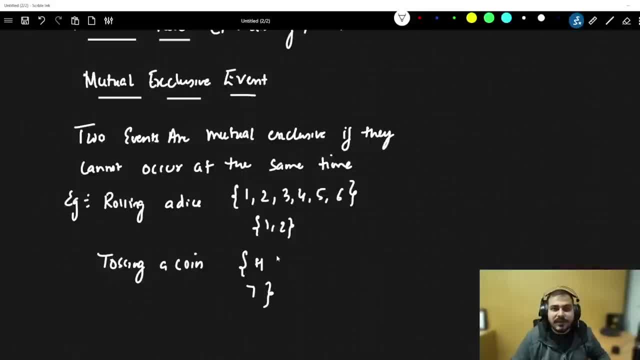 You may either get head or tail. You cannot get both, Unless and until your coin is standing, like shown in the movies. I hope. Which movie am I talking about? Which movies probably I am talking about. You can also consider, you know, good movies like Sholay. 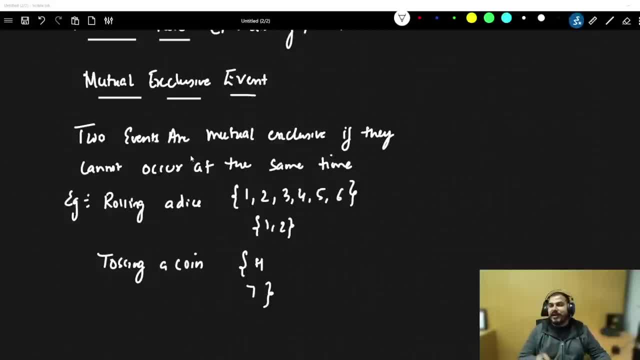 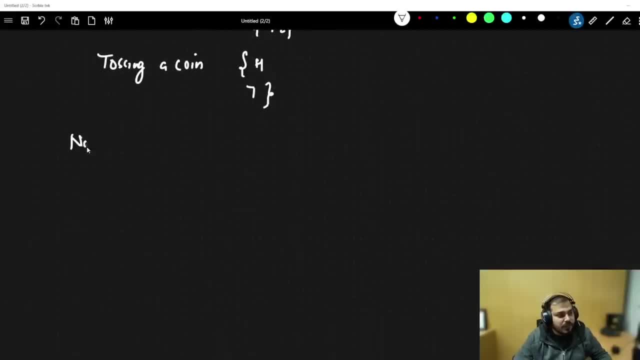 In Sholay, only one type of event occurs at every time, Right. So for this kind of problem scenarios, Now let's discuss. Let's discuss about non-mutual exclusive. Obviously, you understood that. what is mutual exclusive? Now, with respect to non-mutual exclusive? 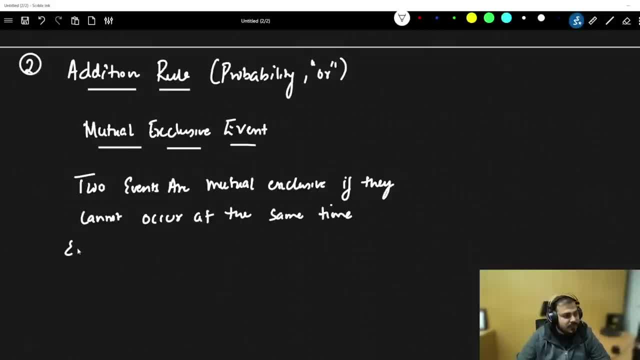 Time if they cannot occur at the same time. let's see an example: rolling a dice. Now, when I roll a dice at a specific time, I can either get one, or I can either get two, or I can either get three, or I can either get four or I can either get five or six. right, 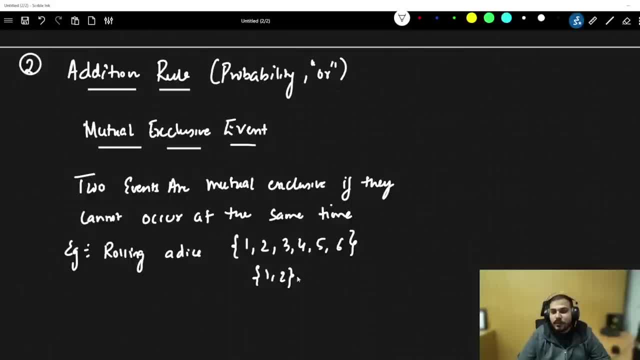 You cannot get one and two at the same time, or you can't get one, two, three, four at the same time. You will only get at one one, probably one experiment or one event that you're probably rolling a dice at a single time. 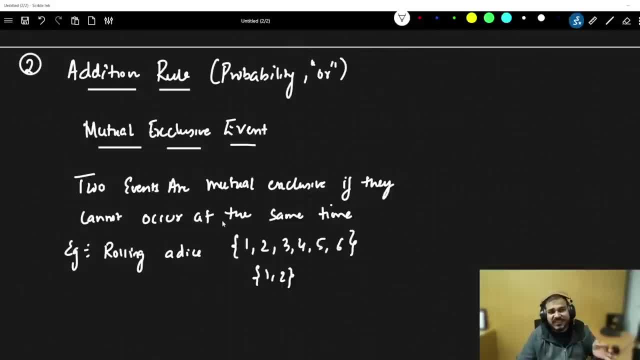 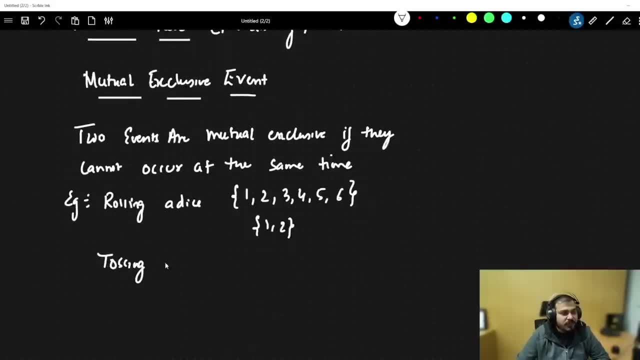 You'll only be To get one number. you will not be able to get two numbers. so this is specifically an example of mutual exclusive. another example again: tossing a coin. in this particular case also tossing a coin, in this particular case, also. what happens? you may either get head or tail. you cannot get both unless and until your coin is standing there, like shown in the movies. I hope. which movie am I talking about? which movies probably I'm talking about? you can also consider, you know, good movies like sholey, and surely only one day, 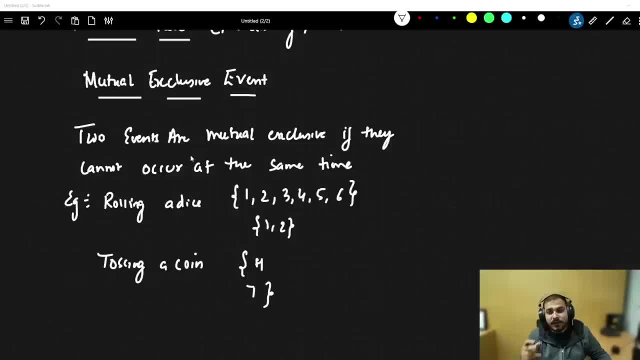 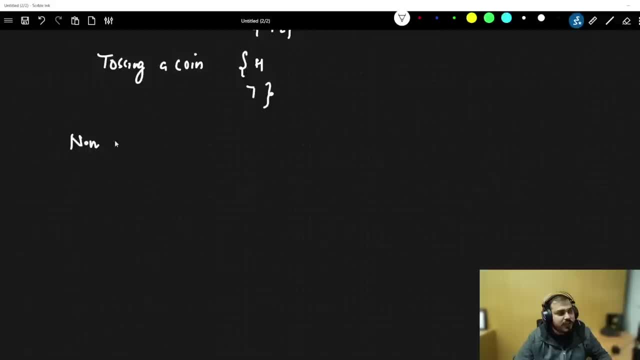 One type of event occurs at every time, right? So for this kind of problem scenarios, now let's, let's discuss, let's discuss on non-mutual exclusive. Obviously, you understood that what is mutual exclusive? now, with respect to non-mutual exclusive, obviously both the events can occur at the same time, multiple events can occur at the same time here. 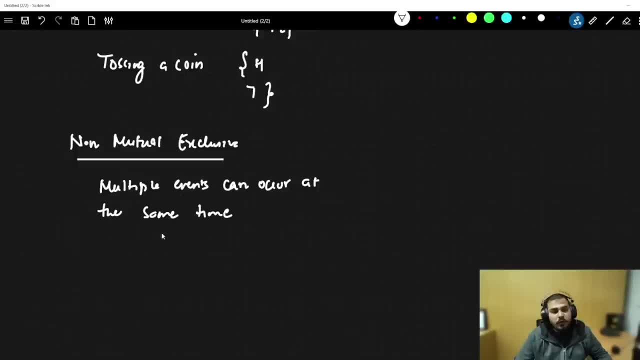 I'll say that multiple events that can occur at the same time, two or more events can occur at the same time. Let's let's say one example. Let's take a deck of cards, a very simple example with respect to this: in deck of cards, 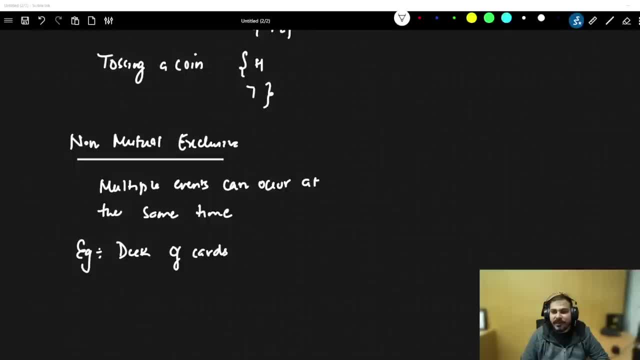 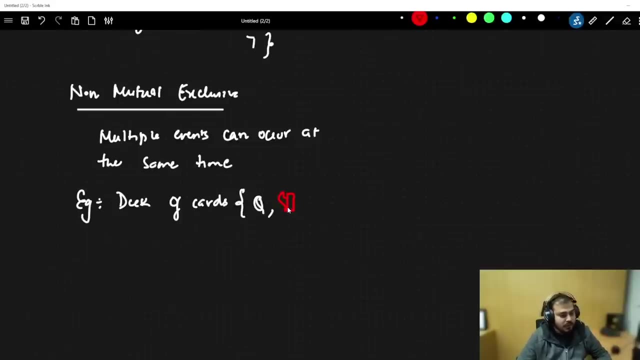 Have you seen, like what will happen in a deck of cards, Two events. Let's consider that from a deck of cards, when I pull out a card, a king can also come. or or let's say that a queen card can come. along with this queen card, a red colored heart card can also come. heart card can also come right. 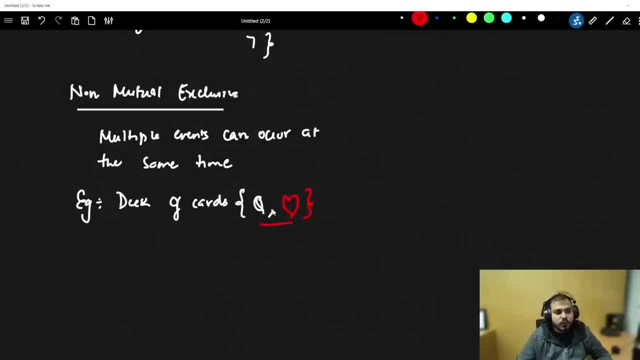 So here multiple events are there. So these two cards are obviously not mutual exclusive. So here you can see that, okay, I can also pick up a king. It can be in black color. It can also be in yellow, Right. It can also be in red color, right. 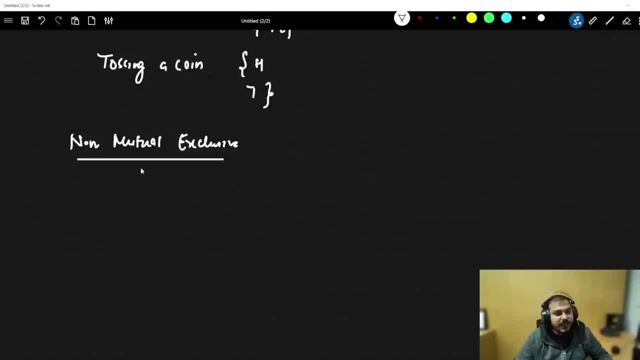 Obviously, both the events can occur at the same time. Multiple events can occur at the same time. Here I will say that multiple events can occur at the same time. Two or more events can occur at the same time. Let's say one example. 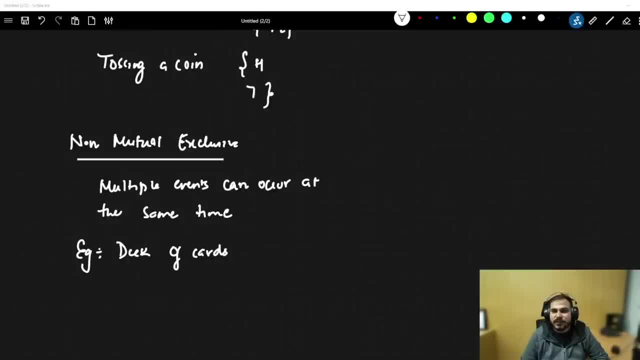 Let's take a deck of cards. A very simple example with respect to this In deck of cards. have you seen like what will happen in a deck of cards? Two events. Let's consider that from a deck of cards. when I pull out a card, 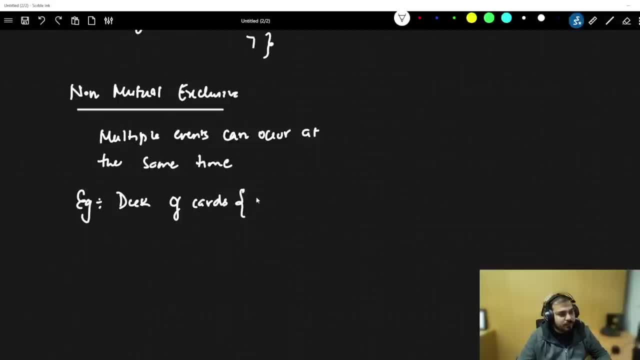 A king can also come. Or let's say that a queen card can come Along with this queen card. A red color heart card can also come, Heart card can also come Right. So here multiple events are there. So these two cards are obviously not mutual exclusive. 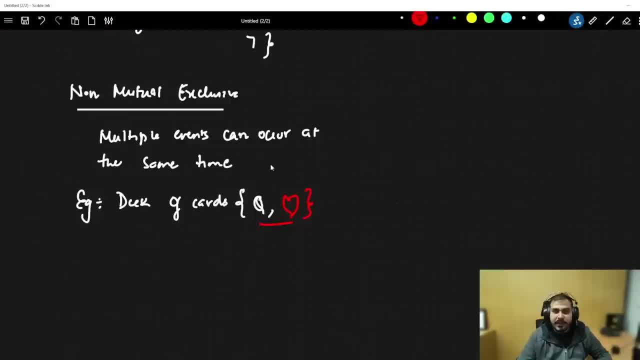 So here you can see that I can also pick up a king. It can be in black color, It can also be in red color. Right, Multiple things are basically happening. So this is an perfect example of a non-mutual exclusive. 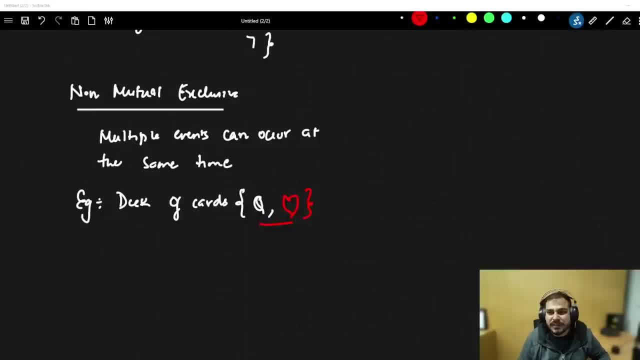 Now, based on this, there is some amazing problem statements that you can basically solve Mutual exclusive Suppose if I toss a coin. So my first question is: If I toss a coin, Which is again a mutual exclusive event, What is the probability of the coin landing on heads or tails? 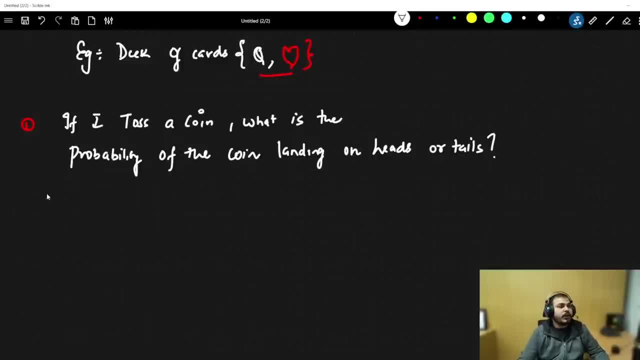 Now, whenever you get this kind of problem statement, First of all you really need to think that, Okay, whether it is mutual exclusive or not. Yes, obviously it is mutual exclusive. Now I need to find out what is the probability of getting heads or tails. 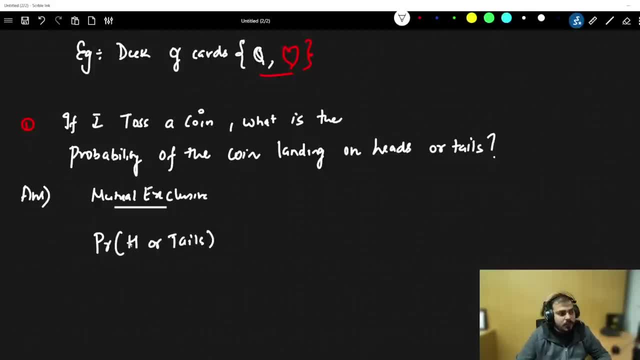 Right. This is what I need to find out. I need to find out, I need to find out what is the probability of getting heads or tails Right From this specific event. So I want to define a common definition, probably for this. 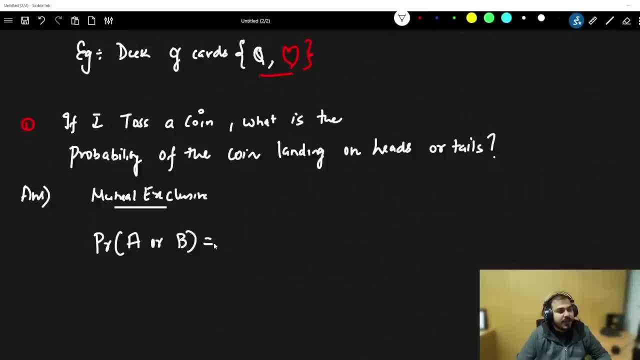 We can write: probability of A or B, Where A and B are events, Is equal to probability of A plus probability of B. So whenever you have a mutual exclusive event, At that point of time you can define this specific definition, Which is also called as additional rule. 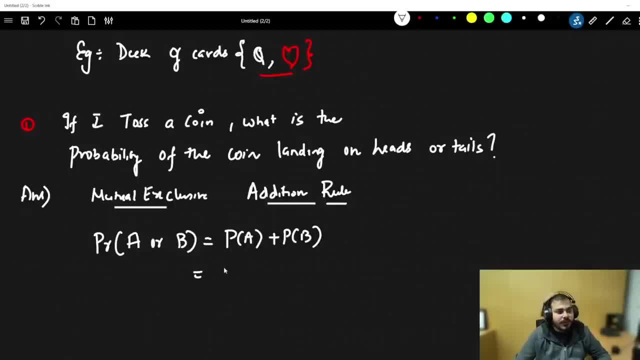 For mutual exclusive. Now here, What is probability of A? You know that it is 1 by 2 plus 1 by 2.. So the answer will be 1.. So probability of A or B to come is basically 1.. 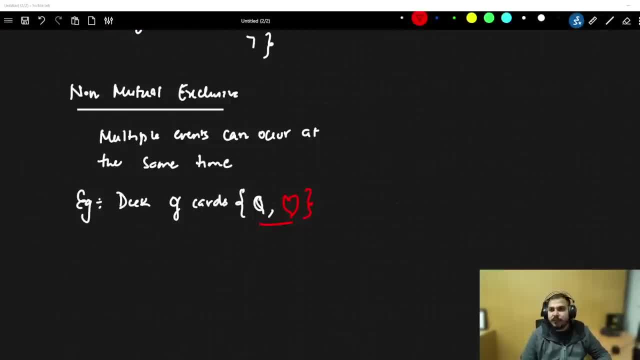 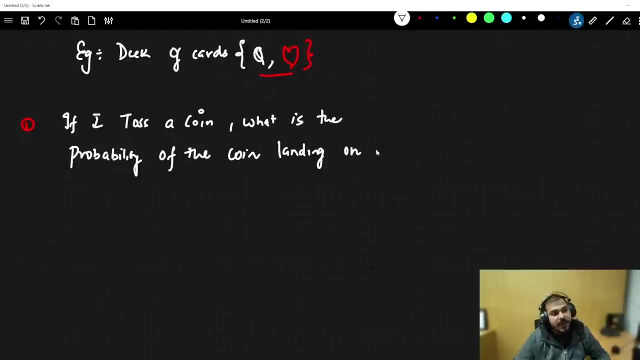 Multiple things are basically happening. So this is an perfect example of a non-mutual exclusive. Now, based on this, there is some amazing problem statements that you can basically solve. Mutual exclusive, Suppose, if I toss a coin. So my first question is: if I toss a coin, which is again a mutual exclusive event, what is the probability of the coin landing on heads or tails? 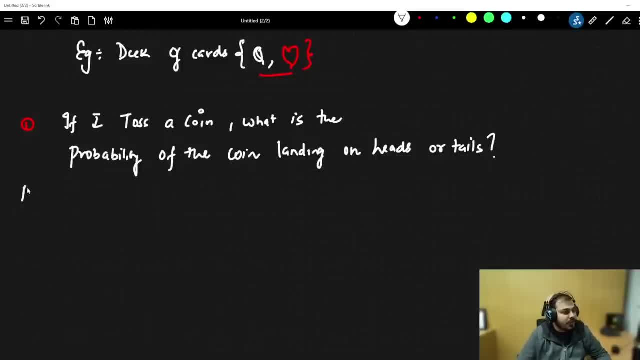 Now, whenever you get this kind of problem statement, First of all you really need to think that, okay, whether it is mutual exclusive or not. Yes, Obviously it is mutual exclusive. Now I need to find out what is the probability of getting heads or tails. 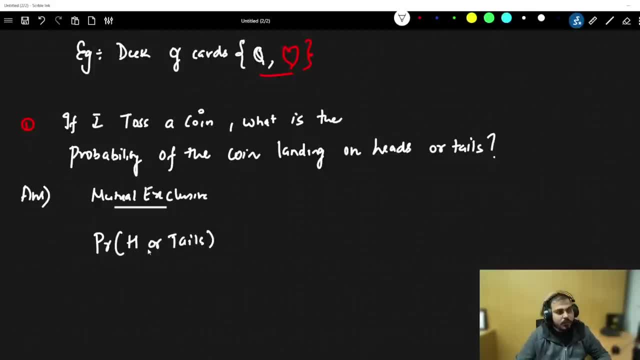 This is what I need to find out. I need to find out what is the probability of getting heads or tails from this specific event. So I want to define a common definition. probably for this We can write: probability of A or B, where A and B are events, is equal to probability. 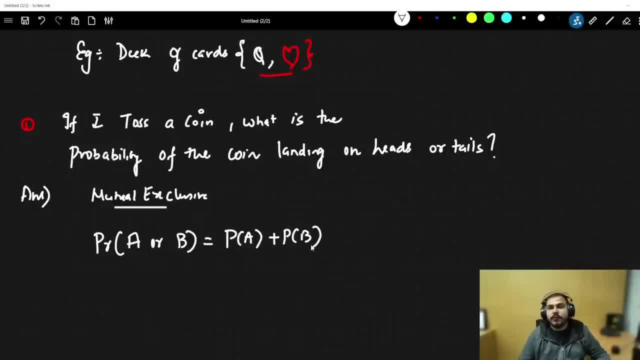 probability of A plus probability of B. So whenever you have a mutual exclusive event, at that point of time you can define this specific definition, which is also called as additional rule for mutual exclusive. Now here, what is probability of A? You know that it is 1. 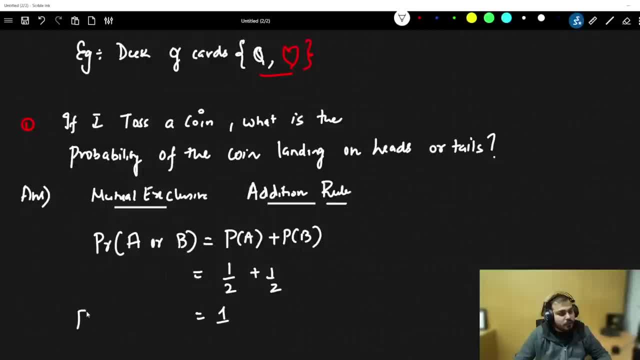 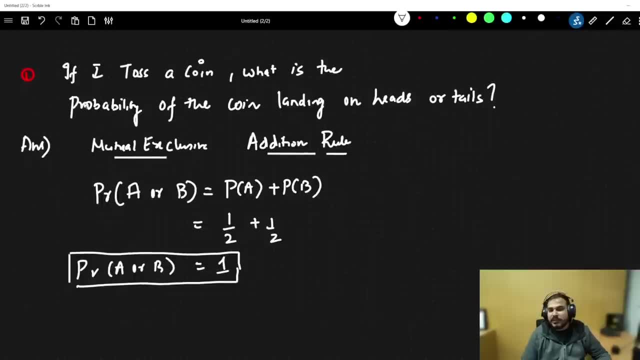 by 2 plus 1 by 2.. So the answer will be 1.. So probability of A or B to come is basically 1.. These are some very, very important things. In exams also you will be getting this In aptitude also. you will be getting it In multiple things. you will basically be getting: 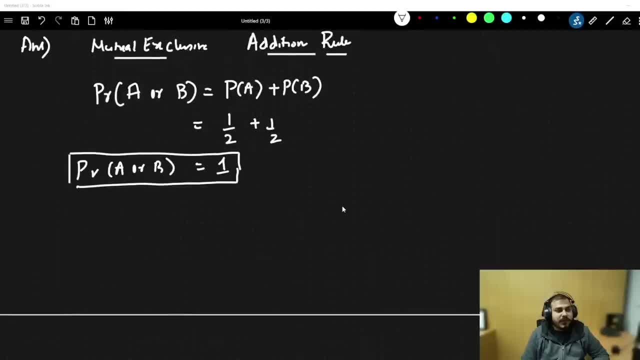 it Now I may also tell you: okay, let's take one more exam. What is the probability, Suppose, if I roll a dice, what is the probability of getting 1 or 3 or 6?? Yes, many people are saying. 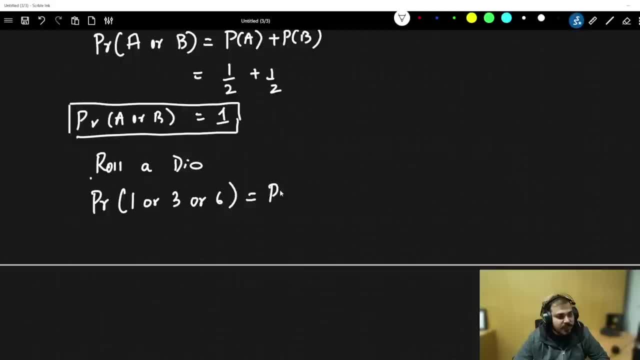 it right, It is 1 by 2.. So here I will basically say that. what is this? I can definitely say it: probability of 1 plus probability of 3 plus probability of 3, 6.. These all are 1 by 6 plus 1 by 6 plus 1 by 6, which is nothing, but 3 by 6,, which is nothing. 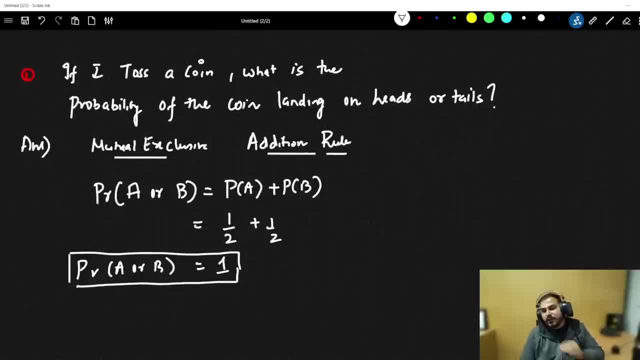 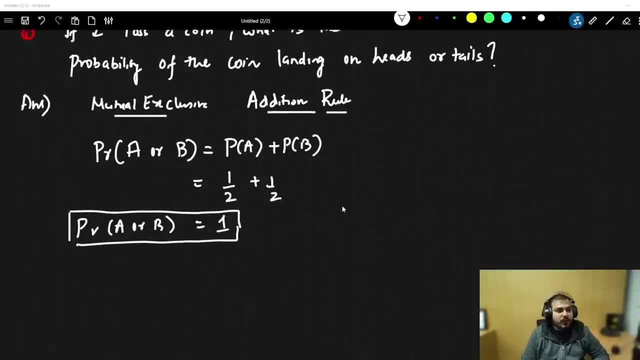 These are some very, very important things. In exams also, you will be getting this. In aptitude also, you will be getting it In multiple things. you will basically be getting it. Now I may also tell you: Okay, let's take one more example. 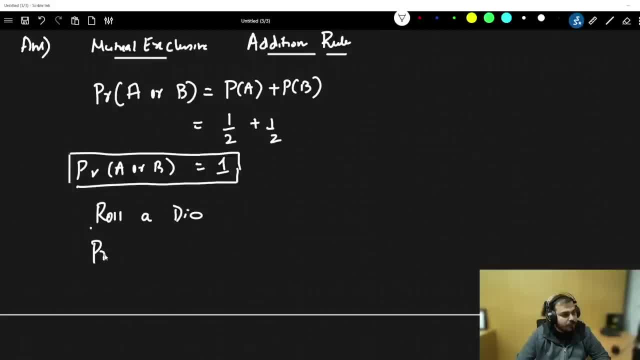 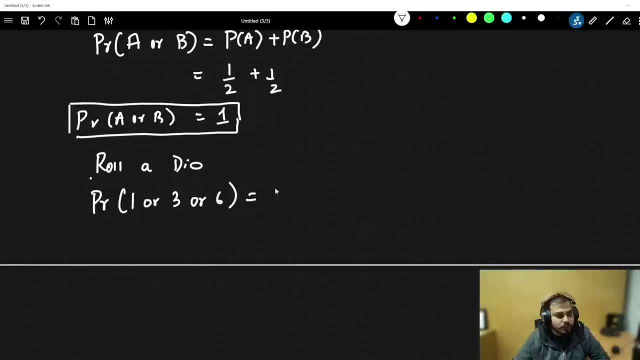 What is the probability, Suppose, if I roll a dice, What is the probability of getting 1 or 3 heads, 1 or 3 or 6.. Yes, many people are saying it right: It is 1 by 2.. So here, 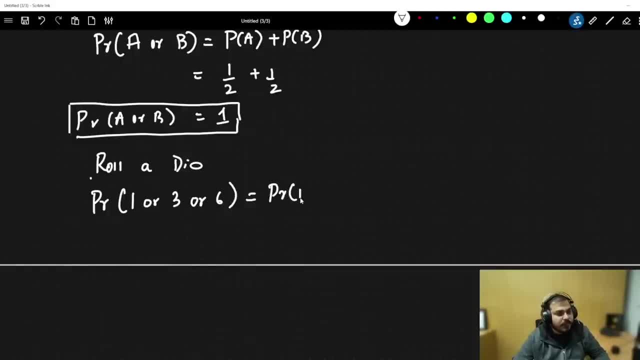 I will basically say that. What is this? I can definitely say it as probability of 1. Plus probability of 3. Plus probability of 3. 6.. These all are 1 by 6. Plus 1 by 6.. 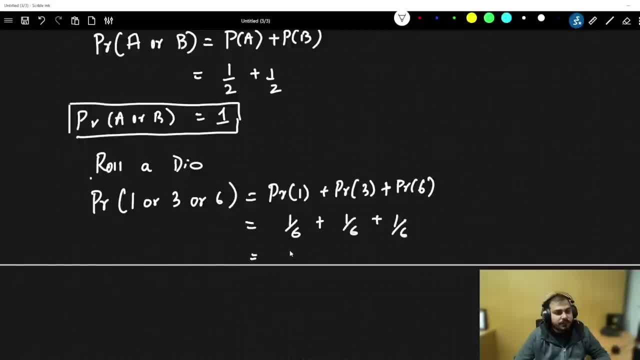 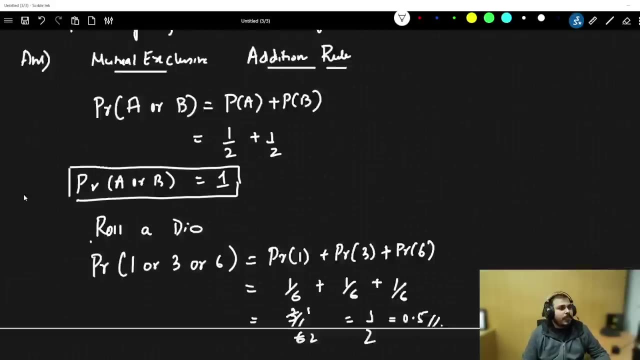 Plus 1 by 6. Which is nothing but 3 by 6.. Which is nothing but 1 by 2. Which is nothing but 0.5.. So 0.5 is basically with respect to this, And here you can easily solve it. 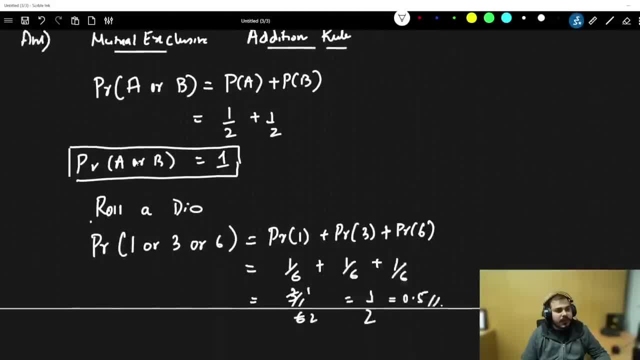 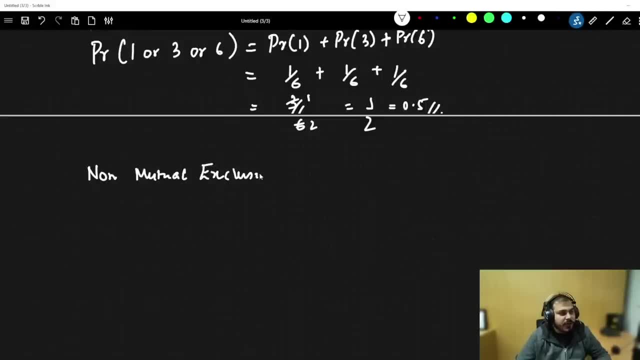 Now, this was with respect to mutual exclusive. This is what we have discussed in mutual exclusive. If I take the next problem, statement For non-mutual exclusive. So, for non-mutual exclusive, Let me take a very good example again. 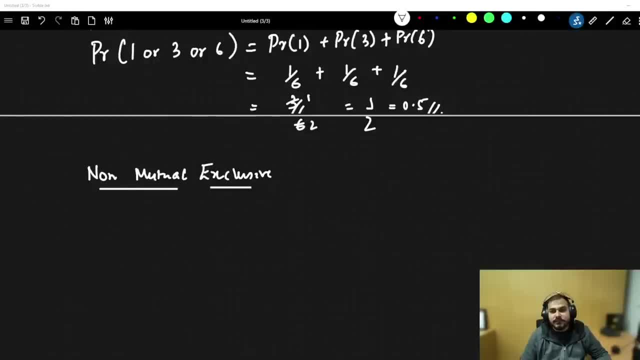 So the question is very much simple Over here. Let's say that You are picking a card. You are picking a card Randomly- This is the question- From a deck. So the question is: What is the probability Of choosing a card? 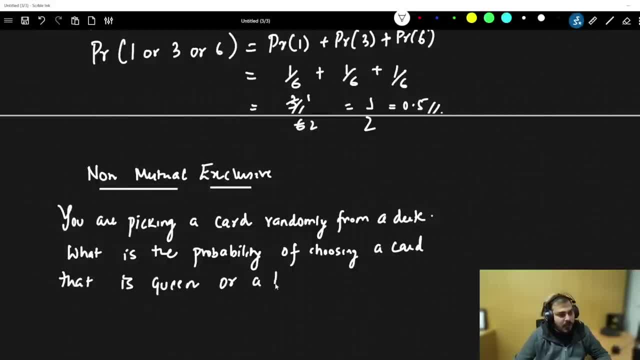 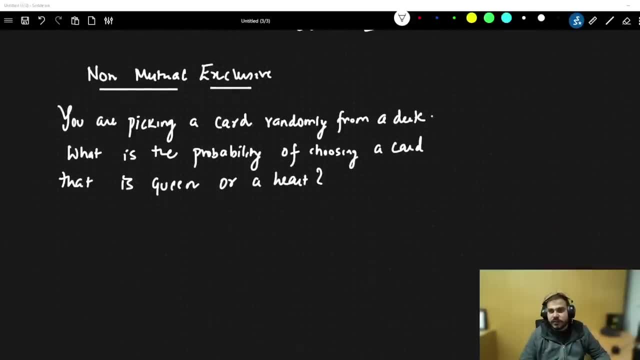 That is Queen Or A heart. So this is the question Very simple. Obviously, first step, You will see that, Whether it is mutual exclusive Or non-mutual exclusive, Obviously you will say that In this particular scenario. 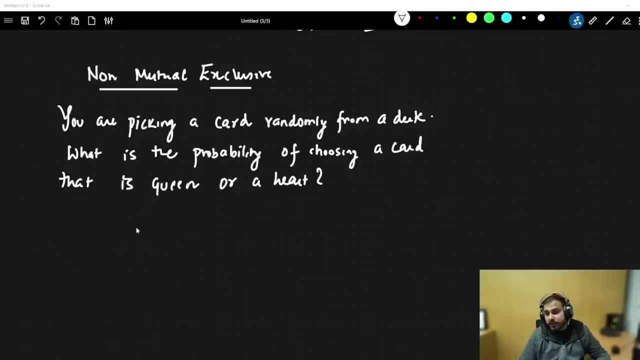 It is Non-mutual exclusive. On mutual exclusive, It is Non-mutual exclusive Right Because it can Occur at the Same time. Now Let's go ahead Towards the answer. Obviously you understood. 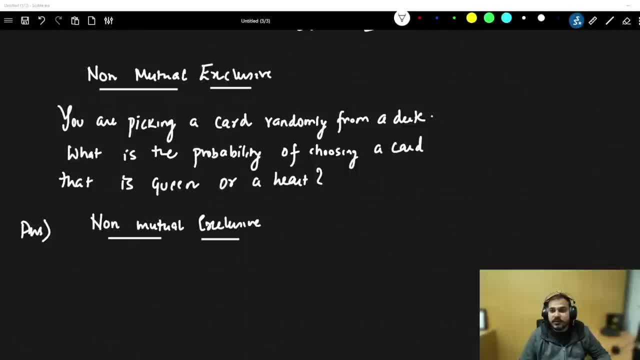 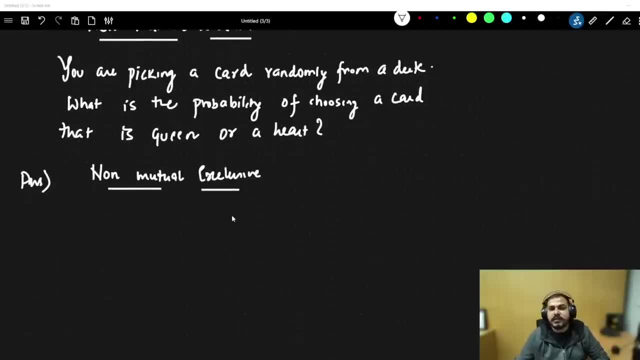 That this is Non-mutual, exclusive. Now, How do you solve This specific problem? Now, In this specific problem, First of all You need to find out What- all Different things- It is basically asked. Let's say that: 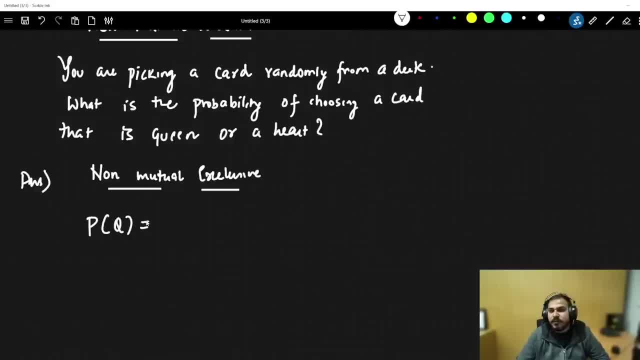 I have got Probability Of getting a queen. What is probability Of getting a queen? Guys, Just think over it. How many cards, How many queen card, Will be in deck of cards? In the total deck of cards There are? 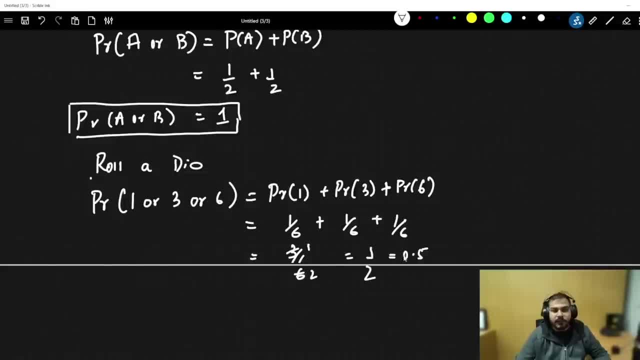 but 1 by 2, which is nothing but 0.5.. So 0.5 is basically with respect to this, And here you can easily solve it. Now, this was with respect to mutual exclusive. This is what we. 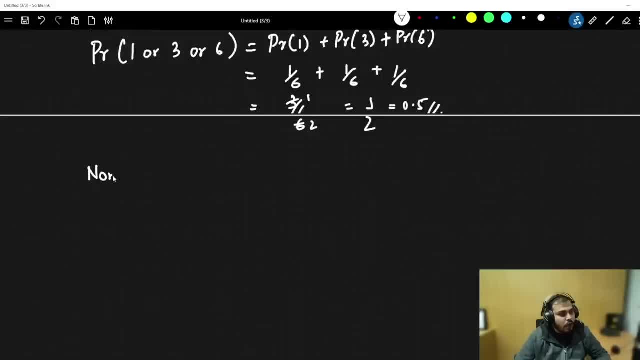 have discussed in mutual exclusive. If I take the next problem statement for non-mutual exclusive, let me take a very good example again. So the question is very much simple over here. Let's say that you are picking a card. You are picking a card randomly. This is the question from a deck. 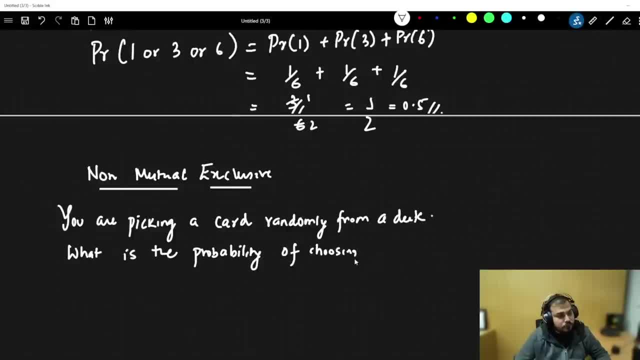 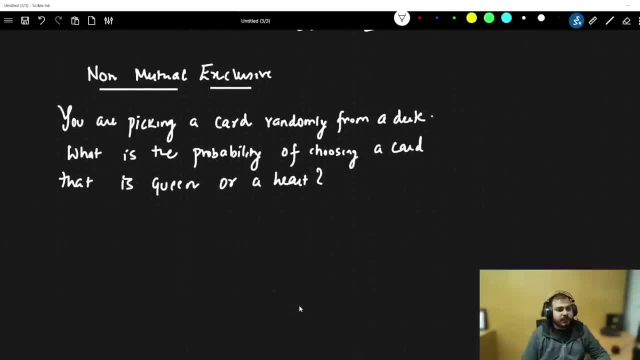 So the question is: what is the probability of choosing a card that is queen or a heart? So this is the question, Very simple. Obviously, first step, you will see that, whether it is mutual exclusive or non-mutual exclusive, Obviously you will say that 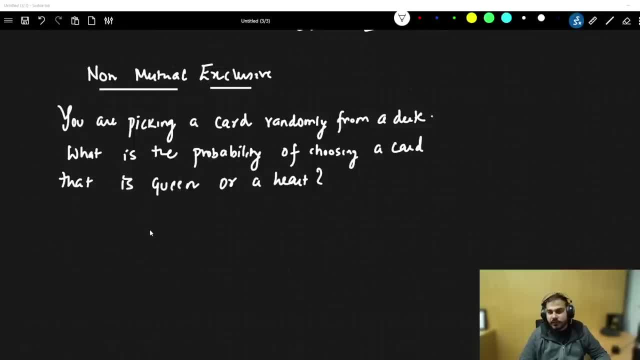 in this particular scenario, it is non-mutual exclusive Or mutual exclusive. it is non-mutual exclusive right Because it can occur at the same time. Now let's go ahead towards the answer. Obviously, you understood that this is non-mutual exclusive. Now how do you solve this specific? 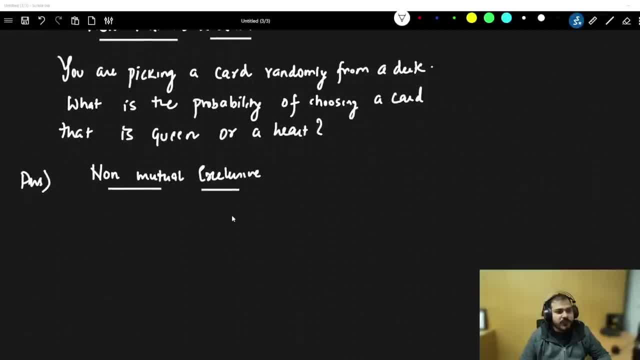 problem. Now, in this specific problem, first of all you need to find out what all different things it is basically asked: Let's say that I have got probability of getting a card, I have got probability of getting a queen. What is probability of getting a queen, guys? Just think over it. How? 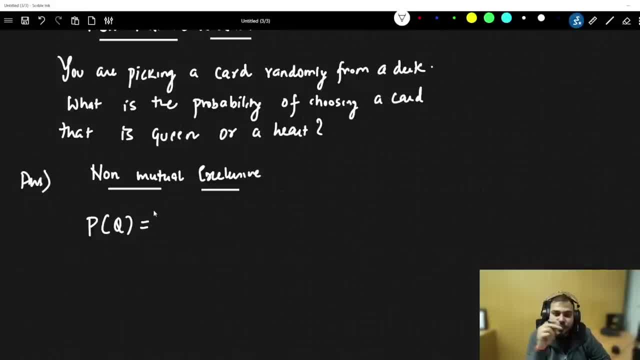 many cards. how many queen card will be in deck of card? In the total deck of cards there are 52 cards, right? If none of you have played cards, please go buy today and see. The probability of getting queen is nothing but 4 by 52, because in every deck there will be 4 queen cards. 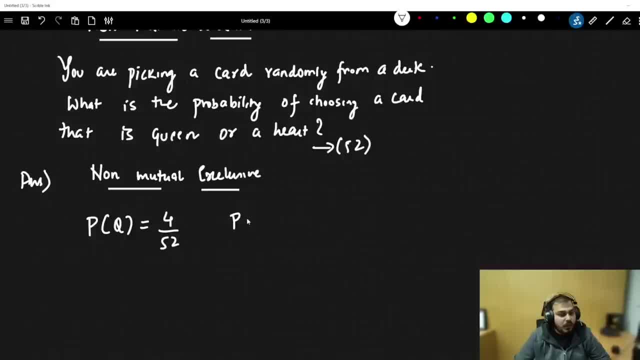 Now the next thing: probability of heart cards. So what is this probability of heart? How many heart cards will basically be there in a deck? Obviously, there will be 13 cards, So I'll say 13 by 52.. Now the next thing is that: probability of 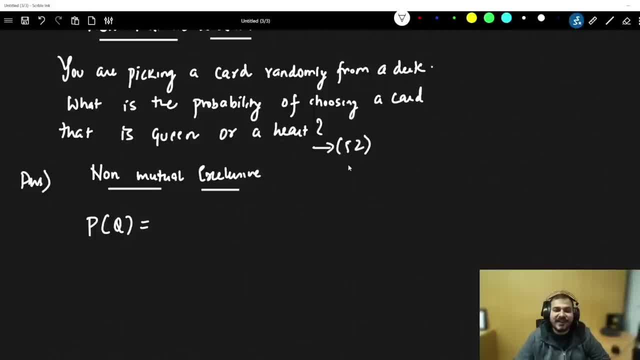 2 cards Right. If none of you Have played cards, Please go buy today And see. The probability Of getting queen Is nothing but 4 by 52. Because in every deck There will be 4 queen cards. 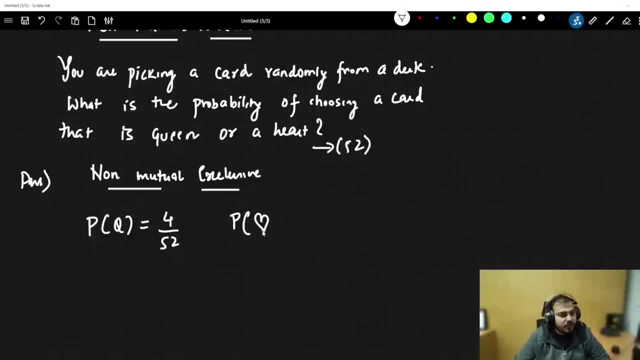 Now The next thing: Probability of heart cards. So What is this Probability of heart? How many heart cards Will basically Be there in a deck? Obviously, There will be 13 cards. So I will say: 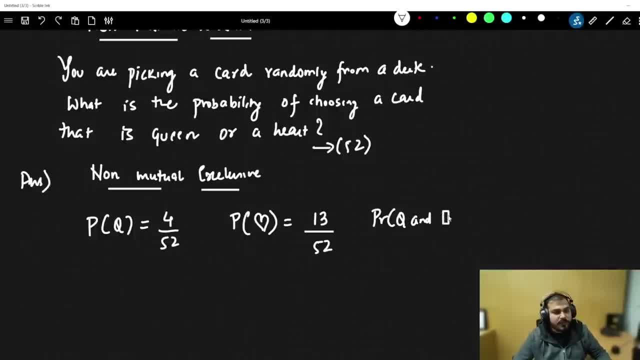 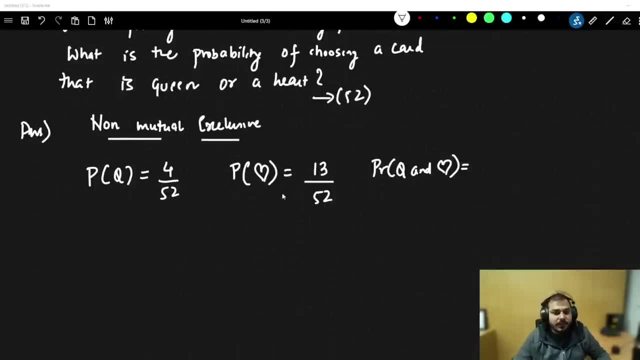 13 by 52. Now, Because this is also One possibility, Right, This is also One possibility. How many queen And heart Will be there? Basically, It will be Only one. So Here I will write. 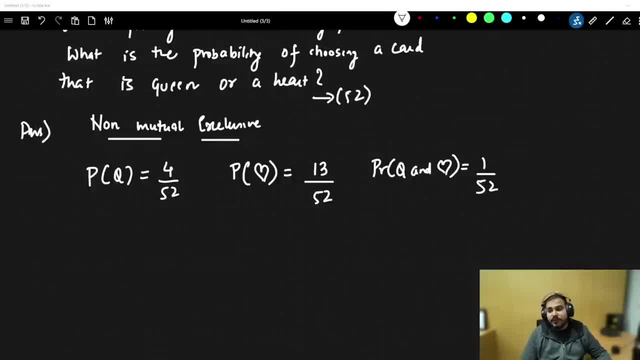 1 by 52.. So These are The possible Things That can Occur, Right, This is the thing. Now, If I come To the formula, And this is the Addition Rule Is equal. 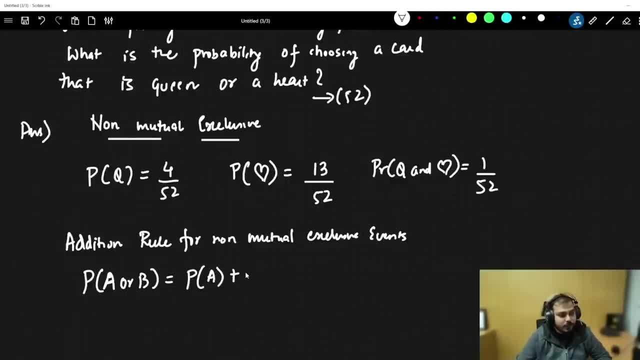 To Probability Of A Plus Probability Of B, There will be One Important Thing Which is This intersection, Which I have to Basically Separate it, So It will be P Probability. 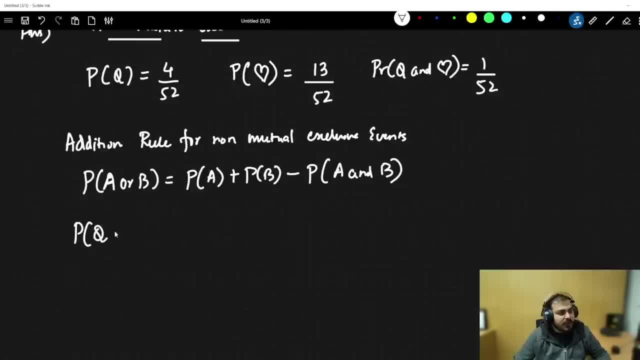 Minus, P Sorry, Minus Probability Of A Color. You Have The Answer With You. This Will Be Probability Of Queen Plus Probability Of Heart Probability. 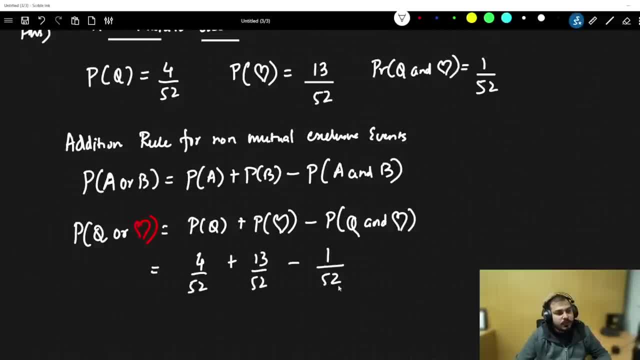 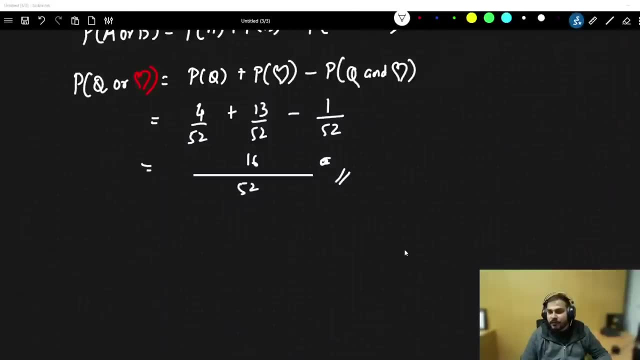 Of Heart Minus Probability Of Queen And Heart. So What Is In How Much The 52. You Can Calculate? This Will Basically Be The Probability. 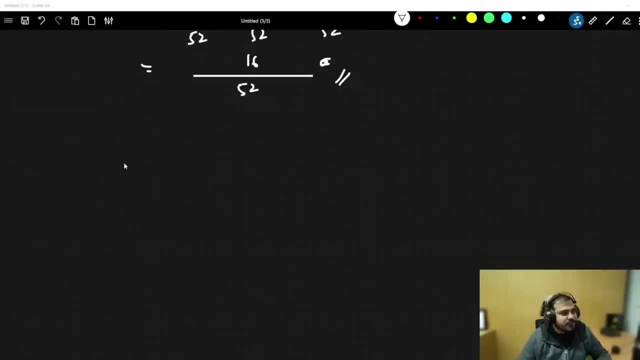 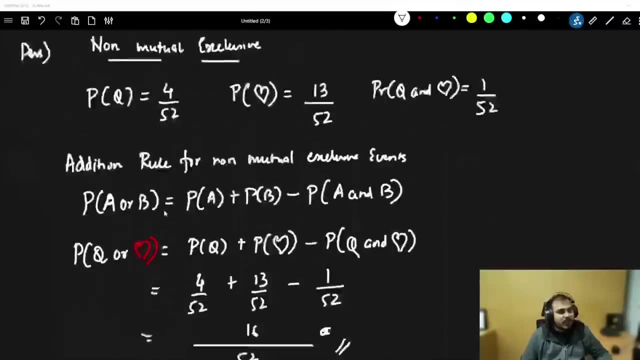 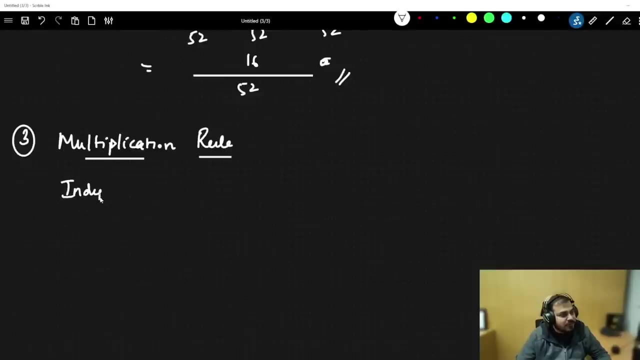 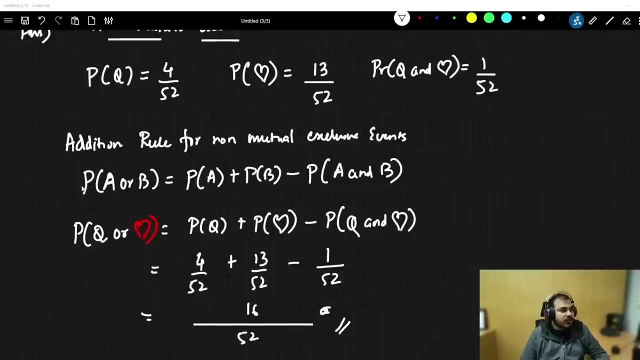 Now You Have Probably Understood Additional Addition. Now We Need To Understand One More Rule To Understand Here. We Need To Understand Something Called As. 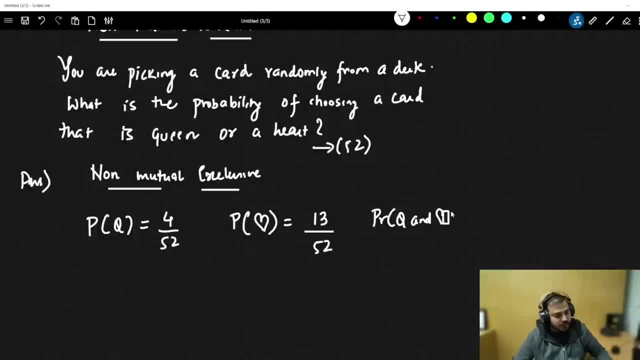 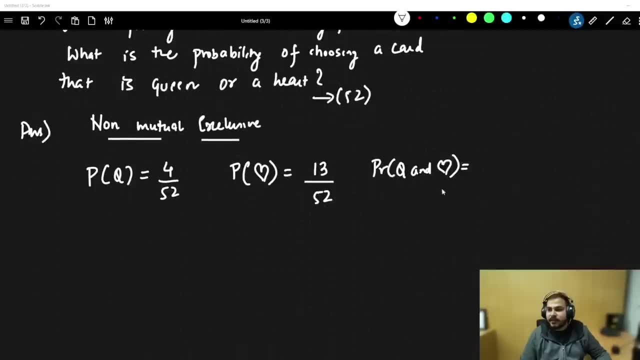 queen and heart, because this is also one possibility. right, This is also one possibility. How many queen and heart will be there? basically, It will be only one. So here I will write 1 by 52.. So these are the possible things that can occur, right, This is the thing. Now, if I come to the 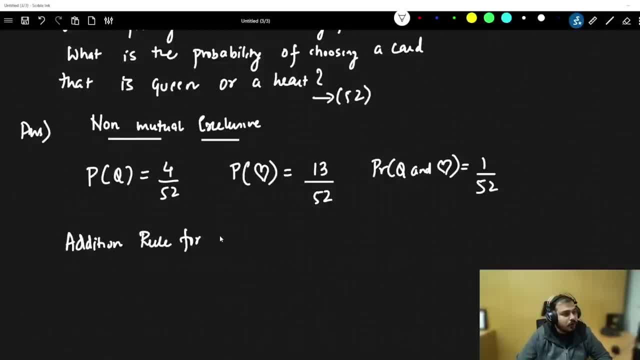 formula and this is the addition Rule for non-mutual, exclusive event, non-mutual, I can write: probability of A or B is equal to probability of A plus probability of B. There will be one important thing, which is this intersection, which I have to basically separate it, So it will be P minus P, sorry, minus probability. 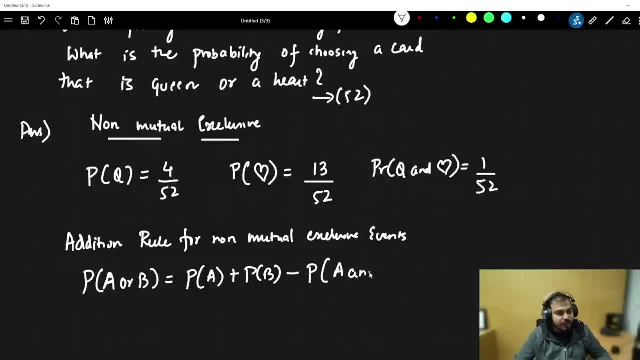 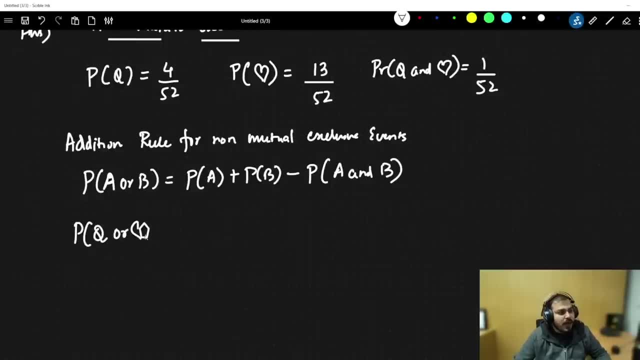 of A intersection B. A intersection B basically means A and B, which is the possibility of both. Now my question is very simple: What is the probability of getting queen or heart? I'll draw it with red color. You have the answer with you. This will be probability of queen plus probability of heart. probability of heart. 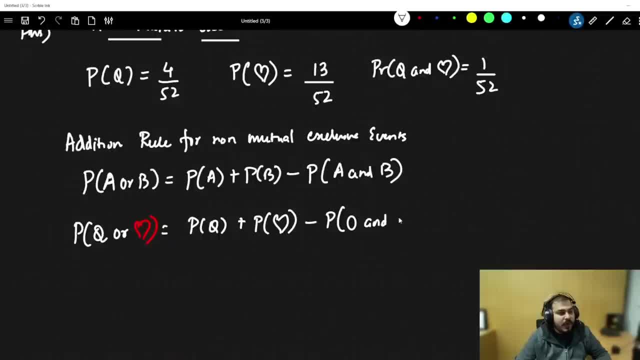 minus probability of queen and heart. So what is probability of Q? 4 by 52.. What is probability of heart? It is 13 by 52.. And what is probability of queen and heart? It is 1 by 52.. 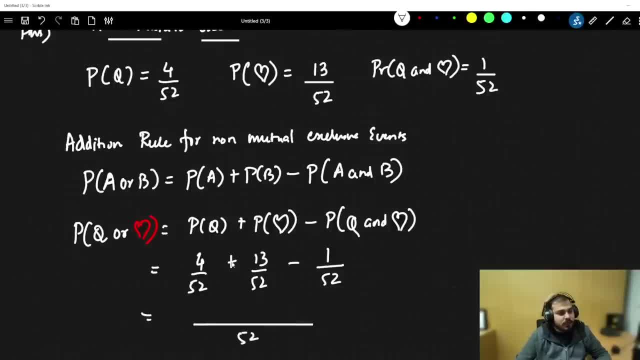 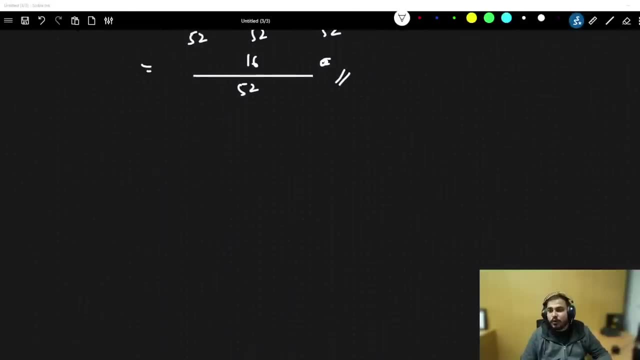 1 by 52.. here I am actually getting 52. this will be 17 minus 1, 16, 16. how much the 52 you can calculate? this will basically be the probability. now you have probably understood additional rule, addition rule. now we need to understand one more rule in probability. see, guys, if you do this much, 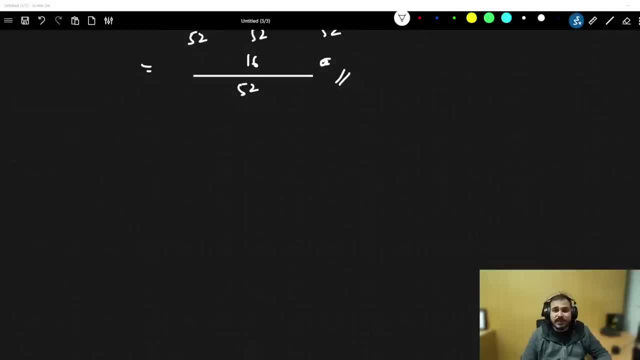 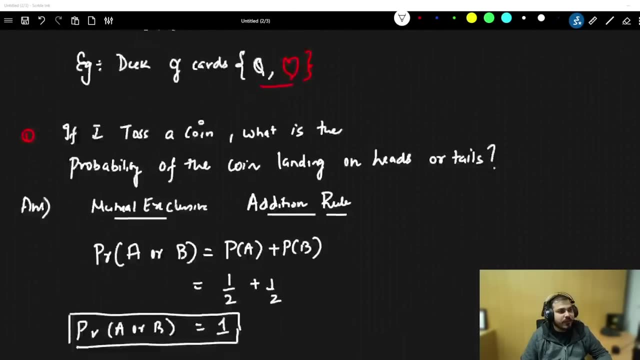 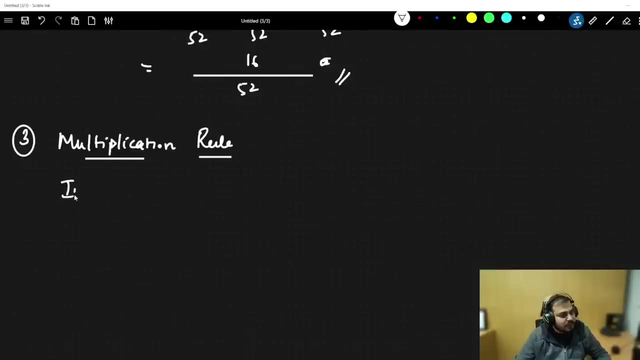 I think you will be able to solve any problem statement that comes in your mind. so here was the problem statement that we did, and this was specifically to something called as addition rule. now coming to the third one, which is called as multiplication rule. in multiplication rule, one thing you need to understand here: we need to understand something called as: 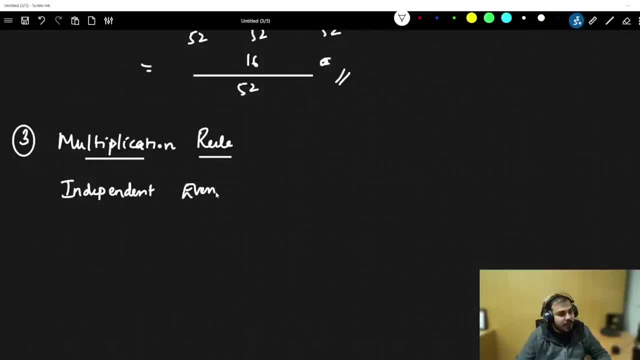 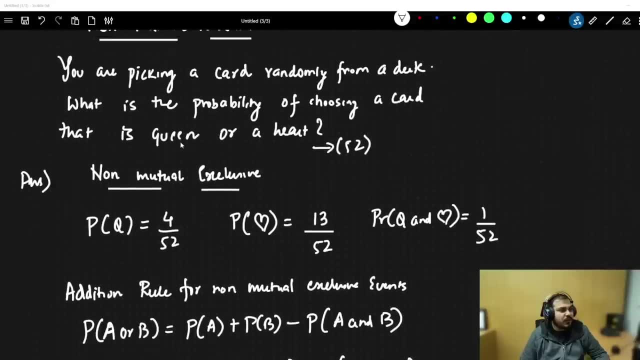 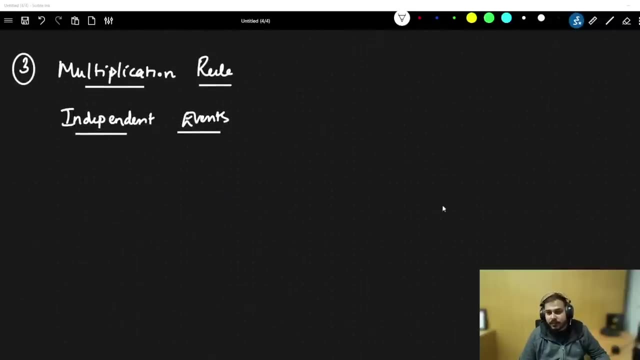 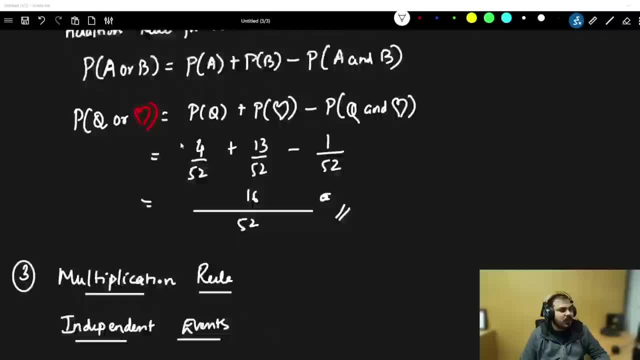 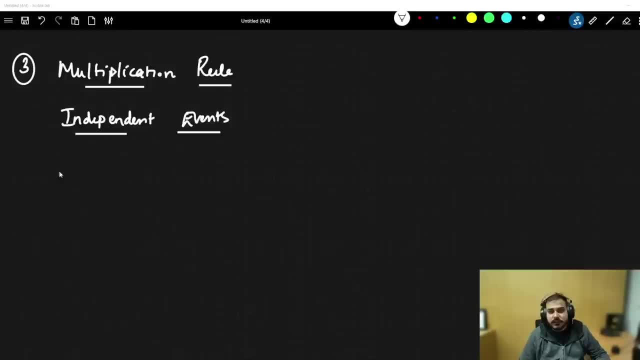 Independent, Independent Events And Non Independent Events. These Are Something Very, Very Important, But It Should Be, And I May Get One, Two, Three, Four, Five. 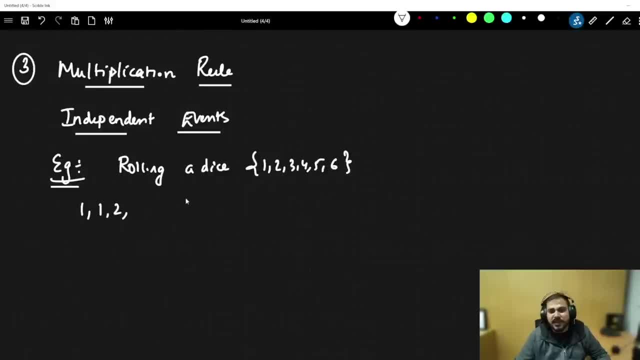 Six Suppose. For The First Instance I Got One. In The Second Instance. It Is Possible I May Get One In The Second Instance In The 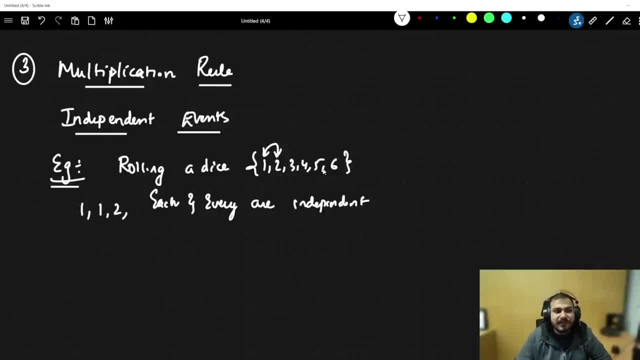 Third, In The Last Time, For Each And Every Events Are Independent: One If One One Comes, Or If Two Comes, Or If Any Events. I 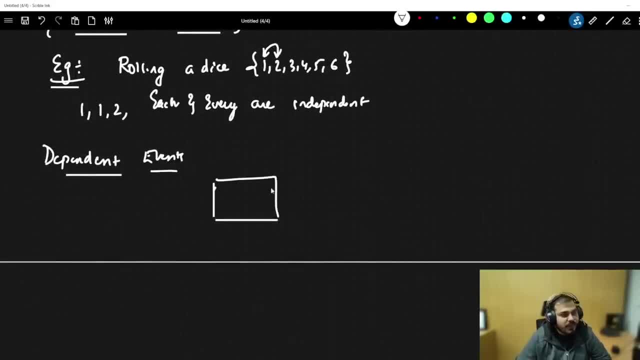 Have A. I Have A Bag In This Bag. Let's Say I Have Three Red Marbles And Two Green Marbles. Now, In The First, 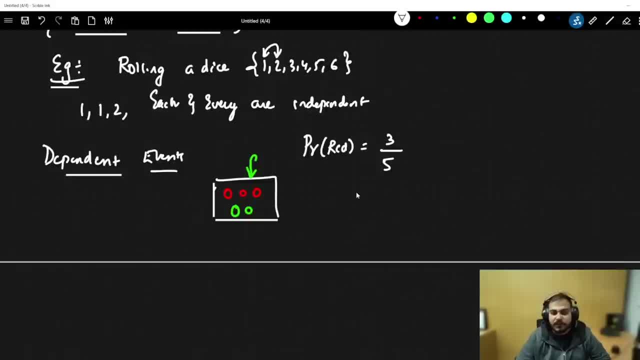 Instance, If I Have Three Marbles, I Have Three Marbles. Now. Let's Consider: In The First Event You Picked Out A Red Marble. Now, 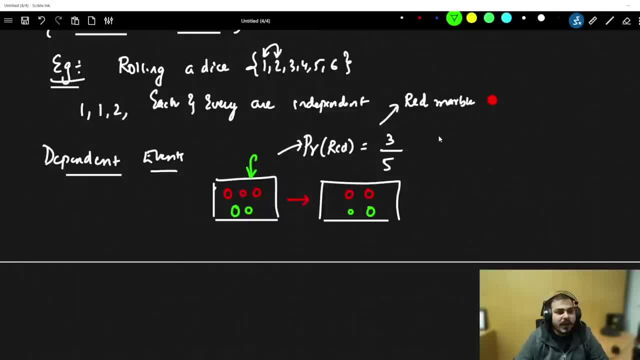 After Taking Out The Red Marble, How Many In Marble? Then How You'll Basically Say, How You'll Basically Say: You'll See That, Okay, How. 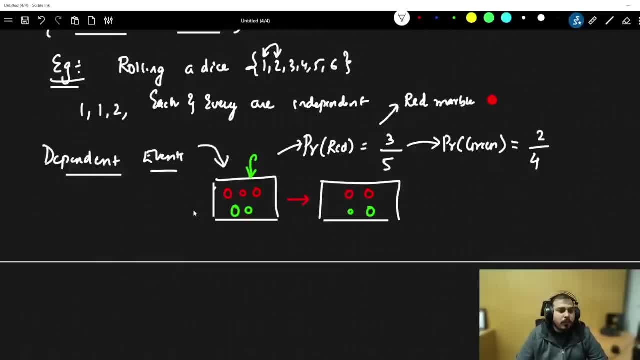 Many Number Of Marbles Are There To Buy For Us. So Here, What Is This? Because Of This Dependent Event, There Is An Amazing Algorithm. 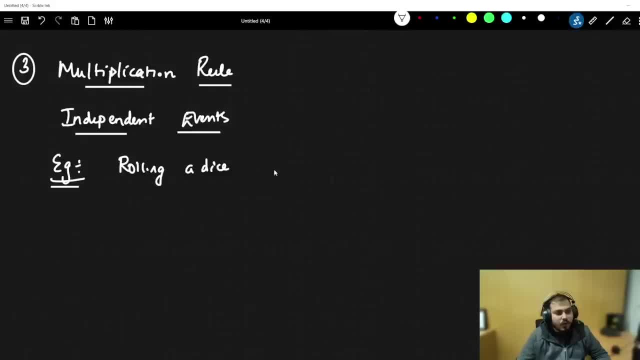 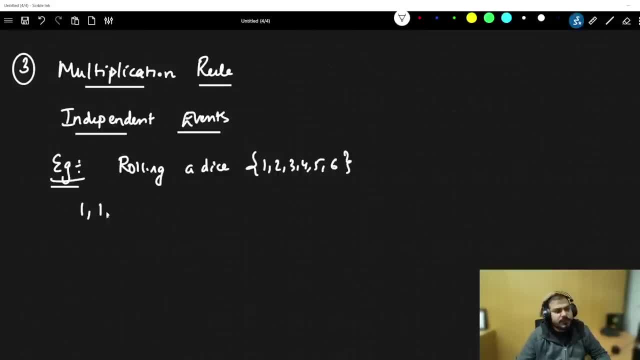 Suppose, for the first instance I got 1.. In the second instance, it is possible, I may get 1.. In the third instance, I may get 2, I may get any number. So one event is not at all dependent on the other event, right? 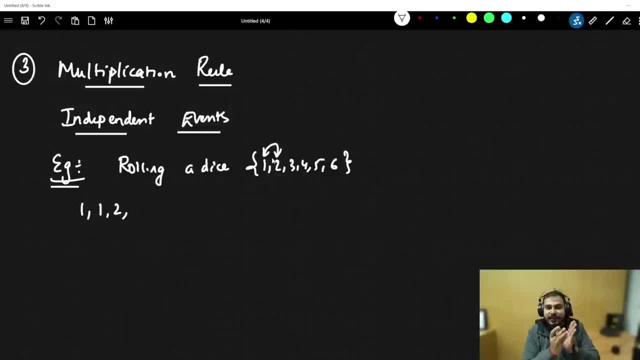 Because anytime we roll, every possibilities or every outcomes has an equal probability to come Over here. what you can understand is that each and every events, each and every events, each and every events are independent, One. if one one comes, or if two comes, or if any events come, it is not going to impact. 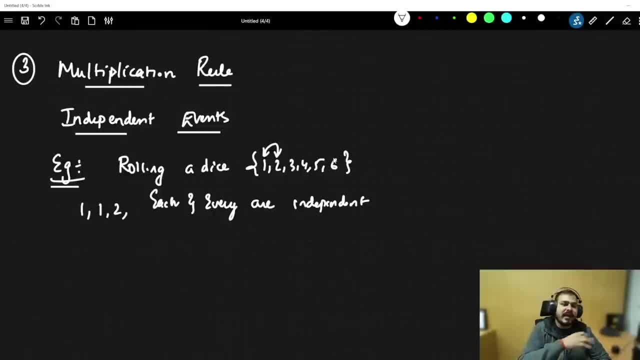 any other event. Every time you probably have to roll and everybody has an equal probability to come over here. This is what is an independent event called. Let me talk about non-independent event, or I will also say it as non, not non-independent, but instead I will say dependent event. 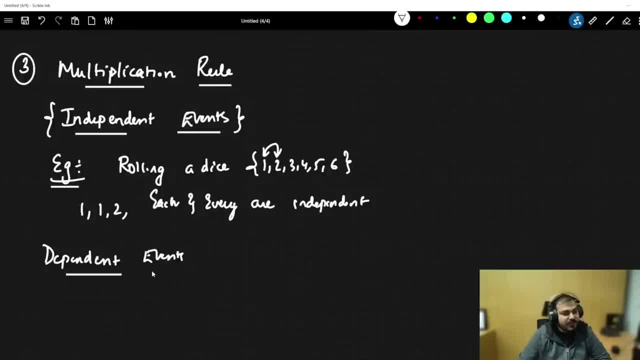 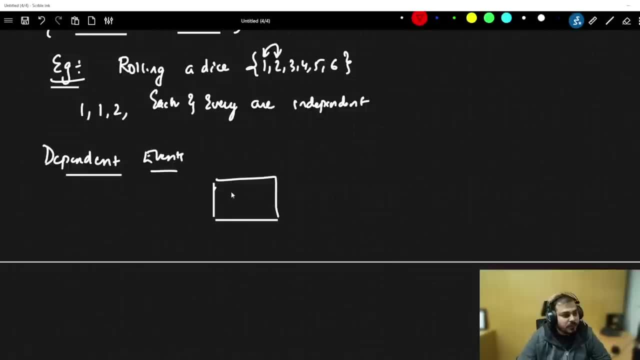 So I will talk about dependent event. Now, in dependent event, suppose let's say that I have a, I have a bag. In this bag, let's say I have 3 red marbles and 2 green marbles. Now, in the first instance, if I pick out, if I, if I pick up a marble, what is the probability? 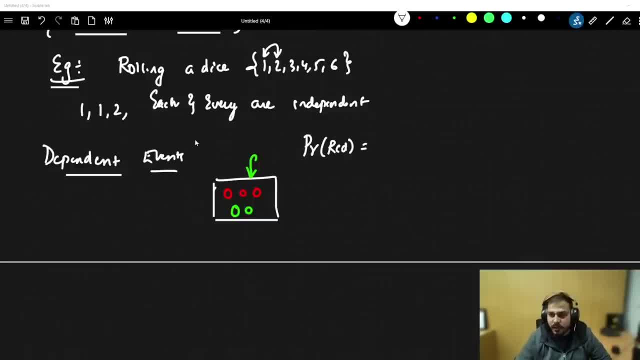 of red marble. What is the probability of taking out the marble? Very simple, You will be seeing that. how many number of marbles are there? They are total 5 marbles And how many number of red marbles are there? There are 3 marbles. 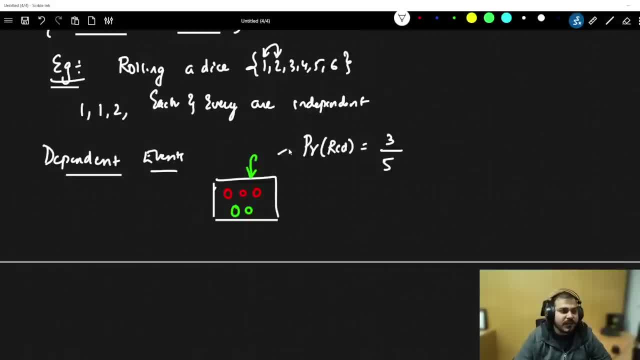 So you are basically able to write 3 by 5.. Now let's consider: in the first event, you picked out a red marble, So you picked out a red marble, So I will make it as red color. Now, after taking out the red marble, how many marbles are remaining? 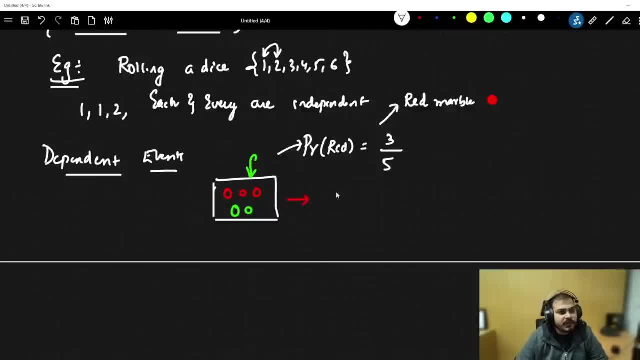 So I will now update this. Okay, So how I will update this. I will update this bag Now. this bag will basically have 2 red marble and 2 green marble. Now, if I try to go ahead and find out, What is the probability, 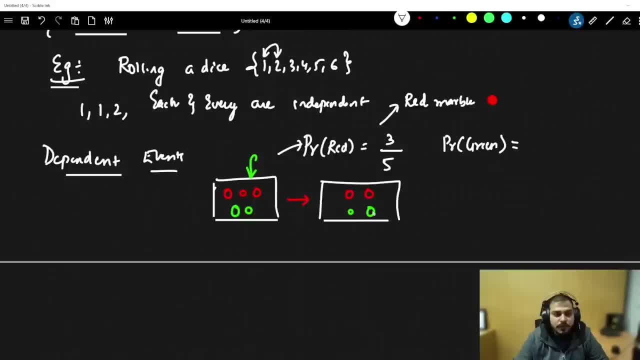 Okay, So I have now taken out a green marble. Then how you will basically say? How you will basically say: You will see that, okay, how many number of marbles are there 2 by 4.. So here, what is happening after this particular event? it has impacted this event. 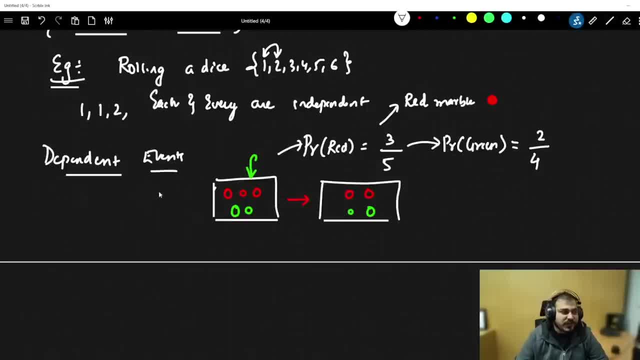 Because the number of marbles are reduced and finally, you got 2 over here. So this is a perfect example of a dependent event. Multiplication rule basically says that in the case of an independent event, we have to solve it in a different way. 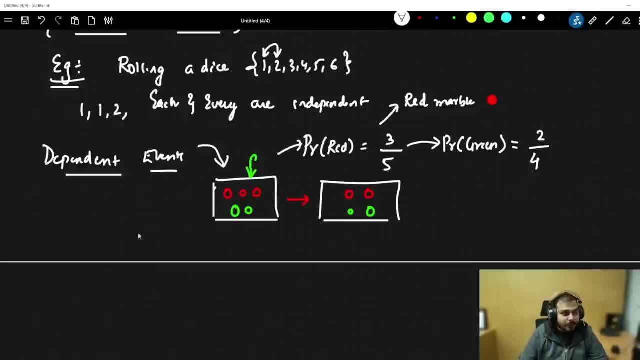 In the case of a dependent event, we have to solve in a different way Because of this dependent event. there is an amazing algorithm which is called as Nape Bias. Have you heard of Nape Bias? I think most of you have heard of. 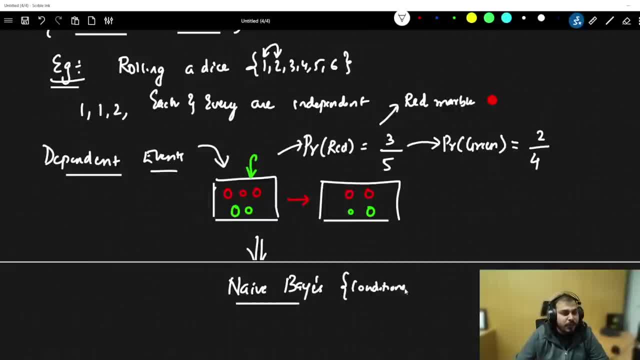 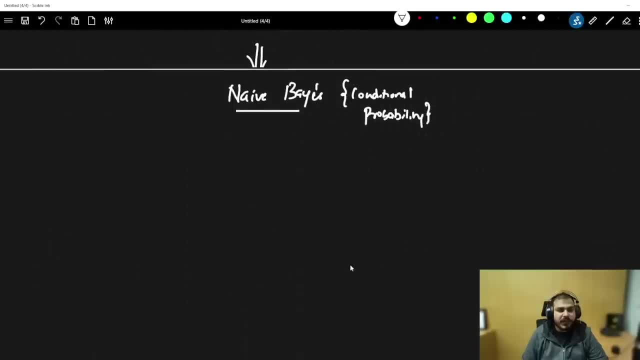 Right, There is a topic which is called as conditional probability. This is where conditional probability will come into existence, So I will talk about it. Okay, So let's go and solve some problems. So let me just go ahead and talk about a problem statement. 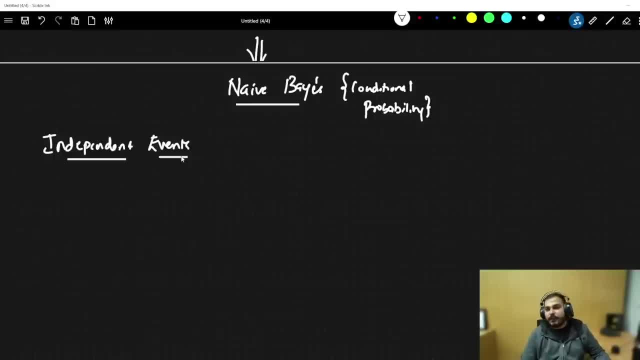 First we will talk about independent events. So independent events, We are going to basically discuss about the problem. First thing, the question is: what is the probability of rolling a 5 and then a 4?? So this is your question, What it is saying. 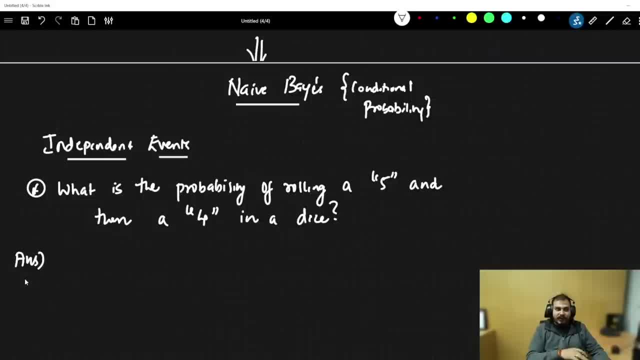 What is the probability? in the first event you have rolled a dice, you are getting 5, and then again you rolled a dice, then you got 4.. So what is the probability of getting 5 and then 4?? This is a simple question. 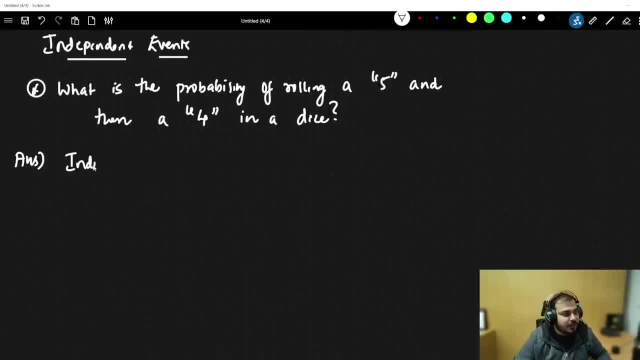 And for this, This, This, basically, is an independent event. You know that. Now how do we solve this particular problem? So I will say independent event. here we will apply the multiplication rule. What is the multiplication rule? What is the probability of A and B? 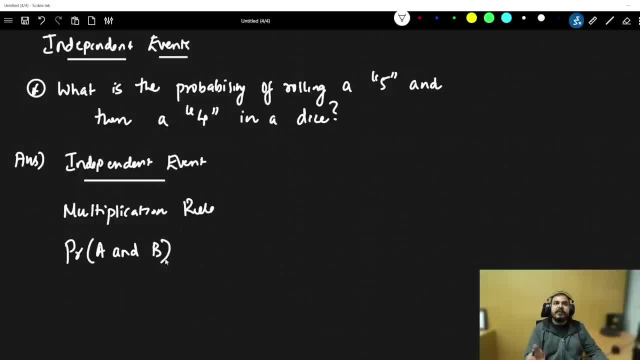 A and basically means first A event has occurred and then B event has occurred. What is the probability of this? So obviously, here I will define the formula over here. First of all I will say probability of A Multiplied by probability of B. 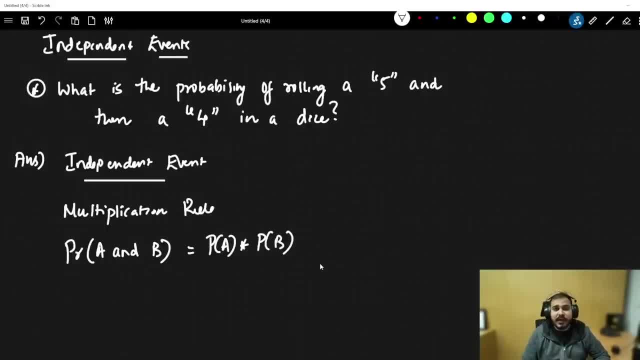 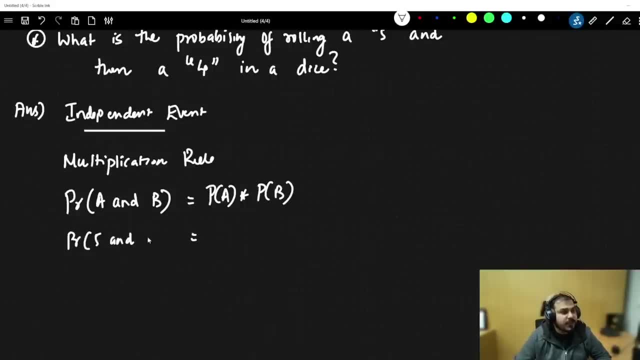 A and then B. Ok, So this is the usual formula that we use for an independent event in a multiplicative rule. So obviously you know what is probability of A. So here I will say probability of 5 and 4.. You know probability of 5.. 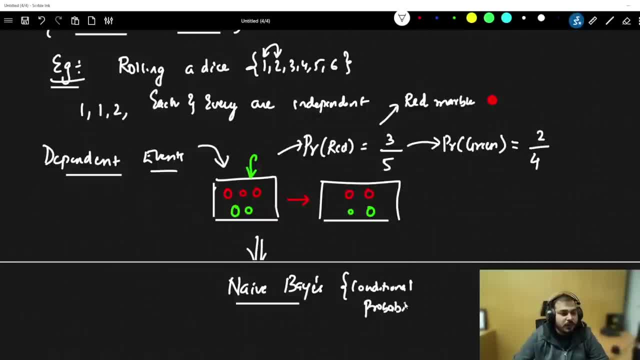 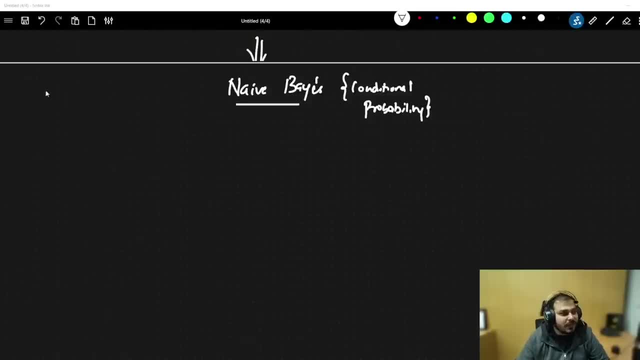 Which Is Called As Nape Bias. Have You Heard Of Nape Bias? I Think Most Of Dependent Events We Are Going To Basically Discuss. 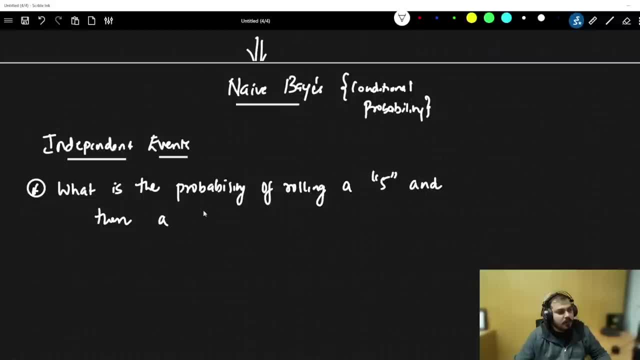 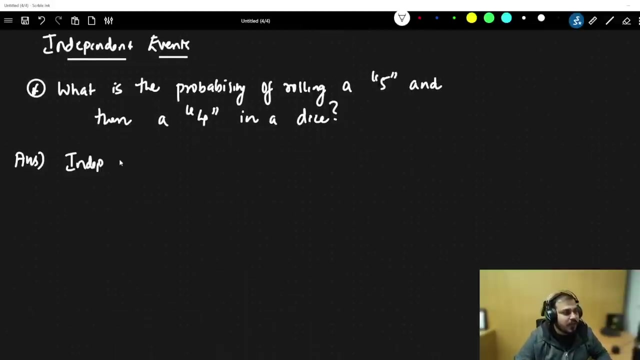 About The Problem. First Thing, The Question Is: What Is The Probability Of Rolling A Five And Then A Four? So This, This Obviously, Is An 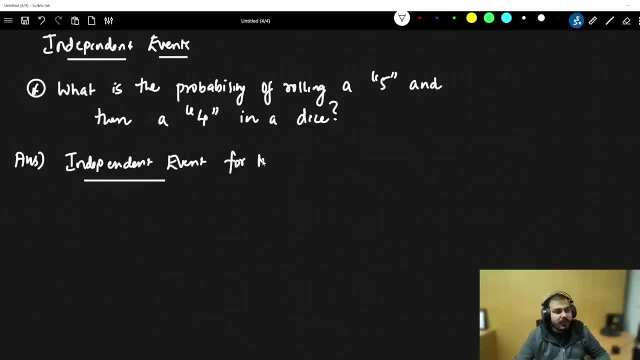 Independent Event. You Know That. Now How Do We Solve This Particular Problem? So I'll Say: Independent Event. Here We'll Apply The Multiplication Rule. 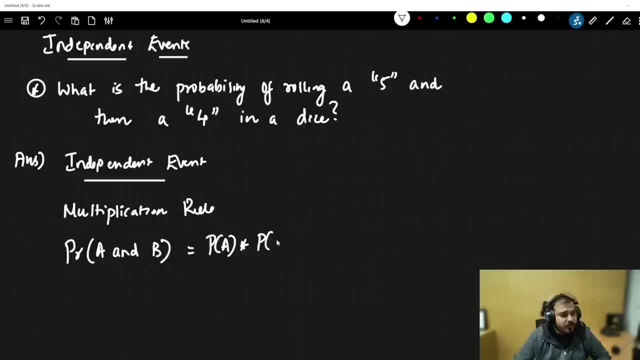 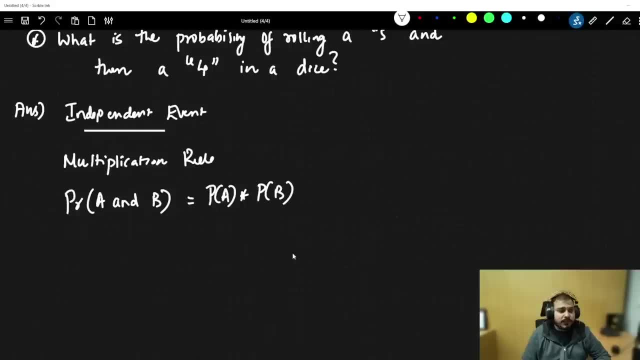 First Of All, I'll Say: Probability Of A Multiplied By Probability Of B, A And Then B. Okay, So This Is The Usual Formula. 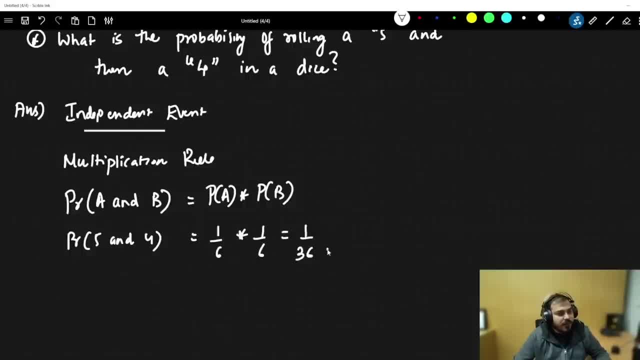 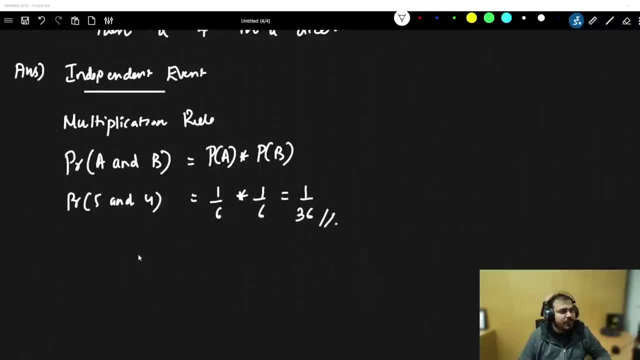 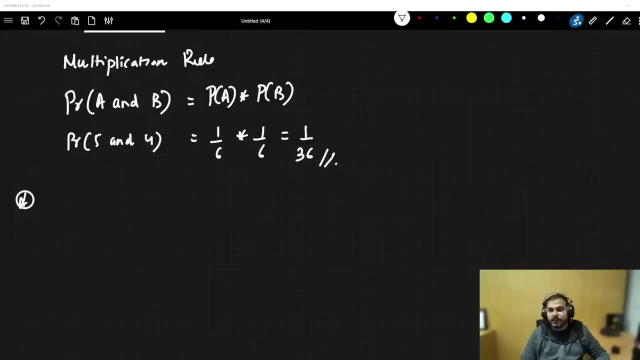 That We Use For An Independent Event. Now Let's Take Another Example, Obviously Because Independent Event Looks Very Simple. So Here I'm Basically Going To. 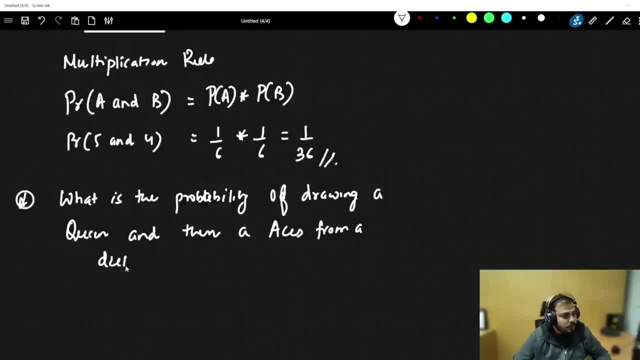 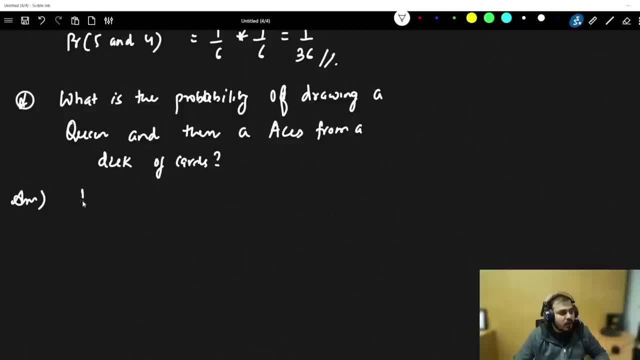 Take Another Example, And This Example Will Be Of Dependent Or Dependent Event. Obviously, In This Case, This Will Be A Dependent Event Because 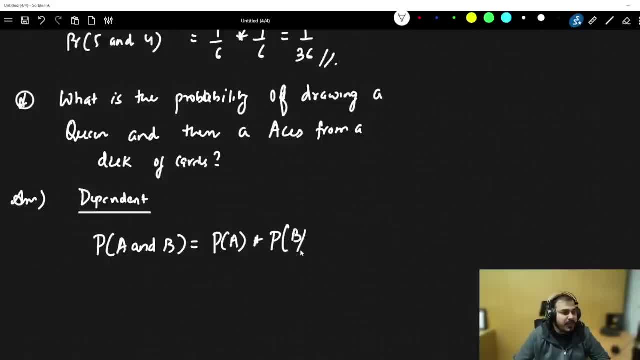 A Deck Of Card Will Get Reduced. So In This Particular Case, I'm Saying: I Have A Bag Over Here. Let's Say That I. 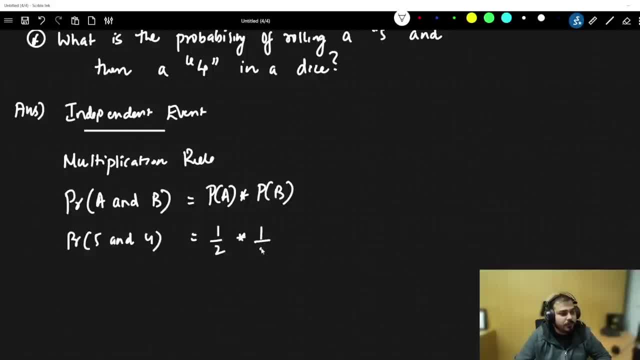 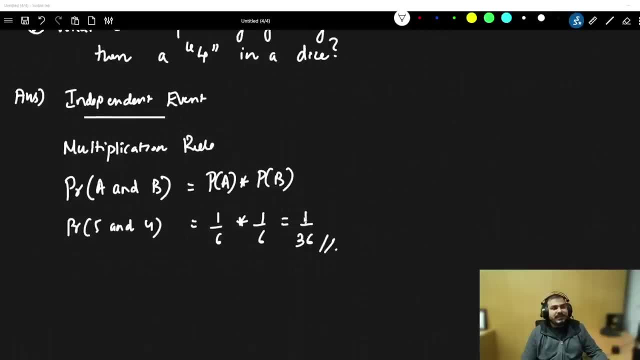 Probability of 5 is nothing but 1 by 2, multiplied by sorry, 1 by 6, multiplied by 1 by 6.. It is nothing but 1 by 36.. Now let's take another example. Obviously, Because 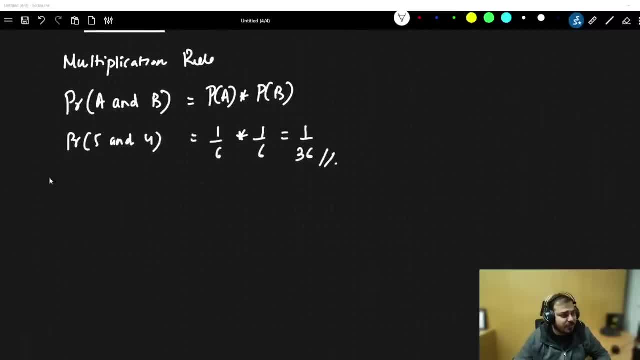 An independent event looks very simple. So here I am basically going to take another example, and this example will be of a dependent event. So let's go ahead and let's try to solve a problem for this. What is the probability of drawing a queen and then a aces from a deck of cards? 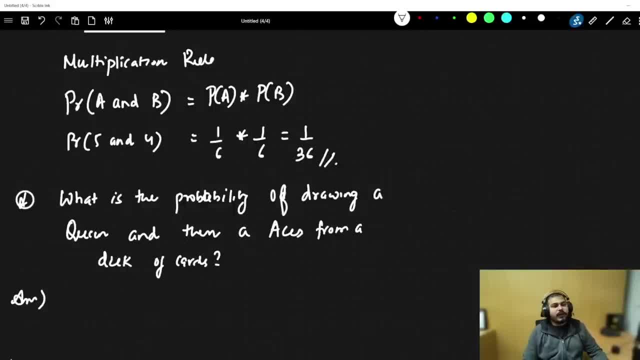 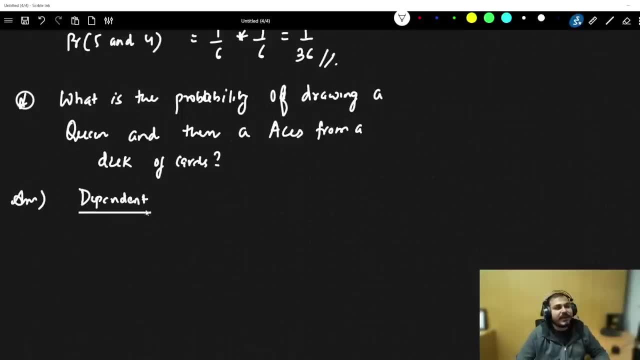 See, over here, two events are actually happening, So let's go ahead. First of all, again, you need to find out whether this is an independent or dependent event. Obviously, in this case, this will be a dependent event, Because a deck of cards will get reduced. 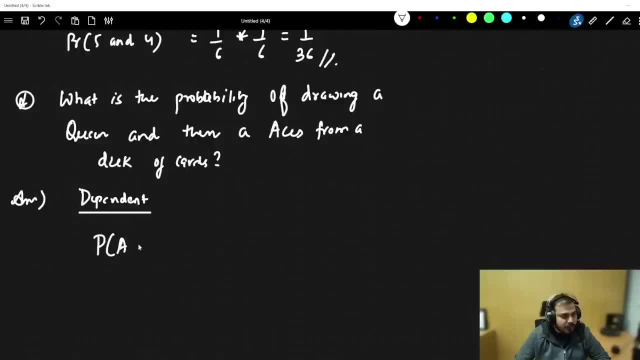 So in this particular case I am saying: what is the probability of A and B in the case of independent event? So here I can basically write: probability of A multiplied by probability of B given A. Now what does this mean? This term is basically called as conditional probability. 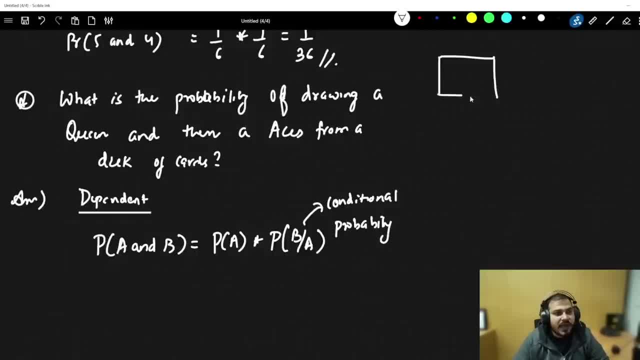 Let me show you an example with respect to the bags. Right, So I have a bag over here. Let's say that I have three marbles, Two red marbles. Okay, Now, in the first instance, I want to find out what is probability of what is probability? 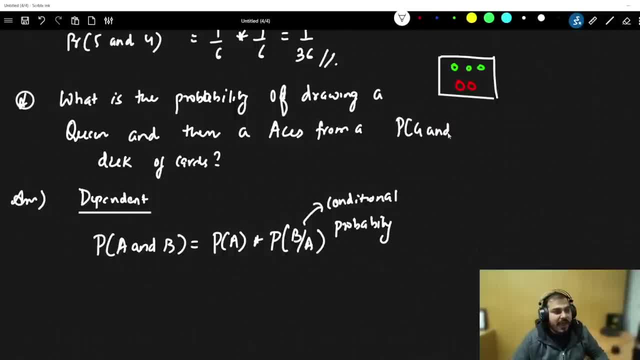 of what is probability of green and then red marble. Now see over here How many marbles are there in the first instance. if I am taking out green, Obviously there is three by five right In the first instance when I took out the green marble. 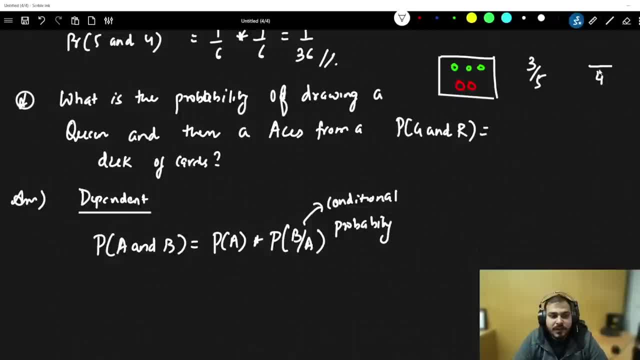 After I take out the green marble, my total number of marbles that will be remaining is four. So the probability of red will be two by four. Now, this term, this term, is basically probability of green. And what is this term? Two by four. 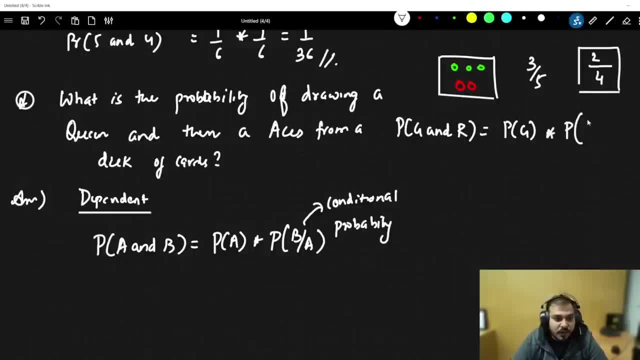 This is nothing but this, only Right, Multiplied by probability of green given red- sorry, probability of red given green Given green basically means this green event has already occurred, Right. So that is the reason the number of marbles has got reduced. 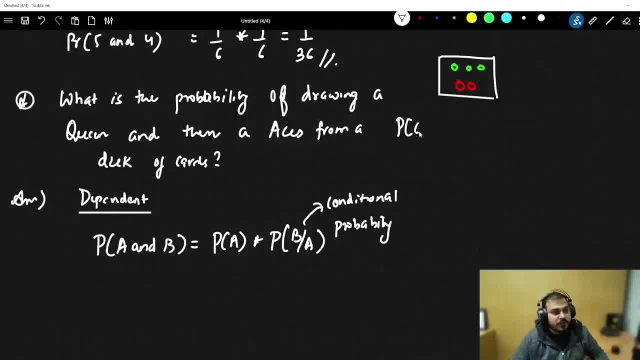 Have Three Marbles, Two Red Marble. Okay, Now, In The First Instance, I Want To Find Out What Is My Total Number Of Marbles. That 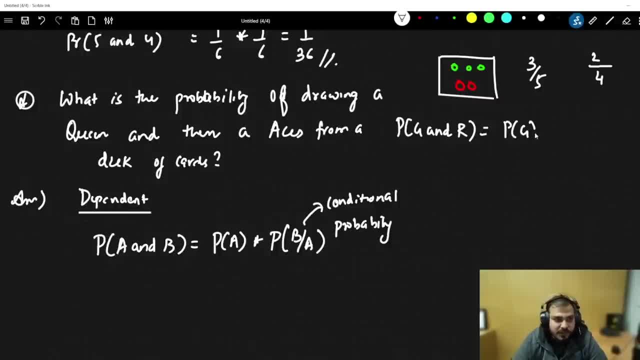 Will Be Remaining Is Four, So The Probability Of Red Will Be Two By Four. Now, This Term, This Term Is Basically Probability, So That Is. 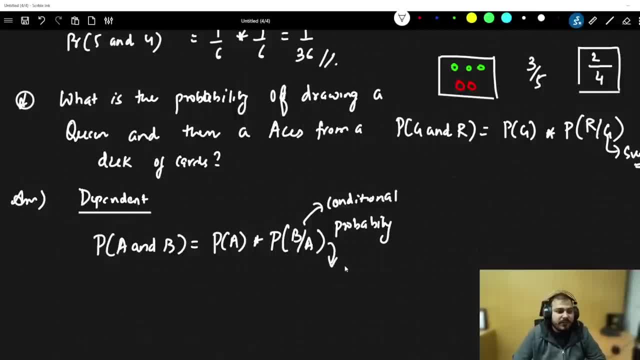 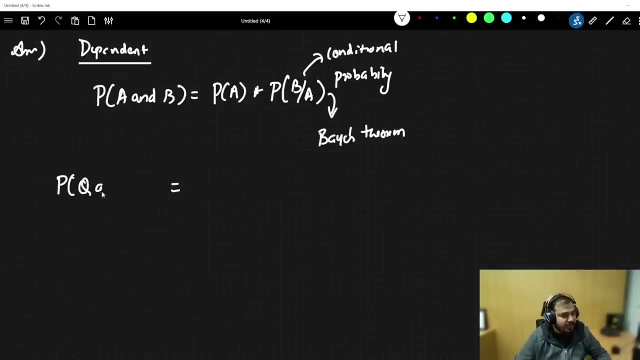 The Reason The Number Of Marbles Has Got Reduced. This Is Called As Conditional Probability, And This Is Very, Very Helpful In Something Called As. 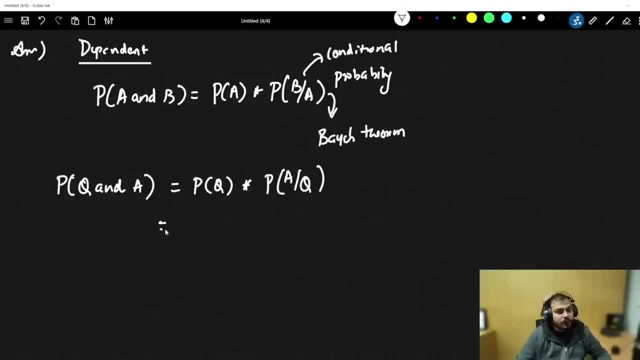 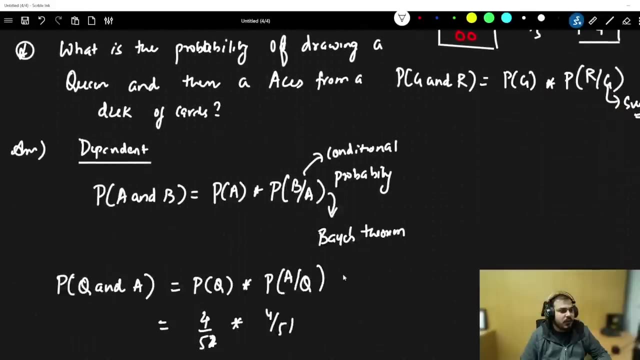 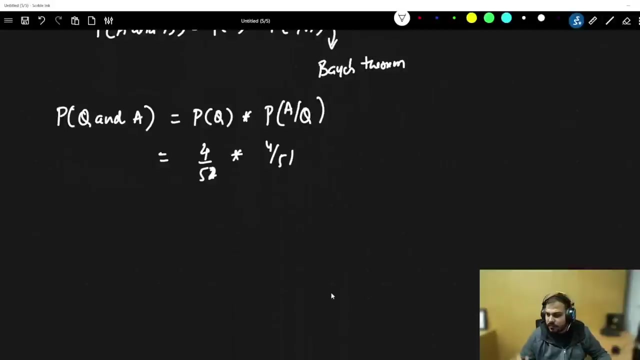 Probability Of Aces Given Queen. So What Is Probability Of Queen? It Is Nothing But Four By Fifty Two Multiplied By Four By Fifty One. 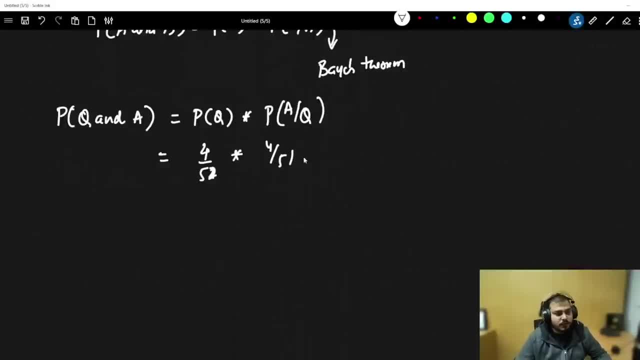 So Sorry, Fifty Three. So This Is Your Answer. You Get Over Here. This Is Basically Your. Now Let's Discuss About Something Called As Permutation. 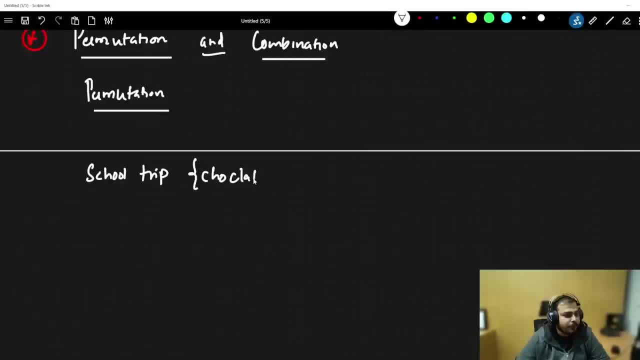 And Combination- A Very Small Topic Probably In The World. They Create Lot Of Chocolates, They Okay, So They, They Make A Lot Of Chocolates. 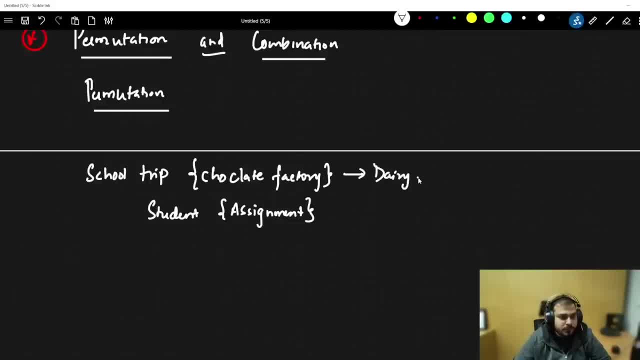 Okay. So I Catch A World Of A Student And I Say How Many? One, Two, Three, Four, Five And One More Chocolate, Normal Toffee. 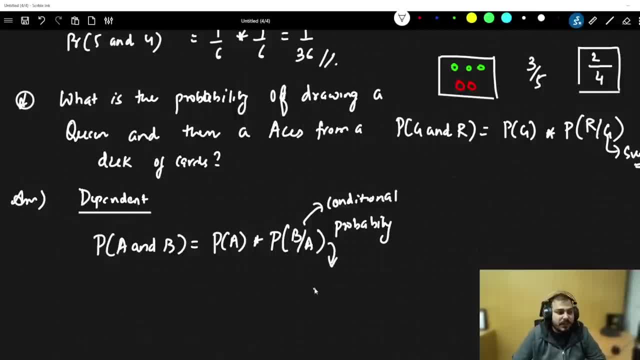 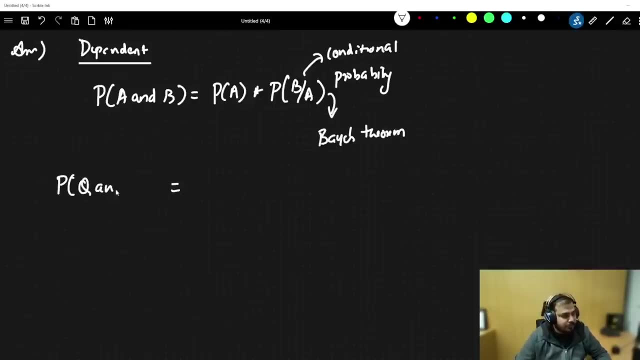 This is called as conditional probability, And this is very, very helpful in something called as naive bias, or I will also say it as bias theorem In bias theorem. this will be very, very important. So here, what is probability of king? sorry, it is queen and king, right. 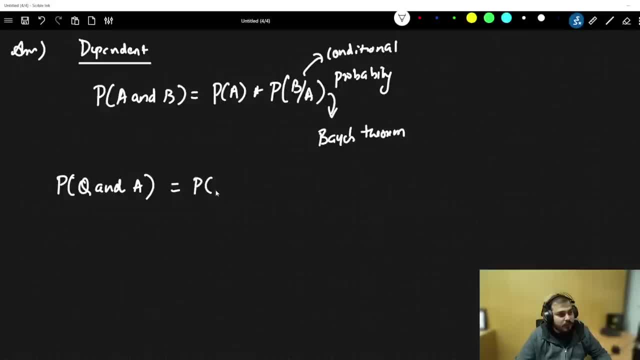 Queen and aces. sorry. So here what I will do: Probability of queen multiplied by probability of aces, given queen. So what is probability of queen? It is nothing but four by four, Right Four by fifty-two multiplied by four by fifty-one. 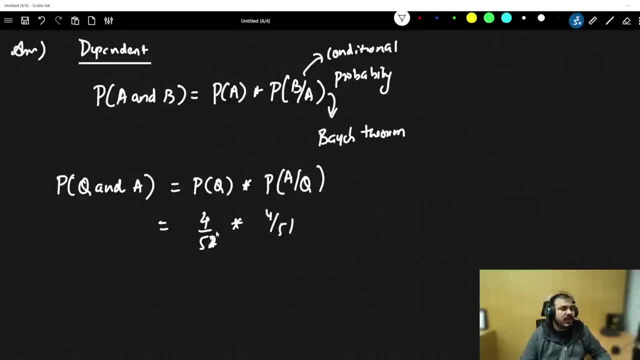 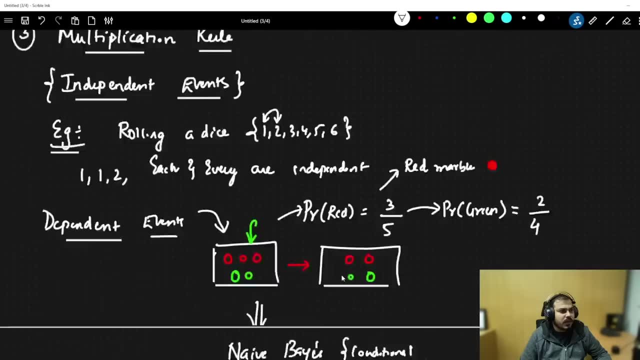 So sorry. fifty-three, how many cards are there? I forgot How many cards will be there in the deck. Fifty-three: right, Where is it? Where is it? No, fifty-two only, Do not confuse me guys. 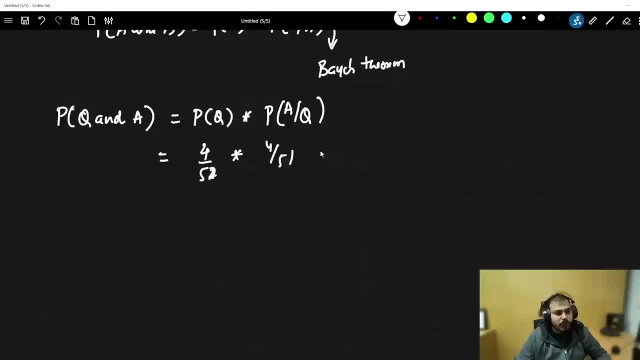 Okay, Four by fifty-two multiplied by four by fifty-one. So whatever answer you get over here, this is basically your answer. Now let us discuss about something called as permutation and combination. Okay, This is another topic. Probably in five minutes I will be able to complete it. 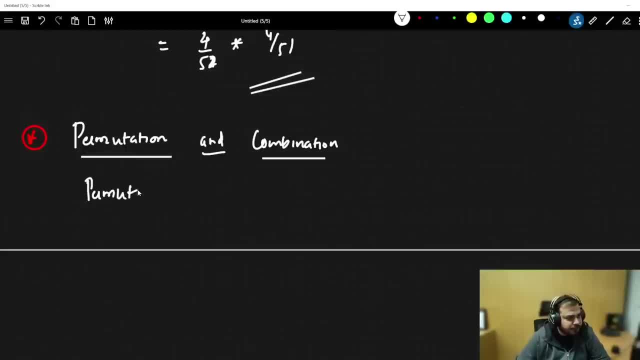 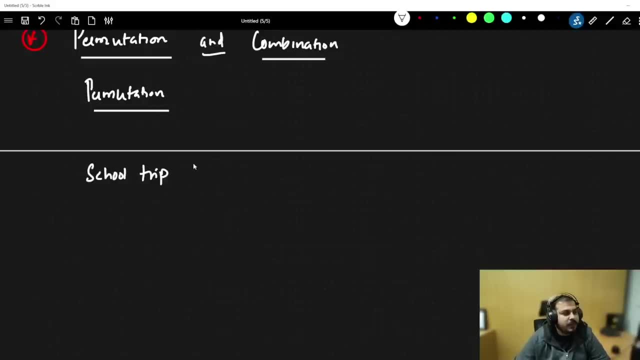 Now let us say that, first of all, let us discuss about permutation. Let us say that I have taken some students to a school trip and then we have gone to something like a chocolate factory in which many chocolates are basically, they create lot of chocolates. they okay, so they make a lot of chocolates. 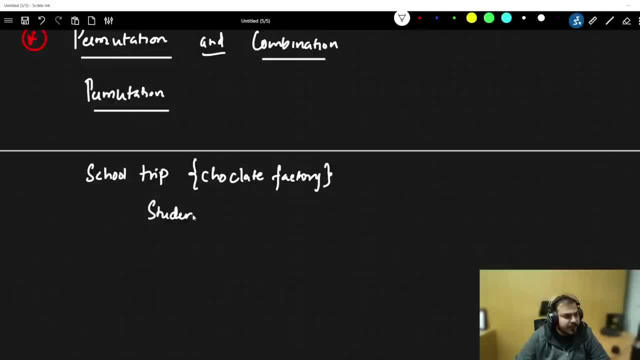 Okay, So I catch hold of a student, Okay. So let us say that, okay, I will give you an assignment. and let us say that, in this chocolate factory, six different types of chocolates are created, like dairy milk right, Like five star, milky bar, and let us say eclairs. okay, jam, how many? one, two, three, four. 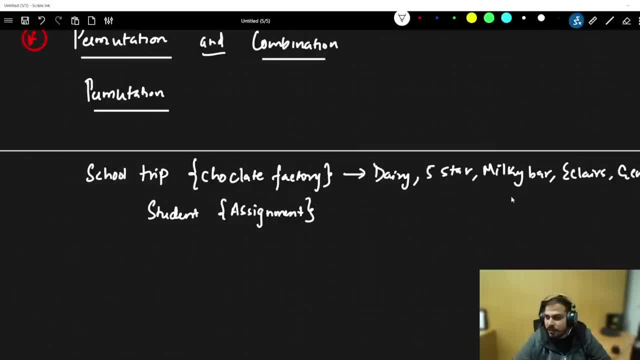 five and one more chocolate, normal toffee. let us say one more category: silk of dairy milk is there? How many chocolates are basically there? So I have given a student an assignment to that, saying that, okay, there are six chocolates that are getting created in this factory. 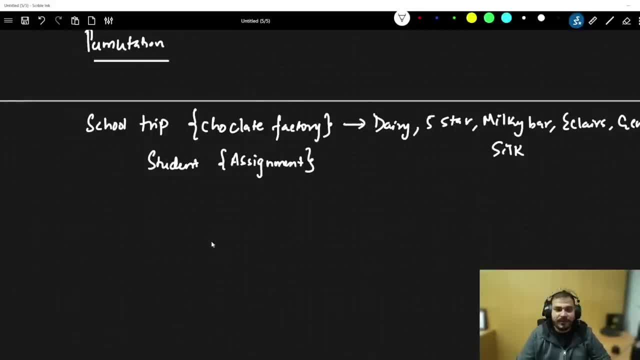 Let's Say One More Category: Silk Of Dairy Milk Is There. So These Many Chocolates Are Chocolates. Whichever Chocolate, You Probably See The 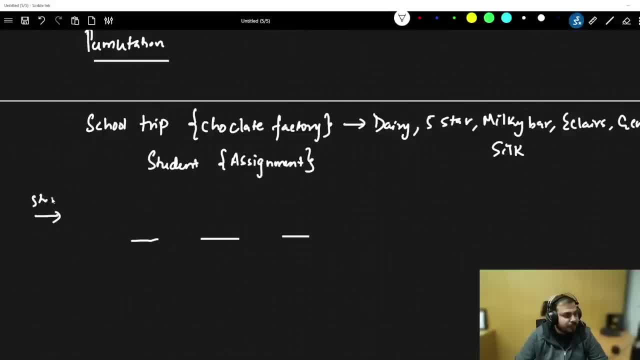 Top Three, The First Three. You Just Write That Name And You Come Up. Come Back To So That Student Went Inside Six Different To Any. 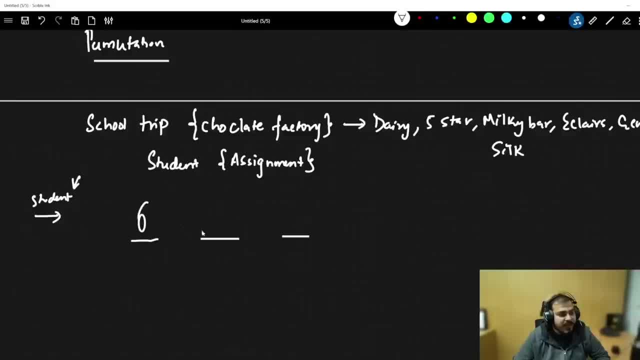 Any Chocolate He May See Right. So Obviously, He May Have Six Options, Out Of Which He Writes One Name Over Here. Let's Say In: 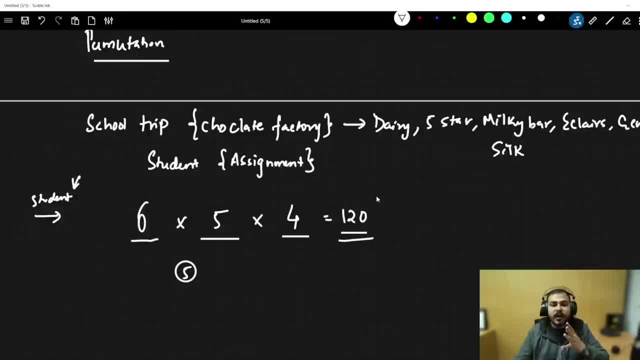 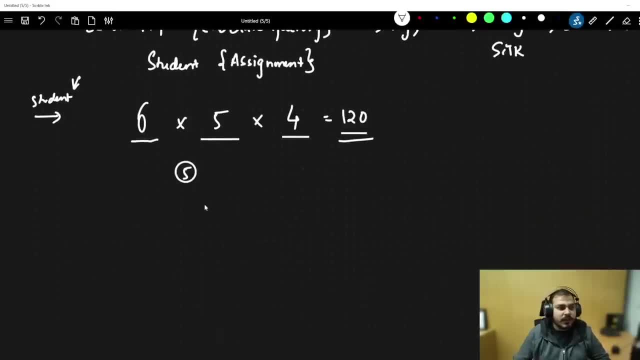 One Twenty, Now One Twenty What It Is. It Is All The Possible Permutations With Respect To The Chocolate Name That He May See All. 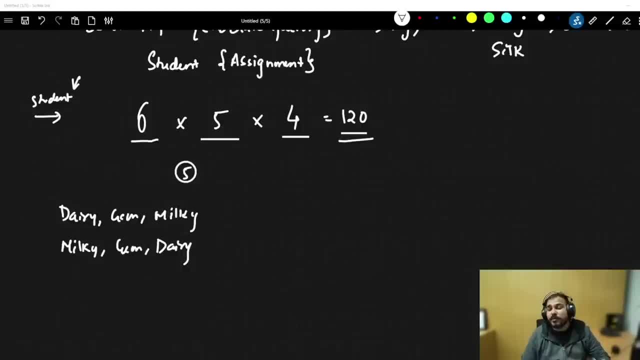 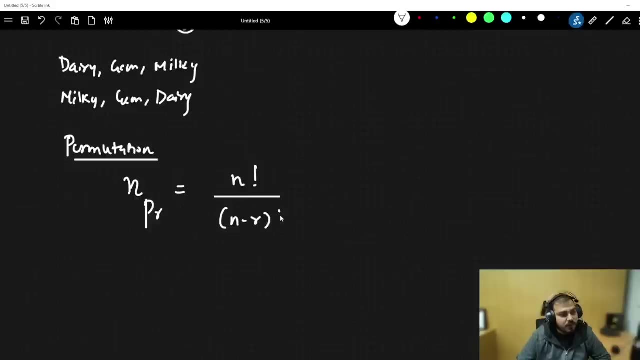 The Possible Permutations Like This. Now, This Is What Permutation Is Permutation Formula? How Do You Write? Now Let's Go Back To School Days. 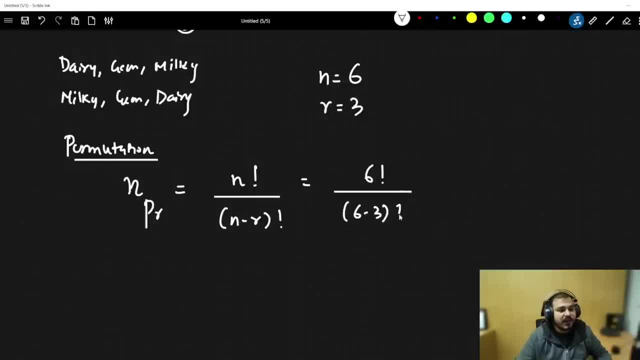 We Are Directly Used To Ratify All The Formulas. This And This Will Get Cut. The Total Answer Is 120.. This Is With Respect. 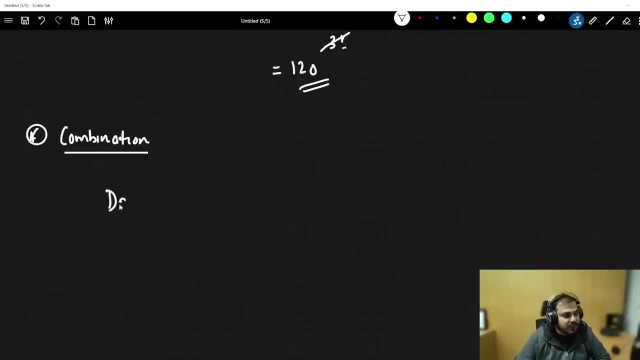 To Permutation. Now, How Does Combination Come Into Existence And What Is The Difference Between The Formulas And The Formulas? So Combination Will Be. 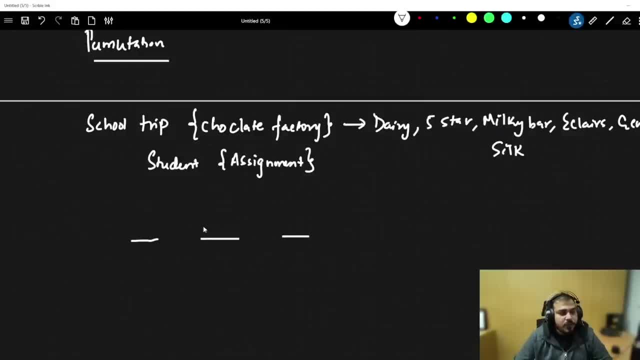 Let us create: in your diary you write the first three chocolates, whichever you see. Whichever chocolates you see once you enter into that factory, whichever chocolate, you probably see the top three, the first three. you just write that name and you come up. 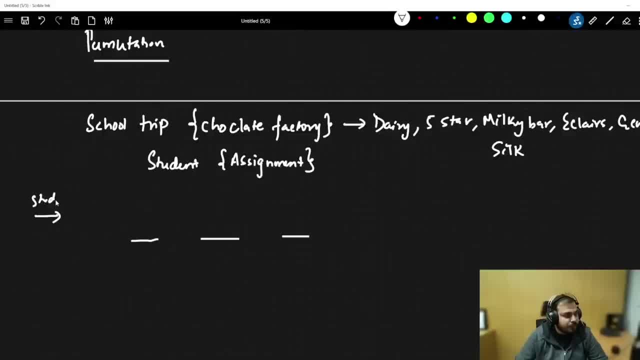 come back to me, Okay, Okay, This is the factory. Now, in the first instance, how many different options this particular student can have of seeing the chocolates? He may definitely have six different options, Now once he sees, probably any one chocolate, right. 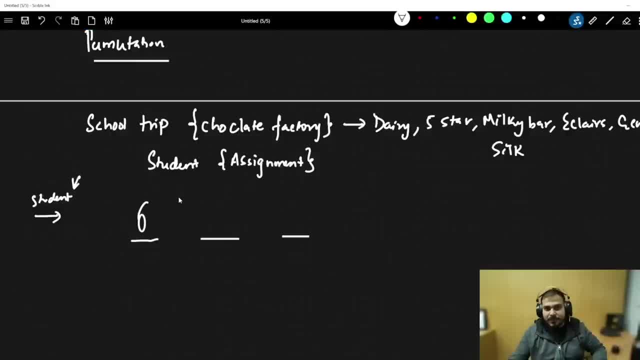 He may have six options, because six different, any, any chocolate he may see, right? So obviously he may have six options, out of which he writes one name over here. Let us say in the next instance how many chocolates will remain. Okay. 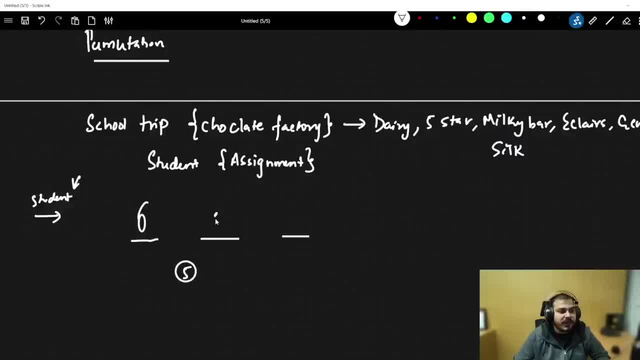 Total five will remain. So how many options he will have to write the name? five: he'll have the right to write the name of the chocolate. Then, finally, here you'll be seeing that when he comes and write the third name over there, they'll be having four options. 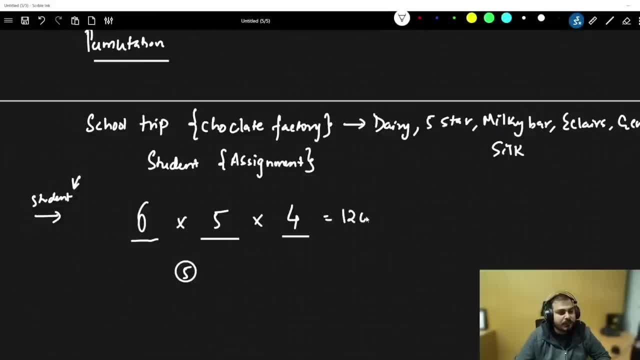 Now, if I try to multiply this, six multiplied by five, multiplied by four, it is nothing but 120.. Now, 120, what it is, it is all the possible permutations with respect to the chocolate name that he may see, All the possible permutations. 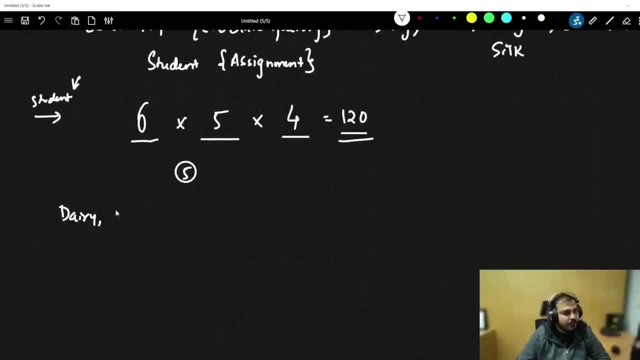 Like he may, he may see. He may see in this way: dairy milk gems, milky bar. He may also see in different way: milky bar, gem dairy milk. So all the possible options that are possible is 120.. 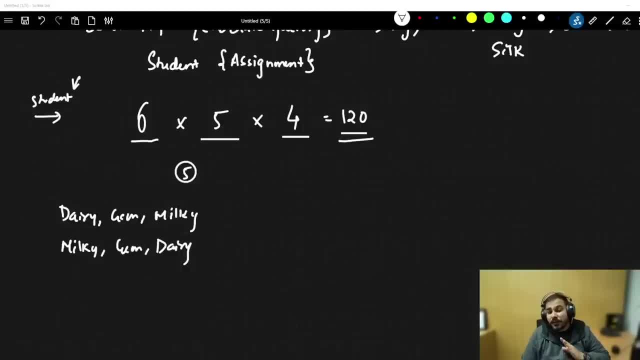 Now when I say 120, okay, these are all the possible options. Now this is what permutation is Permutation formula? How do you write it? Now let's go back to school days. We're directly used to ratify all the formulas. 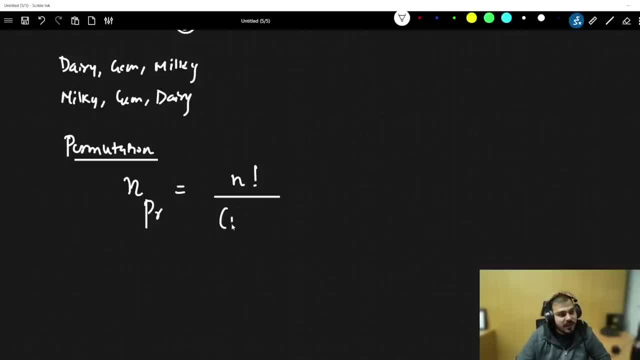 NPR is equal to N factorial divided by four. Okay, Okay, Six. factorial divided by N minus R. factorial Where N is nothing but the total number of chocolates, R is nothing but how many names I have told that person to write. So here you'll be seeing six factorial divided by six minus three. factorial which is nothing. 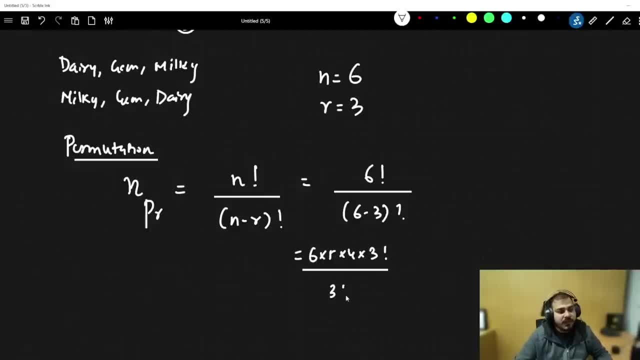 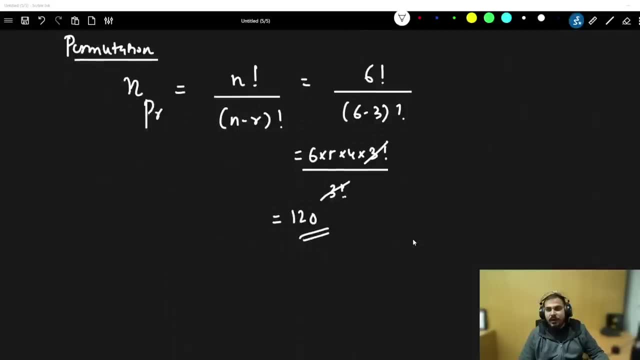 but six into. multiplied by four, multiply by three factorial, divided by three factorial, This and this will get cut, So the total answer is 120.. This is with respect to permutation. Now, how does combination come into existence now, And what is the difference between permutation and combination? 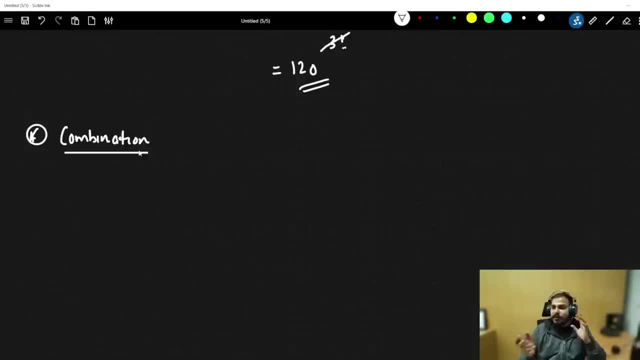 permutation and combination. Now, in combination always understand permutation. if I have the same element like this: I have dairy milk, I have gems, I have probably eclairs. If I have used this element once, this combination, I cannot use this same element and probably make a different. 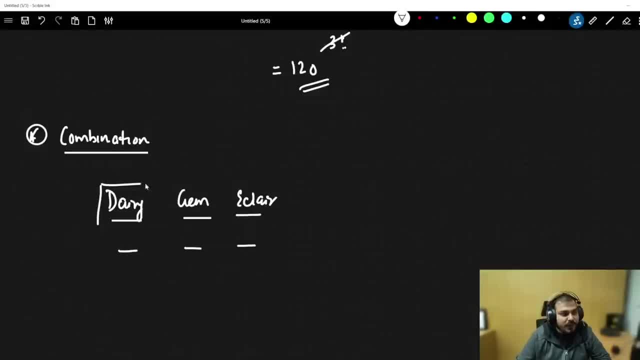 combination. So combination will be unique with respect to the elements that is used. Okay, If I have used dairy milk, gem and eclair, I cannot again reswap it and make it as a different order. So in the case of combination, you have a other formula which will actually help you to. 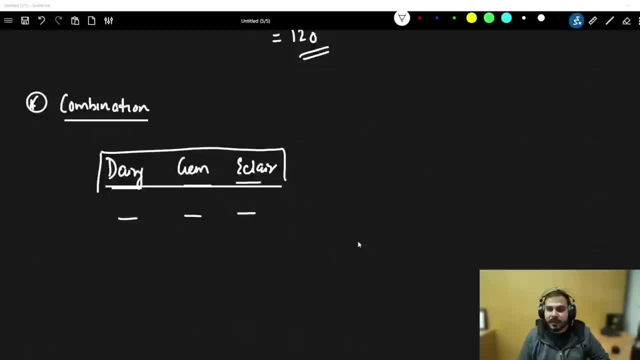 focus on the uniqueness of the objects that you are picking up. So for this, the formula is nCr, which is nothing but n factorial divided by r factorial, n minus r factorial. What is n factorial? You know that There is 6 factorial. What is? 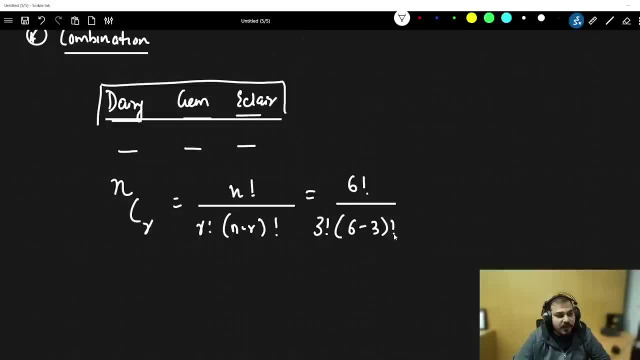 r factorial, 3 factorial and 6 minus 3 factorial. So here you will basically say 5 move 4, and this will be divided by 3 factorial. This I will make it as 3, 2, 1 multiplied by 3 factorial. 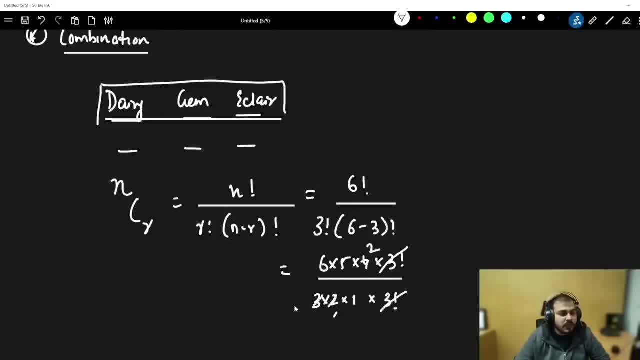 This and this will get cut: 2- 1s are 2, 2s are 3, 1s are 3, 2s are 5, 2s are 10, 10- 2s are 20.. So 20 unique combinations you can basically have. Let's say first of all the first topic. 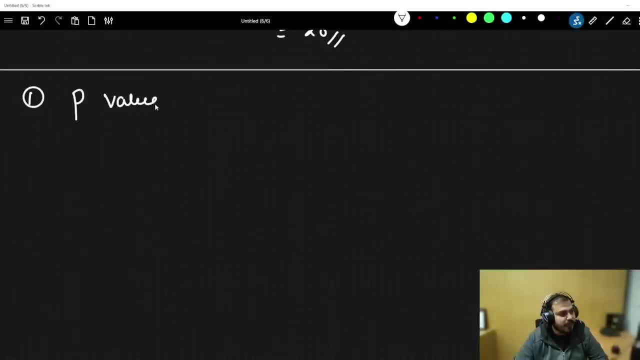 that we are probably going to discuss about is something called as permutation. So permutation is a super, super important topic. Many people get confused. Now let's take one example. Everybody uses a laptop. Let's say that this is my laptop, This is my mousepad, This is. 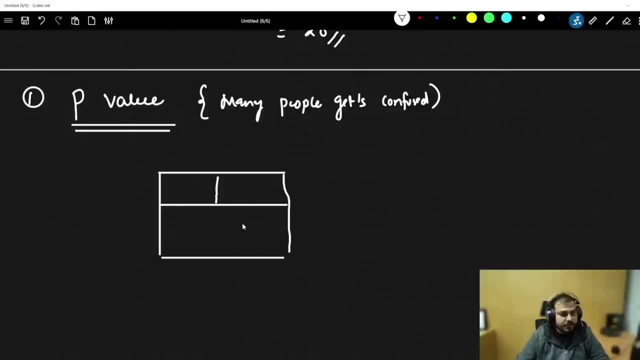 your right button to click. This is your left button to click Your laptop mousepad. over here you will move the fingers. Let's go ahead and let's understand, Don't you think most of the time when you are moving your fingers you will be moving in this specific region? 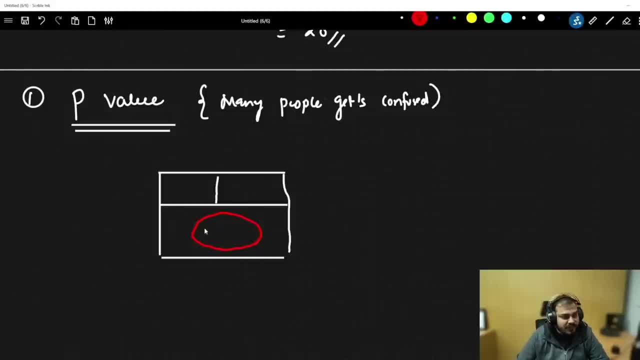 In this specific region. You will be moving your fingers in this specific region, not in the corner. Hardly you will touch somewhere in the corner. Now why I am specifically drawing this? Because this thing will basically specify your distribution of touches And most of 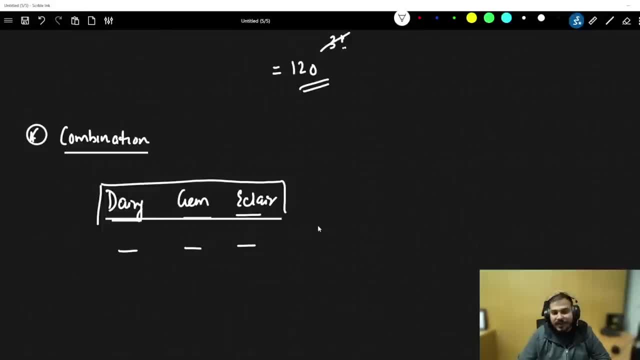 Unique With Respect To The Elements That Is Used. Okay, If I Have Used Dairy Milk, Gem And Eclair, Which Is Nothing But N Factorial, 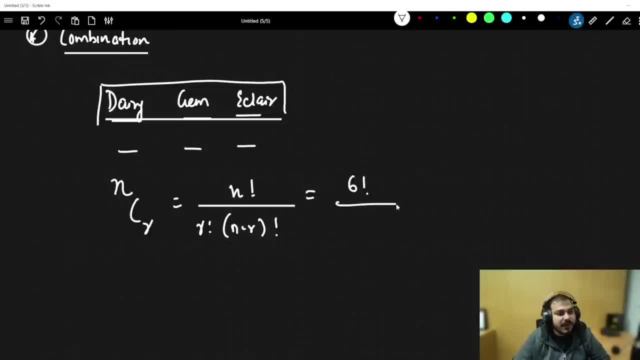 Divided By R Factorial: N Minus R Factorial, What Is N Factorial? You Know That, The Six Factorial, What Is R Factorial? 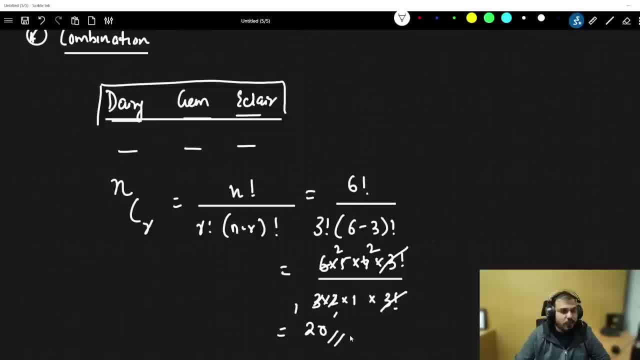 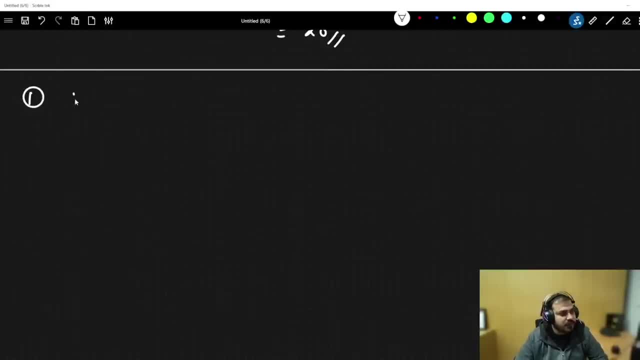 Three Things That You Need To Have. Let's Say First Of All, The First Topic That We Are Probably Going To Discuss About Is Something 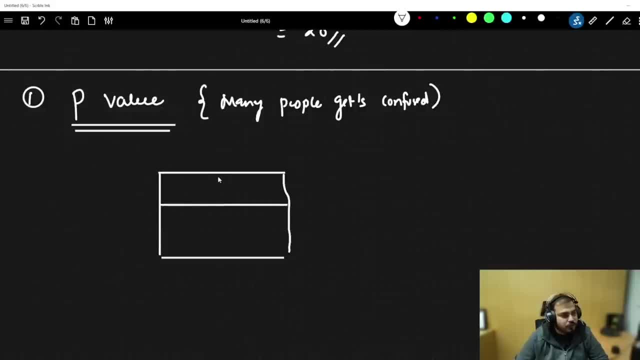 Called As P Value. Super Right Button To Click. This Is Your Left Button To Click Your Laptop Mousepad. Over Here You Will Move The. 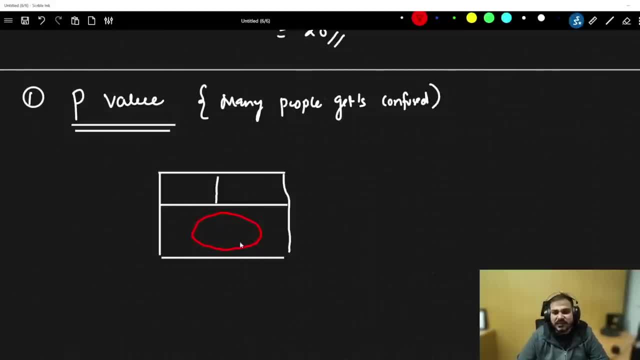 Fingers. Right Here You Will Move The Fingers. Let's Now, Now, Let's Consider That I Say My P Value For This Position Is My. 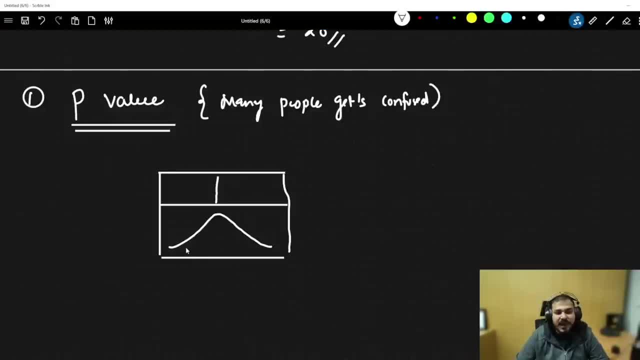 P Value For This Position Is Point Eight. Now Here My P Value For here what I am actually going to do. what does this 0.8 basically means that let's say I am doing hundred times, I am touching this mouse pad hundred times. I. 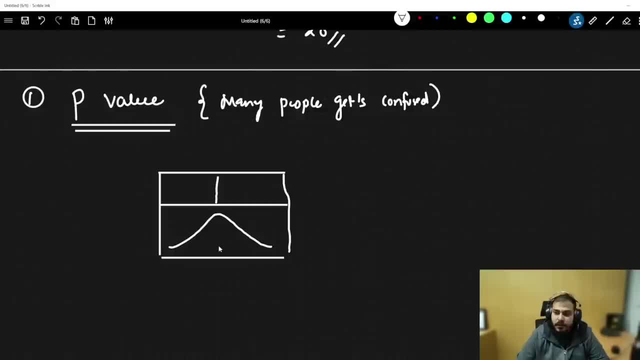 the time, your distribution of touches will be also looking something like this: Now understand one thing: Why this area is bulged. This area is bulged because most of the time, most of the times you will be touching here, This area is less because, over here, hardly you 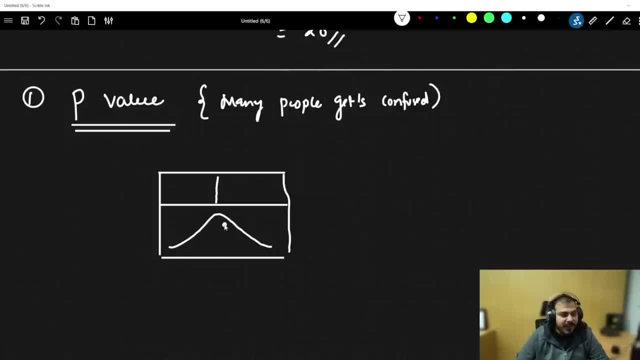 will be touching over here. Now let's consider that I say my p-value for this position is. my p-value for this position is 0.8.. Now here what I am actually going to do. what does this? 0.8 basically means that Let's say I am doing hundred times, I am touching this. 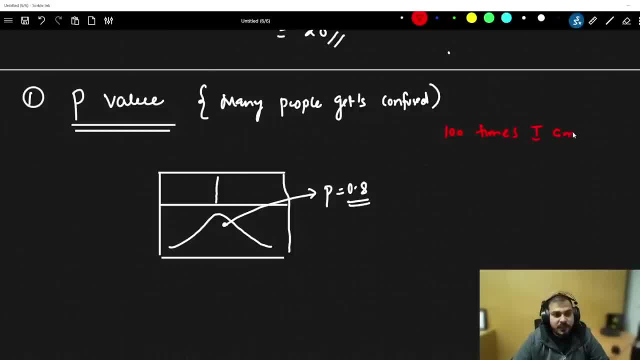 mousepad. Hundred times I am touching. Now let's say that every hundred times. every hundred times. let's, let's remove this. I will write in white color only Every hundred times I touch the mousepad. eighty times out of this hundred. 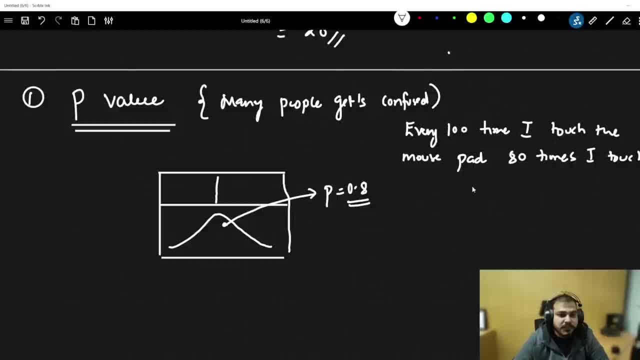 eighty times I touch this specific region. I hope everybody understood this one. Every hundred times probably, I touch this mousepad. The probability of touching this region is eighty times. That is eighty percentage. Similarly, if I say my p-value over here is 0.01.. What does? 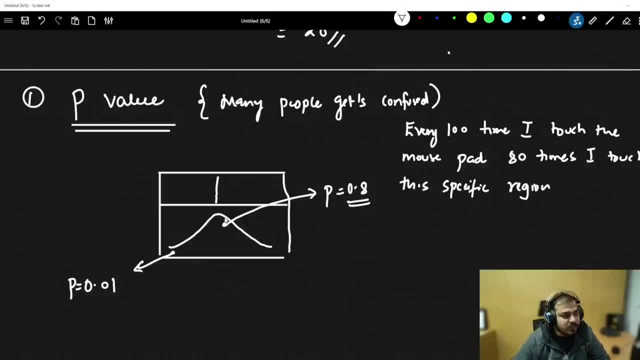 this mean. Similarly, you can consider any region. This region is the tippest like broadest right, So this region may be. p is equal to 0.9.. That basically means out of every hundred touches, I am basically touching ninety times over here. This will be one time This will. 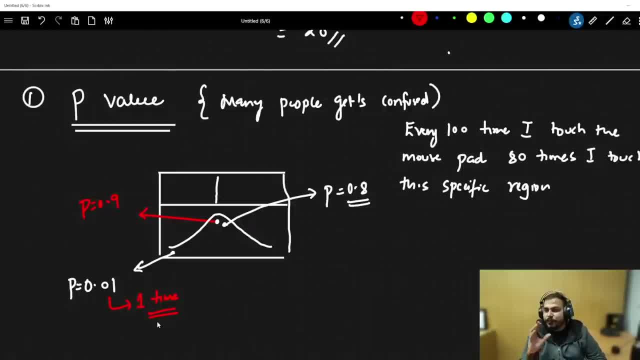 be only one time. So I hope you are getting the understanding Of p-value. P-value basically says most of the time. what is the probability with respect to a p-value for that specific experiment? Now let's go ahead and let's understand something. 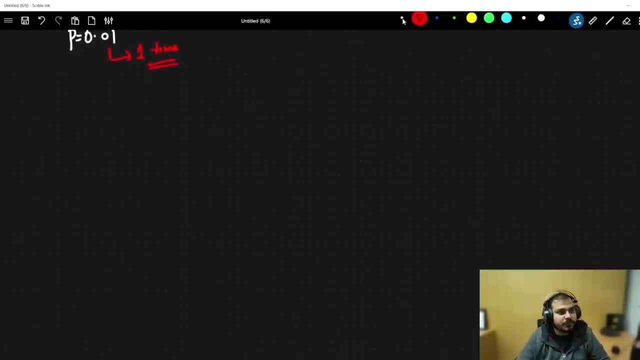 called as now, I am going to combine multiple topics. The first topic that I am going to combine is something called as hypothesis testing, In that I am going to combine confidence interval, In that I am going to combine significance value, In that I am going to combine many things. 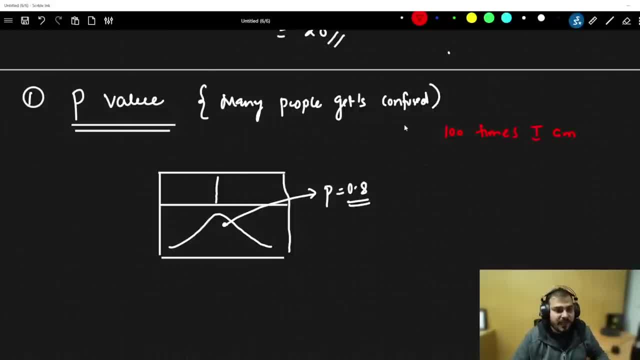 am touching. let's say that every hundred times. every hundred times, let's, let's remove this. I'll write in white color only: every hundred time I touch the mouse pad. 80 times out of this. hundred eighty times I touch this specific region. I hope everybody understood this one. every hundred times probably, I touch 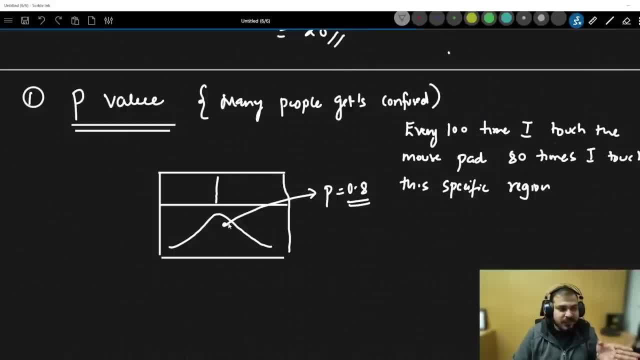 this mouse pad, the probability of touching this region is 80 times, that is, 80 percentage. similarly, if I say my p-value over here is point zero one, what does this mean? similarly, you can consider any region: this region is the tippest like broadest right, so this region may. 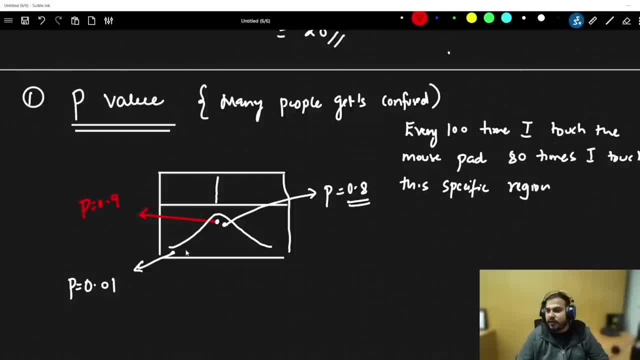 be p is equal to 0.9. that basically means out of every hundred touches, I am basically touching 90 times over here. this will be one time. this will be only one time. so I hope you are getting the understanding of p-value. p-value basically says most of the time what is the probability with respect to a p-value. 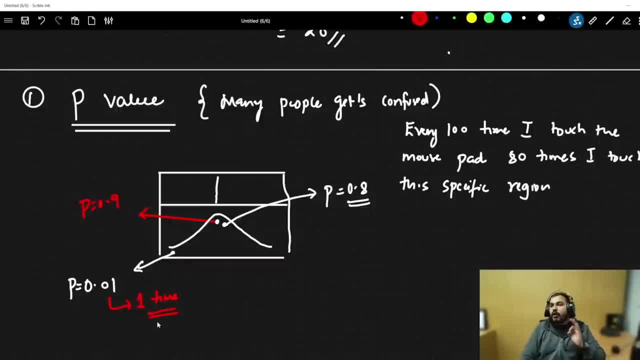 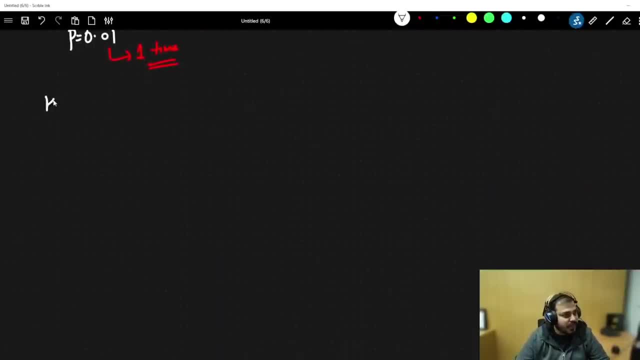 for that specific experience. now let's go ahead and let's understand the probability of touching this specific region. and let's go ahead and let's understand something called as. now I'm going to combine multiple topics. the first topic that I am going to combine is something called as hypothesis. 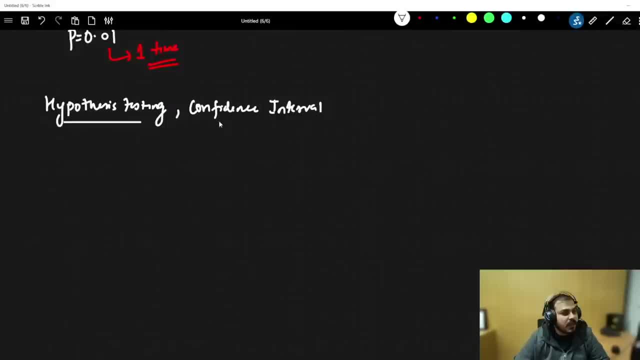 testing, in that I am going to combine confidence interval, in that I am going to combine significance value, in that I am going to combine many things. okay, let's say I am solving a problem. okay, my problem is to. I have a coin. I want to test whether this coin is a fair or a. 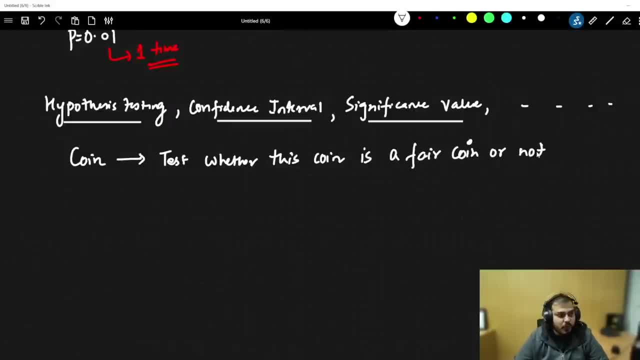 fair coin or not? simple problem statement. I have a coin. I want to test whether this coin is a fair coin or not by performing hundred tosses. now we are entering into inferential statistics. okay, very important, super important. when do you think a coin is a fair coin? obviously, when the probability of heads 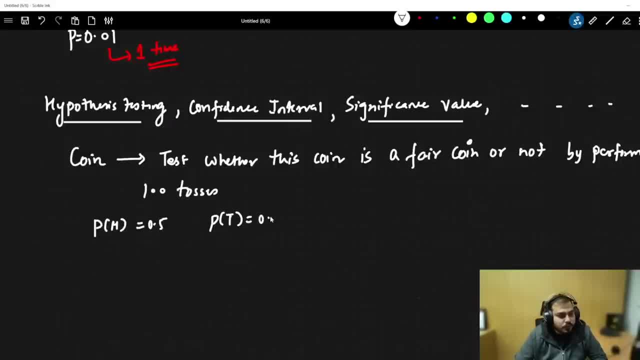 should be 0.5, when the probability of tail should be 0.5. if you have this two condition, definitely you will be saying that yes, in this particular scenario, obviously the coin will be a fair coin. but if you have a shollay coin, if you have a 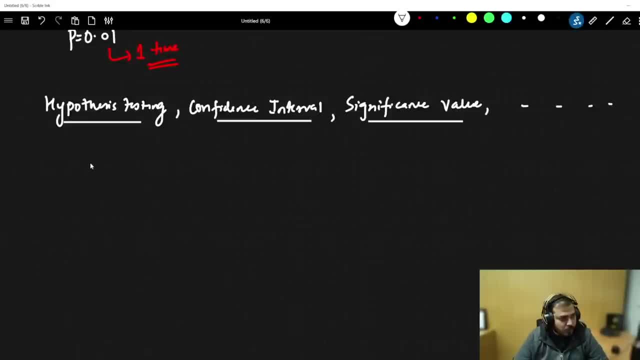 Okay, Let's say I am solving a problem. Okay, My problem is to: I have a coin. I want to test whether this coin is a fair coin or not. Simple problem statement: I have a coin. I want to test whether this coin is a fair coin or not by performing hundred touches. Now we are. 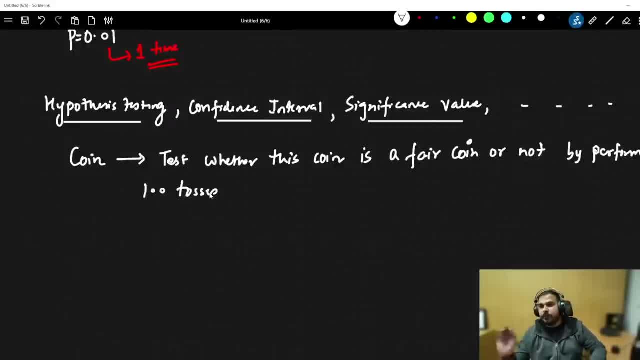 entering into inferential statistics. Okay, Very important, Super important. When do you think a coin is a fair coin? Obviously, when the probability of heads should be 0.5, when the probability of tail should be 0.5.. If you have this two condition, definitely you. 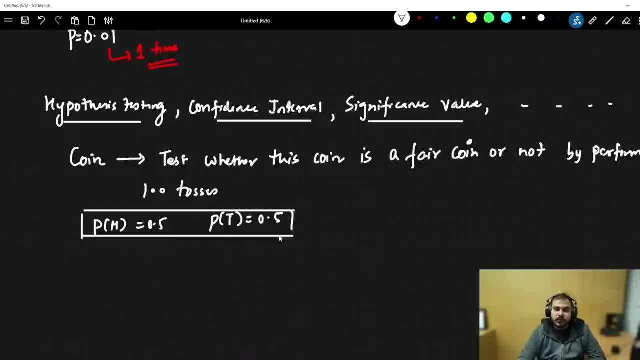 will be saying that yes, in this particular scenario, obviously the coin will be a fair coin, But if you have a shoal coin, if you have a shoal coin, then what will happen? If you have a shoal coin, then probability of heads. 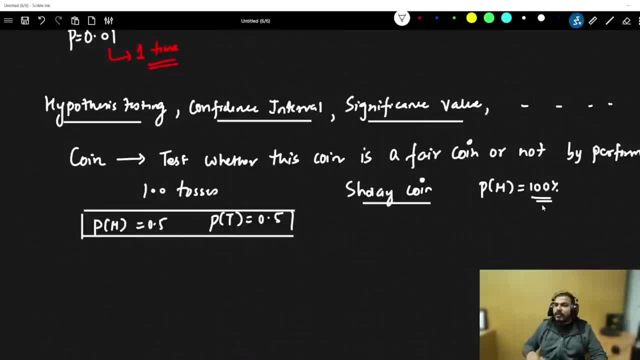 Okay, hundred percent. so for this kind of things, you'll definitely not say that it is a fair coin. now, in order to support this, i am performing hundred experiments. hundred experiment basically means hundred tosses, so hundred tosses i will be performed now. inside this hundred tosses, what i 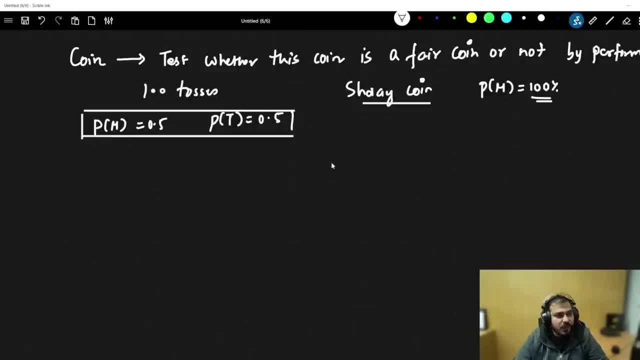 am going to do is that let's say that from this hundred tosses, obviously, what will be the mean? let's say that i'm just focusing on probability of head, i should basically get 50 times. so from this hundred times, from this hundred times, if i'm performing hundred experiment, i can definitely say: 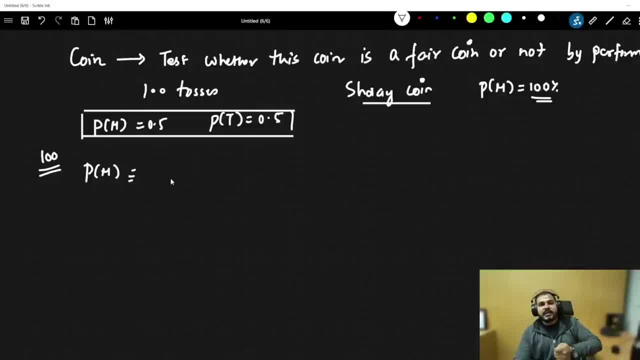 that my probability of head, or probably let's. let's consider that. forget about this probability of head. the number of times i should get head is how much? 50, right, if i get 50 times head, i can definitely say that this coin is. the coin is fair. the coin is fair. i can definitely say this. 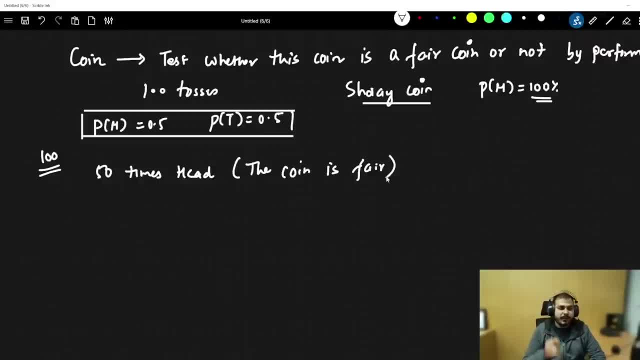 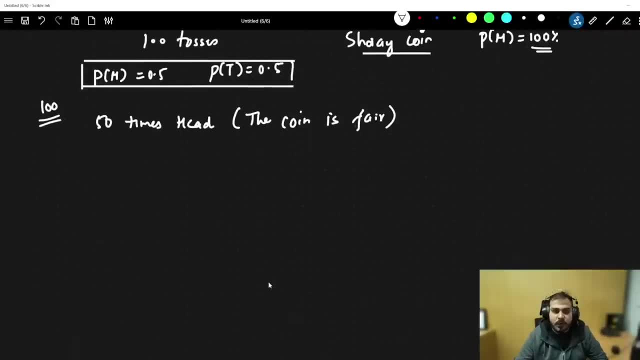 if the number of times after a performing hundred experiment. if i get 50 times head, i can definitely say the coin is fair. now very important. first of all, in this particular scenario, we have to focus on something called as hypothesis testing. you have to focus on hypothesis testing. in hypothesis testing, the first thing is: 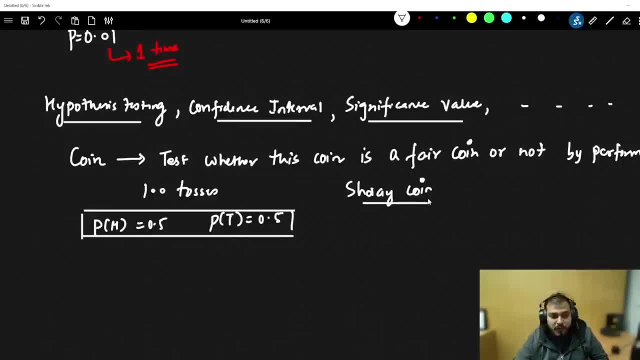 sholey coin, then what will happen if you have a sholey coin, then probability of heads was 100. so, for this point of things, you will definitely not say that it is a fair coin. now, in order to support this, I am performing 100 experiments. 100 experiment basically. 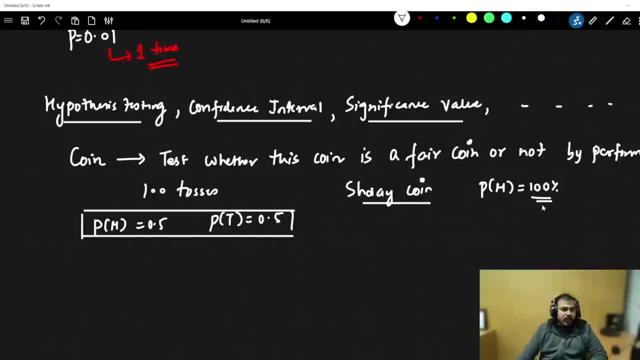 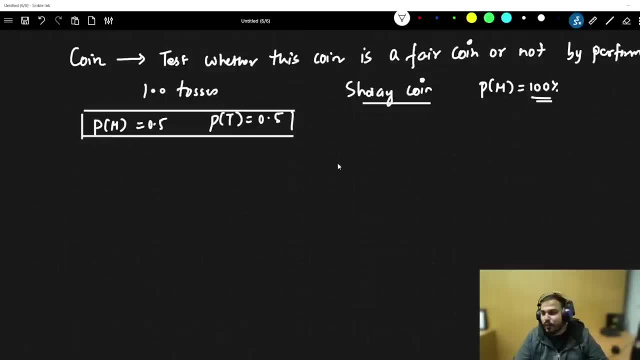 with tosses, So 100 tosses. I will be performing Now inside this 100 tosses. what I am going to do is that let's say that from this 100 tosses, obviously, what will be the mean? let's say that I am just 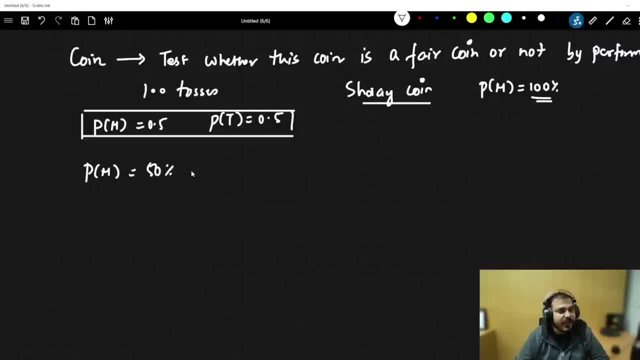 focusing on probability of head, I should basically get 50 times. So, from this 100 times, from this 100 times, if I am performing 100 experiment, I can definitely say that my probability of head, or probably let's- let's consider that, forget about this- probability of head, the number of 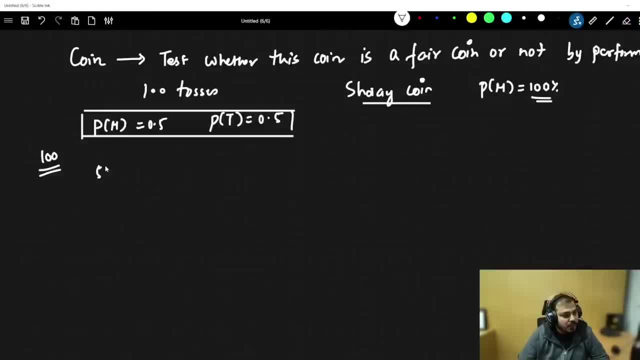 times I should get head is how much? 50 right. If I get 50 times head, I can definitely say that this coin is. the coin is fair. the coin is fair. I can definitely say this If the number of times after performing 100 experiment, if I get 50 times head, I can definitely say the coin is fair. Now, 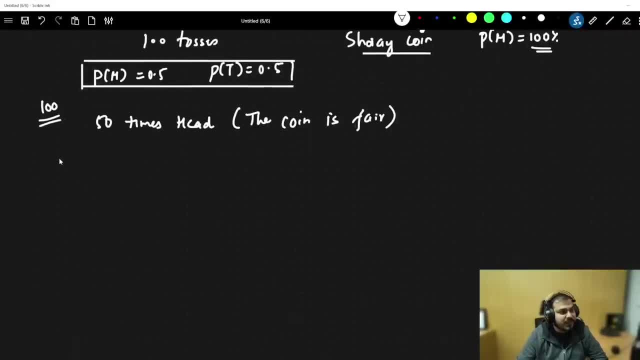 very important. first of all, in this particular scenario, we have to focus on something called hypothesis. You have to focus on hypothesis testing. In hypothesis testing, the first thing is that we need to define our null hypothesis. The null hypothesis is usually given in the problem. 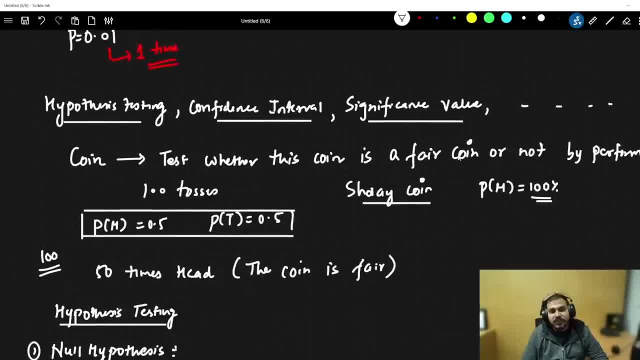 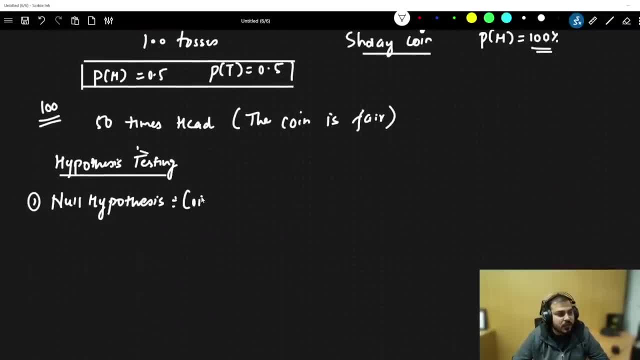 statement: What is? what is? we want to test whether the coin is a fair coin or not. So, whatever the default question is, I am going to use it as a null hypothesis. So here I am saying that the coin is fair. Like one scenario: you have a coin and you have a hypothesis. You have a hypothesis and you 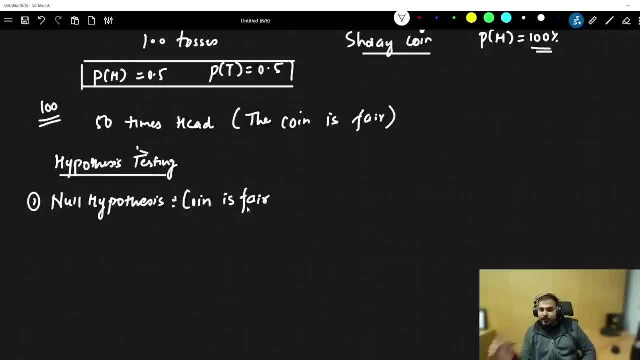 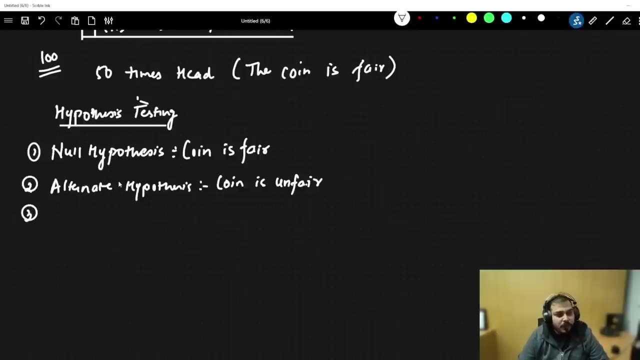 have a right. A person cannot be acquitted as a criminal unless and until it is proved. So the coin is fair. Now the second thing that we basically define is something called as alternate hypothesis. Here I will say: the coin is unfair. Now the third step, and always remember: alternate hypothesis will. 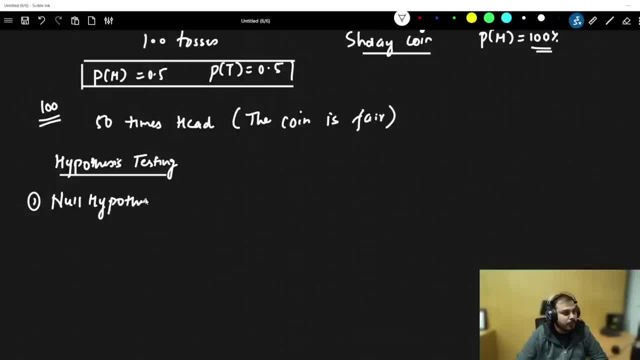 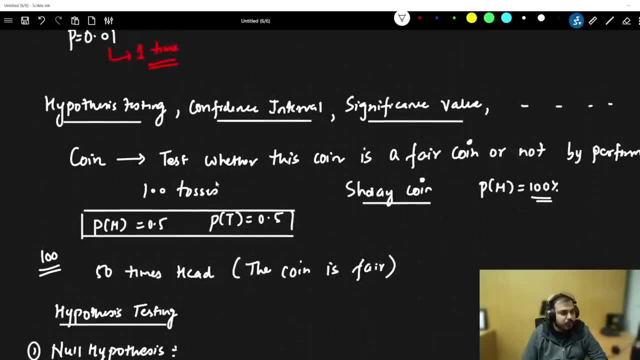 that we need to define our null hypothesis. the null hypothesis is usually given in the problem statement. what is, what is the null hypothesis? the null hypothesis is usually given in the problem statement. what is, what is? we want to test whether the coin is a fair coin or not. so, whatever, the default question is: 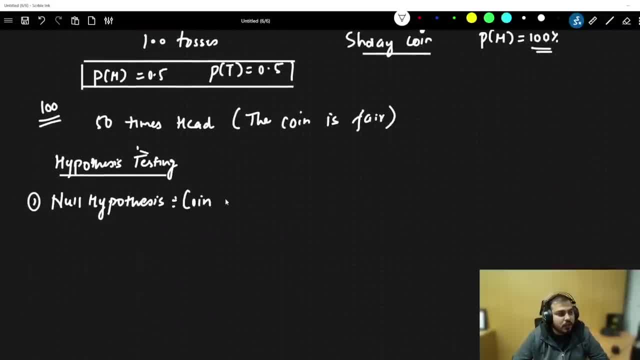 i'm going to use it as a null hypothesis. so here i'm saying that the coin is fair, like one scenario. you have right, a person cannot be acquitted as a criminal unless and until it is proved. so the coin is fair. now, the second thing that we basically define is something: 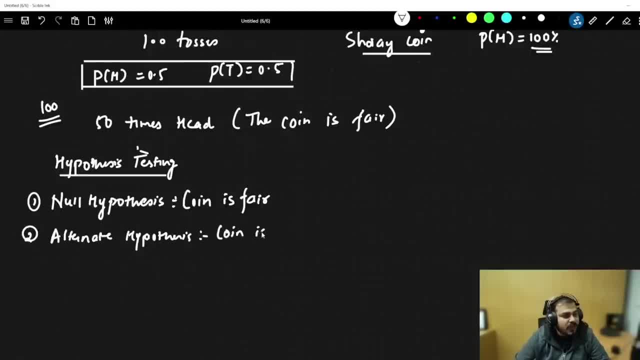 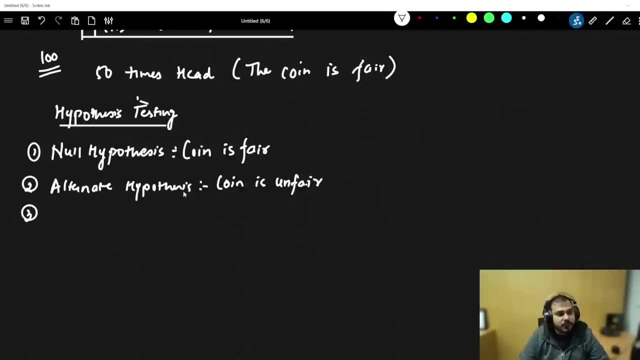 called as alternate hypothesis. here i'll say: the coin is unfair. now the third step, And always remember: alternate hypothesis will be the opposite of null hypothesis, whatever thing we are trying to put. okay. Now the third thing is that we perform the experiments. 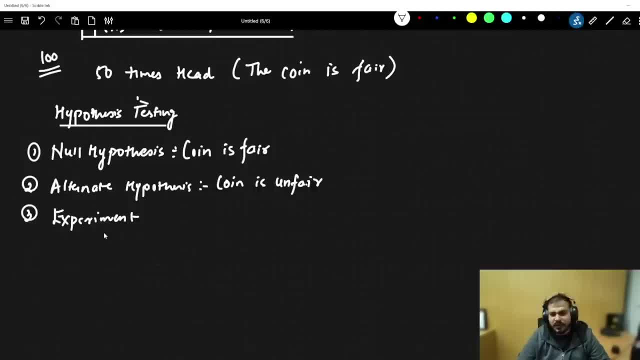 And the experiment can be anything. it can be a Z test, T test, whatever things you want. you can do All this practical. I will discuss it, don't worry. Now, inside this experiment, we see some values and, based on that, the fourth step that we 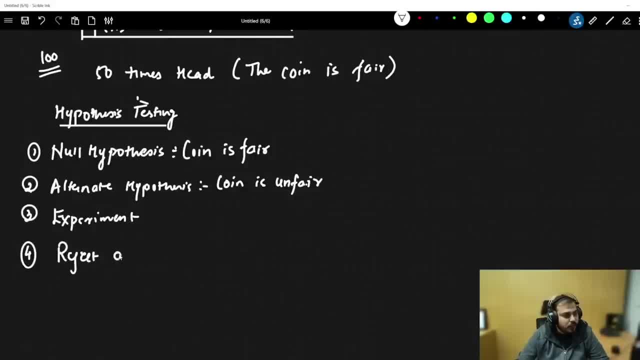 do we reject the null hypothesis Or accept the null hypothesis? null hypothesis- These are the possible steps of the hypothesis testing. Now let's define this guys. Let's say that my mean value is 50, I need to get at least 50 times head right. 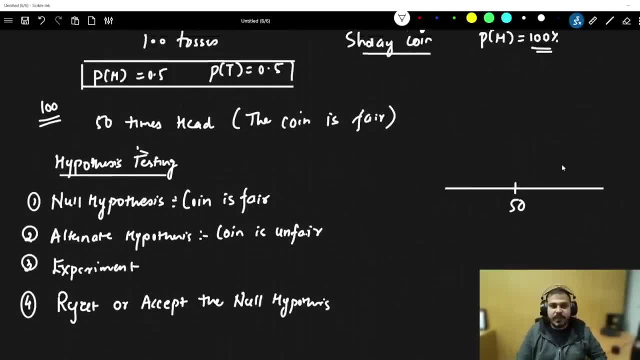 I need to get 50 times head, yes or no? Let's consider that this is my mean. okay, Minimum, 50, not minimum, but 50, 50 I should be getting. in order to say that my coin is fair. Let's say that. 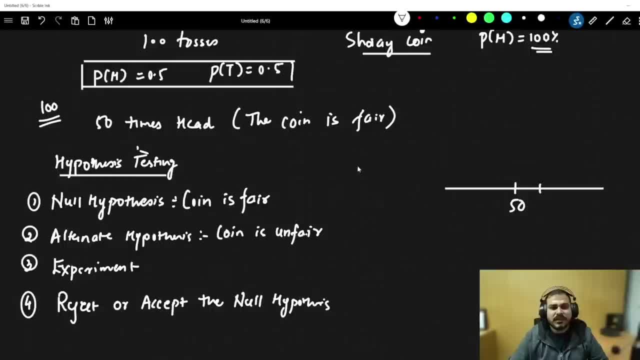 In this problem statement I am just examining. okay, The standard deviation is 10.. So it will come as 60,, 70,, 80,, 90,, 40,, 30,, 20,, 10,. okay, right. 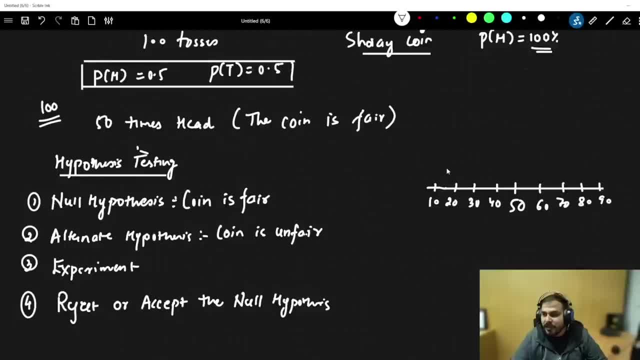 In this particular case it is there and probably, if I know my mean and standard deviation, I may draw a curve which looks like this: What happens? if I want to prove this Now see this. I will perform the experiment. Let's say I have performed 100 times. 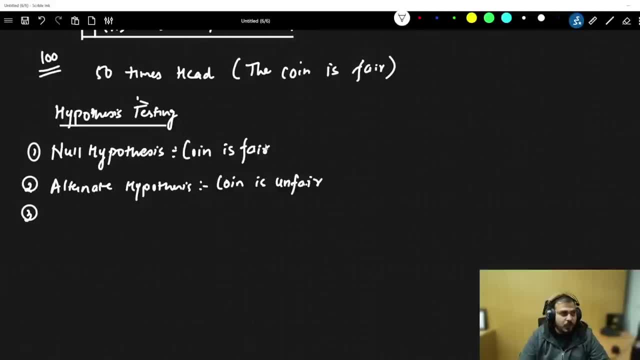 be the opposite of null hypothesis. Whatever thing we are trying to put Okay. Now the third thing is that we perform the experiments, and the experiment can be any kind of experiment, Anything. It can be a Z test, T test, Whatever things you want. you can do All this practical, I will. 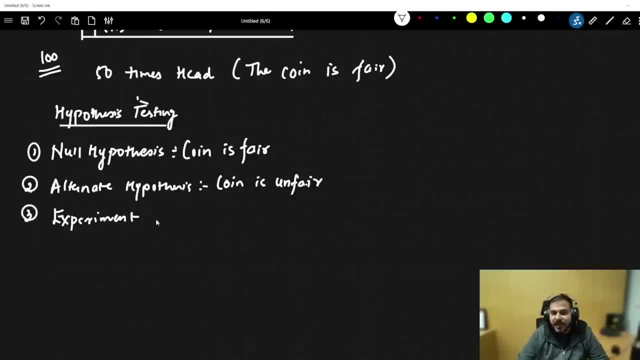 discuss it, Don't worry. Now, inside this experiment, we see some values and, based on that, the fourth step that we do: we reject or accept the null hypothesis, Null hypothesis. These are the possible step of the hypothesis testing. Now let's define this, guys. Let's say that my mean value is 50. I 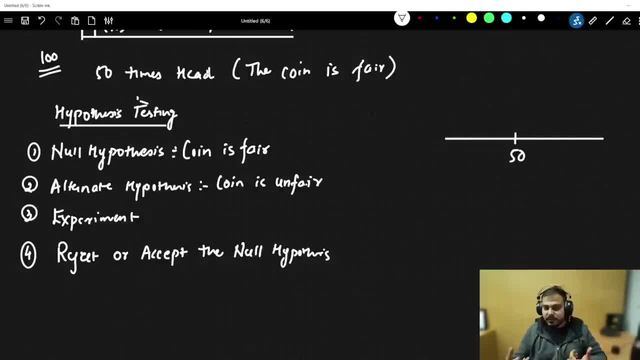 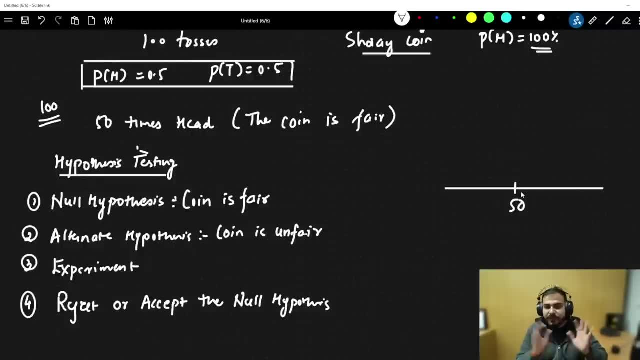 need to get at least 50 times head. right, I need to get 50 times head, Yes or no? Let's consider that this is my mean. Okay, Minimum, 50. Not minimum, but 50. 50 I should be getting in order to say that. 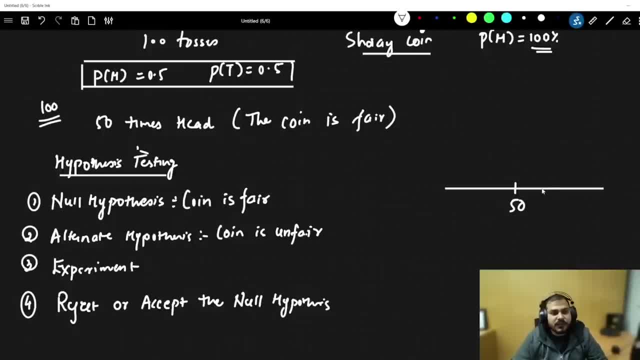 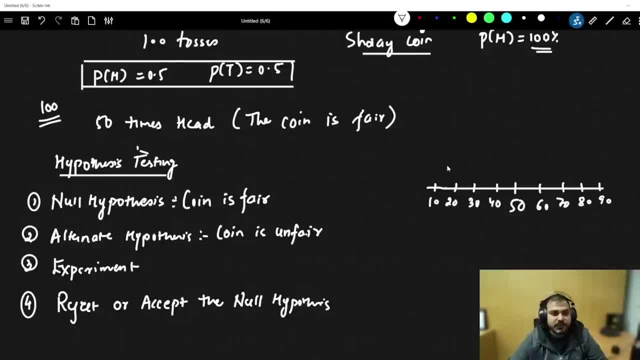 10. Okay, Right, In this particular case it is there and probably, if I know my mean and standard deviation, I may draw a curve which looks like this: What happens? if I want to prove this Now see this. I will perform the experiment. Let's say I have performed 100 times. Now just imagine. 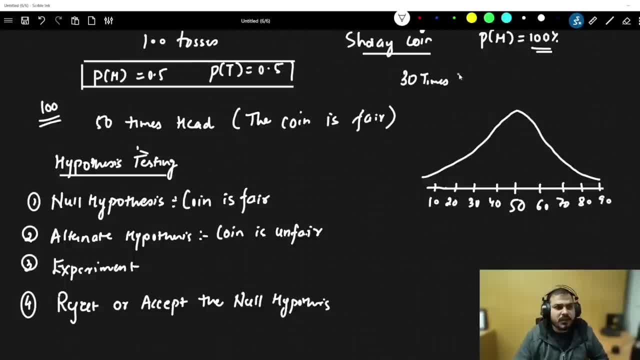 I got 30 times head. Let's imagine I got 30 times head. 30 times head is nothing, but it is somewhere. at this point Can I still say that this coin is fair or not? Can I say the coin is fair or not Or coin is unfair? Can I say: Think over it If I am getting? 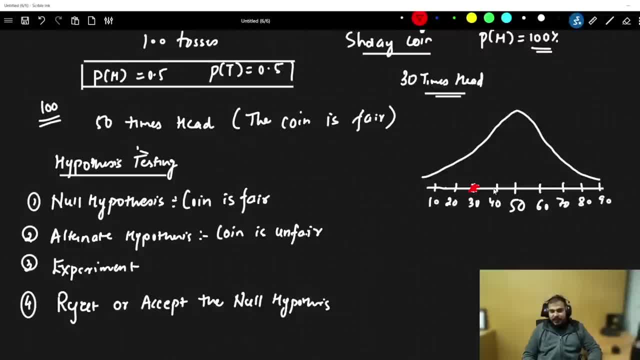 30 times head. Can I say that this coil is unfair? You tell me whether it should be fair or unfair. Tell me. Let's say that I have performed the experiment and I got 30 times head out of 100. So tell me whether this will be fair or no. Many people are saying no, not fair, fair. 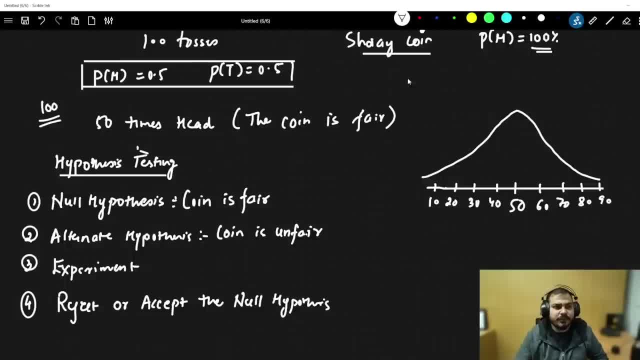 Now just imagine I got 30 times head. Let's imagine I got 30 times head. 30 times head is nothing, but it is somewhere. at this point Can I still say that this coin is fair or not? Can I say the coin is fair or not, or coin is unfair? 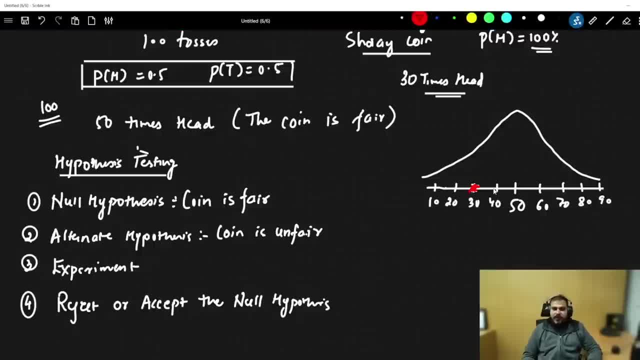 Can I say: Think over it. If I am getting 30 times head, Can I say that this coil is unfair? You tell me whether it should be fair or unfair. Tell me. Let's say that I have performed the experiment and I got 30 times head out of 100. 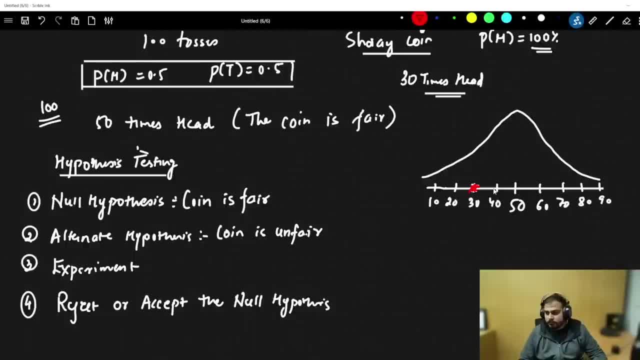 So tell me whether this will be fair or no. Many people are saying no, not fair, fair, fair, not fair. So for this to define, it is always said that Our experiment should be nearer to the mean. nearer to the mean. 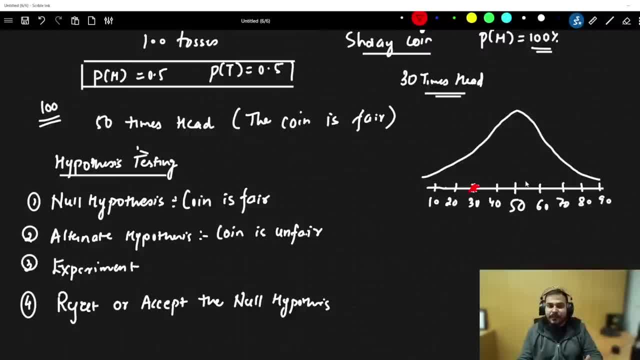 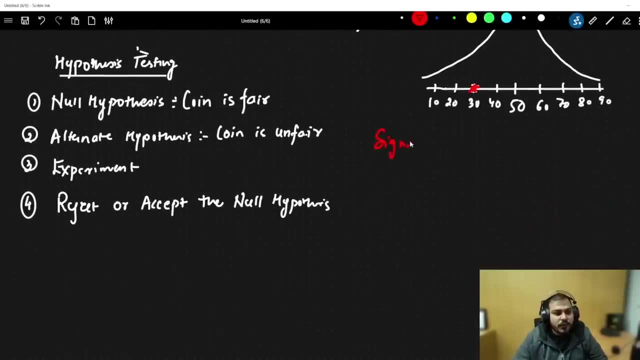 Now, how do we define that? how far it can be away from the mean. We need to define that, how far it may be away from the mean. So for that we use a very important property, which is called as significance value. Now, this significance value is basically given by alpha. 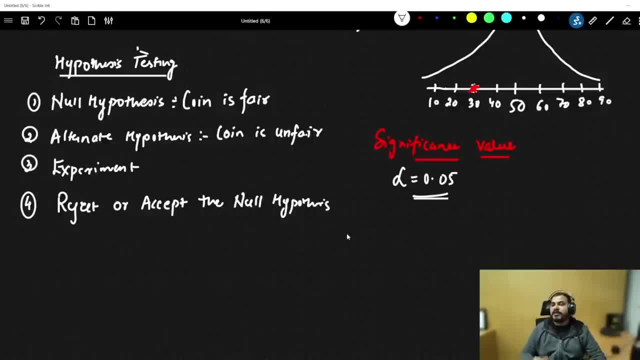 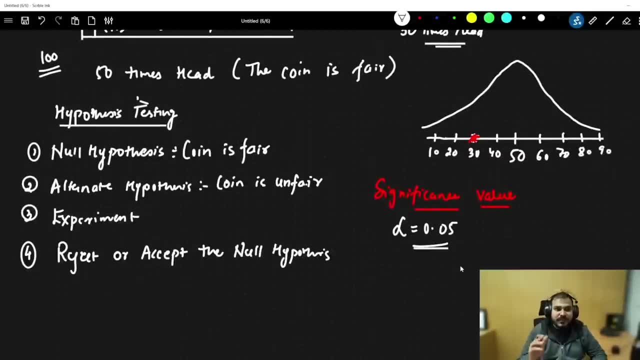 Suppose, let's consider that I am considering alpha as 0.05.. Now, this 0.05, what exactly it is, what exactly it actually means? This means that if I do 1 minus 0.05, this answer. let's say that this answer how much. 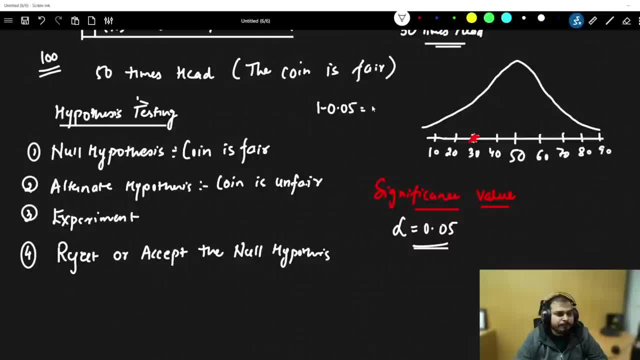 it will come. It will basically come as this: 0.05.. Okay, I have taken my significance value as 0.05.. When I convert this into percentage, it will become 5%- 5%. So from my 100%, if I subtract 5%, this basically indicates that it is 95% confidence. 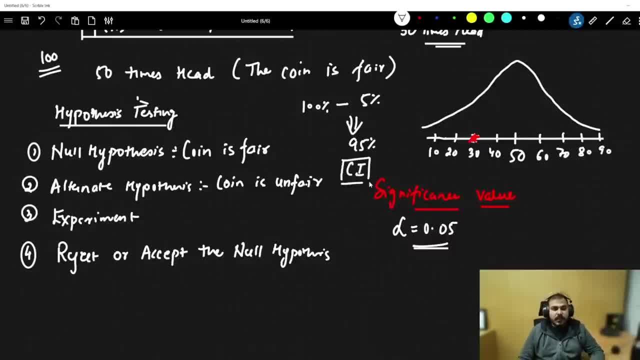 interval. Now, what is this 95% confidence interval? If I probably subtract from 1,, my probably the 95% confidence interval is there. Now, this 95% confidence interval is what part? Let's consider that I know my 2.5 is this part. 2.5 is this part, since this is a two-tailed. 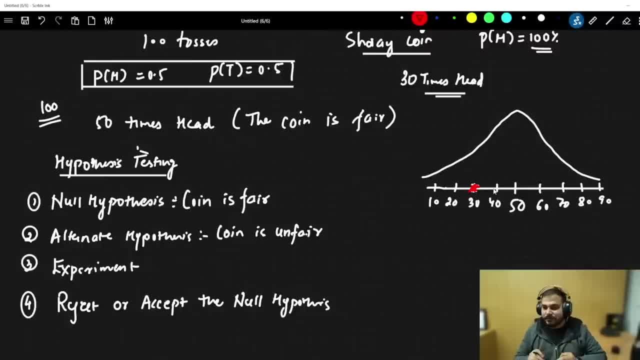 fair, not fair. So for this to define, it is always said that our experiment should be nearer to the mean. Okay, Nearer to the mean. Now, how do we define that? how far it can be away from the mean? We need to define that: how far it may be away from the mean. 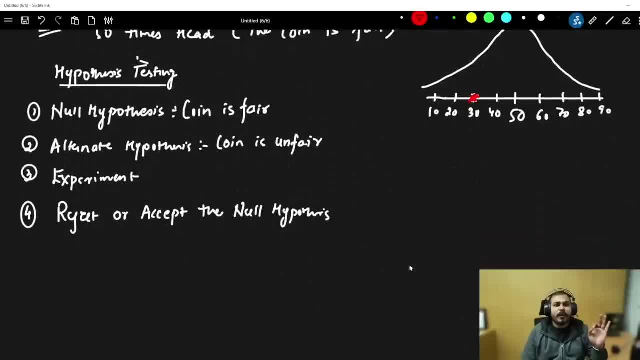 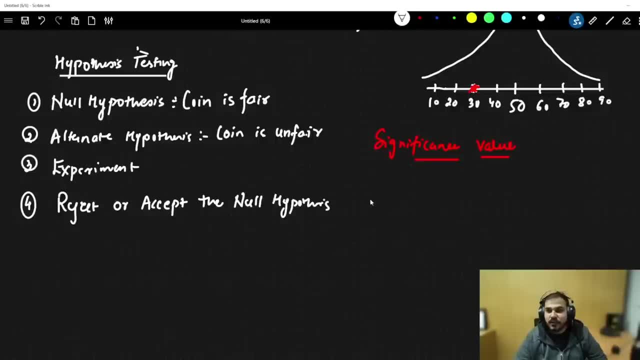 So for that we use a very important property which is called as significance value. Now, this significance value is basically given by alpha. Suppose, let's consider that I am considering alpha as 0.05.. Now this 0.05. what exactly it is, What exactly it actually means? 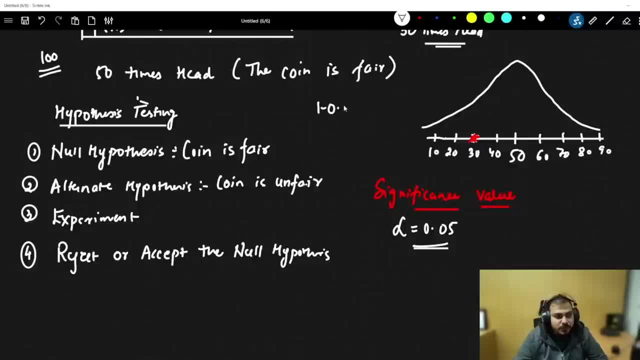 This means that if I do 1 minus 0.05, this answer, let's say that this answer how much it will come? it will basically come as: uh, this 0.05. okay, i have taken my significance value as 0.05. when i convert this into percentage, it will become five. 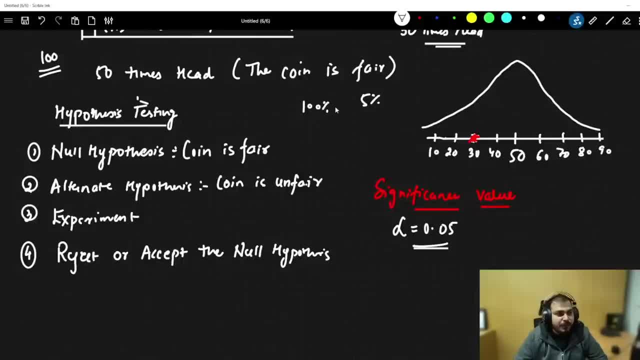 percent, okay, five percent. so from my hundred percent, if i subtract five percent, this basically indicate that it is 95 confidence interval. now, what is this 95 confidence interval? if i probably subtract from one, my probably, the 95 confidence interval is there. okay, now this 95 confidence. 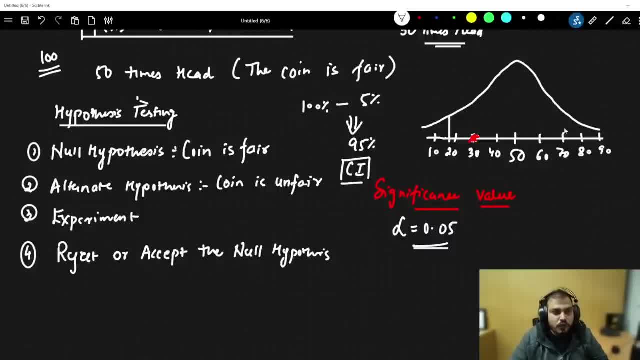 interval is what part? let's consider that. i know my 2.5 is this part. 2.5 is this part. since this is a two tail test, let i'll talk about two tail test also, don't worry. so let's consider that. this part to this part. this is my entire 95 confidence interval. this is defined by a domain expert. 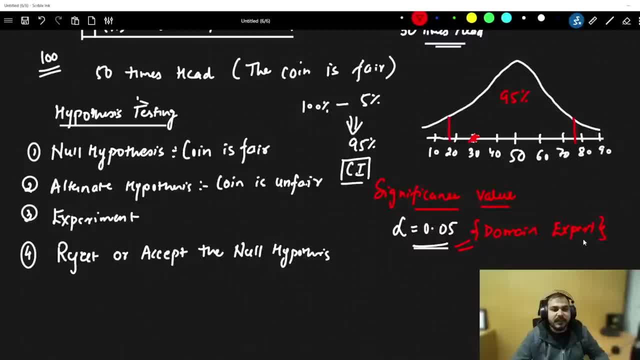 different, defined by a domain expert. but let's consider that it has been defined. now, what does that 0.05 indicate? i'm trying to show it to you when i probably divide this into two parts: here my 2.5 percent will come, here my 2.5 percent. 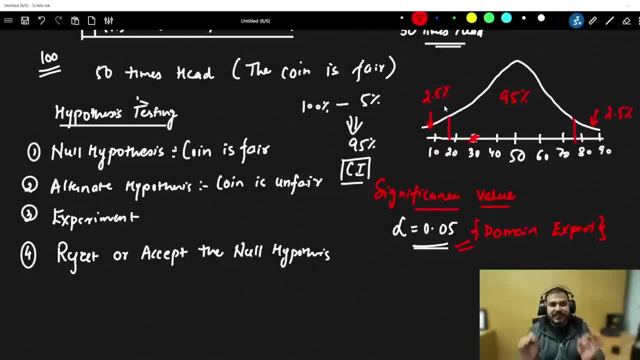 will come now understand one thing very important over here. now let's say that 30, i got 30 over here, so this is my 30 right and i have also defined my confidence interval from this point to this point. whenever we are coming inside this, then we see, we say: 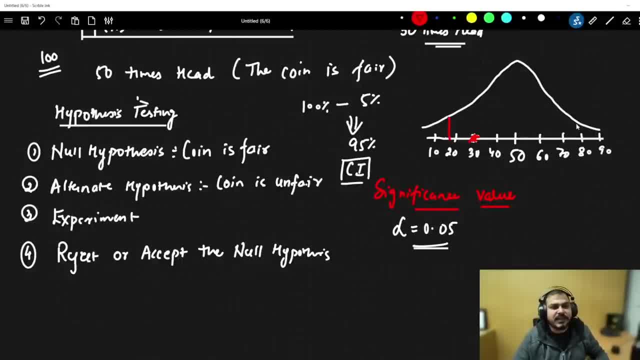 test. I'll talk about two-tailed test also, don't worry. So let's consider that. this part to this part, This is my entire 95% confidence interval. This is defined by a domain expert, Defined by a domain expert. Let's consider that it has been defined. Now, what does that? 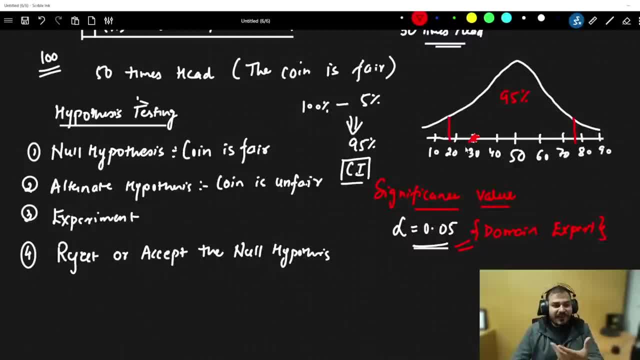 0.05 indicate. I'm trying to show it to you When I probably divide this into two parts: here, my 2.5% will come here, my 2.5% will come Now. understand one thing very important over here Now let's say that. 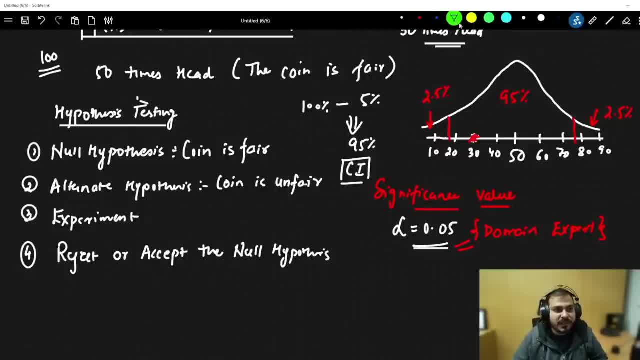 30,. I got 30 over here, So this is my 30, right, And I have also defined my confidence interval from this point to this point. Whenever we are coming inside this, then we see, we say that the coin is fair. Why? Because understand, it is within this interval. Here we need to. 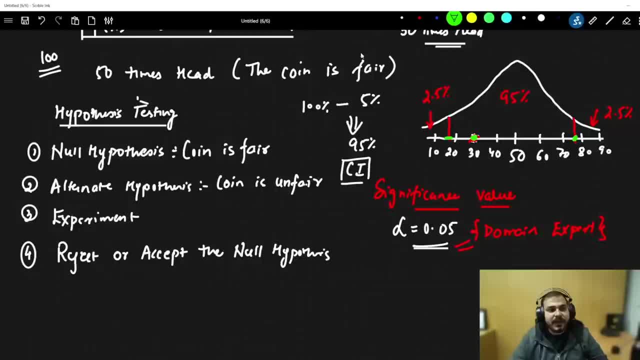 define because we don't know right What should be the number. You said that when I got head 30 times. many people are saying that not fair, But who are we to decide? Domain expert will decide, And how will we decide With the help of this significance value. 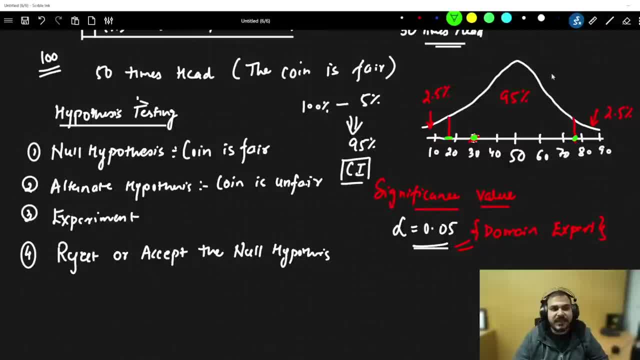 Suppose they say significance value is 0.05.. That basically means that the experiment, if it falls in this 95% confidence interval, that time I will say that that coin is fair. If it falls outside this confidence interval, that time I will say that the coin is not fair. Now tell me. 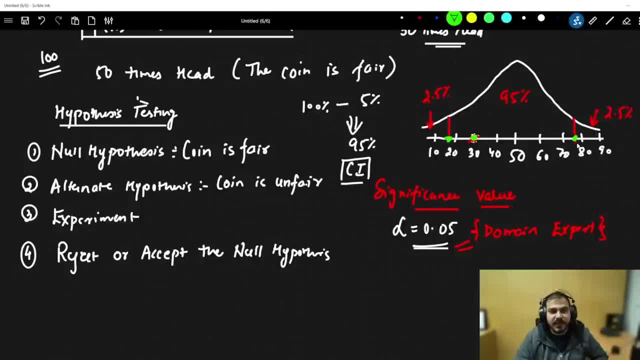 let's say that this number that you are seeing is 20,. let's say: And this number that you are seeing is 75.. 20 to 75 is my confidence interval. Now I perform the experiment If I get 10 heads only out of 100 experiments. should we accept or reject the null hypothesis? 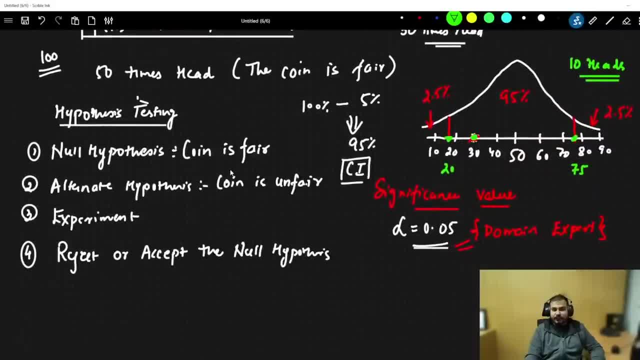 The null hypothesis is basically the coin is fair. The alternate hypothesis coin is unfair. So if I get 10 heads, which region it is falling, It will fall somewhere here. It is not inside the confidence interval So we can definitely say that coin is not fair. So for that particular 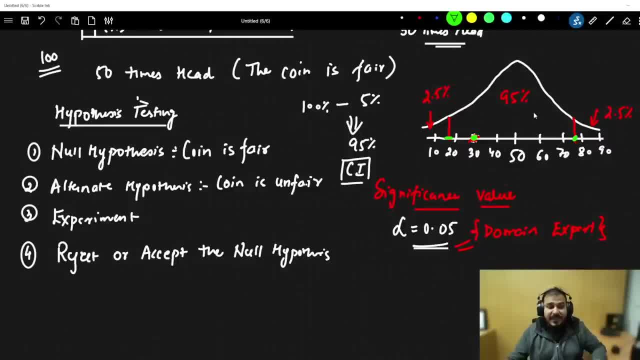 that the coin is fair. why? because understand, it is within this interval. here we need to define because we don't know right what should be the number. you said that when i got head 30 times. many people is saying that not fair. but who are we to decide? domain: the expert will decide and 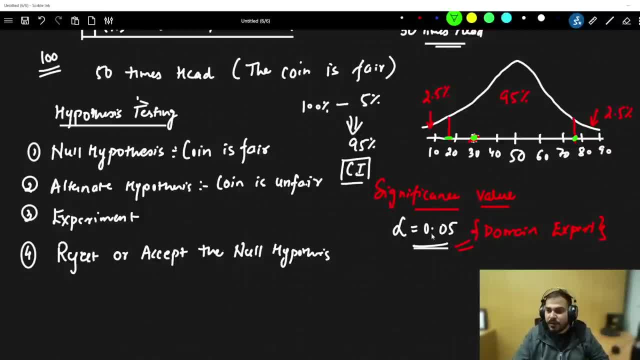 how will we decide with the help of this significance value? suppose they say significance value is 0.05. that basically means that we the the experiment if it falls in this 95 percent confidence interval. that time i will say that that coin is fair if it falls outside this confidence interval. 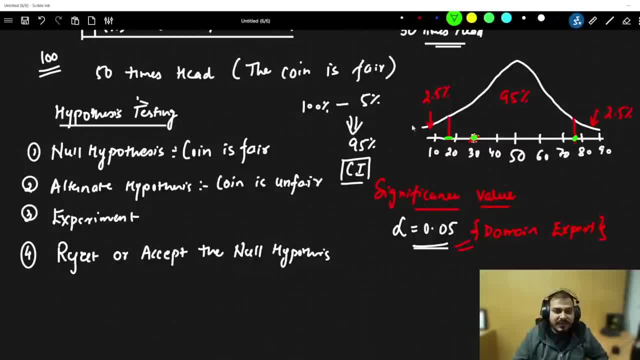 that time i will say that the coin is not fair. now tell me, let's say that this number that you are seeing is 20. let's say, and this number that you are seeing is 75. 20 to 75 is my confidence interval. now i perform the experiment. if i get 10 heads only out of 100 experiments should we accept? 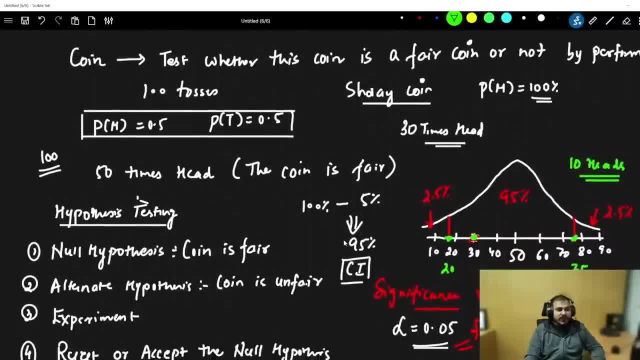 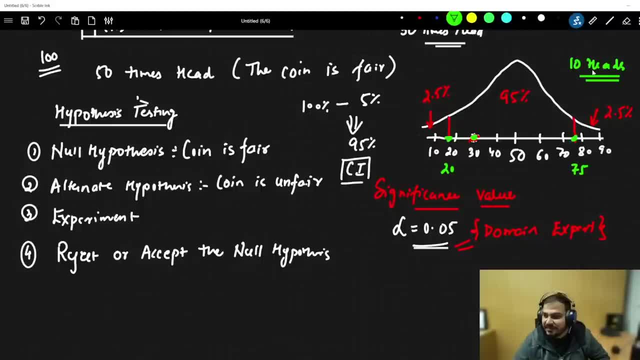 reject the null hypothesis. the null hypothesis is basically: the coin is fair. the null alternate hypothesis coin is unfair. so if i get 10 heads, which region it is falling, it will fall somewhere here. it is not inside the confidence interval, so we can definitely say that coin is not fair. 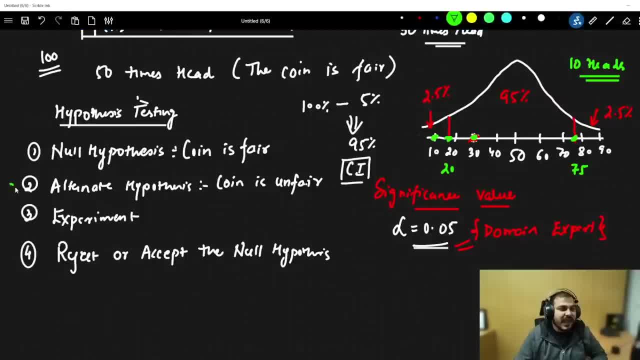 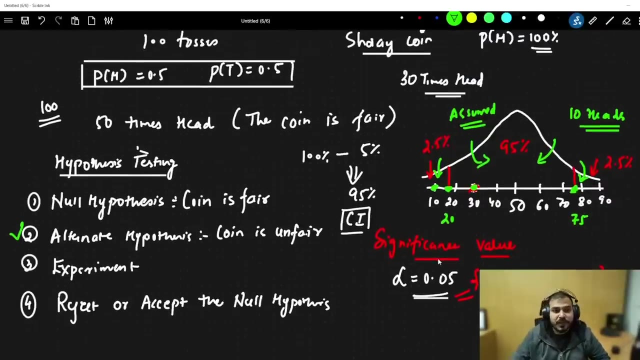 so for that particular case, we reject the null hypothesis and we accept the alternate hypothesis. i hope everybody is able to understand the terminologies that we are using over here. i cannot teach you separate topics understand. i have to combine these topics together to teach you how to do it. what if we have- okay, let's say that, guys, if you have 95 heads. 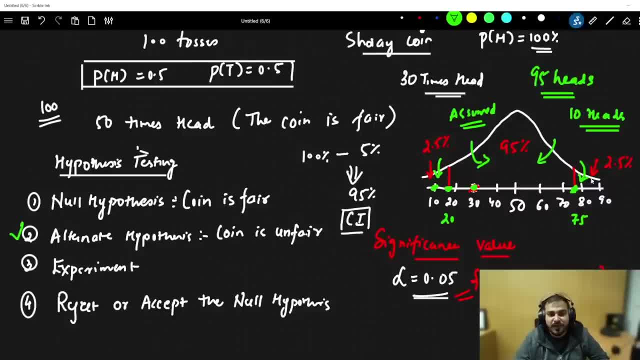 in those 100 experiments. which region it will fall? will it not fall in this region? 95 is somewhere here. so should we accept the null hypothesis or reject the null hypothesis? we have to obviously reject the null hypothesis and alternate hypothesis will be accepted. its very simple. i perform the experiment whatever value i get. i go and check in this. 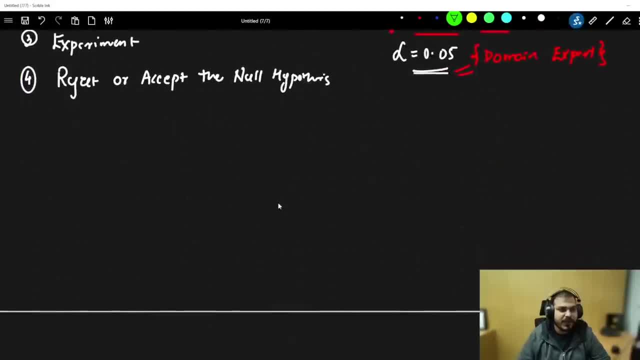 okay, let me tell you now one more, one more scenario. ok, here, let's say that my domain expertise said that, krish, you are a fool, and probably i will now use this: is 50, 60, 70, 80, 90. okay, let's say that, krish, you are a fool. why have you taken alpha 0.05? 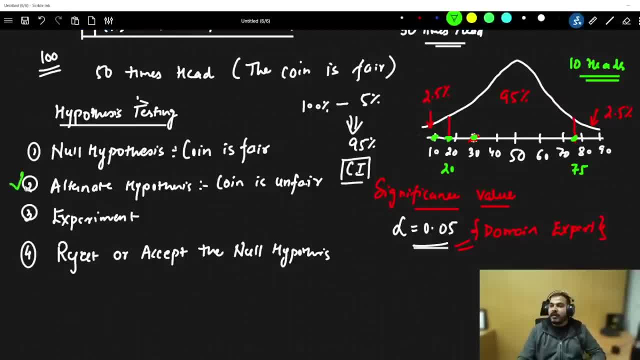 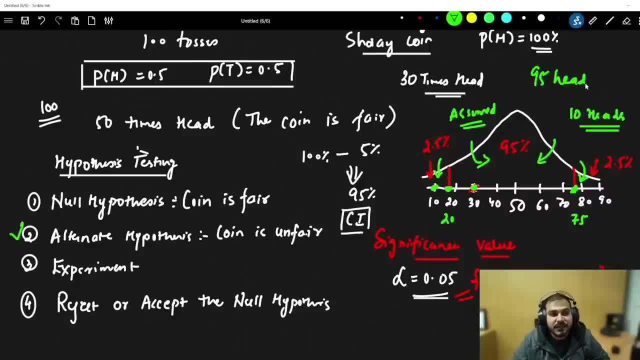 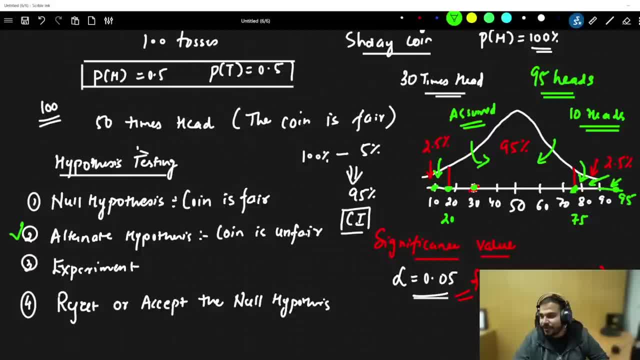 this region. 95 is somewhere here. So should we accept the null hypothesis or reject the null hypothesis? We have to obviously reject the null hypothesis and alternate hypothesis will be accepted. It's very simple. I perform the experiment Whatever value I get. I go and check in this. 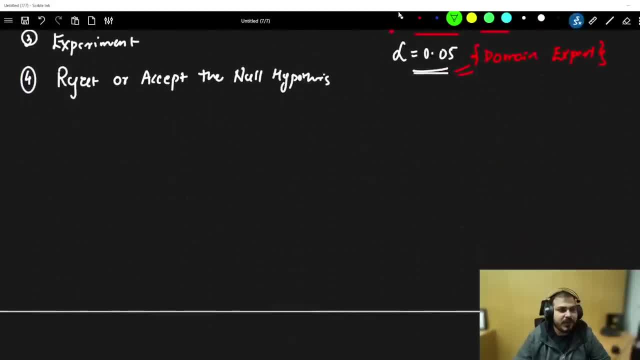 Okay, Let me tell you now one more scenario. Okay, Here let's say that my domain expertise said that, Krish, you are a fool And probably I will now use this- is 50, 60,, 70,, 80, 90.. Okay, Let's say: 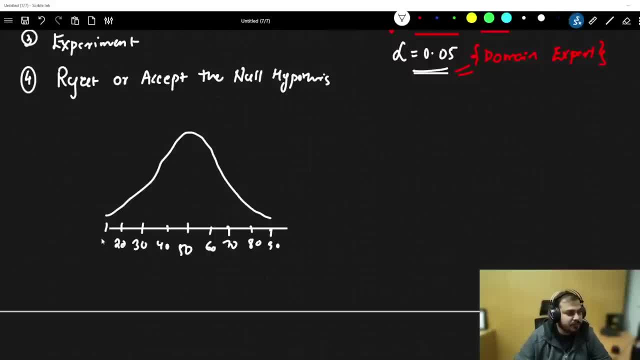 that, Krish, you are a fool. Why have you taken alpha 0.05?? Okay, I don't want that. So let's say that your alpha is 0.20.. Now, what will be your confidence interval? What will be your confidence? 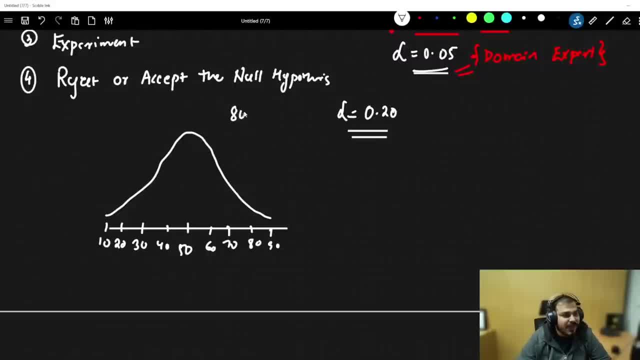 interval. Let's say that your confidence interval will be now 80% instead of 95%. So now your graph will look something like this: Let's say that your confidence interval will be now 80% instead of 95%. So now your graph will look somewhere here like this: It will be still more in this side. 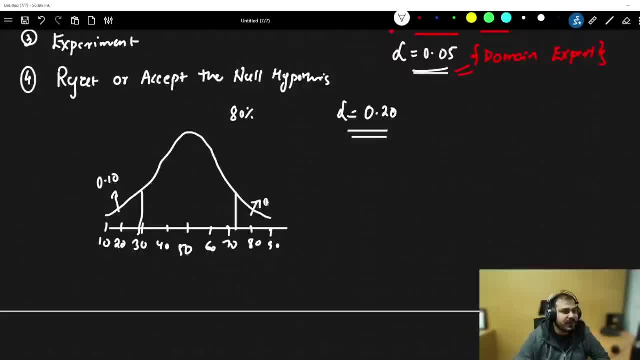 So this side will basically have 0.10.. This side will basically have 0.10.. And this all will be your 0.80%. When you combine all this, when you add up all this, it will be 1.. So at that point, 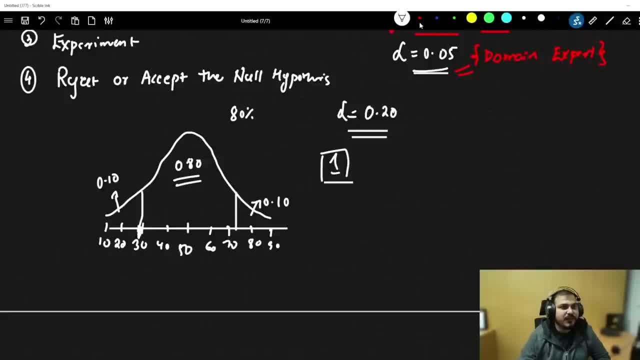 of time. then you can go and find out your confidence interval. This value will give you your lower confidence interval. This value will be giving you a higher confidence interval. You perform the experiment. Now just imagine you got 25 from that experiment. whether you should reject. or accept it. Tell me one more scenario. Let's say that you got 25 from that experiment. Whether you should reject or accept it. Tell me one more scenario. Let's say that you got 25 from that experiment. Let's say that you got 25 from that experiment, Whether you should reject or accept it. Tell me one thing. 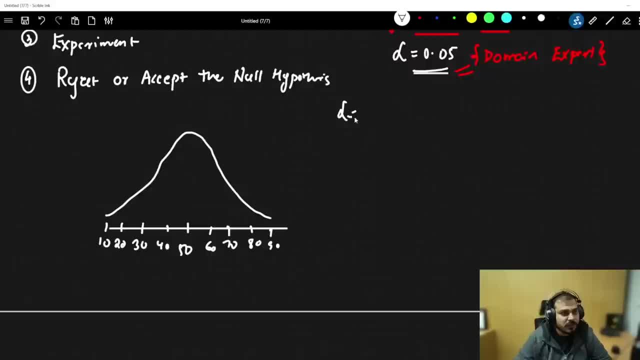 this is 50, 60, 70, 80. okay, let's say that, krish, you are a fool. why have you taken alpha point zero five? I don't want that. So let's say that your alpha is 0.20.. Now, what will be your confidence interval? 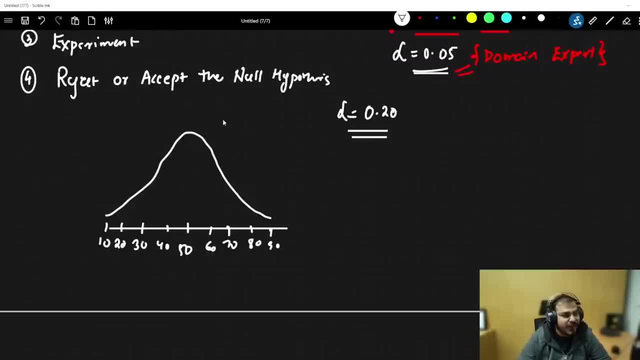 What will be your confidence interval? Let's say that your confidence interval will be now 80% instead of 95%. So now your graph will look somewhere here like this: It will be still more in this side. So this side will basically have 0.10,, this side will basically have 0.10, and this all. 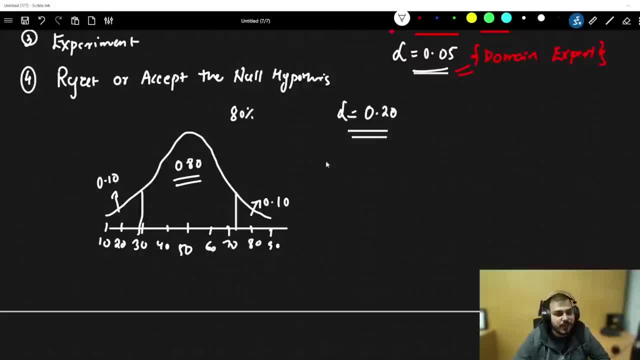 will be your 0.80%. When you combine all this, when you add up all this, it will be 1.. So at that point of time then you can go and find out your confidence interval. This value will give you your lower confidence interval. 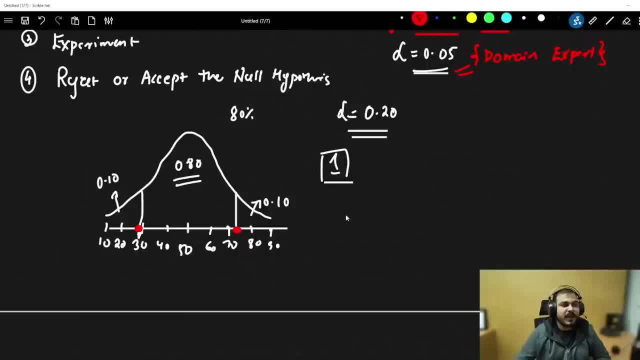 This value will be giving you a higher confidence interval. You perform the experiment. Now just imagine you got 25 from that experiment. whether you should reject or accept it, Tell me one thing: if your alpha value is 0.3,, what is your confidence interval? 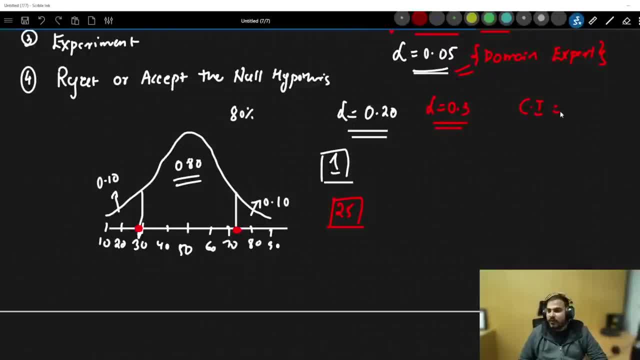 Vishwashwaram, I just took it for heads only, right. So what is your confidence interval if your alpha value is 0.3?? Obviously, you will say that it is 0.7, that is 70% confidence interval. 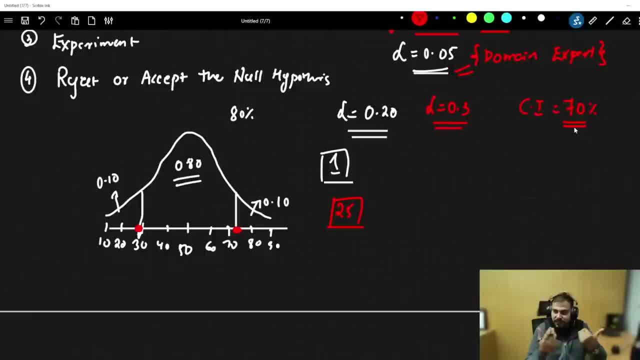 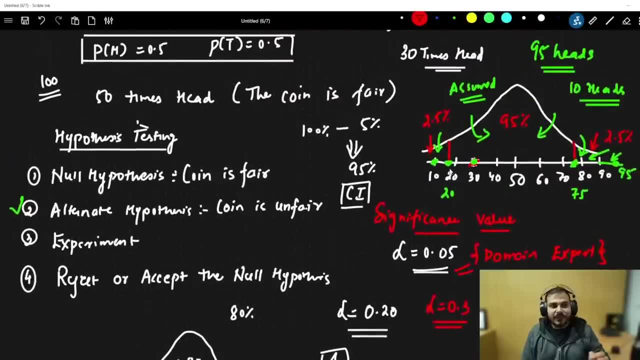 So alpha significance value and confidence interval are reversed right? You need to calculate in that specific way right Now. usually when we say, when we say like p-value, right, Suppose, if it does not follow in the confidence interval, I may say that the p-value is less. 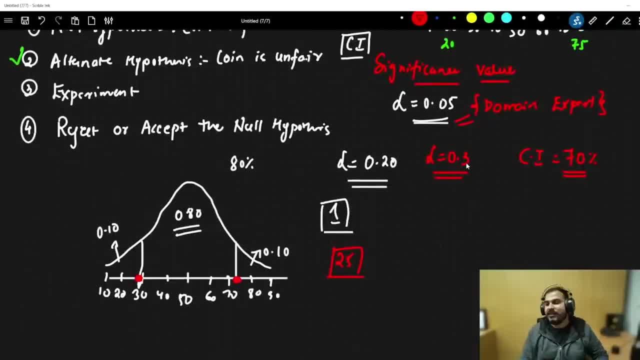 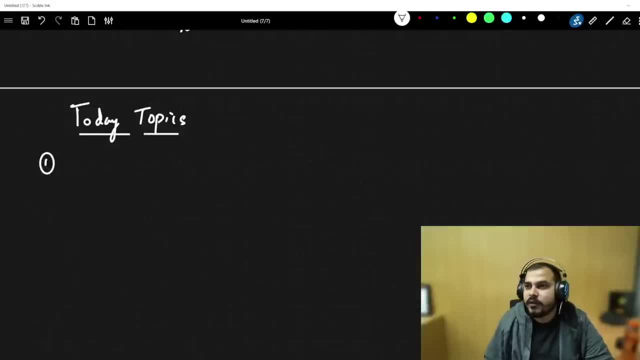 than 0.3.. So because of that, I have to reject the null hypothesis. Hello guys, Today topics- what all things we are going to see- Is that the first thing that we are going to check out is something called as type one. 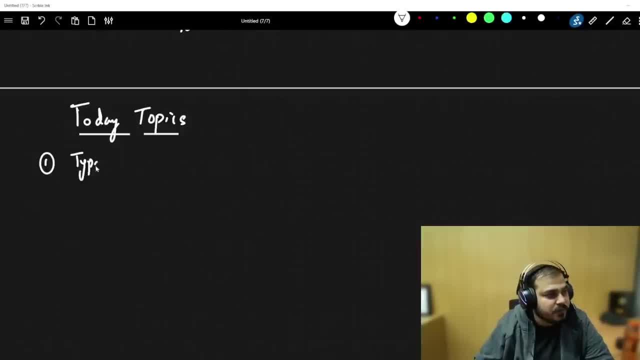 type two error. So the first topic that we are going to see is something like type one and type two error, Very super important, Probably in machine learning. you will be discussing about um, you know, confusion, matrix. Fine guys. if it is not uploaded, don't worry, it will get uploaded today. 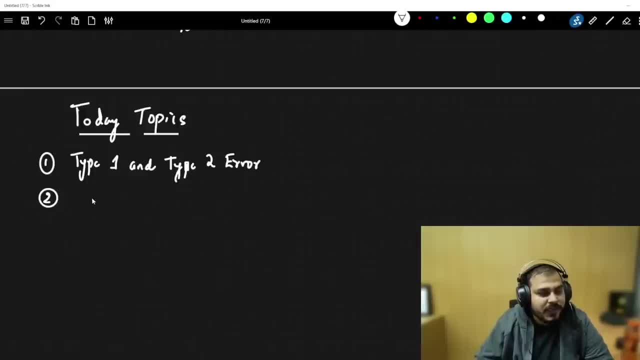 Okay, I will say the backend team to do it. The second thing that we are probably going to discuss about, after one tail of the type one and type two error, is basically your one tail and two tail test. The third topic that we are going to see is that how to find out confidence interval. 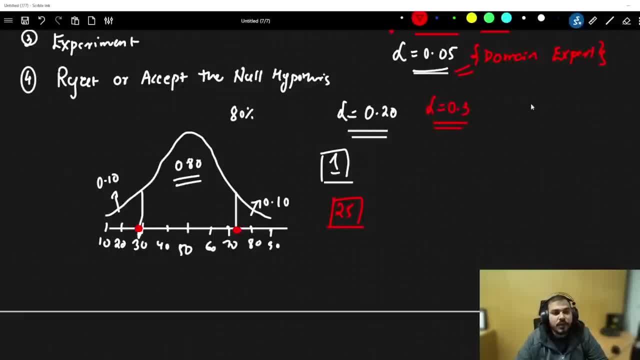 If your alpha value is 0.3,. what is your confidence interval? Vishveshwaram, I just took it for heads only, right? So what is your confidence interval if your alpha value is 0.3?? Obviously you will. 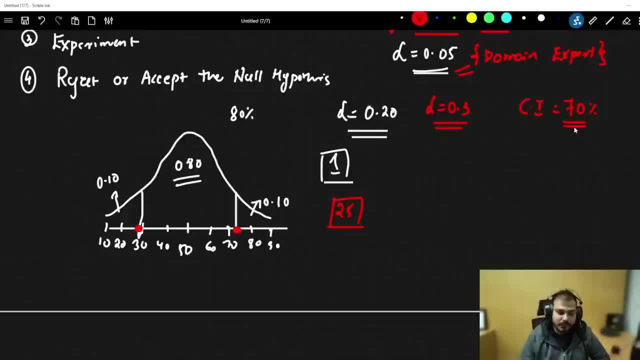 say that it is 0.7.. That is 70% confidence interval. So alpha significance value and confidence interval are reversed right. You need to calculate in that specific way right Now. usually when we say, when we say like p-value, right, Suppose if it. 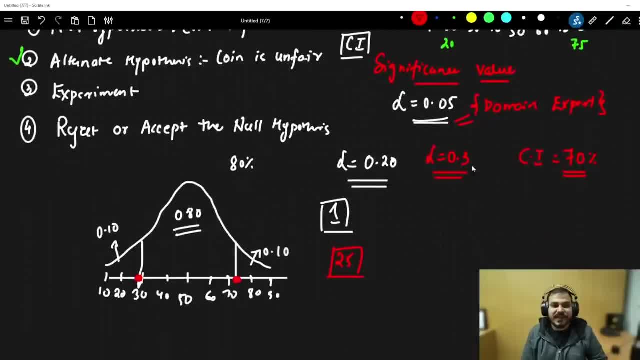 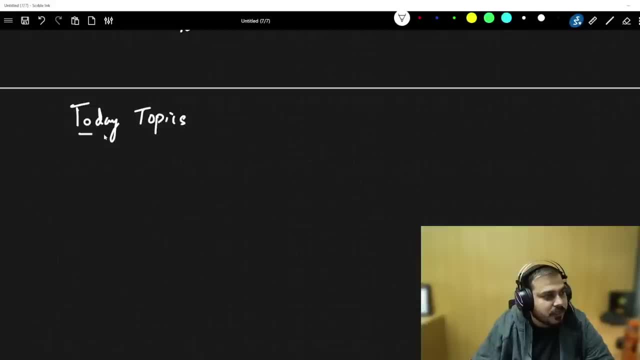 does not follow in the confidence interval, I may say that the p-value is less than 0.3.. So because of that, I have to reject the null hypothesis. Hello guys, today, topics, what all things we are going to see is that the first thing that we are going to check out is something called as type 1,. 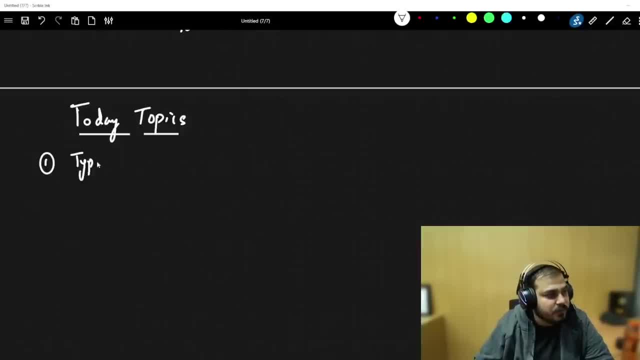 type 2 error. So the first topic that we are going to see is something like type 1 and type 2 error, Very super important, Probably in machine learning. you will be discussing about um, you know, confusion, matrix. Fine guys. if it is not uploaded, don't worry. 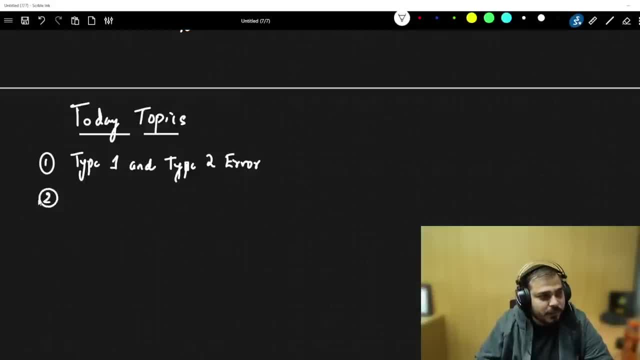 it will get uploaded today. okay, I will say the backend team to do it. The second thing that we are probably going to discuss about after 1 tail, or after type 1 and type 2 error, is basically your one tail and two tail test. The third topic that we are going to see is that how to find out. 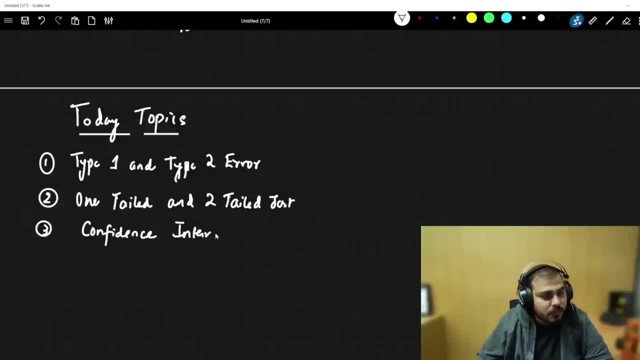 confidence interval. Okay, that is what we are going to see. see now confidence interval. how to calculate this? probably, when an alpha value is given. i told you we need to define some confidence interval in order to solve, uh, you know, some problems. the fourth topic that we will try to see, after confidence interval, is something called as z test. 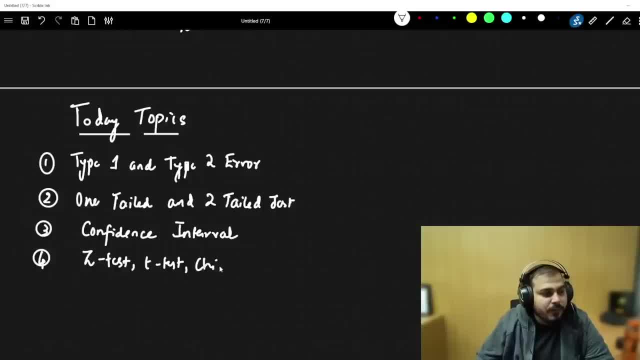 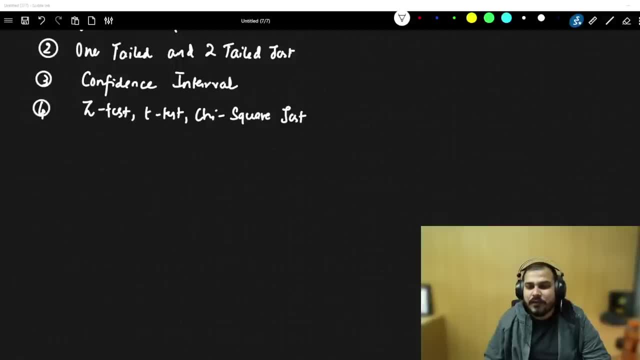 t test and if we get time, we will also finish up chi square test. so let's start. the first topic that we are probably going to discuss about is something called as type 1 and type 2 error always understand whenever we do any kind of hypothesis testing. one very important thing i 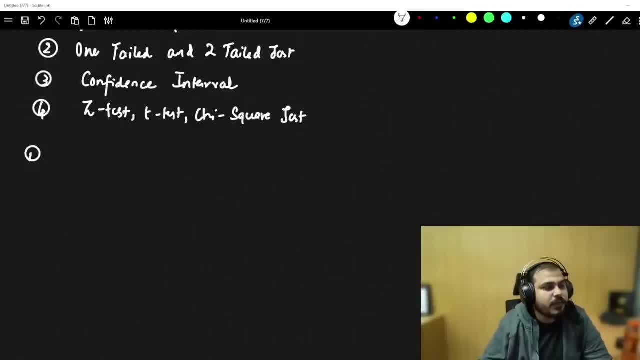 told you that what we have, the first topic that we are probably going to discuss about- is type 1 and type 2 error. type 1 and type 2 error always understand in any kind of hypothesis testing. right, we do have something called as null hypothesis. null hypothesis is usually denoted by: 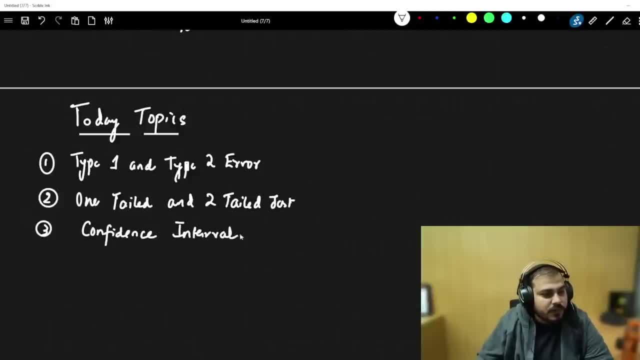 Okay, That is what we are going to see Now. confidence interval: how to calculate this? probably, when an alpha value is given. I told you we need to define some confidence interval in order to solve, uh, you know, some problems. 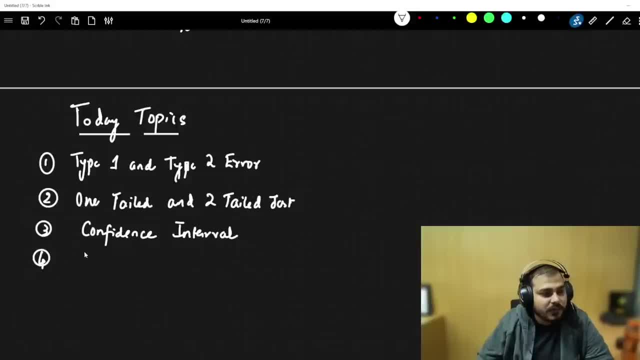 The fourth topic that we will try to see, after confidence interval, is something called as Z test, T test, And if we get time, we will also finish up chi square test. So let's start. the first topic that we are probably going to discuss about is something: 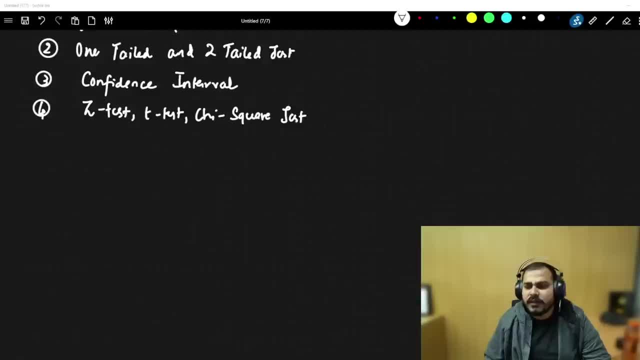 called as type one and type two error, Always understand, whenever we do any kind of hypothesis testing. one very important thing: I told you that what we have, the first topic that we are probably going to discuss about, is type one. Okay, Type one and type two error. 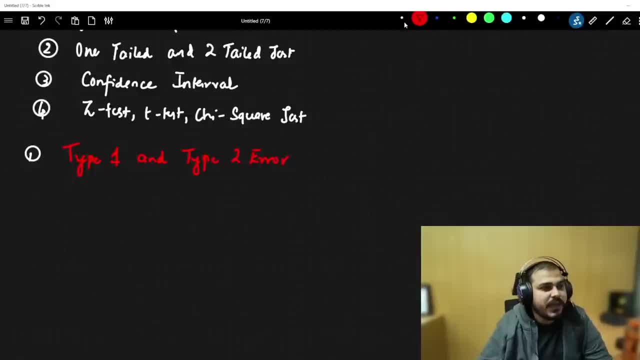 Type one and type two error Always understand in any kind of hypothesis testing. right, we do have something called as null hypothesis. Null hypothesis is usually denoted by H zero. We have something called as alternate hypothesis- Okay, Alternate hypothesis- which is denoted by H one. 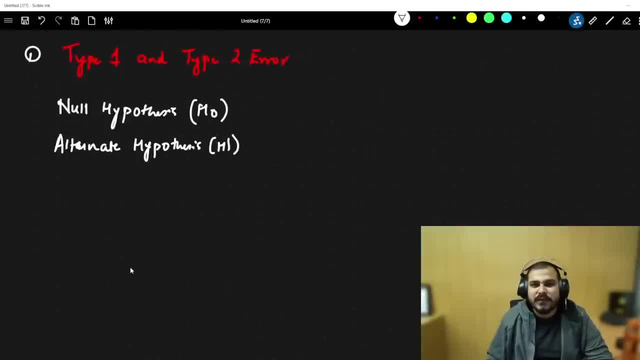 Okay, Now, at the end of the day, after performing any kind of experiments, right, let's say that I'm performing an experiment where to check whether the coin is correct. I'll check whether the coin is fair or not. I'll take the same example: what we have discussed yesterday and coin is not fair. 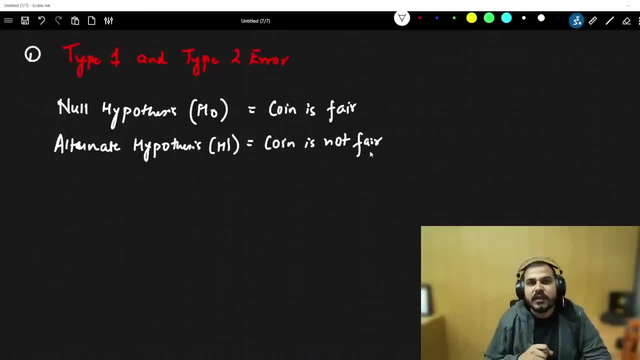 I will probably go and check, check whether it falls within the confidence interval. I'll check the significance value. based on that, the confidence interval will be defined. you know everything we will do And that is what I explained in the yesterday's part. 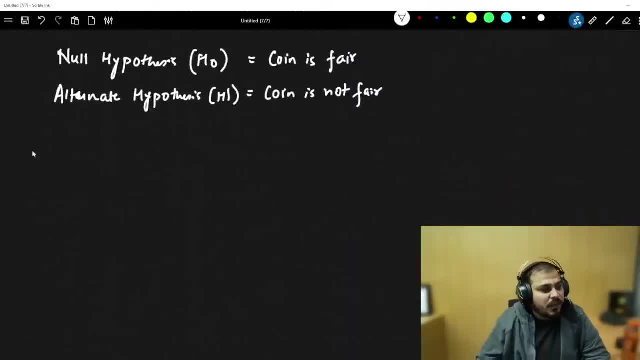 Now, from this, after we perform the experiment, there are two types of decisions that can be made. First of all, we'll go with respect to the reality check. So the reality check will be that either null hypothesis will be true, null hypothesis. 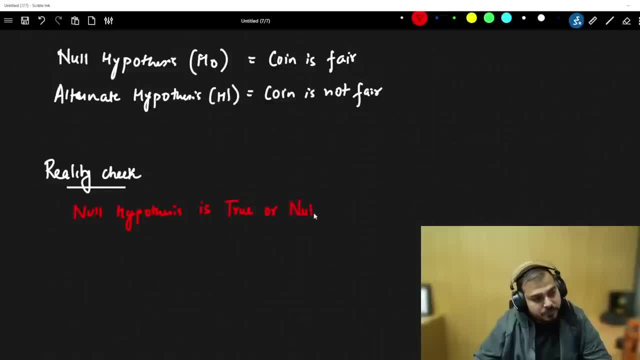 is true or null hypothesis is false right. Only these two things we will be able to see in reality. check right. If I go and check with respect to the decision, because this is what I am actually trying to check- test right in decision, I may either get: null hypothesis is true, null hypothesis. 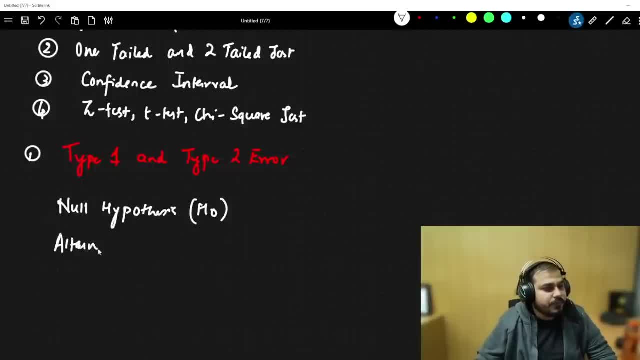 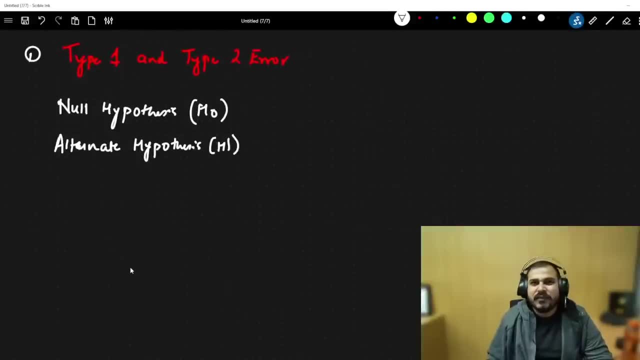 h0, we have something called as alternate hypothesis. okay, okay, alternate hypothesis, which is denoted by h1. okay, now, at the end of the day, after performing any kind of experiments, right, let's say that i'm performing an experiment where to check whether the coin is fair or not. i'll take the same example: what we have discussed yesterday. and coin is not. 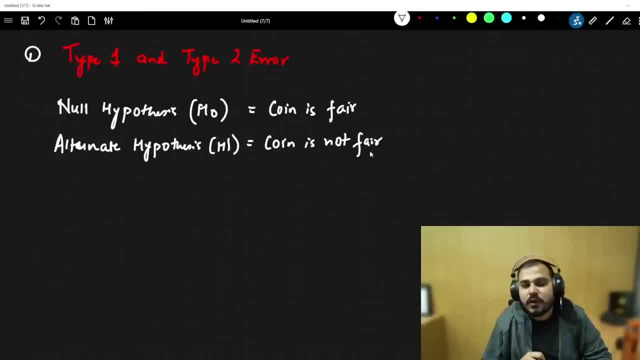 fair. i will probably go and check check whether it falls within the confidence interval. i'll check the significance value. based on that, the confidence interval will be defined. you know everything we will do and that is what i explain to you in this video. so let's start the first topic. 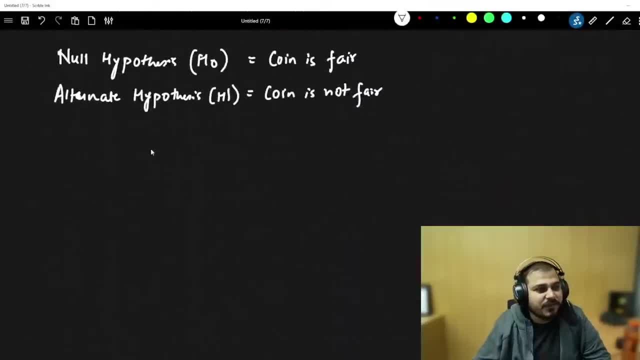 now from this, after we perform the experiment, there are two types of decisions that can be made. first of all, we'll go with respect to the reality check. so the reality check will be that either either null hypothesis will be true, null hypothesis is true or null hypothesis is false. 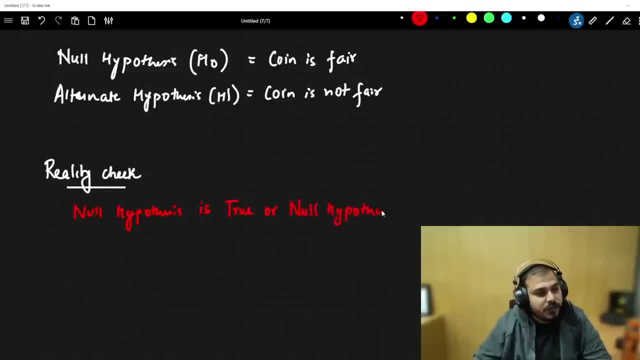 right. only these two things we will be able to see in reality. check right. if i go and check with respect to the decision, because this is what i am actually trying to check- test right in decision- i may either get: null hypothesis is true, null hypothesis is true. 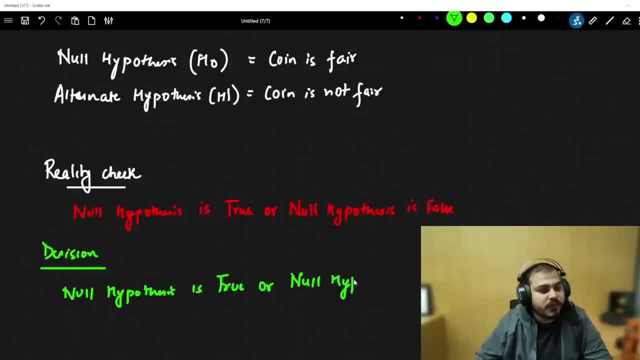 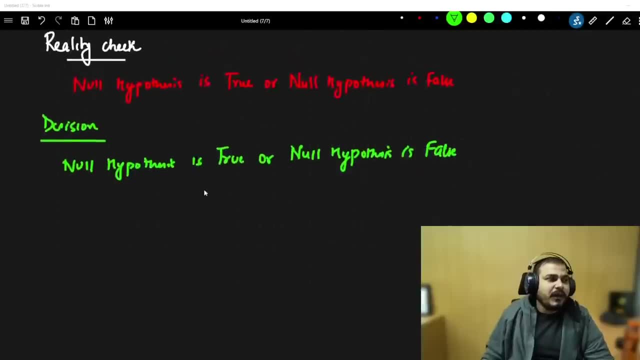 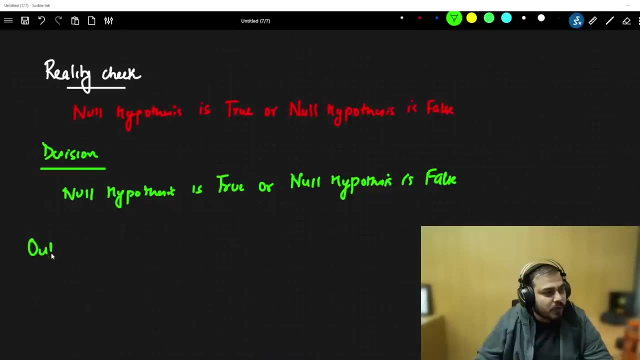 or null hypothesis is false. when null hypothesis is false, i will say that alternate hypothesis is accepted, right, or we reject the null hypothesis. now i, from this two, what you can basically derive is that see this very important first outcome. let's say what, what can, what may be the possible outcome. okay, so what may be the possible outcome, so outcome. 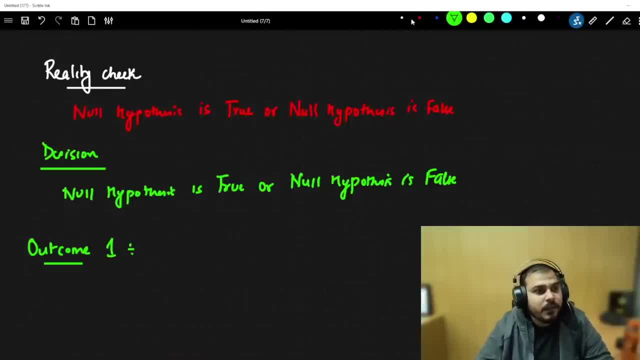 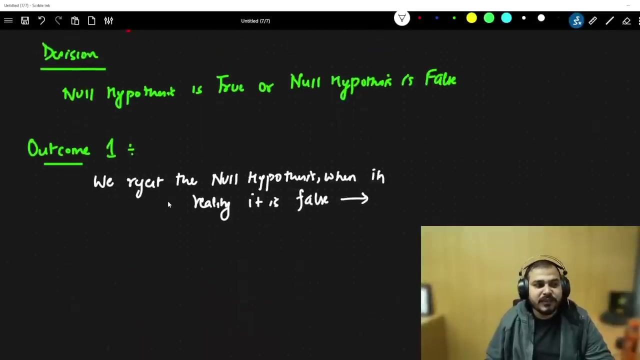 one, i will say that, okay, outcome one is that we reject the null hypothesis with the reject the null hypothesis. that is my decision. when it is when, in reality, it is false, is this is a good decision? yes, we reject the null hypothesis when, in reality, it is false. is this a good decision? 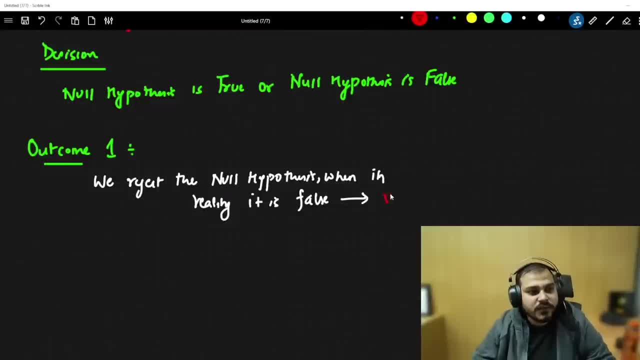 yes, it is obviously a very good decision. this is how we should take a decision now, when, in reality- when i say that, in reality, it is false- obviously we are rejecting the null hypothesis. okay, very good decision. now the second outcome. let's go ahead and discuss the second. 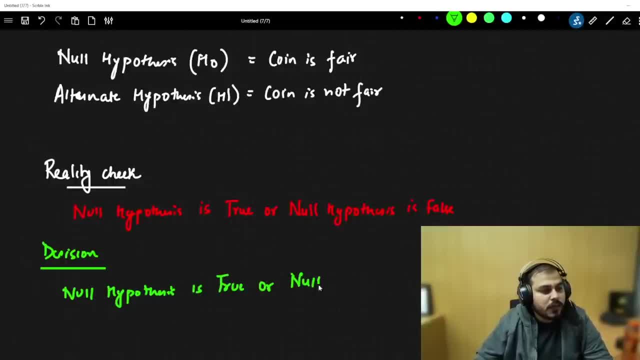 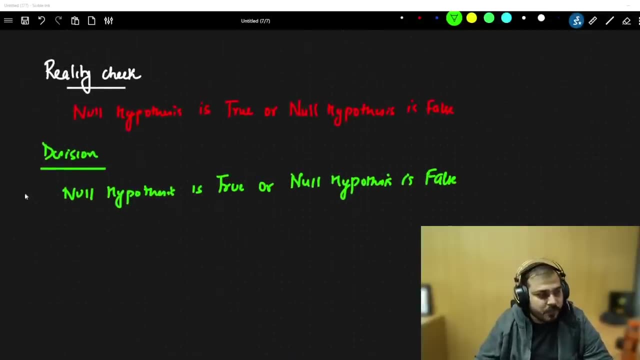 is true Or null hypothesis is false. When null hypothesis is false, I will say that alternate hypothesis is accepted, right, Or we reject the null hypothesis. Now I from this two, what you can basically derive is that see this very important. 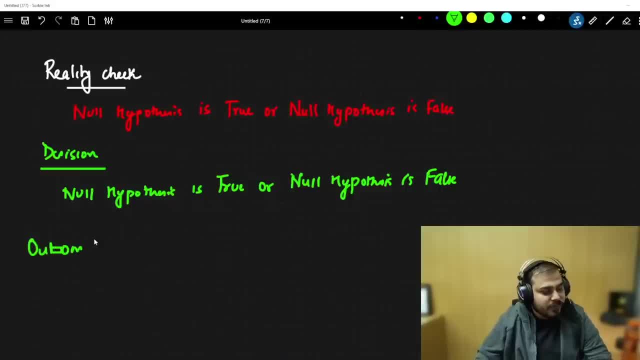 First outcome: let's say what, what can, what may be the possible outcome. okay, So what may be the possible outcome? So, outcome one: I will say that okay. Outcome one Is that we reject the null hypothesis with the reject the null hypothesis, that is my 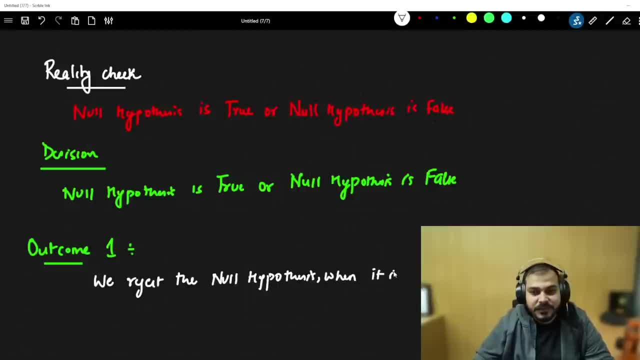 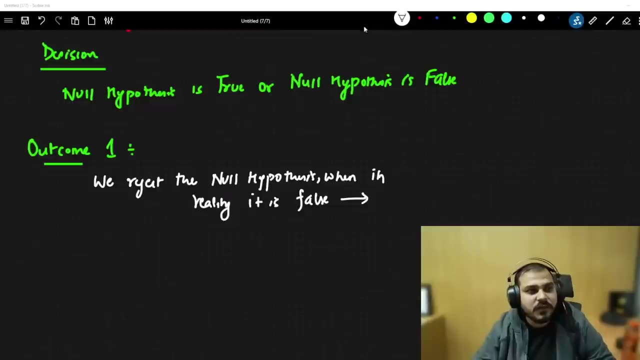 decision when it is when in reality it is false. Is this is a good decision? Yes, We reject the null hypothesis when in reality it is false. Is this a good decision? Yes, It is obviously a very good decision. 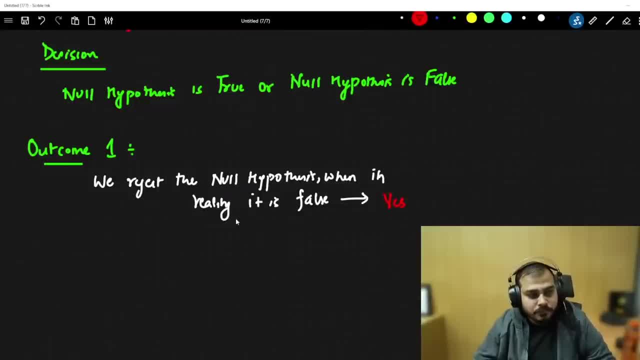 This is how we should take a decision Now, when, in reality- Okay, When I say that in reality, it is false- obviously we are rejecting the null hypothesis. okay, Very good decision. Now the second outcome. let's go ahead and discuss the second outcome. 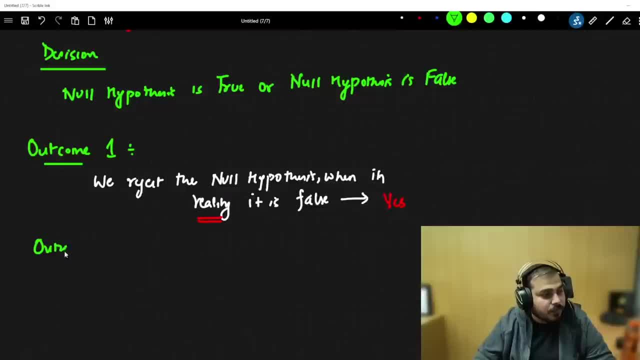 Now suppose I write the outcome two. What are the possible outcomes? I am just trying to show you: okay, We reject the null hypothesis. We reject the null hypothesis When, In reality, Okay, When in reality it is true. so over here, what should be your decision? whether this 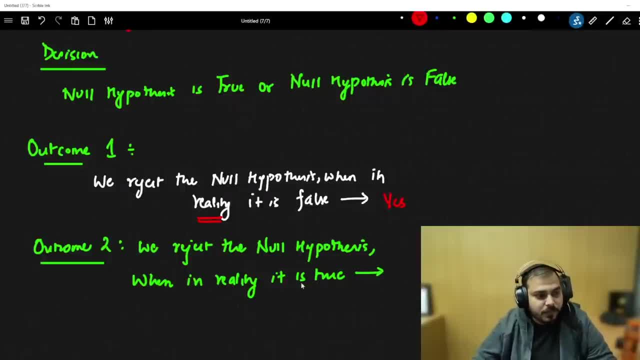 is a good decision or not. Again, I have to note at this particular point, when in reality it is true, if we are rejecting the null hypothesis, is this, is this a correct decision or not? Over here, in this particular case, obviously many people will say that it is a bad decision. 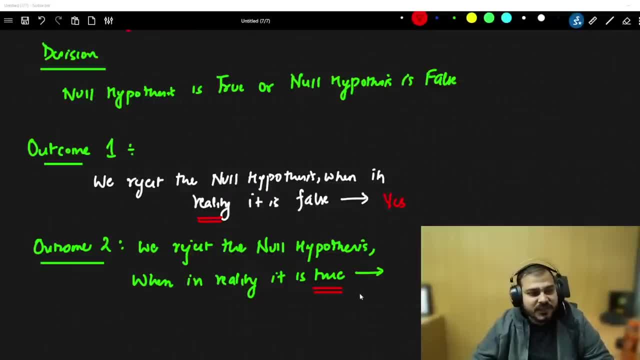 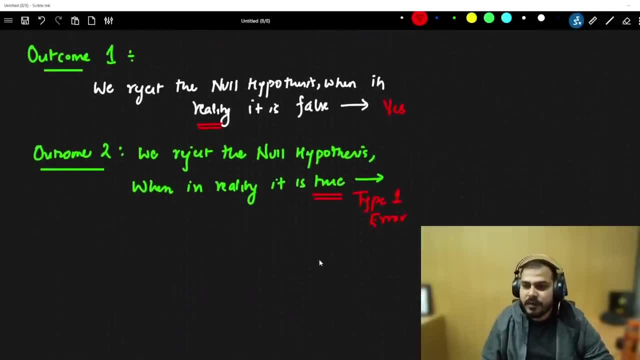 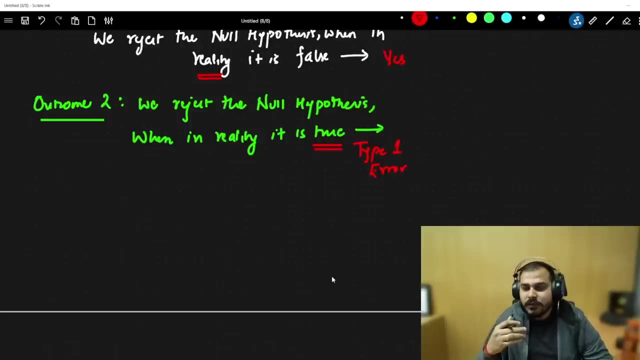 So here I will say no. And this kind of decisions is specifically called as type one error, So this decision is basically called as type one error. Okay, So this decision when we are rejecting the null hypothesis when in reality it is true. 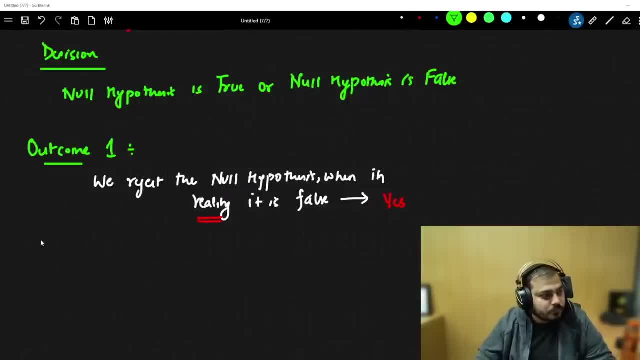 outcome. now suppose i write the outcome two. what are the possible outcomes? i'm just trying to show you. okay, we reject the null hypothesis. we reject the null hypothesis when in reality it is true. so, over here, what should be your decision, whether this is a good decision or not. 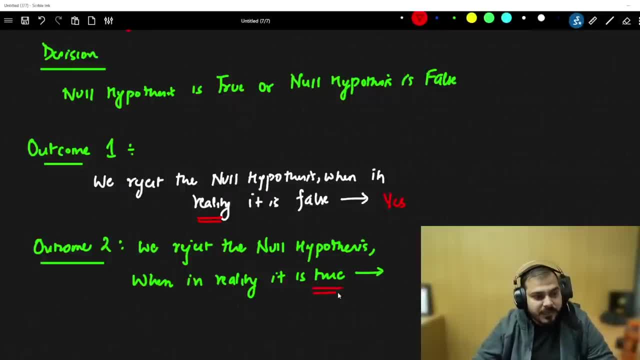 again. i have to note at this particular point, when in reality it is true, if we are rejecting the null hypothesis, is this, is this a correct decision or not? over here, in this particular case, many people will say that it is a bad decision. so here i will say no and this kind of decisions. 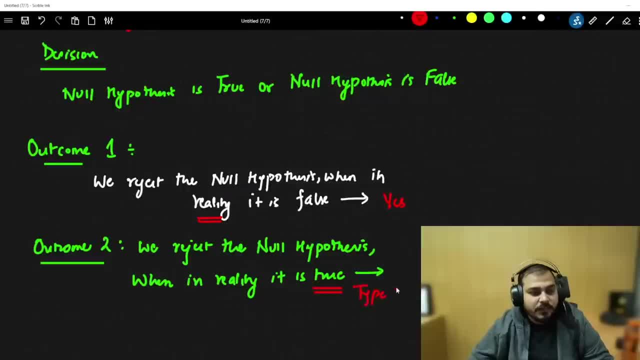 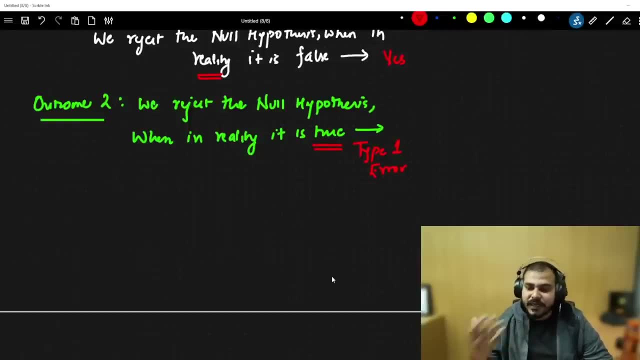 is specifically called as type 1 error, so this decision is basically called as type 1 error, right? so this decision, when we are rejecting the null hypothesis, when they are, when in reality, it is true, let's say that i take my null hypothesis as the person is innocent and my alternate 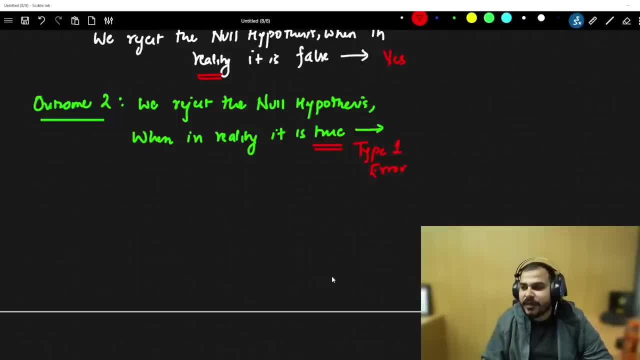 hypothesis is: person is not innocent. now, in this particular case, the person we are just acuity him in movies. you have seen right. many people will just be awarded death sentence even though they have not done anything wrong. so that kind of example is what you are actually. 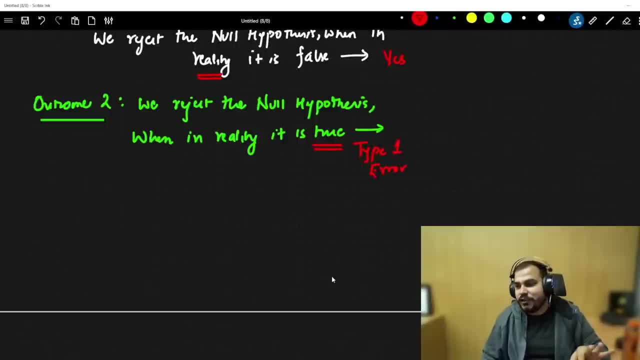 seeing over here we reject the null hypothesis when in reality it is true. that basically means the person is awarded a death sentence even though he did not do anything. so this, for this, is the perfect example example you have seen in movies, right In movies. okay, You will be seeing that a person 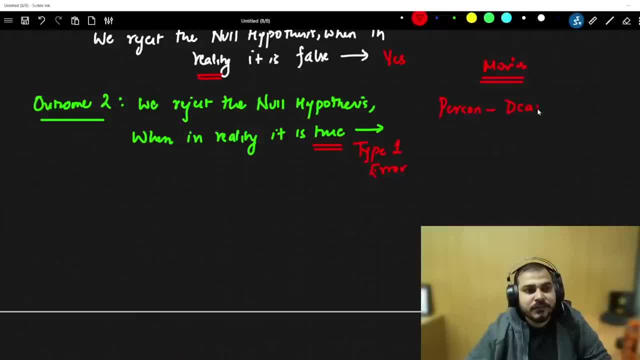 will be awarded a death sentence even though he did not do anything in the case of a fake case. So at that point of time this person is not innocent. But in reality he is innocent. So this becomes a perfect example of type 1 error, Outcome 3.. Outcome 3 basically says that: 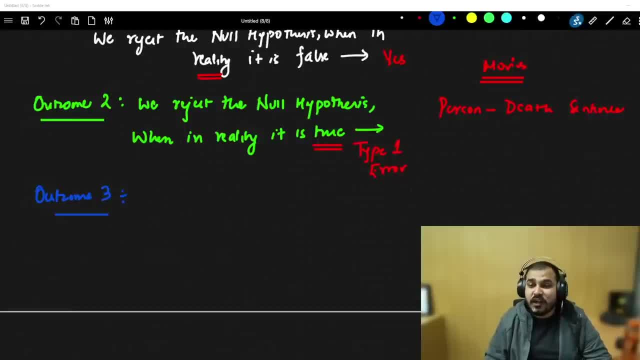 this is also a very important outcome And these all things you will be able to relate in confusion matrix. I do not know how many people knows about confusion matrix. So we retain the null hypothesis or we accept the null hypothesis. Let us say that I am saying 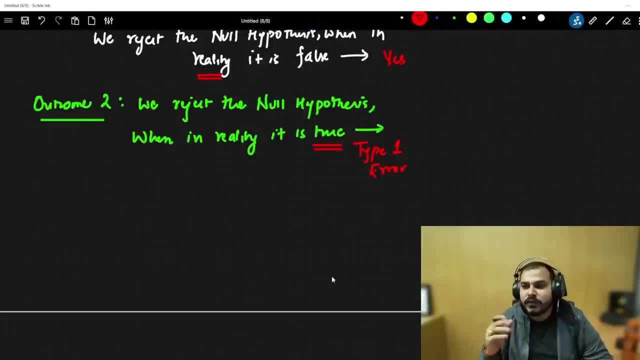 Let's say that I take my null hypothesis as the person is innocent And my alternate hypothesis is: person is not innocent. Now, in this particular case, the person we are just acquitting him in movies we have seen right. many people will just be awarded death sentence even though they have not done. 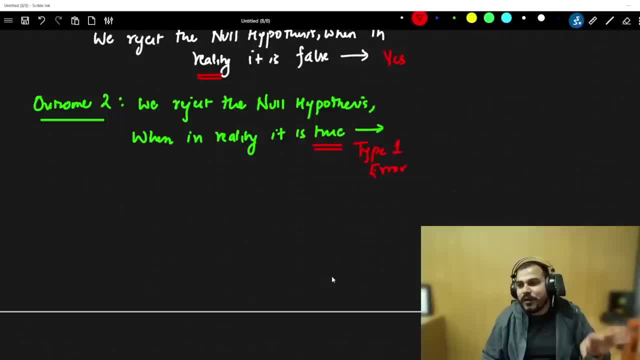 anything wrong. So that kind of example is what you are actually seeing over here. We reject the null hypothesis when in reality it is true. That basically means the person is awarded a death sentence even though he did not do anything. So this is the perfect example. 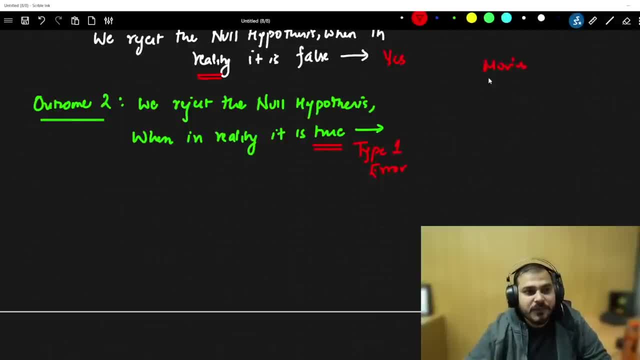 You have seen in movies, right In movies. okay, You will be seeing that a person will be awarded a death sentence even though he did not do anything in the case of a fake, fake case. So at that point you will be seeing that the person is not innocent. 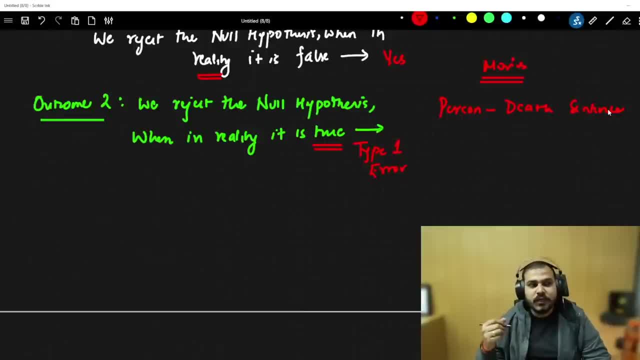 So this is the perfect example. So this is the perfect example. At that point of time, this person is not innocent, But in reality he is innocent, So this becomes a perfect example of type 1 error, Outcome 3.. Outcome 3 basically says that this is also a very important outcome. 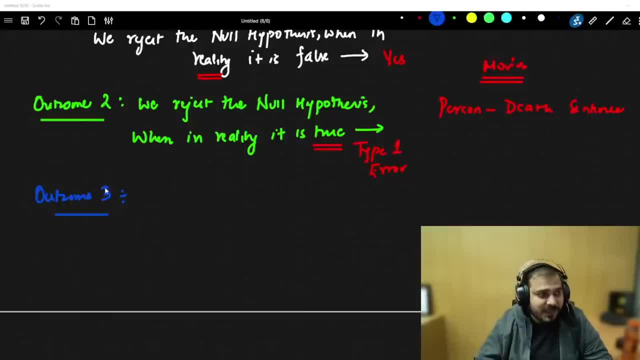 And this all things you will be able to relate in confusion matrix. I don't know how many people knows about confusion matrix. So we retain the null hypothesis or we accept the null hypothesis. let's say that I am saying we accept the null hypothesis. 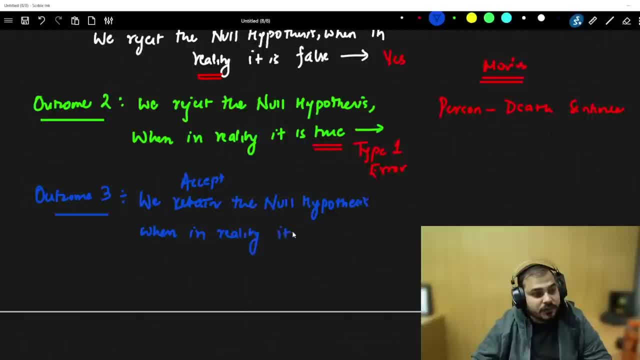 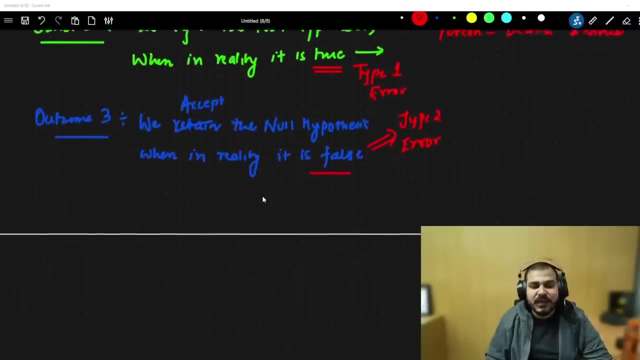 When in reality it is false. Is this a good decision? The answer should be no, So this error is basically called as type 2 error. Only four outcomes will be there. Four outcome will definitely be there. So here you can understand that in this particular case, even though the person has committed, 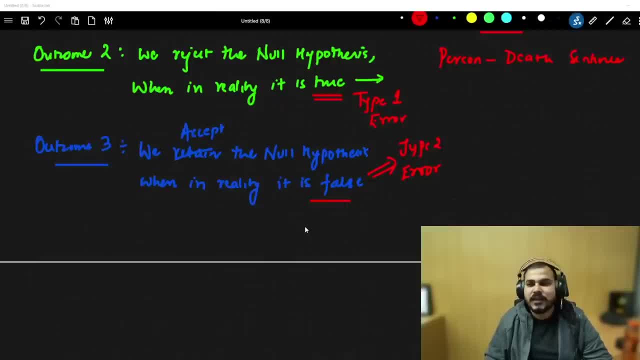 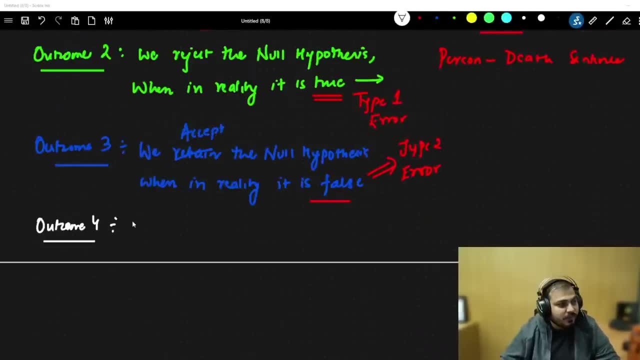 crime. he is not acuted So definitely. this error is basically called as type 2 error. Okay, I hope everybody's got is clear right. Now let's go to outcome 4. Outcome 4. Outcome 4 is that we accept the null hypothesis when in reality it is true. 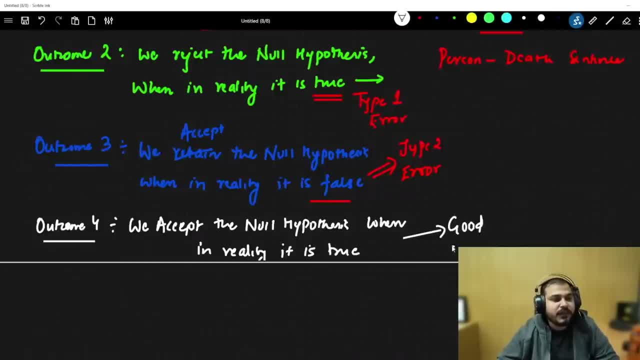 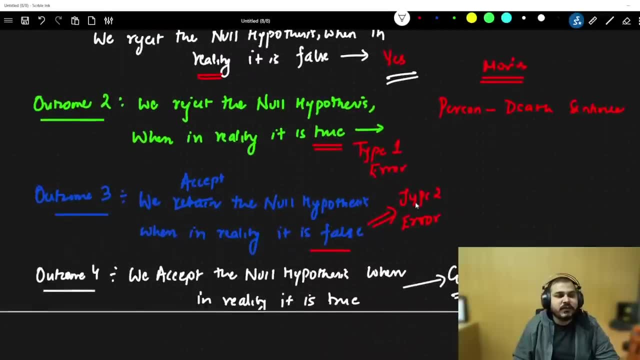 So this is obviously a good case, right? So here I can say that, fine, this decision and this decision are perfectly fine. But whenever we have this scenario, we basically have to consider it as type 1 and type 2 error. So I hope everybody is getting it right. 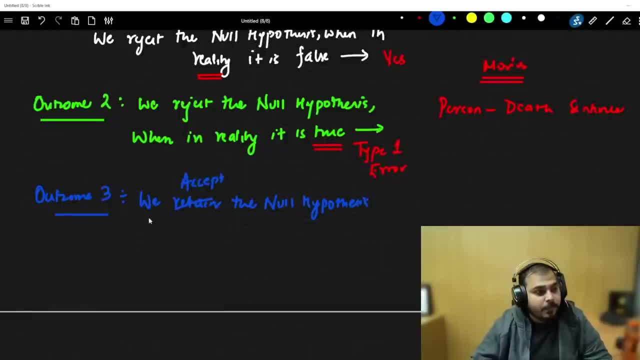 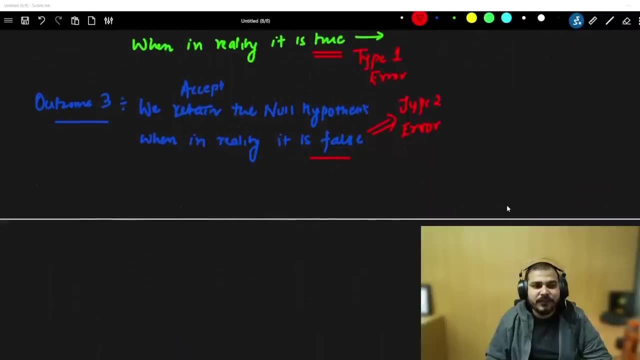 we accept the null hypothesis when in reality it is false. Is this a good decision? The answer should be no, So this error is basically called as type 1 error. Only 4 outcomes will be there. 4 outcome will definitely be there. So here you can understand. 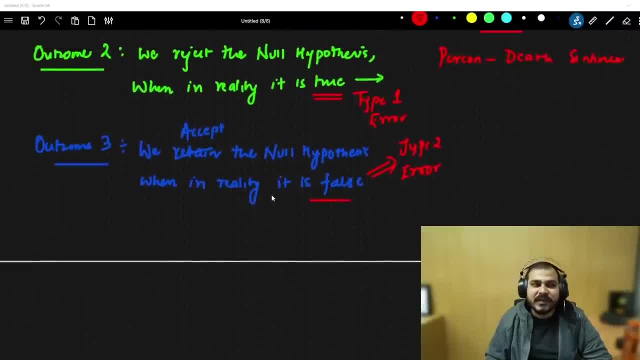 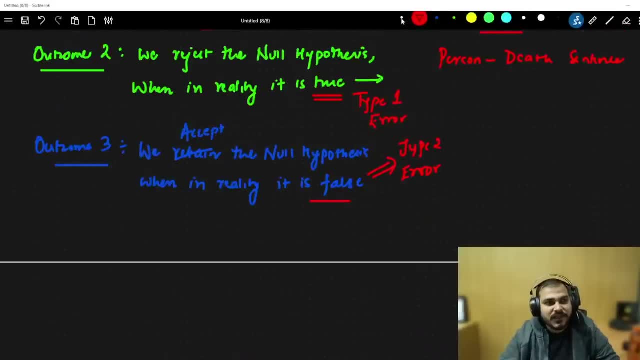 that in this particular case, even though the person has committed crime, he is not acuted So definitely. this error is basically called as type 2 error. Okay, I hope everybody is got is clear right Now let us go to outcome 4.. Outcome 4 is that we accept the 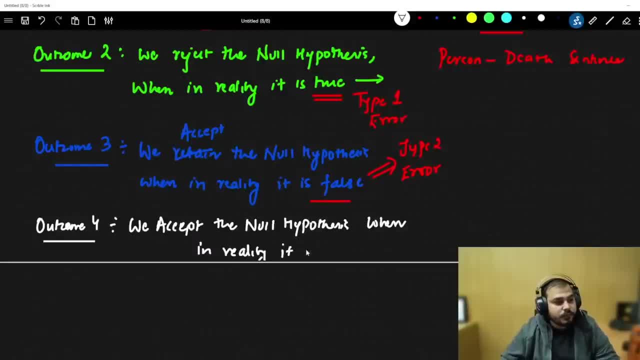 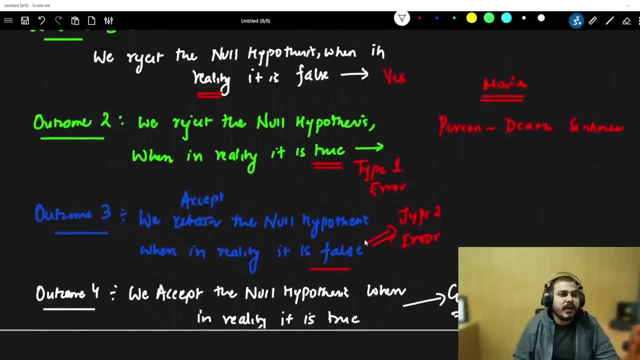 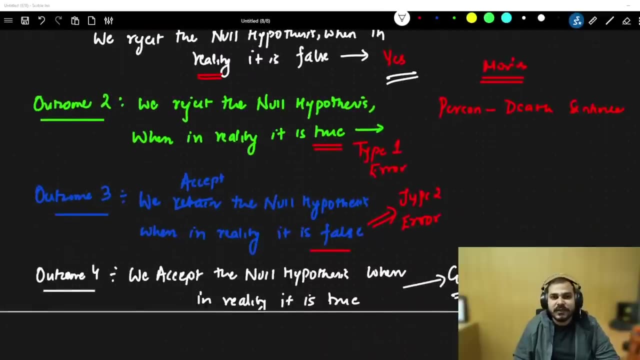 null hypothesis, when in reality it is true. So this is obviously a good case, right? So here I can say that, fine, This decision and this decision are perfectly fine. But whenever we have this scenario, we basically have to consider it as type 1 and type 2 error. So 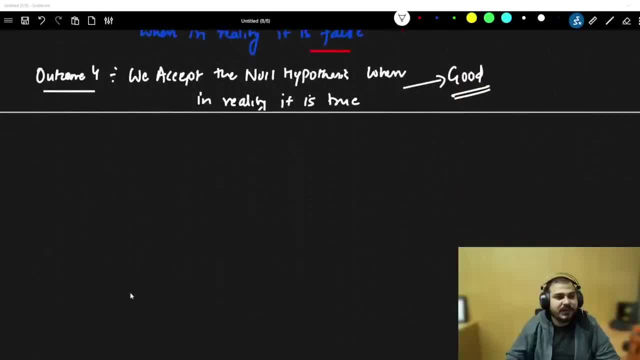 I hope everybody is getting it right. So, similarly, in the real world scenario, you define something called as confusion matrix. right In confusion matrix. what do you have? You have true positive, true positive, right, Sorry, true false and just a second In confusion. 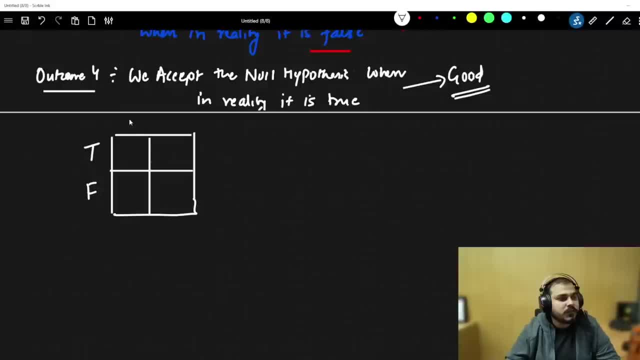 matrix. what you have, You have true, false positive, negative, right. So here you are basically defining your true positive, true negative, false positive, false negative, right. So this basically becomes your true positive, true negative, false positive, false. 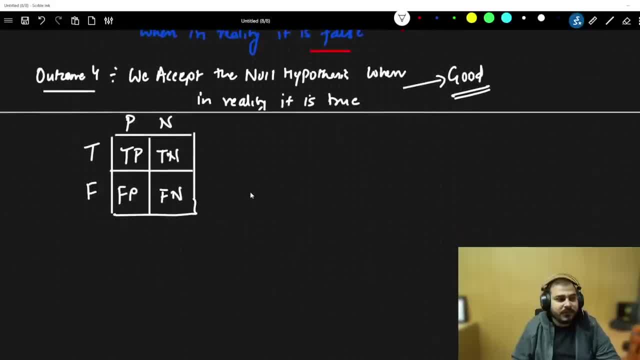 negative. Tell me out of this, which is type 1 and type 2 error. Either this can be type 1 or type 2 error. that will be a answer for you. So you have to tell me, okay, whether. 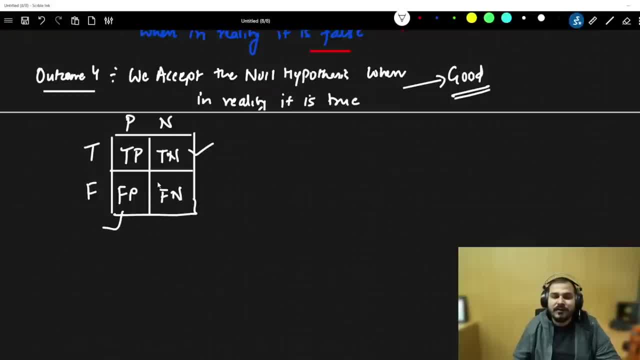 false positive will be a type 1 error. A true negative will be type 2 error or vice versa. Perfect. So this will be one assignment to you. If you don't know, just check out my one of my video. you will be able to see it. 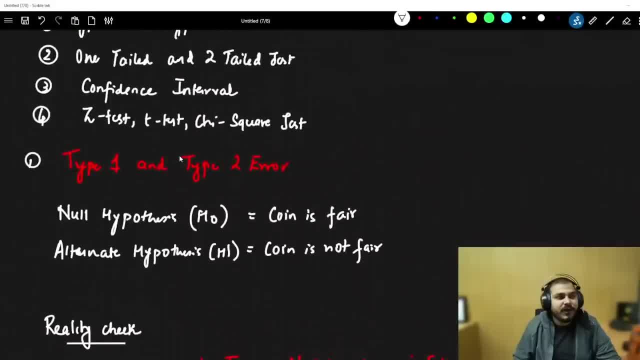 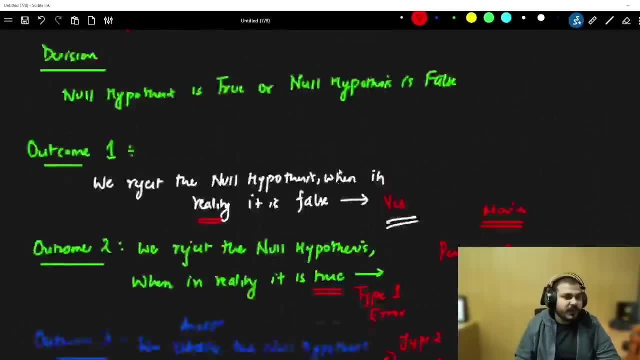 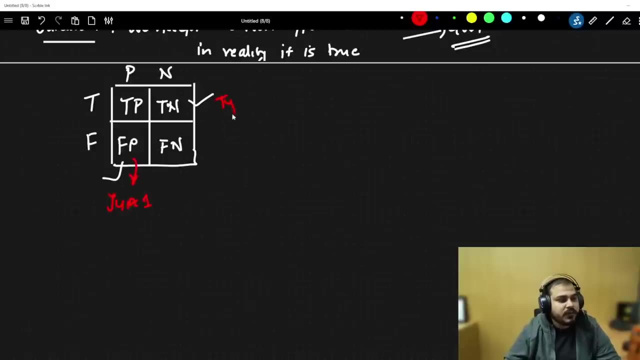 But clear guys, was this explanation good for type 1 and type 2 error? So we have completed this specific topic, that is, type 1 and type 2 error, Perfect. So some people are basically saying false positive is type 1, true negative is, Fp is type 1.. So 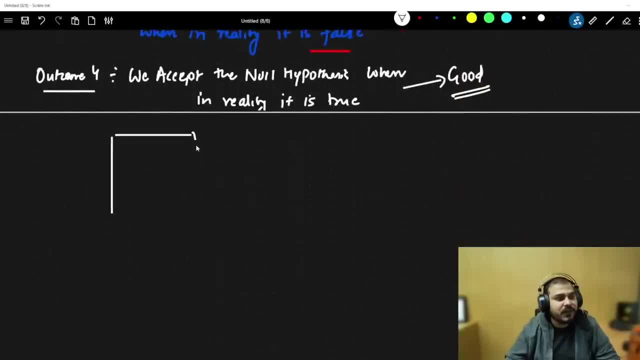 So, similarly, in the real world scenario, you define something called as confusion matrix. Right In confusion matrix, what do you have? You have true positive, true positive right- Sorry, true, false and just a second In confusion matrix. what are? what do you have? 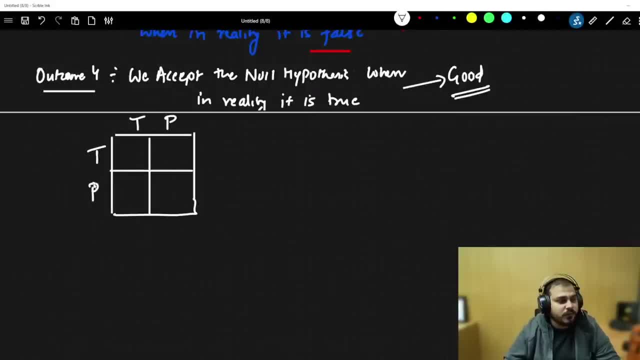 You have true, false positive, negative right. So here you are basically defining your true positive, true negative, false positive, false negative right. So this basically becomes your true positive, true negative, false positive, false negative. 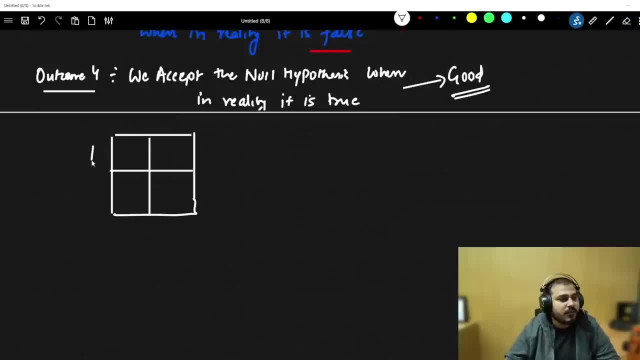 So here you are basically defining your true positive, true negative, false positive, false negative, right, So this basically becomes your true positive, true negative, false positive, false negative. So here you are basically defining your true positive, true negative, false positive, false. 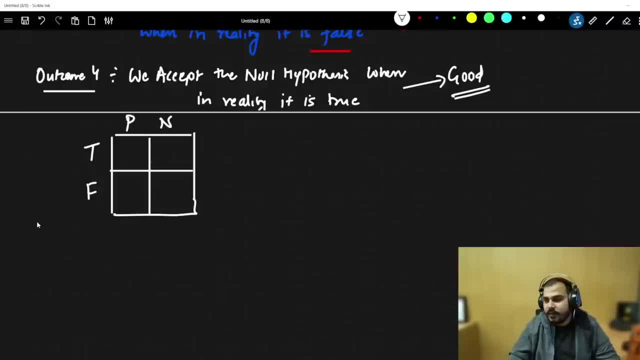 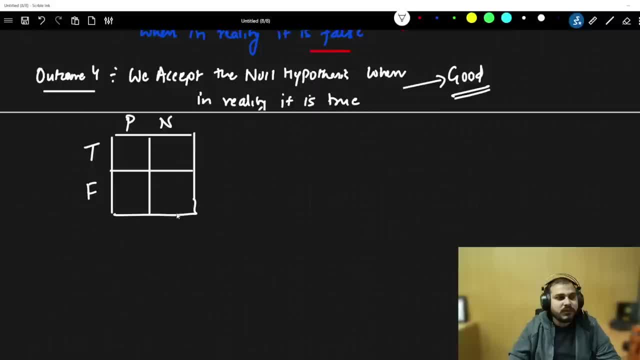 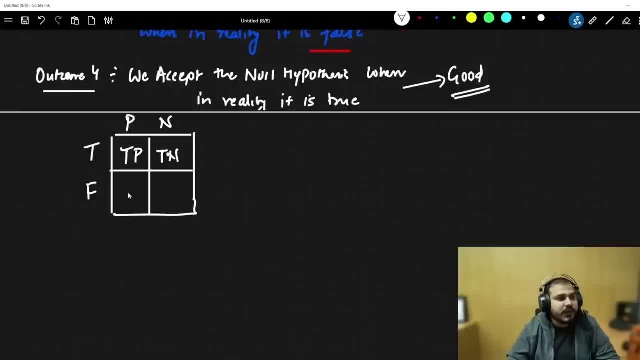 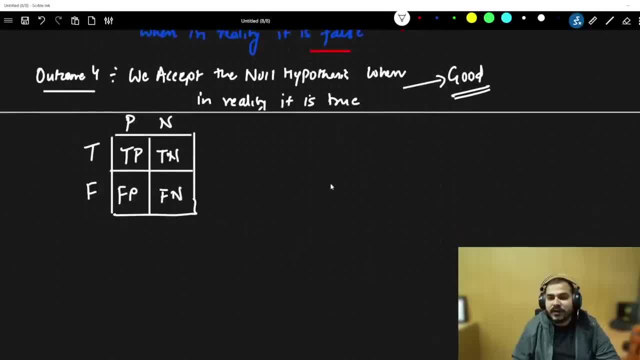 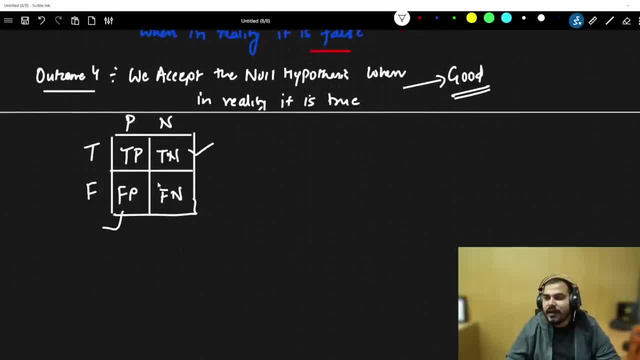 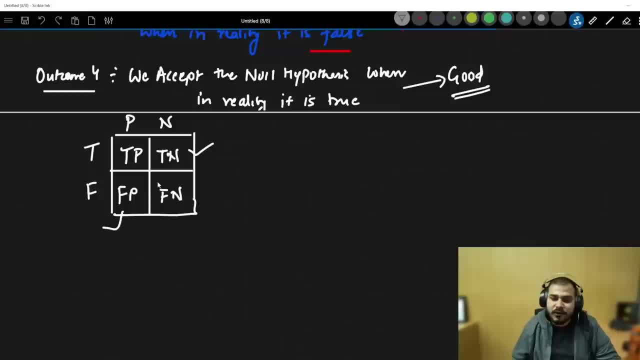 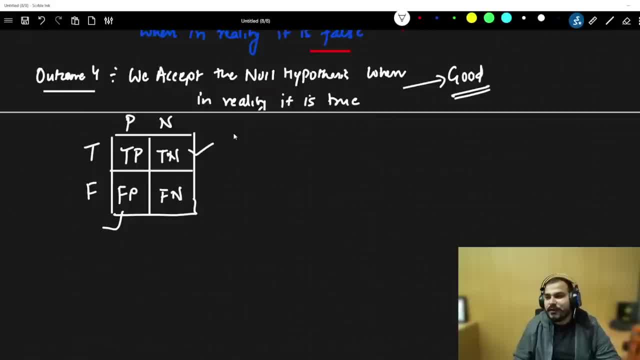 false negative, false positive, right? So here you are basically defining your true positive, true negative, false positive, false negative, false positive, right? So here you are basically defining your true positive, true negative, false positive. 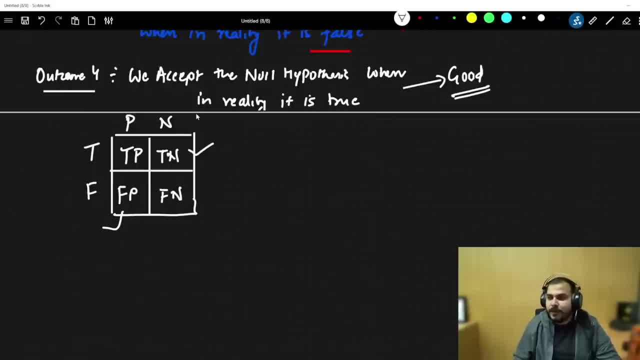 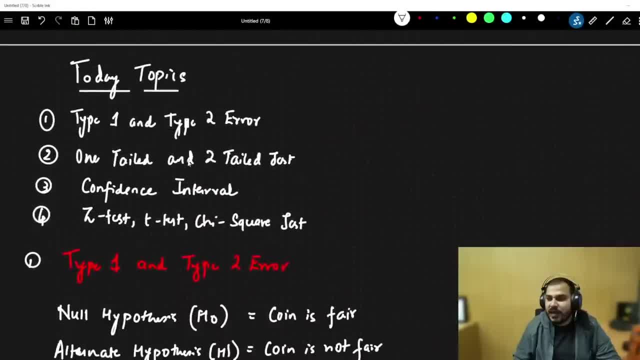 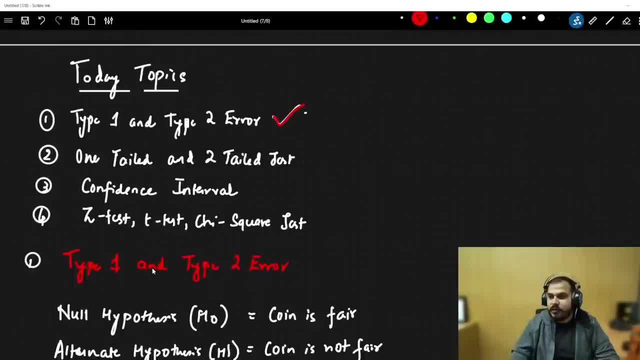 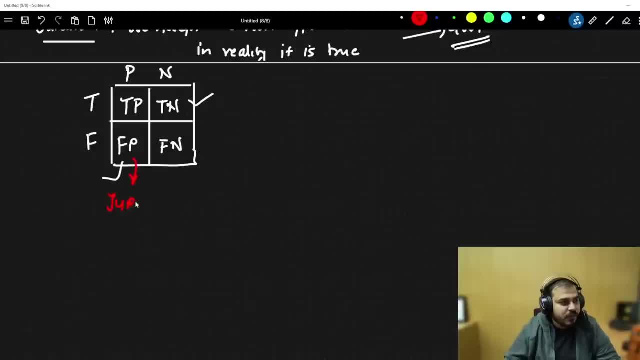 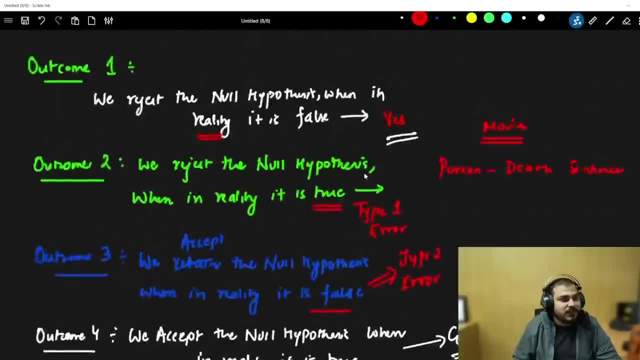 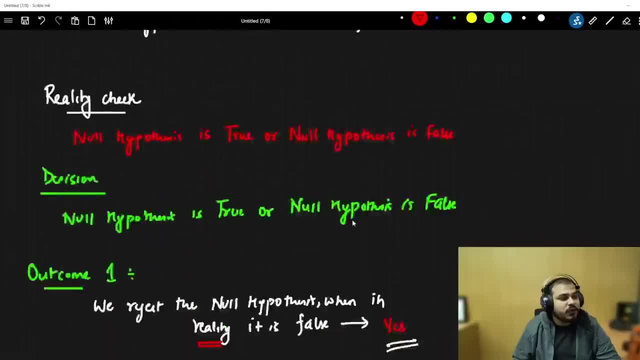 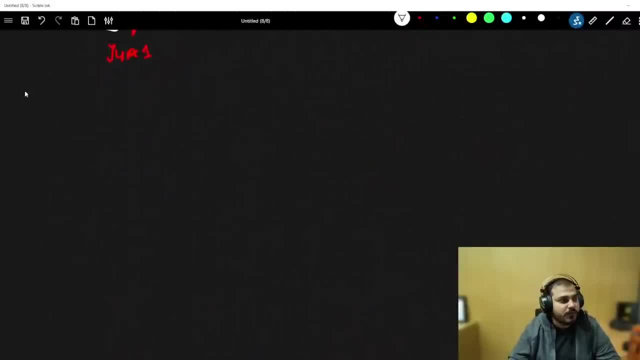 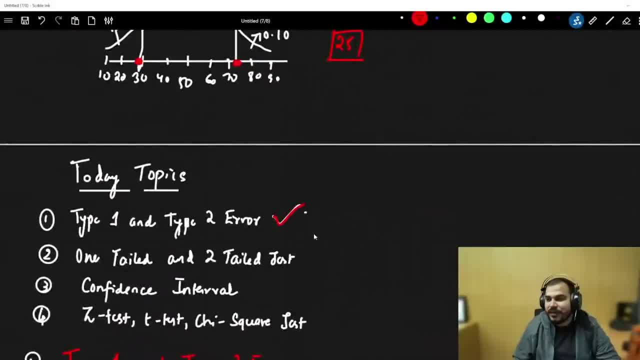 here you have to define your true positive, true negative, false positive, false negative, false positive. So if you have actually solved a very good topic, which is called as type 1 and type 2, error, Now let's go to the next topic that is one-tailed and two-tailed. 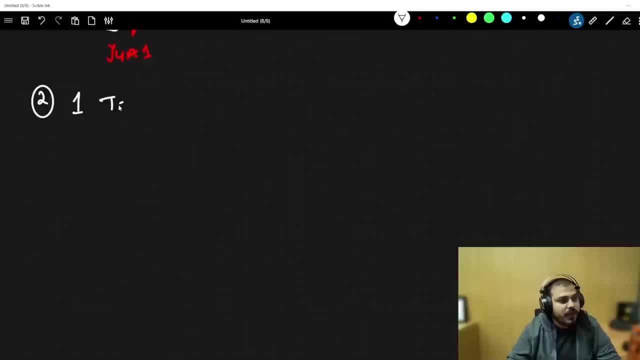 test. This is also very much super important. One-tailed and two-tailed test. So one-tailed and two-tailed test. Now let's go ahead and let's try to understand what is one-tailed and two-tailed test. Now, already you have seen that I have probably drawn a curve, a 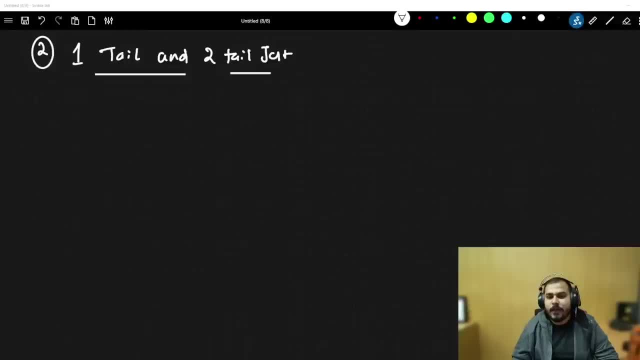 bell curve, and in that I basically define a kind of one-tailed and two-tailed test. Still, you have seen it, but let me give you one good example. Okay, So the example is that a college in let's say a college, or let me write like this, Colleges in Karnataka, 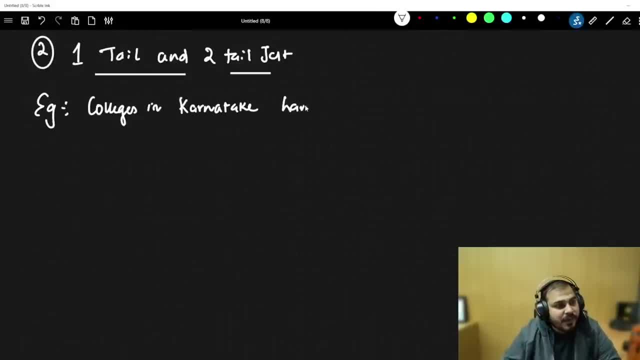 in Karnataka have an 85% placement rate. placement rate in the placements type: A new college. a new college was recently opened and it was found that a sample of 150 students had a placement rate of 88%, with a standard deviation 4%. Does this, does this college have or has? 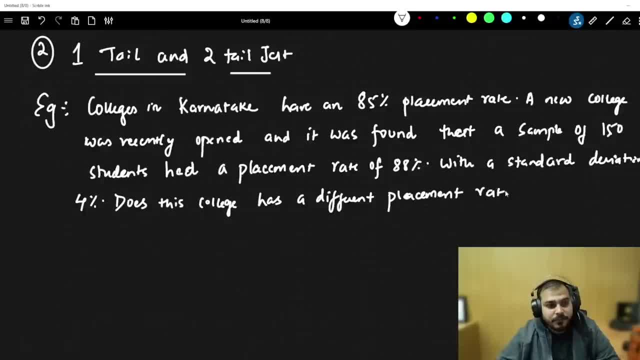 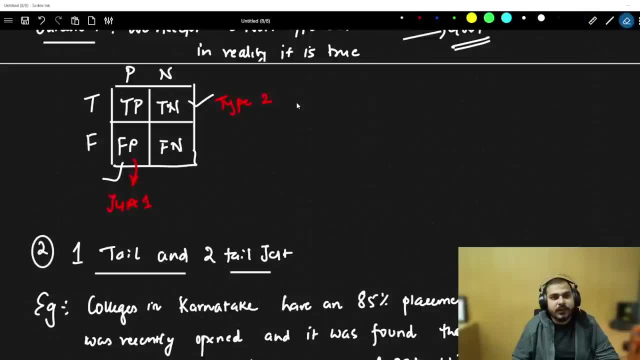 a different placement rate than the other colleges. Okay, So understand this question very much important. Oops, sorry guys, I made one mistake. This should not be type 2.. False negative should be type 2, right, True positive and true negative. 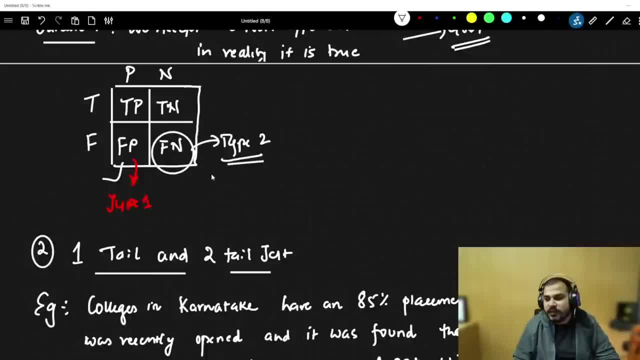 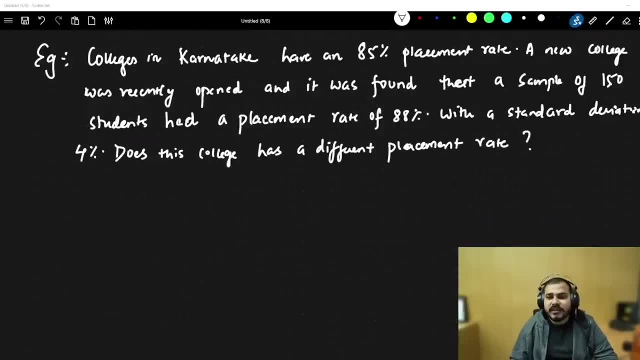 are perfectly fine. Okay, This should be type 2.. True positive and true negative are always right. Let's try to understand some very important thing Now. what does this question basically say? Whether see there are colleges in Karnataka which has 85% placement rate, A new college. 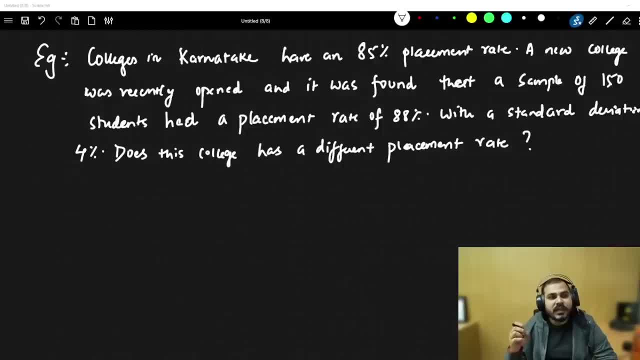 was recently opened and it was found that a sample of 150 students had a placement rate of 88%, with a standard deviation 4%. Does the college has a different placement rate? Does this college? This basically means the new college? Now, in this particular case, first, 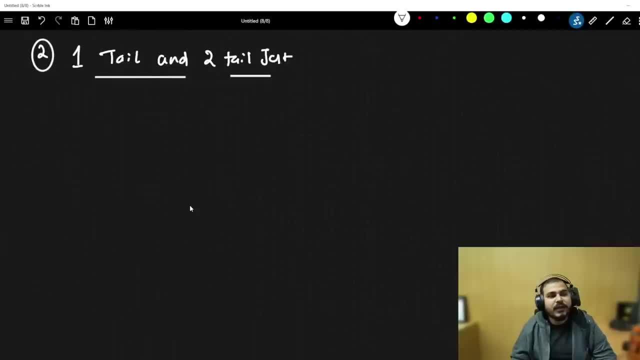 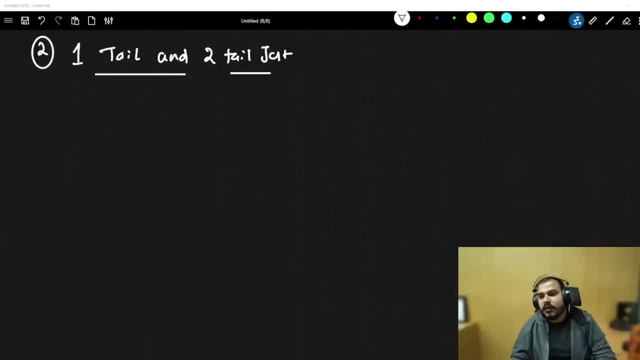 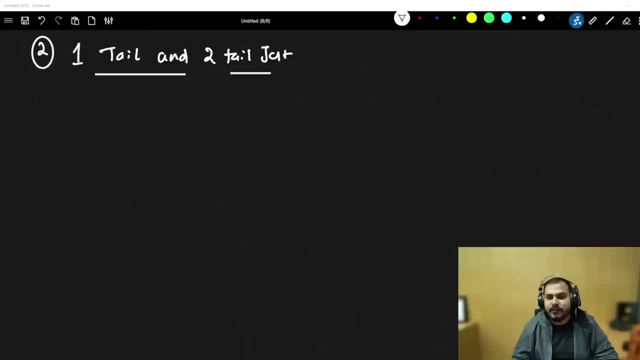 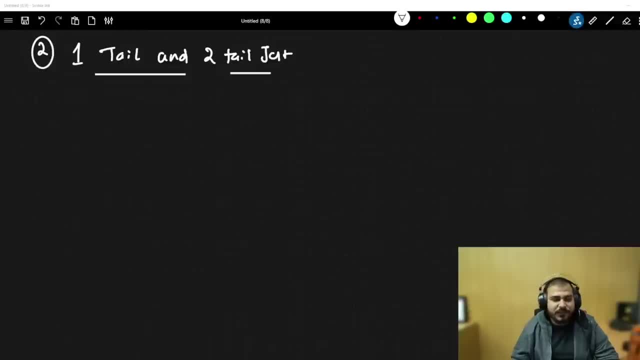 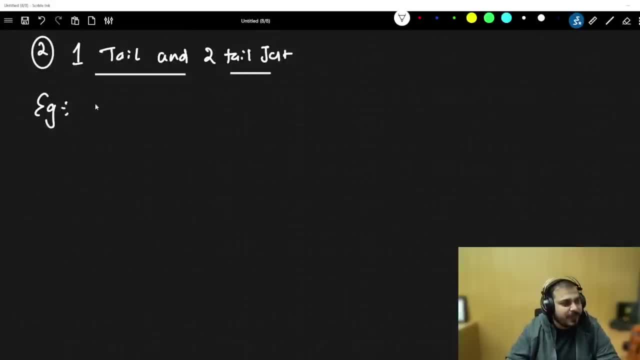 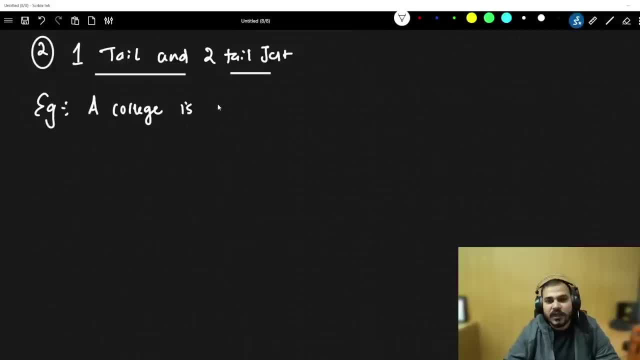 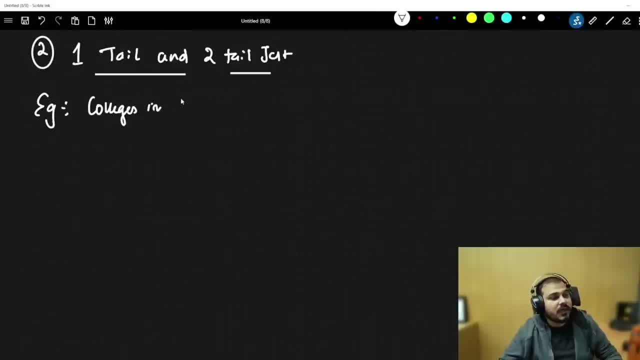 So here you are, basically defining your true positive, true positive, false positive positive, right. So now let me just write it like this: Colleges in Karnataka have an 85% placement rate. A new college was recently opened and it was found that a 90% sample of 150 students had 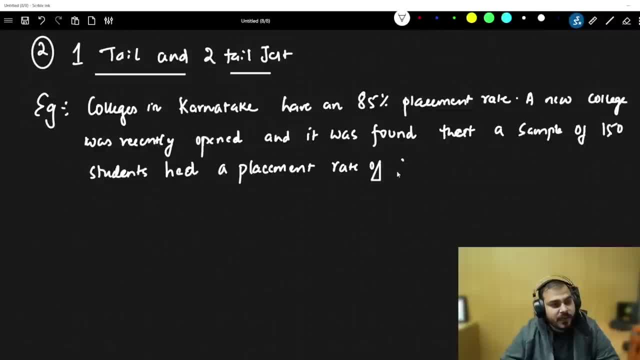 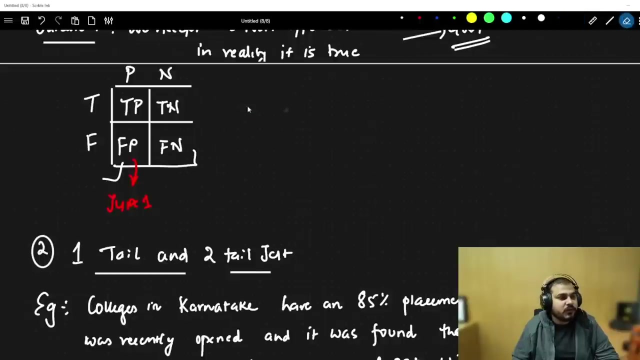 a placement rate of of 88 percent, with a standard deviation four percent. does this? does this college have or has a different placement rate than the other colleges? okay, so understand this question very much important. oops, sorry guys, i made one mistake. this should not be type 2. false negative should be type. 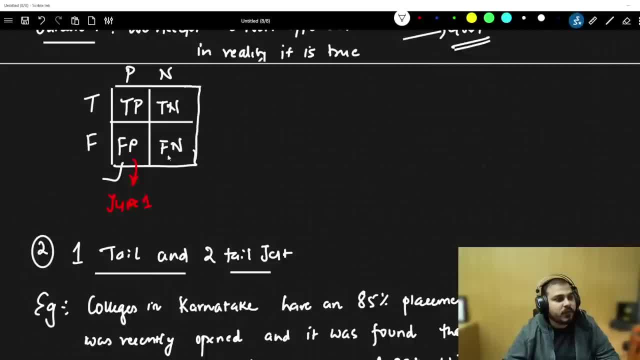 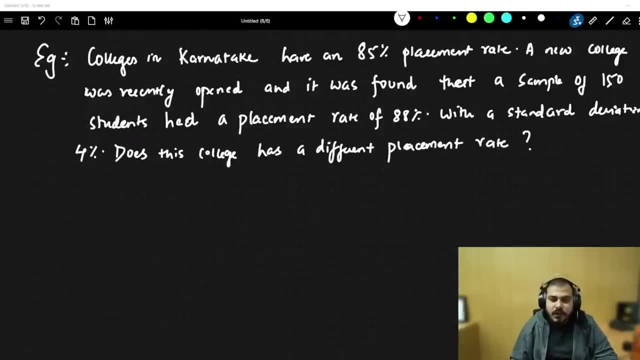 2 right. true positive and true negative are perfectly fine. okay, this should be type 2: true positive and true negative are always right. let's try to understand some very important thing now. what does this question basically say? whether, see, there are colleges in karnataka, which has 85. 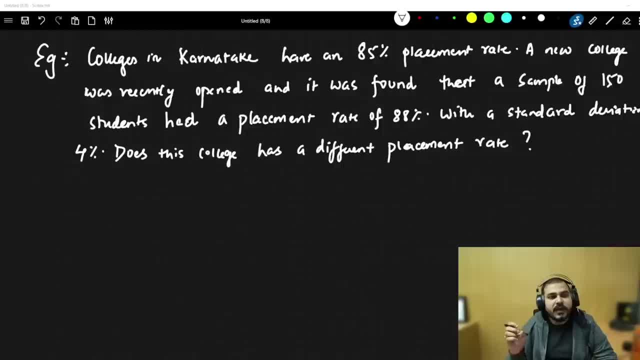 percent placement rate. a new college was recently opened and it was found out that a sample of 150 students had a placement rate of 88 percent, with a standard deviation four percent. thus, the college has a different placement rate. does this college? this basically means the new college? now, in this particular case, first of all, 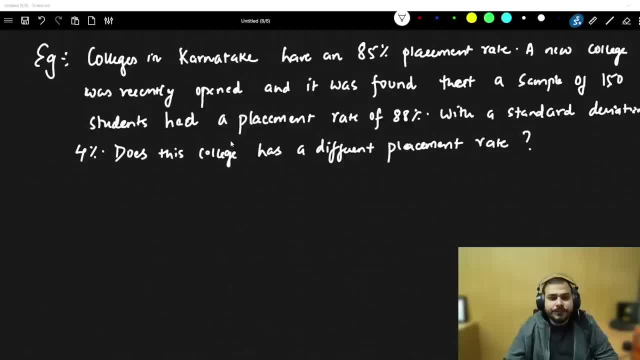 of all, think about the question Now. overhead says: does this college has a different placement rate? What is the placement rate of the entire college? 85%. So does it have a different rate than 85%? That is why I said 85%. Now, you see, in Karnataka there are colleges in. 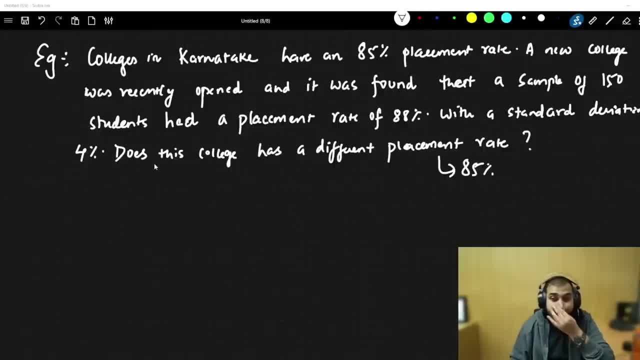 Karnataka, which have 85%. does it mean they have a different placement rate than the other? That is what we really need to check right Now. in this particular case, this becomes a two-tailed test, Why We'll think over it. 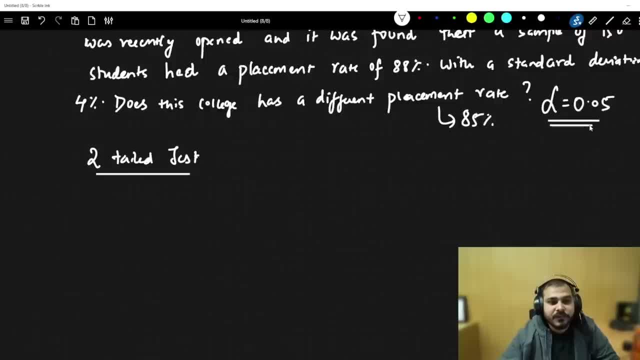 Let's say that here the significance value is given as 0.05.. Let's consider. Let's consider that over here the significance value is given as 0.05.. Now, what we do over here is that we will try to create a graph. 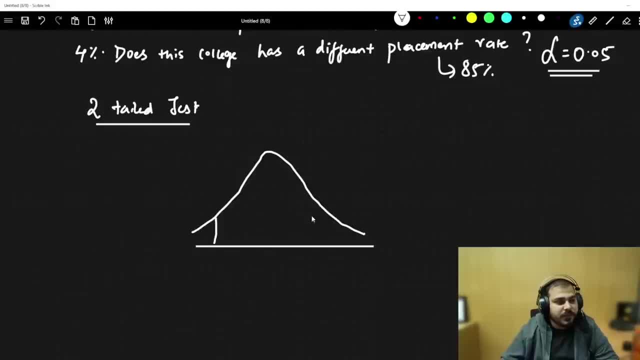 Now when we have 0.05, that basically means if it is a two-tailed test. two-tailed test basically means right now I have a placement rate of 85%, So 85% is you can just consider that. 85% will be what in this particular case? right? 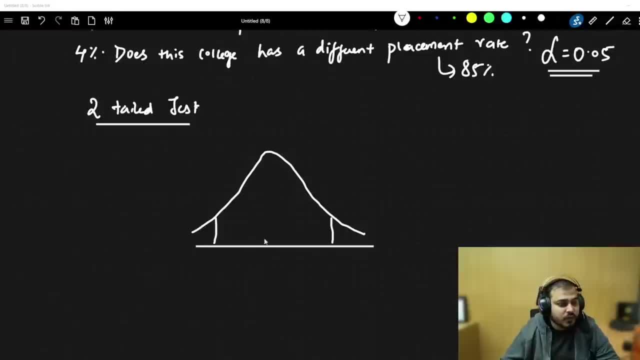 85% passage rate or, sorry, placement rate. right, So 85%, but we need to find out over here when alpha is given, 2.5 will be here and this will be my 95% confidence interval. So 95 will be 0.05.. 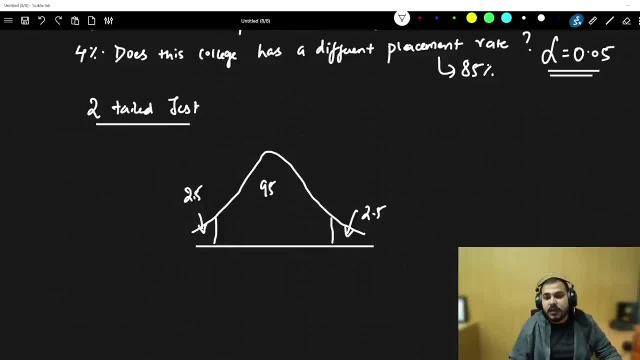 It will basically be here. If I combine all these things, it will become 1.. Now you need to understand whether this will become a two-tailed test or a one-tailed test. This is what is very much simple. Now, this 85% will be my mean. 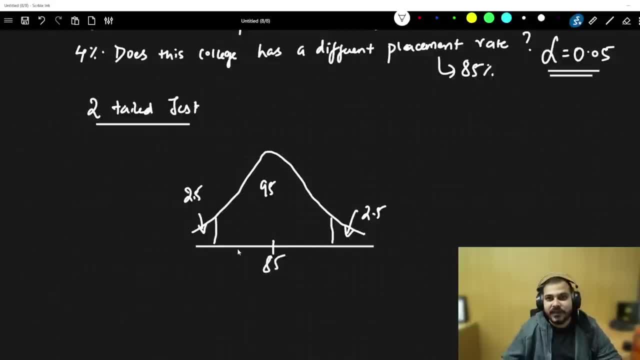 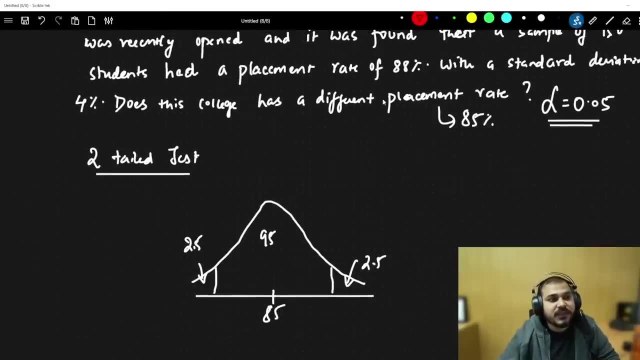 My value can be greater than 85.. It can be less than 85.. It can be greater than 85.. It can be less than 85 because we are just checking whether it has a different placement rate. It can be greater, It can be less also. 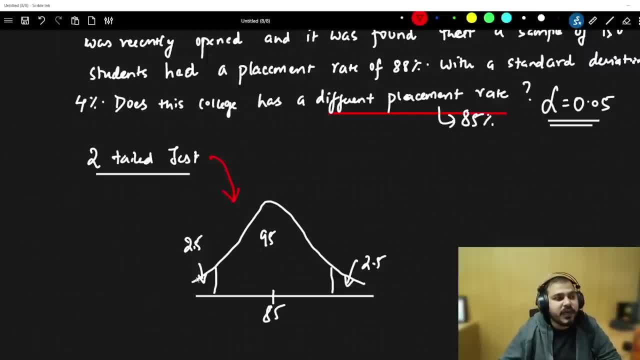 So that is the reason this entire test becomes a two-tailed test, because the new college that gets added, it may fall in this region also. it may fall in this region Right now. you'll be able to see that we are just trying to check whether it is greater. 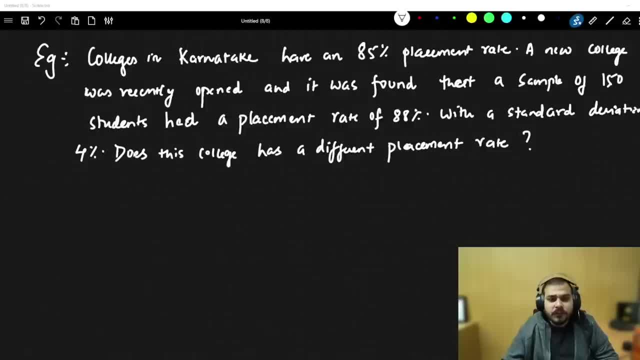 think about the question now. overhead says: does this college has a different placement rate? what is the placement rate of the entire college? 85 percent. so does it have a different rate than 85 percent? that is what we really need to check right now. in this particular case, this becomes a two-tail. 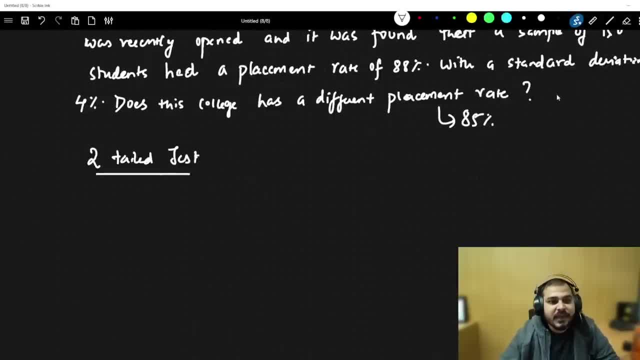 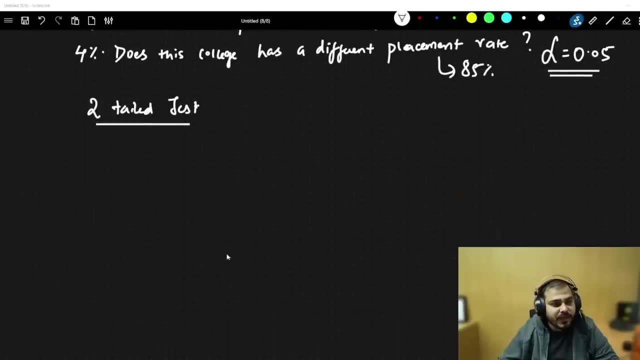 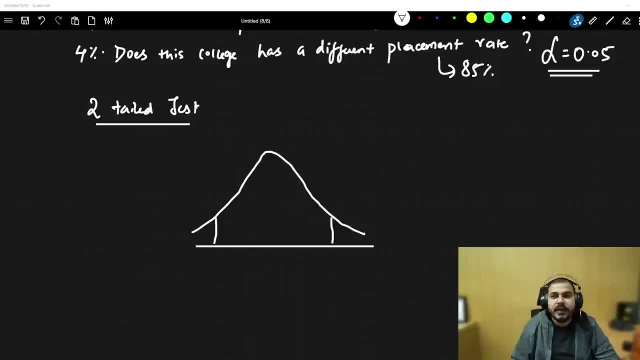 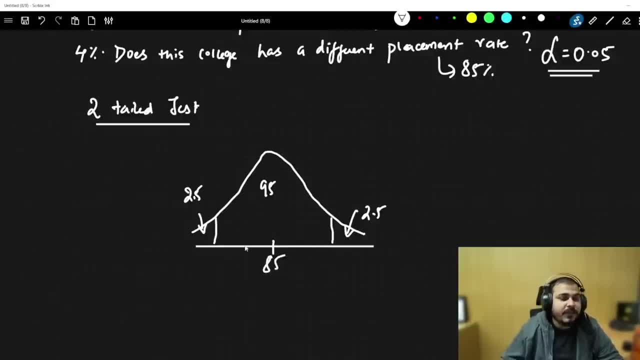 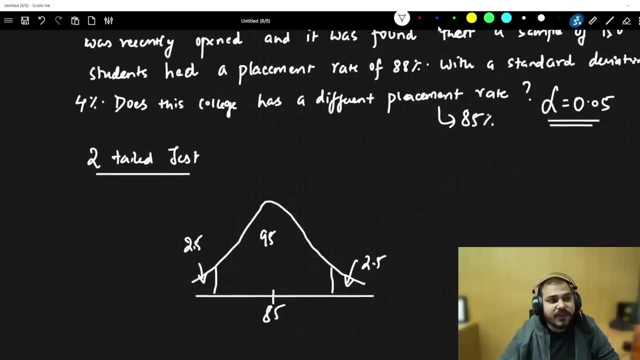 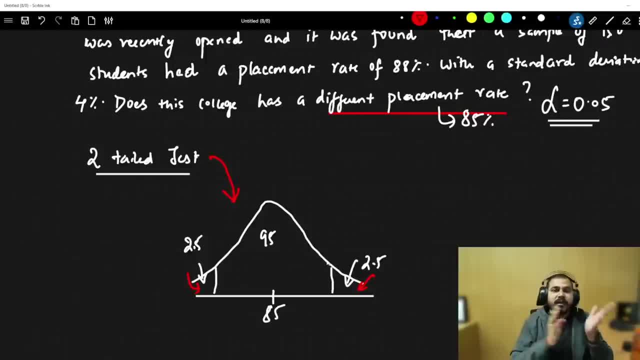 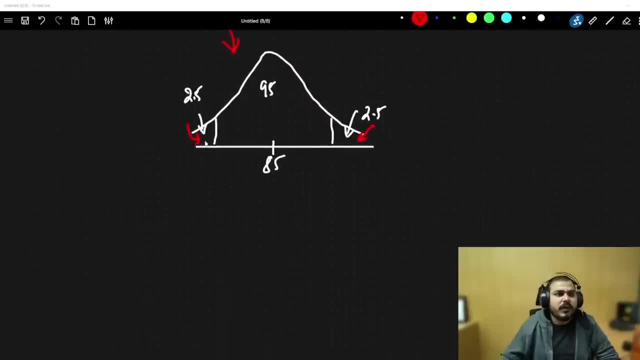 are just trying to check whether it is greater than 85 or whether it is less than 85, so this becomes a two-tailed test. now let me just make a little bit change into the question. now my question says that let's say: let's say that my question- i'll just change the question saying that does. 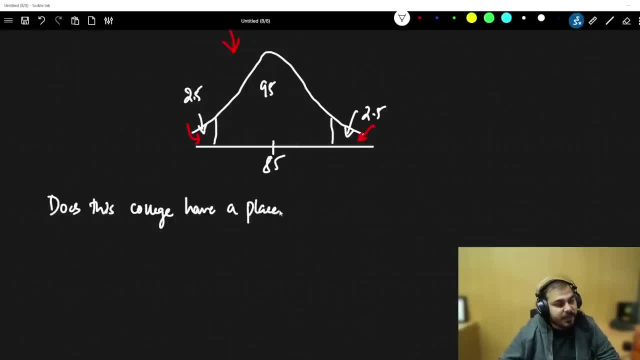 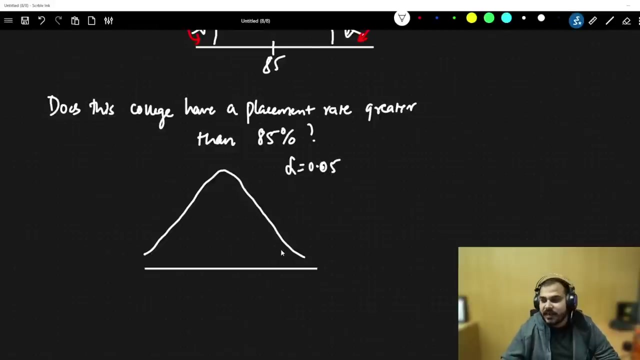 this college have a placement rate greater than 85 percent. now, what now? what will this be? greater than 85 percent. think over it. what this will basically be. yeah, what this will be. now, my question will look like this: this is my, this. my alpha value is 0.05. obviously it is 95 percent. 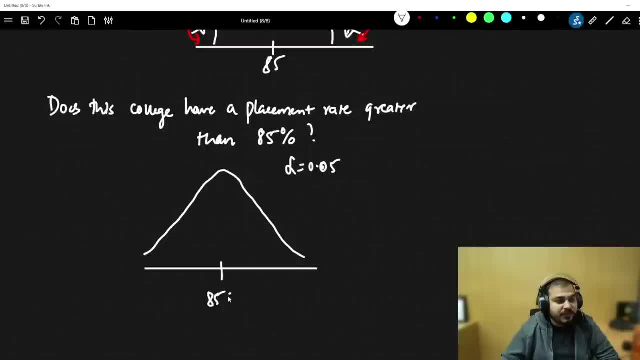 confidence interval, but this is only focused in finding greater. so this entire value i'll put over here and this region will be my five value. this region will be my 95 percent value, so this becomes one. you A one-tailed test. that also in the right hand side, because here the important keyword is: 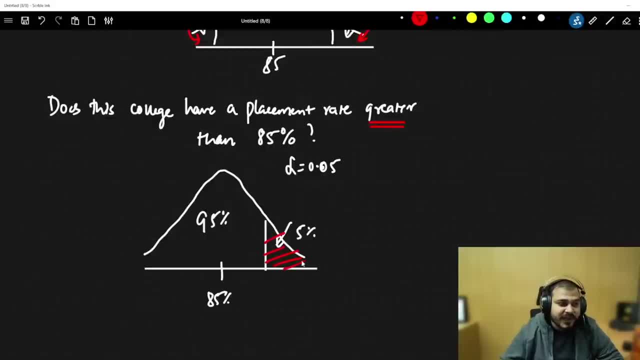 something called as greater. so this becomes a one-tailed test. and remember, we cannot divide this alpha value into two parts. in this case, only in one part. it will be basically present. now just think over it. if this value is lesser, then what will happen? it will come in this: 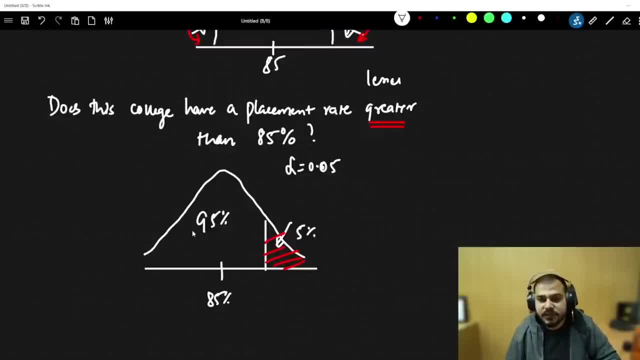 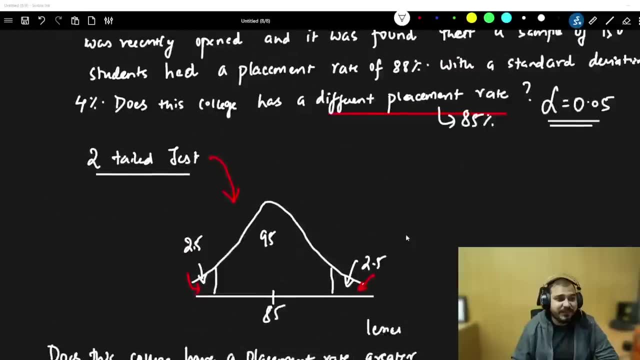 particular side. so i hope you are understanding what is the difference between one tail and two tailed test? so always make sure that focus on the question. what the question is basically said area does this college has a different placement rate from the experiment. any experiment that i may carry on, my answer will be either greater than 85 or less than. 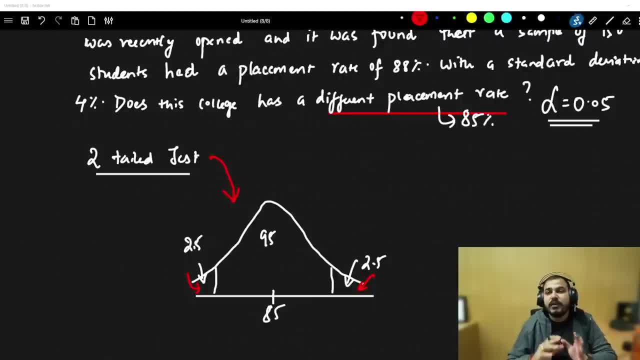 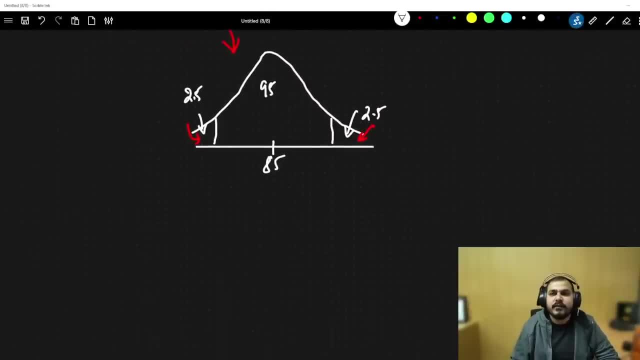 than 85 or whether it is less than 85.. So this becomes a two-tailed test. Now let me just make a little bit change into the question. Now my question says that let's say: let's say that my question, I'll just change the. 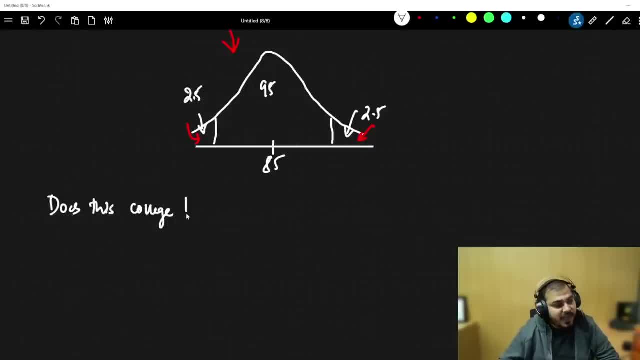 question saying that: does this college have a placement rate greater than 85%? Now, what? now? what will this be Greater than 85%? Think over it. What this will basically be, Yeah, What this will be. Now my question will look like this: 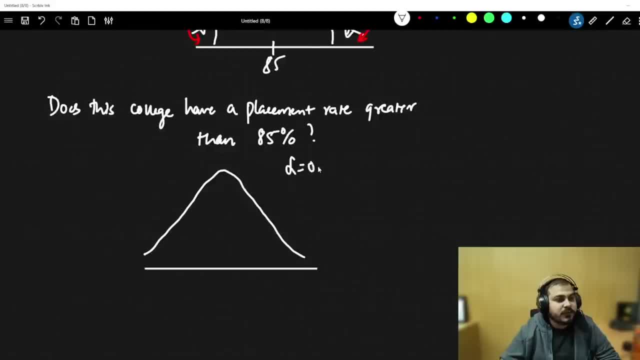 This is my this. My alpha value is 0.05.. Obviously, it is 95% confidence interval, But this is only focused. It is focused in finding greater. So this entire value I'll put over here and this region will be my 5 value. 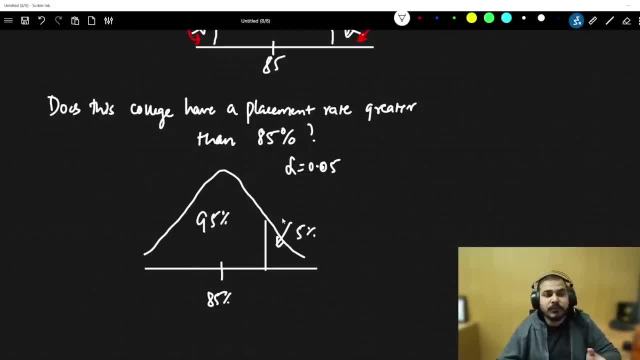 This region will be my 95% value. So this becomes one one-tailed test. That also is the right-hand side, because here the important keyword is something called as greater. So this becomes a one-tailed test. And remember, we cannot divide this alpha value into two parts in this case. 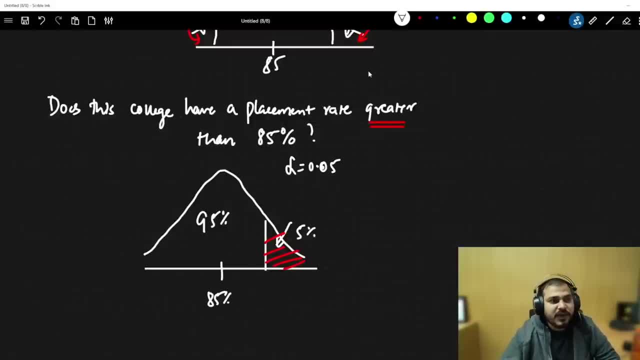 Only in one part. it will be basically present. Now just think over it. If this value is lesser, then what will happen? It will come in this particular side. So I hope you are understanding what is the difference between one-tailed and two-tailed. 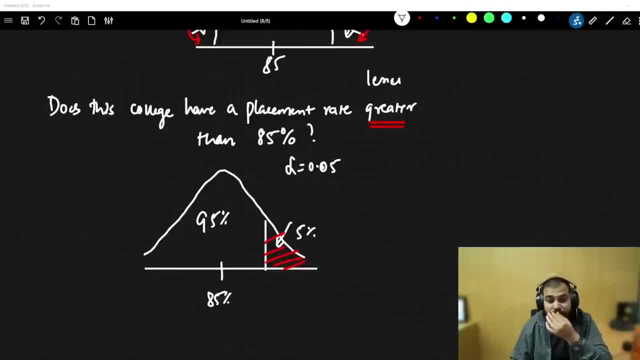 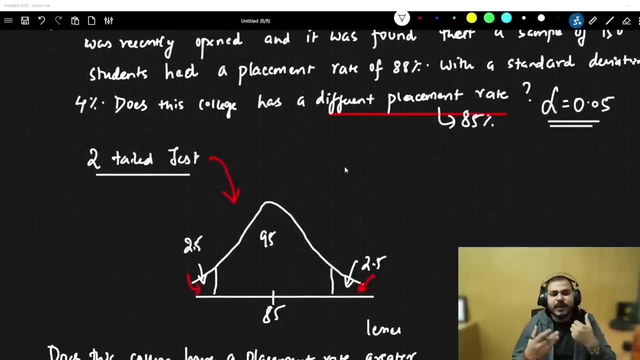 test. So always make sure that focus on the question. what the question is basically said Here does this college has a different placement rate From the experiment. any experiment that I may carry on. my answer will be either greater than 85 or less than 85.. 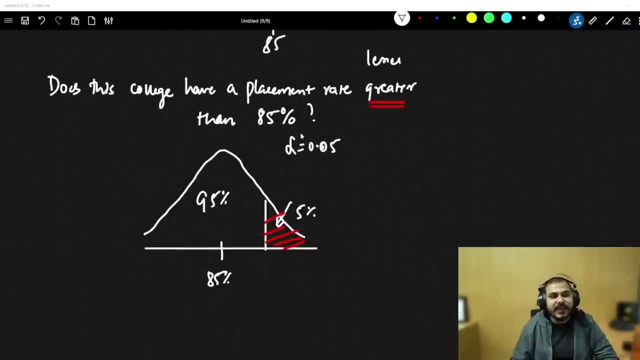 So that becomes a two-tailed test. In this particular case, I'm saying greater than 85%. With alpha values It is 0.05.. So I'm definitely sure that I'm actually checking only this region. I'm not worried at this particular region because I need to check whether it is greater. 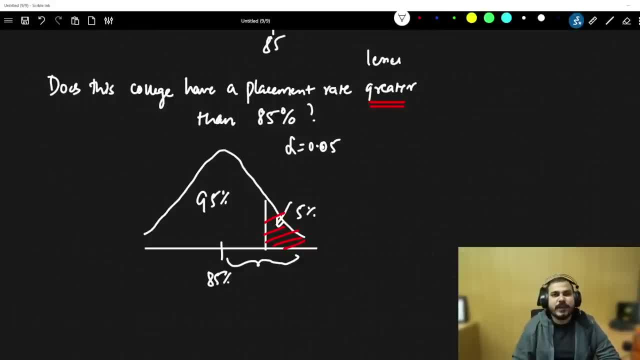 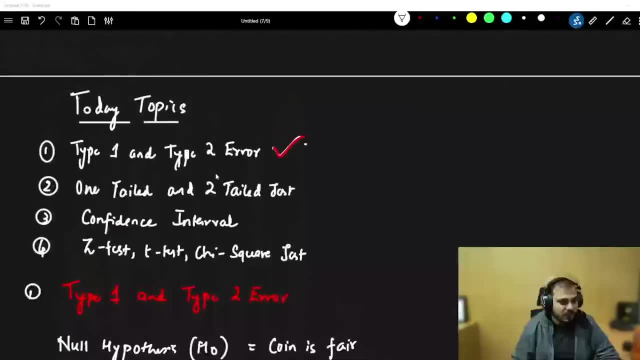 than 85.. This is the most important thing with respect to one-tailed and two-tailed test. Now the next thing that we are going to discuss about is: so we have finished one-tailed and two-tailed also. Now let's go ahead and understand how to find out this confidence interval. 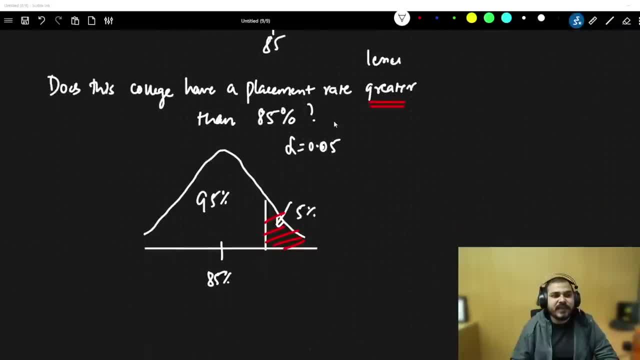 85, so that becomes a two-tailed test. in this particular case i'm saying greater than 85 percent with the alpha value 0.05. so i am definitely sure that i am actually checking only this region. i am not worried at this particular region because i need to check whether it is. greater than 85. this is most important thing with respect to the boiler. this is the most important thing. this is ley kind of. this is why you are going to do the number of case and see the mark. this is not set to the representative. this is what you do not have no information about it, so all you have to Clerk for an. 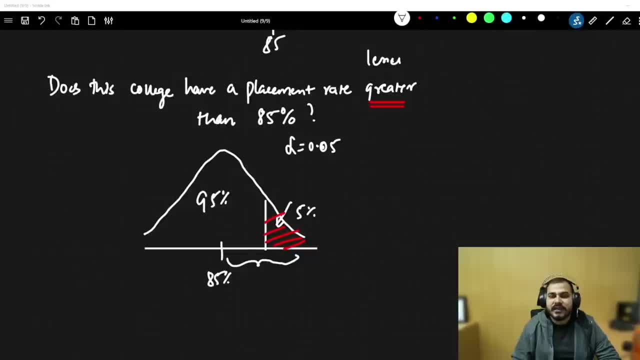 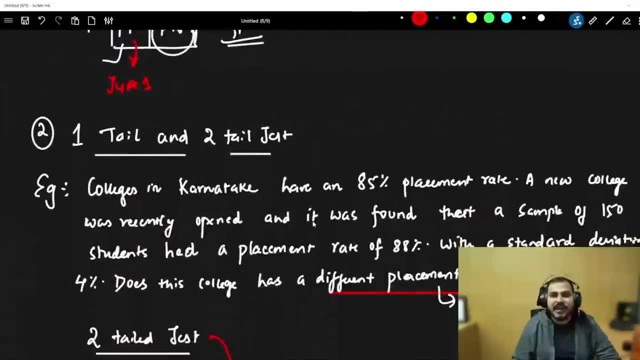 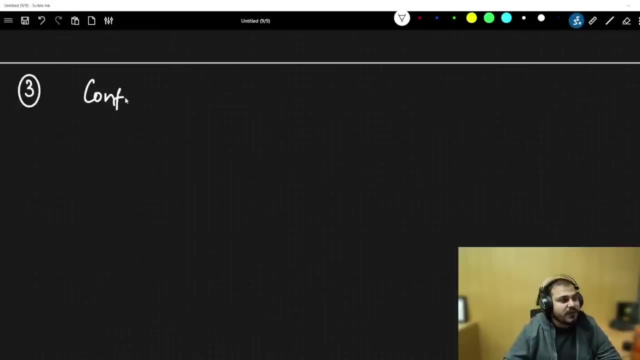 with respect to one tail and two tail test. Now the next thing that we are going to discuss about is: so we have finished one tail and two tail also. Now let's go ahead and understand how to find out this confidence interval. I told you right? See, this is very much important: Confidence. 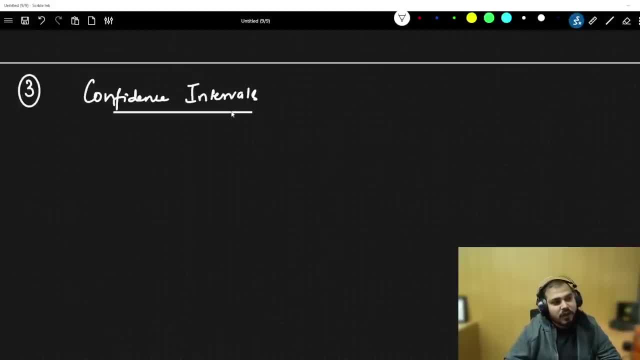 intervals. with respect to means, I told you right Confidence interval, what we do. We basically have this graph. When I say my alpha value is 0.05, then this becomes a two tail test. Suppose I need to find this value right, I need to find these two values. How do I find out these two? 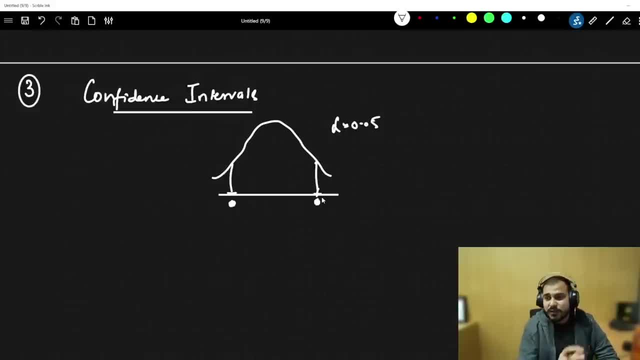 values. That is what we are going to see. We are going to do some kind of calculations which will actually help me to understand. So in order to find out confidence interval, you really need to understand some things. Sir. if it asks less than 85, so it will be considered. 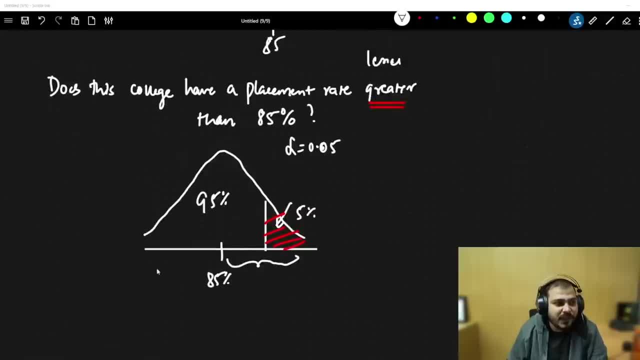 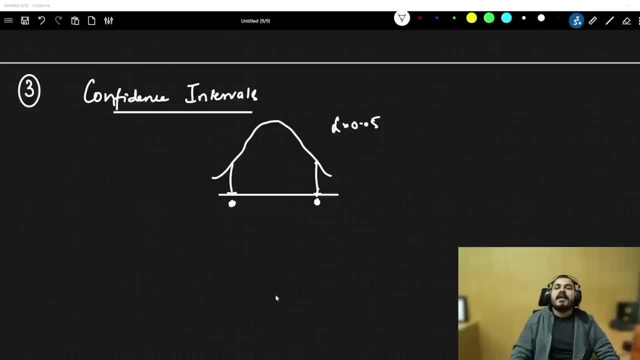 as one tail test. Yes, obviously one tail test, but in the left hand side. Okay, right now, this will be in the right Right hand side. Now let's try to understand. with respect to confidence interval. Now, in order to. 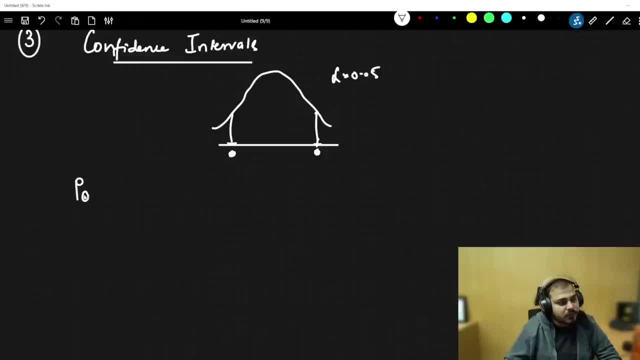 understand confidence interval, you really need to understand a topic which is called as point estimate. Okay, so I will basically give the definition of point estimate. What exactly is point estimate? Point estimate can be defined as a value of any statistic that estimates the value of a parameter is called a point estimate. So a simple definition. 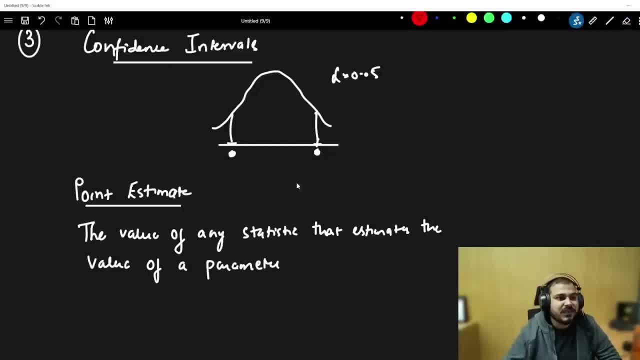 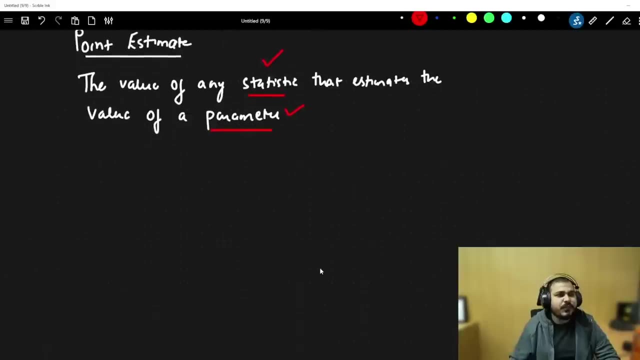 I have written over here. I will define about what is this statistic and which estimates the value of a parameter. So two things: one is statistics and one is parameter. So what exactly is point estimate A value of any statistics that estimates the value of a parameter? Now understand one. 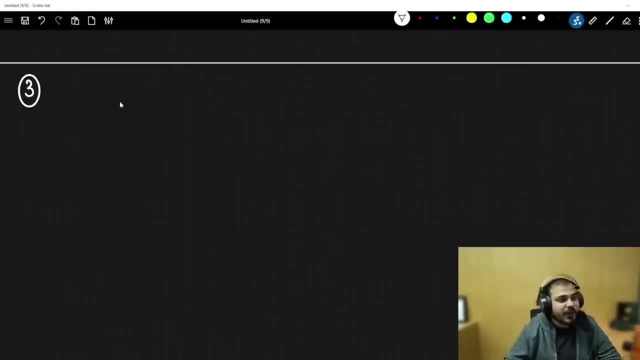 I told you right, See, this is very much important. Confidence intervals: Okay, Confidence intervals with respect to means. I told you right, Confidence interval, what we do, We basically have this graph. When I say my alpha value is 0.05, then this becomes a two-tailed test, suppose. 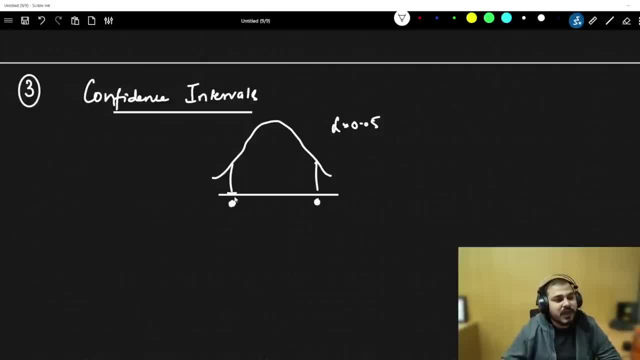 I need to find this value right. I need to find these two values. How do I find out these two values? That is what we are going to see. We are going to do some kind of calculations, which will actually help me to understand. 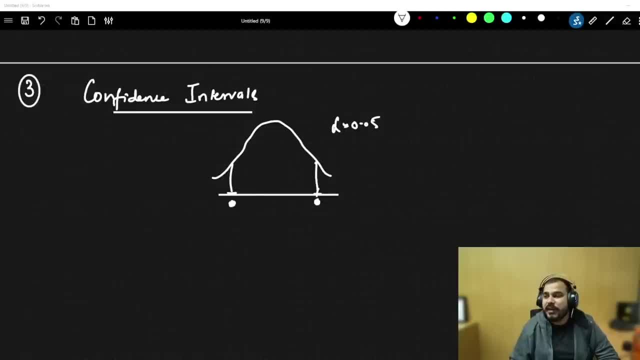 So in order to find out confidence interval, you really need to understand some things, Sir. if it asks less than 85, so it will be considered as one-tailed test. Yes, obviously one-tailed test, but in the left-hand side. 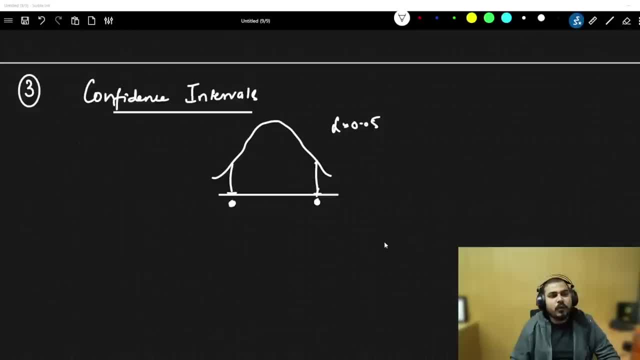 Okay, Right now, this will be in the right-hand side. Now let's try to understand with respect to confidence interval. Now, in order to understand confidence interval, you really need to understand a topic which is called as point estimate. Okay, So I will basically give the definition of point estimate. 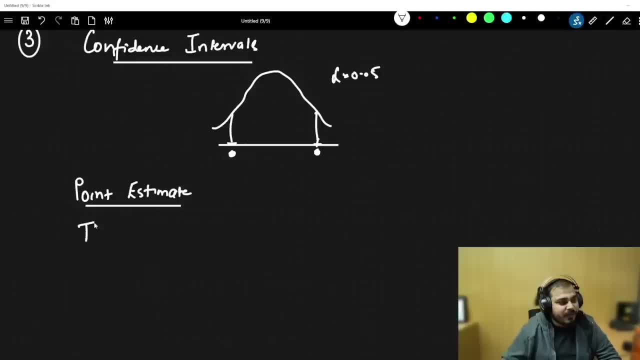 What exactly is point estimate? Okay, So point estimate can be defined as a value of any statistic that estimates the value of a parameter is called a point estimate. So a simple definition I have written over here. I will define about what is this statistic? 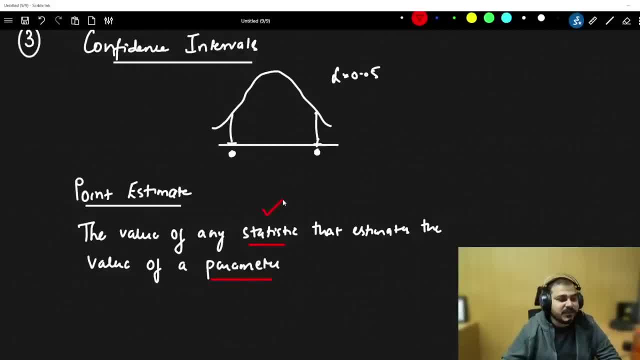 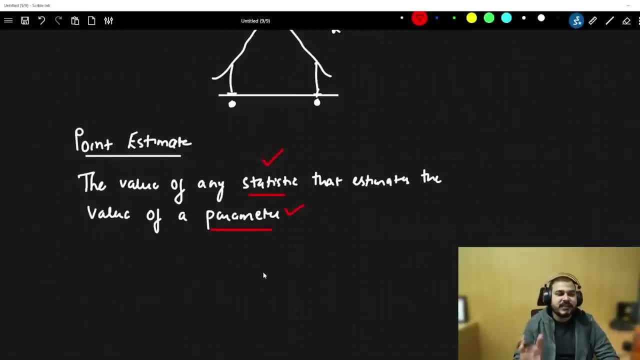 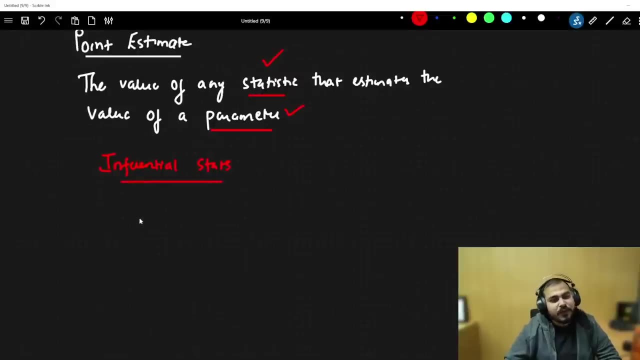 and which estimates the value of a parameter. So two things: One is statistics and one is parameter. So what exactly is point? estimate a value of any statistics that estimates the value of a parameter? Now understand one thing, guys: In inferential statistics, any work that we will be doing, first of all we will be considering 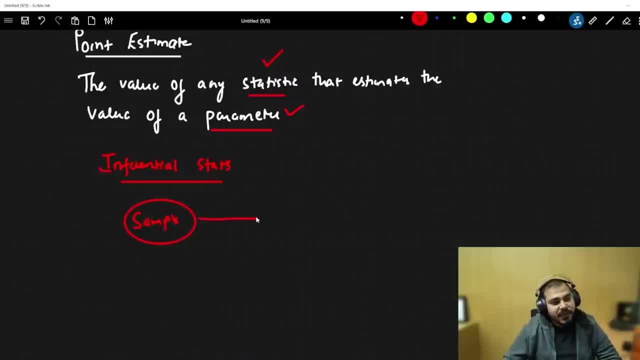 a sample data. Based on this sample data, we will be estimating something for the population data Right In this particular example. let's consider that I will try to. if I have the sample meal, I'll try to estimate the population. 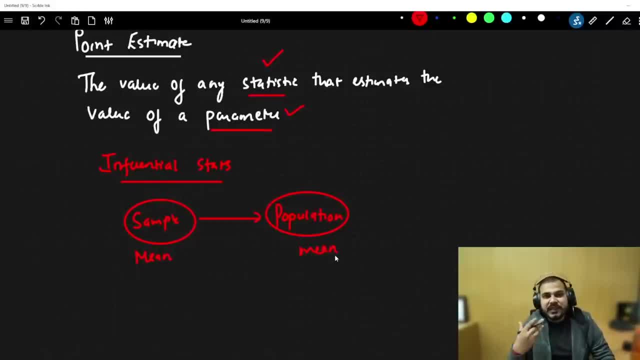 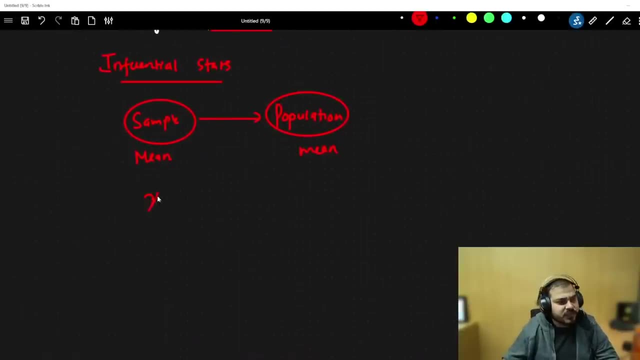 Okay, And usually this only things happens in inferential stats You just have, you'll just have the sample information. probably population standard deviation, you may know, but you really need to find out or estimate the population value And, as you know, like let's say that I'll give one example. 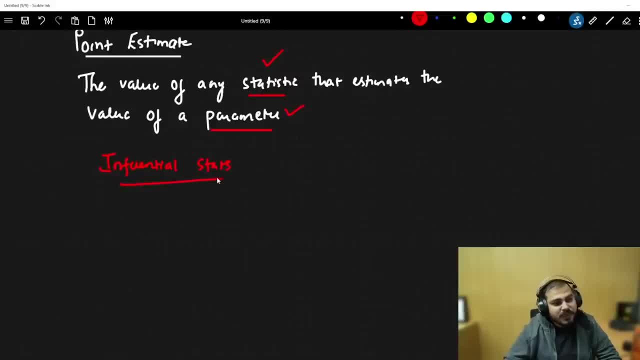 thing, guys: in inferential statistics, the number of parameters is the number of parameters. So any work that we will be doing, first of all, we will be considering a sample data. based on this sample data, we will be estimating something for the population data. 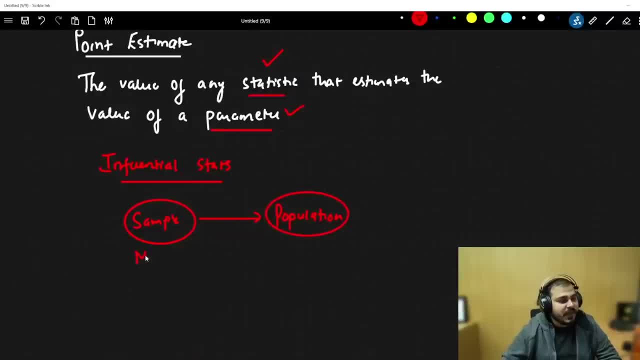 right in this particular example. let's consider that i will try to. if i have the sample meal, i'll try to estimate the population and usually this only things happens in inferential stats you just have. you'll just have the sample information, probably population standard deviation you may. 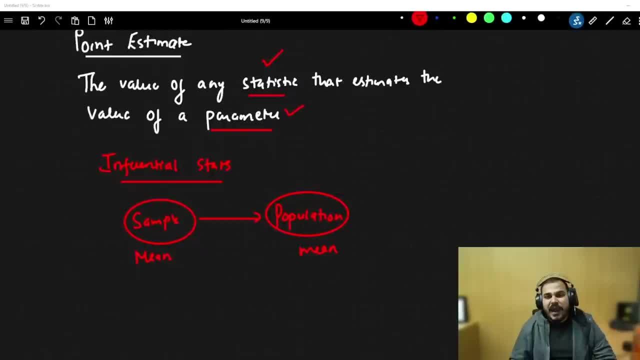 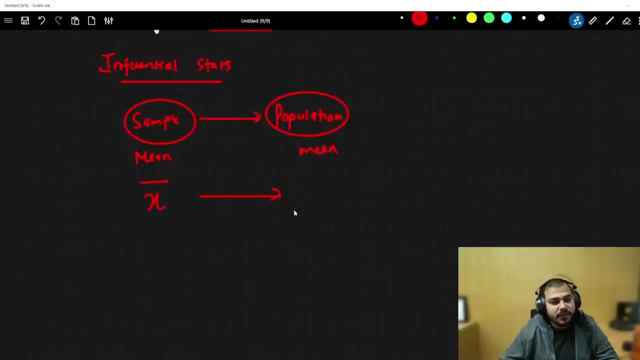 know, but you really need to find out or estimate the population value. and, as you know, like let's say that, i'll give one example, this is my x bar, this x bar, we will try to estimate the value of mu bar right, because if i have a population, with the help of sample, i can definitely estimate mu. 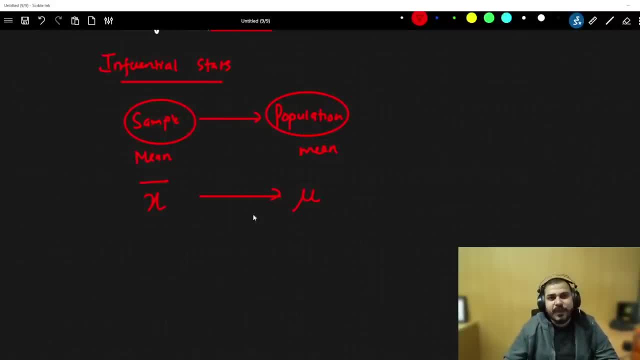 but always remember: this value may be approximately equal to this, it may be also less, it may be also greater. right, let's? in one case, i may say that if my x bar is 2.9 and approximately equal to this, i can always estimate mu, because if i have a population, 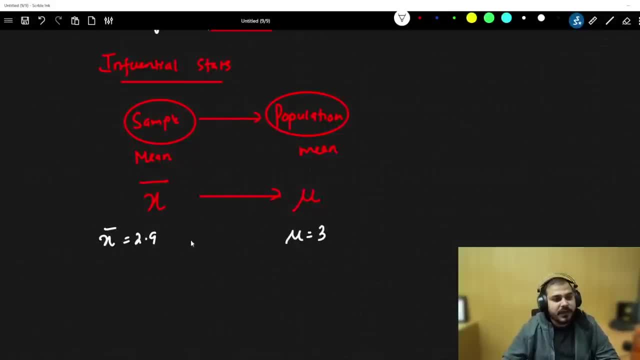 my x bar is 2.9 and approximately equal to this and approximately equal to this. i can always 한번 my population mean is mu is equal to 3, right, This may be equal, this may be less, this may be little bit greater. also, This is what point estimate is all about. So this is the point. 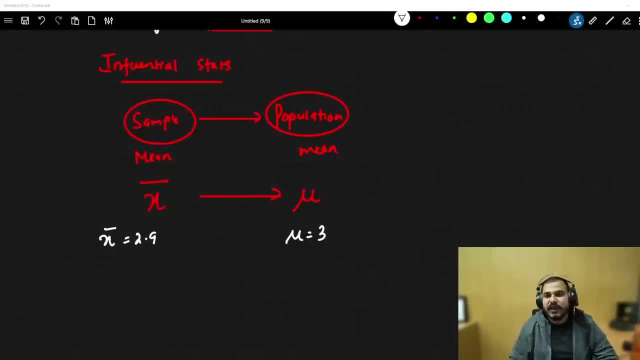 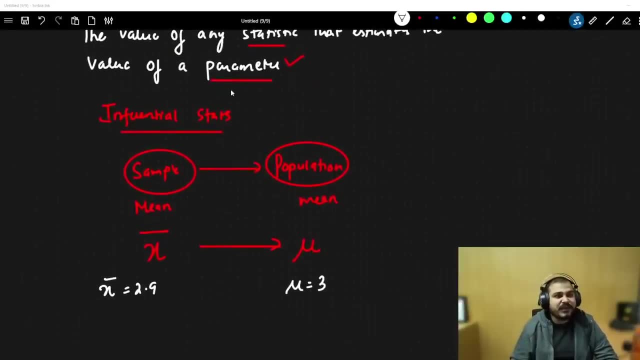 estimate which will be estimating the mu value. So in this particular case, I hope you understood what exactly is point estimate, okay, So point estimate is the value of any statistic that estimates the value of a parameter. So this, through this, we are basically estimating the 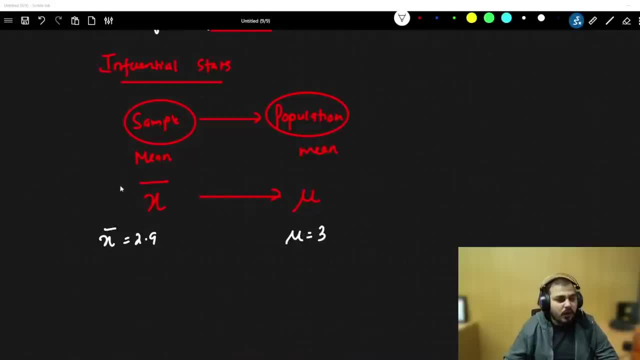 mean. So at least get this specific knowledge. Now, in most of the problem statement I will be given this and I really do need to estimate this. How will I be able to do this? So for that specific case we will try to see a problem statement And here we will something use. 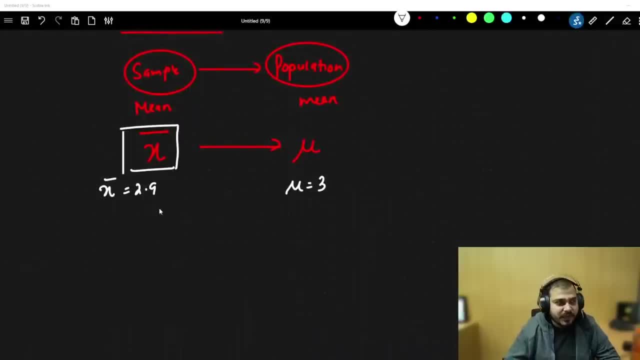 something called as confidence interval. Now understand, I told you that this value will be approximately equal to mean. It may be less than mean, it may be greater than mean. So in this particular scenario, we define something called as confidence intervals So that we will be able to come towards the population mean. So confidence interval is: 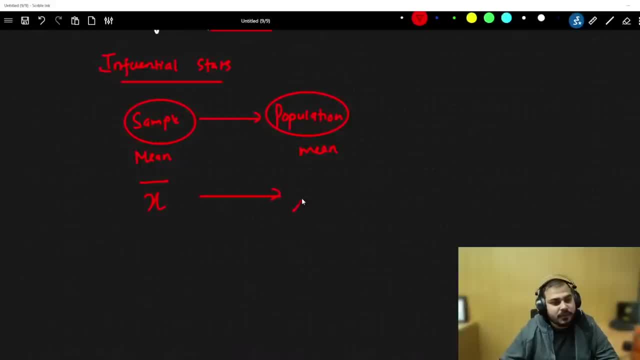 This is my X bar. This X bar, we will try to estimate the value of mu bar right, Because if I have a population with the help of sample, I can definitely estimate mu, But always remember This value. This value may be approximately equal to this. 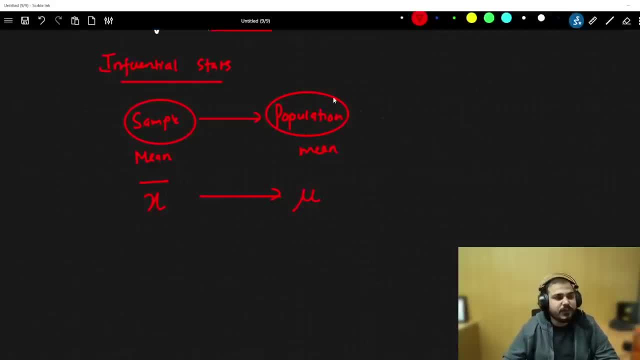 It may be also less, It may be also greater, Right, Let's, in one case I may say that if my X bar is 2.9 and probably my population mean is mu is equal to three, right, This may be equal. 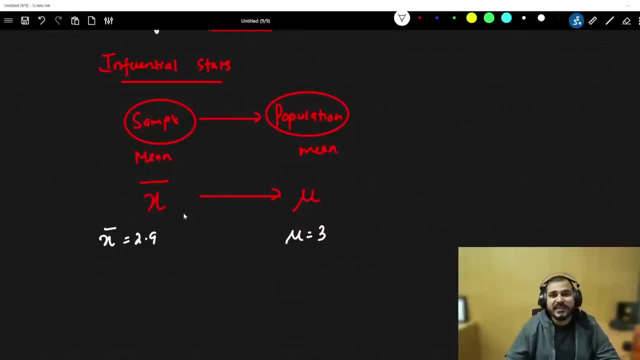 This may be less, This may be a little bit greater. also, This is what point estimate is all about. So point this is the point estimate which will be estimating the mu value. So in this particular case, I hope you understood what exactly is point estimate. 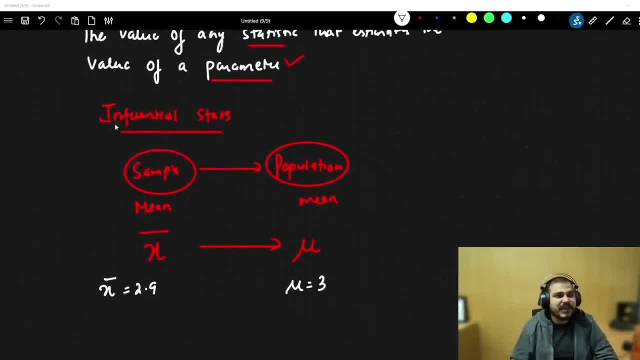 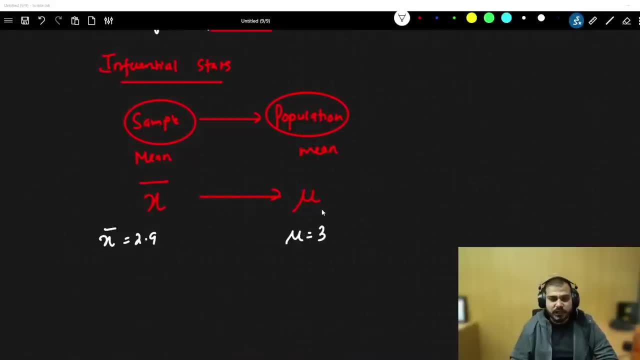 Okay, So point estimate: Okay, So point estimate is a statistic that estimates the value of a parameter. So this, through this we are basically estimating the mean. So at least get this specific knowledge. Now, in most of the problem statement I will be given this, and I really do need to estimate. 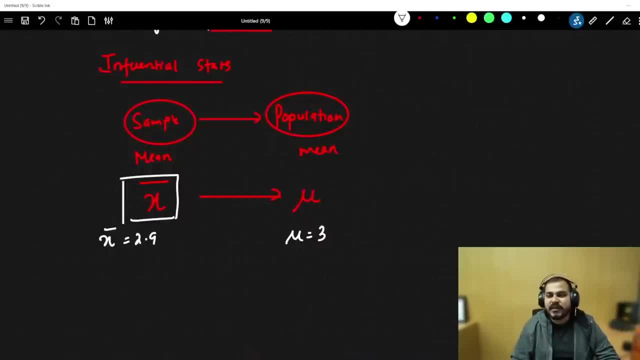 this. How will I be able to do this? So, for that specific case, we will try to see a problem statement And here we will something use, something called as confidence interval. Now understand, I told you that this value will be approximately equal to mean. 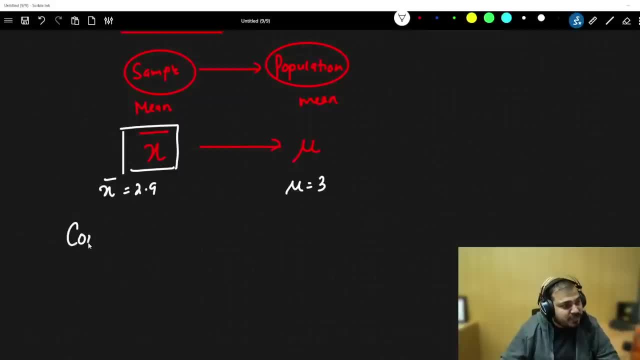 It may be less than mean, It may be greater than mean. So in this particular scenario, we define something called as confidence intervals, so that we will be able to come towards the population mean. So confidence interval is usually given by the formula, which is nothing but point estimate. 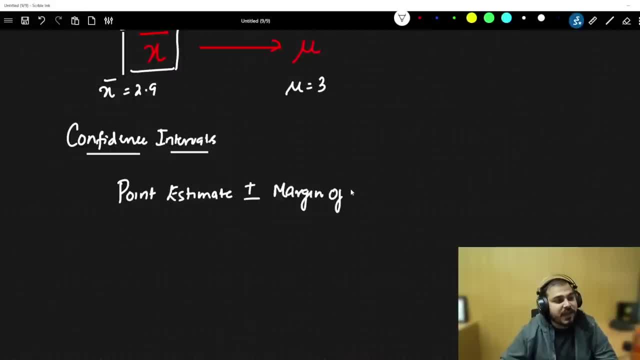 plus or minus margin of error. So there is some margin of error. There is some margin of error because over here you can see 2.9.. This is obviously less. It can also be greater. So I have written plus or minus of margin of error. 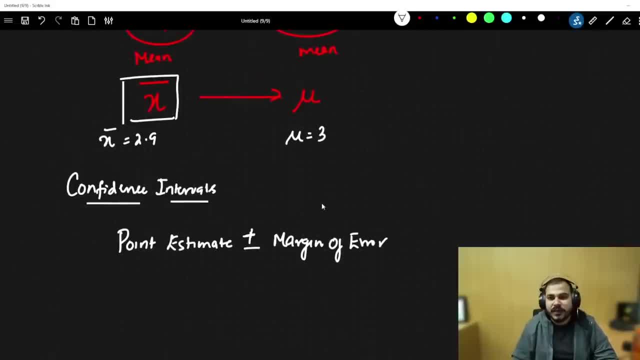 Okay, Because obviously we will not know the exact population mean, right, We don't know. So obviously the point estimate plus margin of error will actually help us to get the same mean, And this is how we determine the confidence interval. Now let's see one problem statement. 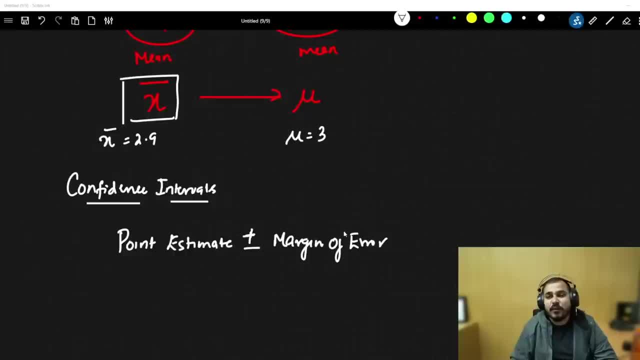 By this you will basically be able to understand what I'm actually saying From this formula. you will be able to understand that how close we are near to the population mean. The second thing is that Suppose if you are given the population standard deviation at that point of time, what formula? 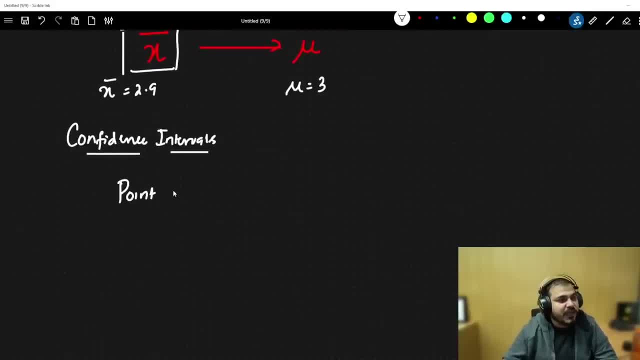 usually given by the formula, which is nothing but point estimate plus or minus margin of error. So there is some margin of error. There is some margin of error Because over here you can see 2.9.. This is obviously less. It can also be greater. So I have written plus or minus of. 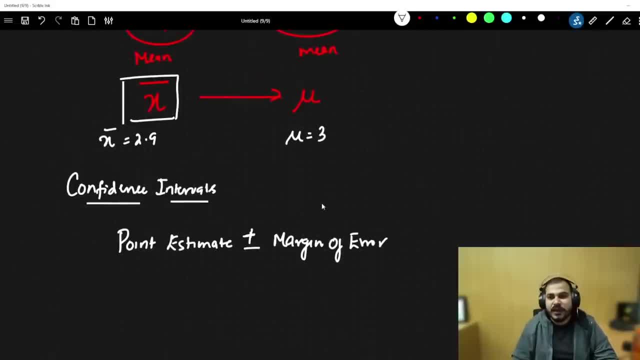 margin of error, Because obviously we will not know the exact population mean, right, We do not know. So obviously the point estimate plus margin of error will actually help us to get the same mean, And this is how we determine the confidence interval. Now let's see one problem statement. 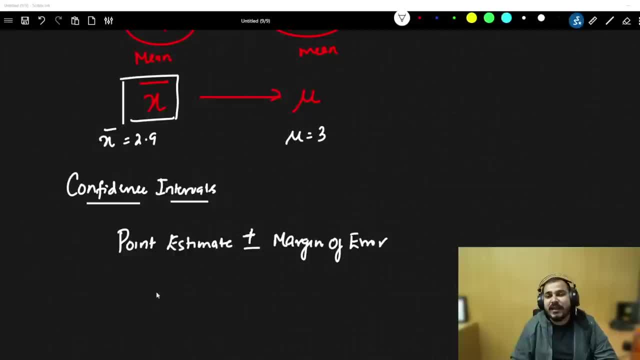 By this you will basically be able to understand what I'm actually saying From this formula. you will be able to understand that how close we are near to the population mean. The second thing is that suppose if you are given the population standard deviation, 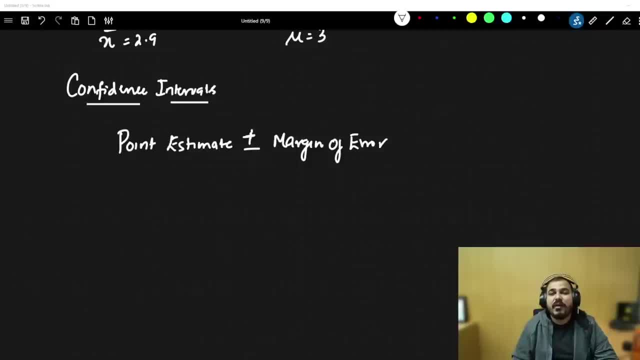 at that point of time what formula you should use to do this and how large your sample size is. So let me just solve one very simple problem and give it to you. So the problem is very, very simple. not that difficult at all. 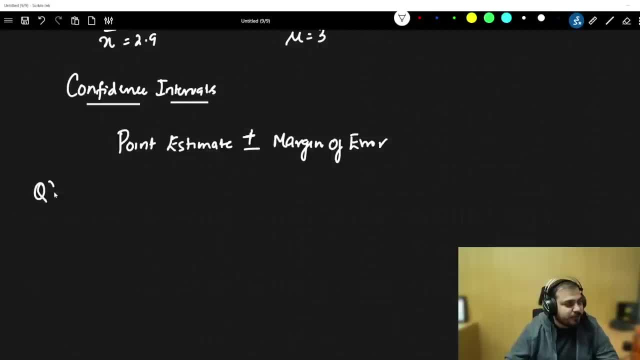 And we'll try to solve that specific problem. So this is my question On the quant test of CAT exam. I hope everybody knows CAT exam. On the quant test of CAT exam, the population standard deviation. the standard deviation is known to be 100.. Now the next thing is that I will take a sample of 25 test-takers. has a mean of 520 score. 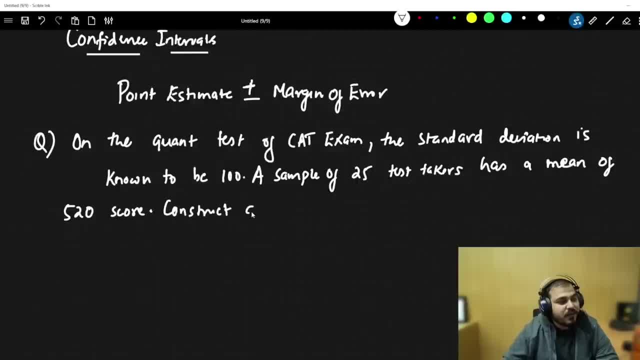 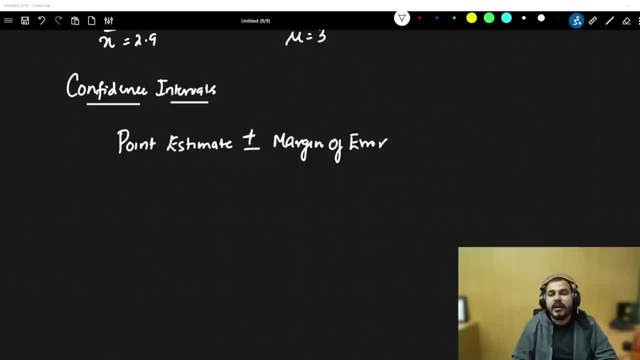 you should use to do this and how large your sample size is. So let me just solve one, one very simple problem and give it to you. So the problem is very, very simple, not that difficult at all, And we'll try to solve that specific problem. 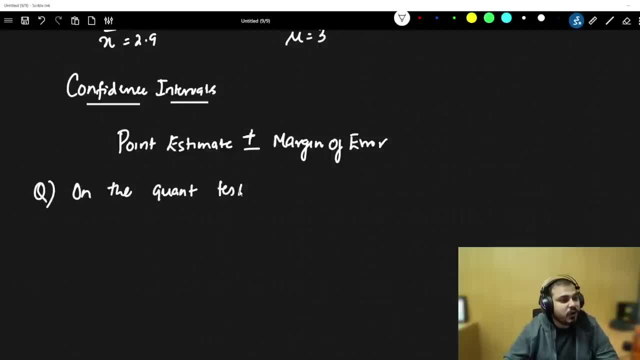 So this is my question on the quant test of CAT exam. I hope everybody knows CAT exam, Okay, So in the quant test of CAT exam, the population standard deviation. the standard deviation is known to be known to be 100.. Now the next thing is that I will take a sample of a sample of 25 test takers. 25 test takers: 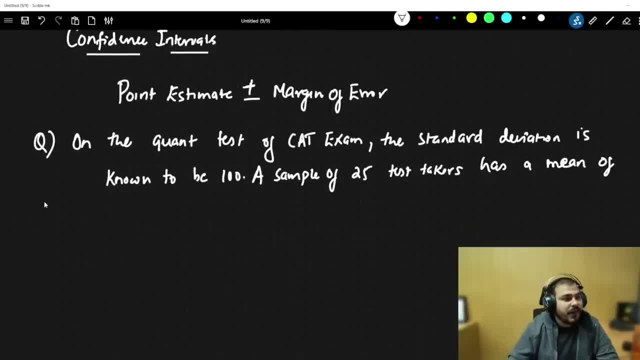 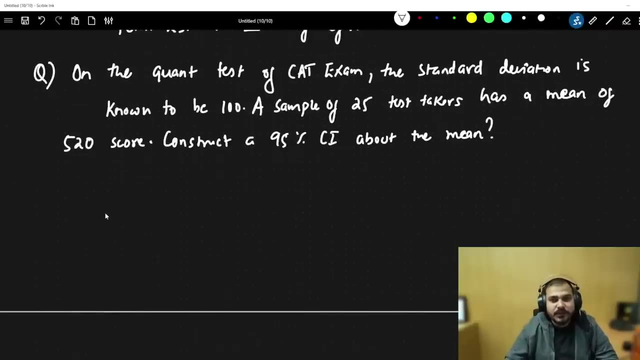 has a mean of, has a mean of 520 score. So here my question is that Construct A 95 percentage confidence interval about the mean? Now let's see what all information is given over here. You know that some information is definitely given. 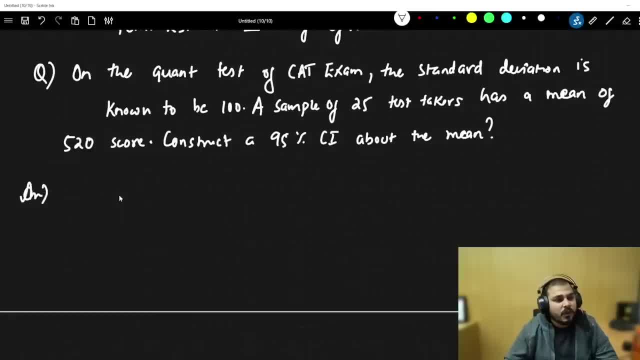 You know that right. So first information: what is given over? here You know, your population standard deviation is given. What is your population standard deviation? here You can see that it is 100,. 100 is the population standard. What is your small n size? 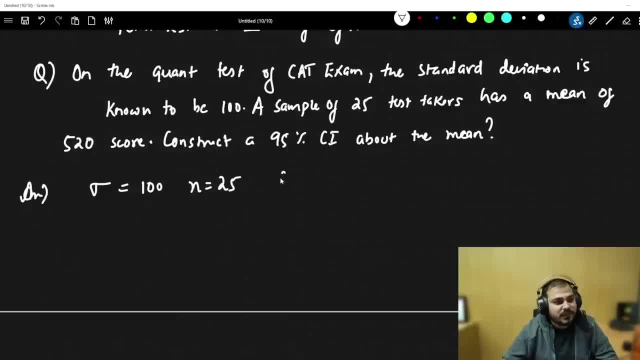 It is nothing but 25.. What is your confidence interval with respect to this alpha? I will get 0.05.. And what is your mean? What is your mean over here? Mean is nothing but X bar, which is nothing but 520.. 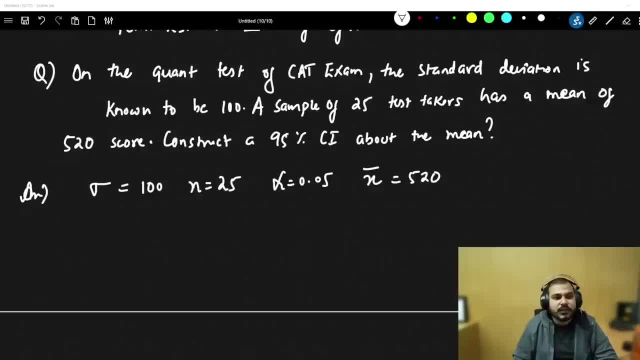 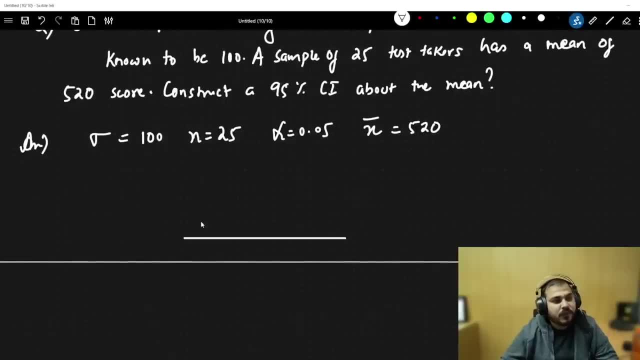 Is this information given in the question? Is this information given in the question? Is this information given in the question? Obviously, it is given. right Now, my graph looks something like this. See this. My graph is looking like this. My mean is basically what is my mean. 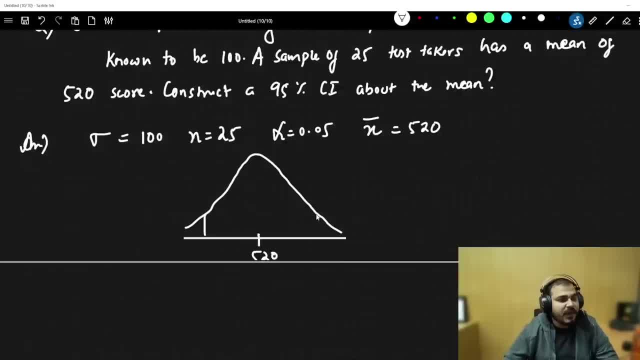 My mean is nothing but 520.. Now my alpha value is 0.05.. So here I have 2.5, here I have 2.5. And this is my 95% confidence interval. Now I need to find out what this value, what this range is basically. 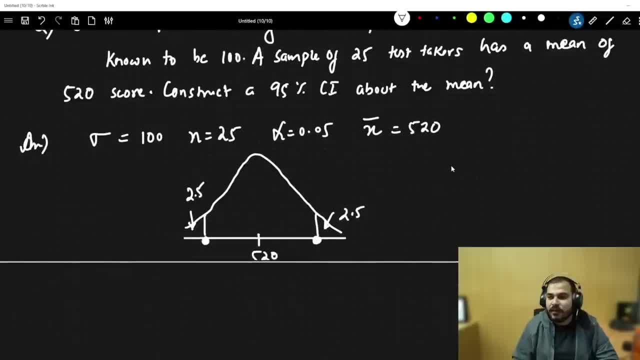 If I say that I want to construct a 95 confidence interval about the mean. what is this value? What value? from here to here it will range. That is what I need to find out. So this is what is my problem statement. 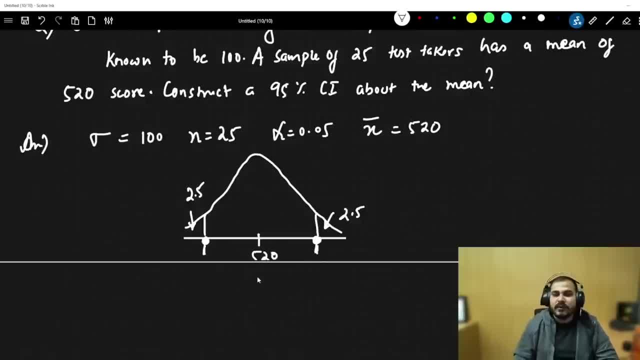 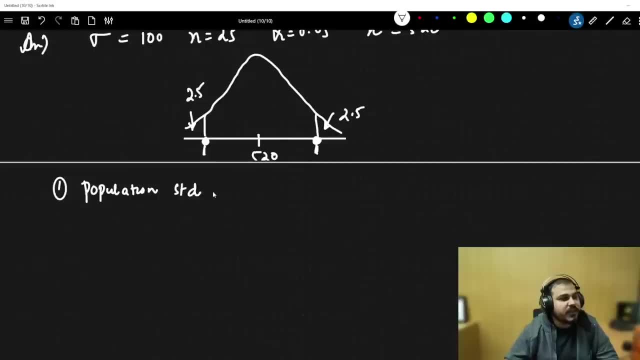 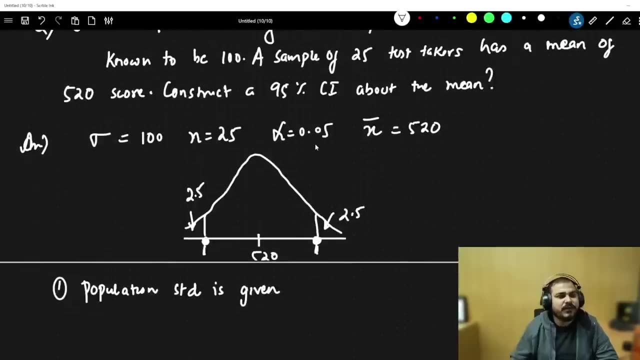 I have also given the standard deviation Now here. whenever population standard, first thing, whenever population standard deviation is given, whenever population standard deviation is given, Guys, why alpha is 0.05?? See, I have given the question as 95% confidence interval, right. 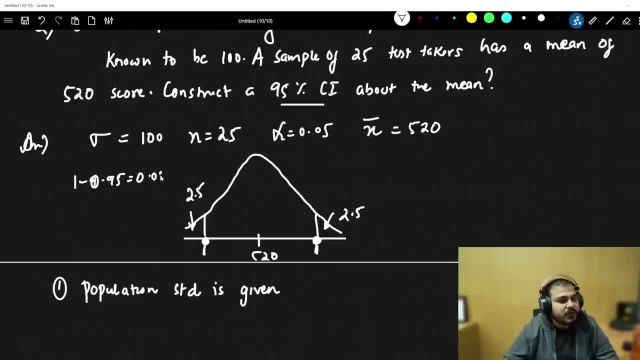 So it is nothing but 1 minus 0.95, which is nothing but 0.05.. So this will be my alpha value. right Alpha and confidence interval are 0.05.. Okay, So this is my alpha interlink, very simple. 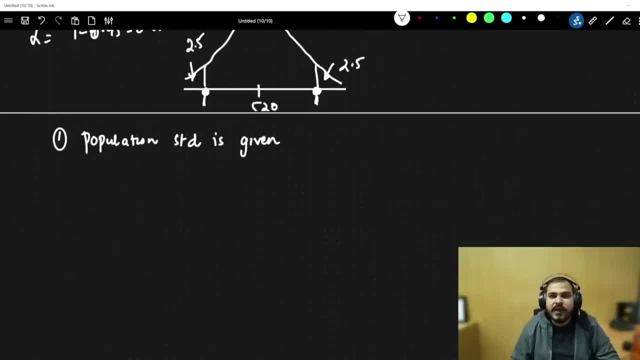 Now, when population standard deviation is basically given, we apply a test. right? What kind of test? Now here I know that this will be my point estimate: plus or minus margin of error. This is for my confidence interval formula. Now, point estimate is obviously your X bar. 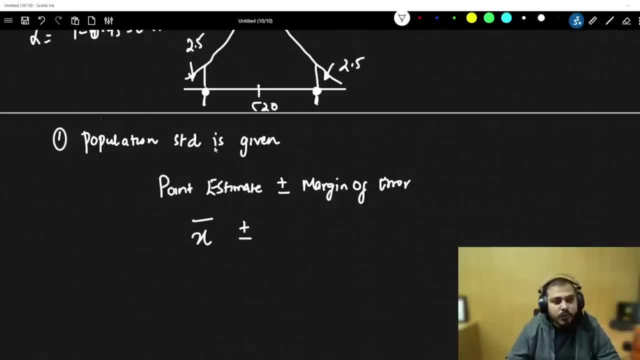 Now, plus or minus, whenever view you have this population, standard deviation, you apply a Z test. So here you will write Z alpha by 2, and the formula will be standard deviation divided by root n. Now this is your formula this term. I will talk about this term. 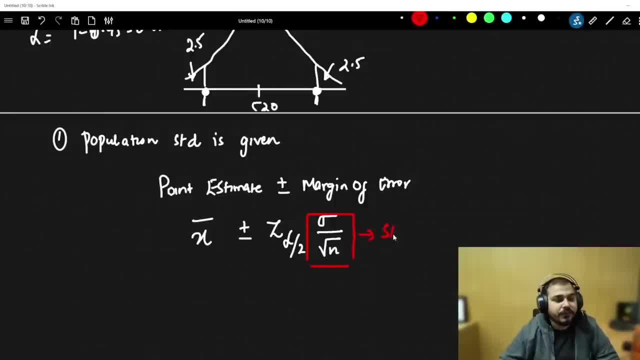 This term that you see, is called as standard error, So in this particular case, one more second point is that when we should use this formula to find out the confidence interval, The next thing is that over here, you will be able to see that I have taken a sample. 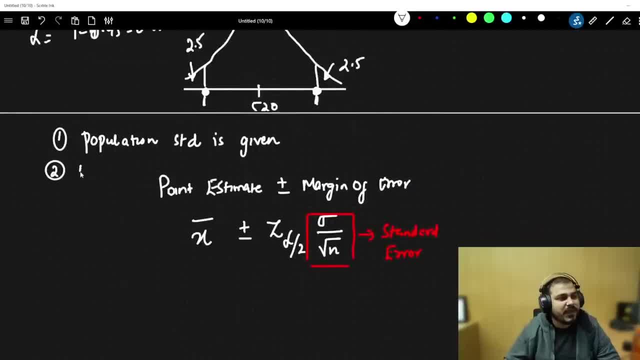 of 25.. But usually the sample size will be greater than or equal to 30.. But just for an example, I have taken as 25, okay, So it's okay. Now don't fight with me, Krish, why I have taken 25.. 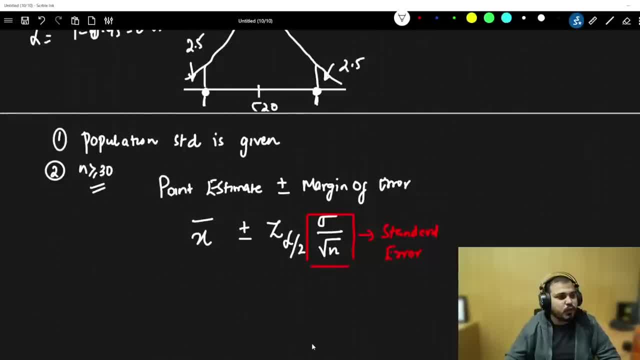 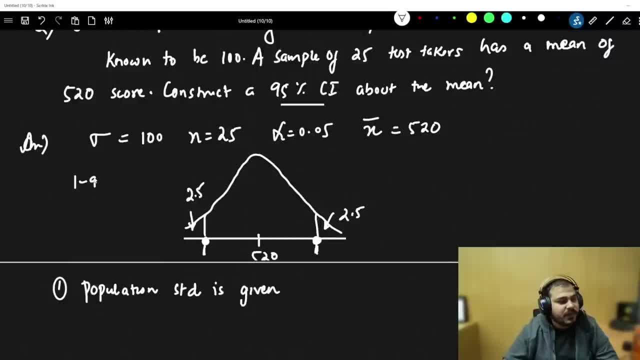 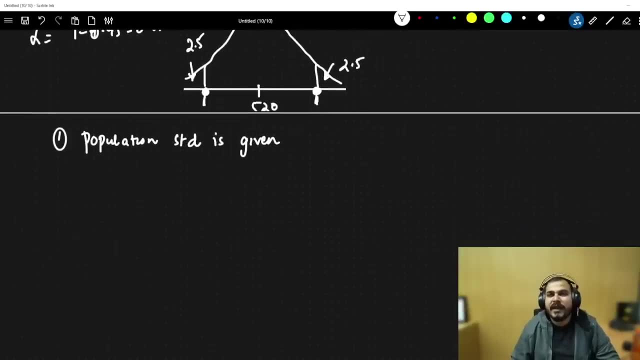 95 percent confidence interval, right? so it is nothing but 1 minus 0.95, which is nothing but 0.05. so this will be my alpha value, right? alpha and confidence interval are interlinked. very simple. now, when population standard deviation is basically given, we apply a test, right? what kind of test? 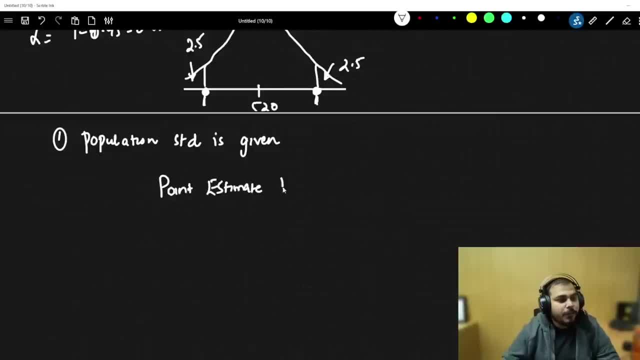 now here i know that this will be my point estimate: plus or minus margin of error. this is my confidence interval formula. now, point estimate is obviously your x bar. now plus or minus. whenever view you have this population standard deviation, you apply a z test. so here you will write z alpha. 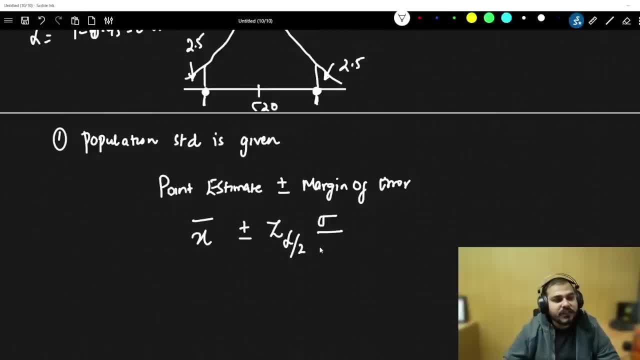 by 2 and the formula will be: standard deviation divided by root n. now this is your formula, this, this term. i'll talk about this term, this term that you see is called as standard error. so you can see that this is the standard error. so if you have this standard error, then you can. 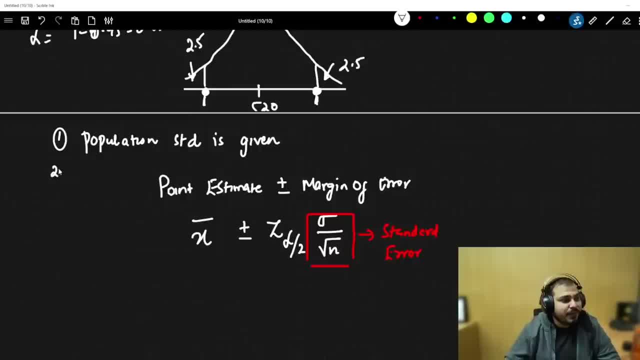 you can see that this is the standard error. so if you have this standard error, then you can, in this particular case, one more, one more. second point is that when we should use this formula to find out the confidence interval, the thing next thing is that over here you will be able to see. 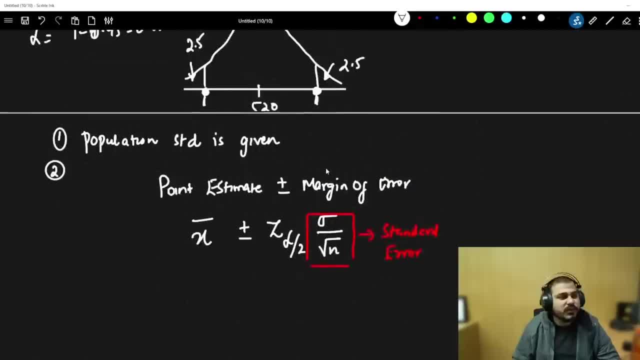 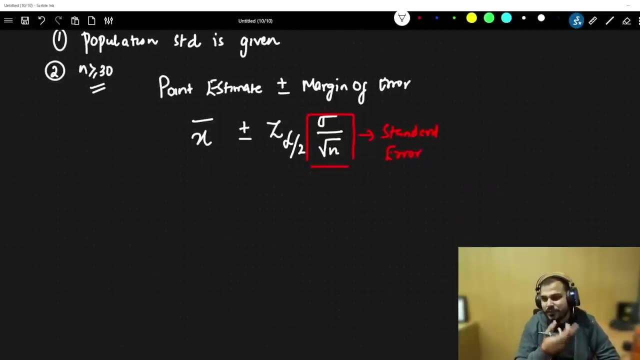 that i have taken a sample of 25, but usually the sample size will be greater than or equal to 30. but just for an example, i have taken uh as 25. okay, so it's okay. now don't fight with me, krish. i have taken 25, take it 30 also. we have to do the calculation, but these two conditions suit. 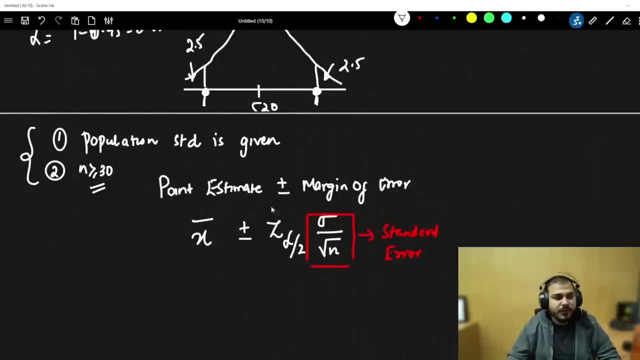 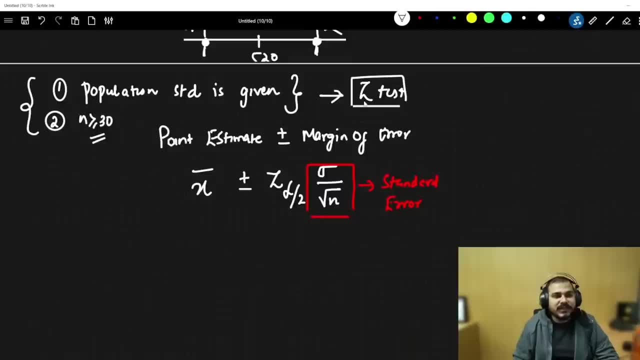 well for this kind of problem statement. okay. so for a z test to happen most of the time, this two condition needs to be approved. now, this z test is nothing but z score. okay, z score to find out the z score. that is what z test is basically used. now understand over here what this alpha is. okay, so 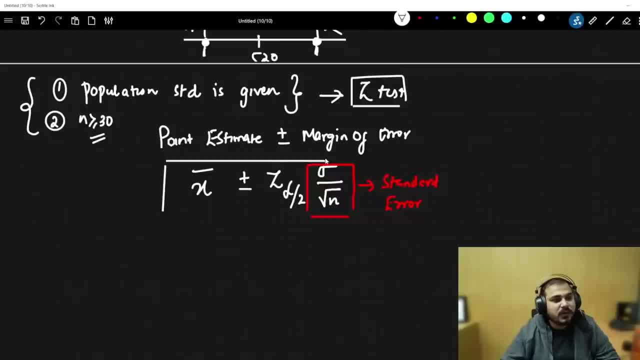 this is the entire formula to find out the confidence interval if your population standard deviation is given. and when you have a z test, you have to find out the confidence interval when your sample size is greater than or equal to 30.. now let's go and solve this particular problem. 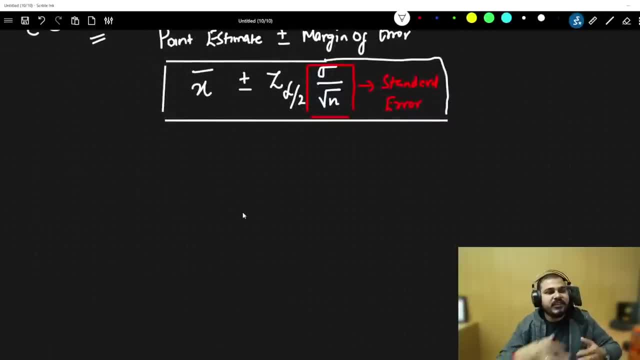 now, when i go and solve this particular problem, the first thing is that i will split this equation into two part. one is: i will get one higher confidence interval. alpha value is 0.05. divide by 2 standard deviation is what is standard deviation over here it is nothing but 100. 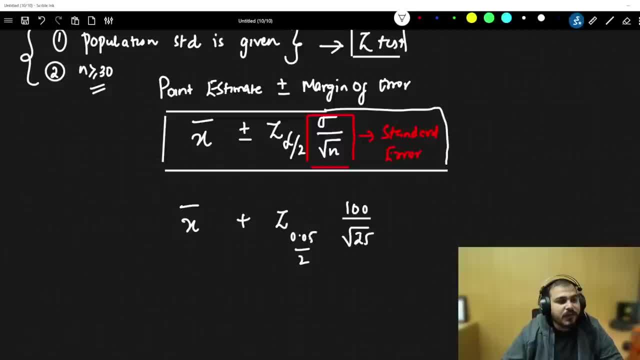 divided by root, 25. now you understood why i have taken 25, because my calculation will be different. the first thing you will find is that over here, you will get the confidence interval, which is the confidence interval plus 0.05. divided by 2, you will get this confidence interval, which is: 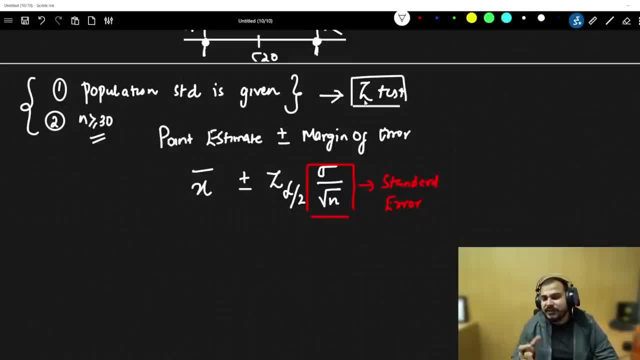 Okay, Z score: to find out the Z score. That is what Z test is basically used. Now understand over here what this alpha is. okay, So this is the entire formula to find out the confidence interval if your population standard deviation is given and when your sample size is greater than or equal to 30.. 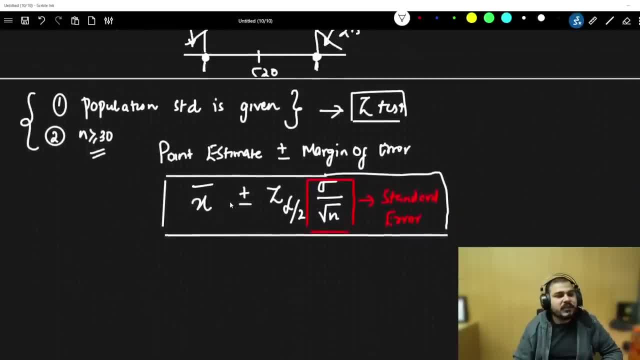 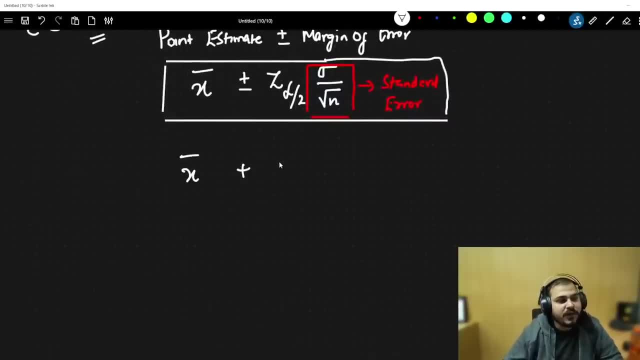 Now, let's go and solve this particular problem. Now, when I go and solve this particular problem, the first thing is that I will split this equation into two part. One is: I will get one higher confidence. Higher confidence interval. alpha value is 0.05 divided by 2.. 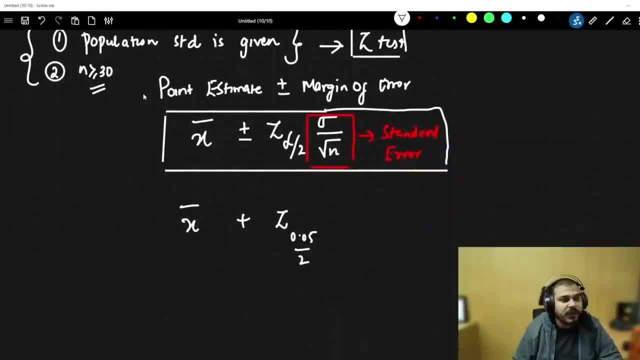 Standard deviation is what is standard deviation over here? It is nothing but 100 divided by root 25.. Now you understood why I have taken 25, because my calculation will become easier. Don't fight with me, guys, I don't have energy to fight. 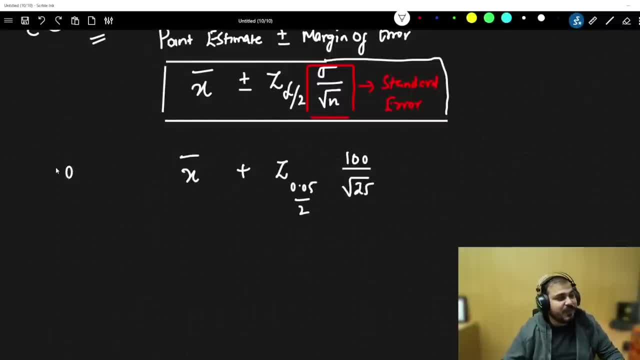 Nowadays I fight with lot of people, So this will basically be my upper bound, upper bound of confidence interval. Similarly, lower confidence interval, Lower confidence interval, Lower bound of confidence interval. I will try to find out. That is x bar minus z, 0.05 divided by 2, 100 divided by root 25.. 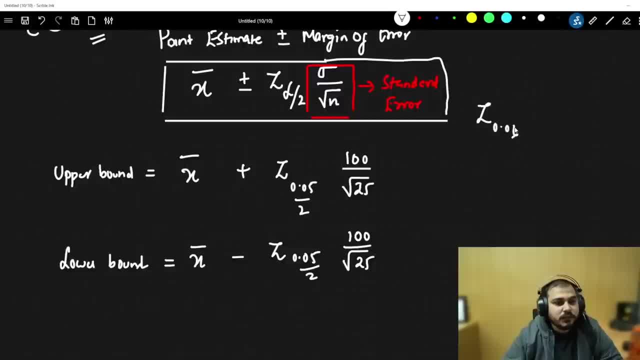 Now here I will write 0.00, sorry. 0.05 by 2 is nothing, but z is nothing but 0.025.. I hope everybody is getting this. Now, how do I find out this particular value for this? Go and open your browser. 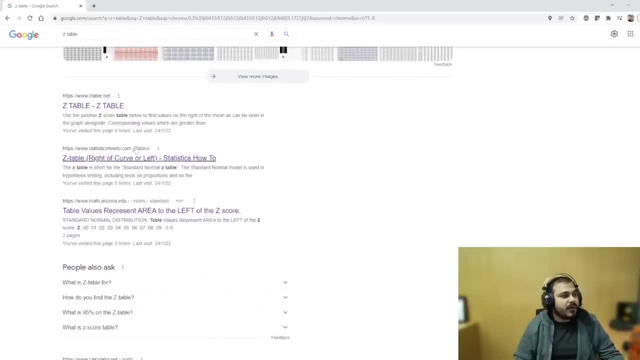 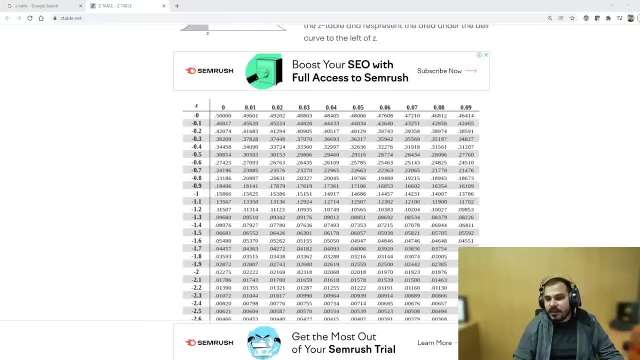 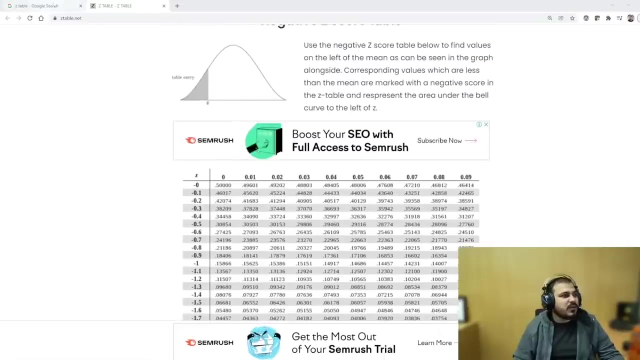 And open z table. So if I go and open z table, if I open z table, let me just open a z table, another z table I will try to open Just a second Point. here all minus are basically shown, So I will not use this z table. I will use the other one because there are only negative. 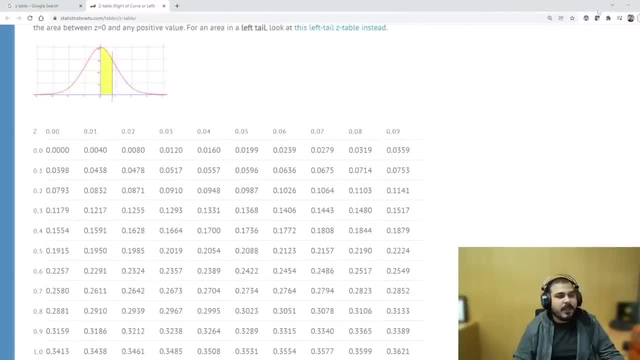 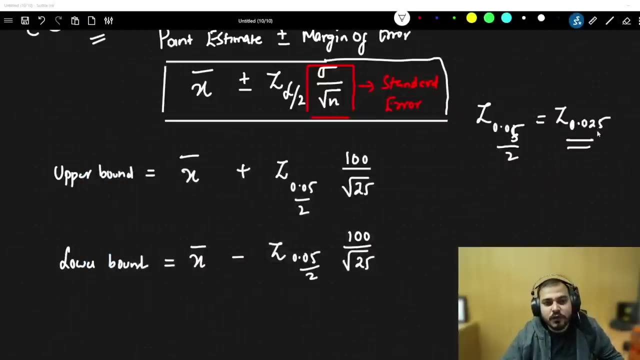 values given Here. probably I will be able to find out. Okay, Now in z table. always understand, Always understand Over here when I say 0.025,. okay, my entire area is how much? So my entire area is 1.. 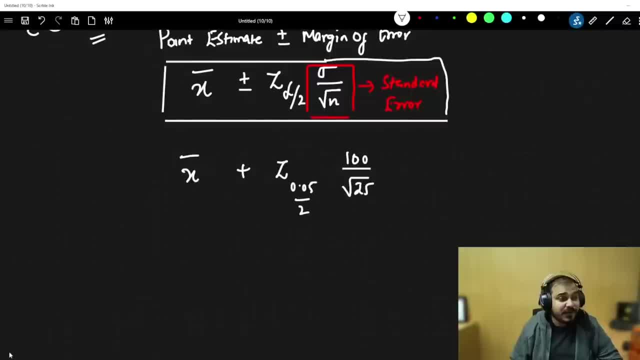 will become easier. Don't fight with me, guys. I don't have energy to fight Nowadays. I fight with lot of people. So this will basically be my upper bound. Upper bound of confidence interval. Similarly, lower bound of confidence interval, I will try to find out. That is x bar minus z. 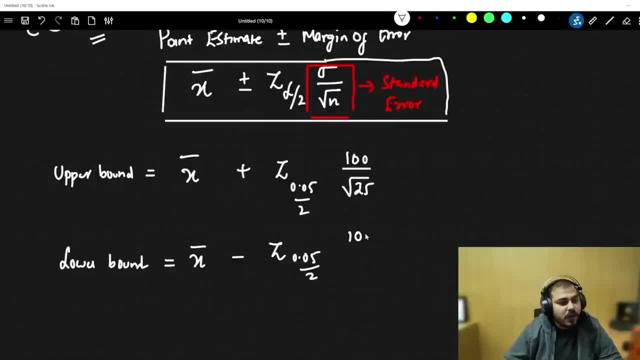 0.05 divided by 2, 100 divided by root: 25.. Now here I will write: 0.05 by 2 is nothing but z is nothing but 0.025.. I hope everybody is getting this. Now, how do I find out this particular value? 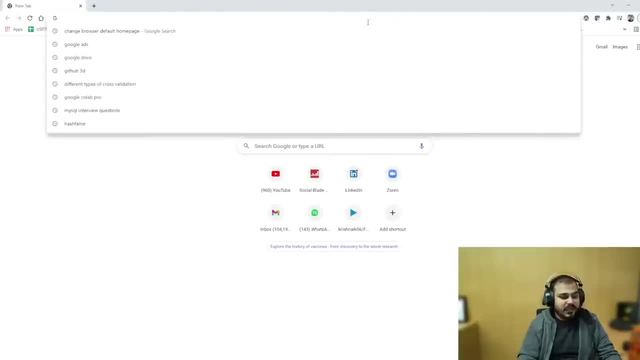 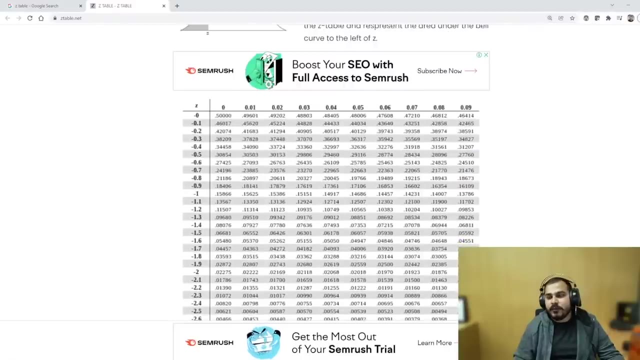 for this. Go and open your browser and open z table. So if I go and open z table, if I open z table, let me Just open a z table, Another z table. I will try to open Just a second Here. all minus are: 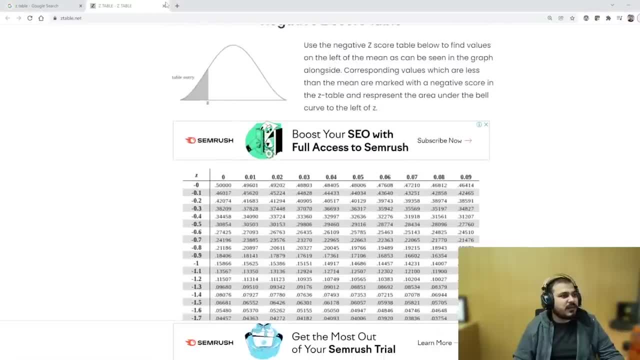 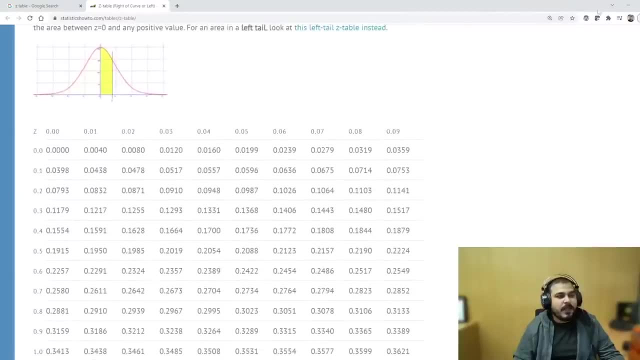 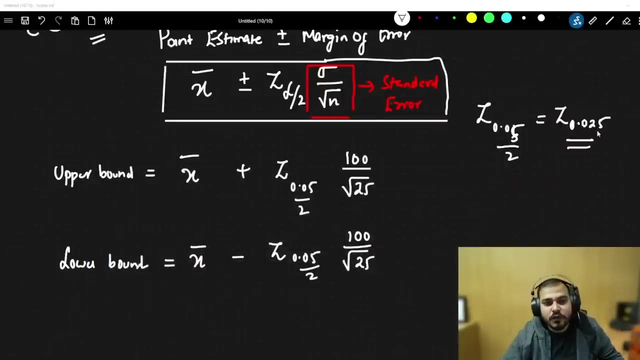 basically shown. So I will not use this z table. I will use the other one because there are only negative values given Here. probably I will be able to find out. Okay Now in z table, always understand, always understand Over here, when I say 0.025, okay, my entire area is how much? 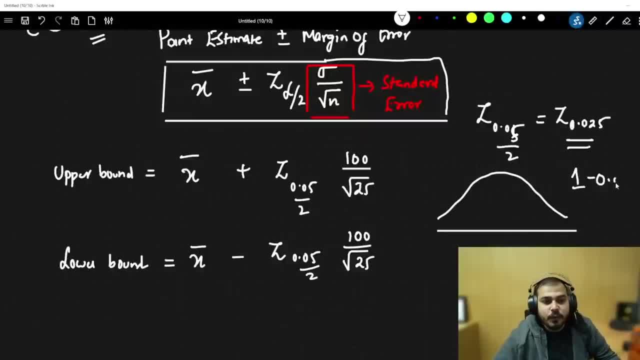 So my entire area is 0.025.. So my entire area is 0.025.. So my entire area is 0.025.. So my entire area is 1.. If I subtract 1 with 0.025, that basically means this part, the entire area, will. 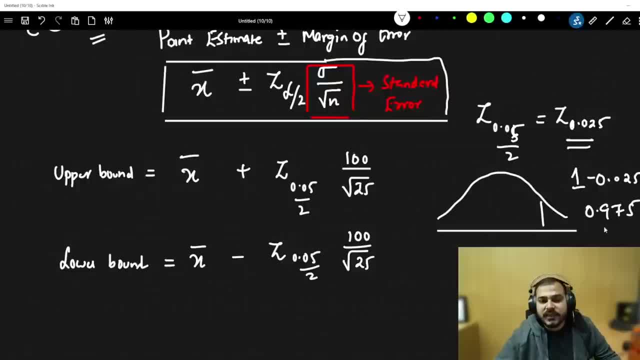 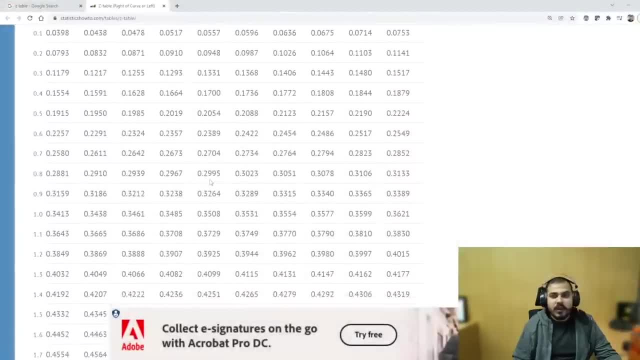 become 0.975.. So 0.975, I have to check in the z table. So for this, what I will do is that I will go to my browser and go and check it. Where is 0.975?? 0.975 is nothing but this specific area. 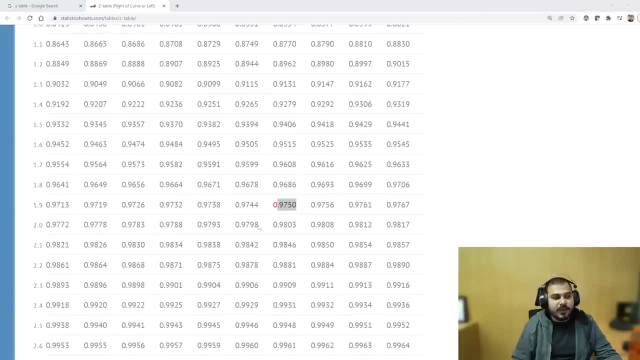 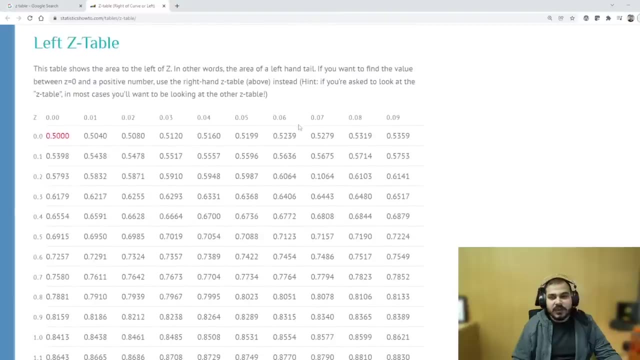 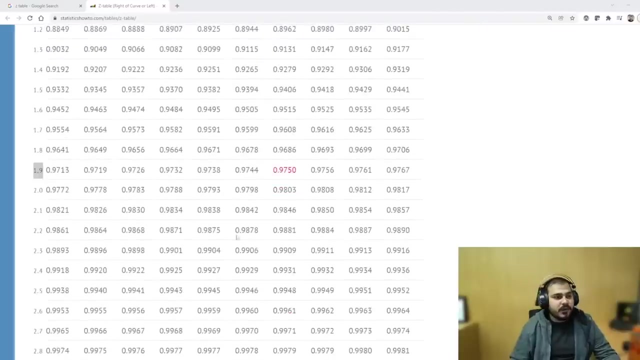 Go and check this: 0.975.. I hope you are able to see this. What is this value? 1.9.. And if I go on top, it is 0.06.. That basically means the z value is 1.96.. So go down over here. you will be able to see 0.9750.. It is nothing but 1.9 and this is. 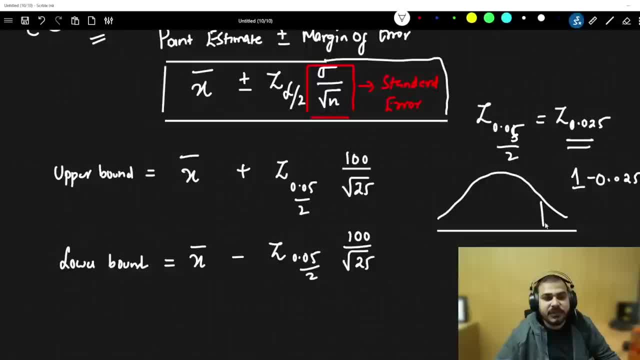 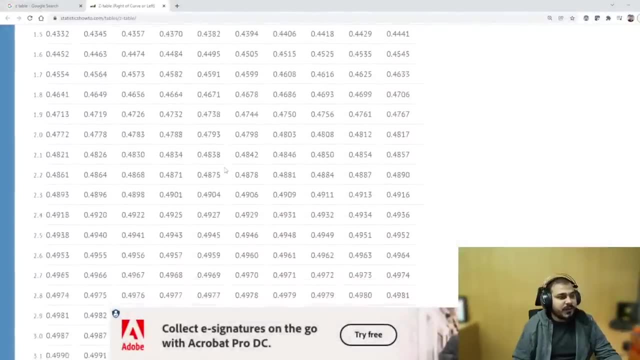 If I subtract 1 with 0.025, that basically means this part, the entire area will become 0.975.. So 0.975, I have to check in the z table. So for this, what I will do is that I will go to my browser and go and check it. 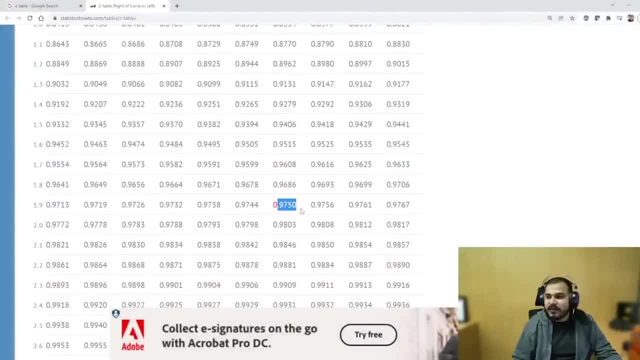 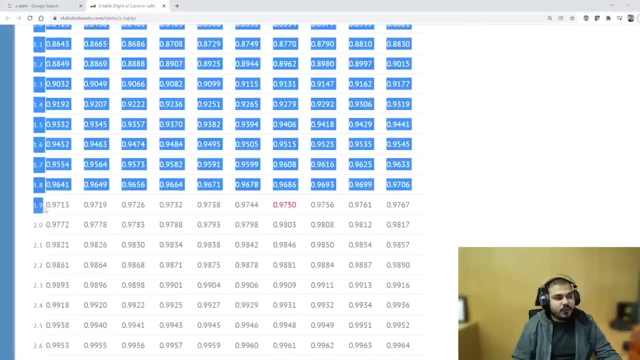 Where is 0.975?? 0.975.. 0.975 is nothing but this specific area. Go and check this: 0.975.. I hope you are able to see this. So what is this value? 1.9, and if I go on top, it is 0.06.. 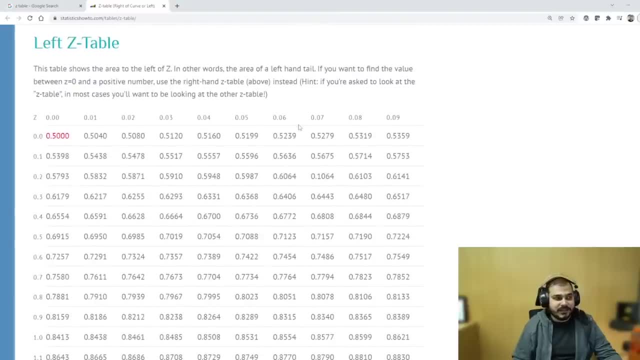 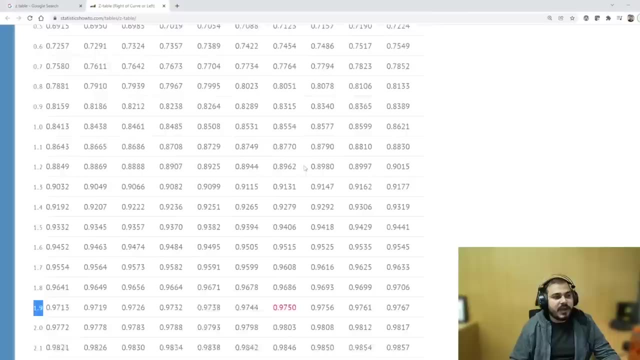 That basically means the z value is 1.96.. So go down over here. you will be able to see 0.9750, it is nothing but 1.9 and this is 0.06.. So this becomes my z score. 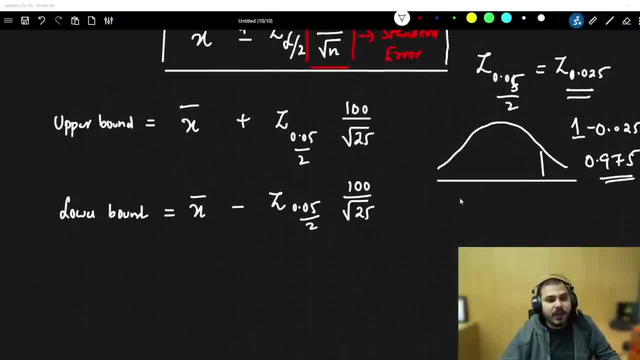 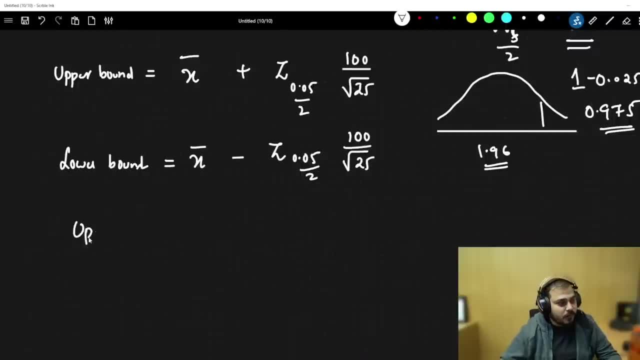 So finally, I will go to my browser. Okay. So finally I get my value as 1.96.. Now go and calculate it. So what is my x bar? For the upper bound? I will say my x bar is nothing. but what is the mean of the sample? 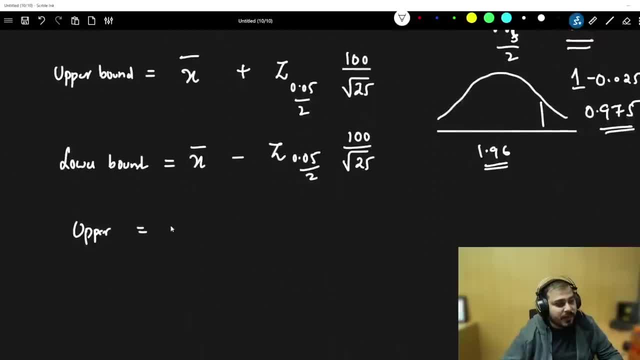 It is nothing but 520.. Okay, So it is 520 plus 1.96 multiplied by 20.. Similarly, the lower bound: it is nothing but 520 minus 1.96.. Okay, So that is the upper bound. 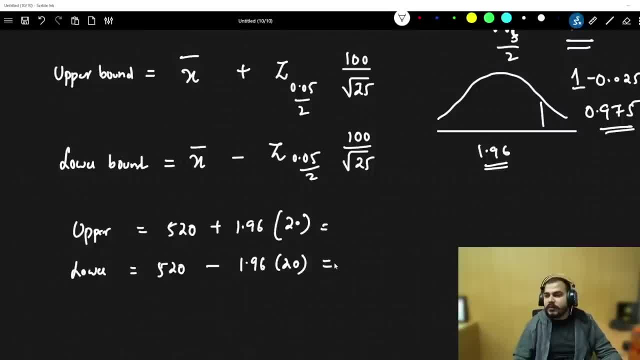 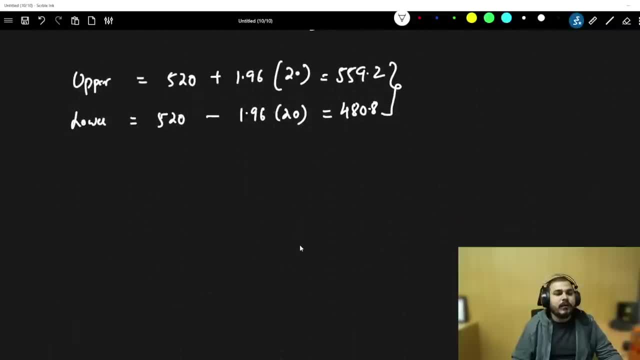 So this is my lower bound and upper bound. that basically means whenever I am defining my confidence interval for this distribution, with alpha is 0.05 and this, this value will be 559.2 and this value will be 480.8 and my mean will basically be 520, right. 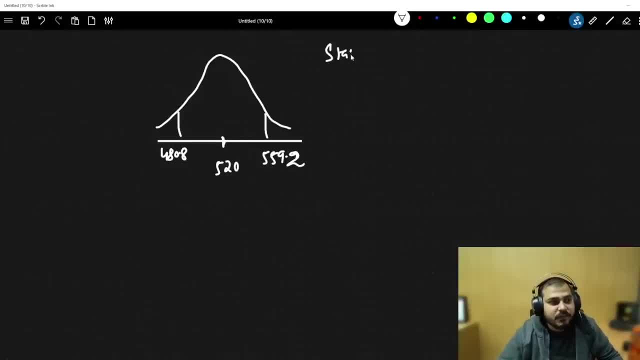 So one stats interview question that I told right: find the average size of the sharks, sharks throughout the world. Can you solve this by taking your own example, Because one of my student solved this particular problem and he gave some confidence interval. He said that let us assume this, this, this, this, this and try to solve in this particular. 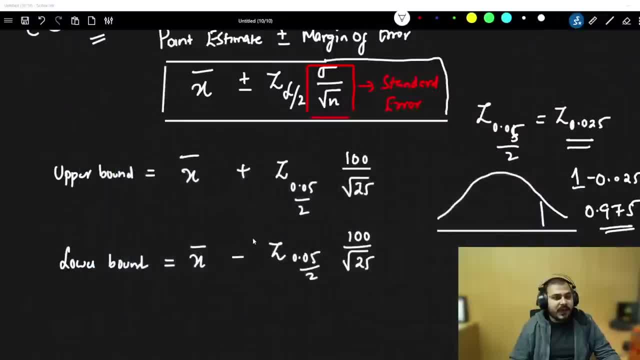 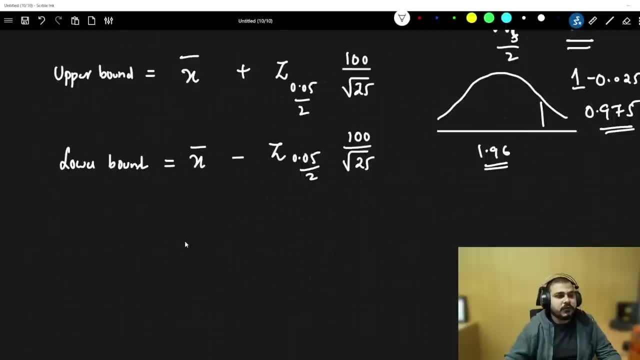 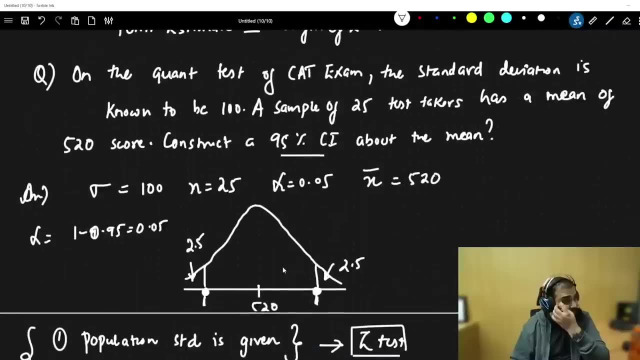 0.06.. So this becomes my z score. So finally I get my value as 1.96.. Now go and calculate it. So what is my x bar? For the upper bound I will say my x bar is nothing. but what is the mean of the sample? 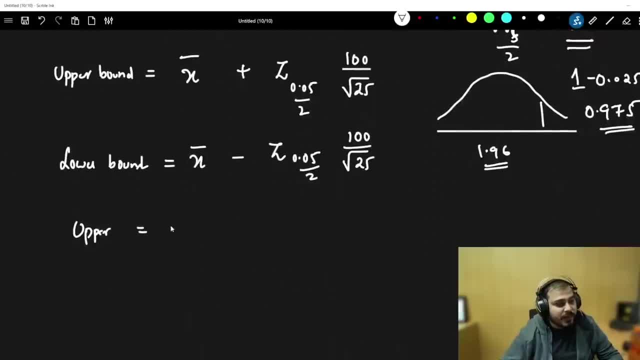 It is nothing but 520.. So it is 520 plus 1.96 multiplied by 20.. Similarly, the lower bound, it is nothing but 520 minus 1.96 multiplied by 20.. Now go ahead and compute this. 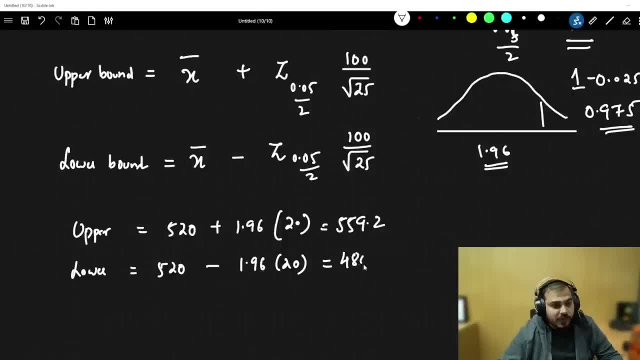 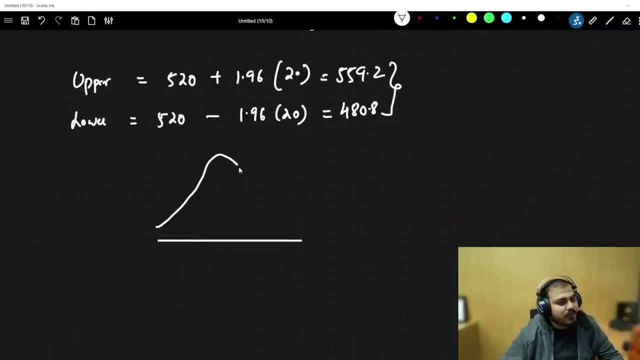 5.59.2480.. So this is my lower bound and upper bound. That basically means, whenever I am defining my confidence interval for this distribution with alpha is 0.05 and this, this value will be 5.59.2 and this value will be 480.8.. And my mean will basically be 520, right? 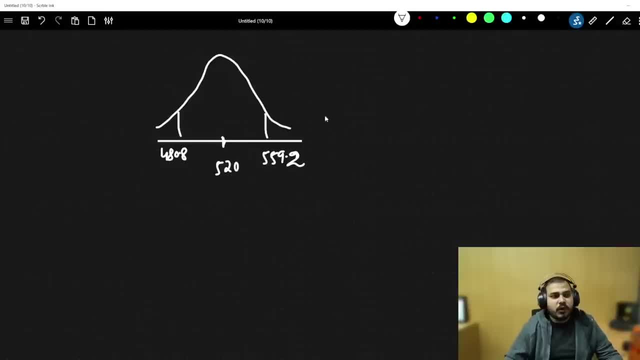 Right. So one stats interview question that I told right: Find the 0.96. Average size of the sharks sharks throughout the world. Can you solve this by taking your own example, Because one of my student solved this particular problem and he gave some confidence. 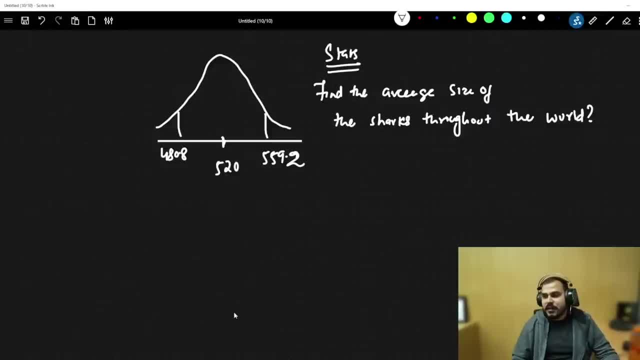 interval. He said that let's assume this, this, this, this this and try to solve in this particular way. He said that, okay, let's consider. oh there, the interviewer said: you know the population standard deviation, you know the x. 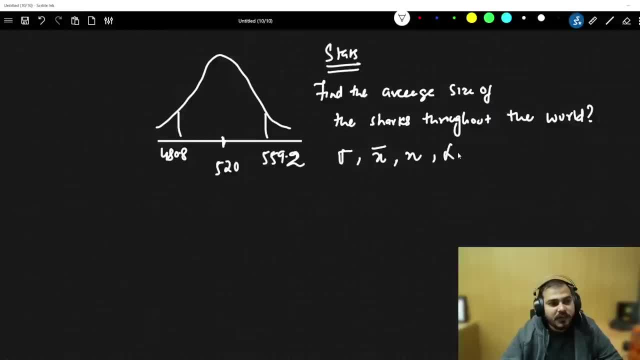 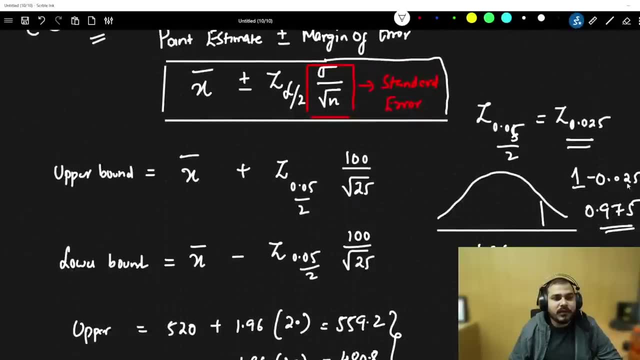 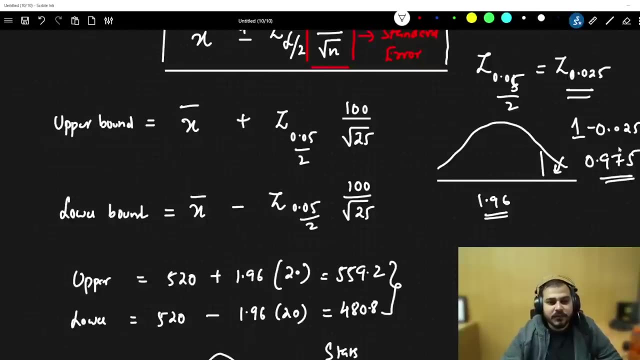 and the z value. you know the n value. try to solve it with alpha as 0.05.. I use naughty- I'll understand that over here- when my alpha value is 0.025.. I am just worried about one tail right this side. this entire area is one. so one minus 0.025 is 0.975.. 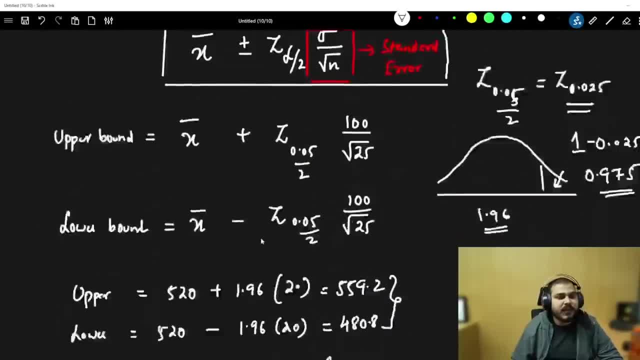 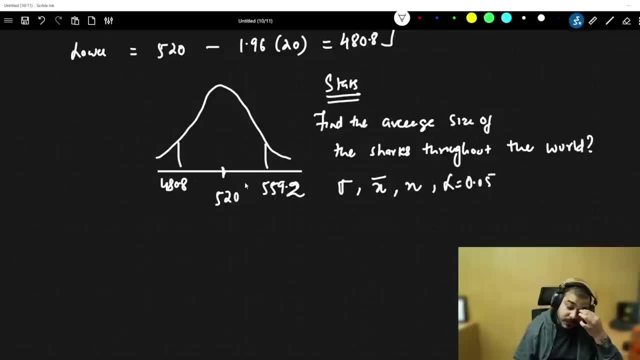 Now, after performing any experiment, if my value falls between this two, at that point of time, I will assume that it is 0.975.. All right, Thank you, It is. we need to accept the null hypothesis and we can go ahead with it. 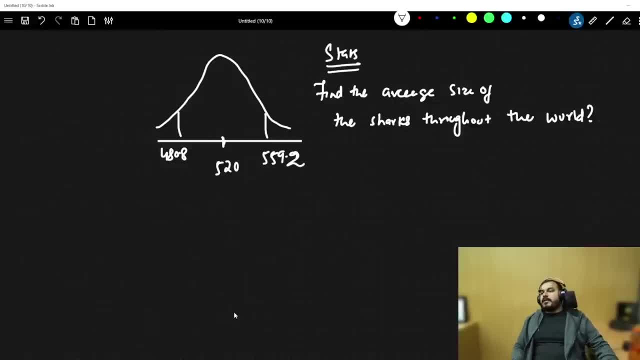 way. He said that. okay, let us consider. oh there, the interviewer said: you know the population standard deviation, you know the X bar value, you know the N value. try to solve it with alpha as 0.05.. 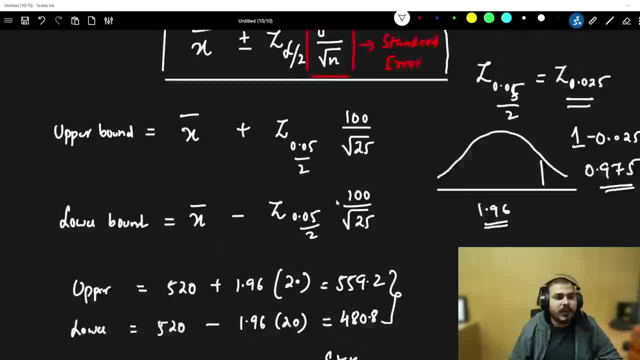 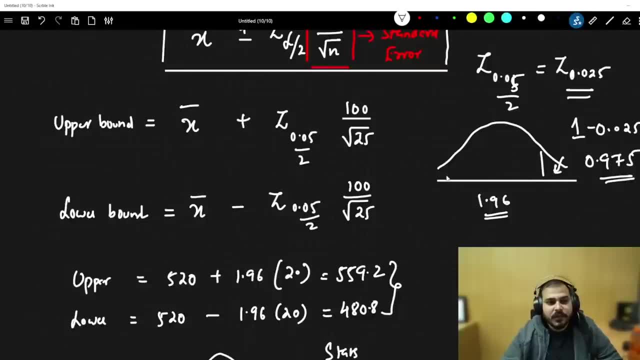 Ayush Nautiyal, understand that over here, when my alpha value is 0.025, I am just worried about one tail right This side. this entire area is one, So one minus 0.025 is 0.975.. 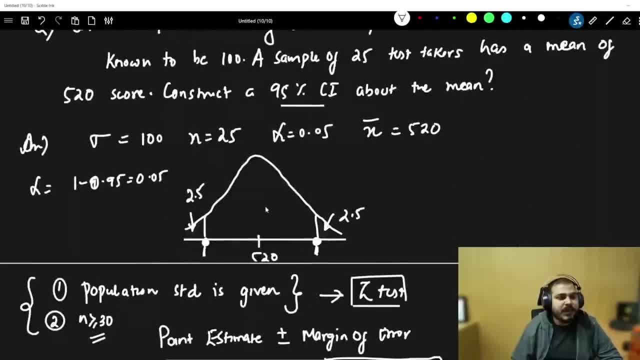 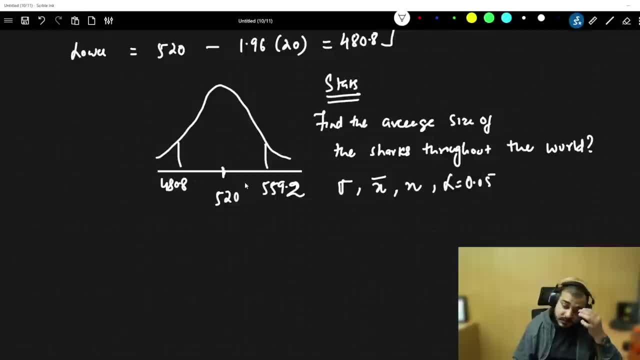 Now, after performing any analysis, I am just worried about one tail right. This entire area is one, So one minus 0.025 is 0.975.. So let me experiment. If my value falls between these two, at that point of time I will assume that it is it. 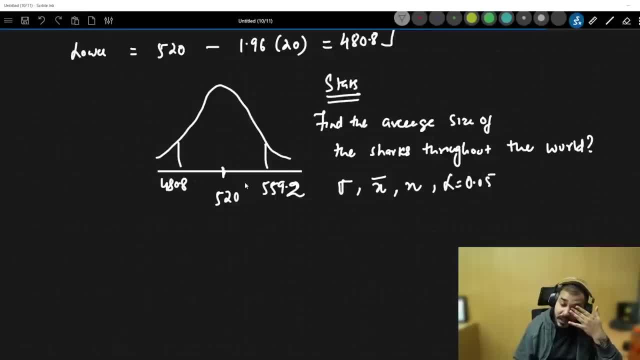 is: we need to accept the null hypothesis and we can go ahead with it. If it does not fall within this range, then it is going to fall away from the well. basically, we need to reject the null hypothesis. Now the next question that we are probably going to see is that what if the population 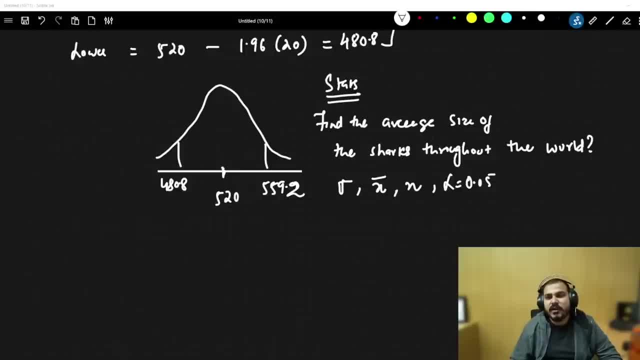 standard deviation is not given. Now, in that particular scenario, what will you do? For that particular case, you really need to use something called as t-test. So let me just show you one very good example and that also we will try to solve. 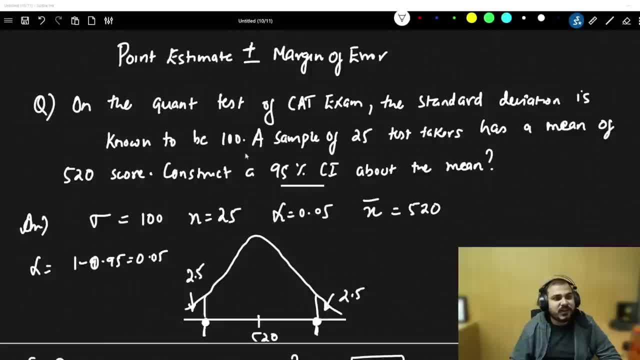 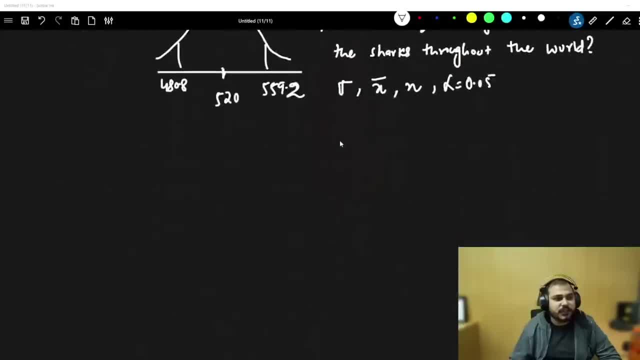 Let us say that the same question: this standard deviation is not given, Standard deviation is not given, Population standard deviation is not given, but sample standard deviation is given. So I will write down the question over here for you, but I hope you are able to understand. 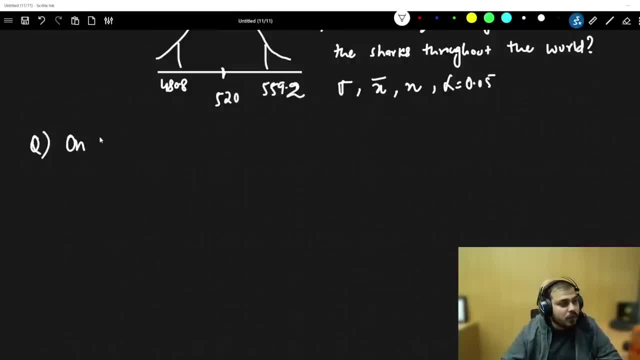 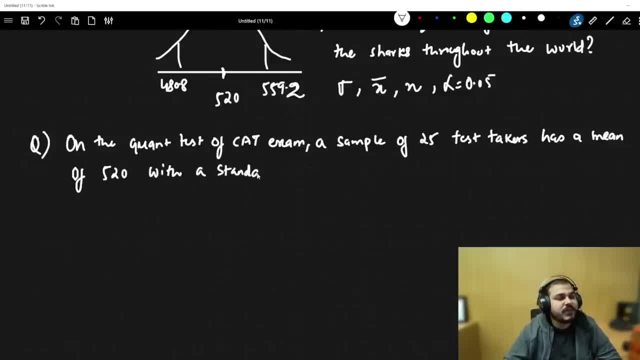 with a standard deviation. Now this standard deviation that is given is basically your sample standard deviation. Has a standard deviation of 80.. Construct 95%, Construct 95%, Construct 95%: Confidence interval about the mean. So this is basically my question. 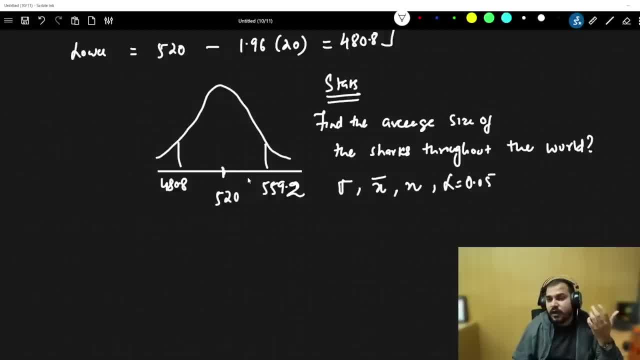 If it does not fall within this range, then it is going to fall away from the hypothesis. Well, basically, we need to reject the null hypothesis. Now, the next question that we are probably going to see is that: what if the population standard deviation is not given? 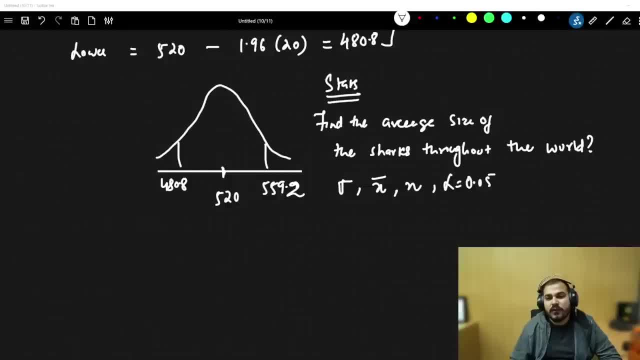 Now, in that particular scenario, what will you do? For that particular case, you really need to use something called as t-test. So let me just show you one very good example and that also we will try to solve. Let us say that the same question, this standard deviation, is not given. 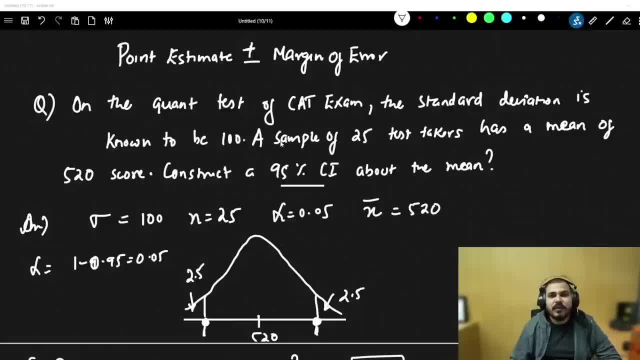 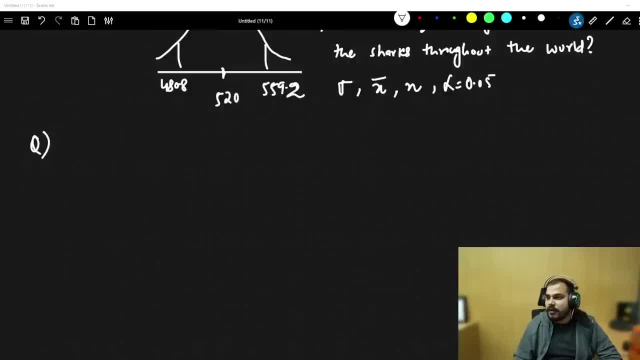 Standard deviation is not given. Population standard deviation is not given, but sample standard deviation is given. So I will write down the question over here for you, but I hope you are able to understand it. So the question is that on the quant test of CAT exam, 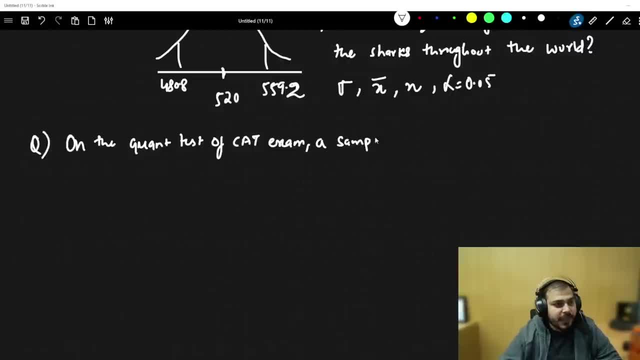 on the quant test. So, on the quant test of a CAT exam, a sample of 25 test takers has a mean of 520, score with a standard deviation. Now this standard deviation that is given is basically your sample standard deviation. 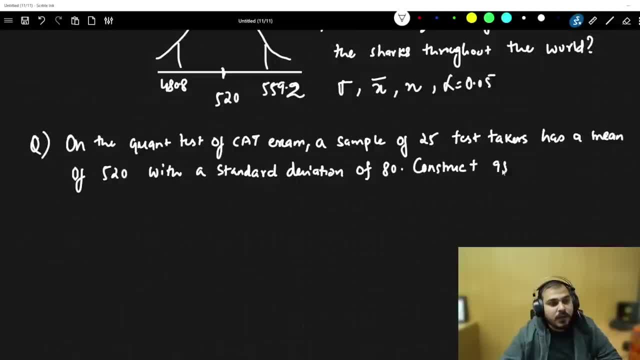 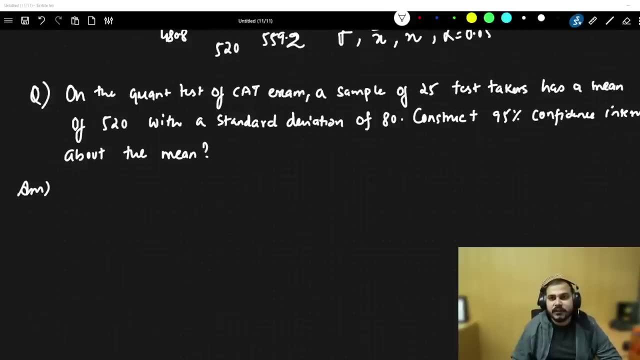 Has a standard deviation of 80.. Construct 95% confidence interval about the mean. So this is basically my question. So over here you can see that population standard deviation is not given. So in this particular case I definitely have to use z-test. 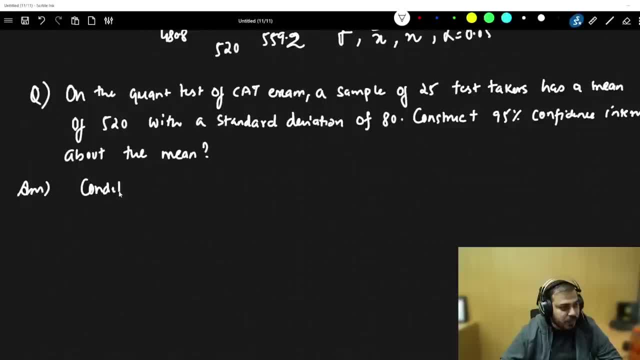 So over here, sorry, t-test condition, I will write, okay. First of all, we will try to see what all things are given. Your n value is given, which is 25.. Your x bar is given, which is nothing but 520.. 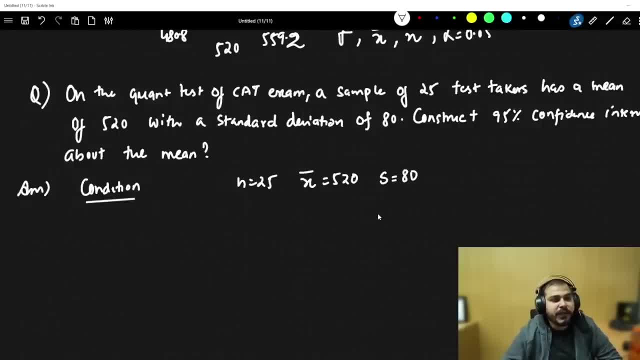 Right. Your sample standard deviation is given. that is 80.. And your alpha is 0.5.. So this is my question. So over here you can see that population standard deviation is not given. So when you see over here, your values have not been given over here. 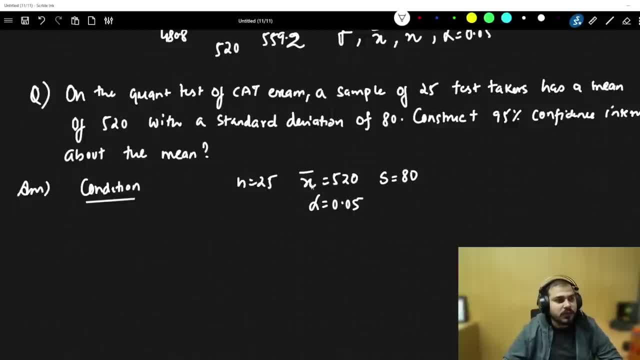 That basically means your you know the conditions. I will not say conditions. But here your population standard deviation is not given. So I can write a condition saying that here population standard deviation is not given. So in this particular case we use something called as t-test. 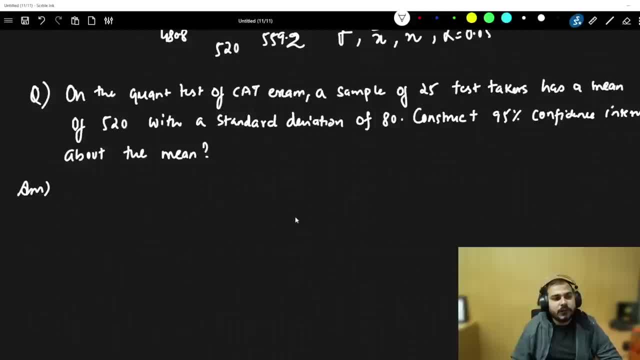 Right. So this is my question. So over here you can see that population standard deviation is not given. So in this particular case I definitely have to use z test. So over here, sorry, t-test Condition- I will write. 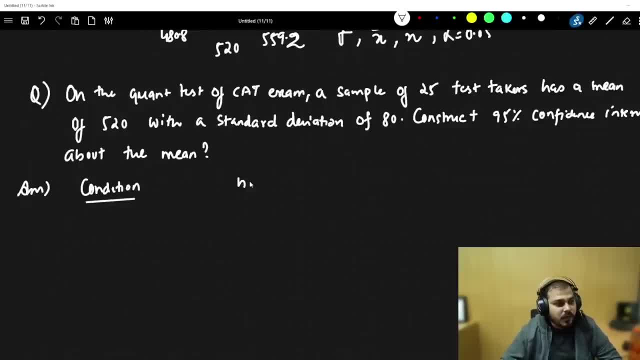 Okay, First of all, we will try to see what all things are given. Your n value is given, which is 25.. Your x bar is given, which is nothing but 520.. Right, your sample standard deviation is given, that is 80, and your alpha is 0.05.. So when you see over here, 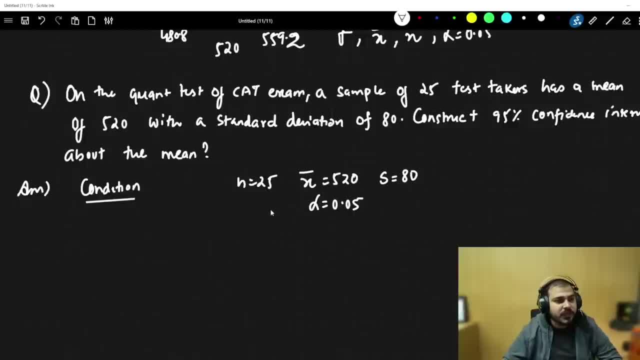 your Values have not been given over here. That basically means you are, You know the the conditions and not the conditions. but here your population standard deviation is not given. So I can write a condition saying that here population standard deviation is not given and In this particular case we use something called as t-test, a population standard deviation given at that point of time. 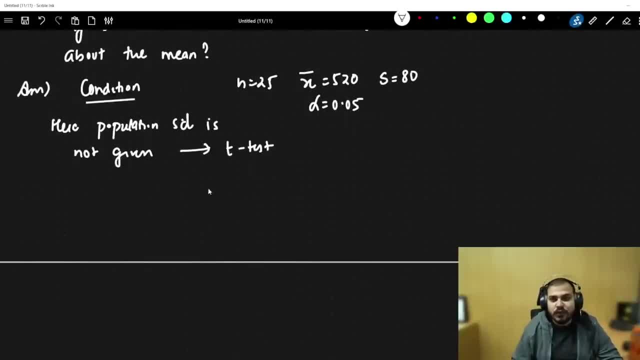 You use t-test, Let's go and try to compute it here. Also, the same formula will be used: point estimate, plus or minus Margin of error. here your margin of error formula will change. Okay, Now what kind of formula it will have? that you need to understand. the formula will be something like X bar. 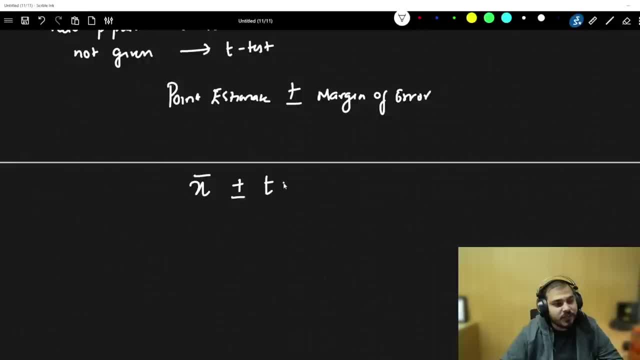 Plus or minus. instead of writing Z alpha by 2 here, You will be writing T alpha by 2, and then you will be using s by root n. This is your standard error. now go and substitute it. So two things you will be basically having. one is upper bound. 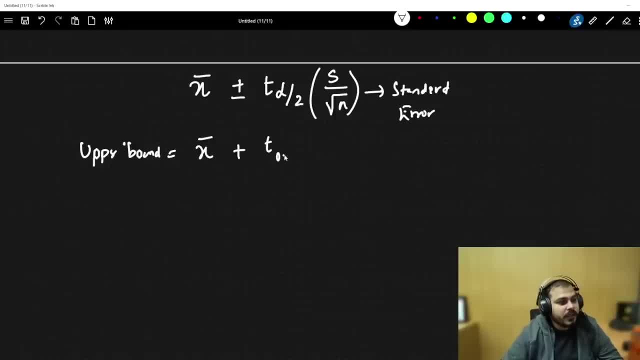 It will be X bar plus T, point 0, 5 by 2 s by root n. right now, first thing, first, Always understand. to calculate the T, Okay, to calculate the T value, you need to find out something called a degree of freedom, because in the T table you will, you will be asked this, and: 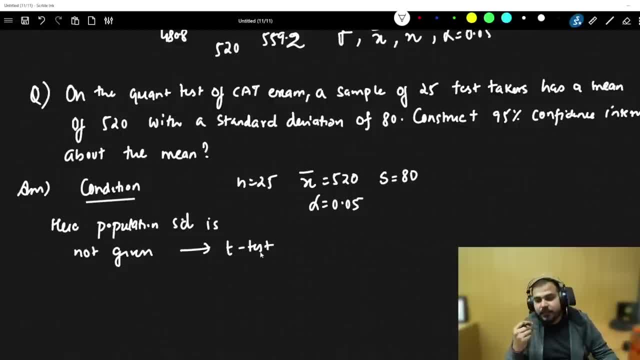 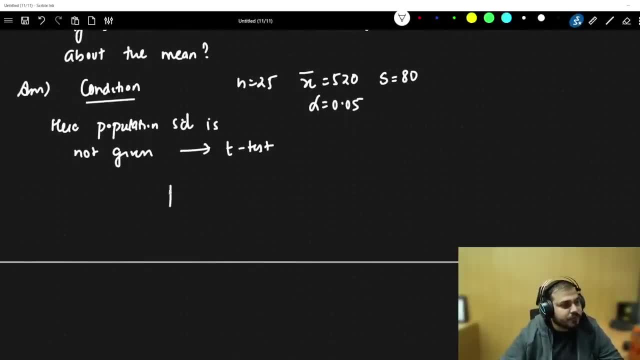 A population standard deviation is given. At that point of time you use t-test. Let's go and try to compute it. Here also the same formula will be used: Point estimate- plus or minus margin of error. Here your margin of error formula will change. okay. 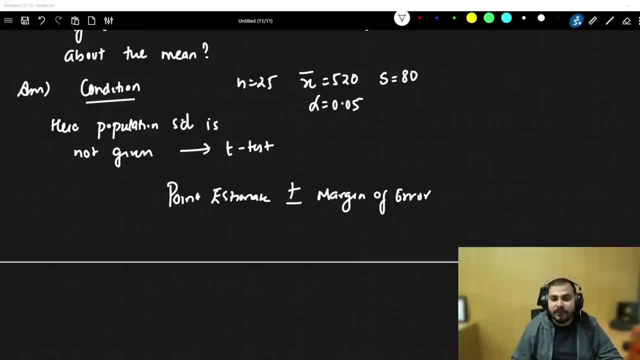 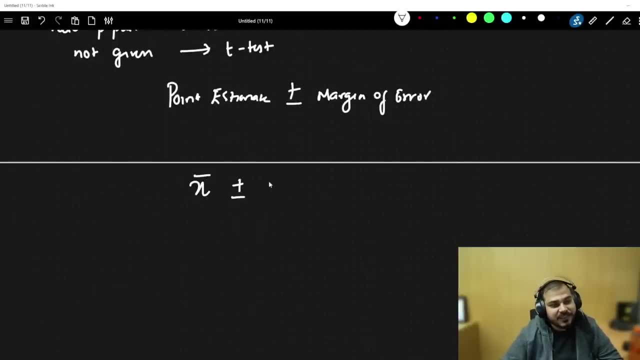 Now what kind of formula it will have. That you need to understand. The formula will be something like x bar plus or minus. instead of writing z alpha by 2, here you will be writing x bar t alpha by 2.. 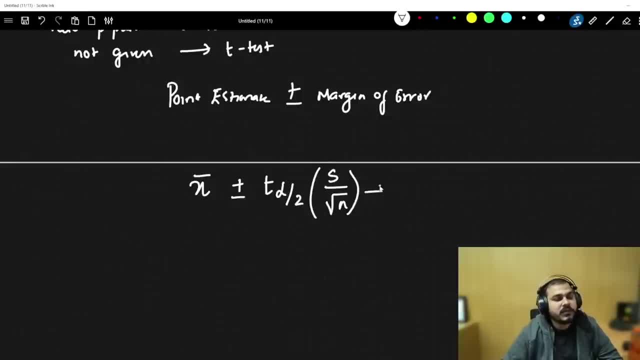 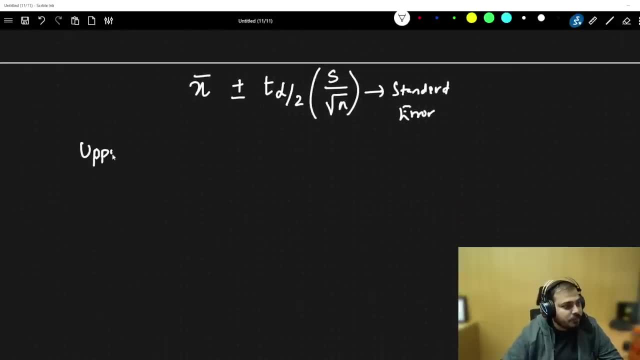 And then you will be using s by root n. This is your standard error. Now go ahead and substitute it. So two things you will be basically having. One is upper bound. It will be x bar plus t 0.05 by 2 s by root n. right. 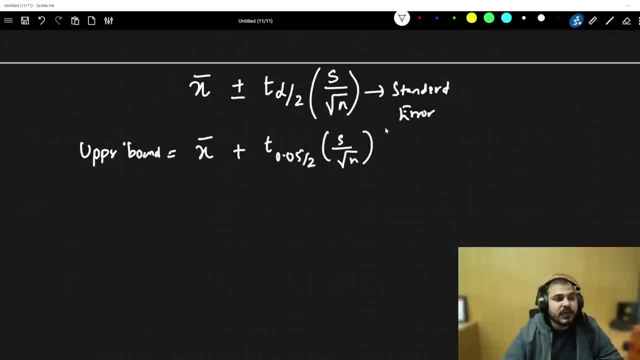 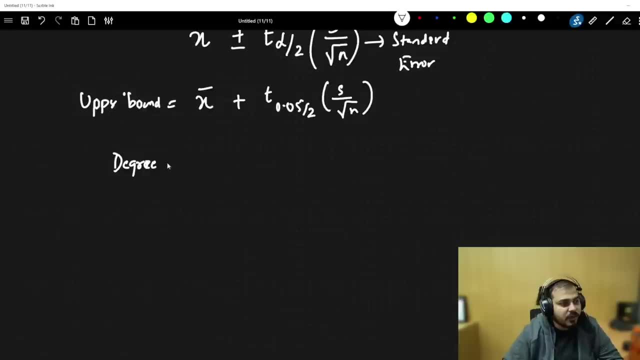 Now, first thing, first always understand. to calculate the t, okay, To calculate the t, To calculate the t value, you need to find out something called a degree of freedom, Because in the t table you will be asked this: And degree of freedom formula is just like your sample variance problem. 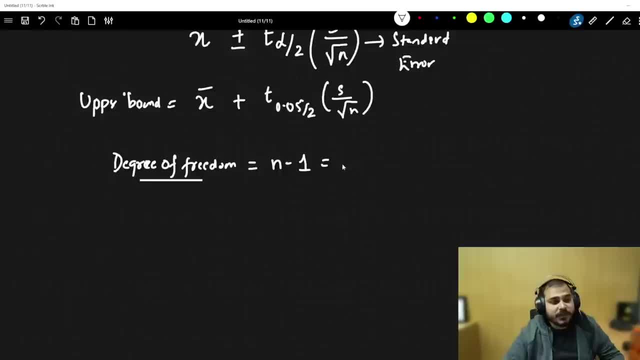 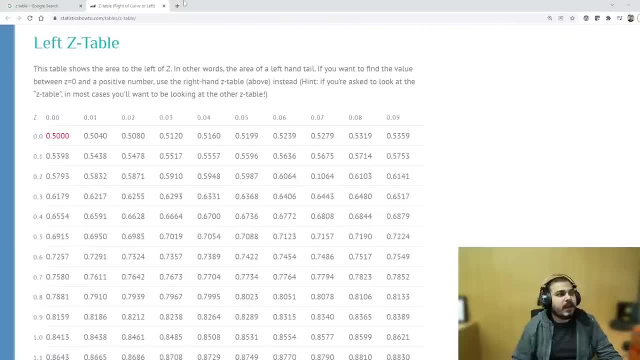 That is n minus 1, which we also use with respect to basal correction. So this will be 25 minus 1, which is nothing but 24.. Now I will go to my browser. I will open over here t table. 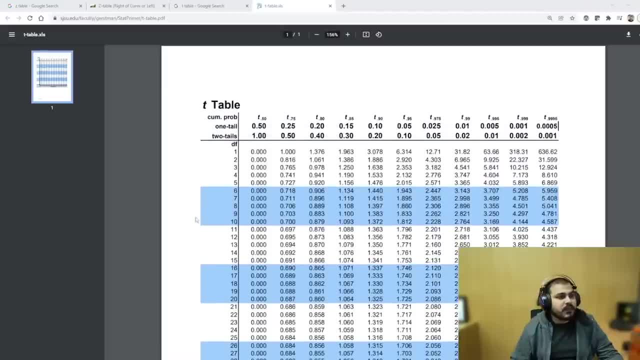 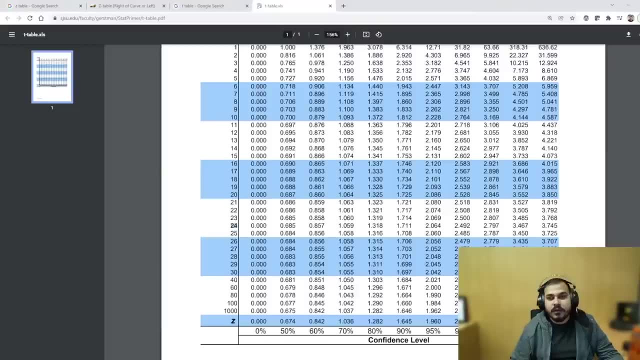 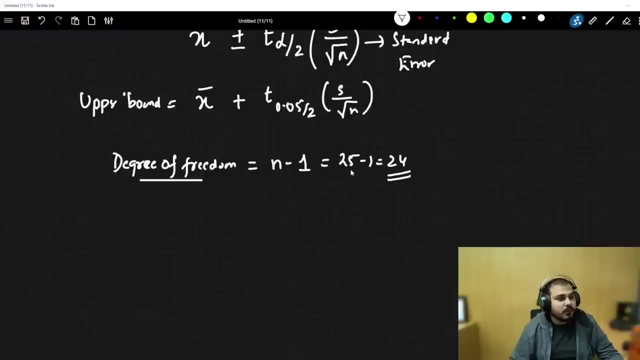 So t table I am having here Now. first thing: first you need to understand, with respect to degree of freedom, What is degree of freedom 24. Degree of freedom is 24. 25. Let's see this: This is 24, right. 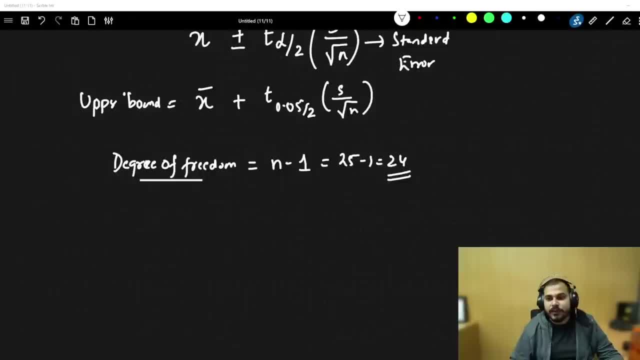 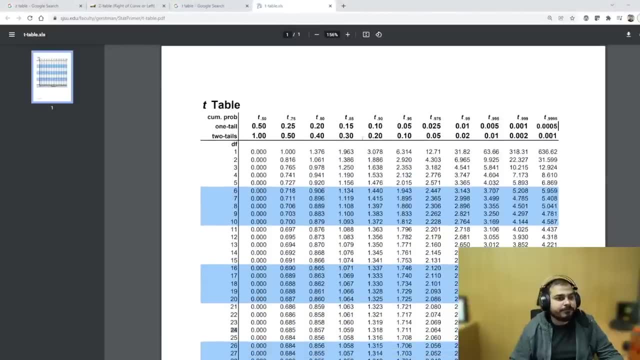 I hope everybody is able to see the degree of freedom over here. Try to have a look on to this table: 0.025. 0.025. 0.025 is nothing but 0.025.. 0.025 is nothing but this one, right. 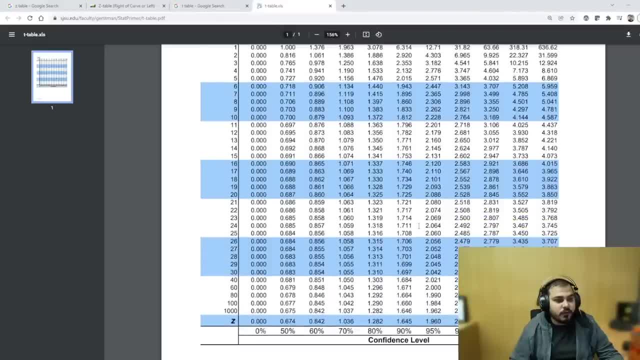 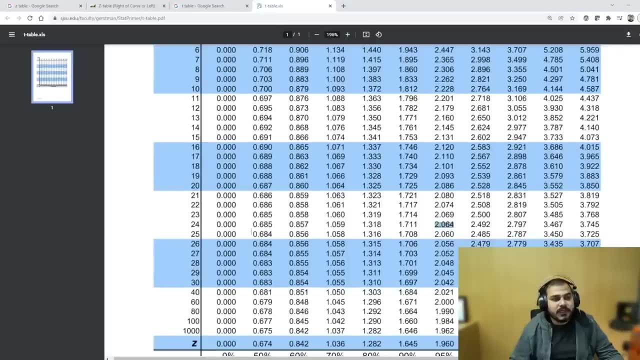 This is what: 0.975.. So if I see with respect to 24, it is nothing but 2.064.. Is everybody getting it? We have to see in this line 24 degree of freedom on the left hand side. 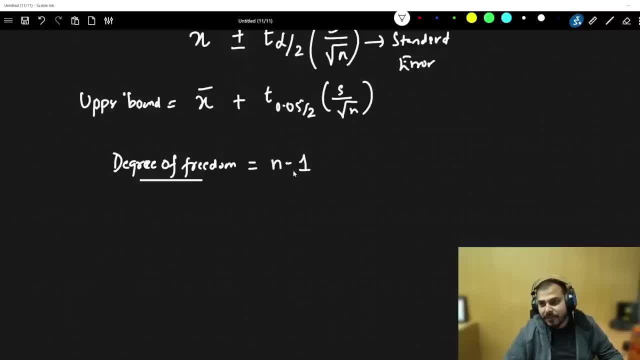 Degree of freedom formula is just like your sample variance problem, That is, n minus 1, Which we also use with respect to basal correction. So this will be 25 minus 1, which is nothing but 24. Now I will go to my browser. I will open over here. 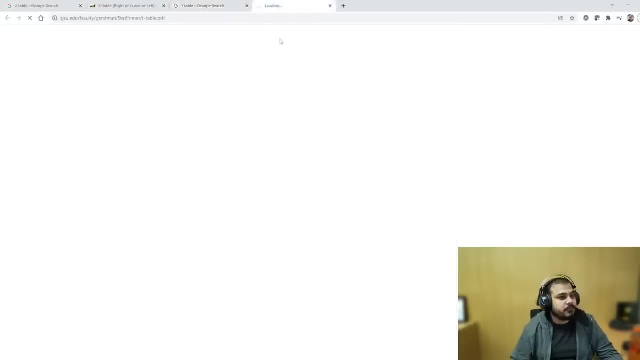 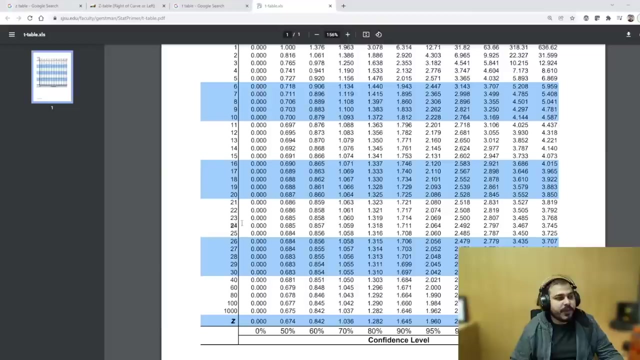 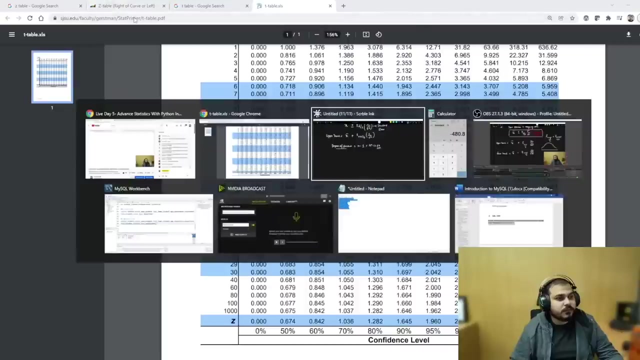 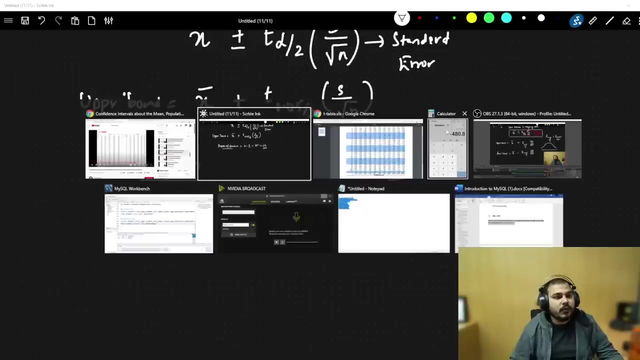 T table. so T table I am having here Now. first thing: first you need to understand, with respect to degree of freedom, What is degree of freedom? 24 degree of freedom is 24, 25. Let's see this. This is 24, right, I hope everybody is able to see the degree of freedom over here. Try to have a look on to this table. 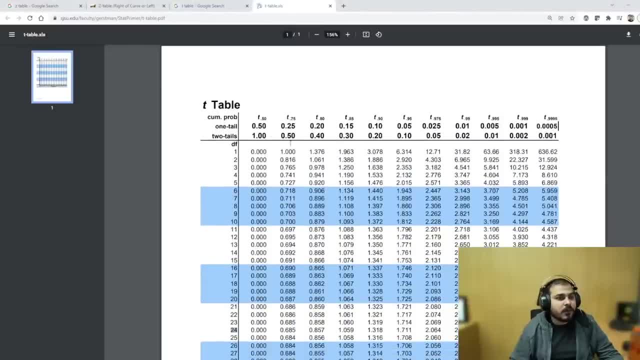 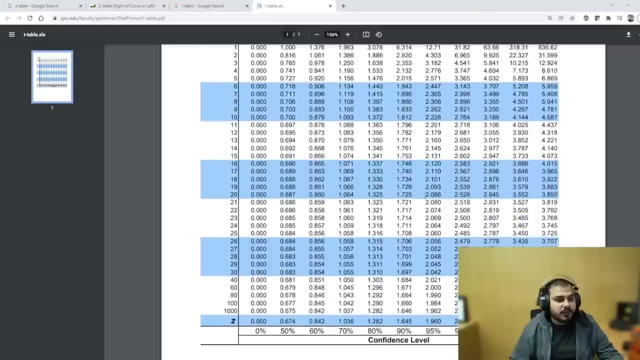 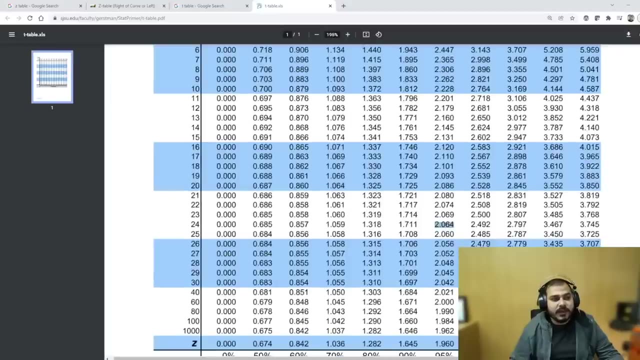 0.0.025, 0.025, 0.025 is nothing but this one, right, This is what point nine, seven, five. So if I see, with respect to two point two, twenty four, It is nothing but two point zero six, four, is everybody getting it? 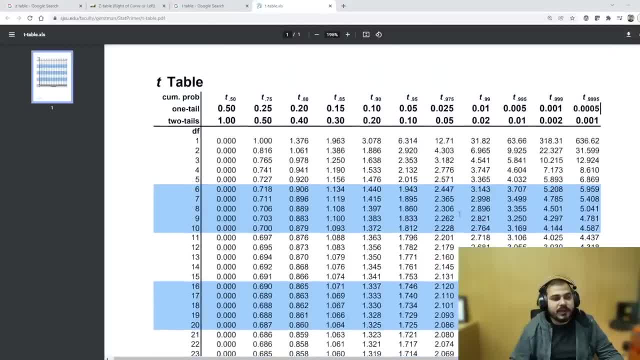 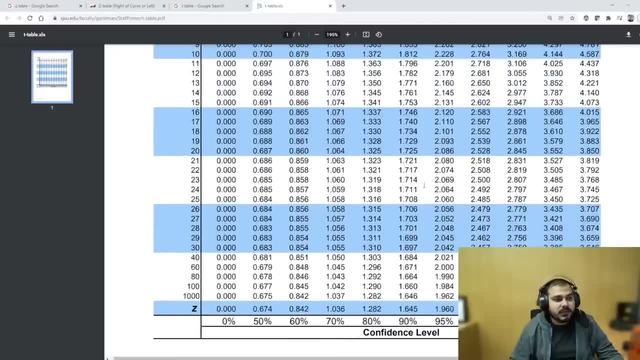 We have to see in this line twenty four degree of freedom on the left hand side, on the right hand side. You can see on top It is point zero two, five, point zero five. So the answer is two point zero six. two point zero six four. 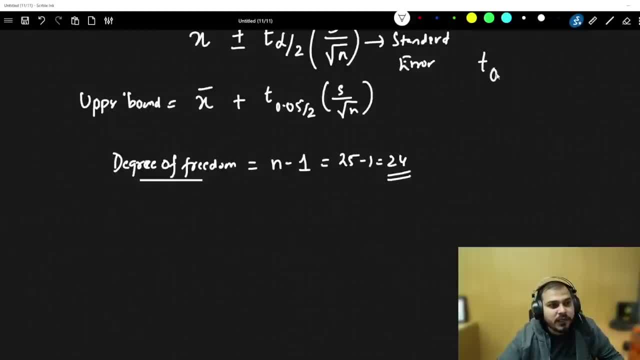 so here I'm basically going to Find your T point zero five divided by two is equal to nothing, but two point zero six four. now the next step. Once you get this, I will go and see what is my X bar. five twenty five, twenty plus two point zero six four multiplied by 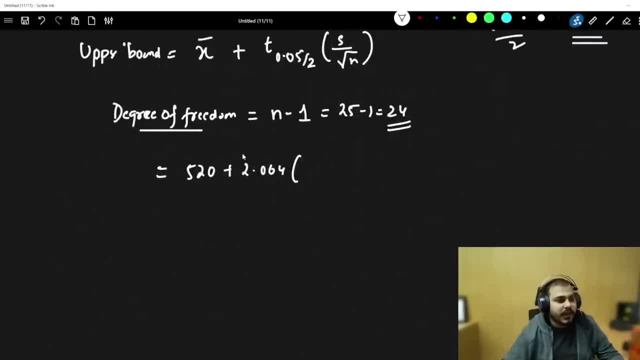 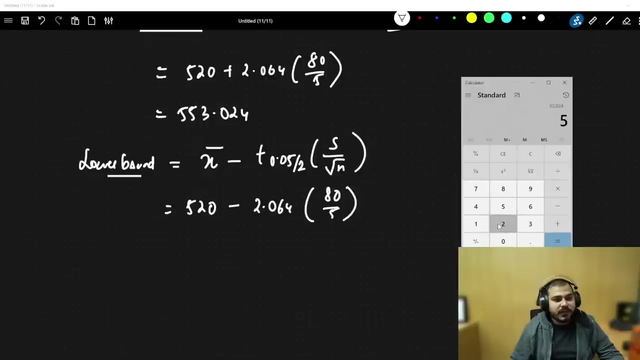 S what is s over here? It is nothing but eighty by five. Five is nothing but root. twenty five is five, Fifty three point zero two, four, and then, if I go and compute the lower bound, 520 minus two point zero six, four. eighty by five, So this minus five twenty. 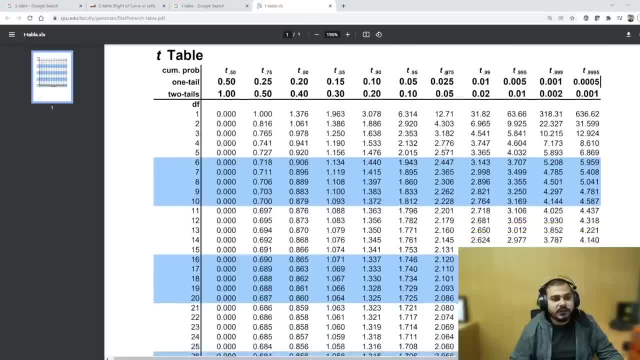 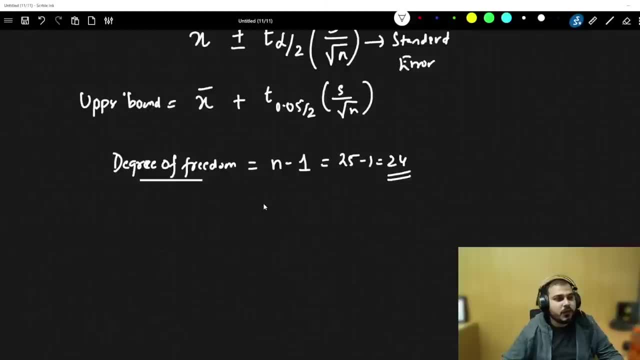 On the right hand side- you can see on top- it is 0.025, 0.05.. So the answer is 2.064.. 2.064.. So here I am basically going to find your t.05.. 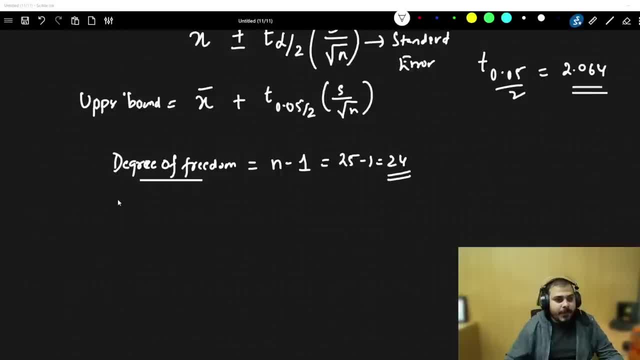 5 divided by 2 is equal to nothing but 2.064.. Now the next step. once you get this, I will go and see what is my x bar 520.. 520 plus 2.064 multiplied by s. 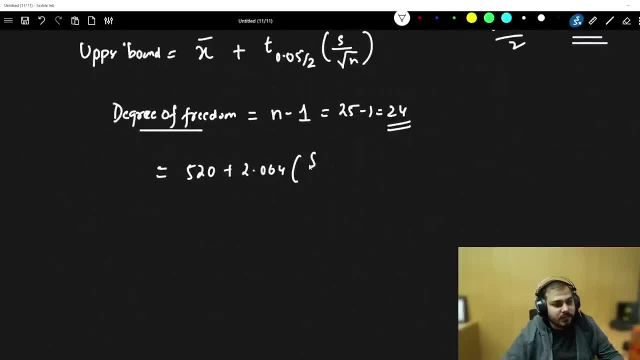 What is s over here? It is nothing but 80 by 5.. 5 is nothing but root. 25 is 5. 553.024. 5.. Then, if I go and compute the lower bound, 520 minus 2.064,, 80 by 5.. 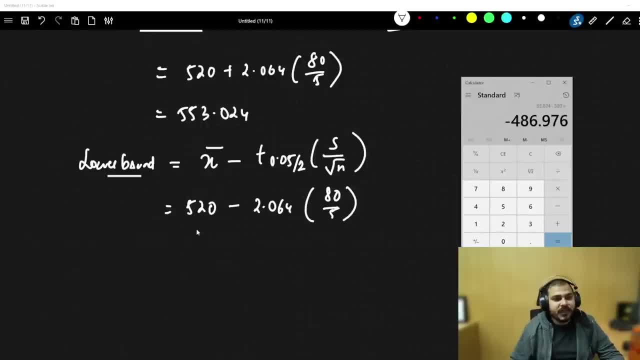 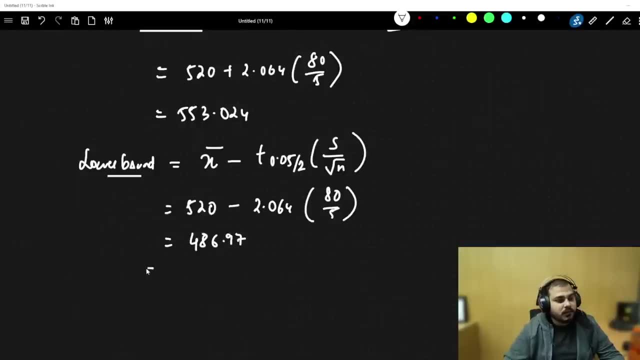 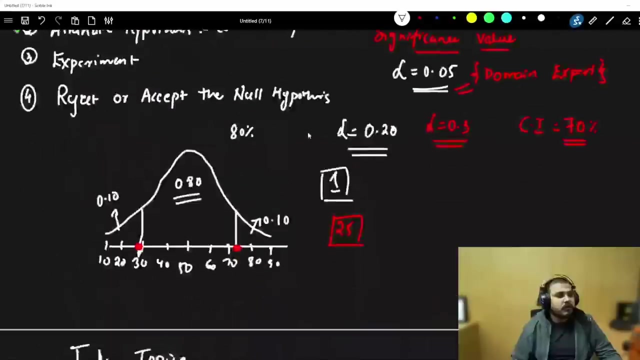 So this minus 520.. So here I am actually getting 486.97.. So my lower bound is nothing but 486.97.. The upper bound of the confidence interval is nothing but 553.024.. So with this we have done. wow, I have written so much today. 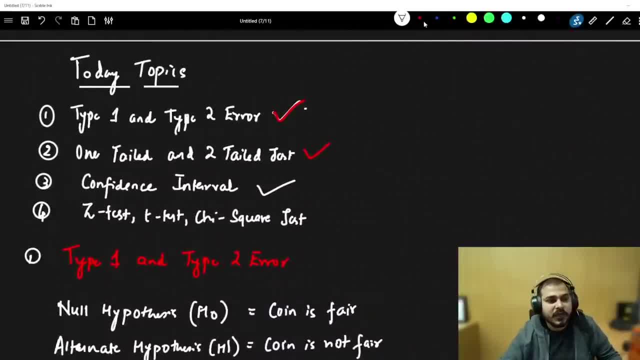 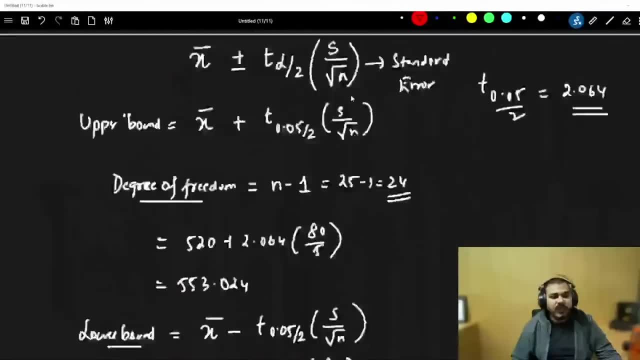 We have finished confidence interval. Congratulations everybody. We have successfully completed. Congratulations. Why? this is not 2 tail, This is 2 tail only. no, I told you. no, This is 2 tail. Why you are getting confused? 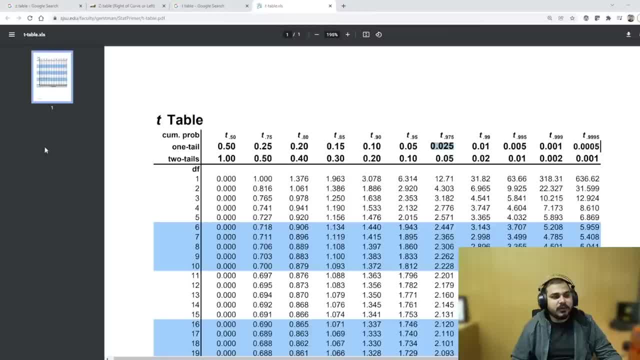 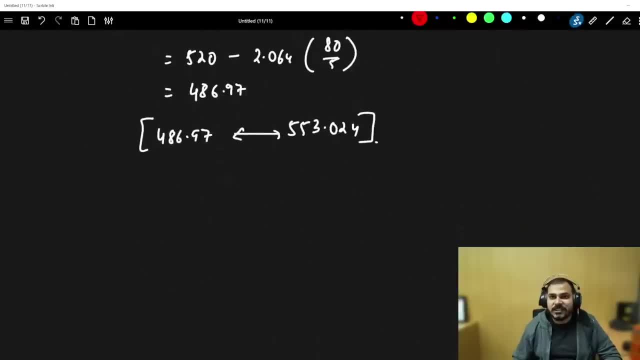 See over here. If I see over here, 0.025 for 1 tail, For 2 tail, this is 0.05.. Now let us go ahead and try to do the first Z test. I hope everybody has understood. why do we use Z test? 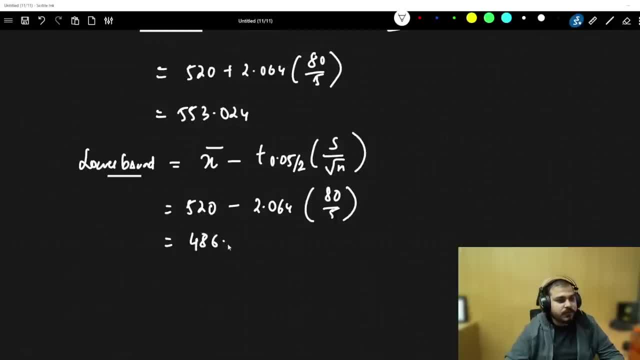 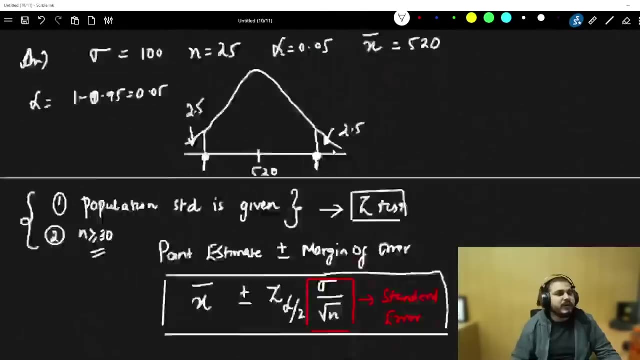 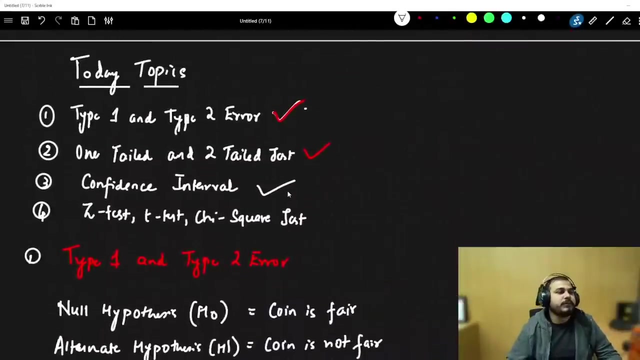 So here I'm actually getting four, eighty six point Nine seven. So my lower bound is nothing but four, eighty six point nine seven. the upper bound of the confidence interval is nothing but five, five, three point zero two. so with this we have done. Wow, I have written so much today. We have finished confidence interval. 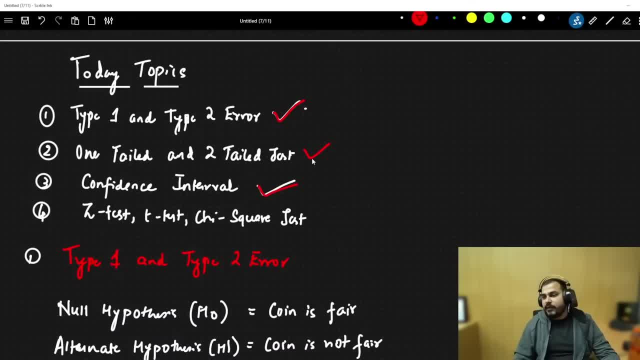 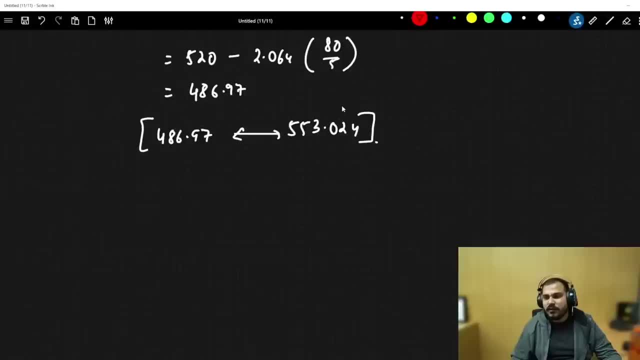 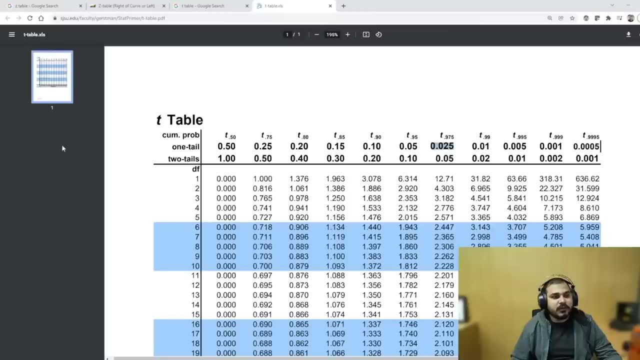 Congratulations everybody. We have successfully completed. Congrats. Why? this is not two tail, This is two tail only. no, I Told you know this is two tail. why you're getting confused? See over here. if i see over here: 0.025 for one tail, for two tail, this is 0.05. now let's go ahead and try to. 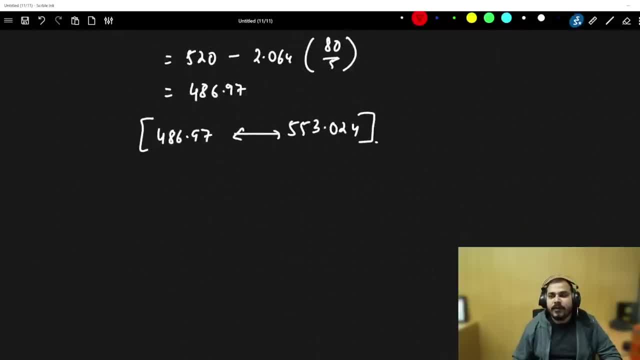 do the first z test. i hope everybody is understood. why do we use z test? so the first question that we are going to solve is one sample z test. now we will perform hypothesis testing. so the first problem that we are going to solve is one sample z test. now we are going to perform hypothesis. 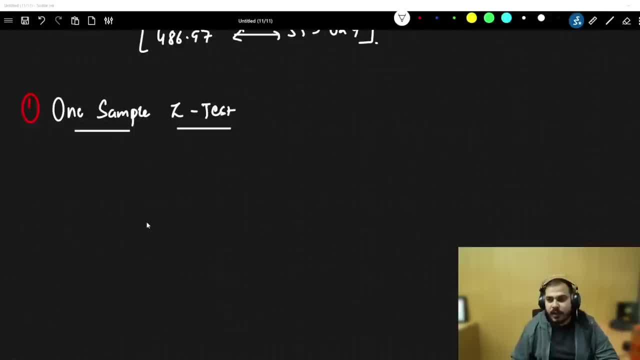 testing. what exactly is one sample z test? first of all, i told you two conditions with respect to z test. the first condition is that the population standard deviation is given at that time you use z test. the second thing is that your sample size should be. sample size should be, have a size at. 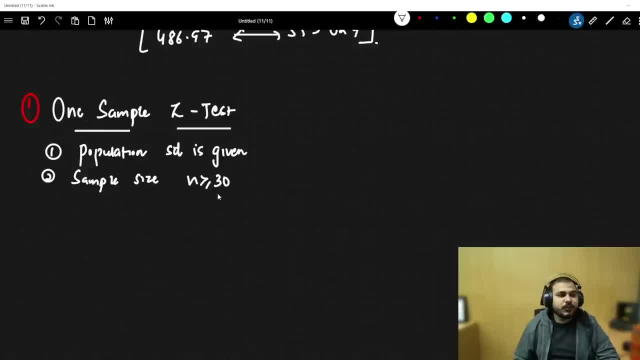 is greater than or equal to 30.. just to make calculation easier, i just put it at n is equal to 25 because root of 25 was 5. so because of that i put it: don't fight with me. i have no energy. i think you will beat me and go. 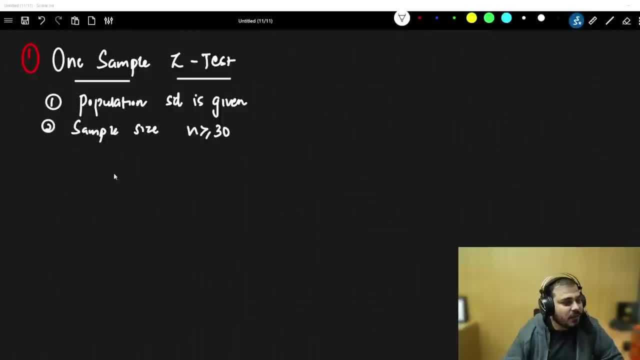 but i don't have any energy. okay, so let's go ahead and let's try to see how to do a hypothesis testing. okay, let's say that i'm writing a problem statement. in the population, the average iq with a you standard deviation of 15. okay, researchers wants to test a new medication to see. 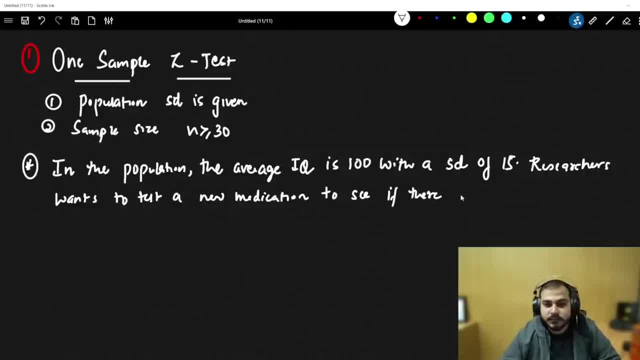 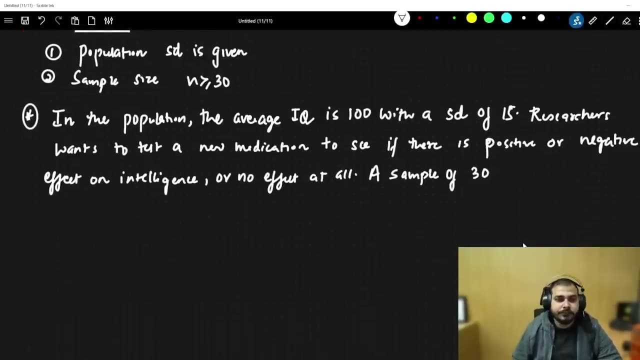 if there is positive or negative effect on intelligence or no effect at all. a sample of 30 participants who have taken the medication has a mean. has a mean iq of. has a mean iq of 140. did the medication the intelligence? just by reading the question. what do you get it from? 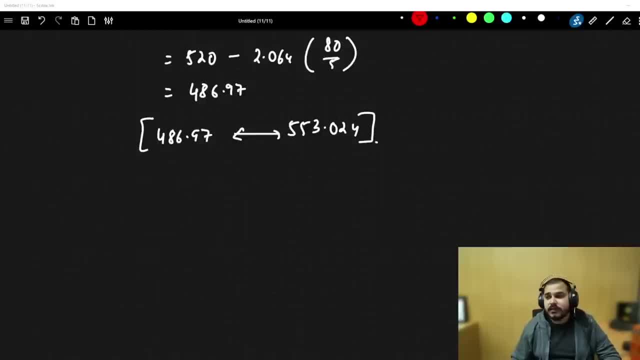 So the first question that we are going to solve is one sample Z test. Now we will perform hypothesis testing. So the first problem that we are going to solve is one sample Z test. Now we are going to perform hypothesis testing. 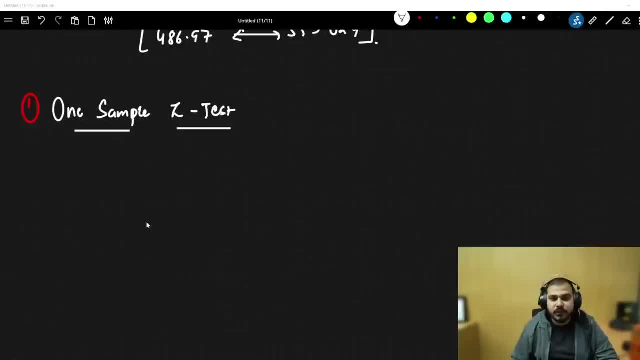 What exactly is one sample Z test? First of all, I told you two conditions with respect to Z test. The first condition is that the population standard deviation is given At that time you use Z test. The second thing is that your sample size should be. sample size should be have a size at least n is greater than or equal to 30.. 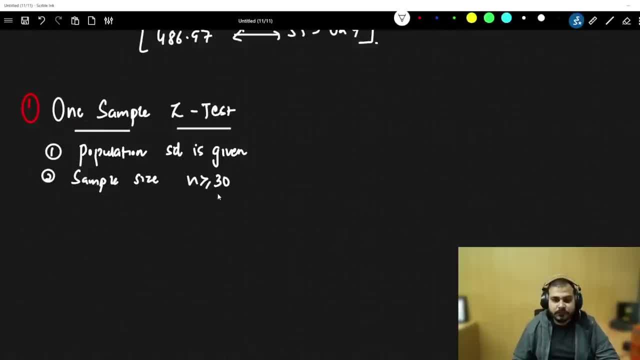 Just to make calculation easier, I just put it at n is equal to 25.. Because root of 25 was 5, so because of that I put it: Do not fight with me. I have no energy. I think you will beat me and go, but I do not have any energy. 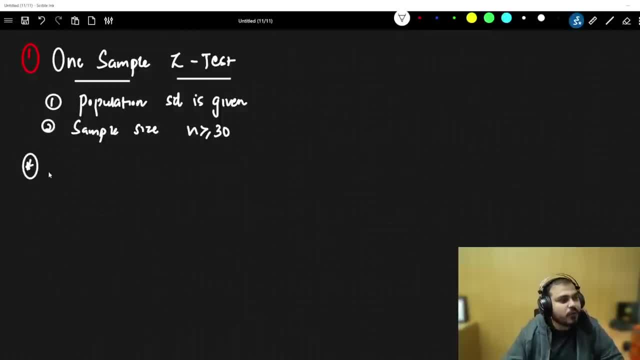 So let us go ahead and let us try to see how to do a hypothesis testing. Let us say that I am writing a problem statement In the population, the average IQ, with a standard deviation of 15.. Researchers want to test a new medication to see if there is positive or negative effect on intelligence. 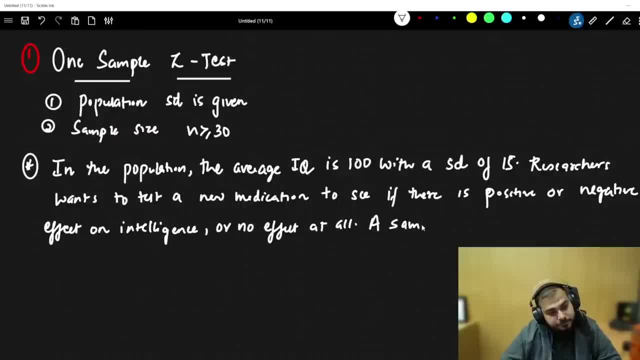 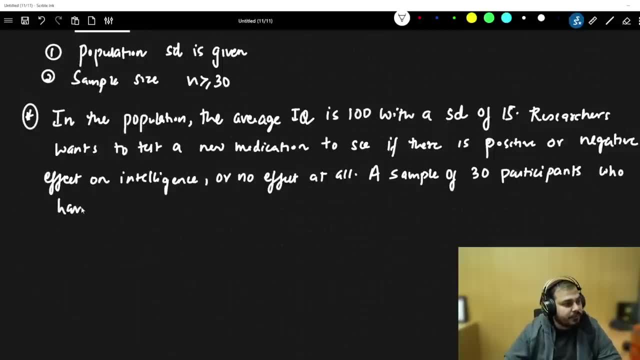 Or no effect at all. A sample of 30 participants who have taken the medication has a mean. has a mean IQ of. has a mean IQ of 140.. Did the medication the intelligence? Just by reading the question? what do you get it from it, guys? 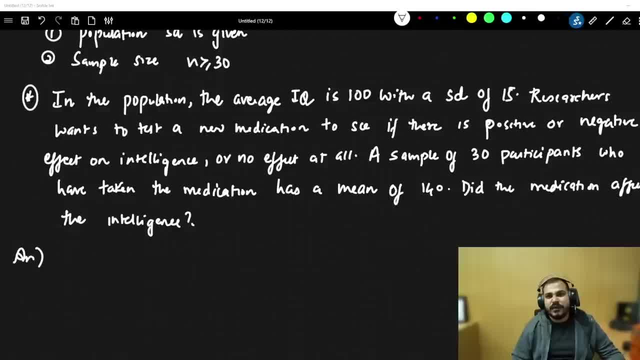 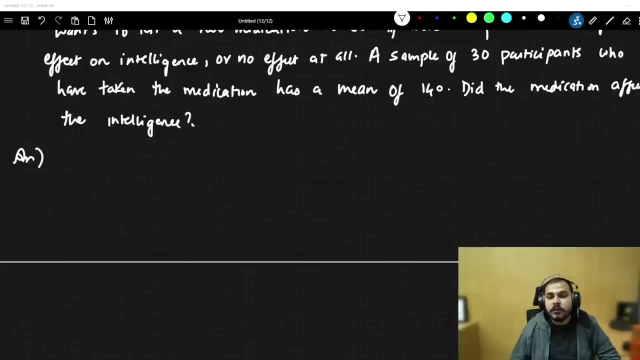 Did the medication improve the improve the intelligence or not? Now I will show you how to perform a hypothesis testing. Okay, Obviously you got to know that, what test it is used. Okay, So let us go ahead, and let us go ahead and discuss it. 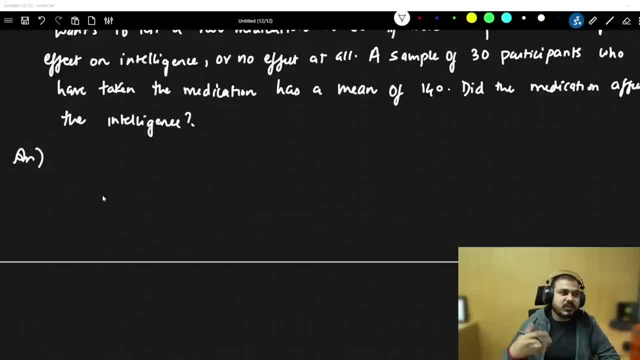 Now, first of all, how to perform a hypothesis testing. Okay, So the first step is that we need to define the null hypothesis. Now, in this particular case, null hypothesis is S0.. Now, in S0, what you will basically say, that: 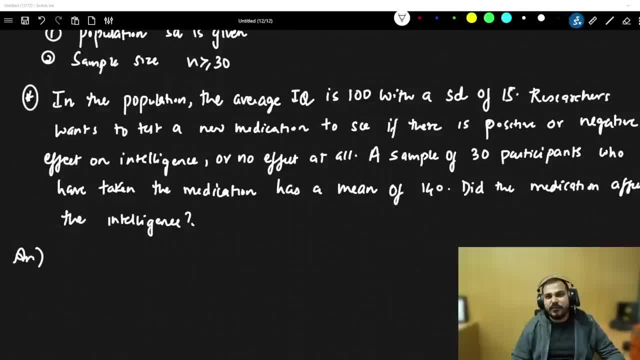 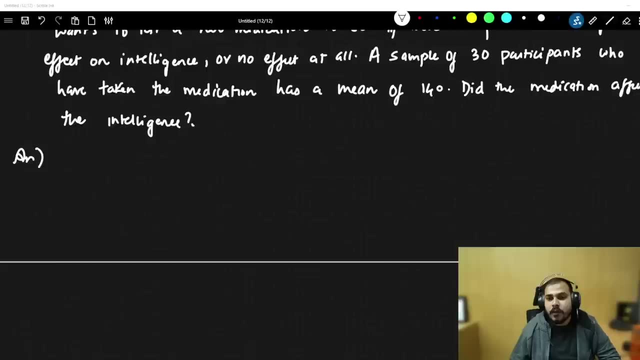 guys, did the medication improve the improve the intelligence or not? now i will show you how to perform a hypothesis testing. okay, obviously you got to know that, what test it is used. okay, so let's go ahead, and let's go ahead and discuss it now. first of all, how to perform a hypothesis testing. okay, so the first. 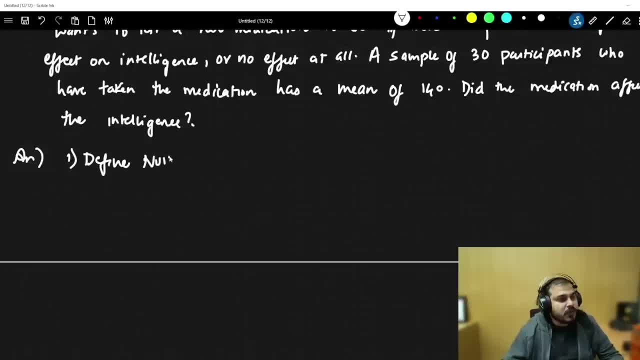 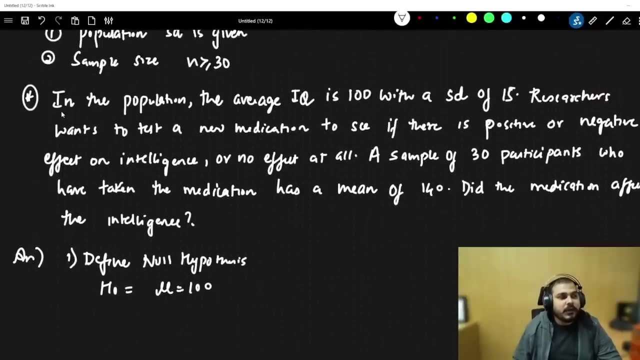 step is that we need to define the null hypothesis now. in this particular case, null hypothesis is s0. now, in s0, what you will basically say that your mean is nothing but 100. can i say your mean is 100 because see the in the. obviously we need to check whether the medication effect the intelligence. 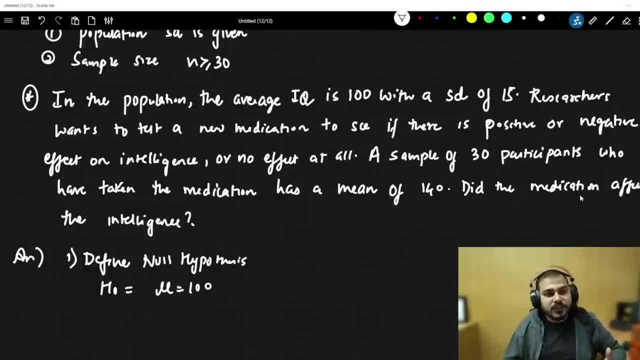 or not. so here i will say that my null hypothesis will be that my mean is my mean iq is 100. my alternate will be that mean is not equal to 100. I hope everybody is agreeing with this, agreeing with this. everybody is agreeing with this. clearly right. so over here. s0 is 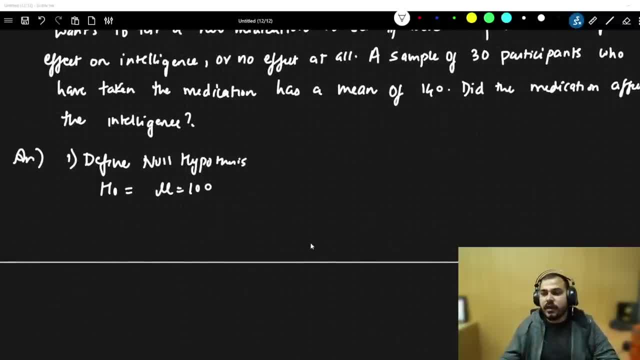 equal to mean is equal to 100. okay, so this basically says that it is your null hypothesis. the second thing is that we need to define our alternate hypothesis. my alternate hypothesis is s0, where my mean is not equal to 100. my mean is not equal to 100 because, if I am saying my null hypothesis in the mean is equal to 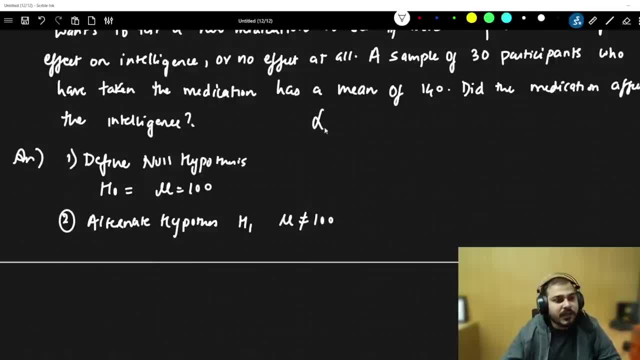 100, then this will not equal to another one important thing that I mentioned forgot to mention: my alpha over here will be 0.05. that basically means my confidence interval is 95. so this is also a part of the question. now the third step. let's go to the third step. okay, mean is not 140, mean is 100. sample. 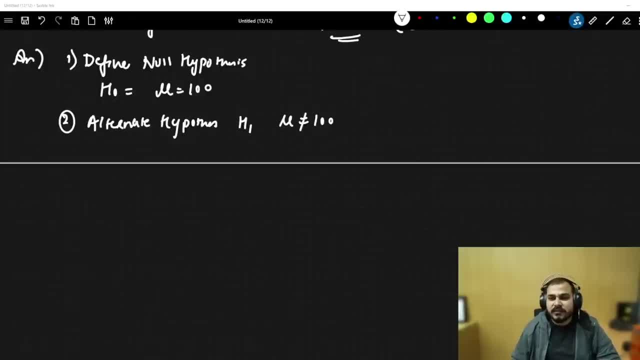 mean is 140. you can apply in any concept, guys. it need not be that you can only apply in something. okay? the third step: we basically state our alpha value, state alpha value. so my alpha value is negative. so my alpha value is negative, value is 0.05.. The fourth step: Let's go to the fourth step now. What do you think? the fourth: 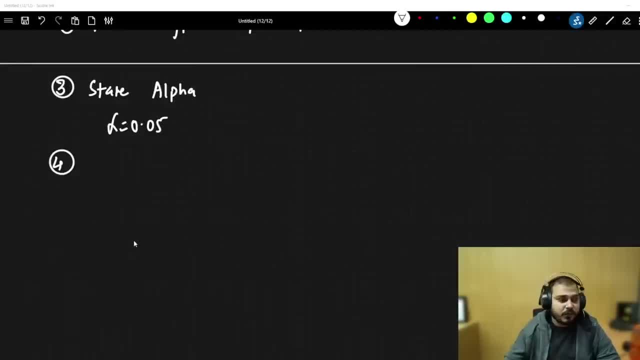 step is. In the fourth step I need to provide my decision rule. So here I will say state decision rule And always understand: in the decision rule you need to specify this graph And here you will basically say that since my alpha is 0.05, what kind of test this will be? 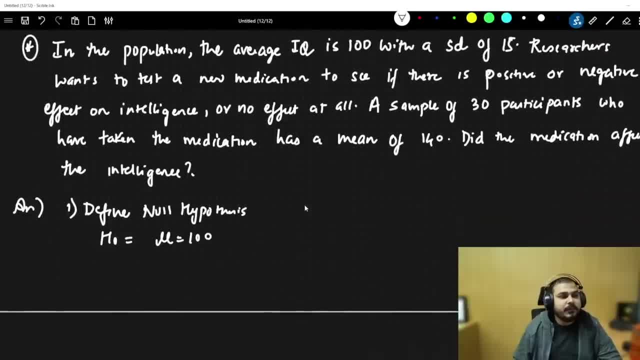 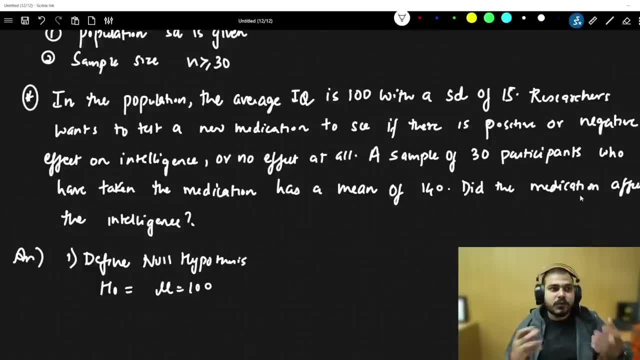 your mean is nothing but 100.. Can I say your mean is 100?? Because see the in the, obviously we need to check whether the medication affect the intelligence or not. So here I will say that my null hypothesis will be that my mean is my mean IQ is 100.. 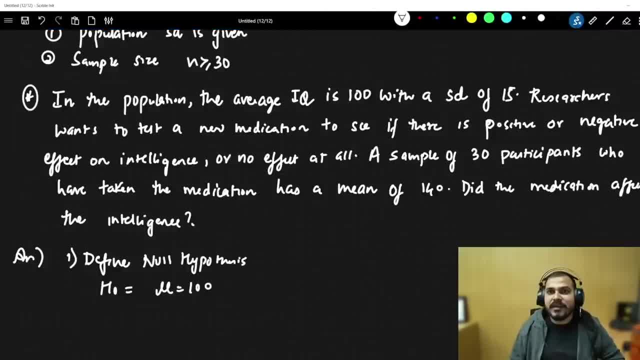 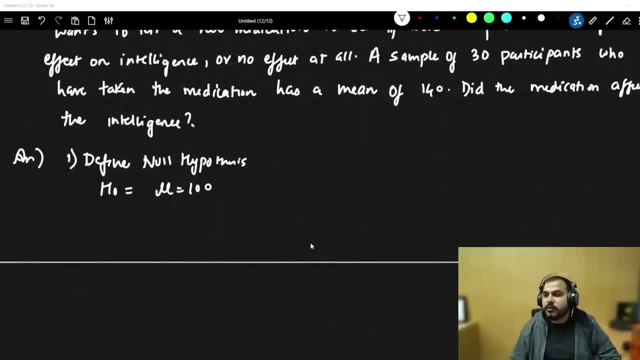 My alternate will be that my mean is not equal to 100.. I hope everybody is agreeing with this, Agreeing with this. Everybody is agreeing with this, clearly, Right? So over here, S0 is equal to mean is equal to 100. 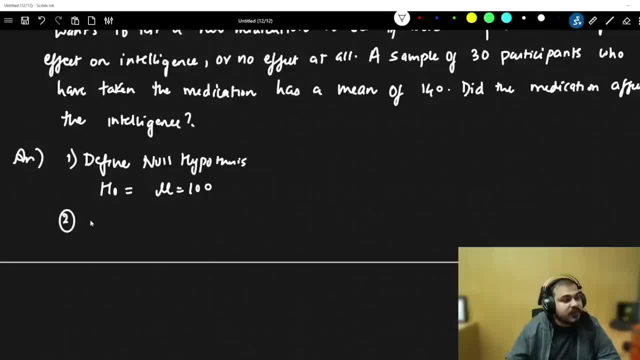 Okay, So this basically says that it is your null hypothesis. The second thing is that we need to define our alternate hypothesis. My alternate hypothesis is S0, where my mean is not equal to 100.. My mean is not equal to 100. 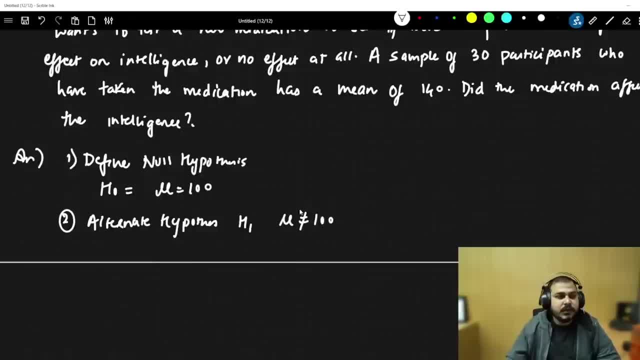 Because if I am saying my null hypothesis is a mean is equal to 100, then this will not equal to 100.. One important thing that I mentioned forgot to mention: my alpha over here will be 0.05.. That basically means my confidence interval is 95%. 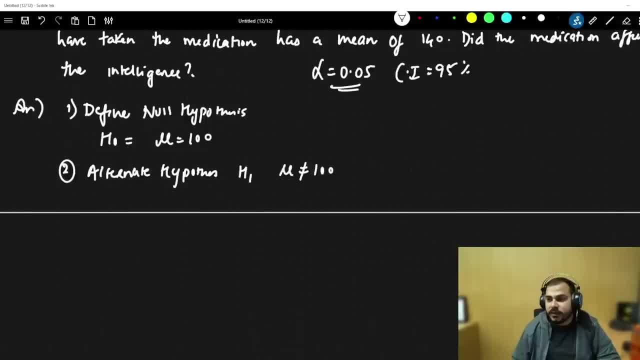 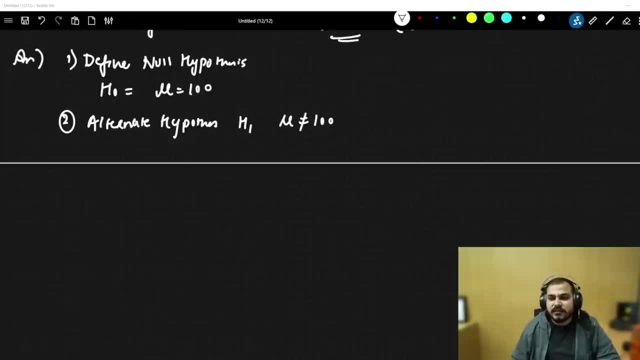 So this is also a part of the question. Now the third step. Let us go to the third step. Mean is not 140.. Mean is 100.. Sample: mean is 140.. You can apply in any concept, guys. It need not be that you can only apply in something. 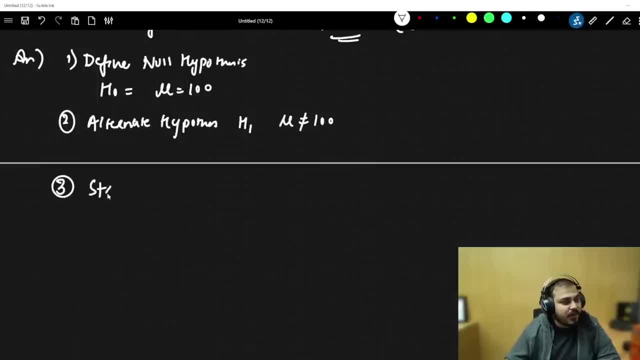 Okay, The third step. we basically state our alpha value. State alpha value. So my alpha value is 0.05.. The fourth step. Let us go to the fourth step. now What do you think the fourth step is? In the fourth step, I need to provide my decision rule. 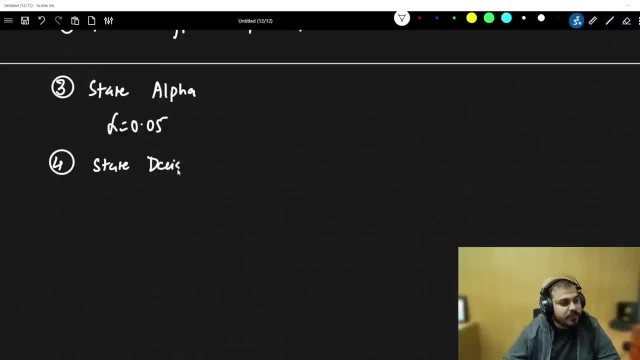 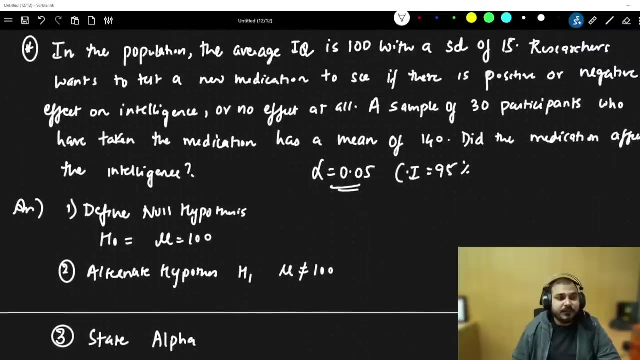 So here I will say state decision rule And always understand: in the decision rule you need to specify this graph, And here you will basically say that, since my alpha is 0.05.. What kind of test this will be? Did the medication affect the intelligence? 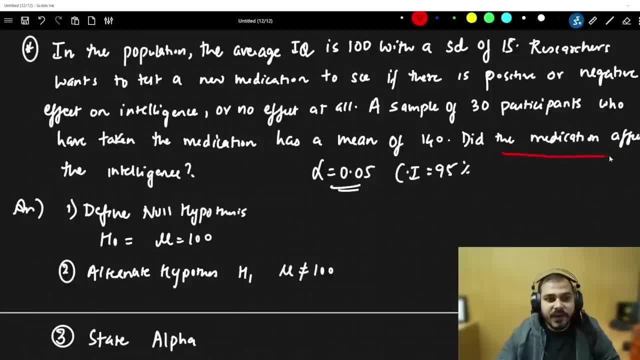 The question. Understand this question: Did the medication affect the intelligence? So here we are just focusing on that: whether the medication increase your intelligence or whether it decreased your intelligence. Okay, So either it can be. So this definitely will become a two tail test. 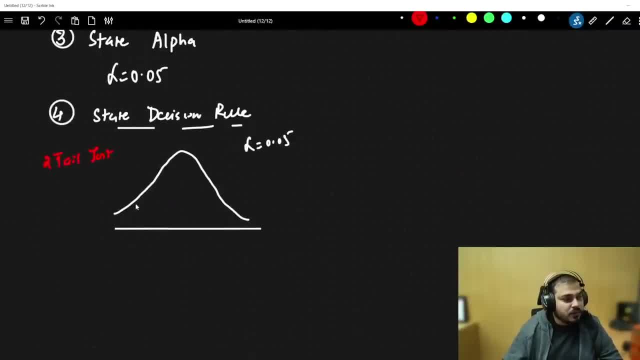 So two tail test. So here I will be having 2.5.. Here I will be having 2.5.. So this will be 2.5.. This will be 2.5. And this will be 95%. 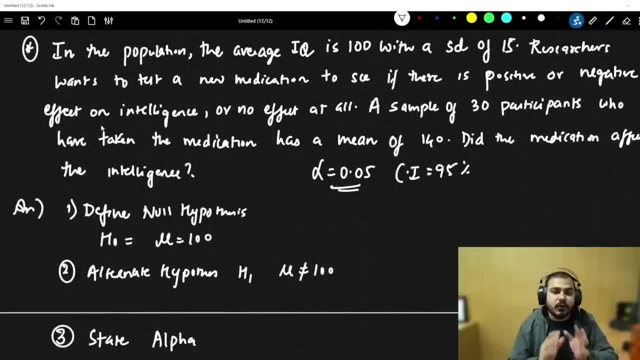 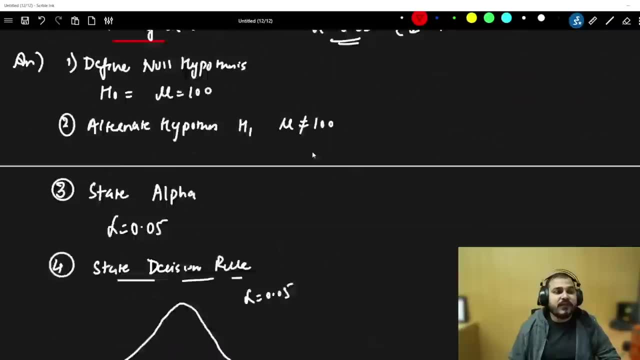 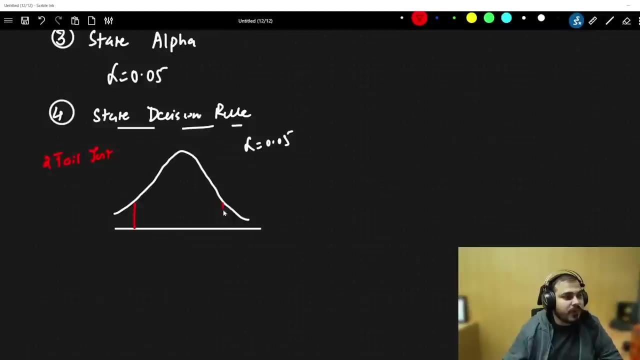 Did the medication affect the intelligence? The question, understand this question: Did the medication affect the intelligence? So here we are just focusing on that: whether the medication increase your intelligence or whether it decreased your intelligence. So either it can be. So this definitely will become a two-tailed test. So two-tailed test. So here I will be having 2.5.. 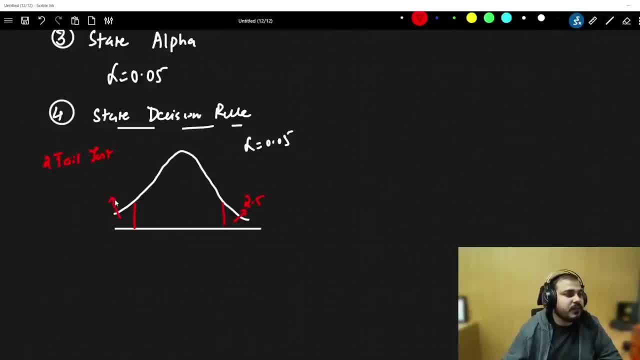 Here I will be having 2.5.. So this will be 2.5. This will be 2.5. And this will be 95%, Right? Everybody is clear with this. Can I get a quick yes? Right, This will definitely become a two-tailed test. And one more important thing over here. 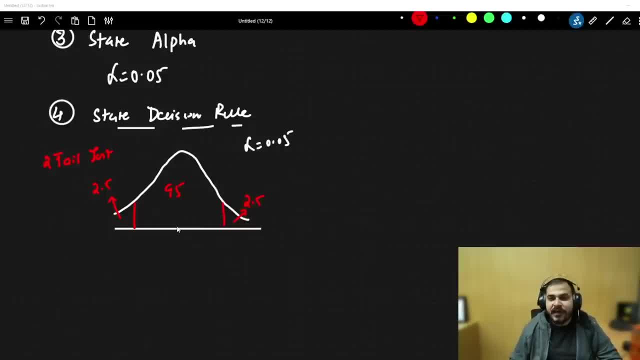 when I say 2.5,, then if I really want to find out, with the help of Z test, what will be this value, I have to check it for 1 minus 0.025.. Right, So this will be 0.975.. In this particular value, 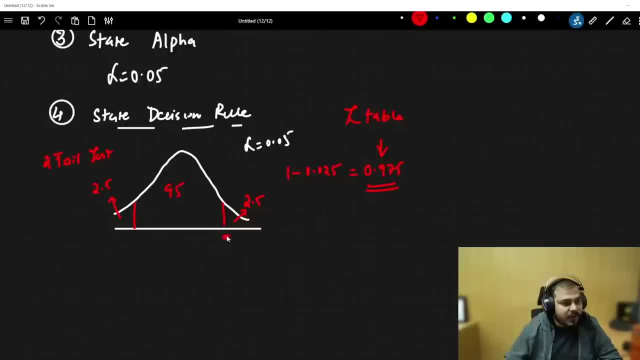 I need to check in my Z table, So I need to find out this value and this value Right, Go ahead and check it. Go ahead and check it. What will be the value over here? This will be plus 1.96.. This will. 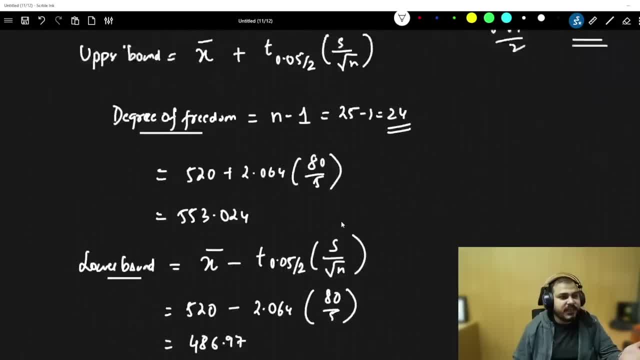 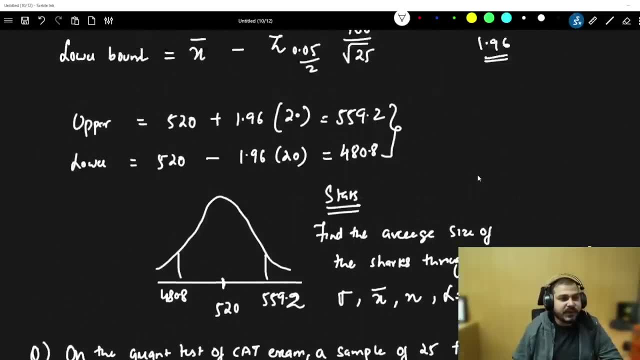 be minus 1.96.. We just checked it Right. We just checked it over here. You can see over here, Right, Where did it go Here? we got this. This was for T Right. This was for Z For Z. we got this Right. 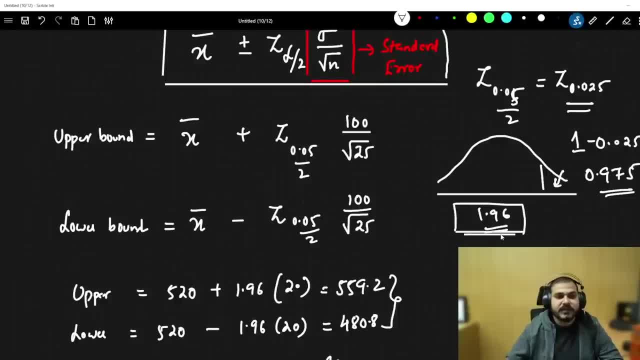 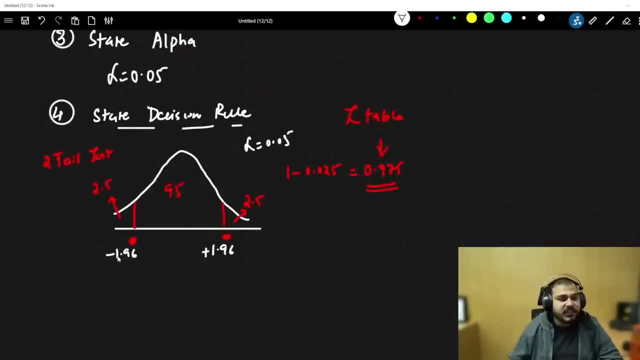 1.96.. See this, We got 1.96.. Okay, So 1.96 plus minus 1.96.. Now I know my decision rule, My whatever experiment I will perform later on, whatever Z score value I will be getting, I should be getting within this minus. 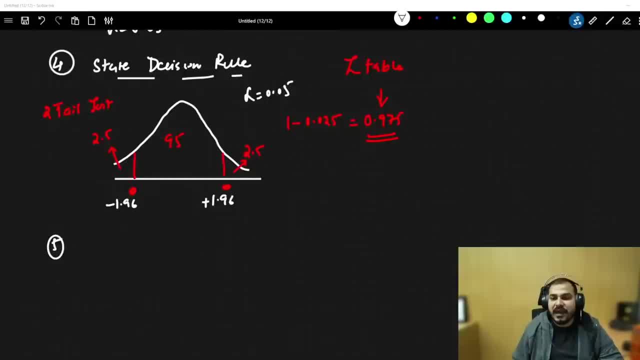 1.96 to plus 1.96.. Now here I will use my test statistics. Now, what will be my test statistics over here? It's very simple. What is the Z score formula? we basically use Calculate test statistics And this will be T test, Right? So the formula that we basically use. sorry, Z test. I am extremely 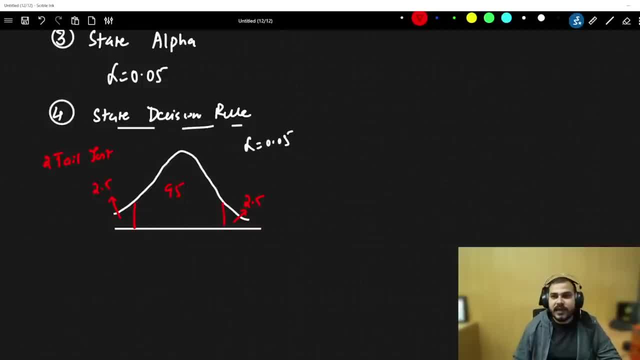 Right, Everybody is clear with this. Can I get a quick yes? Right? This will definitely become a two tail test. And one more important thing over here When I say 2.5.. Then If I really want to find out with the help of Z test. 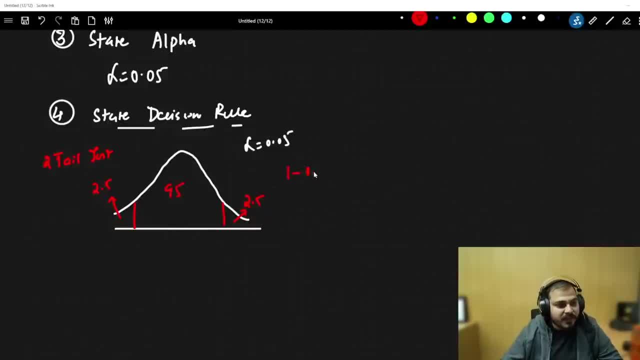 What will be this value? I have to check it for 1 minus 0.025.. Right, So this will be 0.975.. In this particular value, I need to check in my Z table. So I need to find out this value and this value. 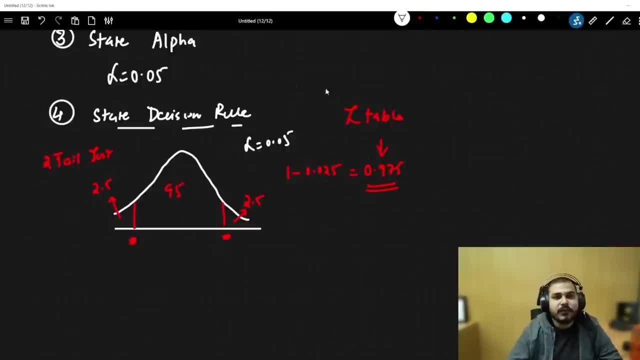 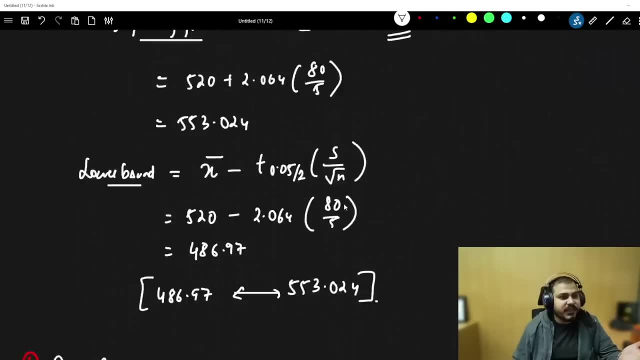 Right, Go ahead and check it. Go ahead and check it. What will be the value over here? This will be plus 1.96.. This will be minus 1.96.. We just checked it Right. We just checked it over here. 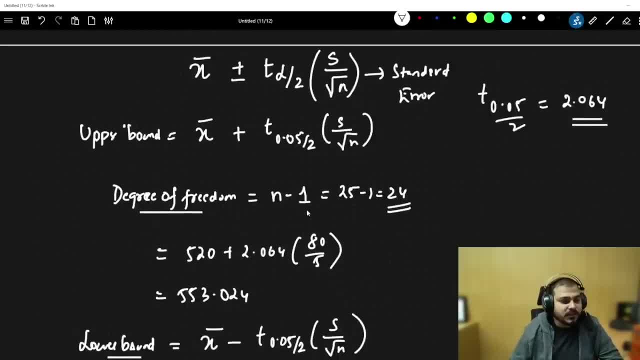 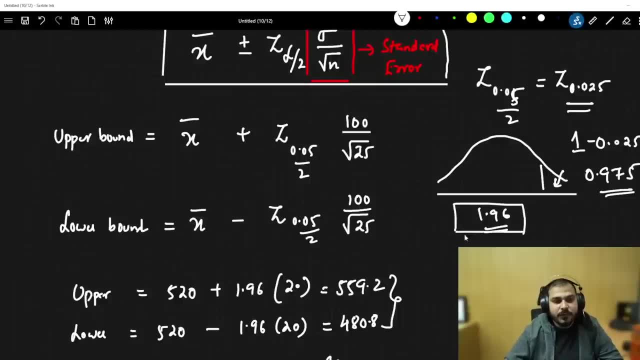 You can see over here, Right, Where did it go? Here, we got this. This was for T Right. This was for Z For Z. we got this Right: 1.96.. See this: We got 1.96.. 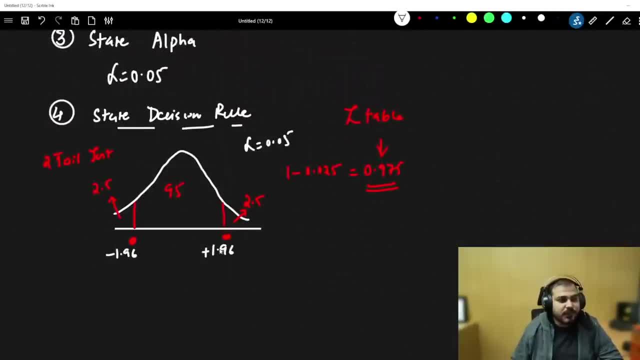 Ok, So 1.96 plus minus 1.96.. Now I know my decision rule, My Whatever experiment I will perform later on, Whatever Z score value I will be getting, I should be getting Getting within this minus 1.96 to plus 1.96.. 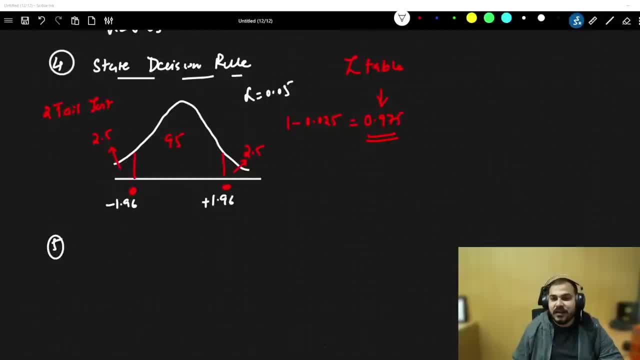 Now here I will use my test statistics. Now, what will be my test statistics over here? It is very simple. What is the Z score formula? we basically use Calculate test statistics And this will be T test, Right? So the formula that we basically use. 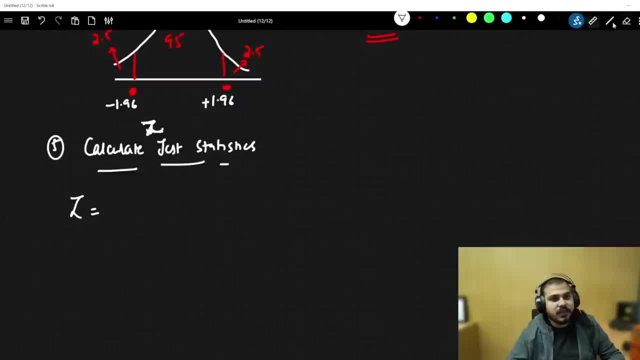 Sorry, Z test. I am extremely sorry. This will be Z test, Not T test. Z test, Z test: Calculate Z. What is the formula that we basically use? X minus mu divided by standard deviation. I hope everybody remembers this formula. 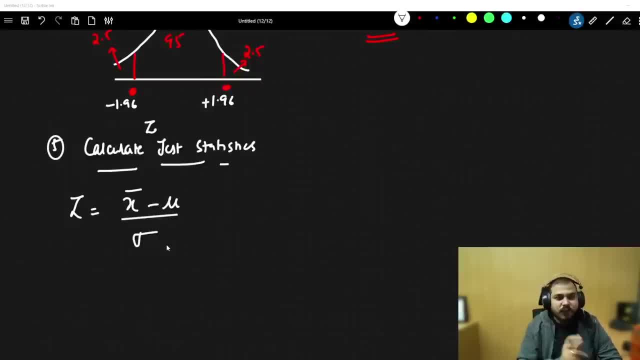 Right. But understand one thing: The real formula of Z square is Z test. is This divided by root N, The reason why we did not consider before root N? Understand: For every sample, my N value will be 1.. So whenever I write root of 1.. 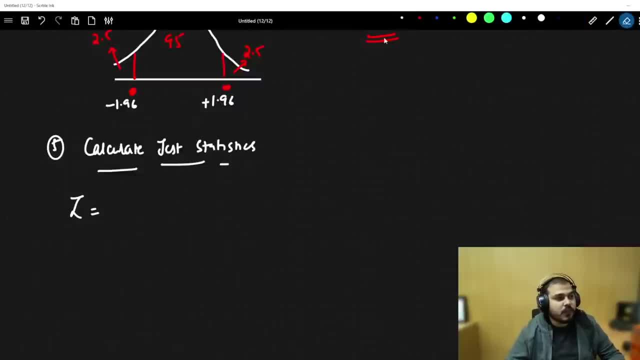 sorry, This will be Z test, not T test. Z test: Calculate Z. What is the formula that we basically use? X minus mu divided by standard deviation. I hope everybody remembers this formula Right, But understand one thing: The real formula of Z square is Z test. is this divided by root n. 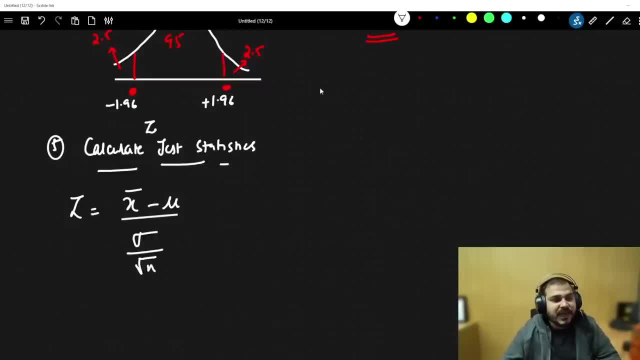 And the reason why we did not consider before root n understand. for every sample, my n value will be 1.. So whenever I write root of 1, it will be 1.. Right, But when we are working with a huge sample, 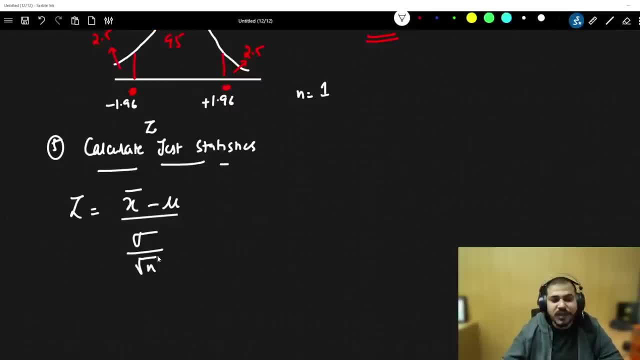 right. When we are working with a huge sample, we have to basically use root n And this is called as standard error. Standard error Like how we divide something by, you know, n minus 1.. There is some reasons why we do it, But when we are working with a huge sample, we have to basically. 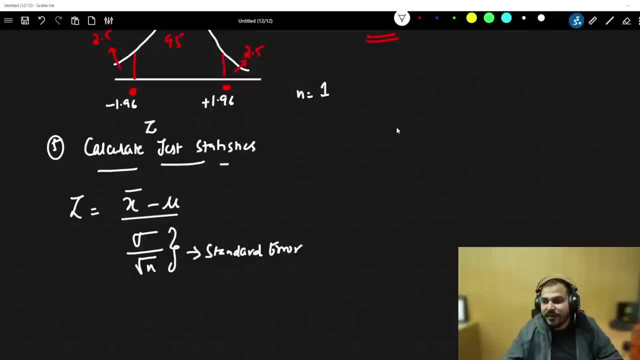 do it. Okay, And probably I do not know whether you have seen my video or not- Okay, So this is basically called as standard error. So we have to divide by root n. Always understand. for one sample, this root n will already be 1.. So we have to use this particular formula. Okay, To do this. 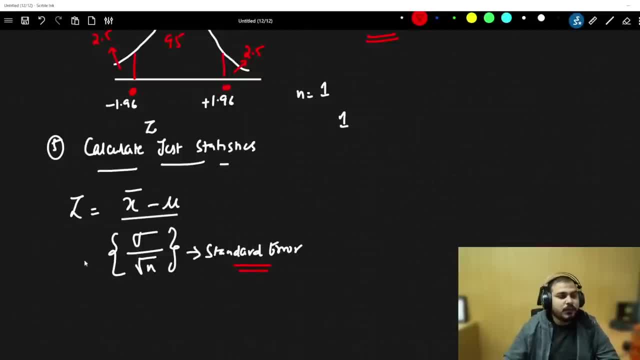 Okay, So this is basically my standard error formula, which is specified by this And always remember. because why do we use this? I will just give you one example. Suppose I take 5 samples. right, I take 5 samples, 5 different, different samples from a population 5,, 5, 5. 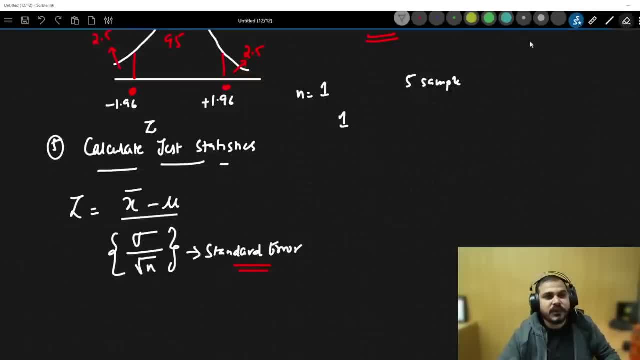 samples from different different. Let us say that I have a population of 1000 points. Okay, Let us say that I have a population of 1000 points, 1000 points. Let us consider that I am considering a sample of 100 points. Every time I come, I take. otherwise, just wait for it, guys, I will teach. 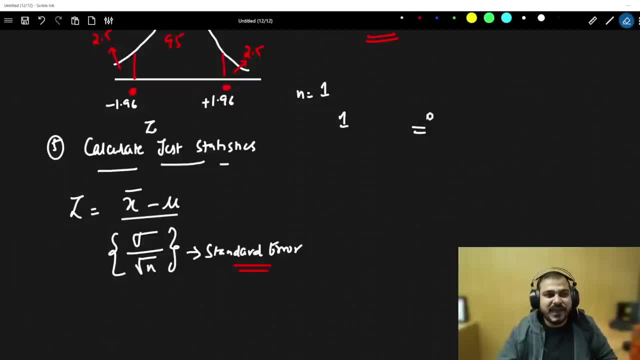 you. There is a topic which is called a central limit theorem. I will discuss that and then probably I will teach you this particular topic. But just right now understand that to make our standard error become very less, because here we are working with sample data. 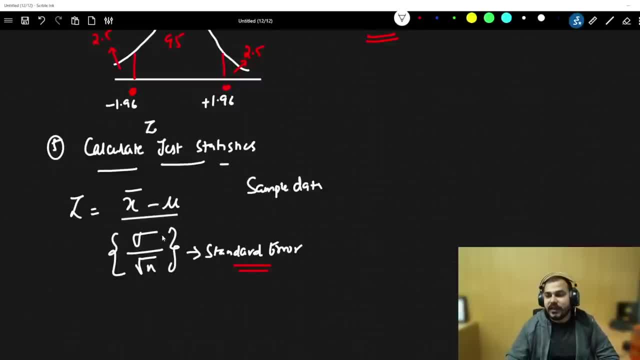 If we are working with population data directly, we can write standard deviation like this. But since we are working with sample data, we have some kind of standard error. And by dividing it by root, n, as the sample size keeps on increasing our values, our mean. 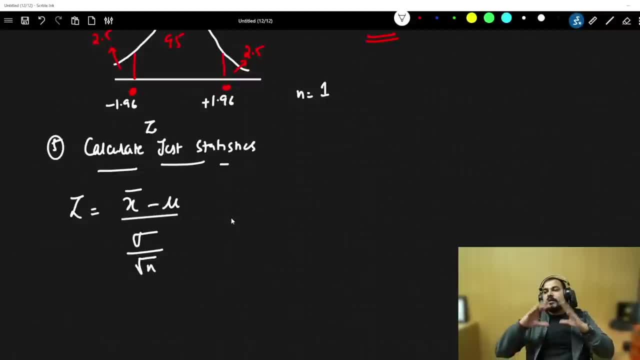 It will be 1. Right, But when we are working with a huge sample- Right, When we are working with a huge sample- We have to basically use root N And this is called as standard error. Standard error, Like how we divide something by. 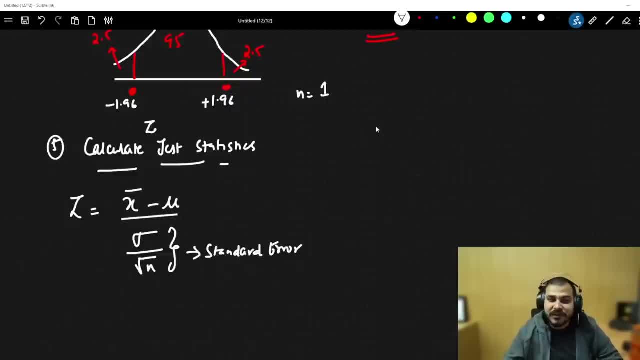 You know, N minus 1.. There is some reasons why we do it. Okay, And probably I do not know whether you have seen my video or not. Okay, So this is basically called as standard error. So we have to divide by root: N. 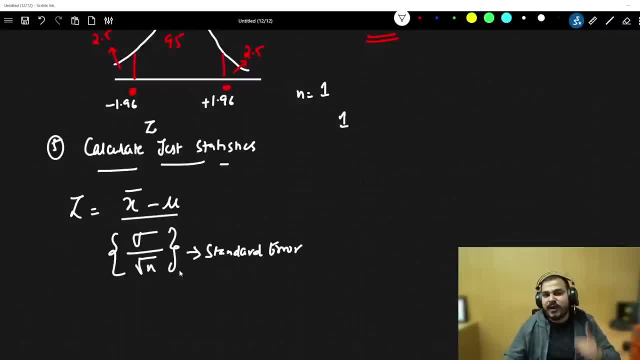 Always understand. For one sample, This root N will already be 1.. So we have to use this particular formula. Okay, To do this. Okay, So this is basically my standard error formula, Which is specified by this, And always remember. 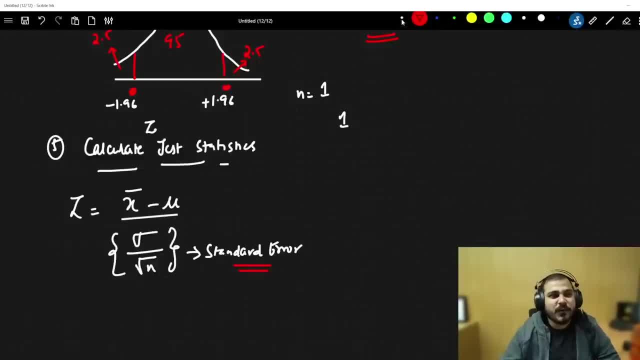 Because why do we use this? I will just give you one example. Suppose I take 5 samples. Right, I take 5 samples, 5 different, different samples from a population, 5, 5, 5 samples from different, different. 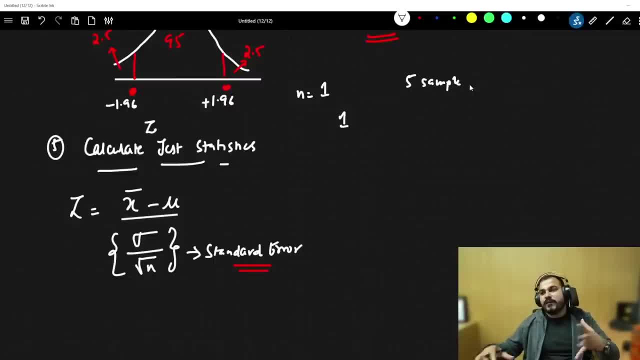 Let us, Let us say that I have a population of 1000 points. Okay, So I take 5 samples, 5 different, different samples from a population: 5, 5, 5 samples from different, different. Let us say that I have a population of 1000 points. 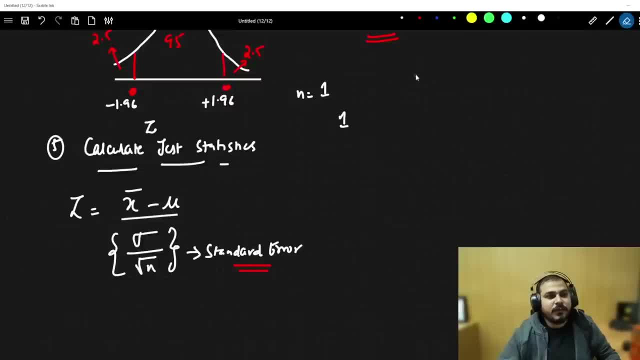 Okay, Let us say that I have a population of 1000 points. 1000 points. Let us consider that I am considering a sample of 100 points. Every time I come, I take. Otherwise, Just wait for it, guys. 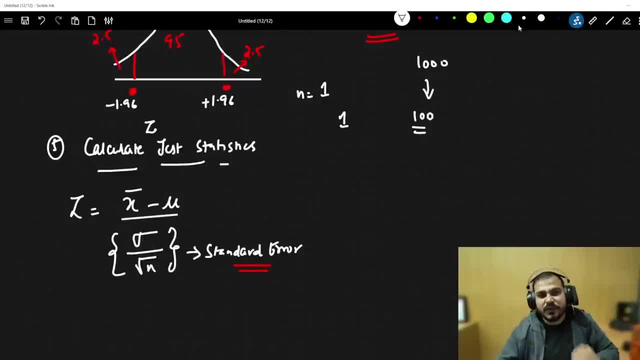 I will teach you. There is a topic Which is called a Central Limit Theorem. I will discuss that And then, Probably, I will teach you this particular topic. But Just right now Understand that To make our standard error become very less, 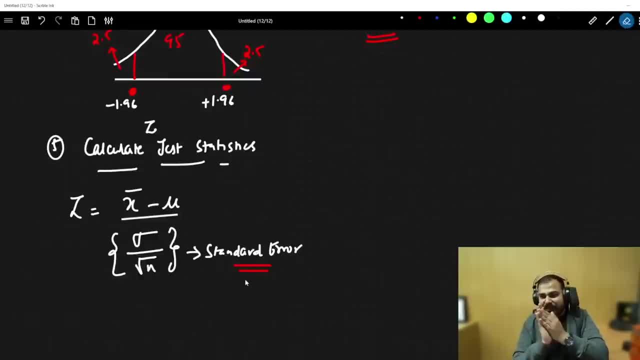 Because Here We are working with sample data. If You are working with population data, Then We take the standard error From 0 to 100. And directly we can write standard deviation like this. But since we are working with sample data, 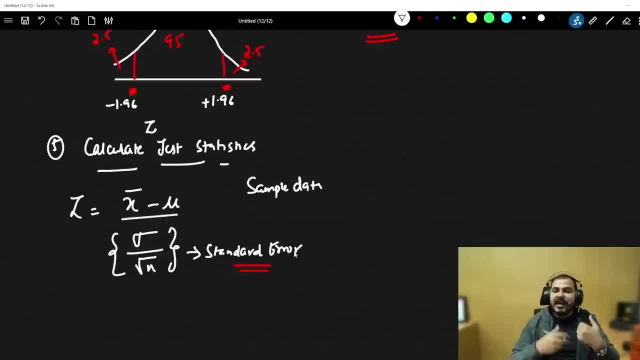 we have some kind of standard error and by dividing it by root n, as the sample size keeps on increasing, our values, our mean values, will be matching with the population. So don't worry, just give some time and I will explain you this. For right now, just consider that it is standard. 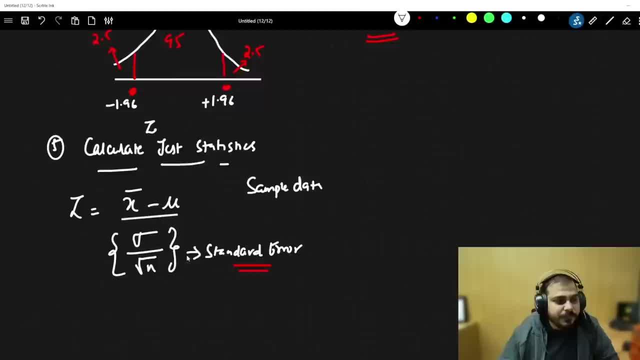 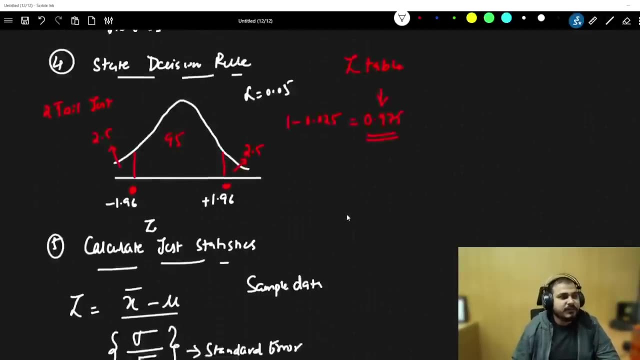 values will be matching with the population. So do not worry, Just give some time and- And I will explain you this For right now, just consider that it is standard deviation divided by root n, If I go ahead and calculate this particular thing. so what is my x bar? 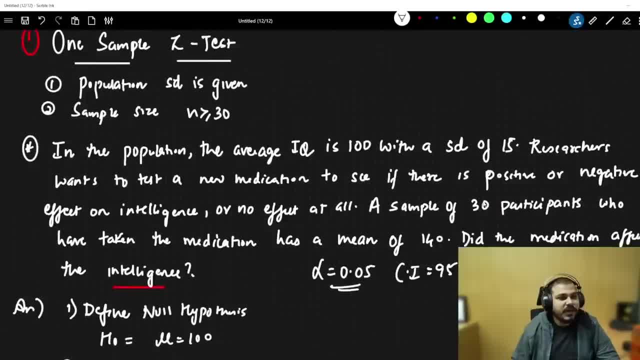 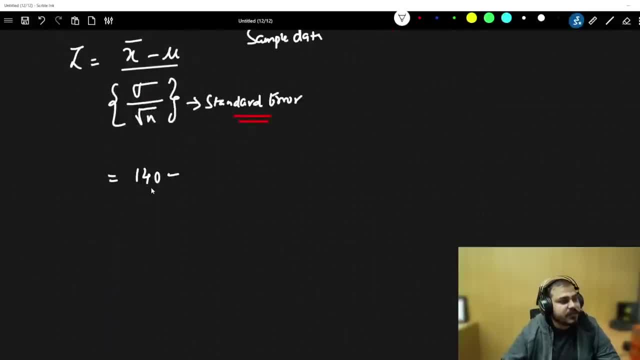 My x bar is obviously what. Let's see what is my mean. a sample of 30 participation is nothing but 140, okay, So 140 minus what is the population mean IQ? the average IQ is 100.. So here I will say 100.. 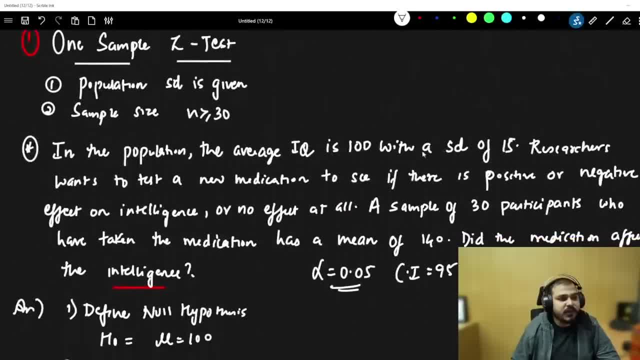 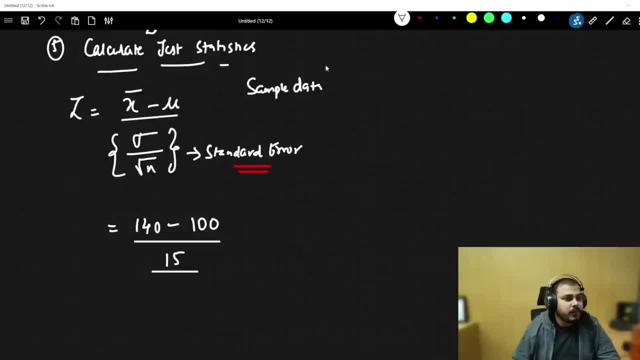 Divided by what is standard deviation? population standard deviation with a standard deviation of 15.. So here I have 15.. Divided by root n: what is n? What is the sample that we have taken, 30. So here it will be root of 30.. 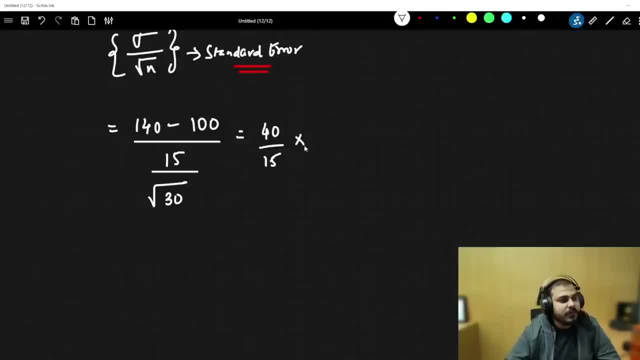 So this will basically be 40 divided by 15, multiplied by root, 30.. I hope I am right. It is 14.3.. Okay, 14.60.. Finally, we state our decision. Now, this is a very important step because from this particular step, I will be able. 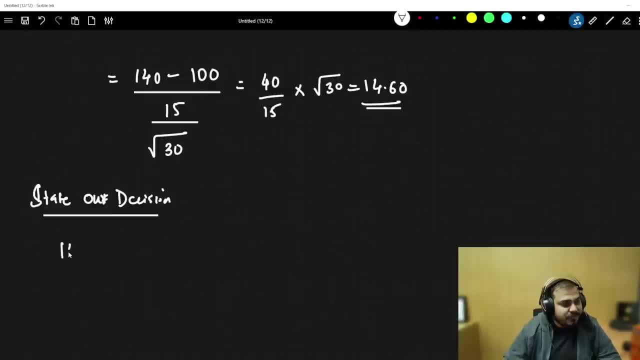 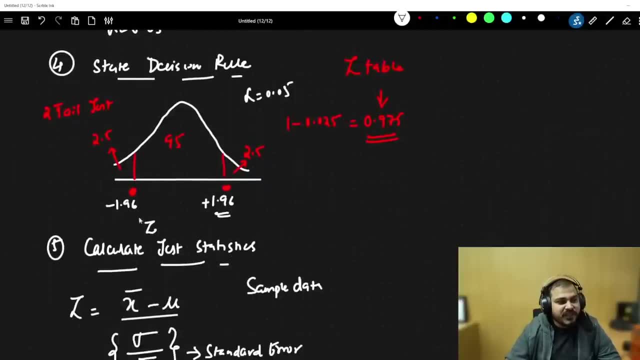 to understand something I got from my Z test, 14.60.. Now let's go and see our decision rule. What did our decision rule basically say? It should be between minus 1.96 to plus 1.96.. Is this greater than 1.96 or not? 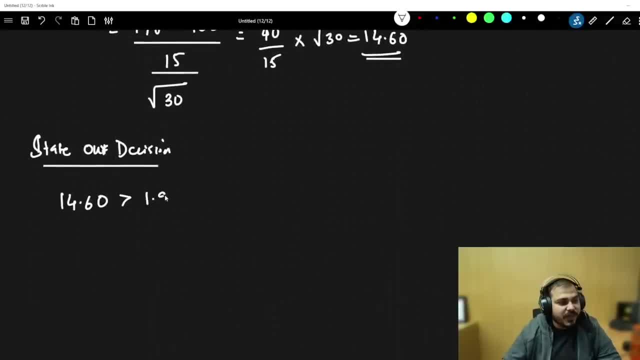 So 14.96 over here, 14.60 is greater than 1.96.. Which is obviously that my condition will be that if Z is less than minus 1.96 or greater than 1.96, then what we have to do 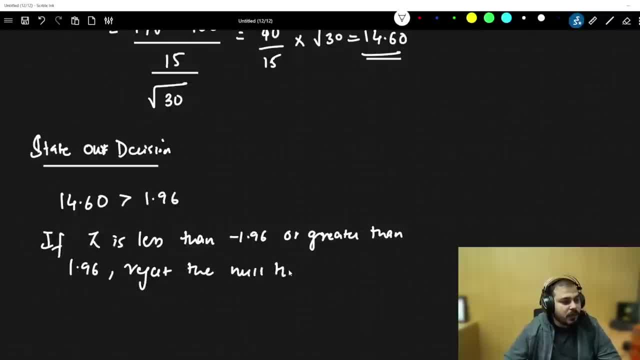 We have to just reject the null hypo-ASS because my Z value over here is 14.60.. But we are going to have to do something. We are going to have to reject the null hypo-ASS. Let's take out one amazing thing from this. 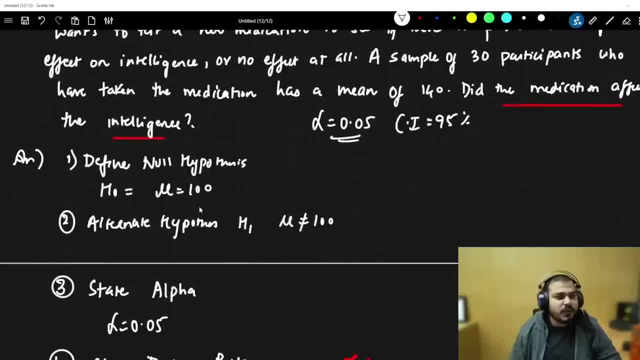 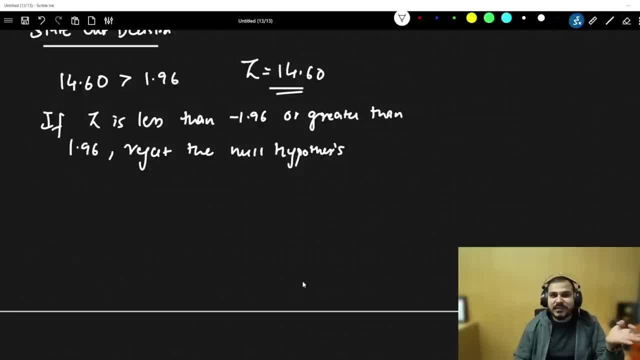 So when I reject my null hypothesis, that basically means my mean is not equal to 100, right, I'm accepting this. Now tell me one very important question: Does this medication improve the intelligence or did it decrease the intelligence? My next question is that: did the medication improve the intelligence or decrease? 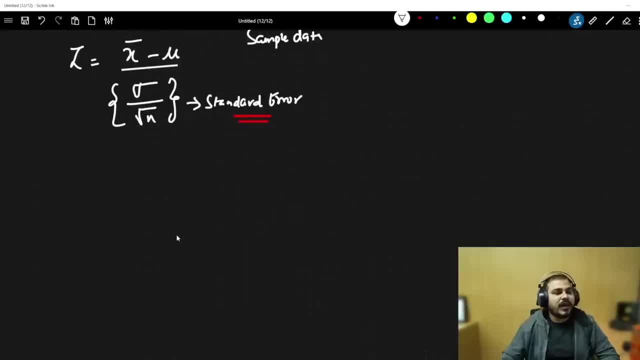 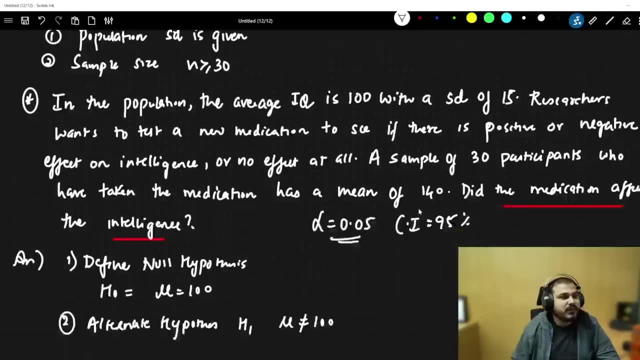 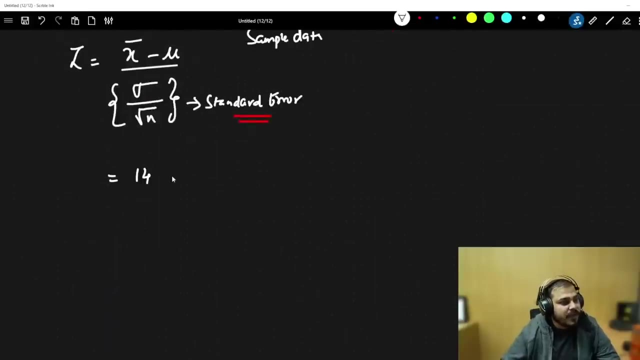 deviation divided by root n, If I go ahead and calculate this particular thing. so what is my x bar? My x bar is obviously what. Let's see what is my mean. A sample of 30 participation is nothing but 140.. Okay, so 140 minus what is the population mean IQ? the average IQ is 100. So here I will say: 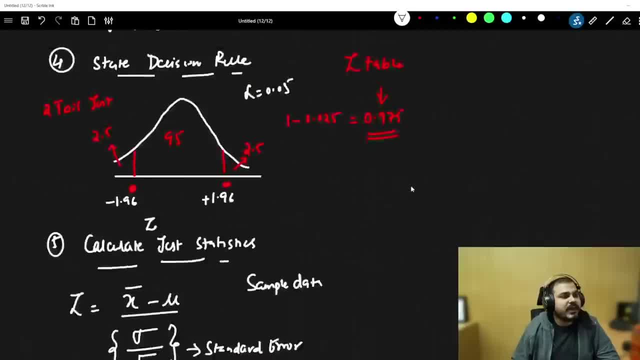 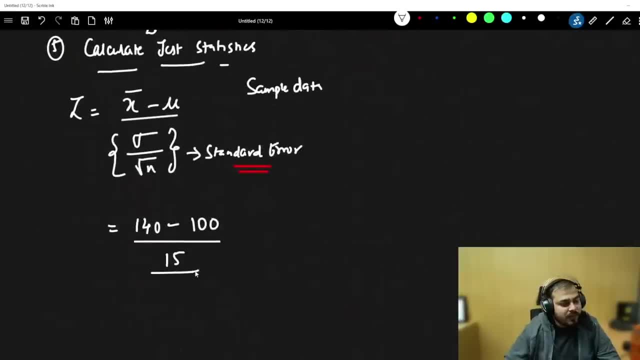 100 divided by what is standard deviation, Population standard deviation, with a standard deviation of 15.. So here I have 15. Divided by root n, what is n? What is the sample that we have taken? 30. So here it will be root of 30. So this: 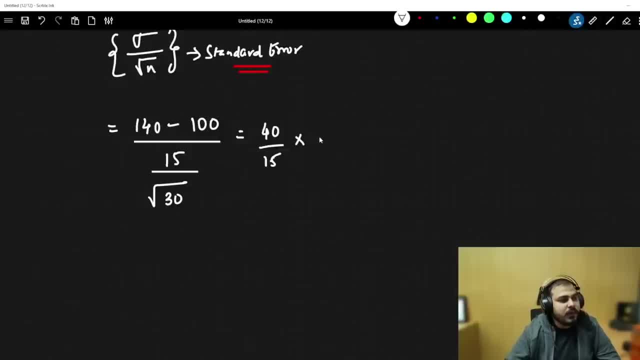 will basically be 40 divided by 15, multiplied by root, 30.. I hope I am right. It is 14.60.. Finally, we state our decision. Now. this is a very important step because from this particular step, I will be able to understand something I got from my z test. 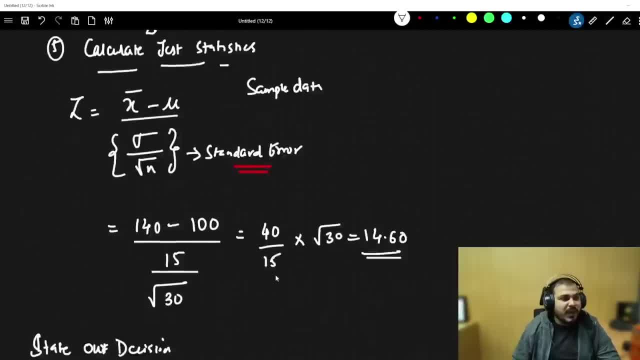 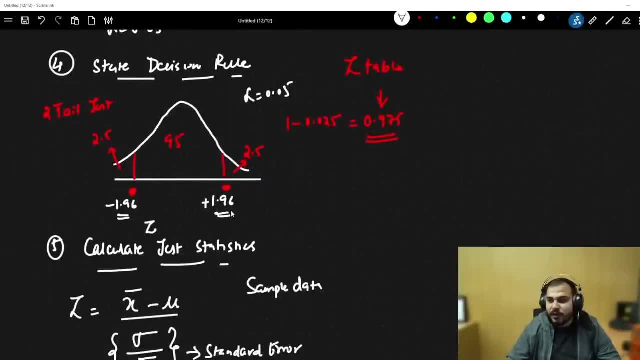 14.60.. Now let's go and see our decision rule. What did our decision rule basically say? It should be between minus 1.96 to plus 1.96.. Is this greater than 1.96 or not? So 14.96 over here. 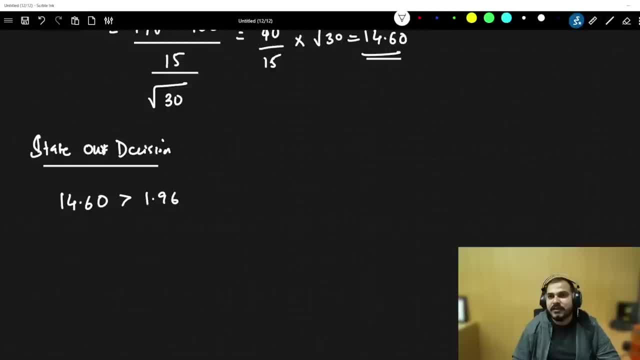 14.60 is greater than 1.96, which is obviously that my condition will be that if its less than 1.96.. So if z is less than minus 1.96 or greater than 1.96, then what we have to do, We have to just reject the null hypothesis, Because 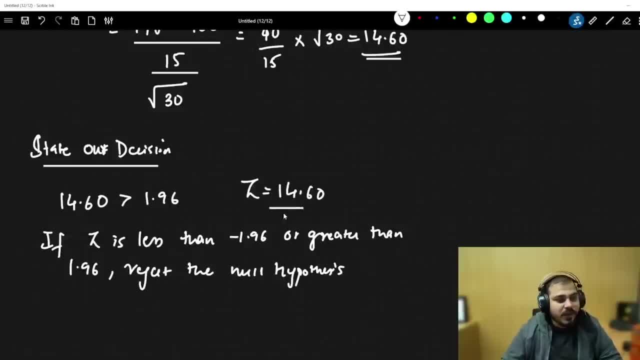 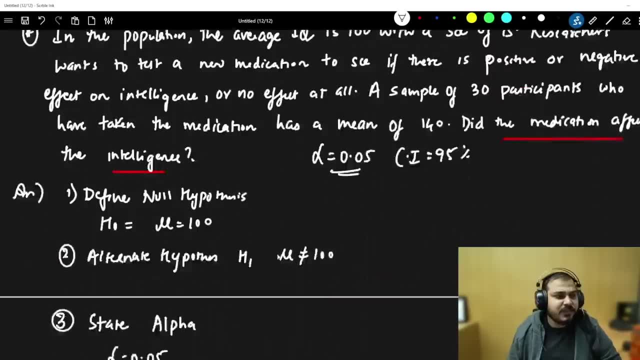 my z value over here is 14.60,. but let's take out one amazing thing from this. Now, let's take one amazing thing from this. So when I reject my null hypothesis, that means basically mean my mean is not equal to 100. right, i'm accepting this. now tell me one very important. 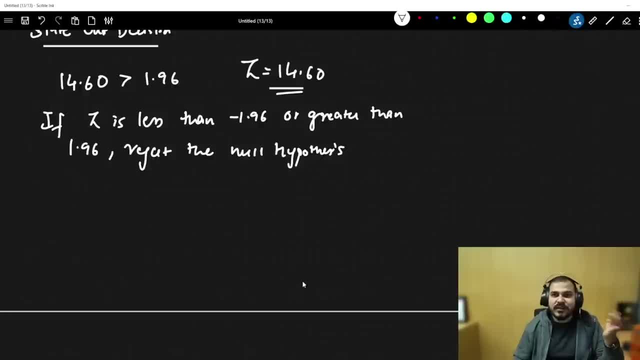 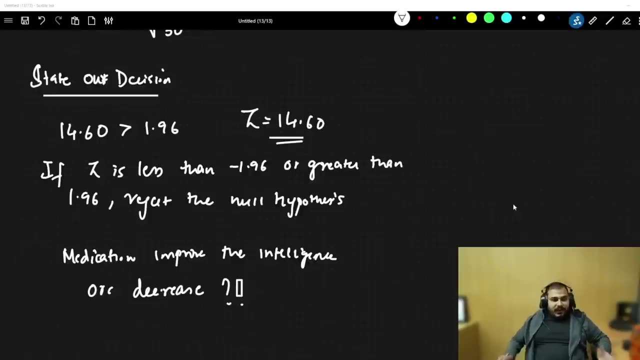 question this: this medication improve the intelligence or did it decrease the intelligence? my next question is that: did the medication improve the intelligence or decrease? now this you have to answer me after solving this much. obviously it is improved. improved, guys. improved the intelligence, not decreased. improved the intelligence. very simple. if i was getting the 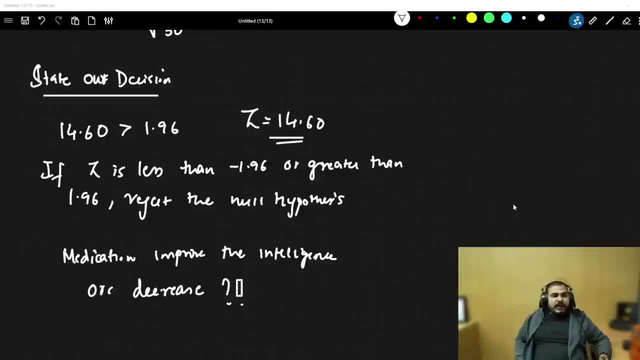 Now this you have to answer me after solving this much. Obviously, it is improved. Improved guys. improved the intelligence, not decreased. improved the intelligence. Very simple, If I was getting the Z value as minus 0.2, that time what was happening? 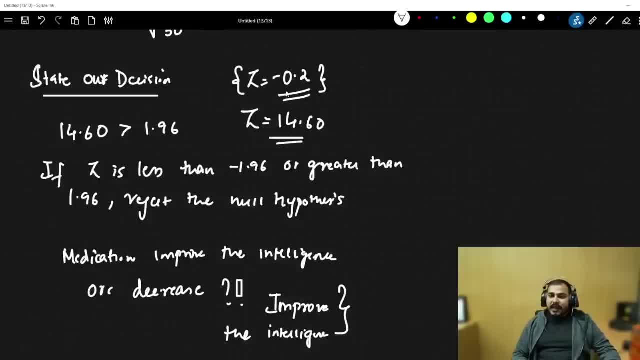 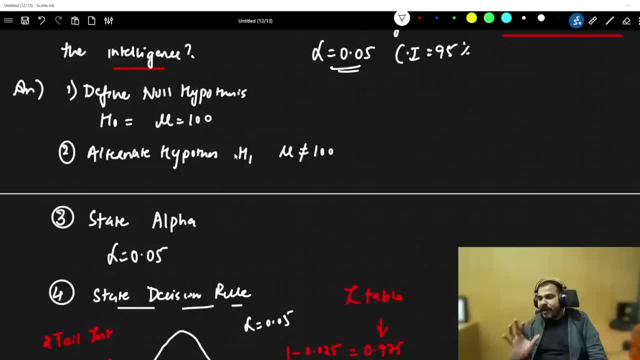 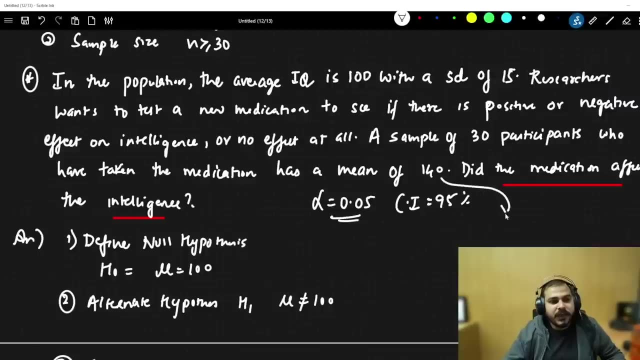 Then what would happen? It would have decreased the intelligence. It has increased the intelligence. Rejecting the null hypothesis is saying that the medicine had an impact. Now do the same problem. I will just change one value over here. This mean will be 110.. 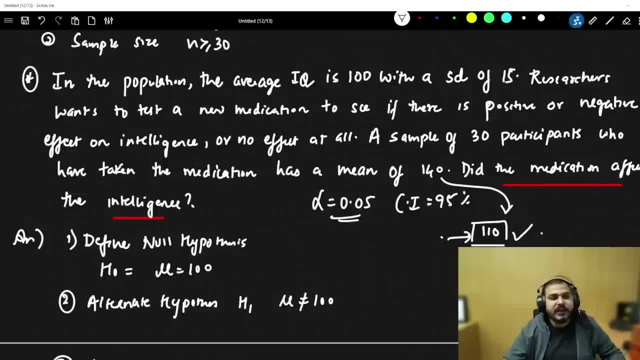 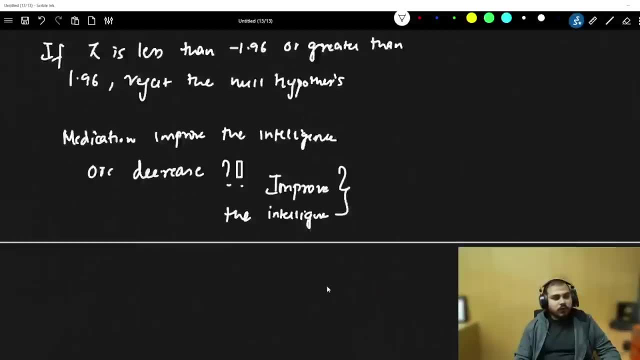 This mean of this, 30 participants will be 110.. Try to solve the problem and tell me whether the null hypothesis is accepted or the alternate hypothesis, Whether the null hypothesis is accepted or rejected. Okay, So do this from your side. So do the problem statement. 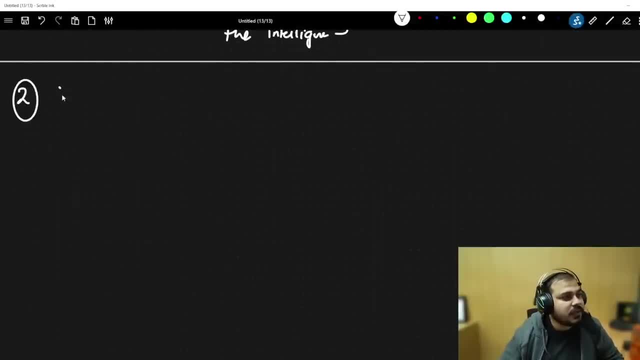 So we will start our second test, which is called as one sample t-test. Now I hope You like the session. So, guys, see, I like to teach in this particular way. you know, like write everything. I never prepare PPTs. probably you have seen my YouTube videos. 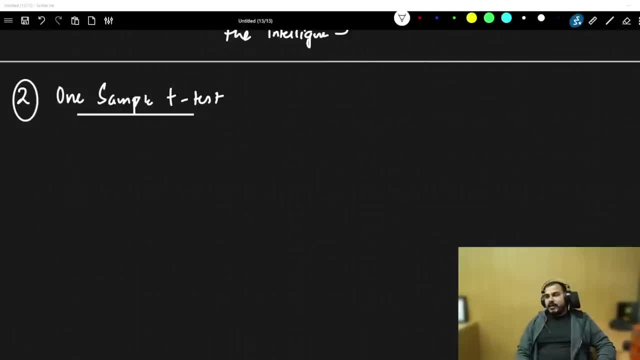 Hardly I prepare any kind of PPTs, you know. I write it like this. The reason I write it like this? because it also helps me to practice. It also helps me to see that what mistakes I'm probably making, I'll become perfect in this. 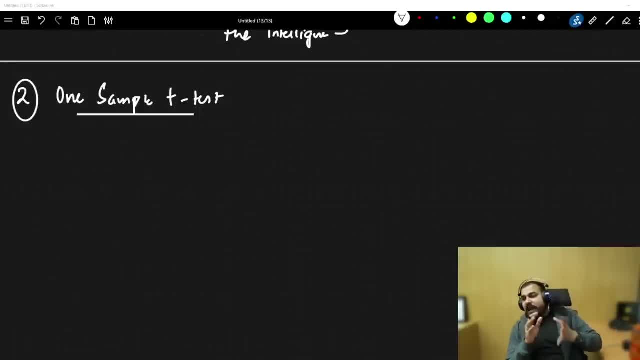 So tomorrow, if you call me in any session, Krish probably teach statistics or machine learning. You know, I will just go and start explaining everything over here. Now let's go towards the next problem. Second problem statement, which is called as. which is called as one sample t-test. 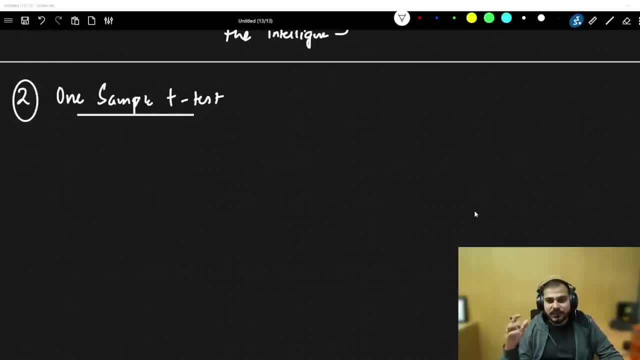 Now I hope you understood what is t-test right. First of all, let me say Z test. Whenever you have population standard deviation, you use this right. You really need to remember this If you don't have population standard deviation. 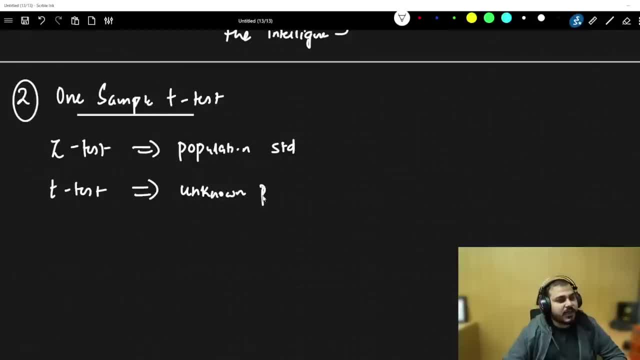 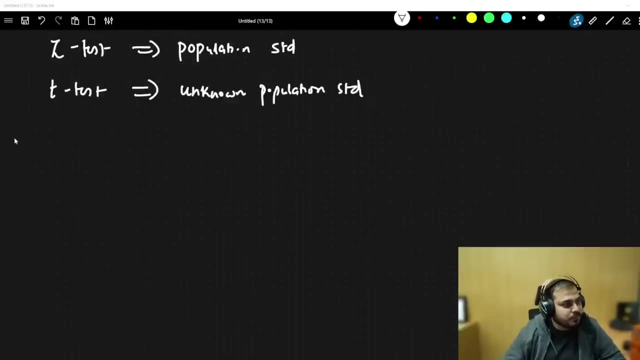 That is an unknown case of population standard deviation. then what do you do? You use t-test, okay? So this is the basic difference between t-test and all. okay, Now I'll take the same problem, okay? So let's solve the same question, okay. 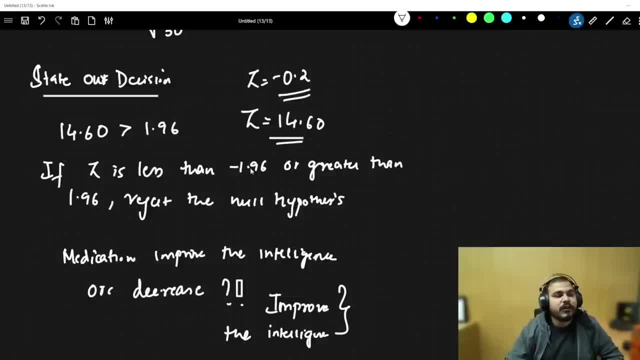 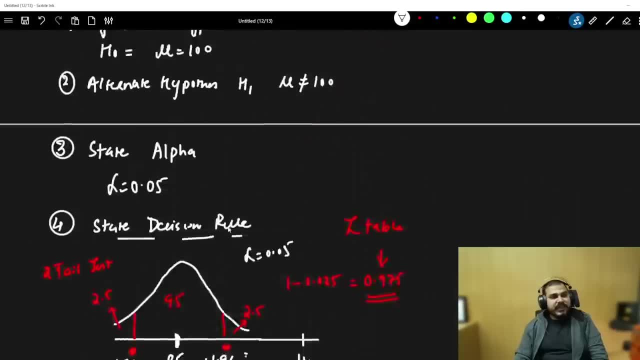 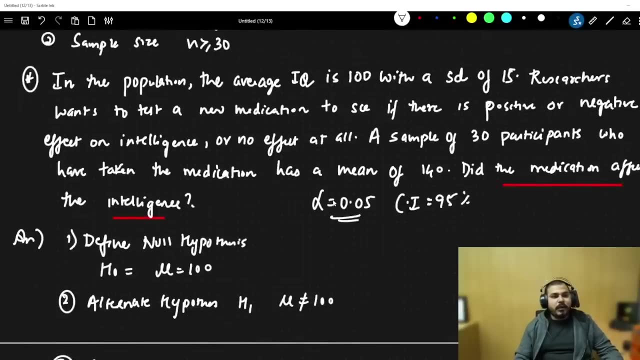 z value as minus 0.2. that time, what was happening then? what would happen? happen? it would have decreased the intelligence. it has increased the intelligence. rejecting the null hypothesis saying is saying that the medical, the medicine had an impact. now do the same problem, i will just change. 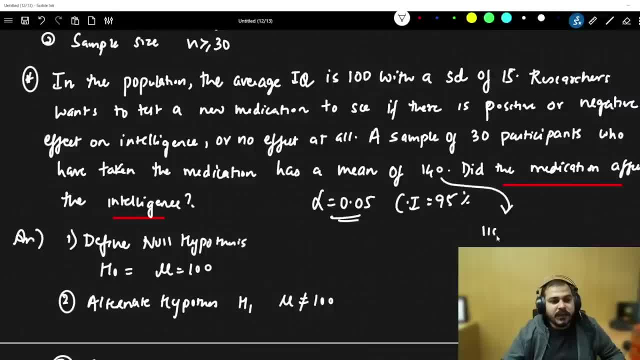 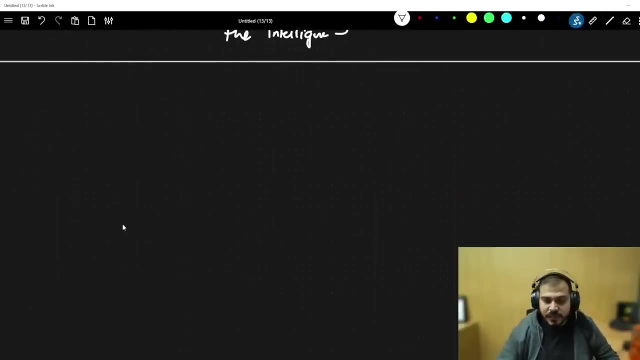 one value over here. this mean will be 110. you- this mean of this, 30 participants will be 110. try to solve the problem and tell me whether the null hypothesis is accepted or the alternate hypothesis, whether the null hypothesis is accepted or rejected. okay, so do this from your side. so do the problem statement. so we will start. 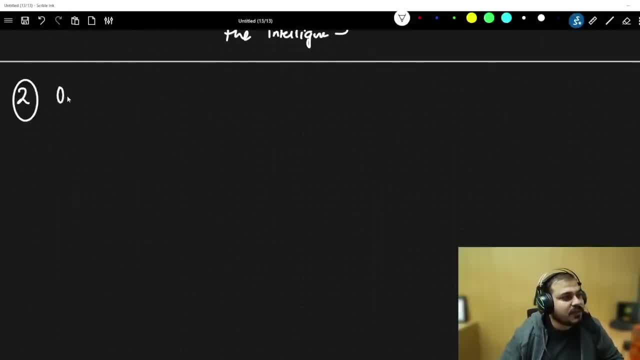 our second test, which is called as one sample t test. now i hope you like the session. so, guys see how was the video. it helped you. i am happy that you are enjoying this video. so if you have liked it, share the video. so please considering by liking and sharing it. that would be great. 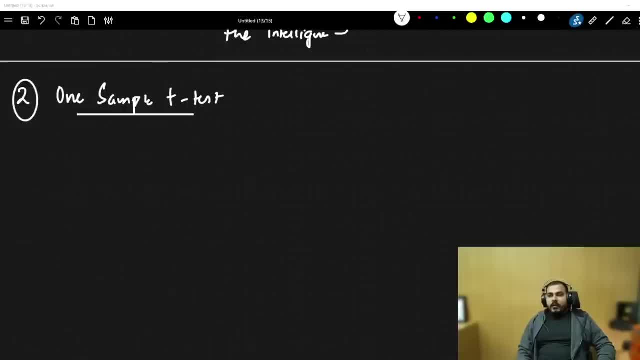 i will try to answer more positive questions in future pilot videos. I like to teach in this particular way. right, you know like write everything. i never prepare ppts. probably you have seen my youtube videos. hardly i prepare any kind of ppts, you know, i write it like. 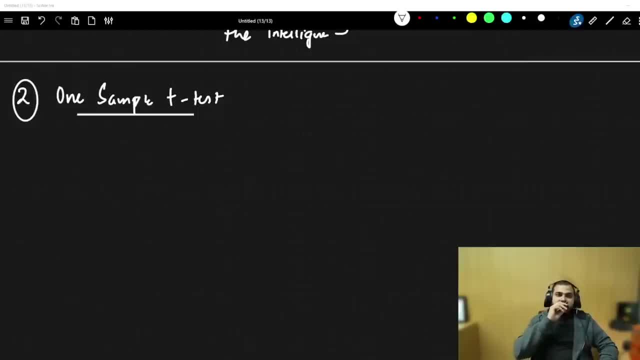 this the reason i write it like this, because it also helps me to practice. it also helps me to see that what mistakes i am probably making, i will become perfect in this. so tomorrow, if you call me in any session, Krishh probably teach statistics or machine learning, you know. 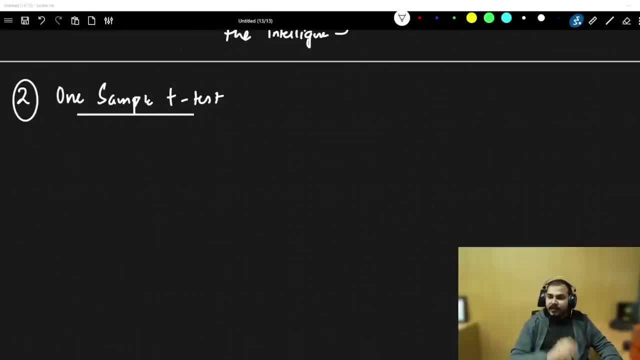 i will just go and start the метhod thoroughly and you will find will honest answer your questions. I will just go and start explaining everything over here. now let's go towards the next problem, second problem statement, which is called as, which is called as one sample t test. now I hope you. 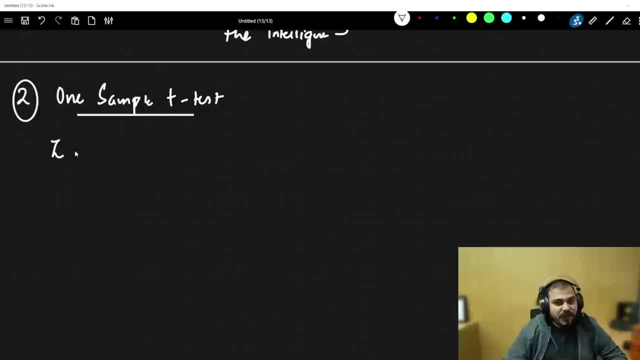 understood. what is t test right? first of all, let me say z test. whenever you have population standard deviation, you use this right. you really need to remember this. if you don't have population standard deviation- that is, in unknown case of population standard deviation- then what you do? 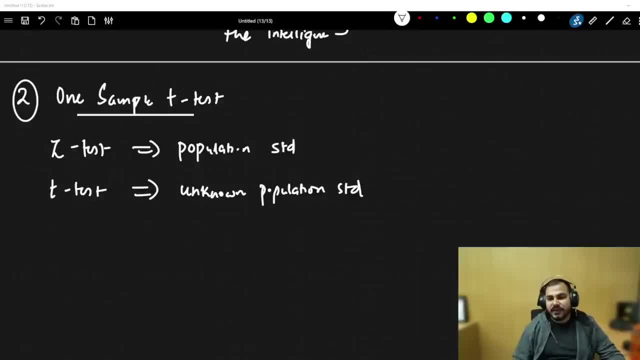 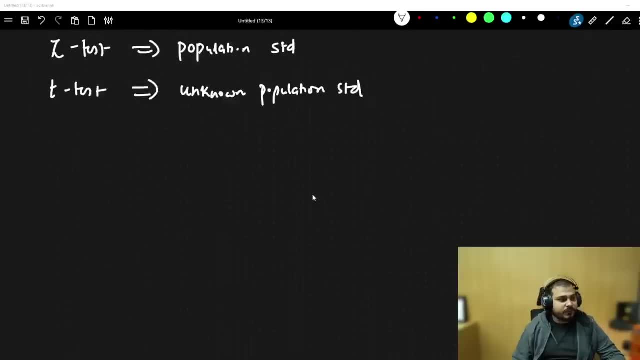 you use t test, okay. so this is the basic difference between t test and all. okay, now I'll take the same problem, okay, so let's solve the same question, okay. first of all, in a population the average IQ is equal to 100. then a team of researchers: 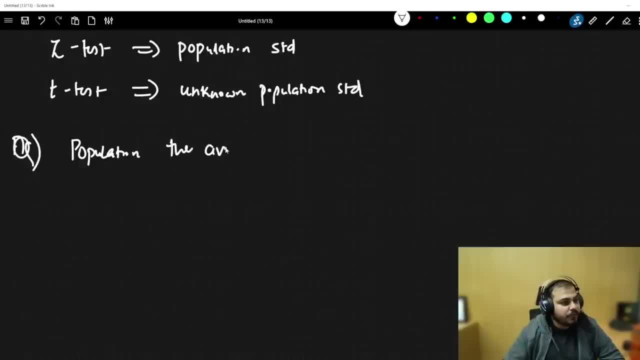 First of all, in a population, the average IQ is equal to 100.. Then a team of researchers Tried a medication to see whether there is a positive or negative effect. A sample of 30 participants were taken And they have a mean of mean of mean IQ of 140, with a sample standard deviation of 20.. 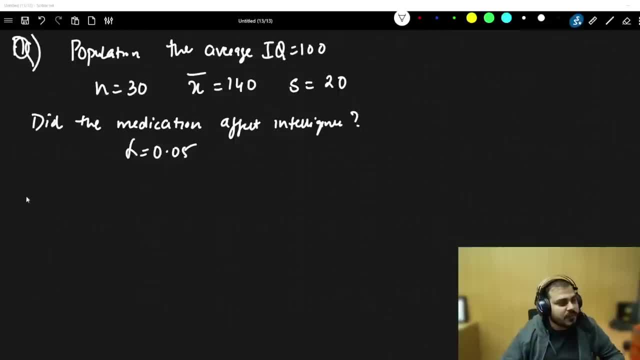 So did the medication affect the intelligence? The first thing, first answer. What is your null hypothesis? Your mean is equal to 100.. What is your H1?? Mean is not equal to 100.. The second step, the first step. the second step is done. 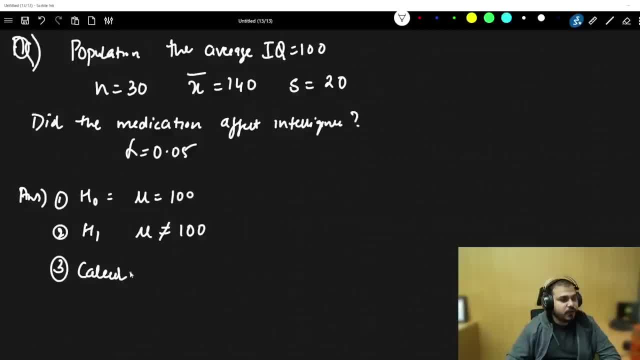 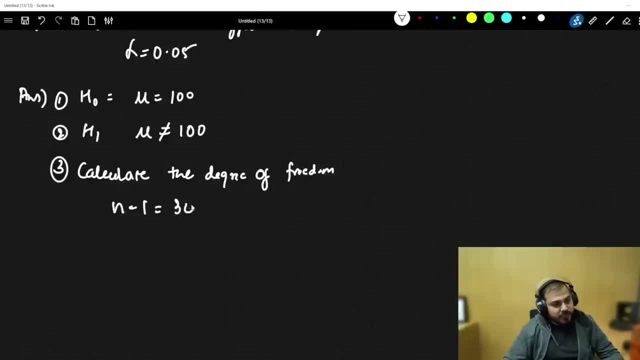 Now the third step that we do in t-test, which I have discussed before, also Calculate the degree of freedom. Here I basically use n minus 1.. So this will be 30 minus 1, which is nothing but 29.. 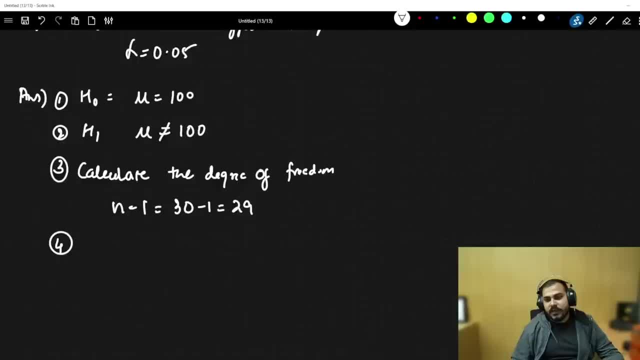 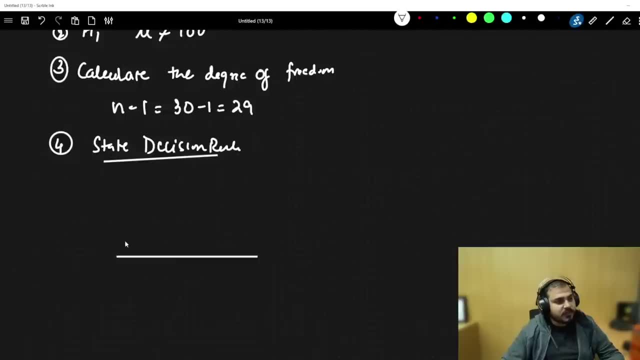 Fourth step. What is my fourth step? I will go ahead with the decision rule. Now, my decision rule is nothing, but It's very, very simple. I will go and define this graph. I know what is my alpha value: 0.05.. 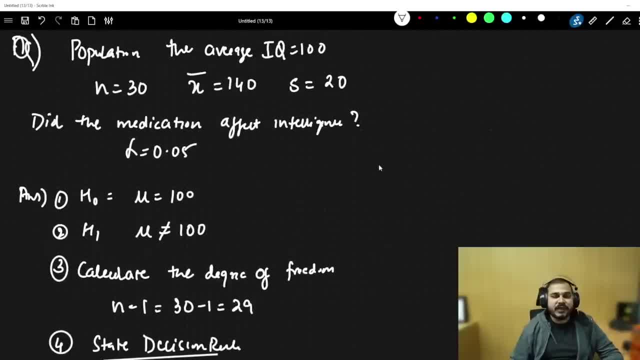 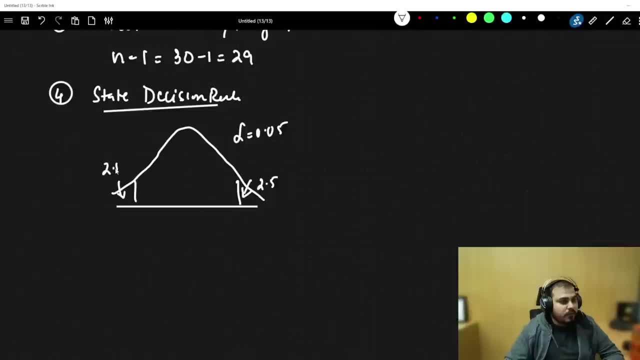 I know my question. Did the medication affect the intelligence? It can either increase or decrease, So it will become a two tailed test. So here you have 2.5.. Here you have 2.5.. Here is your 95.. 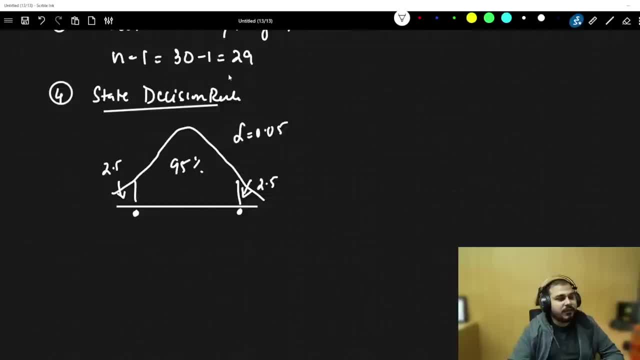 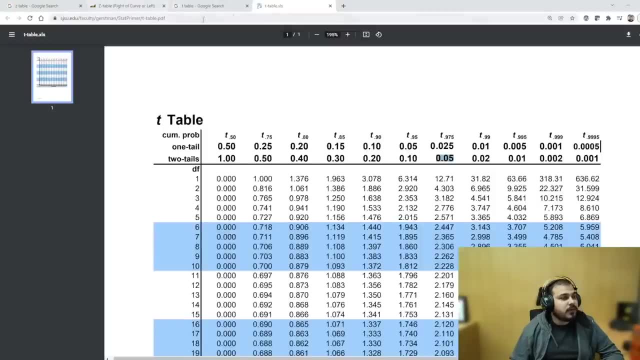 What is this value? We have probably found it out with degree of freedom 29.. So let's go and try to find out with degree of freedom 29.. What will be the value? So it is t-tailed. This is the variable degree of freedom 29.. 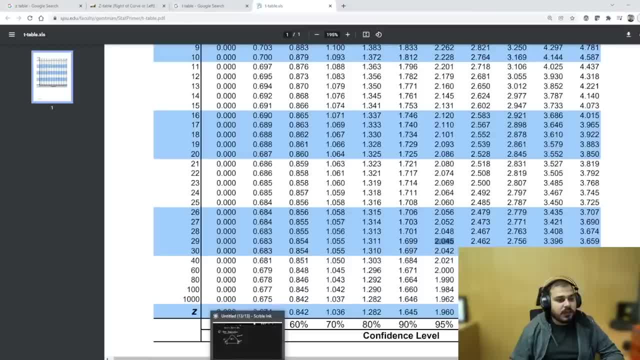 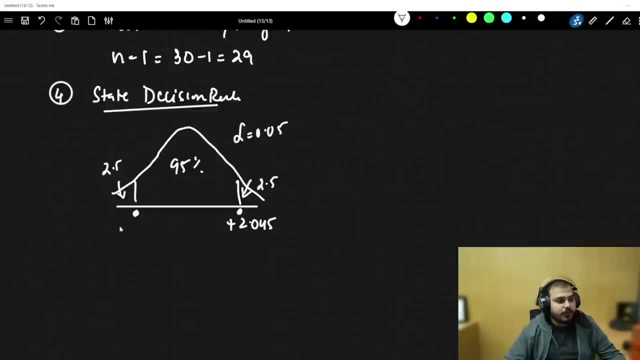 So 2.045,, so 2.045.. So here you will be able to see plus 2.0,. what was that? 2.045, sorry, and minus 2.045, right. So this is your decision rule. 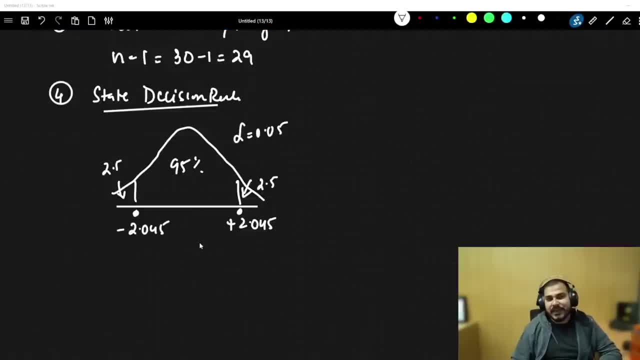 Now your t value that you should be getting should be between this: If it is greater or lesser than this, you reject the null hypothesis, So you have to probably do. Finally, we go to the test statistics formula of t-test. The formula will be almost same. 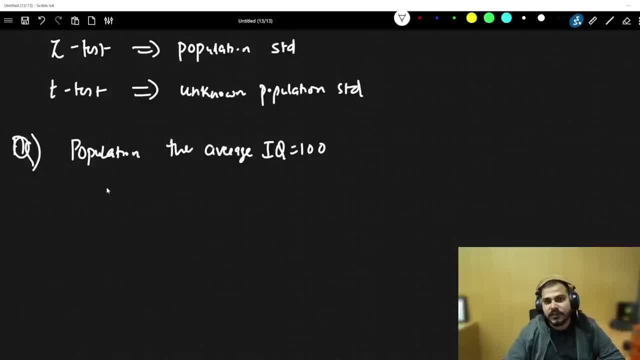 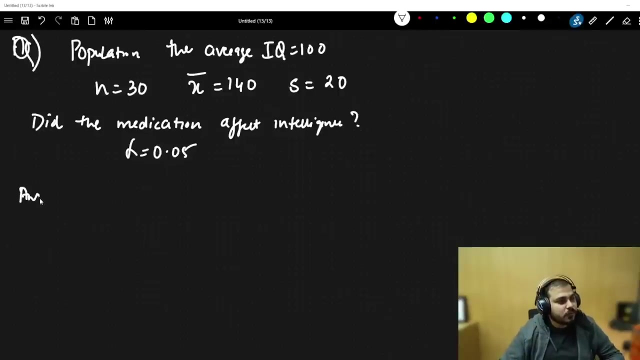 tried a medication to see whether there is a positive or negative effect. a sample of 30 participants were taken and they have a mean of mean of mean IQ of 140, with a sample standard deviation of 20. so did the medication affect the intelligence? the first thing, first answer. what is? 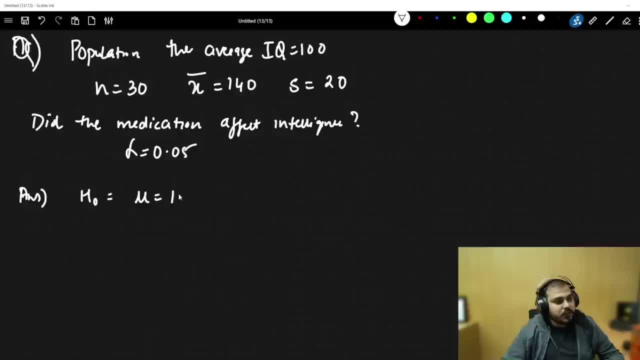 your null hypothesis, your mean is equal to 100. what is your h1 mean is not equal to hundred. the second step: with the first step, the second step is done. now the third step that we do in t test, which I have discussed before: also calculate the. 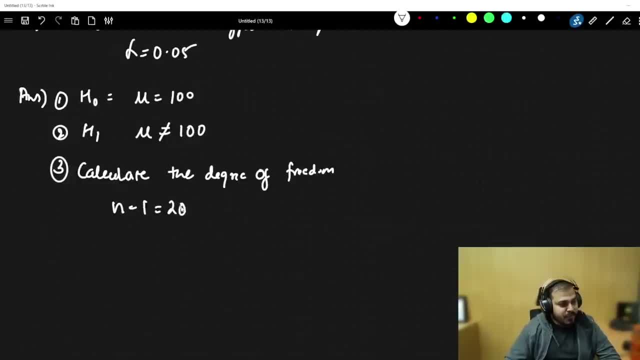 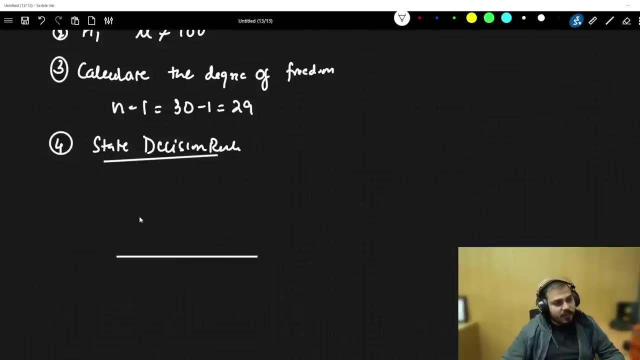 degree of freedom. here I basically use n minus one, so this will be 30 minus 1, which is nothing but 29. fourth step: what is my fourth step? I will go ahead with the decision rule now. my decision rule is nothing but 0.. It's very, very simple. I will go and define this graph. I know what is my alpha value. 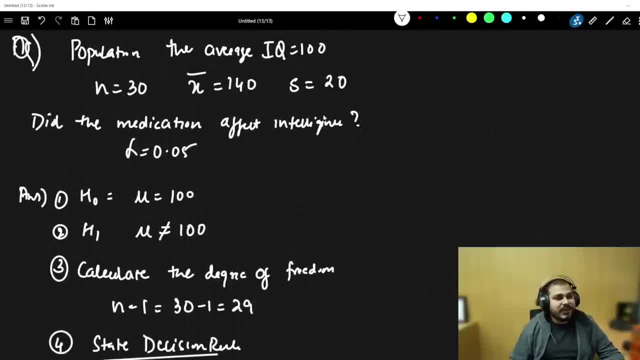 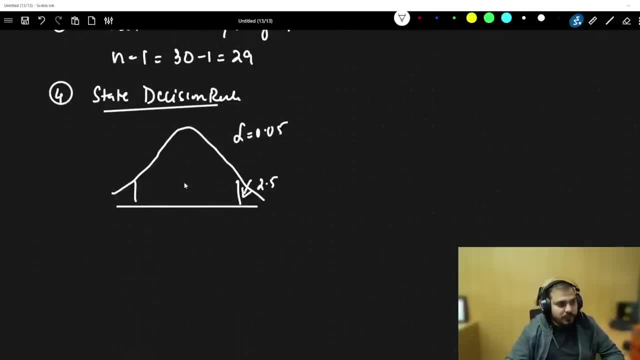 0.05,. I know my question. did the medication affect the intelligence? it can either increase or decrease, so it will become a two tailed test. so here you have 2.5, here you have 2.5, here is your 95.. 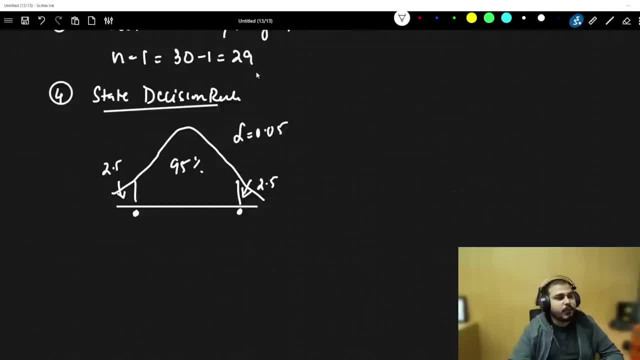 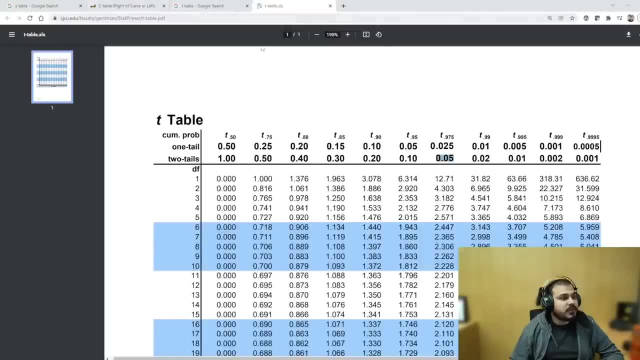 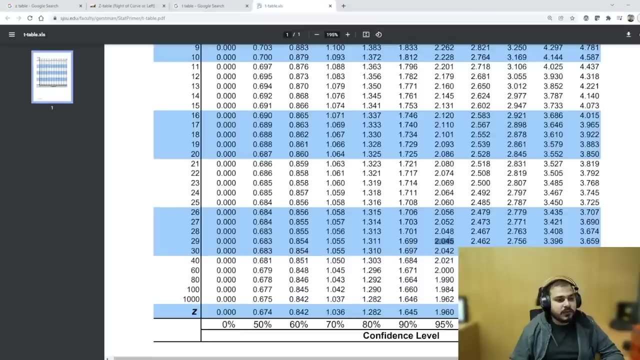 What is this value? We have probably found it out with degree of freedom 29,. so let's go and try to find out with degree of freedom 29,. what will be the value? so it is t table, degree of freedom 29,. so 2.045,, so 2.045, so here you will be able to see plus 2.0,. what was that 2.045,? 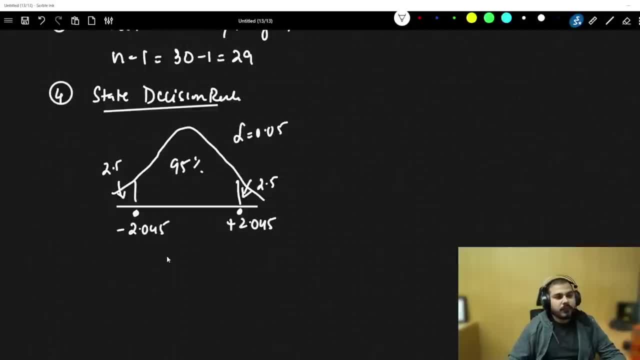 sorry, and minus 2.045, right. so this is your decision rule. Now, your t value that you should be getting should be between this: If it is greater or lesser than this, you reject the null hypothesis. That is what you have to probably do. 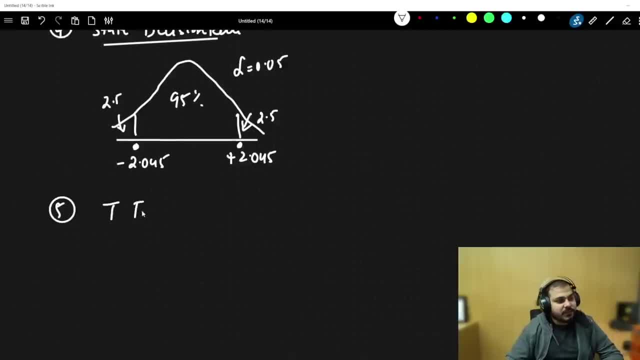 Finally, we go to the test statistics formula of t test. The formula will be almost same. t is equal to x bar minus mu divided by population. standard division is not given, sample is given and this will be root n. So try to compute the values, guys: x bar is nothing but 140, mu is nothing but 100, s. 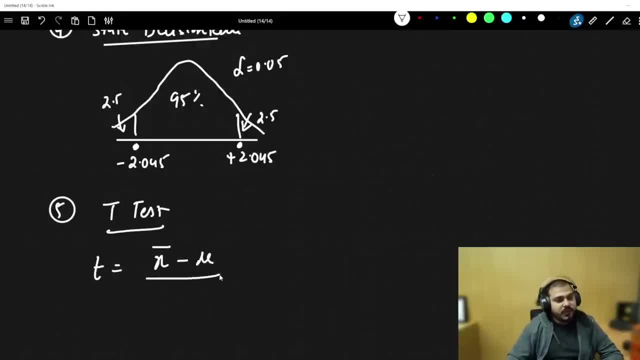 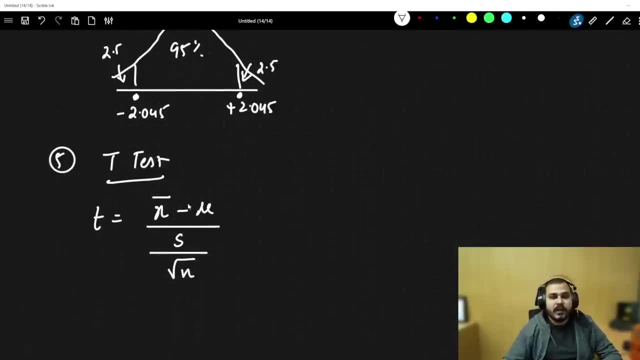 t is equal to x-bar minus mu divided by population. standard division is not given. Sample is given and this will be root n. So try to compute the values, guys. x-bar is nothing but 140.. Mu is nothing but 100.. S is nothing but 20.. 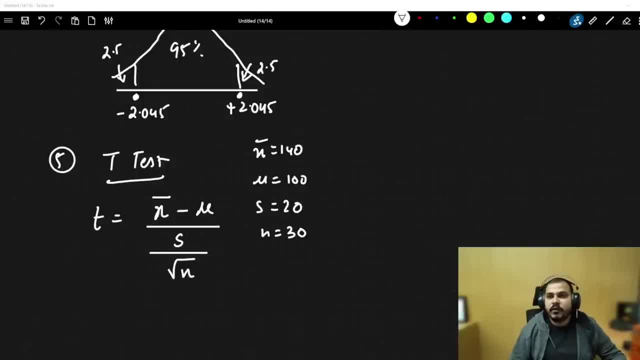 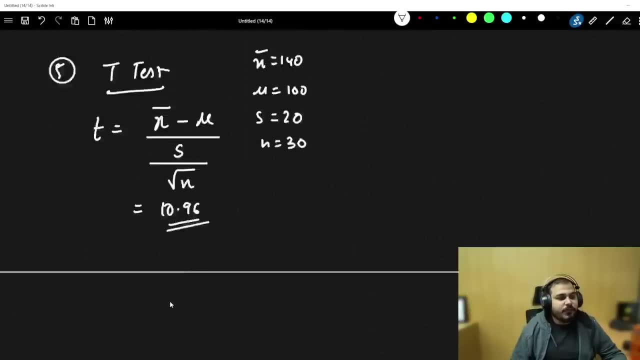 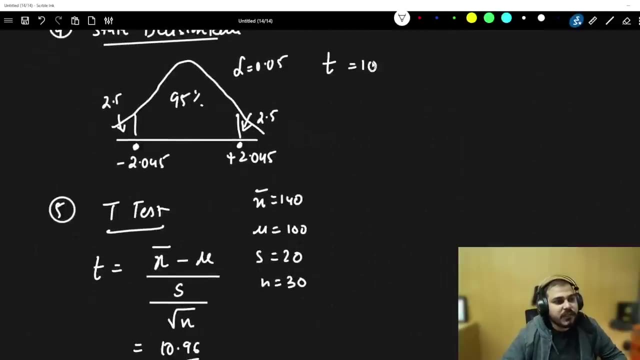 N is nothing but 30. So compute it. If I try to do the calculation entirely, this entire answer will be 10.96.. Now, since we have got 10.96, it is obviously greater than 2.05.. So the t value, which is nothing but 10.96, is greater than 2.05.. 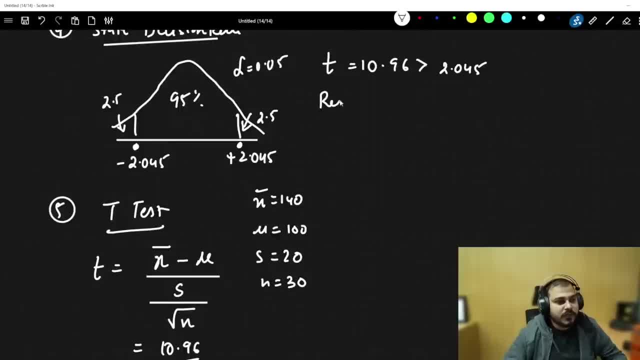 And it is also greater than this particular value. So what we do? We reject null hypothesis. Now, when we reject null hypothesis basically means my p value is less than or equal to the significance value, That is, I am falling in this region or in this region. 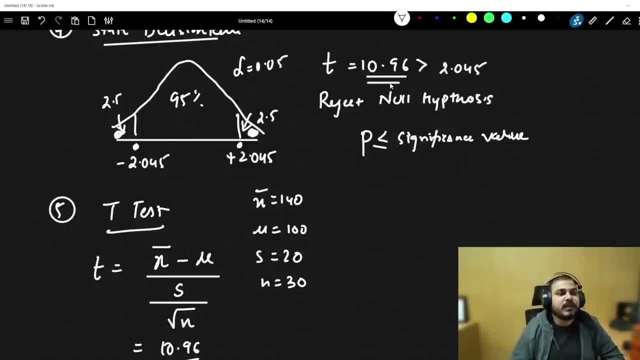 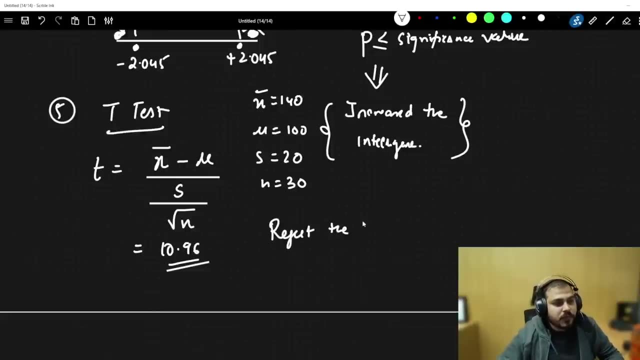 Now, since I am getting 10.96, what do you think? whether my intelligence increased or not, So obviously. final conclusion: you can see that it has increased the intelligence. So what you do? You reject the null hypothesis, Except the null hypothesis. 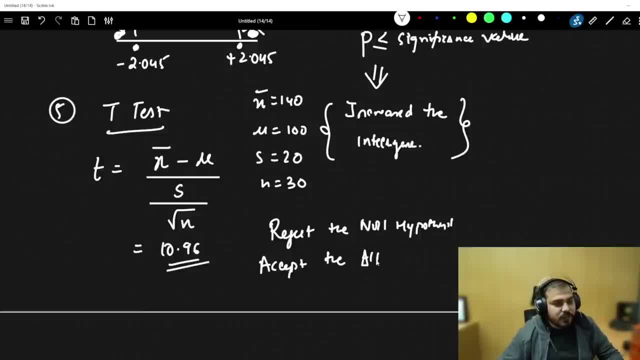 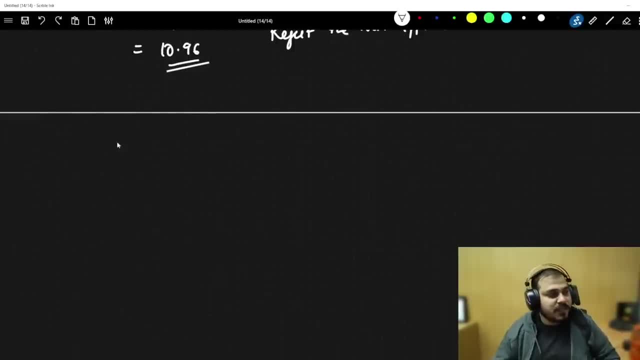 Sorry, reject the null hypothesis except the alternate. So, from my teaching, did your IQ increased or not? Now let's see a real world problem, And probably you can do this from yourself. A bank wants to open an ATM machine in a specific area. 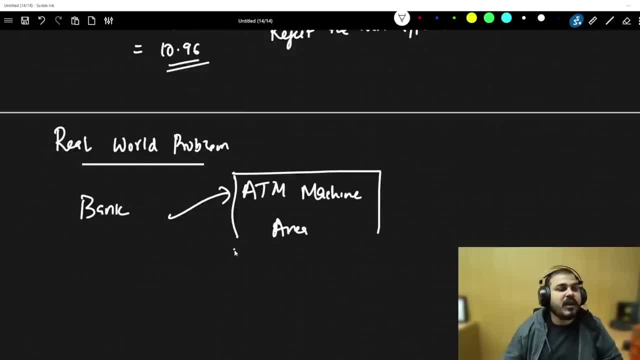 So this problem- you have to solve This problem- you have to formulate, and you have to think over it, How we can apply hypothesis testing. You can consider any values that you want, Like you can say that average money people take out from the ATM machine. 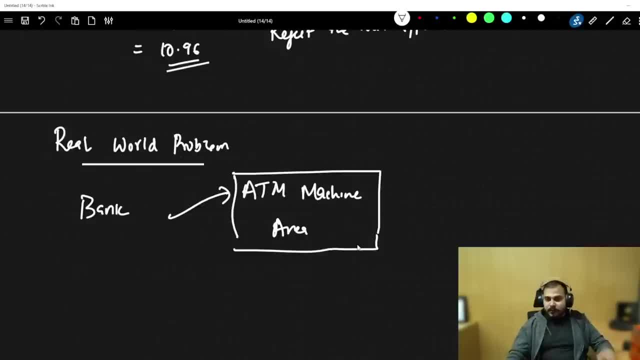 With 95% confidence interval, You can formulate- Because this was one interview question in one bank that is called as standard charted Interview question- from there, Think over it- What all things basically required. Think over it and try to solve it. 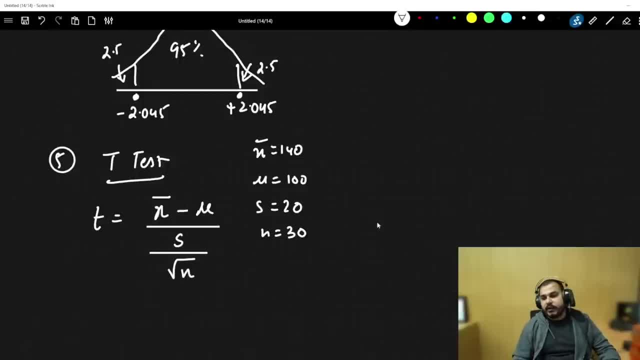 is nothing but 20.. Let's see, n is nothing but 30. So compute it. So, if I try to do the calculation entirely, this entire answer will be 10.96.. Now, since we have got 10.96, it is obviously greater than 2.05.. 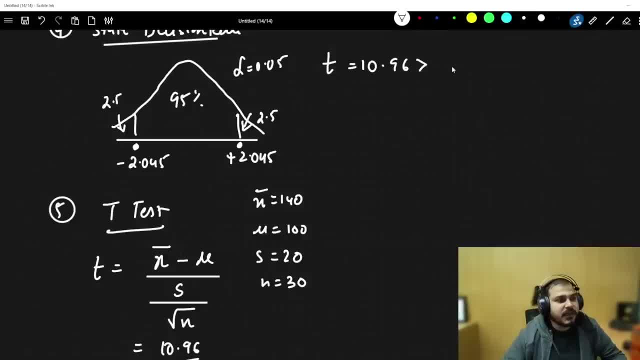 So the t value, which is nothing but 10.96, is greater than 2.05, and it is also greater than this particular value. so what we do? we reject null hypothesis. Now, when we reject null hypothesis, we reject null hypothesis. 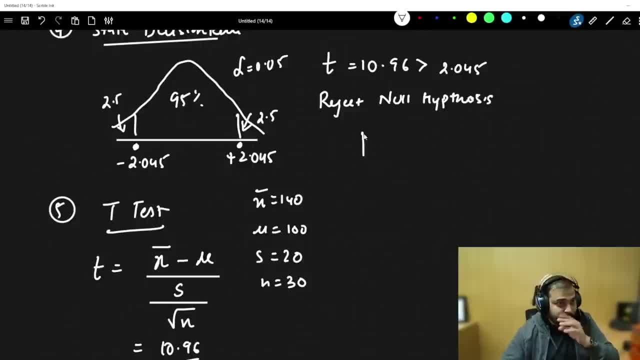 That basically means my p value is less than or equal to the significance value, That is, I am falling in this region or in this region. Now if, since I am getting 10.96,, what do you think? whether my intelligence increased or 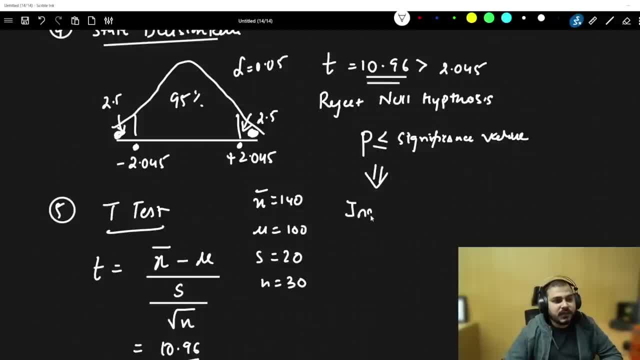 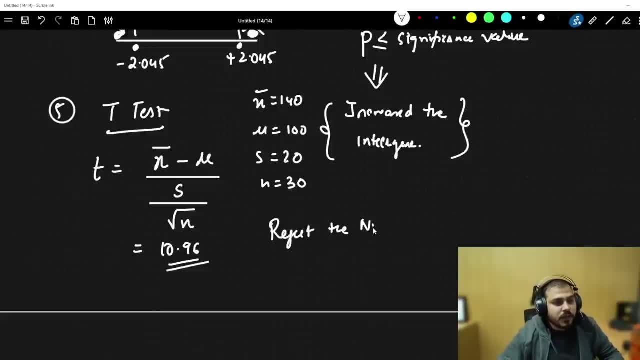 not So obviously. final conclusion: you can see that it has increased the intelligence. So what you do? You reject the null hypothesis. Okay, So you reject the null hypothesis, accept the null hypothesis. sorry, reject the null hypothesis. accept the alternate. 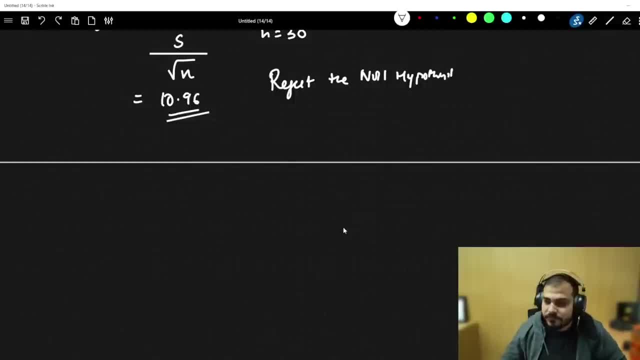 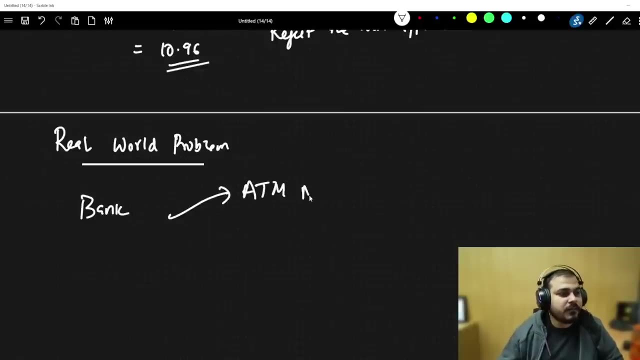 So, from my teaching, did your IQ increased or not? Now let's see a real world problem, And probably you can do this from yourself. A bank wants to open an ATM machine in a specific area, So this problem is not solved. The problem is solved. 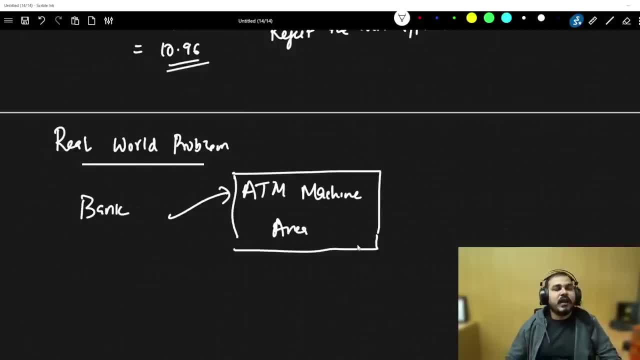 The problem is solved. The problem is solved. You have to formulate, and you have to think over it, how we can apply hypothesis testing. You can consider any values that you want. Like you can say that average money people take out from the ATM machine with 95% confidence. 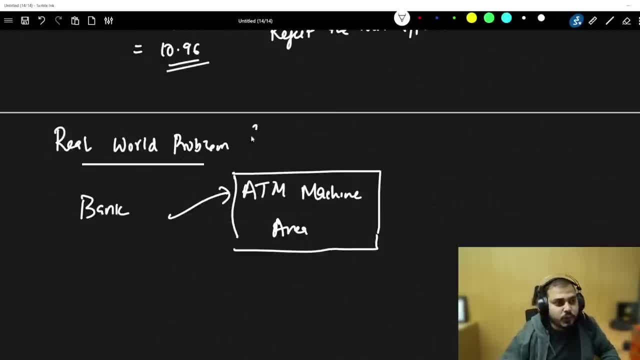 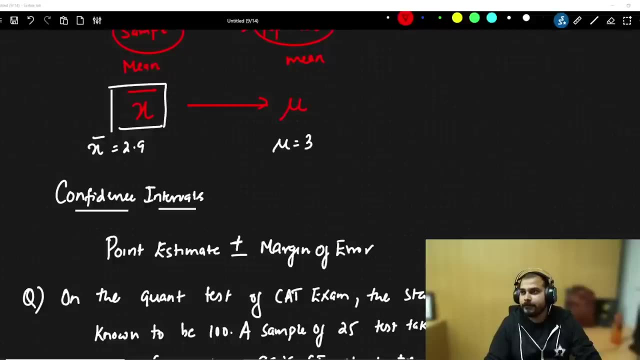 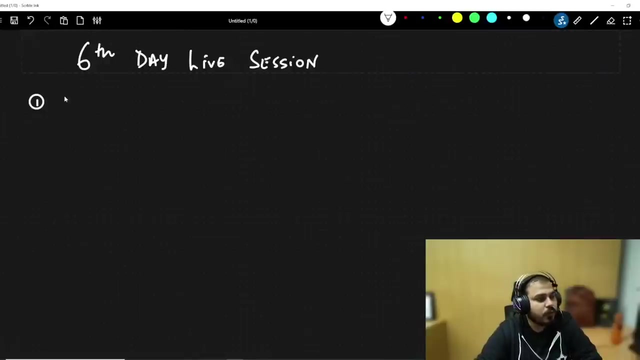 interval you can formulate, Because this was one interview question in one bank that is called as Standard Chartered Interview question. from there, Think over it. What all things basically required. right, Think over it and try to solve it. hello guys, i hope you are doing fine today. first of all, we will continue with the discussion. 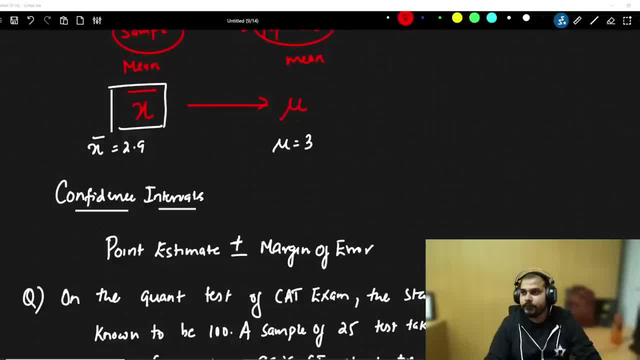 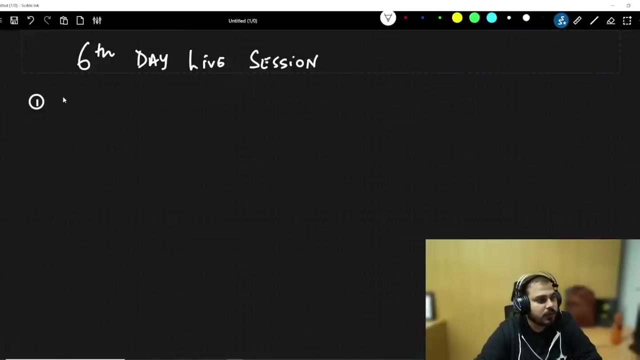 Okay, Hello guys, I hope you are doing fine Today. first of all, we will continue with the discussion where we left, So we will solve a chi-square problem. The second thing that I forgot about some of the topics over here Is with respect to covariance correlation, Pearson correlation coefficient. 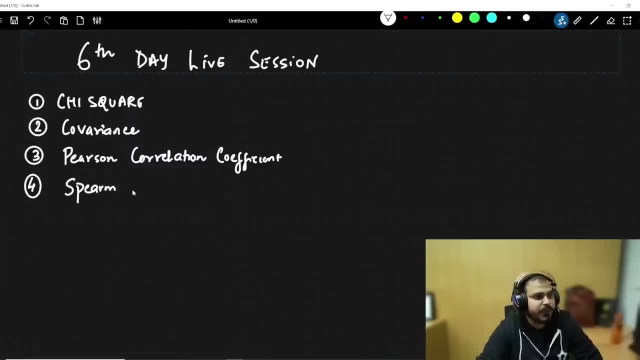 And the fourth topic that we are going to see is nothing but Spearman rank correlation coefficient. Spearman rank correlation coefficient- We are going to discuss about this. Then probably we are also going to see practical implementations, Okay, So we are also going to check out some practical implementation things. 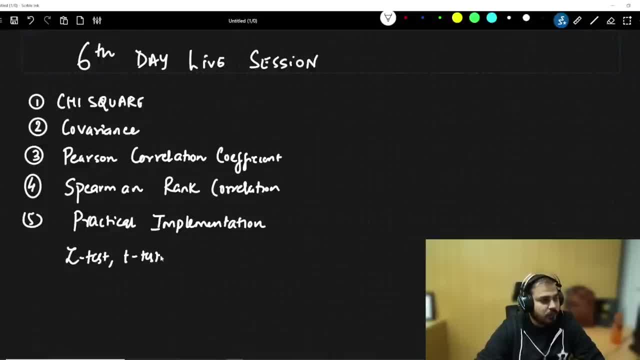 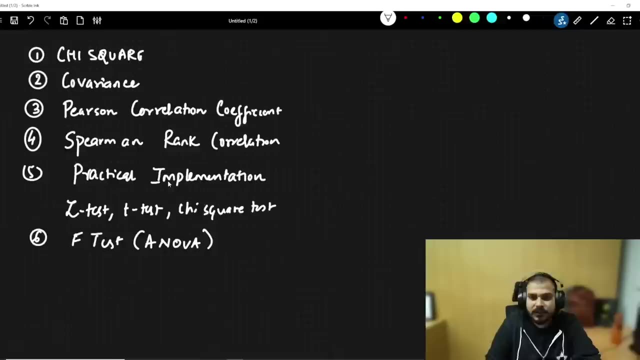 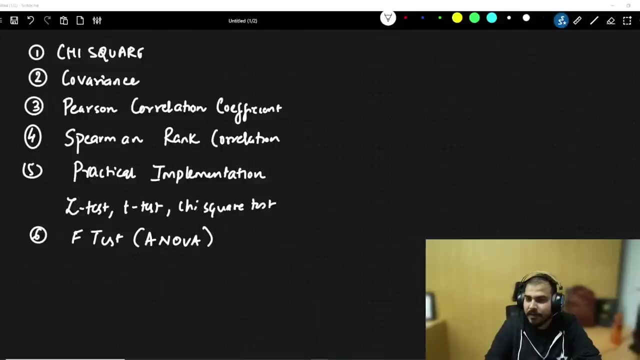 In this practical implementation. we will try to perform Z test, T test and probably also see how to perform chi-square test- This topic- we will also see F test, which is the last topic, which is also called as ANOVA test. The reason why I have kept F test as last, because the calculation will be very, very the calculation is quite complex in that particular case. 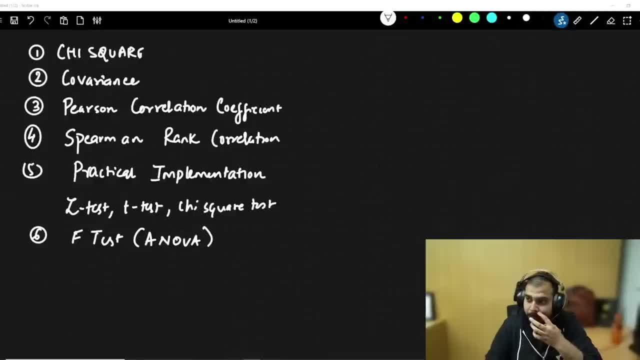 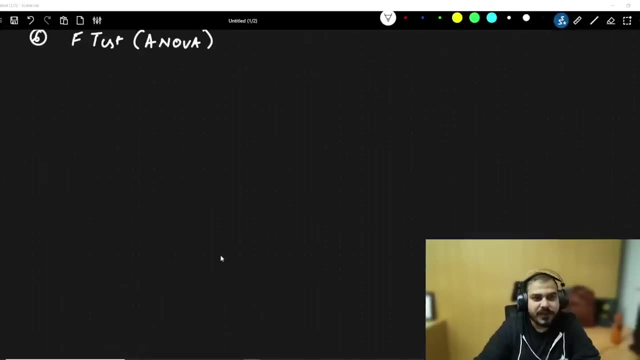 So now let's go ahead and let's try to discuss about the chi-square test. Chi-square test has quite amazing problem statement. So if I really want to discuss about chi-square test, it is mostly. I will talk about it. okay, right now. So let me just define what is exactly chi-square test. 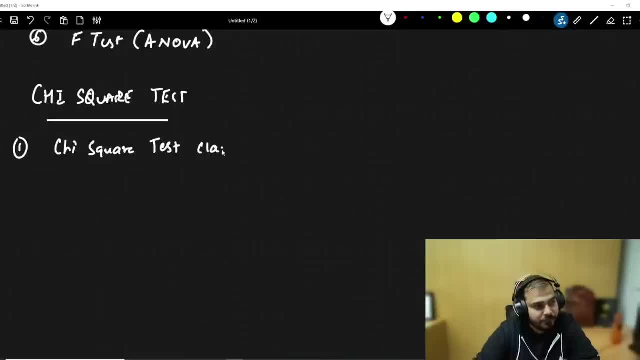 The chi-square test claims about population proportions. That basically means if someone ask you Krish- Okay, Someone ask you Krish, Someone ask you in the interview: why is chi-square test use that, Why it is used- you can just say that it is a non-parametric test that is performed on categorical variables. 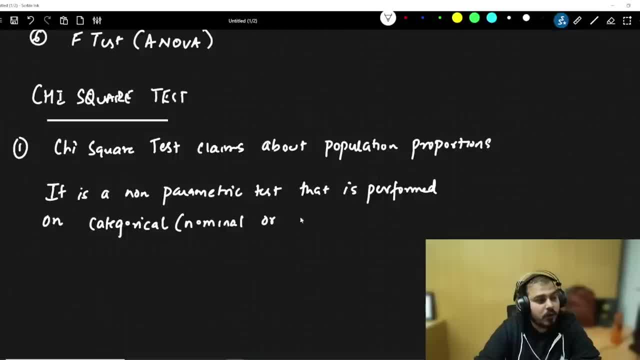 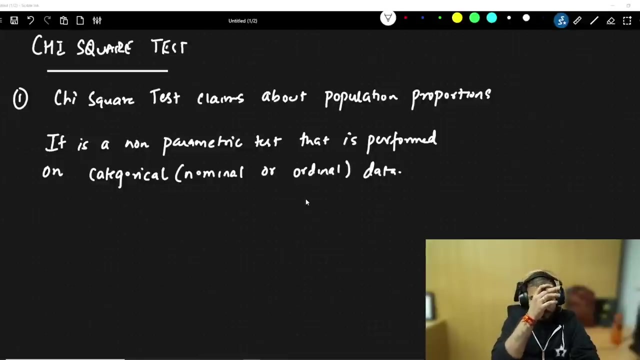 Categorical. it can be nominal or ordinal data. So this is how you basically define a chi-square test. So it is a non-parametric test that is performed on categorical or ordinal data. So this is what chi-square test is basically used. So if probably they ask you in the interview, make sure that you are basically understanding why a specific test is actually done. 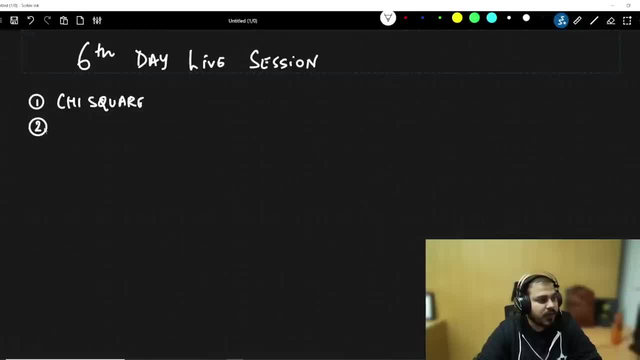 where we left, so we will solve a chi-square problem. the second thing that i forgot about some of the topics over here is with respect to covariance correlation, pearson correlation, coefficient, and the fourth topic that we are going to see is nothing but spearman rank correlation. 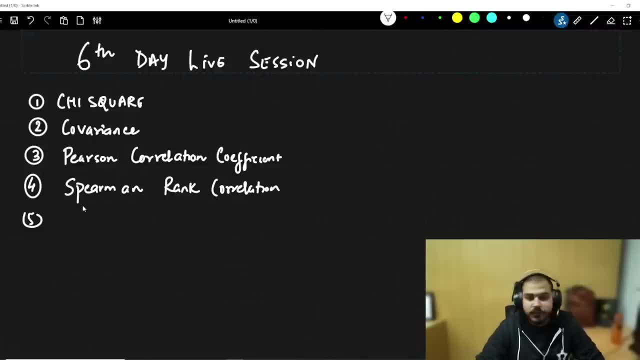 coefficient- spearman rank correlation coefficient- we are going to discuss about this. then probably we are also going to see practical implementations, okay, so we are also going to check out some practical implementation things. now, in this practical implementation, we will try to perform z test, t test and probably also see how to perform chi-square test. this topic we will also see. 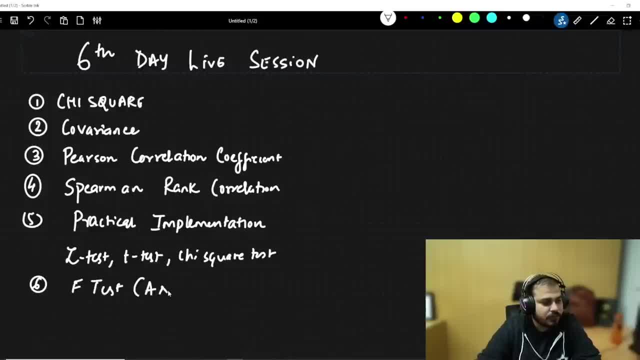 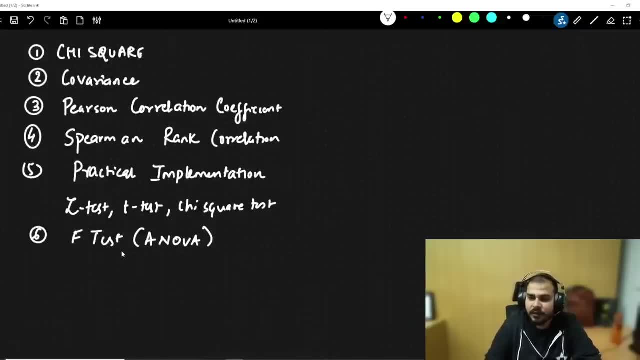 f test, which is the last topic, which is also called as anova test. the reason why i have kept f test as large, because the calculation will be very, very the calculation is quite complex in that particular case. so now let's go ahead and let's try to discuss about the 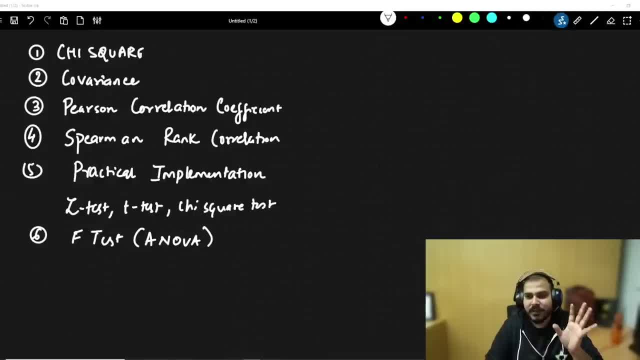 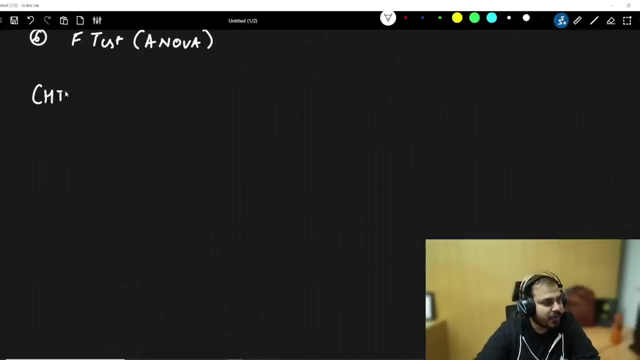 chi-square test. chi-square test has quite amazing, uh problem statement. so if i really want to discuss about chi-square test, it is mostly. i'll talk about it, okay, right now. so let me just define what is exactly chi-square test. the chi-square test claims about population proportions. that basically means if someone 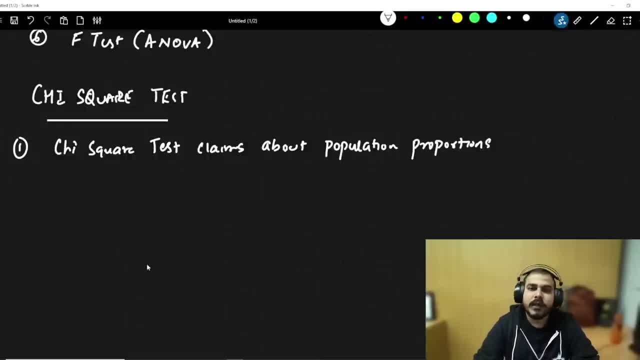 asks you krish. okay, someone asks you in the interview: why is chi-square test use that is used? you can just say that it is a non-parametric test that is performed on categorical variables. categorical, it can be nominal or ordinal data. so this is how you basically define a chi-square. 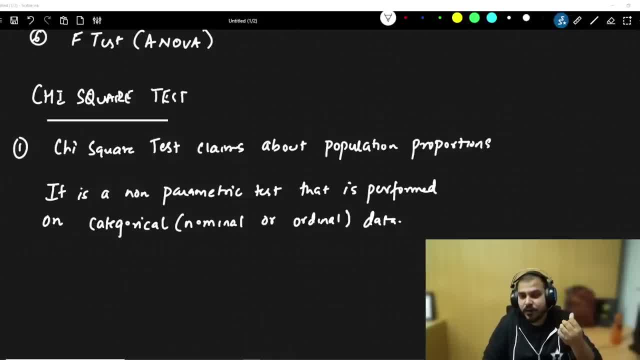 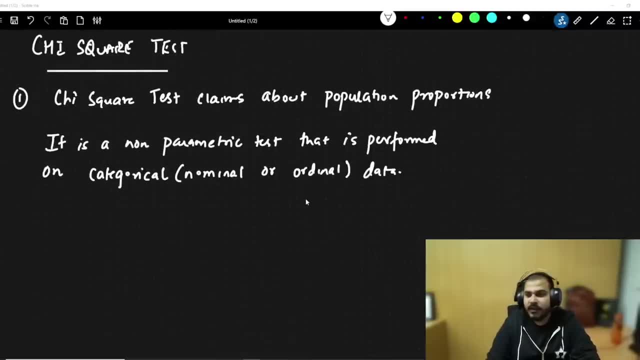 test. so it is a non-parametric test that is performed on categorical or ordinal data. so this is what chi-square test is basically used. so if probably they are using a chi-square, ask you in the interview. make sure that you are basically understanding why a specific test is. 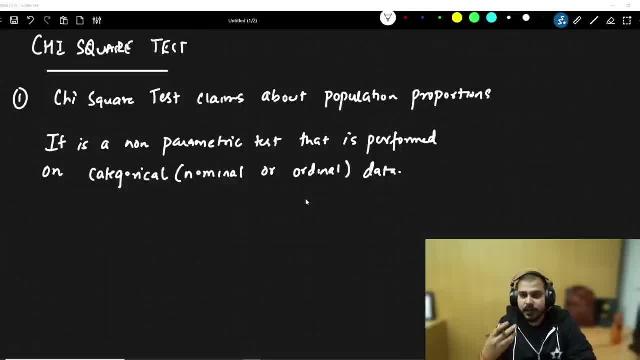 actually done. this is very, very important. okay, because in the interview they'll not. they may give you a problem statement and they may ask you what will be your plan to solve that specific problem statement, but with respect to definition, you should definitely be able to tell them. let's. 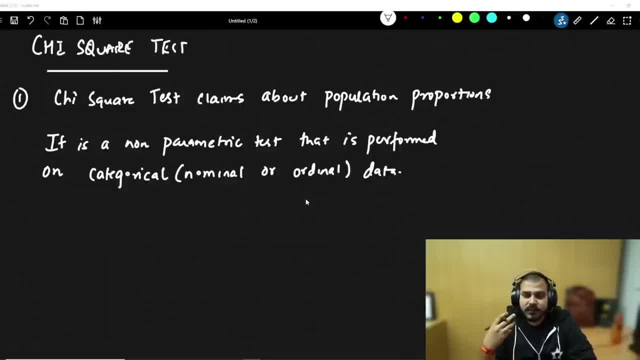 This is very, very important, okay, Because in the interview they may give you a problem statement and they may ask you what will be your plan to solve that specific problem statement. But with respect to definition, you should definitely be able to tell them: Let's go ahead and let's solve a specific problem. 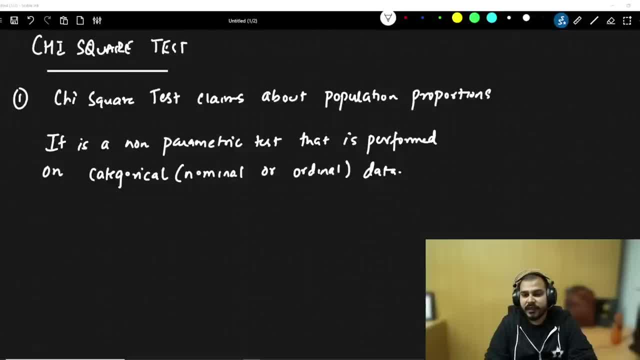 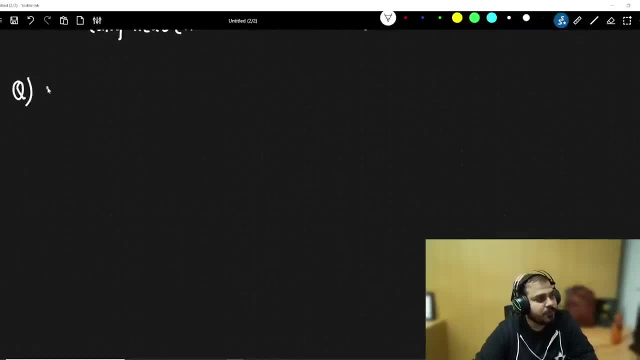 For solving this specific problem. I am just going to take a chi-square test problem. okay, Let's say that I will take a very good example. So this is my question: In 2000: Indian census: the ages of the individual. The ages of the individual in a small town. 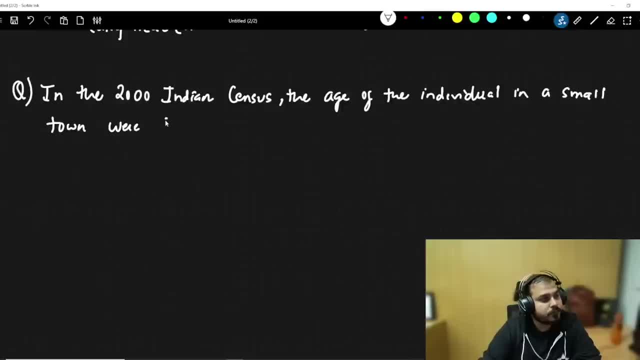 In the small town were found to be the following: Now over here you have three categories: Less than 18 years, 18 to 35 years And greater than 35 years. So you had this information in the 2000 census. 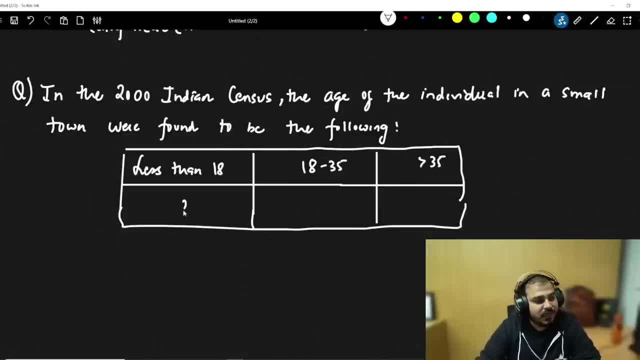 That basically means Less than 18 years. Less than 18 years were basically 20%, 18 to 35 were somewhere around 30% And greater than 35 was somewhere around 50%. Okay, so this is the information that is given from the complete census. 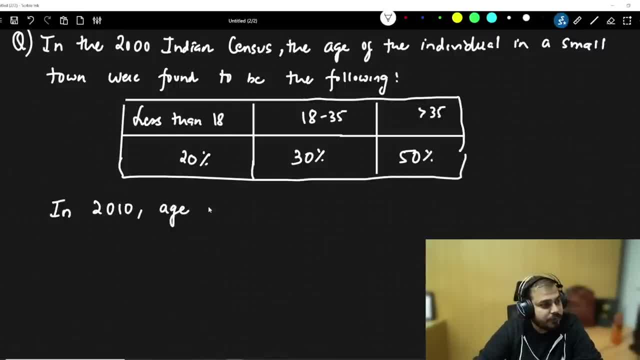 Considering this, in 2010, ages of sample n is equal to 500. individuals were sampled. Below are the results. So we basically have three columns again. That basically means in 2010. again they took a sample of 500 people And they found out. this was the basic results. 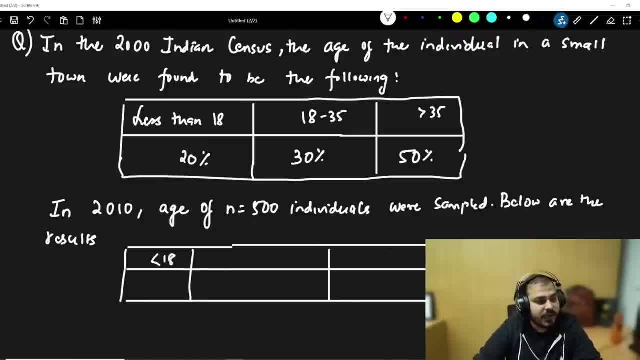 Let's see So out of those 500.. Less than 18. 18 to 35. And greater than 35. So less than 18 were 121 people, 18 to 35 were 288 people, And this was 91 people. 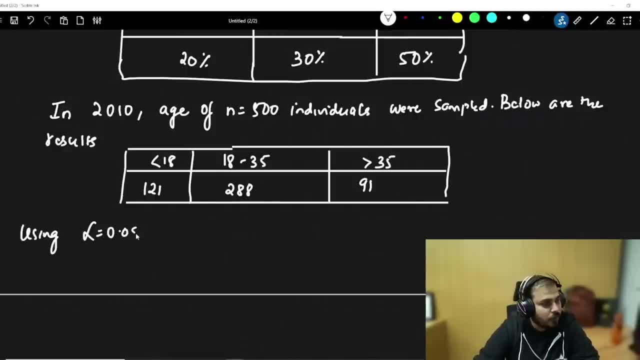 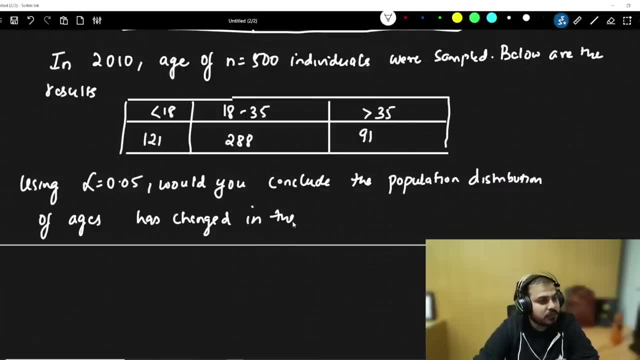 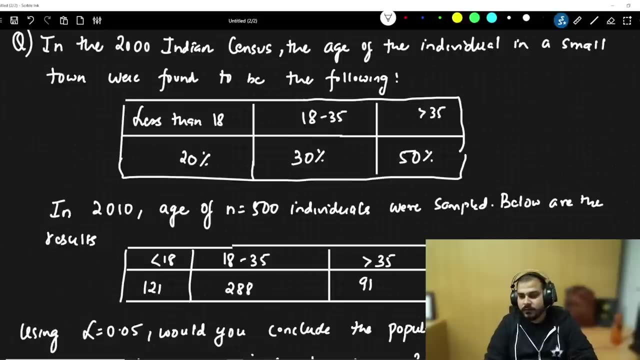 So the question is Using alpha as 0.05.. Would you conclude? the population distribution of ages has changed in the last 10 years, So this is the question that is basically given to you. The question is very much simple. It is saying that in 2000.. 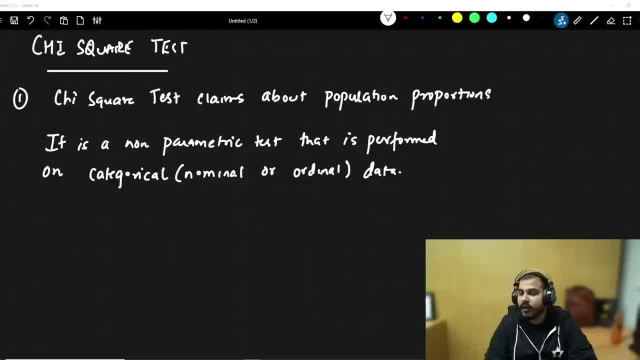 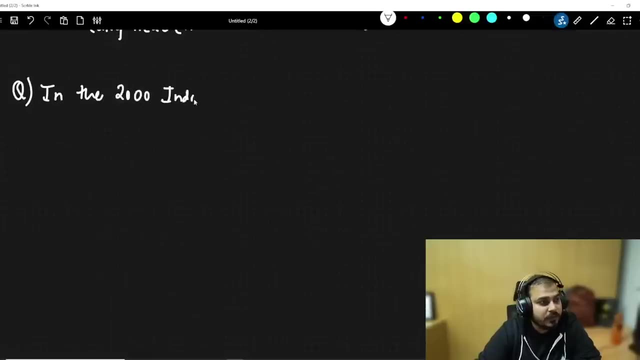 go ahead and let's solve a specific problem. for solving this specific problem, i am just going to take a chi-square test problem. okay, let's say that. uh, i'll take a very good example. so this is my question: in 2000, indian census, the ages of the individual. the ages of the individual. 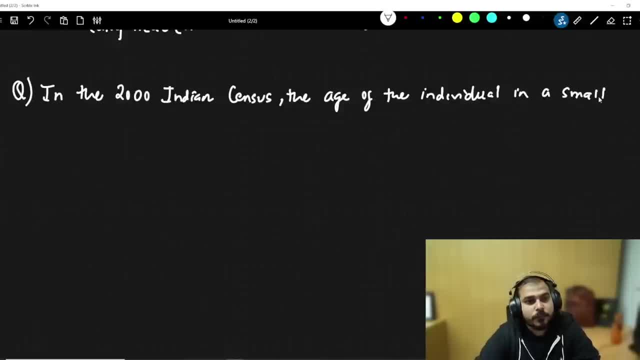 in a small town. in the small town were found to be um the following now over here you have three categories: less than 18 years, 18 to 35 years and greater than 35 years. so you had this information in the 2000 census. that basically means less than 18 years were basically 20 percent, 18 to 35 were somewhere. 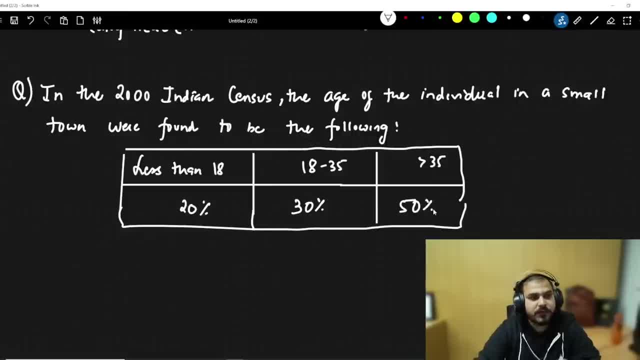 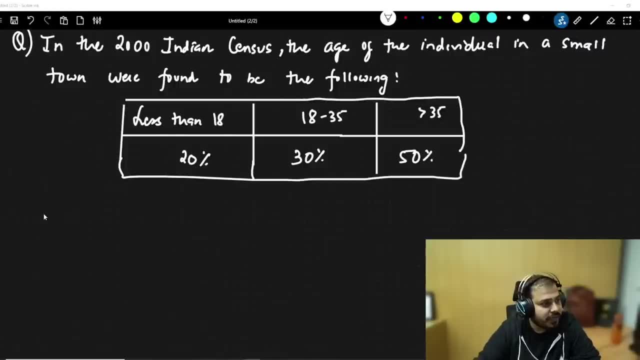 around 30 percent and greater than 35 was somewhere around 30 percent and greater than 30 percent around 50 percent. okay, so this is the information that is given from the complete census. considering this in 2010, ages of sample n is equal to 500 individuals were sampled. below are the results: 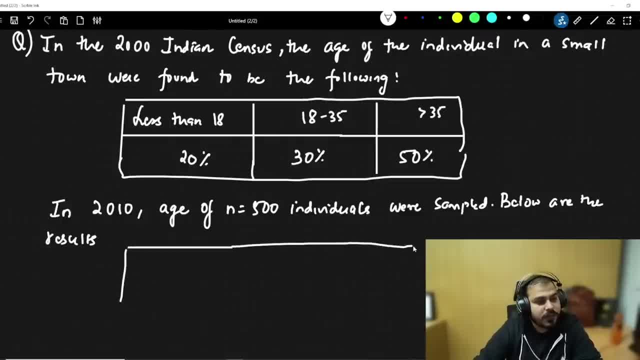 so we basically have three columns. again, that basically means in 2010. again, they took a sample of 500 people and they found out. this was the basic results let's see. so, out of those 500, less than 18, 18 to 35 and greater than 35. 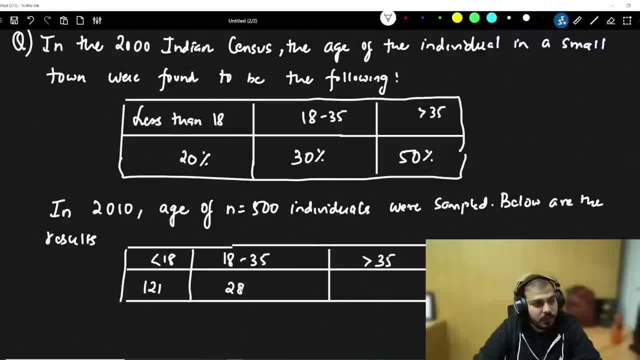 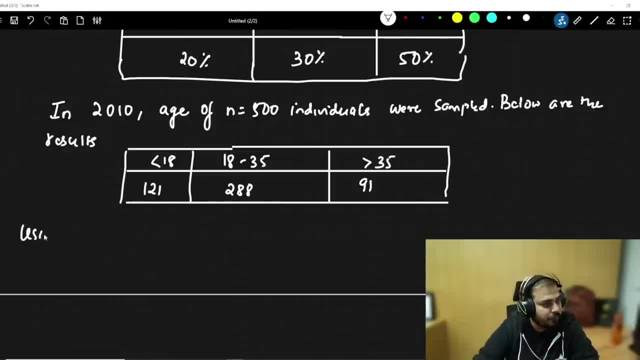 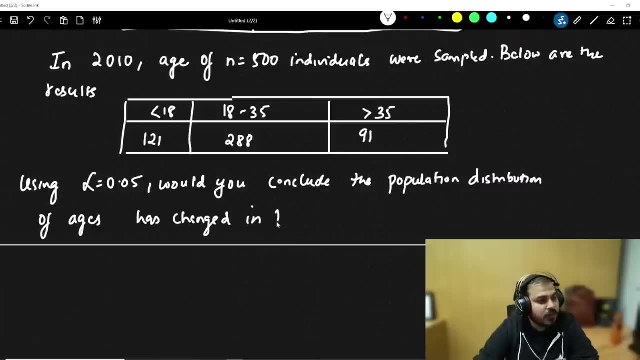 so less than 18 were 121 people. 18 to 35 were 288 people and this was 91 people. so the question is: using alpha as 0.05, would you conclude? the population distribution of ages has changed in the last 10 years, so this is the question. that is basically. 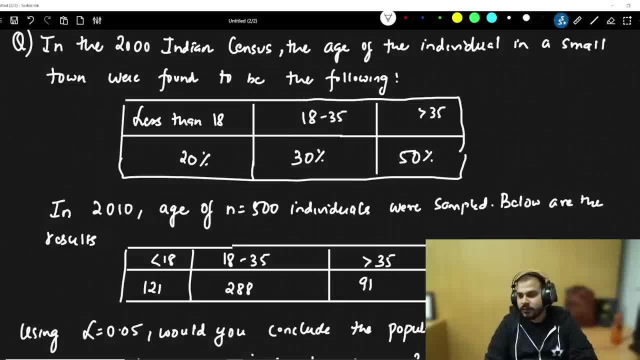 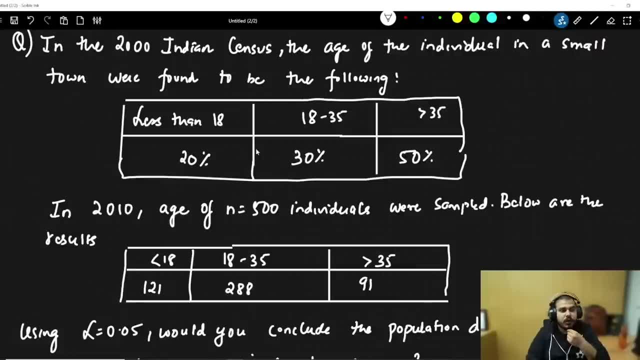 given to you. the question is very much simple. it is saying that in 2000- uh, in 2000 census, in 2000 census, the indian census, the age of the individual in a small town were less than this is basically the data. this is the population information like less than 18 percent were 20 percent, 18 to 35 were. 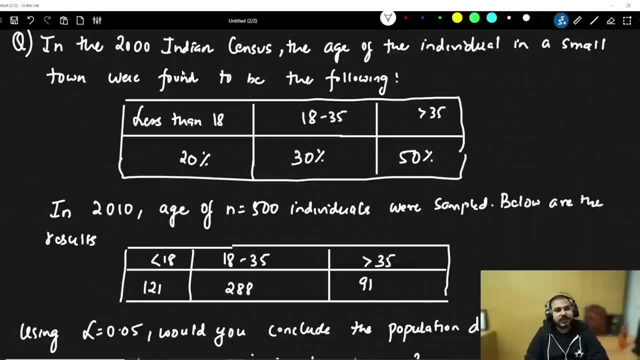 In 2000 census. In 2000 census, The Indian census, The age of the individual in a small town were less than. This is basically the data. This is the population information. Like less than 18% were 20%. 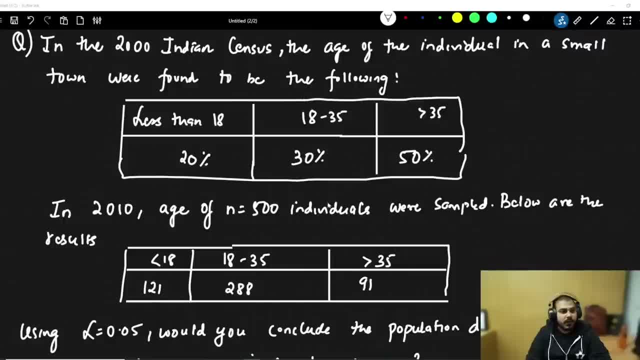 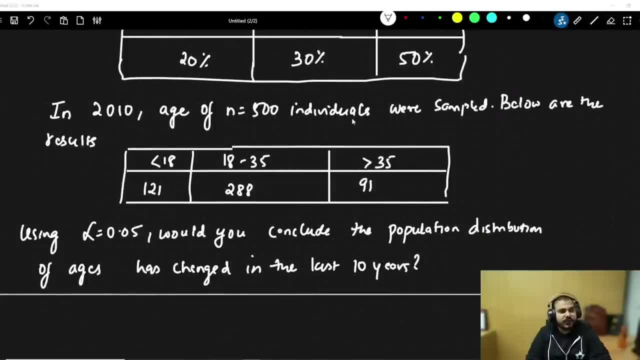 18 to 35 were basically 30%, and greater than 35 was 50%. Okay, Then in 2010, the ages of n is equal to 500- individuals were sampled. Below are the results. Then, in 2010, what happened is that. 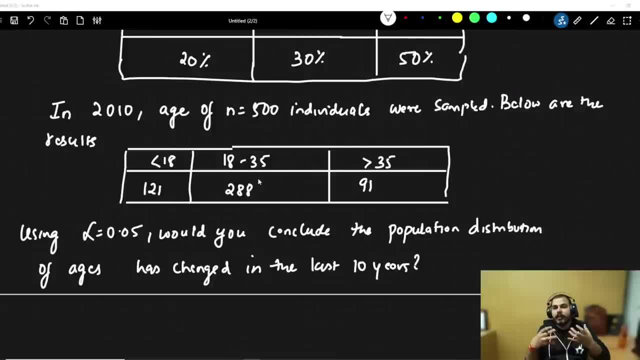 You know This again. They again found out by picking up 500 people As a sample data, And they found out that less than 18 were 121 people, 18 to 35 were 288 people And greater than 35 were 91 people. 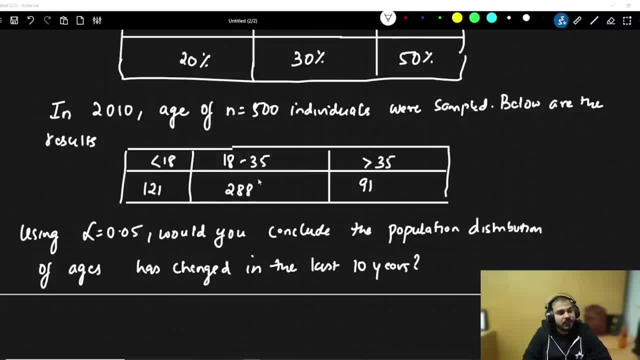 So using alpha is equal to 0.05.. Would you conclude: the population distribution has changed in the last 10 years. Now what we are going to do over here is that We are basically going to solve this particular problem. Now you may be thinking that 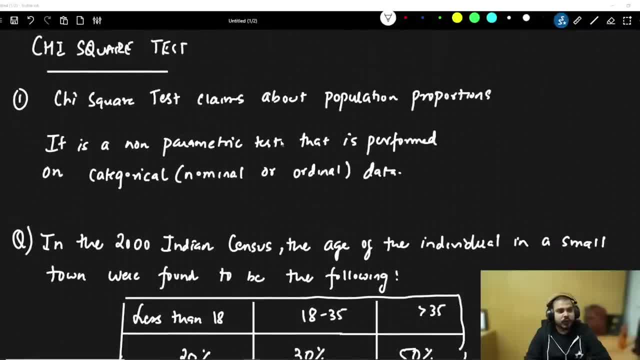 Krish, you have told that it is a non-parametric test that is performed on Categorical- That is, nominal or ordinal- data. Now, what exactly is non-parametric test? Non-parametric test usually occurs In the case of non-parametric test. 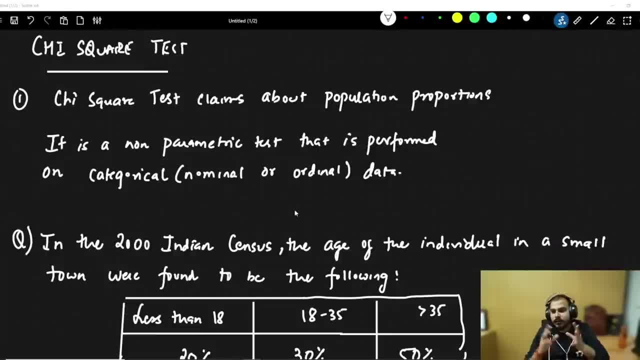 Non-parametric test usually occurs with respect to population proportion. Whenever you are given some kind of proportions of data, At that point of time You cannot specifically use a kind of parametric test, So you have to go with non-parametric test. 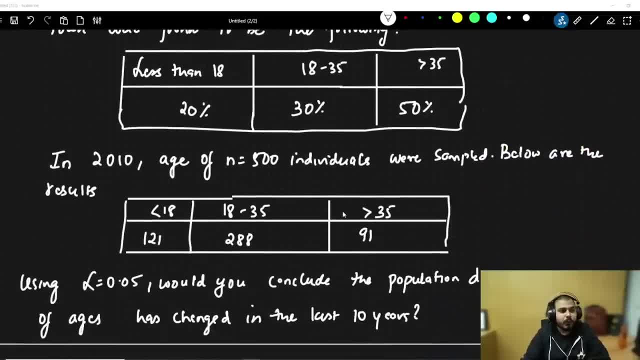 Now here you can actually see that This is the original data with respect to the population. Then you sample the data and you found it out Right, And then we are just trying to see that What is the difference between this to this? 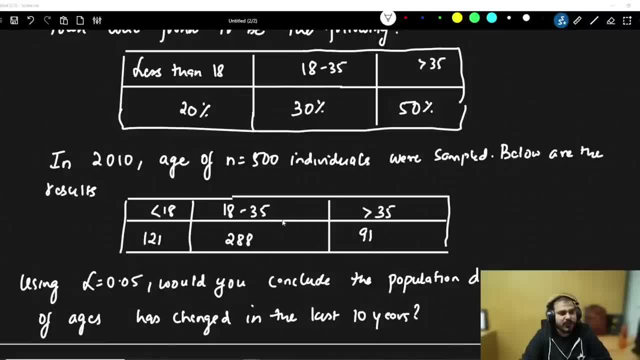 This to this. Do you think The population may have probably changed just by seeing the specific data? Or Still, you will probably Just say that Yeah, So it may be. population has changed Probably 18 to 35. You can see a huge quantity or number. 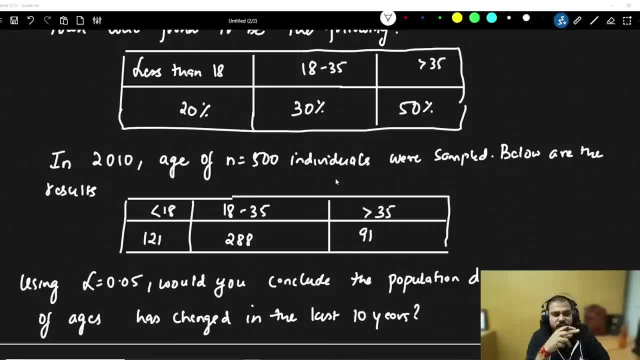 Greater than 35. Just seeing the percentage, It shows a very less number. Obviously, from the above population proportion You should be saying that greater than 35 should be more. In this particular situation, In this particular scenario, What kind of assumptions we can make? 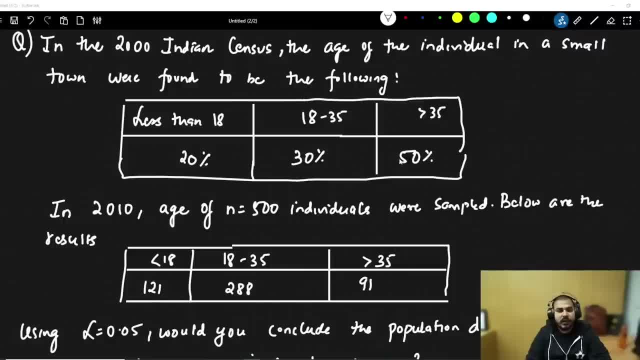 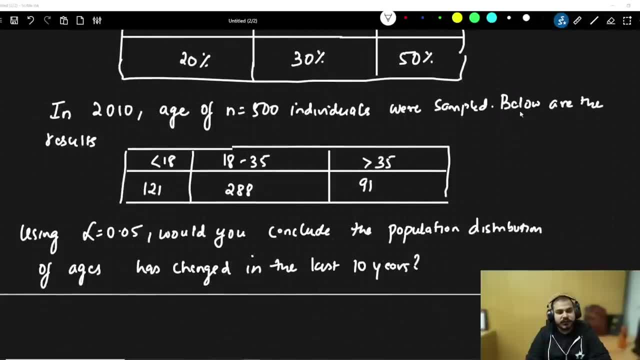 basically, uh, 30 percentage and greater than 35 was 50 percentage. okay, then, in 2010, the ages of n is equal to 500- individuals were sampled. below are the results: then, in 2010, what happened is that? you know? uh, this again sam. they again found out by picking up 500 people as a sample data, and 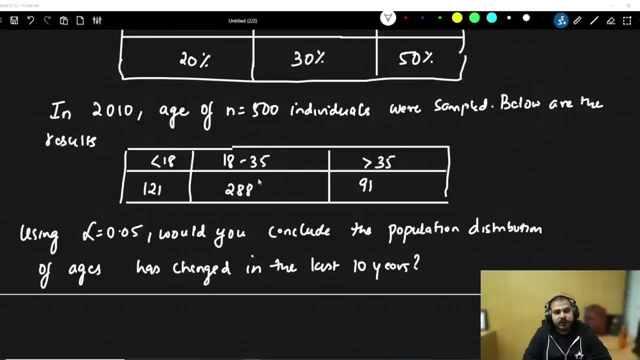 they found out that less than 18 were 121 people, 18 to 35 were 288 people and greater than 35 was 91 people. so, using alpha is equal to 0.05. would you conclude? the population distribution has changed in the last 10 years. now what we are going to do. 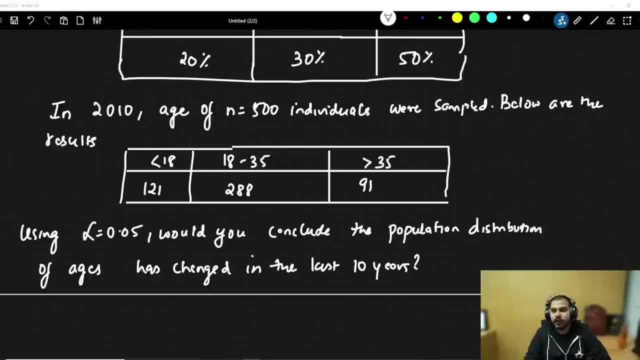 over the next 10 years. we are going to use the population distribution distribution to. over the next 10 years. we are going to use the population distribution distribution to. here is that we are basically going to solve this particular problem. Now you may be thinking that 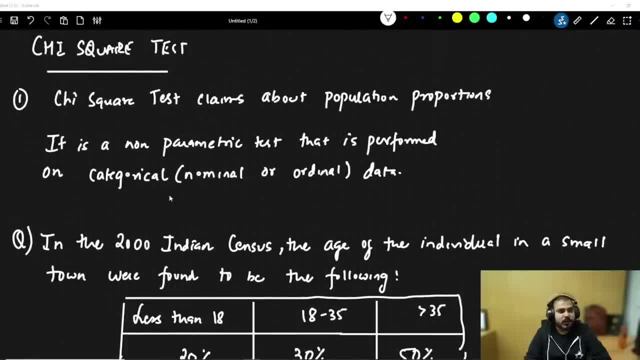 Krish, you have told that it is a non-parametric test that is performed on categorical- that is, nominal or ordinal- data. Now, what exactly is non-parametric test? Non-parametric test usually occurs with respect to population proportion. Whenever you are given some kind of proportions. 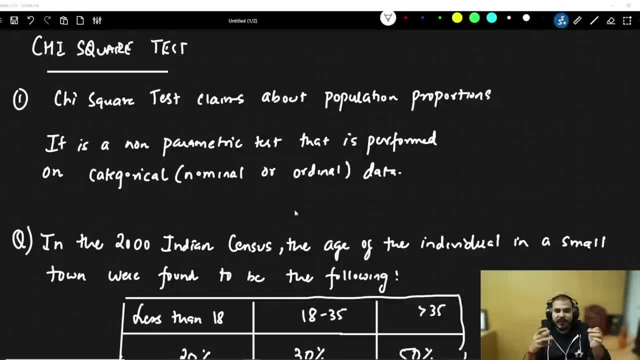 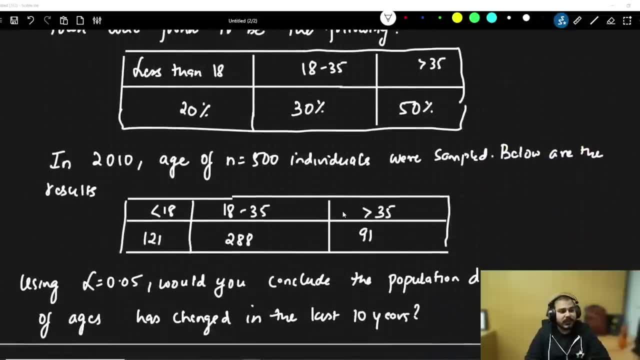 of data. at that point of time you cannot specifically use a kind of parametric test, so you have to go with non-parametric test. Now, here you can actually see that when this is the original data with respect to the population, then you sample the data and you found it out. 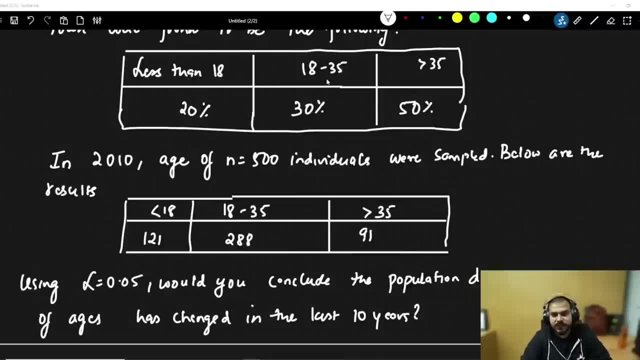 right, and then we are just trying to see that. what is the difference between this to this, this to this? do you think the population may have probably changed just by seeing this specific data? or you, Still, you will probably just say that yeah, sir, it may be. population has changed probably. 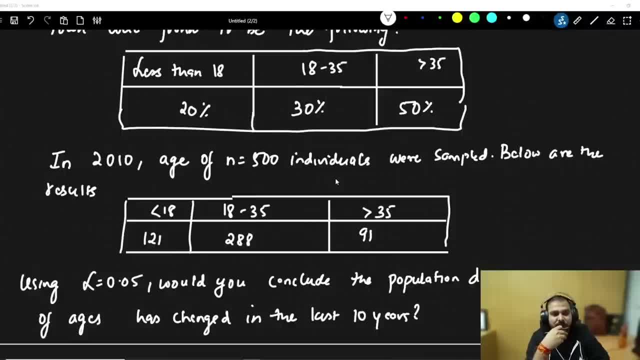 18 to 35, you can see a huge quantity or number greater than 35. just seeing the percentage, it shows a very less number. obviously, from the above population proportion you should be saying that greater than 35 should be more. In this particular scenario. what kind of assumptions we can make? 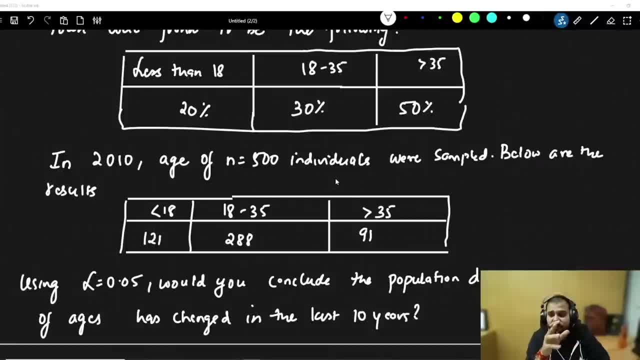 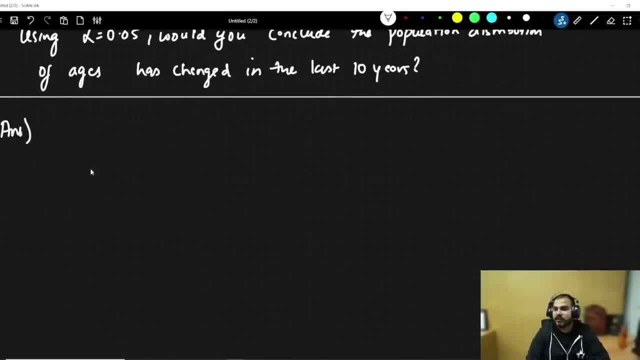 there is two kind of assumptions: whether the population distribution has changed or whether it has not. So let's not need to go into that. you'll have this big bar chart restarts. what we've done for now is that we have a quick demo of what this is. 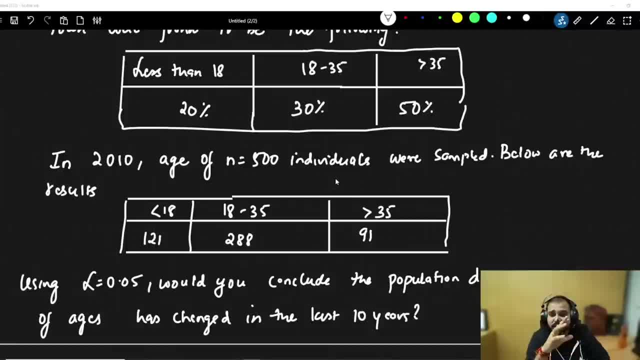 There is two kinds of assumptions: Whether the population distribution has changed Or whether it has not. So how to go ahead and approach and solve this particular problem. So here I am going to basically start the answer. So the first step, What we are going to do. 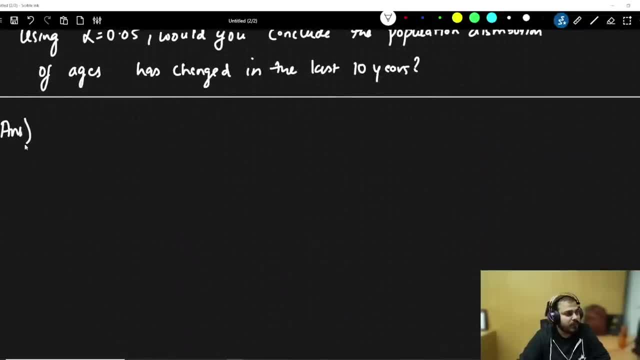 As usual, You can, Let's let's go ahead and let's make two tables First of all. So this is my first table. This is my second table, Because this table will play a very important role, Guys. Okay, The first table. 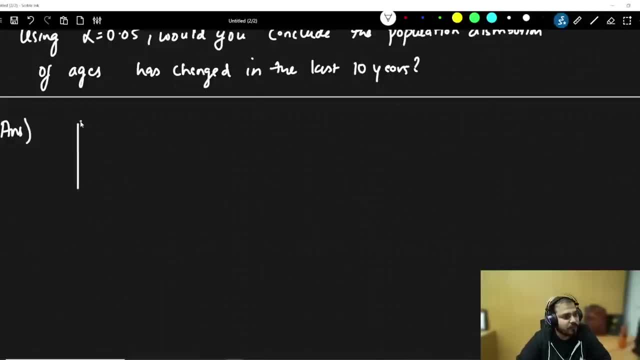 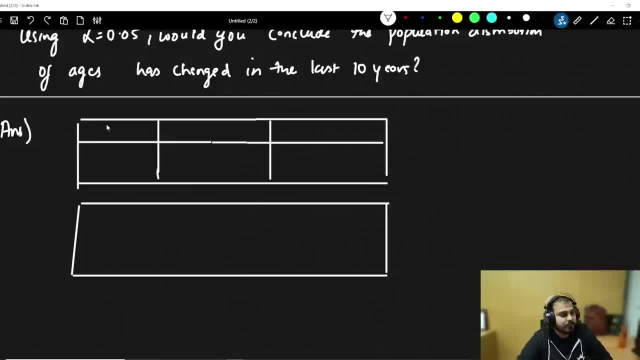 Basically have The population information, So I am just going to Draw it over here. Here I am going to basically say: Less than This is Less than 18.. 18 to 35. And greater than 35.. 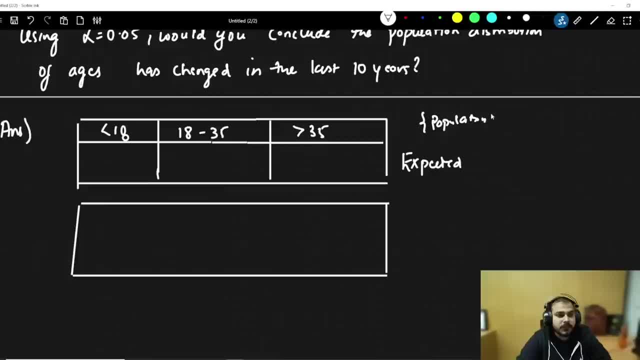 Now, this is the Expected. See Why I am saying expected, Because this is the population information. This is the population information. So here, Less than 18 is 20 %, This is 30 % And this 60 % and this is 50%. Now, this is what your entire distribution is expected to be, because in 2000, 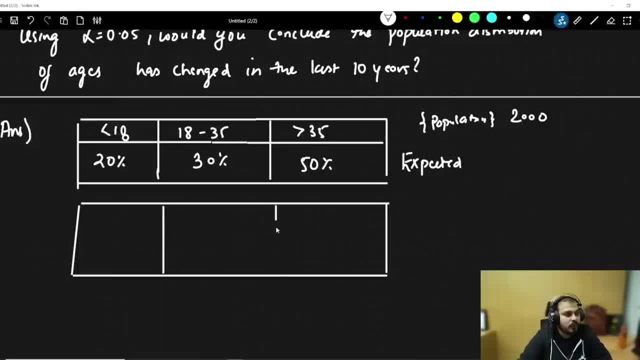 US census. they found out this data Now, right now, after 10 years, when they took the sample of n is equal to 500, this is the observed one. So the observed one was less than 18, less than 18 was 121, 18 to 35 was 288 and greater than 35 were 91.. So this two information you. 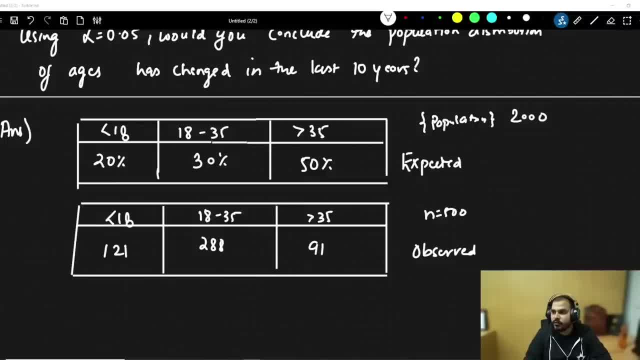 definitely have The reason why I am drawing this two, or writing this two, information. okay, we will be able to understand it Now. we will create one more table, and the table is something called as expect based. This is the observed one right Now, what I'll do. 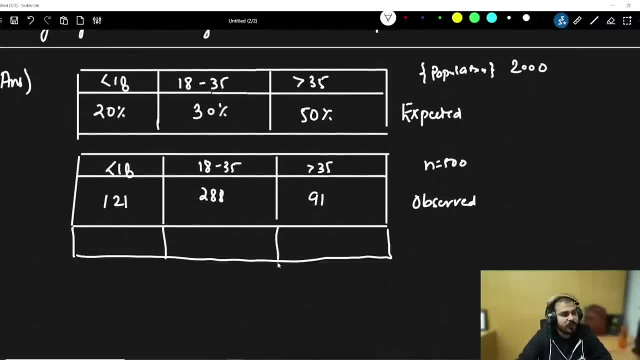 I'll create one more field And let's say, based on this- suppose, if I take, n is equal to 500, based on this, what should be our expected? What should be our expected distribution based on this data, If I am picking up 500.. So we will try to divide this based on this percentage, right? So here my 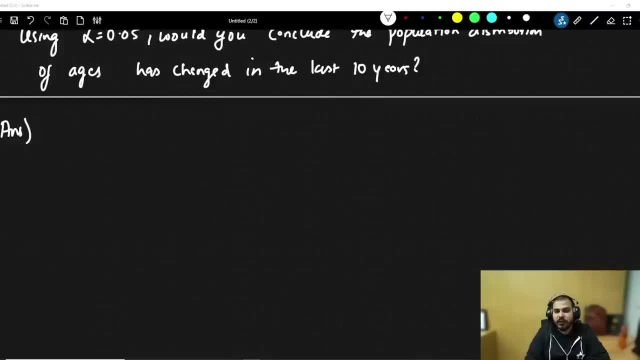 So, if the pressure is your default- and, as you can see, your pressure is set to your default, yeah, in terms of the universal limit. So I just needed to start the session with you, know, know, your data here, cryptogram, and I ll draw a picture, and this could heat it up once or twice as I draw it down as a whole. I don't feel like we're gonna mess this up, so go with me. 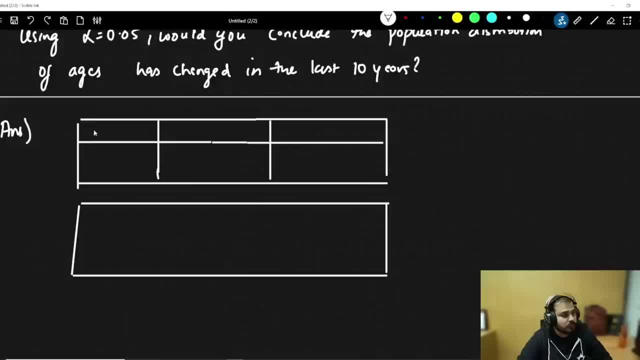 Here I am going to basically say: less than this is less than 18, 18 to 35 and greater than 35.. Now, this is the expected. see why I am saying expected, because this is the population information. this is the population information. 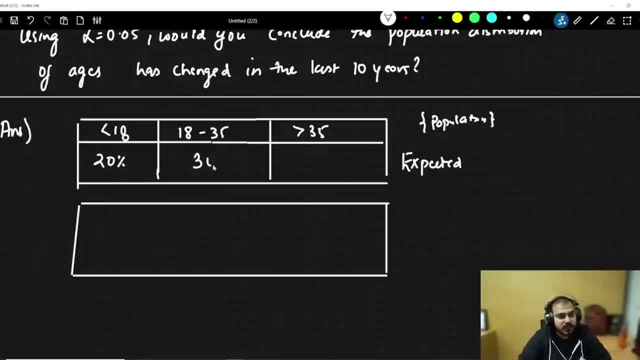 So here, less than 18 is 20%, this is 30% and this is 50%. Now, this is what your entire distribution is expected to be, because in 2000 you have since said they found out this data Now, right now, after 10 years, when they took the sample of n is equal to 500,. this is the. 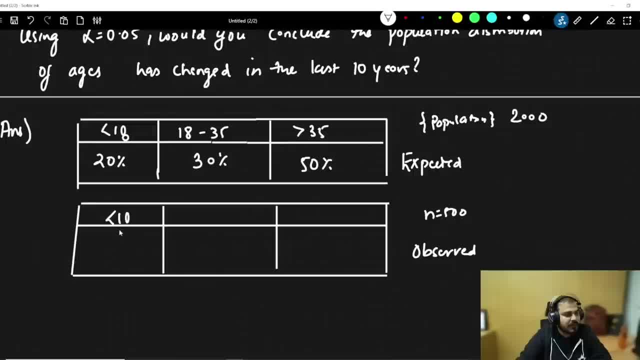 observed one. So the observed one was less than 18, less than 18 was 121, 18 to 35 was 288 and greater than 35 were 91. So this two information you definitely have The reason why I am drawing this. 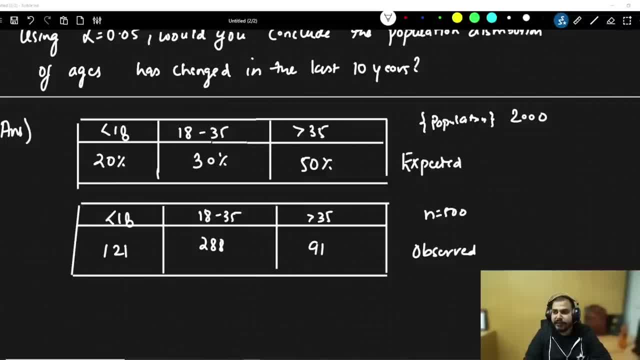 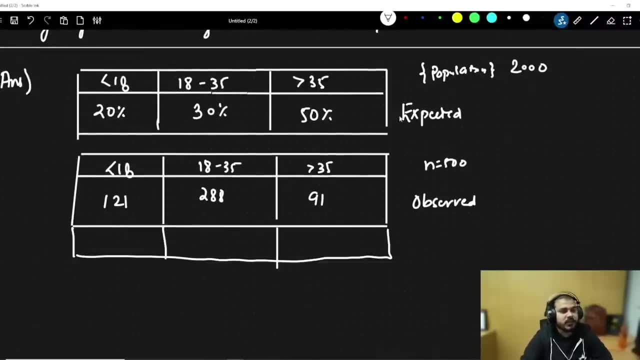 This two, or writing this two, information. okay, we will be able to understand it Now. we will create one more table and the table is something called as expect based. This is the observed one right Now. what I will do. I will create one more field and, let's say, based on this suppose, 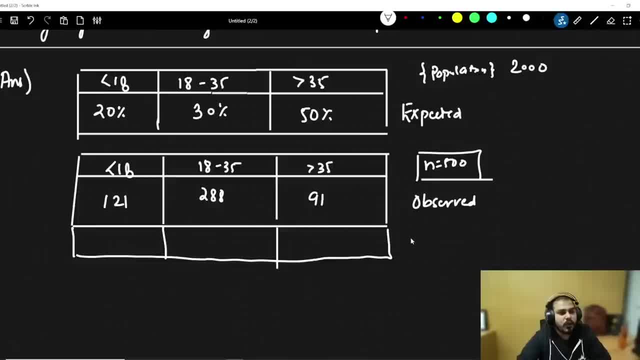 if I take n is equal to 500,. based on this, what should be our expected? What should be our expected distribution based on this data, if I am picking up 500?? Okay, So we will try to divide this based on this percentage, right. 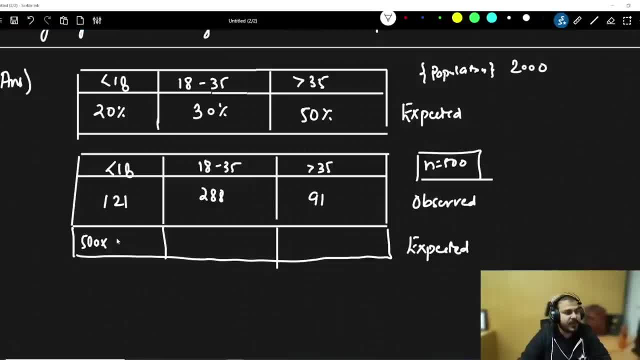 So here my value will be 500,. 500 multiplied by what is 20% is less than 18.. So I will multiply by 0.2.. Here I will say 500 multiplied by 0.3.. Here I will say 500 multiplied by 0.5.. 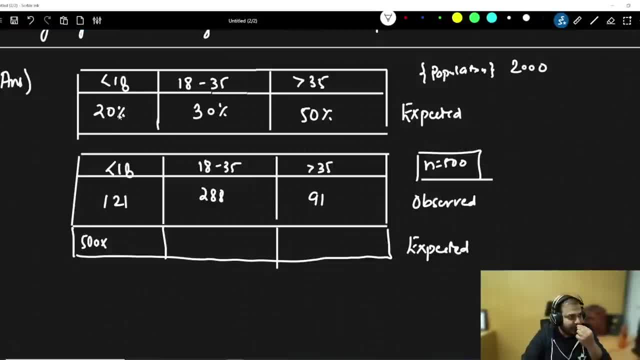 value will be 500 multiplied by what is 20% is less than 18.. So I will multiply by 0.2.. Here I will say 500 multiplied by 0.2.. So my most expected distribution will be 500 multiplied by 0.3.. Here I will say: 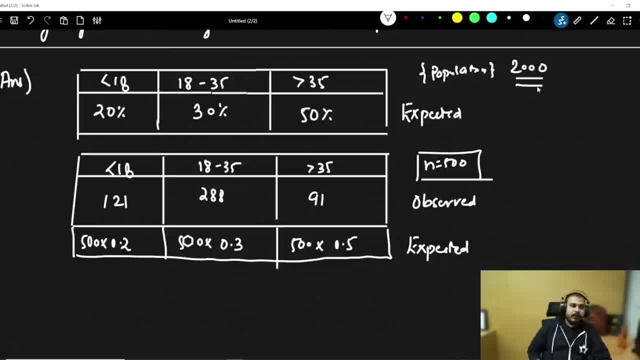 500 multiplied by 0.5.. So this should be my expected distribution based on 2000 census Observed. is this one that is fine, but we really need to find out our expected also. So if I multiply this two, so if I multiply 500 multiplied by 0.2, this is basically 100.. So here I'm. 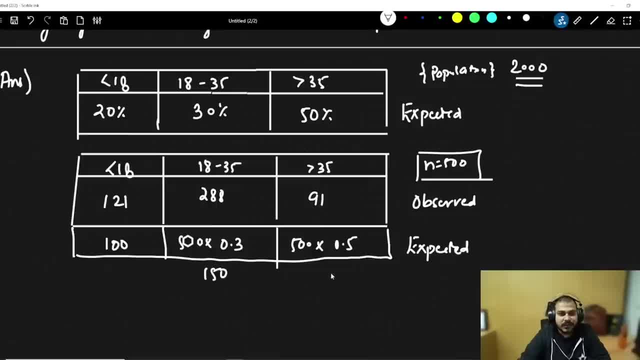 basically going to write hundred. This will be how much. This will be 150.. was what was the? what was the distribution i needed to have based on the 500 data, based on this 2000 census? but this is what is observed. so now let's go and focus on this. two table right. 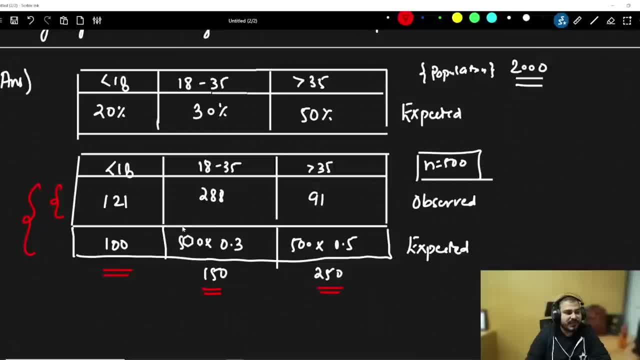 now. okay, so we have got 100, 150, 250. obviously there is a huge difference. by seeing this, only you will be able to say that: okay, krish, there is a huge difference here. only i can definitely say that, okay, just reject the null hypothesis, but understand over here. alpha is basically given. 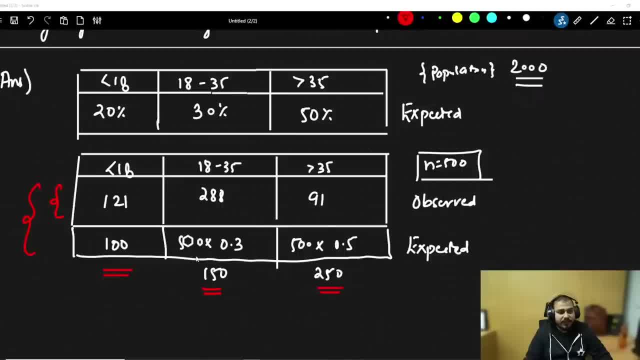 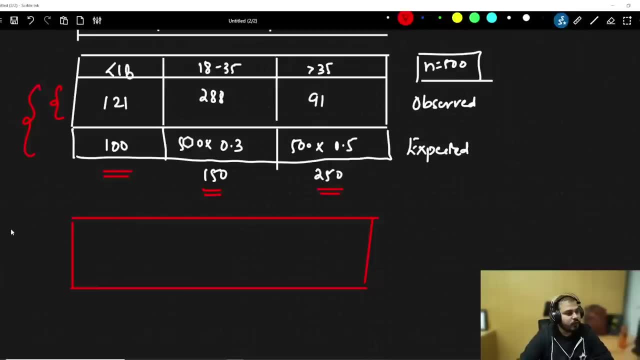 i want 95 percentage confidence interval. why multiplied? again, understand why multiplied: because we need to find the expected distribution based on this data from this 500 sample. so if i consider 500 sample in 2010 also, i need to get this data: 100, 150, 250. so i'm basically going to. 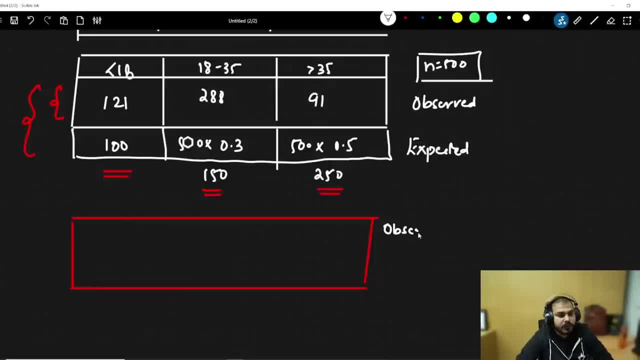 say: this is my, this is my observation and this is my expected. so this here has less than 18, 18 to 35 and greater than 35. so less than 18 is how much i have, basically 121, 288, 91. this is the observation, and then i have 100. 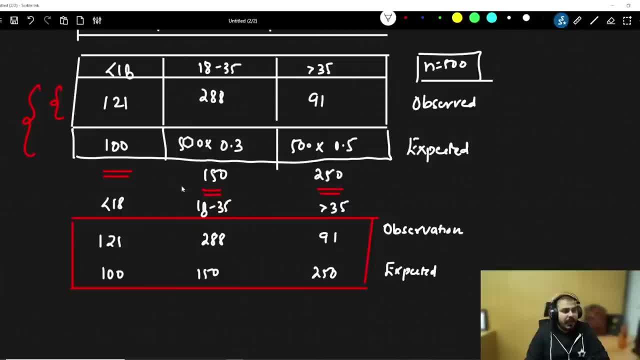 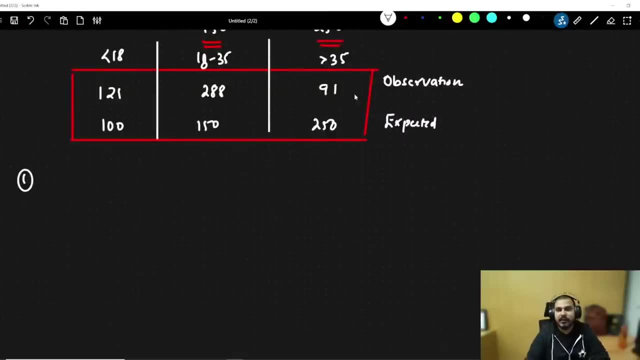 150 and 250. now, these are my three categories. this is one category, this is two category and this is the third category. now let's go ahead and let's try to understand what is the next step. now, next step, i will first of all- obviously you know you have to define your null hypothesis, alternate- 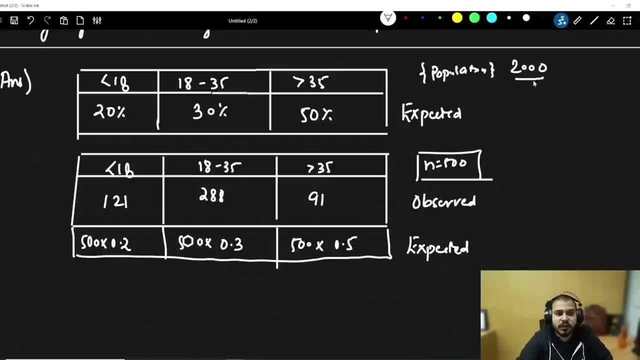 So this should be my expected distribution based on 2000 census. Observed is this one. That is fine, But we really need to find out our except expected only. So if I multiply this too, so if I multiply 500 multiplied by 0.2, this is basically 100. 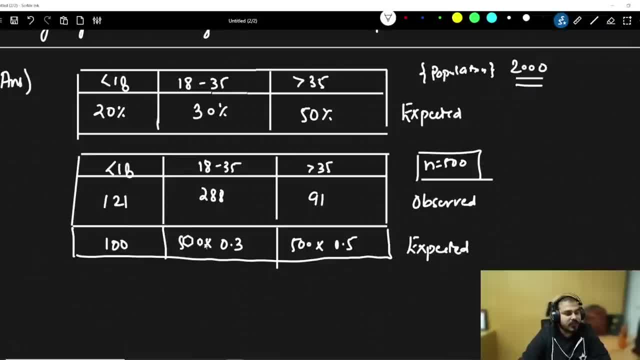 So here I'm basically going to write 100.. This will be how much. This will be 150 and this will be 250.. This was what was the distribution I needed to have, based on the 500 data, based on this 2000 census. 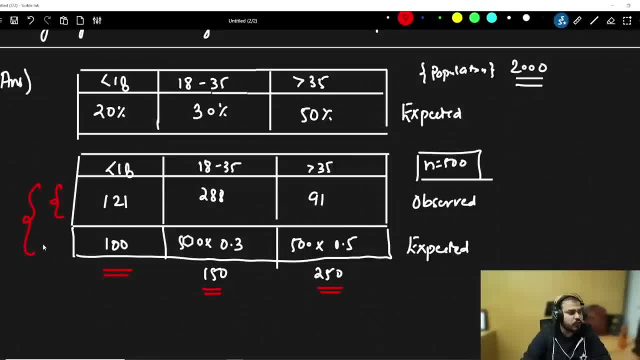 But this is what is observed. So now let's go and focus on this two table right now. Okay, So we have got 100.. 150, 250, obviously there is a huge difference. by seeing this only you'll be able to say: 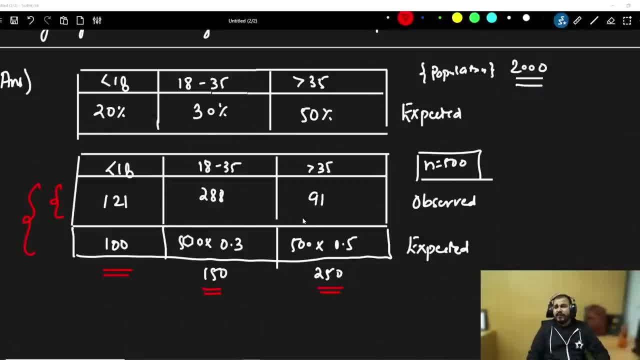 that. okay, Chris, there is a huge difference here. Only I can definitely say that, okay, just reject the null hypothesis. but understand over here: alpha is basically given. I want 95 percentage confidence interval. Why multiplied? again, Understand why multiplied. 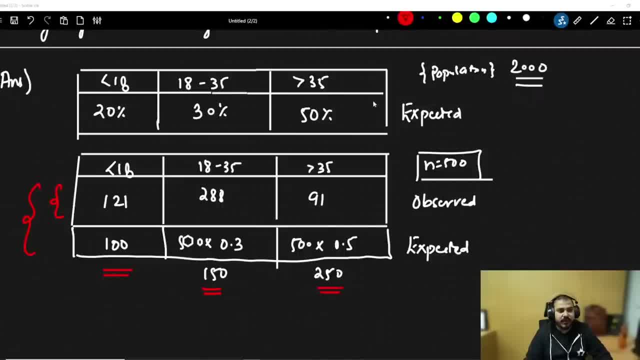 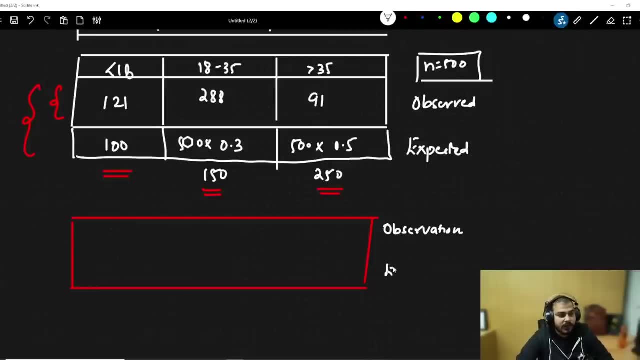 Because we need to find the expected distribution based on this data from this 500 sample. So, if I consider 500 sample in 2010, also, I need to get this data: 100, 150, 250.. So I'm basically going to say: this is my, this is my observation and this is my expected. 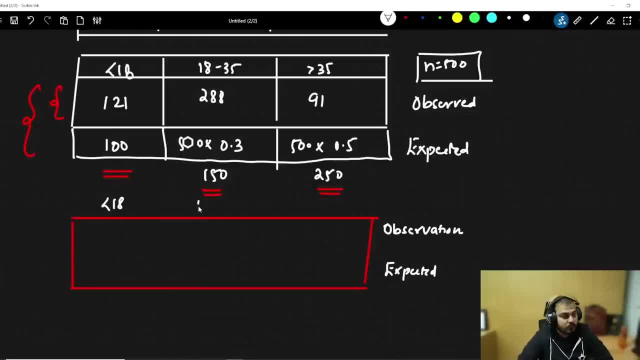 So this here has less than 18, 18 to 35 and greater than 35.. So less than 18 is how much. I have basically 121, 288, 91.. This is the observation, And then I have 100.. 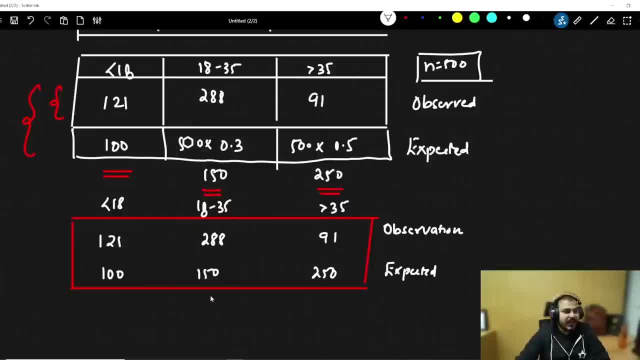 150 and 250.. Now, these are my three categories. This is one category, This is two category and this is the third category. Now let's go ahead and let's try to understand what is the next step. Now, next step, I will first of all, obviously, you know, you have to define your null hypothesis. 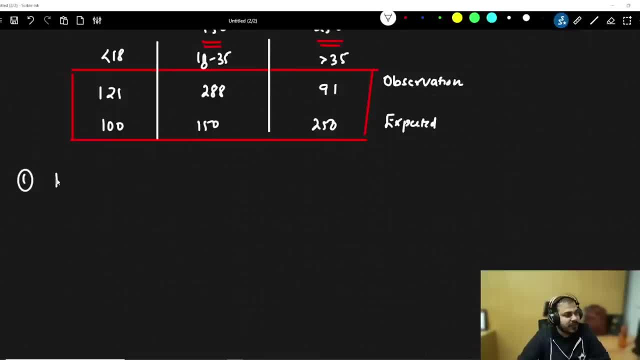 alternate hypothesis when you start the hypothesis testing. So let's say that my null hypothesis is that the data meets the distribution, meets the distribution. This is the data right. This is the data observation data. it meets the distribution of 2010 census, of- sorry- of 2000 census. 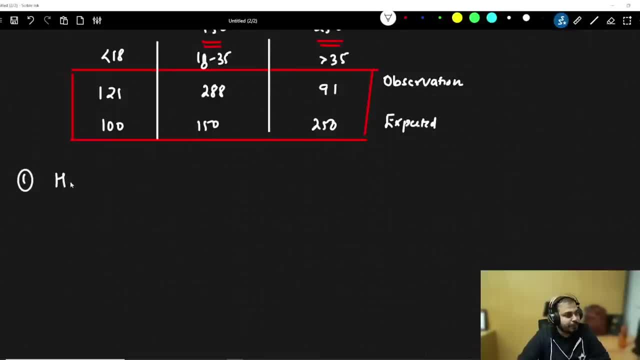 hypothesis when you start the hypothesis test. you have to define your null hypothesis when you start testing. so let's say that my null hypothesis is that the data meets the distribution, meets the distribution. this is the data right. this is the data observation data. it meets the distribution. 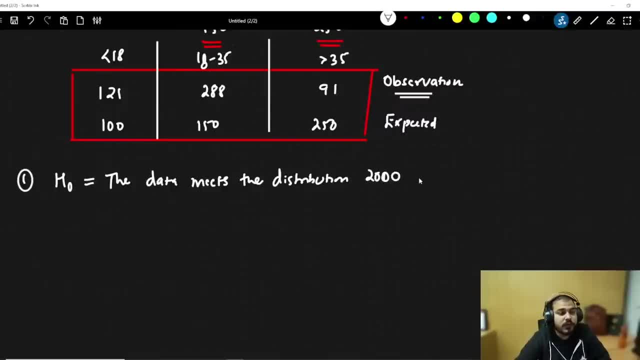 of 2010 census, of- sorry- of 2000 census. my alternate hypothesis will say that the data does not meet the distribution of 2000 census. so i hope everybody is able to understand the null hypothesis and the alternate hypothesis. so i'm going to start the observation and then i'm going to 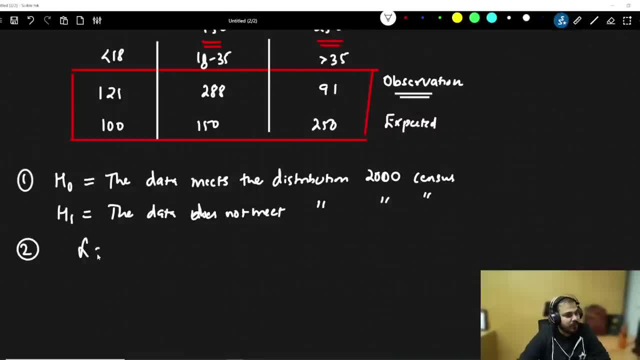 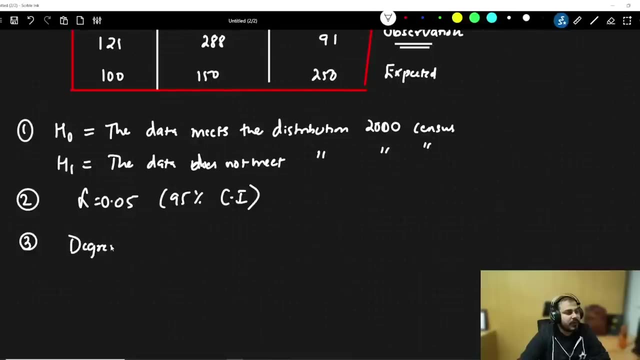 type of this. then the second step is my alpha value. my alpha is 0.05. that basically means 95 percentage confidence interval. now the third step in this is that whenever we do a chi-square test, we also need to know the degree of freedom. so how do we calculate degree of freedom? 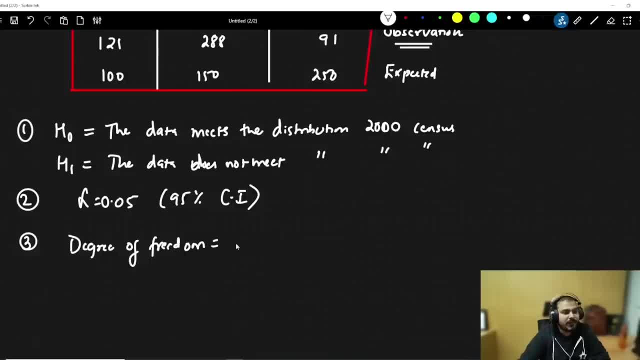 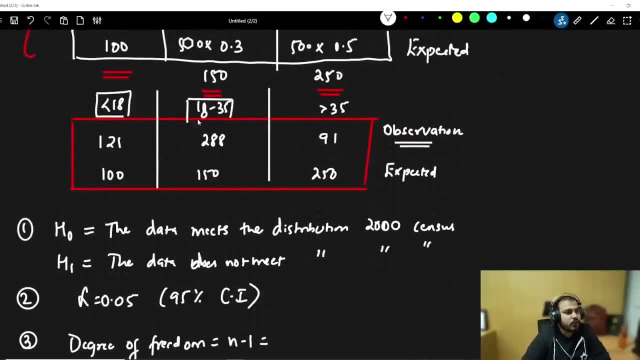 this is the steps, guys, and always this will be like this: one n minus 1. what is n over here? n is nothing, but this is 1, 2 and 3. this is where number of categories are coming into picture. categories are coming into picture: 1, 2 and 3. so 3 minus 1 is basically 2. age is now categorical. 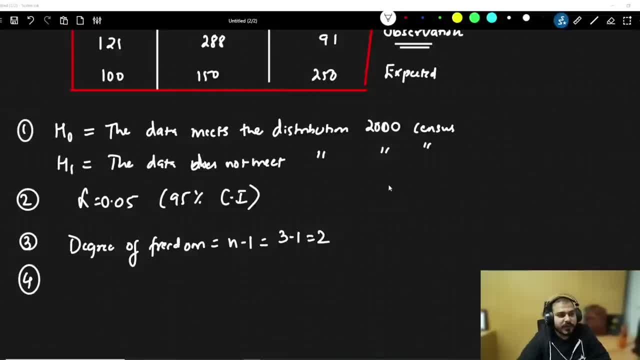 right, absolutely perfectly fine. you know your degree of freedom. your degree of freedom is 2 and your alpha value is 0.05. all you have to do is that go and check in the chi-square table, okay, to find out your decision boundary. is this a one tail test or two tail test? the data may be less than your. 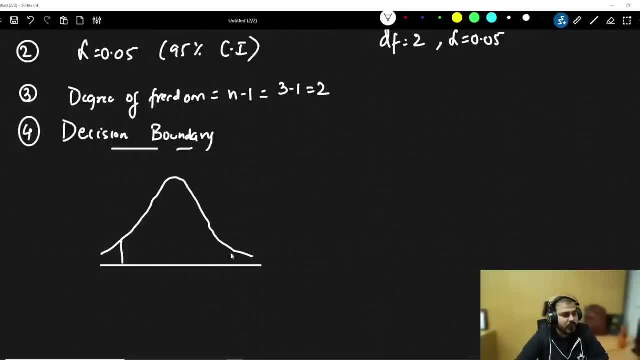 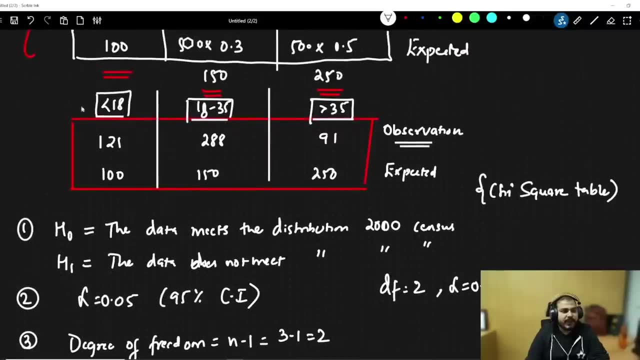 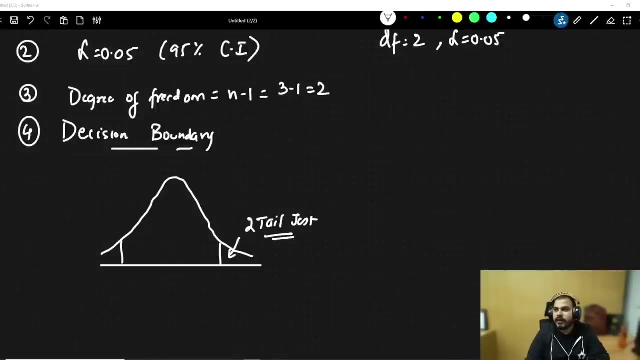 distribution, it may be more right. so here is this: a two tail test. because alpha is 0.05, guys, we have to pick three as n, because there are three age categories. so this will become a two tail test. now in two tail test, all i have to do is that open a chi-square table. let's see now this is: 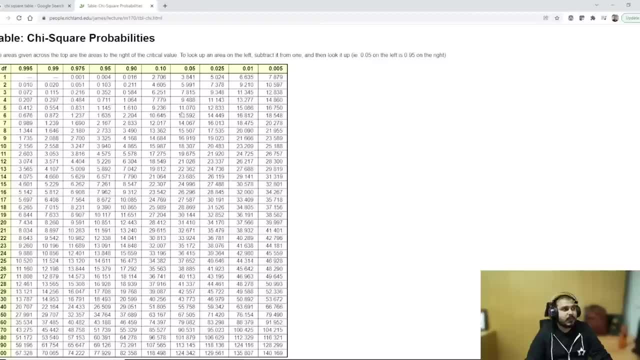 my chi-square table. hope so i get the answer quickly. so df is 2. or to look upon a area on the left, subtract it from the 1.05, see 0.05 is here and degree of freedom is here, so it just becomes 5.991. so over here your we usually mention. 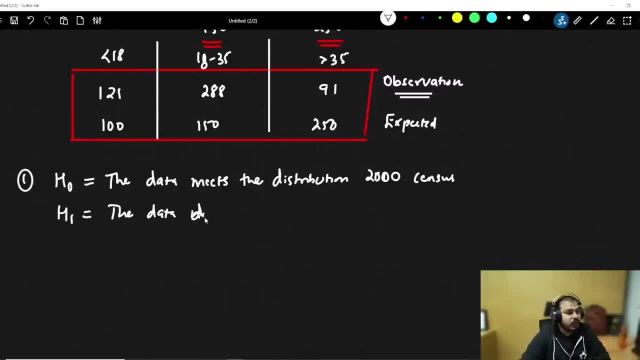 My alternate hypothesis will say that the data does not meet the distribution of 2000 census. So I hope everybody is able to understand the null hypothesis and the alternate hypothesis. Then the second step is my alpha value. My alpha is 0.05.. 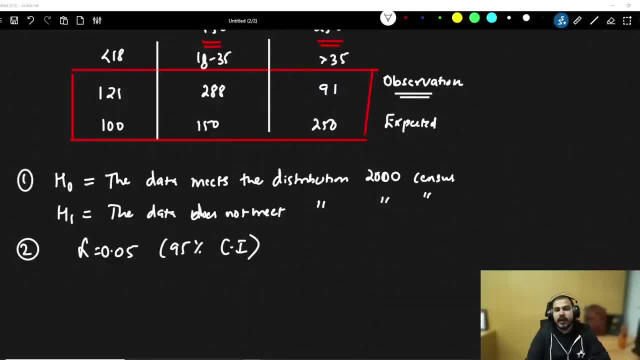 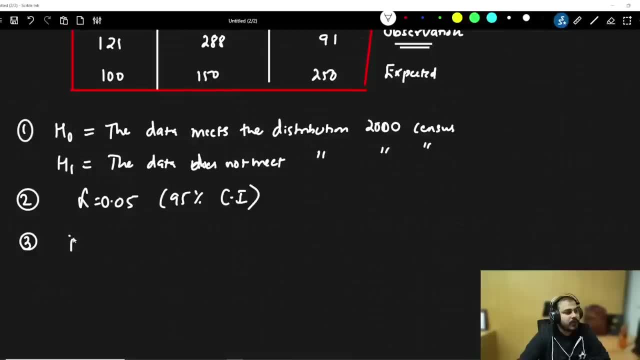 That basically means 95% confidence interval. Now the third step, And this is that whenever we do a chi-square test, we also need to know the degree of freedom. So how do we calculate degree of freedom? This is the steps, guys, and always this will be like this: one n minus one. 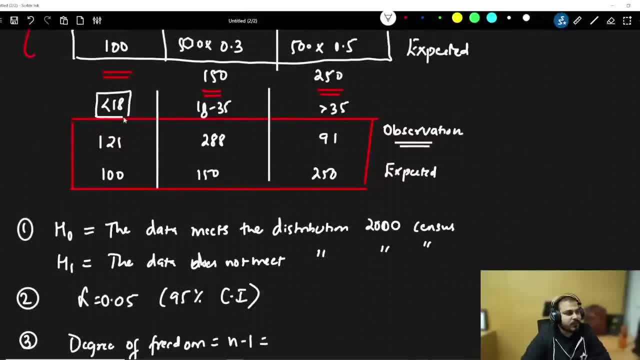 What is n over here? N is nothing, but this is one, two and three. This is where number of categories are coming into picture. Categories are coming into picture One, two and three. So three minus one is basically two. 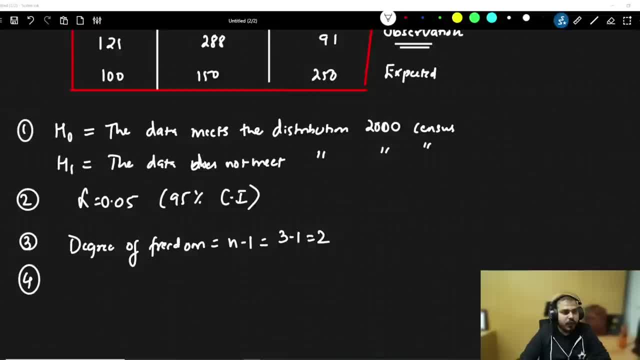 Age is now categorical right, Absolutely, Perfectly. fine, You know your degree of freedom. Your degree of freedom is two and your alpha value is 0.05.. All you have to do is that. go and check in the chi-square table, okay, to find out your decision boundary. 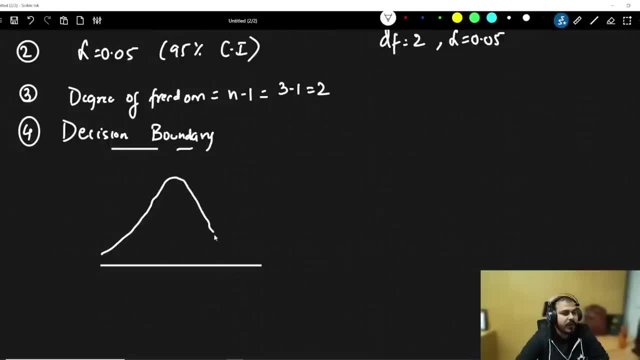 Is this a one-tailed test or two-tailed test? The data may be less than your distribution. It may be more right. So here is this a two-tailed test because alpha is 0.05.. Guys, we have to. 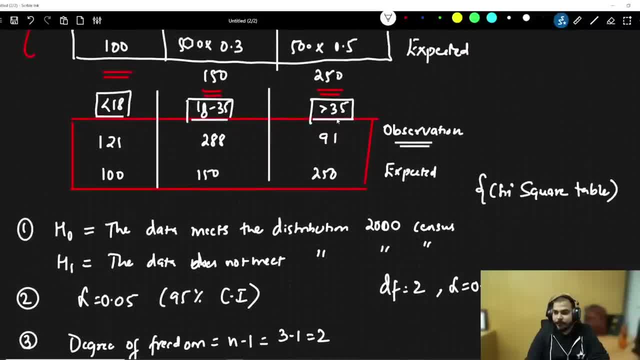 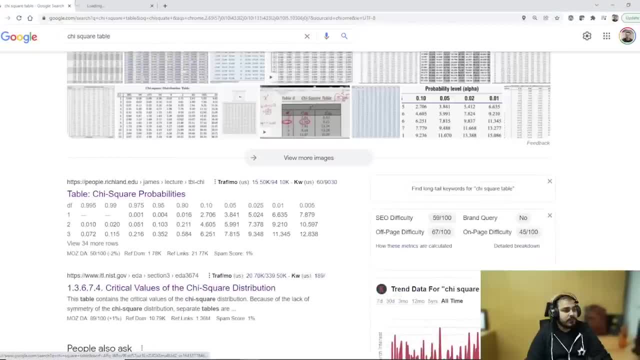 Pick three as n, because there are three age categories. So this will become a two-tailed test. Now, in two-tailed test, all I have to do is that open a chi-square table. Let's see Now, this is my chi-square table. 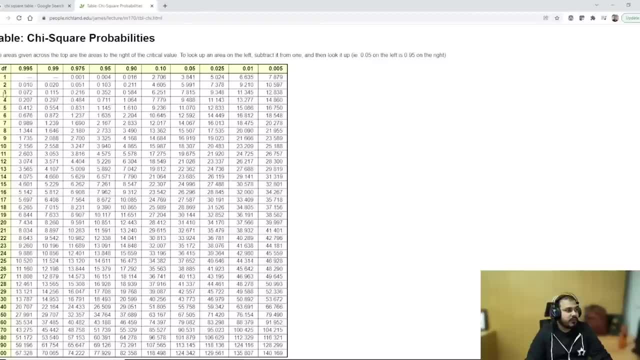 Hope so I get the answer quickly. So df is two. or to look upon an area on the left, subtract it from the one, 0.05.. See, 0.05 is here and degree of freedom is here, So this becomes 5.95.. 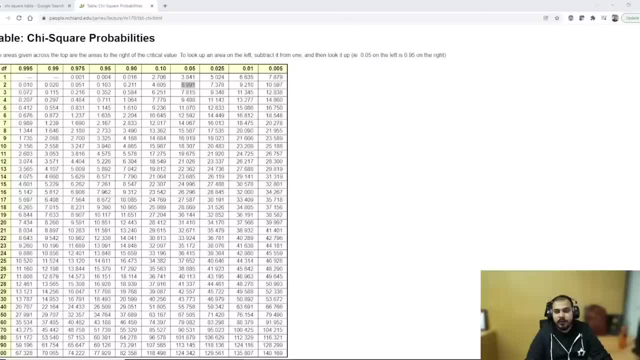 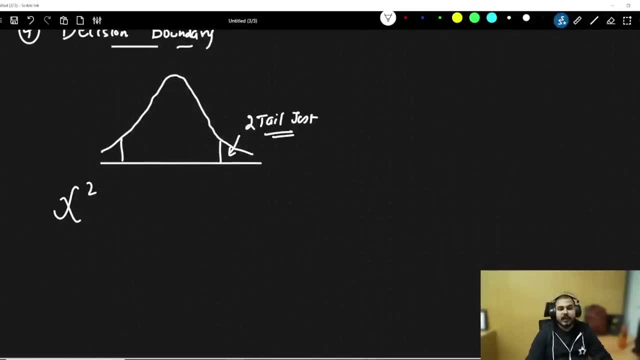 Okay, 0.991.. So over here we usually mention chi-square by x-square and chi-square is basically denoted by x-square, and my decision boundary is that if chi-square is greater than 5.99, I have to reject h0. 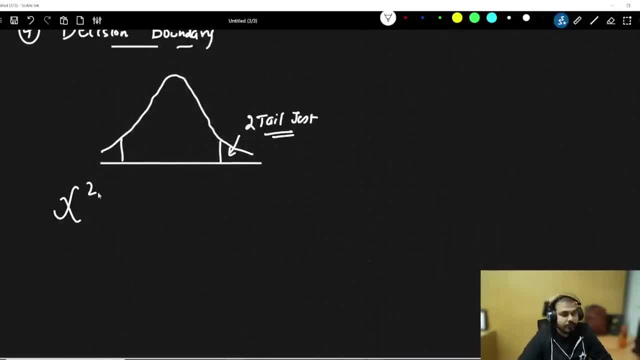 chi-square by x square and chi-square is basically denoted by x square, and the decision boundary is that if chi-square is greater than 5.99, i have to reject a zero. now let's go and compute the chi-square test as usual. very simple definition. so my definition will be that fifth is: calculate the test statistics, which is called a chi-square test. this is nothing, but x square is equal to summation of f0 minus f0.. 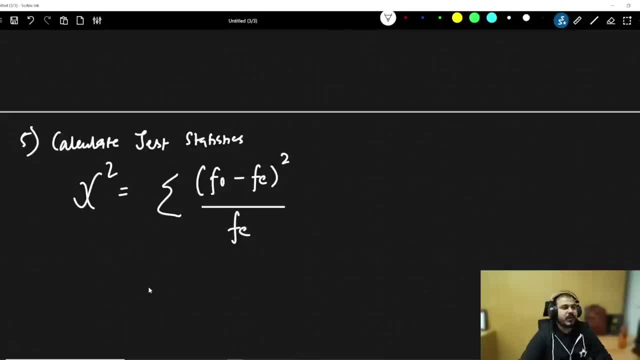 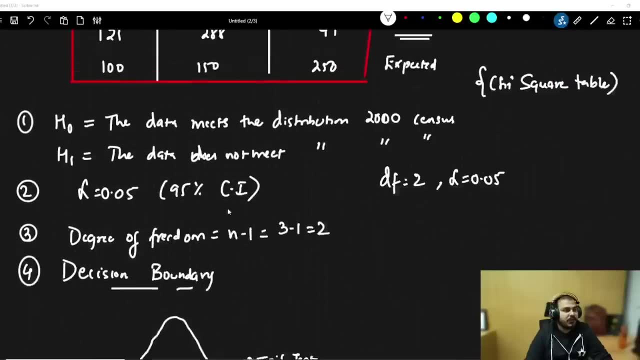 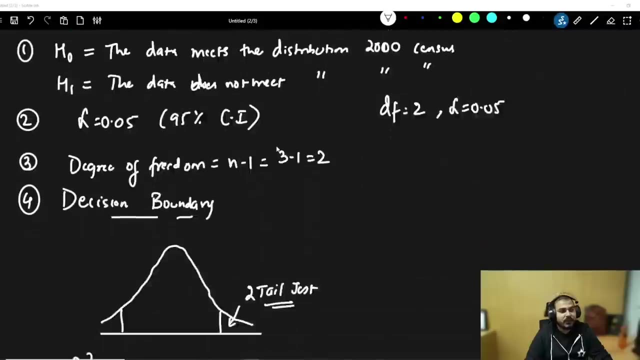 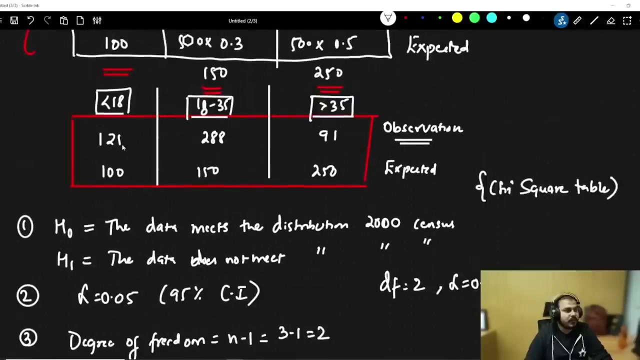 e, whole square divided by fe. again, notation can be used in all different ways, but let me talk about what is f0. f0 basically means observed, okay, observed. fe basically means expected. so i am going to do the summation of all these three values. so here i will first of all write: 121 is my first observed value, see 12100. so 121 minus 100.. 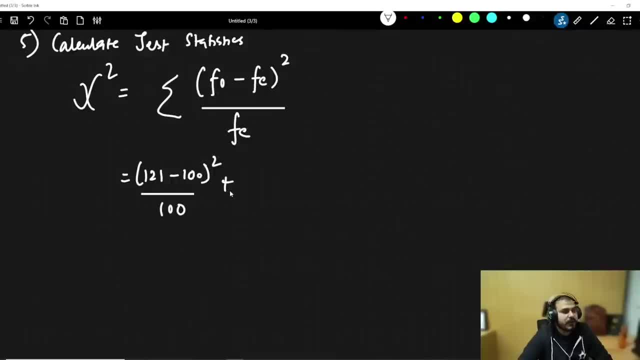 whole square divided by 100. then if i go to the second element over here, you can see 288 minus 150 divided by 150. so 288 minus 150 divided by 150, okay, whole square. then third one will be 91 minus 250, whole square divided by 250. so this will be 91 minus 250.. 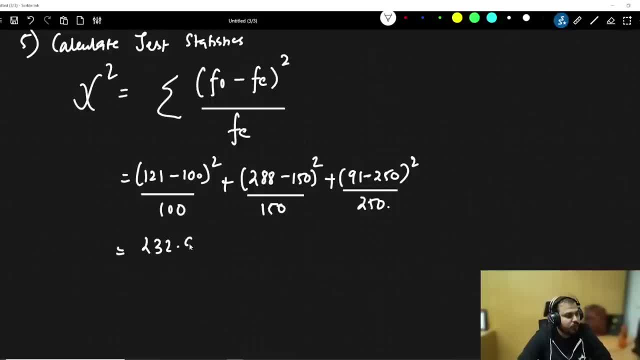 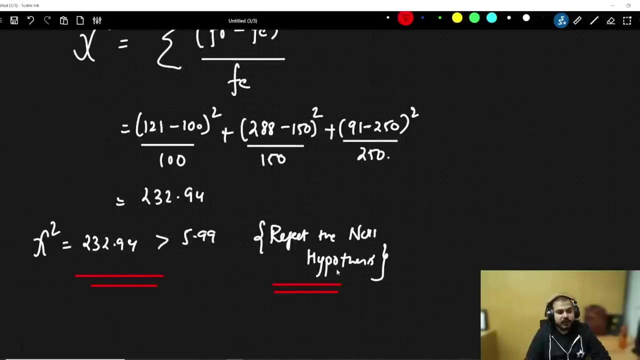 whole square divided by 250: 232.94. that basically means my x square is 232.94, which is obviously greater than 5.99. so what we have to do, we have to reject the null hypothesis, and which is absolutely true, because the population distribution has changed. so 232 is greater than 5.99. so we are rejecting the null hypothesis. okay, it is 494.. 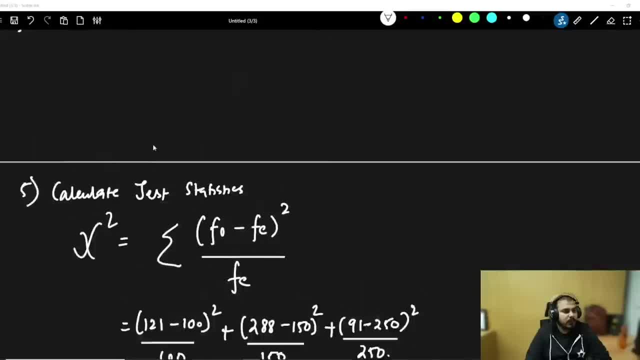 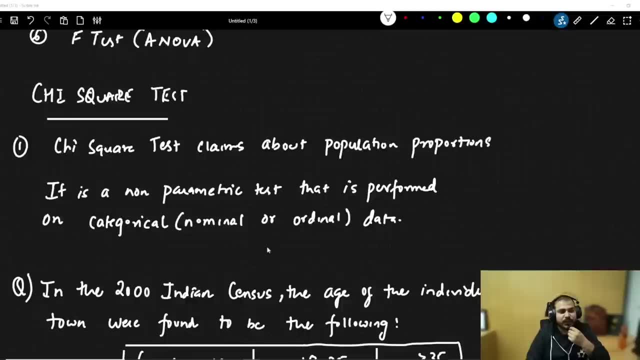 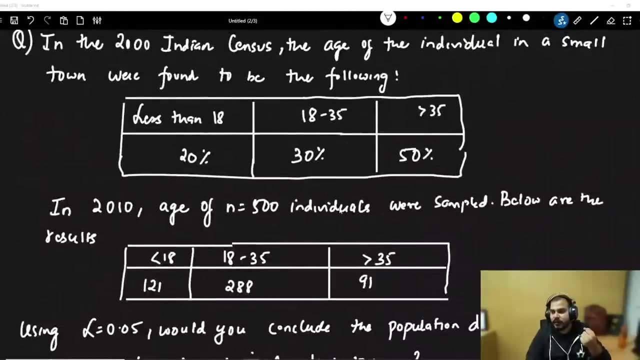 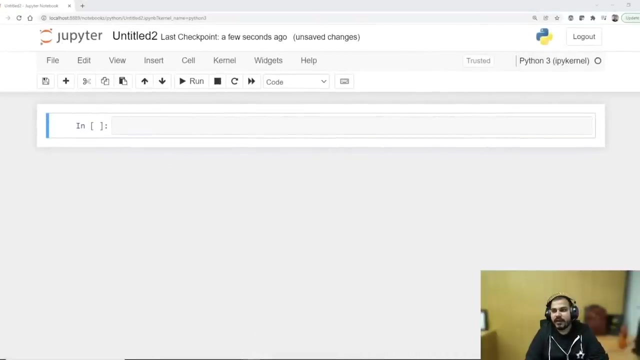 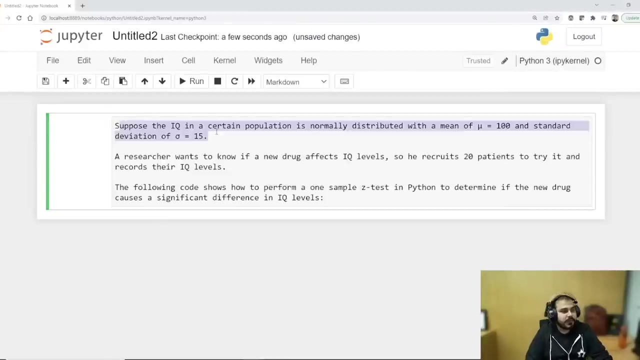 okay, let me write 494.. 494. so if you want to define chi square, it claims about population proposition. you can just say that it is a non parametric test that is performed on categorical, nominal or ordinal data. it is specifically applied on nominal or categorical data. okay, let's see one python example. okay, so i am just opening this. okay, let's say that in my i want to perform z test. okay, so let's say that i have some values like this. so this is my question: suppose the iq value is 0.. 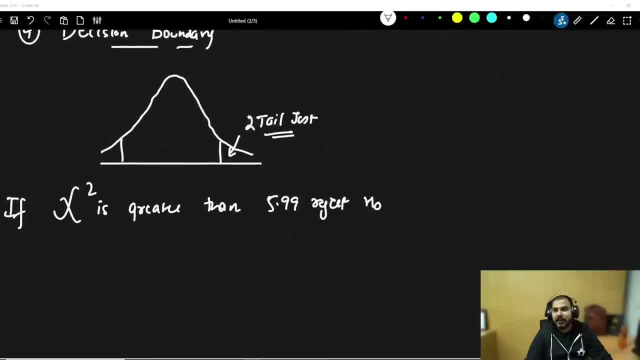 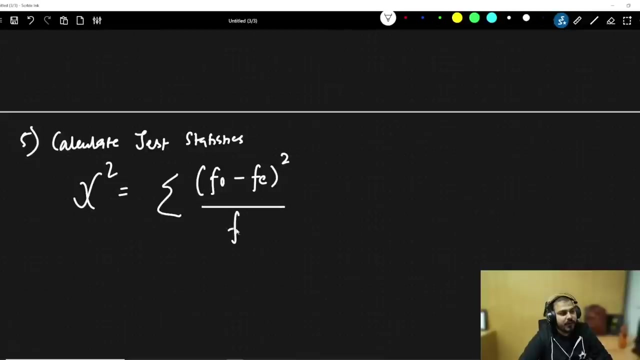 Now let's go ahead and compute the chi-square test. as usual, Very simple definition, So. So my definition will be that fifth is calculate the test statistics, which is called a chi-square test. This is nothing but x-square is equal to summation of f0 minus fe, whole square divided by fe. 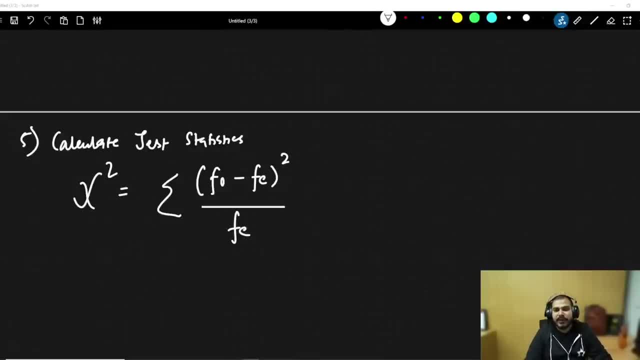 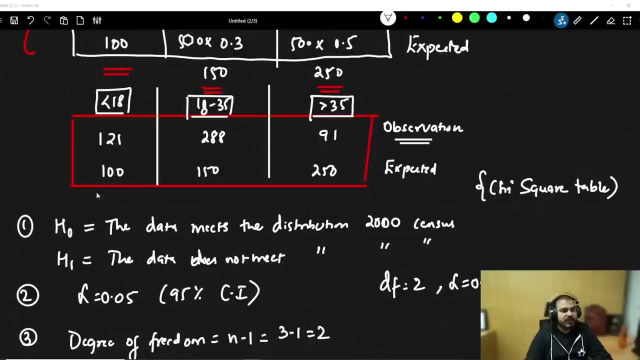 Again, notation can be used in all different ways, But let me talk about what is f0.. F0 basically means observed, Okay, Observed. Fe basically means expected, So. So I am going to do the summation of all these three values. 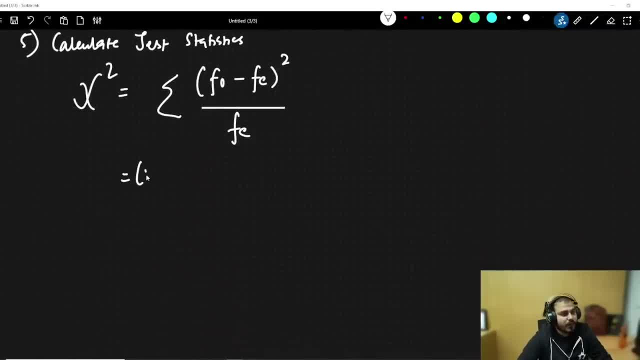 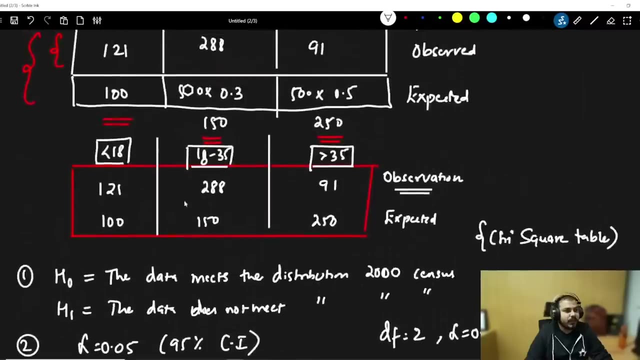 So here I will first of all write: 121 is my first observed value. See 121, 100.. So 121 minus 100, whole square divided by 100.. Then if I go to the second element over here, you can see 288 minus 150 divided by 150.. 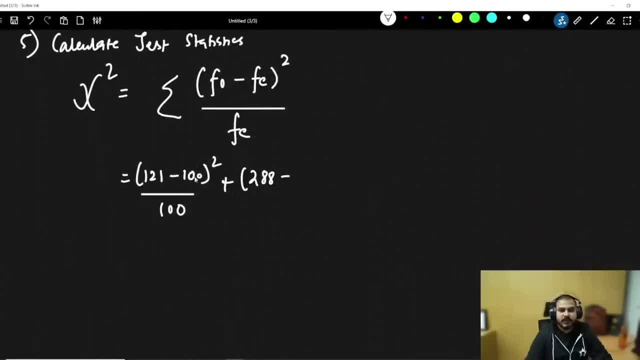 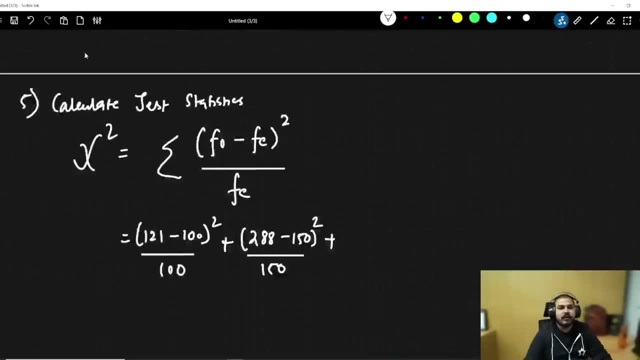 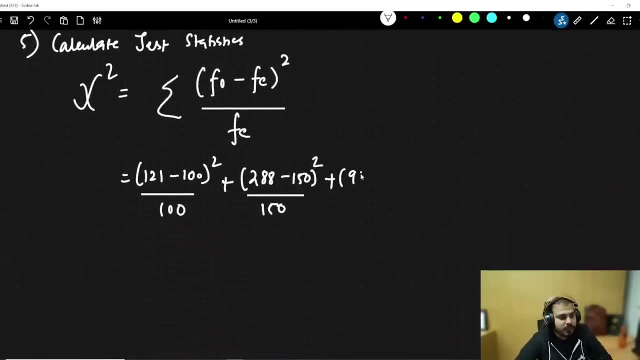 So 288 minus 150.. Okay, whole square. Then third one will be 91 minus 250 whole square divided by 250.. So this will be 91 minus 250, whole square divided by 250, 232.94.. That basically means my x-square is 232.94,, which is obviously greater than 5.99.. 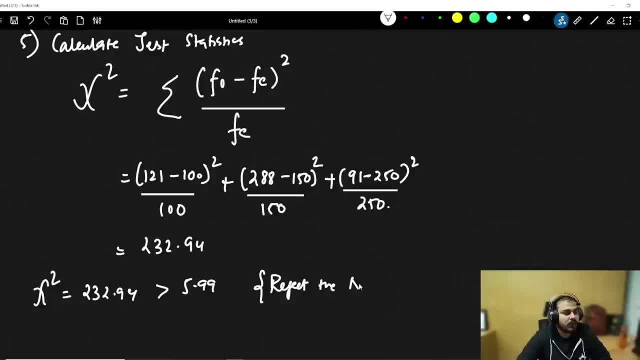 So what we have to do, We have to reject the x-square. So what we have to do, We have to reject the x-square. So what we have to do, We have to reject the null hypothesis, and which is absolutely true, because the population distribution has changed. 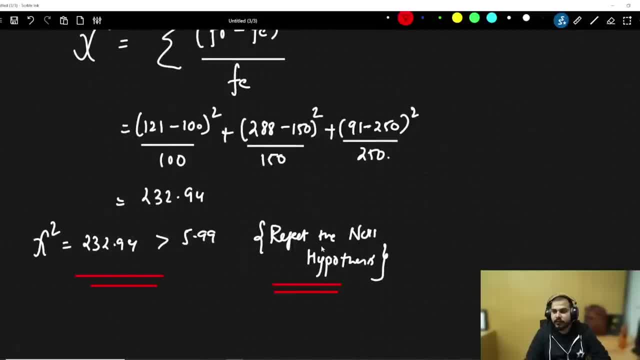 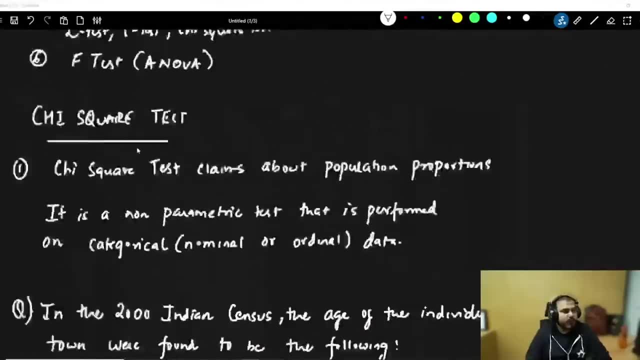 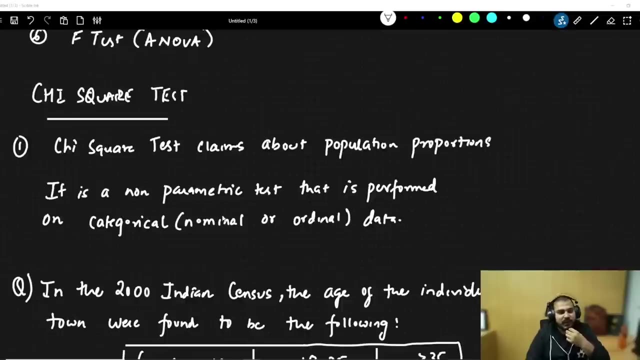 So 232 is greater than 5.99.. So we are rejecting the null hypothesis. Okay, it is 494.. Okay, let me write 494.. So if you want to define chi-square- it claims about population proportion- You can just say that it is a non-parametric test that is performed on categorical, nominal or ordinal data. 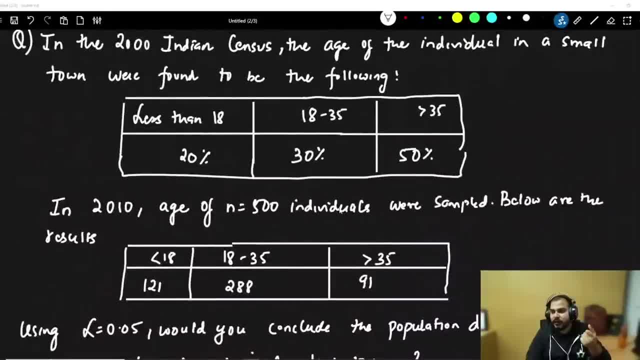 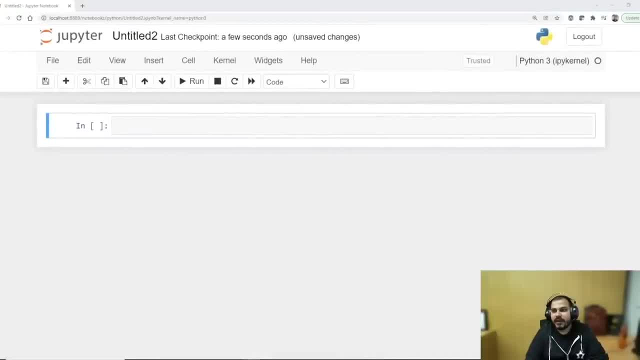 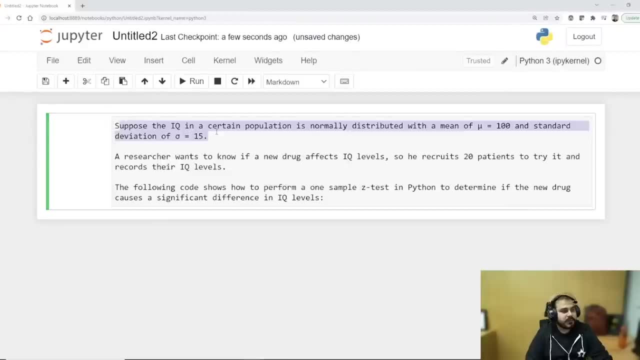 It is specifically applied on nominal or categorical. Okay, let's see one python example. So I am just opening this. So let's say that in my, let's say, I want to perform z-test. So let's say that I have some values like this: 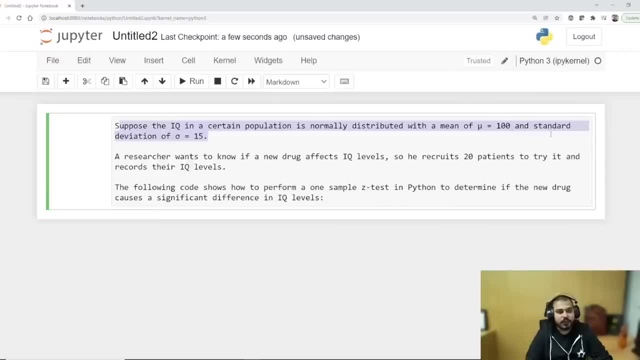 okay, let me write 494.. okay, let's say that in my i want to perform z test. okay, so this is my question. suppose the iq value is 0.. okay, let me write 494.. okay, let me write 494.. okay, let me repeat this: iq value in certain population is normally distributed with a mean of mu is equal to hundred and standard deviation of 15. a researcher wants to know if a new drug affects iq level, so he recruits 20 patient to try it and record the iq level. now i am going to show you the code in python to determine if the new drugs causes a significant effect or not. so i am just going to execute this and let's say that i have this: 20 records for z test. we use this library, which is called as stat models, dot, stach, dot, weight, stat, import, z test, as z test. so this will be the z test of the new drugs. 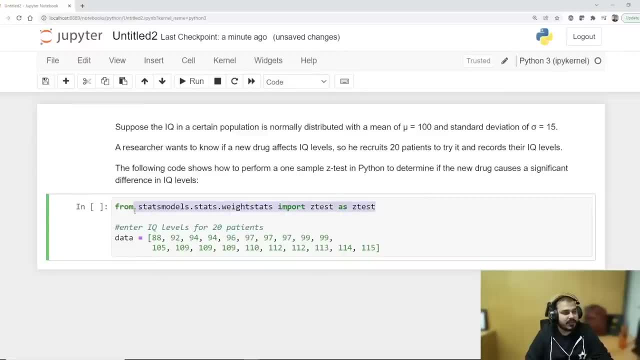 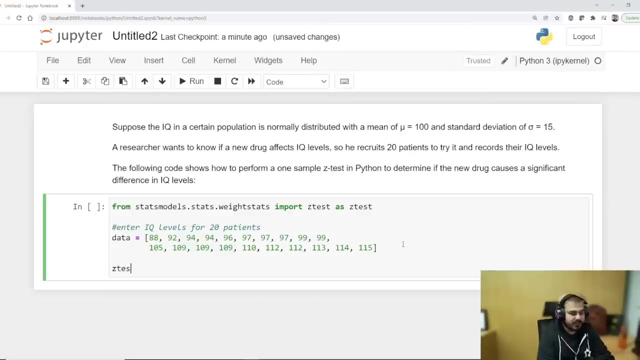 okay, let me write 435.. okay, let's see this. okay, let's see this. these are my 20 patients and i have recorded their iq after the medication is basically applied. now, in order to apply z test, no need to do that much calculation, just write z test and here, just. 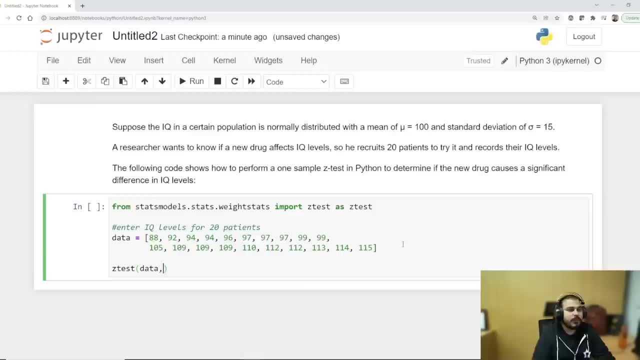 give the data and the next parameter that you will probably be giving is, uh, this iq, that is 100. okay, which which you are actually trying to compare, to basically reject a null hypothesis or not. in this, the null hypothesis will: be mean is equal to 100, mean is not equal to 100. now, when 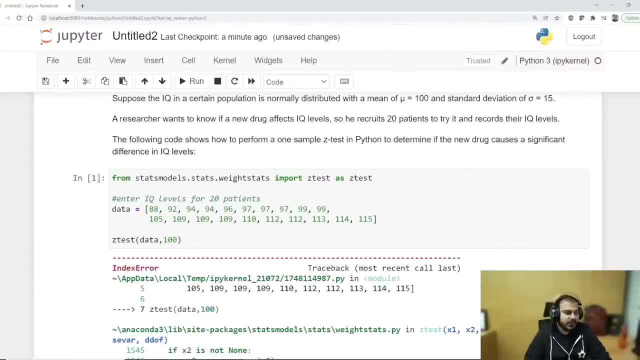 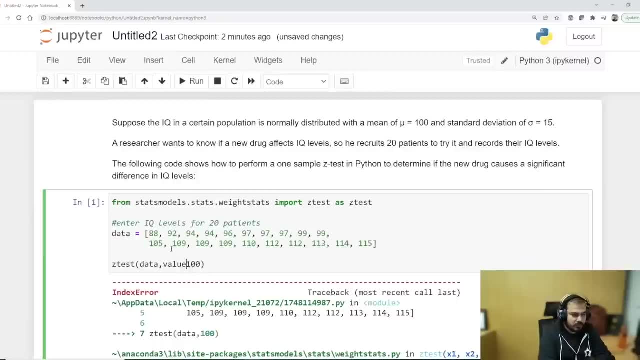 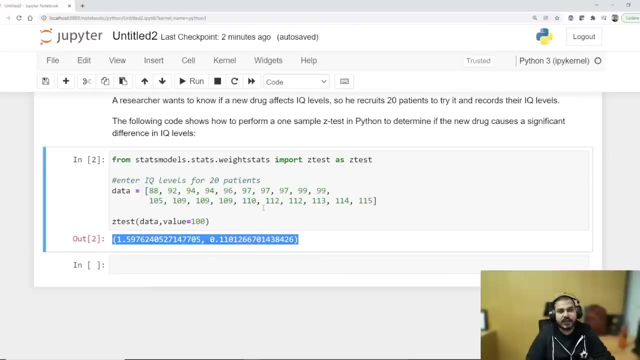 you execute this now here. let's consider that i think the library is not there. or tuple index, tuple index. what is the problem? value is equal to 100. i have to write, so here let's consider that my alpha value is: see, let's see this. these are the two values that i'm getting. the first value: 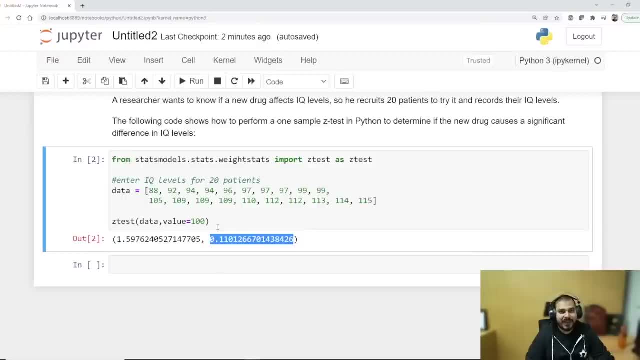 is the z test value. the second value is the p value. what does this p value basically mean? now, many people were asking the difference between significance and p value. you In Z-test they try to give us some kind of p-value. here they also give the Z-test value. 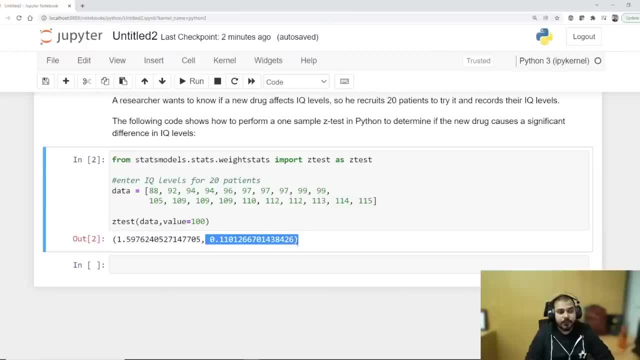 the Z-score that you are able to see is here, and this p-value. This p-value can be used along with significance value, and suppose right now the p-value is 0.001, let's say that 0.11.. 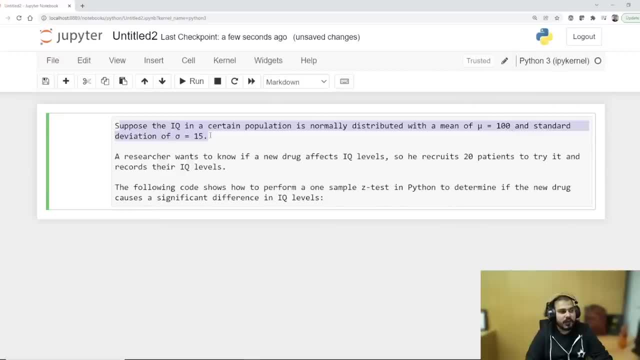 So this is my question: Suppose the IQ in certain population is normally distributed, with a mean of mu is equal to 100 and standard deviation of 15. A researcher wants to know if new drop affects IQ level, So he recruits 20 patient to try it and record the IQ level. 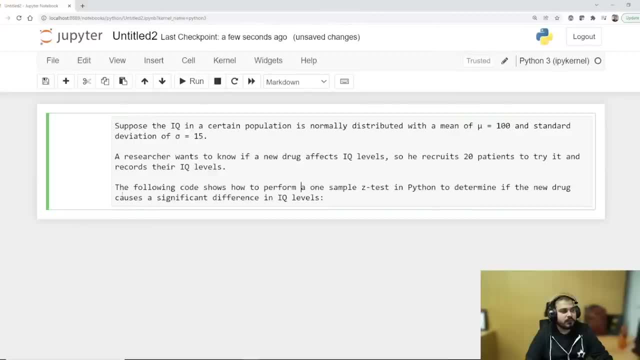 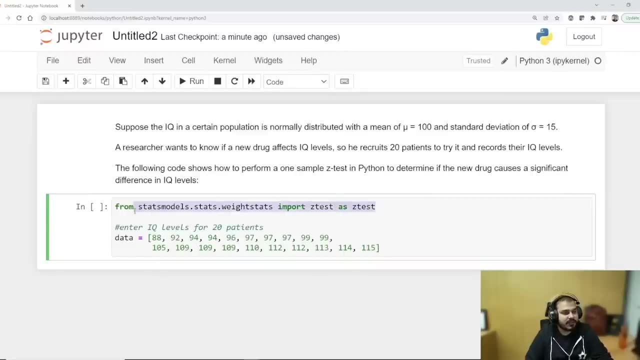 Now I am going to show you the code in python to determine if the new drop will be greater than 50.. drugs causes a significant effect or not. so i'm just going to execute this and let's say that i have this: 20 records for z test. we use this library, which is called, as stat models, dot stats. 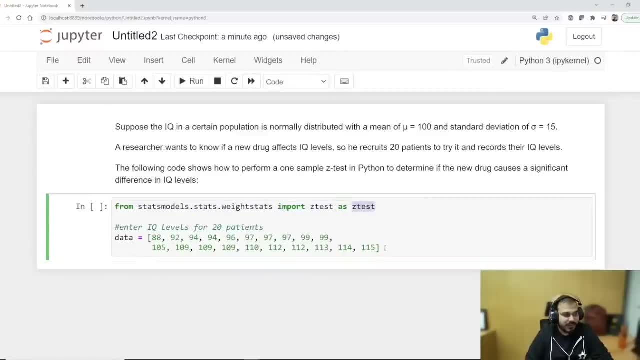 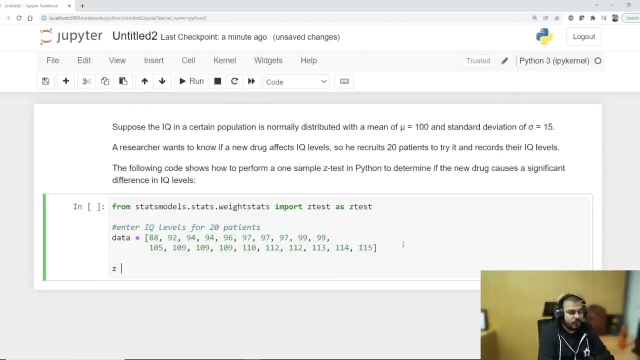 dot weight stats. import z test as z test. so these are my 20 patients and i have recorded their iq after the medication is basically applied. now in order to apply z test, no need to do that much calculation. just write z test and here just give the data and the next parameter that you will. 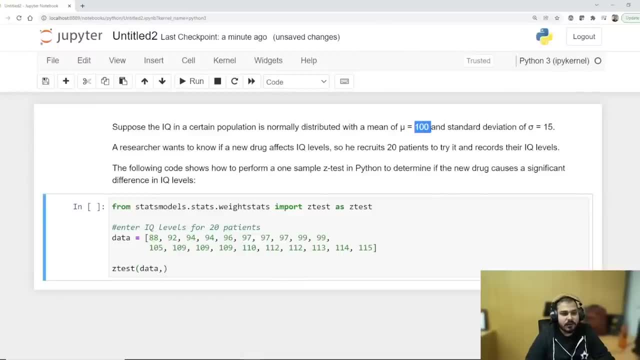 probably be giving is: uh, this iq that is 100. okay, which which you are actually trying to compare, to basically reject a null hypothesis or not? in this, the null hypothesis will: be mean is equal to 100, mean is not equal to 100. now, when you execute this now here, let's consider that i. 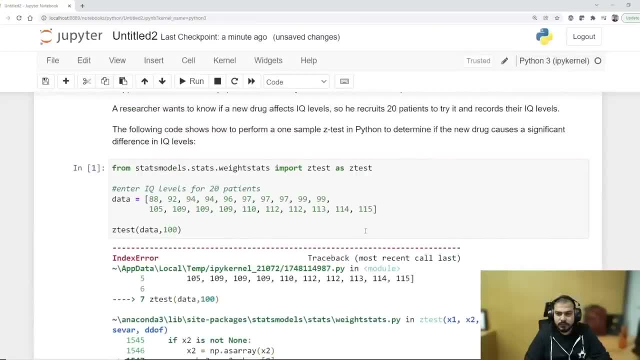 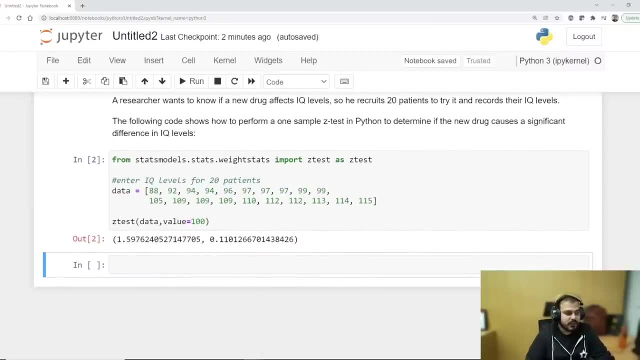 think the library is not there- or tuple index. tuple index: what is the problem? value is equal to 100. i have to write, so here. let's consider that my alpha value is: see. let's see this. these are the tuples. tuples values, two values that I am getting. The first value is the z-test value. The second value is the p-value. 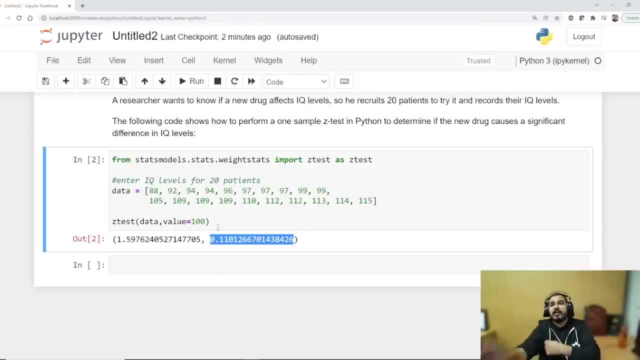 What does this p-value basically mean? Now, many people were asking the difference between significance and p-value. In z-test they try to give us some kind of p-value. Here they also give the z-test value. The z-score that you are able to see is here And this p-value, This p-value. 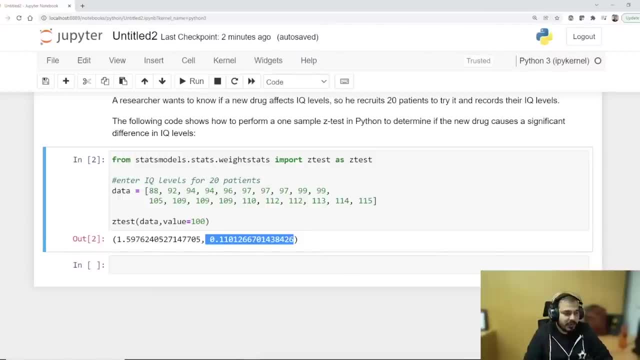 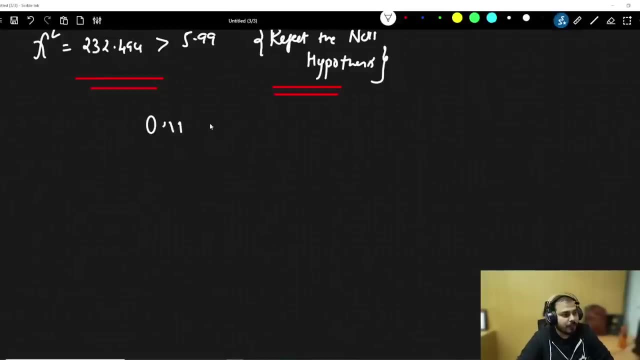 can be used along with significance value. and suppose right now the p-value is 0.001.. Let's say that 0.11.. This 0.11, suppose if it is less than significance level. Now, in this particular case, let's consider that I am going to take a significance level of 0.05.. So if this is less, 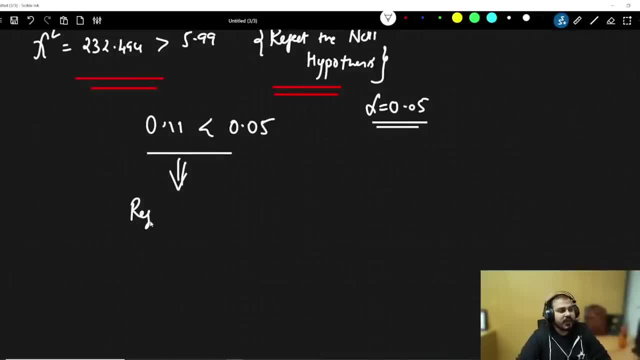 than this, then obviously this: we reject the null hypothesis. This is just saying that, based on this p-value, it is based on the significance level. So if this is less than this, then obviously this is just saying that, based on this p-value, it is based on the significance level. So if this is 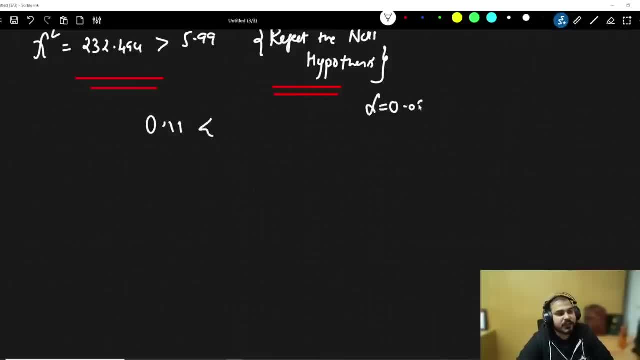 This 0.11, suppose if it is less than significance level. now, in this particular case, let's consider that I am going to take a significance level of 0.05.. So if this is less than this, then obviously this: we reject the null hypothesis. 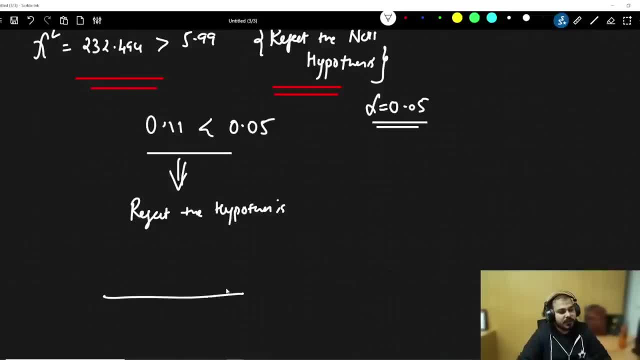 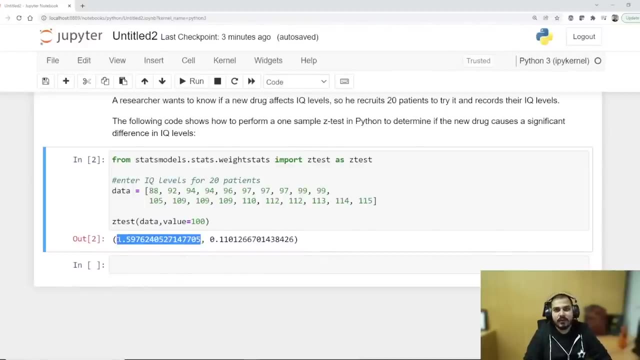 This is just saying that, based on this p-value, it is basically falling in this region. So that is the region. it is less than 0.05.. So it obviously gives two values here. just for understanding purpose, we can definitely use this value and try to do the remaining calculations if you want, because this is 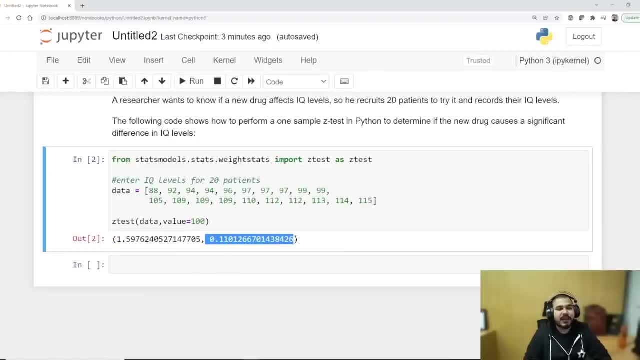 my real job. This is the Z-test value. Other than that, this value will basically help you to compare with the p-value and then decide whether it has got rejected or not. So I can give you the entire code in the ok. since it is 0.11,, this is less than 0.05,. 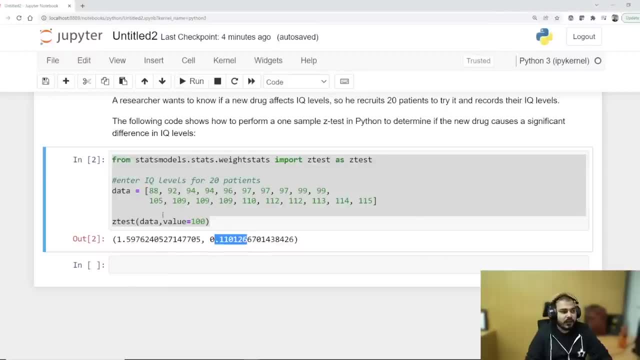 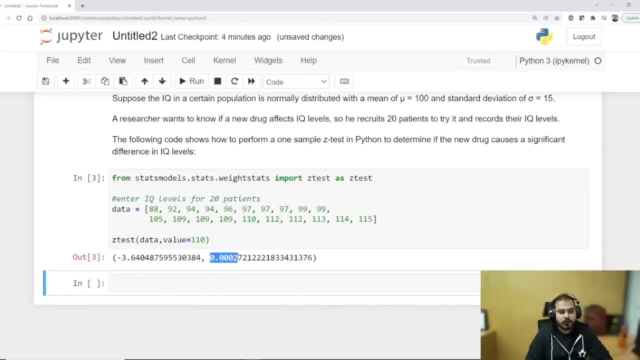 we are going to reject it. Suppose, if we get 0.005, let's say that in this particular case I am going to use the mean as 110.. Now you see, I am getting 0.002.. So do we reject or accept the null hypothesis? 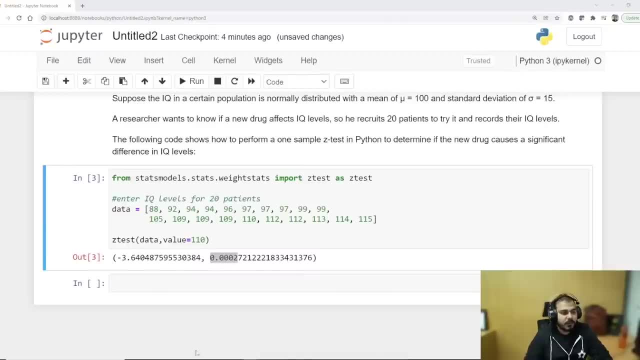 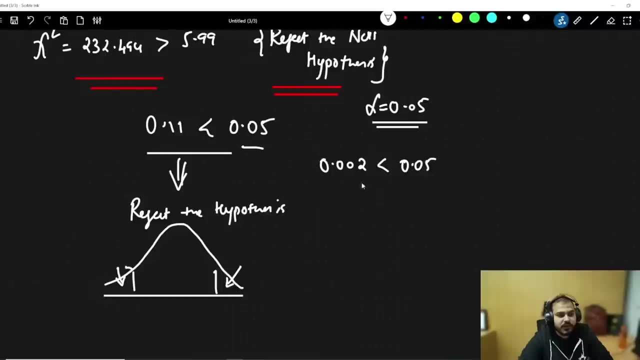 Here. in this particular case, if I go and probably see, you will be able to see I am getting 0.0002, 0.002, which is obviously less than 0.05.. So we accept the null hypothesis. This is obviously not right, not less than so we reject the null hypothesis. 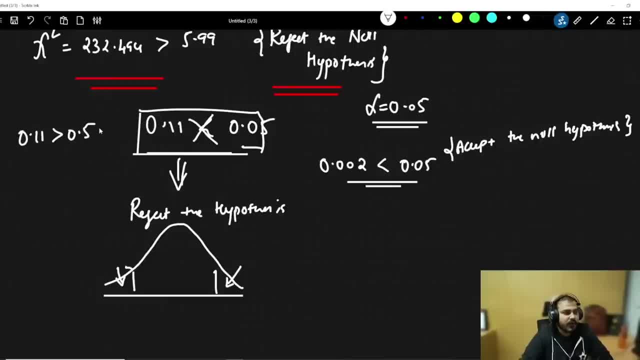 This is not less than 0.11 is greater than 0.05.. So we reject the null hypothesis. Alpha can vary. You can have 0.01.. You can have 0.10.. It depends on the domain. 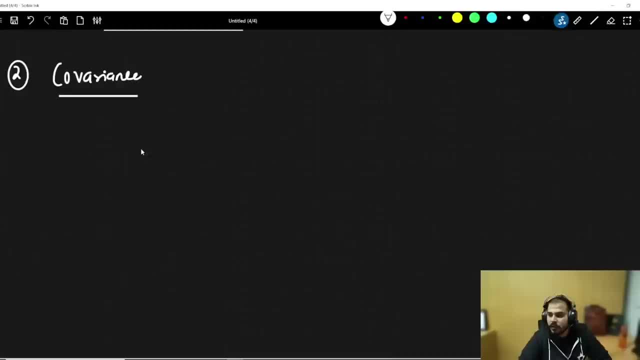 Now let me discuss about the next point, which is called as covariance. Yes, if p-value is less than, if p-value is less than significance value, that basically means it falls in the tail region. So we reject the null hypothesis. If it is greater, then we accept the null hypothesis. 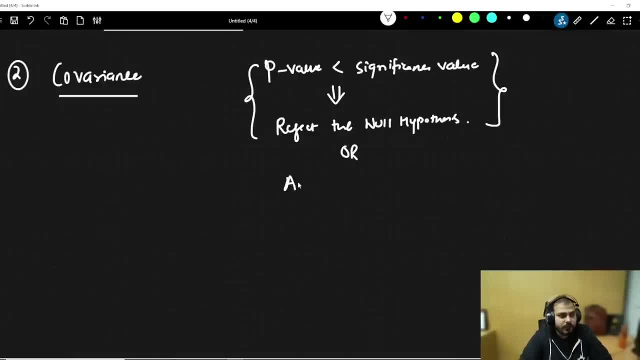 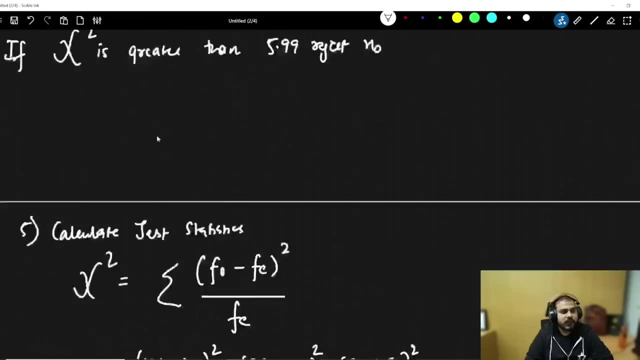 If it is greater we have to accept, Or I will say 0.10.. We accept the null hypothesis. Yes, in medical domain it can be. depending Now, like that you can do for t-test, what all data you require. 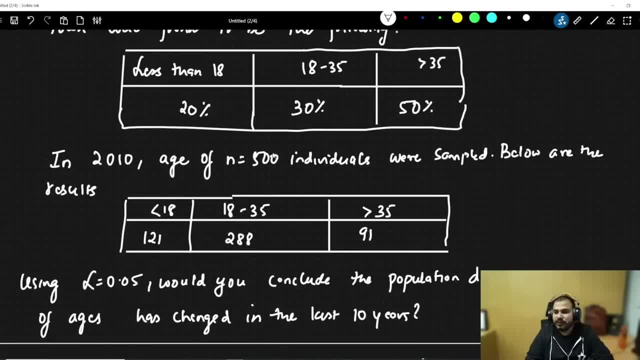 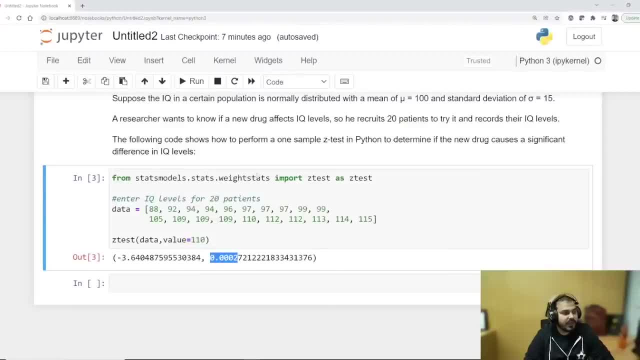 See, whatever a question I am writing with respect to this, that kind of data you require Now in this case also, when I gave this problem statement, when I gave this problem statement here. you can see that, right, I have written the same type of question. 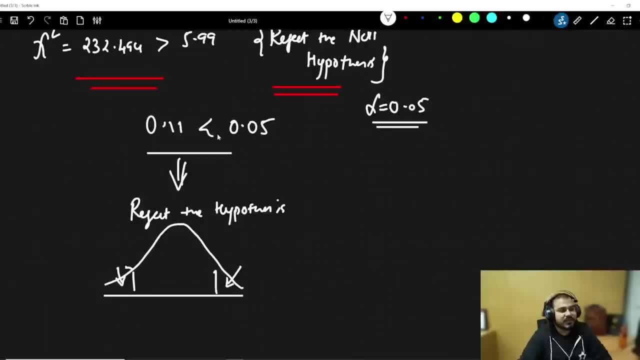 based on this p-value, it is based on the significance level. So if this is less than 0.11, then obviously this is based on the significance level. So if this is less than 0.11, then basically, following falling in this region, So that is the region- it is less than 0.05.. So it obviously gives. 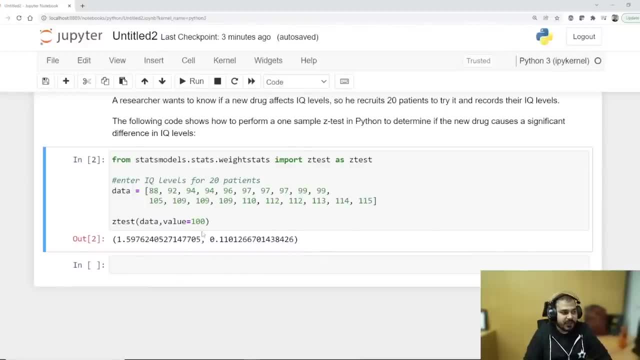 two values Here, just for understanding purpose. we can definitely use this value and try to do the remaining calculations if you want, because this is my real z-test value. Other than that, this value will basically help you to compare with the p-value and then decide whether it has got rejected. 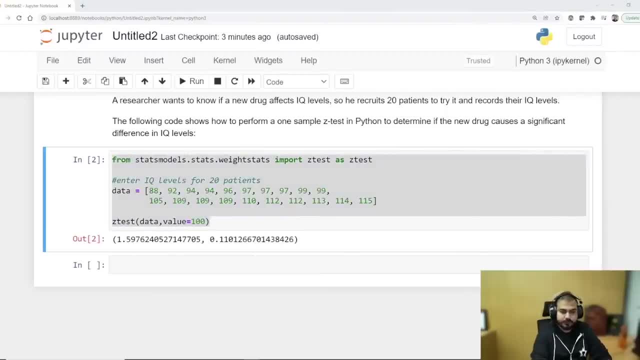 or not. So I can give you the entire code in the okay, Since it is 0.11, this is less than 0.05, we are going to reject it, Suppose, if we get 0.005, let's say that in. 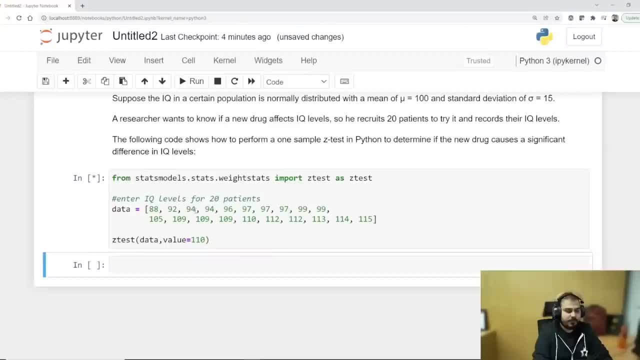 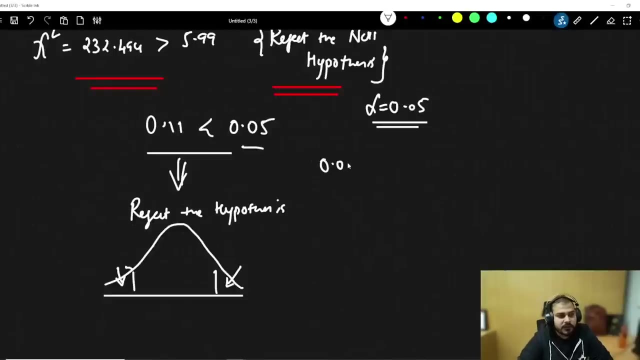 this particular case, I am going to use the mean as 110.. Now you see I am getting 0.002.. So do we reject or accept the null hypothesis Here in this particular case? if I go and probably see, you will be able to see I am getting 0.0002.. 0.002, which is obviously less than 0.05.. 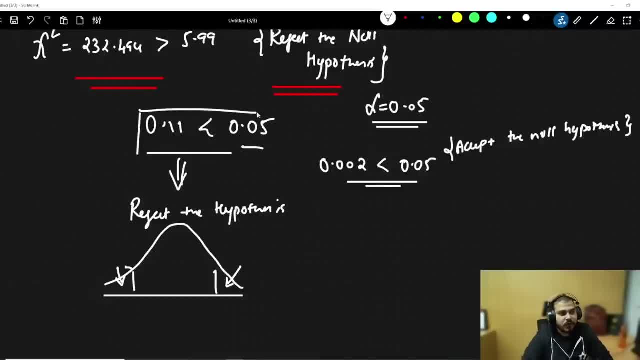 So we accept the null hypothesis. This is: This is obviously not right, not less than so. we reject the null hypothesis. this is not less than 0.11, is greater than 0.05, so we reject the null hypothesis. 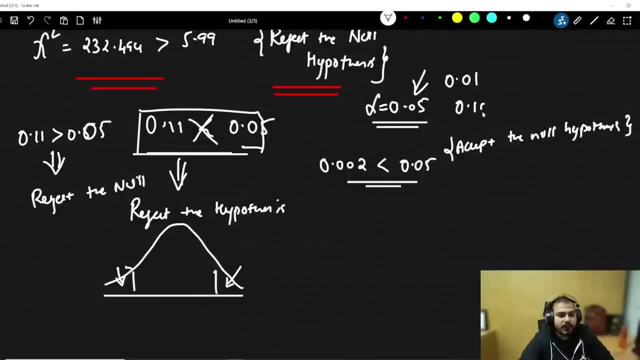 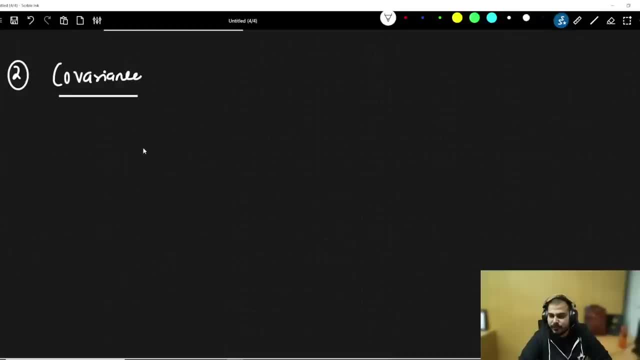 Alpha can vary. you can have 0.01,, you can have 0.10, it depends on the domain. Now let me discuss about the next point, which is called as covariance. yes, if p-value is less than, if p-value is less than significance value, that basically means it falls in the 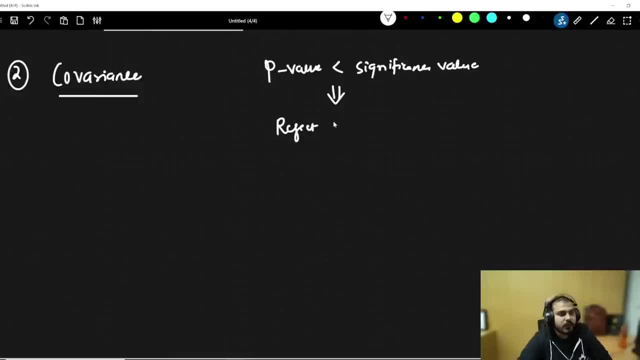 tail region. so we reject the null hypothesis. if it is greater, then we accept the null hypothesis. if it is greater, we have to accept. or I will say: we accept the null hypothesis. yes, in medical domain it can be depending. Now, like that you can do for t-test. 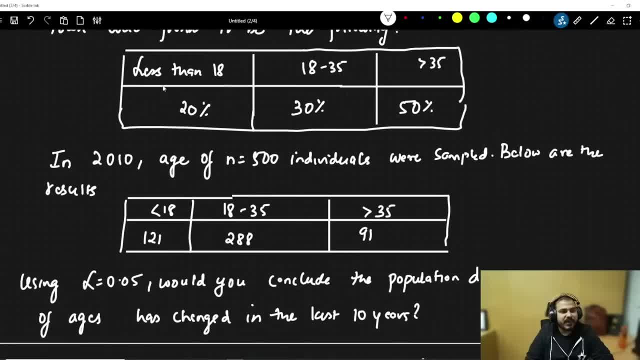 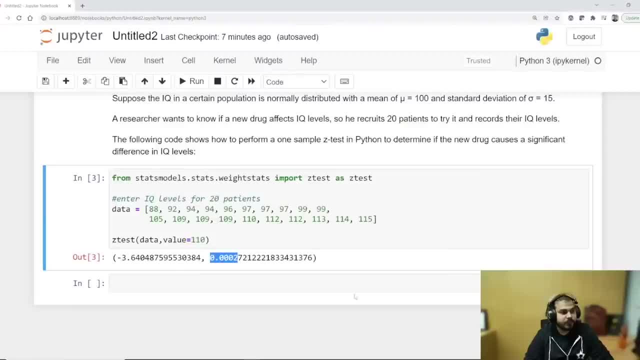 What all data you require. see whatever a question I am writing with respect to this, that kind of data you require now, in this case also, when I gave this problem statement, when I gave this problem statement here. you can see that, right, I have written the same. 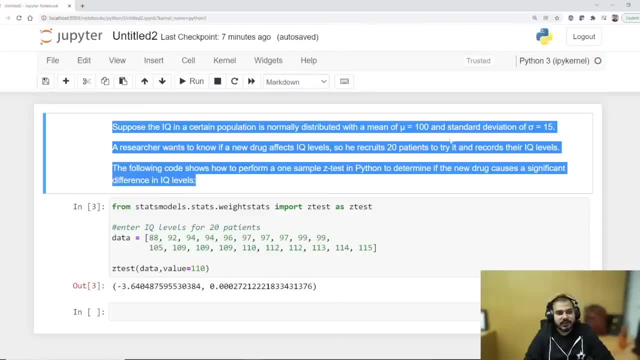 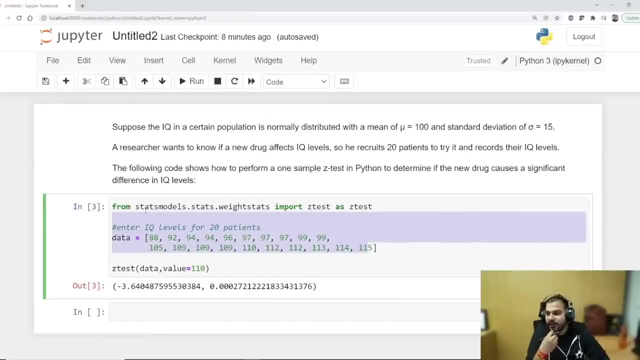 type of question. suppose the IQ in this, this, this, this is there. so it across 20 patient. this is the 20 patient data and I am basically checking out the z-test. so if mean IQ before meditation is 110 and p-value is 0.002.. 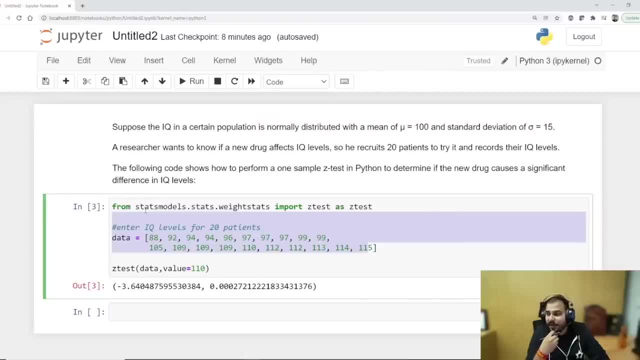 It means that Even after taking medication, the IQ will be around 110, it means medication has no effect. yes, With respect to that specific thing, let's say that it has got. medication has been applied. before, the IQ was 110 and after giving this medicine also, it was near 110,. alpha and significance. 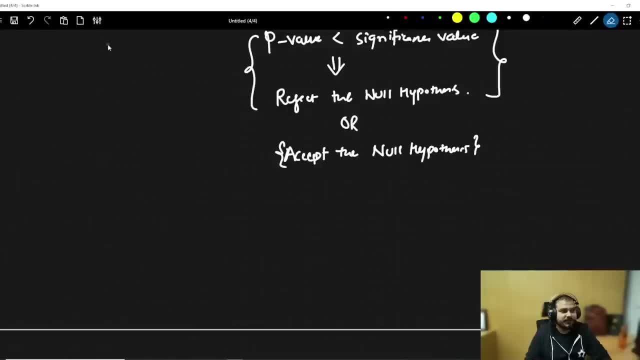 value are one and the same. ok, Let me define once again. this is my graph. ok, this is this. initially, I got 1- 1, this was my p-value. This is obviously greater than p-value. This is obviously greater than 0.05.. 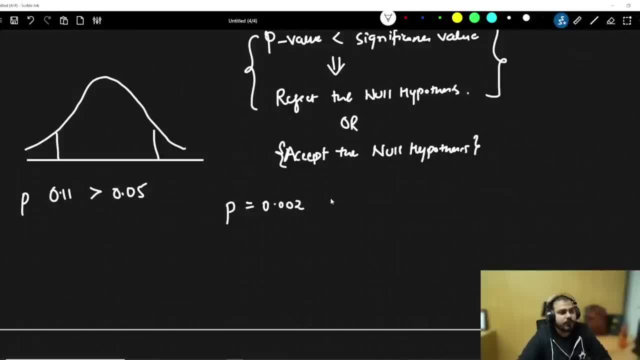 And let's consider about p-value as 0.002, which is less than 0.05.. When I have this scenario, this basically means I am in the confidence interval. If I am having this scenario where it is greater than 0.05, I am falling in this in the tail. 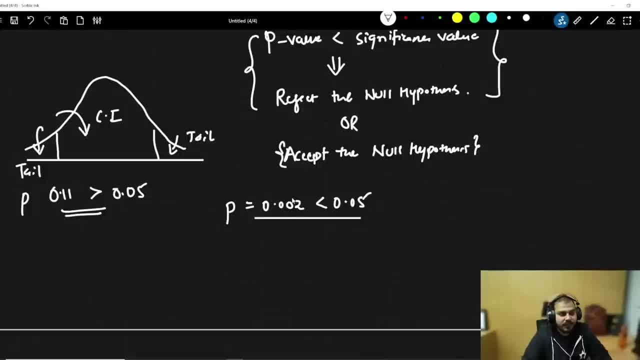 region. I hope now you are able to understand If I am having this scenario where the p-value is less than significance value. I am in the confidence interval In this 95%. if I am over here, that basically means it is greater than the significance. 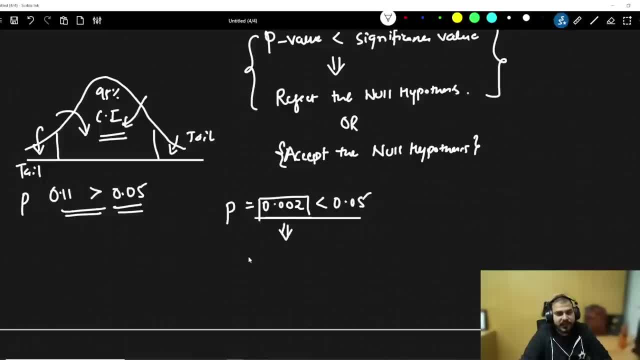 level: Yes, if p-value is less than we do not reject, right. In this case, we accept the null hypothesis. We fail to reject the null hypothesis. We accept null hypothesis. ok, In this particular case, we reject. 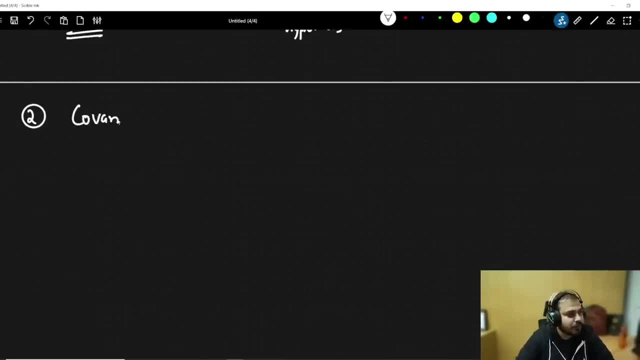 Now let's go ahead and discuss about the next topic, which is called as covariance. Let's say that I have two data sets, two columns- Ok, X and Y. So if I have these two columns, let's say that this is basically my weight and this 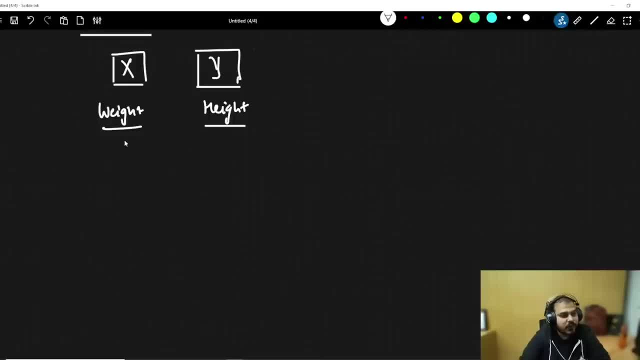 is basically my height feature. ok, In this particular scenario, let's consider that you have some weights. Let's say you have like 50, you have height like 160 cm, then you have 60,, 170 cm, then you have 70,, then you have 180 cm and then probably you have 175,, you have 181 cm. 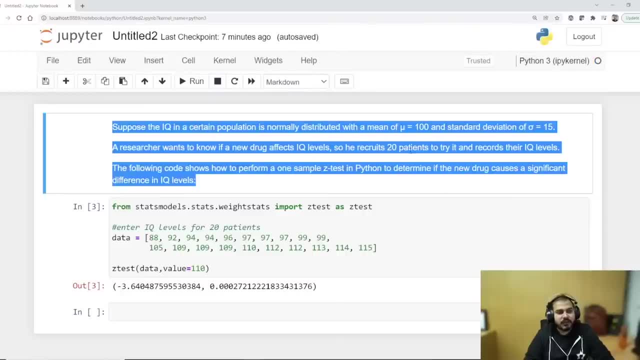 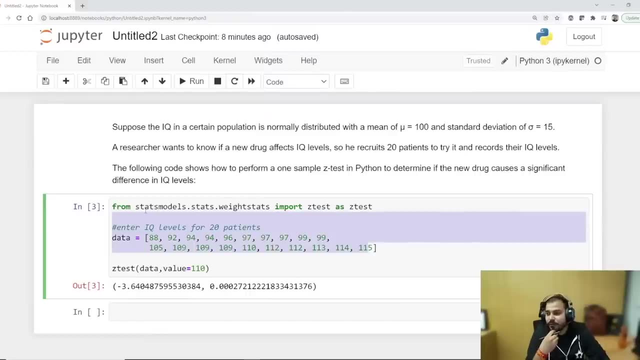 Suppose the IQ in this, this, this, this is there. So you reproach 20 patients. This is the total. It will be 10,000.. Alright, the 20 patient data, and i am basically checking out the z test. so if mean iq before meditation. 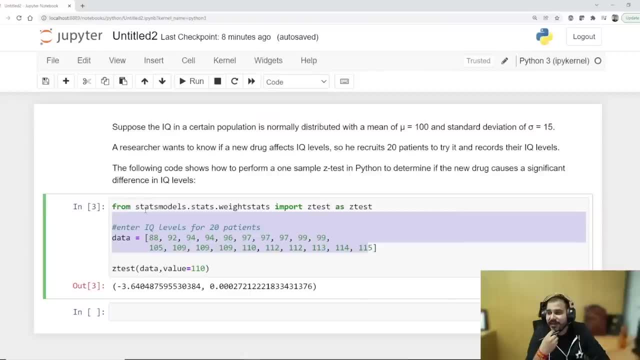 is 110 and p value is 0.002. it means that even after taking medication, the iq will be around 110. it means medication has no effect. yes, with respect to that specific thing, let's say that it has got. uh, medication has been applied. before the iq was 110 and after giving this medicine also it 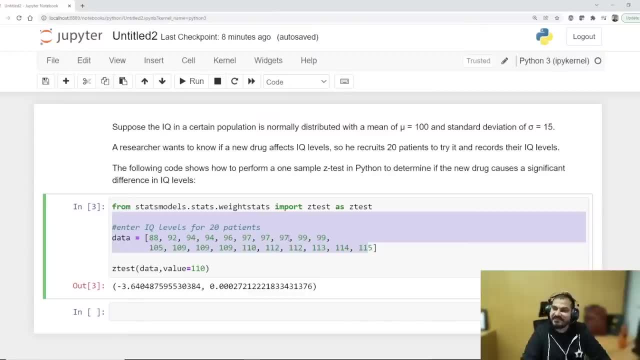 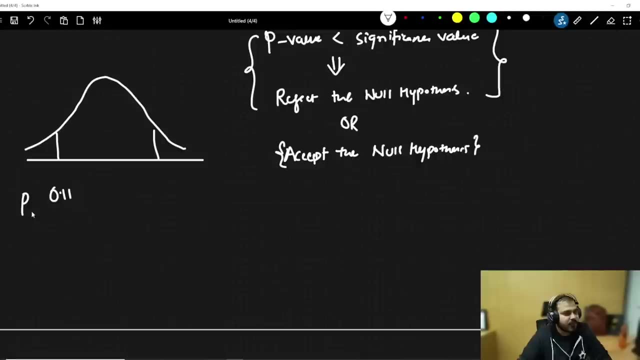 was near 110. alpha and significance value are one in the same. okay, let me define once again. this is my graph. okay, this is this. initially, i got 1- 1. this was my p value. this is obviously greater than 0.05, and let's consider about p value as 0.002, which is less than 0.05. when i have this scenario, 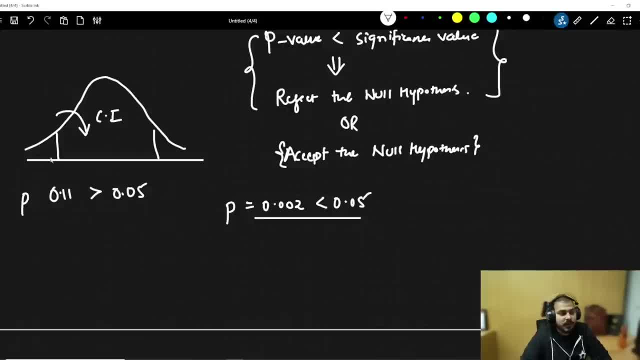 this basically means i am in the confidence interval if i am having this scenario where it is greater than 0.05. i am following this scenario in this in the tail region. i hope now you are able to understand. if i am having this scenario where the p value is less than significance value, i am in the confidence interval in this 95 percent. 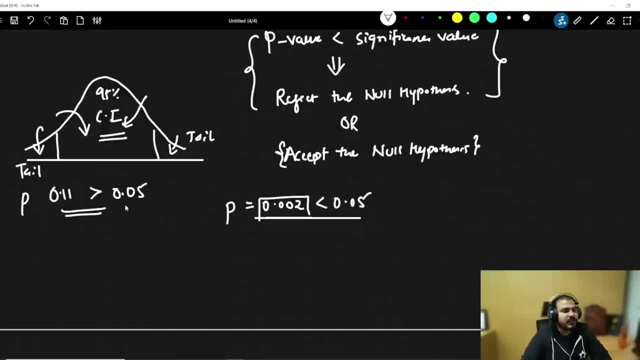 if i am over here, that basically means it is greater than the significance level. yes, if p value is less than we do not reject, right, in this case, we accept the null hypothesis. we fail to reject the null hypothesis. we accept null hypothesis. okay, in this particular case, we reject. now let's go ahead and discuss about the next topic, which. 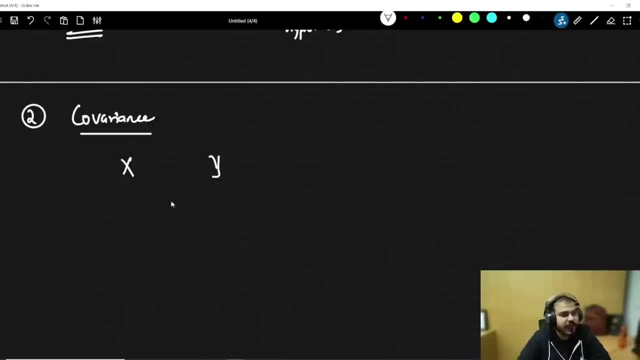 is called as covariance. let's say that i have two data set, the two columns x and y. so if i have these two columns, let's say that this is basically my weight and this is basically my height feature. okay, in this particular scenario, let's consider that you have some weights. let's say you have. 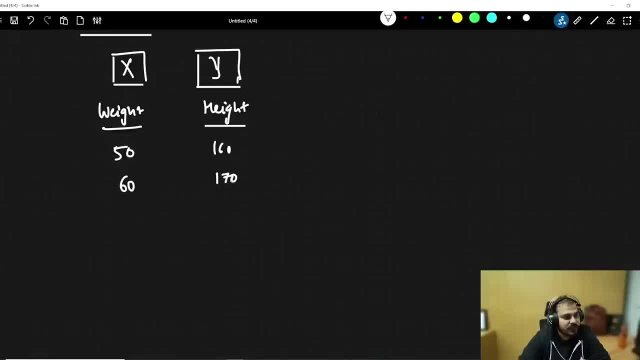 160 centimeters, then you have 60, 170 centimeters, then you have 70, then you have 180 centimeters and then probably you have 175, you have 181 centimeters. now, in this particular thing, you can what, what kind of things you are seeing, what kind of relationship you are seeing when x is. 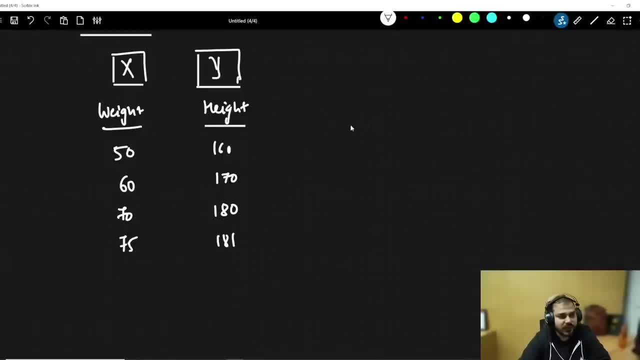 Now, in this particular thing, you can what kind of things you are seeing, What kind of relationship you are seeing. When X is increasing, Y is increasing, And similarly can I say, when X is decreasing, Y is decreasing. So both this relationship will basically follow this specific thing based on this. 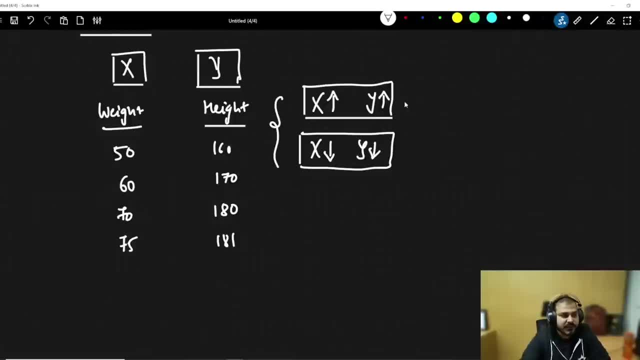 particular data. So when X is increasing, Y is increasing. when X is decreasing, Y is decreasing. Suppose let's say that I have one more data set: weight and height only. Let's say I have- let's consider that- number of hours study and number of hours play. 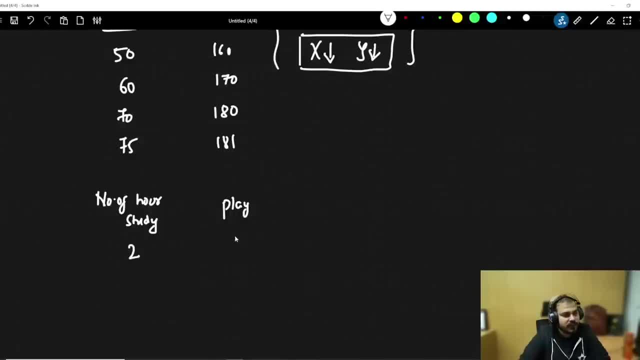 Now, in this particular case, if I am studying for 2 hours, let's say I am playing for 6 hours. if I am studying for 3 hours, I am playing for 4 hours. If I am studying for 4 hours, I am playing for 3 hours. 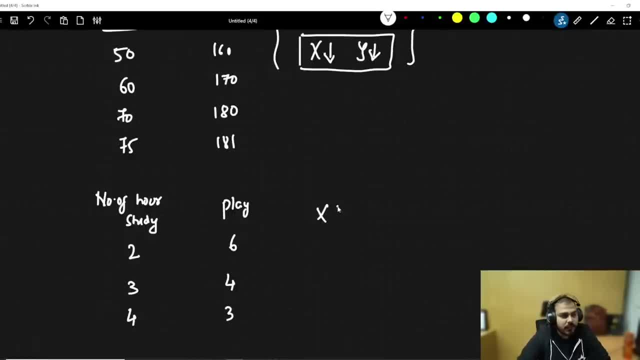 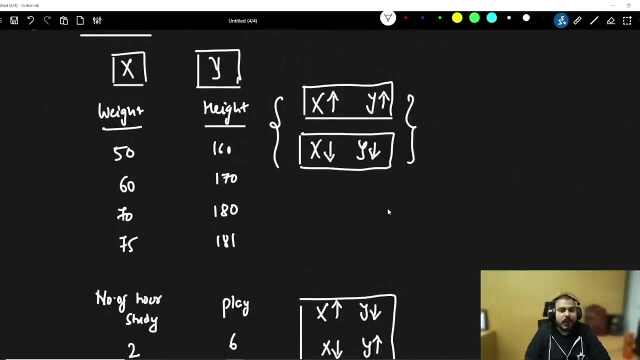 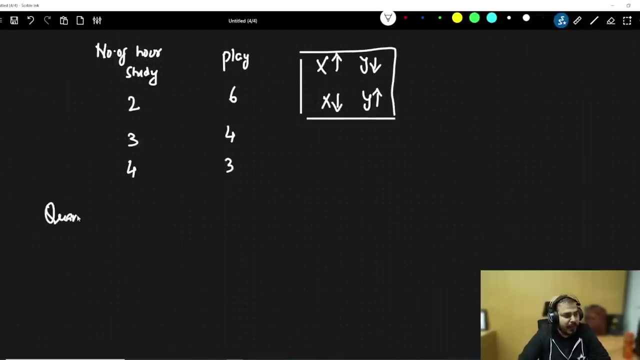 In this particular case, what is the relationship? You can see that when X is increasing, Y is decreasing, or when X is decreasing, Y is increasing is basically used over here. so here you can see these two conditions, right, these two conditions. now, this is what you can observe. but the main thing is that: how do i quantify? how can i quantify? 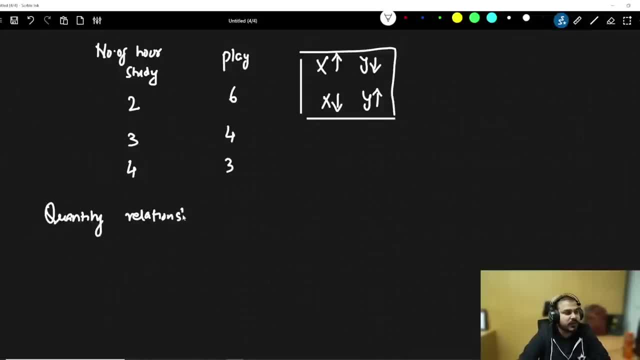 or show some relationship, quantify relationship through numbers between x and y. now, in that particular case, i can use a formula which is called as covariance. now, covariance is basically given by cov, x comma y, which is nothing but summation of i is equal to 1 to n, x of i minus x. 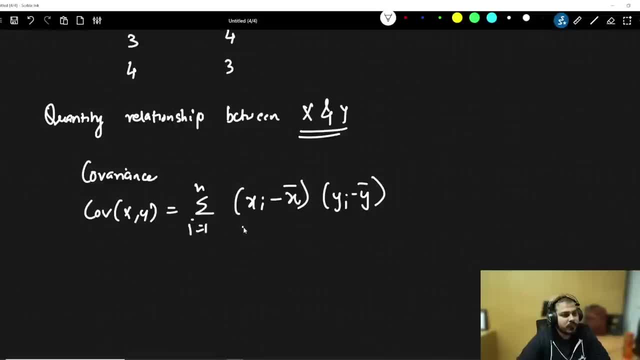 bar y of i minus y bar divided by divided by n. so this is basically the formula with respect to covariance. if you are working with sample again, this would be the formula for covariance. so this is basically the formula for covariance. so this will be n minus 1 right now. let's consider that we are working with sample now in this. 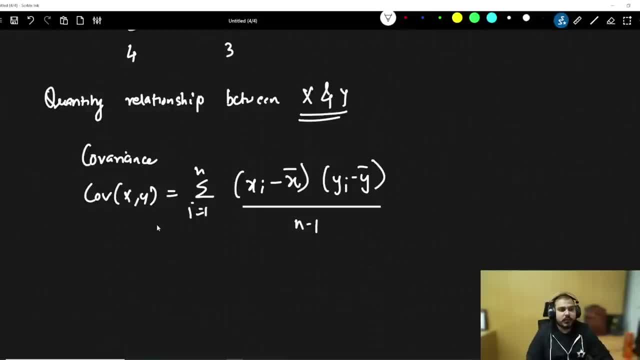 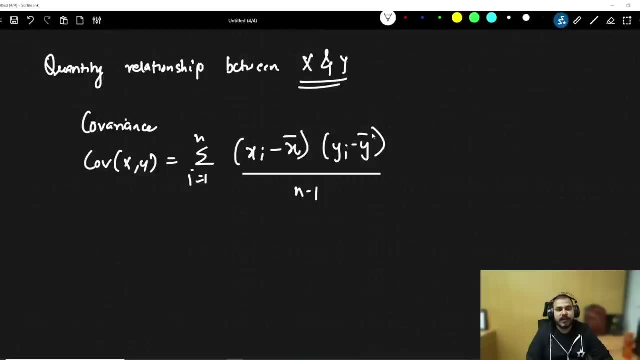 particular case, you can see what is happening. covariance of x comma y, covariance of x comma y is nothing but x minus x bar. x bar is nothing but the mean of x. y minus y bar is y bar is the mean of y. now, when we calculate, you will be able to see either we will get a positive number or a. 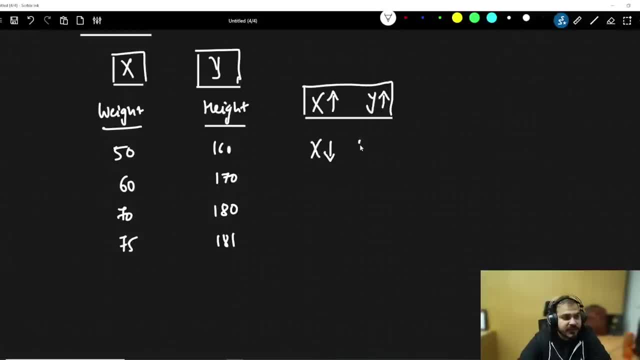 increasing, y is increasing. and similarly can i say: when x is decreasing, y is decreasing. so both this relationship will basically follow this specific thing and this particular data. so when x is increasing, y is increasing. when x is decreasing, y is decreasing. suppose let's say that i have one more data set. 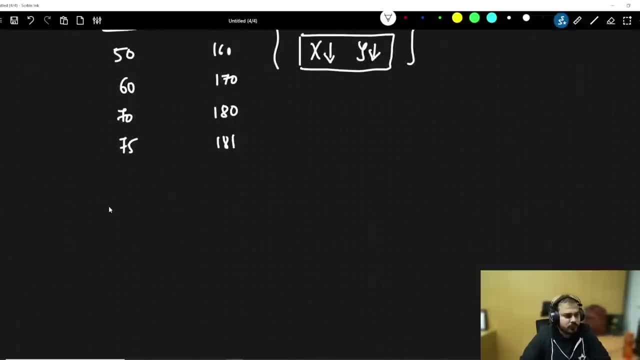 weight and height only. let's say i have- uh, let's consider that number of hours study and number of hours play. now, in this particular case, if i am studying for two hours, let's say i'm playing for six hours. if i'm studying for three hours, i'm playing for four hours. 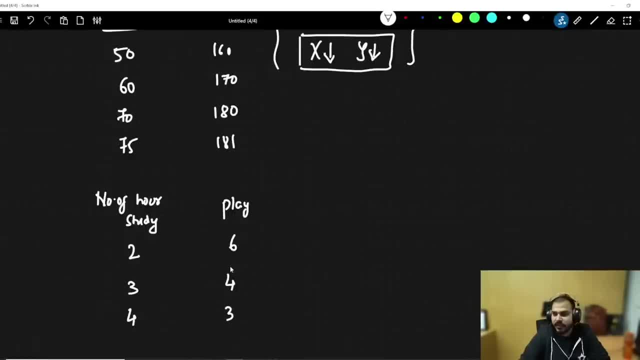 if i'm studying for four hours, i am playing for three hours. in this particular case, Universalhoric-Sag意思ем은 점된 적용. name: 재료 개선 z failing out, which inequality is the place Midst fashion length and microwave meat verification? 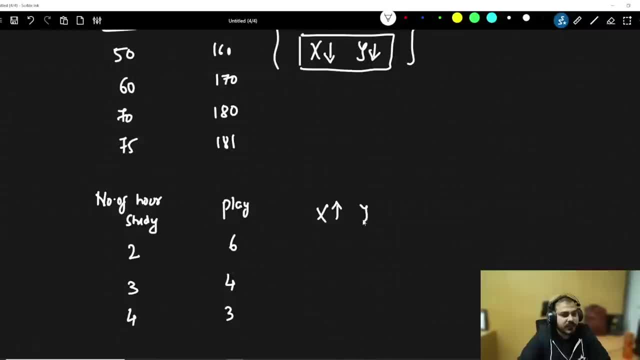 from read unclean language and whatever other. mathematics now in this particular case, is very simple. trouble not only have any computational, but this also requires further drams of labor and memory. what is the relationship? you can see that when x is increasing, y is decreasing, or where x is. 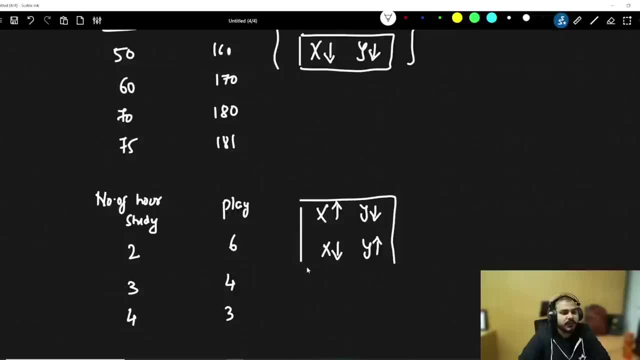 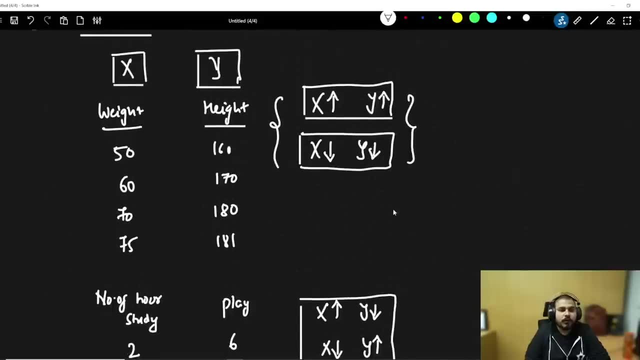 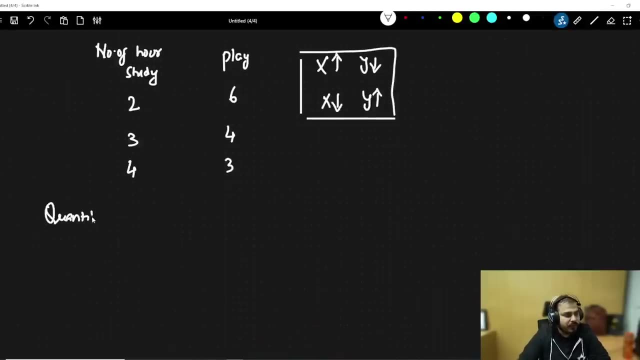 decreasing y is increasing. so this relationship is basically used over here. so here you can see these two conditions, right, these two conditions. now, this is what you can observe. but the main thing is that how do i quantify, how can i quantify or show some relationship, quantify relationship. 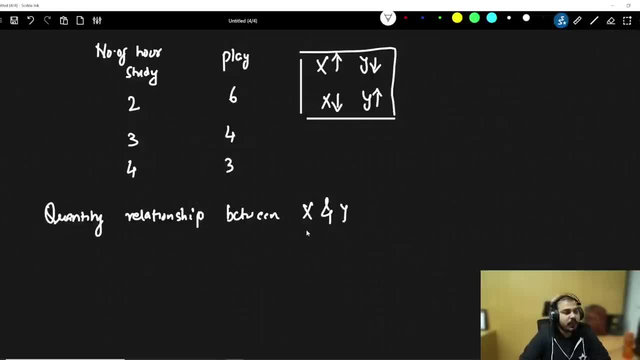 through numbers between x and y. now, in that particular case, i can use a formula which is called as covariance. now covariance is basically given by cov x comma y, which is nothing but summation of i is equal to 1 to n. x of i minus x bar, y of i minus y bar, divided by, divided by n. 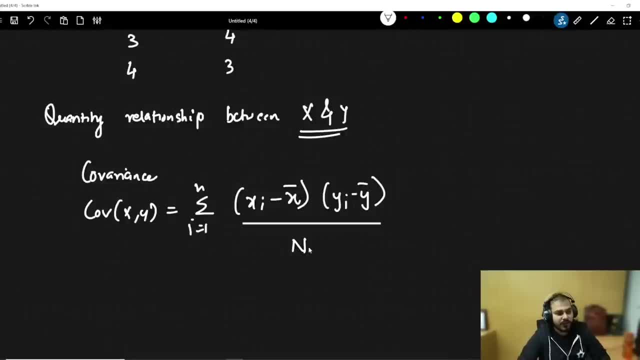 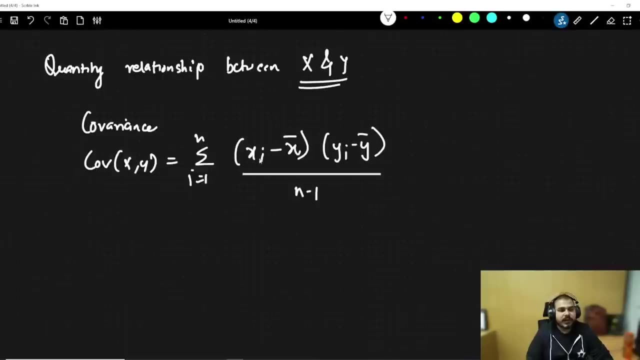 so this is basically the, the, the with respect to covariance. if you are working with sample again, this will be n minus 1 right now, let's consider that we are working with sample. now, in this particular case, you can see what is happening: covariance of x comma y. covariance of x comma y is nothing but x minus x bar. x bar is nothing. 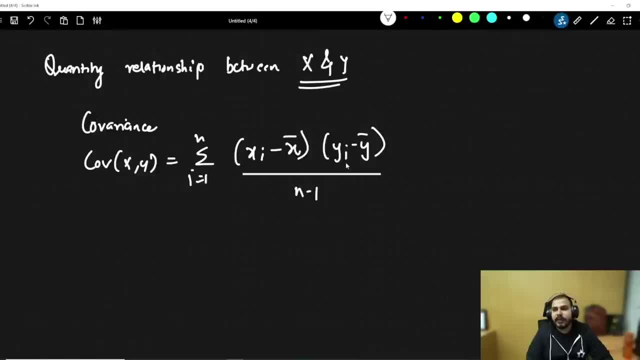 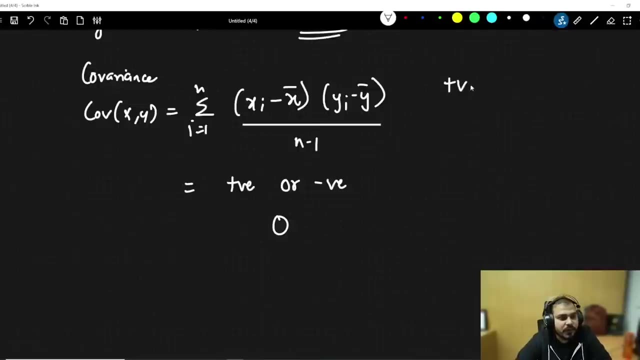 but the mean of x, y minus y bar is y bar is the mean of y. now when we calculate, you will be able to see either we will get a positive number or a negative number, or i may get zero. now tell me, what does the positive number basically indicate? so positive number, positive value, indicate two things. one is: when x is increasing, y is also increasing. when x is decreasing, y is also decreasing. so this shows if this positive number is basically coming. it basically shows or it basically quantifies the relationship between x and y in this particular way. that basically means when x is increasing, y is increasing. when x is decreasing, y is decreasing. so this shows if this positive number is basically coming. it basically shows or it basically quantifies the relationship between x and y in this particular way. that basically means when x is increasing, y is increasing. when x is decreasing, y is decreasing. so this shows if this positive number is basically coming. it basically shows or it basically quantifies the relationship between x and y in this particular way. that basically means when x is increasing, y is increasing. when x is decreasing, y is decreasing. so this shows if this positive number is basically coming. it basically shows or it basically quantifies the relationship between x and y in this particular way. that basically means when x is increasing, y is increasing. when x is decreasing, y is decreasing. so this shows if. 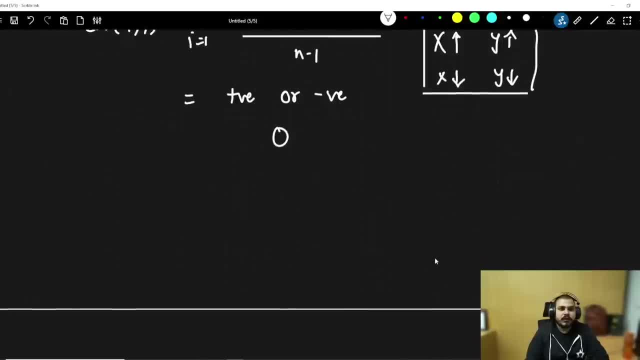 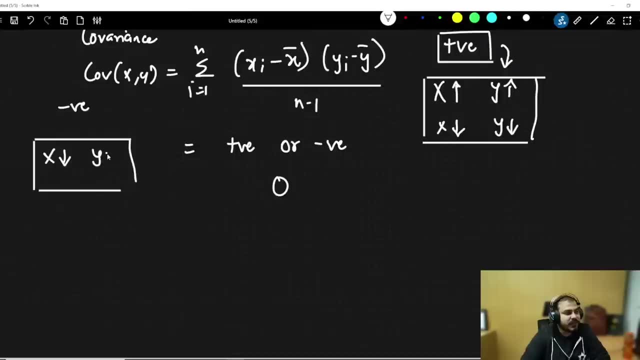 here you will be able to see with this, with a positive, now similarly with a negative number, so with a negative number. here you can find out that when X is decreasing, Y is increasing. with X is increasing, Y is decreasing. so this relationship you will be able to find out. so this is nothing but positive. 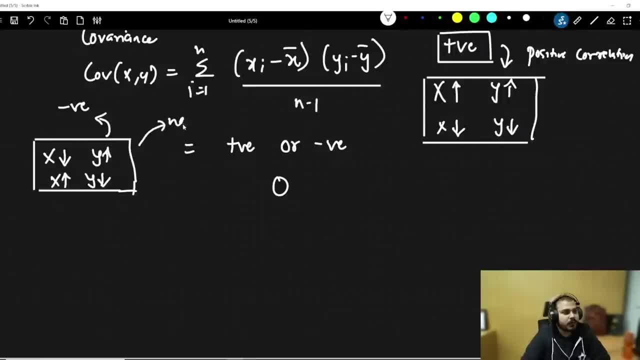 correlation, I'll say, and this will basically be negative correlation. so here you will be able to see this: if it is zero, that basically means when X is increasing, Y is not increasing a, probably there is no relationship between X and Y. so understand this particular thing. but let's understand. 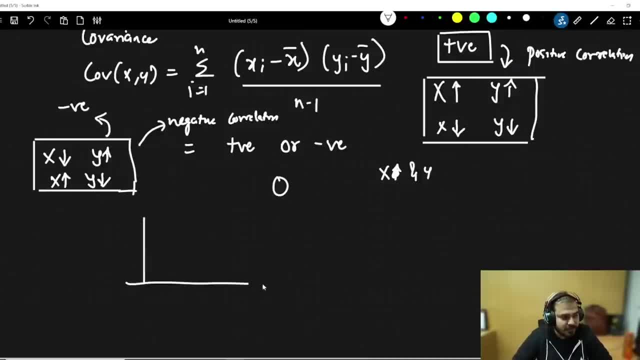 with respect to covariance, like, suppose, if I have a data set which looks like this: now, in this particular case, if this is my X and Y, what do you think will this be? whether it will have a positive correlation, a negative correlation? think over it. it will obviously have a positive correlation, right? because here? 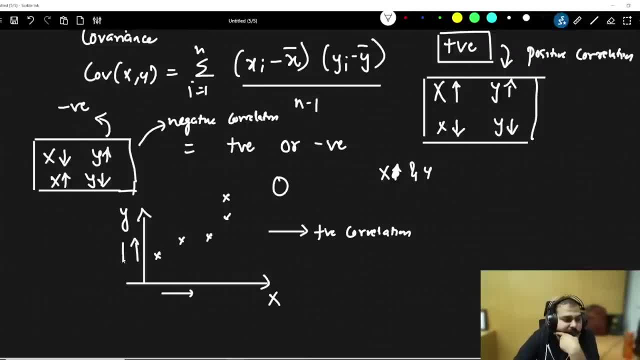 when the X is increasing, Y is also increasing. if the X, Y is decreasing, increasing and the negative correlations. but suppose now, when the X is increasing, Y is increasing. if the X is decreasing, if the X is decreasing, x is also decreasing, right, both this condition are getting several. so here you can definitely 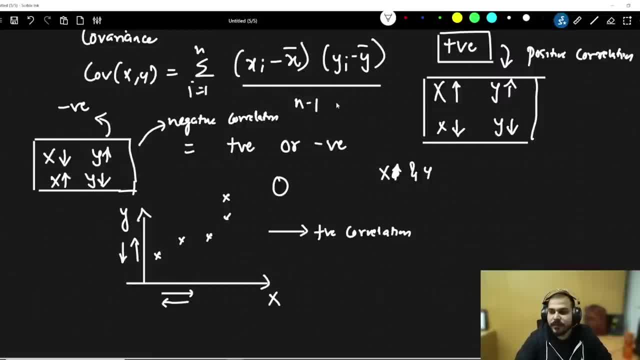 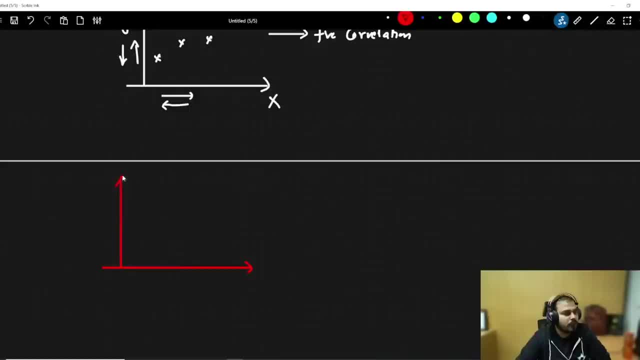 see this positive correlation is there and when you are trying to apply this particular formula, you will either get a positive value in this particular case, suppose if i have another graph which looks like this, which looks like this: this is my x and this is my y, if i have some data points. 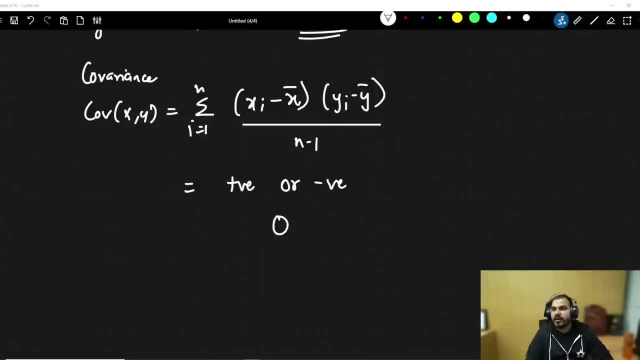 negative number or i may get zero. now tell me, what does the positive number basically indicate? so positive number, positive value, indicate two things. one is, when x is increasing, y is also increasing. when x is decreasing, y is also decreasing. so this shows if this positive number is basically coming. it basically shows or it basically quantifies a relationship between x. 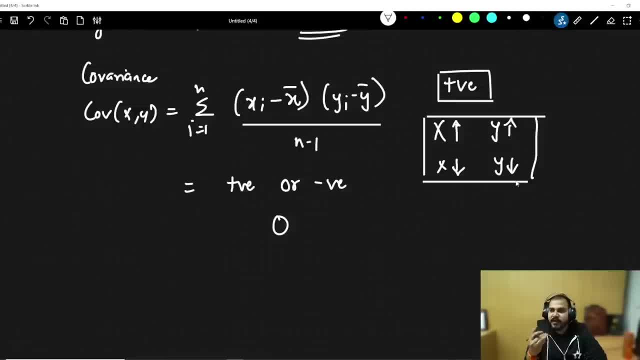 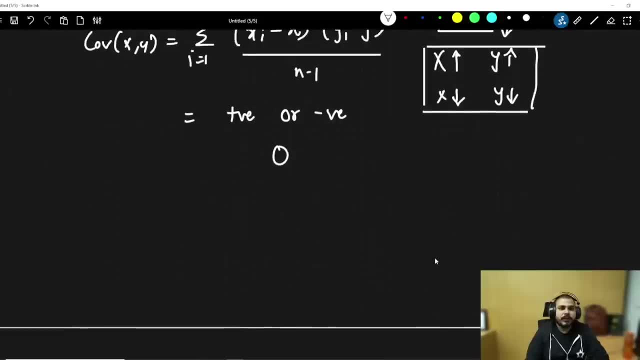 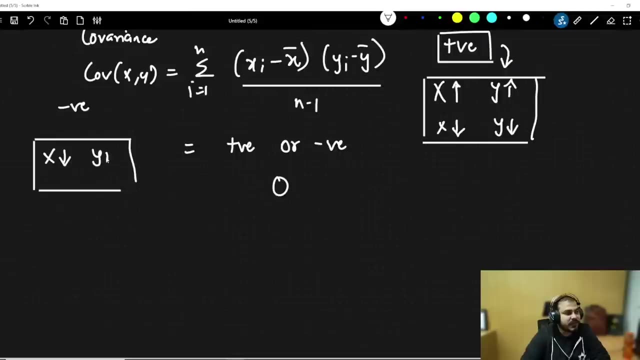 and y in this particular way. that basically means when x is increasing, y is increasing. when x is decreasing, y is decreasing. so here you will be able to see with this with a positive, now similarly with a negative number, so with a negative number. here you can find out that when x is decreasing, 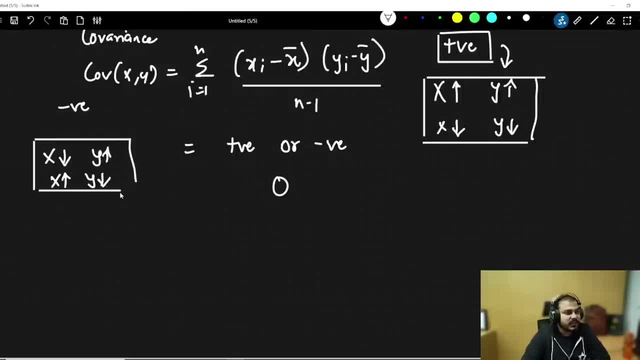 y is increasing, whereas x is increasing, y is decreasing. so this relationship you will be able to find out. so this is nothing but positive correlation. i'll say, and this will basically be negative correlation. so here you will be able to see this: if it is zero, that basically means 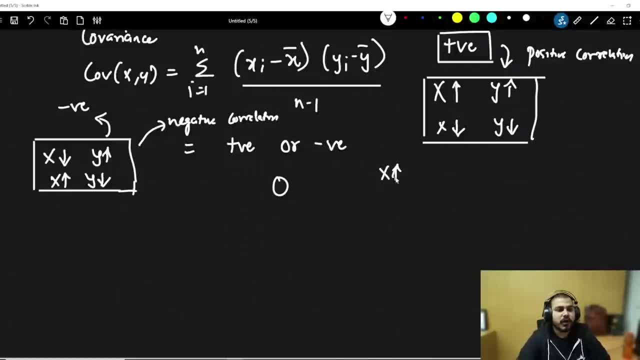 when x is increasing, y is not increasing, or probably there is no relationship between x and y. so understand this particular thing, but let's understand with respect to covariance. like, suppose, if i have a data set which looks like this: now, in this particular case, if this is my x and y, 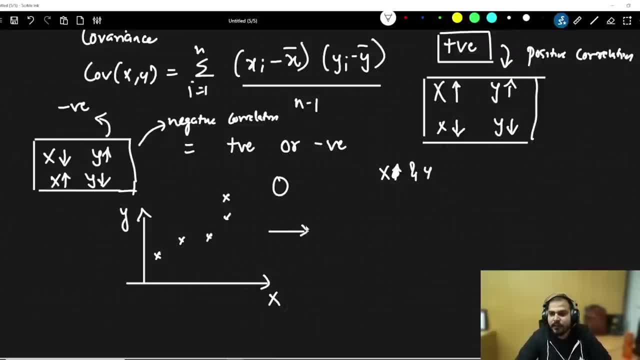 what do you think will this be? whether it will have a positive correlation or negative correlation? think over it. it will obviously have a positive correlation, right? because here, when the x is increasing, y is also increasing. if the x, y is decreasing, x is also decreasing, right? both this? 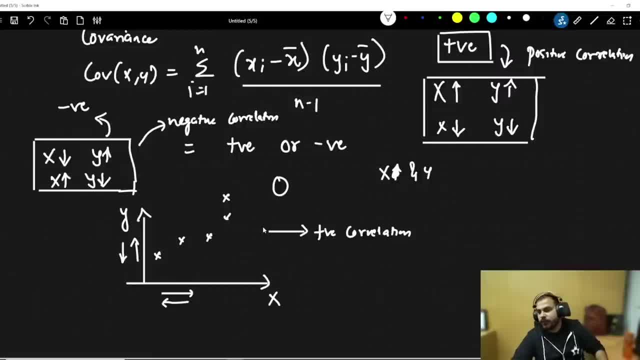 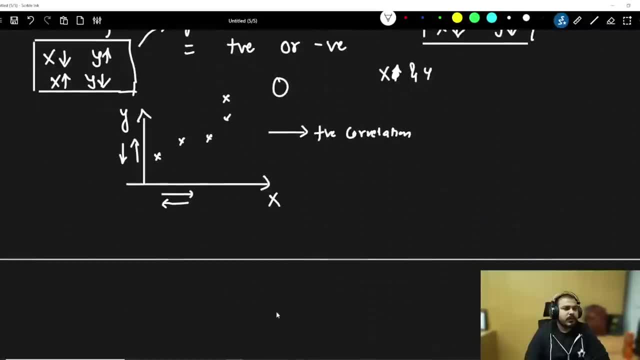 condition are getting separated. so here you can definitely see this positive correlation is there and when you are trying to apply this particular formula, you will either get a positive value. in this particular case, suppose if i have another graph which looks like this, which looks like this: this is my x and this: 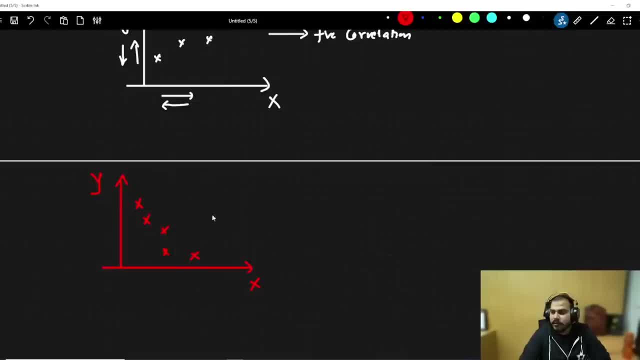 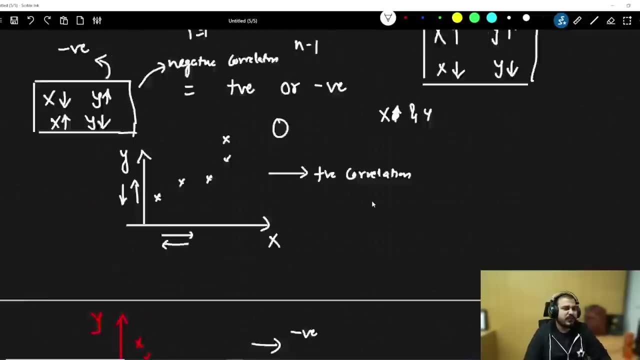 is my y, if i have some data points which looks like this: now, in this particular case, what type of correlation you will have? you will basically have a negative correlation. sorry, i should not say correlation over here. i'll say negative for now, because we have not started correlation. 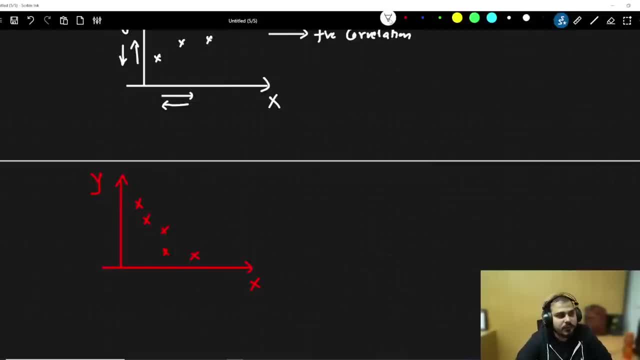 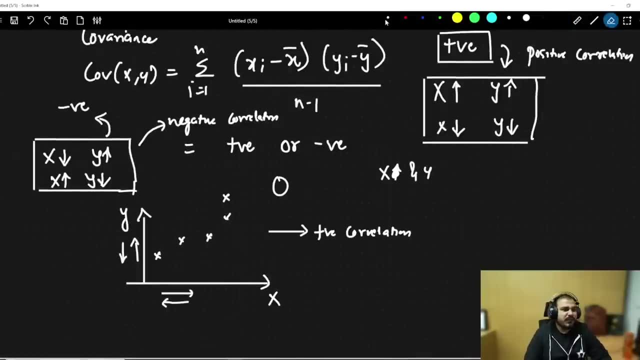 which looks like this: now, in this particular case, what type of correlation you will have? you will basically have a negative correlation. sorry, i should not say correlation over here. i'll say negative for now because we have not started correlation. but here you will be having a some. 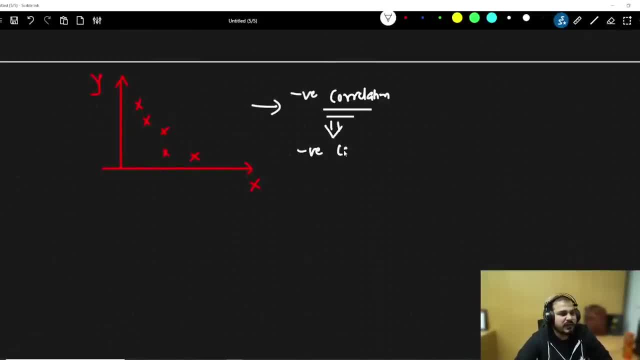 negative correlation. okay, i can also say it as negative covariance. suppose if i have another data set which looks like this with respect to x and y: if my data set is like this, then what will be the my value of covariance? covariance will be zero because there is no relationship covariance. 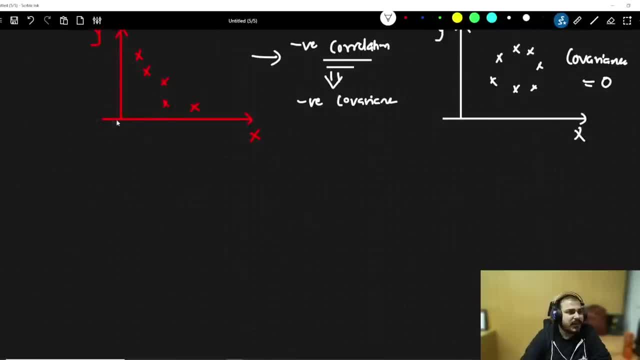 will be basically zero. now let's understand one basic disadvantage of covariance. now covariance over here you'll definitely be able to see positive or negative, you'll be able to find out the positive or negative correlation. but with respect to the disadvantage, there is no fixed value you may have. 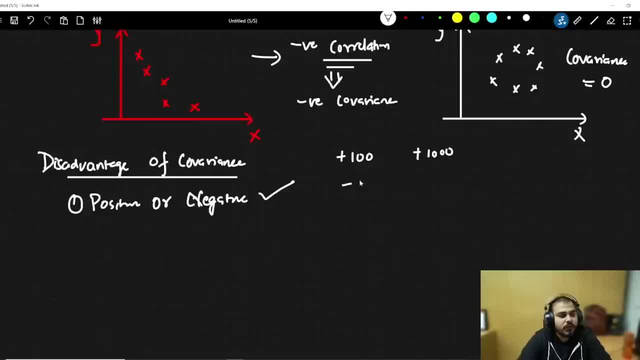 plus hundred also, you may have plus thousand also. you may find out minus 200 also, minus 2000 also, like this. with respect to the magnitude, there is no such limit. you will definitely be able to see the direction, whether it is positive or negative, but this magnitude is not limited. so if we have 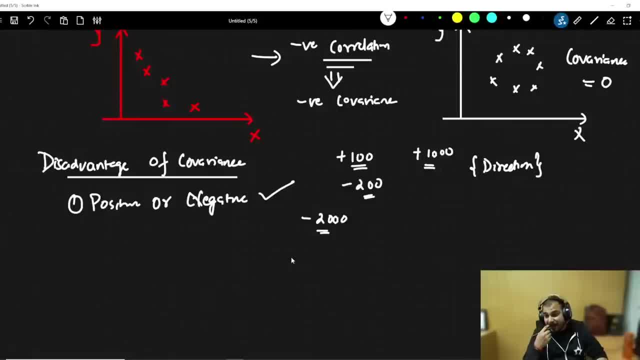 one portion positive, how much positive, how much negative that part, if, probably, if you have two distribution- one is plus hundred, the other one is plus thousand- you'll not be able to identify because it is just a magnitude value. it is just a magnitude value now. that is the reason we really 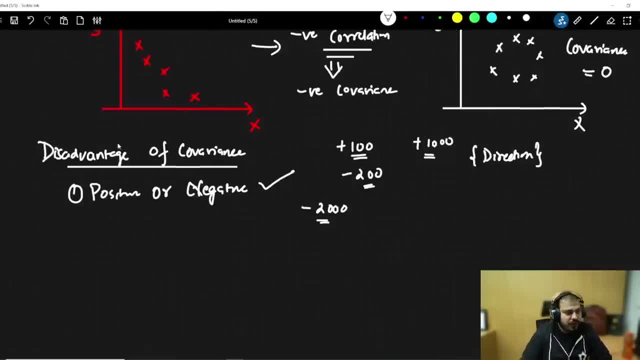 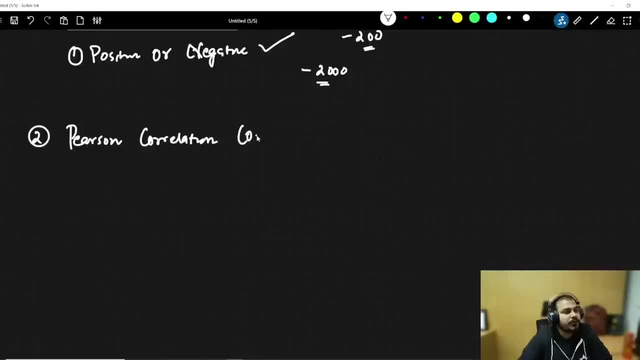 need to restrict this values between some range. so for that specific region we use another one which is called as pearson correlation, a pearson correlation coefficient. what it does is that it basically restricts all your value between minus one to plus one, the more towards plus one or minus one. 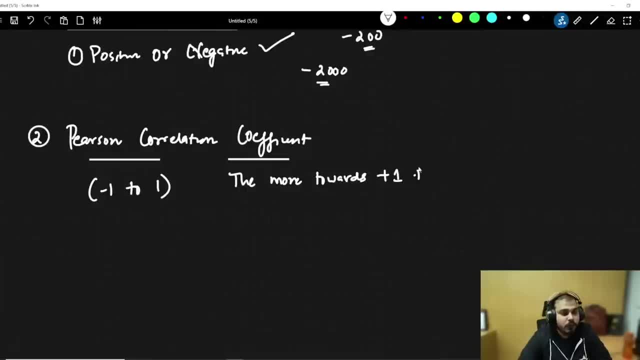 more positively it is correlated. sorry, the more towards plus one, more positively it is correlated. the more towards minus one, more negatively it is correlated. you should be able to see that. okay, then what is the difference between covariance with respect to the formula? now for the peers correlation, you can basically use something like this: x comma y. it is nothing, but it is very simple. 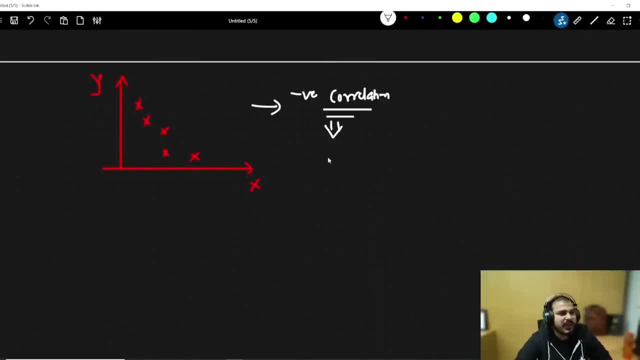 but here you will be having a negative correlation. okay, i can also say it as negative covariance. suppose if i have another data set which looks like this with respect to x and y, if my data set is like this, then what will be the my value of covariance? covariance will be zero because there is no relationship covariance. 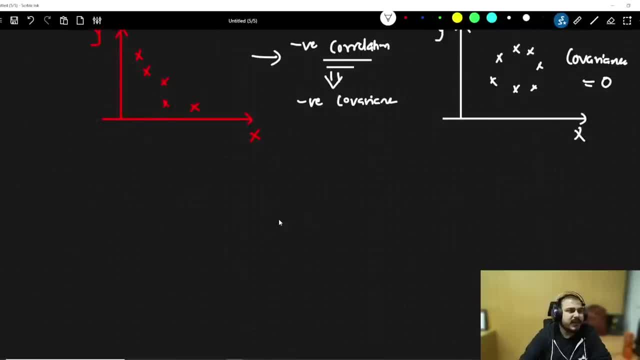 will be basically zero. now let's understand one basic disadvantage of covariance. now covariance over here you will definitely be able to see positive or negative, you will be able to find out positive or negative correlation. but with respect to the disadvantage, there is no fixed value. you may have plus hundred also. you may have plus thousand also. you may find out minus 200 also. 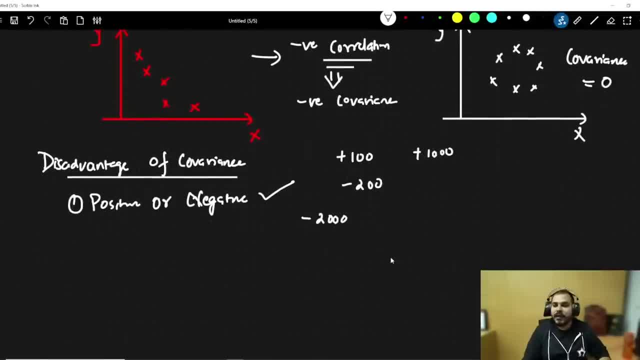 minus 2000 also like this. with respect to the magnitude, there is no such limit. you will definitely be able to see the direction, whether it is positive or negative, but this magnitude is not limited. so if we have two distribution, how much positive, how much negative that part, if it probably 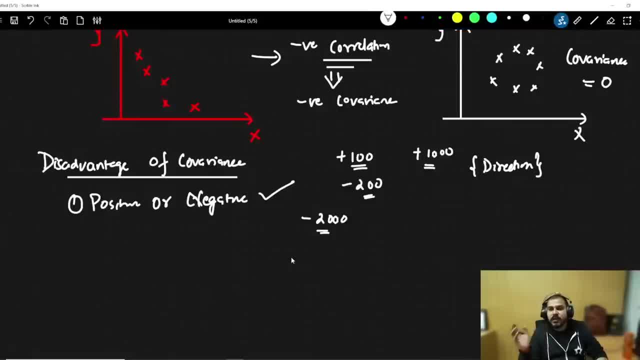 has two distributions. one is plus hundred, the other one is plus thousand. you will not be able to identify because it is just a magnitude value. it is just a magnitude value now. that is the reason we really need to restrict this values between some range. so for that specific region. 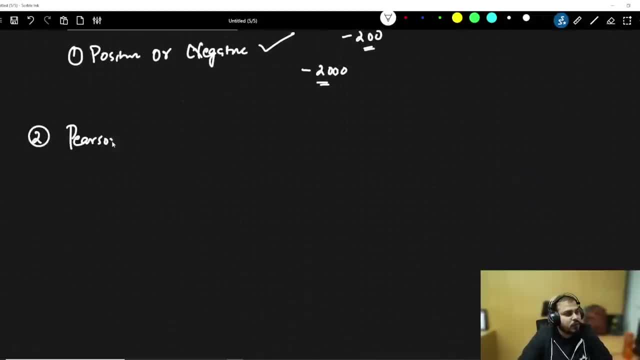 we use another one which is called as pearson correlation, a pearson correlation coefficient. what it does is that it basically restricts all your value between minus one to plus one, more towards plus 1 or minus 1. more positively it is correlated, sorry, the more towards plus 1. 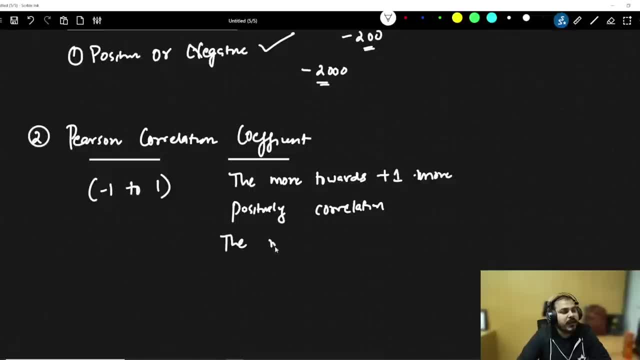 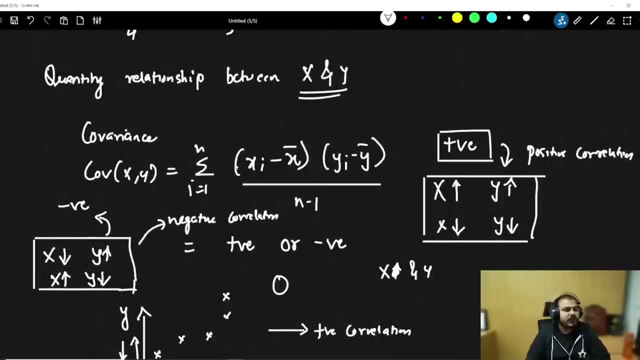 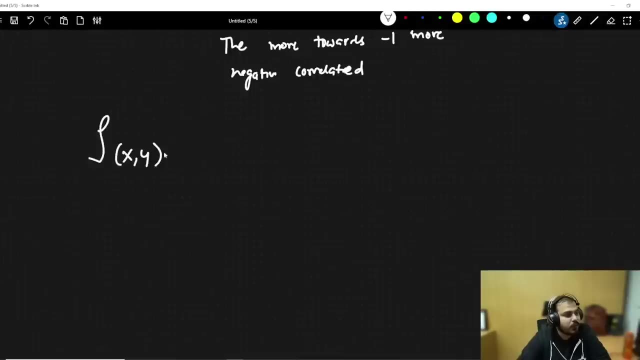 more positively it is correlated, the more towards minus 1, more negatively it is correlated. you should be able to see that. okay, then what is the difference between covariance with respect to the formula? now for the peers correlation. you can basically use something like this: x comma y. 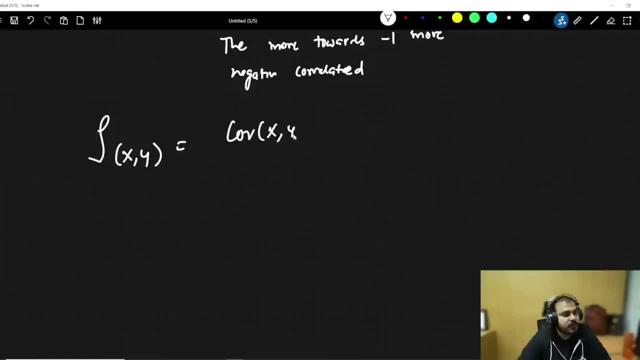 it is nothing, but it is very simple: covariance of x, comma y divided by standard deviation of x and standard deviation of y. because of this multiplication, all your values will be between minus 1 to plus 1. so here you will be able to see that it is always between minus 1 to plus 1. 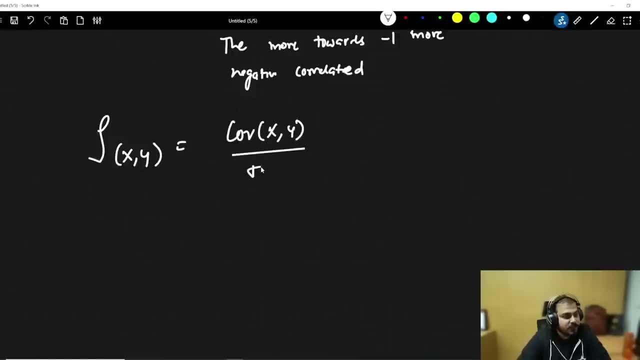 covariance of x comma y divided by standard deviation of x and standard deviation of y. because of this multiplication, all your values will be between minus one to plus one. so here you will be able to see that it is always between minus one to plus one. now let me show you some examples in wikipedia, so if you go and search for 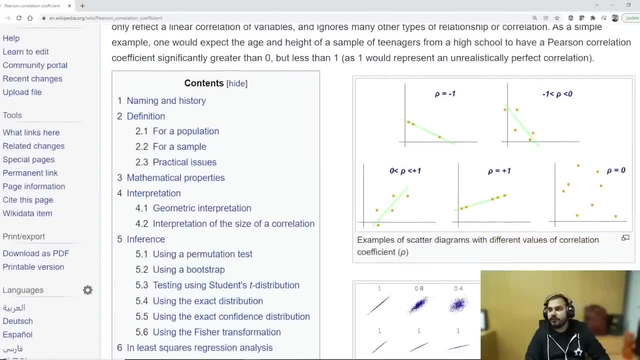 pearson correlation coefficient. here you will be. you will be able to see that it is always between minus one to plus one. you will be able to see this. okay, now tell me this particular diagram. here you can see all the points are in one, one straight line. so when you draw this particular line, your correlation. 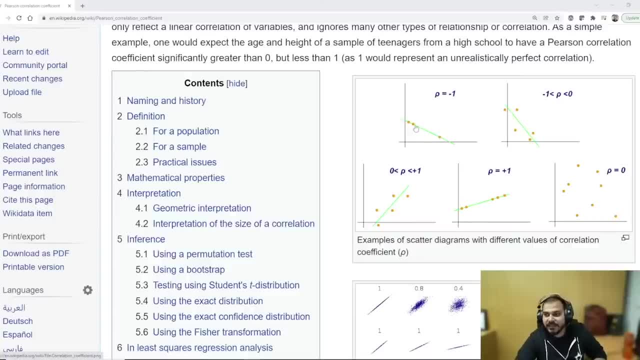 obviously, in this particular case, when x is decreasing, y is increasing, right, in this particular case, if x is decreasing, y is increasing. if x is increasing, y is decreasing. this is the relation that it is found, so it is negatively correlated and if it falls all in the straight line, it is. 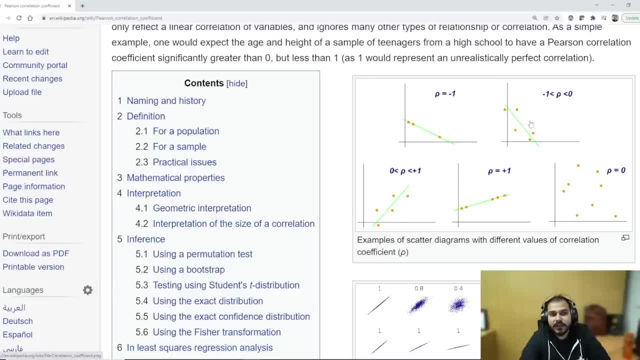 minus one, then here you will be able to see that over here you have some of the data points distributed in this. here also you can actually see negative correlation, but not all are in the straight line, so your value, your correlation, will be ranging between minus one to zero. similarly, in: 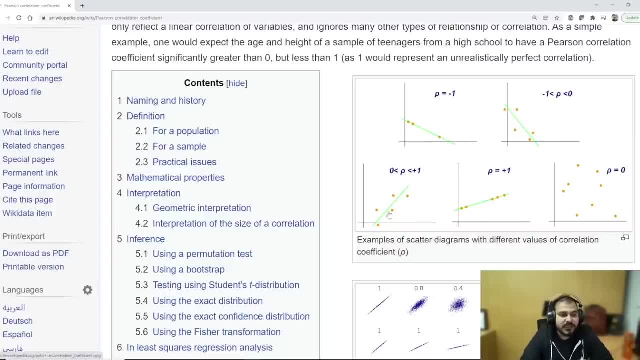 this particular case. here you can see that when x is increasing, y is also decreasing, so here will have a positive correlation. since it does not follow in the straight line, it is between zero to one. if it falls in the straight line, then it is plus one, so it 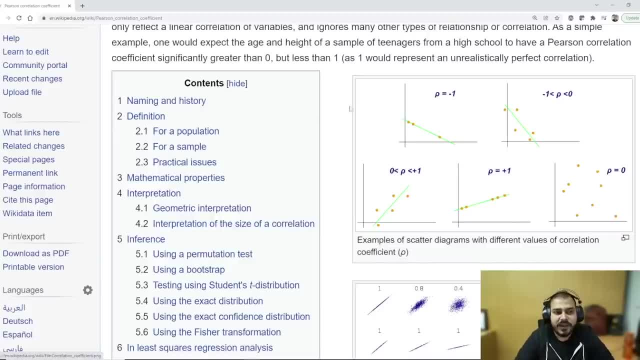 captures the linear properties very well, because everywhere you can see that there is a linear line, it captures it in an amazing way. that is the most advantageous things with respect to Pearson correlation. now, in this particular case, here you can see that the correlation is zero. why? because 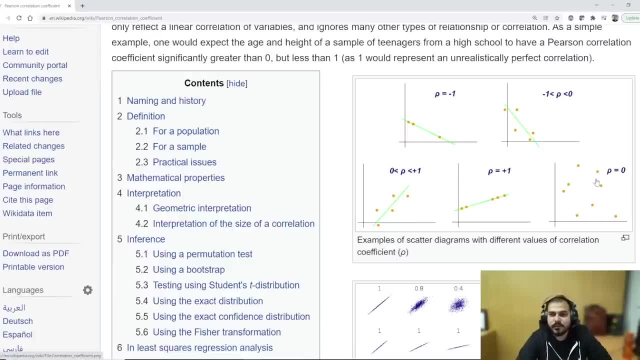 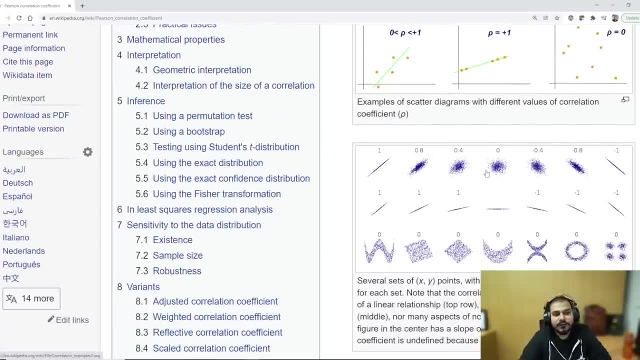 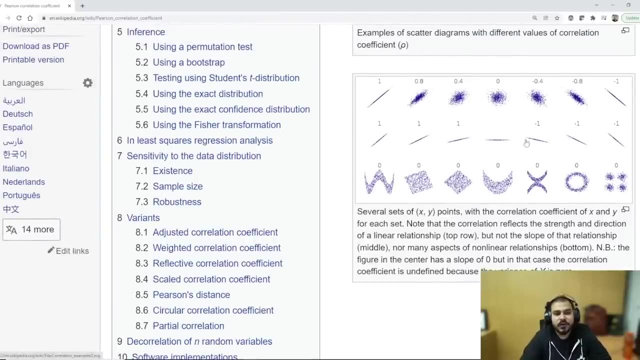 we cannot identify when x is increasing, y is also increasing. the data is completely distributed here and there. now some more examples here you can see: this is one. this is point eight, point four. zero minus point four, minus point eight and minus one. and similarly, these all are one one, one one. this is zero minus one, minus one. 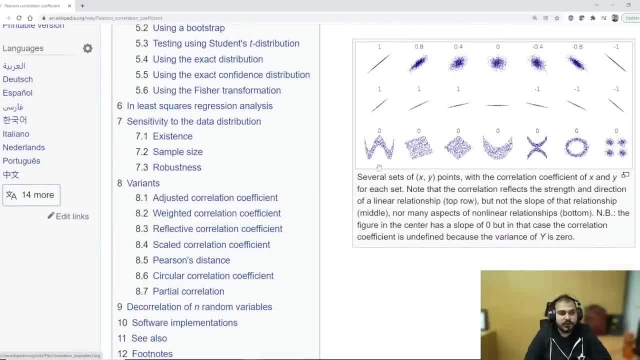 minus one and similarly, here you can see some more zeros. you can also see some more zeros. this you cannot definitely identify. what exactly is this? there is a lot of difference between covariance and correlation, so here your values will always be between minus one to plus one, and nothing more. 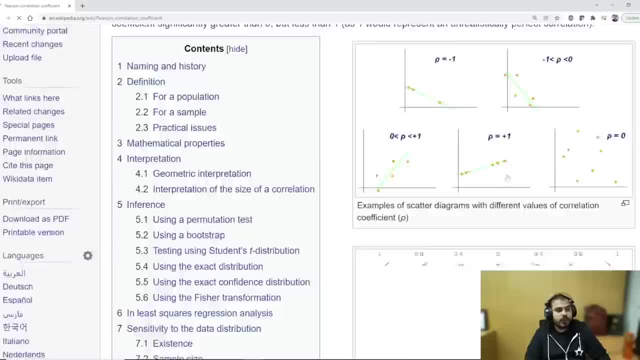 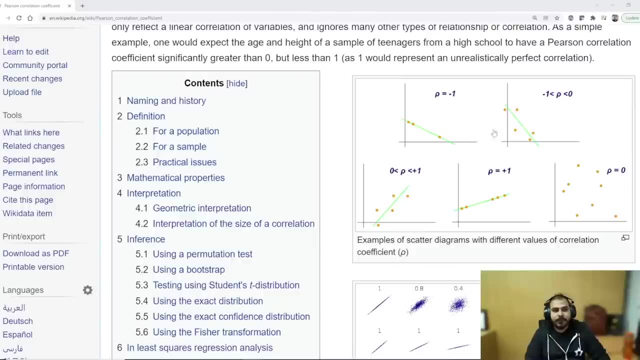 now let me show you some examples in wikipedia. so if you go and search for pearson correlation coefficient here, you will be able to see this. okay, now tell me, this particular data is not the same as the data of the previous data. so if you go and search for 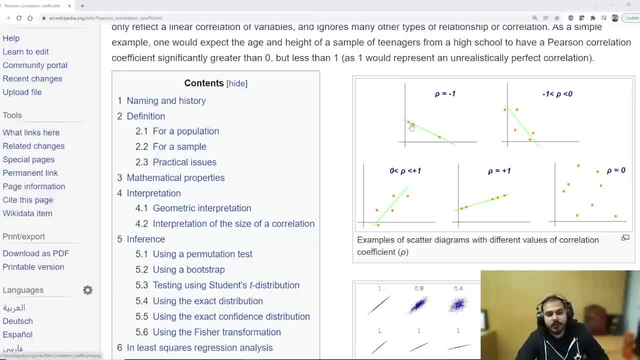 diagram here you can see: all the points are in one, one straight line. so when you draw this particular line, your correlation, obviously, in this particular case, when x is decreasing, y is increasing, right, in this particular case, if x is decreasing, y is increasing. if x is increasing y. 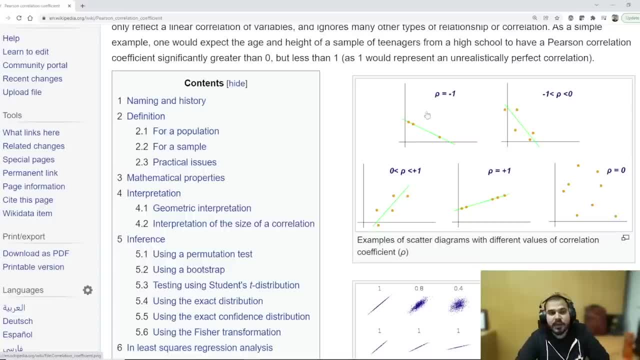 is decreasing. this is the relation that it is found, so it is negatively correlated. and if it falls all in the straight line, it is minus 1. then here you will be able to see that. over here you have some of the data points distributed in this. here also you will be able to see that. 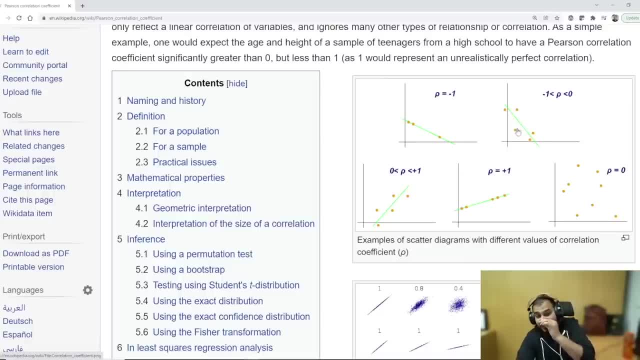 you can actually see negative correlation, but not all are in the straight line, so your value, your correlation, will be ranging between minus 1 to 0. similarly, in this particular case, here you can see that when x is increasing, y is also decreasing. so here we'll have a positive. 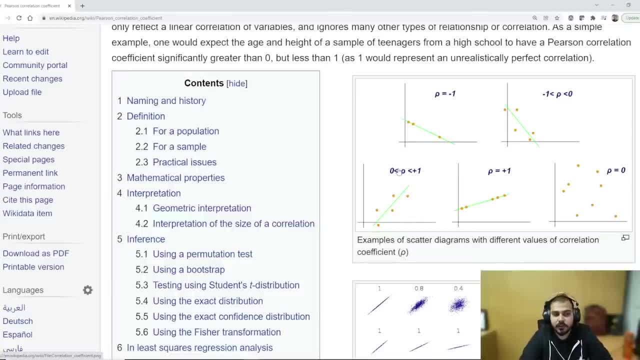 correlation. since it does not follow in the straight line, it is written 0 to 1. if it falls in the straight line, then it is plus 1. so it captures the linear properties very well, because everywhere you can see that there is a linear line, it captures the linear properties very well. 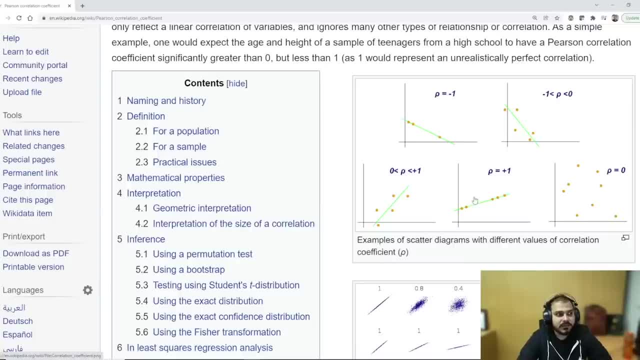 so you can use it in an amazing way. that is the most advantageous things with respect to Pearson correlation. now, in this particular case, here you can see that the correlation is 0. why? because we cannot identify when x is increasing, y is also increasing. the data is completely distributed here. 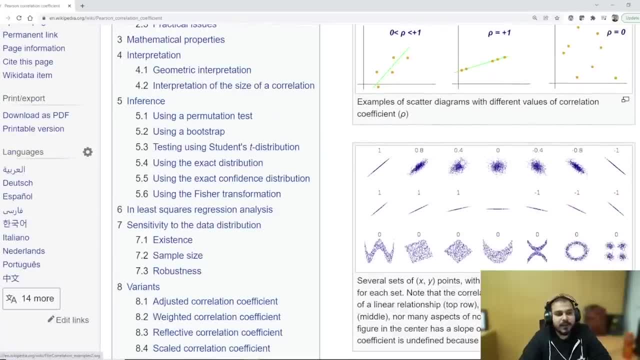 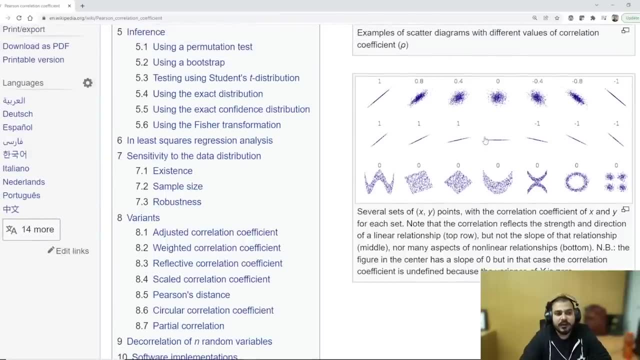 and there. now some more examples here you can see: this is 1, this is 0.8, 0.4, 0 minus 0.4, minus 0.8 and minus 1, and similarly, these all are 1, 1, 1, 1. this is 0 minus 1 minus 1, and this is 0 and this is. 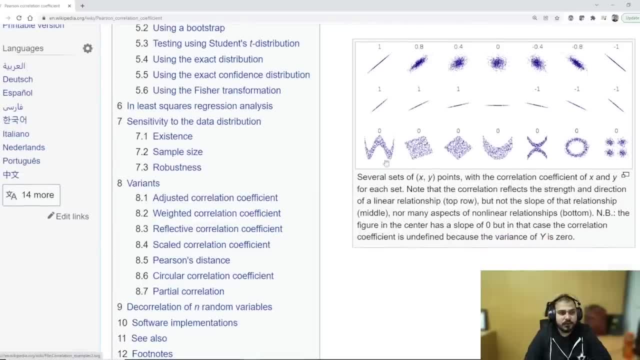 1 minus 1, and similarly, here you can see some more zeros. you can also see some more zeros. this you cannot definitely identify. what exactly is this? there is a lot of difference between covariance and correlation, so here your values will always be between minus 1 to plus 1, and 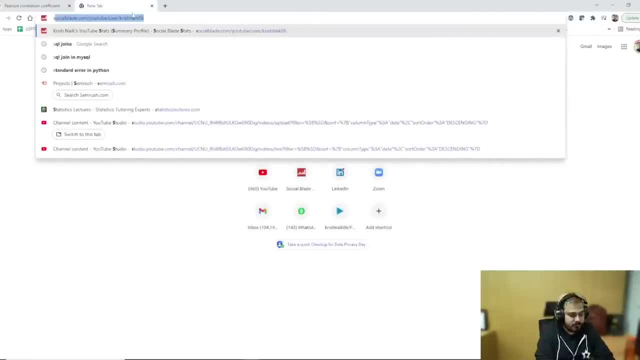 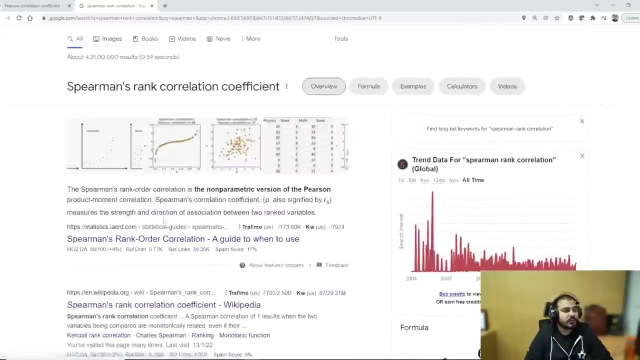 nothing more than that. okay, let me search for one more thing, something called a Spearman rank correlation. now you'll be understanding why do we specifically use Spearman rank correlation also, so I'll go to Wikipedia here. 1 and 2 are the values of the correlation between minus 1 and. 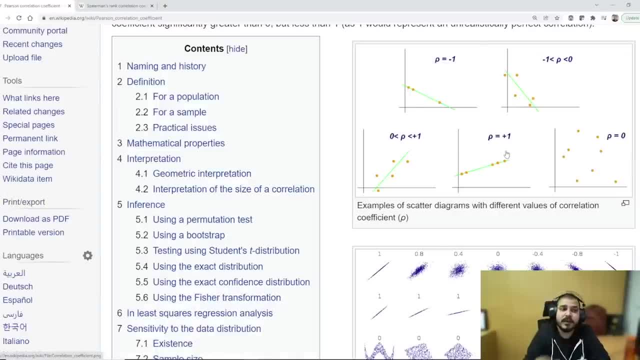 minus 1 and after you create this correlation, you can see that this line can be interpreted as 1 and when it is interpreted as minus 1, it means 1. you have to identify it captures the linear properties. well, linear. when the line is linear, obviously it'll say you 1, even though the 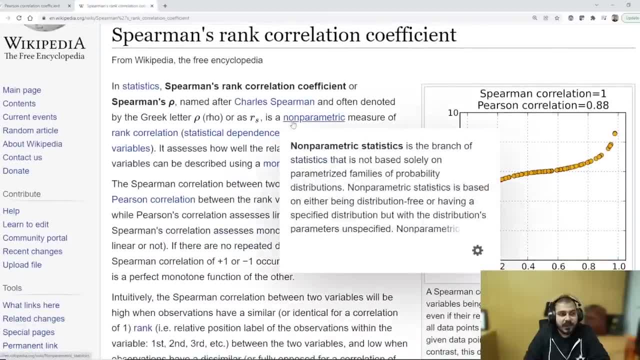 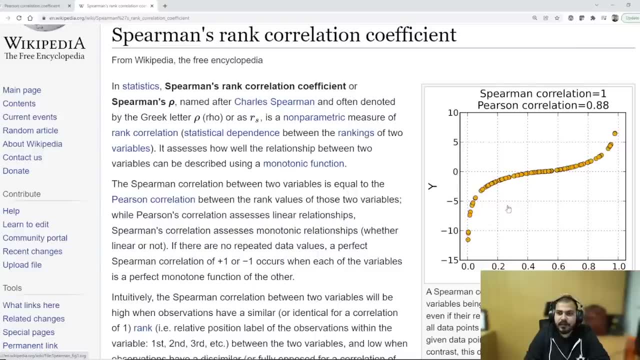 distribution is like this: it will try to create a linear line and your it will tell you the value. now let's go to Spearman rank correlation. now, in Spearman rank correlation, just see this graph, everybody, this graph over here that you are actually being able to see. this is obviously having a 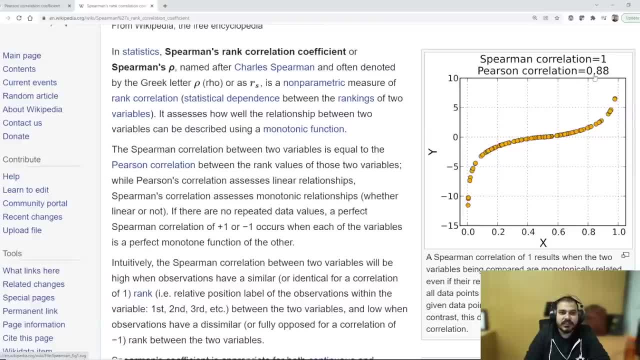 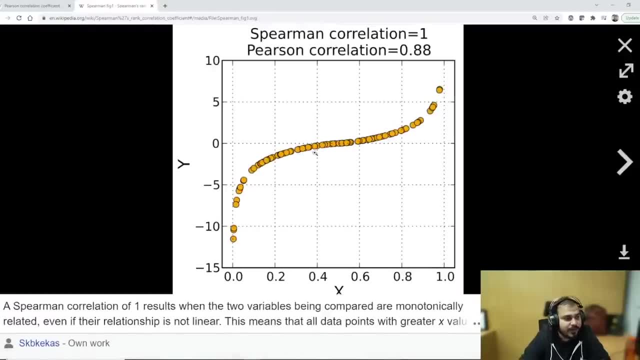 positive correlation, because when the x is increasing, y is increasing. and when I try to calculate with respect to Pearson correlation, it is giving me 0.88.. You will be able to see that at every point, at every point over here, at every point when x is increasing, y is definitely. 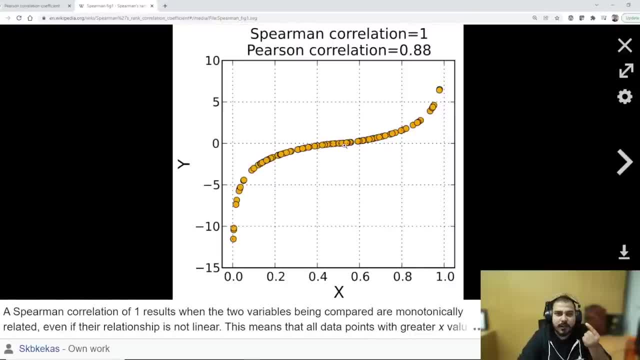 increasing In this region. it is increasing by a small amount, So this property is not being able to capture by Pearson correlation. So that is the reason it is showing you 0.88, even though when x is increasing, y is also increasing. We need to get 1, and that is where Spearman 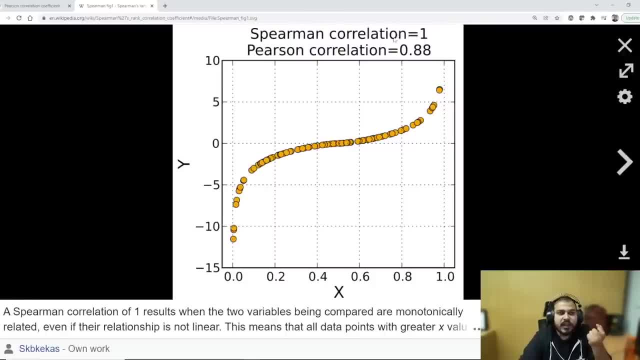 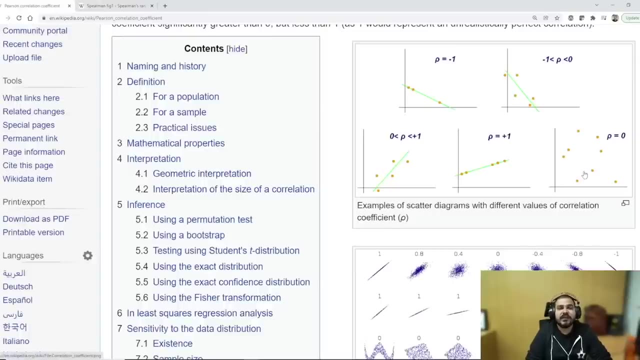 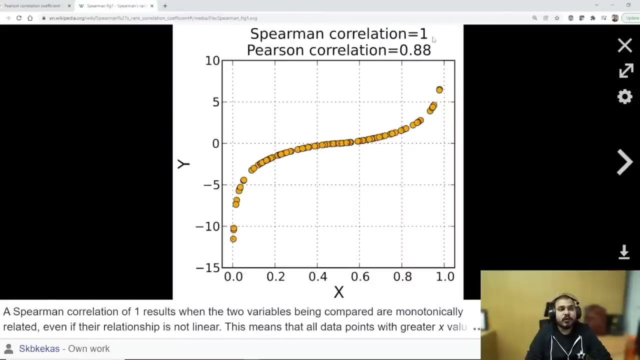 rank correlation will come, Because Spearman rank correlation will also satisfy non-linear properties. Pearson correlation is good at satisfying linear properties. that we have already seen Because, if you see this example, it tries to determine the linear properties and tries to give the value. In this case, non-linear properties will also work well. Okay, so Spearman. 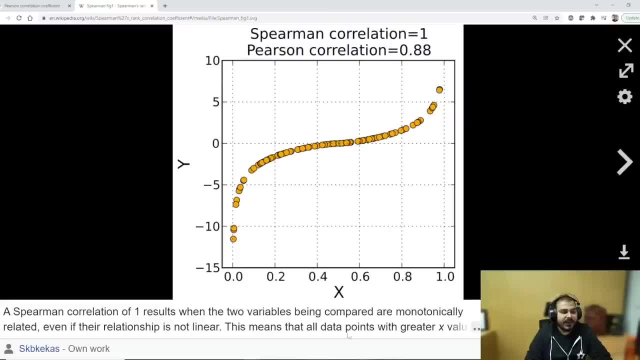 correlation. And what is the formula? Probably they will try to change it to the following: So Spearman rank correlation will also satisfy non-linear properties. So the formula. only one difference is there. Instead of writing, suppose let's say that I am? 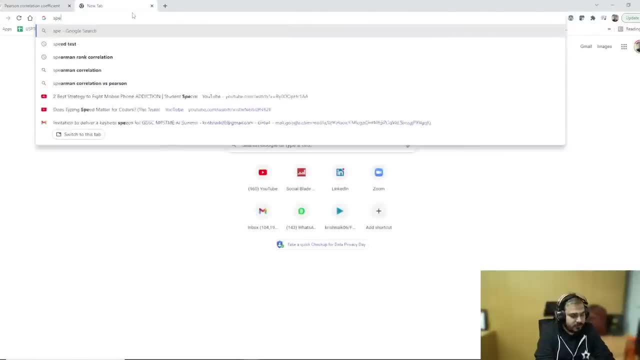 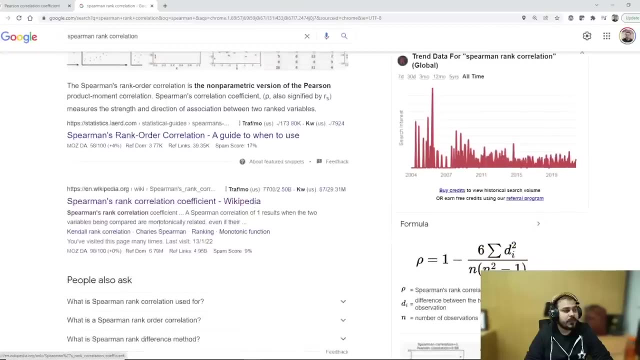 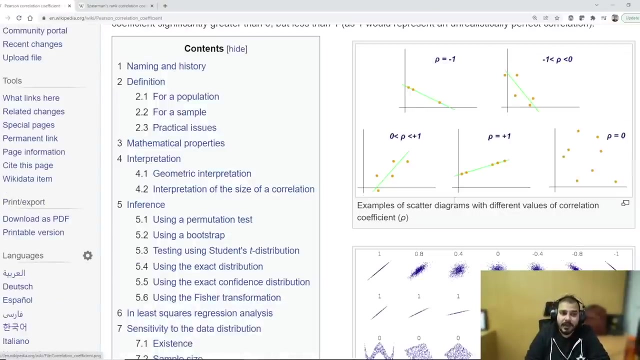 than that. okay, let me search for one more thing, something called a spearmann rank correlation. now you will be understanding why do we specifically use spearmann rank correlation also, so I will go to Wikipedia here. one thing that you have to identify: it captures the linear properties. well, 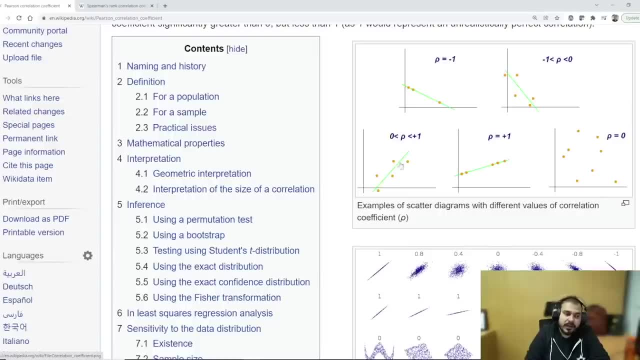 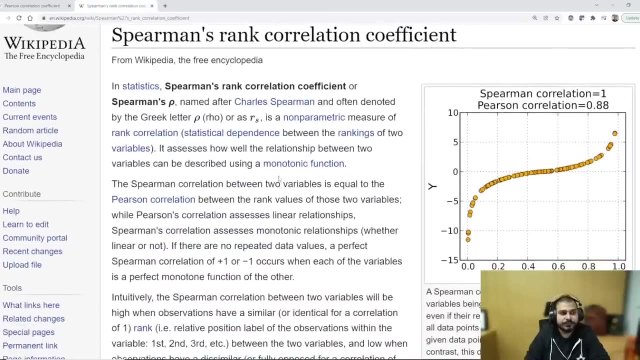 linear. when the line is linear, obviously it will say you won, even though the distribution is like this. it will try to create a linear line and your it will tell you the value. now let's go to spearmann rank correlation. now, in spearmann rank correlation, just see this: 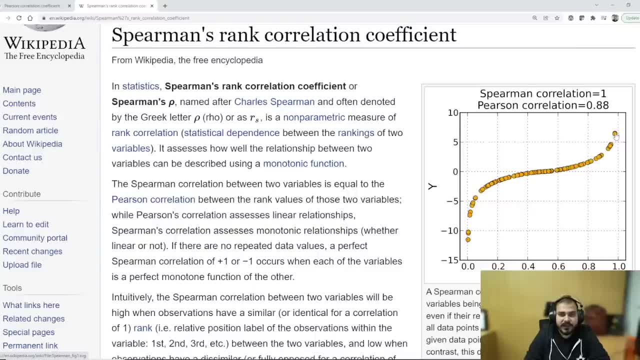 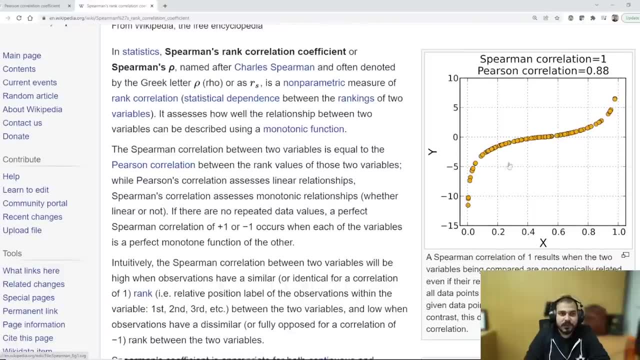 graph everybody, this graph over here that you are actually being able to see. this is obviously having a positive correlation, because when the x is increasing, y is increasing And when I try to calculate with respect to Pearson correlation, it is giving me 0.88.. 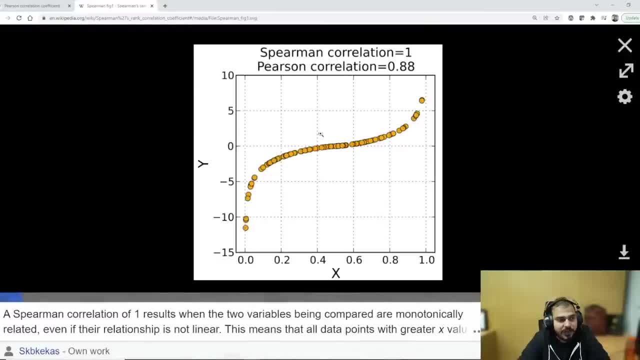 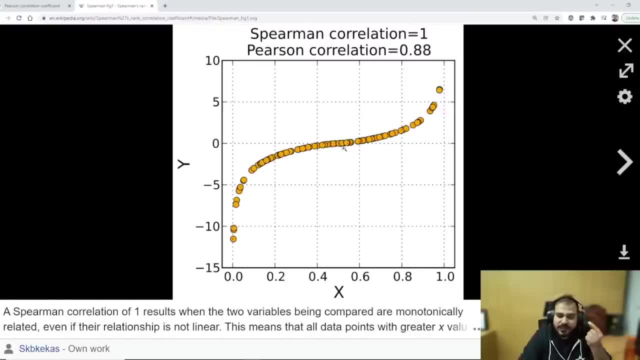 You will be able to see that at every point, at every point over here, at every point when x is increasing, y is definitely increasing In this region. it is increasing by a small amount. So this property is not being able to capture by Pearson correlation. 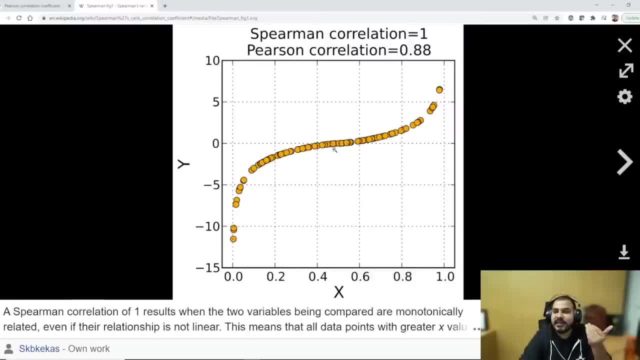 So that is the reason it is showing you 0.88, even though when x is increasing, y is also increasing. We need to get 1, and that is where Spearman rank correlation will come, Because Spearman rank correlation will also satisfy non-linear properties. 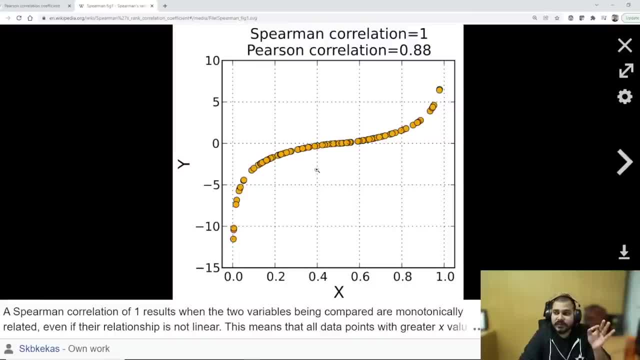 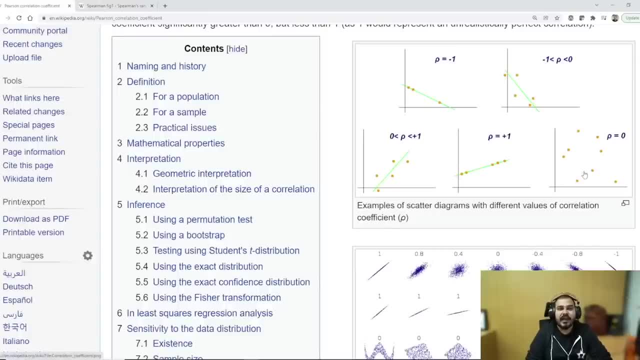 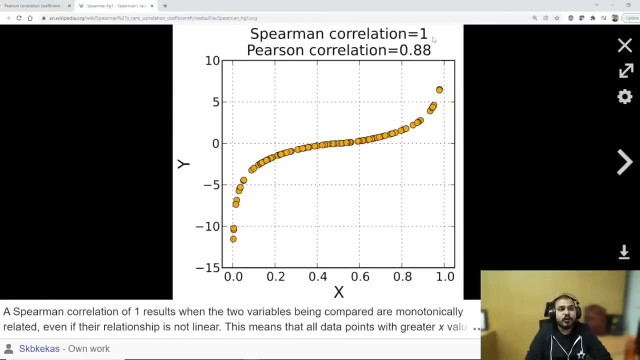 Pearson correlation is good at satisfying linear properties. that we have already seen because if you see this example, it tries to determine the linear properties and tries to give the value. In this case, non-linear properties will also work well. So Spearman correlation, and what is the formula? probably they will try to change it to. 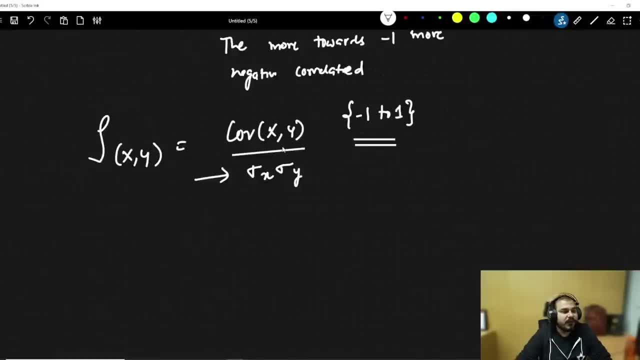 The formula. only one difference is there? Instead of writing, suppose let's say that I am going to find out the Spearman rank correlation between x and y. Here everything will be same. Here, instead of standard deviation of x, here you will be having rank of standard deviation. 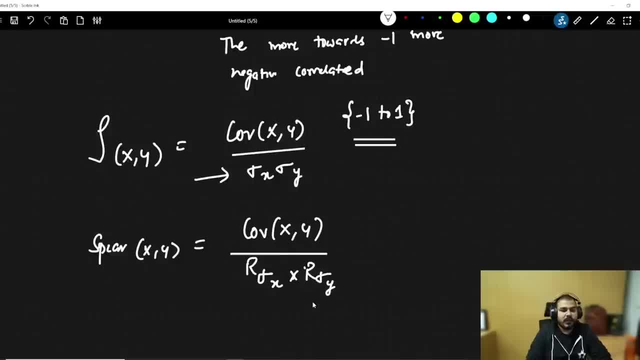 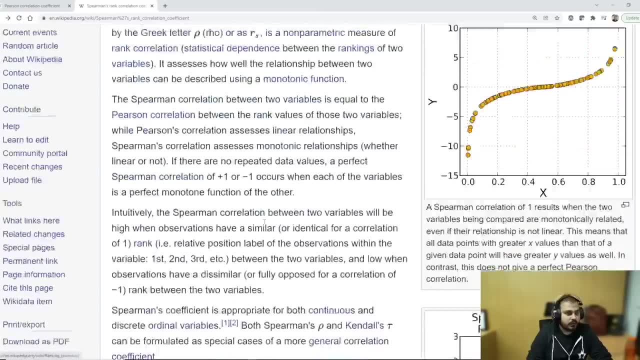 of x multiplied by rank of standard deviation of y. Now you may be thinking: What is this rank of standard deviation of x and standard deviation of y? Let me just show you that also. So this is the formula. Okay, I missed one more thing. 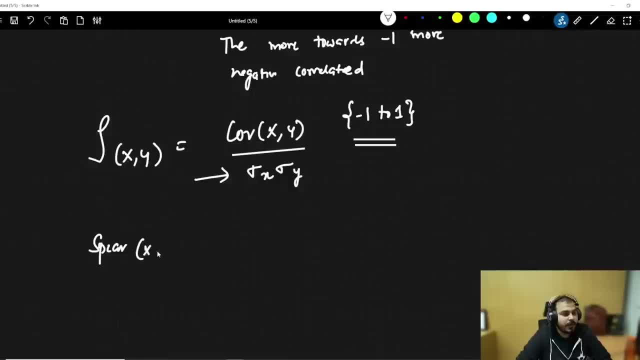 going to find out the Spearman rank correlation between x and y. Here. everything will be same. Here, instead of standard deviation of x, here you will be having rank of standard deviation of x multiplied by rank of standard deviation of y. Now you may be thinking: what is this rank of? 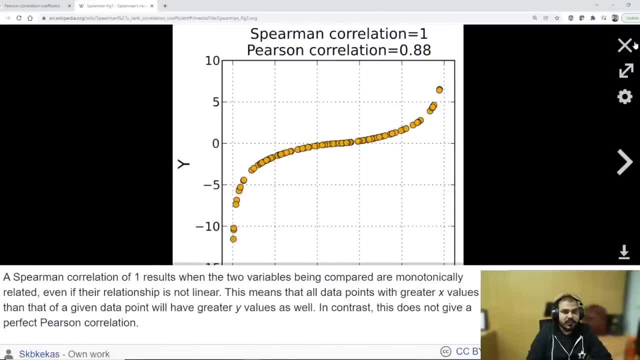 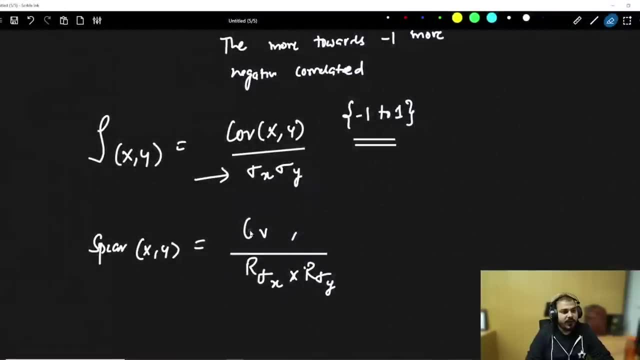 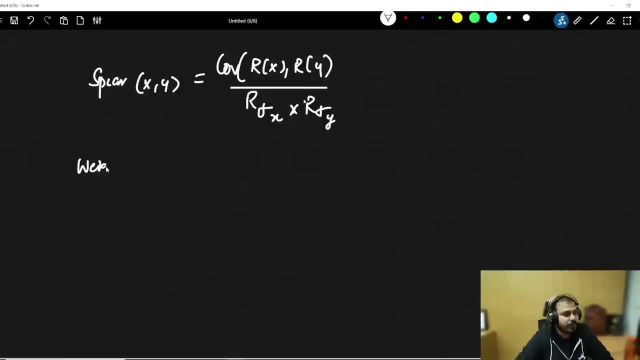 Now, what is this? rank of x and rank of y? Let's consider that I have this feature: weight and probably age. If this is 170, the weight may be 45. If it is 160, the weight- sorry, weight is too high. This is not possible, So I will just say height and weight. let's say: 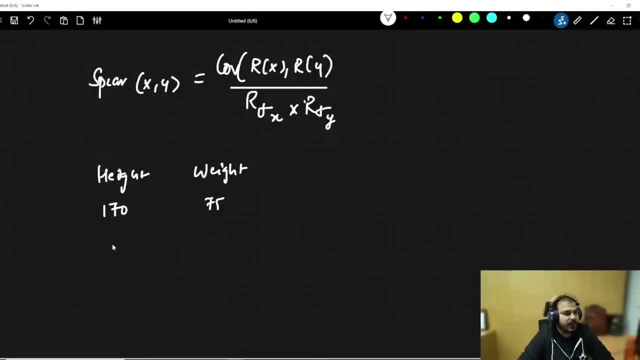 say the height is 170, the weight may be 75 kgs. if i say height is 160, then the weight may be 62- 150. the weight may be 60- 145. the weight may be 55. now, in this particular case, how do i define my? 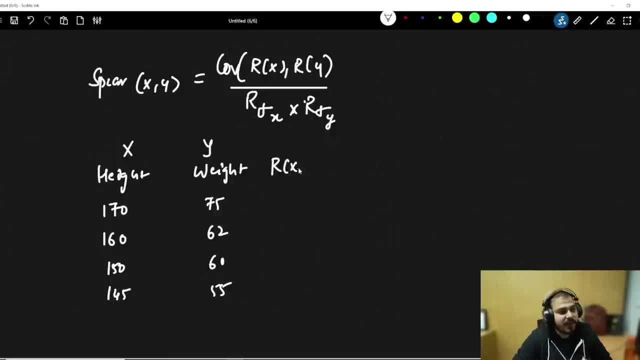 rank. this is my x, this is my y. how do i define my rank of x? now, rank of x is very, very simple. you just assign rank over here. you have four points. okay, which one, which value you want to give the highest rank? go and see over here, this is having the highest value, right, highest value. now let's. 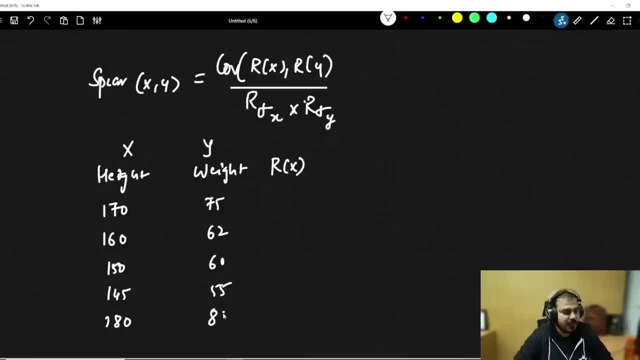 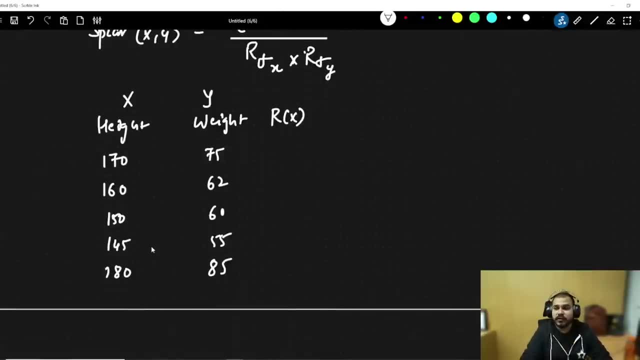 say: let's consider that i have one more 180 and this will be 85. let's consider in this you just need to convert this or you just need to assign rank to this particular data. now rank basically gets applied to this in height. if i say rank of x, 180 is the highest right, so i may give this rank. 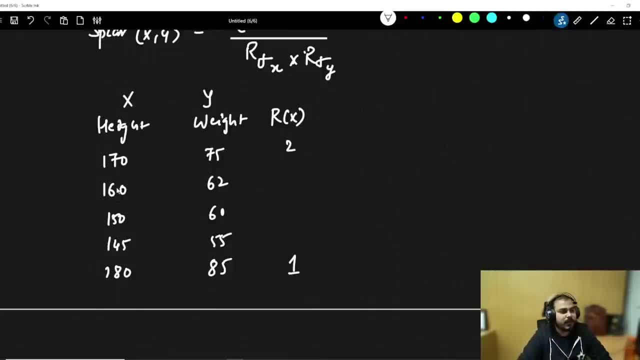 as one, then 170 is the next highest, then 160 is the next highest. you can see that i have one more value right now. i have one more value right now. i have one more, then 150, then 150, 45, right. so here you will be able to see that i'm assigning rank and similarly. 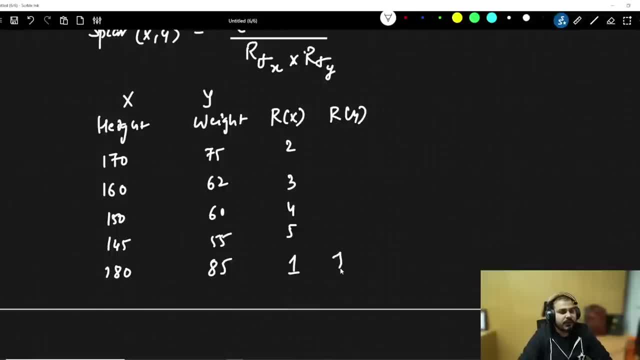 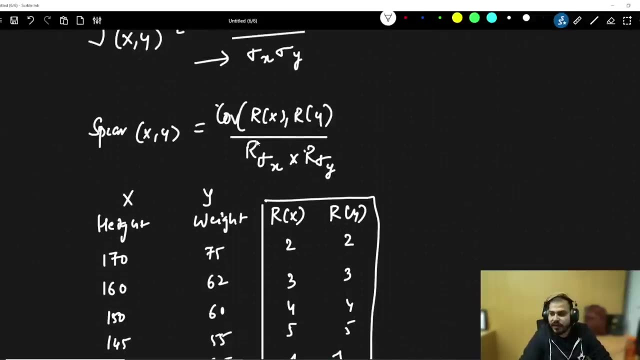 i'll go and assign rank for y in this particular case. my one rank is 85, then you have two, then you have probably three, then four, then five, like this: this rank will be basically used to do this calculation. that is the reason i told right: covariance of rank of x and rank of y divided by 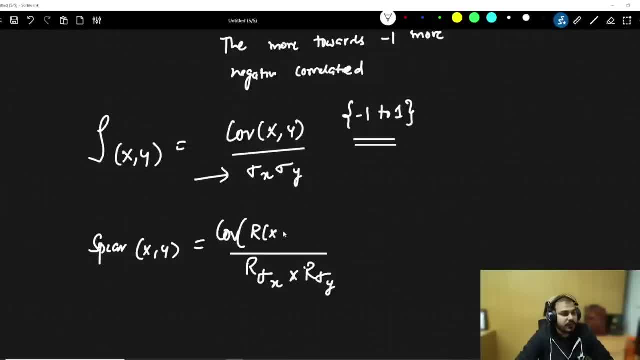 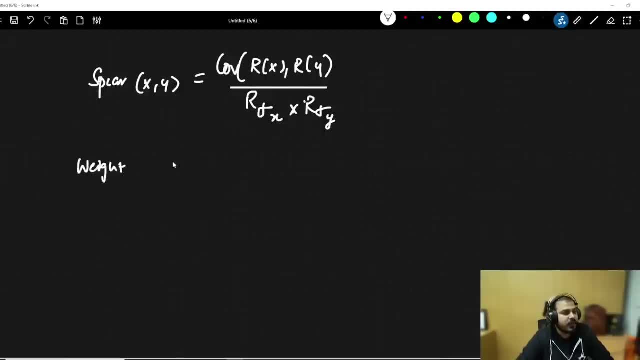 This will be covariance of covariance of rank of x, comma rank of y. Now, what is this? rank of x and rank of y? Let's consider that I have this feature: weight and probably age. If this is 170, the weight may be 45.. 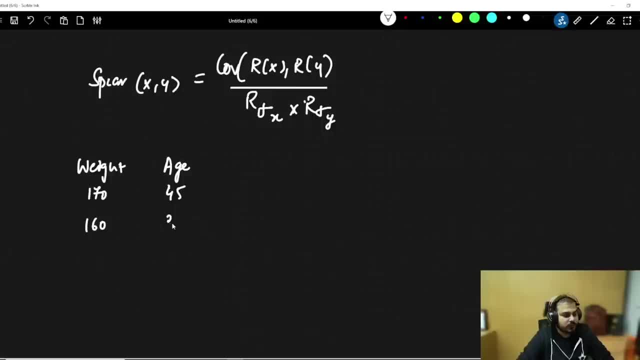 If it is 160,, 35. If it is 160, the weight- sorry, weight is too high. this is not possible. So I will just say height and weight. let's say So, if I say the height is 170, the weight may be 75 kgs. 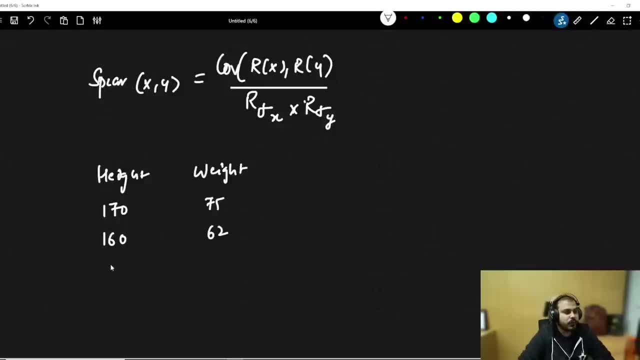 If I say height is 160, then the weight may be 62, 150, the weight may be 60, 145, the weight may be 55. Now, in this particular case, how do I define my rank? of this is my x, this is my y. 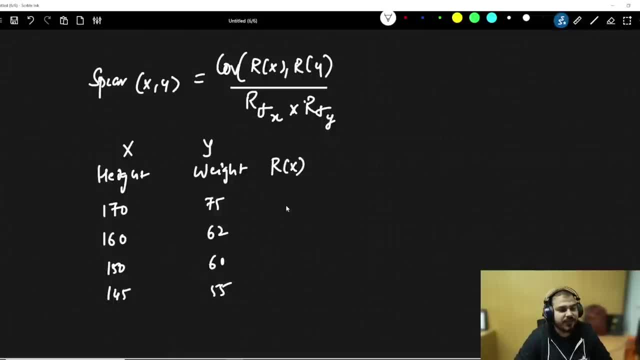 How do I define my rank of x? Now, rank of x is very, very simple. You just assign rank Over here. you have 4 points. Okay, which one? which value you want to give the highest rank? Go and see over here. this is having the highest value, right. 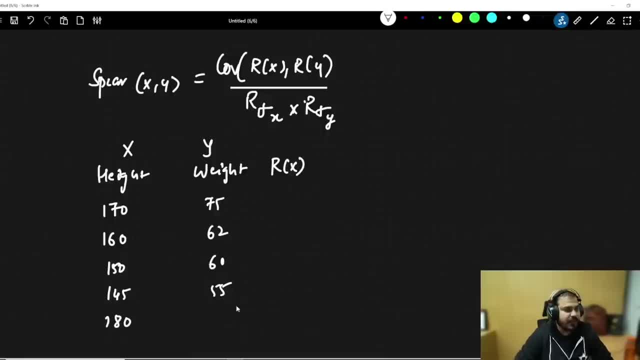 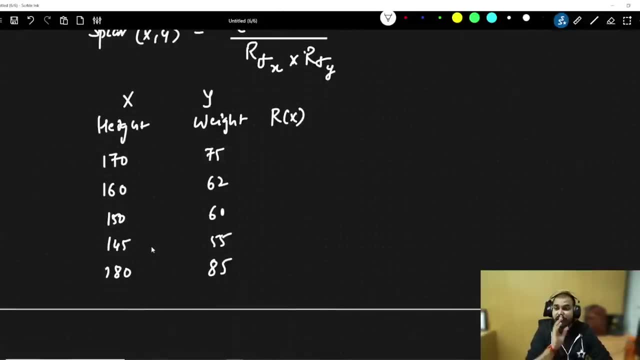 Highest value. Now let's say: let's consider that I have one more 180 and this will be 85.. Let's consider: in this you just need to convert this or you just need to assign rank to this particular data. Now rank basically gets applied to this. 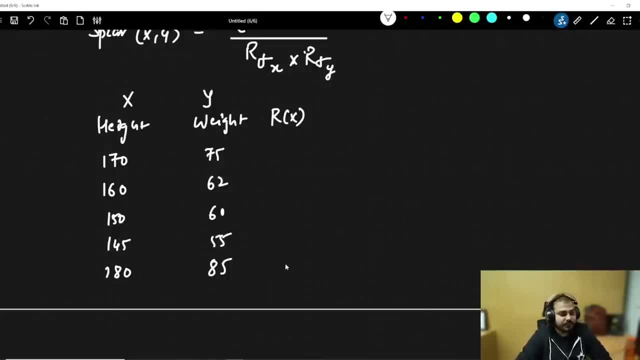 In height, if I say rank of x 180.. 180 is the highest right, So I may give this rank as 1. Then 170 is the next highest, Then 160 is the next highest, Then 150,, then 150,, 45, right. 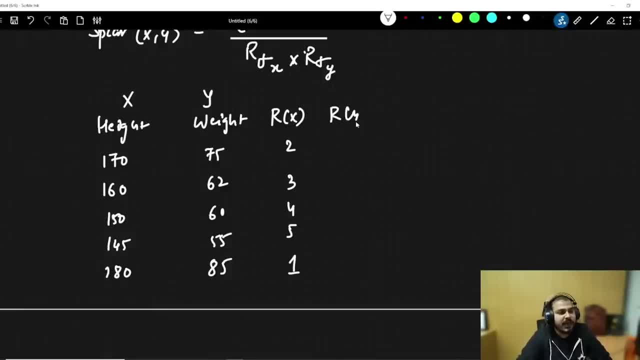 So here you will be able to see that I am assigning rank, And similarly I will go and assign rank for y. In this particular case my one rank is 85. Then you have 2, then you have probably 3,, then 4,, then 5,, like this: 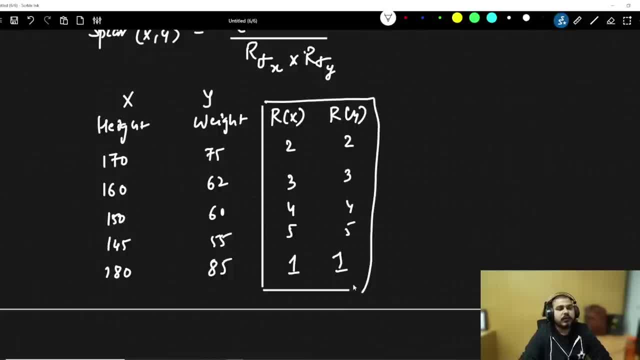 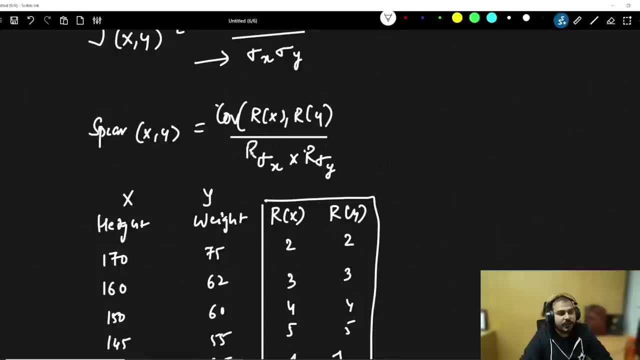 This rank will be basically used To do this calculation. That is the reason I told right: Covariance of rank of x and rank of y divided by standard deviation of rank of x and rank of y. So this value will be taken. this will be completely ignored. 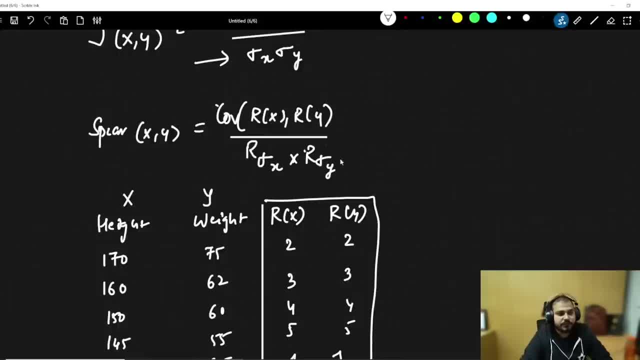 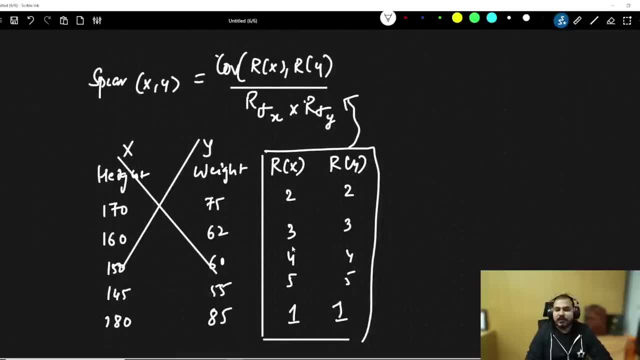 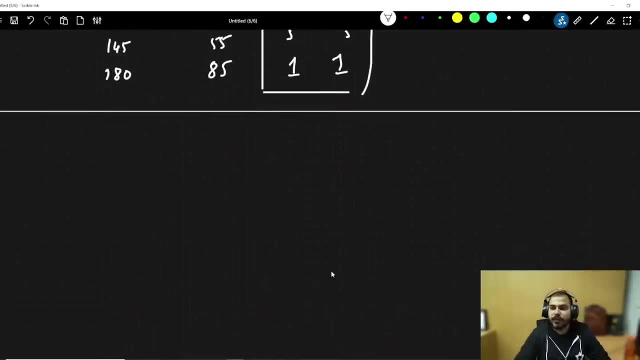 standard deviation of rank of x and rank of, so this value will be taken. this will be completely ignored. so this is what is basically the entire spearmint rank correlation and i hope you have understood. but understand if someone asks you: why do you use spearmint rank correlation coefficient? 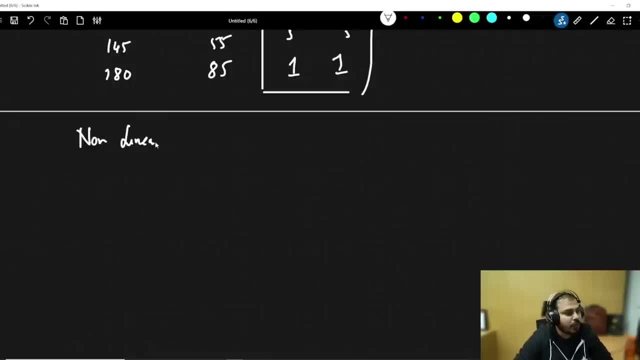 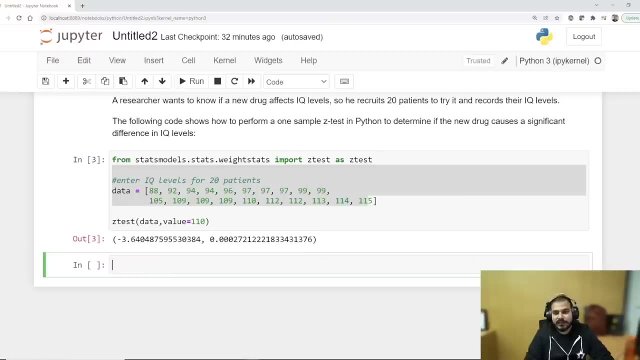 you should basically say that it captures the non-linear properties. it captures the non-linear properties. now let's go ahead and let's try to do this. one example: let's go and see something like t test and try to do it. let's say: let's see whether 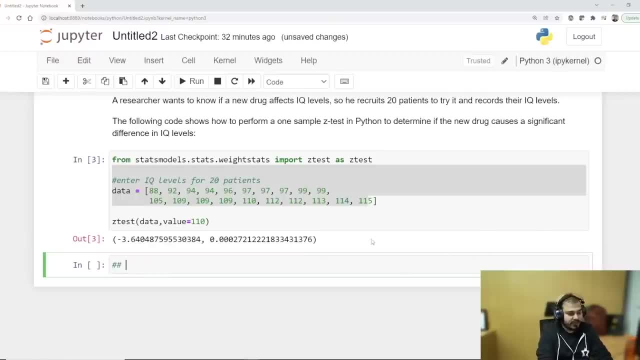 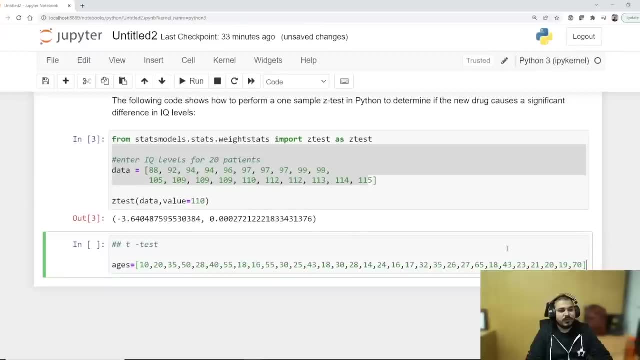 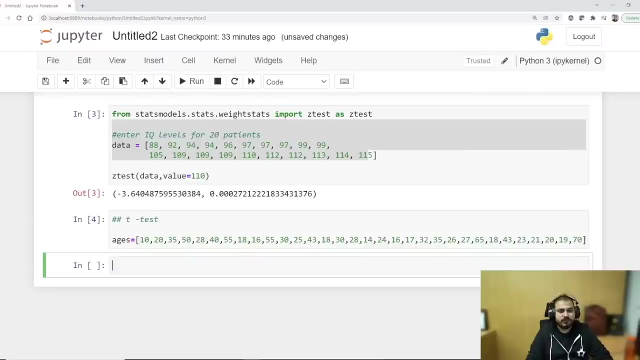 we'll be able to get or not. so here i'm actually going to show you t test, so suppose i have this ages. let's consider. i want to initialize this ages, so this is my ages. you can randomly initialize whatever you want, because we are just doing a hypothesis testing. okay, so it's up to you if you. 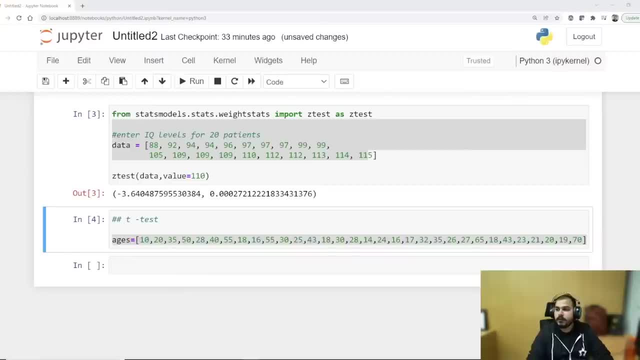 want this ages also, i can ping it in the chat. so this is the ages. now my main aim is that let's compute the mean of this ages. so ages underscore mean is equal to np dot mean of ages. so if i go and probably print ages underscore mean, so this is 30.34. 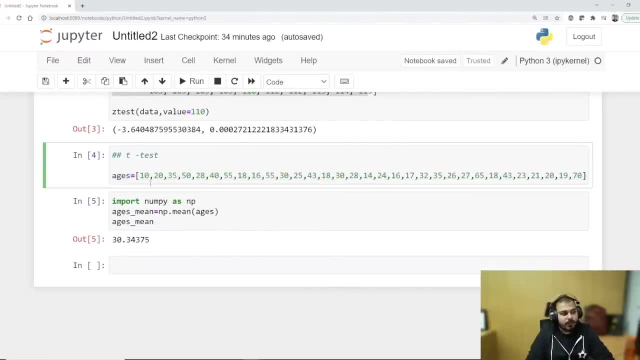 now let's, let's do one thing very simple from all these ages. let's consider that these are my population. i will just take a sample of age and then we will try to verify whether we are coming here to this mean or not using t test, because here we don't know the population standard. 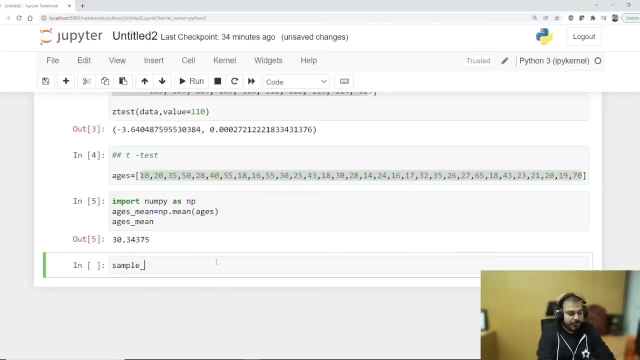 deviation. so let's do one thing. i'm just going to take my sample size as 10. this will basically be my sample size and i will just pick up all the sample from this particular ages. so i'm going to say np, dot, random dot choice. so here i'm just going to give my ages and this will basically. 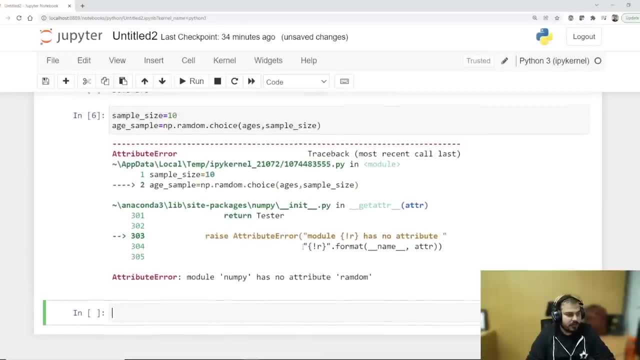 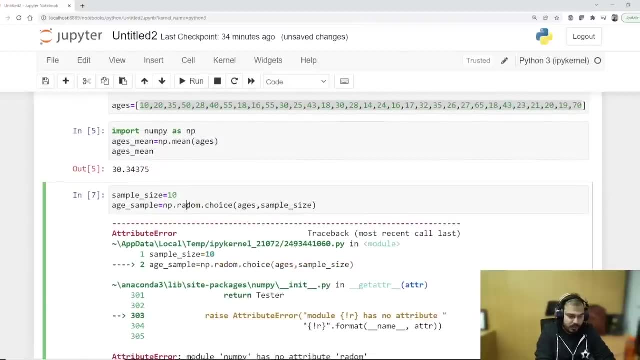 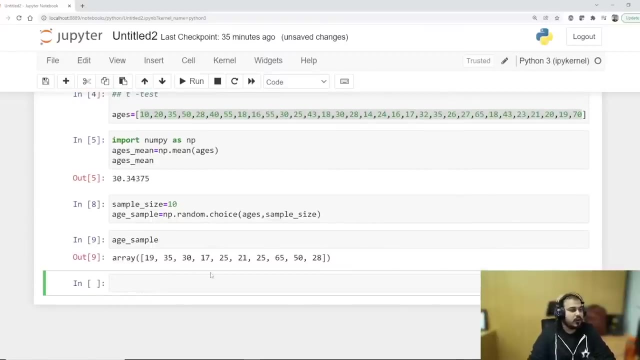 be my sample size. so if i, okay, i'm getting an error, okay, random, random, np dot- random, still error. okay, random, it became now insert, random, my goodness. so here now, if i go and show you my age underscore sample here, you'll be able to see that this ages have been picked. 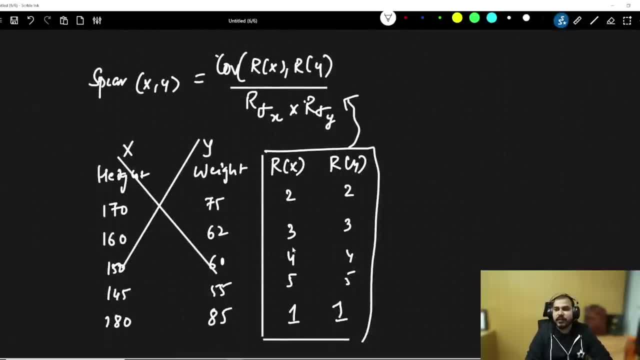 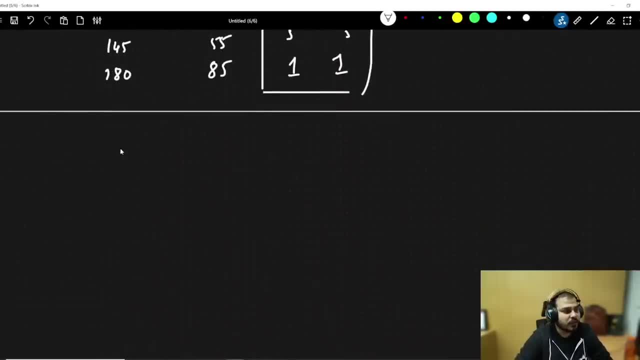 This is what is basically the entire Spearman Rank Correlation. I hope you have understood, But understand. if someone asks you why do you use Spearman Rank Correlation coefficient, you should basically say that it captures the nonlinear parameters. So I am just going to add this and this. 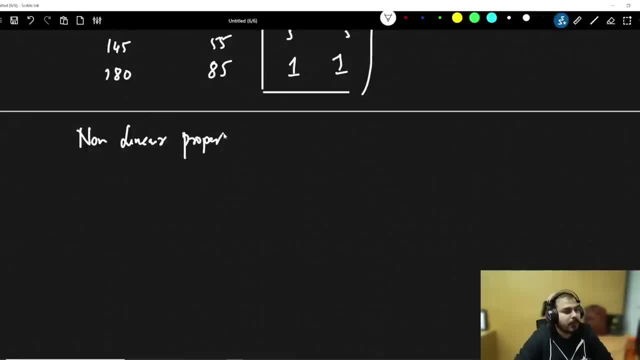 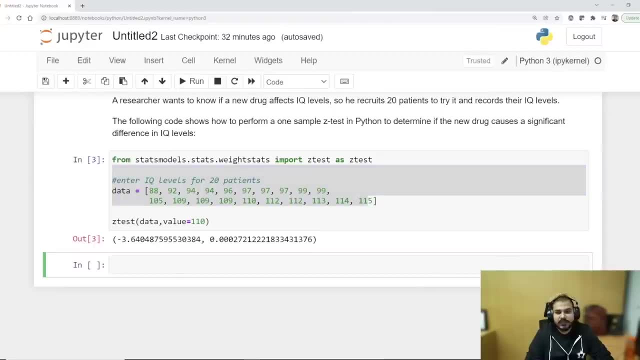 Here I have this properties: it captures the nonlinear properties. now let's go ahead and let's try to do this. one example: let's go and see something like t test and try to do it. uh, let's say, let's see whether we'll be able to get or not. so here i'm actually going to show you t test. so suppose i have this. 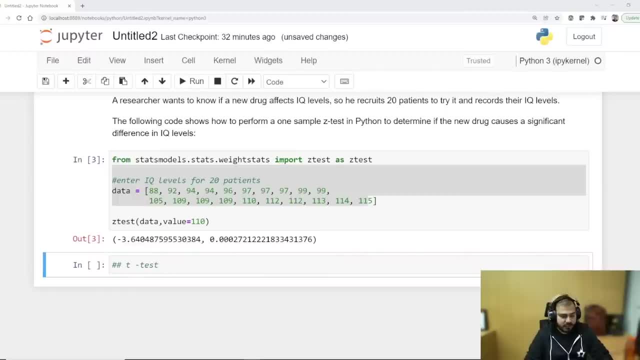 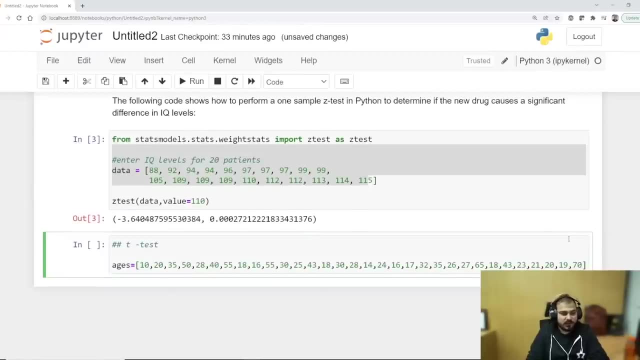 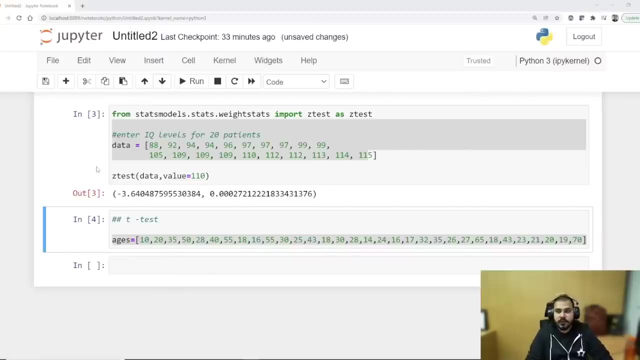 ages. let's consider: i want to initialize this ages, so this is my ages. you can randomly initialize whatever you want, because we are just doing a hypothesis testing, okay, so it's up to you. if you want this ages also, i can ping it in the chat. so this is the ages now. my main aim is that let's. 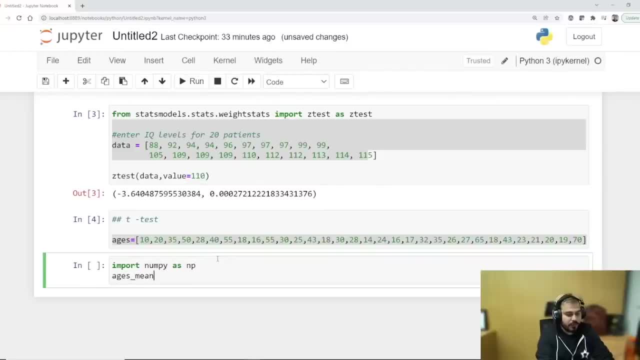 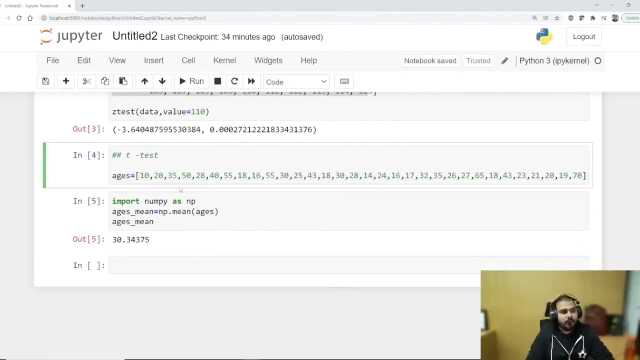 compute the mean of these ages. so ages underscore mean is equal to npmean of ages. so if i go and probably print ages underscore mean, so this is 30.34. now let's let's do one thing very simple. from all these ages, let's consider that these are my population. 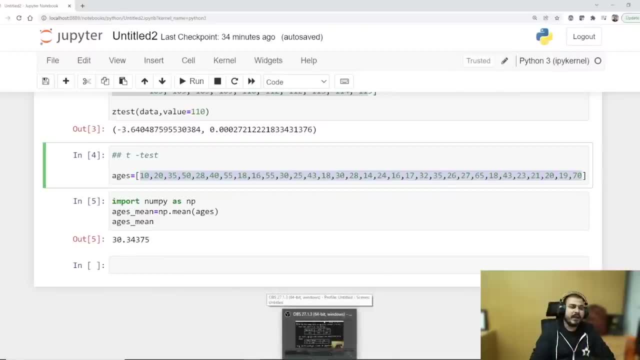 i will just take a sample of age and then we'll try to verify whether we are coming nearer to this mean or not using t test, because here we don't know the population standard deviation. so let's do one thing: i'm just going to take my sample size as 10. this will basically be my. 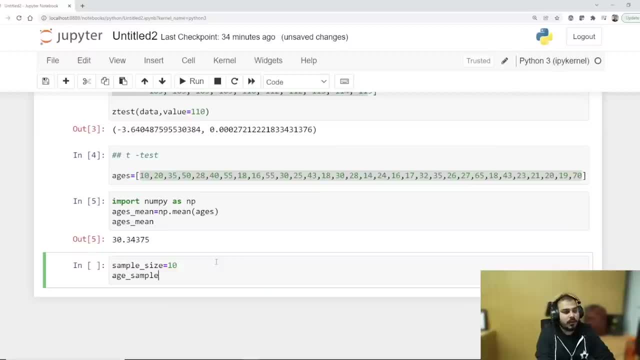 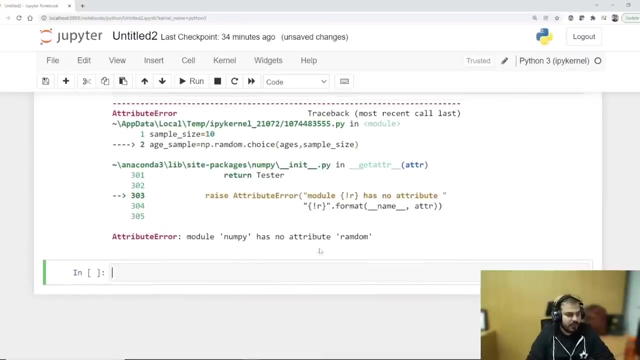 sample size and i will just pick up all the sample from this particular ages. so i'm going to say np, dot, random, dot, choice. so here i'm just going to give my edges and this will basically be my sample size. so if i okay, i'm getting an error. okay, random, random, np, dot, random, still error. 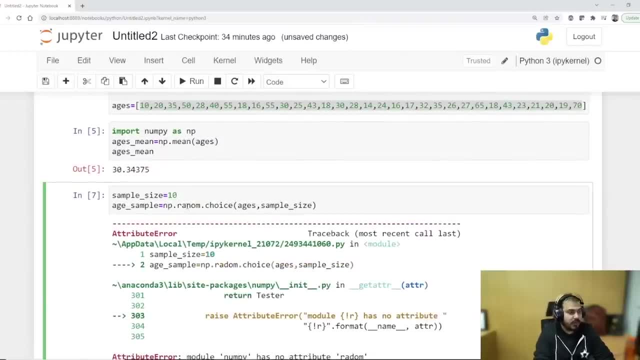 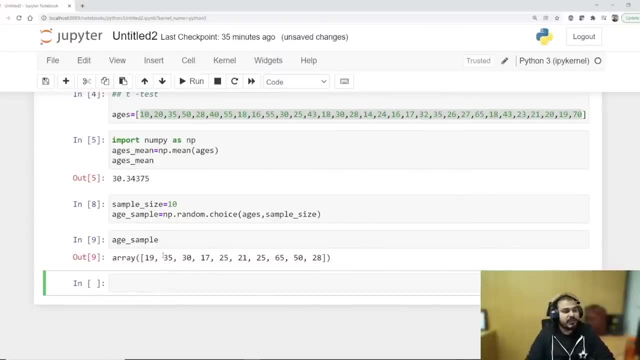 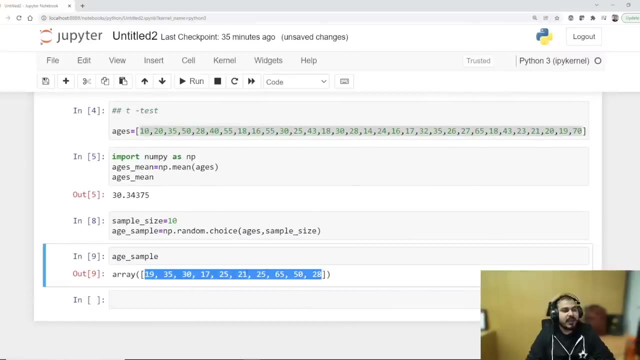 okay, random, it became now insert random, my goodness. so here now, if i go and show you my age underscore sample here, you'll be able to see that this ages have been picked. now can i basically whatever mean is basically coming from this? can i actually come near to this population, mean, with the help? 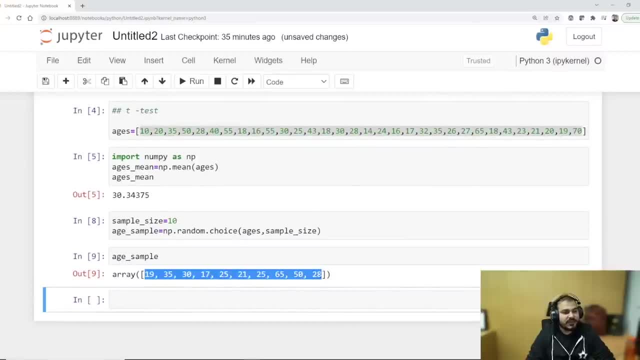 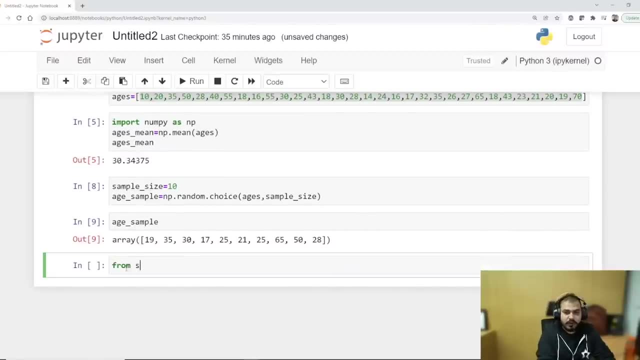 now, can i basically whatever mean is basically coming from this- can i actually come near to this population, mean with the help of t test? that is what i'm actually going. so i'm going to say from skypie dot stats import t test. underscore one sample. this we have done yesterday, okay. t test underscore one sample. 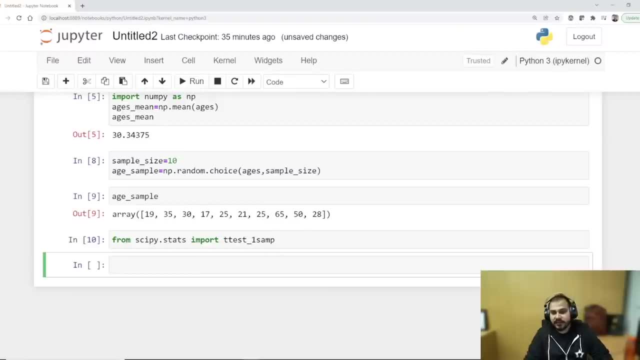 basically means one sample t test. that we have probably done yesterday. that is what we are going to do now: t test underscore one sam. here i'm basically going to give you two things. one is my age underscore sample and probably i want to give and compare with respect to this mean. 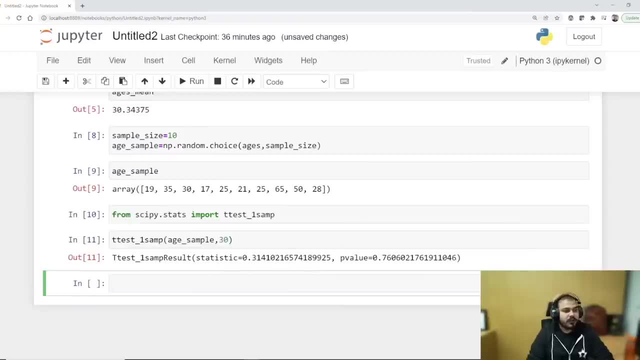 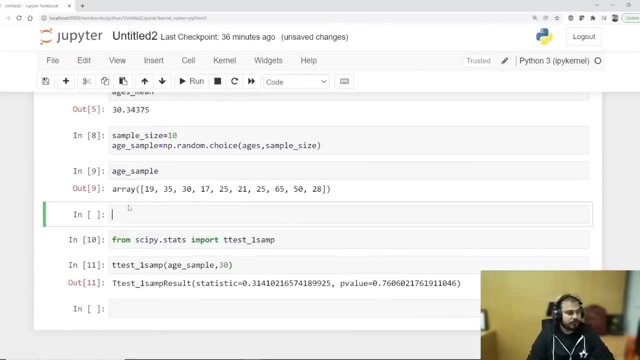 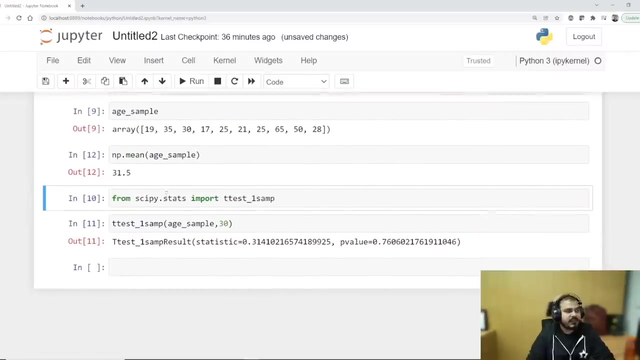 okay. so here i'm just going to give you 30. so here you can see that i'm getting the p value as 0.76. if you don't believe me, just go and compute the np dot mean of age underscore sample. i'm getting 31.5 right, which is little bit away from here. now it is up to you. i got the p value as: 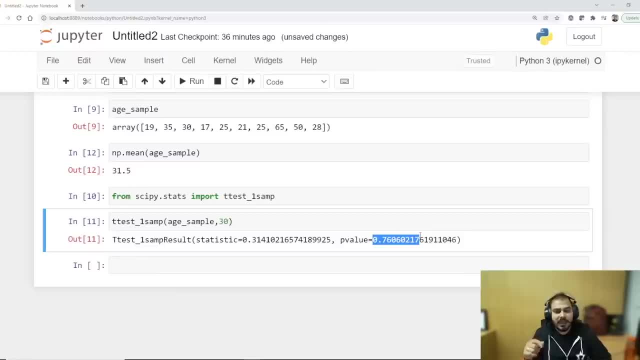 0.76. now, if i say my alpha value, my alpha value is 0.05. in this particular case, my p value is 0.75, so i'm getting the p value as 0.76. so i'm getting the p value as 0.75, so i'm getting the. 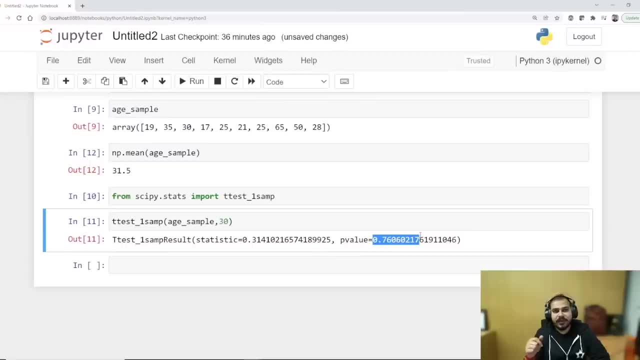 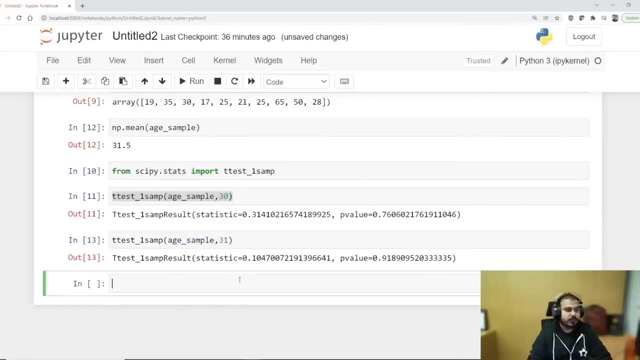 greater than the alpha value. so tell me whether it should be accepted or rejected. suppose if i execute the same code and i write sample size with respect to 31, now i'm getting 0.918. suppose if i execute with respect to this and i take up with my sample as 28, now i'm getting 0.48. 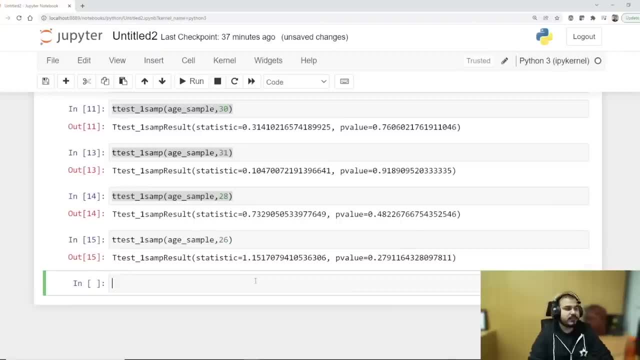 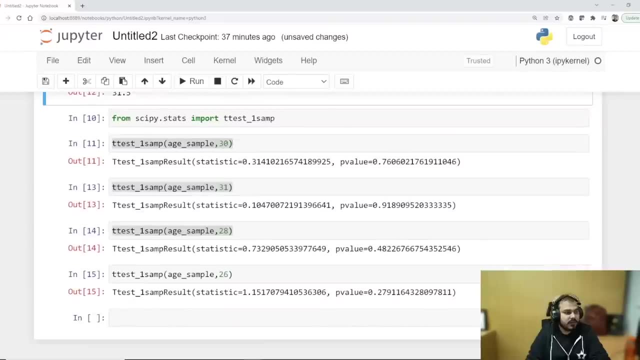 if i keep on doing this and make it to 26, here you'll be able to see 0.27. so this is with respect to different, different things. i can also even change this. now, if i go and execute this, here i'm getting 0.60. here i'm getting 0.45. here i'm getting 0.96. 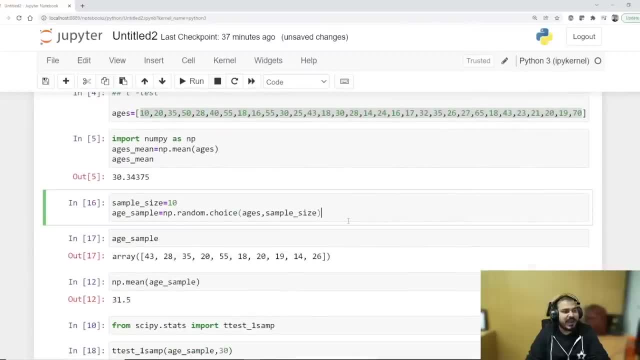 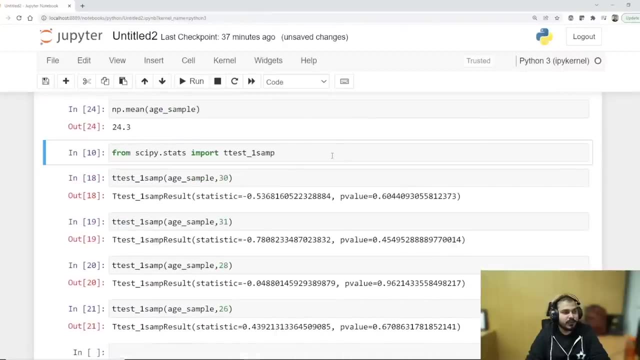 here i'm getting 0.67. if i try to change this random value again and again. let's say that i've taken now different sample. my sample is mean is nothing but 24.3. now if i execute this, this is 0.015. 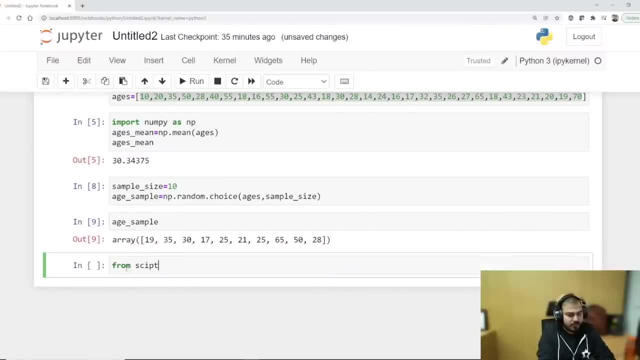 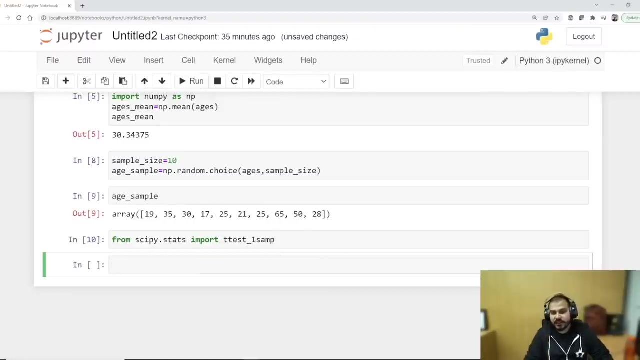 of t test. that is what i'm actually going. so i'm going to say: from skypy dot stats import t test underscore one sample. this we have done yesterday. okay, t test underscore one sample basically means one sample t test that we have probably done yesterday. that is what we are going. 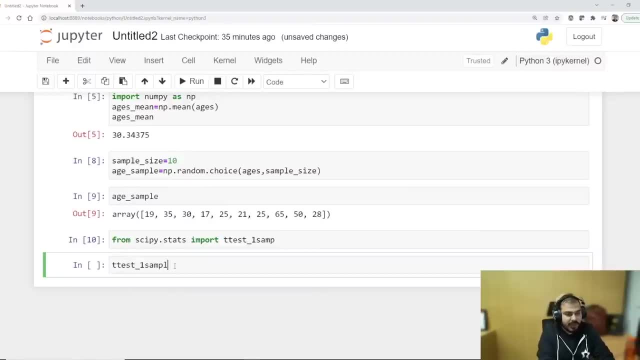 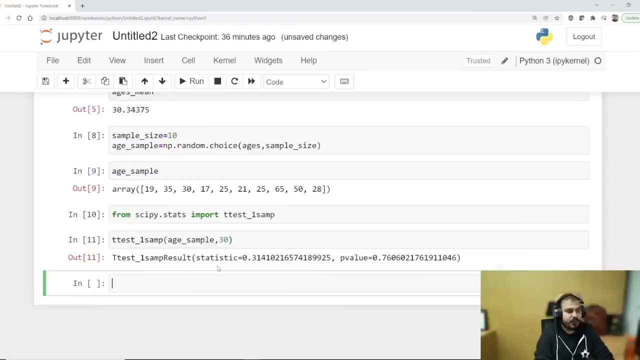 to do now: t test underscore one stamp. here i'm basically going to give you two things. one is my age underscore sample. i'm probably. i want to give and compare with respect to this mean okay, so here i'm just going to give you 30. so here you can see that i'm getting the p value as 0.76. 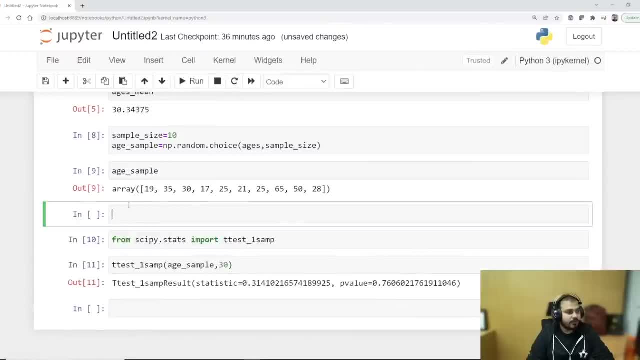 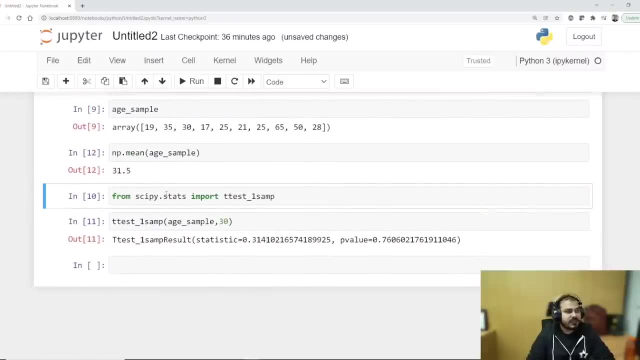 if you don't believe me, just go and compute the np dot mean of age underscore sample. i'm getting 31.5, right, Which is little bit away from here. Now it is up to you. I got the p-value as 0.76.. 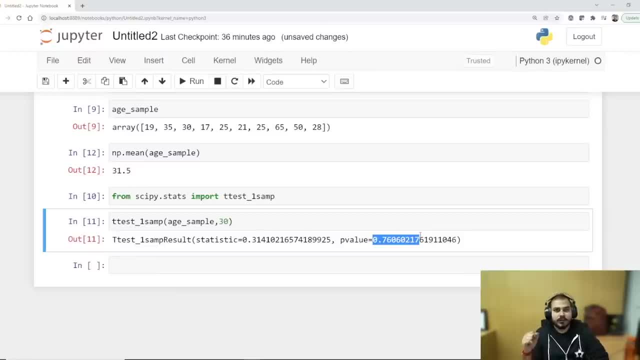 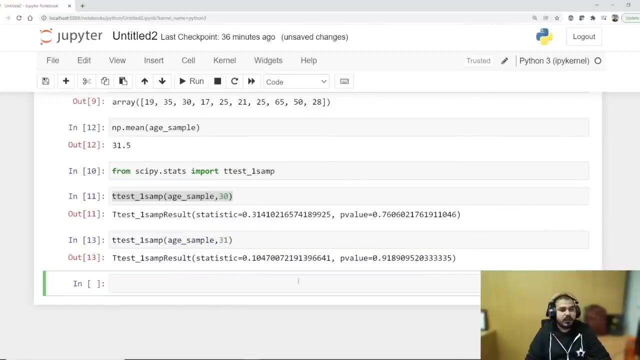 Now, if I say my alpha value, my alpha value is 0.05.. In this particular case, my p-value is greater than the alpha value, So tell me whether it should be accepted or rejected. Suppose if I execute the same code and I write sample size with respect to 31.. Now I'm getting 0.918.. Suppose 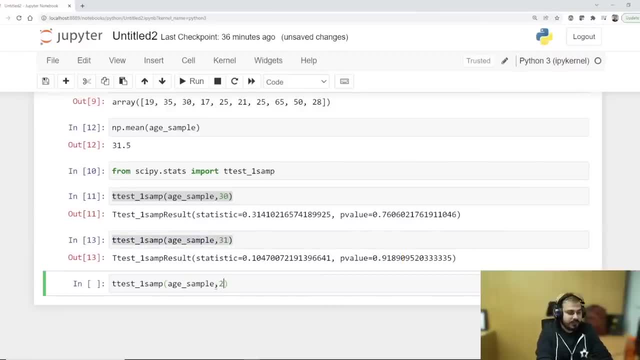 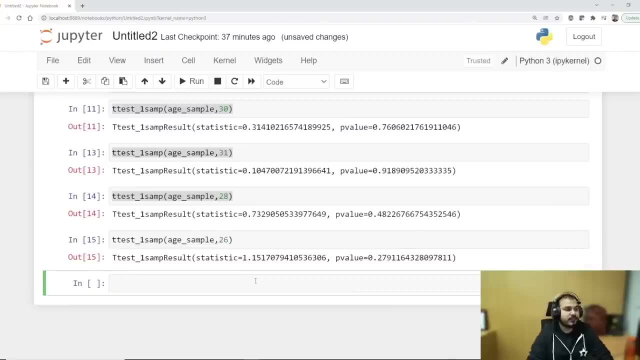 if I execute with respect to this and I take up with my sample as 28.. Now I'm getting 0.48.. If I keep on doing this and make it to 26,, here you'll be able to see 0.27.. So this is with respect. 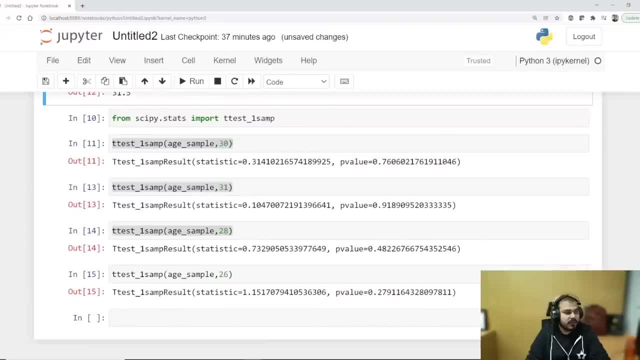 to different, different things. I can also even change this. Now, if I go and execute this, here I'm getting 0.60.. Here I'm getting 0.45.. Here I'm getting 0.96.. Here I'm getting 0.67.. If I try to, 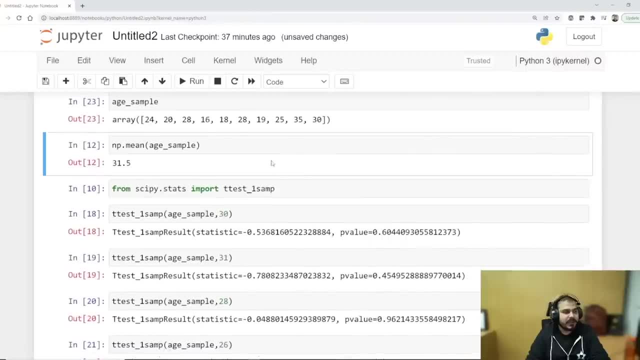 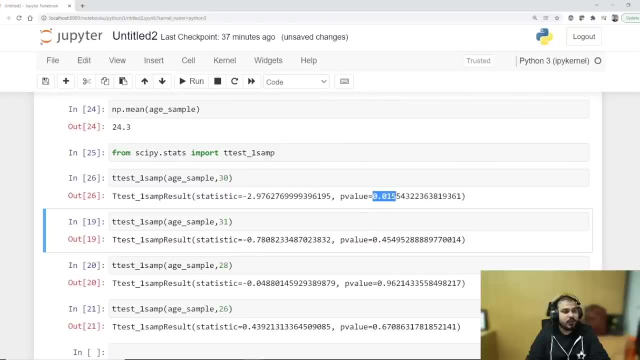 change this random value again and again. Let's see. Let's say that I have taken now different sample. My sample is mean is nothing but 24.3.. Now, if I execute this, this is 0.015.. It is, tell me, 0.05, right, Greater than 0.05. 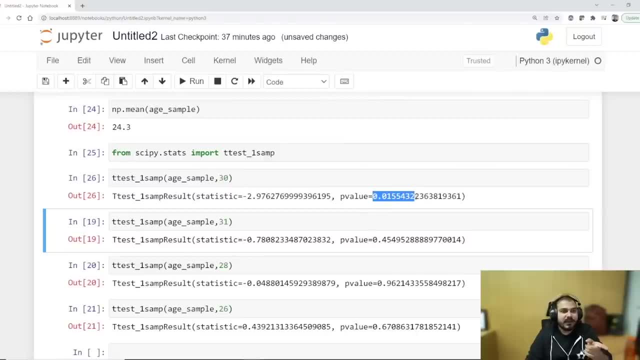 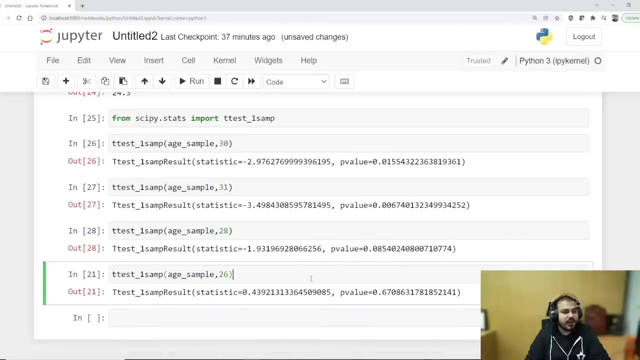 it is, tell me 0.05 right, greater than 0.05 or less than 0.05? now, in this particular case, it is equal to 0.006. if i say with respect to 31, this is 0.006. it is within that confidence interval or not? similarly, if i go and see with respect to 28, 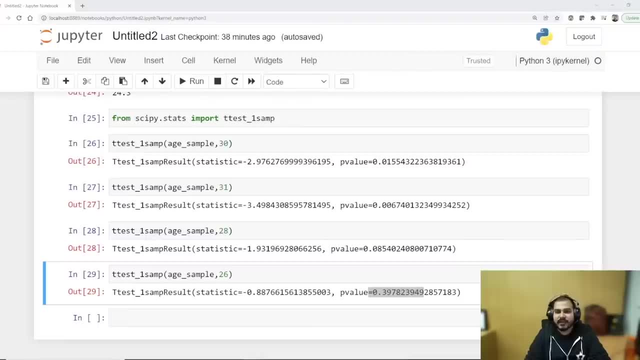 0.085- 0.397. so here you can basically see- and here i have just taken a small example, here i have just taken a small example- usually, in the main scenario, you will basically have a huge data set to check out all this particular things. so this was an example with respect to t-test. 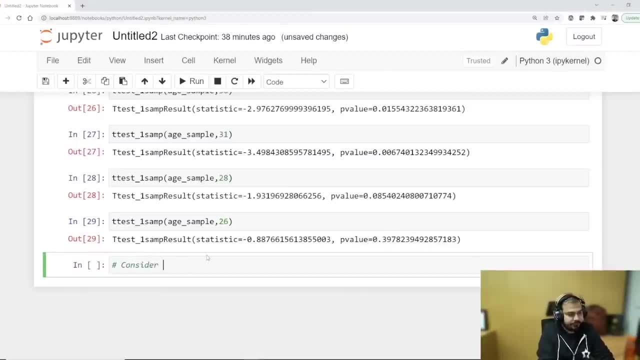 have a problem statement. i will consider. so. my example is that suppose i take college, the ages of the entire college student. suppose i take ages of the college student, of the college student. now what i'm going to do? i'm going to take the class, let's say one class students ages. i'm going to 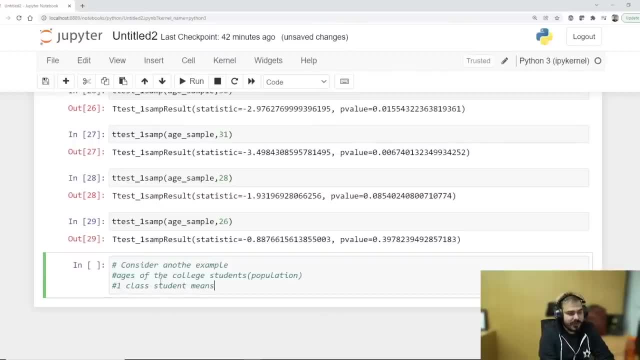 take student i'm going to take, and then i'll probably find the mean of all the ages and then we'll try to compare whether this will be able to give that specific output. basically, can we come to the population mean ages of the college student? that is what i'm actually trying to. so, first of 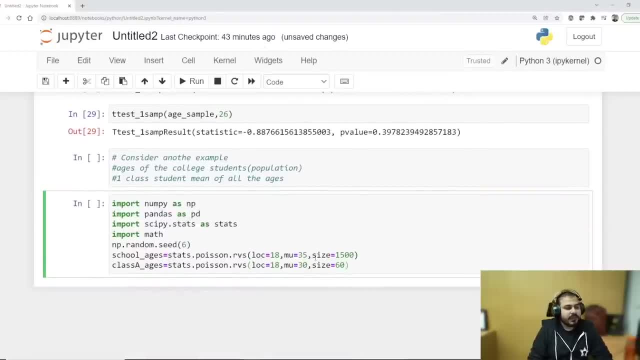 all. let's say that i'm having this code. let's say this is there now. everybody focus on the code here. this is a poison distribution. it is just saying that you have to start from 18 age and the mean is 35 and we are going to consider our population ages as 1500. then we are basically considering class a, with 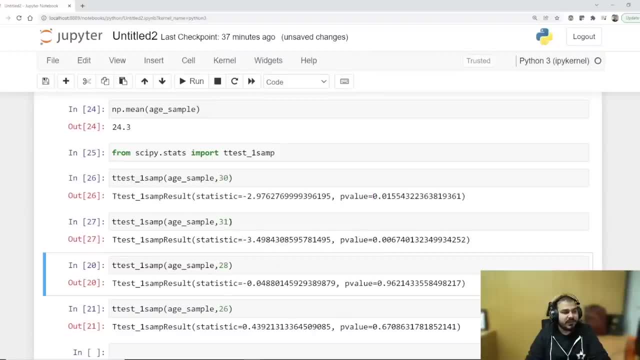 or less than 0.05.. Now, in this particular case it is, if I say with respect to 31,, this is 0.006.. It is within that confidence interval or not? Similarly, if I go and see with respect to 28,, 0.085,, 0.397.. So here you can basically 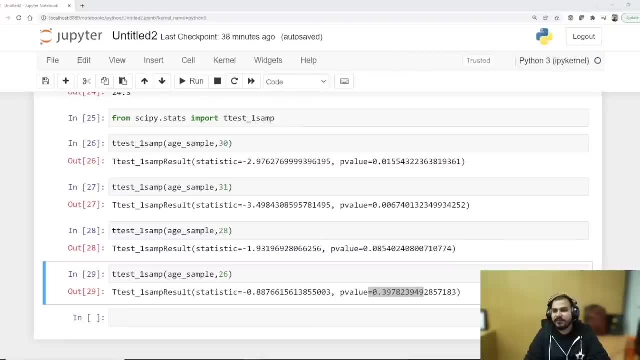 see- and here I've just taken a small example- here I have just taken a small example- Usually, in the main scenario, you will basically have a huge data set to check out all this particular things. So this was an example with respect to Ttest. 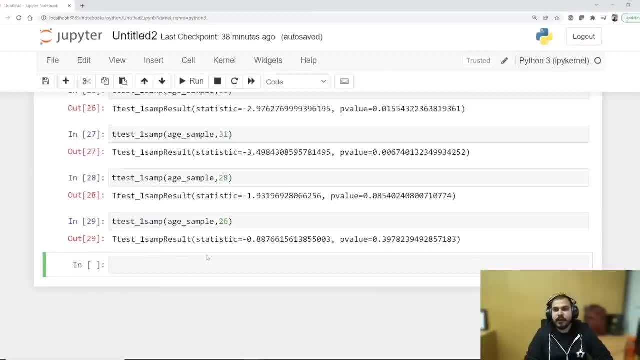 Let's take one more example. Now I have a problem statement I will consider. So my example is that suppose I take college, that ages of the entire college student. suppose I take ages Here they are excellent fotos of 4 correct questions. All They are in their own. 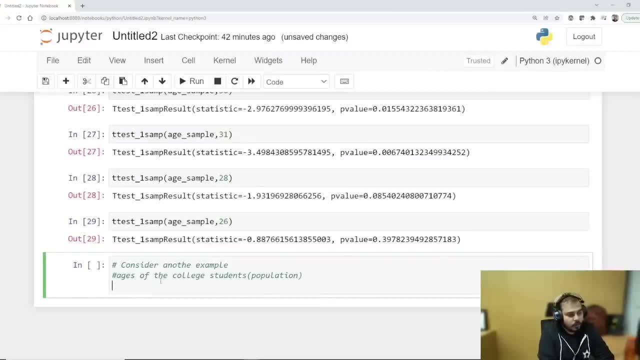 the college student of the college student. now what i'm going to do, i'm going to take the class. let's say one class, students ages i'm going to take, student i'm going to take, and then i'll probably find the mean of all the ages and then we'll try to compare whether this will be able. 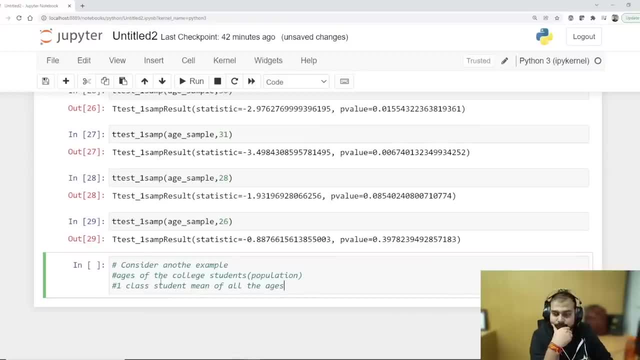 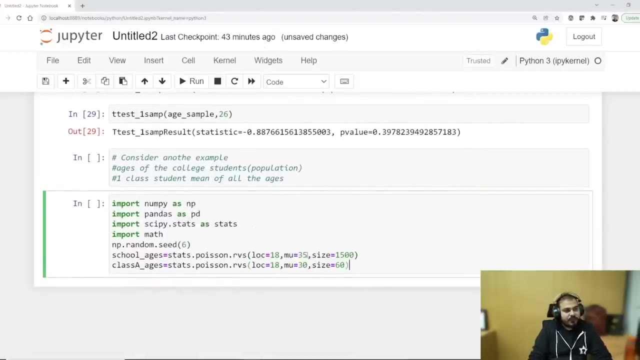 to give that specific uh output. basically, can we come to the population- mean uh ages- of the college student? that is what i'm actually trying to do. so first of all, let's say that i'm having this code. let's say: this is there now. everybody focus on the code here. this is a poison distribution. 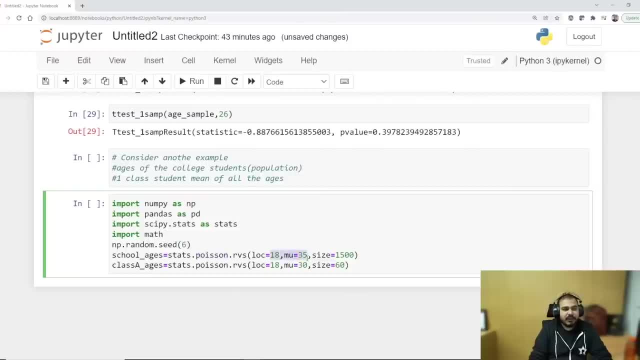 uh, it is just saying that you have to start from 18 age and the mean is 35 and we are going to consider our population ages as 1500. then we are basically considering class a with, uh, starting age as 18, mean as 30 and size: that's the last class class. we're going to consider our population ages as 1500. 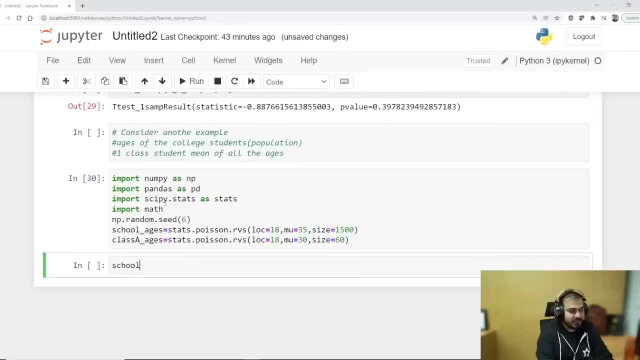 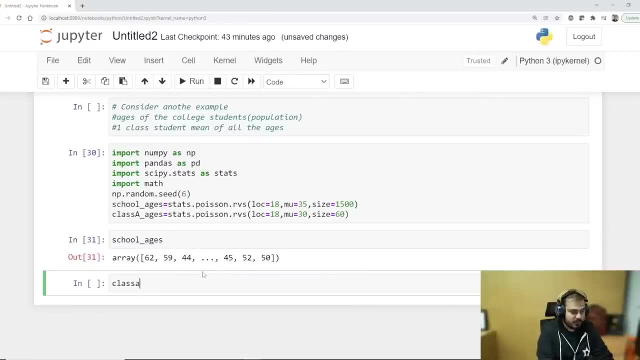 and the mean is 35 and we are going to consider our population ages as 1500. that's the last class. class is only 60 sample. so in this particular case, if i go and see school underscore ages, here is my value and similarly, if i go and see class a underscore ages, so this is my class a underscore ages, which. 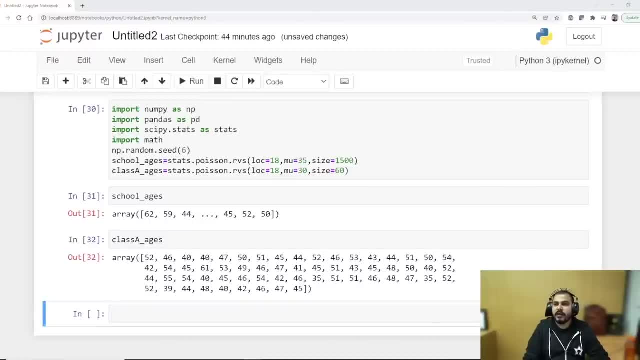 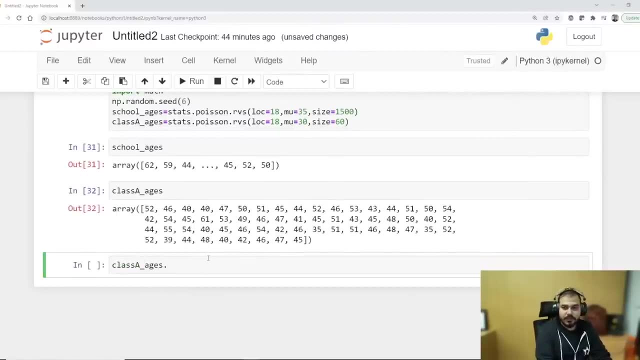 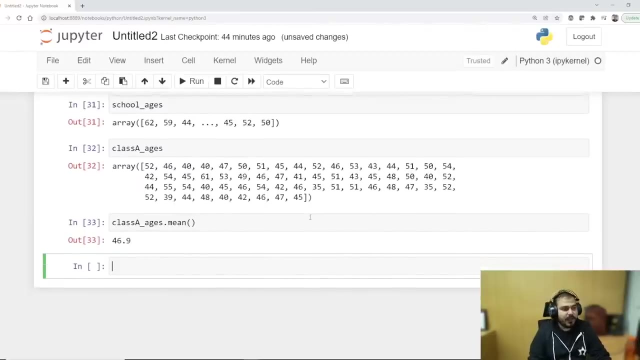 are basically my 60 data. now let's do something. uh, one amazing thing. first of all, let's try to find out the class a underscore, ages dot mean. so here you can see that it is 46.9. now what i am actually going to do? i'm basically going to apply again this t test, t test one, sam, and here my first. 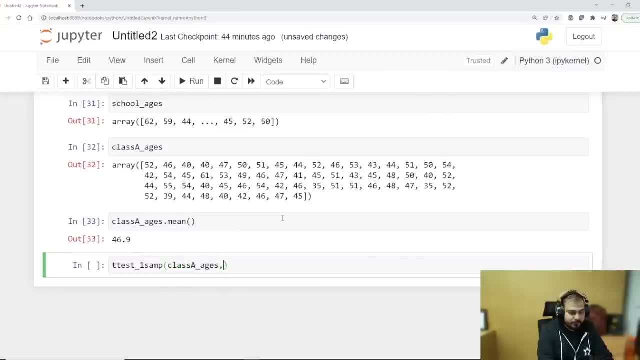 data will basically be my class, a, ages, and then the second parameter will basically be my mean, my mean. i will try to give this specific mean, school underscore ages, dot mean. so this will be a parameter. if i go and see away and press shift tab, you will be able to see that. the second 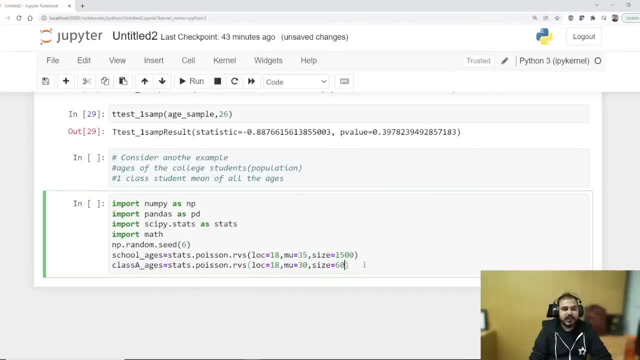 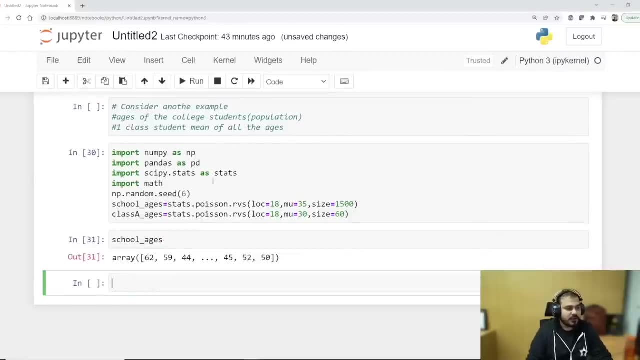 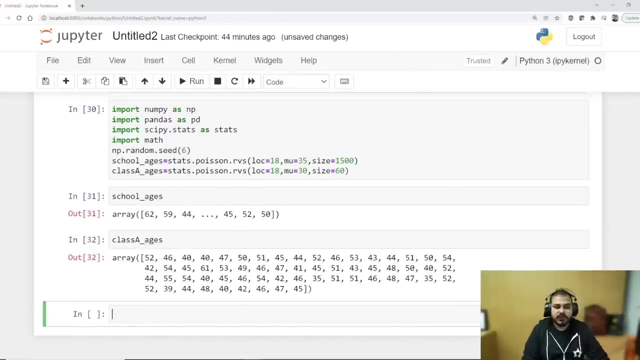 starting age as 18, mean as 30, and size: that is only 60 sample. so, in this particular case, if i go and see school underscore ages, here is my value and similarly, if i go and see class a underscore ages, so this is my class a underscore ages, which are basically my 60 data. now let's do something. 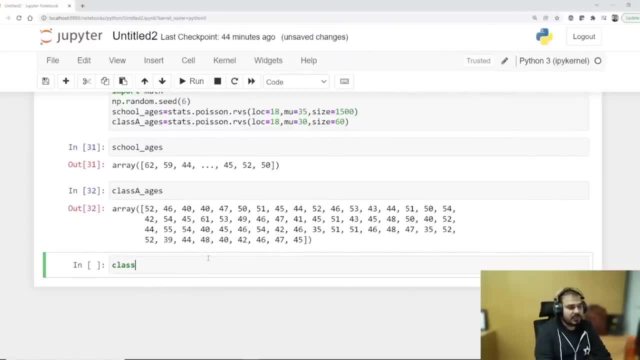 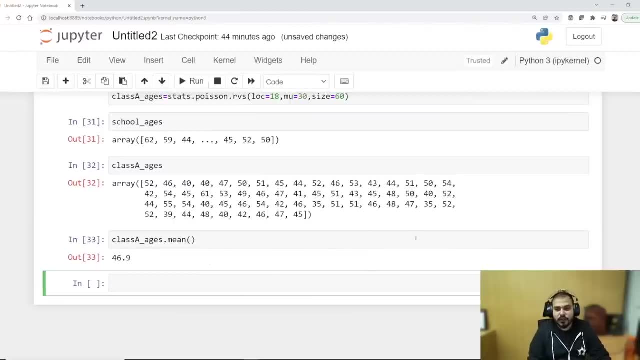 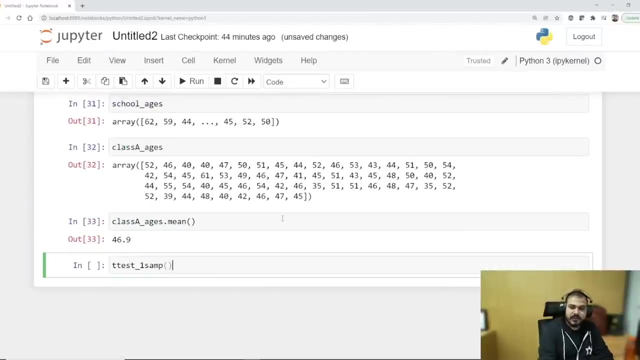 first of all, let's try to find out the class a underscore ages dot mean. so here you can see that it is 46.9. now what i am actually going to do? i'm basically going to apply again this t test, t test one, sam, and here my first data will basically be my class a, ages, and then the second parameter will. 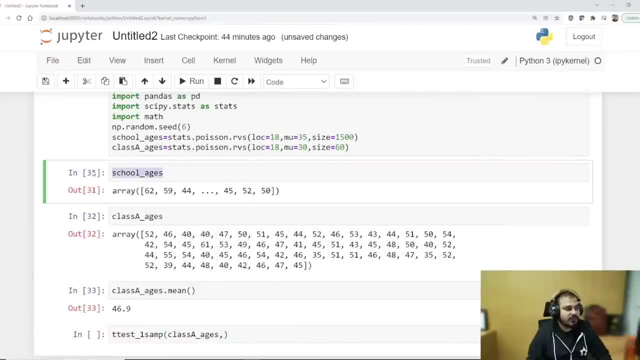 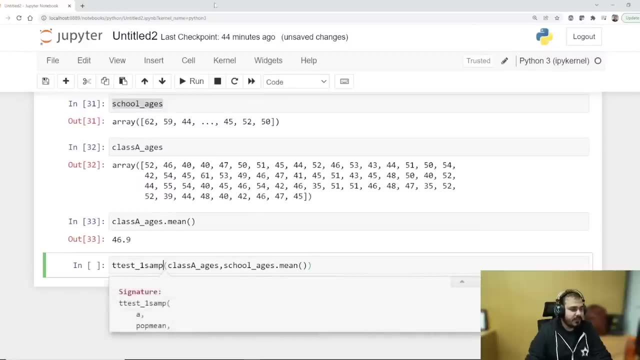 basically be my mean, my mean. i will try to give this specific mean, school underscore, ages, dot mean. this will be a parameter. if i go and see away and press shift tab, you will be able to see that the second parameter i have to give as mean, this is nothing but my pop mean. now, here you can see that i am getting. 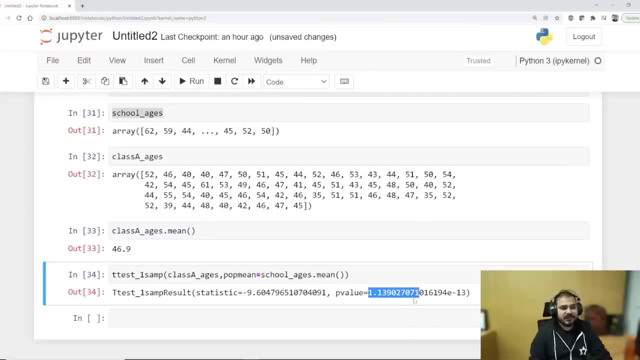 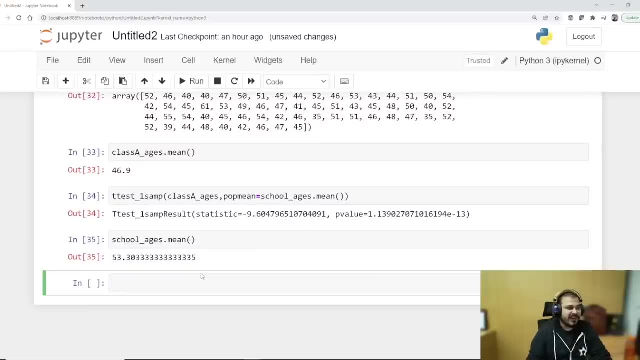 the p value as this one. so tell me whether this needs to be accepted or rejected. and if i go and probably see the school ages mean this far away. right, it is 46.9 and this is 53. if you are considering, alpha is 0.05, it will obviously be very, very so. similarly, you have to reject it, guys. 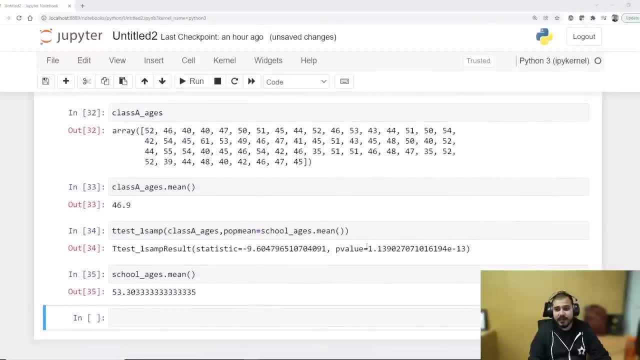 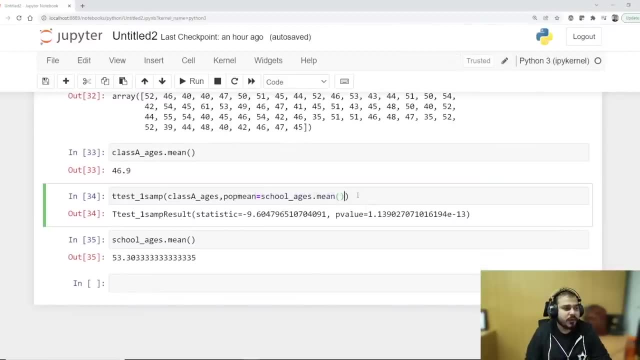 not accept it. okay, because this is way higher than that. you have to basically get p value less than the significance. let's say that i am putting this nearer to nearer to the class a. mean let's see what will happen. 47- it is coming, coming somewhere here. oh sorry, i have to give this as my sample mean. so 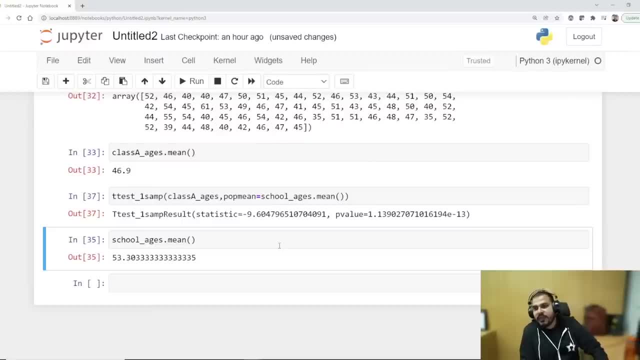 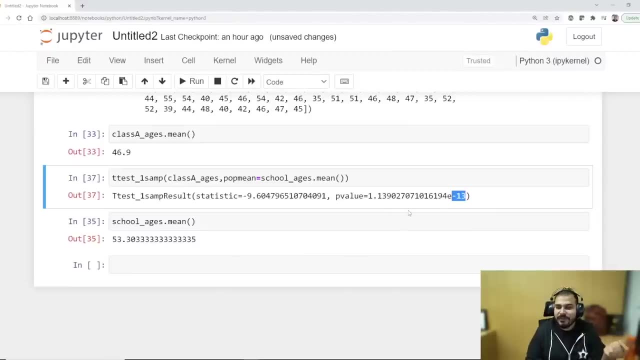 like this. you can basically check out all the things and verify it. whatever we have done, we have done. it is 10 raised to minus 13. it should not be rejected. guys, it is 10 raised to minus 13. i'm extremely sorry. it should not be rejected. so that is the. 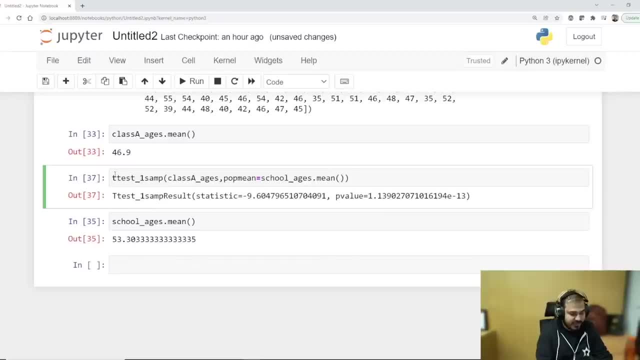 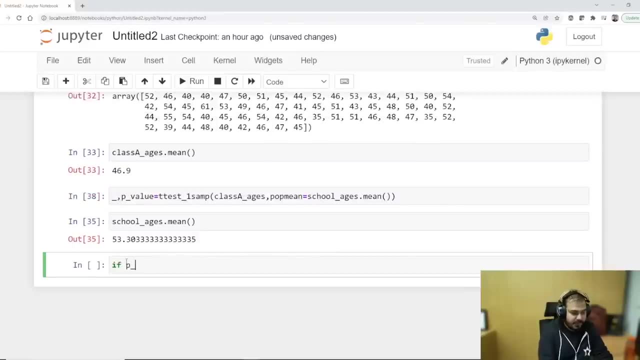 reason what we do we can put. if so, here i will just say underscore comma: p underscore value is equal to this. so if i say if p underscore value is less than 0.05, then what we do print accept h0. so what i am actually getting over here? 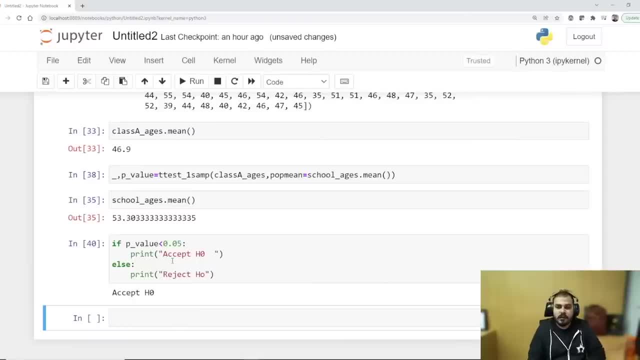 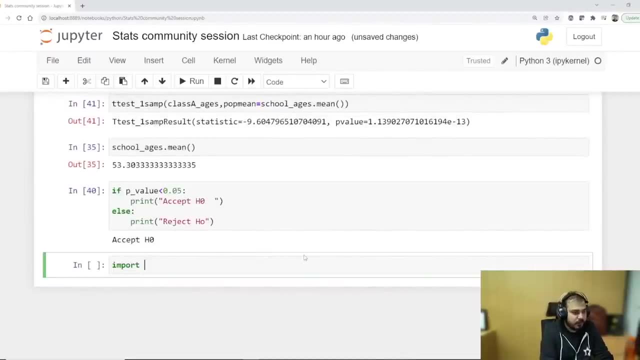 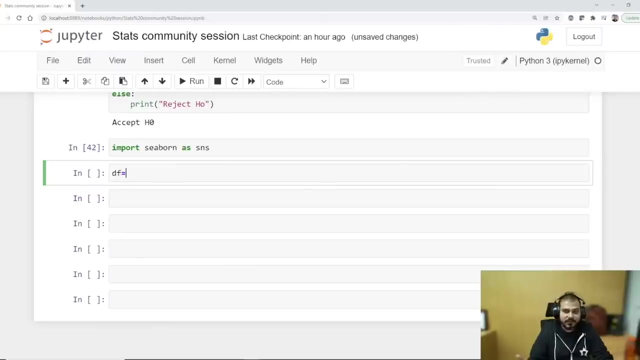 okay, guys. okay, one more final thing that i probably missed out. let's say that i'm using c bond, so df is equal to, because i need to show you correlation and all also, so we'll check out that also, so that you'll be able to check it out. okay, so sns dot load underscore data set. let's consider: 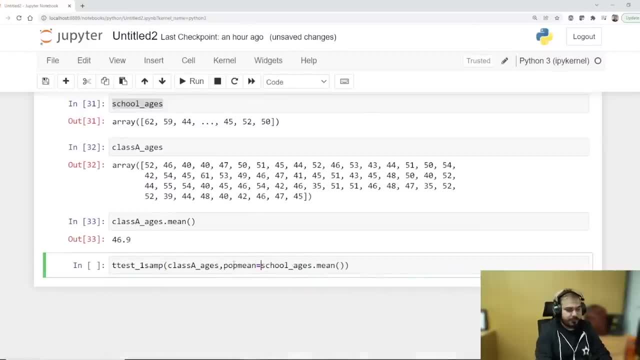 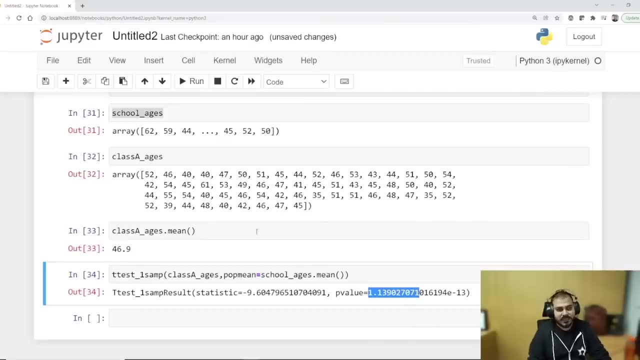 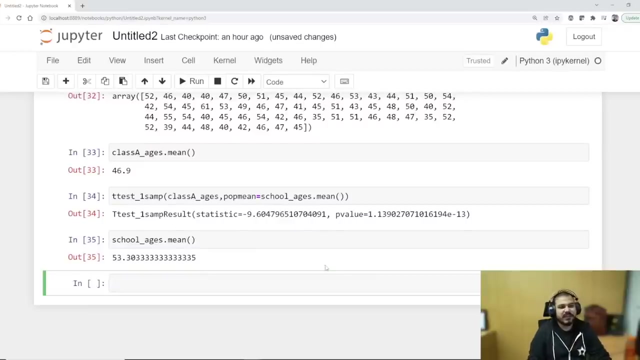 parameter i have to give us mean this is nothing but my pop mean. now here you can see that i'm getting the p value as this one, so tell me whether this needs to be accepted or rejected. and if i go and probably see the school ages mean this far away, right, it is 46.9 and this is 53 if you're considering alpha. 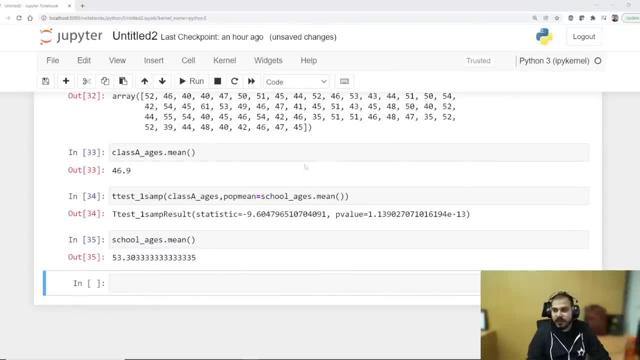 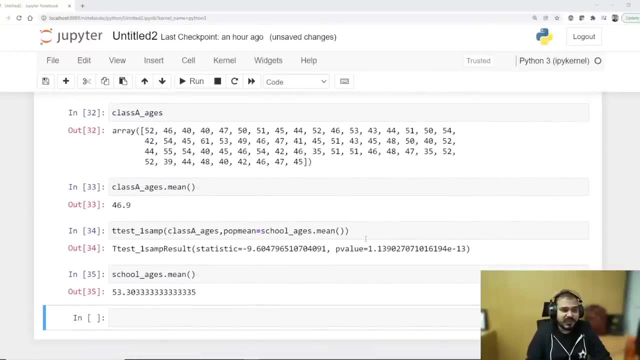 is 0.05, it will obviously be very, very so. similarly, you have to reject it, guys, not accept it, okay, because this is way higher than that. you have to basically get p value less than the significance. let's say that i am putting this nearer to. 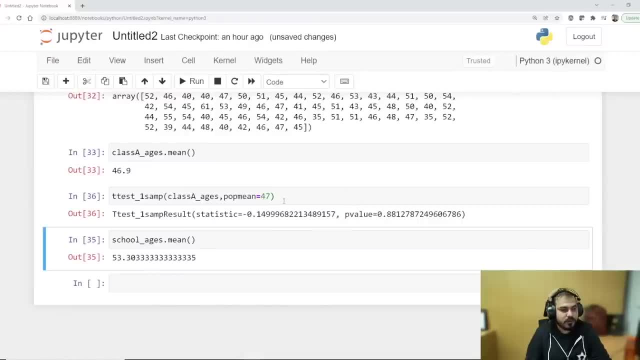 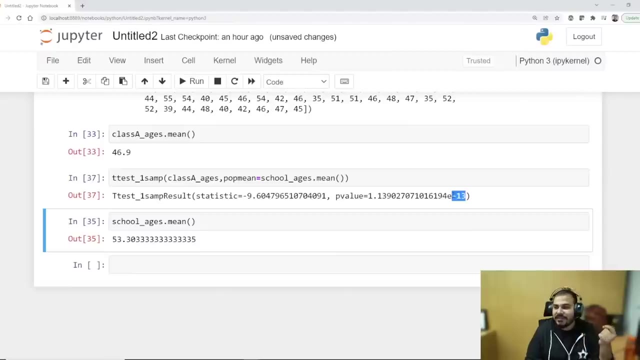 nearer to the class a mean. let's see what will happen. 47. it is coming coming somewhere here. oh sorry, i have to give this as my sample mean. so like this, you can basically check out all the things and verify it. whatever we have done, we have done. it is 10 raised to minus 13. it should. 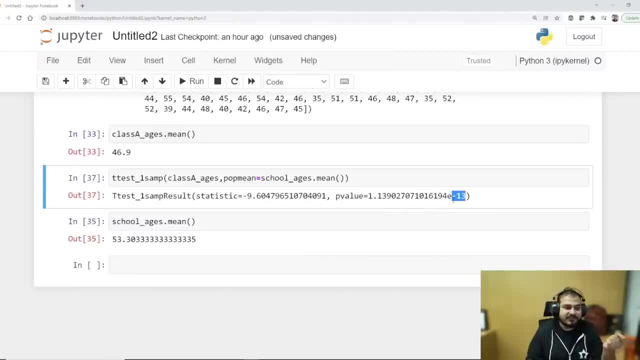 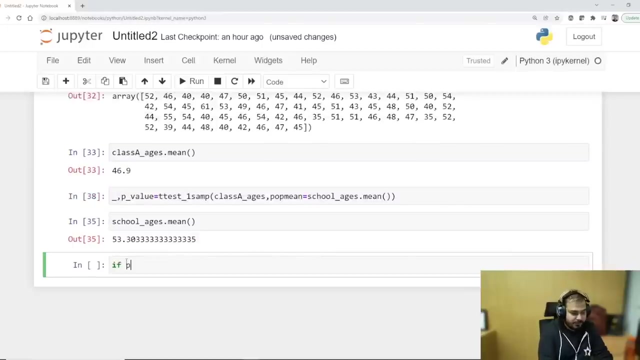 not be rejected, guys. it is 10 raised to minus 13. i'm extremely sorry, it should not be rejected. so that is the reason what we do. we can put, if so, here i will just say: underscore comma: p underscore value is equal to this. so if i say if p underscore value is less, 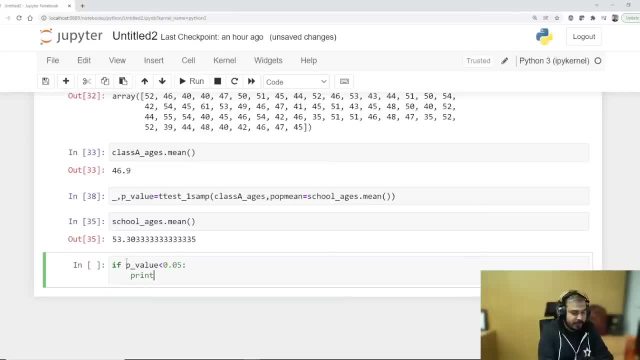 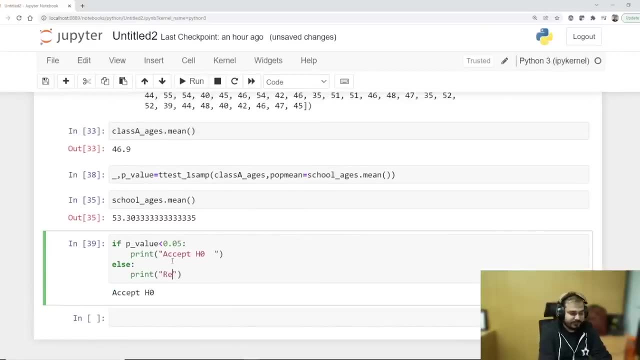 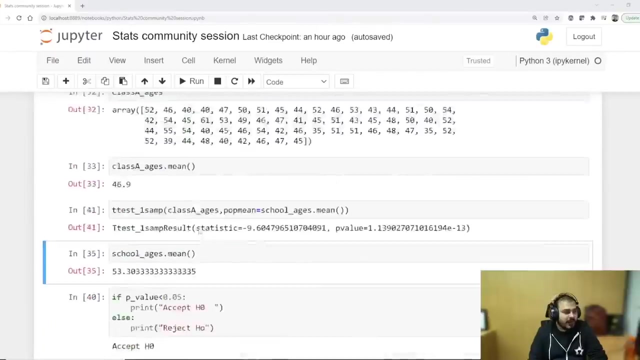 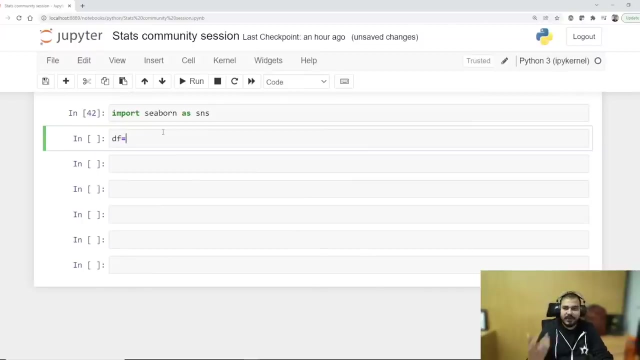 than 0.05, then what we do print accept h0. so what i'm actually getting over here, okay, guys? okay, one more final thing that i probably missed out. let's say that i'm using c bond, so df is equal to, because i need to show you correlation and all also, so we'll check out. 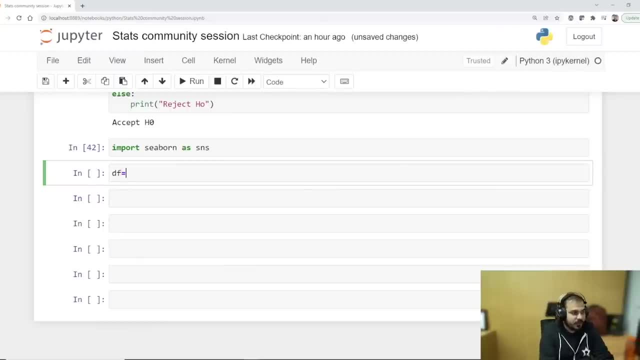 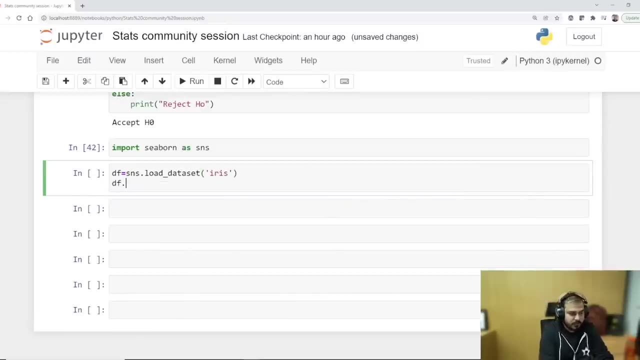 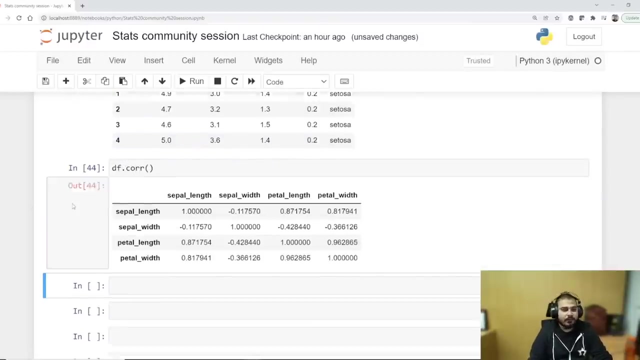 that also, so that you'll be able to check it out. okay, so sns dot load underscore data set. let's consider that i'm going to use iris data set, so this will be my df dot head. so if i use the correlation df dot corr. so this is how my diagram looks like. here you can see that it is basically. 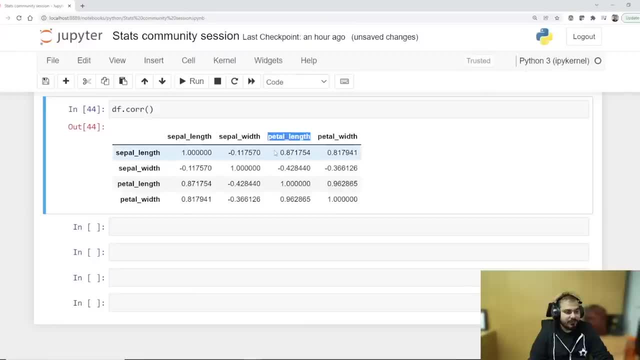 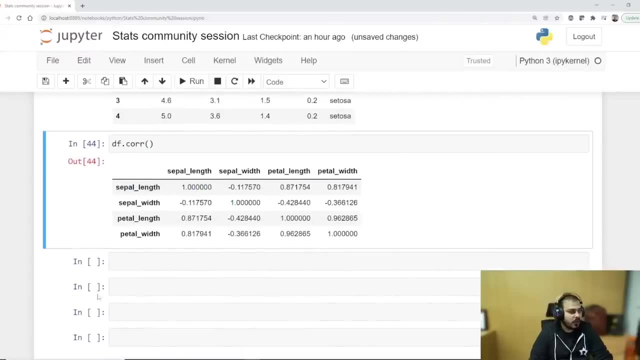 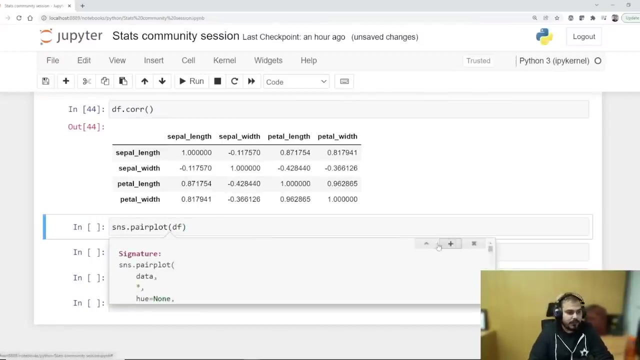 showing you the correlation with sepal length and petal length. it is positively correlated. now see, with respect to correlation also, we have various ways. okay, i'll not use in this. instead i can also use sns, dot, pair, plot, df. so here also you have a way to see. 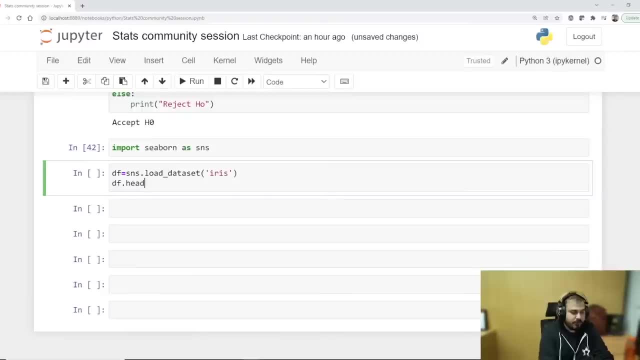 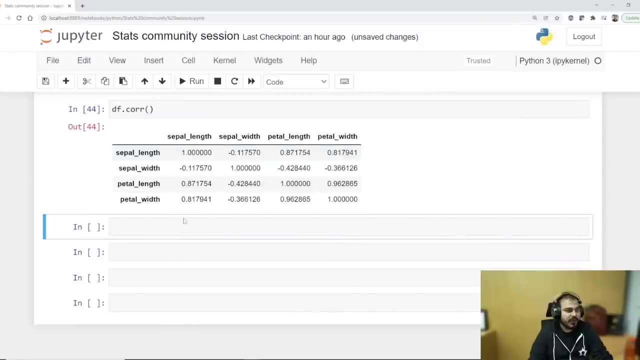 that i'm going to use iris data set, so this will be my df dot head. so if i use the correlation df dot corr. so this is how my diagram looks like. here you can see that it is basically showing you the correlation with sepal length and petal length. it is positively correlated. now see: 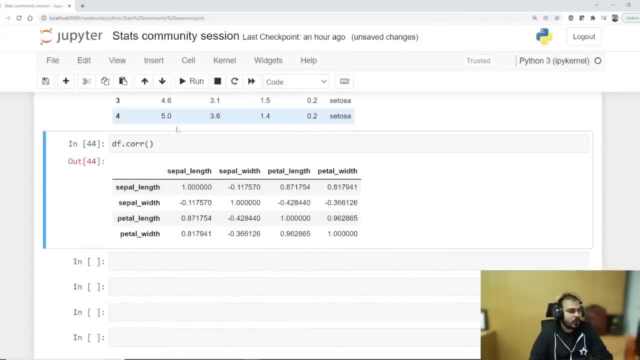 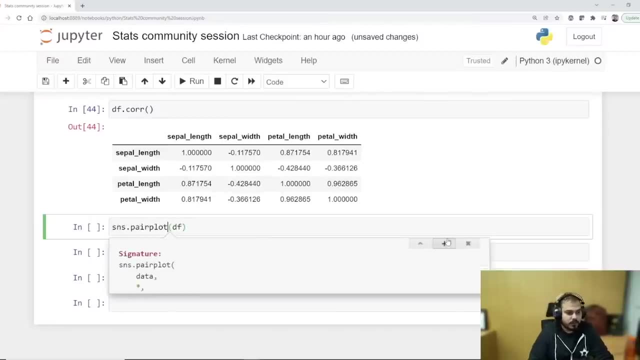 with respect to correlation also, we have various ways. okay, i'll not use in this. instead i can also use sns, dot, pair, plot, df. so here also you have a way to see in a diagrammatic way. so here you can see. this is how your diagram looks like. 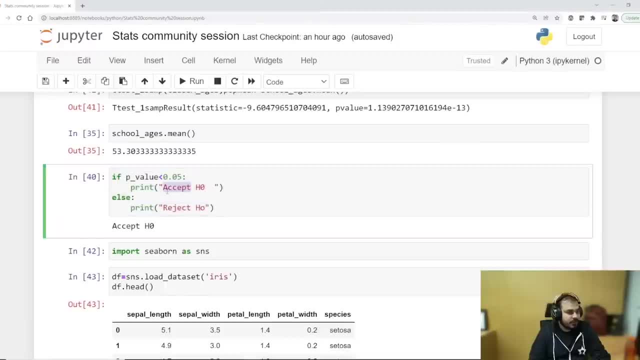 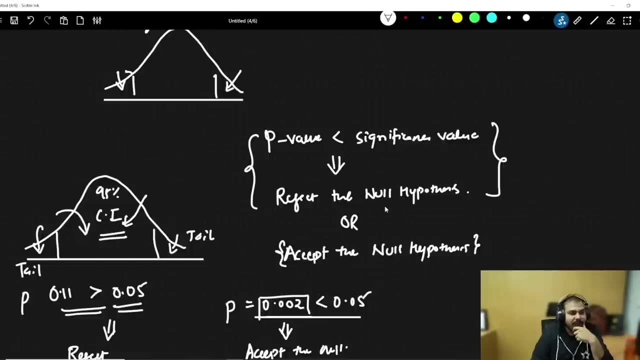 okay, the entire correlation in visualized way. guys, this will be reverse. sorry, i should basically write less than or equal to 0.05. so i have written it correctly over here, but in the code i have written wrong. okay, if p value is less than the significance value, we reject. okay, code wise. but 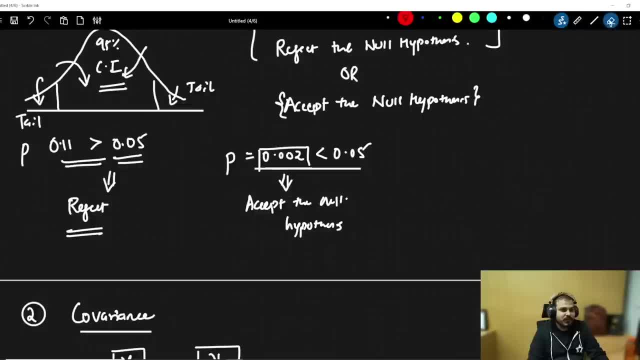 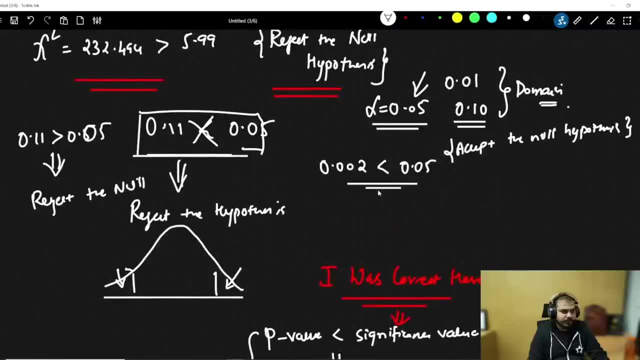 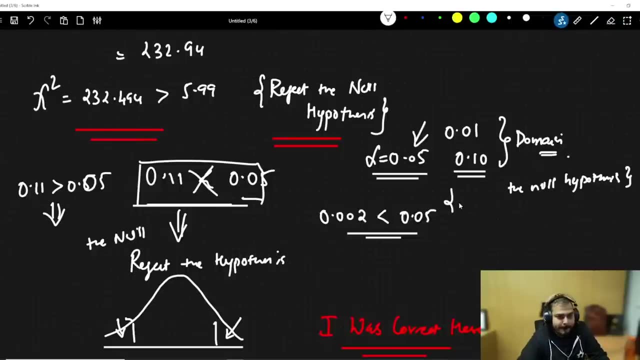 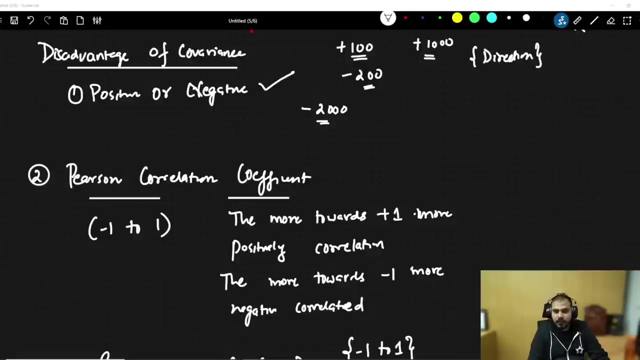 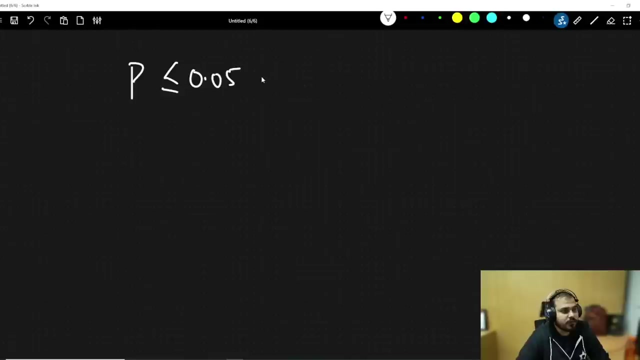 this wise. uh, i've written it correctly, sorry. this should also be rejected. this should be reject. this should be accept anywhere. i made a mistake here again. okay, here also, i think, accept here, reject. i made one mistake, guys. again i'm going to repeat it. see, if p value is less than or equal to 0.05. 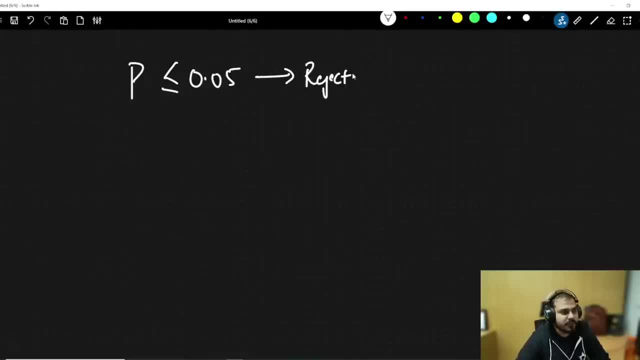 in this particular case, we reject the null hypothesis. the reason why we do this? because p. p is basically defining the probability part right now. in this particular case, they are just saying that it is less than five percent probability that the null is correct. it basically says that five percent probability, the null hypothesis. 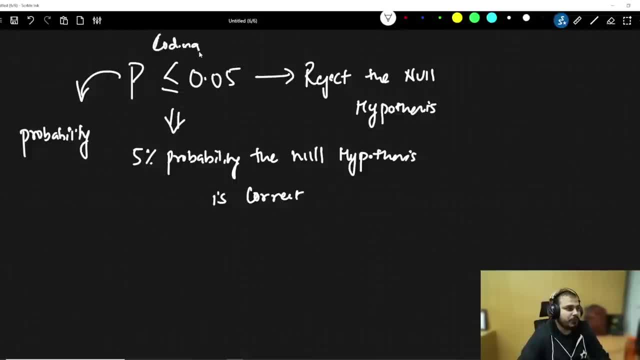 is correct. this will be applicable in coding guys, so don't worry in coding. so this is what it is basically saying. okay, so if p is greater than or equal to 0.05, here we accept the null hypothesis, which in turn is saying that more than 5% probability there is a. 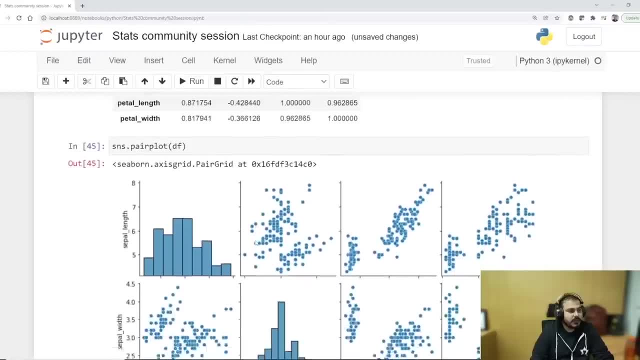 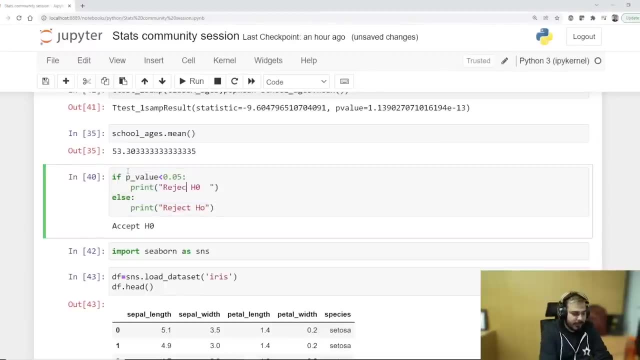 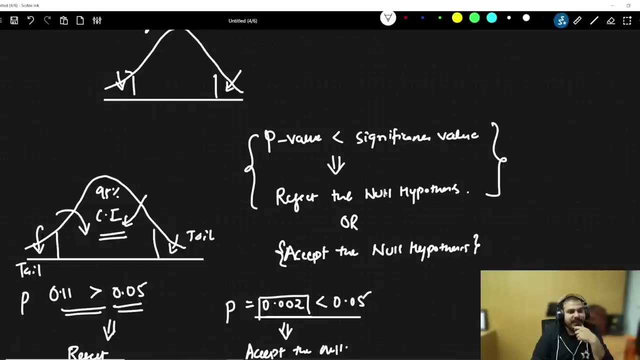 in a diagrammatic way. so here you can see. this is how your diagram looks like. okay, the entire correlation in visualized way. guys, this will be reverse. sorry to basically write less than or equal to 0.05. so i have written it correctly over here, but in the code i have written wrong. okay, if p value is less than the significance. 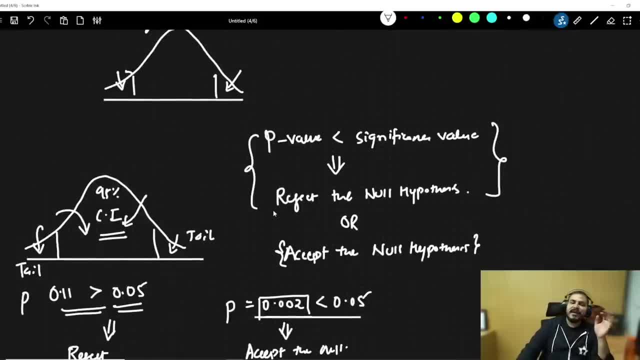 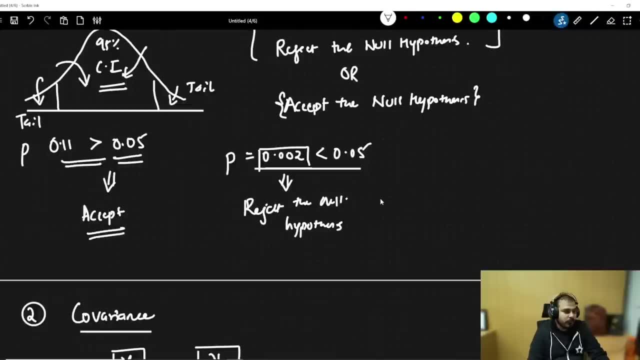 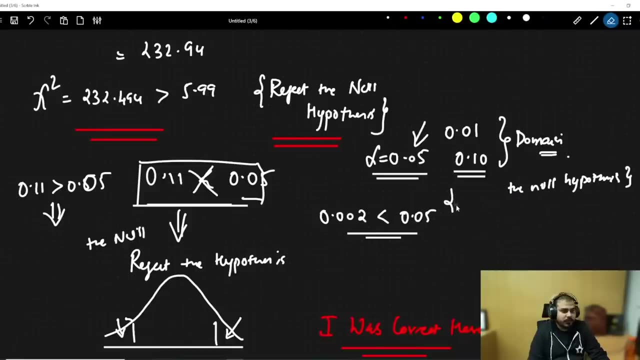 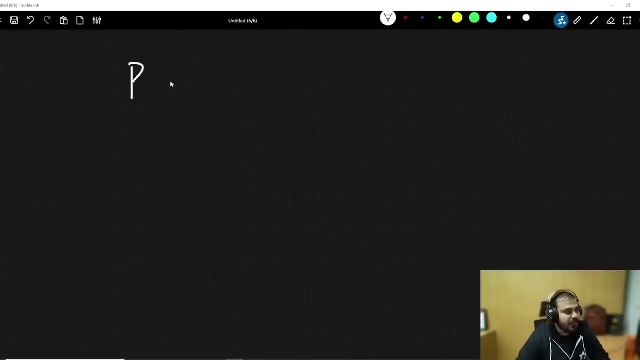 value. we reject. okay, code wise, but this wise. uh, i've written it correctly, sorry, this should also be rejected. this should be reject. this should be accept anywhere. i made a mistake here again. okay, here also, i think, accept here, reject. i made one mistake, guys. again i'm going to repeat it. see, if p value is less than or equal to 0.05 in. 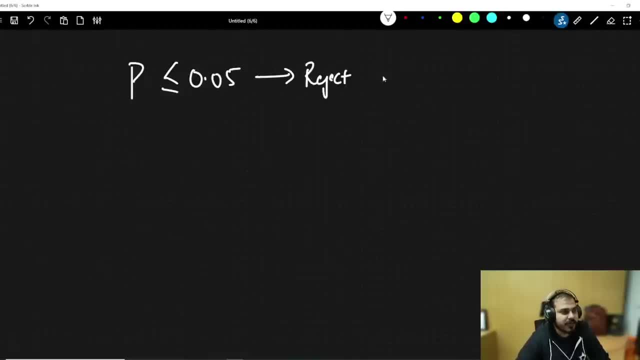 this particular case, we reject the null hypothesis. the reason why we do this? because p, p is basically defining the probability part right now. in this particular case, they are just saying that it is less than five percent probability and if p is less than or equal to 0.05, then we reject the null hypothesis. 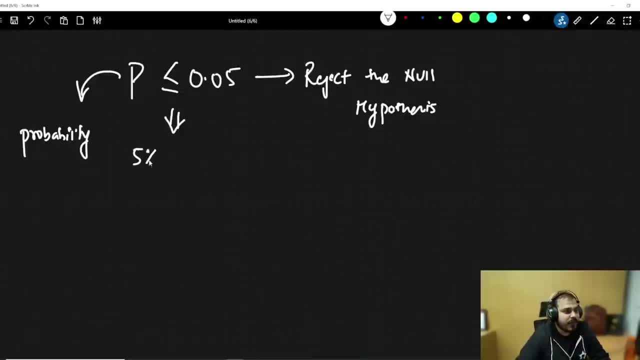 right now. in this particular case, they are just saying that it is less than five percent probability probability that the null is correct. it basically says that five percent probability, the null hypothesis is correct. this will be applicable in coding guys, so don't worry in coding. so this is. 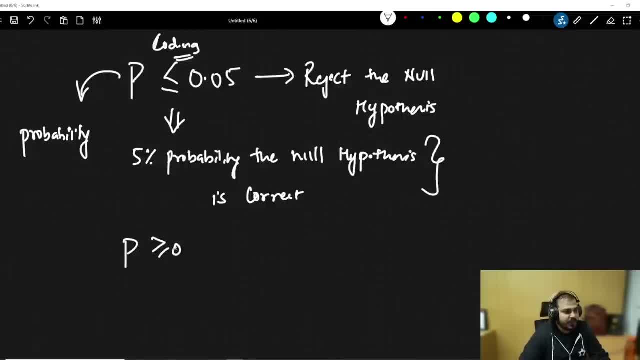 what it is basically saying. okay, so if p is greater than or equal to 0.05, here we accept the null hypothesis, which in turn is saying that more than five percent probability, there is a chances of more than five percent probability for the null hypothesis, correct? so this is basically. 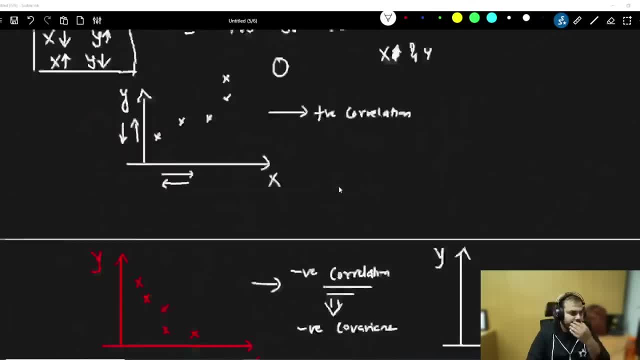 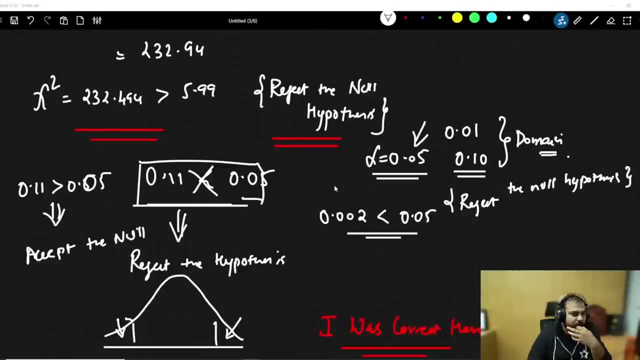 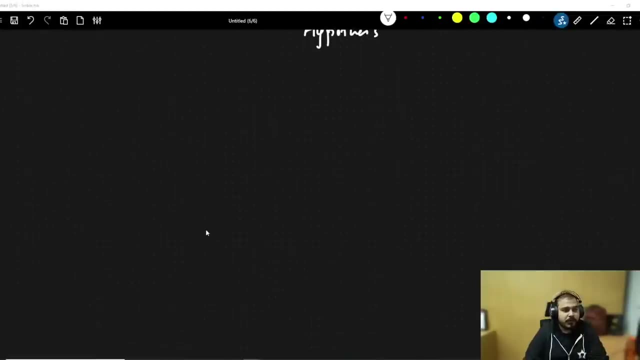 for alpha 0.05. i hope now it is clear here i have written it anywhere wrong so that this gets solved. this is fine, because this is greater than 5.99. only the relationship between alpha, p value and alpha is important. guys see, in coding we always get a p value. so here also, if i go and 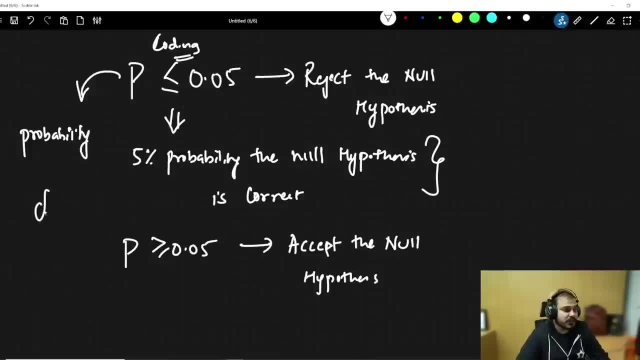 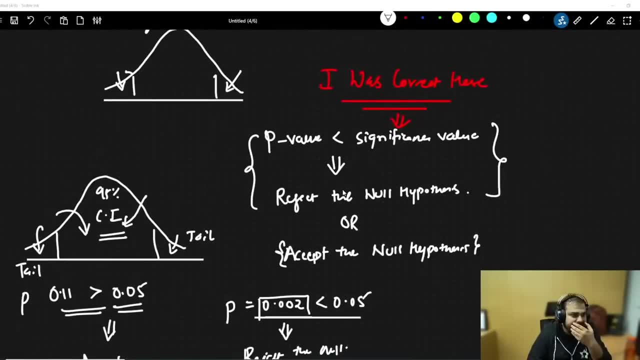 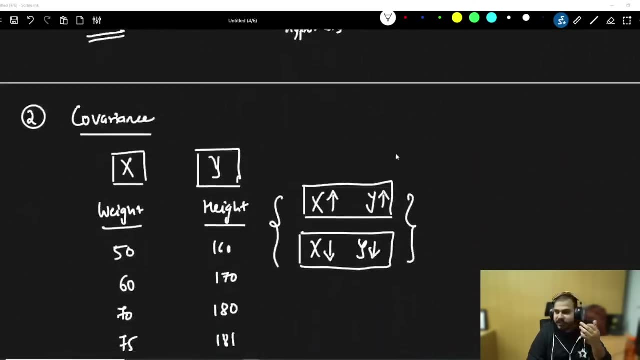 chances of more than 5% probability for the null hypothesis, correct. so this is basically for alpha 0.05. i hope now it is clear here i have written it anywhere wrong so that this gets solved. this is fine because this is greater than 5.99. only the relationship between alpha p value and alpha 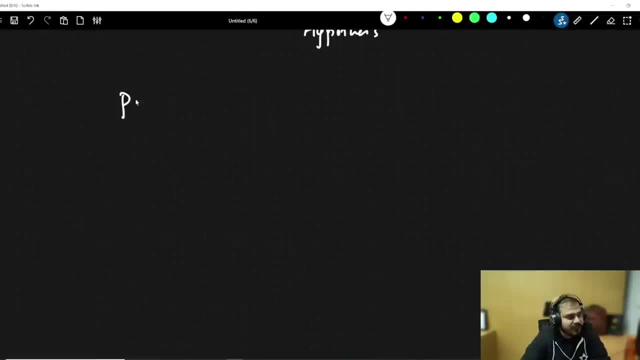 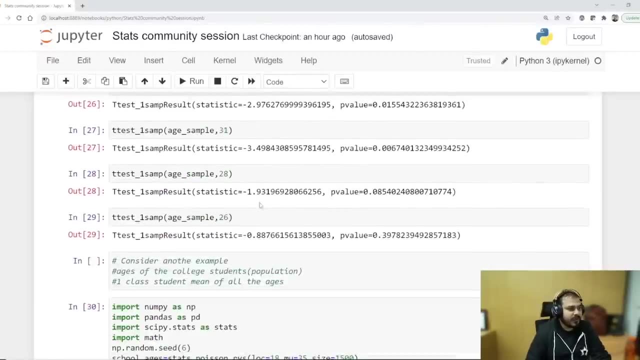 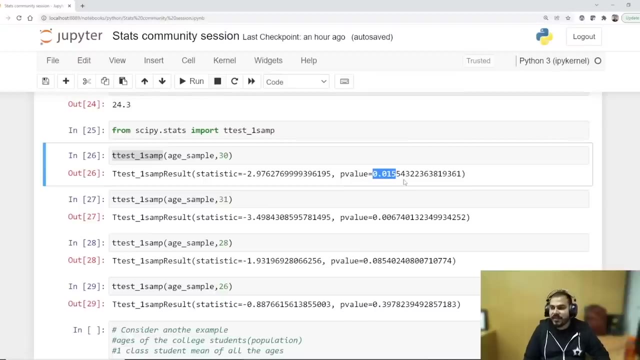 is important. guys see, in coding we always get a p value. so here also, if i go and see with respect to the coding, let's say in this particular case, if i am getting 0.015, this basically indicates that. what does it indicate? we have to reject the null hypothesis. so here also i will just write a. 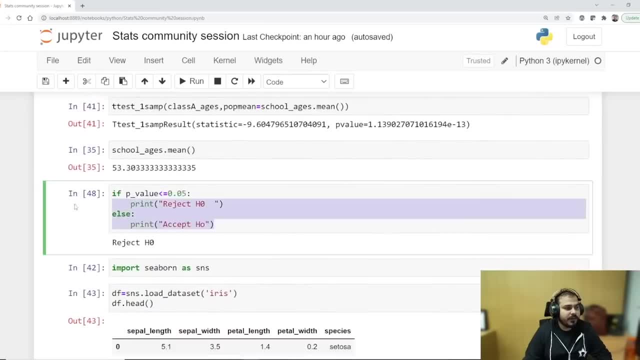 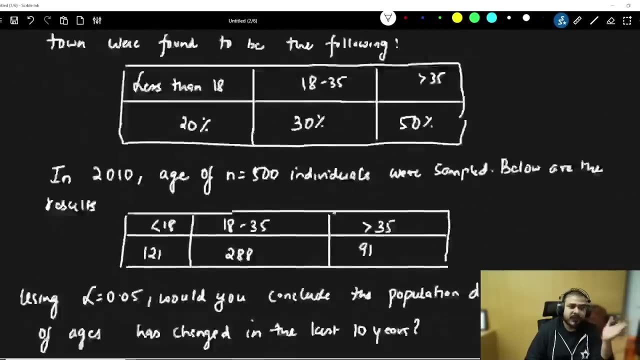 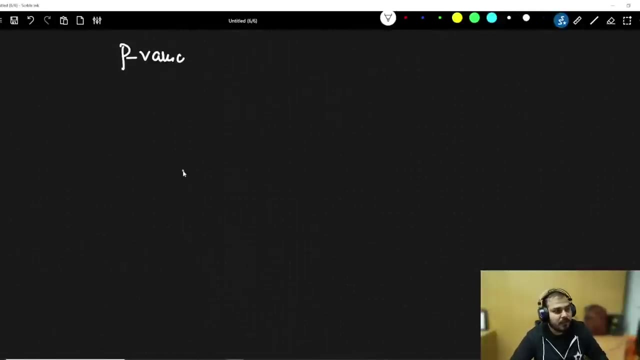 condition saying that this condition will work over here. it is always a confusing thing. p value, because p value i defined in that condition particular way. everything is correct because see what, what exactly p value basically specifies. i'll talk about it. i told you an example of mouse bar. right, if i have like this here, if i say p value. 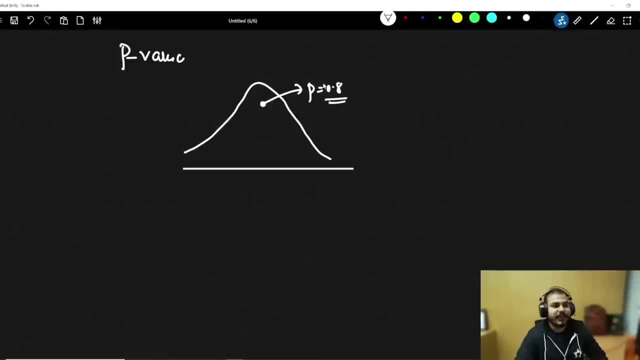 is 0.8. that basically means out of all the 100 touches, 80 percentage of time you're going to touch over here. out of all the 100 criteria, if you say p value is 0.01, over here one time, you are saying now, if you are saying p value is less than 0.05, that basically means 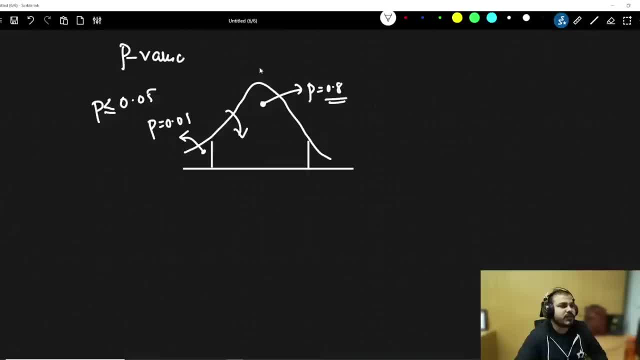 you have less than five percent probability for the null hypothesis to be true, which is basically present over here. p value less than or equal to 0.05 basically is specifying your tail region and this is specifying your this confidence interval region when the p value is greater. 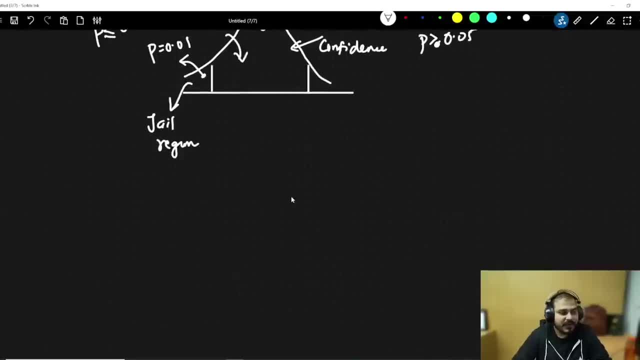 than or equal to 0.0. greater than 0.0. always understand this relationship between p value and significance value. significance value specifies your confidence interval. p value is result. if this is less than or equal to ci, the confidence interval or, in this particular case: 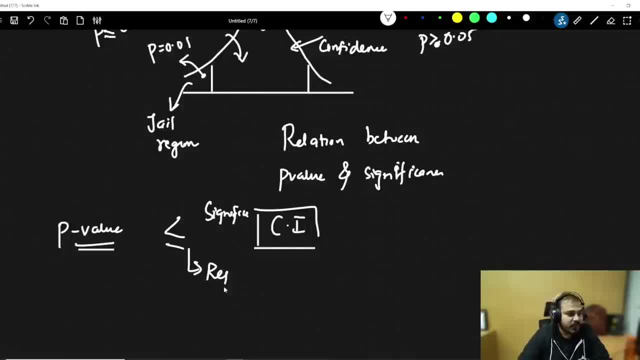 the significance value. here you specifically reject the null hypothesis because it is just saying that less than five percent probability it is there. so we reject the null hypothesis and in the other case we accept the null hypothesis. okay, when the p value is greater than alpha- the first topic that we will discuss about p value and significance values. so today i'm going to talk. 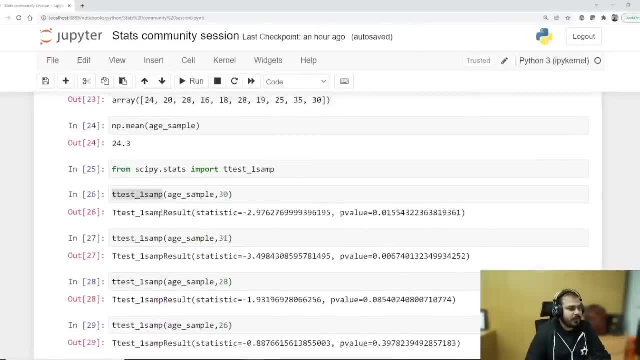 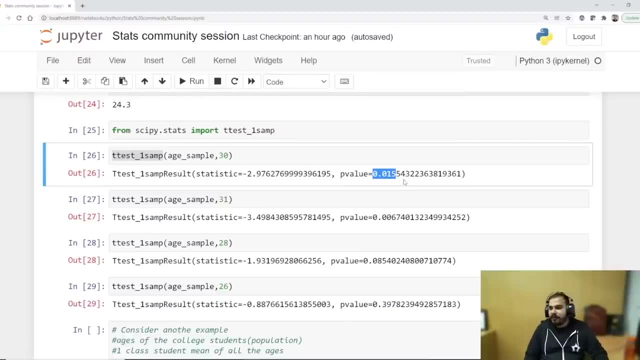 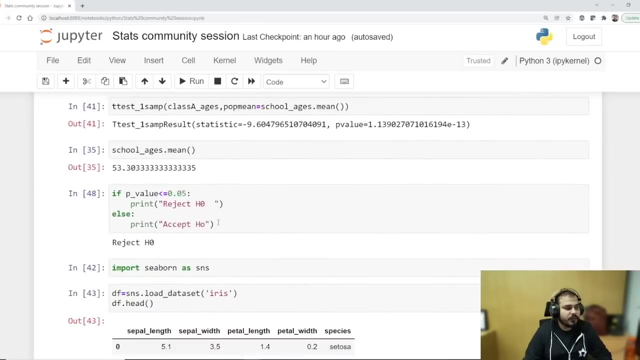 see with respect to the coding, let's say you in this particular case, if i am getting 0.015, this basically indicates that. what does it indicate? we have to reject the null hypothesis. so here also i will just write a condition saying that this condition will work over here. it is always a confusing thing. p value because 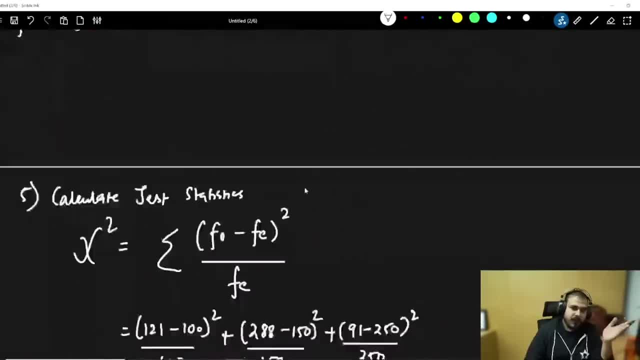 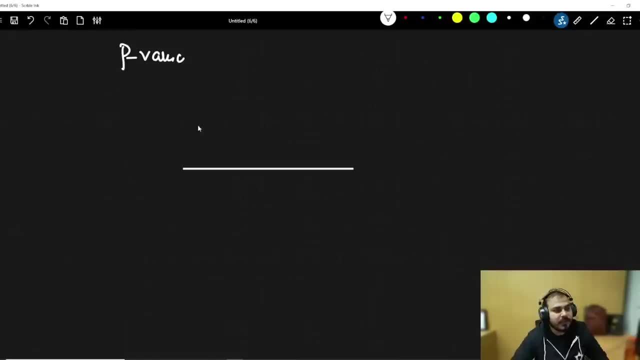 p value i defined in that particular way. everything is correct because see what, what exactly p value basically specifies. i'll talk about it. i told you an example of mouse bar. right, if i have like this here: if i say p value is 0.8, that basically means out of all the 100 touches 80. 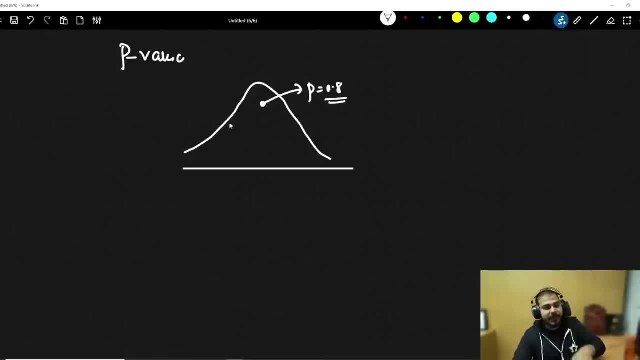 percentage of time you're going to touch over here out of all the hundred criteria. if you say p value is 0.01- over here one time- you are saying now, if you are saying p value is less than 0.05, that basically means you have less than five percent probability for the null hypothesis to be true. 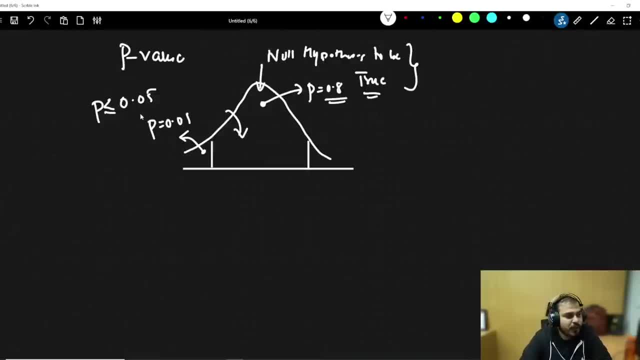 which is basically present over here. p value less than or equal to 0.05 is specifying your tail region and this is specifying your this confidence interval region when the p value is greater than or equal to 0.0. greater than 0.0. always understand this. relationship between p value and significance value. significance value specifies your confidence interval. p value is from the test result. if this is less than or equal to ci, the confidence interval or, in this particular case, the significance value. here you specifically reject the null hypothesis because it is just saying that less than 5 percent probability it. 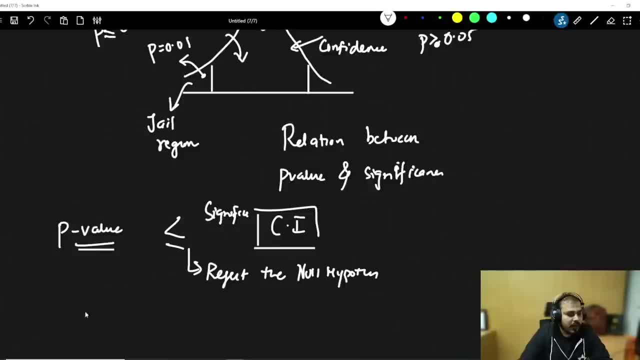 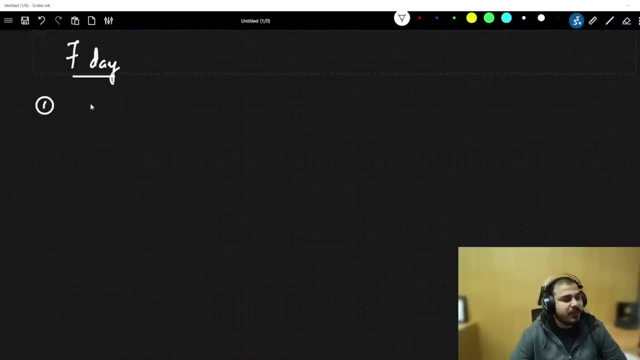 is there. so we reject the null hypothesis and in the other case, we accept the null hypothesis. okay, when the p value is greater than alpha. the first topic that we will discuss about p value and significance value. so today i am going to talk about the exact relationship between this p value. 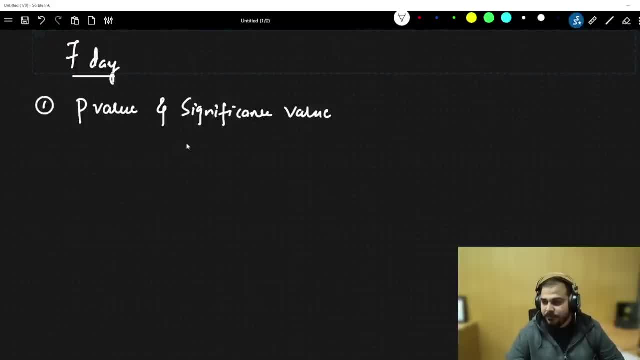 and significance value. the first topic that we will discuss about p value and significance value. significance value because from the tests that we were doing, you know we were seeing that, okay, most of the tests from that test, how do we derive this p value? that is what i'm actually going to. 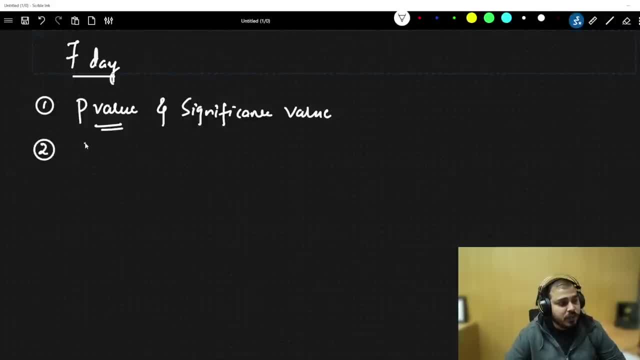 discuss about it and practically also one example will be shown. then we'll move towards distribution. first we will discuss about central limit theorem, central limit theorem, or then we are going to discuss about distributions like bernoulli's distribution, bernoulli distribution. then fifth, we are basically going to discuss about binomial distribution and then sixth, we'll also be seeing 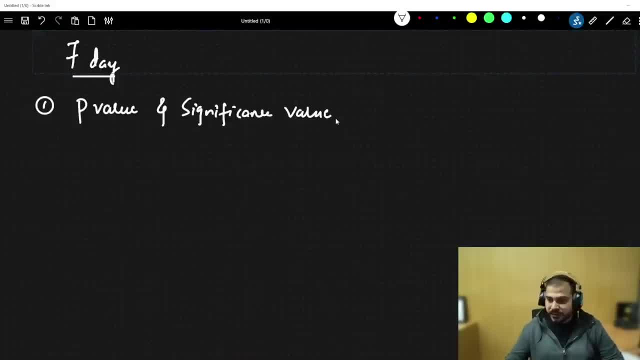 about the exact relationship between this p value and significance value, because from the tests that we were doing, you know, uh, we were seeing that, okay, most of the tests from that test- how do we derive this p value? that is what i'm actually going to discuss about it, and practically also one example. 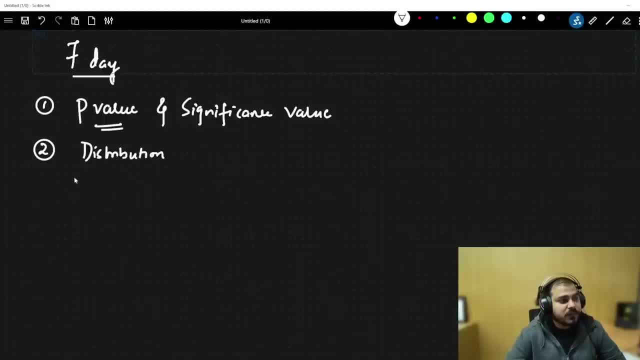 will be shown. then we'll move towards distribution. first we will discuss about central limit theorem, central limit theorem, or then we are going to discuss about distributions like bernoulli's distribution, bernoulli's distribution, and then we are going to discuss about distribution like bernoulli's distribution. 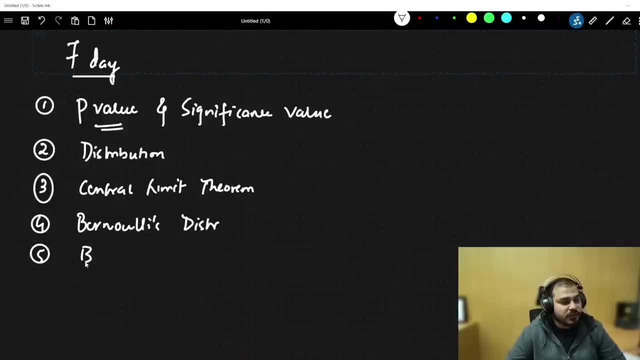 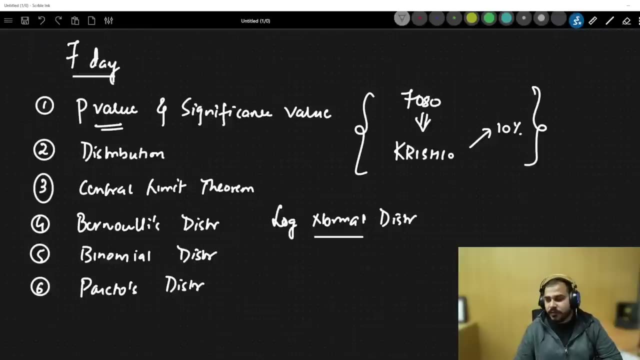 bernoulli's distribution. then fifth, uh, we are basically going to discuss about binomial distribution, uh, and then sixth, we'll also be seeing something called as parito's distribution. okay, i'll include log normal also. right, log normal distribution, poison, uh, parito distribution there. 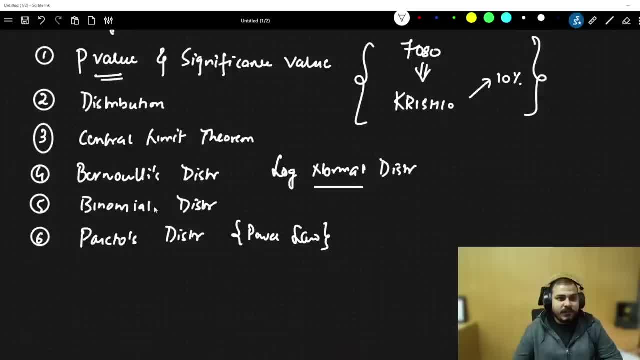 is something called as power law. we'll discuss about it one. one final thing that is pending is called as f test, which is also called as anova test. this will take one hour time, guys. just to do this, i will upload a separate video. okay, i'll upload a separate video. 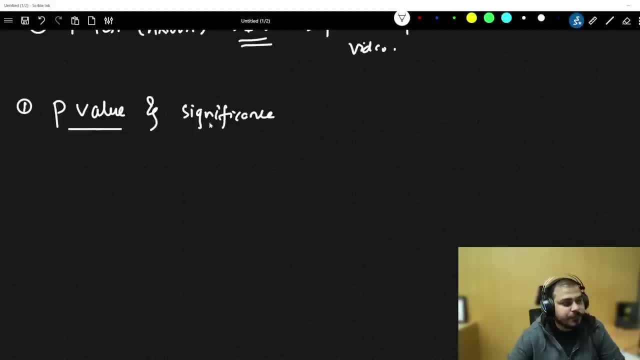 on the same today, i will show you how you will derive the p value. so we are basically going to see how do we derive the p value and what is the relationship between p value and significance value. so this all things we will be discussing. let's take a problem statement, the problem. 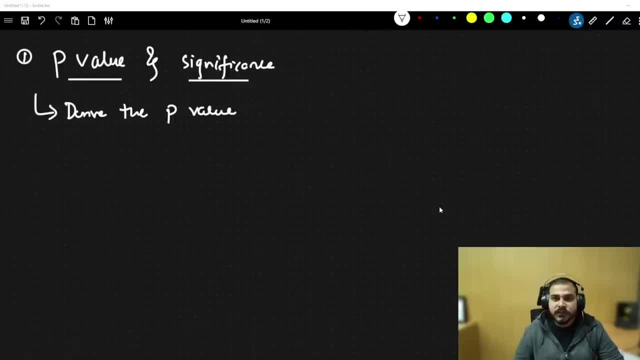 statement: uh, i'm going to take it off a z test and uh, let's, let's take the. let's try down the question before that. everybody ready, take up your book and pen. i've already discussed about permutation and combination guys in the previous session. the question is nothing but it. 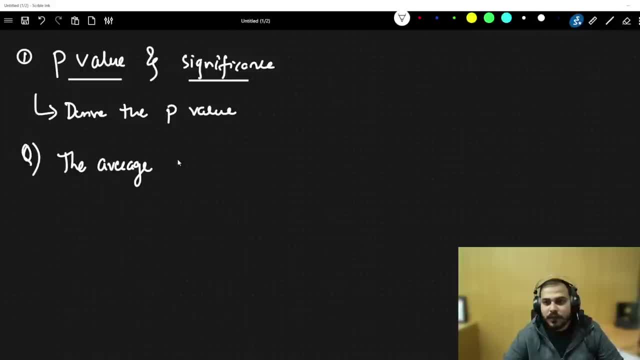 is very simple: the average. we'll do a z test problem and then we'll try to derive this. the average weight of all residents in bangalore city. in bangalore city is 168 pounds. we take a sample now. we take a sample. okay, one, one data i have missed. so over here: the average weight of all residents in bangalore city. 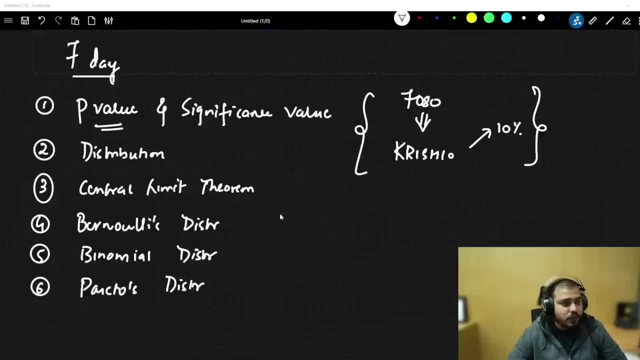 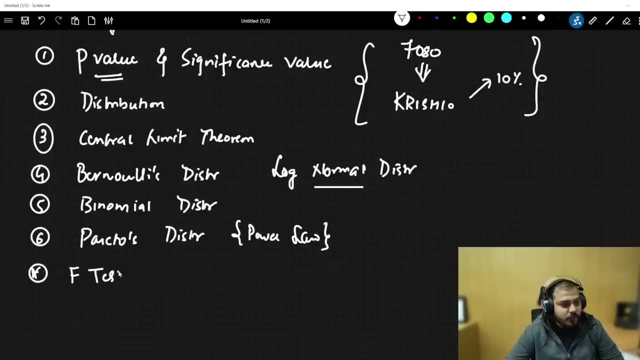 something called as parito's distribution. okay, i'll include log normal also, right, log normal distribution, poison parito distribution. there is something called as power law. we'll discuss about it one. one final thing that is pending is called as f test, which is also called as anova test. 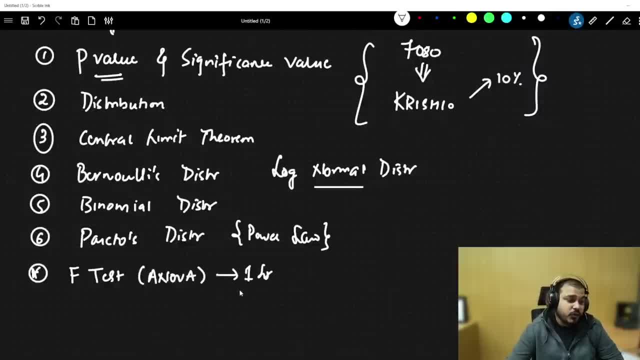 this will take one hour time, guys. just to you do this, i will upload a separate video. okay, i'll upload a separate video on the same today. i will show you how you will derive the p value. so we are basically going to see how do we derive the. 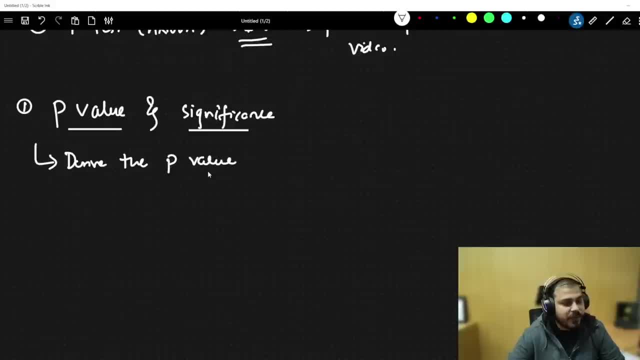 p value and what is the relationship between p value and significance value? so this, all things we will be discussing. let's take a problem statement, the problem statement, uh, i'm going to take it off a z test and uh, let's, let's take, let's write down the question before that. 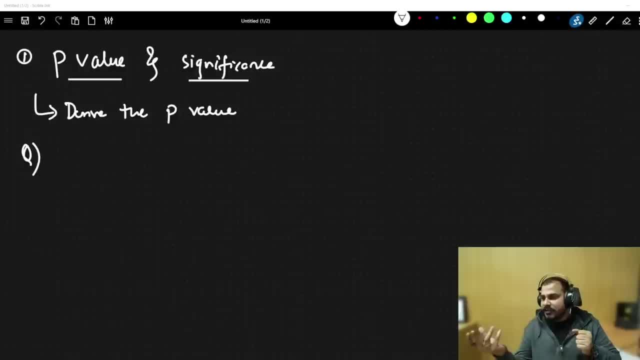 everybody ready, take up your book and pen. i've already discussed about permutation and combination guys in the previous session. the question is nothing, but it is very simple: the average. we'll do a z test problem and then we'll try to derive this, the average weight of all. 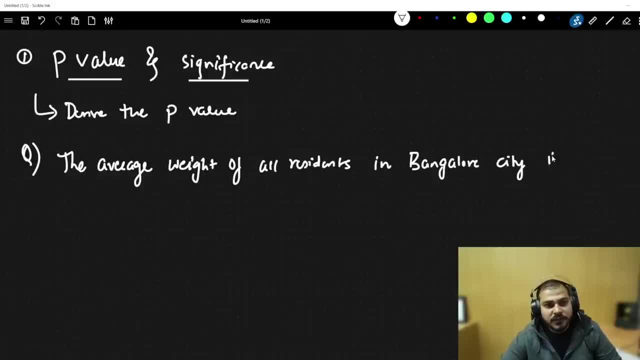 residents in bangalore city. in bangalore city is 168 pounds. we take a sample now. we take a sample. okay, one, one data i have missed. So over here. the average weight of all residents in Bangalore city is 168 pounds, with a standard deviation 3.9.. 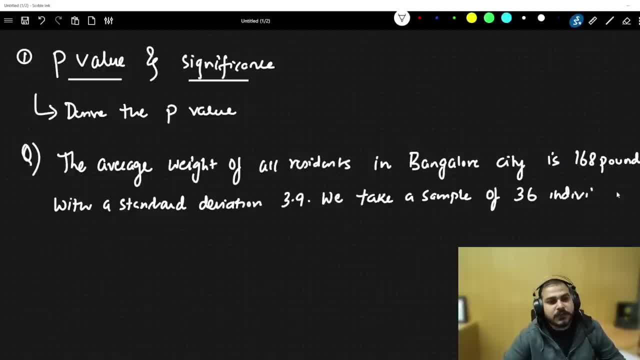 Now what we are saying. we take a sample, 36 individuals and the mean is 169.5 pounds. From this information, we really need to check whether this sample is being able to tell us the weights are same or not. So this is what it is given and our confidence interval is basically 95%. 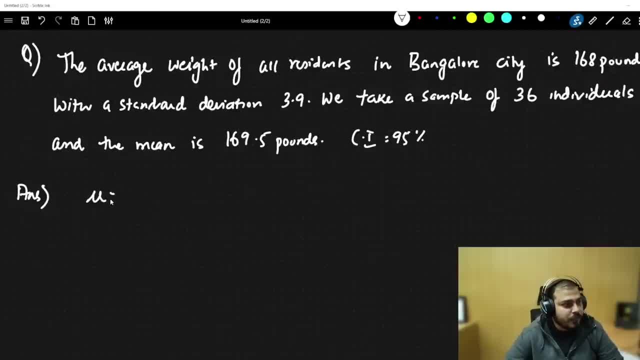 So over here, you know what is my, what is your mean. my mean is 168 points, the standard deviation is 3.9, the x bar is nothing but 169.5 and my n sample is greater than 36 and obviously my n sample is given. 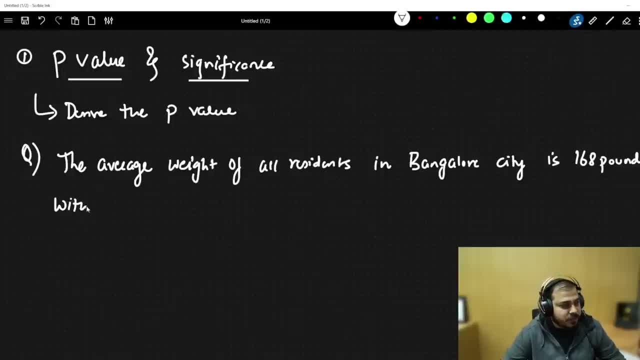 is 168 pounds, with a standard deviation 3.9. now what we are saying. we take a sample, 36 individual and the mean is 169.5 pounds. from this information, we really need to check whether whether the sample is being able to tell us. 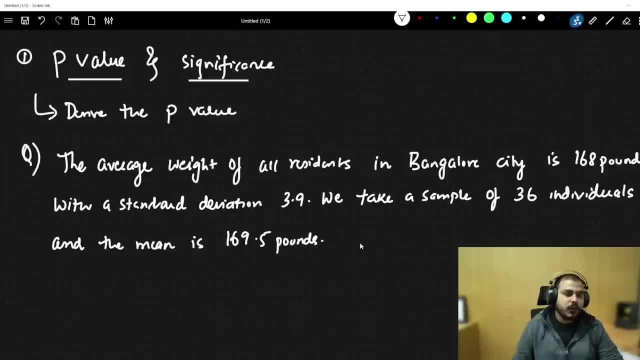 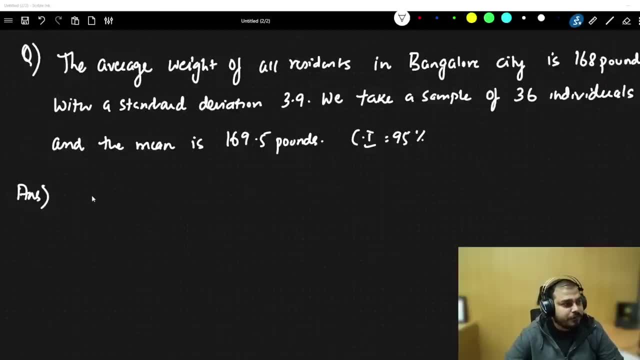 the weights are same or not. okay, so this is what it is given, and our confidence interval is basically 95 percentage. so over here, you know what is my, what is your mean? my mean is 168 points. the standard deviation is 3.9, the x bar is nothing but 169.5 and my n sample is greater than 36. 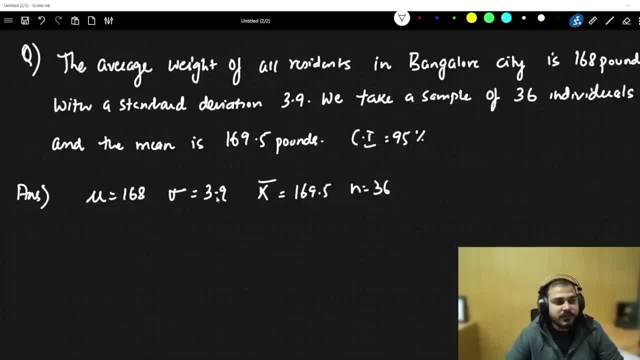 and obviously my n sample is given, my population standard deviation is given. so i'm going to take a sample and i'm going to basically use z test. very good, the alpha value is 0.05. 1 minus 95 percent is one zero point, zero five. let's go ahead and solve this particular problem. so what is your null? 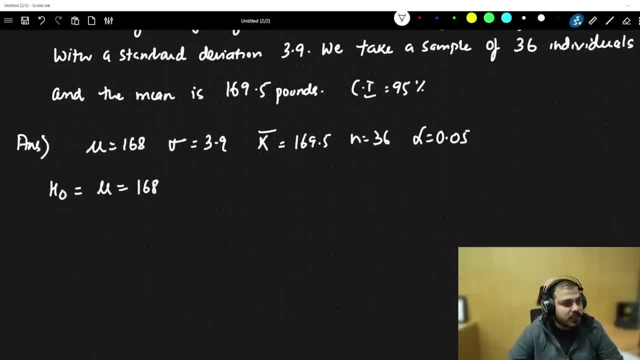 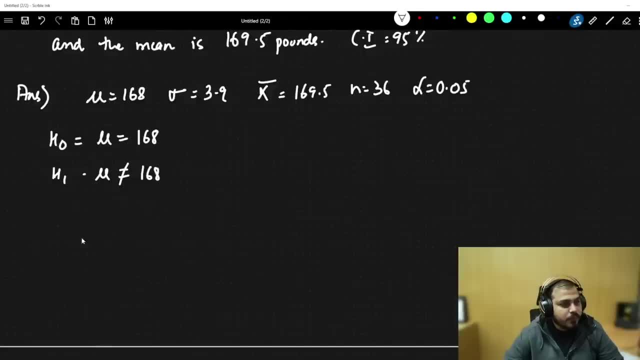 hypothesis: mean is equal to 168. what is your alternate hypothesis? your mean is not equal to 168. then what we do? we basically come to the second step, where we specify our alpha 0.05. the third step: we basically find out our decision value and we define the decision boundary. so my decision boundary is, quickly, how much? 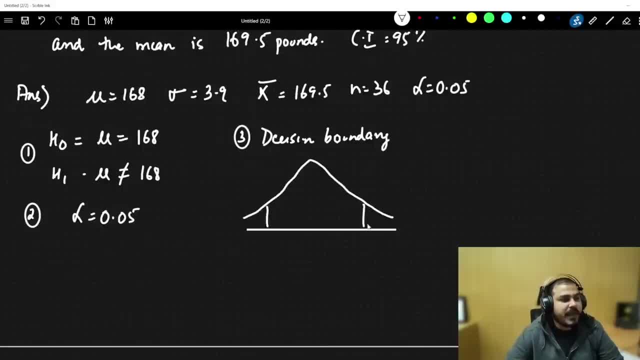 it is nothing, but it is this graph. it is a two-tail test. it can be greater than 168, less than 168. so here i have basically 0.025, here i have 0.025, here i have 95. now, what is this value that i can get from? 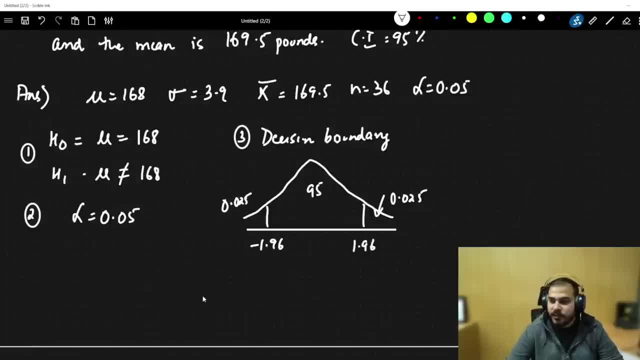 the z table that we see. can i say one point nine six plus minus one point nine six. so if you open a z table with respect to one minus point zero, two five, you will be getting 0.9750. we are going to check this area of curve and usually we get one point nine six and minus. 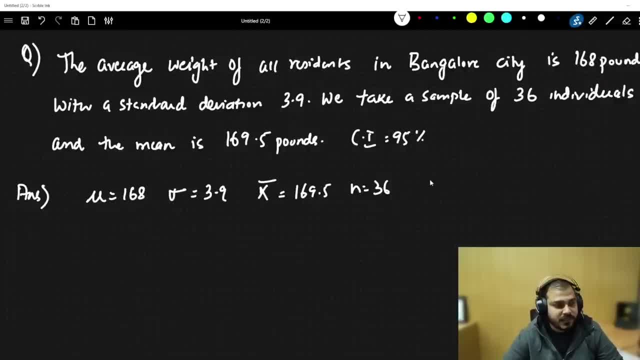 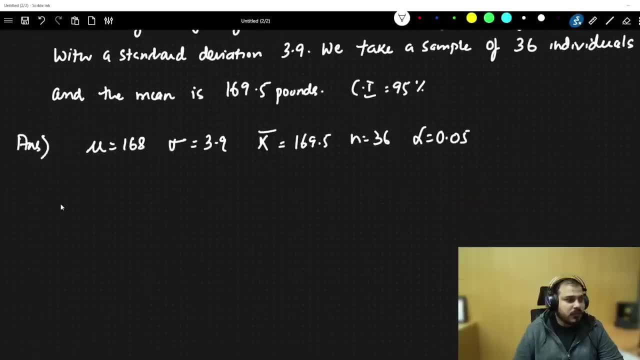 My population standard is 3.9.. My standard deviation is given, so I am going to basically use Z test. Very good, The alpha value is 0.05. 1 minus 95% is 0.05.. Let's go ahead and solve this particular problem. 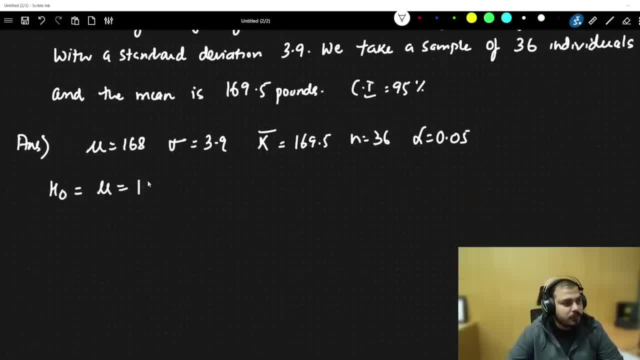 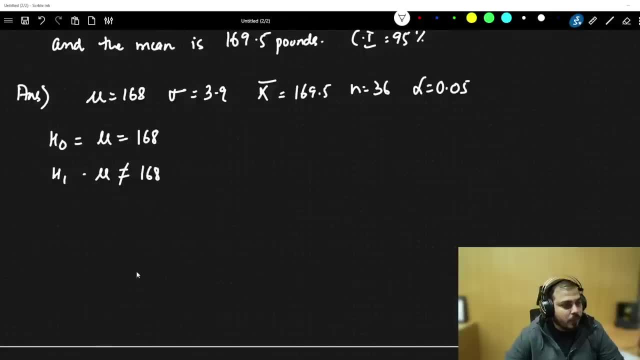 So what is your null hypothesis? mean is equal to 168.. What is your alternate hypothesis? your mean is not equal to 168.. Then what we do? we basically come to the second step, where we specify our alpha 0.05. the third step. 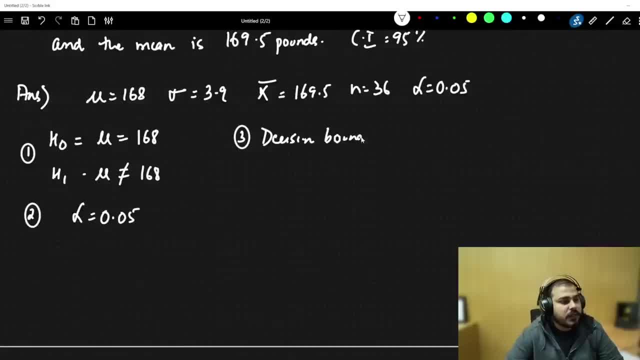 We basically find out our decision boundary. so my decision boundary is: quickly how much? it is nothing, but it is this graph. it is a two tail test. it can be greater than 168, less than 168.. So here I have basically 0.025. here I have 0.025. here I have 95%. 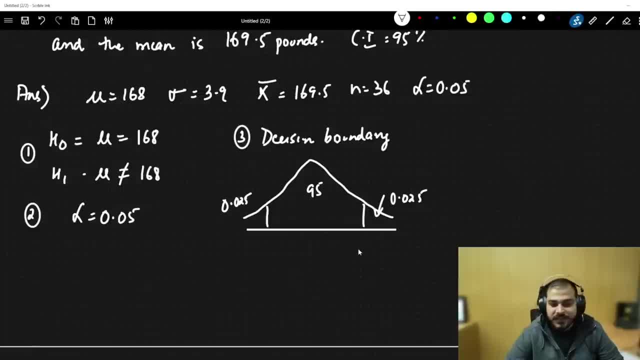 Now, what is this value that I can get from the Z table that we see? can I say 1.96 minus 1.96.. 1.96.. If you open a Z table with respect to 1 minus 0.025, you will be getting 0.9750. we are going. 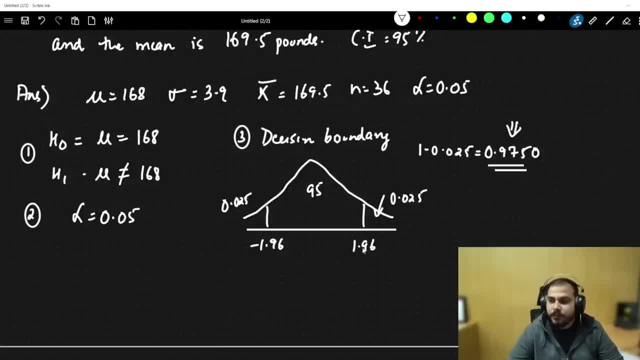 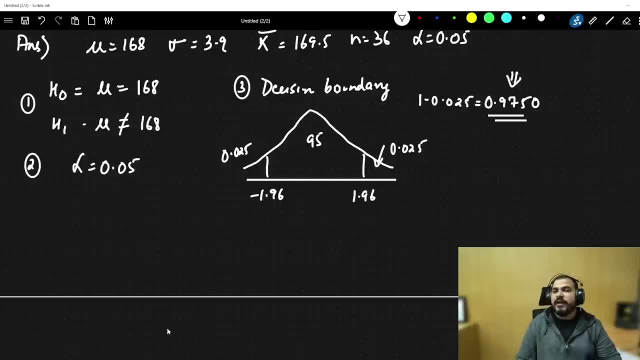 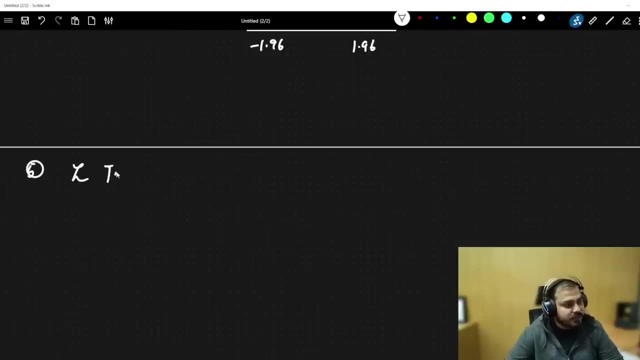 to check this area of curve and usually we get 1.96 and minus 1.96.. Now the next step. I hope everybody is clear because we have already done this in our previous session. Next step: we do the. that is my fifth step. we calculate the Z test. 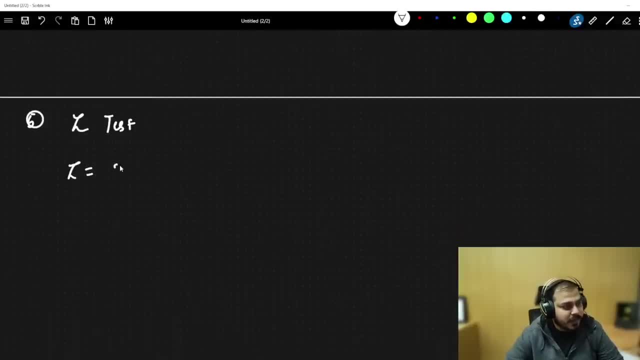 Now Z test formula is very much simple. I hope everybody remembers X minus mu divided by standard deviation of root n. What is X, 169.5 minus 168 divided by what is standard deviation? 3.9 root by 169.5, not 1 root of. 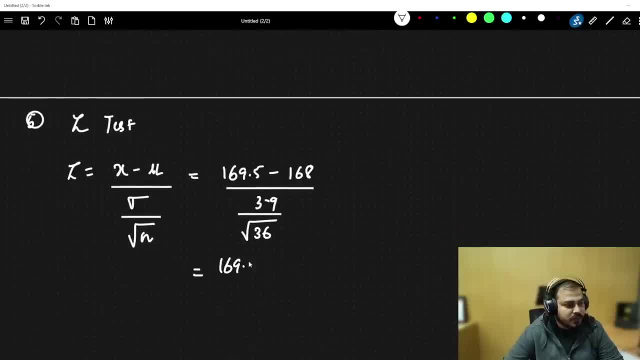 36.. So here we are basically going to get 169.5, 1.5 divided by 3.9, multiplied by 169.5.. So this is the result. So this is the result. So this is the result. I am going to calculate the size of this unit. 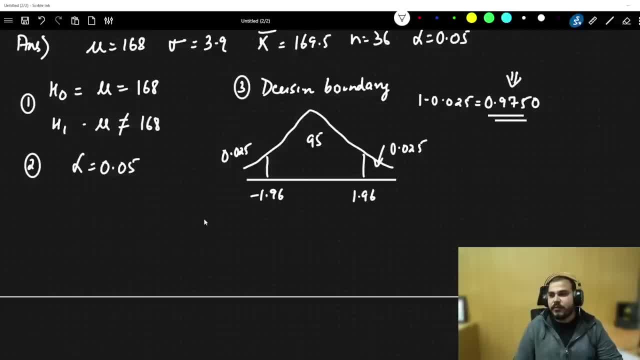 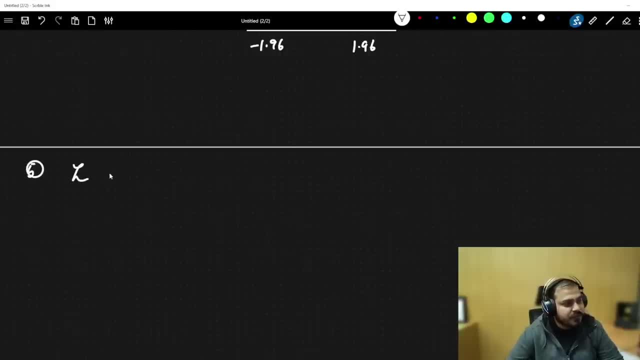 one point nine six. now the next step. i hope everybody is clear because we have already done this in our previous session. next step: we do the. that is my fifth step. we calculate the z test and also calculate it as u's or u's and as all our Lean, as our do it. and the last step is: 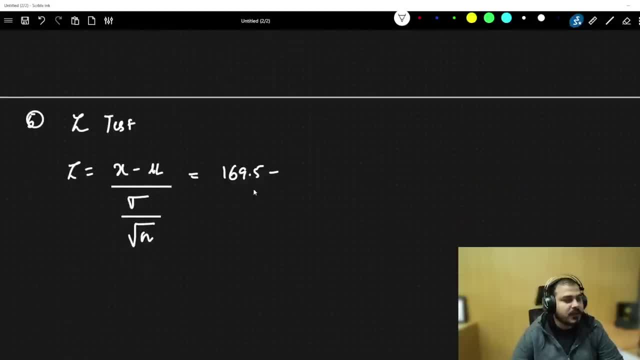 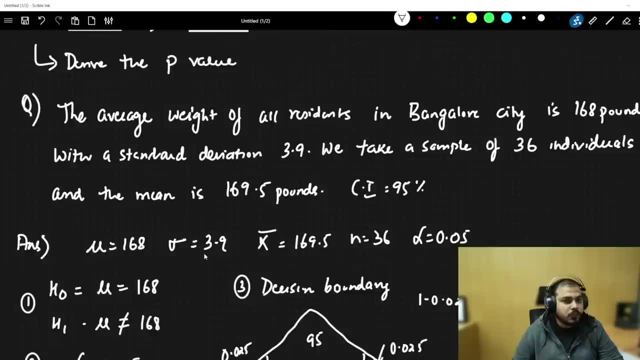 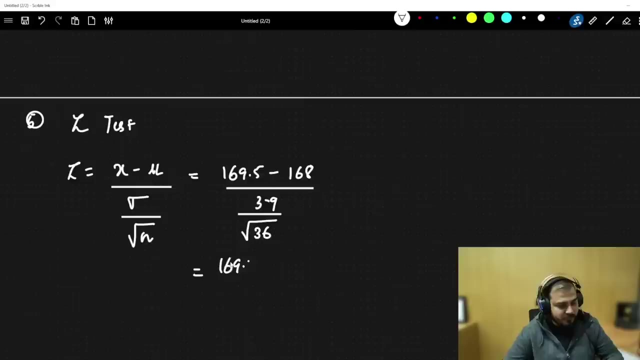 How much will be with respect to the z side, and the last set of that is our capital Z, so that we we will calculate the z side as we know it and we will declare the z as any other z for our common । combined losses. all will from 1 to 0.. д1.. So what will it give us as a result? there will be this. 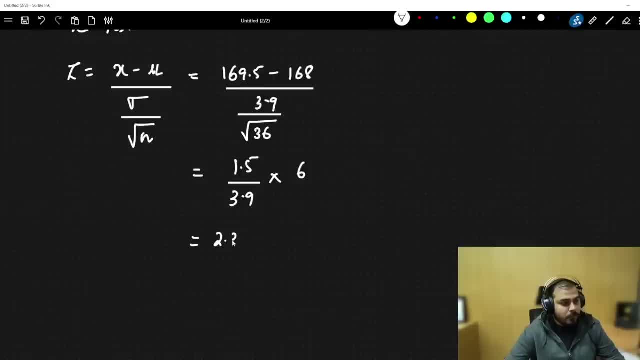 equation. i am going to write it here: p, that is the number of that z are alright, i will just alsoA: So 2.307,. so right now, let's go to our decision rule. my Z value is 2.307, is it greater than? 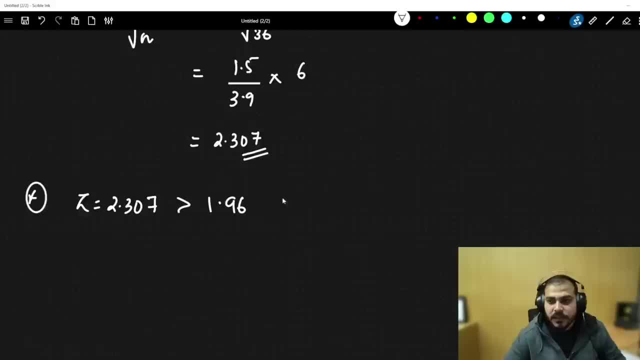 is it greater than 1.96,? it is greater than 1.96, so we reject the null hypothesis. But this is already. we have done many number of times. okay, we have done many number of times, but now one step will go ahead. this is fine. this is one way of solving this problem. 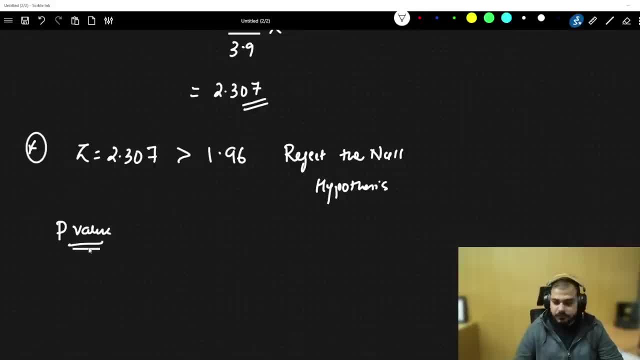 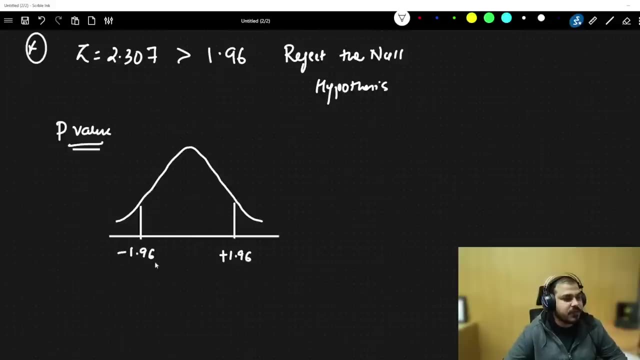 but where does P value comes into existence? where does P value comes into existence in this particular case? Now, what it is saying is that initially, my this graph- I was checking it for this- to this, where it was plus 1.96, minus 1.96, and obviously I got 2.307, so it is falling somewhere here. 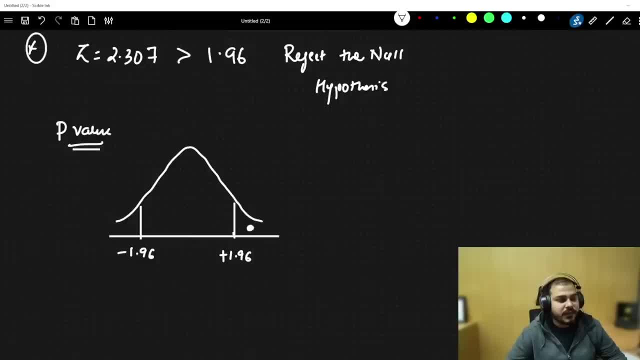 it is falling somewhere here- right, If I am, if I am considering 2.307, it is falling somewhere here. it is on the top and side, so we are rejecting the null hypothesis. Now, if I really want to find out the P value, what I am actually going to do, I am going 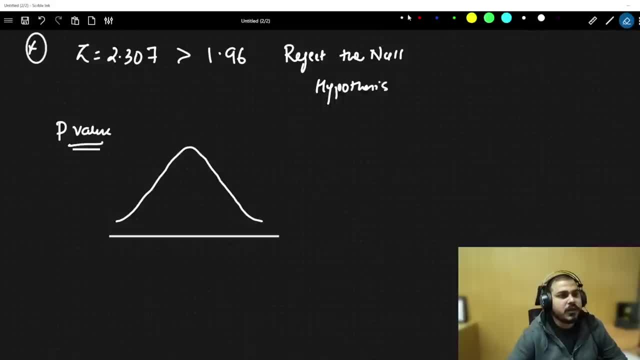 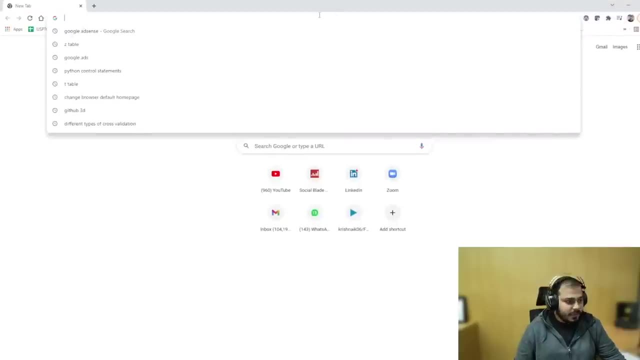 to remove this. and now my curve will be little bit bigger because, based on this, I got the Z value as 2.307 and here also I got minus 2.307, because both are symmetrical. Now the next step. what I will do: I will take out my Z table. I will take out my Z table. 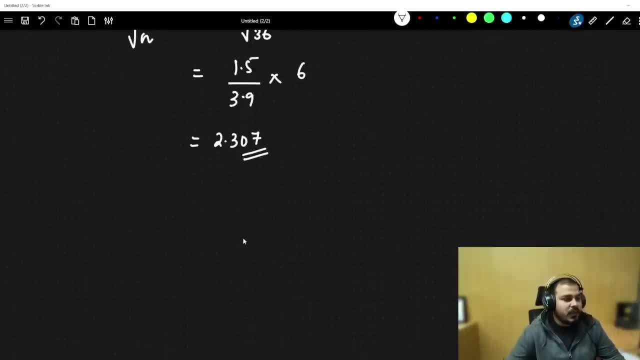 So the reason why we are like this will be because in the article we want to have 6.. So going to get, We got the value. this is fine. this is one way of solving this problem. but where does p value comes into existence? where does p value comes into existence in this particular case? now, what it is saying is: 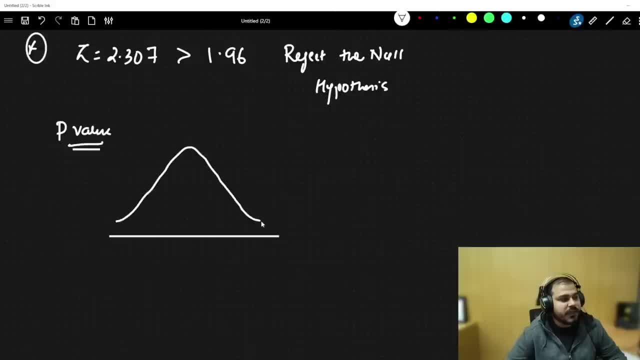 that initially my this graph- i was checking it for this- to this, where it was plus 1.96, minus 1.96 and obviously i got 2.307. so it is falling somewhere here. it is falling somewhere here, right, if i'm, if i'm considering 2.307, it is falling somewhere here. it is on the top one side. 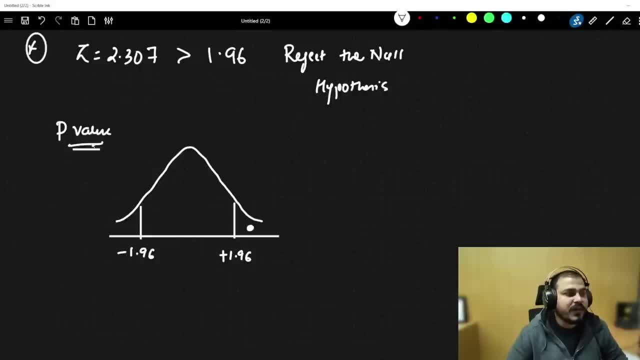 so we are rejecting the null hypothesis. now, if i really want to find out the p value, what i am actually going to do, i'm going to remove this, and now my curve will be little bit bigger because, based on this, i got the z value as 2.307, and here also i got minus 2.307, because both are. 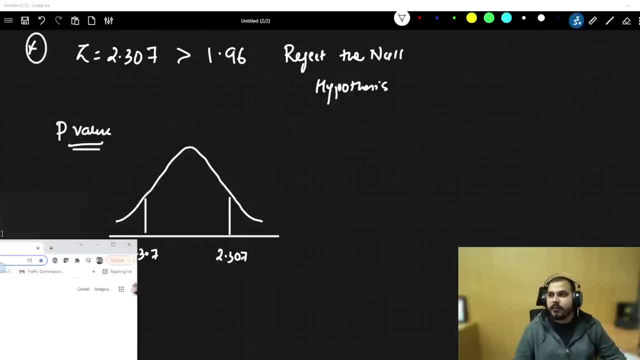 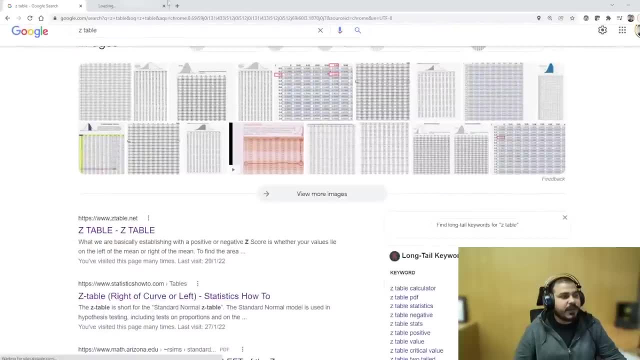 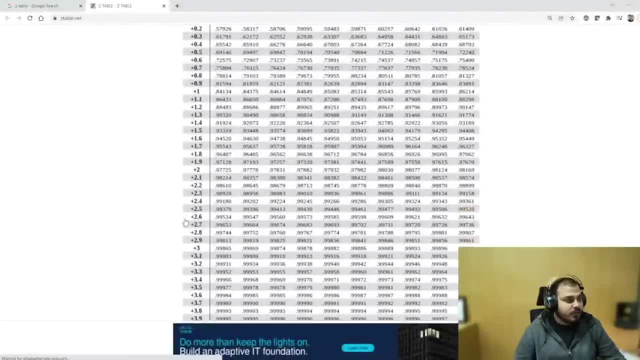 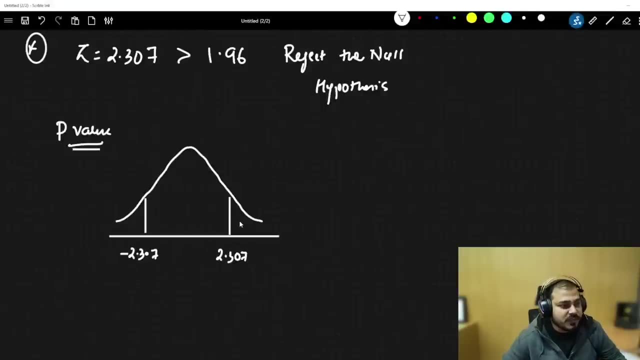 of 2.307, right. so what i'm going to do over here- 2.3- i'll check based on this z score. what is the area under the curve? what is this specific area? what is this specific area? i really need to find out and i don't know what is the area right now, so i will go ahead and calculate it now based on 2.307. 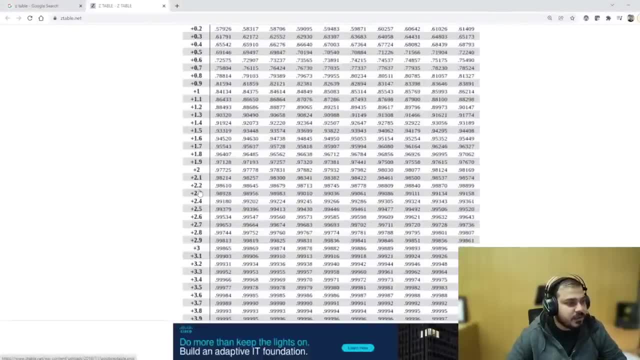 okay, so 2.3 is here and 07. if i say 07, it is somewhere here, so 2.307, i am getting somewhere around 0.99111. i hope everybody is able to understand what i am getting over here. 0.99111. 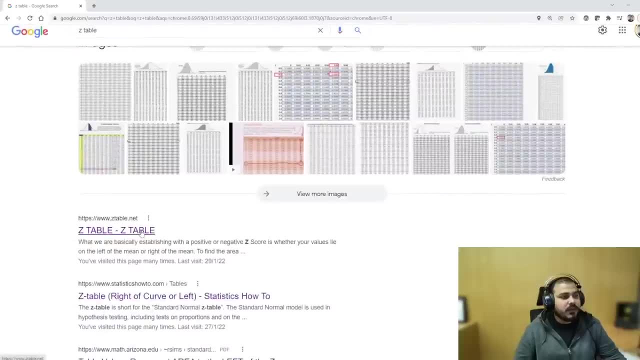 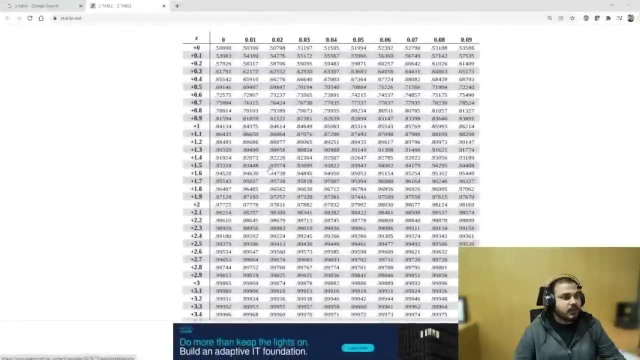 and I will try to find out what is those values with respect to my Z score, with respect to my Z score of 2.307, right, So what I am going to do over here- 2.3,. I will check based on this Z score. what is the? 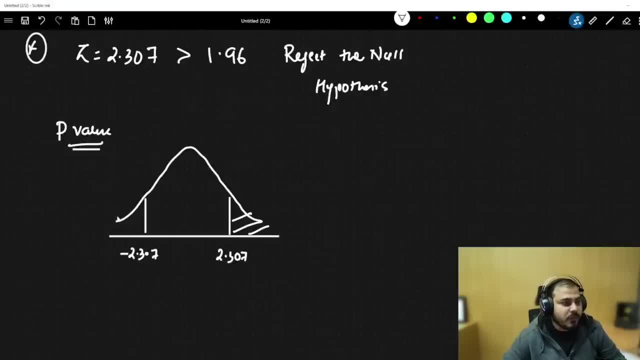 area under the curve. what is this specific area? what is this specific area? I really need to find out and I do not know what is the area right now, So I will go ahead and calculate it Now, based on 2.307, ok. 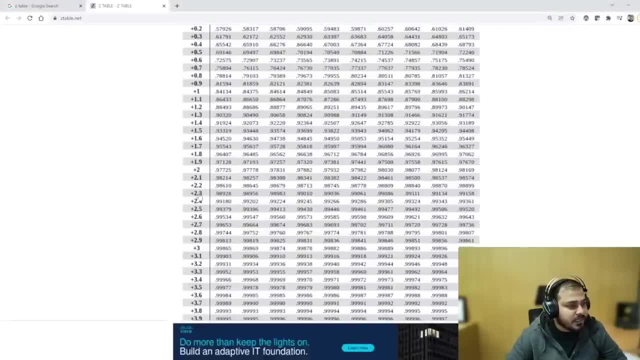 So I will go ahead and calculate it Now based on 2.307,. ok, So 2.3 is here and 07, if I say 07, it is somewhere here. so 2.307, I am getting somewhere around 0.99111,. I hope everybody is able to understand what I am getting over here. 0.99111, right. 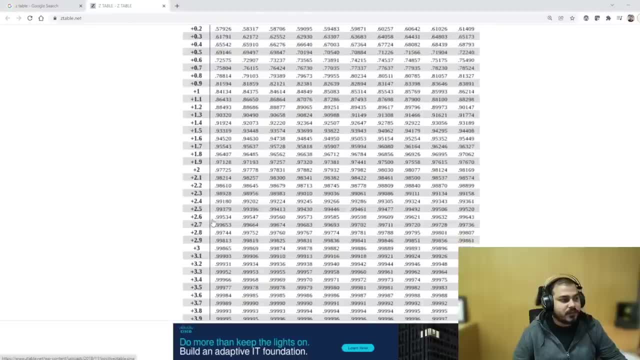 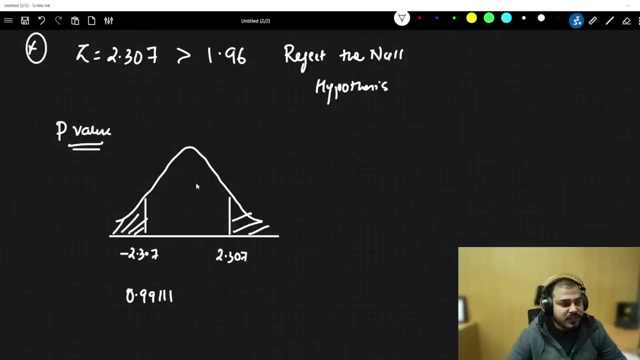 So what I am getting over here, it is nothing but 0.99111,. so here, based on this, my area under the curve is basically 0.99111,. so this with respect to the area under the curve, I am actually getting this. 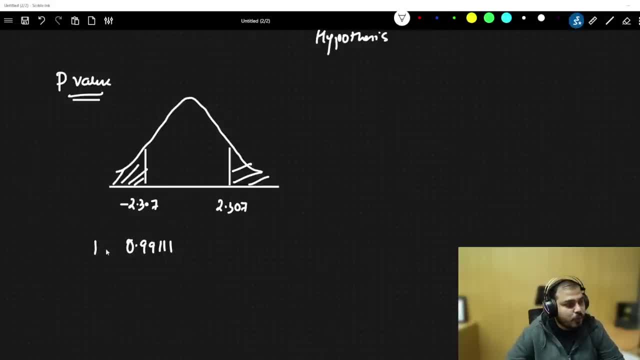 Now understand one thing: if I subtract with 1, see, 0.99111 is basically the area under the curve of this particular curve. Now, if I subtract this with this, how much I will be getting? so this area is nothing but 0.0089 and this is nothing but 0.0089.. 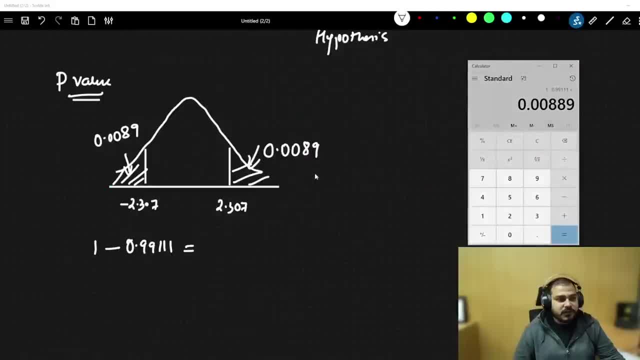 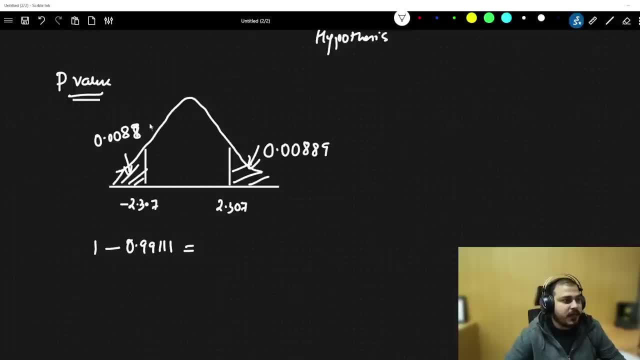 So I am getting 0.0089,, 0.0089, right, So this, you can see this- 889,- sorry, it is 889.. 889.. 889. 889.. So here I get 8, 9,, here also I am getting 8, 9.. 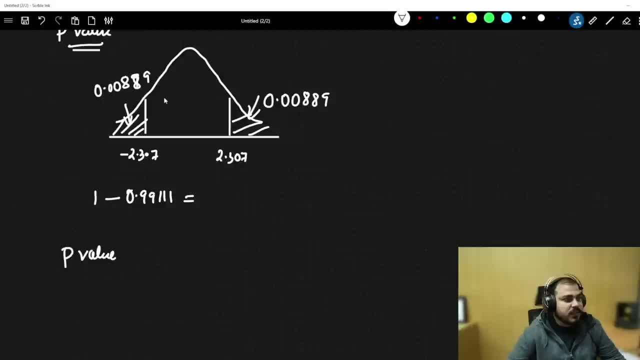 Now, according to the p-value- now see this- this middle one is 0.99111,. if I add up all this particular value I should be getting 1, and if you add it up I am probably will be getting 1.. P-value is nothing, but I have to add this area of curve of this tail and this tail because 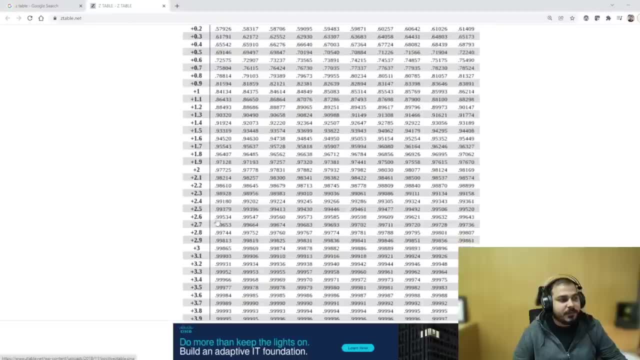 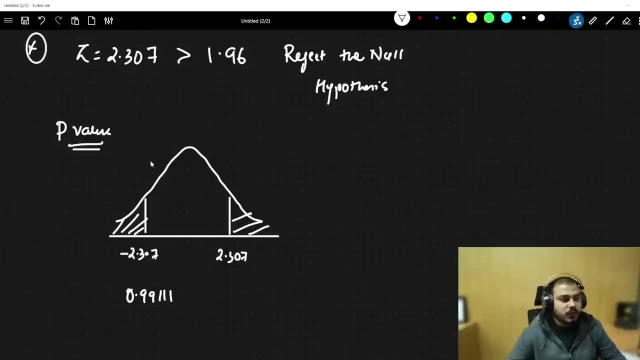 right. so what i am getting over here, it is nothing but 0.99111. so here, based on this, my area under the curve is basically 0.99111. so this with respect to the z score, i am getting the area under the curve. i am actually getting this now understand one thing: if i subtract: 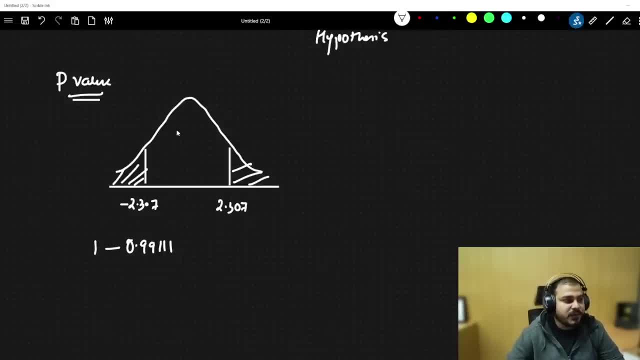 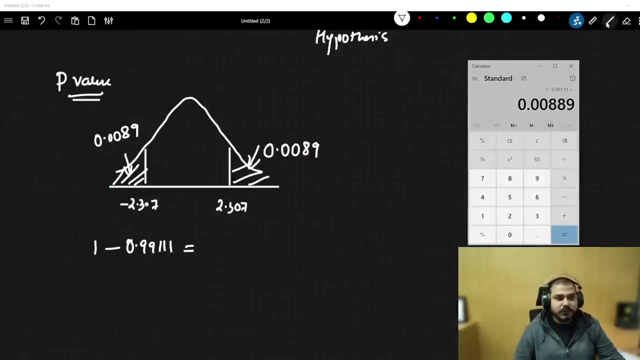 with 1, see 0.99111 is basically the area under the curve of this particular curve. now, if i subtract this with this, how much i will be getting. so this area is nothing but 0.0089 and this is nothing but 0.0089. so i am getting 0.0089, 0.0089, right? so this, you can see this- 889. sorry, it is. 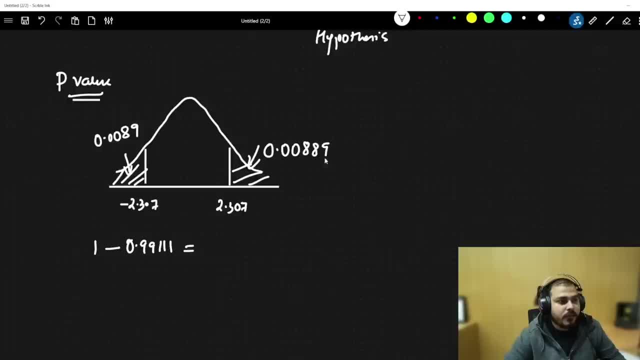 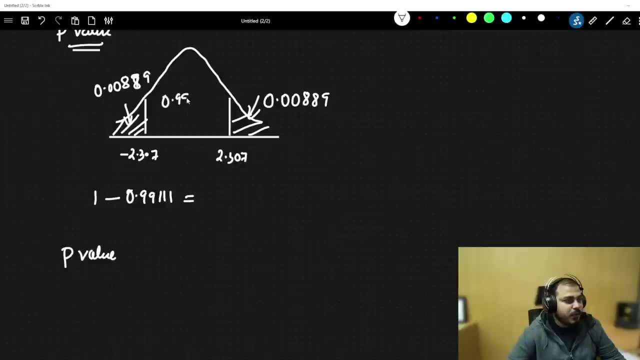 889, 889. so here i get 8- 9. here also i am getting 8, 9 now according to the p value. now see this: this middle one is 0.99111. if i add up all this particular value, i should be getting. 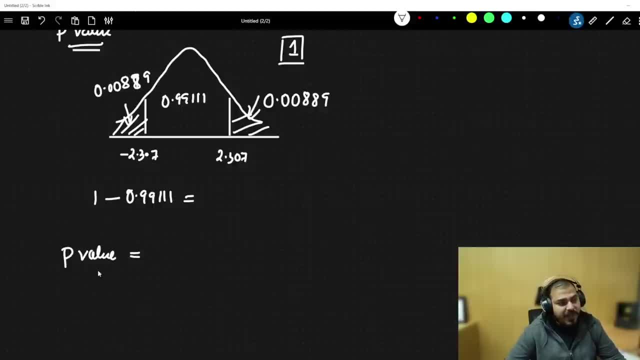 one and if you add it up, and probably you will be getting one p value is nothing. but i have to add this area of curve of this tail and this tail because it is two tail. i have to add this up and then this will basically give my p value. 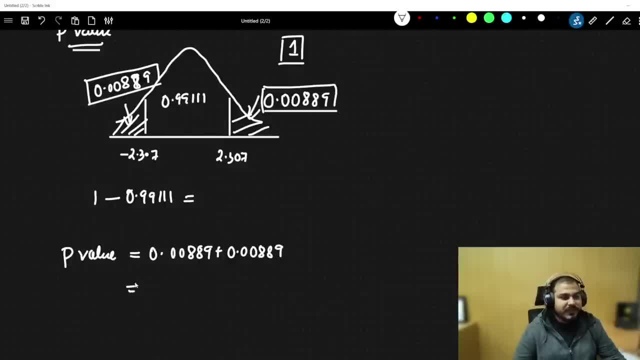 0.00889. so once i add this particular value, i am actually going to get 0.01778. is it not 0.889 divided by 2? no, because see both the, both the area are symmetrical. understand one thing: both the area are symmetrical. if i am getting one value over there, if i am getting one value, 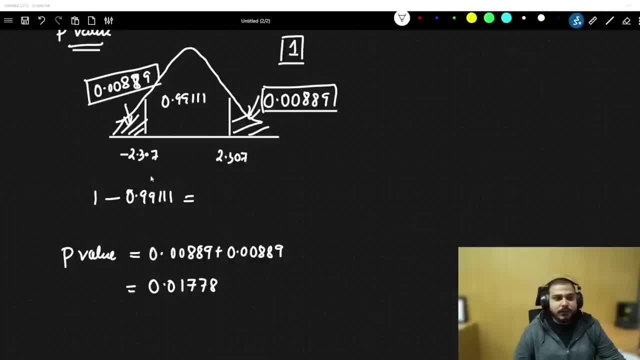 over there. probably i will be able to see that specific part right, because this part is symmetrical to this part. do you think it is divided by two? do you think it is divided by two? no, i don't think so. it should be divided by two. it should. it is basically. 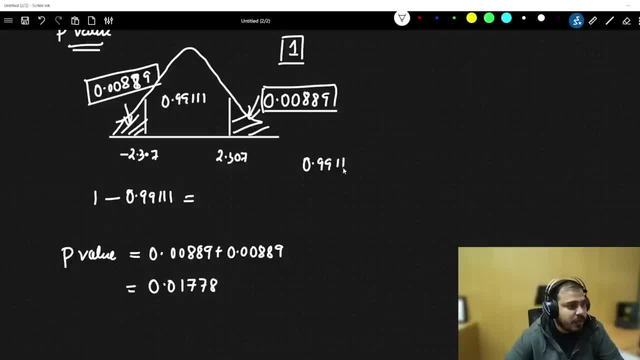 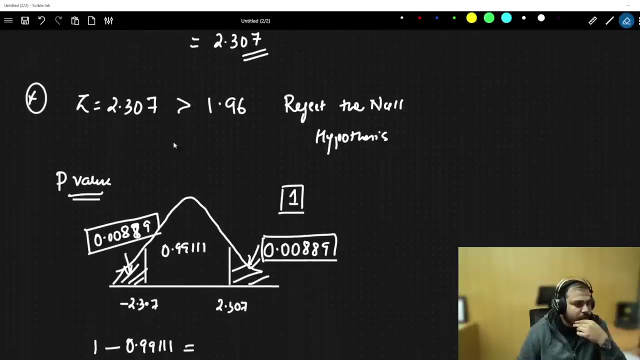 considered at this part and this part, right: 0.99111. oh yeah, should we divide by two? yes, yes, then only probably i will be able to. okay, so probably we are getting more than one. so over here i am getting 2.307. 2.307 is greater than 1.96. 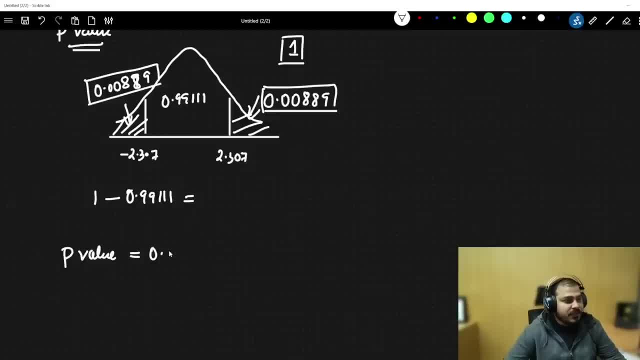 it is two tail. I have to add this up and then this will basically give my p-value 0.00889.. So once I add this particular value, I am actually going to get 0.01778, is it not 0.889 divided by 2?? 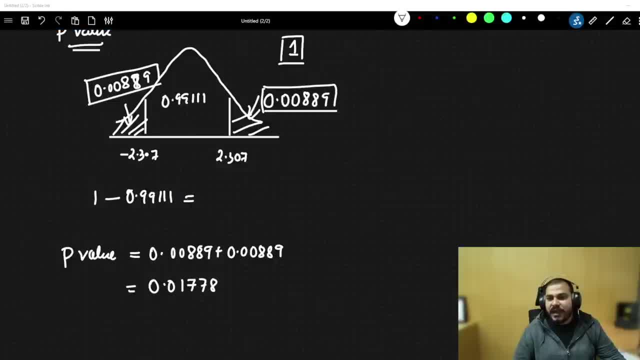 No, because see, both the area are symmetrical. understand one thing: both the area are symmetrical. If I am getting one value over there, if I am getting one value over there, probably I will be able to see that specific part right. 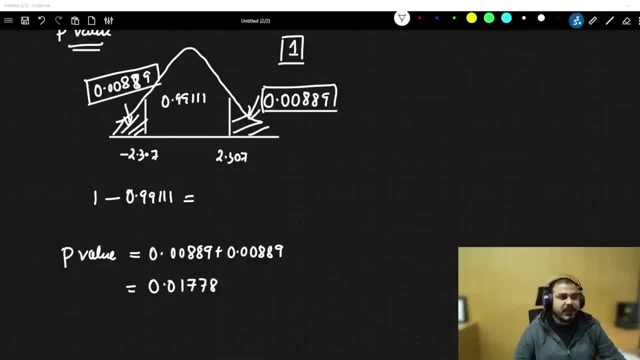 So I will be able to see that specific part right, Because this part is symmetrical to this part. Do you think it is divided by 2?? Do you think it is divided by 2?? No, I don't think so. it should be divided by 2.. 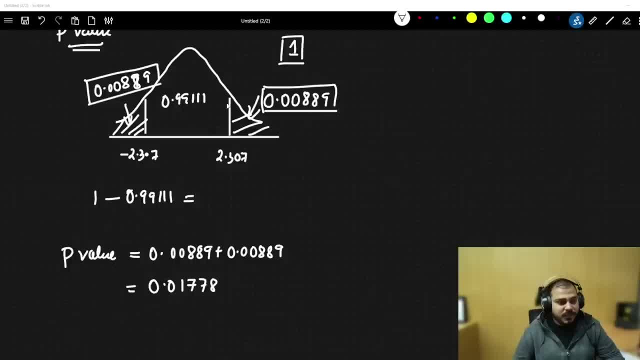 It should. it is basically considered at this part and this part right: 0.99111,. oh yeah, should we divide by 2?? Yes, yes, then only probably I will be able to. okay, So probably we are getting more than 1.. 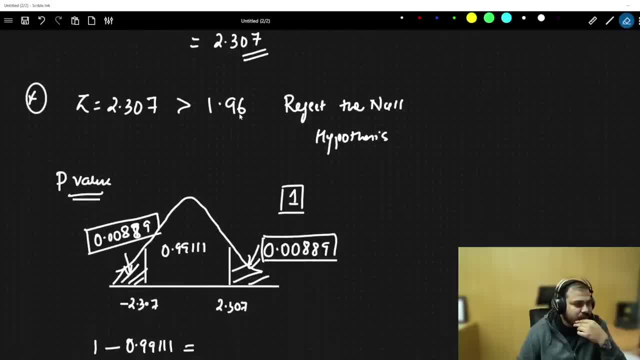 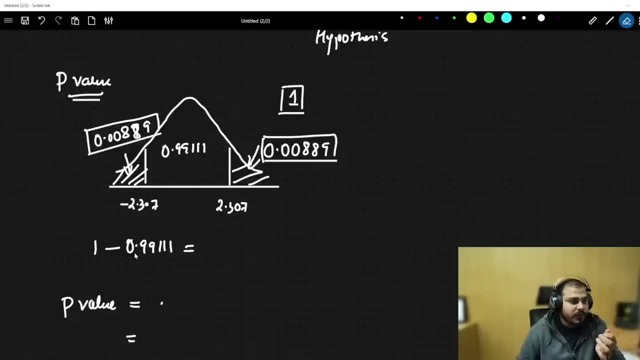 So over here I am getting 2.307,. 2.307 is greater than 1.96,. with respect to 2.3007, I am actually getting the value as 0.99111, okay, So 1 minus 0.99111 will be nothing, but so 0.0044,, this area, 0.0044.. 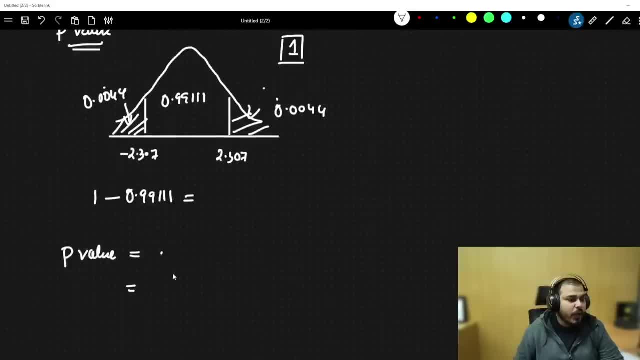 Now, if we add it, we will be getting till 1.. Now, in order to add the p-value, Okay, To get the p-value, I will take this area 44 plus 0.0044.. Now here you can see that I am getting 0.0088.. 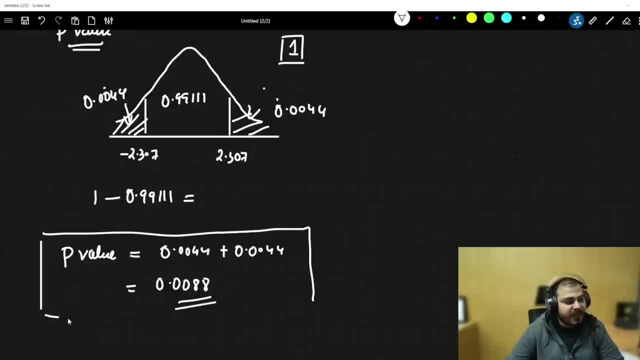 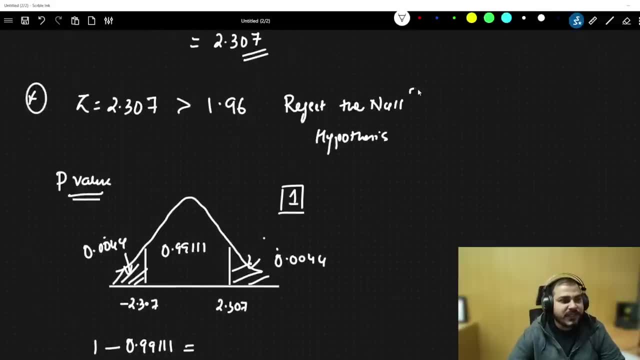 Now this is basically my p-value. okay, Because based on the real z-score that I have got, I will be deriving my p-value from here. Now, obviously, we know that we have to reject the null hypothesis Now from the p-value also, we can actually verify. 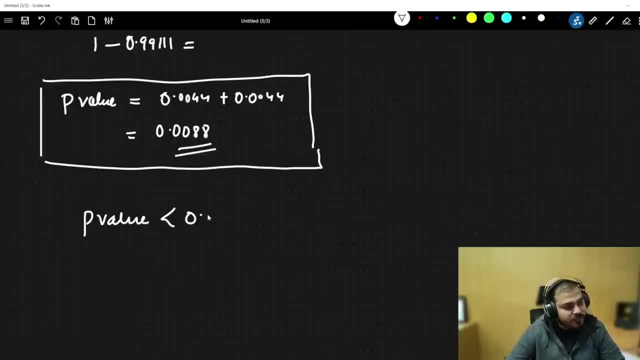 Here now. this p-value is obviously less than 0.05, right, which is my significance value. So obviously 0.0088 is less than 0.05.. So what happens over here? we basically reject the null hypothesis. 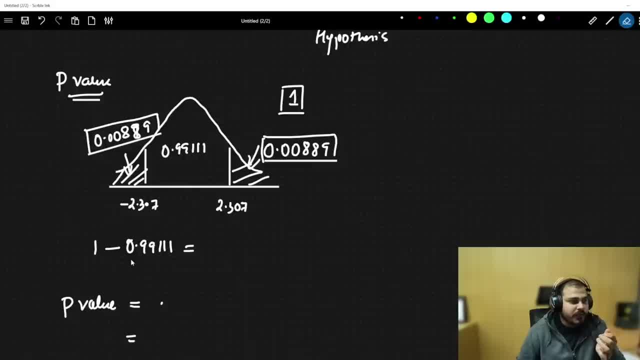 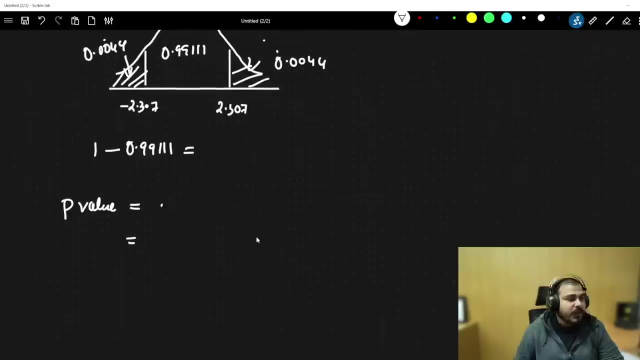 with respect to 2.3007, i am actually getting the value as 0.99111. okay, so one minus 0.99111 will be nothing, but so 0.0044, this area, 0.0044. now, if we add it, we will be getting till one. 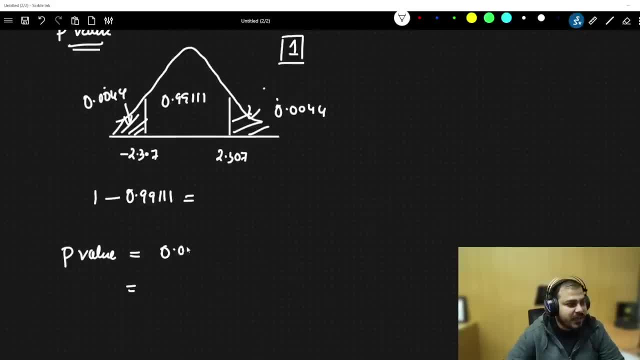 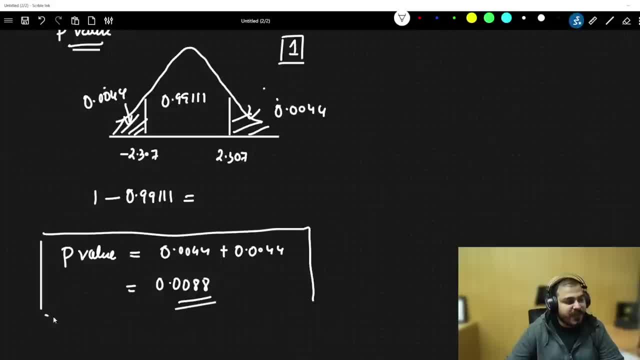 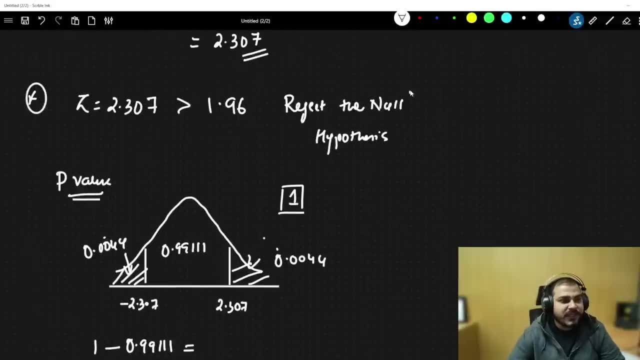 now this is basically my p-value. okay, because based on the real z-score that i have got, i will be deriving my p-value from here now. obviously, we know that it we have to reject the null hypothesis now from the p value. also, we can actually verify here now this p-value. 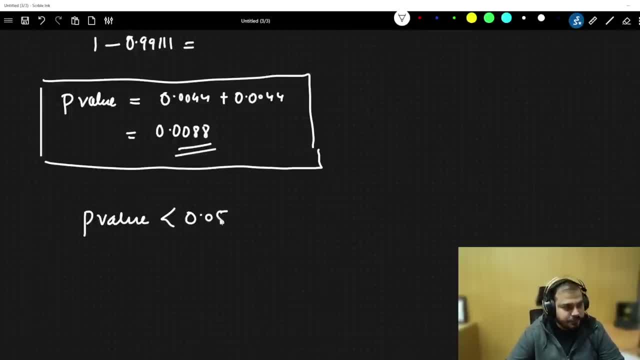 is obviously less than 0.05, right, which is my significance value. so obviously 0.0088 is less than 0.05.. So what happens over here? We basically reject the null hypothesis. So here we are rejecting the null hypothesis. Suppose if this p-value is greater than 0.05, always understand. 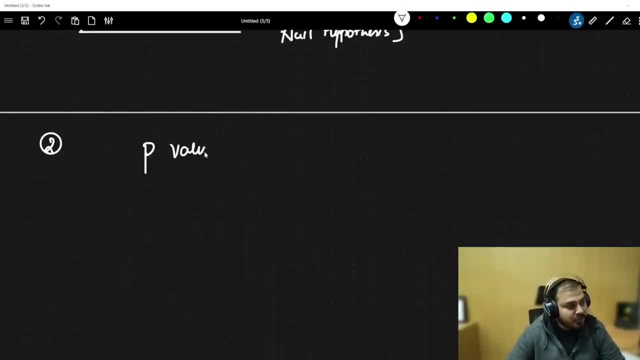 two important points. One is: p-value is less than your significance value. I hope you understood how to calculate the p-value right. So if this is less than or equal to the significance value, this means we have to reject the null hypothesis If the p-value is greater than. 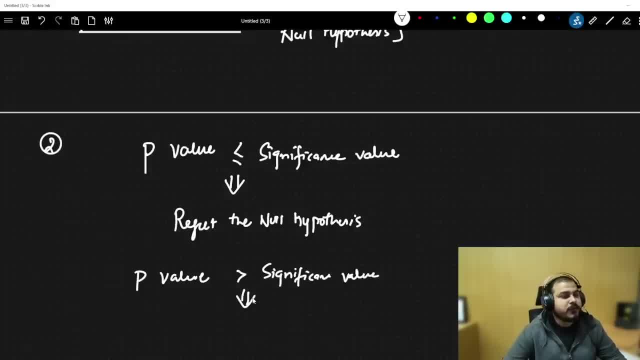 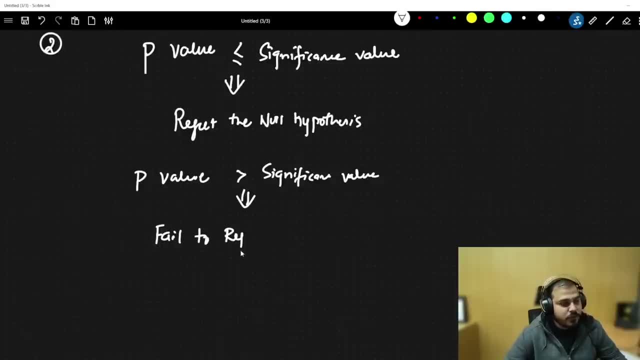 significance value. then what we do? We fail to reject the null hypothesis. We fail to or accept the null hypothesis. We fail to reject the null hypothesis. Now it is clear, guys from the yesterday's session. Now you can try out in every problem that we have probably discussed this many days. 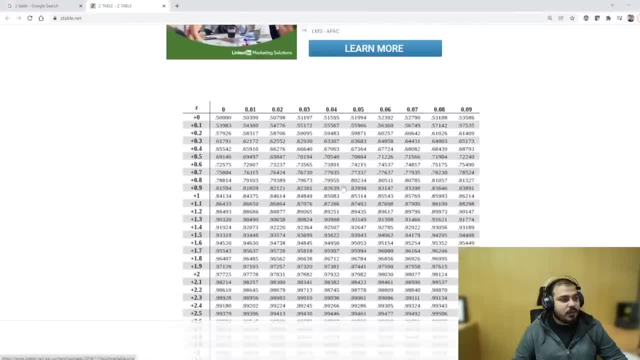 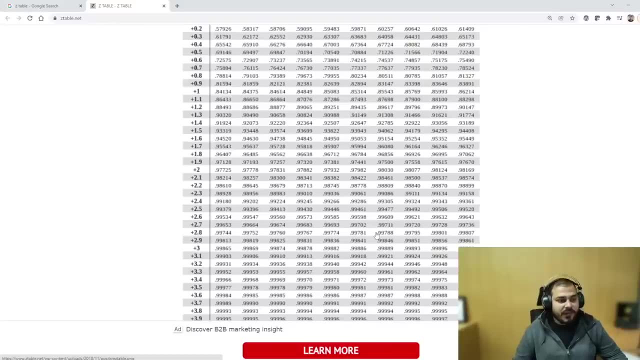 Okay, guys, whenever we have, Okay guys, whenever we have a z-table right Right now. one thing is that, first of all, I'll check with 0.025.. 1 minus 0.025 is 0.9750.. So if I go and see, probably somewhere you'll be able. 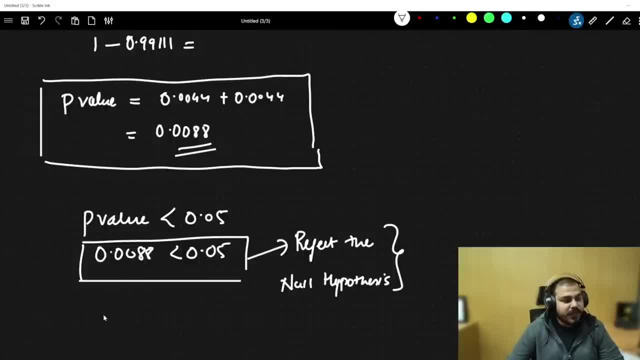 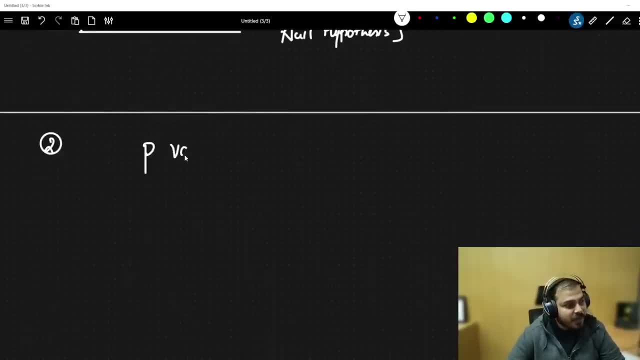 So here we are, rejecting the null hypothesis, Suppose if this p-value is greater than 0.05, always understand one two important points. One is: p-value is less than your significance value. I hope you understood how to calculate the p-value right. 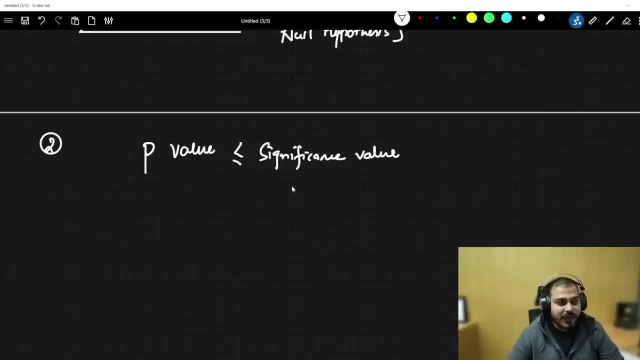 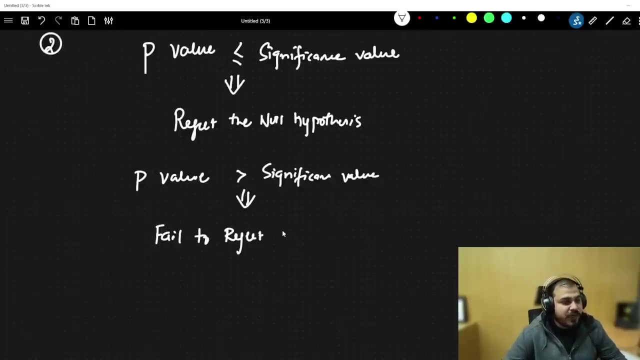 So If p-value is less than or equal to the significance value, this means we have to reject the null hypothesis. If the p-value is greater than significance value, then what we do? we fail to reject the null hypothesis. We fail to or accept the null hypothesis. we fail to reject the null hypothesis. 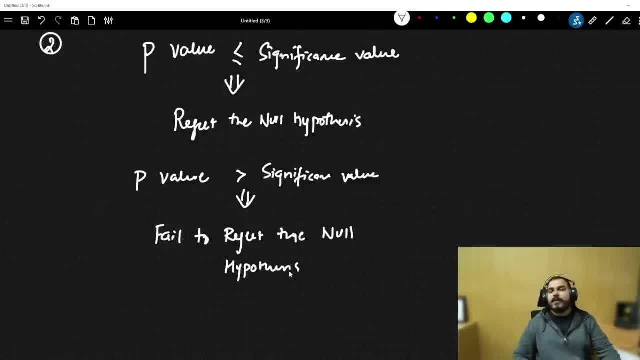 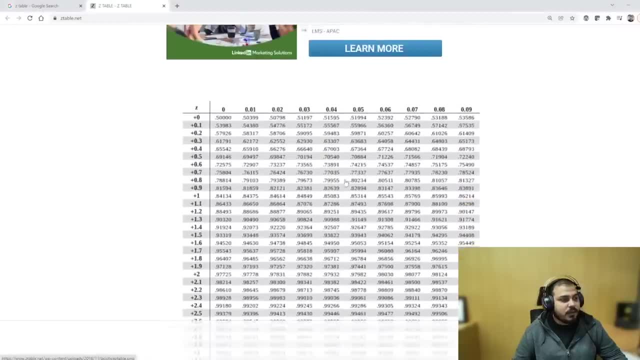 Now it is clear, guys, from the yesterday's session: now you can try out in every problem that we have probably discussed. See, guys, whenever we have a z-table right right now, one thing is that, first of all, I will check with 0.025.. 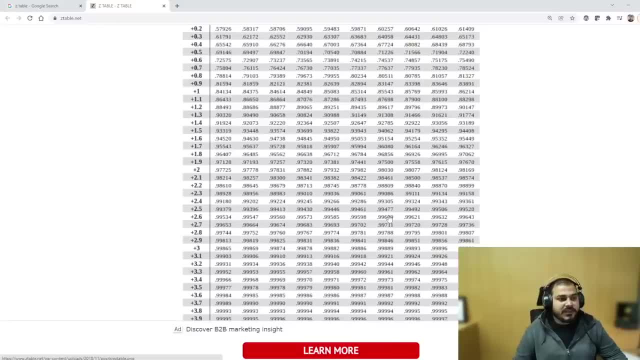 1 minus 0.025 is 0.9750.. So if I go and see probably somewhere you will be able to see 0.9750, where it is here. So it is nothing but plus 1.9 and this is 6.. 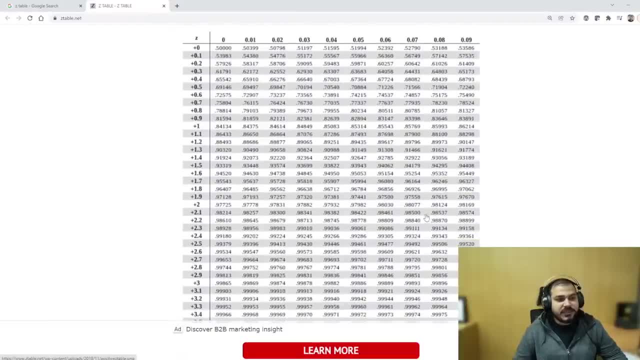 But we saw that our real z-score was coming as 2.37.. 2.30.. 2.30.. 2.30.. 2.30.. 2.37., 2.30.. 2.30.. 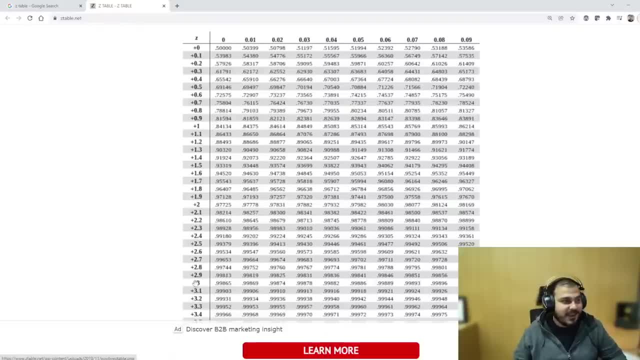 2.30 is this one. Okay, guys, 2.30 is this one. I took 2.307, okay. So again, there was a confusion over here. You can also take this one, See 1 minus 0.9828.. 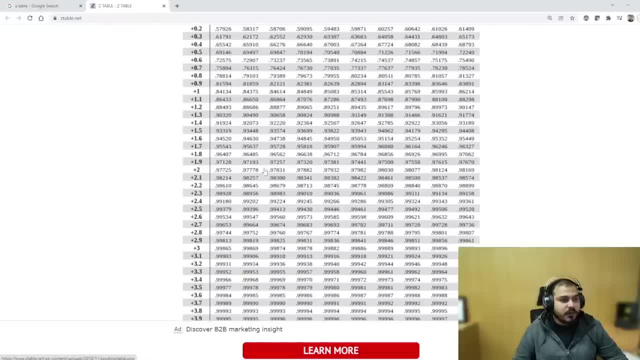 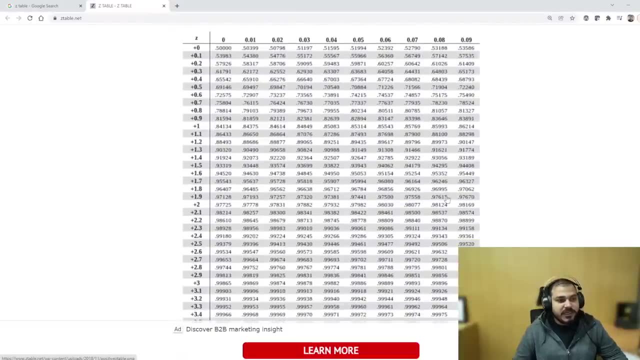 to see 0.9750 where it is here. So it is nothing but plus 1.9 and this is 6.. But we saw that our real z-score was coming as 2.37.. 2.30.. 2.30 is this one? Okay, guys, 2.30 is this one. 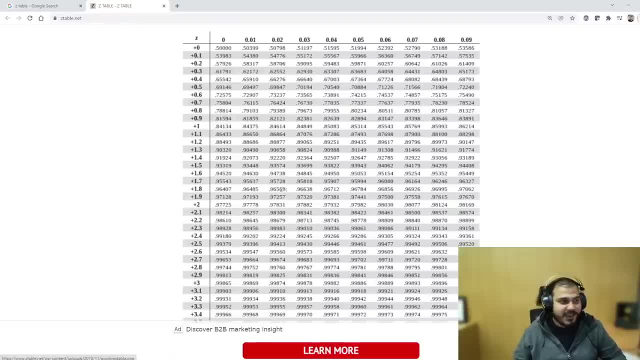 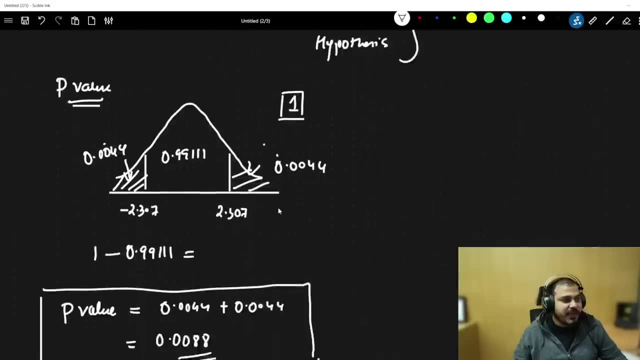 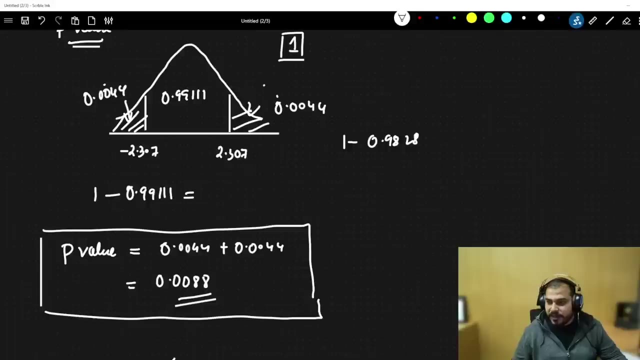 I took 2.307.. Okay, so again, there was a confusion over here. You can also take this one, See 1 minus 0.9828.. 1 minus 0.9828.. You can also do this: 1 minus 0.9828.. So if I subtract this: 1 minus 0.9828,. 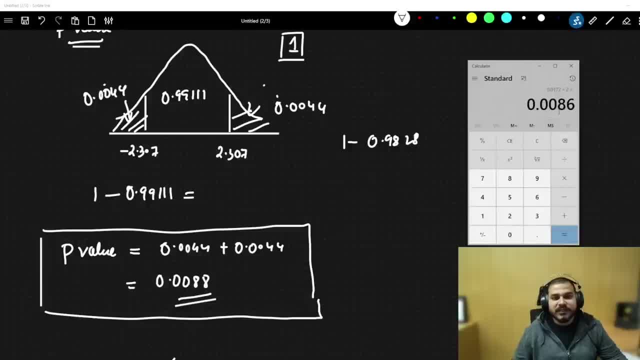 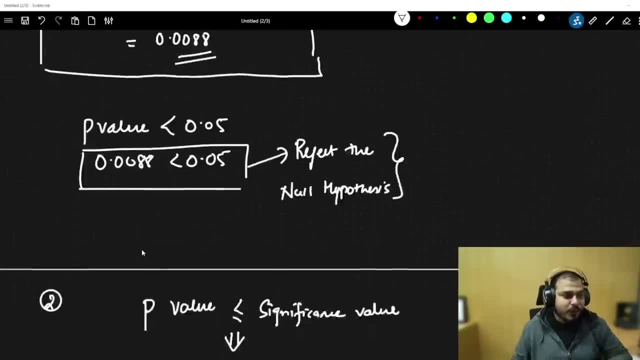 0.0172.. If I divide by 2,, this will be 0.0086.. You can take this up. Okay, again, I'm going to repeat this. Okay, let's see, I'm planning to repeat it. Okay. 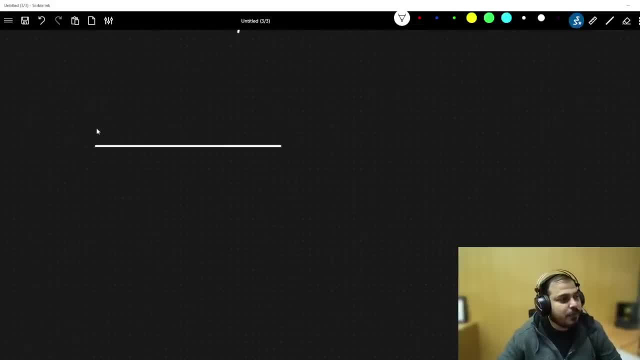 fine, Not a problem. See initially what I got. my value was this: right, I got this as minus 1.96.. This as plus 1.96.. But based on the z-score calculation, how much we got with. 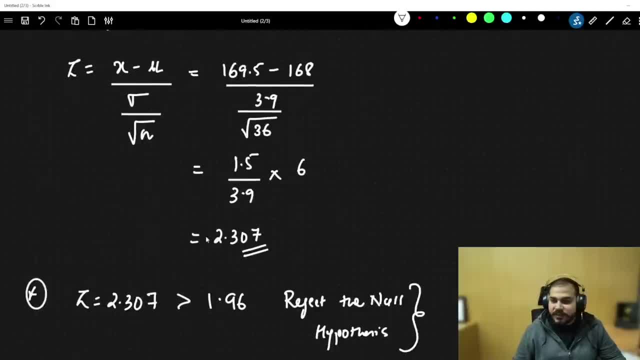 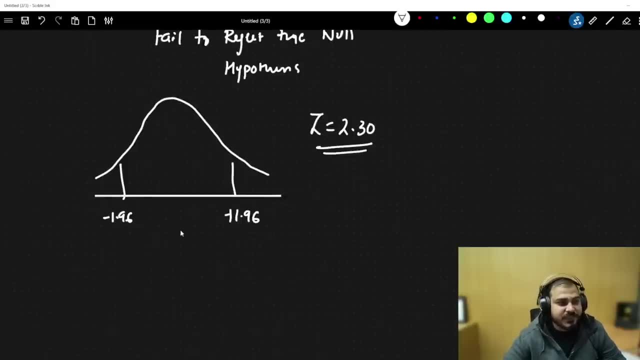 respect to z-score calculation. Here you can see I got 2.307.. Okay, 2.307.. So here I'm actually going to get 2.30.. Okay, let's take this. So obviously my z is 2.30.. It is greater. 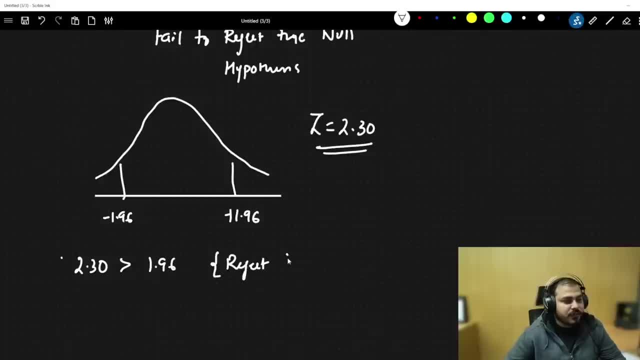 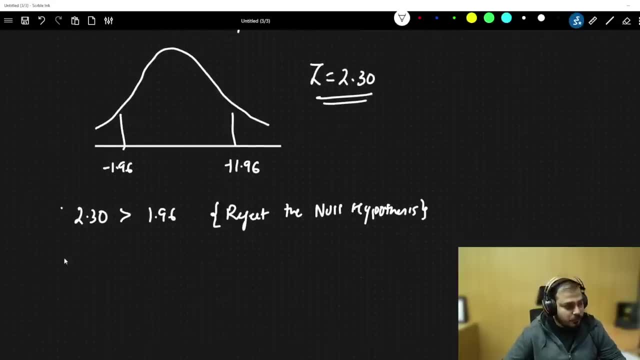 than 1.96.. So I've told you, we have to reject the null hypothesis in this case. This is, with the help of z-score Now, what I'm actually going to do. Let's calculate the p-value Now in order to. 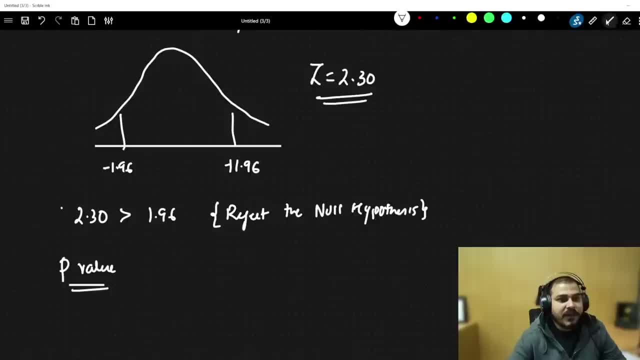 calculate the p-value. okay, what I will do, I will rub this and I'll try to find out the area with respect to this z-score That is 2.30.. So plus 2.30, minus 2.30.. And I will try to find out. 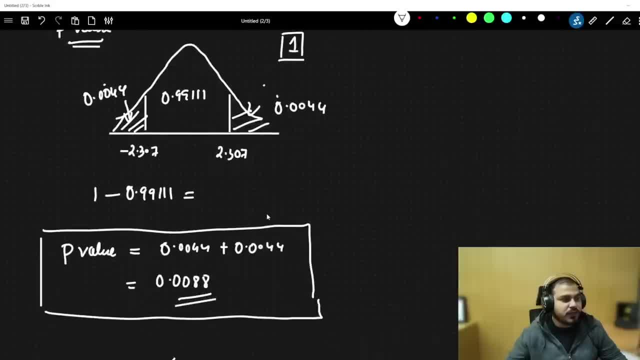 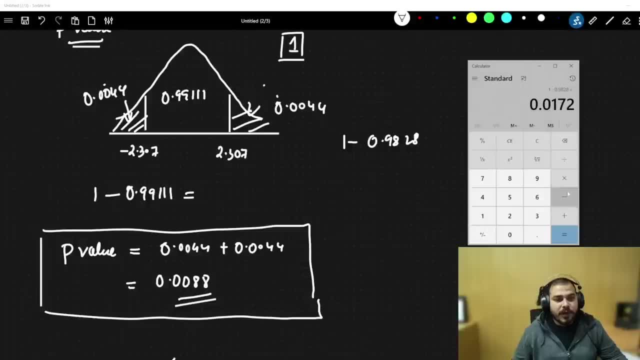 1 minus 0.9828.. You can also do this: 1 minus 0.9828.. So if I subtract this, 1 minus 0.9828, 0.0172,, if I divide by 2, this will be 0.0086.. 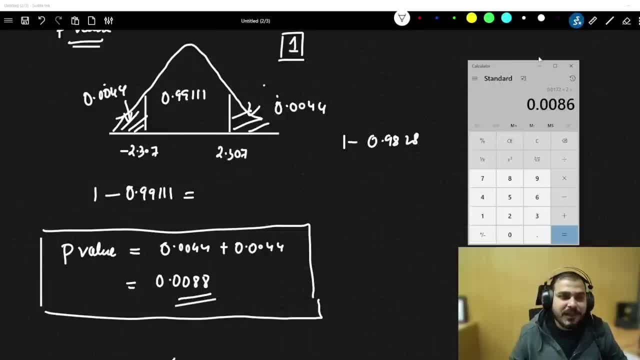 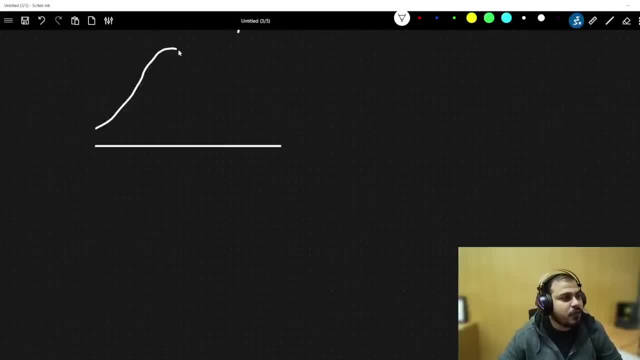 You can take this out, okay, and I'm going to repeat this. okay, Let's see, I'm planning to repeat it, okay, Fine, not a problem. See initially what I got. my value was this: right, I got this as minus 1.96, this as: 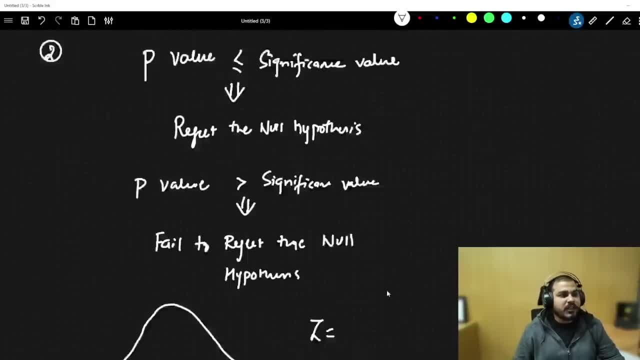 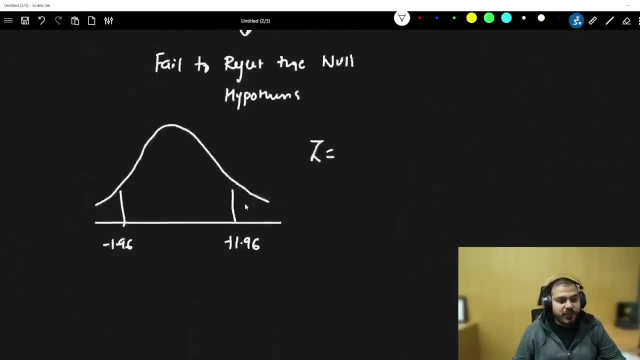 plus 1.96.. But based on the z-score calculation, how much we got with respect to z-score calculation? Here you can see I got 2.307, okay, 2.307.. So here I'm actually going to get 2.30, okay, Let's. 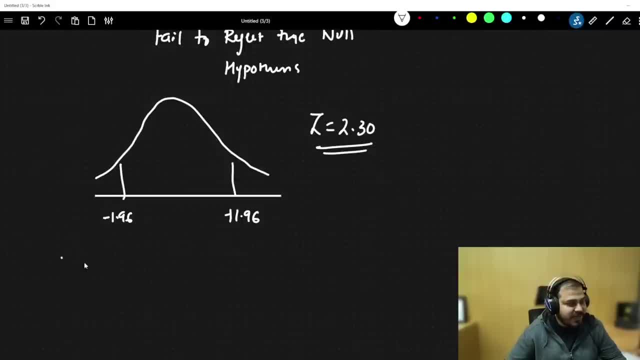 take this: So obviously, my z is 2.30, it is greater than 1.96.. So I've told you we have to reject the null hypothesis in this case. This is, with the help of z-score, Now, what I'm actually. 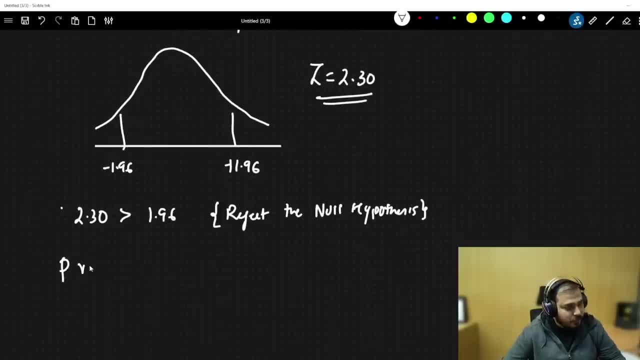 going to do. let's calculate the p-value Now. in order to calculate the p-value, okay, what I will do, I will rub this and I'll try to find out the area with respect to this z-score, that is 2.30.. 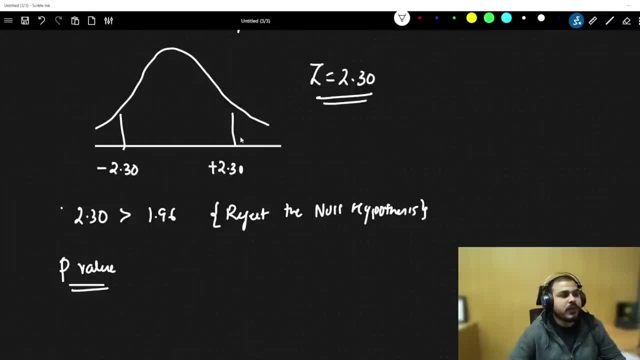 So plus 2.30.. Minus 2.30.. And I will try to find out what is this area And based on this, I'll be able to find out this area also. So let's go ahead in the z-table now. So this is my z-table: 2.30, okay. 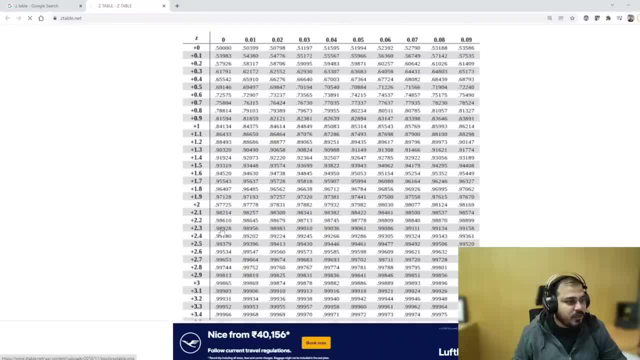 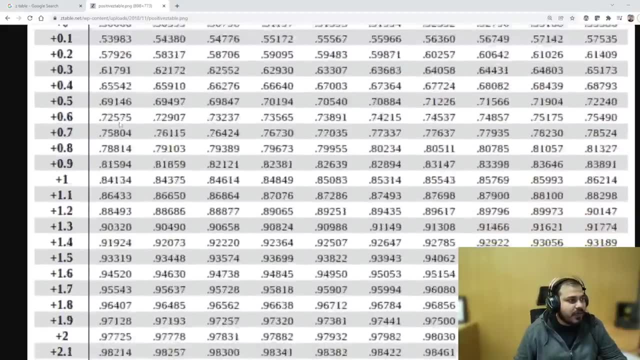 2.30.. So here is my value: 0.98.. See this, guys. I'm again repeating it: 2.30, right, This is my z-score value, So 0.98928.. So here I'm actually going to get 2.30.. So this is my z-score value. 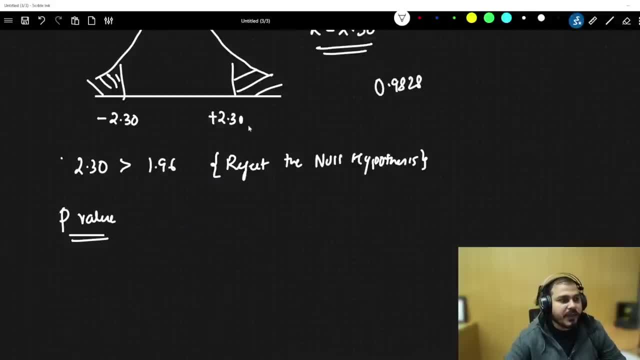 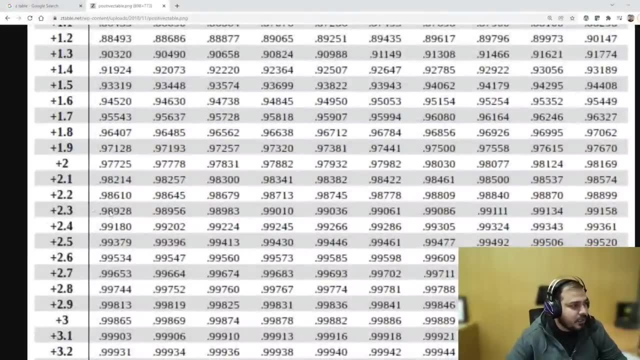 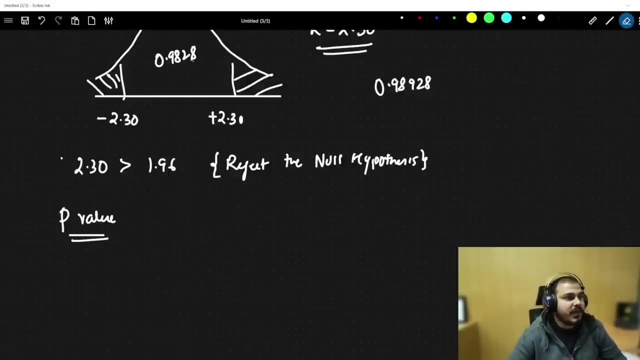 So I will be getting 0.9828, right? So this is my area under the curve: 0.9828.. I guess 0.9828, only 2.30, 0.98, 928, okay, 0.98, 928.. Now, when I subtract 1 minus 0.9828,, then I will be getting 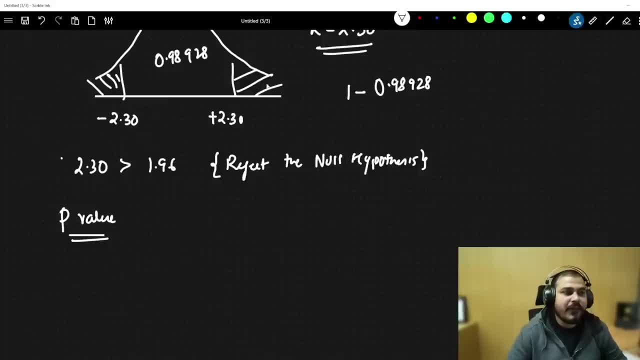 this area and this area right, Since I will be getting 0.9828, I will be getting 0.9828.. So this will have to get this particular area. So I have to subtract with the whole 1.. So if I go and 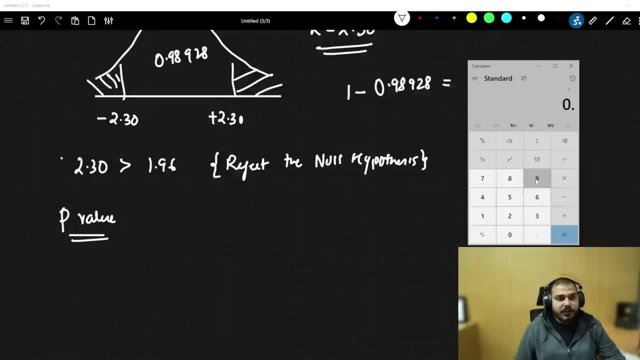 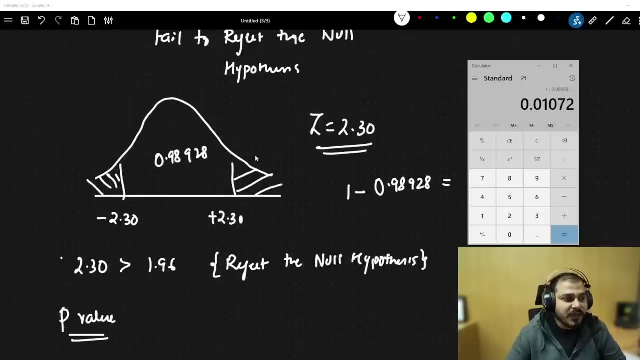 calculate now: 1 minus 0.98928.. So it is nothing but 0.01772.. Now understand, this is not one-tail test, This is two-tail test. So I have to divide the area from here to here also. So that is the. 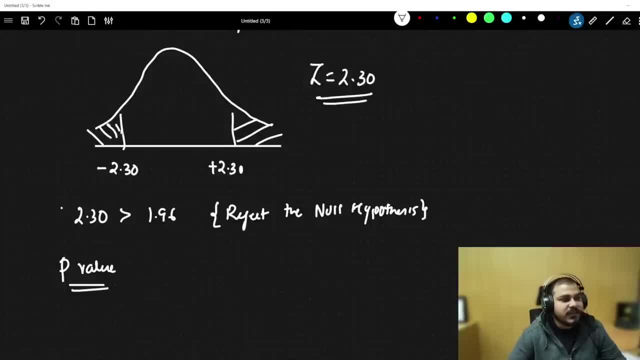 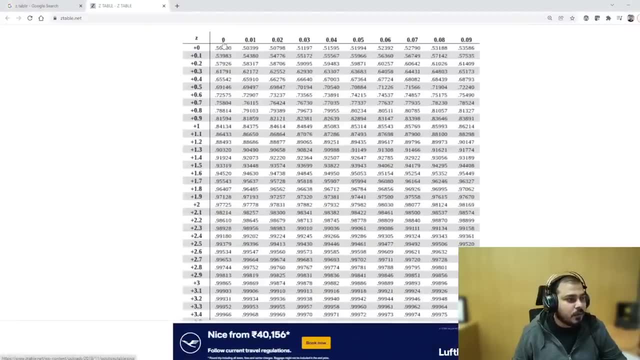 what is this area And based on this, I will be able to find out the area with respect to this area. So let's go ahead in the z-table now. So this is my z-table: 2.30.. Okay, 2.30.. So here. 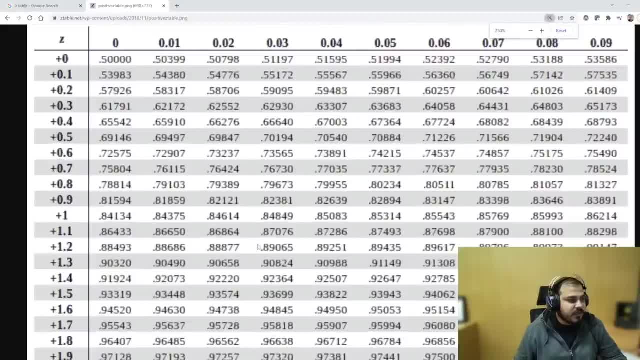 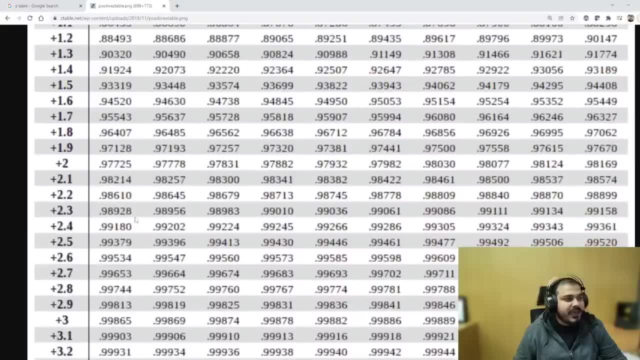 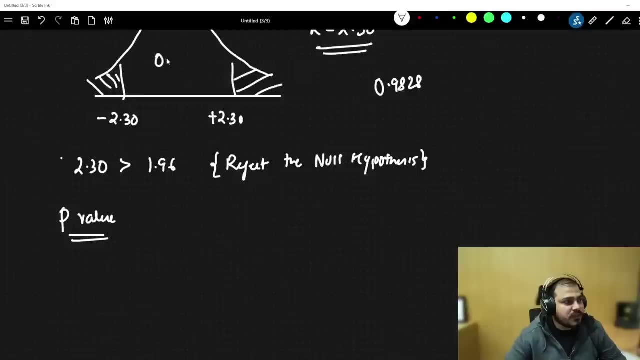 is my value 0.98.. See this, guys. I'm again repeating it: 2.30.. Right, This is my z-score value, So 0.98928.. So here I'm actually getting 0.9828.. Right, So this is my area under the 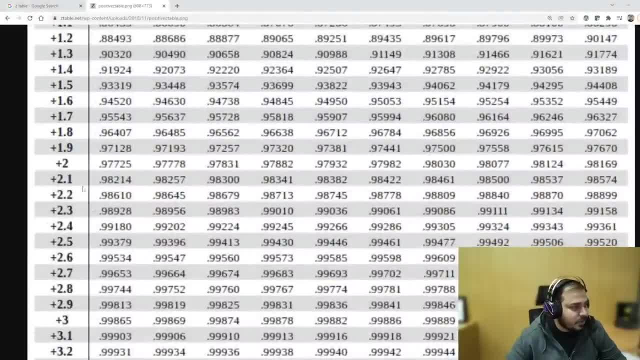 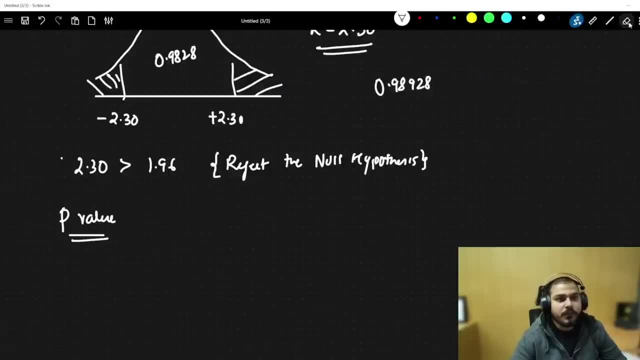 curve 0.9828.. I guess 0.9828, only 2.30.. 0.9892.. 0.928.. Okay, 0.98928.. Now, when I subtract 1 minus 0.9828, then I will be getting this area and this area Right, Since I will have to get. 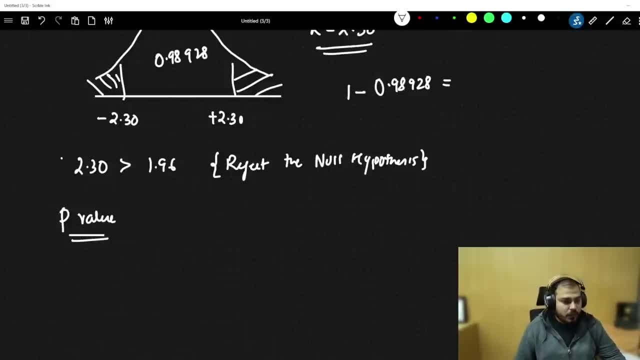 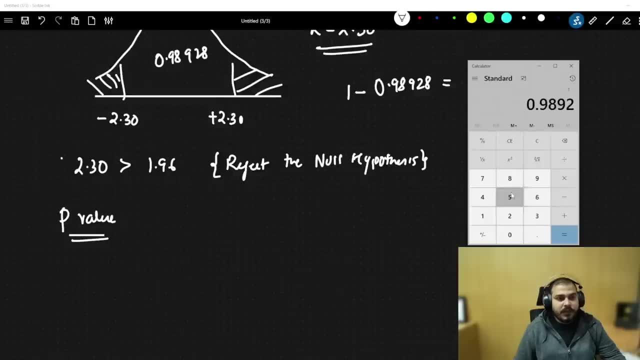 this particular area. so I have to subtract with the whole 1.. So if I go and calculate now, 1 minus 0.98928.. So it is nothing but 0.017.. 1072.. Now understand, this is not. 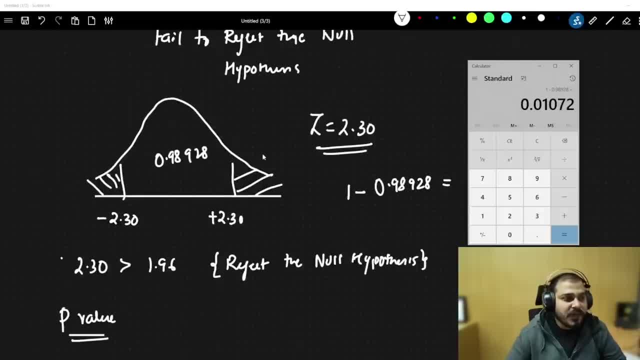 one-tailed test. This is two-tailed test, So I have to divide the area from here to here also. So that is the reason why I divide by 2.. So I'm going to divide by 2.. So I'm actually going to. 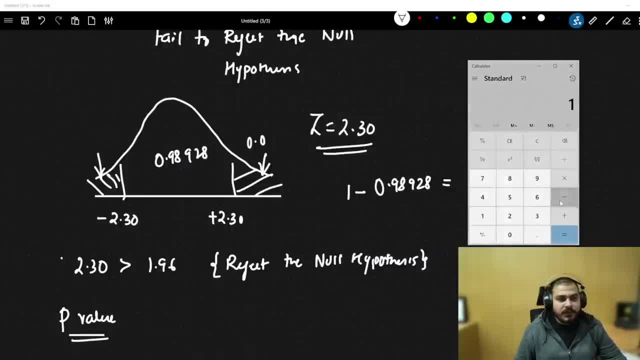 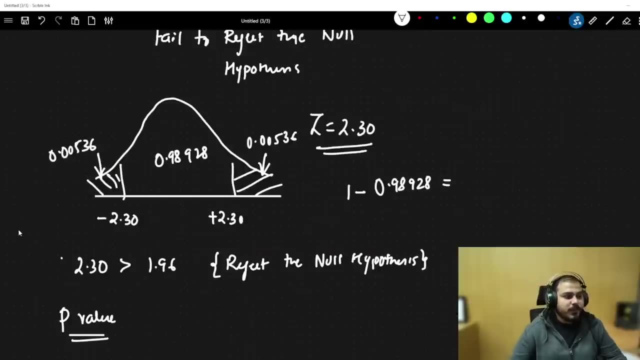 get this as 0.001 minus 0.98928.. So I'm actually going to get this as 0.001 minus 0.98928.. So I have to divide by 2.. So it is nothing but 0.00536.. Then 0.00536.. In p-value I will add: 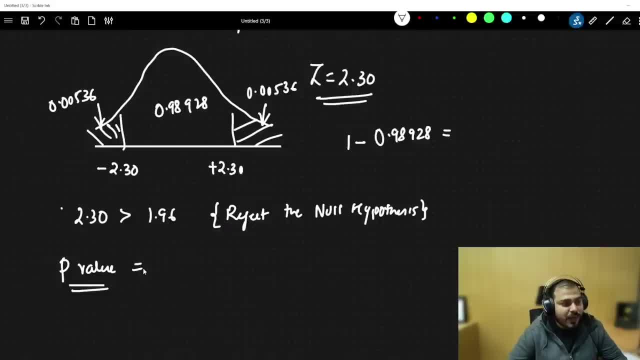 this two term. Understand, guys, what I am actually trying to do. You have to check out the z-table. So if I add this, probably then I will be getting some value, And then check whether this is less than significance value, Less than alpha, Less than or equal to 0.017.. 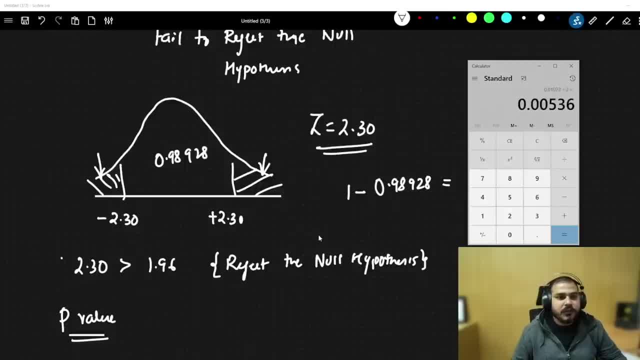 reason why I divide by 2.. So I'm going to divide by 2.. So I'm going to divide by 2.. So I'm going to divide by 2.. So I'm actually going to get this as 0.001 minus 0.98928 divided by 2.. So it is. 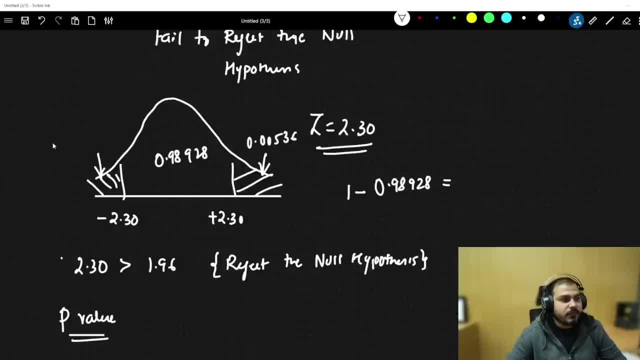 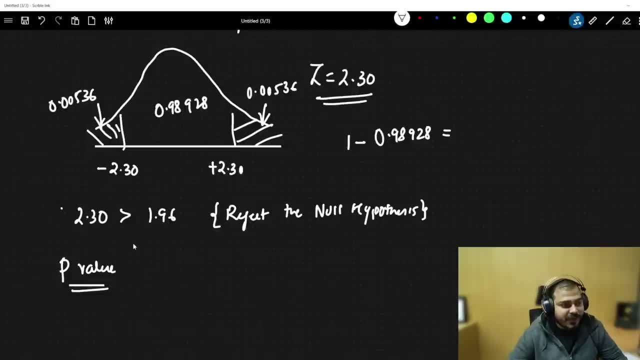 nothing but 0.00536.. Then 0.00536.. In p-value I will add this two term. Understand, guys, what I'm actually trying to do. you have to check out the z-table. So if I add this, probably, then I will. 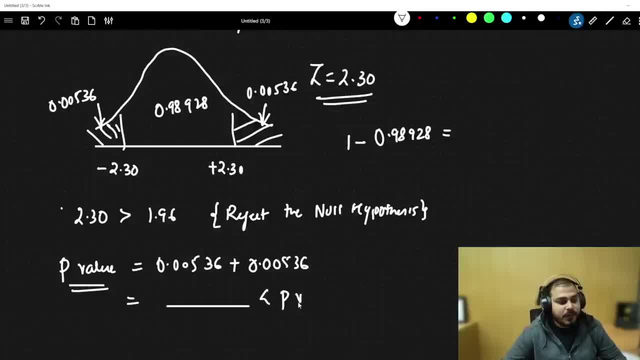 be getting some value, And if I add this, then I will be getting some value. So if I add this, then I will be getting some value. So if I add this, then I will be getting some value, And then check whether this is less than significance value Less than alpha, less than or equal to alpha. 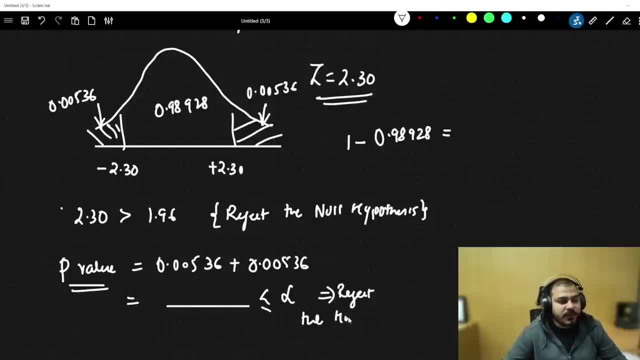 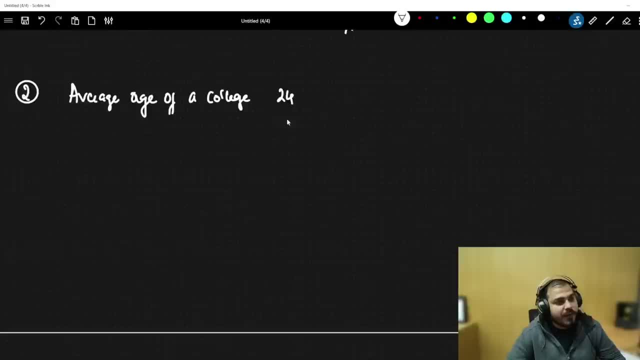 then you reject the null hypothesis And obviously this case also. it will be less than Let's solve this problem. So the average age of a college: 24 years, with a standard deviation 1.5.. So this is. 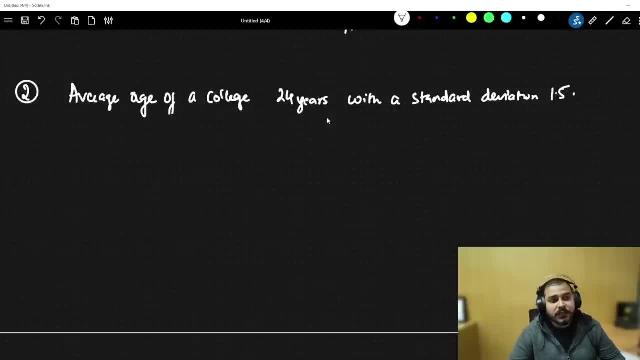 a college. over here, The average age of a college is 24 years, with a standard deviation of 1.5.. Now what I'm actually going to do is I'm going to add this to here. So I'm going to add this to. 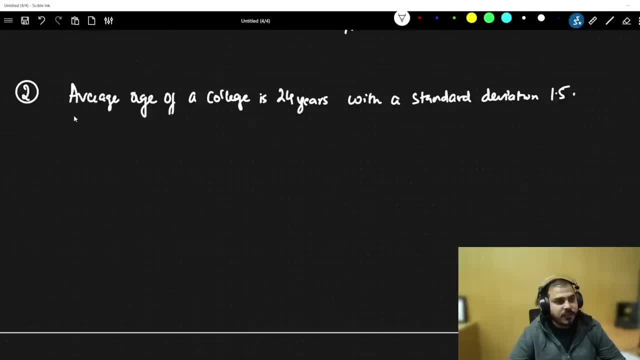 here. So what I'm actually going to do over here is that I'm just going to say that, okay, fine, the average age of the college is this much, this much. So we take a sample of 35 students, Let's. 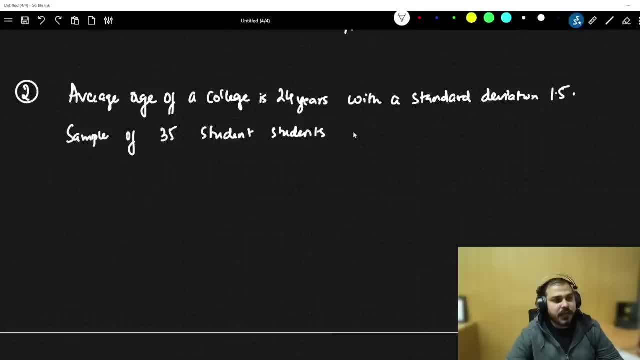 say that the mean. we take a sample of 35 students and we find out that the mean is 25 years. Then with alpha as 0.05, that is the confidence interval as 95%, With alpha as 1, point: alpha. as 0.5, that is the confidence interval as 95%. So that is the confidence interval as 0.5.. And then with alpha as 1.5, that is the confidence interval as 0.5.. So that is the confidence interval as 0.5.. 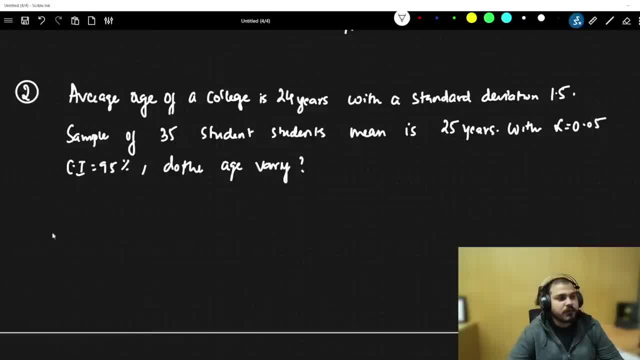 0.05 and confidence interval. do the age vary? okay? so this is the question. h0, you'll say: mean is equal to 24. h1, you'll say: mean is equal to mean is not equal to 24. you know your standard deviation, it is 1.5. you know your n value: it is 35, let's take it as 36, okay. and then your x bar is 25. 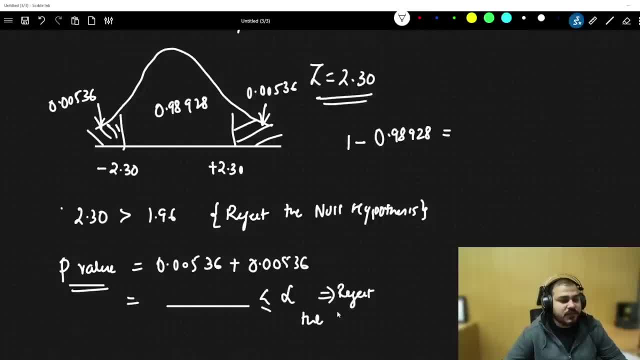 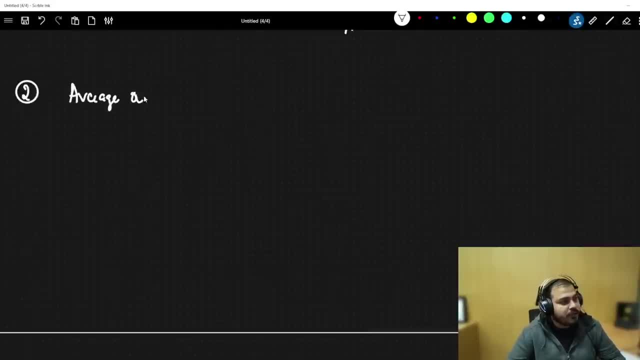 to alpha, then you reject the null hypothesis and obviously this case also. it will be less than let's solve this problem. so, uh, the average age of a college: 24 years with the standard deviation 1.5. so this is a college. over here, the average age of a college is 24 years with a standard. 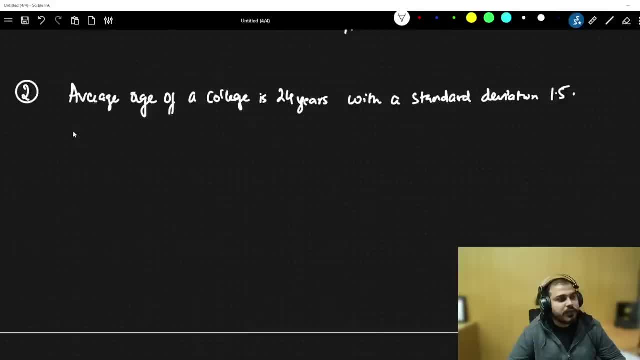 deviation of 1.5. now, what i am actually going to do over here is that i am just going to say that, okay, fine, uh, the average age of the college is this much, this much. so, uh, we take a sample of 35 students, let's say that the mean. we take a sample of 35 students and, uh, we find out that 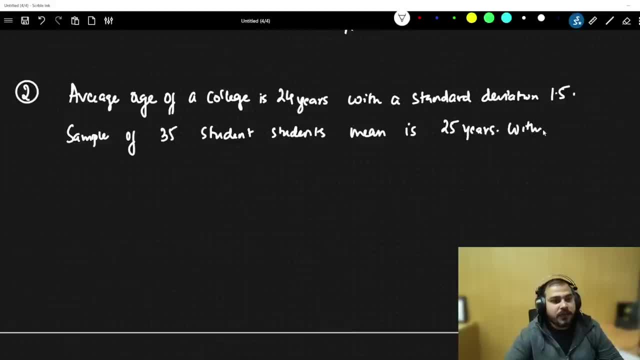 the mean is 25 years, then with alpha as 0.05, that is the confidence interval as 95 percent, with alpha as one point, alpha as 0.05 and confidence interval do the age, oh oh, vary, okay, so this is the question. h0, you'll say mean, is equal to 24. h1, you'll say mean is equal. 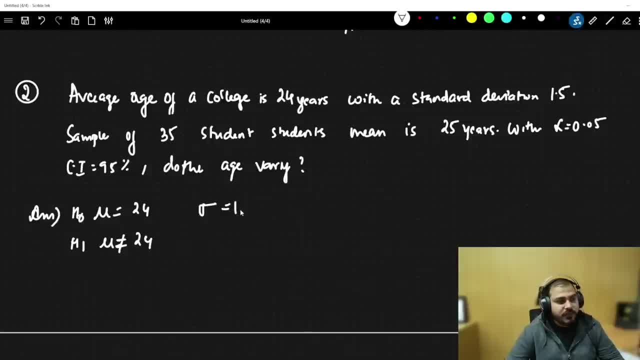 to mean is not equal to 24? you know your standard deviation: it is 1.5. you know your n value: it is 35, let's take it as 36, okay. and then your x bar is 25 and your alpha value is 0.05. now tell me. 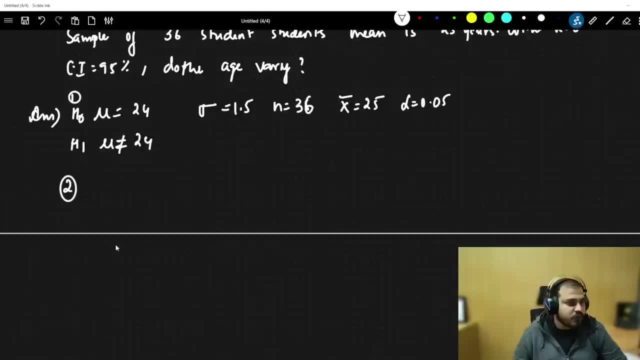 whether this is a two-tailed test or one-tailed test. it's a two-tailed test. so here you have your alpha as 0.05. now, if i make my confidence interval, my decision tree- sorry, my decision over here- this will be 0.025. why 0.025? this 0.05 will be divided into two regions, since it is. 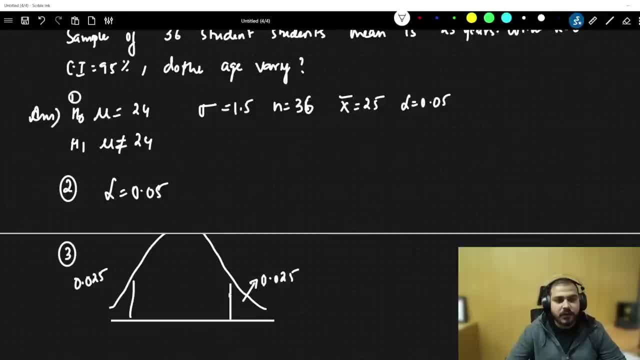 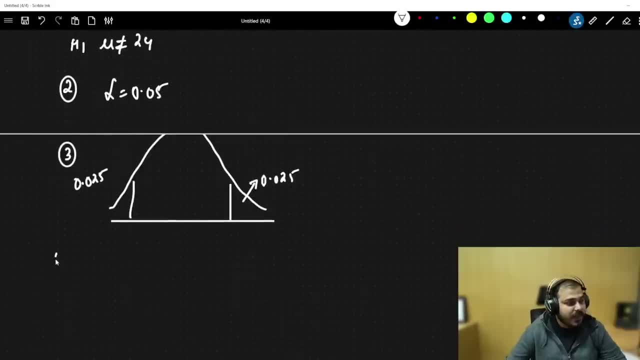 two-tailed test. if it is a one-tailed test, focus over here only. no focus over here only to solve it, why you don't have to worry about all those things you know. then let's go and solve. with respect to z score: you z score, x bar minus mu, divided by standard deviation, by root f. so what is my x bar? it is: 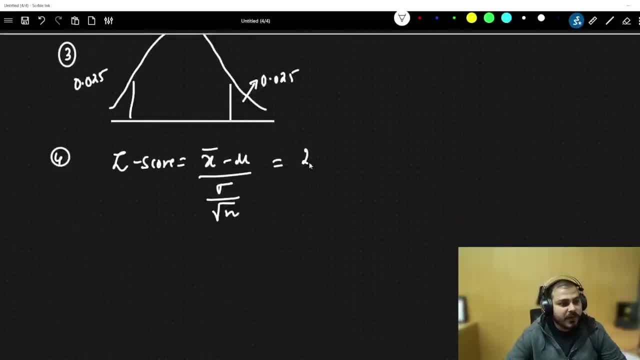 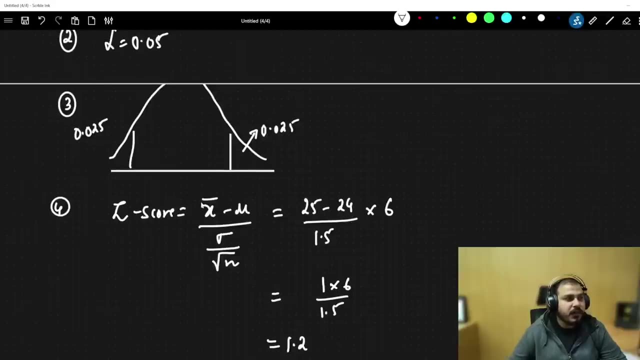 nothing but 25, 25 minus 24 divided by 1.5, multiplied by 6. so it is 1 multiplied by 6 divided by 1.5. go and calculate it. the z score is 1.2. you know the decision boundary. what is the decision boundary? 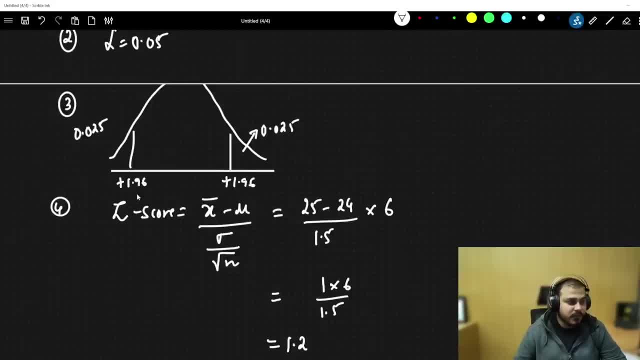 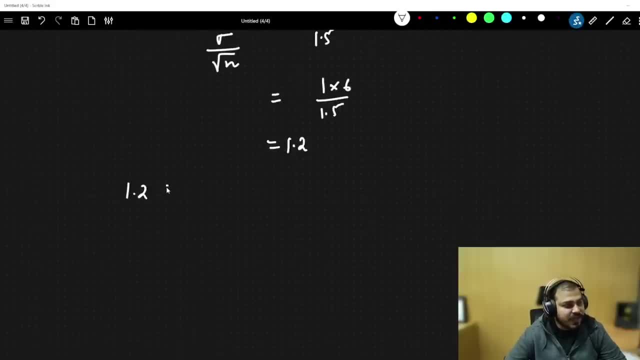 plus 1.96 plus 1.6, right now you are getting 1.2. if you are getting 1.2, then obviously 1.2 is less than 1.96. should we reject or accept the null hypothesis 4? are we getting 4? oh sorry, it is 4, extremely sorry now. 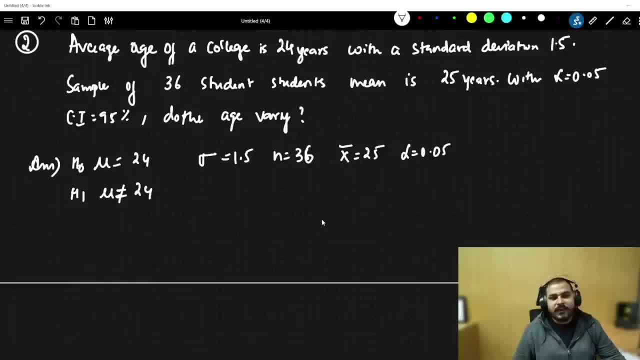 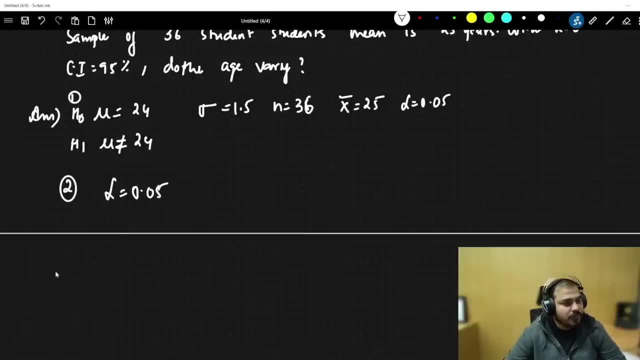 and your alpha value is 0.05. now tell me whether this is a two-tailed test or one-tailed test. it's a two-tailed test. so here you have your alpha as 0.05. now, if i make my confidence interval, my decision tree- sorry, my decision over here- this will be 0.025. why 0.025? this 0.05 will? 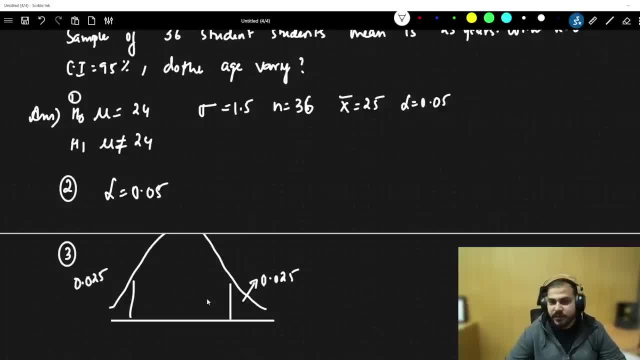 be divided into two regions, since it is two-tailed test. if it is a one-tailed test, focus over here only no focus over here, only to solve it, why you don't have to worry about all those things you know. then let's go and see. 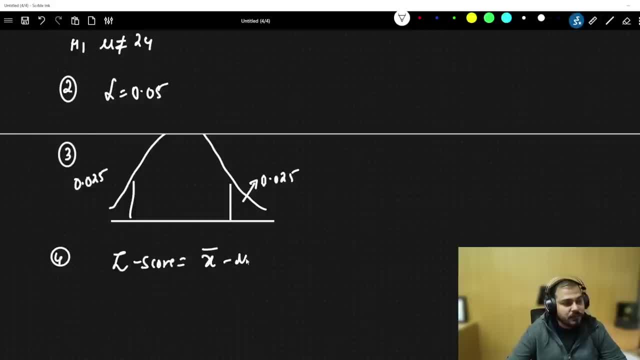 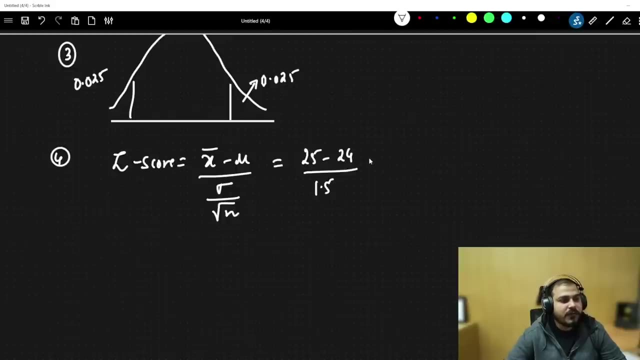 solve with respect to z score, z score, x bar minus mu, divided by standard deviation, by root f. so what is my x bar? it is nothing but 25, 25 minus 24 divided by 1.5 multiplied by 6, so it is 1. 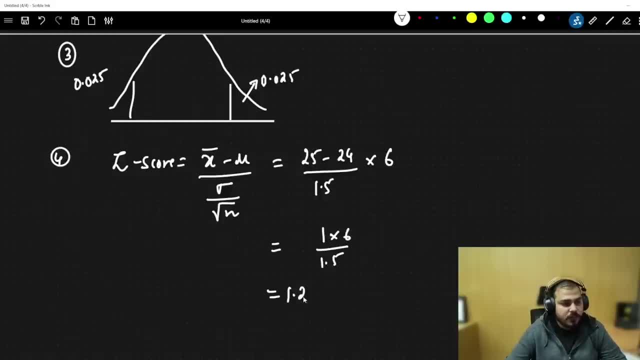 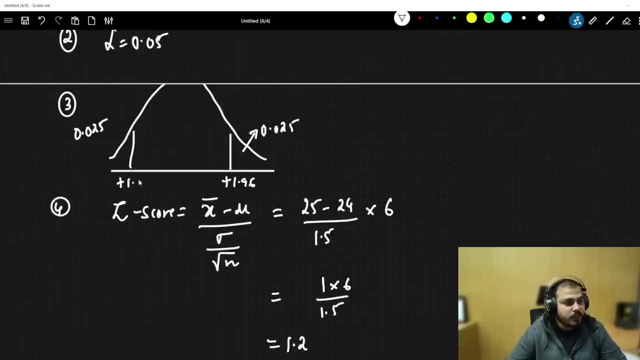 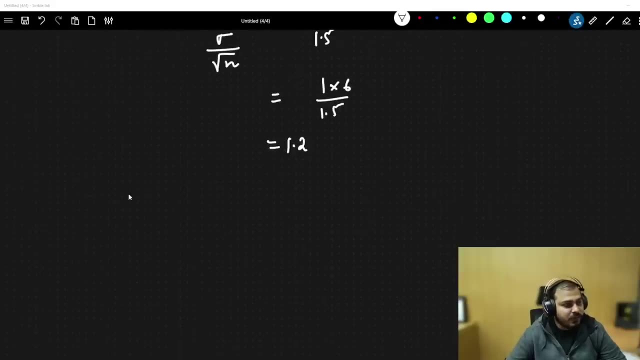 multiplied by 6, divided by 1.5, go and calculate it. the z score is 1.2. you know the decision boundary. what is the decision boundary? plus 1.96, plus 1.96: right now you are getting 1.2. if you are getting 1.2, then obviously 1.2 is less than. 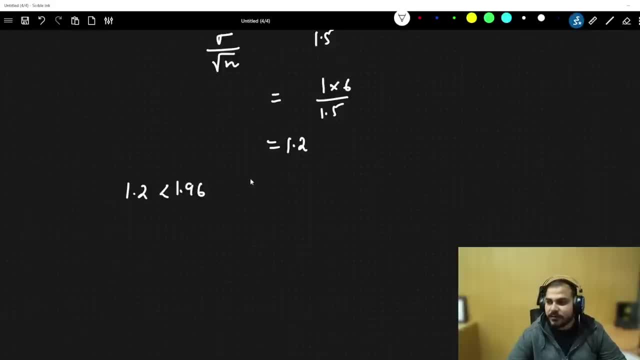 1.96. should we reject or accept the null hypothesis 4? are we getting 4? oh sorry, it is 4, extremely sorry. now, if you are getting 4, the 4 is greater than 4 is greater than 1.96. so we reject. 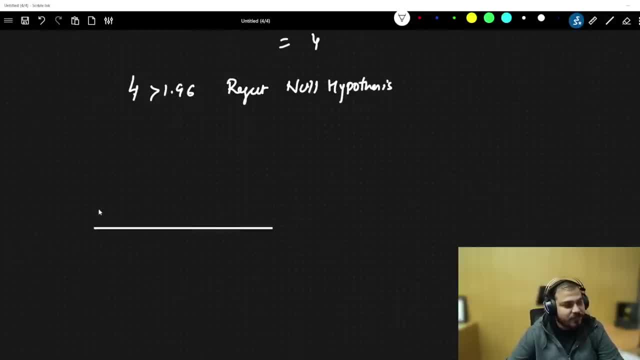 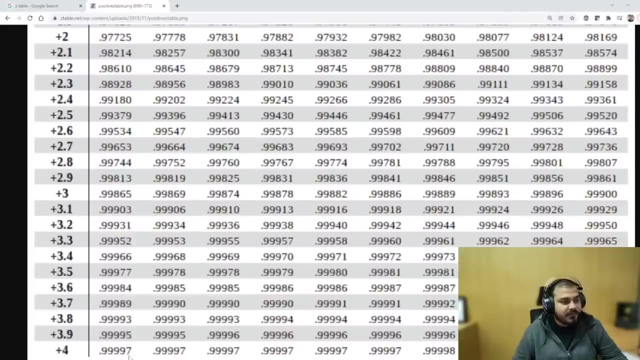 null hypothesis. now what you are going to do for this particular 4. you have got a 4 value, right, so this will be your plus 4. this will be your minus 4. now go to the z table. try to find out what is the 4 value. so go over here. try to find out what is 4. it is 0.99997 497, right, so it is 0.9997. 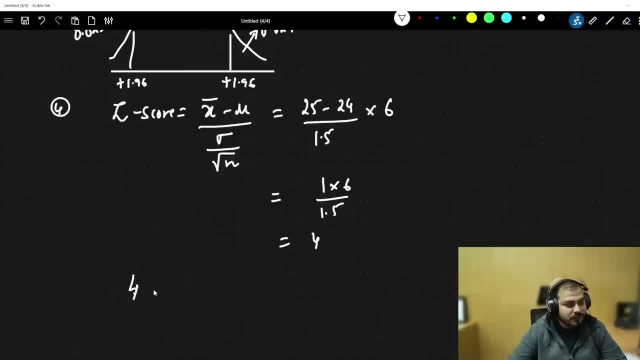 if you are getting 4, the 4 is greater than 4 is greater than 1.96, so we reject null hypothesis. now what you are going to do for this particular 4. you have got a 4 value right, so this will be a. 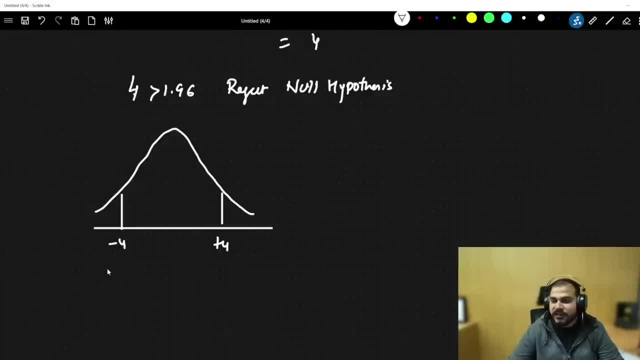 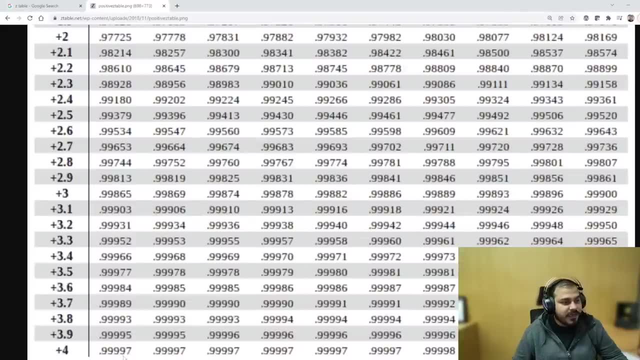 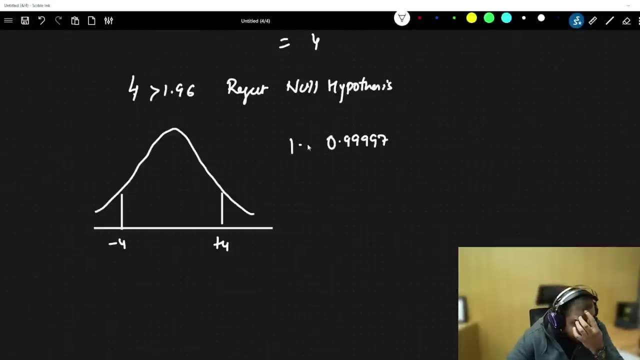 plus 4. this will be a minus 4. now go to the z table. try to find out what is the 4 value. so go over here. try to find out what is 4. it is 0.99997, 4, 9, 7, right, so it is 0.9997. so i will go and subtract. 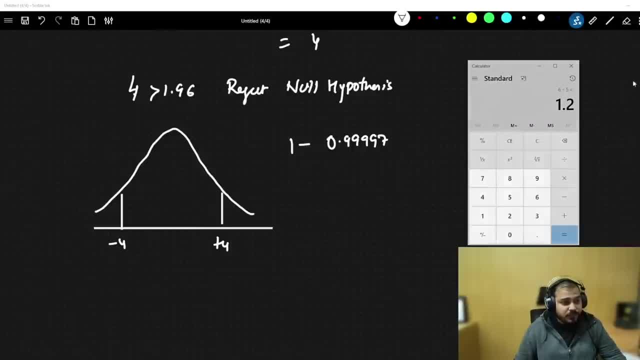 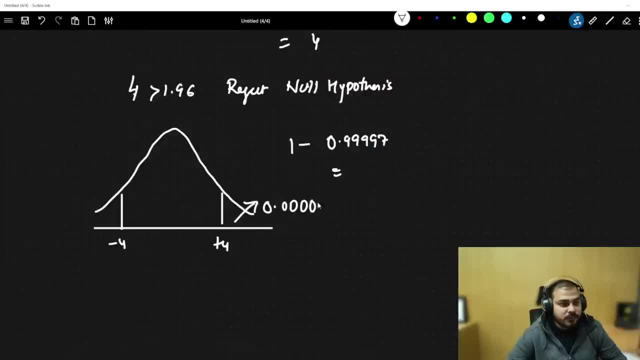 side will be 2 tilted, so this side will be 2 tilted, so this side is 2. 5 on B right now. so the truth you can write this: aggravated with 0 is 0. it is here because one is hidden as 0, saying so: the real problem is that when we add 0 as 0, difficult problem. 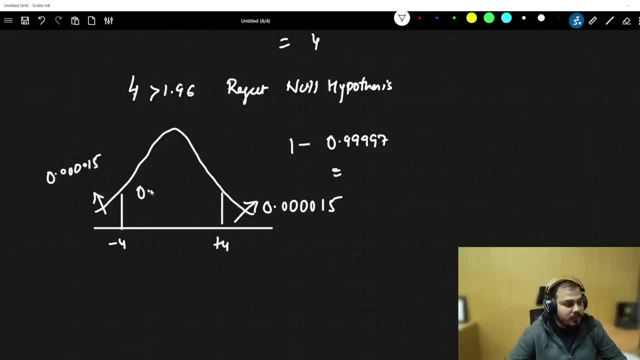 this positive Equ propia error when we add 0 as 0, such that all these key points are strongly. and this is the real problem, because it makes us feel that no, no, no, no, no, there is no guide, there is no guide to get rid of the errors there. your half will. 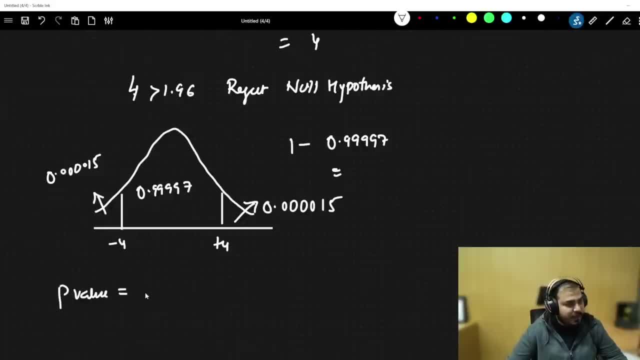 often people point 0 times, but there is a point here and there will be twopoints. 1 can be equal between 0, 0, F and 3 equals to 0, because this also gets rid of two points in standard Alfonzo, 1 for mu, so B of also has mean and 2 it is OK. this means B, F. 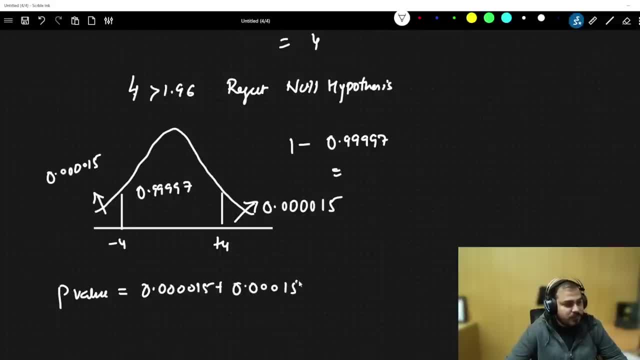 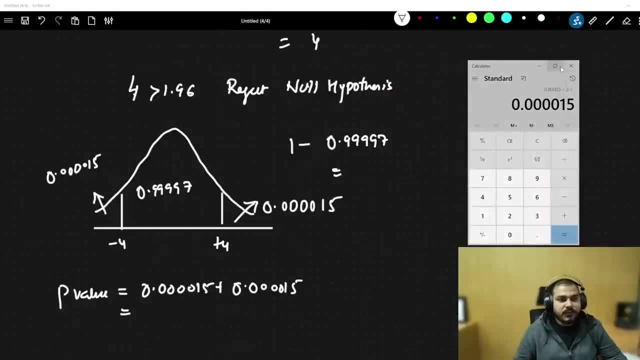 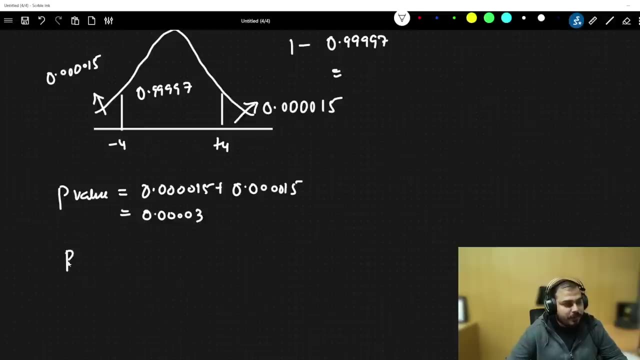 plus 0.00015. so what this will be? this will be nothing but the same thing: 0.403, 0.403.. Now, my p-value is obviously very, very lesser than significance value. so what we have to do? we have to reject the null hypothesis. reject the null hypothesis. 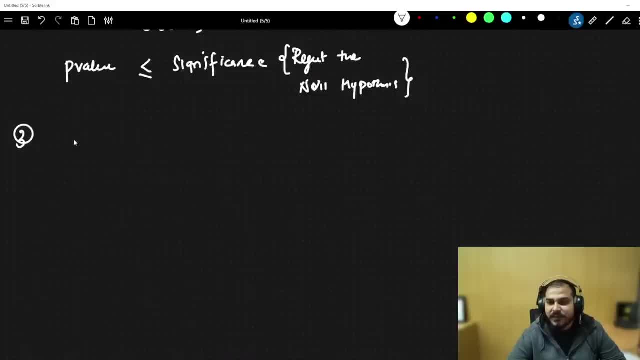 So here you can definitely say that with the sample size that we have taken, definitely we will not be able to conclude that the mean is that much. So let's go ahead with log normal distribution. ok guys, so log normal distribution. usually log normal distribution will have this kind of shape. obviously we have seen lot of examples. 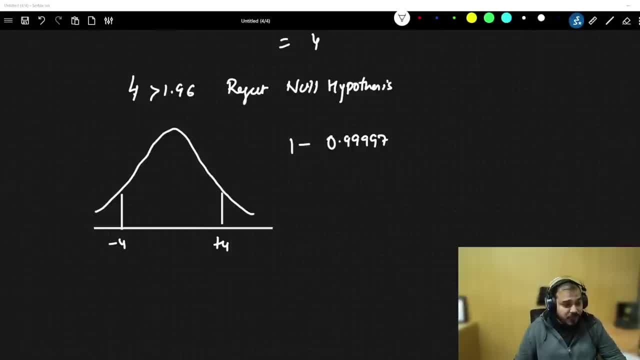 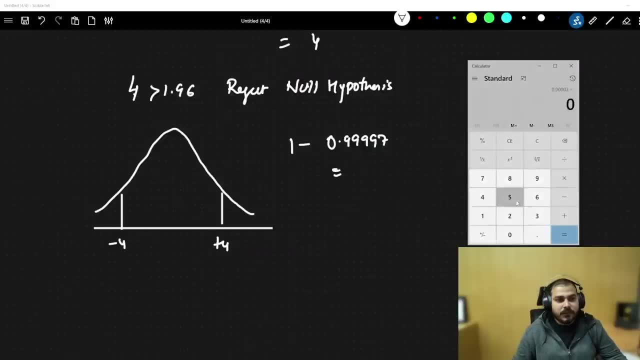 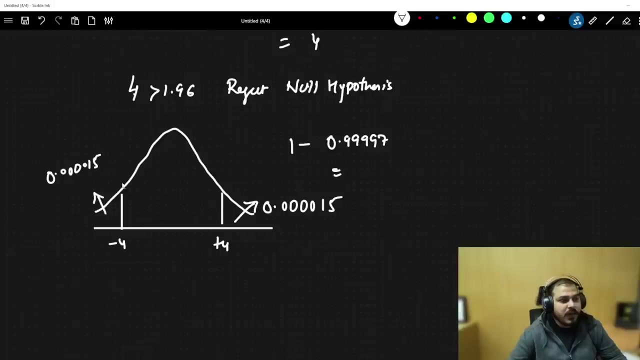 so i will go and subtract this to this. now, if i subtract this to this, what will happen? and i have to divide this by 2, since this is, since this is what two tail test- this side will basically be my area as 0.004015 and this will be my area as 0.4015, and this middle. 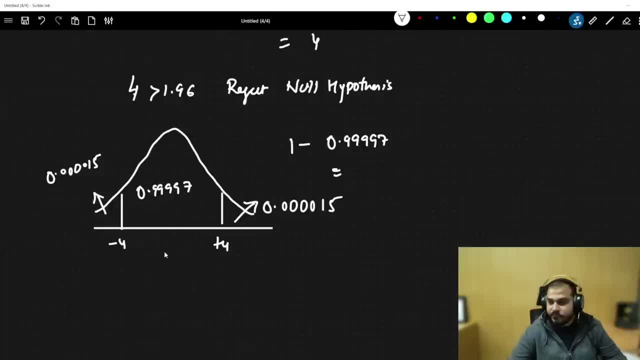 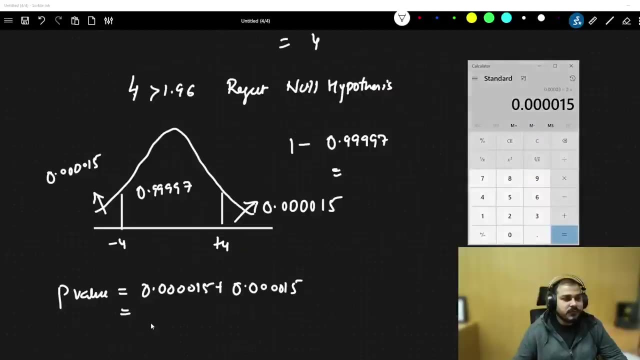 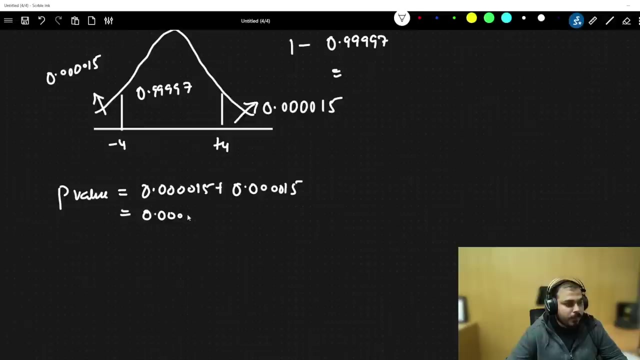 one will basically be 0.9997. now, what is my p-value? my p-value is 0.00015 plus 0.00015, so what this will be? this will be nothing but The same thing: 0.403,, 0.403,. now my p value is obviously very, very lesser than significance. 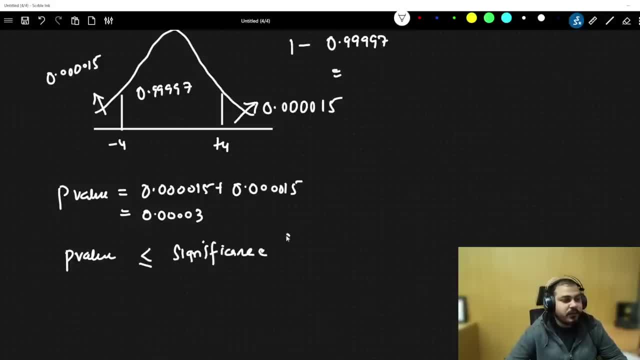 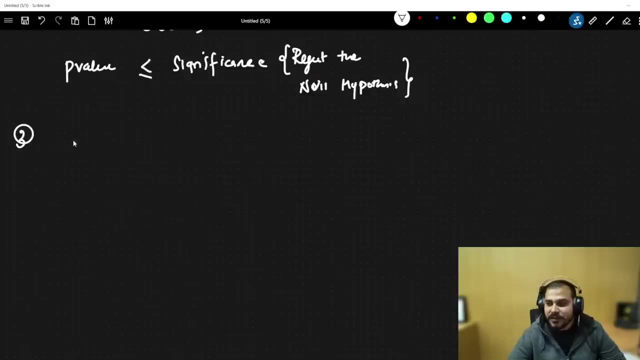 value. so what we have to do, we have to reject the null hypothesis. reject the null hypothesis. So here you can definitely say that with the sample size that we have taken, definitely we will not be able to conclude that the mean is that much. 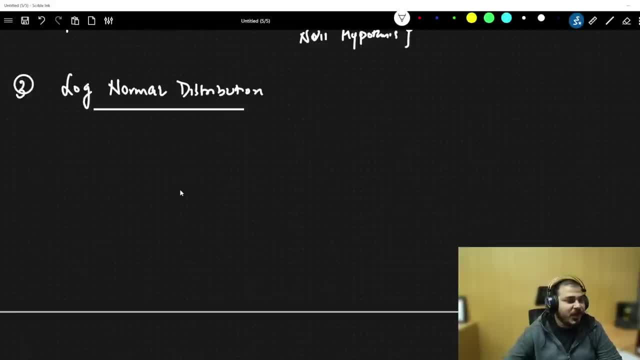 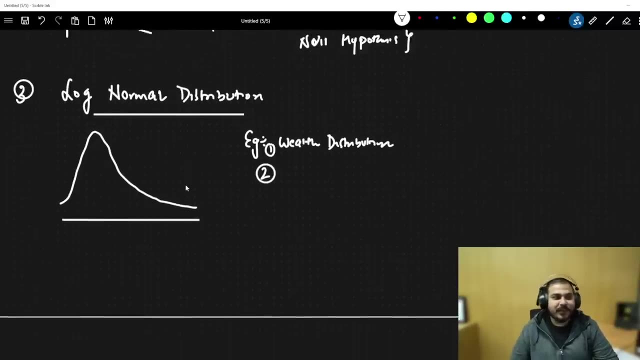 So let's go ahead with log normal distribution. okay guys, so log normal distribution. usually log normal distribution will have this kind of shape. obviously we have seen lot of examples like Welter distribution. these all things are actually there. so this was the example. 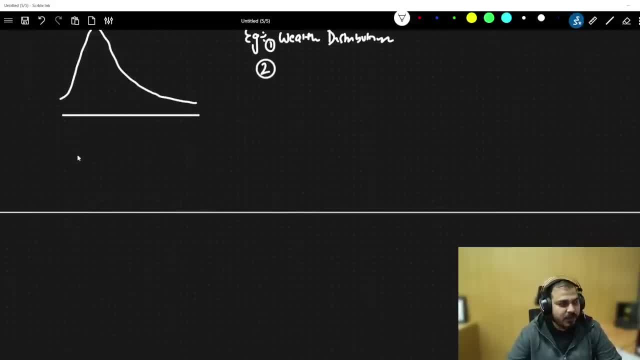 of log normal distribution. Now suppose I say that if y is a random variable that belongs to a log normal distribution, let's say that y is a random variable that belongs to a log normal distribution. let's say that with mean, as with some mean, let's say that this is there, it belongs to a log. 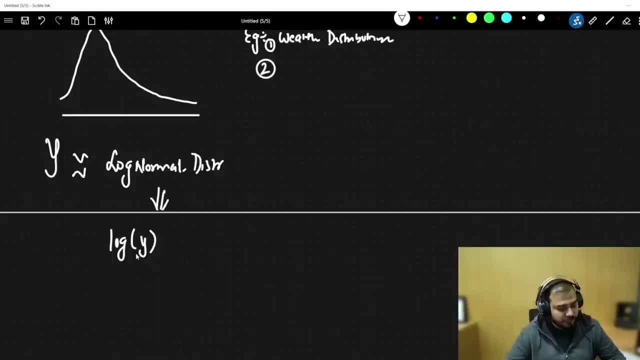 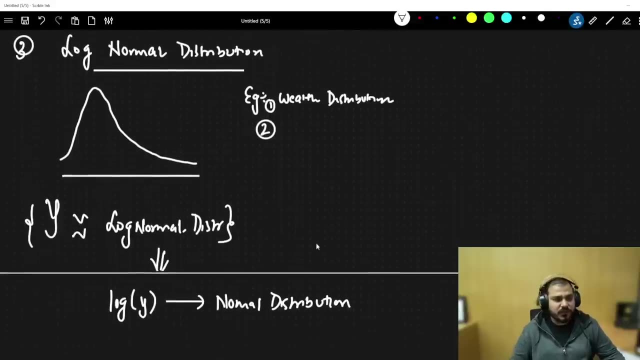 normal distribution then if I apply, if I apply log of y, then it should follow a normal distribution. So if it is satisfying this condition we can say a distribution is basically in this kind of log normal distribution. So log normal distribution I have already discussed in the previous session also lot. 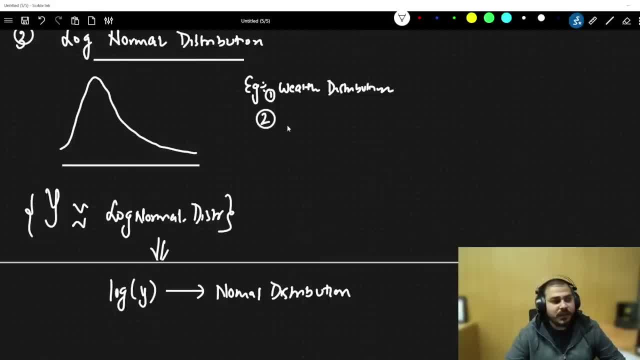 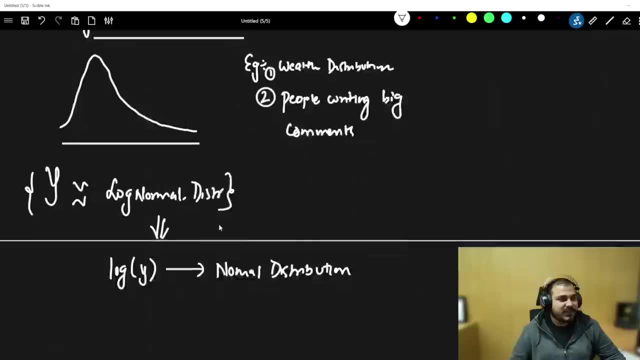 of examples: are there people writing comment session, people writing bigger comments, people writing? there will be very less number of people who write big comments, right, big comments. So this is one example and again, this is also. I have uploaded a detailed video in my stats. 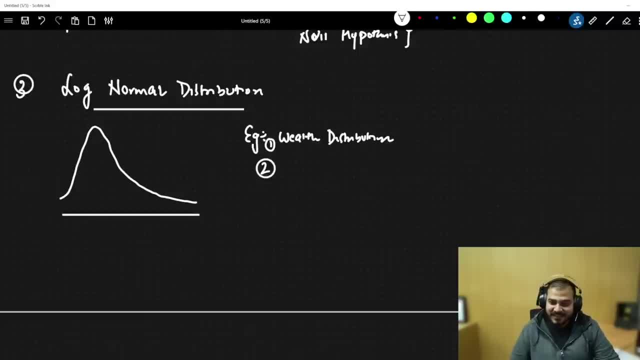 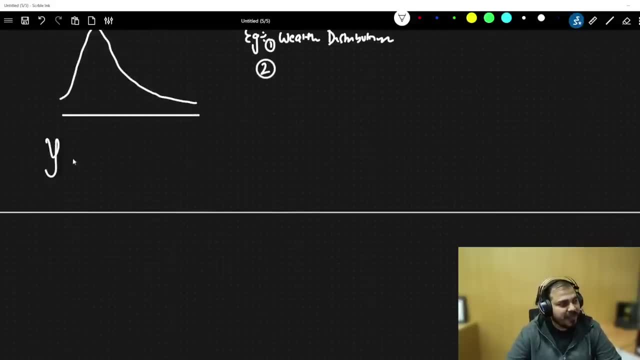 like wealth distribution. These all things are actually there. so this was the example of log normal distribution. Now suppose I say that if, if y is a random variable, that belongs to a log normal distribution, with mean, as with some mean, let's say that this is there, it belongs to a log normal distribution. 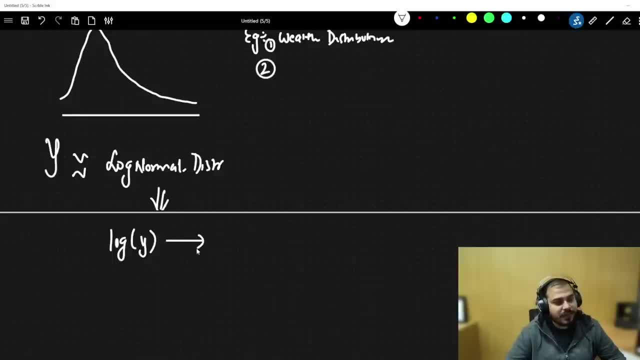 then if I apply, if I apply log of y, then it should follow a normal distribution. So if it is satisfying this condition we can say a distribution, So log normal distribution is basically in this kind of log normal distribution So log normal distribution. I have already discussed in the previous session also lot. 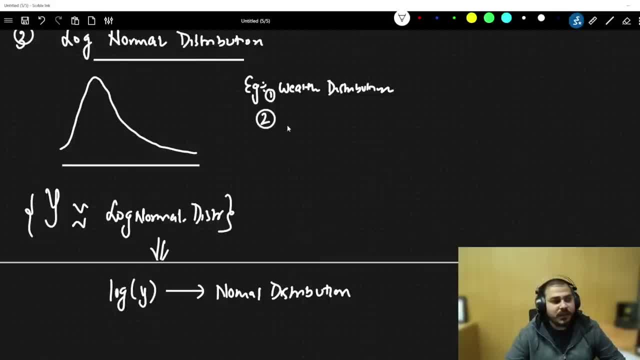 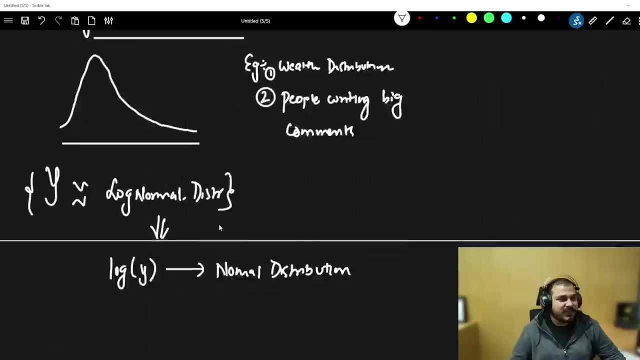 of examples. are there people writing comment session, people writing bigger comments, people writing there will be very less number of people who write big comments, right, big comments. so this is one example, and again, this is also. I have uploaded a detailed video in my stats playlist. Let's go to the next distribution. 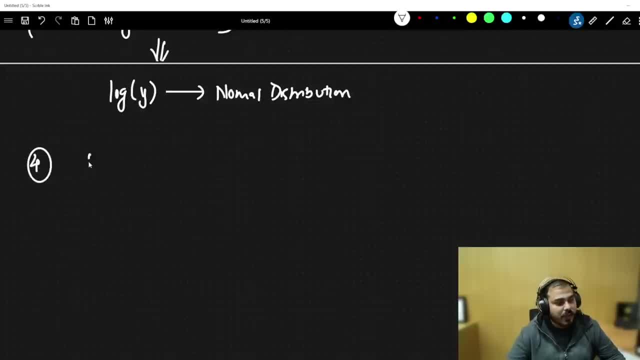 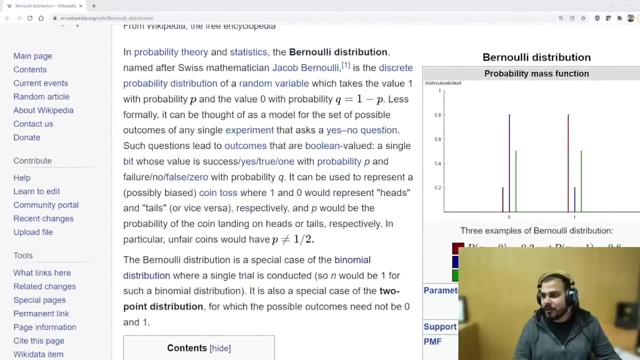 If I say that next distribution is 0.403.. So I will talk about Bernoulli's distribution. So let's talk about Bernoulli distribution. okay, let's start away and talk about Bernoulli distribution Now, in Bernoulli distribution you can see that it's more about p and q. it's more about 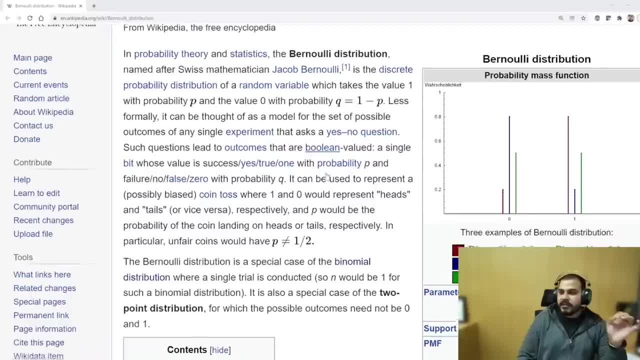 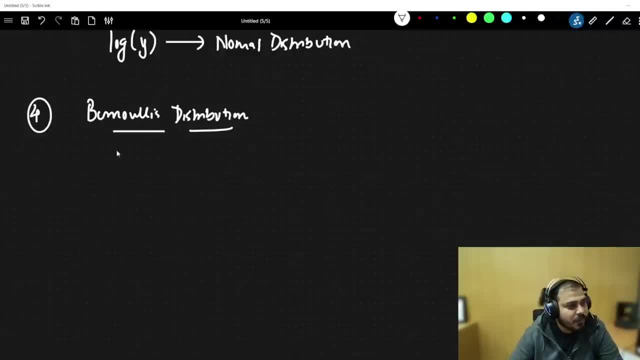 see, whenever you have a Bernoulli distribution, that basically means you need to understand there are only two outcomes. So if I go and probably open it over here, In Bernoulli distribution They are specifically two outcomes. two outcomes basically means that it can be either zero. 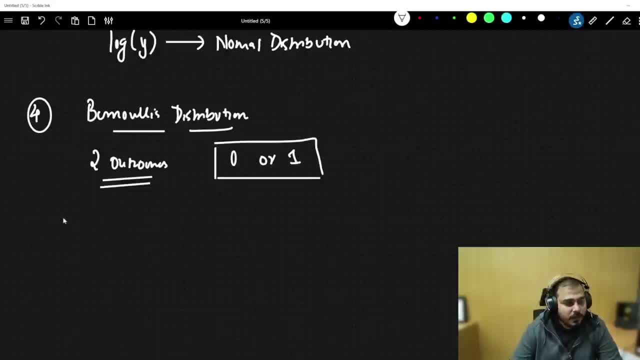 or one, let's say that I have two outcomes of zero. but I really need to find out the probability. you know when? when we need to focus on probability with respect to Bernoulli distribution, we define by two values: one is p and one is q. 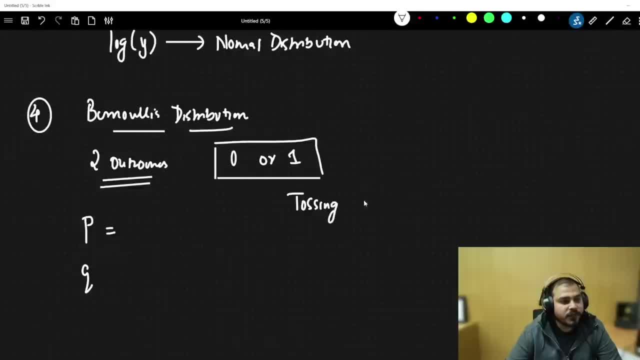 Suppose I say I'm considering an experiment which is called as tossing a coin. in tossing a coin, What is the probability of head? let's say that I'm getting probability of head as 0.5.. So this will basically become my p value. okay, when I talk about the p value, q value, it will 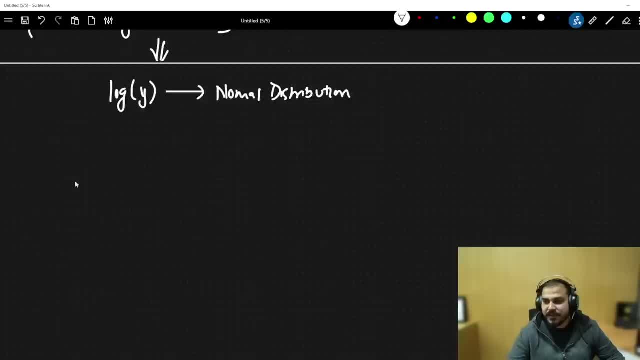 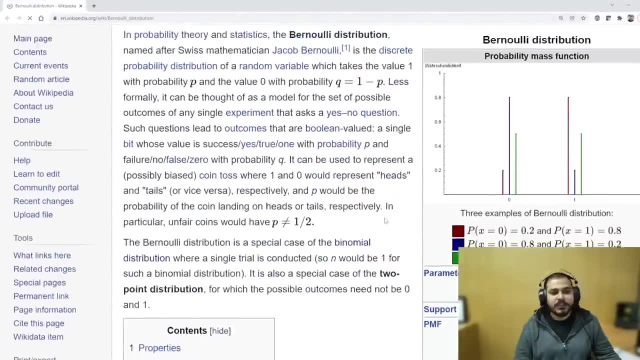 playlist. let's go to the next distribution. if I say that next distribution is there, so I will talk about Bernoulli's distribution, So let's talk about Bernoulli distribution. okay, let's start away and talk about Bernoulli. 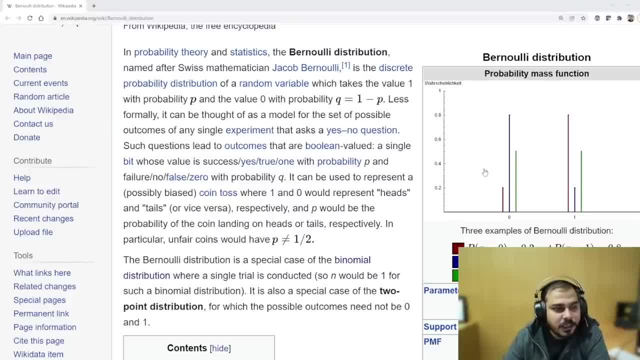 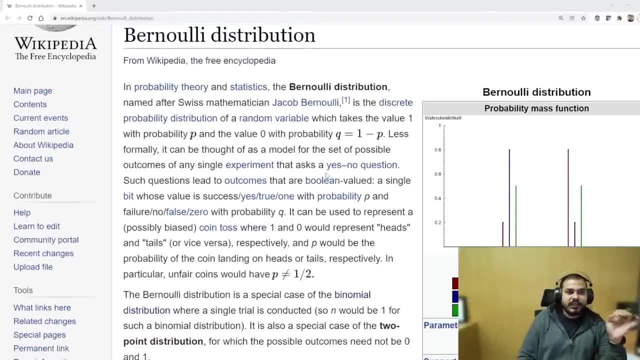 distribution 9.. In Bernoulli distribution you can see that it's more about p and q, it's more about c. Whenever you have a Bernoulli distribution, that basically means you need to understand there are only two outcomes. 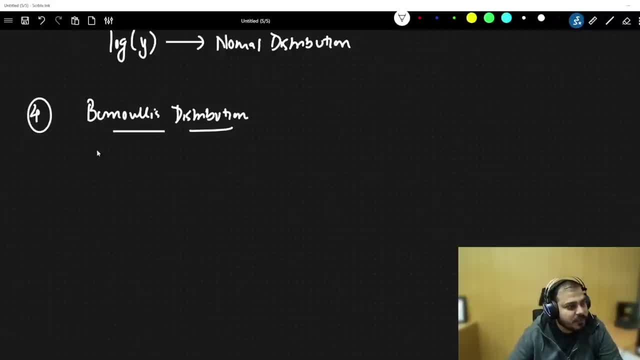 So, if I go and probably open it over here, in Bernoulli distribution there are specifically two outcomes. Two outcomes basically means that it can be either 0 or 1.. Let's say that I have two outcomes of 0 or 1, but I really need to find out the probability. 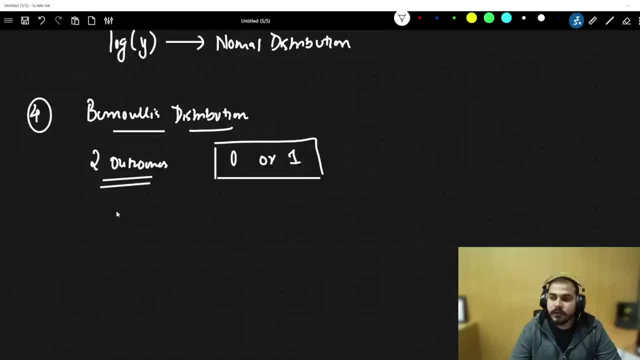 you know When we need to focus on probability with respect to Bernoulli distribution, we define by two values, one is p and one is q. Suppose I say I am considering an experiment which is called as tossing a coin. In tossing a coin I know what is the probability of head. let's say that I am getting probability. 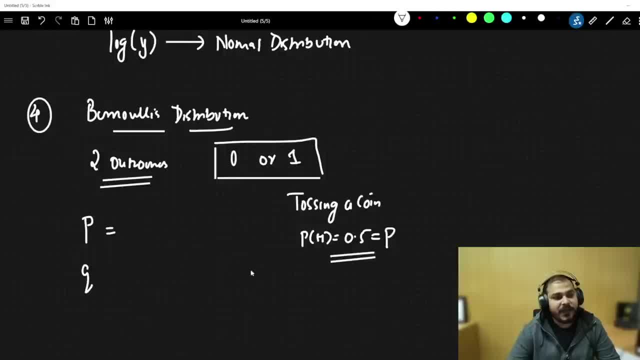 of head as 0.5.. So this will basically become my p value. okay, When I talk about the p value, q value, it will become 1 minus p. okay, that basically means it's the probability of head, because when we are probably tossing a coin there, 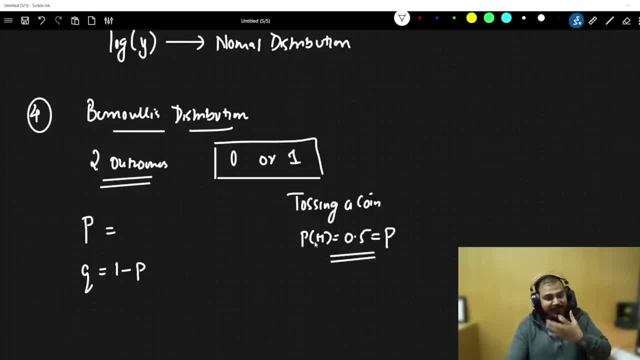 are two choices: either you get head or either you get p. So when I say probability of head is 0.5, so this is what one outcome probability is there? What about the other outcome? So that is nothing but 1 minus p. 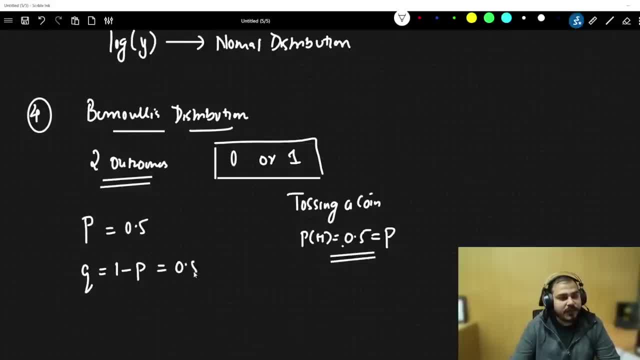 So here, if I have 0.5,, then q will be 1.5,, then this will be 0.5.. Suppose I do not have a fair coin. I do not have a fair coin, do not have a fair coin. 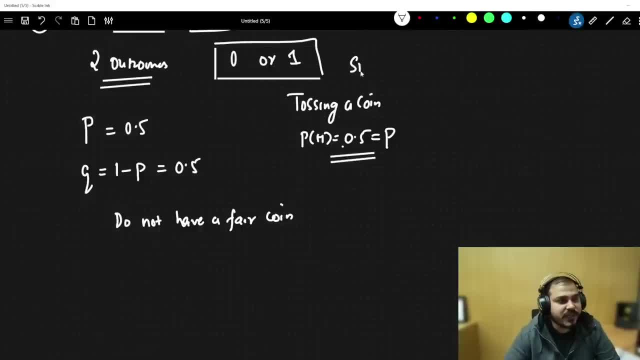 Now, in this particular case- And this is the only relationship- Okay, This is related to single trial, not multiple trials, single trial distribution. Now, let's say that I do not have a fair coin. Let's say that my probability of head is 0.3.. 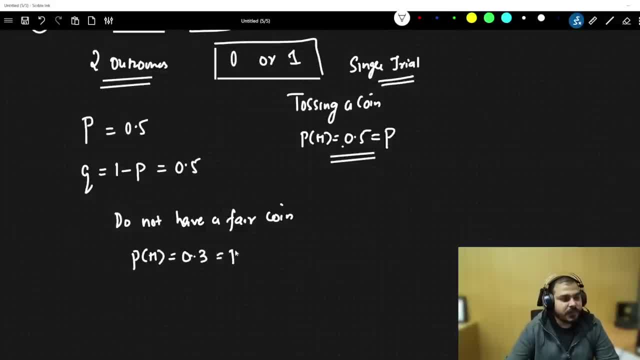 Now, in this particular case, what will be my probability of tail? This is basically p. then my probability of tail will obviously be q, which is nothing but 1 minus p, which is nothing but 1 minus 0.3, 0.7.. 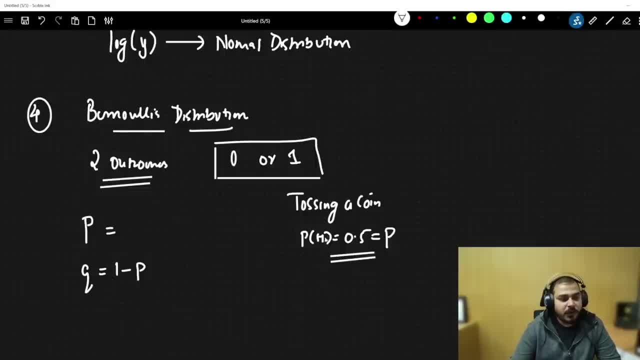 be 1 minus p. okay, that basically means it's the probability of head, because when we are probably tossing a coin, there are two choices: either you get head or either you get tail. So when I say probability of head is 0.5, so this is what one outcome probability is there. 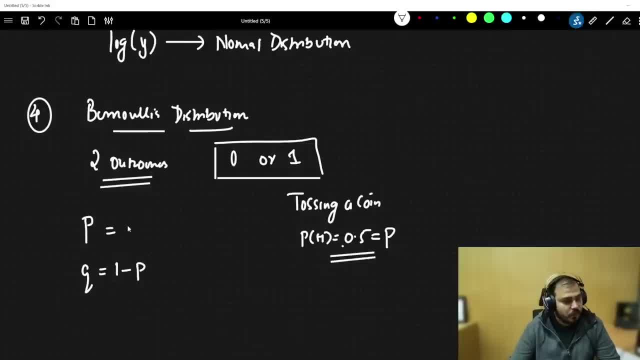 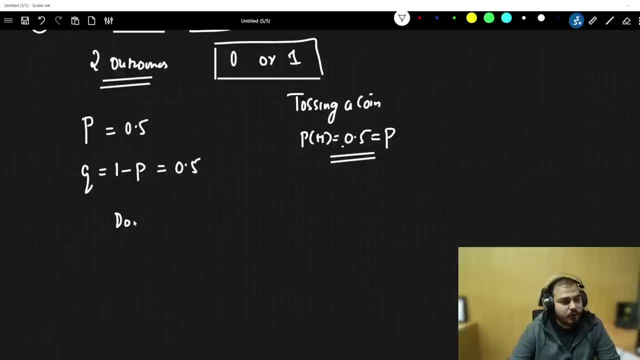 What about the other outcome? so that is nothing but 1 minus p. So here, if I have 0.5, then q will be 1.5, then this will be 0.5.. Suppose I do not have a fair coin. I do not have a fair coin. do not have a fair coin now. 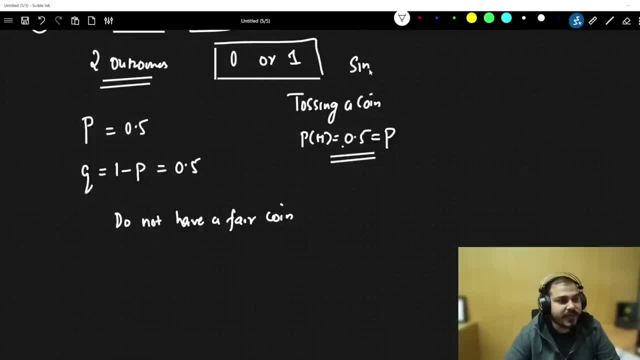 in this particular case- and this is only related to single trial, not multiple trials- single trial distribution. Now, let's say I do not have a fair coin. let's say that my probability of head is 0.3. now, in this particular case, what will be my probability of tail? this is basically p. then my probability. 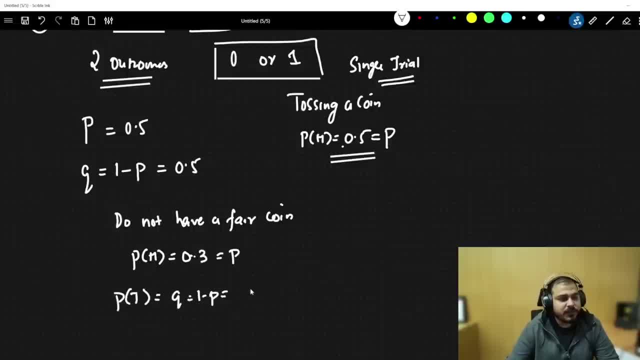 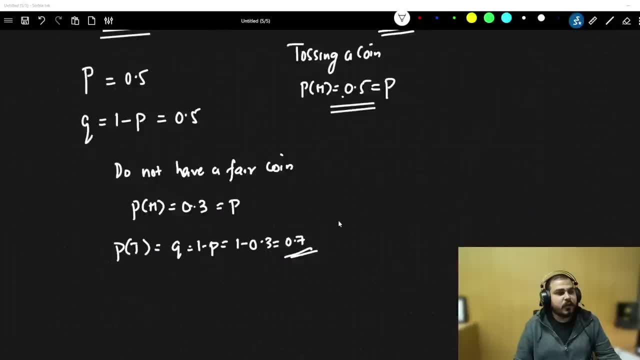 of tail will obviously be q, Which is nothing but 1 minus p, which is nothing but 1 minus 0.7.. So this is basically 0.7 over here. you can see over here Now. similarly, if I go and probably discuss with respect to this here, you can see that. 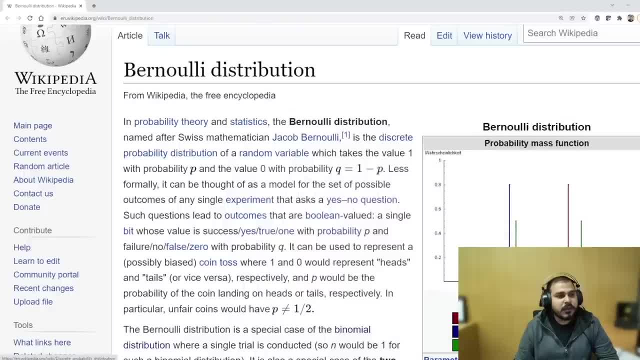 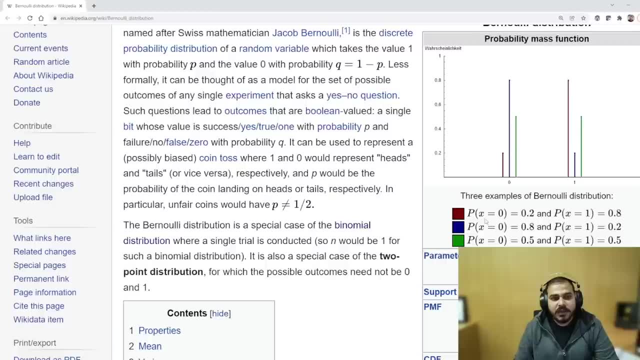 a Bernoulli distribution named after Swiss mathematician, Jacobi Bernoulli, as a discrete probability distribution. Now here you see this. okay, three examples of Bernoulli distribution. here the probability of x is equal to 0 with one of. the outcome is 0.2. 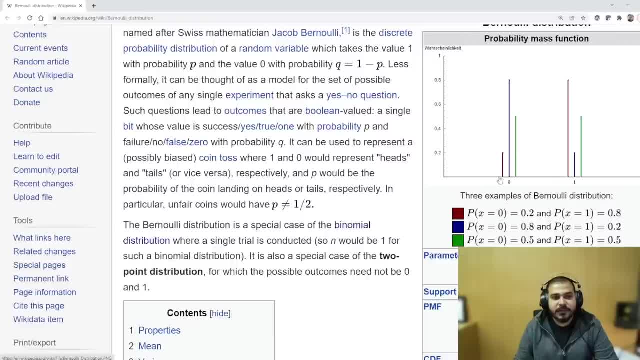 So we are drawing this graph, this line. See, This will come as 0.2, this will come as 0.8.. Over here, next outcome you can see over here, is 0.8 and 0.2.. So this is how you basically create: in this 0.8 and this is 0.2.. 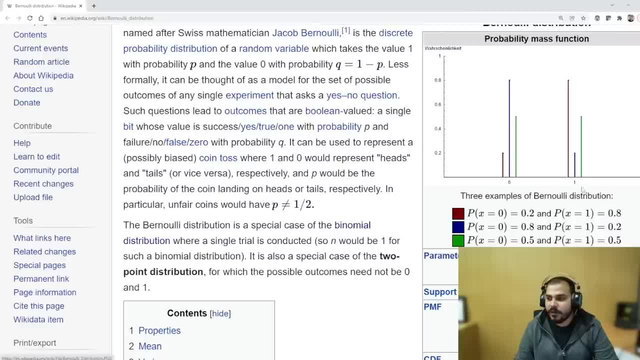 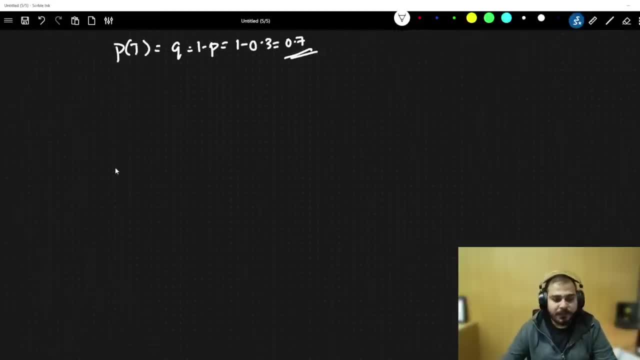 In the green color you can see 0.5 and 0.5. so this is my 0.5 and 0.5.. Now understand one important thing: whenever we draw this kind of like, this kind of experiment, if we draw in the form of graphs on the left hand side, obviously you know what will be. 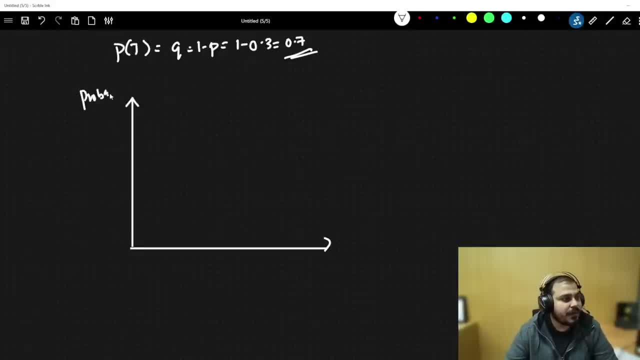 there. with respect to this and the right hand side, there will be probability. So this is basically 0.2, 0.4, 0.6, 0.8 and 1.. Now, suppose let's consider that I have three. I have one coin over here. 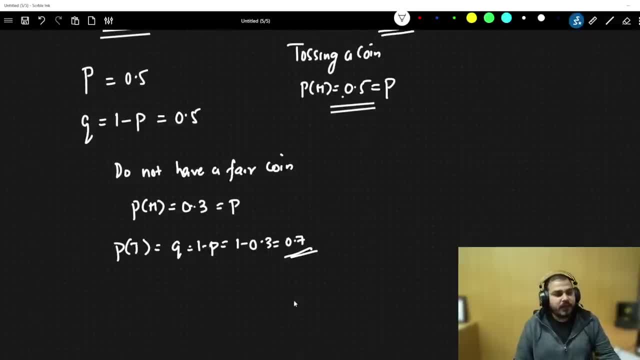 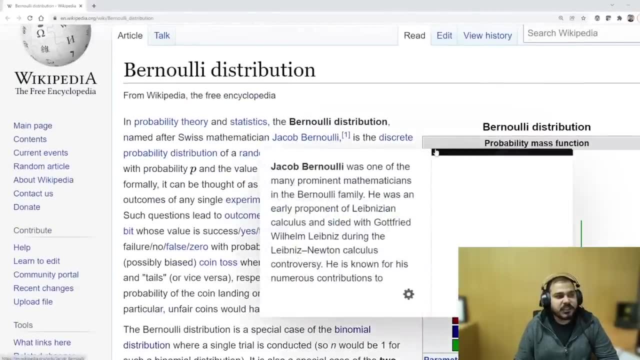 So this is basically 0.7 over here. you can see over here Now. similarly, if I go and probably discuss with respect to this here, you can see that a Bernoulli distribution named after Swiss mathematician, Jacobi Bernoulli Bernoulli has. 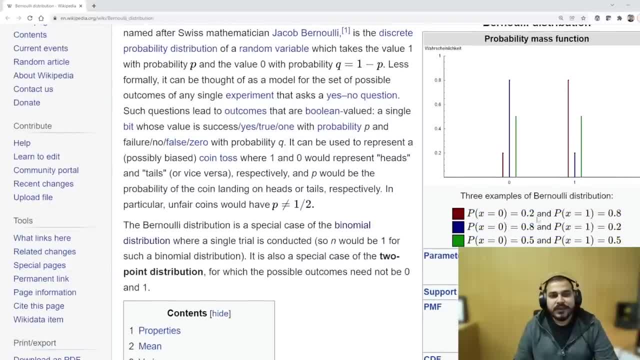 a discrete probability distribution. Now here you see this. Okay, Three examples of Bernoulli distribution. Here, the probability of x is equal to 0, with one of the outcome is 0.2.. So we are drawing this graph, This line. 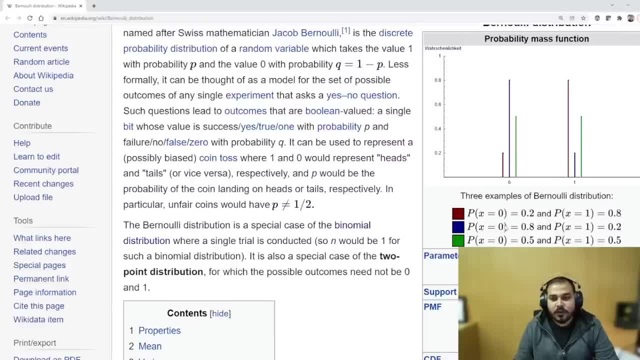 See, this will come as 0.2, this will come as 0.8.. Over here, next outcome you can see over here, is 0.8 and 0.2.. So this is how you basically create: in this 0.8 and this is 0.2.. 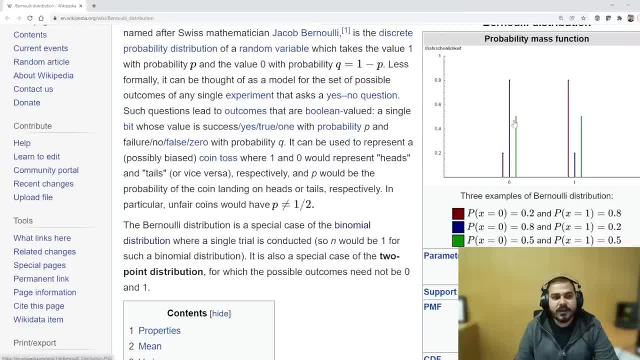 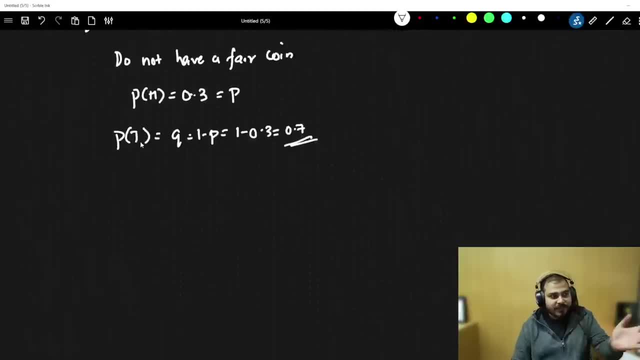 In the green color, you can see, You can see 0.5 and 0.5.. So this is my 0.5 and 0.5.. Now understand one important thing: Whenever we draw this kind of like, this kind of experiment, if we draw in the form of graphs, 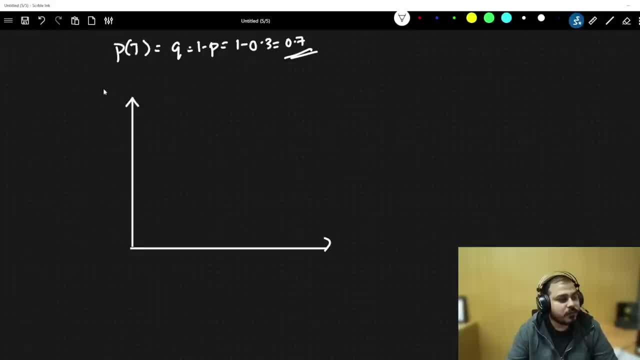 On the left hand side. obviously, you know what will be there with respect to this and the right hand side, there will be probability. So this is basically 0.2, 0.4,, 0.6, 0.8 and 1.. 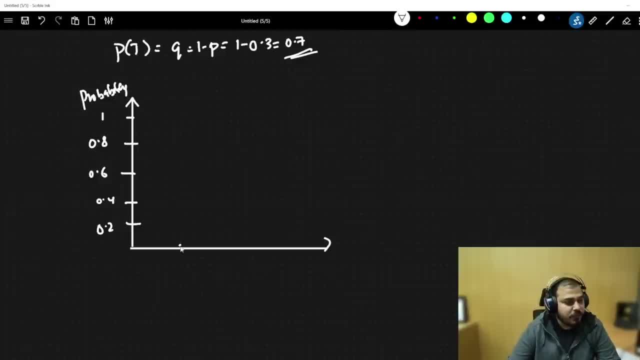 Now suppose let's consider that I have three. I have one coin over here. this one coin is: this one coin is basically head, this is basically tail. Now, if I try to show you with respect to the probability of head and tail, I can basically: 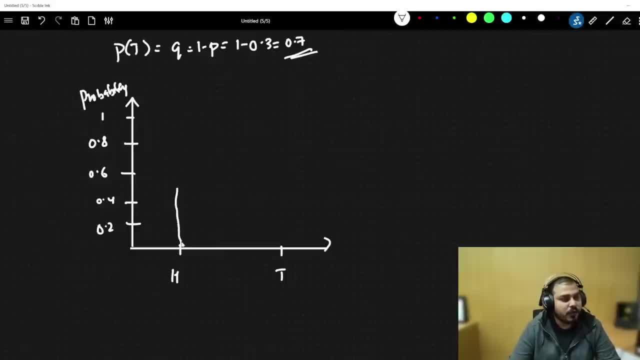 draw. Suppose if I say this probability of head is 0.5, so I can draw this line like this, I can basically draw this line with respect to this and this. Then if I am drawing this line, then probability of tail will also be 0.5.. 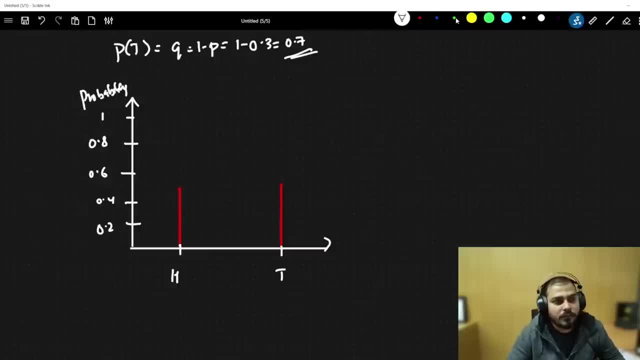 Suppose if I say the probability of head of not a fair coin is nothing but 0.8. Then we will draw a line like this Here. So we say then what will happen? if this is 0.8, then this will become 0.2.. 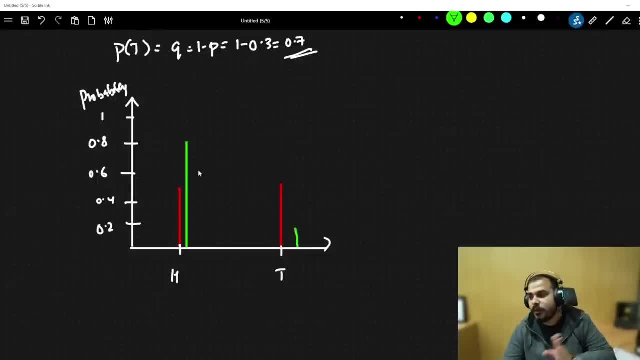 So this is how we basically draw this, and this is not a probability density function. Understand: this is a probability mass function. In probability density function it is completely different. Probability density function is for continuous variable. This is specifically for categorical variables. So this probability mass function that we have over here, we will basically say it as: 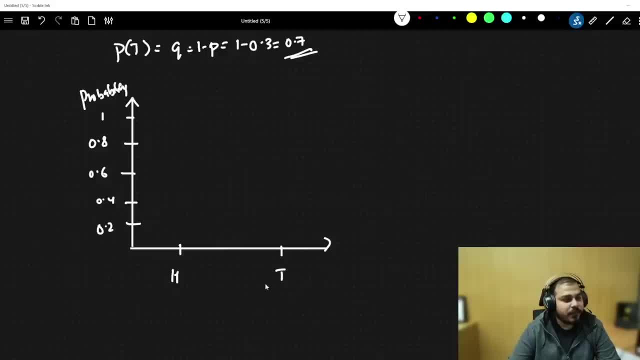 This one coin is basically head, This is basically tail. Now, if I try to show you with respect to the probability of head and tail, I can basically draw. suppose, if I say this probability of head is 0.5, so I can draw this line like: 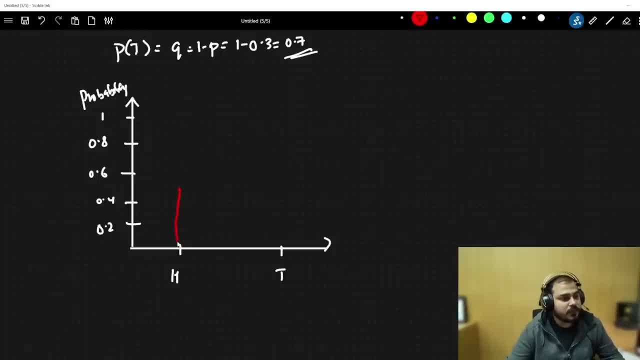 this: I can basically draw this line with respect to this and then if I'm drawing the, the red line, same thing- and then rounded it by missing this line, this line, then probability of tail will also be 0.5.. Suppose, if I say the probability of head of 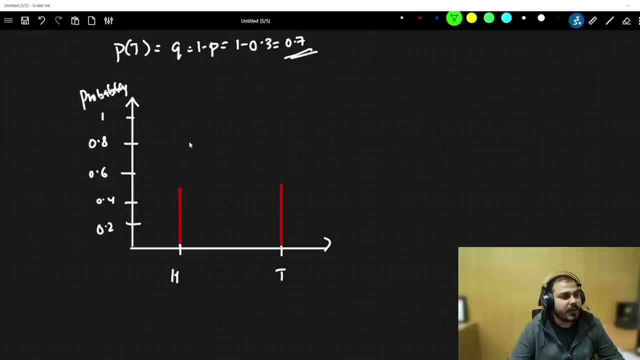 not. a fair coin is nothing but 0.8, then we will draw a line like this Here. I can basically say: then what will happen? if this is 0.8, then this will become 0.2.. So this is how we basically draw. 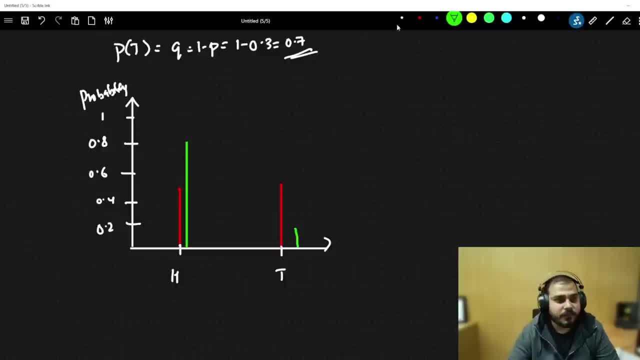 this and this is not a probability density function. Understand: this is a probability mass function, A probability density function. it is completely different. Probability density function is for continuous variable. This is specifically for categorical variables. So this probability mass function that we have over here, we will basically say it as PMF. before we used to. 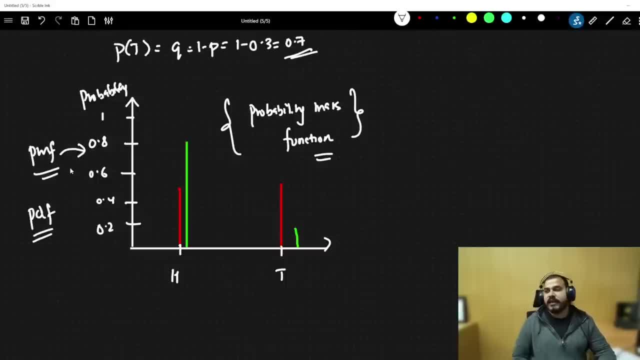 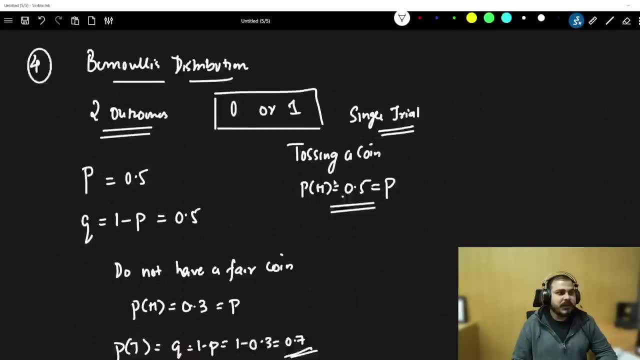 say it as PDF. So whenever we have this kind of variables, categorical variables, at that point of time this is basically called as probability mass function. So I hope everybody is able to understand with respect to this. Now let's go to the Wikipedia page. So here you can see probability. 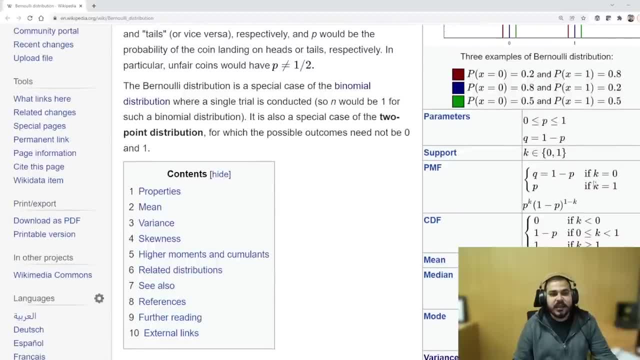 mass function and the same thing. probability. mass function is saying: If k is equal to 0.5, I will write: q is equal to 1 minus p. if k is equal to 1, and the PMF is basically defined in this particular manner. Any probability that I want to form, I want to find out. this is how the formula. 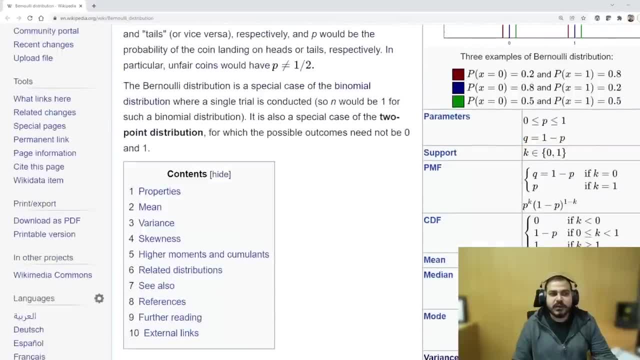 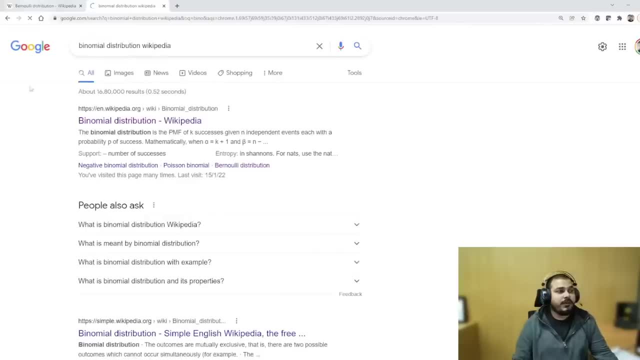 is basically utilized. We really need to know only this much things about the distribution and one probability formula. This was with respect to Bernoulli distribution. Now let's go ahead and try to discuss about binomial distribution. See. binomial distribution is also very much good. 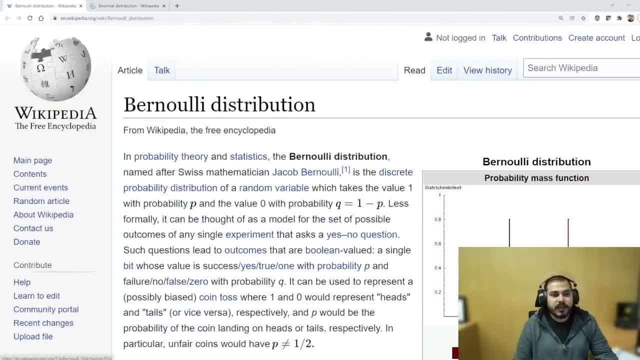 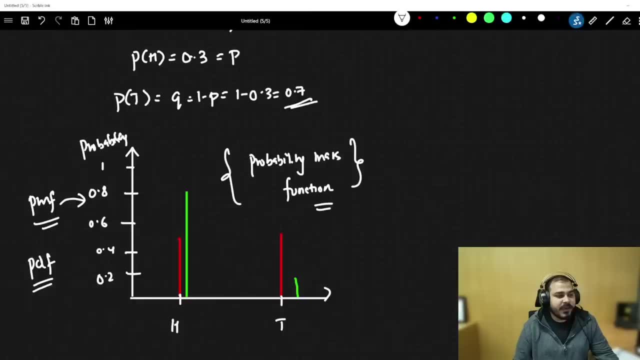 Till now we discussed about single trial right. Single trial: whenever we take up multiple trial, then it becomes a binomial distribution Inside this. let me write it down over here. So if I go and see with respect to binomial distribution, Binomial distribution. 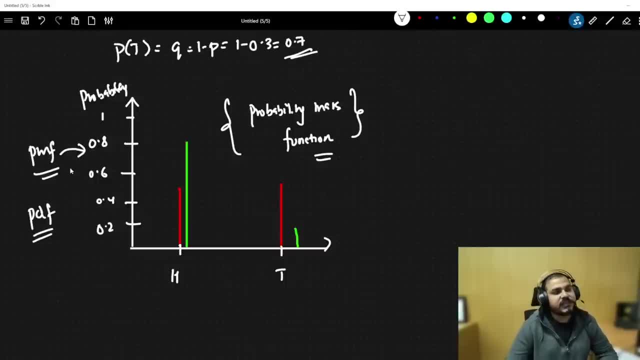 PMF. Before we used to say it as PDF. So whenever we have this, This kind of variables, categorical variables, at that point of time This is basically called as probability mass function. So I hope everybody is able to understand with respect to this. 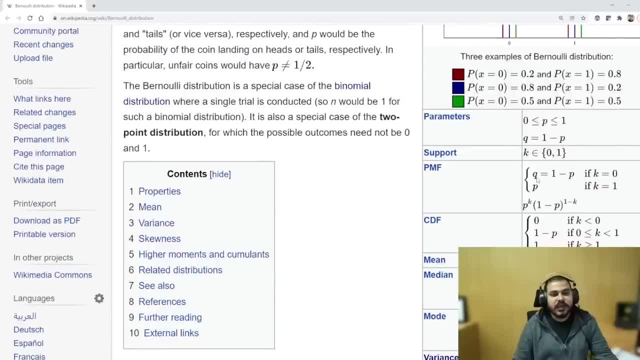 Now let's go to the Wikipedia page. So here you can see probability mass function. And the same thing probability mass function is saying: If K is equal to 0, I will write: Q is equal to 1 minus P, P, if K is equal to 1.. 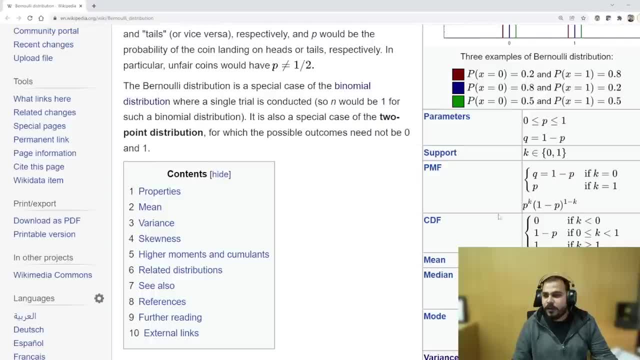 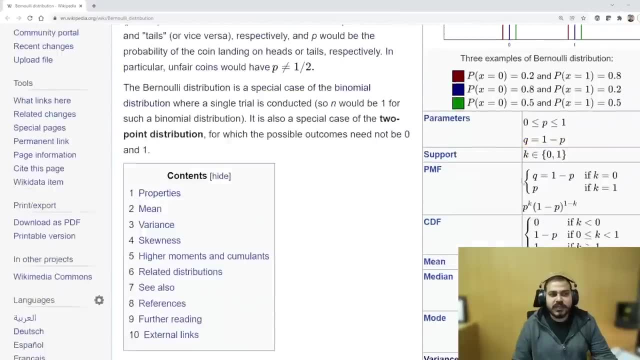 And the PMF is basically defined in this particular manner. Any probability that I want to form, I want to find out. this is how the formula is basically utilized Before we start the discussion. we already know that we need to know only this much things. 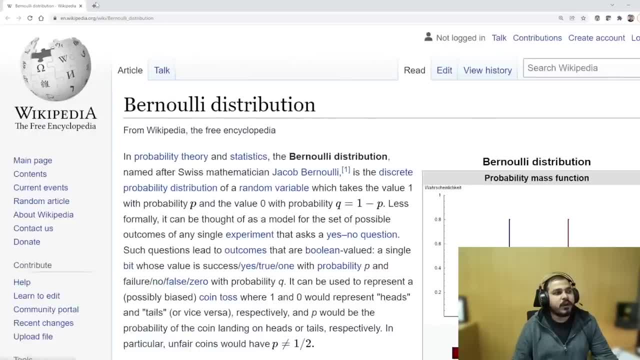 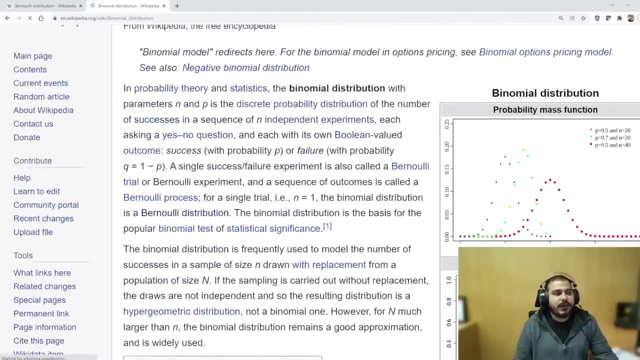 about the distribution and one probability formula. This was with respect to Bernoulli distribution. Now let's go ahead and try to discuss about binomial distribution, See binomial distribution is also very much good. Till now, we discussed about single trial, Right? 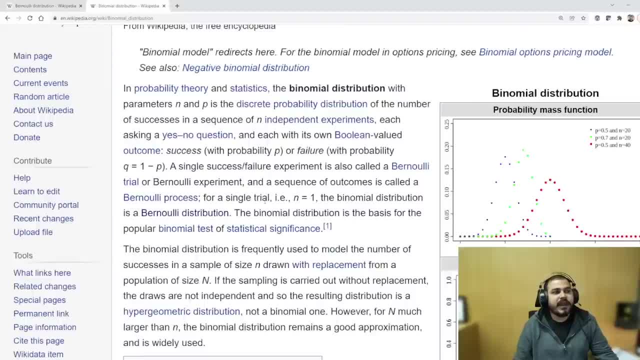 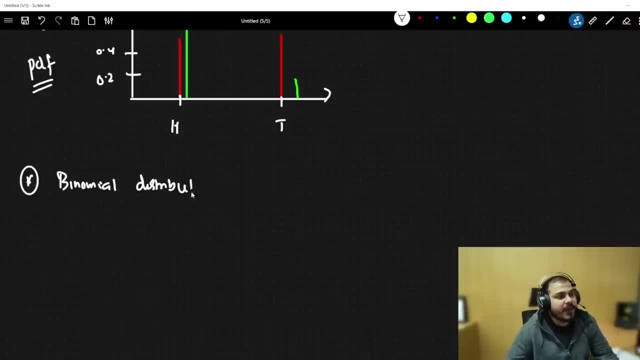 Single trial. whenever we take a multiple trial, then it becomes a binomial distribution Inside this. let me write it down over here. So if I go and see with respect to binomial distribution, binomial distribution says that obviously with respect to every trial. 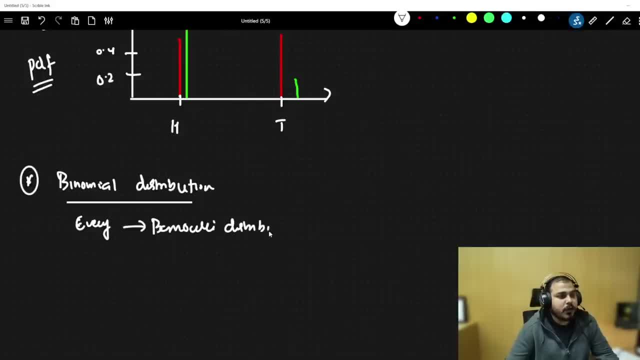 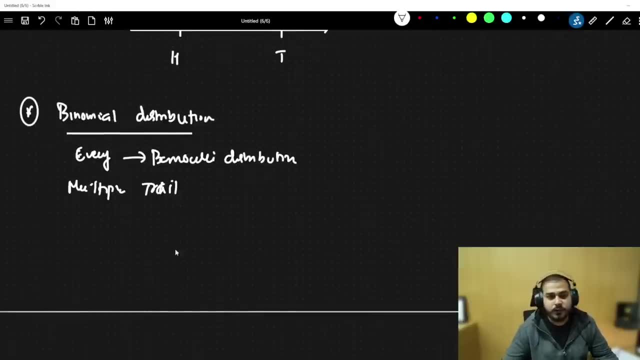 This is the distribution. There will be a Bernoulli distribution, Bernoulli distribution, but here we have multiple trials. That basically means we have the combination of many Bernoulli's distribution over here. Suppose in this trial my probability of head is this much: 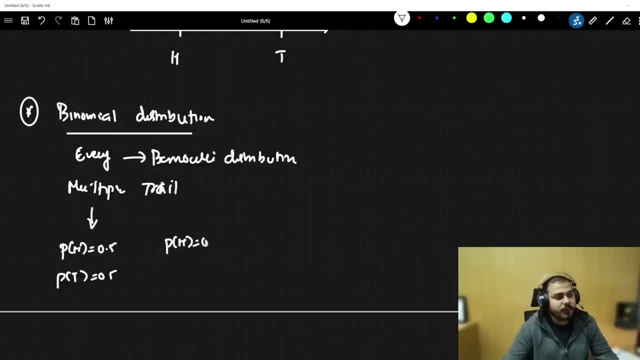 Suppose, in one more trial I will go and write: probability of head is 0.6,, this is 0.4.. Like this, I will be having many trials combined together in one kind of binomial distribution Whenever you have a categorical variable and whenever we try to draw this kind of diagram. 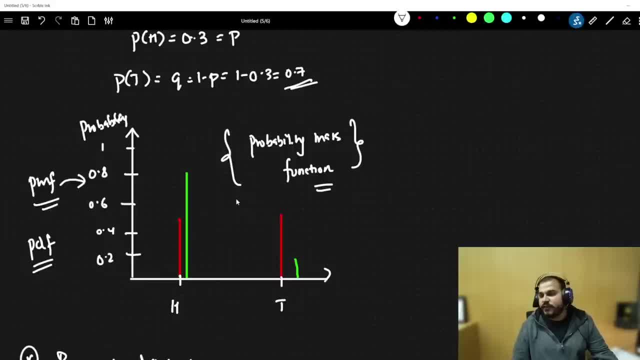 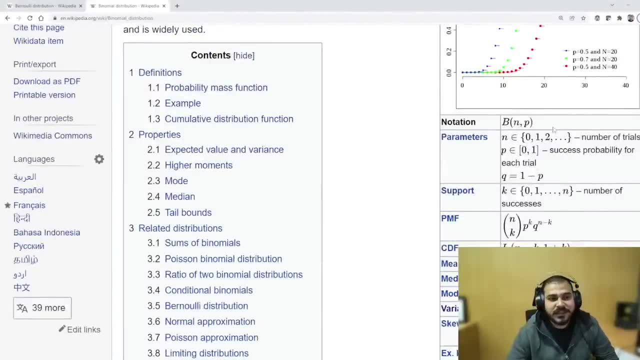 then it is called as a probability mass function. In the case of a continuous variable we have probability density function. So, if I go and probably see this, the binomial distribution is given by two notations: n, p. So n is nothing but number of trials, p is nothing but success or probability for each trial. 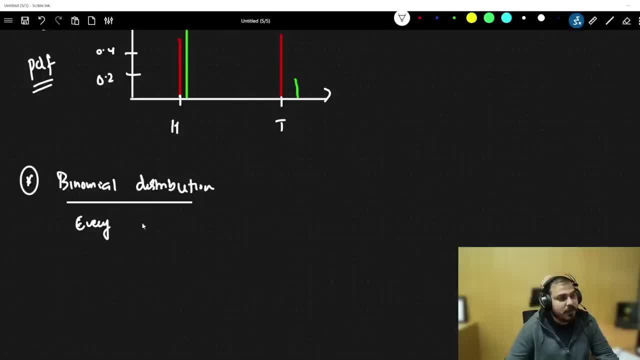 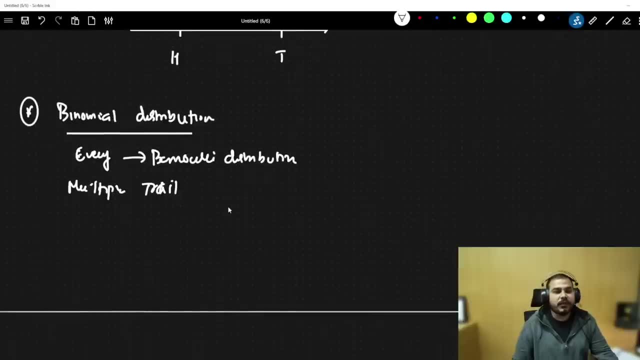 says that obviously, with respect to every trial there will be a Bernoulli distribution, Bernoulli distribution, but here we have multiple trial. That basically means we have the combination of many Bernoulli's distribution over here. Suppose in this trial my probability of head. 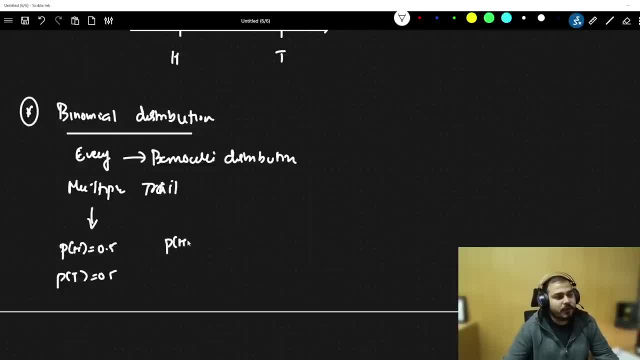 is this much? Suppose in one more trial, I will go and write: probability of head is 0.6, there is 0.4.. Like this, I will be having many trials combined together in one kind of binomial distribution, Whenever you have categorical variable and whenever. 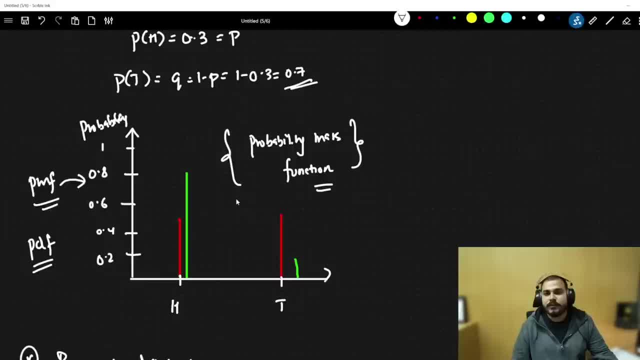 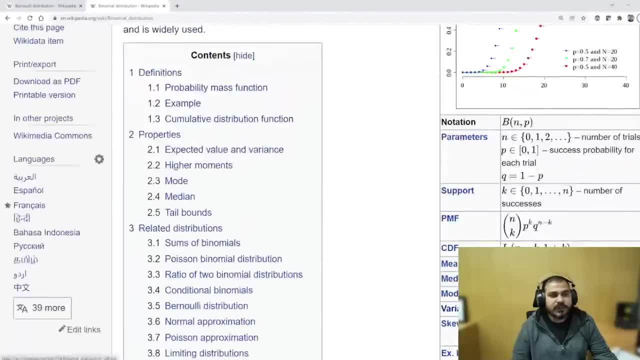 we try to draw this kind of diagram. it's called as probability mass function. In the case of drains we have probability density function. So if I go and probably see this, the binomial distribution is given by two notation: n, p. So n is nothing but number of trials, p is nothing but success of probability. for 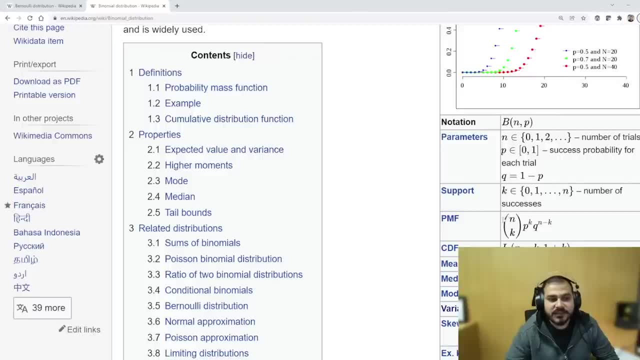 each try, where q is equal to 1 minus e, okay, and this is the formula with respect to the probability mass function, to calculate the probability of a binomial distribution. Now, this is done. now let's go to one very important distribution, which is called as Pareto distribution. Now, Pareto distribution. 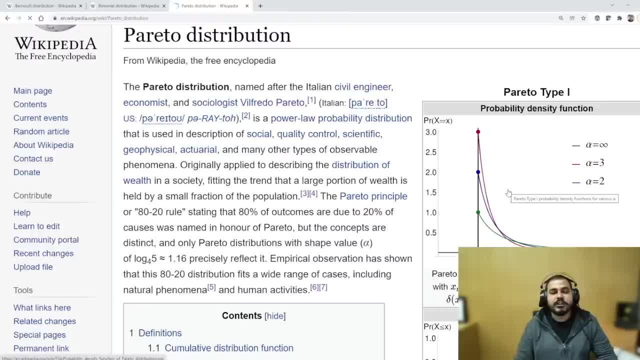 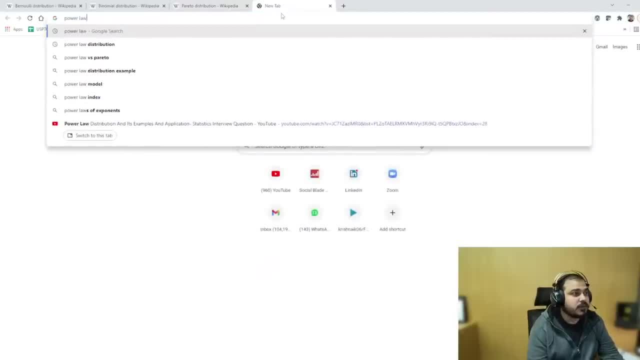 is a non-Gaussian, it is not a Gaussian distribution. it looks something like this: one application of Pareto distribution is nothing but power law distribution. so if I show you power law, so here everybody see this diagram with respect to this. I am just going to take a snippet of it. 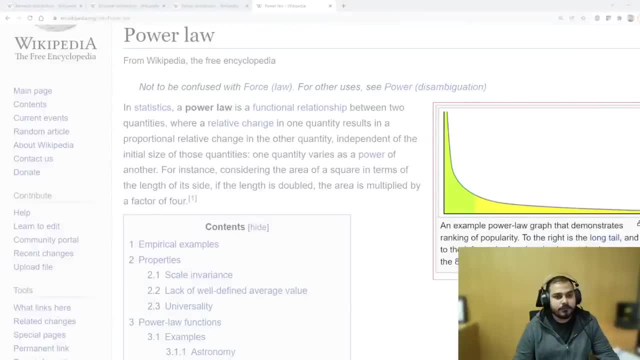 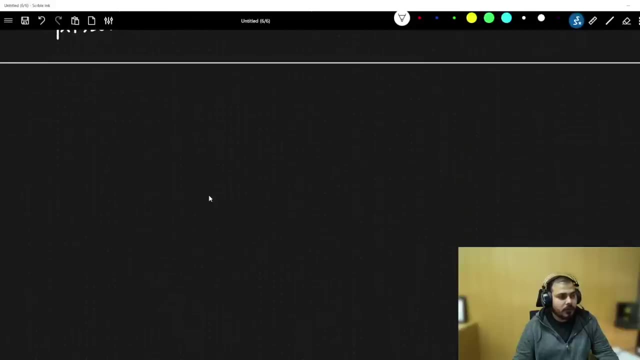 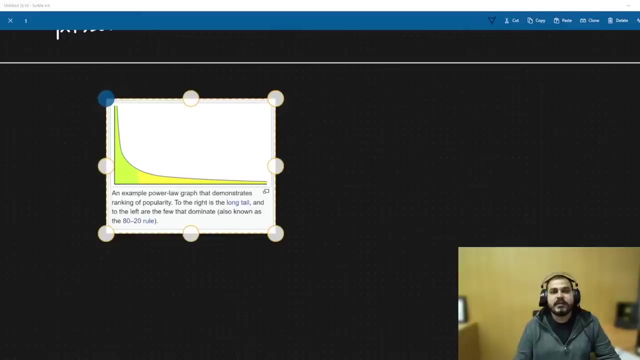 we'll discuss about this. this is something very much important. okay, let's let's paste it over here now. in this particular case, when we are discussing about power law distribution, let's see that what important information we can take out from this. power law distribution basically says that you 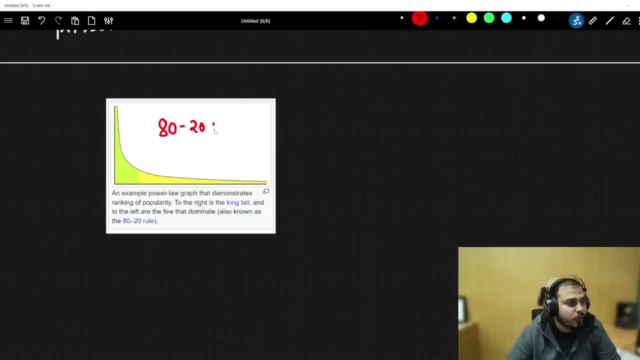 have to remember this. power law distribution is a non-Gaussian distribution. Now, in this particular case, let's take a look at this rule, which is called as 80-20 rule. you can see that this is probably my 80 percentage of this entire value and this is my 20 percentage of the entire value. my x-axis may be: 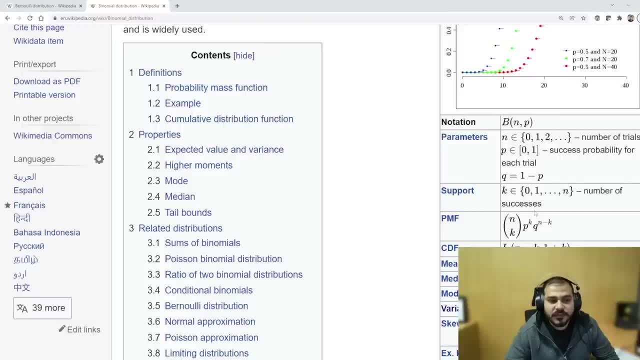 where q is equal to 1 minus p, And this is the formula, with respect to the probability mass function, to calculate the probability of a binomial distribution. Now, this is done. Now let's go to one very important distribution, Which is called as Pareto distribution. 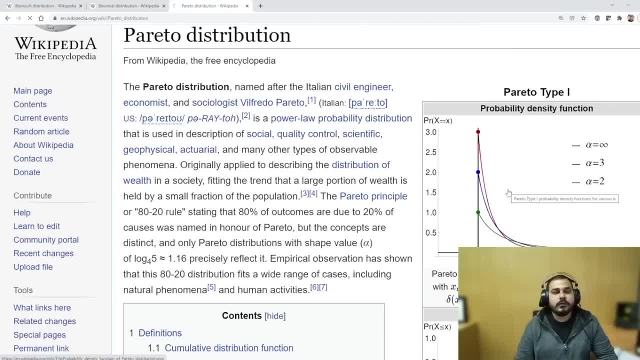 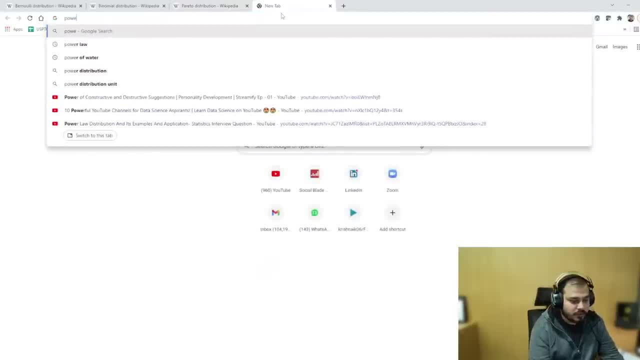 Now, Pareto distribution is a non-Gaussian. it is not a Gaussian distribution. It looks something like this: One application of Pareto distribution is nothing but power law distribution. So if I show you power law, So here everybody see this diagram with respect to this. 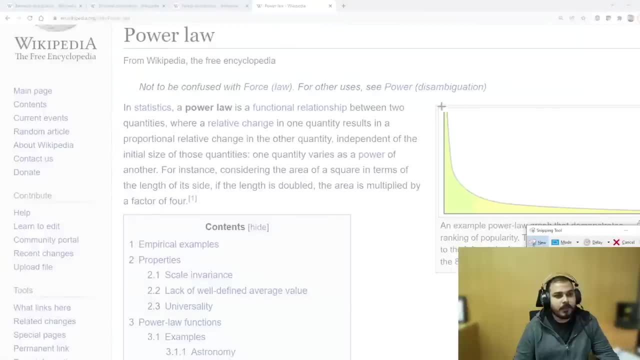 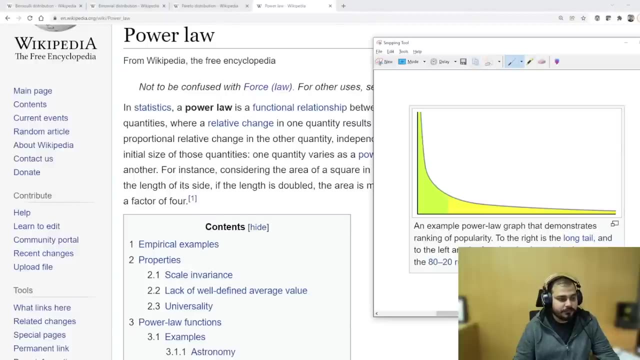 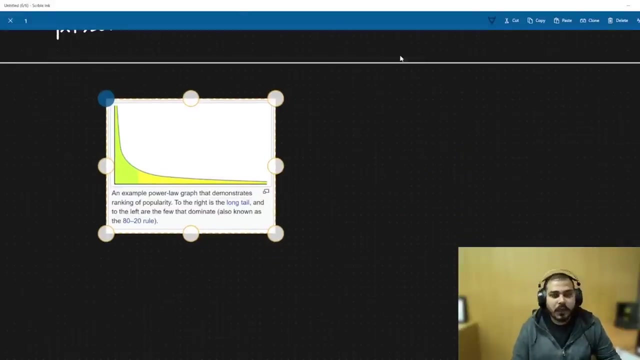 I am just going to take a snippet of it. We will discuss about this. This is something very much important. Okay, Let's paste it over here. Now, in this particular case, when we are discussing about power law distribution, let's see that what important information we can take out from this. 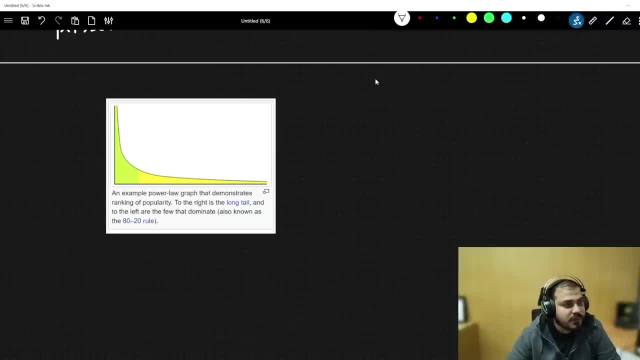 Power law distribution basically says that you have to remember this rule, which is called as 80-20 rule. You can see that this is probably my 80% of this entire value and this is my 20% of the entire value. 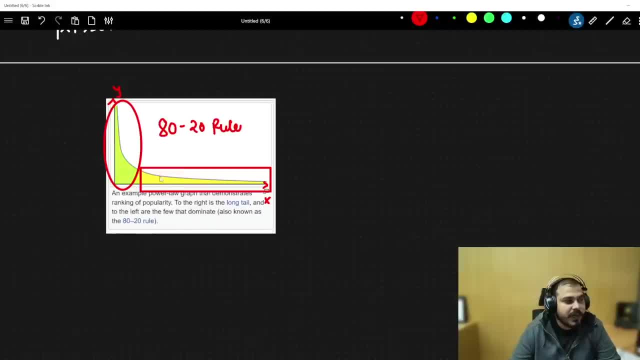 My x-axis may be something, my y-axis may be something, But understand, the 80 of one kind of distribution will be falling here and the remaining 20 will be falling here. Let's take some examples. Okay, Now suppose if I say that 80% of the wealth is distributed with 20% of the people? 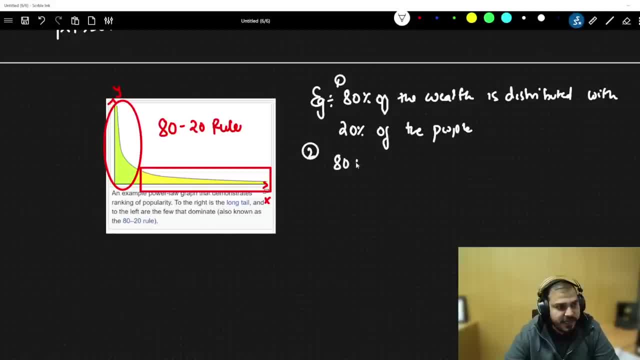 The second question: Any example, any other example? Can I say: 80% of the company projects are done by 20% of the people, 20% of people in a team, 80% of sales Is done by 20% of the most famous project. 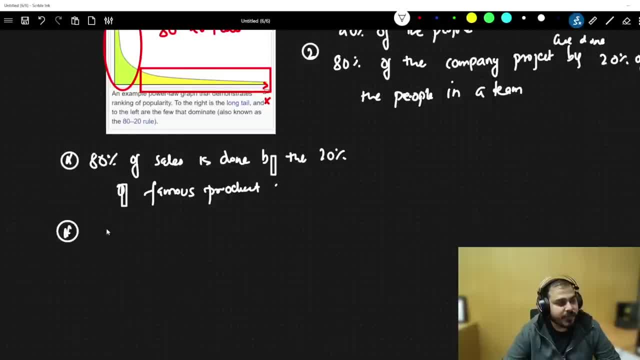 Any example More. One more example I can take: 80% of the match- cricket match, Okay, let's say- Is won by 20% of the 20% of the team. 80% of videos are completed by 20%. 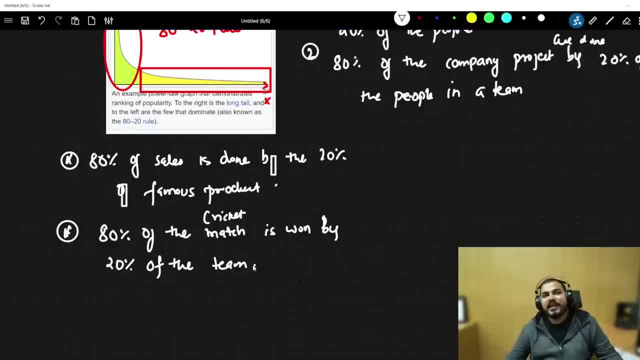 80% are serious out of all the 100%. Like 80% of the syllabus are completed by 20% of the people. 80% spamming on YouTube video has been done by 20% of the people. Yes, 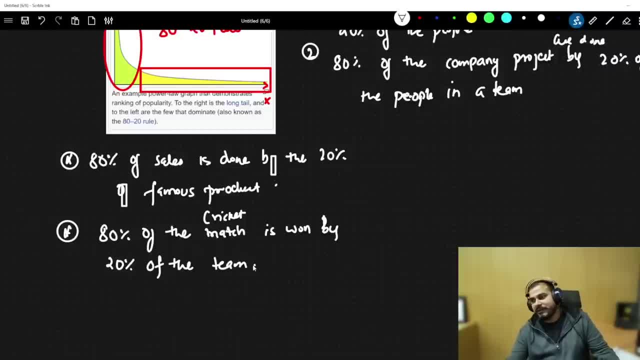 Any kind of examples you can basically take. You can also consider salaries. You can also consider, Yes, 80% of oil coming from 20% of the land. So whenever you have what this kind of distribution, it is called as power law distribution- 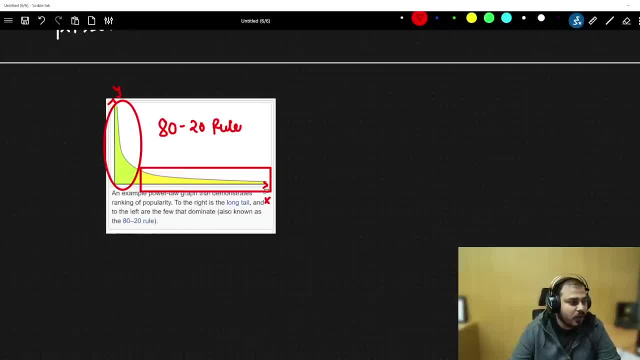 something. my y-axis may be something, but understand the 80 of one kind of distribution will be falling here and remaining 20 will be falling here. Let's say some, take some examples. okay, now suppose if I say that 80 percentage of the wealth is distributed with 20 percentage of the people, 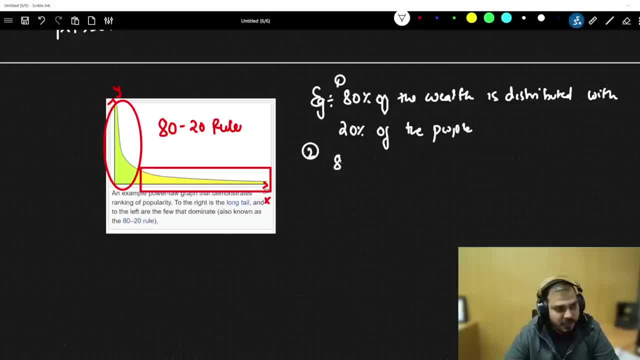 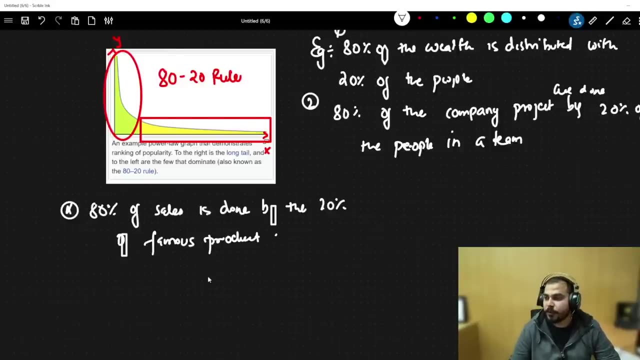 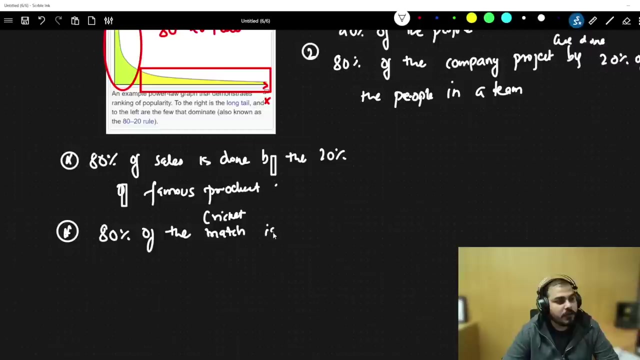 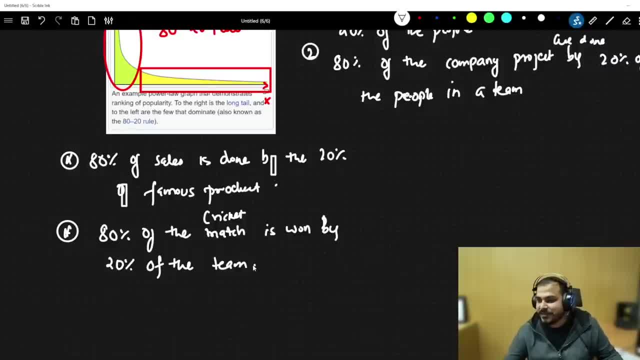 of videos are completed by 20 percent. 80 percentage are serious out of all the 100. like 80 percentage of the syllabus are completed by 20 percentage of the people. 80 percent spamming on youtube video has been done by 20 percentage of the people. yes, any kind of examples you can. 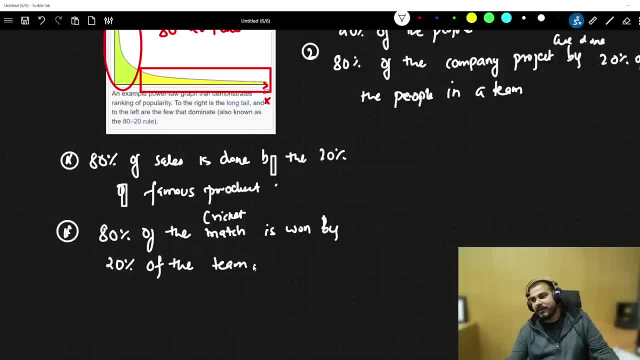 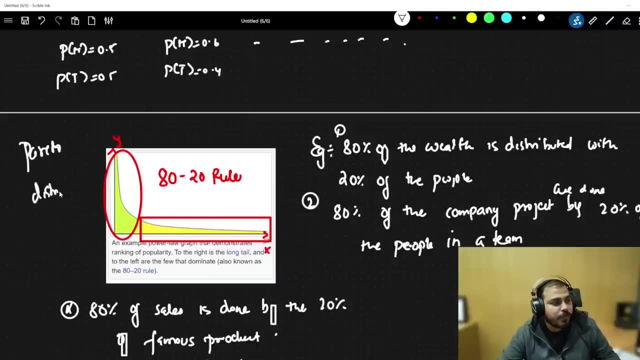 basically take. you can also consider salaries. you can also consider, yes, 80 percentage of oil coming from 20 percentage of the land. so whenever you have what this kind of distribution, it is called as power law distribution and this is also called as a parito distribution. now listen to me one. 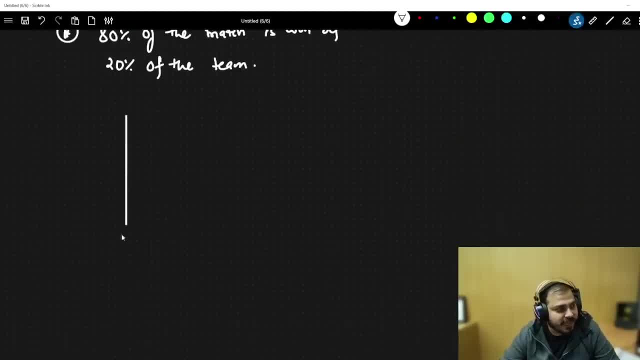 thing, guys. this is something very much amazing right now. this diagram that you see looks something like this, looks something like this. right, if i extend this diagram and probably make it like this, if i probably extend this diagram, if i extend this diagram and make it like this. 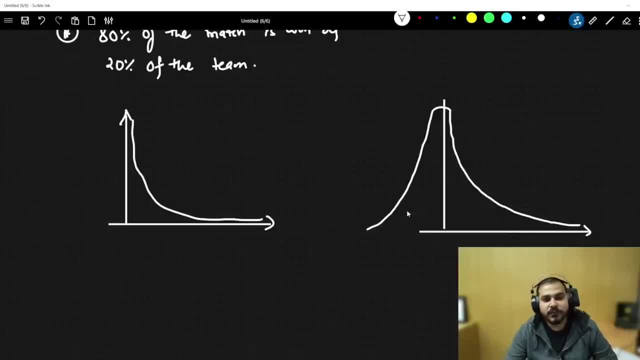 see this. this is a very important thing. then, what kind of distribution this is? this is my power law distribution. what distribution is this? this is not normal. this is, can i say this is log, normal distribution, log, normal guys, not normal. the right hand side over here. this will get extended by a lot log. 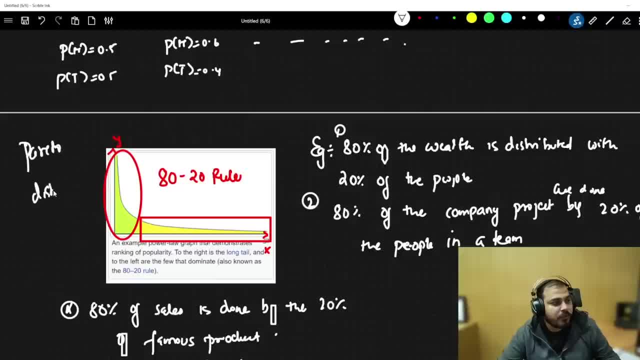 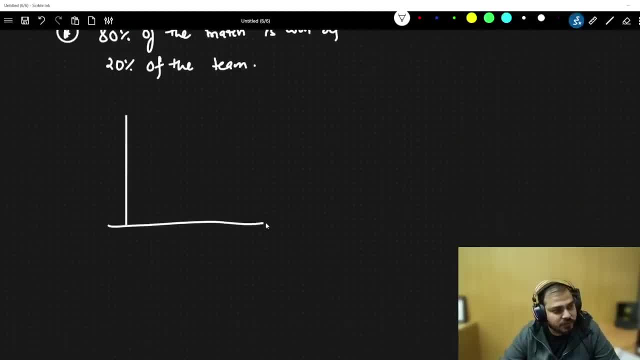 And this is also called as a Pareto distribution. Now listen to me one thing, guys. This is something very much amazing. Right now, this diagram that you see looks something like this, Looks something like this. right, If I extend this diagram and probably make it like this, 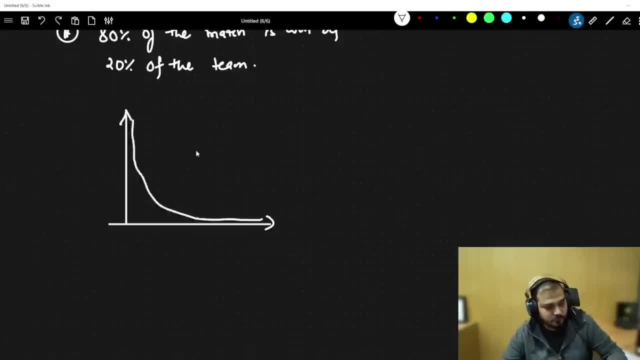 If I probably extend this diagram, If I extend this diagram and make it like this- See this, this is a very important thing- Then what kind of distribution this is? This is my power law distribution. What distribution is this? This is not normal. 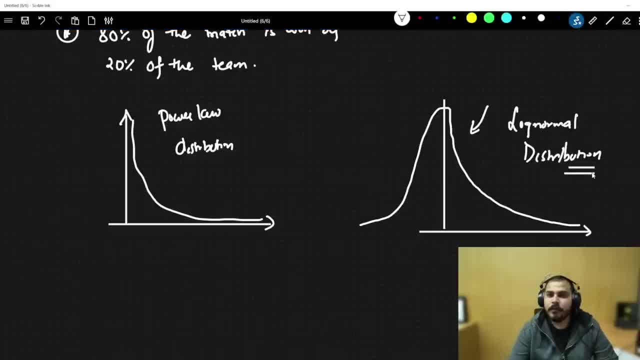 This is. can I say this is log normal distribution. Log normal guys, not normal The right hand side over here. This will get extended by a lot: Log normal distribution. Probably I did not draw the diagram properly, but it is a log normal. 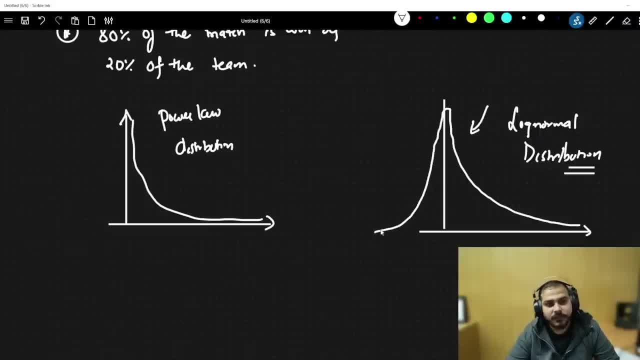 Log normal Right skewed data, Something like this. Let's say So: this specifically is a log normal distribution. So there is a very good relationship between log normal and power law distribution and Pareto distribution. So, mathematically, if I talk about 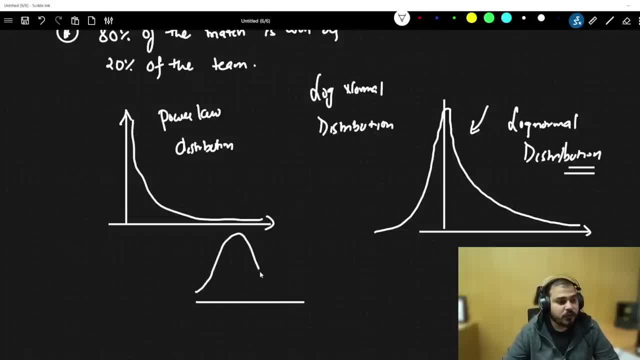 you can also convert this distribution into normal distribution also, And for this you have to watch one of my video which is called as transformation- data transformation. So definitely check out those video, And probably this is what is basically spoken about it, you know. 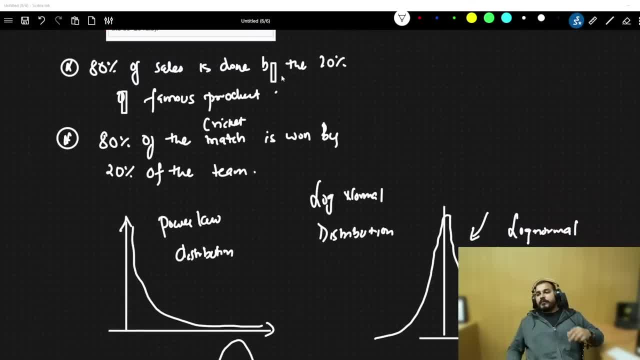 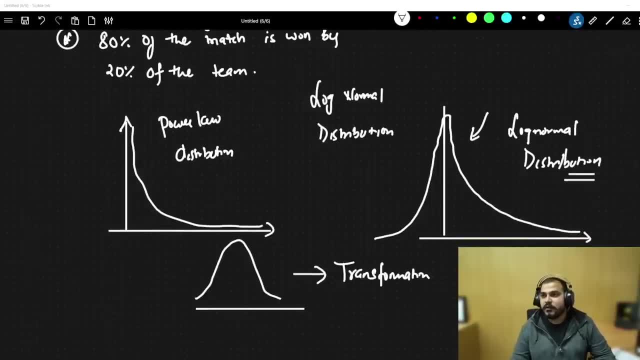 So that is called as Pareto distribution. with respect to this, Now, guys, yes, box cost transformation is basically used in order to convert this data into normal distribution. So probably you will be able to see from that video link that I have actually given. 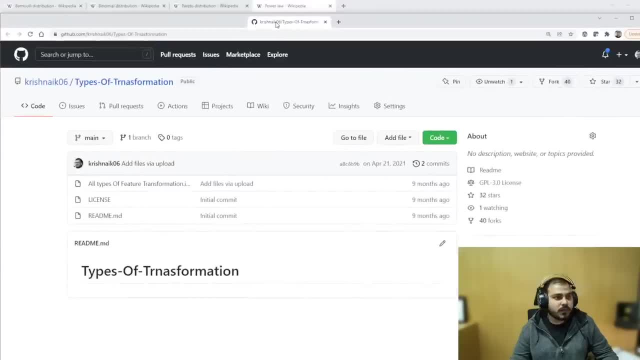 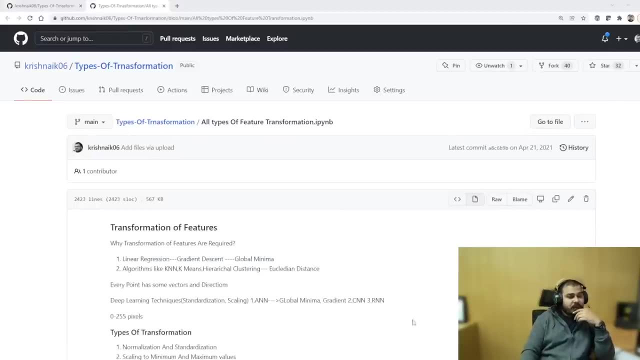 I can also show you the code, So this is how the code looks like. I have covered everything, guys. Now it's your time to flourish and learn everything. See over here all the transformation, normalization, standardization, scaling- this- this. 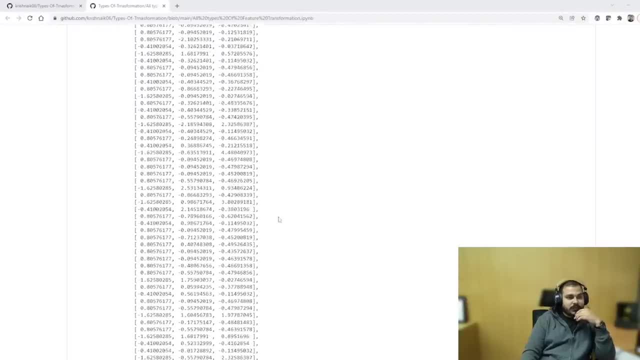 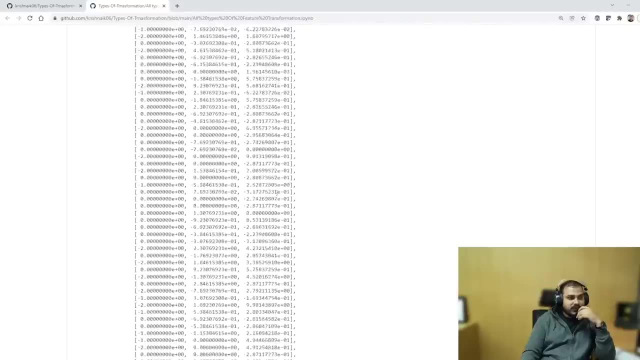 this square root. everything is given over here. So this is here. I have also discussed about QQ plot, So if I go and probably show you, So all the transformation is basically used, I have used all the transformation in this. You have to follow that video, guys. 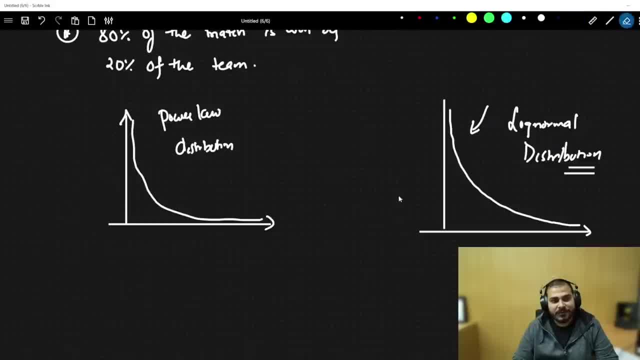 normal distribution. probably i did not draw the diagram properly, but it is a log norm, log normal right skewed data, something like this, let's say. so this, specifically, is a log normal distribution, so there is a lot of power law distribution, and this is a very important thing. then what kind of 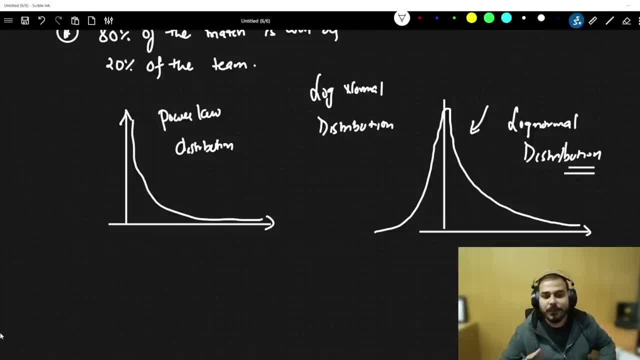 distribution is this: this is a very good relationship between log, normal and power law distribution of parito distribution. so mathematically, if i talk about, you can also convert this distribution into normal distribution also, and for this you have to watch one of my video which is called as transformation- data transformation. so definitely check out those. 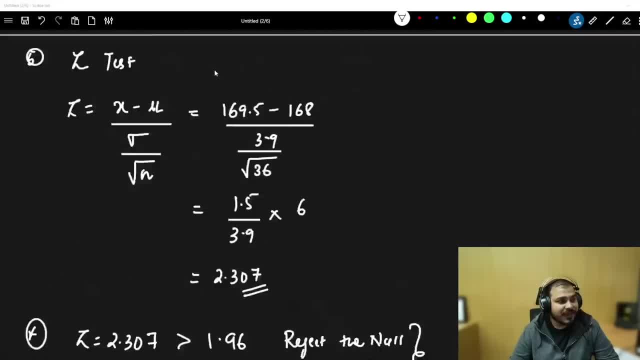 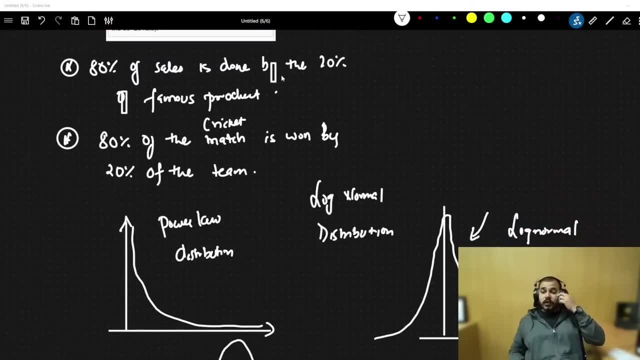 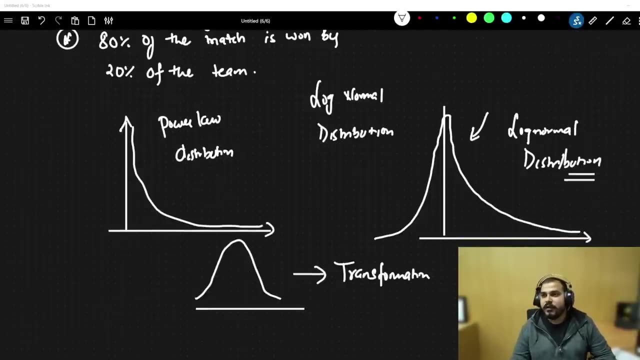 video and probably this is what is basically spoken about it. you know, so that is called as parito distribution. with respect to this, now, guys, uh, yes, box cost transformation is basically used in order to convert this data into normal distribution. so probably you will be able to see from that video link that i have actually given. i can also show you the code. so 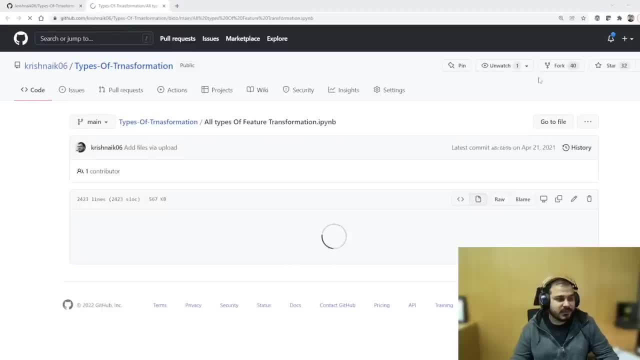 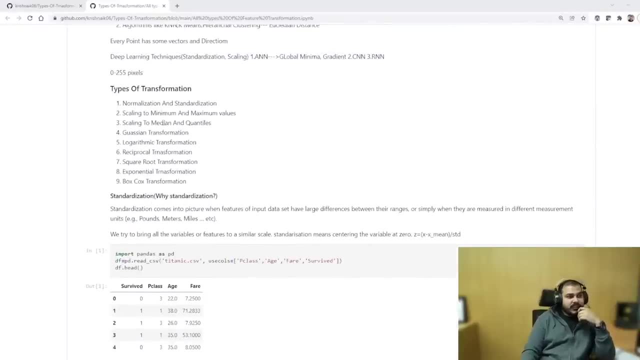 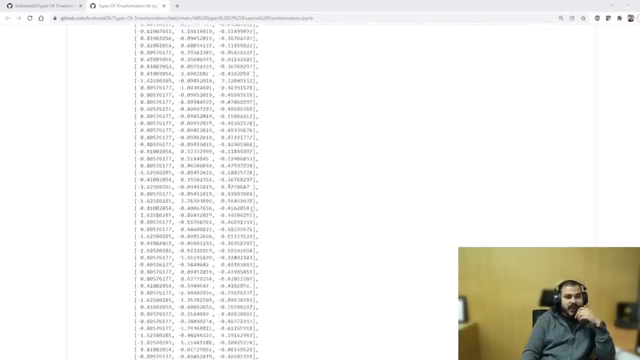 this is how the code looks like. i have covered everything, guys. now it's your time to flourish and learn everything. see over here all the transformation: normalization, standardization, scaling, this, this, this square root- everything is given over here. so this is here. i have also discussed about qq plot, so if i go and probably show you so, all the transformation is basically. 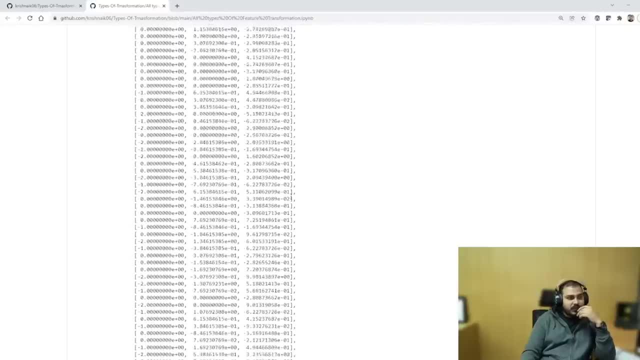 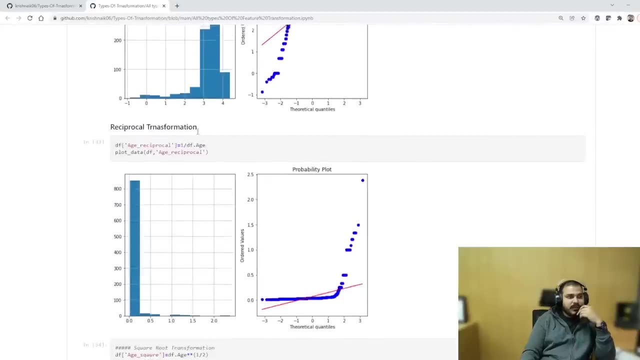 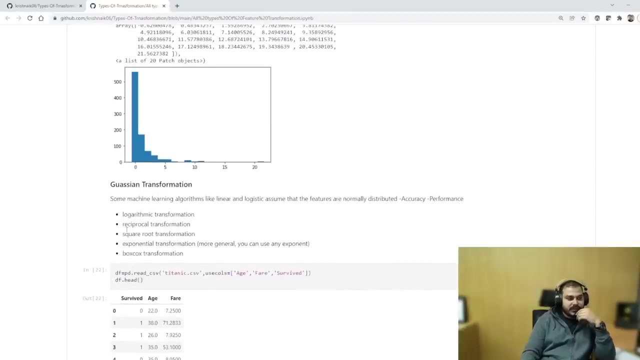 used. i've used all the transformation in this. you have to follow that video, guys, because it will probably take me one hour to explain all these things. see, this is what is qq plot is reciprocal transformation, logarithmic transformation. then you have gaussian transformation. these all transformation are the logarithmic reciprocal square root. 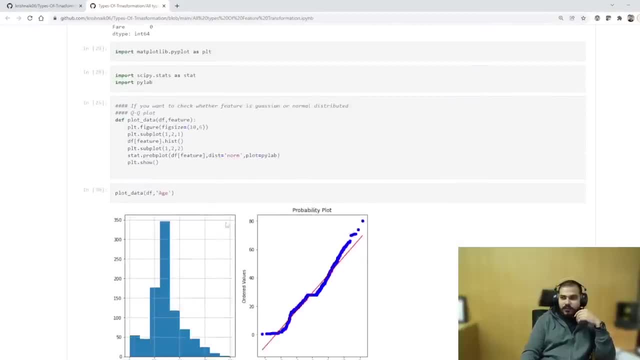 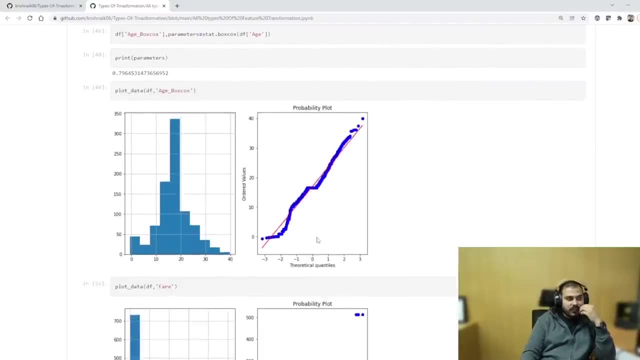 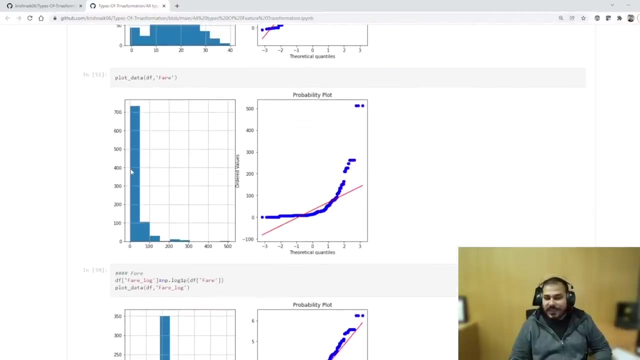 exponential transformation, boxcox transformation. so all this transformation is basically used in. in the initial stages we basically apply with respect to all the features and then we'll be able to. can i say this distribution follows what? what kind of distribution this image follows? so it is in the same link in the youtube channel that i've actually given what kind of distribution this. 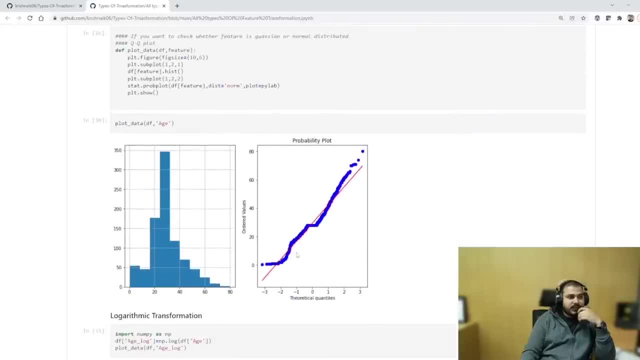 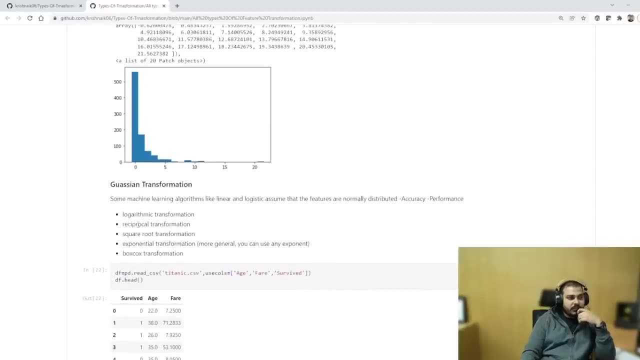 because it will probably take me one hour to explain All these things. See, this is what is QQ plot is Reciprocal transformation, logarithmic transformation. Then you have Gaussian transformation. These all transformation are there, Logarithmic, reciprocal. 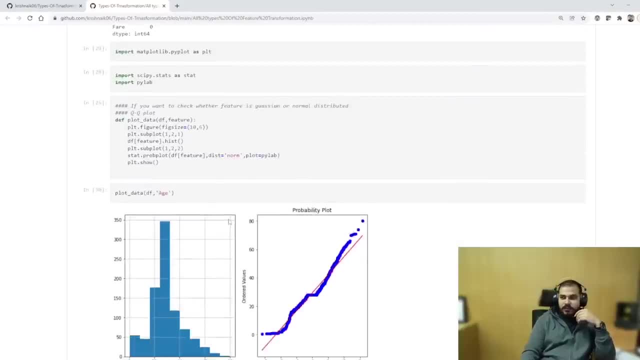 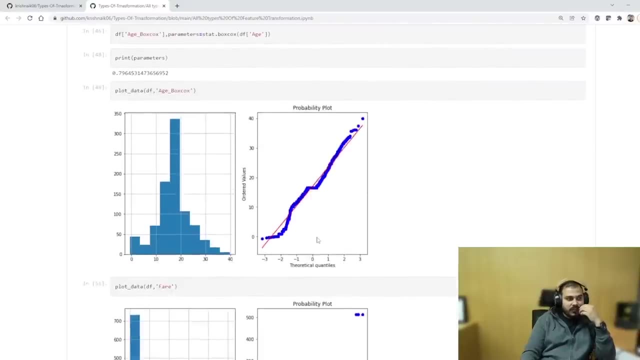 square root, exponential transformation, box cost transformation. So all this transformation is basically used in. in the initial stages We basically apply with respect to all the features and then we'll be able to. can I say this distribution follows what? what kind of distribution this image follows? 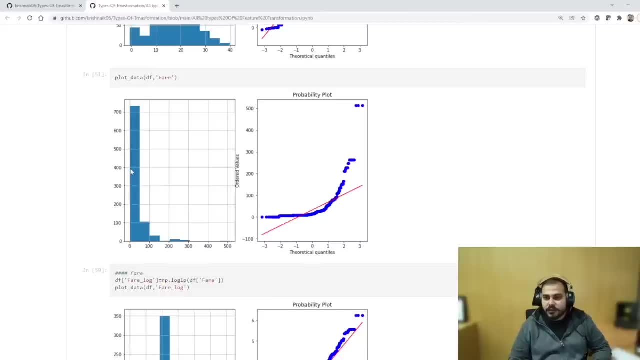 So it is in the same link in the YouTube channel that I've actually given What kind of distribution this follows. This follows a Pareto distribution, a power law distribution right, So we can basically use a box cost transformation to convert this data. 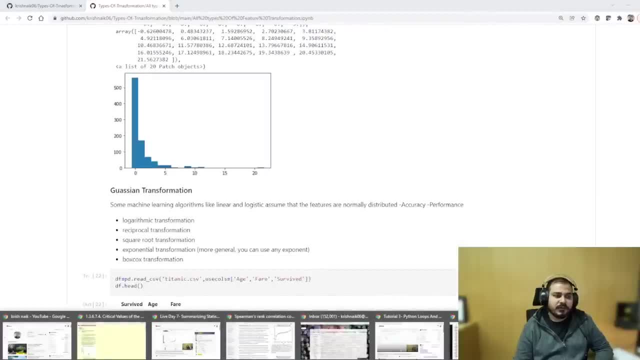 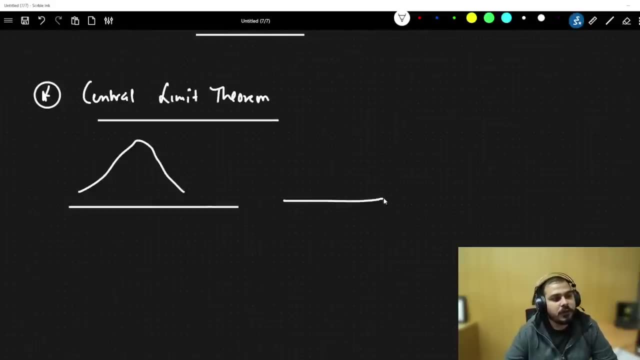 So if you, if you go through this, you are well covered with respect to everything. So central limit theorem basically says that if I have a distribution that is either normal, that is not normal or that is any kind of distribution that I have, 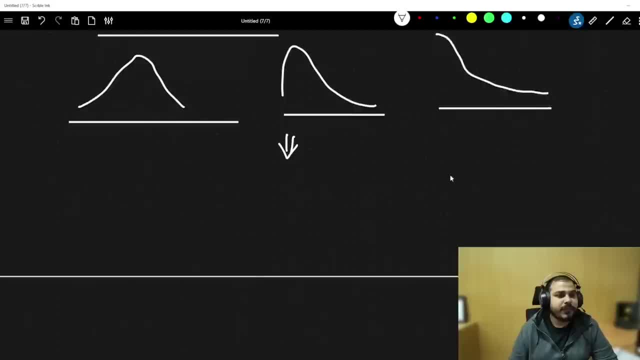 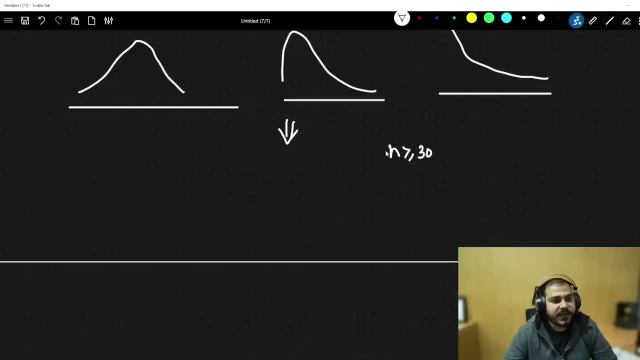 Whenever we basically take up multiple samples. let's say that I have this distribution or this distribution, this distribution. If I take up some multiple samples, let's say that n is greater than or equal to 30. If I start taking multiple samples from this particular data, 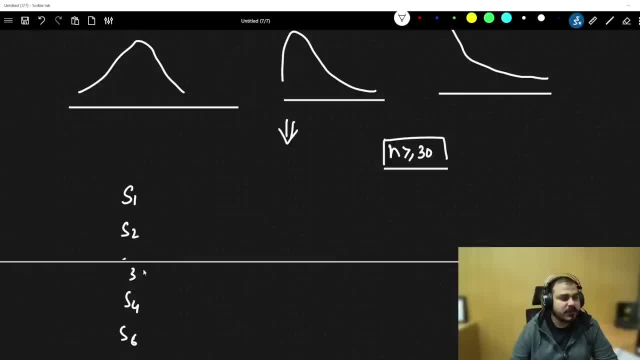 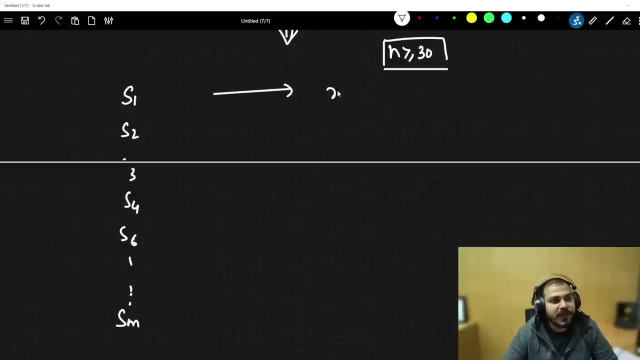 let's say that I have taken multiple samples like this, like this: up to n is greater than or equal to 30, like many, many samples. Okay, And for every sample, if I start finding the mean, if I start finding the mean. 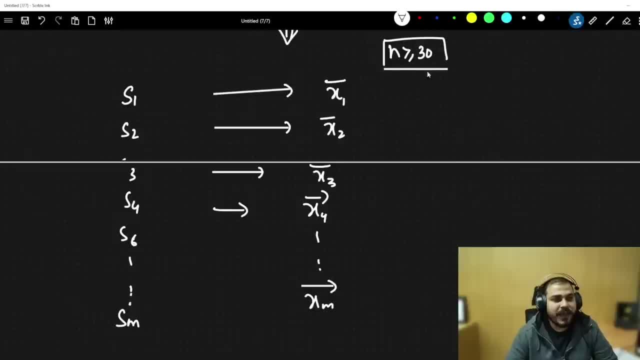 like this up till x of n. why I'm saying n should be greater than or equal to 30, because the more greater than or equal to 30,, the more the central limit theorem holds. Okay, So if I take this entire data of this sample mean, 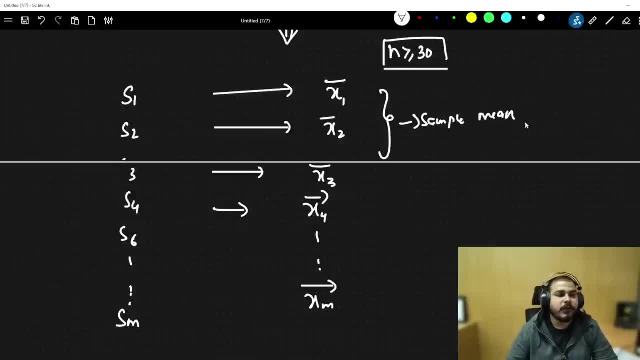 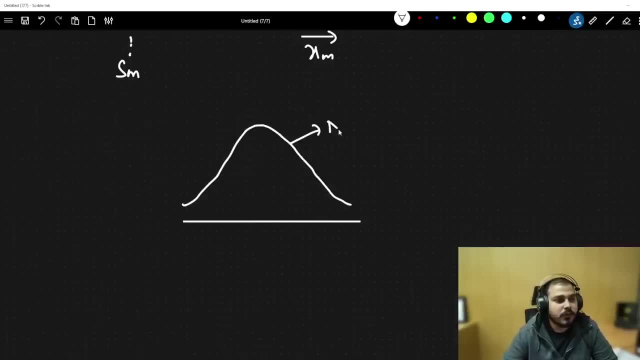 all the sample mean and if I populate it in the form of PDF, then that basically says that it will get converted into a normal distribution. So this will basically be a normal distribution. All the sample mean will follow. this sample mean will follow a normal distribution. 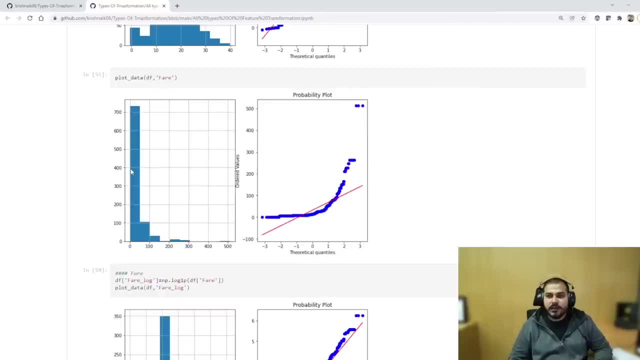 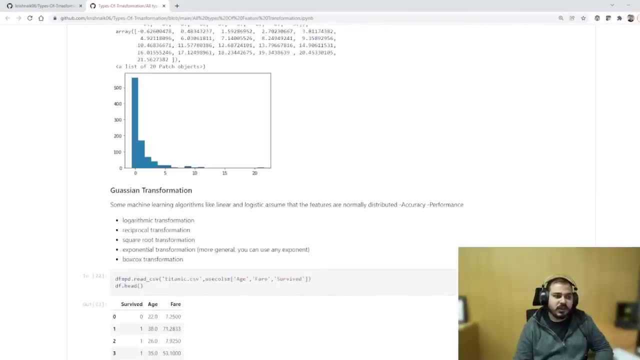 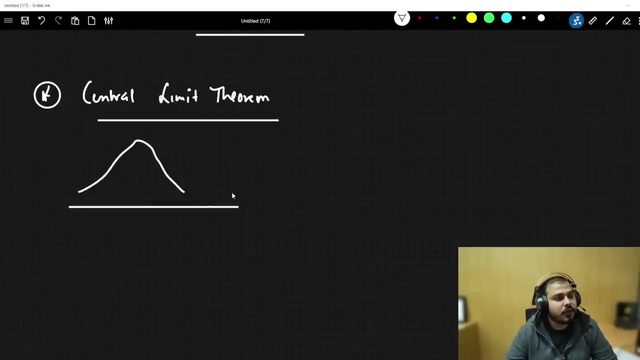 follows? this follows a pareto distribution, a power law distribution, right, so we can basically use a boxcox transformation to convert this data. so if you, if you go through this, you are well covered with respect to everything. so central limit theorem basically says that if i have a distribution that is either normal, that is not normal or that is any kind of 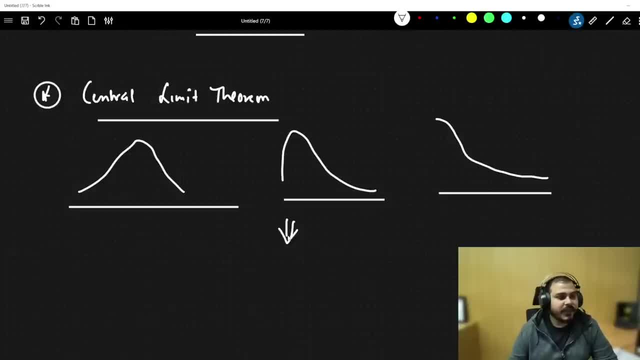 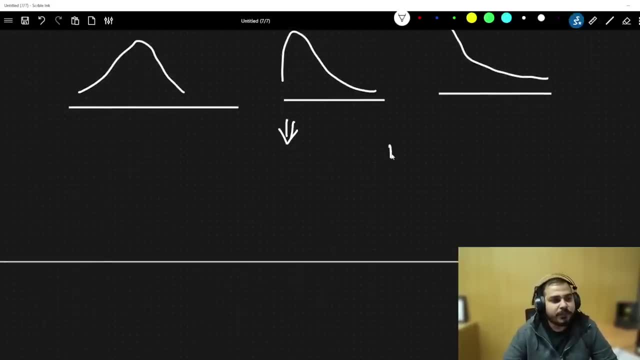 distribution that i have whenever we basically take up multiple samples. let's say that i have this distribution or this distribution, this distribution, if i take up some multiple samples. let's say that n is greater than or equal to 30, if i start taking multiple samples from this. 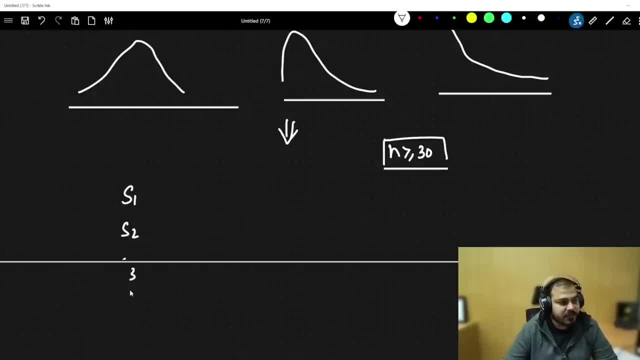 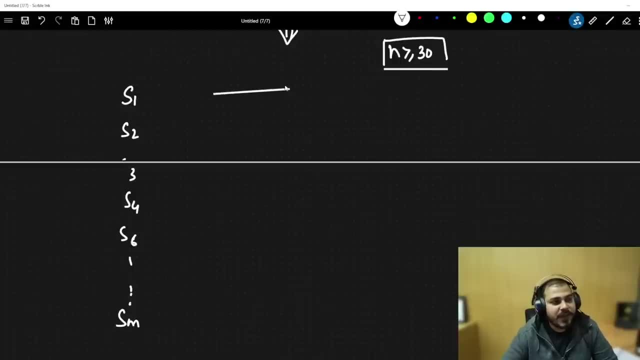 particular data. let's say that i have taken multiple samples like this, like this, up to greater than or equal to 30, like many, many samples. okay, and for every sample, if i start finding the mean, if i start finding the mean, like this, up till x of n, why i'm saying uh, n should be greater than. 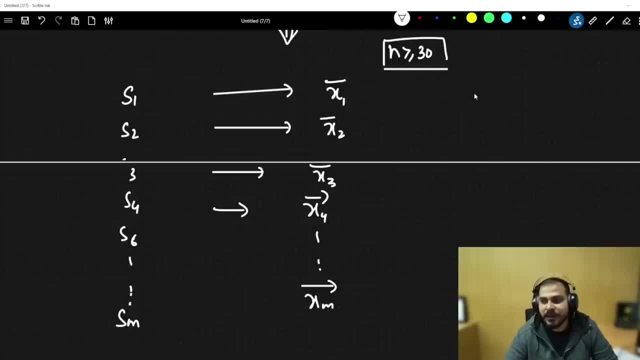 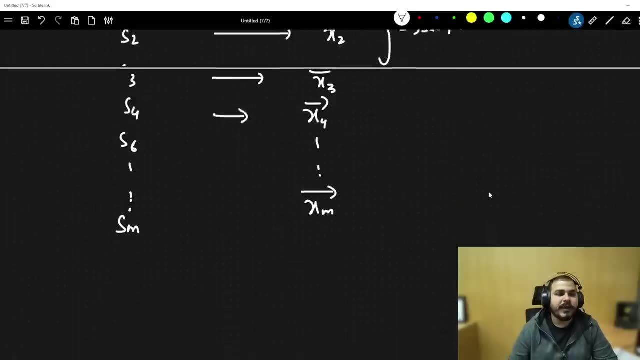 or equal to 30, because the more greater than or equal to 30, the more the central limit theorem holds. okay, so if i take this entire data of this sample mean, all this sample mean, and if i populate in the form of pdf, then that basically says that it will get converted into a normal distribution. 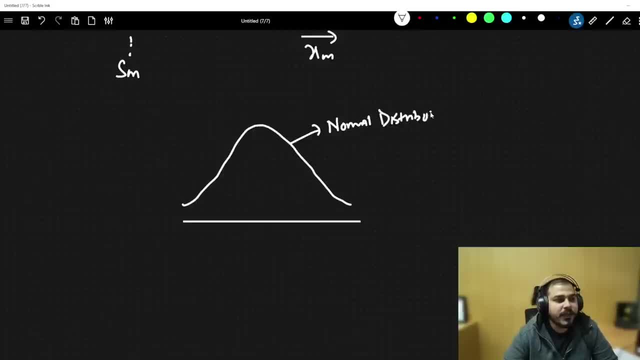 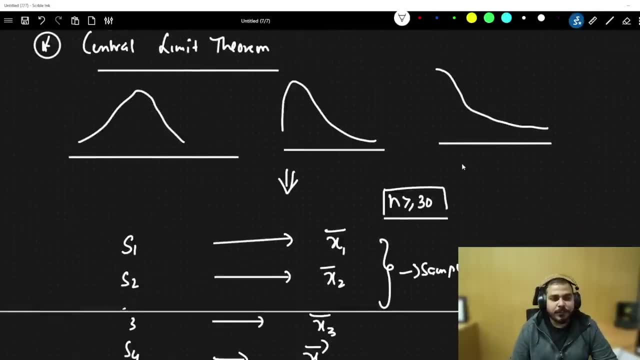 so this will basically be a normal distribution. all the sample mean will follow this sample mean will follow a normal distribution. so here you can see that, whatever distribution it may be, if we take some samples specifically, n is greater than or equal to 30 for each and every sample. if 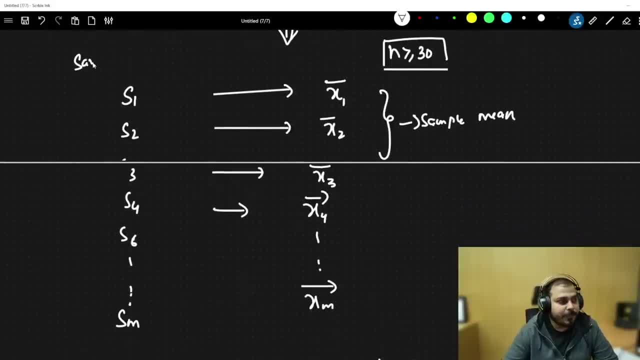 i try to find out the sample mean, sample size. so see sample size. i told you it should be n is greater than or equal to 30.. sample size: the number of elements over here that we are picking should be greater than or equal to 30, and let's consider that we have taken. 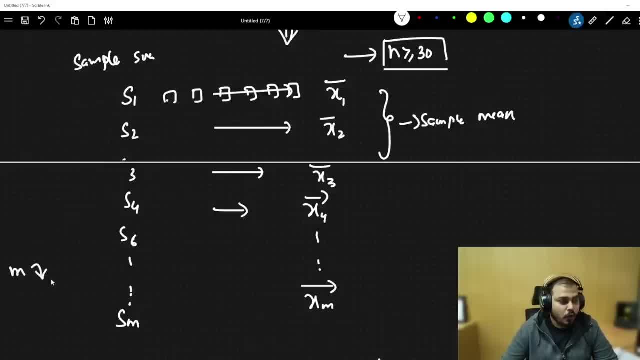 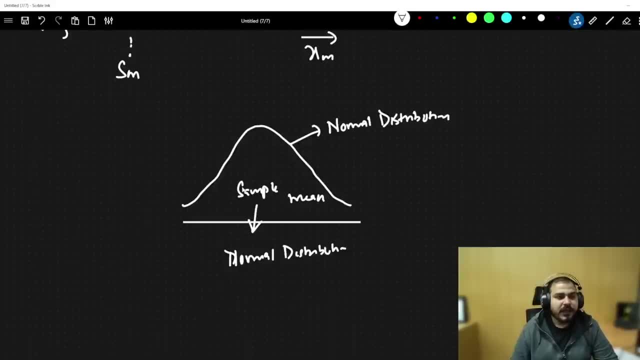 m samples. m samples can be anything but more the bigger value, more better. we will be able to solve this particular central limit here. so here you will be able to see that as we go on doing this, finally you will be able to see that if we populate all the sample mean we get this normal.